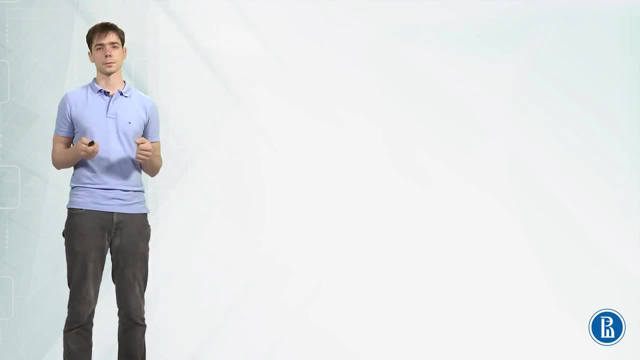 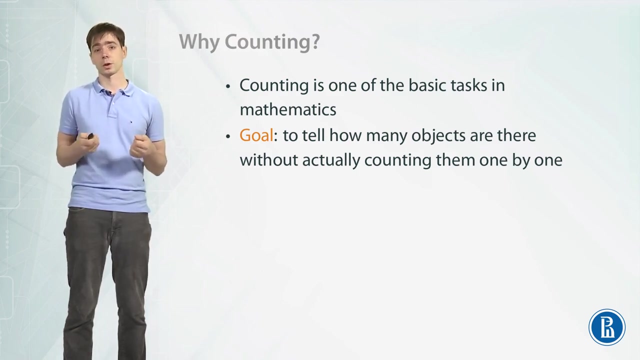 Hi, I'm Vladimir Podolsky, and today we are going to discuss basics of counting. Counting is one of the basic tasks in mathematics, And the main goal here is to tell how many objects are there of certain type, without actually counting them one by one. 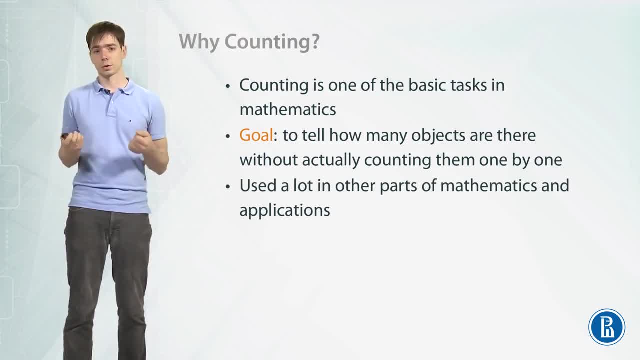 Counting is used in many other parts of mathematics and in applications, so it's a very important area, and there are two applications that are important for us. The first one is counting number of steps of algorithms. to estimate the running time of an algorithm. 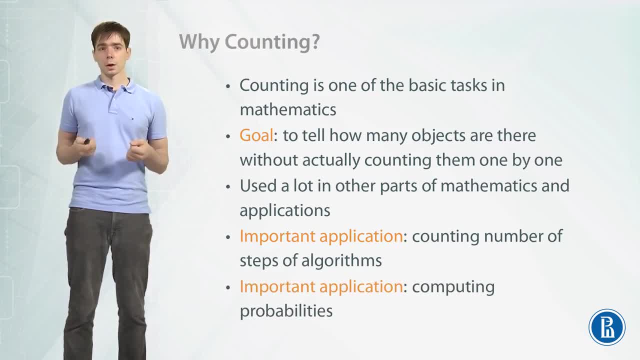 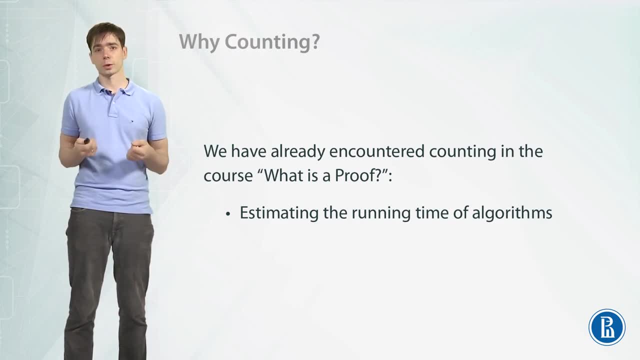 And the second one is counting probabilities. If you have seen the first course of our specialization- what is a proof? then you can note that we have already encountered counting twice there: First time when we tried to estimate the running time of some algorithms, and the second time. 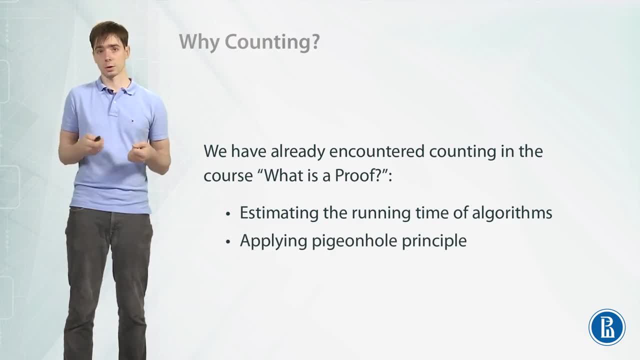 when we tried to estimate the running time of some algorithms And we tried to apply pigeonhole principle. To apply pigeonhole principle, we have to count the number of pigeons and the number of pigeonholes, But counting turns out to appear even in simple real-life situations. 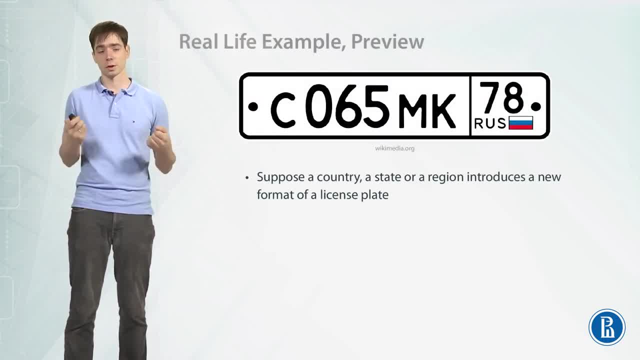 Consider the following example of license plates. Suppose there is some country or state or region that introduces a new format of their license plates- And here is a right example. This is a Russian example. The new form of license plates, which was introduced about maybe 20-25 years ago, is the following: 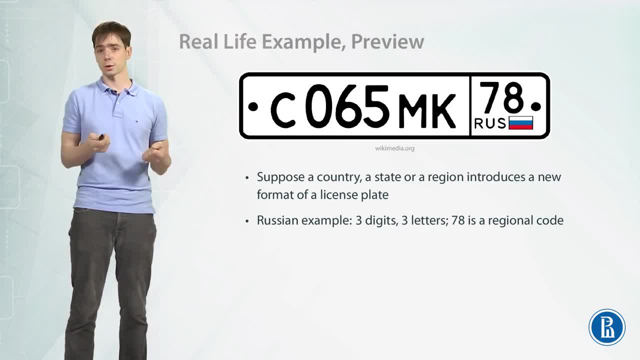 So there are three digits, three letters, and here 78 is a regional code. So for a fixed region this code is fixed. So we have 10 options for digits, from 0 to 9.. And we have 12 options for letters. 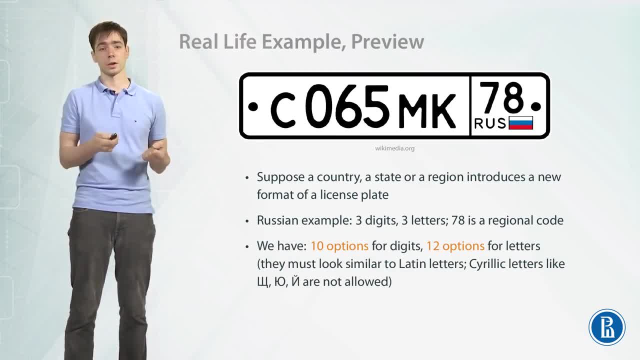 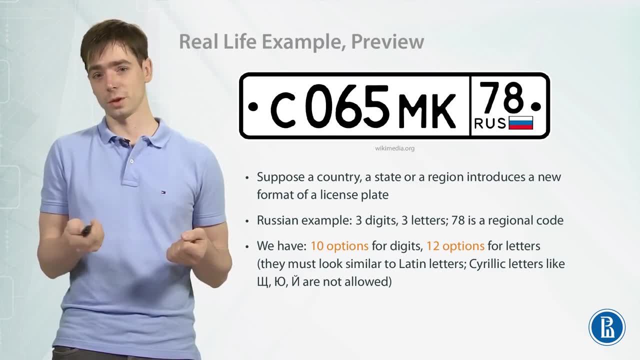 Because these are Cyrillic letters and they must look similar to Latin letters. So some Cyrillic letters, like those listed here, are not allowed. So how many possible license plates do we have with this format of a license plate? Is it enough for everyone? 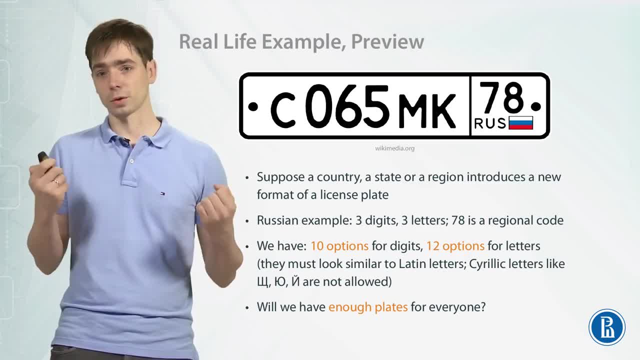 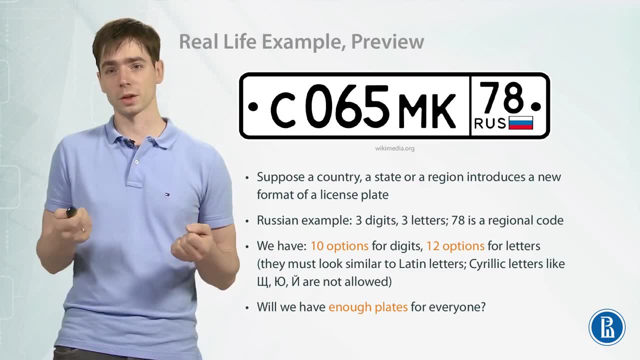 And what should we do in this situation? if we are a government, or Okay, So if we are introducing this license plate, should we hire someone who will just list all possible license plates and count them one by one, Or should we do something smarter? 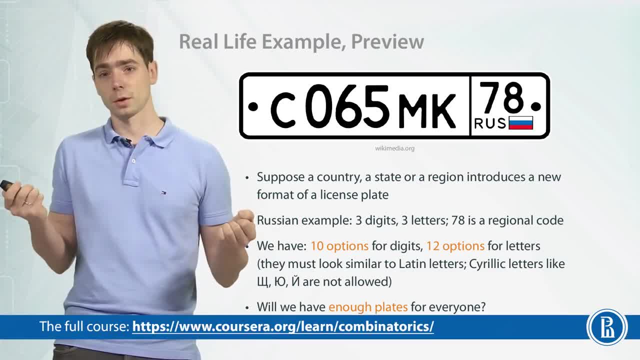 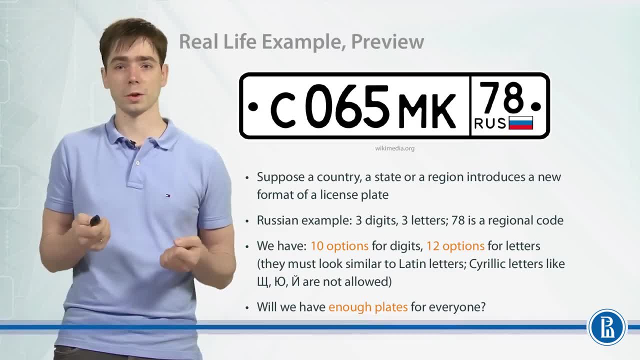 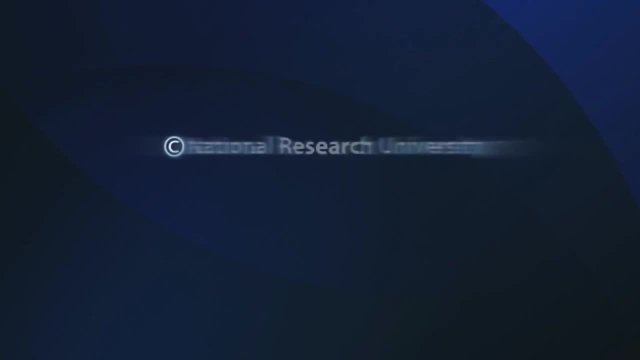 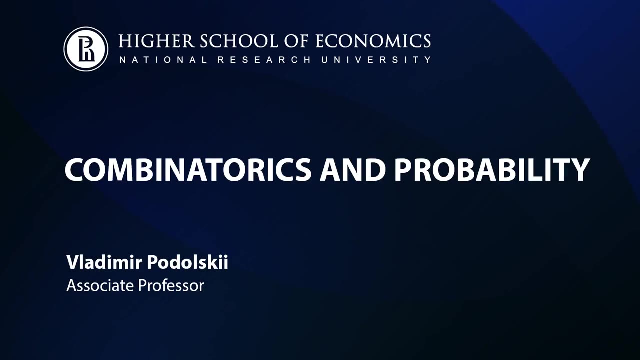 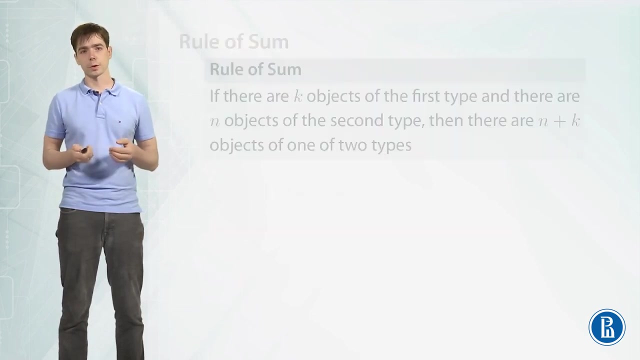 So that's what we are going to discuss in this course, And in the end of this week we will be able to answer these questions about license plates. So we will start with our most basic building block rule of sum. Suppose we have k objects of the first type and we have n objects of the second type. 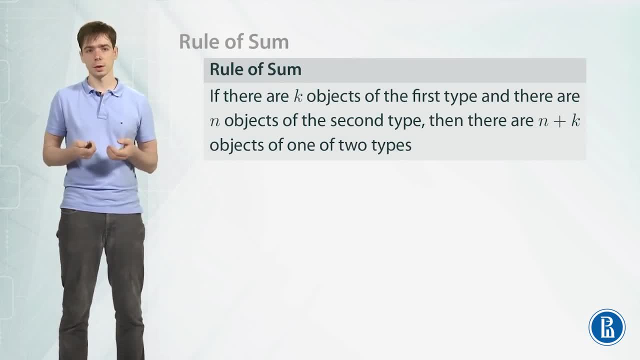 Then we have n plus k objects of one of the two types, of the first one or of the second one. So this rule is very simple. Here is a simple example. Suppose we are looking for a place to eat And we are looking for a place to eat. 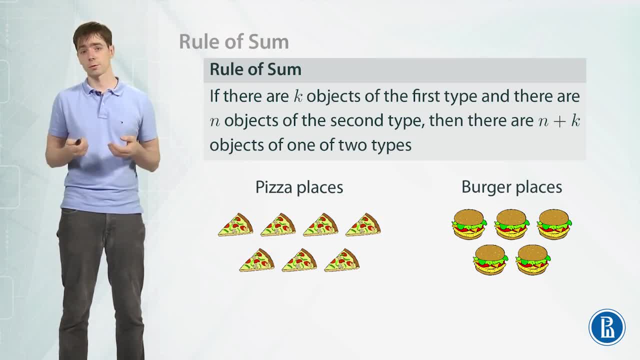 And we are looking for a place to eat And we have 7 options for the pizza place And we have 5 options for the burger place. So in total, then, we have 7 plus 5 places to eat today. So that's the basic example. 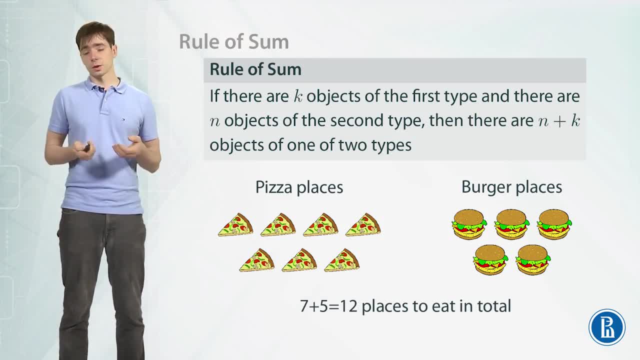 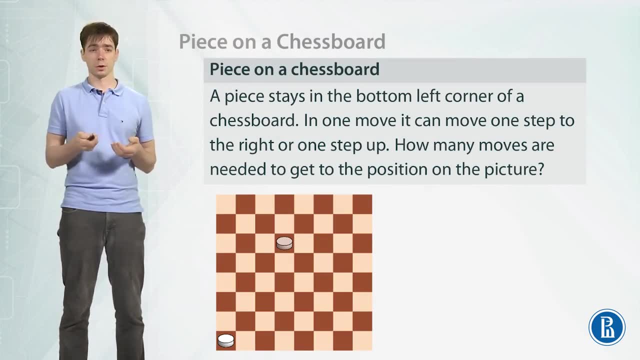 The rule is indeed very simple. Let's consider the following simple problem. Suppose we have a piece on the chessboard And it is positioned in the bottom left corner And we need to move the piece to the position indicated on the picture, And in each move the piece can move one step right or one step up. 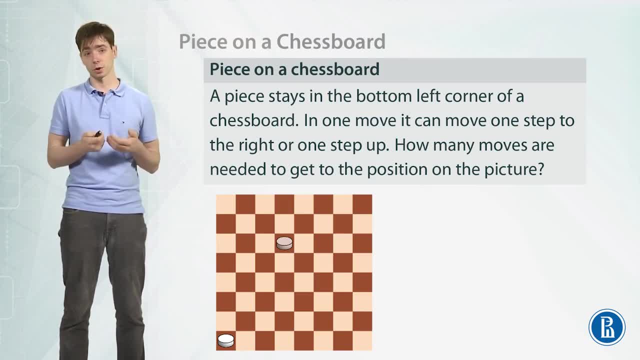 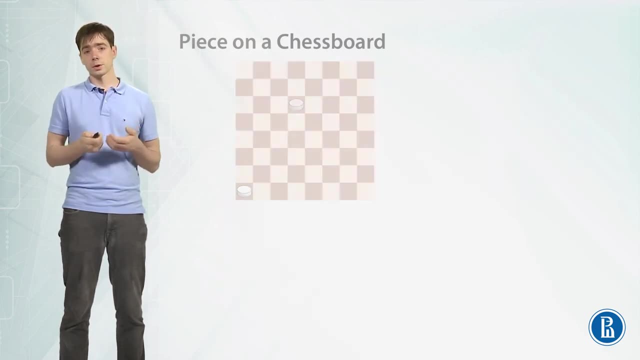 So how many moves do we need to get to the desired position? And if you have seen our first course, what is a proof? then you can recall that we have considered. we have encountered this problem there as well. Okay, let's see how we can get to this position. 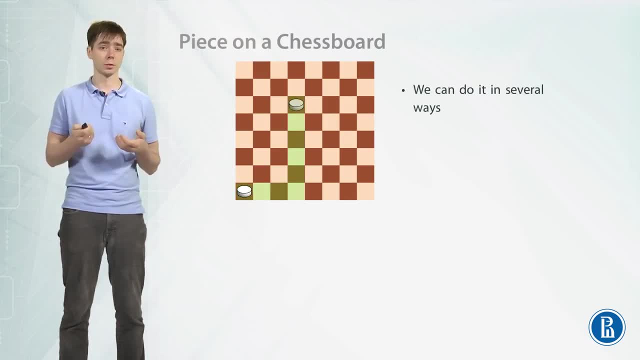 And there are several ways to do it And, for example, we can do it this way: So in this case we need eight moves. Okay, we can do it, for example, this way: We can move up first, then to the right, then up, then to the right again. 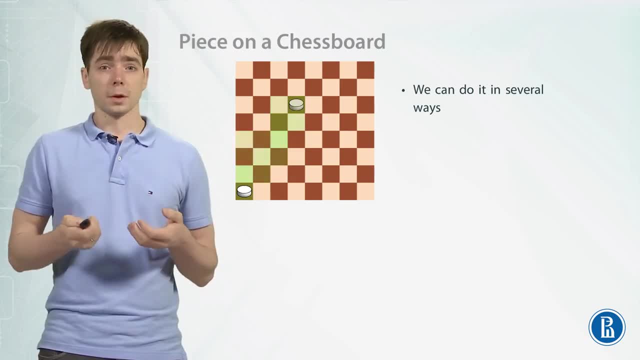 And we need eight moves. again, We can do it this way, So we go up, then right, then up, then right, then up again, and then right, then up again. So Again, we need eight moves. So in all cases we needed eight moves. 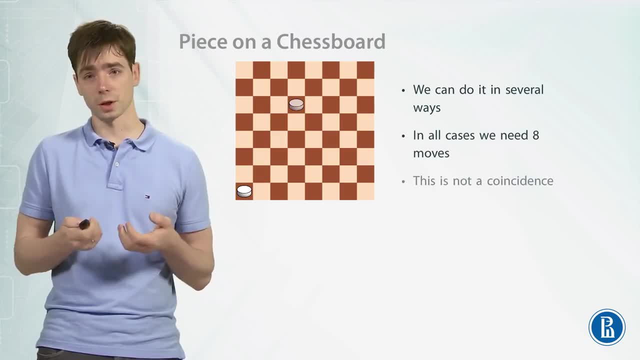 We can try some other cases And again we will need eight moves, because this is not a coincidence. So it turns out that we always need eight moves, And here is the reason why There are two types of moves: Moves to the right and moves up. 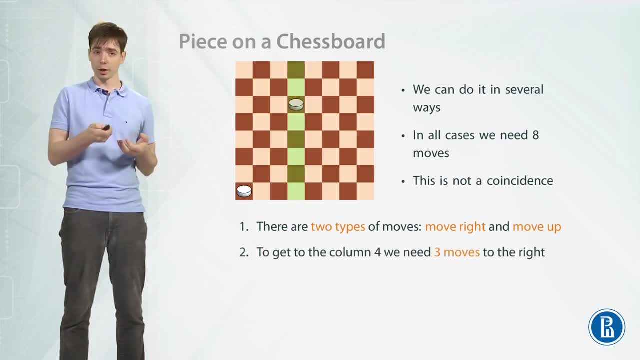 So let's see, We would like to get to the third column of the board. So to get to the third column, moves up doesn't help us. So if we move up, we stay in the same column And moves to the right helps us. 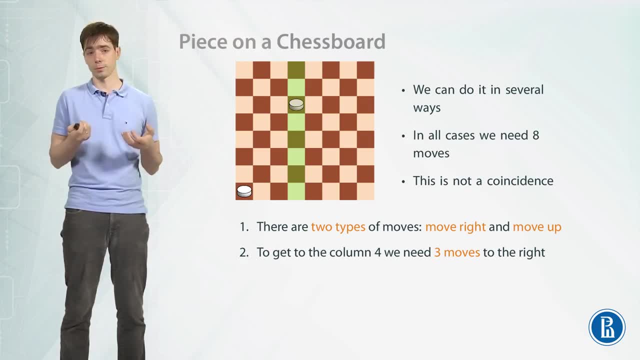 And we need three moves to the right to get to the fourth column. It's the fourth column, Okay, So now we need to get to the sixth row of the table of the chessboard. So again moves to the right. now doesn't help. 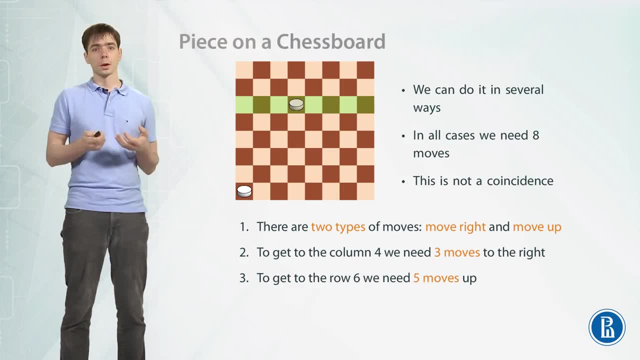 We stay in the same row But moves up helps, And we need five moves up to get to the right row. So there are two types of moves. We need three moves of the first type. We need five moves of the second type. 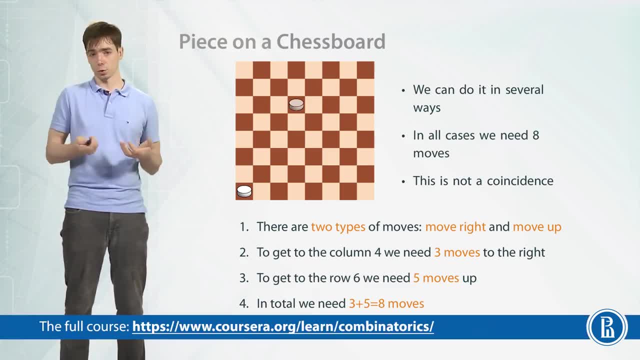 So in total, by the rule of thumb, we need eight moves. So note that we are actually using the rule of thumb. It's very simple, But still we are using it in this case. It's a simple argument. 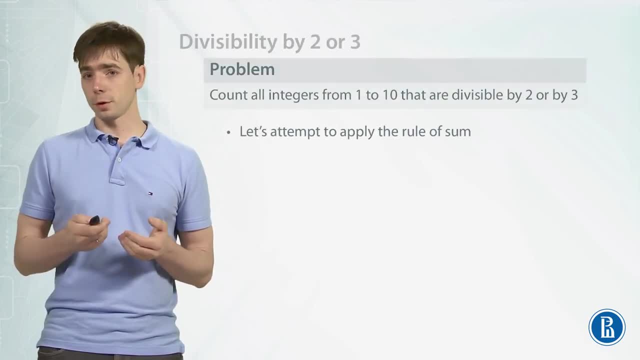 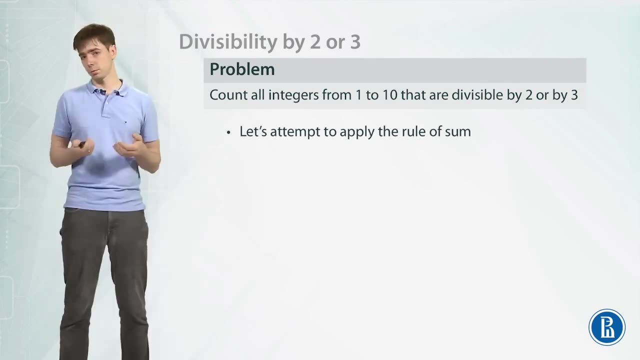 Okay, Let's consider the next problem. Suppose we have integers from one to ten And we would like to count how many of them are divisible by two or by three. And okay, This looks like a situation where we can apply the rule of thumb. 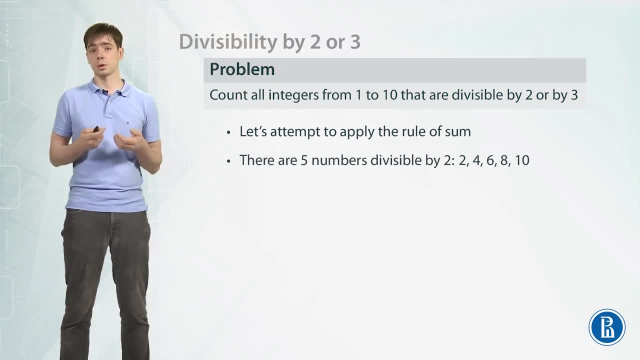 And let's try to do it. Let's see how many of integers are divisible by two, And we can just list all of them: Two, four, six, eight and ten. These are integers from one to ten which are divisible by two. 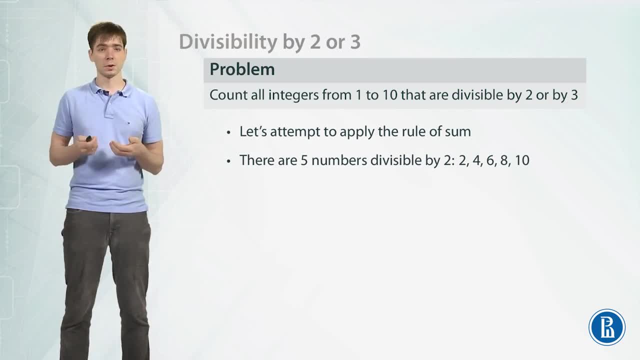 Okay, So now let's see how many integers are divisible by three. There are three of them, Three, six and nine. These are all integers that are divisible by three, from one to ten. Okay, So now we can apply the rule of thumb. 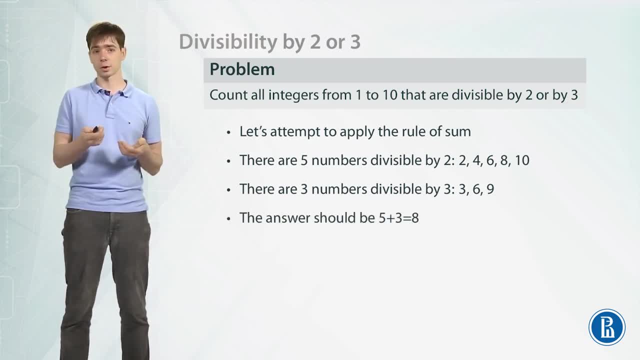 There are two types of integers And we can apply the rule of thumb and get the result. There should be eight integers, from one to ten, that are divisible by two or divisible by three. Okay, But let's check. Ten is a small number. 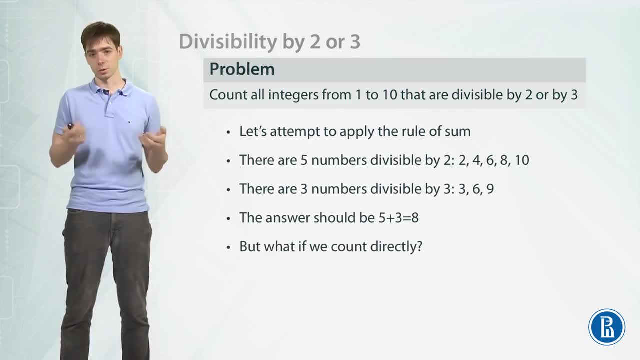 So let's just count all these numbers directly, Let's see what happens. So here are all numbers, from one to ten, And let's see how many of them satisfy our property. Okay, Two is good. So two is divisible by two. 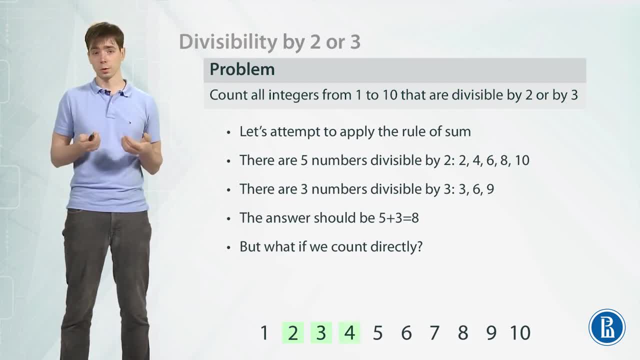 Three is also good, Three is divisible by three, Four is also good, Six is also good. Five is not good because it's not divisible by two or three. Seven is not good, Eight is good, Nine is divisible by three And ten is good. 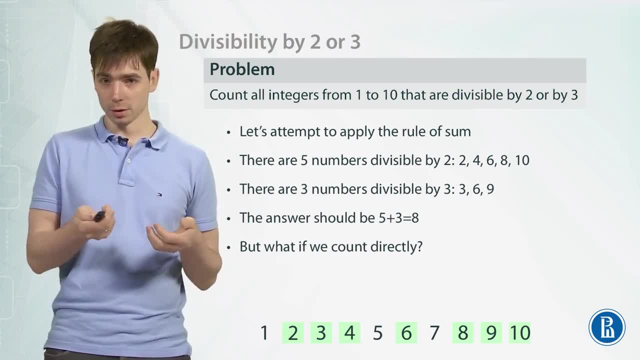 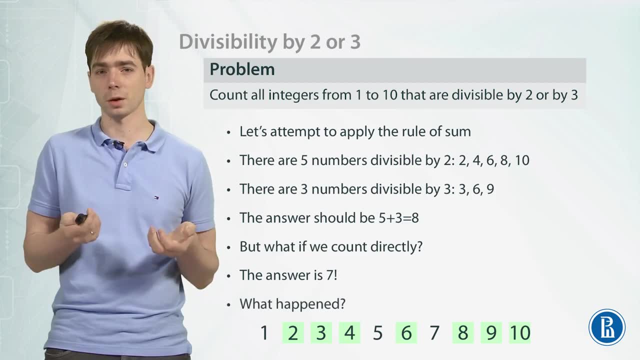 So now, if we count the number of green squares, we see that there are seven of them, So the answer is actually seven. And so what happened? How it happened that our rule of thumb, a very simple and trivial rule, gave us the wrong answer? 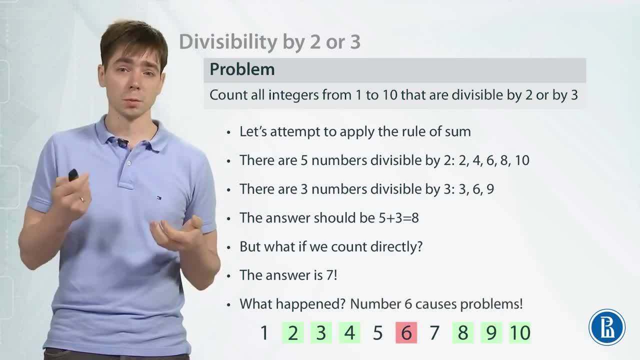 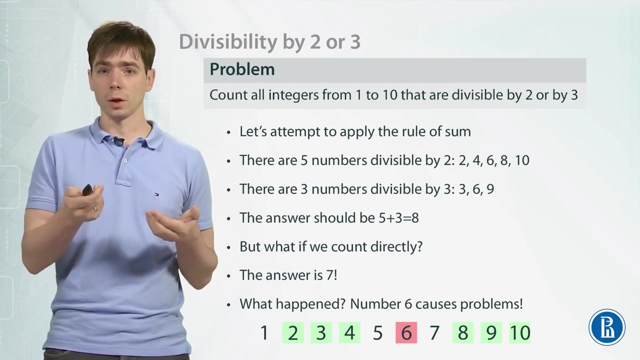 So actually the problem is with number six. Note that if you look at the list above, the list of numbers divisible by two and the list of numbers divisible by three, number six occurs twice there. So when we summed up five and three, we have counted six twice. 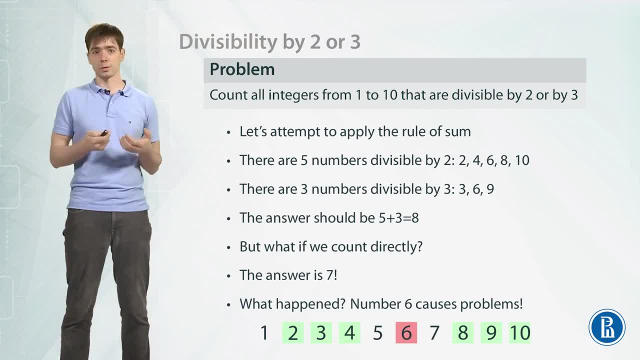 And this is the problem. So we applied the rule of thumb in the wrong way, So we should not do it. And let's recall the rule of thumb and let's see what actually we shouldn't do. Let's learn our lesson. 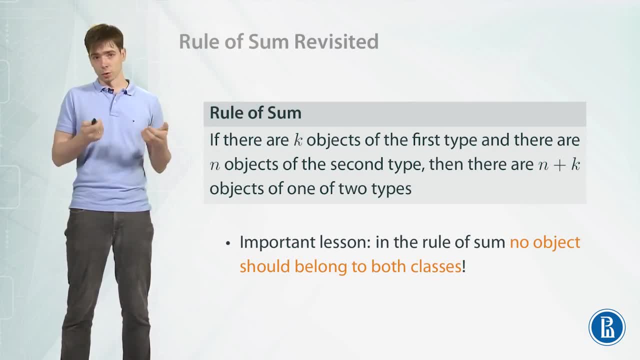 Let's recall our lesson from this example. So let's recall the rule of thumb. So we have k objects of the first type, There are n objects of the second type, And then we can say that there are n plus k objects of one of the two types. 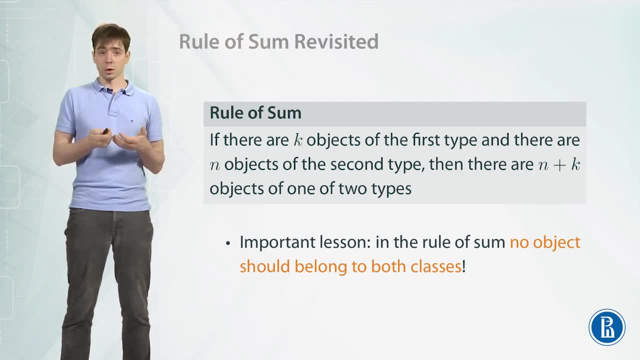 But now an important remark. No objects should belong to both types, Should have both types, should belong to both classes. in the rule of thumb They should be disjoint. Objects of the first type should be different objects from objects of the second type. 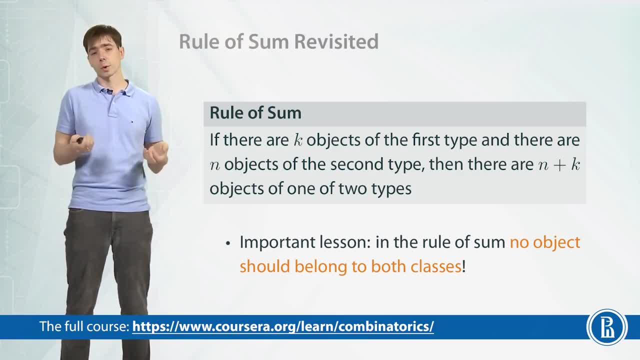 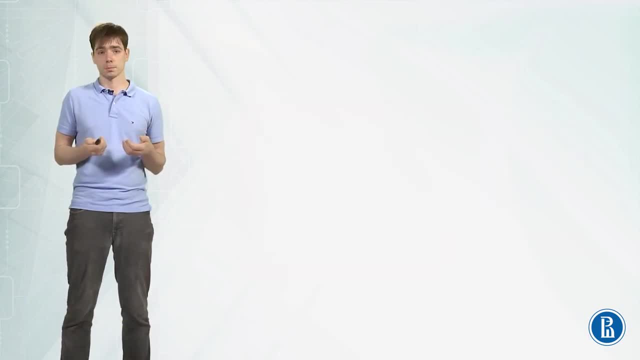 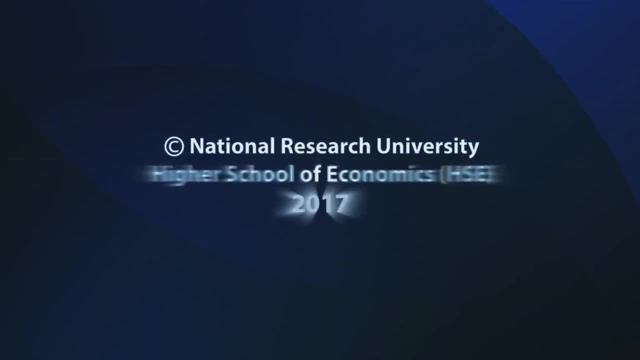 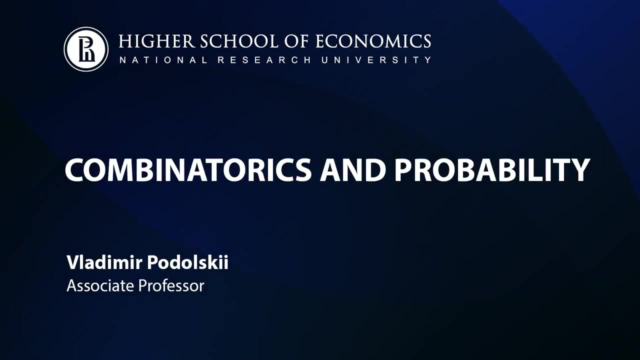 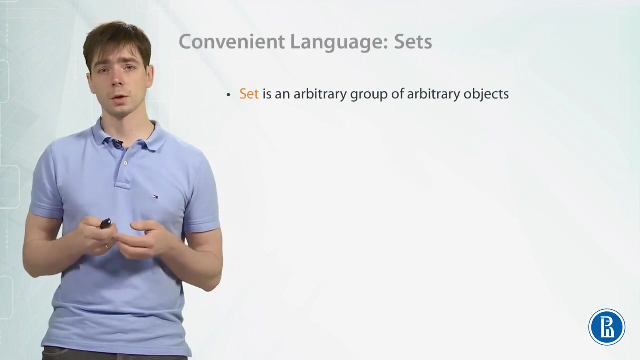 Then we can apply rule of thumb. Otherwise it gives us wrong results, like in the previous example. So we have to be careful when applying rule of thumb. It is a good time to introduce a convenient language. we will use Language of sets. 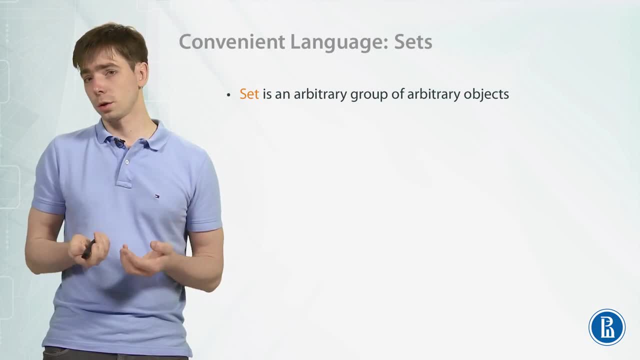 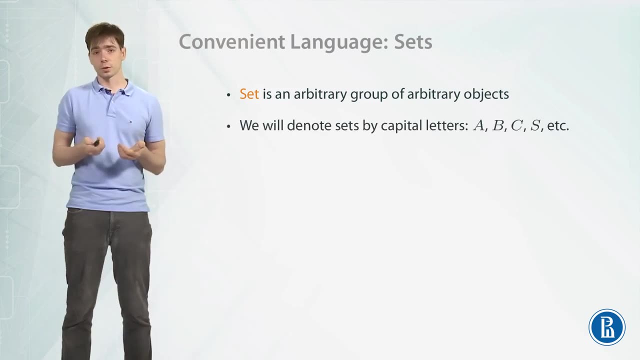 Set is a very simple object. It's an arbitrary group of arbitrary elements, arbitrary objects. So we will denote sets by capital letters: A, B, C, S and so on. And sets can be given, for example, by listing all of their elements. 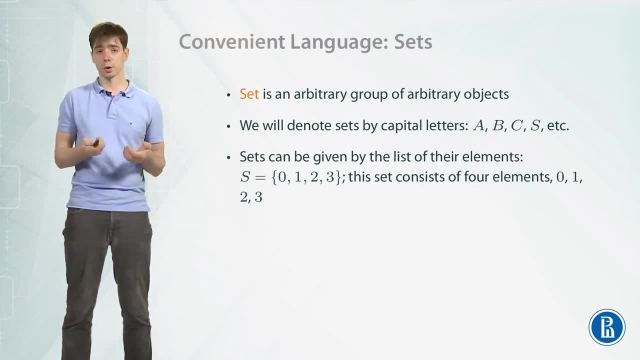 Sets are given by their elements And we can to define some set. we can just give a list of elements. For example, this set consists of four elements: 0, 1, 2, 3.. Okay, In this notation the order doesn't matter. 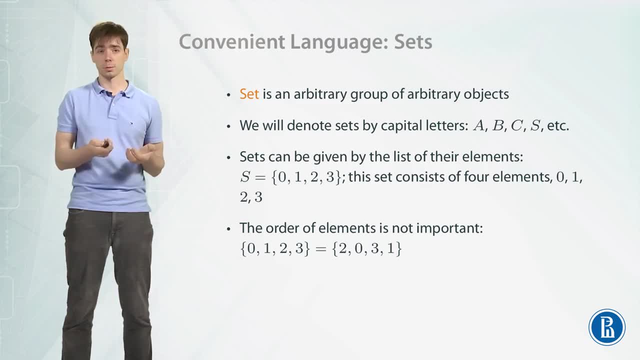 The order of elements in the set doesn't matter, So we can give the same set by the list 0, 1,, 2,, 3.. And by the list 2,, 0,, 3,, 1.. It's the same set. 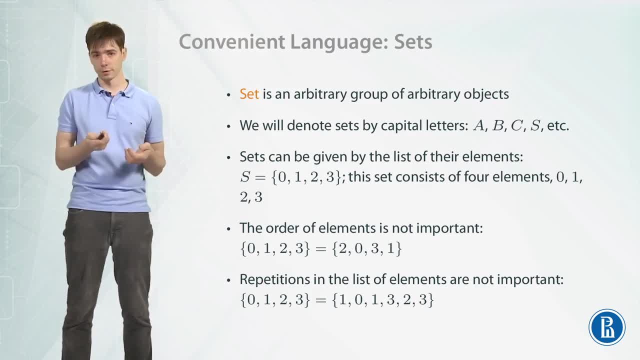 And we allow repetitions in the list when we give a set in this way, So each element either belongs to the set or doesn't, So it cannot belong there twice. So the set: 1, 0,, 1, 3,, 4.. 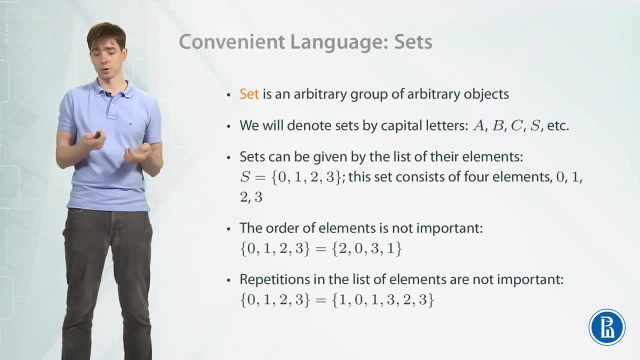 0,, 1,, 3,, 2, 3.. The set of these elements is the same as just the set of elements 0,, 1,, 2,, 3.. So each element either belongs to the set or not. 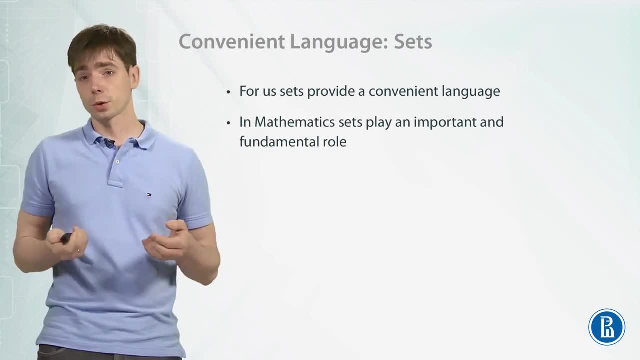 For us, sets provide a convenient language In mathematics. sets are very important. They play a fundamental role. They are the foundation of mathematics. For us, sets can be just any list of any elements. For example. this is a set for us. 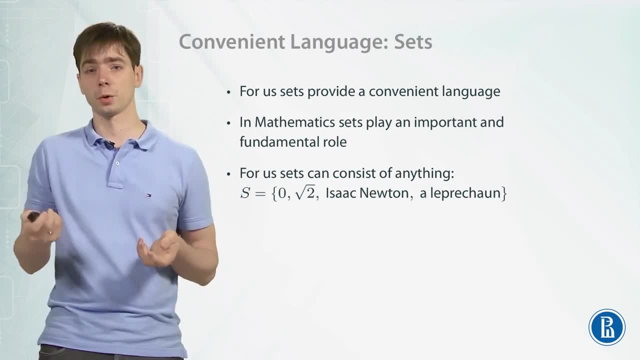 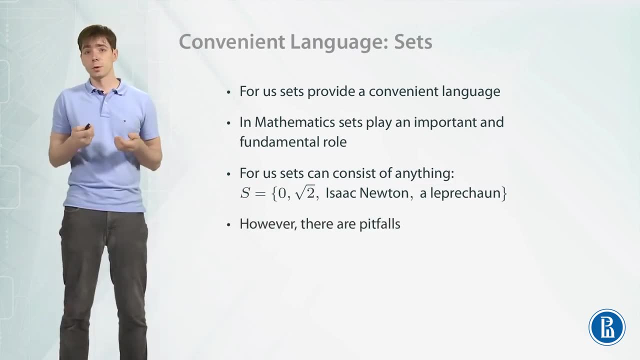 0, square root of 2. Isaac Newton: A leprechaun. This set consists of four elements. Here is the list of them. So this is a legitimate set for us. So in mathematics it is known that there are pitfalls there. 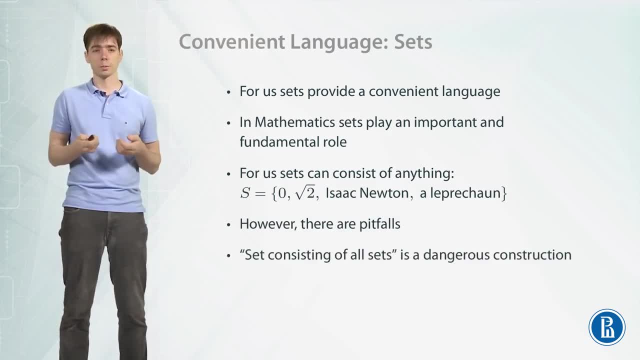 So you cannot just consider anything you want, For example, the construction like this Set consisting of all sets. It is a dangerous construction. You should be very careful with it. But we will not encounter these difficulties in this course And we will not discuss them. 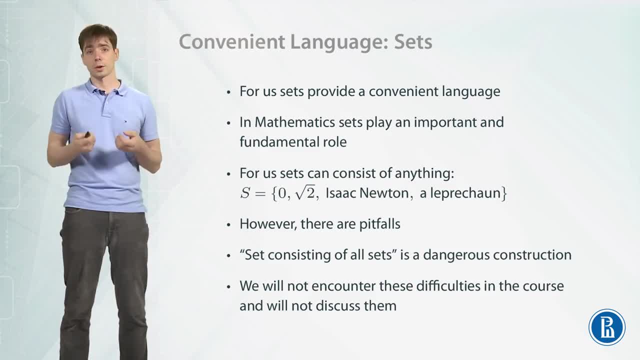 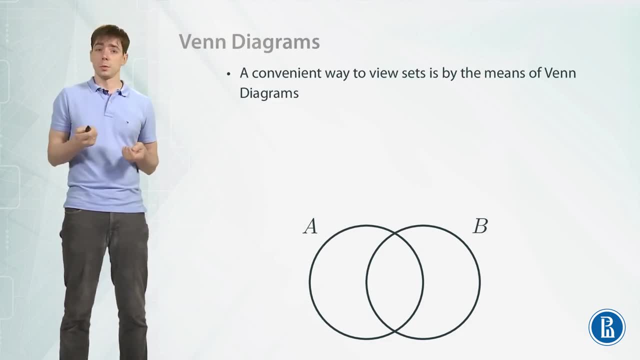 We will not have this problem. For us, set is an arbitrary group of arbitrary elements. Okay, So a convenient way to view sets is by the means of Venn diagrams. So here is a Venn diagram for two sets, And here there are two sets, A and B. 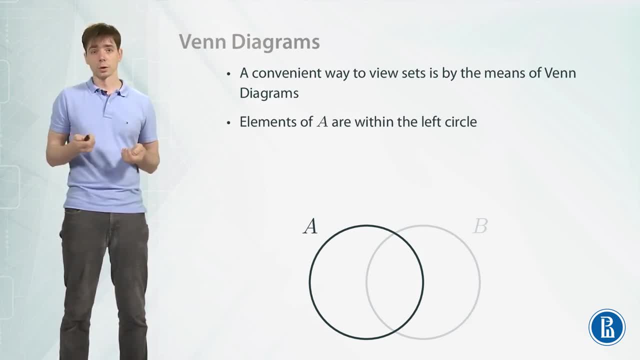 Elements of A are depicted within the left circle. Elements of B are depicted within the right circle. So note that the circles are intersecting And the intersection corresponds to elements that belongs to both sets. So if there are elements that are in both sets, they will be in the intersection of two circles. 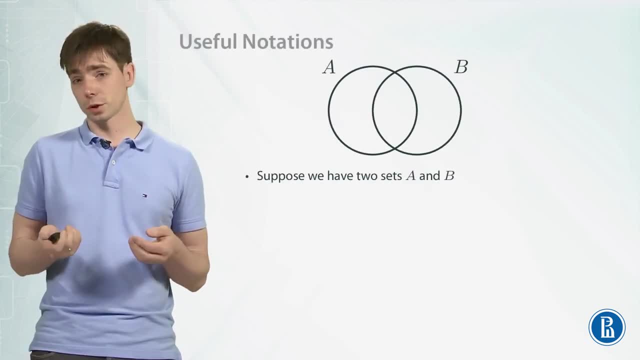 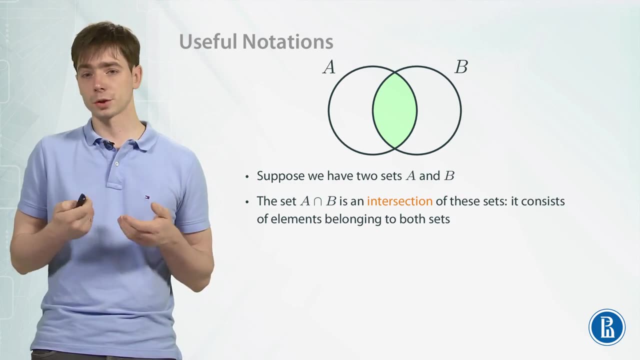 So suppose there are two sets, And here is a picture, And we would like to introduce a couple of operations over sets. First, the intersection of two sets. And the intersection of two sets is again a set And it is a set of all elements that belong to both sets. 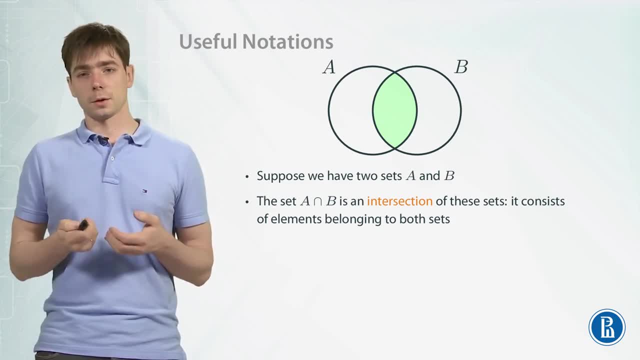 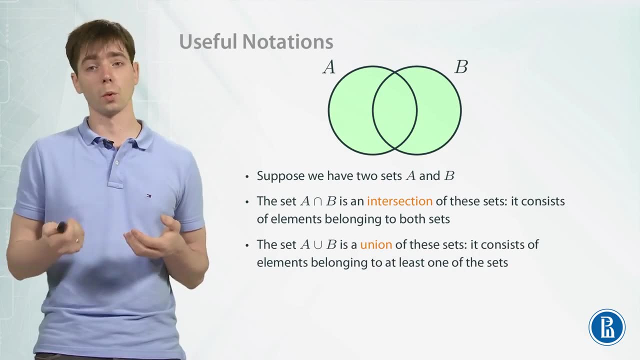 A and B. Next operation is a union of two sets, And this is the set that consists of all elements that belong to either A or B. If you have seen our first course, What is a Proof Note that Recall that we had Boolean logic there? 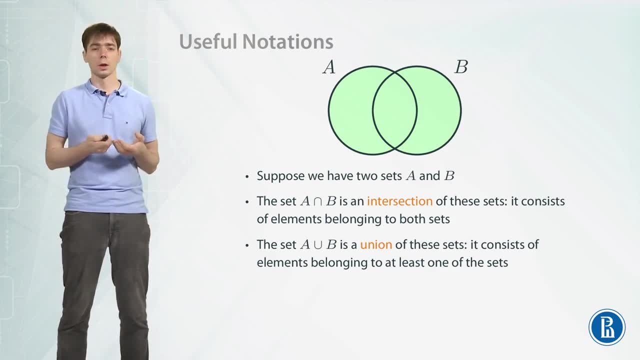 And operations, AND and OR on Boolean variables, And note that operations for intersection and union are similar in their looks By And operations in Boolean logic, And this is And recall also that we have Venn diagrams there as well And the Venn diagram for AND operation looked like that. 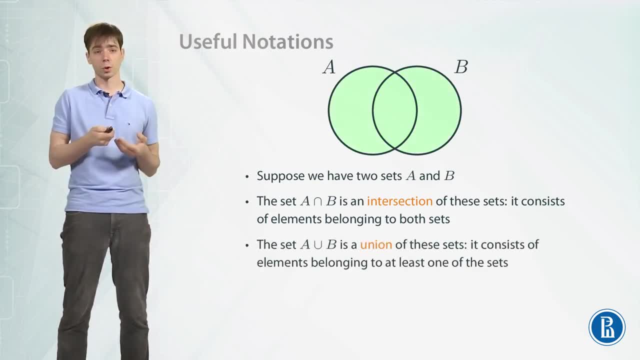 Like for intersection, And the Venn diagram for OR operation looked like the Venn diagram for union. This is not a coincidence. There is a correspondence between Boolean operations and operations over sets. We will not discuss it in details, But there is a 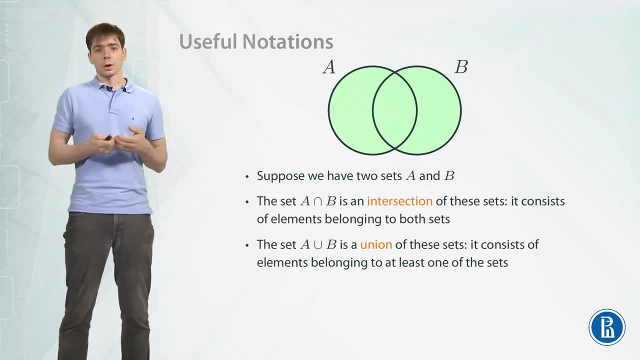 There is a connection there, There is a correspondence. Okay, And the last definition we would like to introduce is the number of elements in the set, Which is denoted like this: Note that the set can be infinite, For example, the set of all natural numbers. 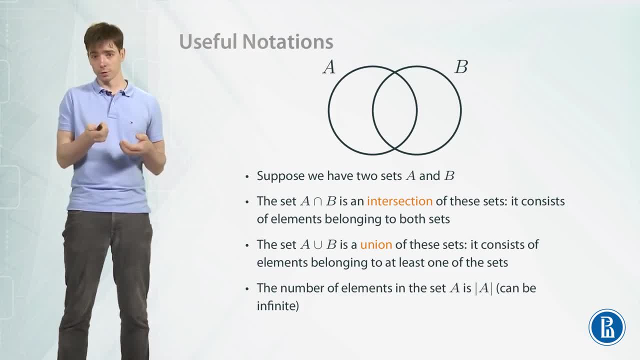 It is an infinite set, So this number, The number of elements in the set, can be infinite. It can also be zero. There is a set with no elements, A so-called empty set. So this is our last notation here. 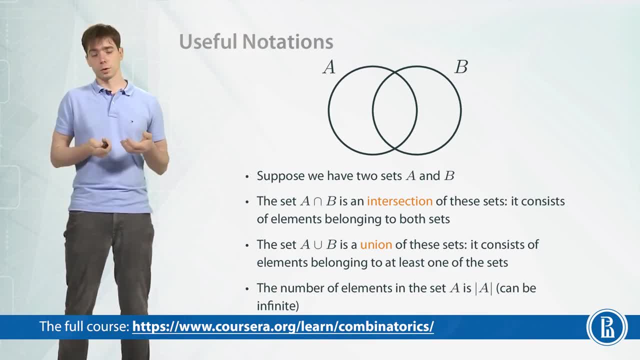 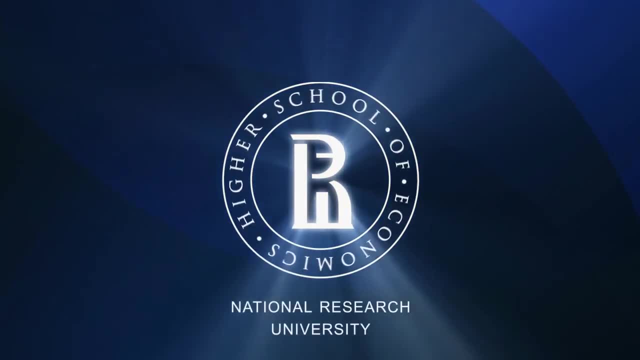 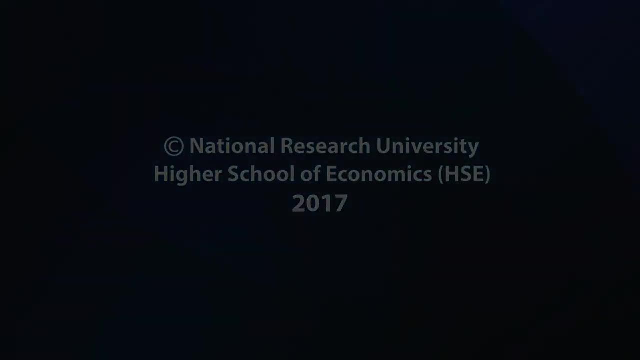 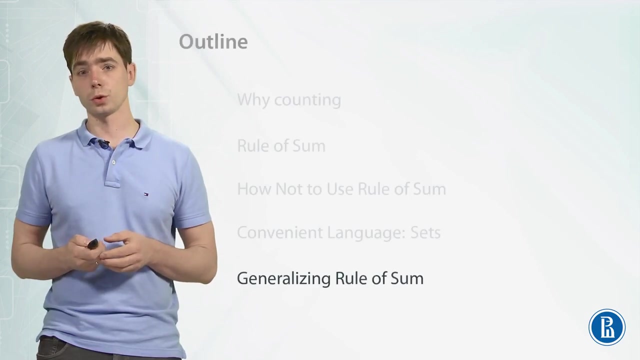 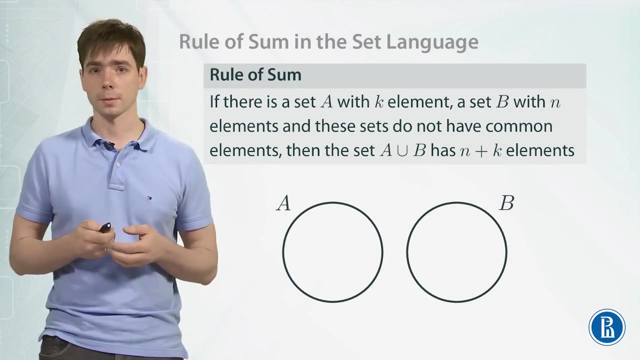 Okay, And now we can proceed back to combinatorics. Okay, Now we are going to generalize our rule of sum a little bit, But first let's state the rule of sum in the language of sets. So in the language of sets this rule sounds as follows: 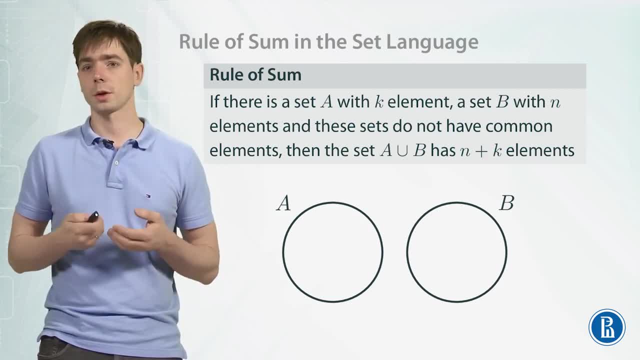 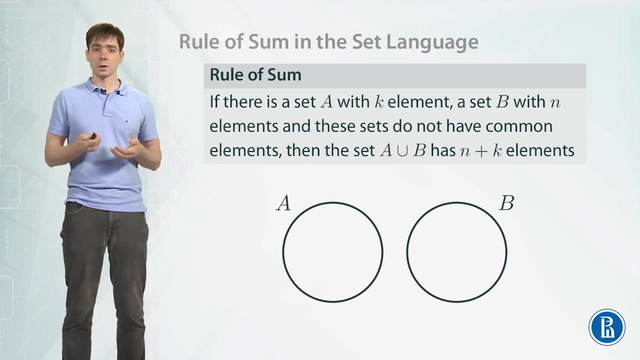 So suppose there is a set with K elements And there is a set B with N elements And what is important, This set do not have common elements. We have seen that this is important before. Then the set, The union of sets A and B, contains N plus K elements. 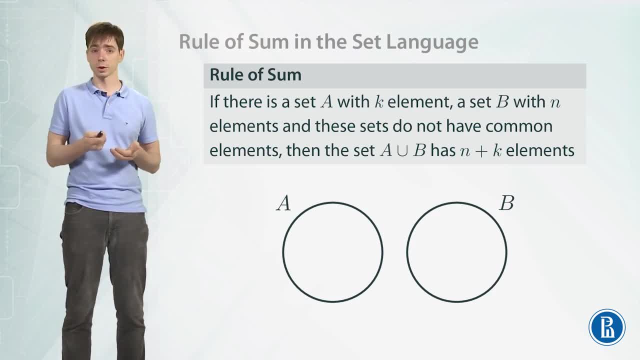 And here is a picture. There is a circle for A, There is a circle for B. They do not intersect, So there are no elements in the intersection. And so here is the set of all elements in the union of A and B. 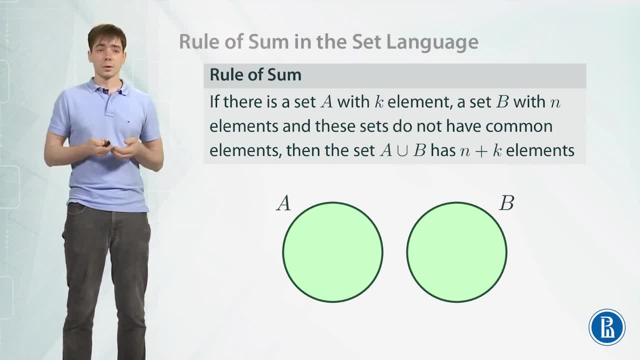 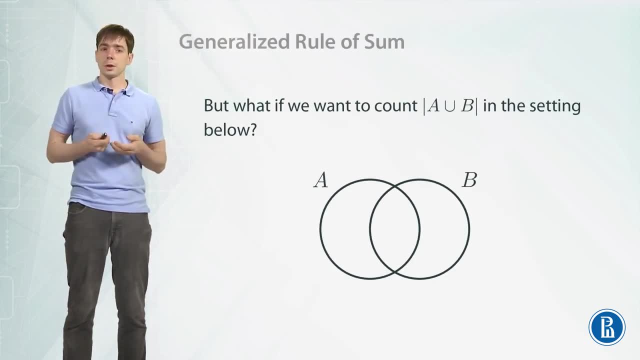 It is denoted by green color. So there are N plus K elements there. So here is the rule of sum. But what if sets A and B are intersecting? Okay, we cannot apply the rule of sum now, But what if we still would like to count how many elements belong to one of the sets A or B? 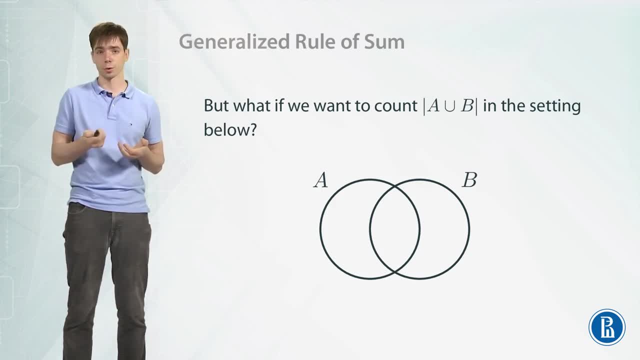 What if we want to count the number of elements in the union of A and B? Okay, let's see what we can do. So we would like to count the number of elements here. Let's see what we can do. Okay, let's start with the rule of sum. 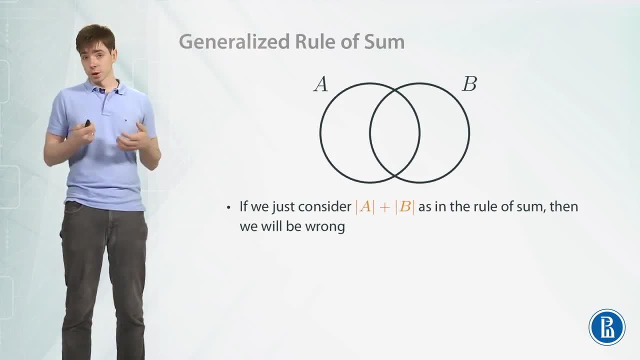 We can just consider the number of elements in the union of A and B. Okay, We can just consider the number of elements in A plus the number of elements in B, Just as in the rule of sum, And we know that the answer will be wrong if there is something in the intersection. 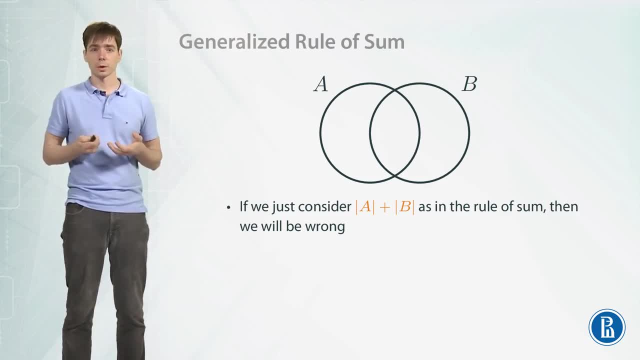 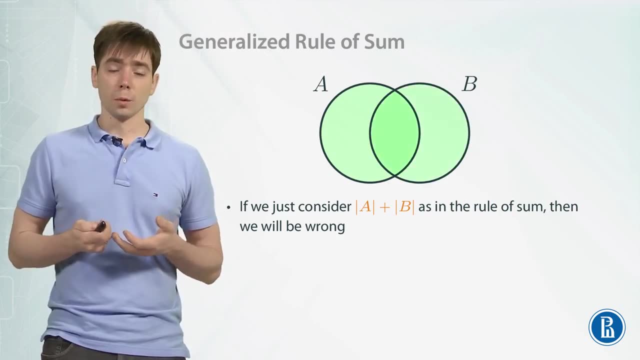 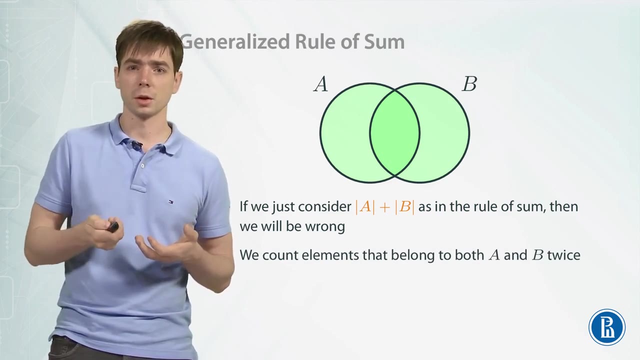 Okay, let's see what we have done here. We have counted all elements of A And then we have counted all elements of B. And why is this wrong? We have counted elements in the intersection twice. Note that the color there is a bit more intense. 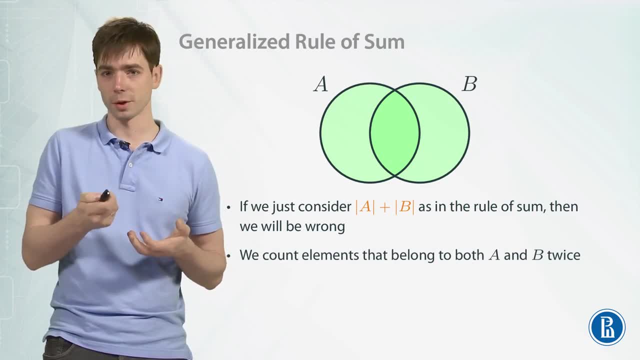 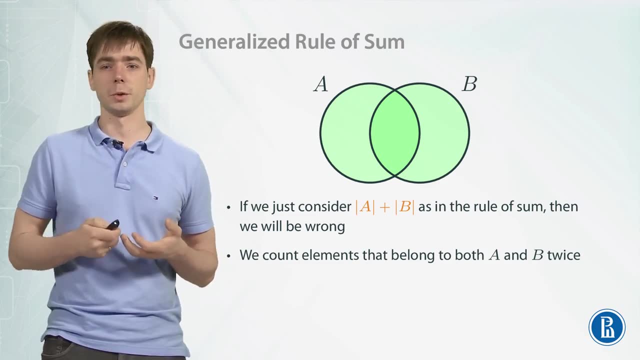 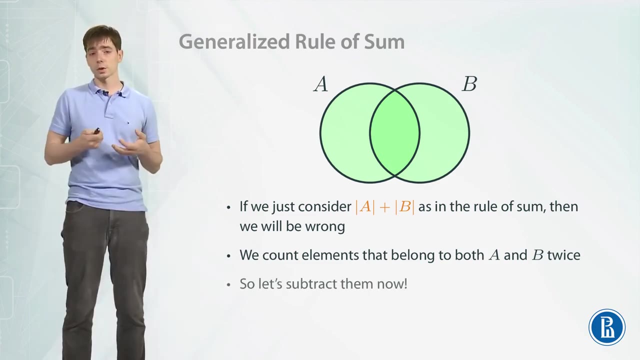 So it denotes that we have counted them twice. We have colored this area first when coloring A and second when coloring B. Okay, now we are wrong, We have the wrong number, But what we can do? Okay, we can just subtract what we have counted twice. 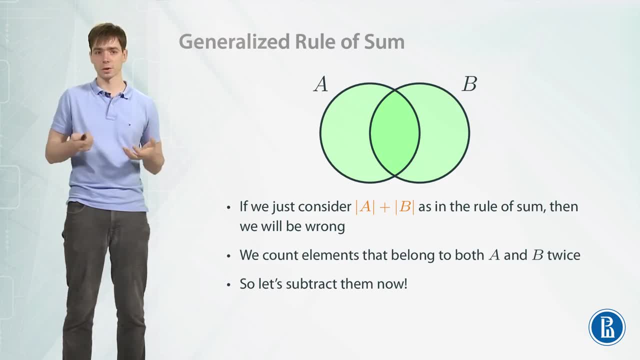 If we counted twice and now we subtract the number of elements there, then we will have the right answer. So that's what we can do. And the number of elements there is just the size of the intersection of A and B. So this gives us the following result: 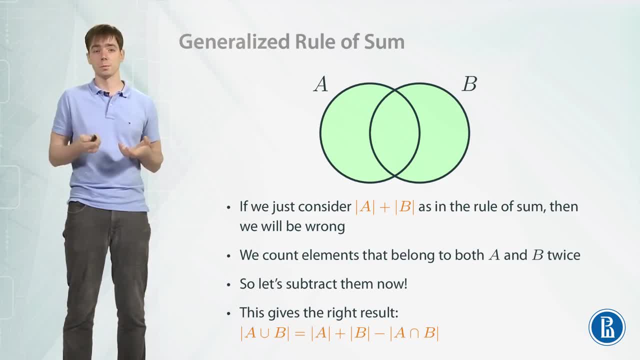 The size of the union of A and B is the size of A plus the size of B minus the size of the intersection. So that's how we still can compute the number of elements in the union, even if the sets are intersecting. Note that the rule of sum is the special case of these equations, when the size of the intersection is zero. 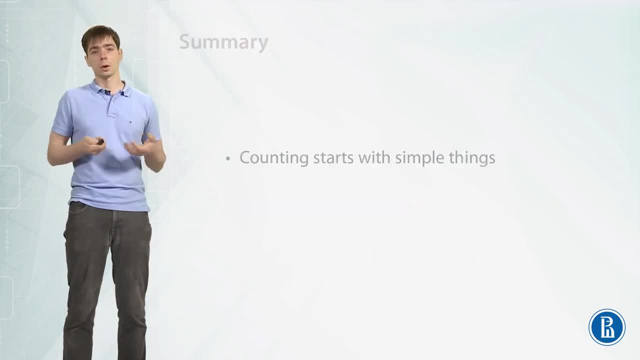 The intersection is an empty set. Okay, let's summarize what we have learned in this lesson. Counting starts with a very simple thing, Just the rule of sum, And we can build everything else from it. But note that even these simple things can be tricky. 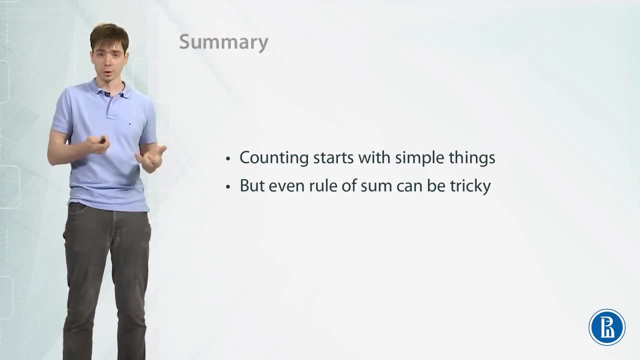 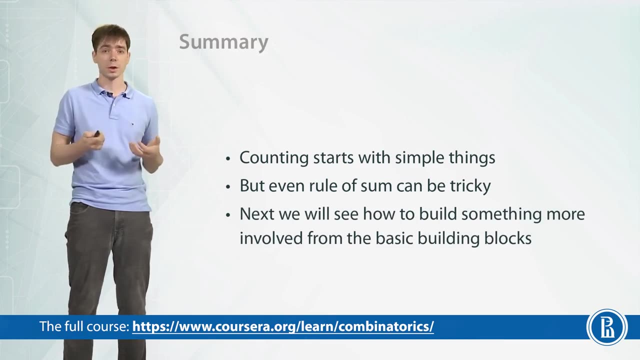 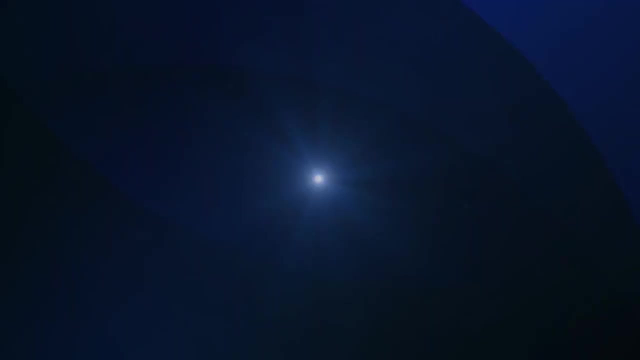 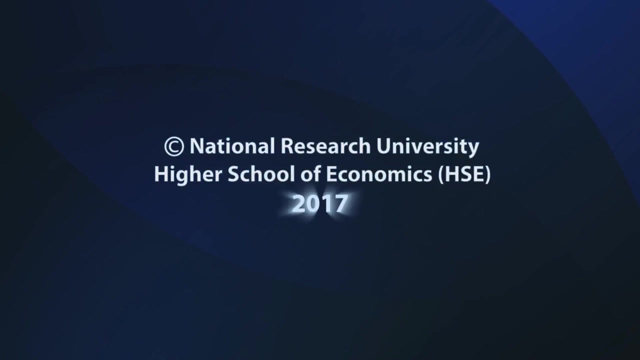 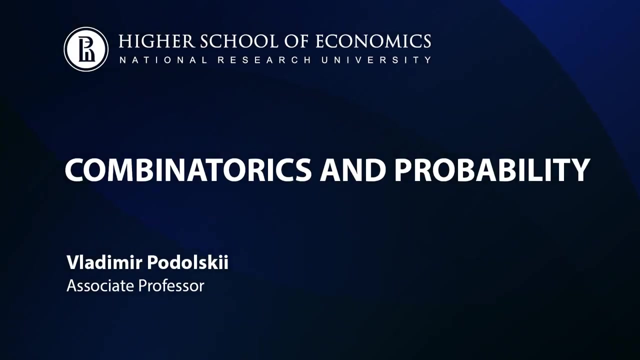 Rule of sum can be tricky. We have to be careful when we are applying it. And next, in the next lesson, we will see how we can build something more complicated, more involved, from the basic building blocks. Hi, I'm Vladimir Podolsky, and today we are going to discuss recursive counting. 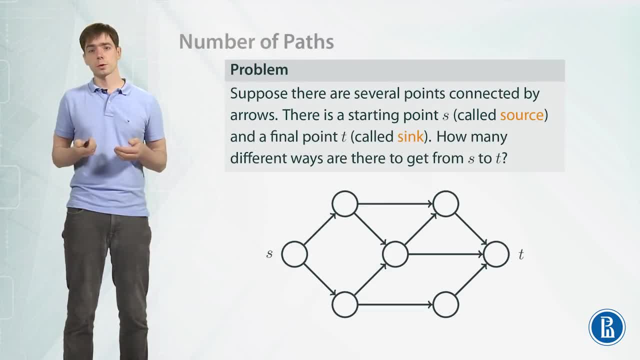 Let's start with the following problem. Suppose there are several points which are connected by arrows, And points are represented by circles. here There is a starting point S, which is called source, And there is a final point T, which is usually called sink. 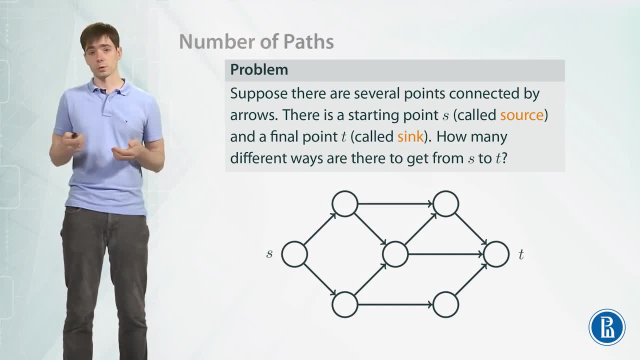 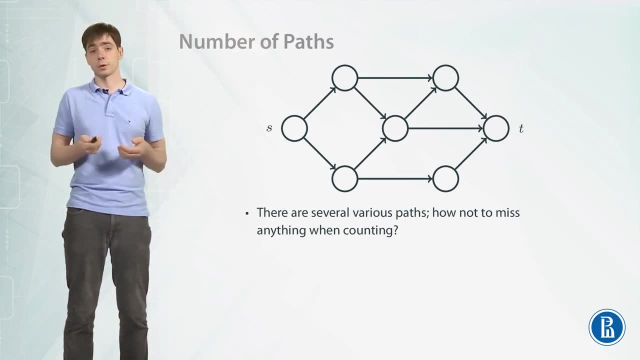 How many different ways are there to get from S to T following these arrows? Okay, let's try to consider this problem. There are several different paths here and they look completely differently. And the main problem if we try to do it by hand. 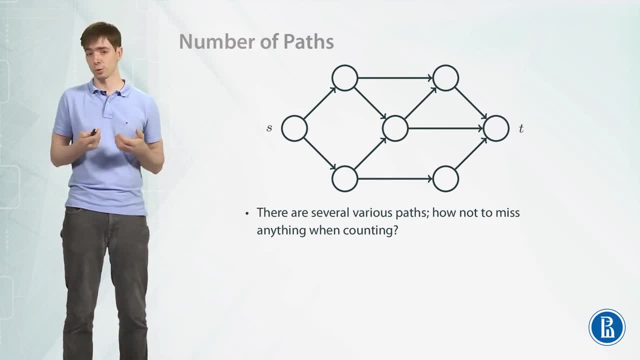 is how not to miss anything when you just list all possible paths. And, by the way, this is one of the advantages of using mathematics here. Mathematics comes with proof, So if you use some formula, then you know it is correct and you know you haven't missed something. 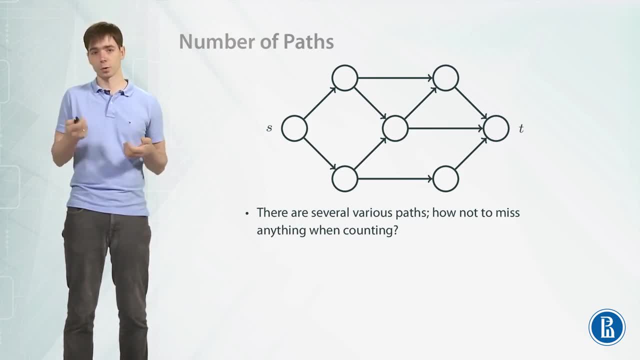 If you try to count by hand, then you can miss something. where you have a long list of paths, It is easier not to notice something, So mathematics reduces the number of places where you can make a mistake. Okay, so what can we do with this problem? 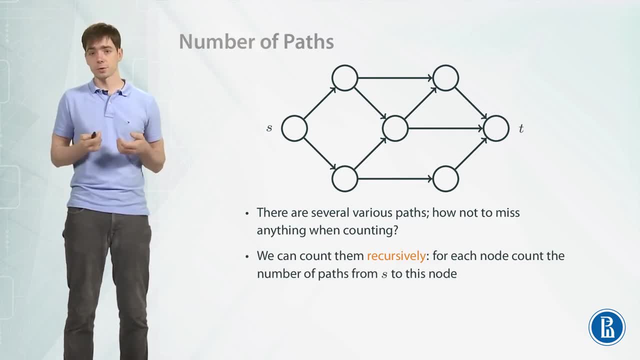 Okay, we can count this number of paths recursively For each node. we will count how many paths do we have to this node from S, And we do it for all nodes, one by one, And on our way we will use the rule of sum. 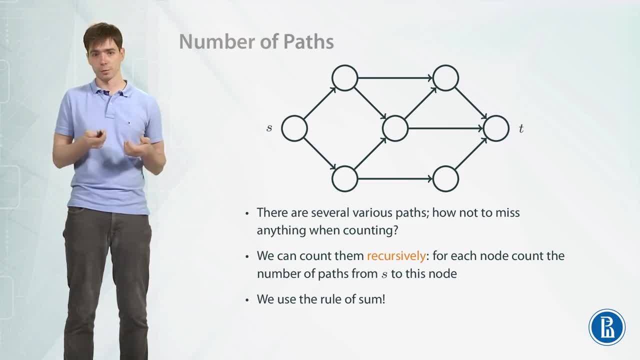 Let's note it. So here we will use our basic building block, the rule of sum. Okay, we will start with the simplest possible node, S. So there is exactly one way to get from S to S: Just do nothing, Just stay there. 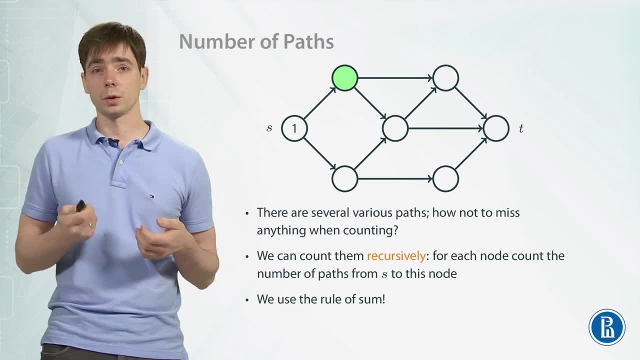 And so the answer is one. Okay, let's consider the next node, This one. There is only one way to get to this node. There is only one arrow incoming to this node, And it goes from S. So there is one way to get to S. 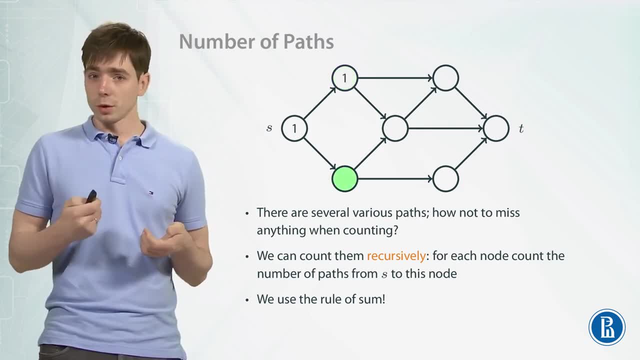 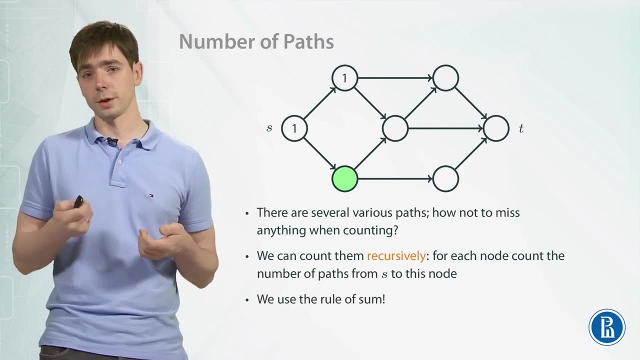 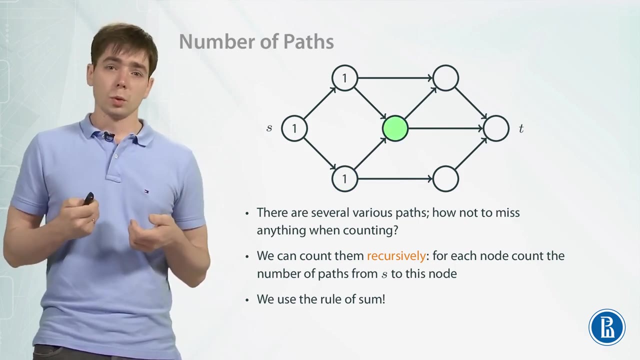 And so there is one way to get here. Here, There is only one arrow which goes into this node, So again, there is only one way to get here from S. Okay, now we get to something more interesting. There are two possible ways to get. 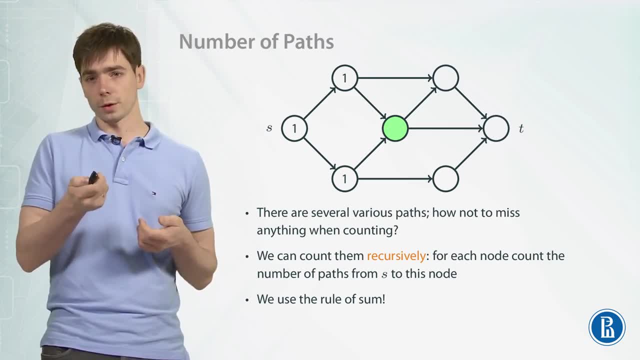 To this node. So we can go here from above and from below, And in both cases there is one possible way to get to the corresponding node, So to the node on the top and the node on the bottom. So we have, to sum up, ways of two types. 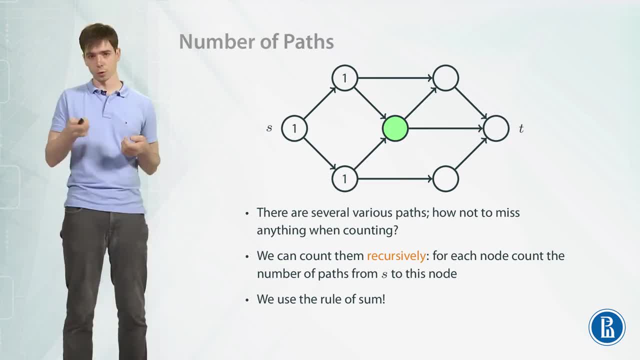 Which go through the vertex above and the paths that go through the vertex below. So we apply the rule of sum And one plus one is two. Okay, let's proceed to the next node. Again, for this node, we have two ways to get here. 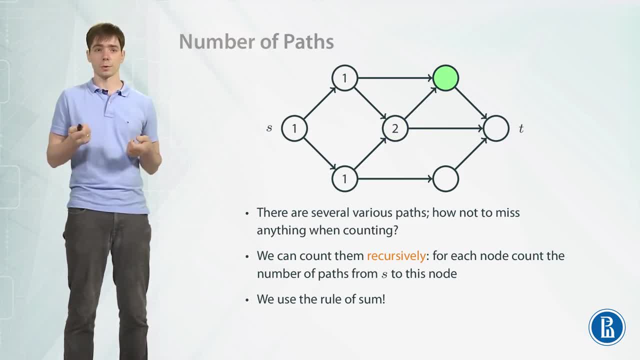 There are paths of two types: The one which goes from the node, which is labeled by one currently, And the other which goes through the node, which is labeled by two. So there are two types of paths here, And there is exactly one path of the first type. 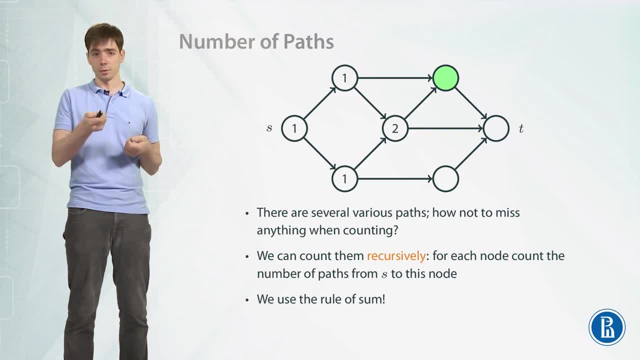 And there are two ways to get to the node in the middle. So there is one path of the first type And there are two paths of the second type. So we have to add this up by the rule of sum And we get three. 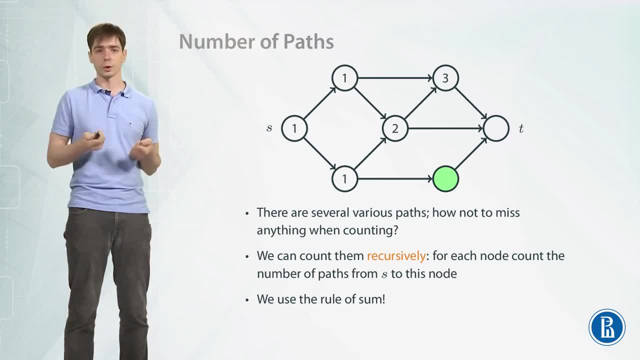 Now, this node is simple. There is only one edge going here And there is only one path to get to the previous vertex, To the previous node. So there is only one way to get here. Okay, and now the final node. There are three edges which go into T. 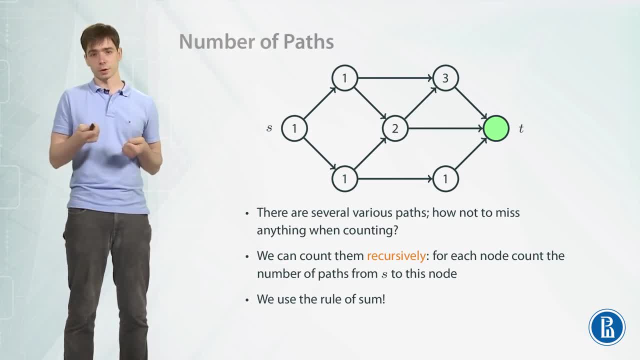 And so there are three types of paths. There are three types of paths by which we can get to T: The one which gets to T from above, The one which gets to T from the middle And the one which gets to T from below. 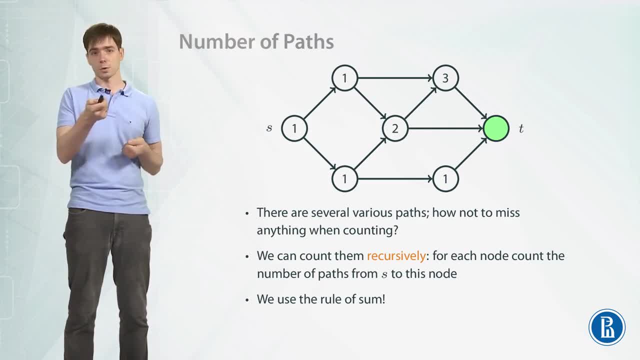 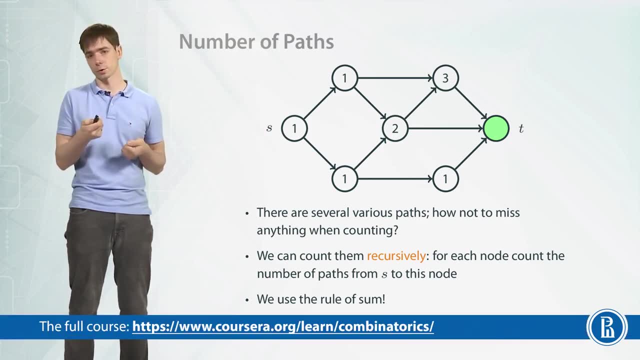 And there are three paths to. There are three ways to get to the vertex above. So there are three paths of the first type, There are two paths of the second type And there is one path of the third type. So we sum this up by the rule of sum. 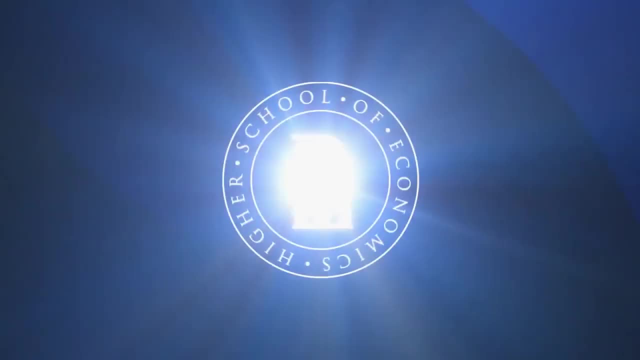 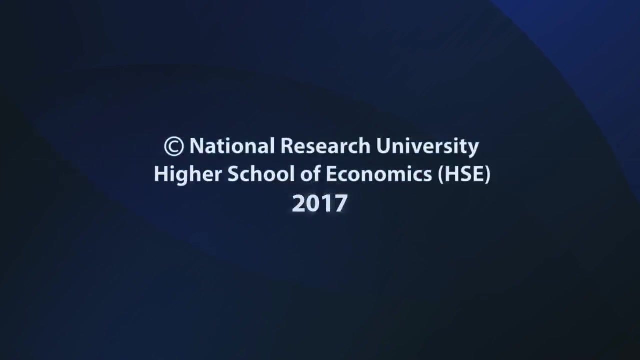 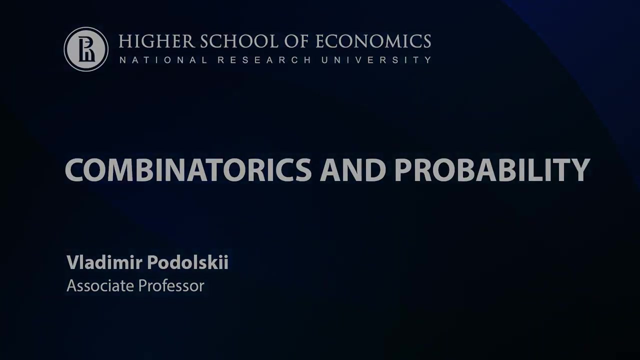 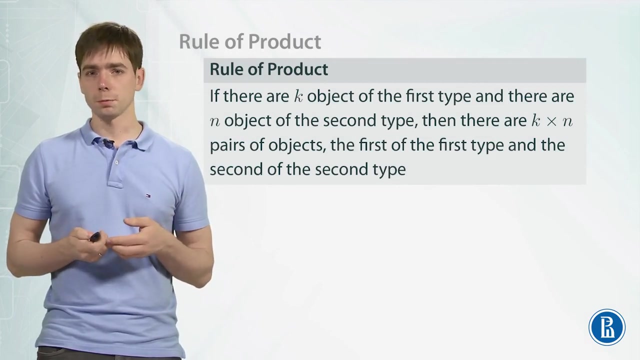 And we get six. Now let's proceed to our second basic rule of counting, Rule of product. Suppose there are k objects of the first type And there are n objects of the second type. Then there are k times n pairs of objects. 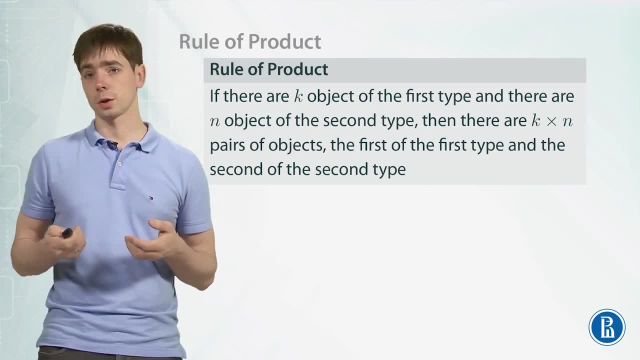 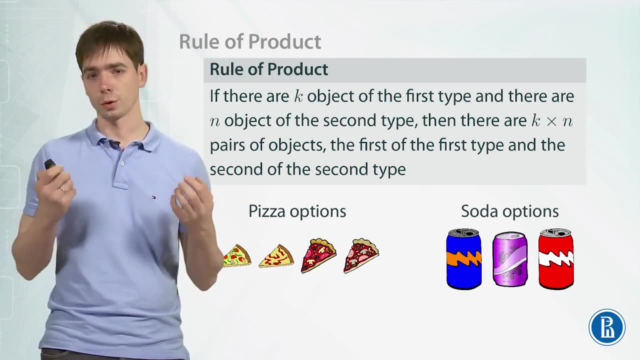 Where the first object is of the first type And the second object is of the second type. Here is a simple example. Suppose you got to some place to eat And there are four options for pizza in menu And there are three options for soda. 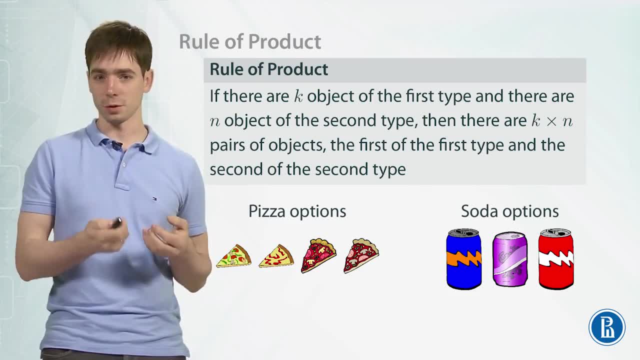 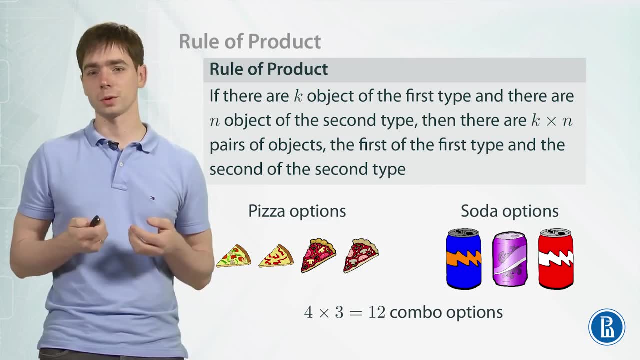 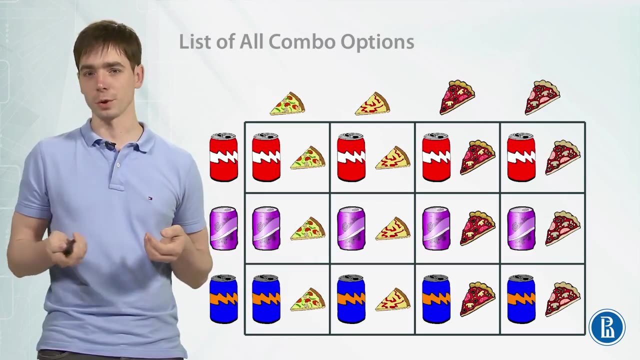 Then you can pick a pair consisting of a pizza And a soda in four times three ways. So there are twelve possible ways to pick your menu, And just for clarity Let's just draw the picture of all of these options here in this table. 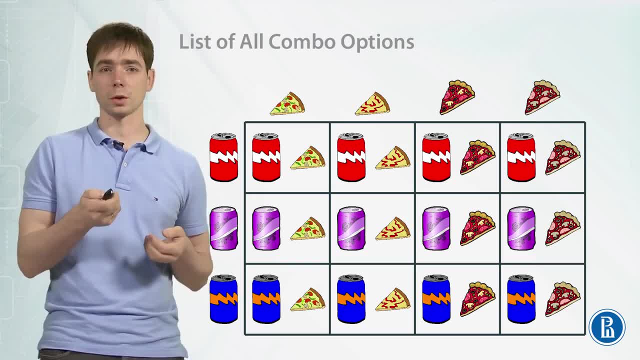 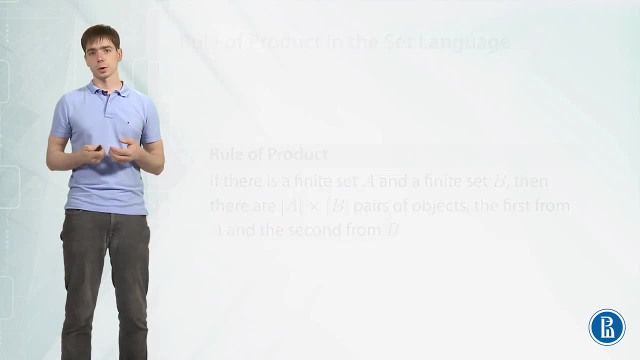 Columns correspond to pizzas And rows correspond to sodas, And in each cell we have the corresponding pair of soda and pizza. So here are twelve options. Let's state the rule of product in the set language. So there is a finite set A. 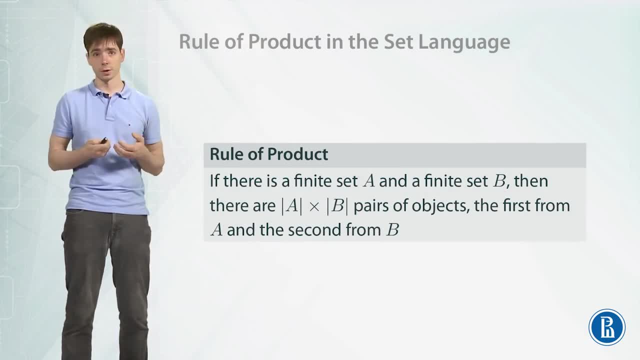 And there is a finite set B. This means that both sets have finitely many elements. Then there are A times B, Meaning the number of elements in A Times the number of elements in B Of pairs of objects. The first object in the pair is from A. 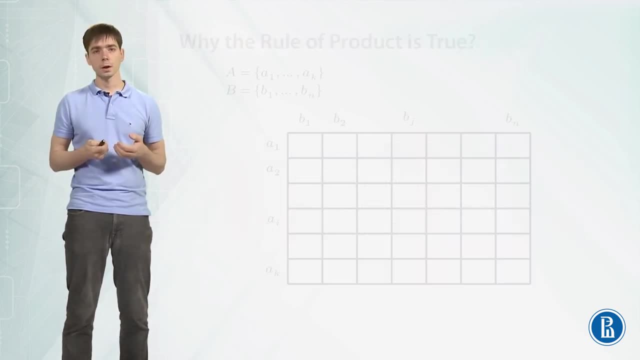 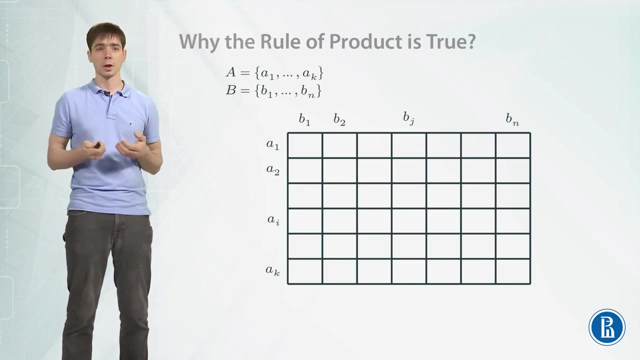 And the second object in the pair is from B. Okay, Let's get some intuition Why the rule of product is true. It also looks rather simple, But still, Let's see. Suppose we have the set A With elements A1 and so on. 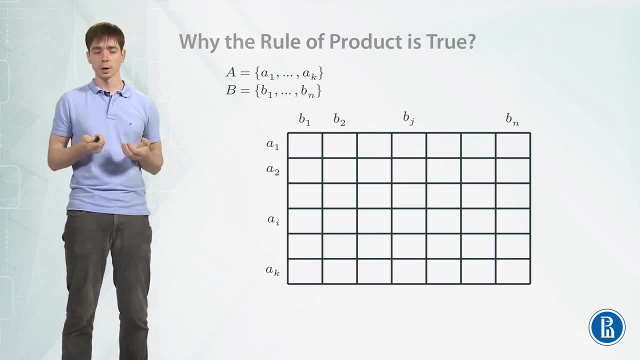 A, K, And there is a set B, B1 and so on, B, N. And let's draw the same table we have drawn in our previous example. Let's enumerate all columns by elements of B And let's enumerate all rows by elements of A. 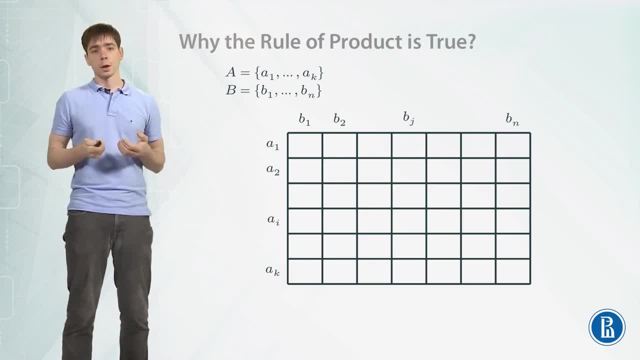 So we have N columns and K rows And in each cell of the table, In cell on the intersection of the row E, I and the column J, We place the pair A- I and B- J And then note that the number of all pairs is the same as the number of cells in this table. 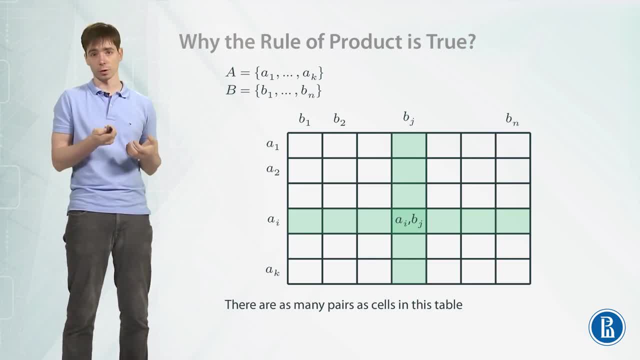 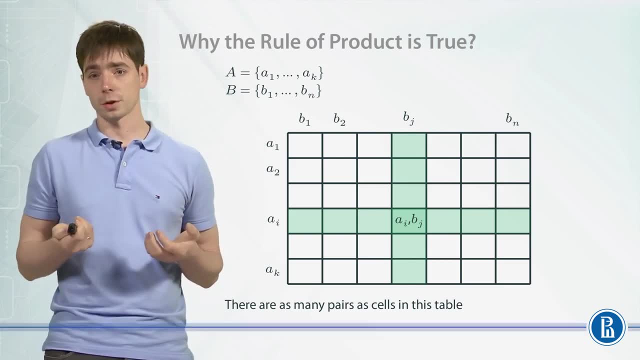 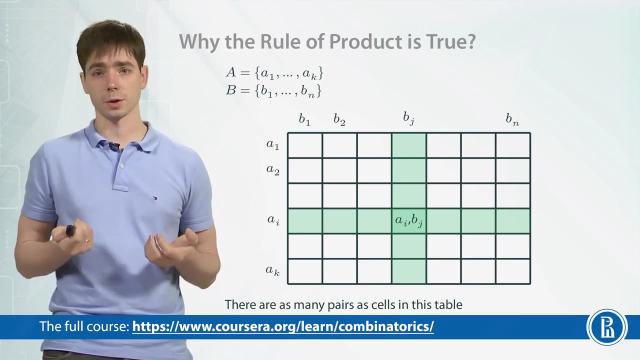 And how can we count the number of cells in the table? We can just multiply the number of columns by the number of rows, Rows, Rows. So the number of pairs is the same as the number of cells in the table. So to count the number of pairs is the same as to count the number of cells in the table. 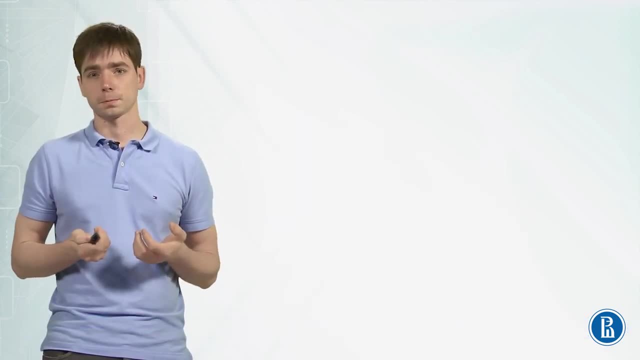 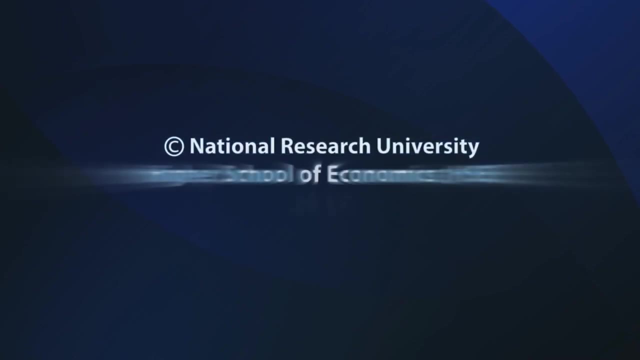 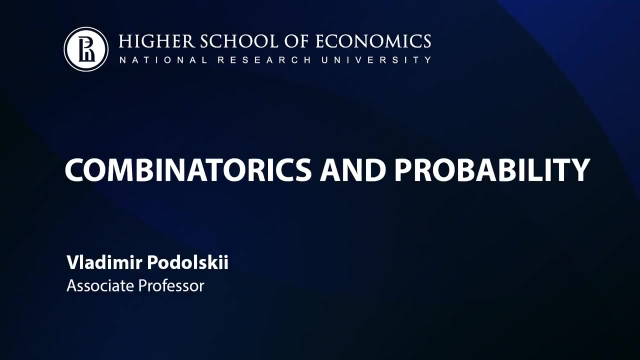 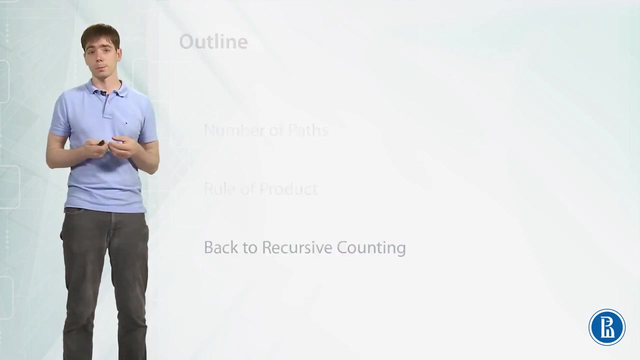 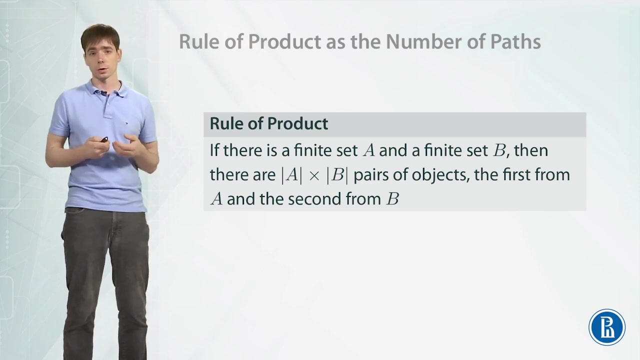 So that's why the rule of product is true. In the beginning of this lesson, we discussed how we can count the number of paths in the picture with nodes and arrows recursively. Let's try to look at the rule of product from this point of view. 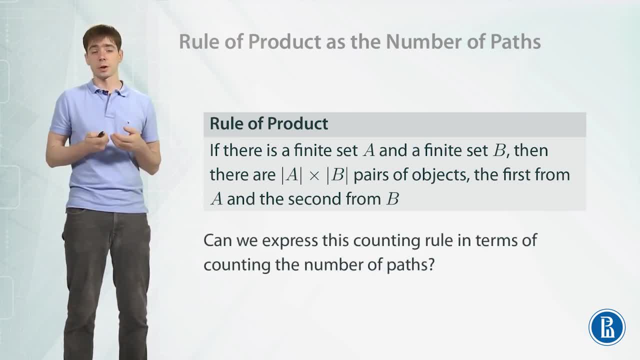 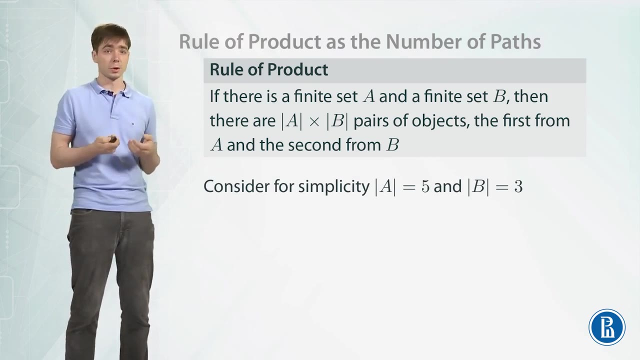 So here is the rule of product, And let's see whether we can express this rule in terms of counting paths in some picture with nodes and arrows. Okay, so here is the rule of product And let's consider the following example, just for simplicity of the presentation. 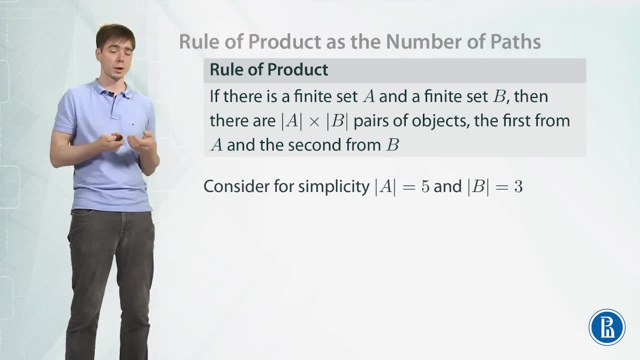 It doesn't matter really, but just let's fix some numbers. Suppose the size of A, the number of elements in A is 5 and the number of elements in B is 3.. And let's consider the following picture. We have three nodes: S, T and the node in the middle. 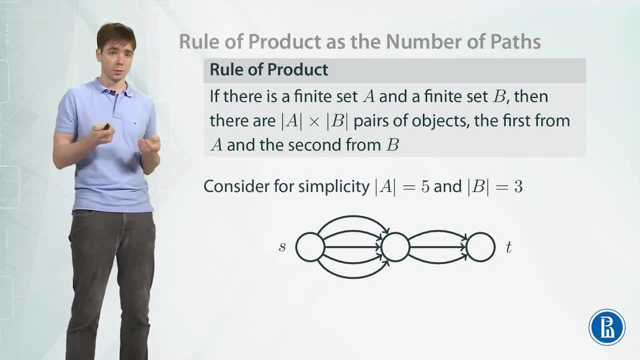 There are five arrows going from S to the middle node And there are three arrows going from the middle node to T. Okay, and let's count how many nodes, that Five arrows correspond to the size of A and three arrows correspond to the size of B. 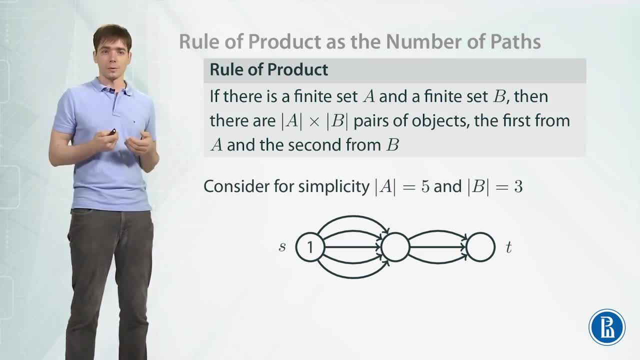 And now let's count. how many paths do we have in this picture? There is only one way to get from S to S, which is just stay where we are. There are five ways to get from S to the middle node. We can pick one of the five arrows from the middle node. 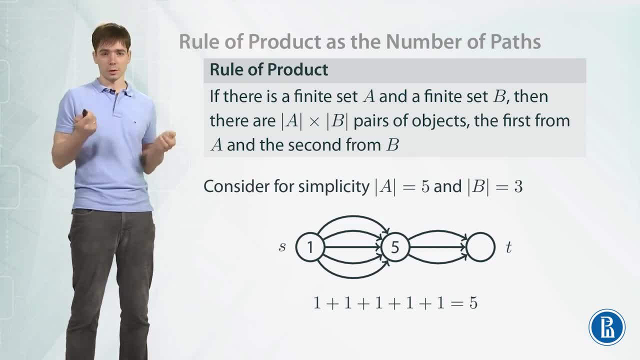 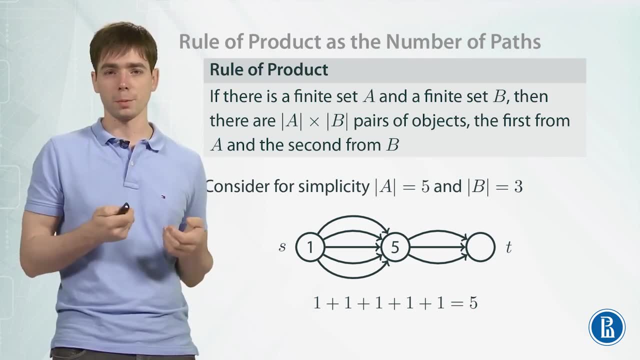 And okay, if you recall how we did it before. so we have to apply rule of sum. There are five types of paths, one path of each type, So we add one to itself five times and we obtain the result five. Now let's proceed to the node T. 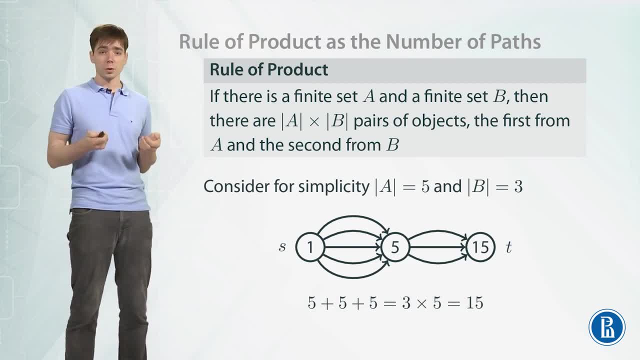 There are three edges going to T. So there are three types of paths that goes to T, One for each edge in going to T, And there are five ways to get to the middle node. So there are five paths of each type. So we add five plus five plus five, which is three times five, which is fifteen. 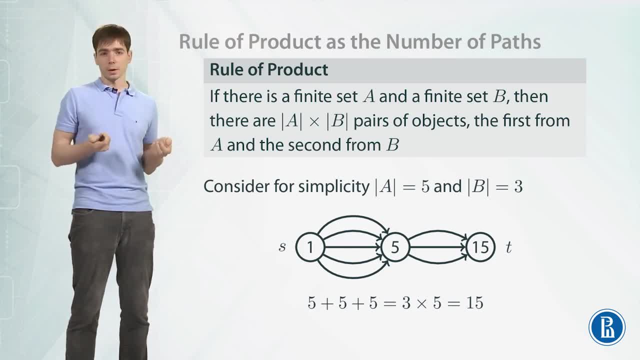 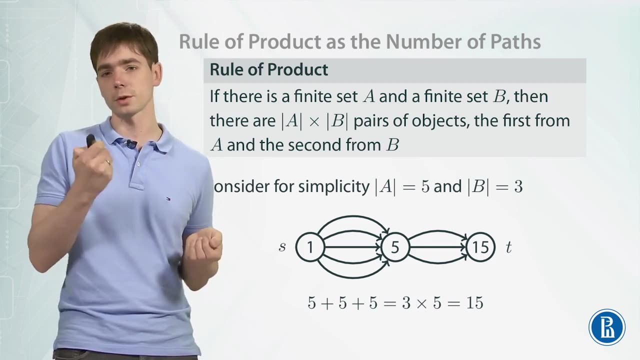 So we have fifteen ways to get from S to T, And okay, and this corresponds to the rule of product. Indeed, if you look at this path, what does it do? Let's recall our example. A is the choices of pizzas. say pizza, 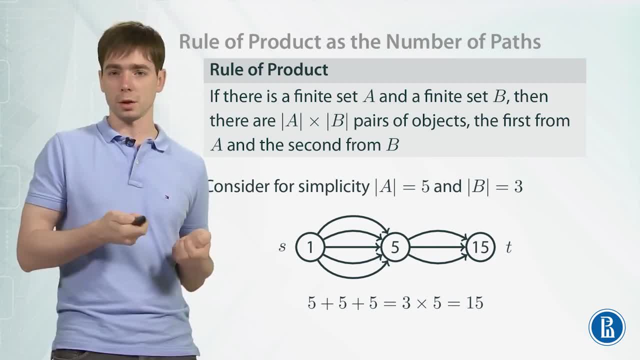 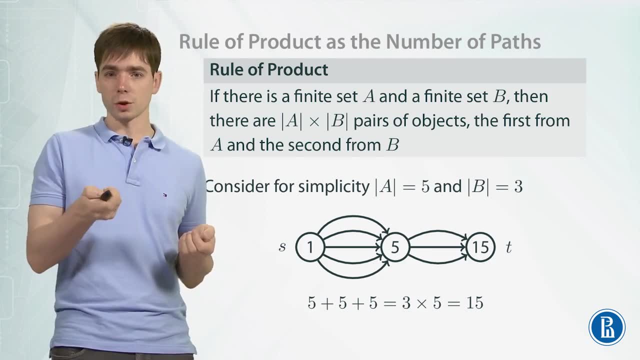 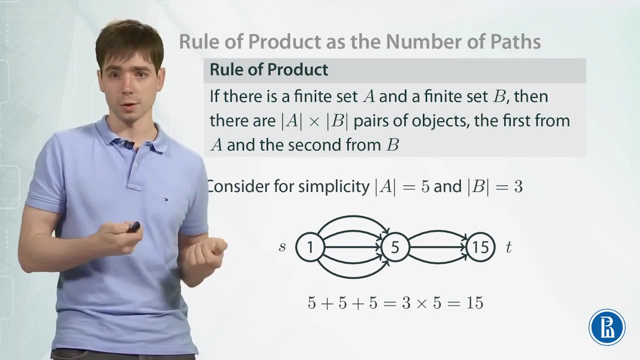 And B is the set B of our options for soda. So each path from S to T consists of two steps, And on the first step we pick an edge from A And this means that we pick our option for pizza. And on the second step, we pick one of the edges corresponding to A. 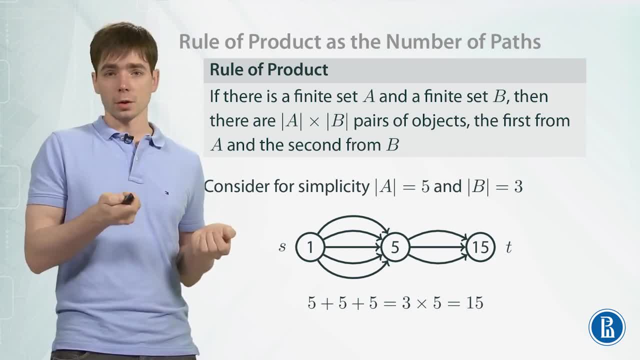 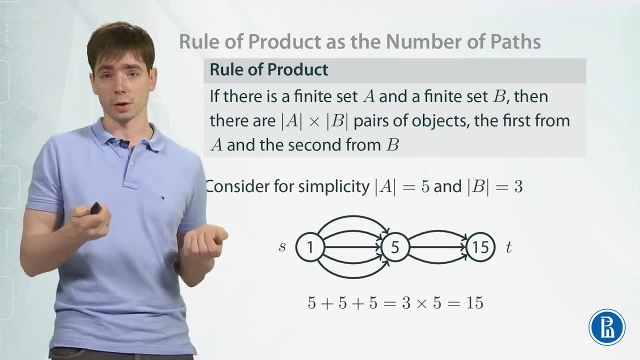 And on the third step we pick one of the edges corresponding to B. So here we pick our choice of soda. So this path exactly corresponds to pairs of where the first element is from A and the second is from B. This path corresponds to pairs of elements and A and B. 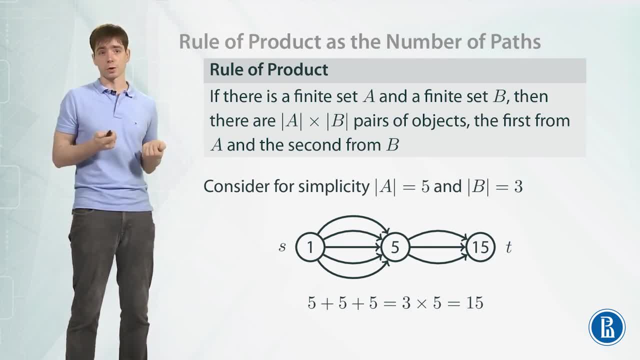 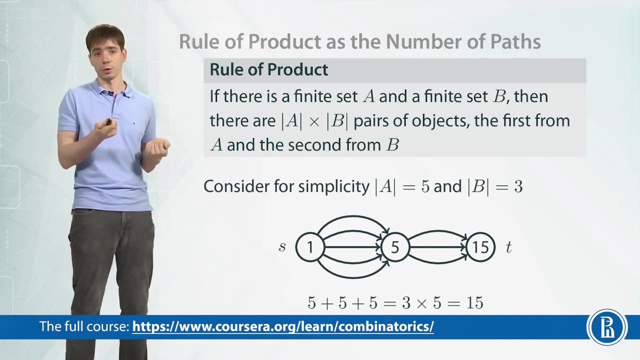 And so this picture exactly represents the rule of product. In particular, we see that to show the rule of product, all we need is the rule of sum, And that's exactly the only thing that we use when we count the number of paths in this picture. 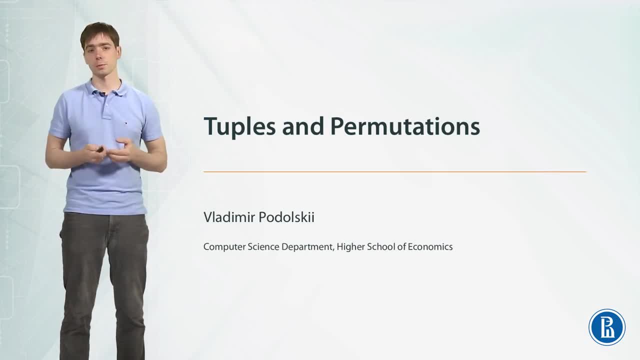 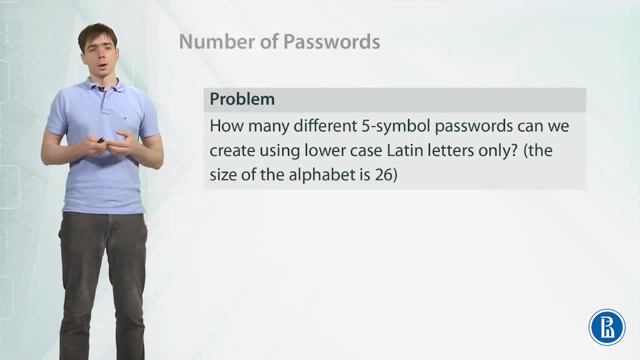 Hi, I'm Vladimir Podolsky, And today we are going to discuss how to compute tuples and permutations. Let's start with tuples And let's consider the following problem: How many different five-symbol passwords can we create if we can use only lowercase Latin letters? 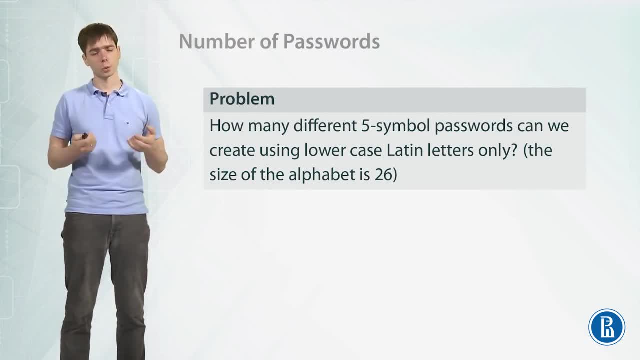 And so the size of the alphabet is 26.. So how many passwords are there? And it turns out that to solve this problem we need only the rule of sum And that's it. But we need to solve this problem step by step. 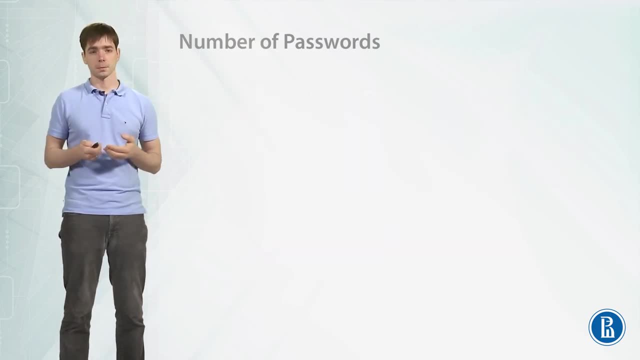 And we should apply the rule of sum, The rule of sum step by step. So let's see how to do it. And let's start with not five-letter password, but just with one-letter password. Then clearly, there are 26 options for one letter. 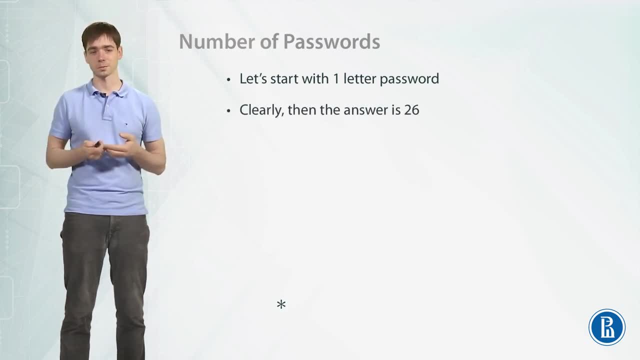 And so there are 26 possible passwords of one letter. So this is not much. Okay, let's proceed to two letters. Now we have two letters And we have 26 options to pick each of them, And this is exactly the setting for the rule of sum. 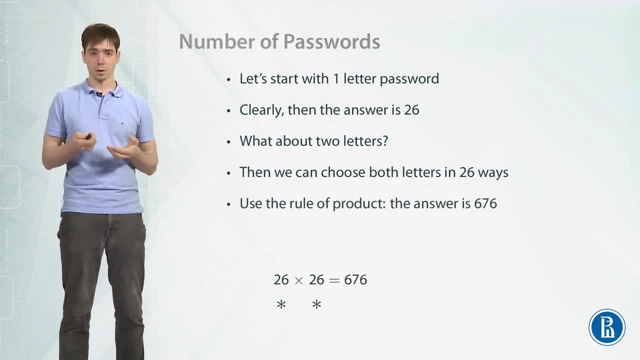 We need to pick the pair of objects. The first one we can pick in 26 ways, And the second one we can pick in 26 ways as well. So the rule of product tells us that there are 26 times 26 pairs. 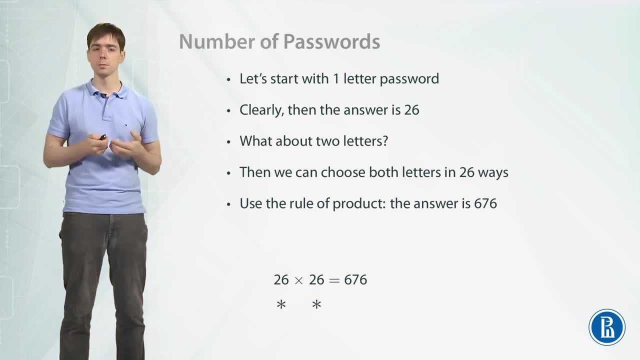 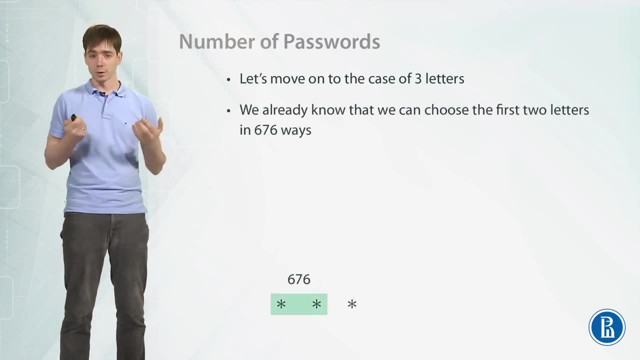 This is 676.. Okay, let's proceed to third letters now. And what we have already known from the previous calculations is that we can pick the first two letters in 676 ways. Okay, now we can pick the third letter in 26 ways. 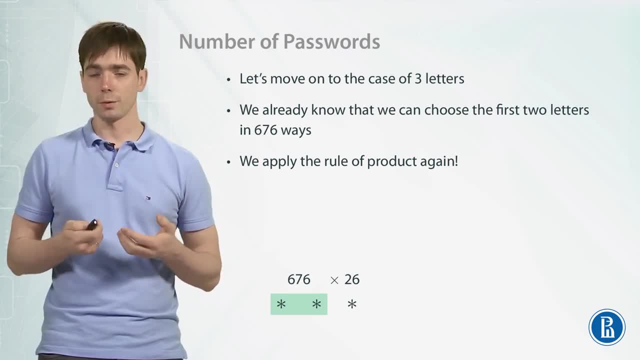 So we can apply the rule of product again. Now, the element of the first set is already the pair of the first two letters, And the element of the second set is the third set. Okay, And the element of the second set is the third letter. 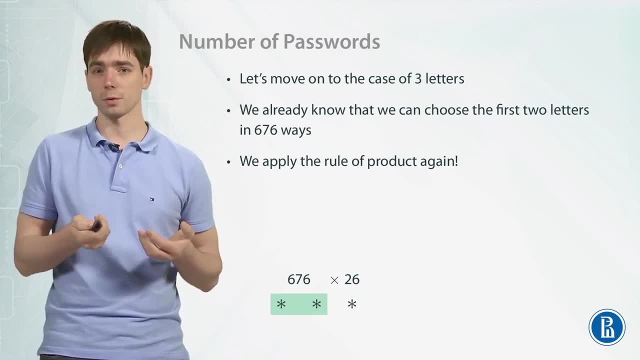 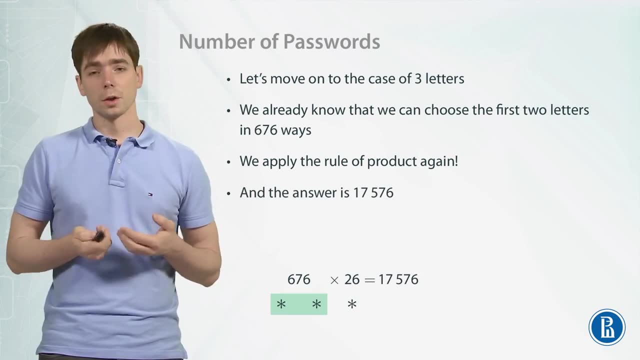 So we have to multiply the number of elements in the first set the number of elements in the second set. So we multiply 676 times 26.. And here is the answer. That's already something. Again, not a lot. There are not many passwords of three letters. 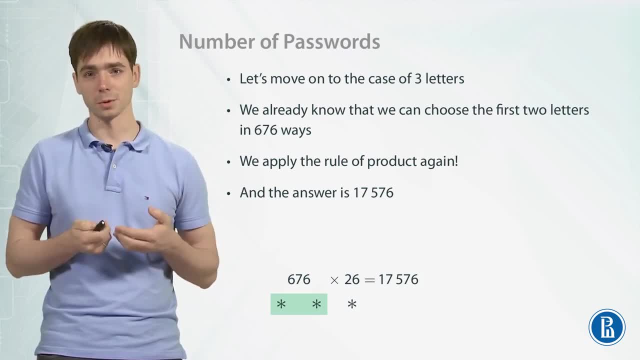 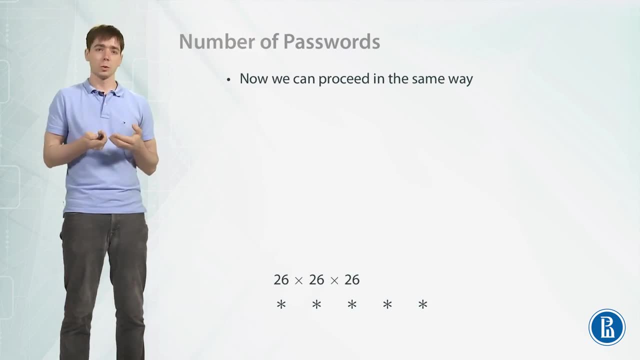 But already we have some considerable number. Okay, let's proceed further And we can just argue by the same way. We now know that the number of passwords, the number of sequences of three letters- We have already calculated the number of sequences of three letters. 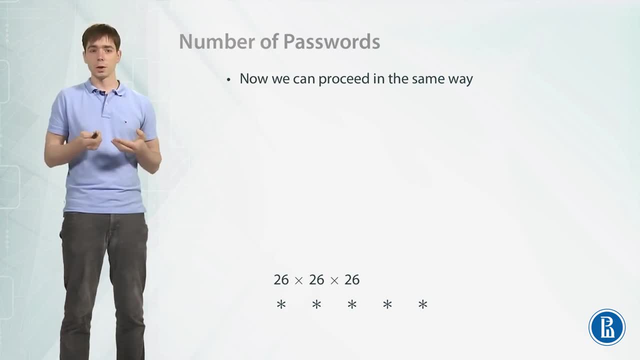 It is 26 times 26 times 26.. We can pick the fourth letter in 26 ways. So now we can pick, So we can apply the rule of sum again. The element of the first set is a triple of the first three letters. 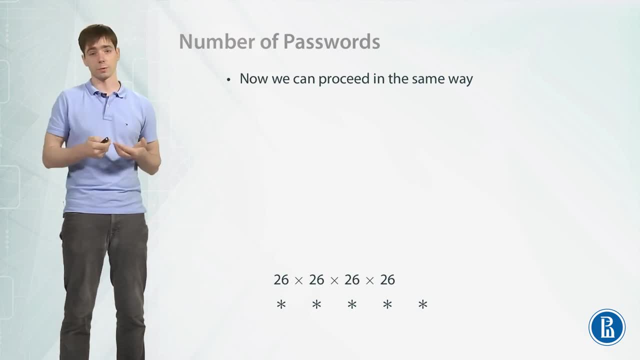 And the element of the second set is the fourth letter. So now for four letters, we have 26 times 26 times 26 times 26 possible passwords, And we make this step again. So for five letters we now have 26 multiplied by itself five times. 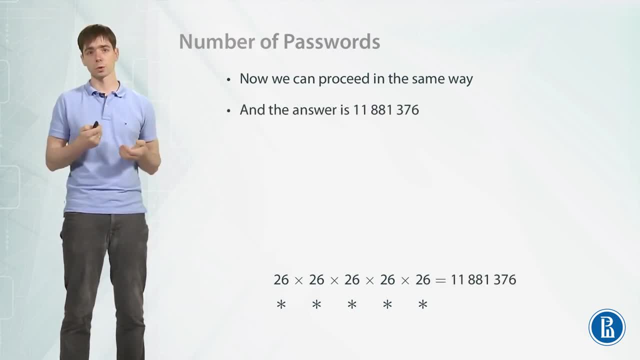 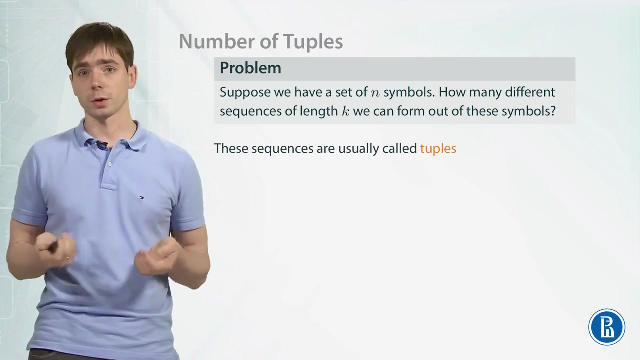 And this is this number. So this is how many passwords we need to. So we have, If we are only allowed five letters And we can only use lowercase Latin letters. Okay, so we have shown this argument on some specific example, But this is a general argument. 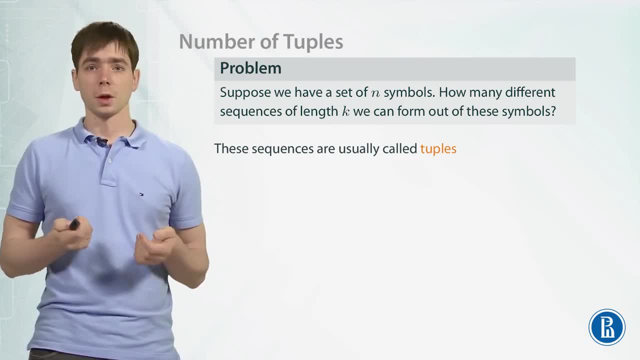 Suppose now we have the following setting: Suppose we have a set of n symbols. So we choose from n symbols now And we ask the following question: How many different sequences of length? How many different sequences of length? How many different sequences of length k? 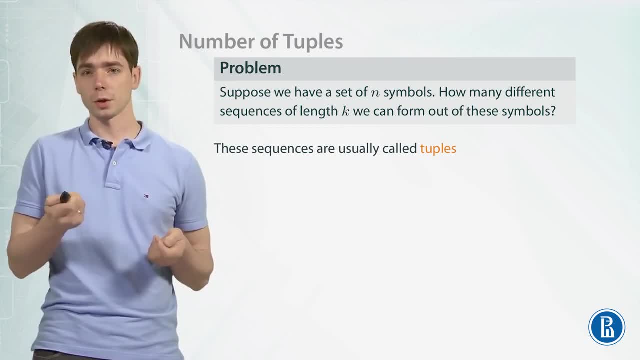 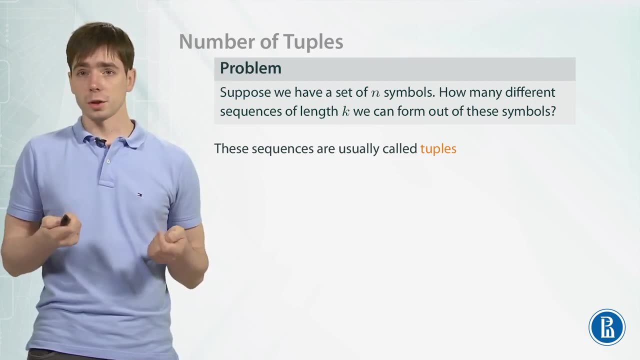 We can form out of these n symbols. So n and k are parameters Here. they can be anything. These sequences are usually called tuples, And this is the first standard setting we have to consider in combinatorics. This is an important setting. 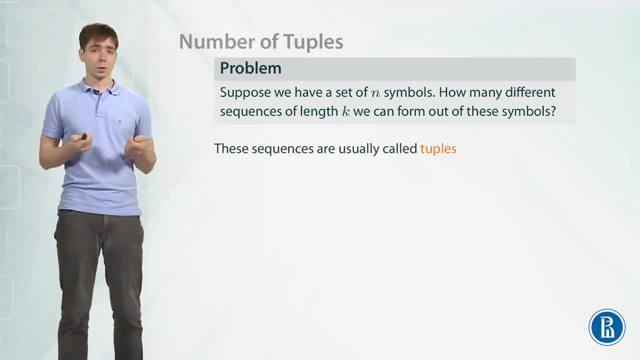 And we will use it later on. Okay, So Let's see, We can just apply the same argument. Just instead of 26 for n and 5 for k, We can now have arbitrary parameters. Let's quickly go through this argument again. 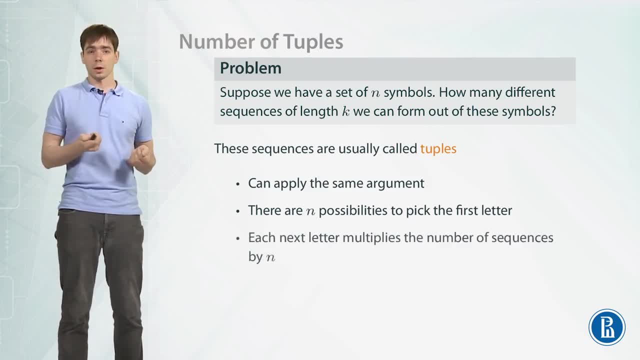 There are n possibilities to pick the first letter, And for each next letter there are again n possibilities. So we apply the rule of product repeatedly, And each time we multiply by n. So in the end the answer is the product of n by itself. 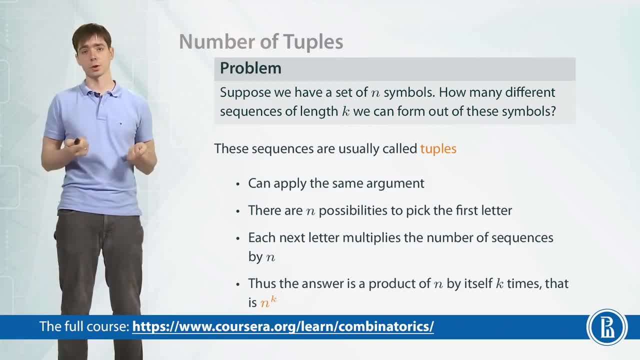 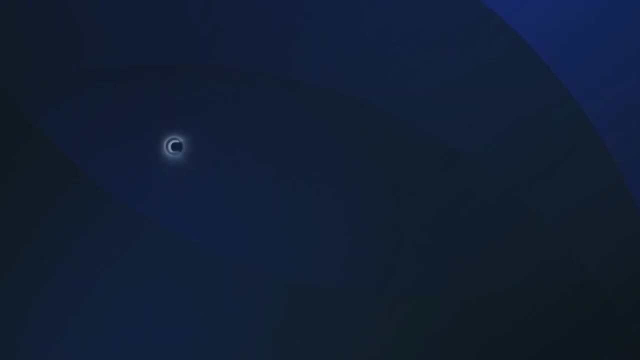 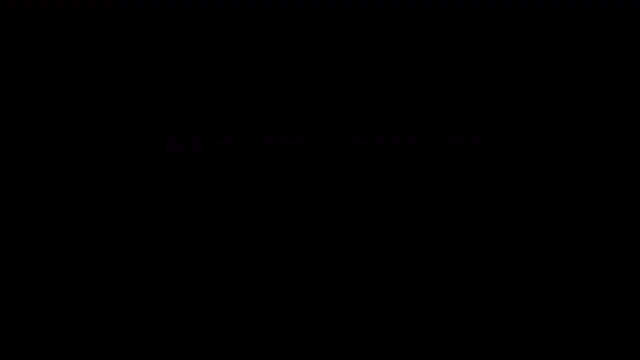 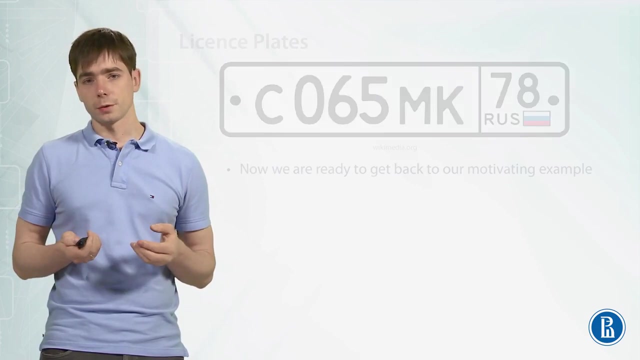 k times, That is n to the k. So this is the answer in general form. So This is the answer in this standard setting of computing tuples. Now we are ready to get back to our motivating example from the beginning of this lecture. 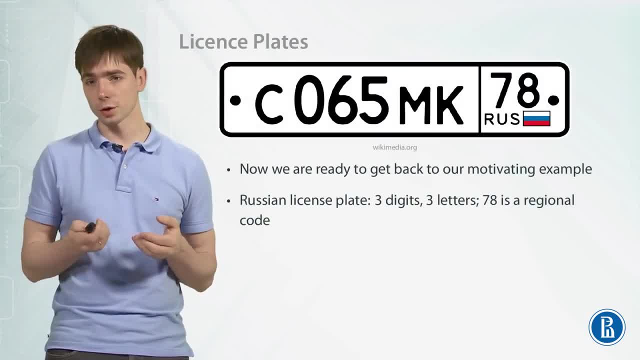 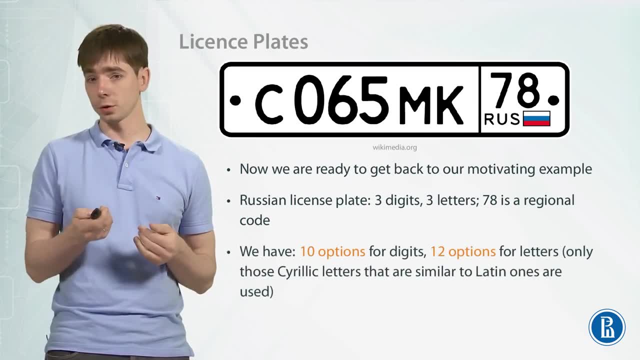 Consider Russian license plates. There are 3 digits there, There are 3 letters And 78. here is the original code. So we have 10 options for each digit, from 0 to 9.. We have 12 options for letters. 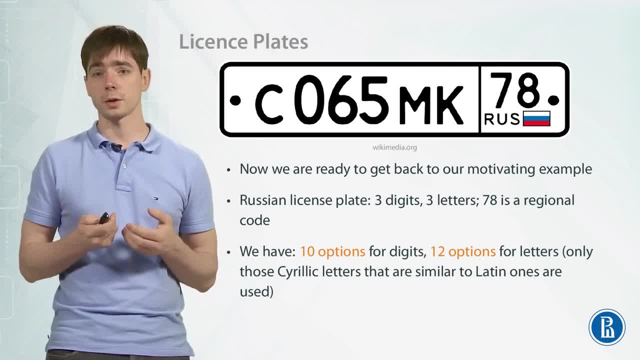 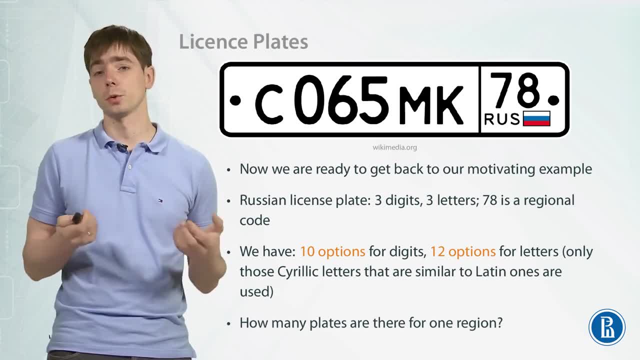 This is because we can use only those Cyrillic letters that are similar to some Latin letters. And now, how many plates do we have for a certain region? How many possible plates do we have? Okay, Let's see. For each digit, we have 10 options. 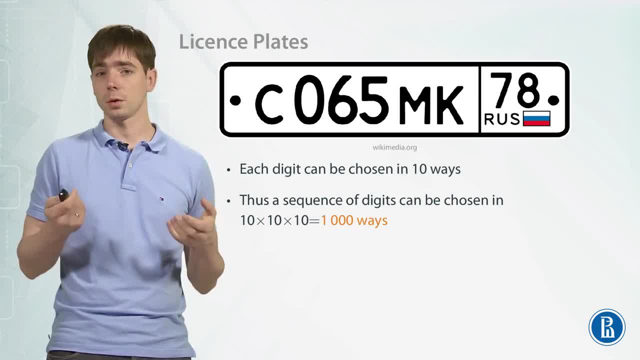 So now we have to pick a tuple of 3 digits And it can be chosen by the previous result, by the previous statement. It can be chosen by 10 times 10 times 10, by 1000 possible ways. Okay, Next we have to pick 3 letters. 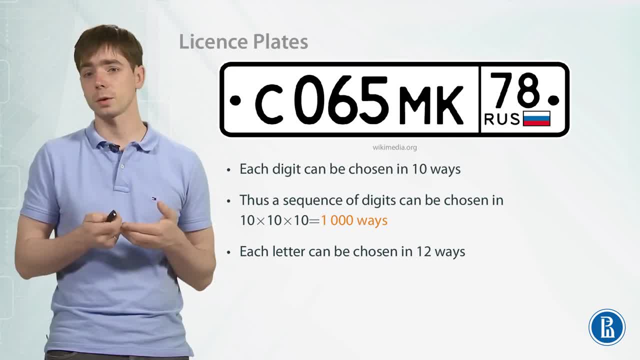 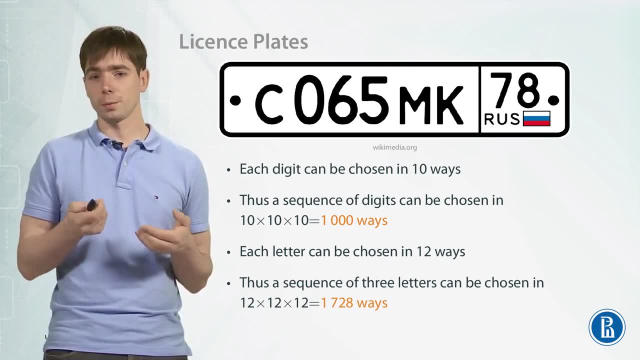 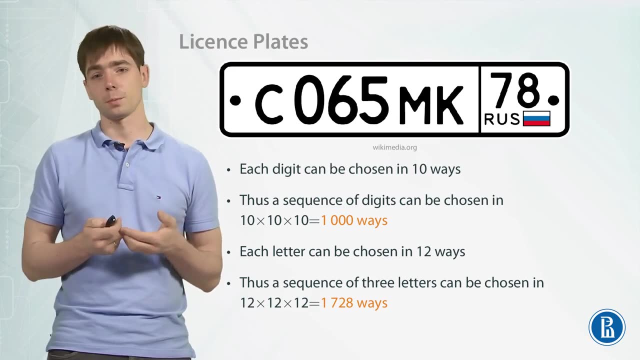 And each letter can be chosen in 12 ways. So we have a tuple of 3 letters And it can be chosen by 12 times. 12 times 12, which is 1728 possible ways. Okay, Now, how many ways do we have to choose a sequence of digits and a sequence of letters? 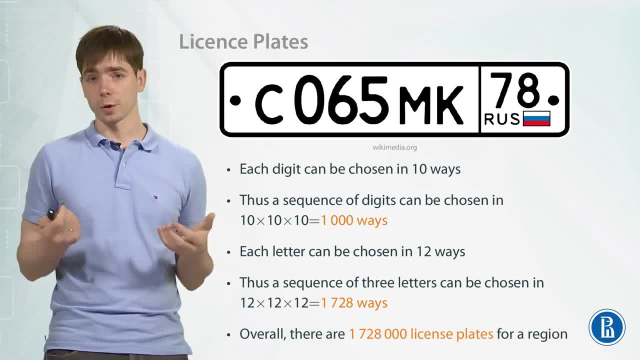 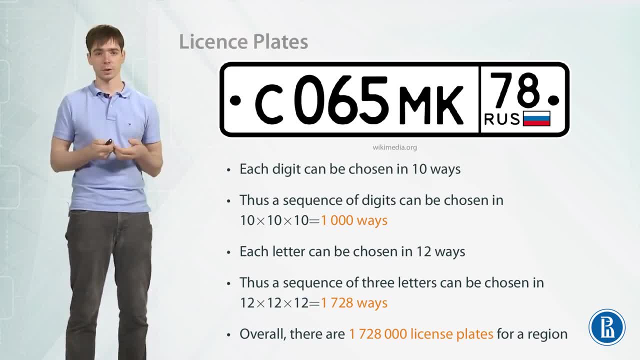 Again we can apply a rule of product. We have to choose a tuple of length 3 of digits and a tuple of letters of also length 3.. We have to multiply these two numbers And so in total we have 1,728,000 license plates for a region. 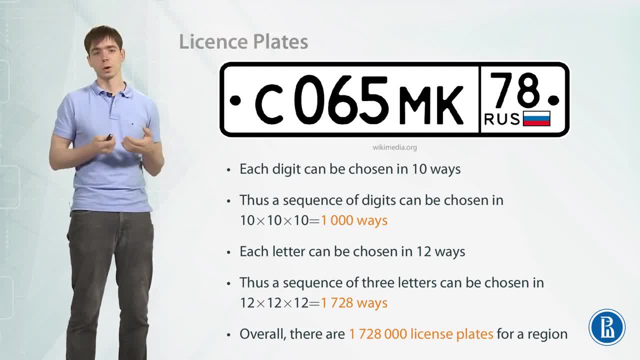 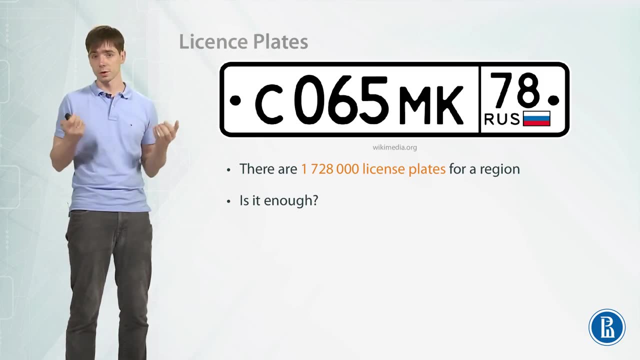 Okay, So we have done the calculations. We do not need anyone to list all of the license plates. Here is the answer. We have done this in just two slides. Okay, Is it enough? So we have this number of license plates. 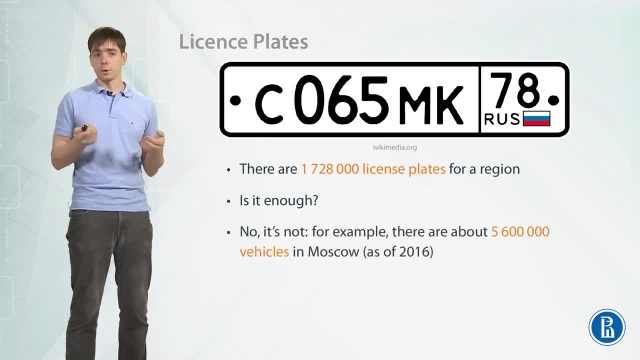 Is it enough? It turns out it's not. For example, if we look at Moscow, it's one of the regions We have more than 5 million vehicles in Moscow as of 2016.. Now, in 2017, it's even more. 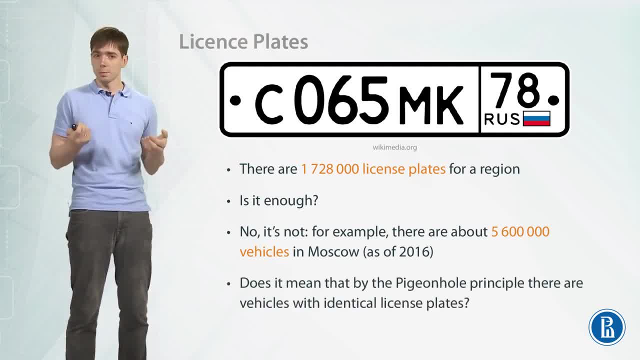 So it's not enough, Okay, Does it mean that by pigeonhole principle we're Okay? So vehicles here are pigeons and license plates are pigeonholes. Recall that we have a pigeonhole principle. If there are more pigeons than pigeonholes, then there should be at least two pigeons. 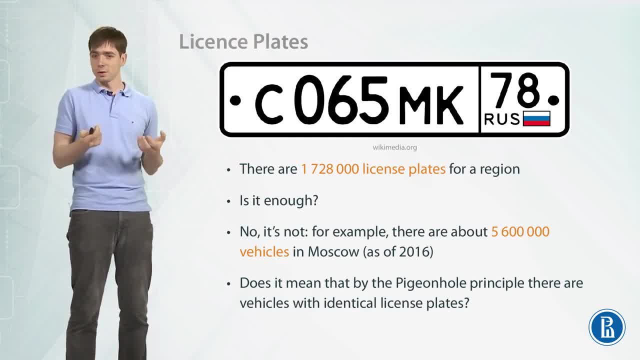 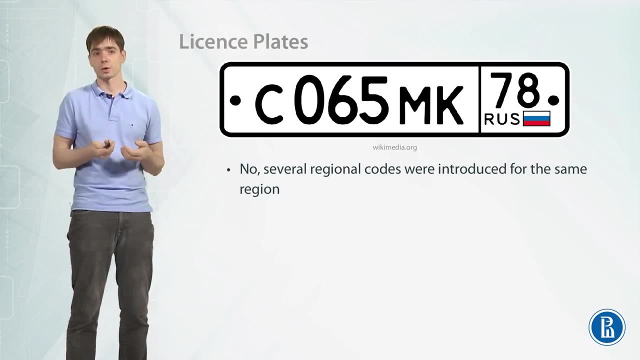 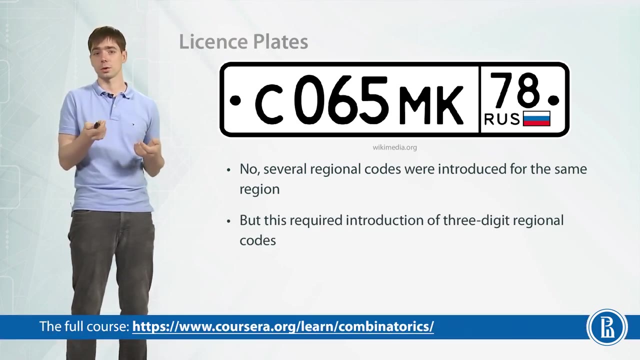 in one pigeonhole. So does it mean that there are two vehicles with identical license plates? No, it doesn't. So the solution was that there were several regional codes introduced for the same region. Still, this required introduction of not two-digit regional code like on the picture. 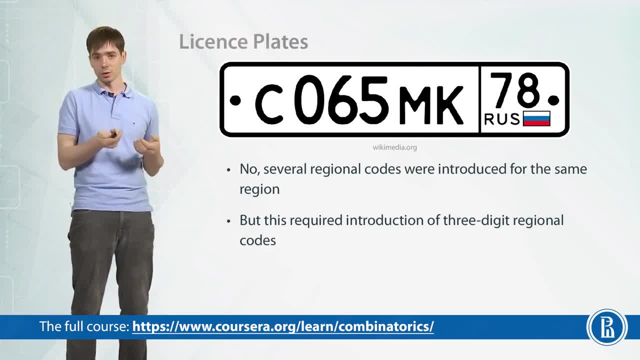 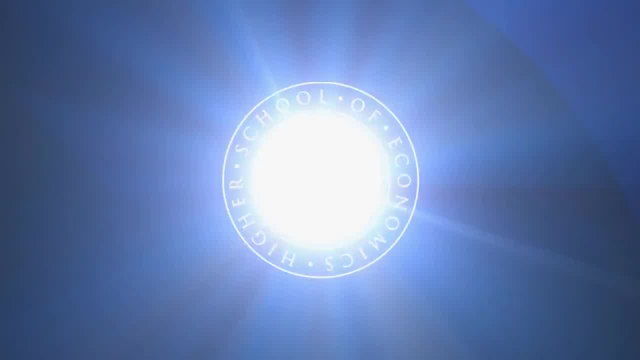 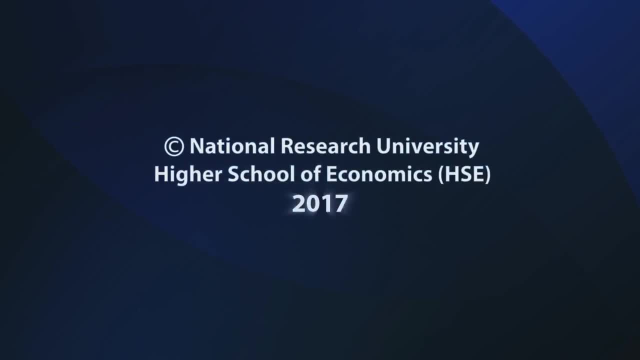 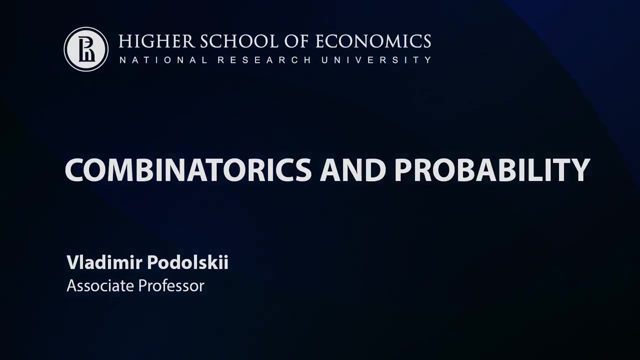 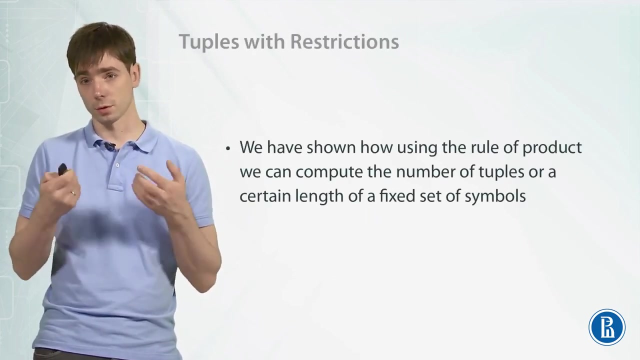 78, or instead we had to introduce three. So now we have three-digit regional codes as well. So we have seen that the rule of product allows us to compute the number of tuples of a certain length over a certain size of alphabet, But this rule can give us much more. 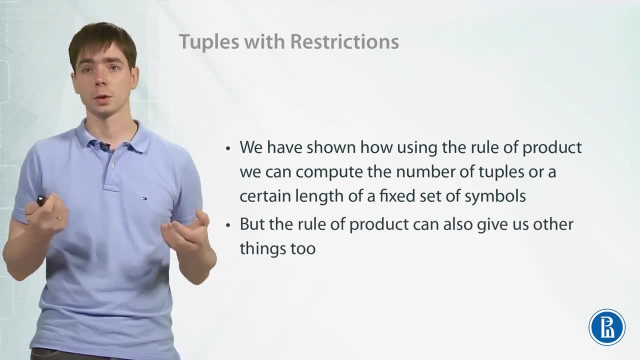 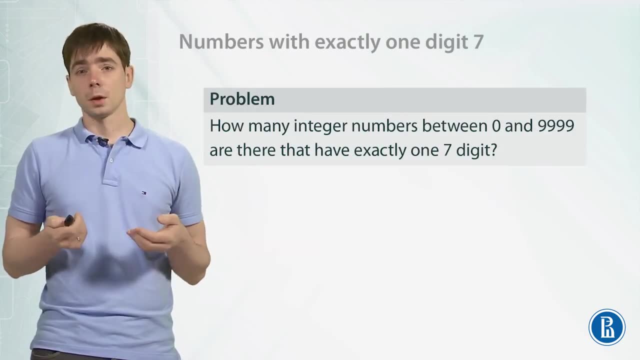 In the next example we will see how it allows us to compute the number of tuples with certain additional restrictions. Consider the following problem: Consider integers below 10,000 and above or equal to 10,000. That has exactly one digit, 7.. 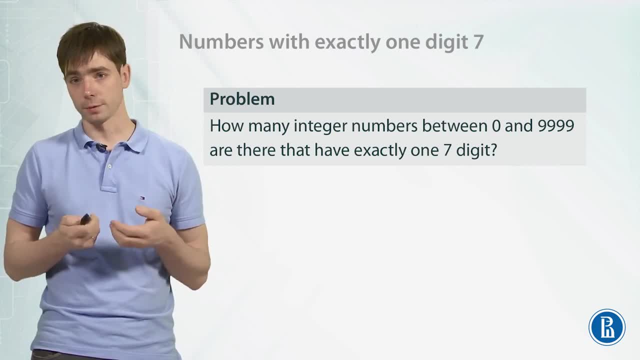 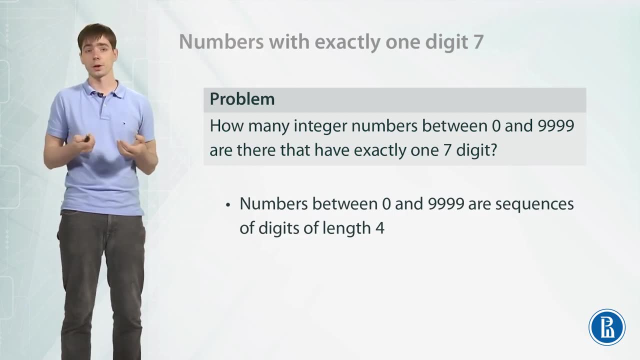 So how many integers with this restriction do we have? Okay, So first of all, let's note that we can represent the integers of this form by a sequence of digits of length 4.. Why of length 4?? So note that numbers below 10,000 can be represented of length 4, but there are also numbers with 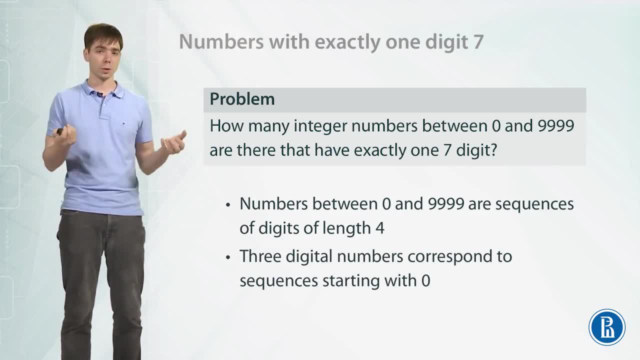 3 digits, How can we represent them by a sequence of digits of length 4?? Note that this is easy. They just correspond to sequences starting with 0. So, indeed, there is a correspondence between numbers below 10,000 and sequences of digits. 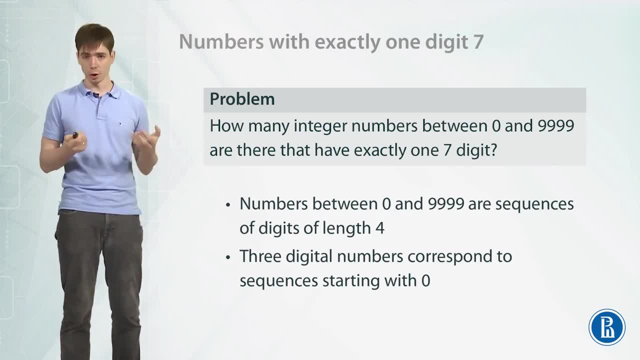 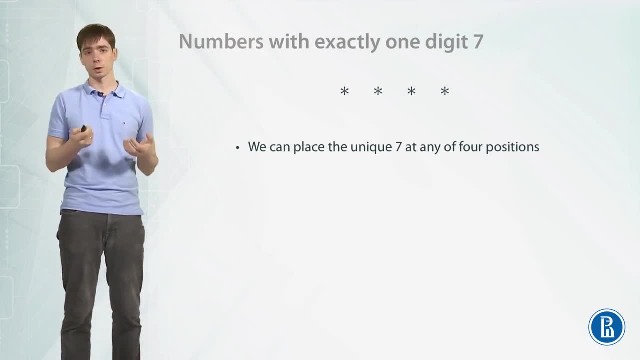 of length 4.. Okay So now we need to compute sequences of digits of length 4, that has exactly one digit, 7.. Okay So let's start with this unique digit 7.. We can place it to any of four positions. 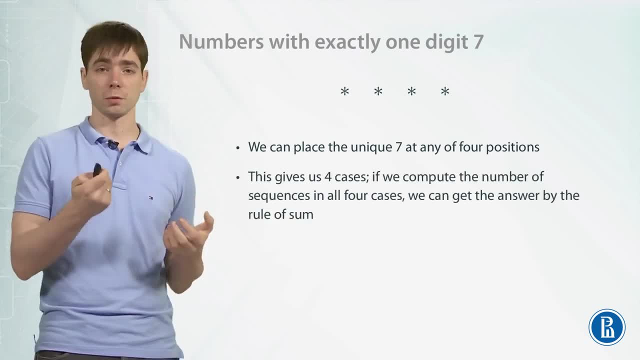 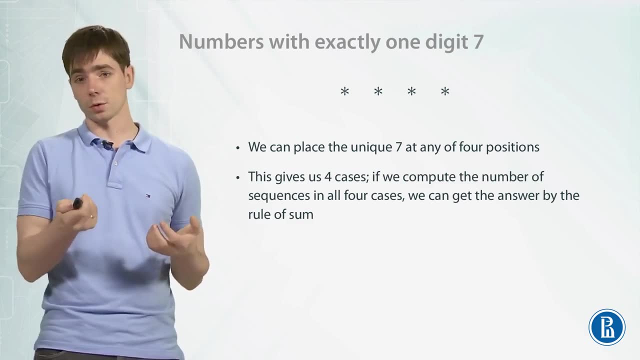 So there are four cases. we can place it to The first position, to the second one, to the third one and to the fourth one. And if we compute the number of sequences of length 4, the number of tuples of length 4 in all four cases, then we can sum these numbers up and get the answer just by the rule. 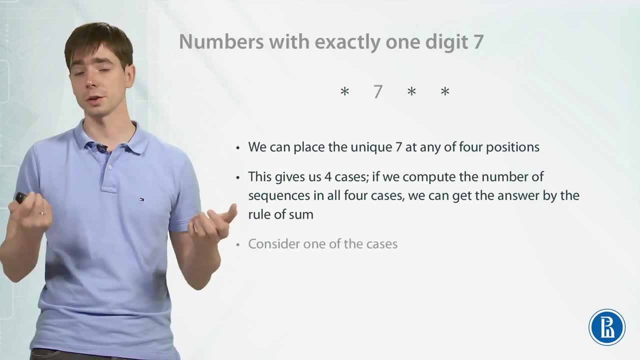 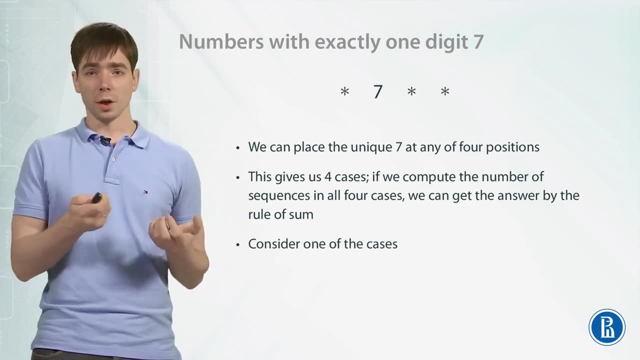 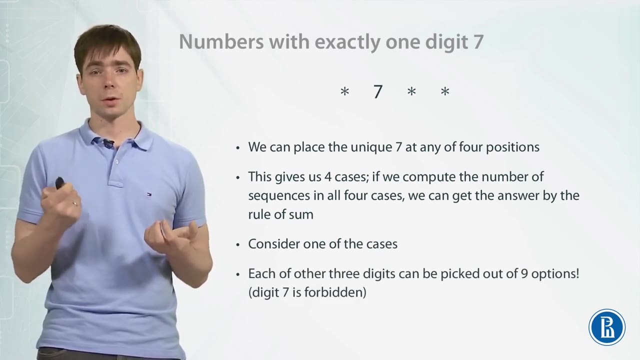 of sum. Okay, So let's do it. Let's consider one of the examples. So let's place 7,, for example, on the second position. Okay, How many tuples do we have with 7 in the second position? Note that we can pick each other digit in nine ways. 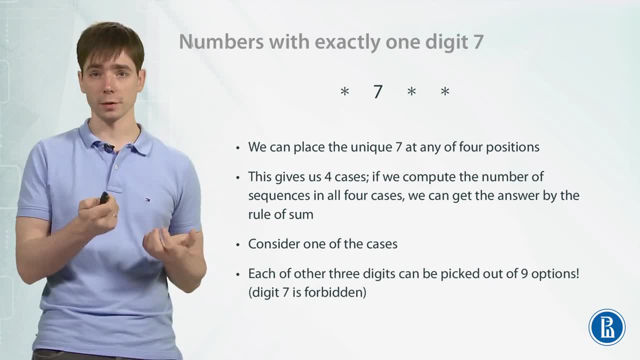 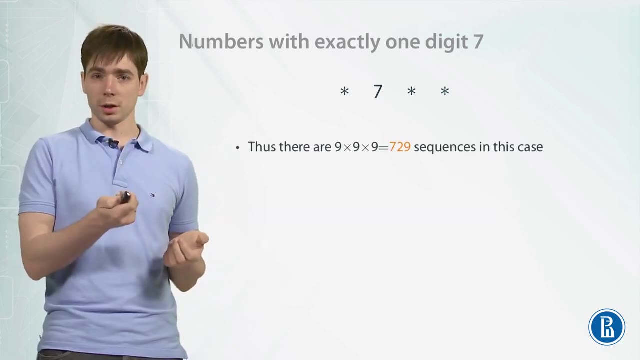 Why? Because 7 is forbidden. There is exactly one, 7, in this sequence, So 7 is already there. So for other positions, 7 is forbidden. So it leaves us with nine options. Okay, So now we need to pick a tuple of length- 3,, where each digit can be picked from nine. 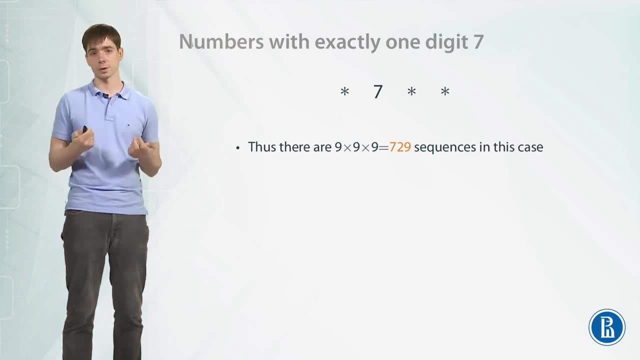 options. So we apply our previous result and we can say that there are 9 times 9 times 9.. This is 729 sequences in this case, And note that this argument doesn't matter that 7 is in the second position. It's the same if it is in the first position, the third or in the fourth. 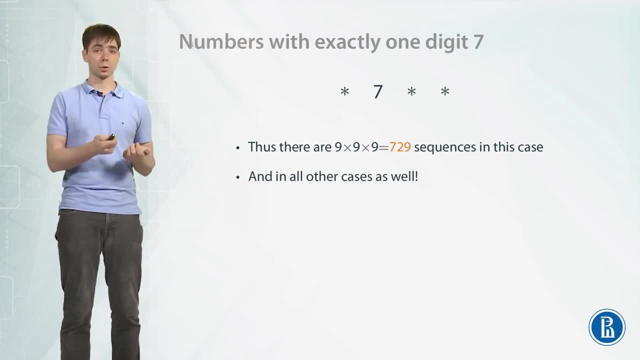 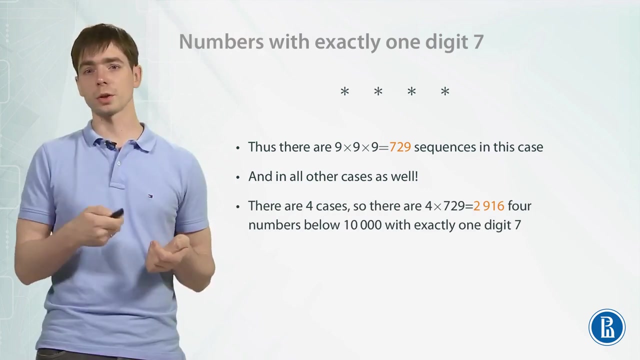 The answer is the same, no matter where we put digit 7.. So in all cases, in each of four cases, we have 729 sequences. Okay, So there are four cases. We have 729 sequences in each of them. No sequence can occur in two different cases. 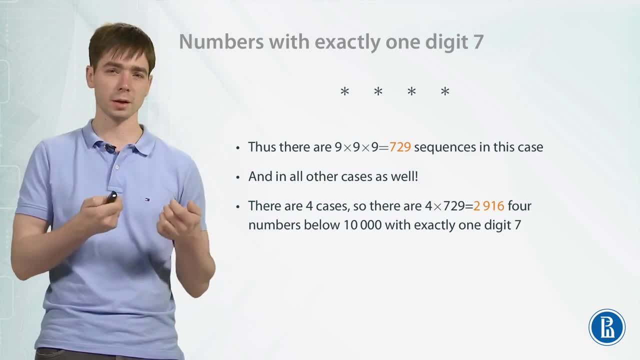 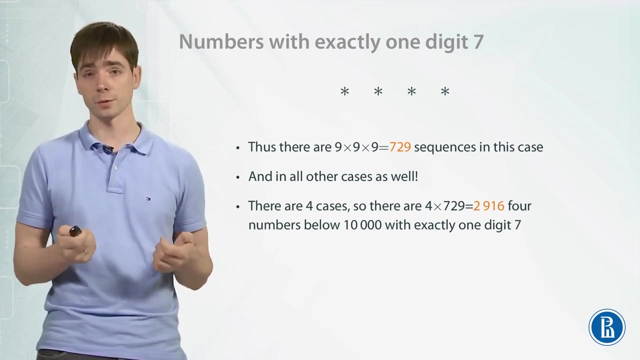 Because sequences in two different cases has number 7 on different positions, So we can safely apply rule of sum. We sum up elements of sets and there is no element in the intersection of any sets, So we can safely apply rule of sum. And so the number of sequences in all four cases is 4 times 729, which is 2916. 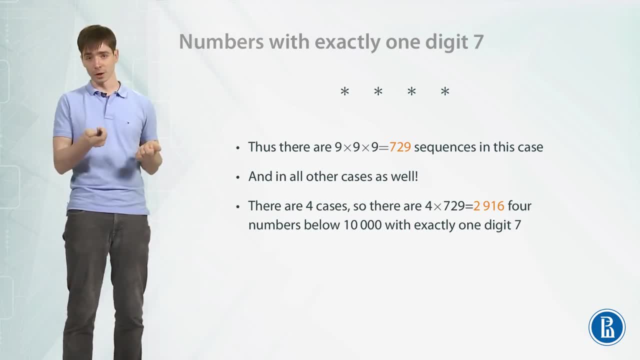 So there are these numbers, There are these many numbers below 10,000, with exactly one digit: 7.. Okay, Is it a lot or not? So we can see that in total, we have 10,000 numbers below 10,000.. 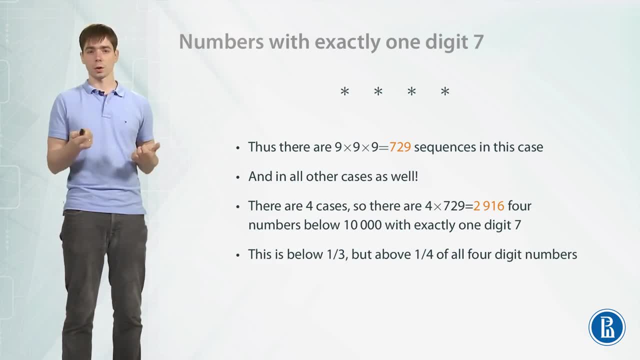 Note that we are also considering zero, So the fraction of numbers with exactly one 7 is 2916 divided by 10,000.. This is below one third, But above one fourth, So this is somewhere in between. These are rough estimations. 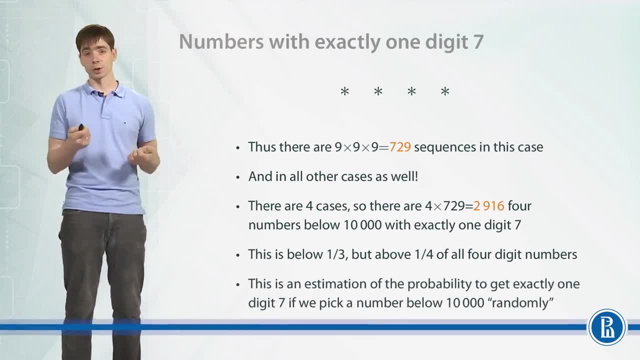 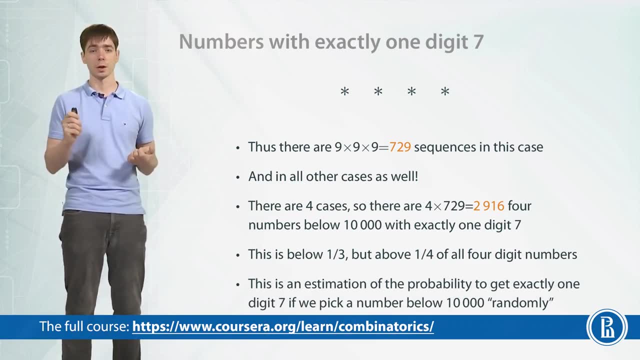 And these estimations give us. Note that these estimations give us the following: This is the probability So we have. So this is an estimation for the probability to get exactly one digit, 7, if we pick number below 10,000 randomly. 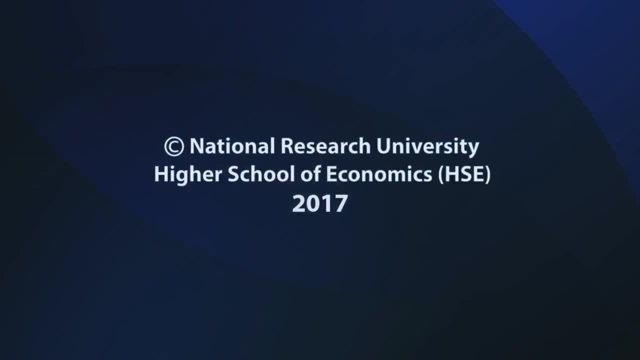 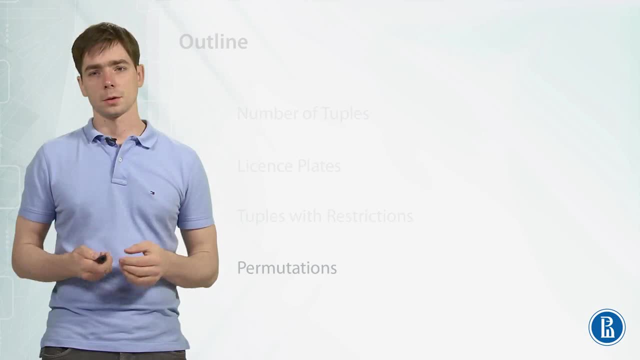 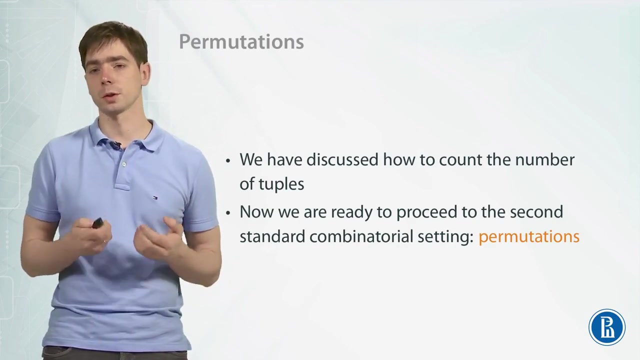 And this is the probability to get exactly one digit, 7, if we pick number below 10,000 randomly. So we have discussed how to count the number of tuples And now we can move on to our next standard combinatorial setting, Our second standard combinatorial setting. 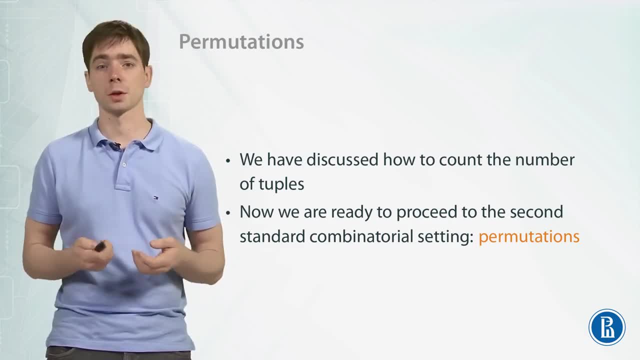 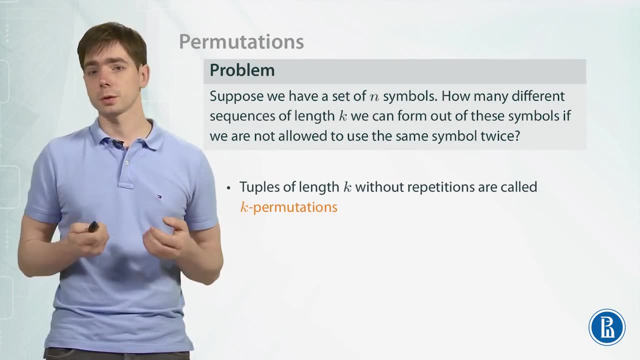 Permutations, We will count how many permutations are there. Okay, So consider the following general problem: Suppose we have a set of n symbols And we would like to count how many different sequences of length k are there Consistent of these n symbols. 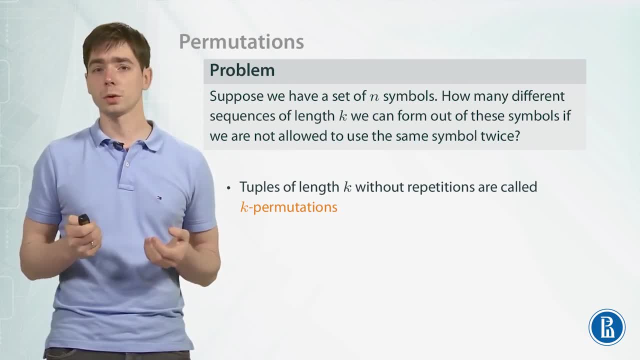 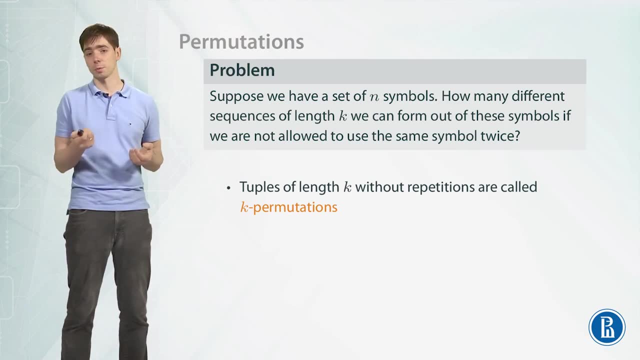 But with additional restriction: We are now not allowing to use the same symbol twice. Okay, So tuples of length k, without repetitions of letters, are called k permutations, And that's what we are going to compute in this problem: The number of k permutations we are going to compute in this problem. 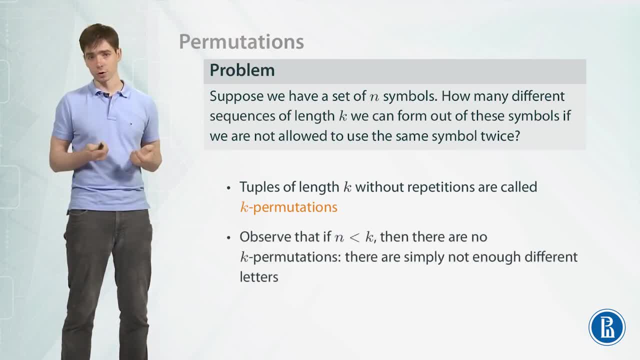 And let's make the following observation, Useful observation: If n is less than k, If the number of symbols in our disposition is less than the length of sequence we are trying to construct, And we are not allowed to repeat letters, Then the answer is simple. 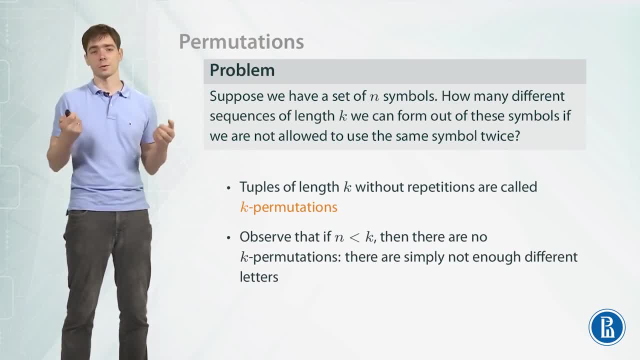 There are just no permutations there. There are just not enough different letters to construct a sequence of length k. So in this case the answer is zero And this case is simple. So let's, further on, assume that k is at most n, And let's consider this case. 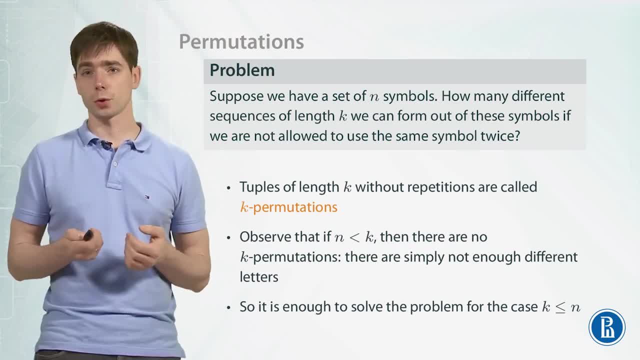 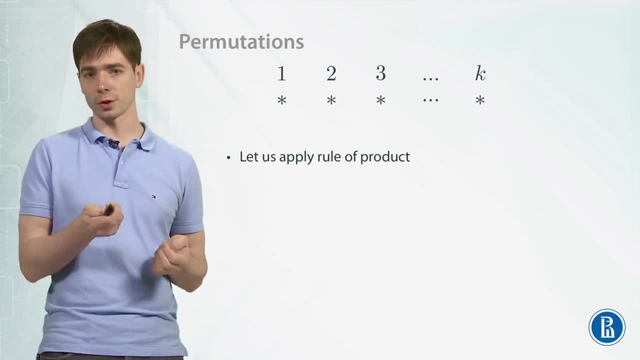 The non-trivial case. So let's proceed to the solution to our problem. Okay, So here we see our sequence. We denote the symbols by stars, Let's enumerate them from 1 to k And we will apply the rule of product. 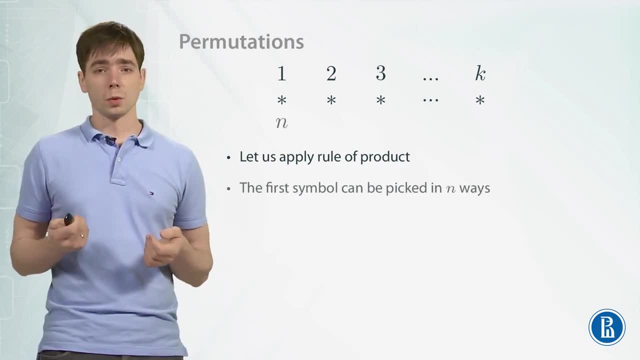 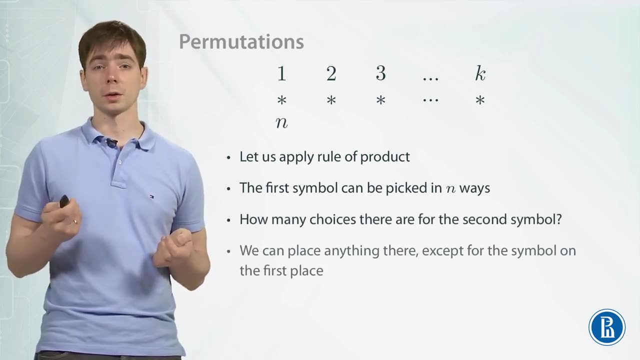 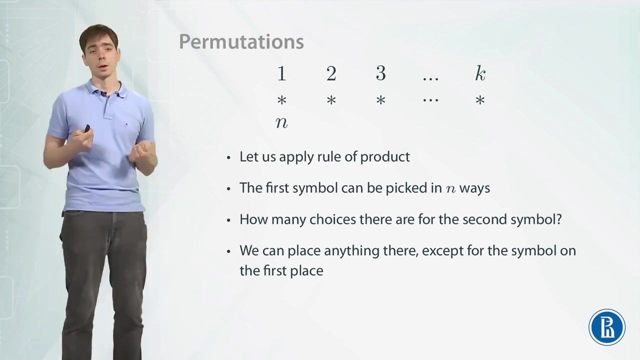 So we will solve this problem using the rule of product. So the first symbol we can pick in n ways. So what about the second symbol? How many choices do we have there? And note that we can place there anything except the symbol we already placed in the first position. 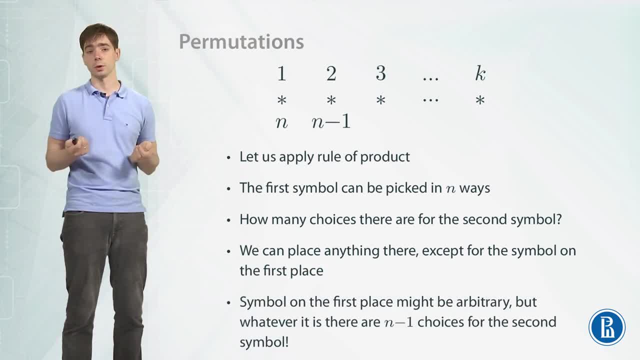 So there are n-1 options for the second symbol. The symbol in the first position might be any symbol, But for any symbol in the first position There are n-1 possibilities for the second symbol. So there are n possibilities for the first symbol. 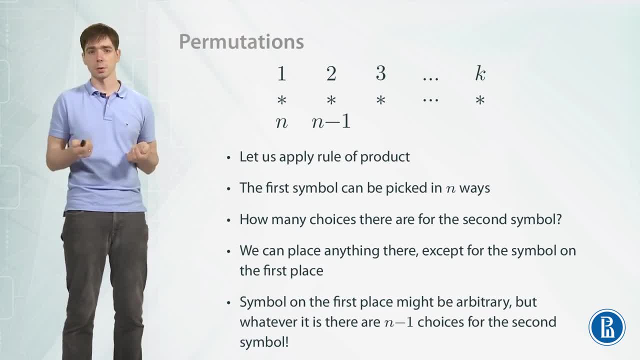 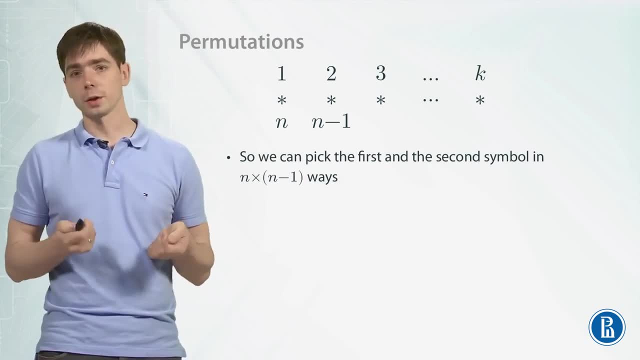 For each of them, there are n-1 possibilities for the second symbol. So in total we have n times n-1 possibilities to pick the first and the second symbol. Okay, And now we can proceed in the same way. Consider the first symbol. 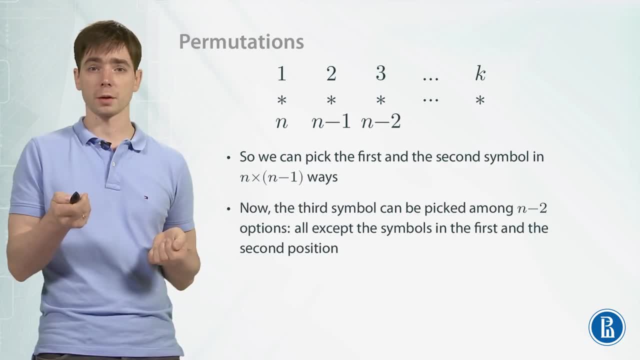 We can pick the first two symbols by n times, n-1 ways. And for the third symbol, Whatever the first and the second symbols are. For the third symbol we have n-1 options: All symbols except the symbol in the first position and the symbol in the second position. 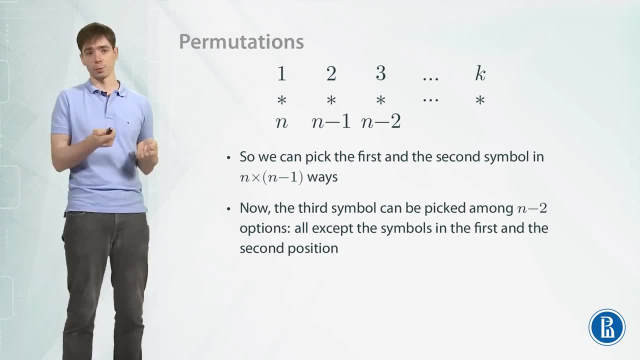 So there are n-2 possibilities for all ways to pick the first and the second symbol. So for the first three symbols we have n times n-1 times n-2 possibilities, And so on. For each next symbol we have one less option. 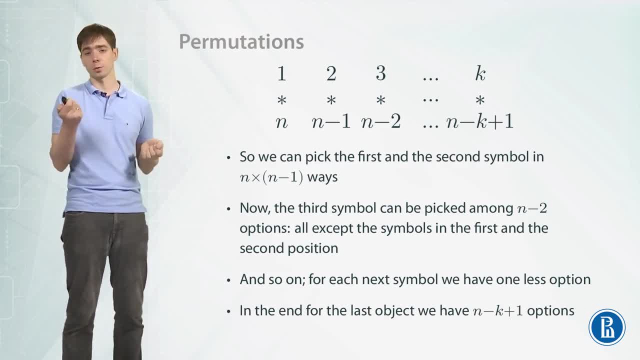 And in the end- So for the last symbol- we will have n-k plus 1 option. So this might require a moment's reflection Why it's n-k plus 1 and not n-k. One easy way to observe it is to look at. 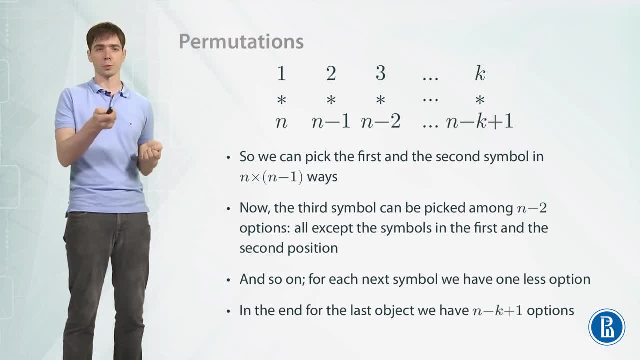 So let's see Near the first symbol, we have one number above and one number below: 1 and n. For the second symbol, it's the same. We have two numbers: 2 and n-1.. Note that for each symbol, 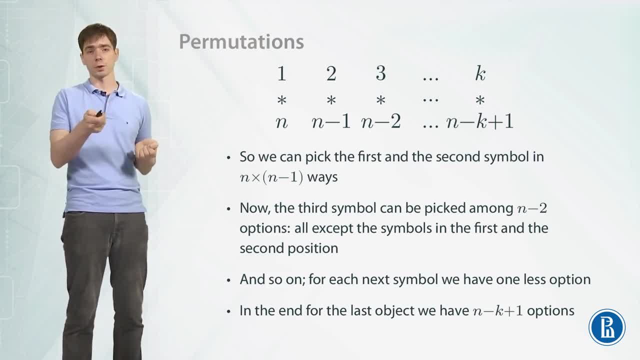 For the first, for the second, for the third, and so on. The sum of these numbers is n plus 1.. And when we move to the right, The first number increases, The second number decreases, So the sum of these numbers always stay to be equal to n plus 1.. 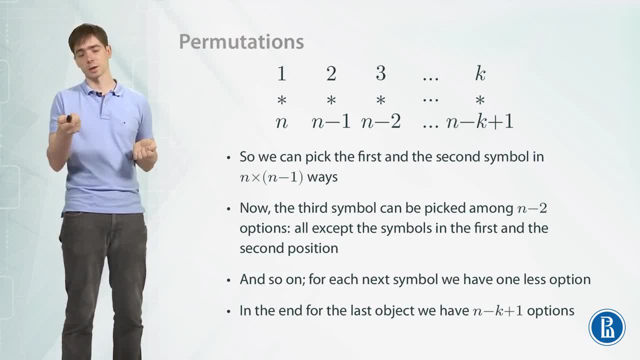 So in the end it also should be equal to n plus 1.. So it should be n-k plus 1 below there. So that's the easy way to observe that this is n-k plus 1.. There are n-k plus 1 options there. 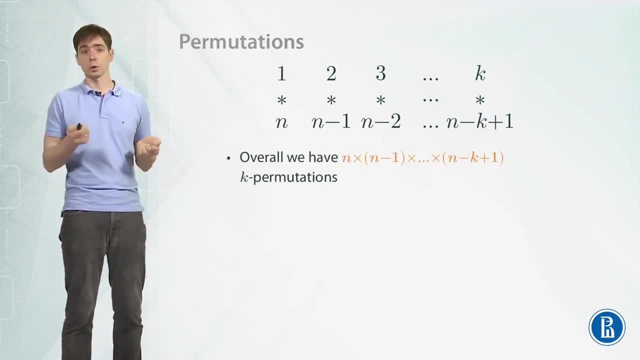 For the last symbol. Okay, So in total we have. So now we have to multiply all of these options, And so we have n times n minus 1.. And so on, Times n minus k plus 1.. K. permutations of symbols of length: n. 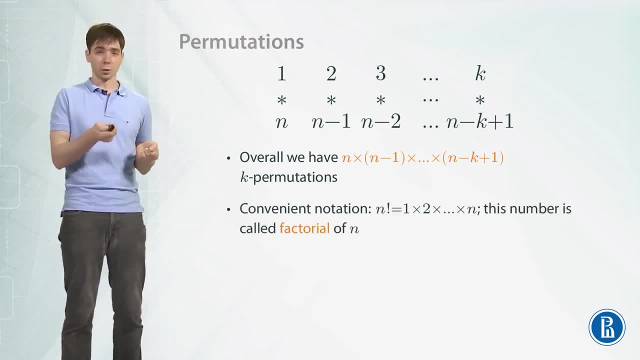 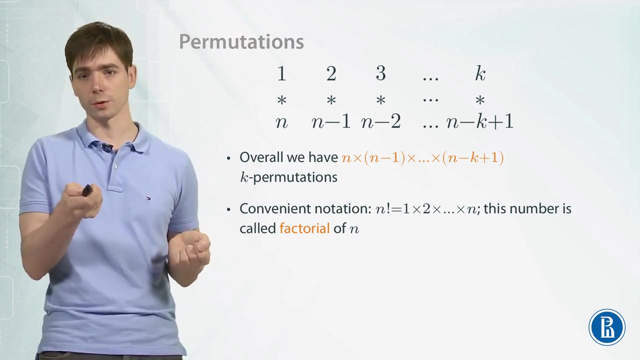 Okay, So this is not a very nice looking formula. So there is a convenient notation to make it look more simple. Simple and more short. A convenient notation is n factorial. So by n, factorial Is just the product of numbers from 1 to n. 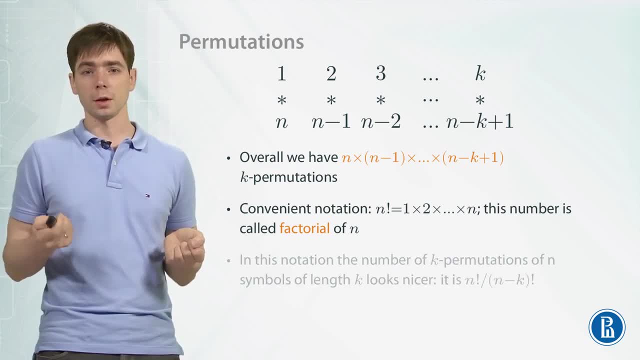 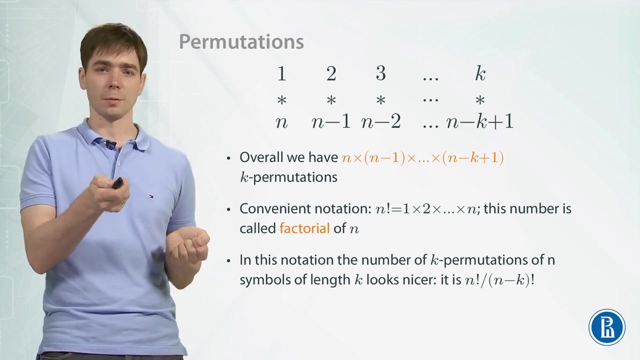 1 times 2 and so on times n, And in this notation The number of k permutations of n symbols Look, Looks nicer. It is. Note that we have Product of. The answer to our problem was The product of all numbers. 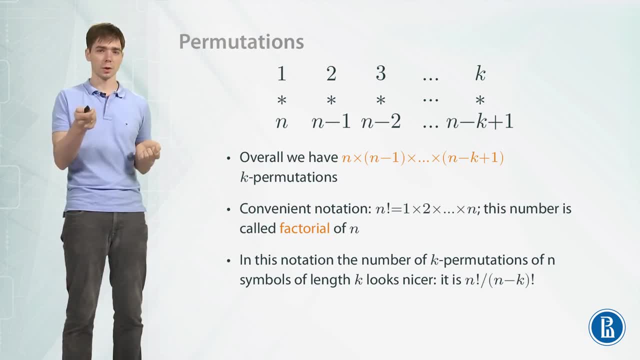 We multiply n by n minus 1., By n minus 2. And so on. But we stop on n minus k plus 1. So we can write it as n factorial Divided by n minus k factorial. So we consider n factorial. 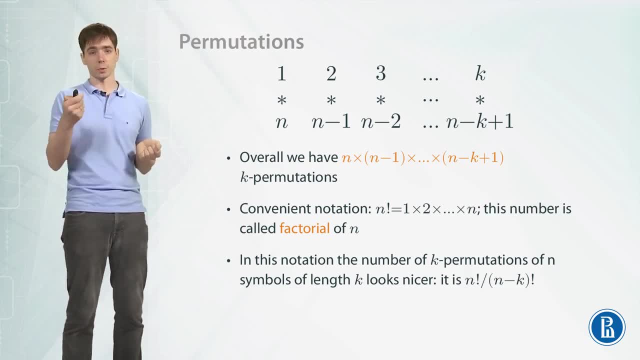 And we divide it by all multipliers We do not want in our product. So the answer in these terms is n factorial Divided by n minus k factorial. And Okay, One important observation to make. And what if n minus k is equal to 0.. 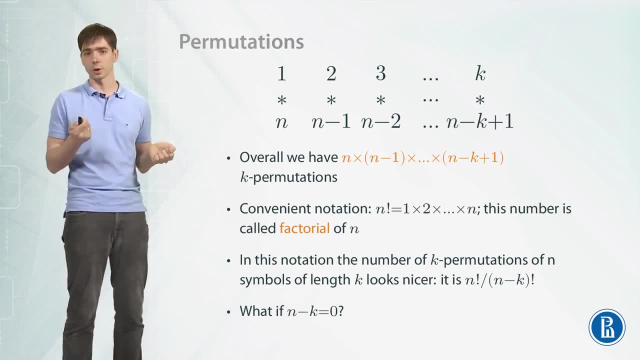 This is possible. So What if a is n is equal to k, Then in this formula We have- It looks like we have- We try to divide by 0.. n minus k is 0. So We try to divide something. 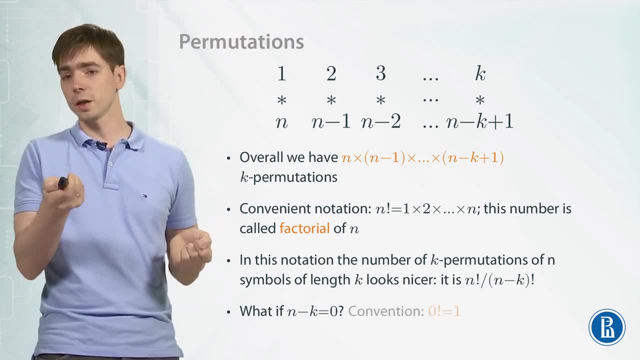 Is this an attempt to divide by 0?? No, it's not. It's an attempt to divide by 0, factorial, And we haven't said what it is yet. And the standard convention here To make this formula True only Also for this case. 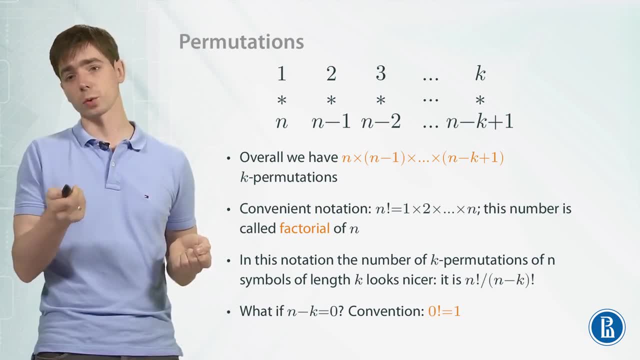 The standard convention is To say that 0 factorial is 1.. So That's what we will agree, Agree upon, And then this formula works also for the case of n equals k. So And we are done. The answer to this problem is n factorial. 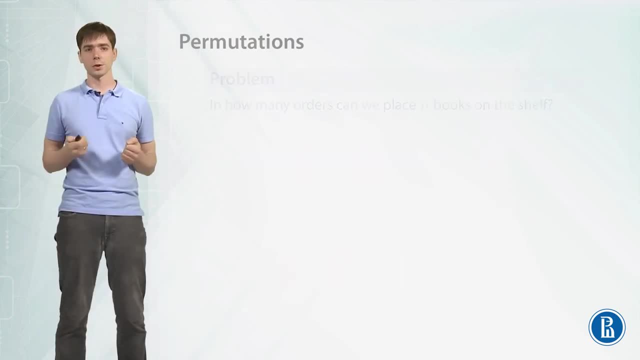 Divided by n minus k factorial. So Now let's consider the following specific example. So We have n books, n different books, And we would like to place them on the shelf In some order. So How many different orders? 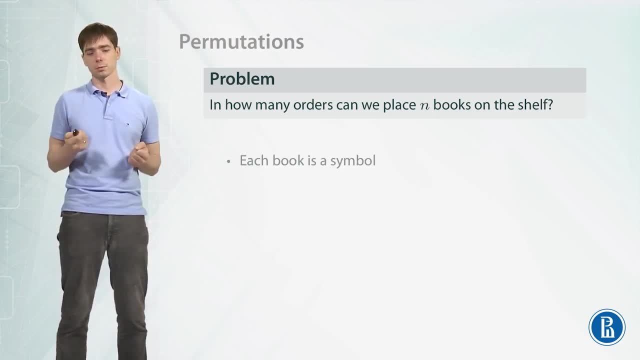 In how many different orders we can do it. Okay, We can think of each book as a symbol. And now What we need to do? We need to Count. how many sequences of n symbols Do we have? Do we have? 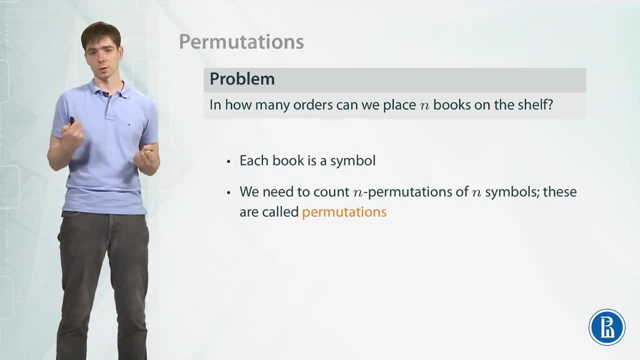 And Again, As in the previous Previous problem, We are not allowed to repeat the symbol twice. We cannot place the same book in two places simultaneously On the bookshelf, So We need to count n permutations Of n symbols. 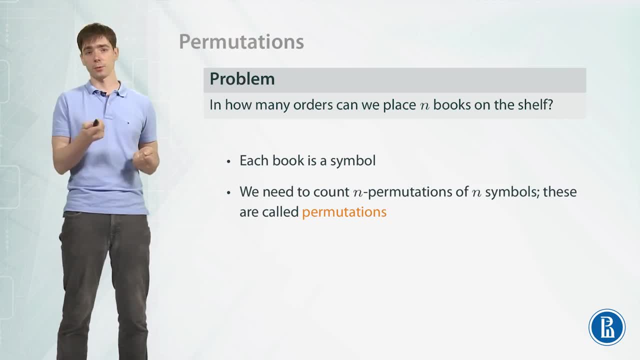 And these Are called Just permutations. If We have n permutations of n symbols, Then we can just omit The prefix n there And Talk about Just permutations. This is A very standard object In combinatorics. 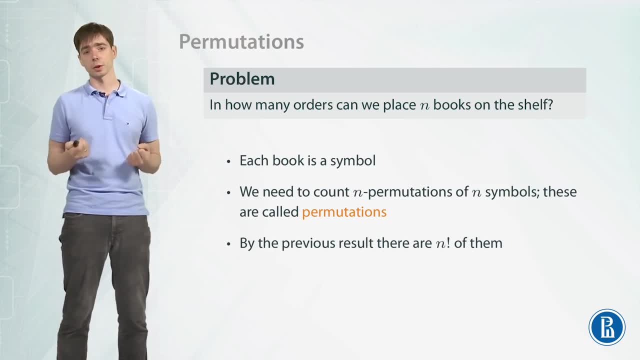 And By the previous result, We have n factorial of them. So We have shown: Our previous problem Shows That there are n factorial Of such Permutations And so There are n factorial ways To place. 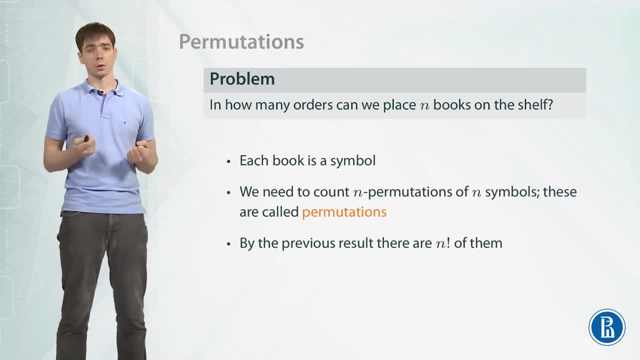 n books On the shelf. There are n factorials Orders To place n books On the shelf And Recall. So If you have seen Our First course, What is a proof Recall That we have used? 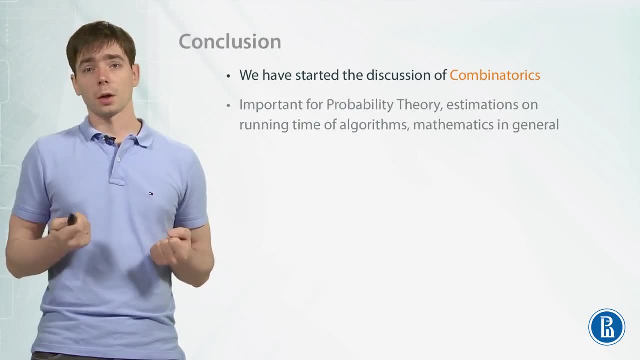 This formula When discussing Magic squares. Okay, So In this week We have started The discussion Of combinatorics, The theory. It will be important For estimation Of running time Of algorithms And it is also important. 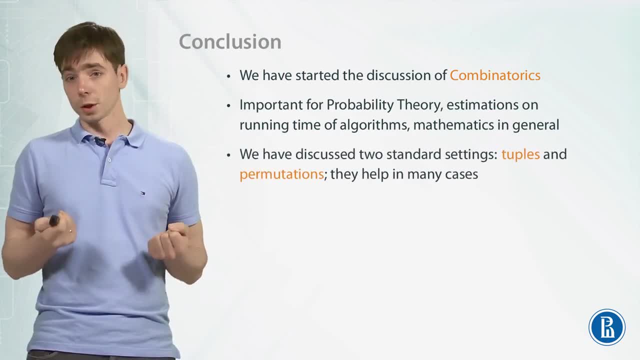 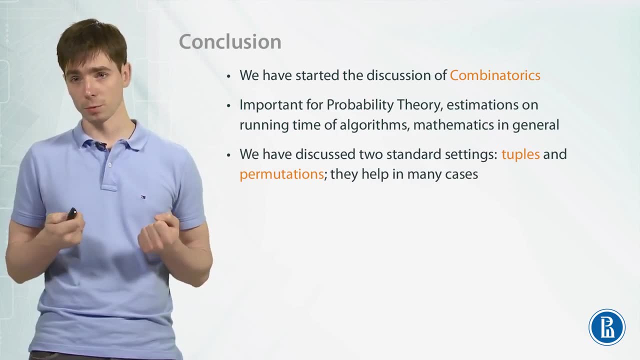 In mathematics In general And We have Already discussed Two standard settings In combinatorics: Tuples And permutations. We have discussed Discussed How We can compute How many tuples Are there Of certain length. 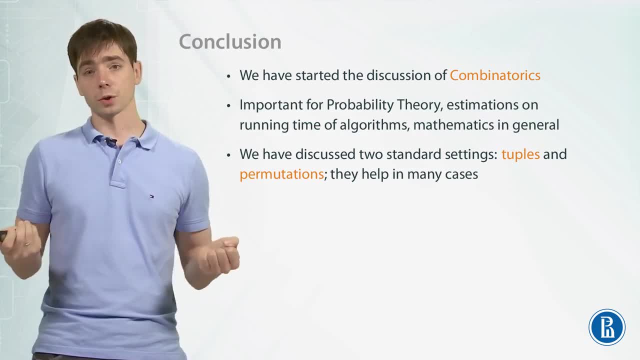 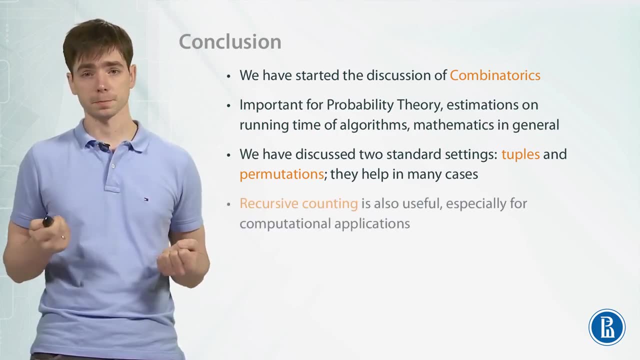 Over certain alphabet And How many permutations Are there Of certain length Over certain alphabet? And Already Help Help us In many settings. We also Have discussed Recursive counting. It is Also useful, Especially. 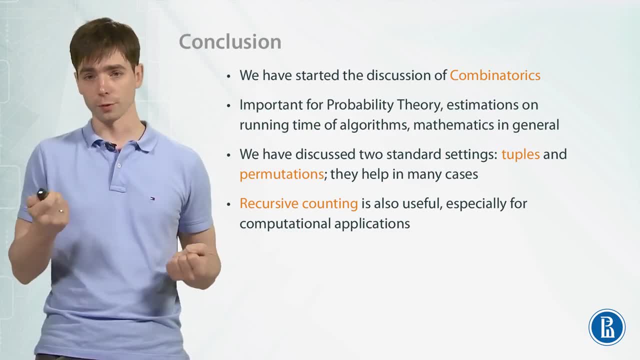 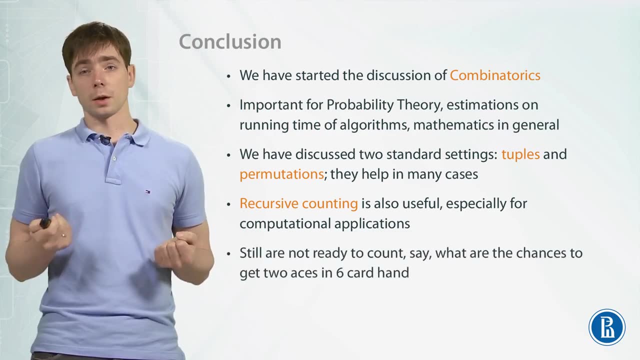 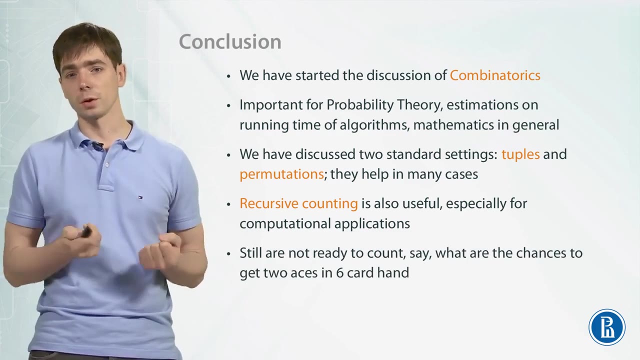 If We are trying To compute Something- Not To produce A formula, But To compute Something By an algorithm. Recursive Counting Is Very useful There, But We still Do not Count. 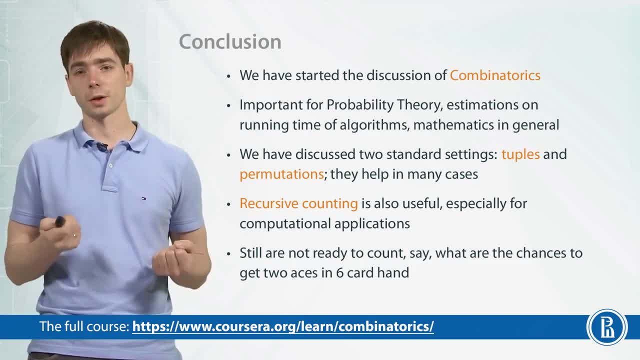 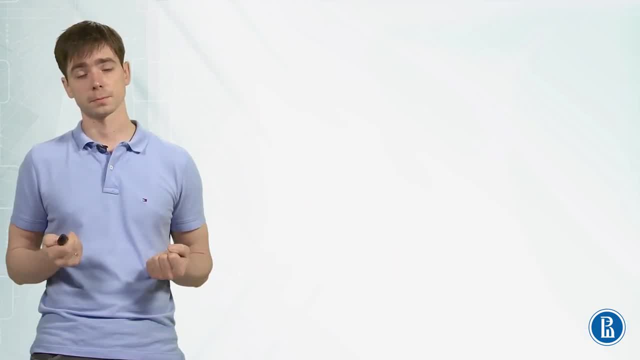 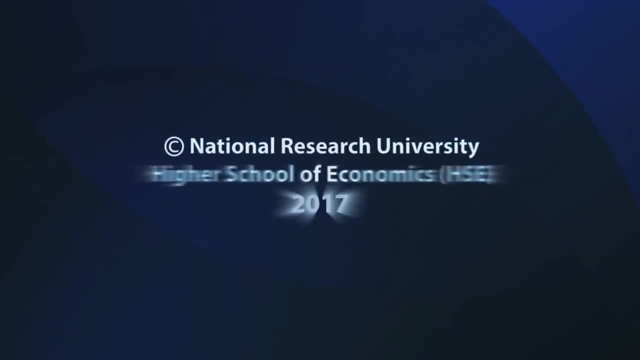 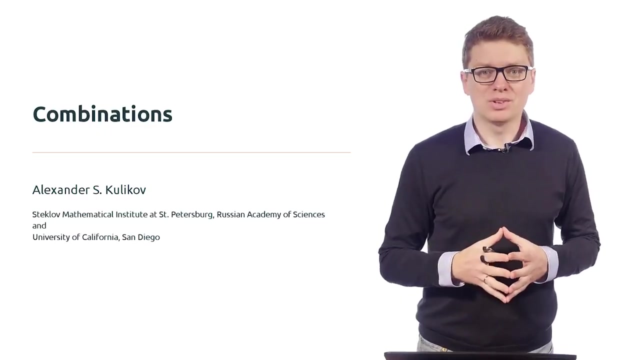 What Are Our Chances To Get Two Aces In The Card Game If We Have Six Card Hand? We Still Do Not Know How To. 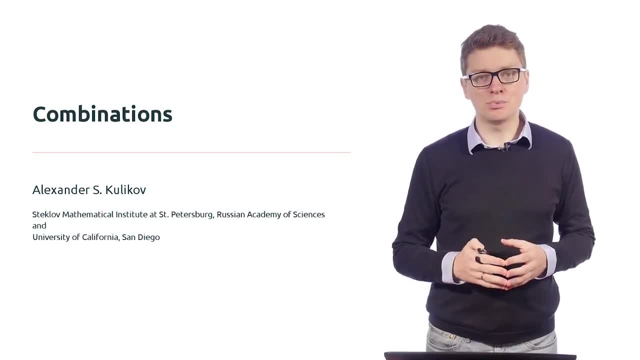 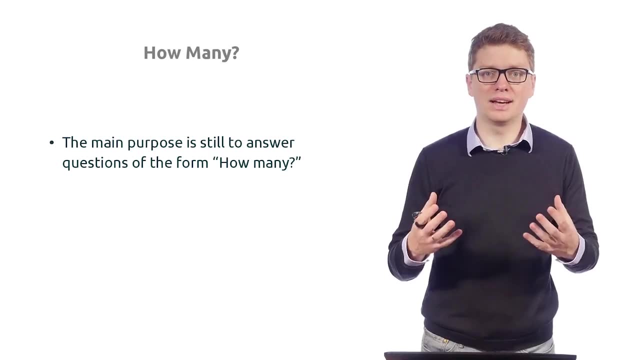 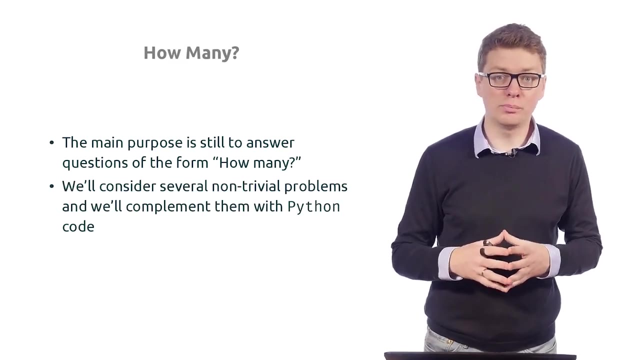 Do It, And In This Module We Are Going To Still Discuss Questions Of The Form: How Many Objects Are There Satisfying Some Particular? 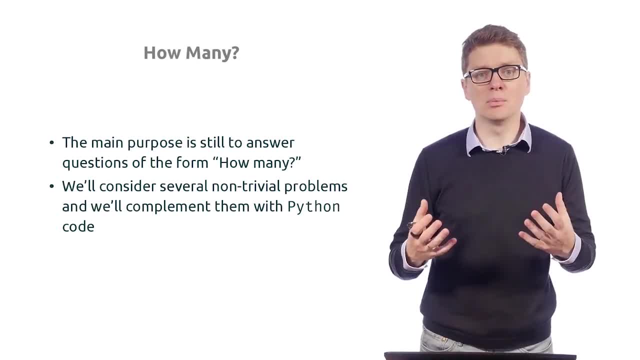 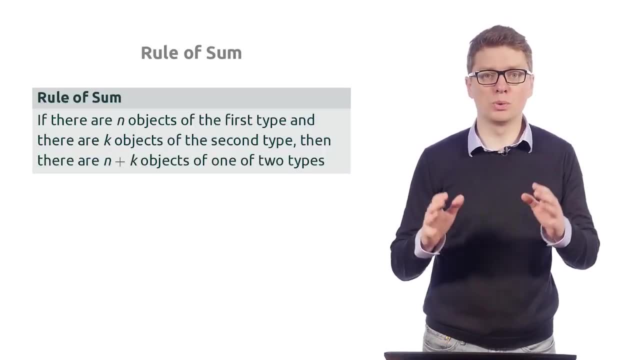 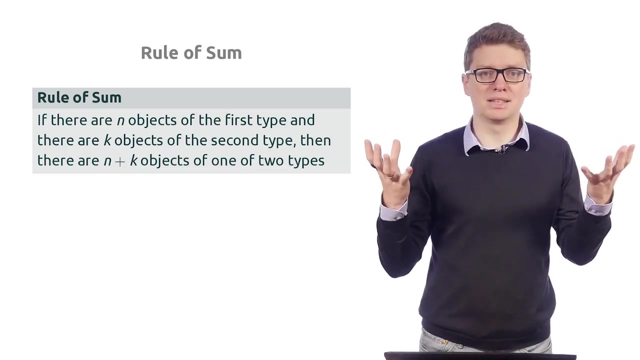 Properties. We Will See Many Interesting Questions And Details. Let's First Review What We've Learned Already In The Previous Module. So The First One Is: 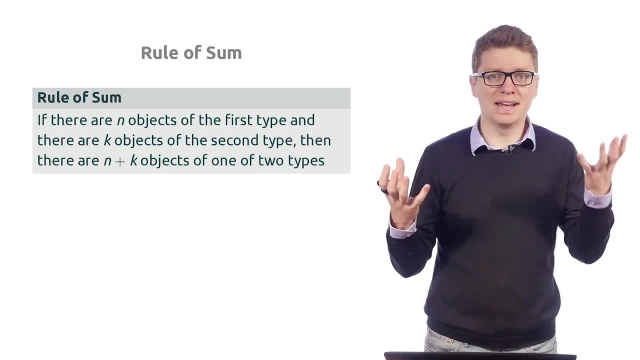 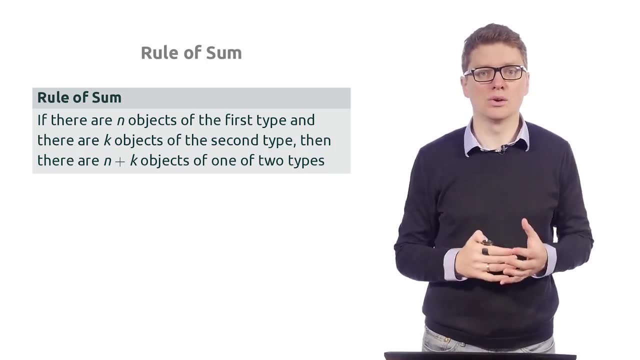 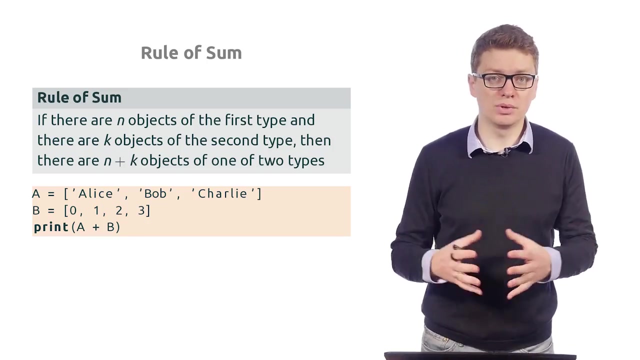 The Rule Of Sum. So If We Have N Objects Of First List It Consists Of Alias, Bob And Charlie And The Second List Is: 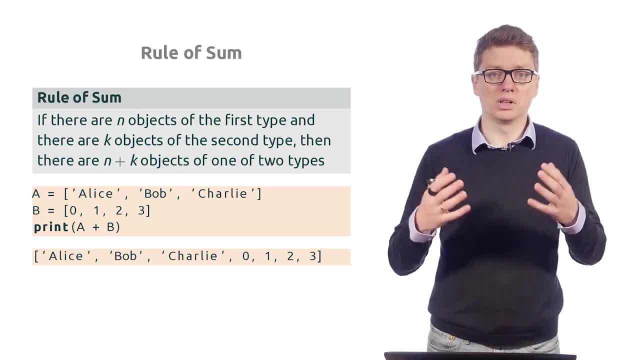 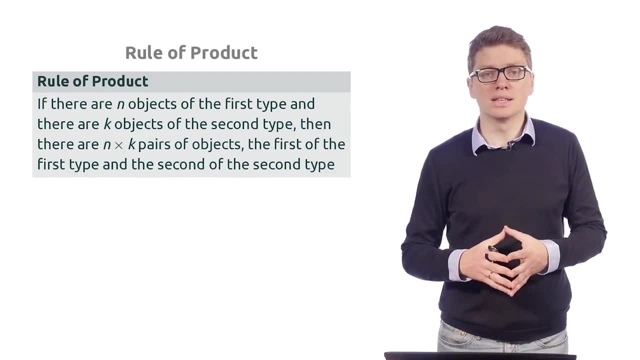 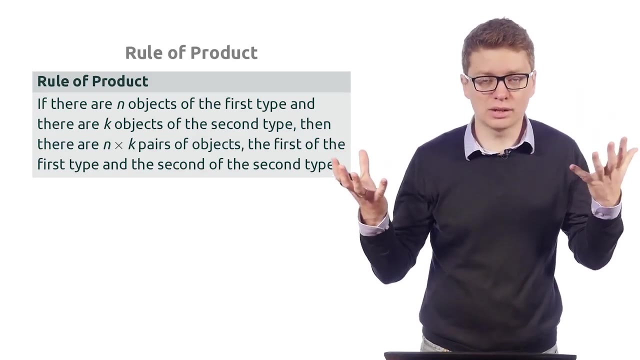 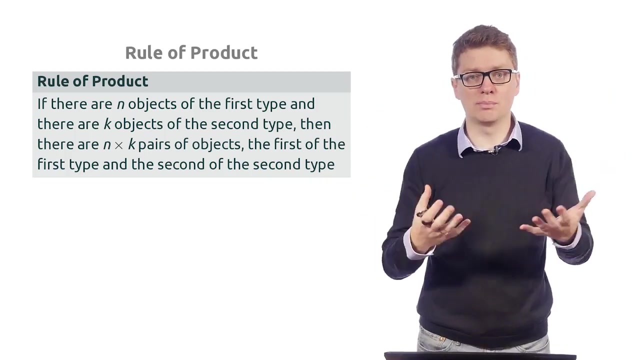 B And It Consists Of Four Digits: Zero, One, Two And Three. Then If You Have Two Objects On The Other Hand And You Would 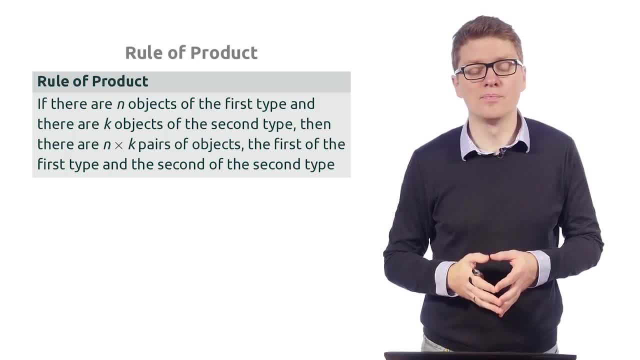 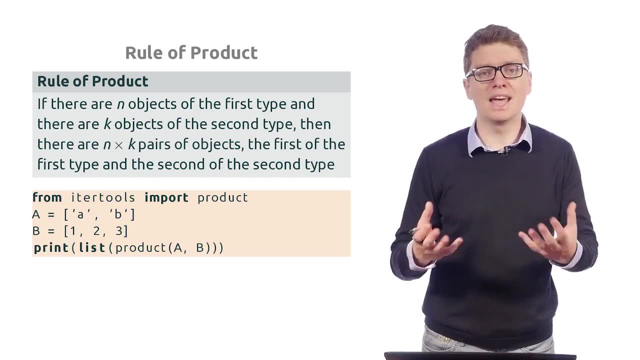 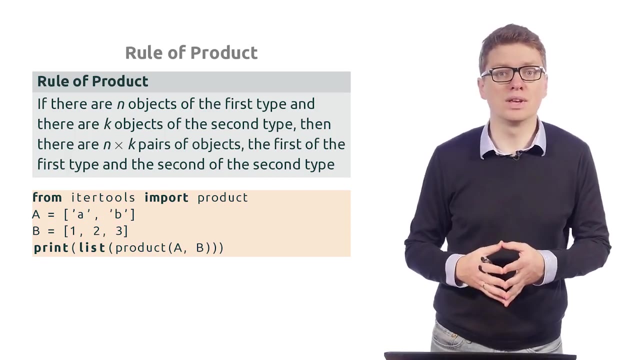 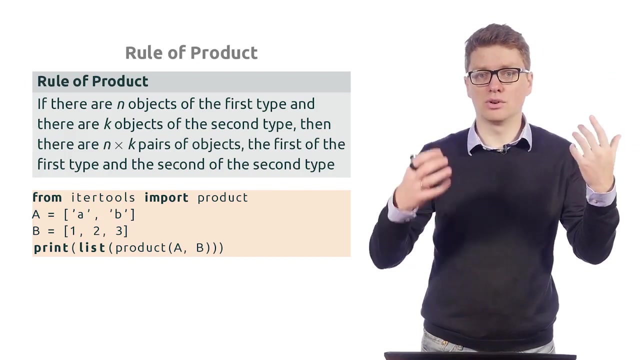 Like To Select The Pair Of Two Objects, One Of The First Type And One Of The Second Types, And Forming A Pair Of An 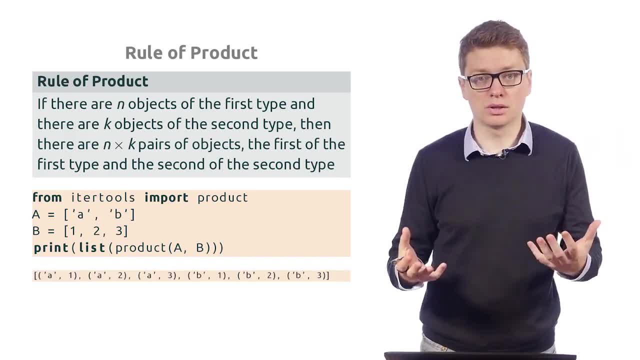 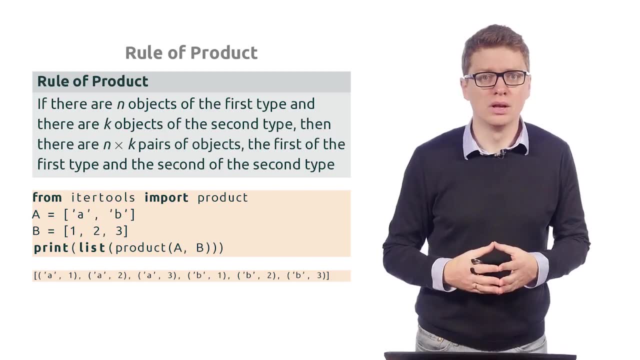 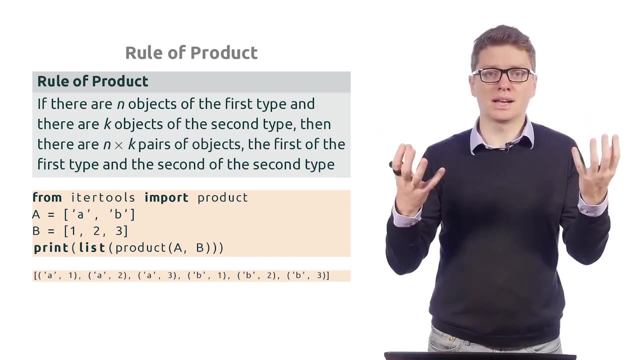 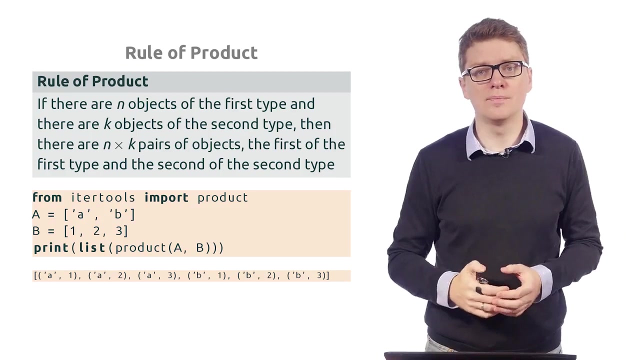 Object From The List A And An Object From The List B Is Equal To Six, That Is, To The Product Of The Length. Okay So 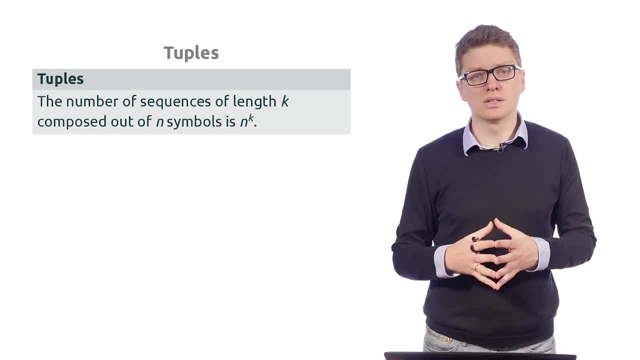 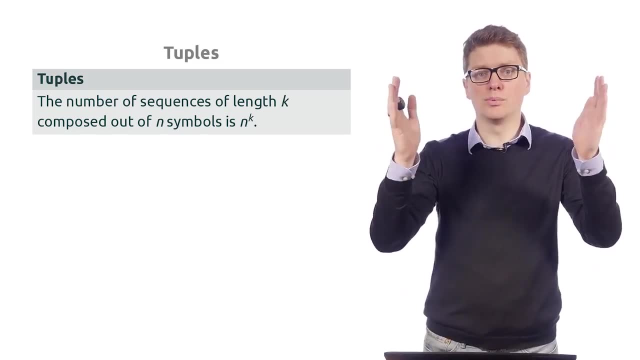 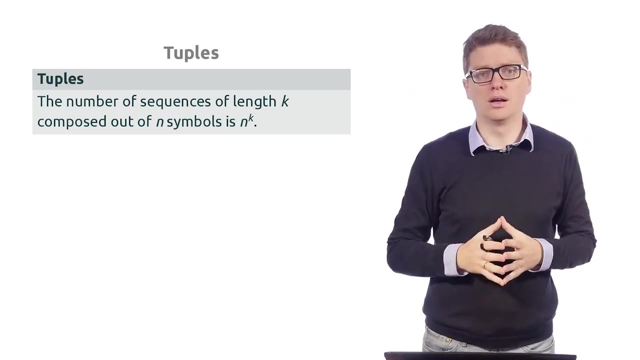 The Next. The Next Important Object Is Topples, So The Number Of Way Of If You Have An Object And You Would Like To Form. 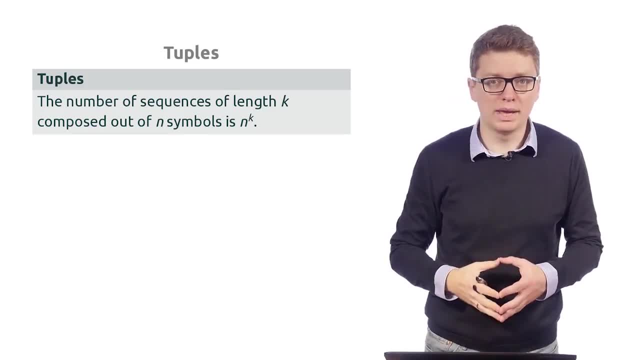 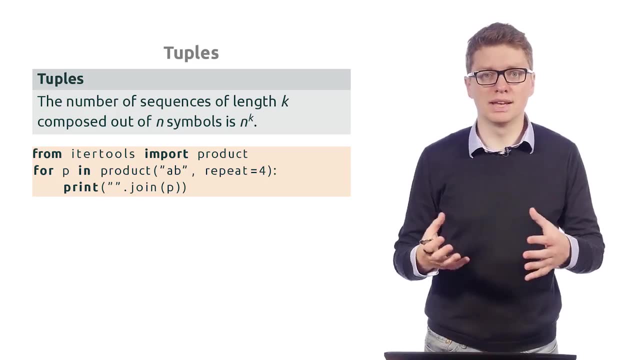 A Topple Consisting Of Way Of Doing So Is N To The K Once Again. Let's Show An Example. Assume That We Have Two. 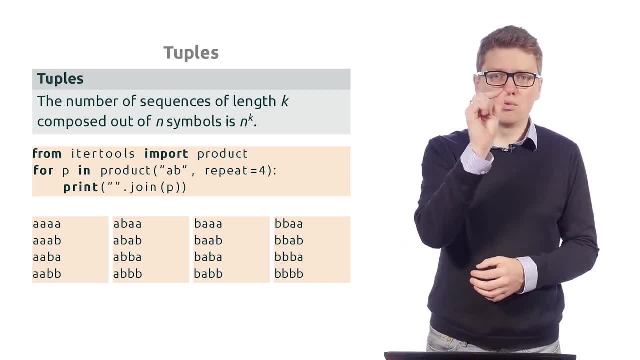 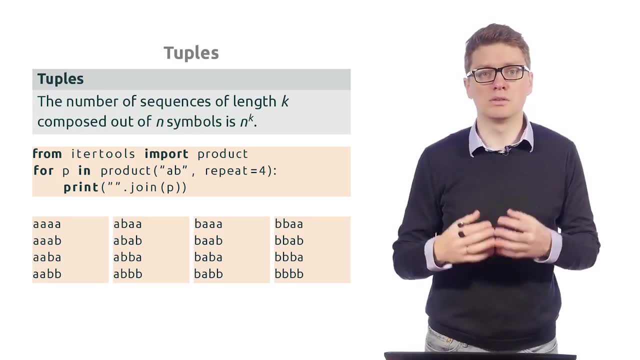 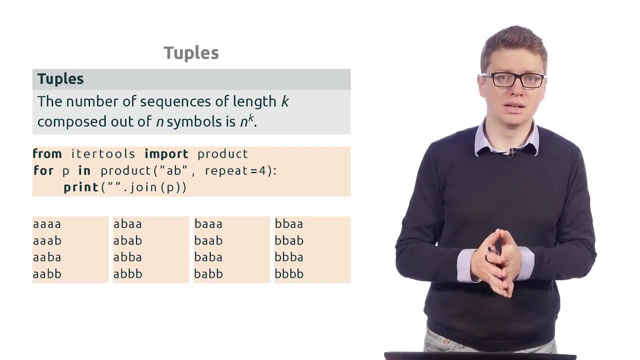 Letters A And B And We Would Like Take A Or You Take B. So By The Product Rule, The Number Of Ways Of Doing So. 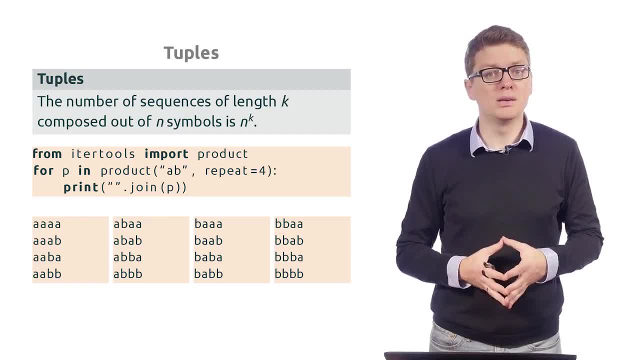 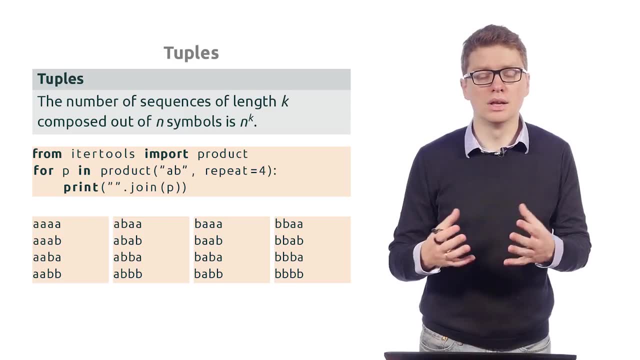 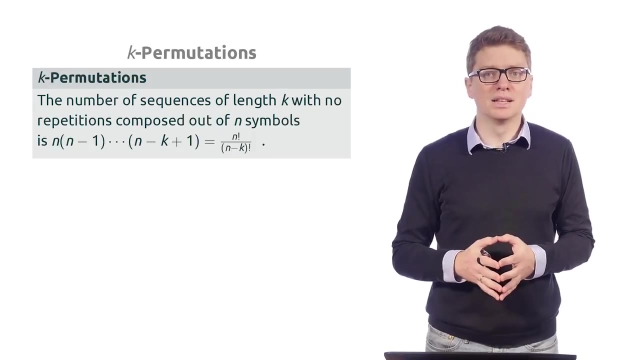 Is Two Times Two Times Two Times Two, Which Is Nothing. The Product Method Of The Library. Okay, So Finally Let's Discuss K Permutations In: 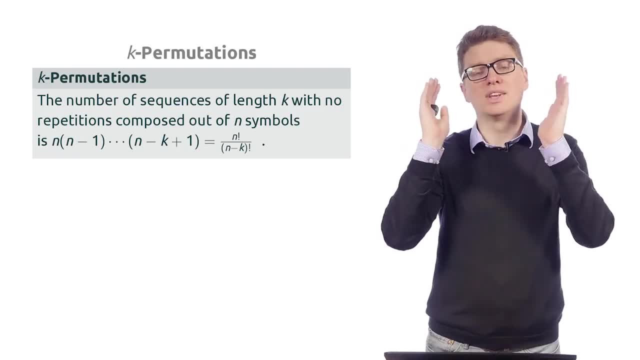 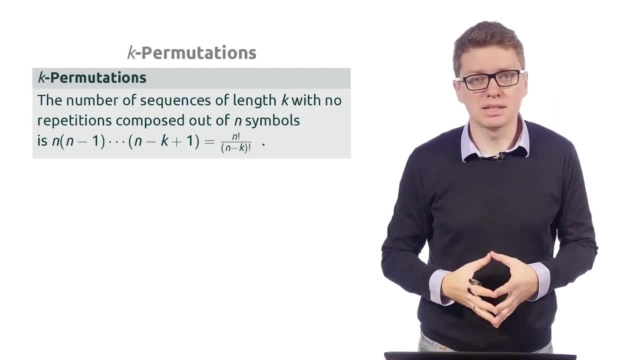 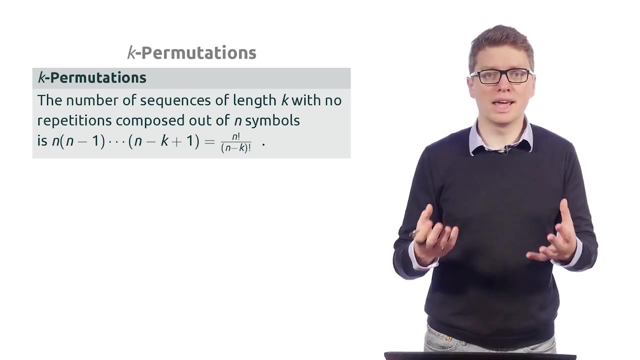 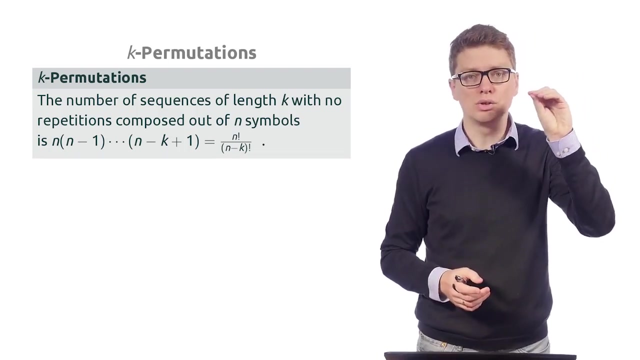 This Case, What You Would Like To Do Is To Given An Elements You Would Like To To Construct The K Permutation. Okay, So In 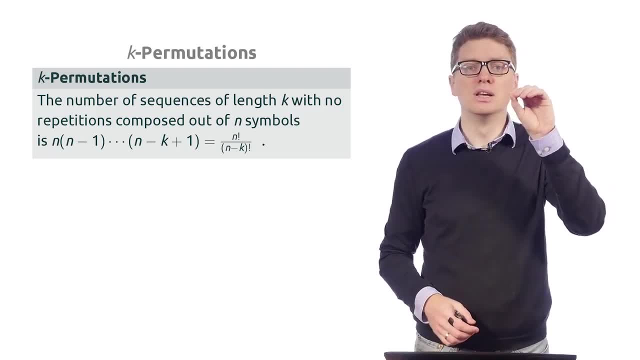 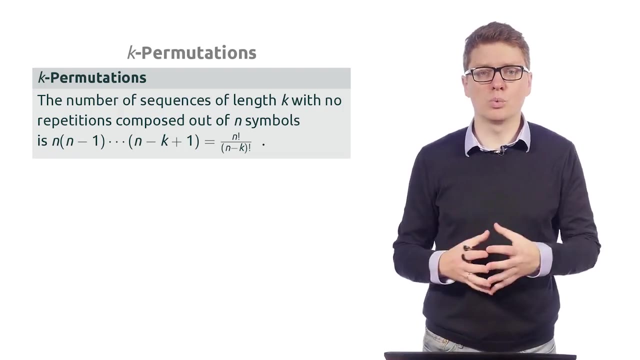 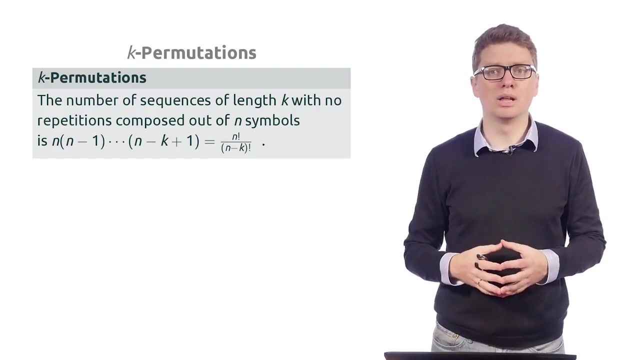 This Case, For The First Position, You Have N Choices Because You, Because You Can Select Any Of N Elements, You Have N Sum In The 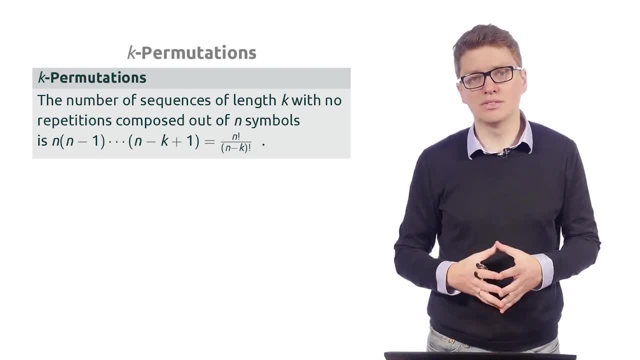 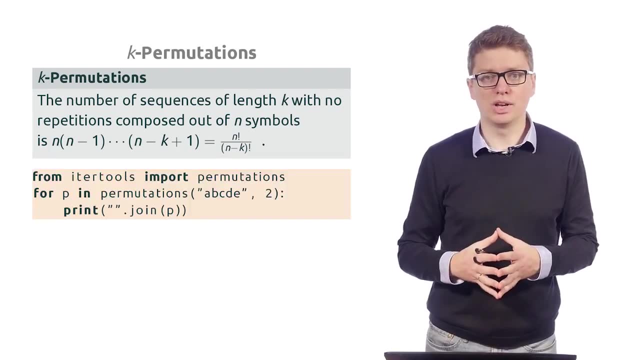 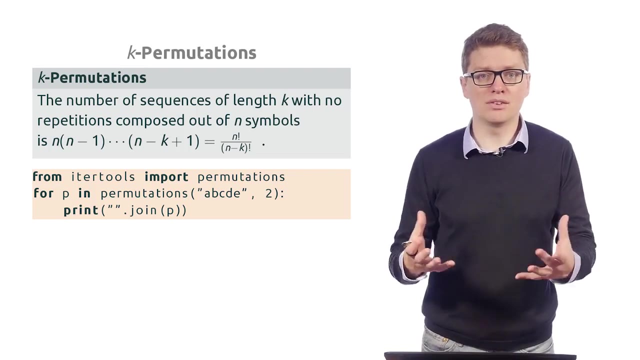 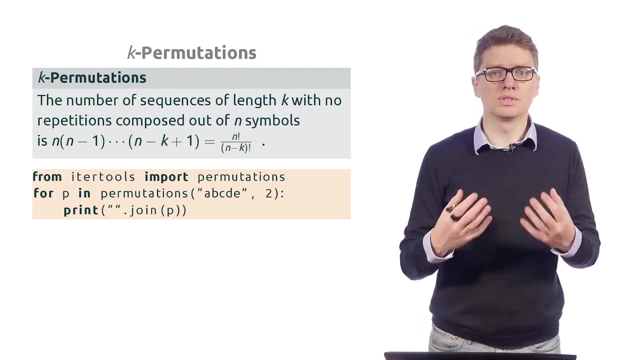 K Permutations. Okay, So You See That In This Case Is N And You Have A Term, This Problem, And You Can Dec of size 2.. So for the first position we have 5 choices. for the second, 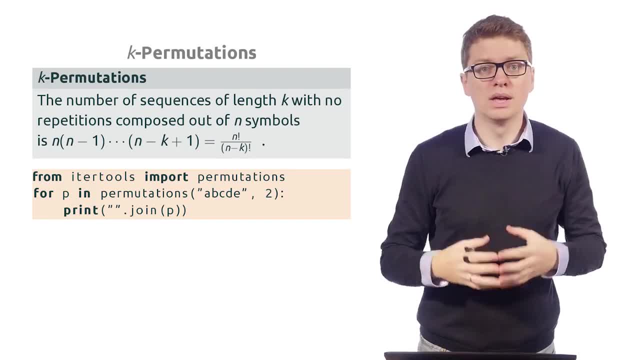 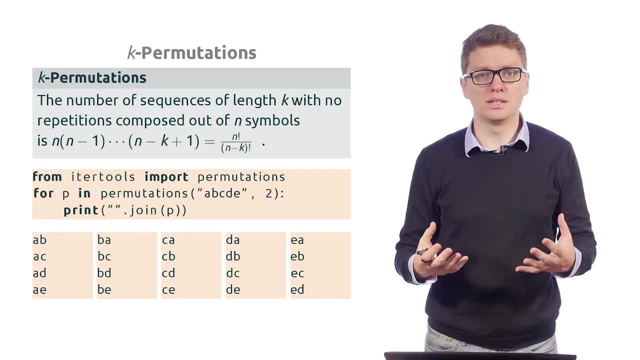 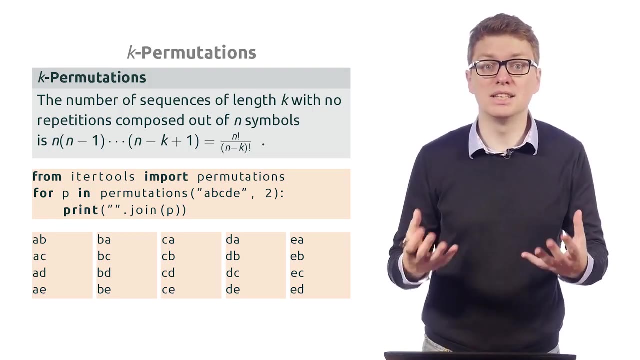 position. we have 4 choices, So the number of ways of doing so is equal to 20.. Let's check it. and indeed the following code produces us all 20 such 2 permutations. So it all starts with AB and it all ends with ED. Let's now. 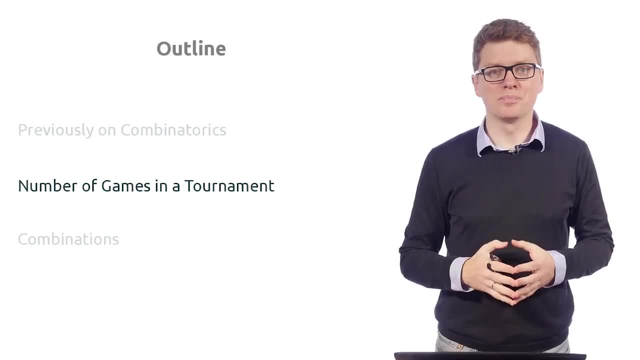 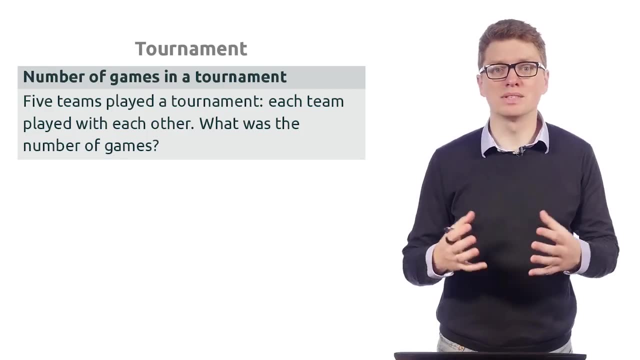 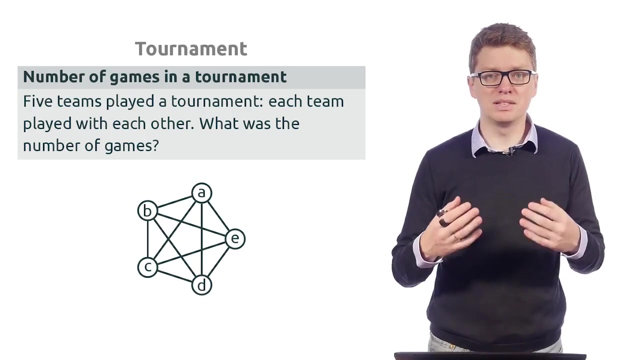 count the number of games in the tournament. More precisely, the setting is the following: We have 5 sport teams and they play the tournament, meaning that each team played with each other. So the question is: what was the number of games in this tournament? So visually it looks as follows: There are 5 teams: A, B, C, D and 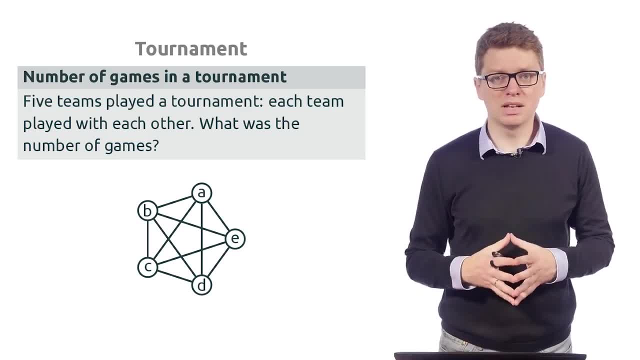 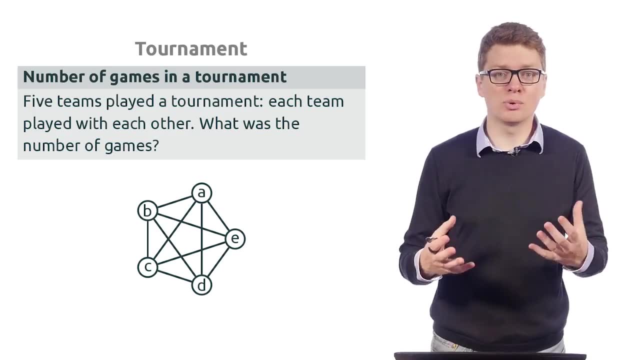 E, and every two of them are connected by a segment, meaning that they play the game. Basically, our goal is just to compute the number of segments. This is essentially a toy problem, but what we're going to do is to design a general formula, not for five teams, but for any number of teams. So let's start to. 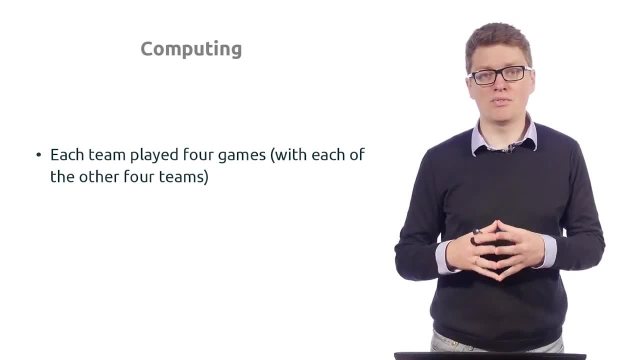 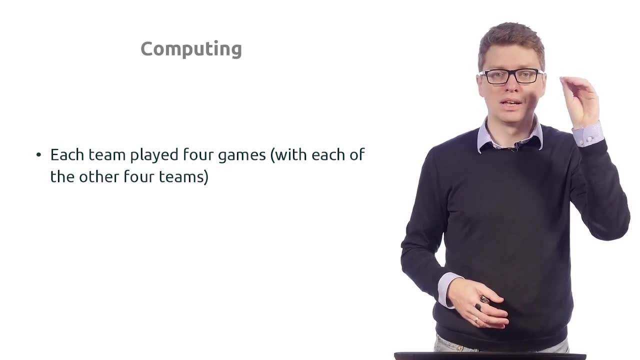 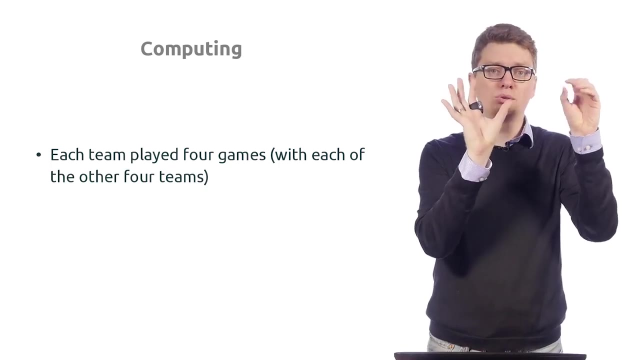 count. What we know is that there are five teams, so if we select any of them, then we know that each team played exactly four games. Why is that? Well, just because if a team is fixed, then there are four teams remaining and we know that this team played with every of these four teams. 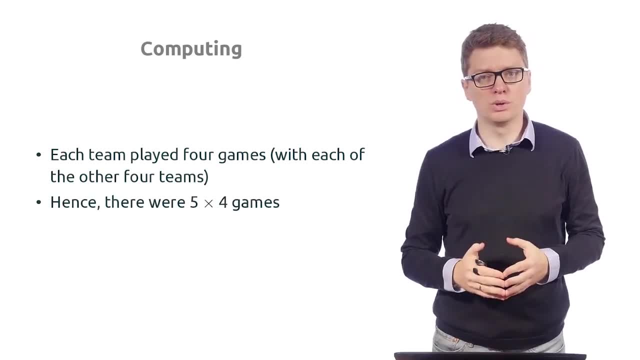 right, Which means that, by the product rule, what we know is that there are five teams and each of them played four games, which gives us 20 games, But there is actually a flaw in this argument, so let's try to catch it and let's try to. 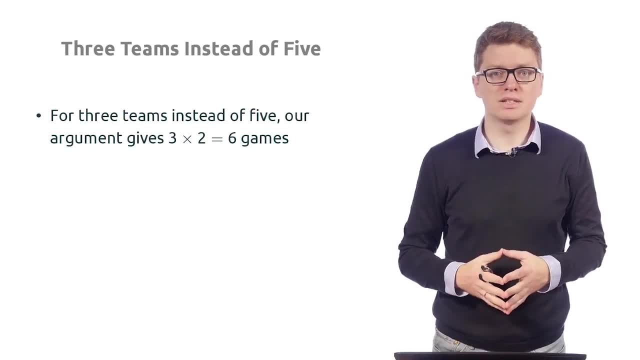 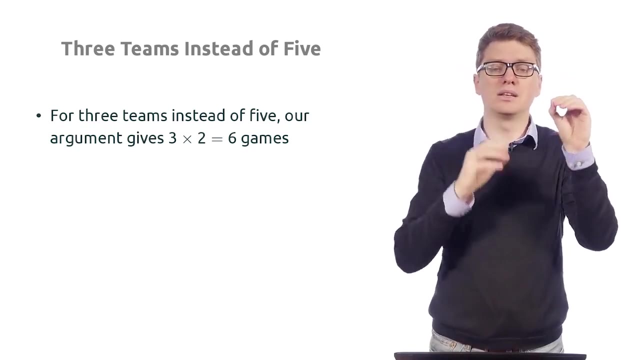 fix it, Okay. so first of all, let's decrease the number of teams. So imagine if we had just three teams, so what would happen? It actually gives that there are six games. Why is that? Well, there are three teams and each of them played two games with each of the remaining two teams, So the 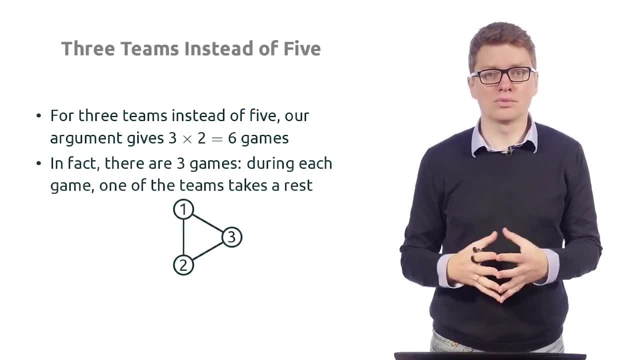 number of games is six, but this is not correct, of course, which can be just easily seen by considering this simple picture. So we have three teams, there is a segment between any of them, and the number of segments is three instead of six. right To understand? where is the flaw? let's just: 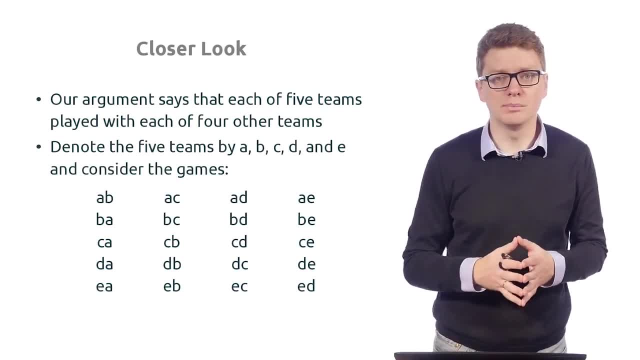 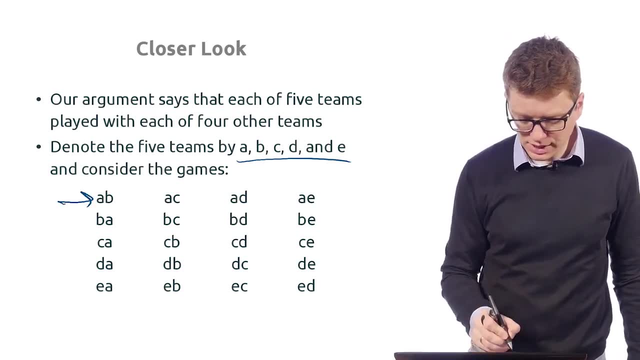 draw all possible games. Okay, so we have five teams: A, B, C, D and E. So in the first row we have all the games played by the team A. So we played, indeed, with AB, with AC, with AD and AE. Makes sense, right. So for the second row. 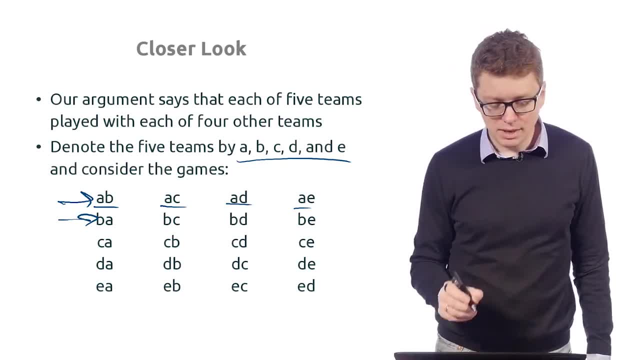 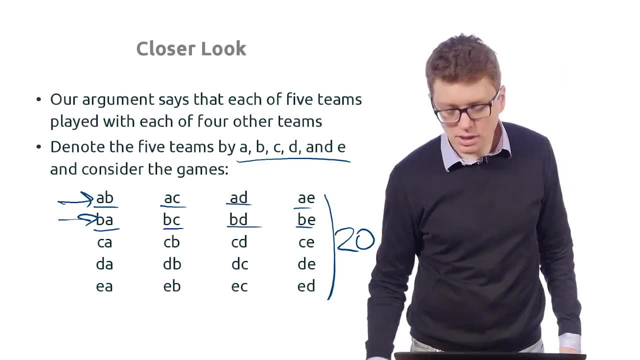 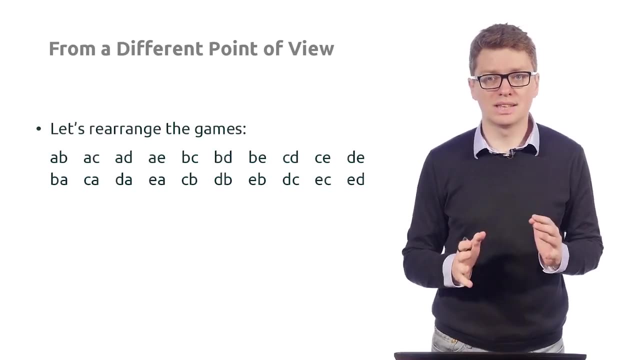 lists all the games played by the team B. It played with A, with C, with D and with E. So still it for some reason gives us 20 games in total. To understand what went wrong, let's try to rearrange all these games as follows. So we still have two rows and ten columns. 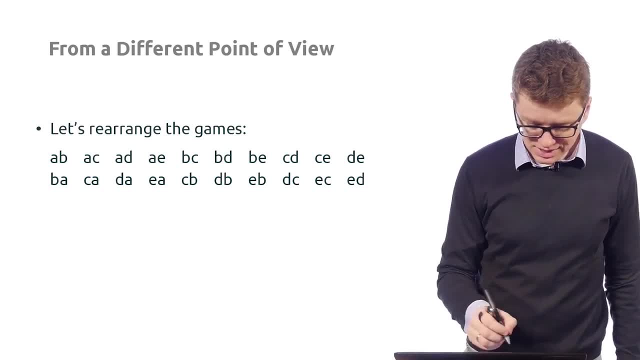 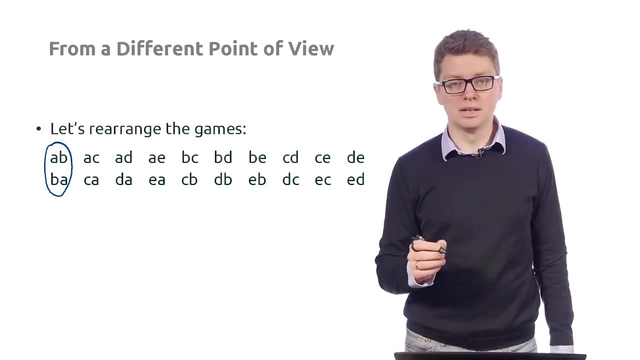 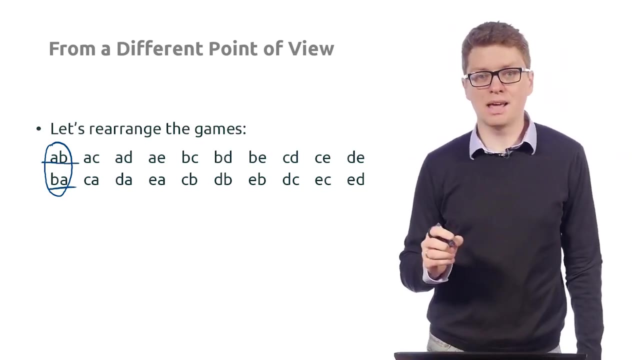 so there are still 20 games At the same time. in this table it can be easily seen that each game is actually counted twice. So we see that we counted the game between the teams A and B as AB and BA, And this happened actually with every game, For example, the game between 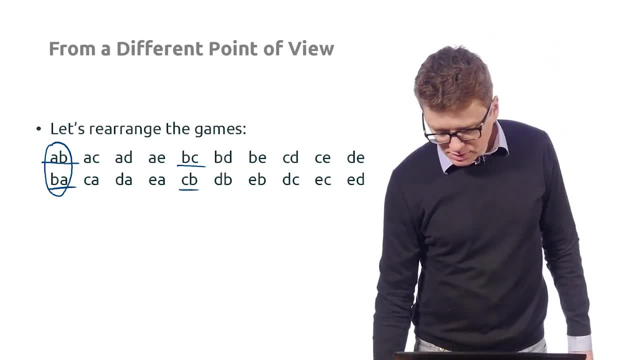 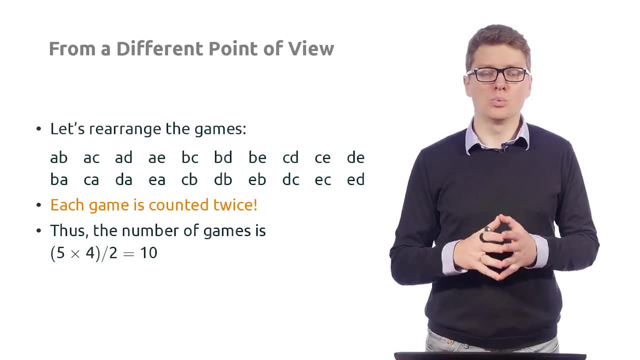 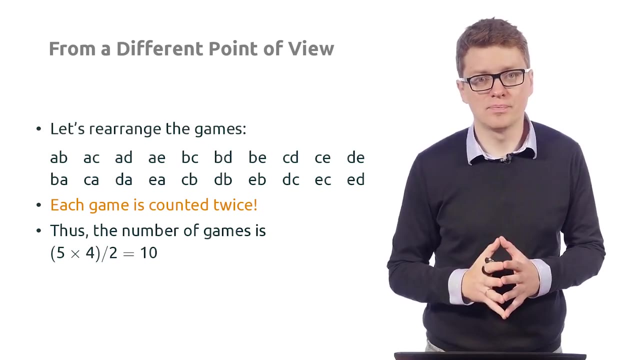 B and C was counted as BC and CB, So this was our overestimation. So each game was counted exactly twice, which means that we actually need to divide our resulting count by two, which finally gives us a correct result: It is 10.. Okay, So there is an important message. 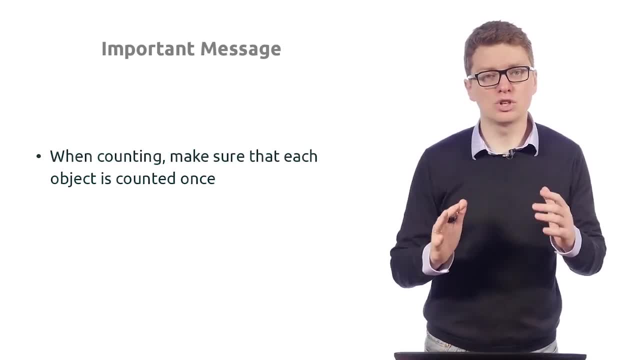 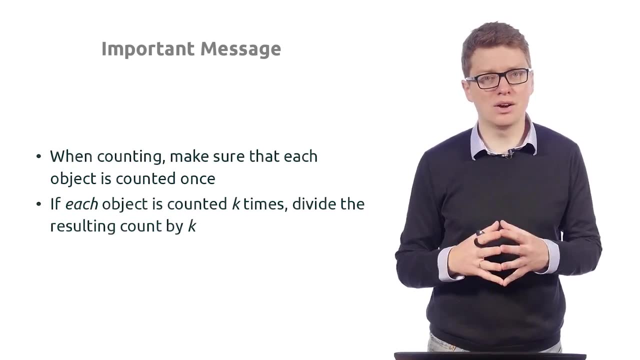 for us. When we count something, we need to make sure that each object was counted exactly once. But if it turned out, as in our example, that we for some reason counted each object exactly K times, then it is easy to get the correct result. What we need to do is just to divide by K, So in. 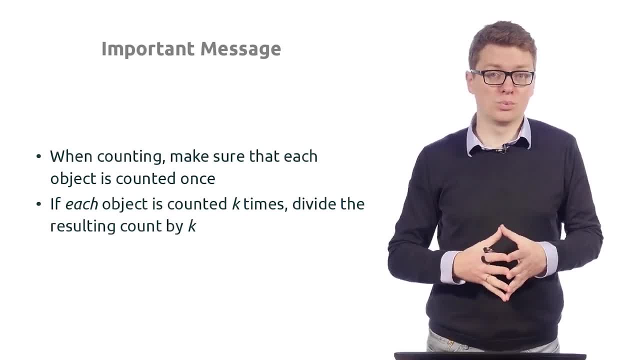 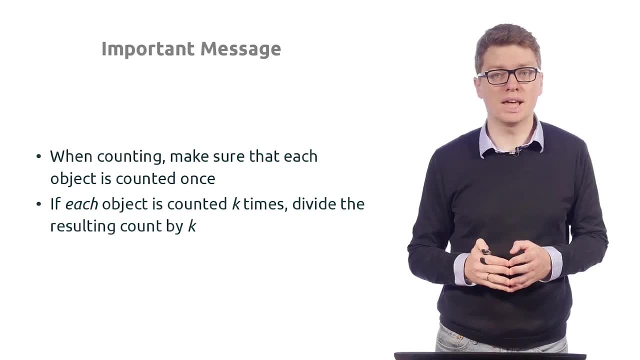 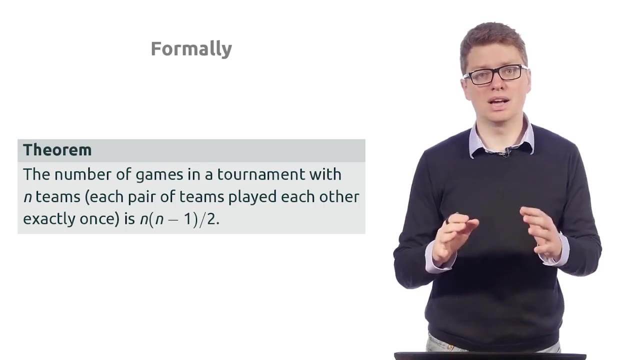 our case, we counted each game two times, So what was need to be done is to divide everything by two. Okay, Now let's generalize it to arbitrary number of teams. The theorem here on the slide states that if we have n teams, then the number of games in a tournament where each game plays 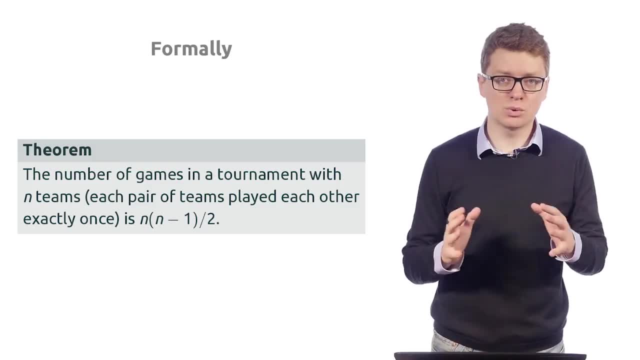 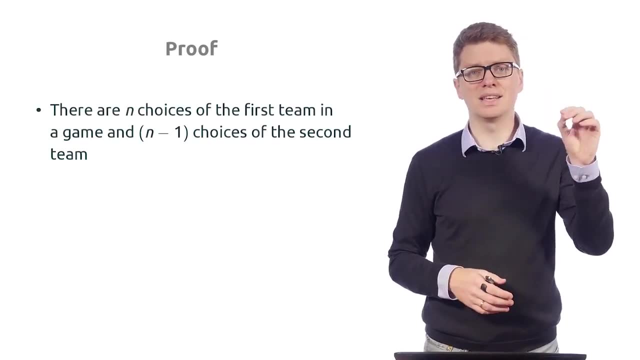 with each other exactly once is equal to n times n minus one divided by two. Okay, Let's prove it. So there are n teams. Each of them plays exactly n minus one games, because there are exactly n minus ones, And so we need to divide by two. Okay, So let's generalize it to arbitrary number of teams. 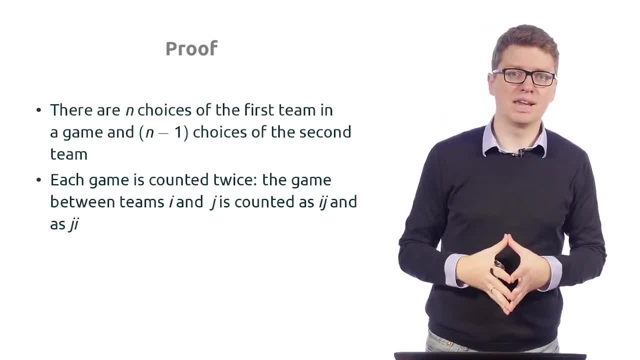 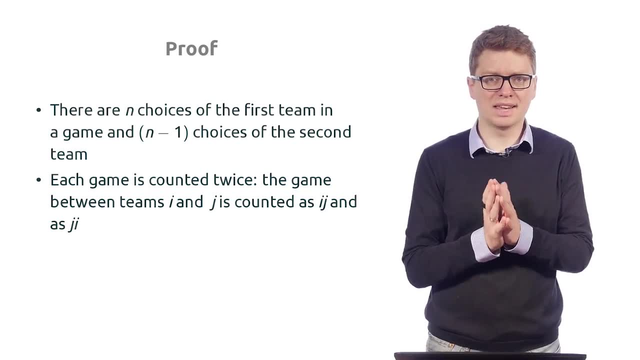 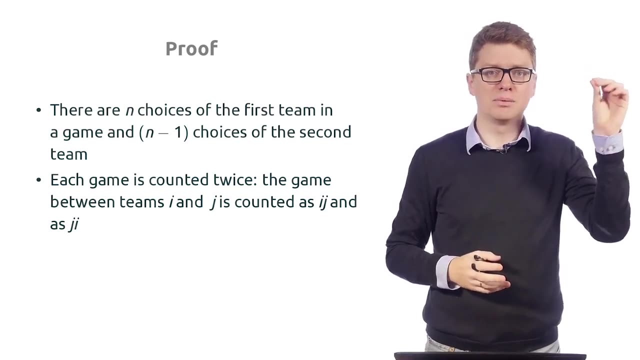 teams remaining okay. so the total number of games, is is n times n minus 1, but at the same time each game is counted twice, because if a game involves teams I and J, then it was counted twice, first when we fixed the team I, and then it was playing. 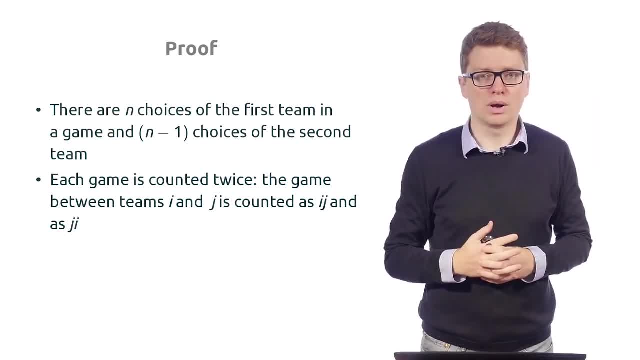 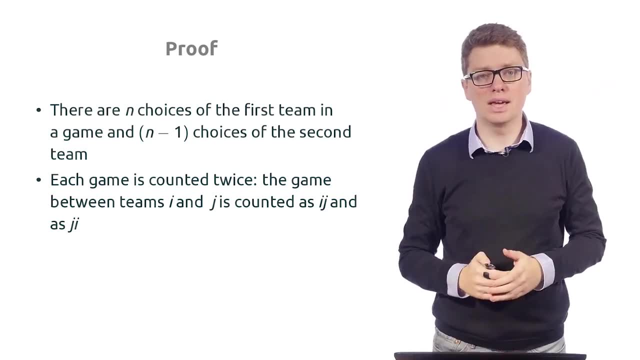 with the game with the team J, and on the other hand, it was also counted when we fixed a team J, the team J, and then we counted the game as J I. okay, so we need to compute the product of n and n minus 1, and then divided by 2, this is the. 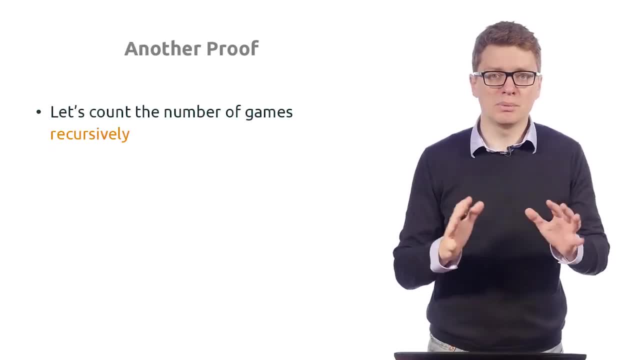 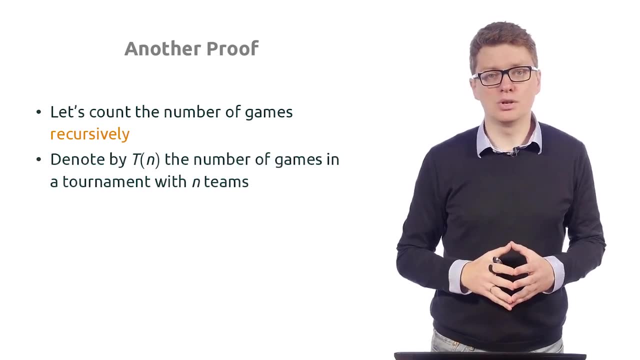 resulting number. okay, let's also complement it, this, with a recursive proof of the same formula. okay, so for this, let's denote by T of n the number of games in a tournament with n teams. okay, then we need to compute the number of games in a tournament with n teams. okay. 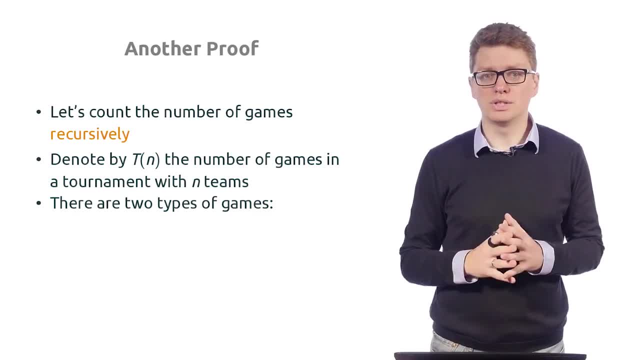 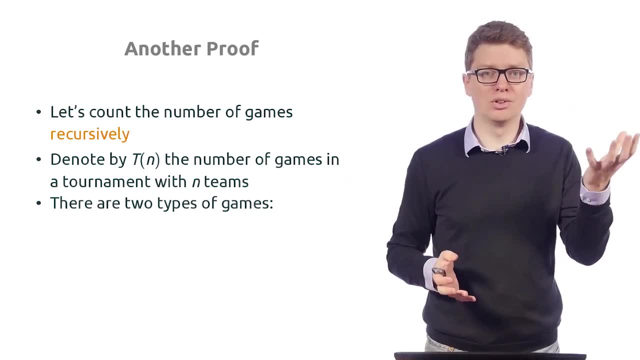 then we need to compute the number of games in a tournament with n teams. okay, to get a recurrence relation for T of n, let's do the following: let's split all the games into two parts. on one hand, we have all teams involving the first team. okay, so there are exactly n minus 1 such games. why is that? well, because the 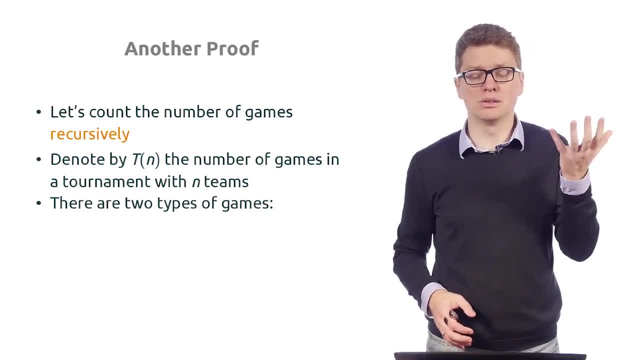 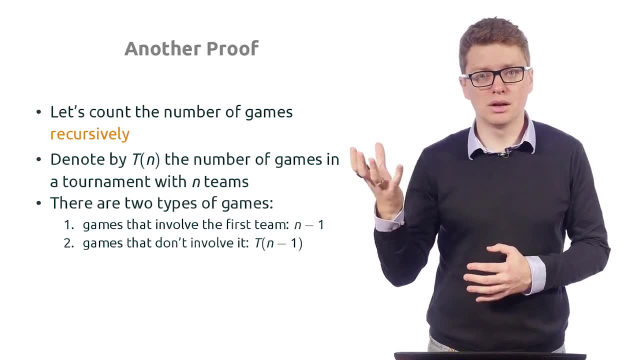 first team played exactly n minus 1 games. we know this already. on the other hand, we have all the remaining games, that is, all the games that do not involve the first team, but this is the same as exact as just all the games played by all the. 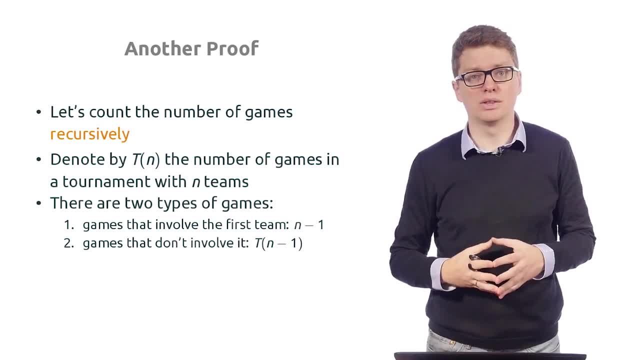 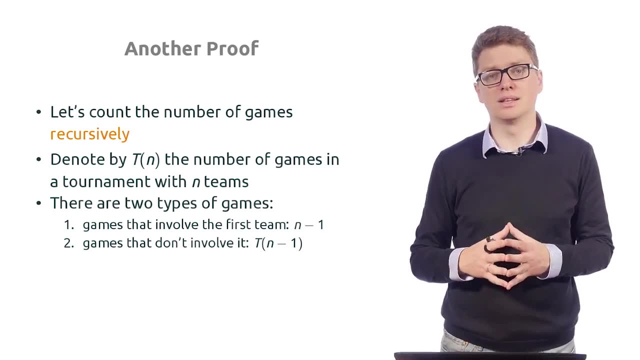 remaining teams, but this is nothing else as T of n minus 1, right? so just by definition, we need to count all the games played by the, by the teams 2, 3 and so on: n, so there are n minus 1 such teams. so, and we know that by: 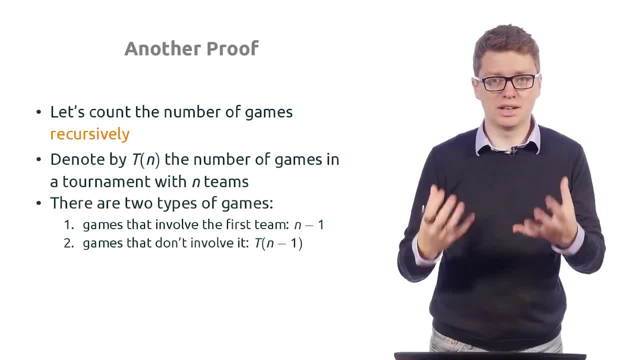 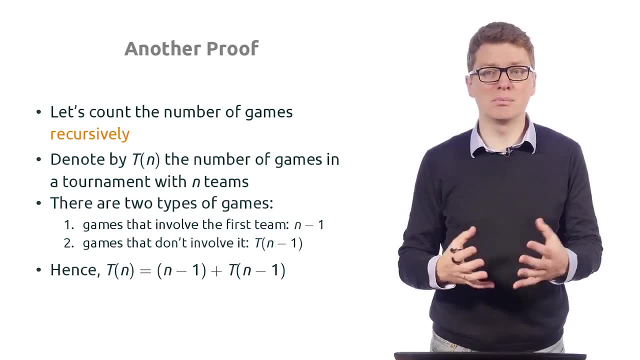 definition. T of n minus 1 is exactly. this number is exactly the number of games played by n minus 1 teams. this gives us the following recurrence relations: your fan is equal to n minus 1 plus T of n minus 1. so now we need to somehow get a formula for T of n from this recurrence relation. okay, 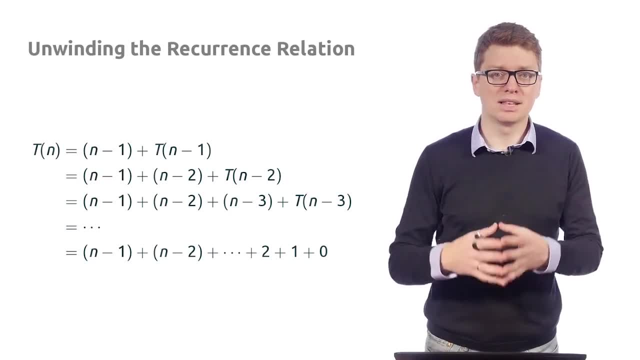 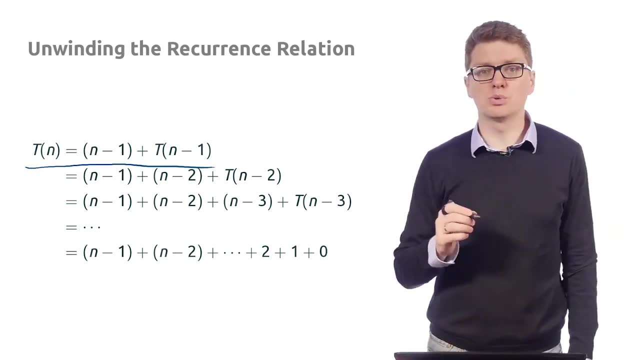 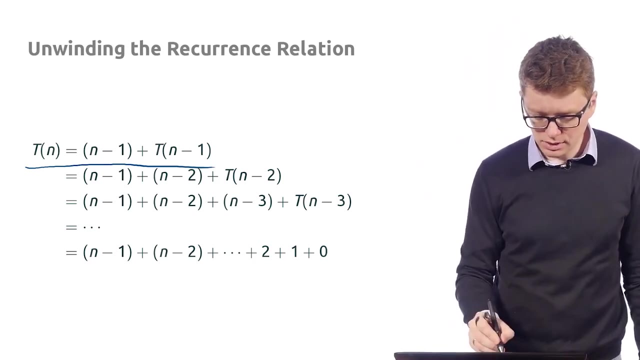 and for this we are going to apply the method, the so-called method of unwinding. mainly, let's first write our formula: T of n is equal to n minus 1 plus T plus T of n minus 1, but then we can apply the same formula for T of n minus 1, so we leave. 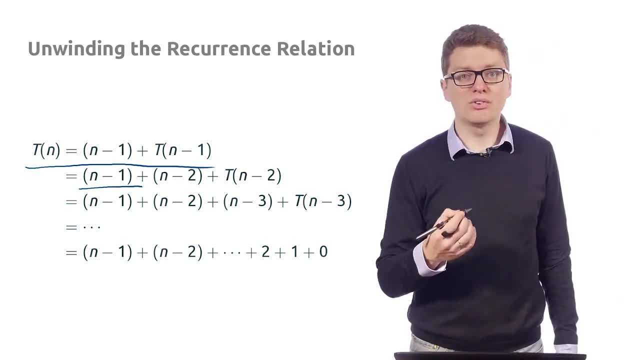 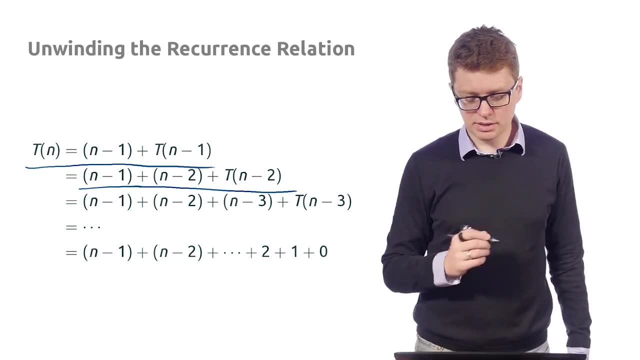 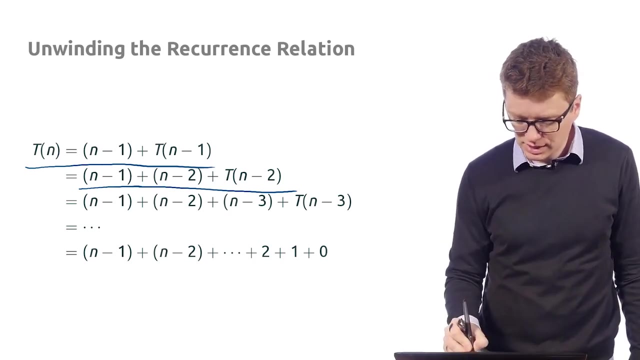 n minus 1, but for T of n minus 1 we rewrite it as n minus 2 plus T of n minus 2. so we apply the same formulas. this gives us n minus 2 plus T of n minus 2. okay, but then we do the same with T of n minus 2. okay, this gives us n. 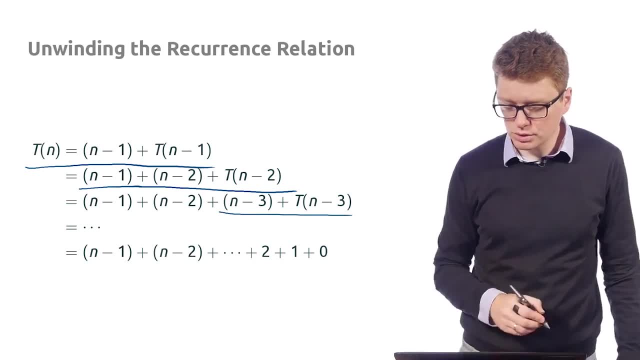 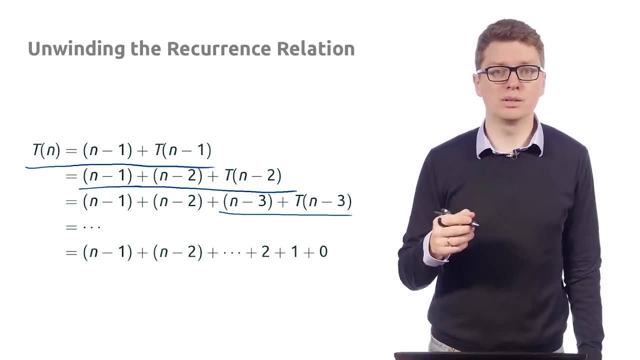 minus 3, plus T of n minus 3, and so on. so we keep repeating this until we reach T of 1 or T of 0, which is in any case equal to 0, right, because if we have 0 T teams or if we have 1 team, then the number of games is in any case equal to. 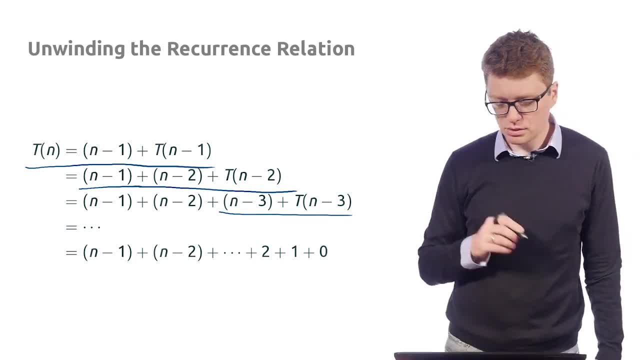 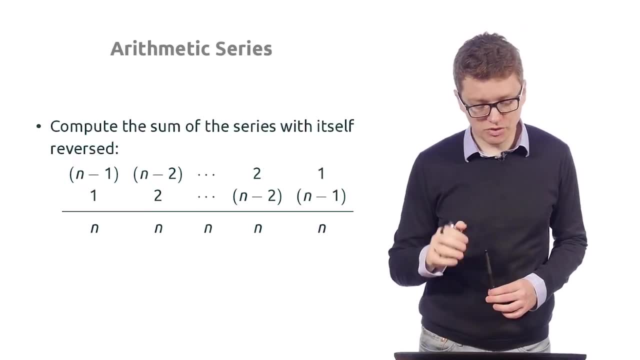 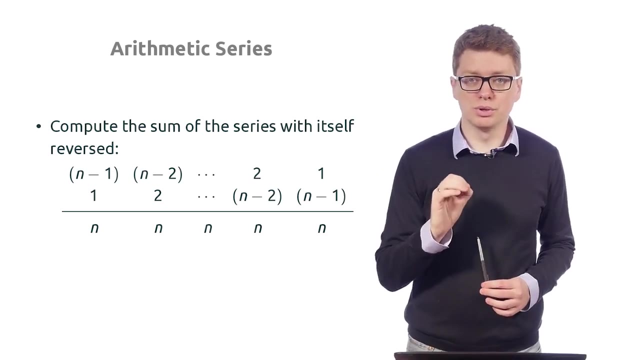 0. what remains is n minus 1 plus n minus 2 plus, and so on: plus 2 plus 1 plus 0. this is the so-called arithmetic series. okay, let me remind you how to compute the sum of such series, then. a simple but but useful trick to remember. here is the: 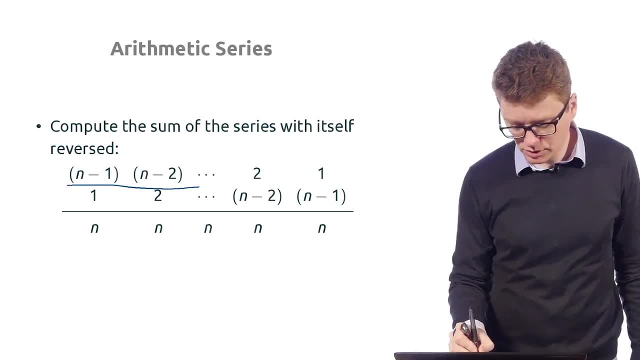 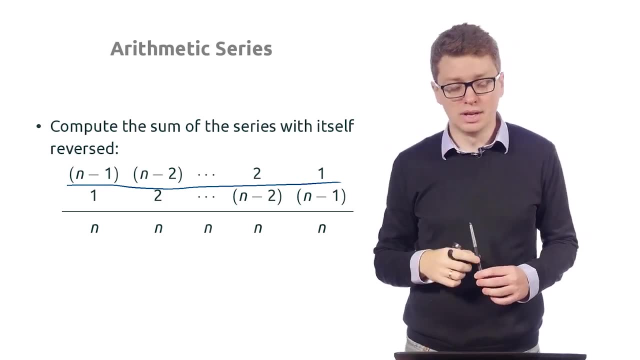 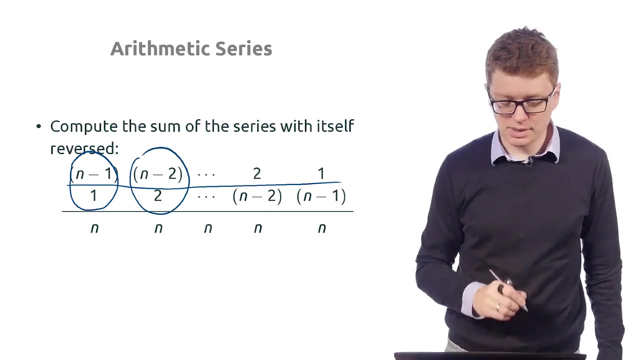 following: if you write all the all the terms in your arithmetic series and then you write the series once again, but in the reverse order, then what is convenient is that in every, in every column, the sum is going to be the same and it is going to equal. it is equal to just N, which means that it is very easy. 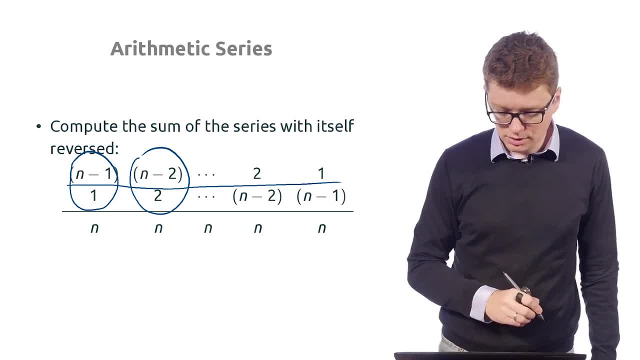 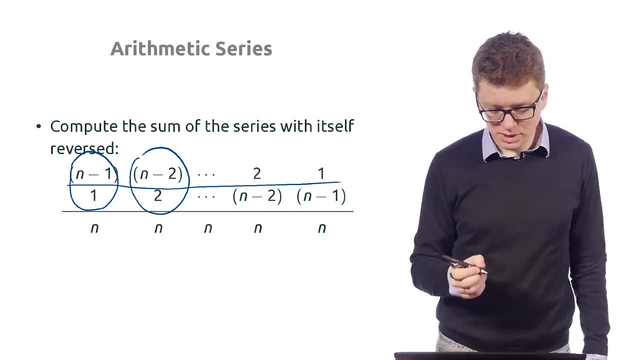 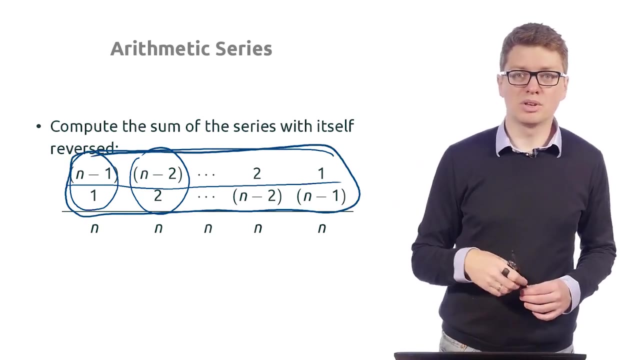 to compute the sum of all the numbers shown here on the slide. so we have N minus 1 columns right and then each column. the sum is equal to Jack, which means that the sample of the numbers that we have at the in the order of two of all these numbers is equal to n times n minus 1.. At the same time, to get the 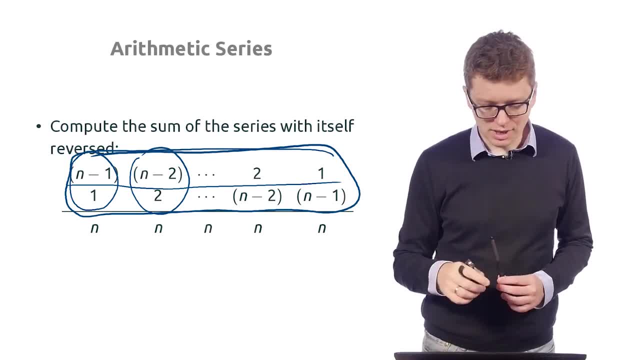 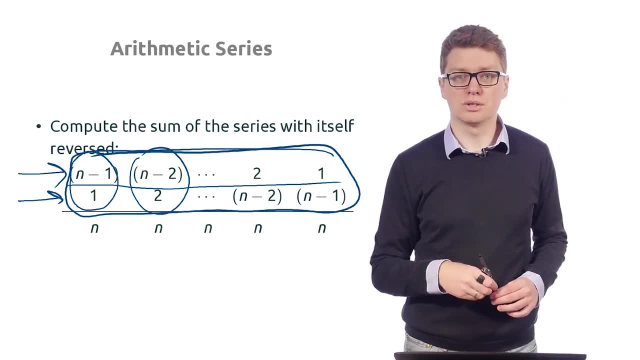 sum for arithmetic series. we need to remember that we counted it twice here, right? So this is our original series and it is the reversed original series, So the sum in these two guys are the same, of course, which finally means that for: 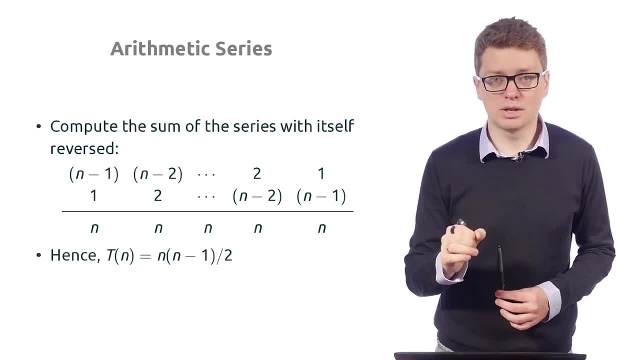 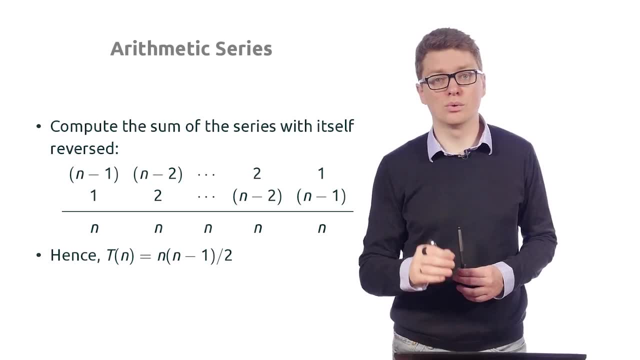 the arithmetic series, the sum is equal to n times n minus 1, divided by 2.. And this also is the answer for t of n. So this is another proof of the same formula. The number of games in the tournament is equal to n times n minus 1. 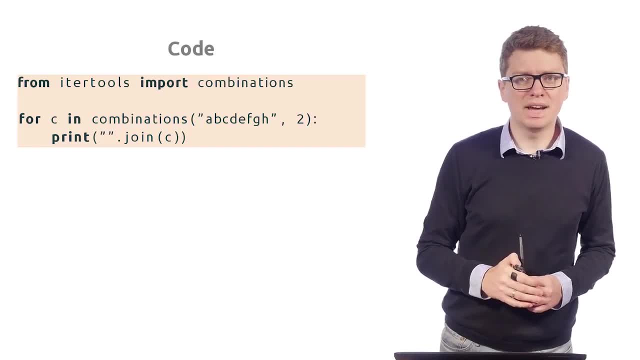 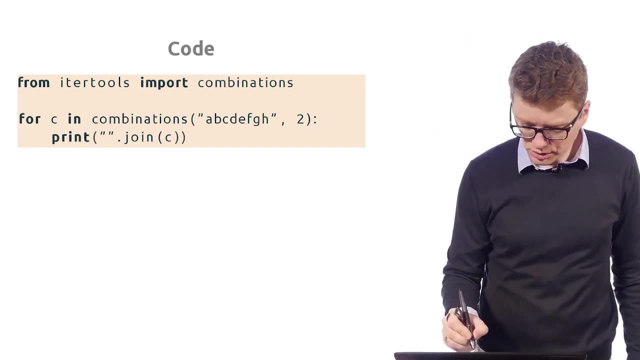 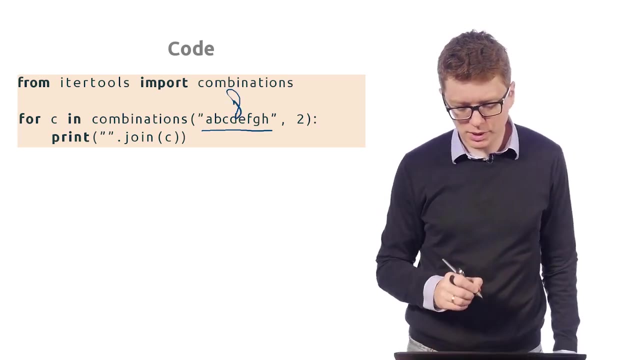 divided by 2, okay, So finally, let me complement it, as usual, with a simple script in Python. So, for this, what we're going to do here is to take eight teams: A, B, C, D, E, F, G, H. So there are eight teams and we are going to using the. 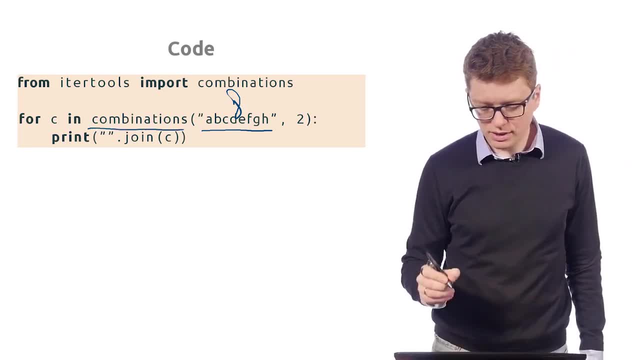 combination of these two. we are going to take eight teams and we are going to use the combination of these two. we are going to take eight teams and we are going to take eight teams and we are going to use the combination of these two. So, in this next explanation method, we're going to generate all possible. 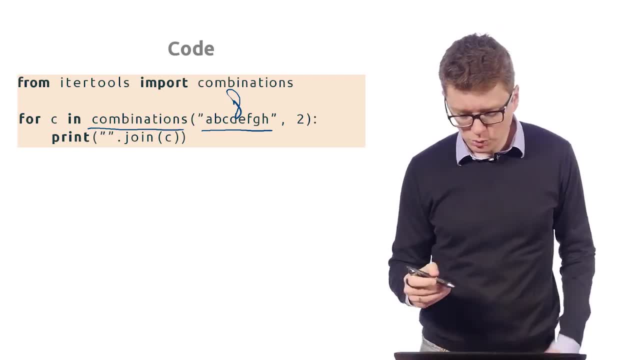 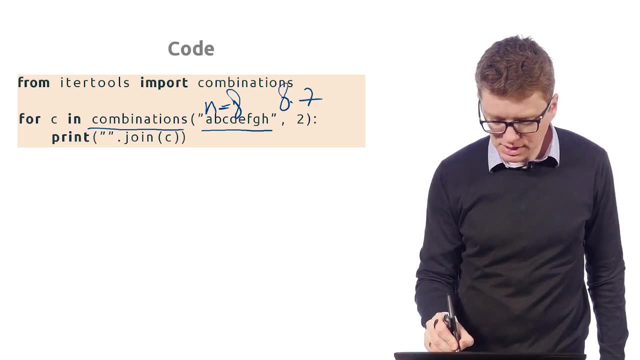 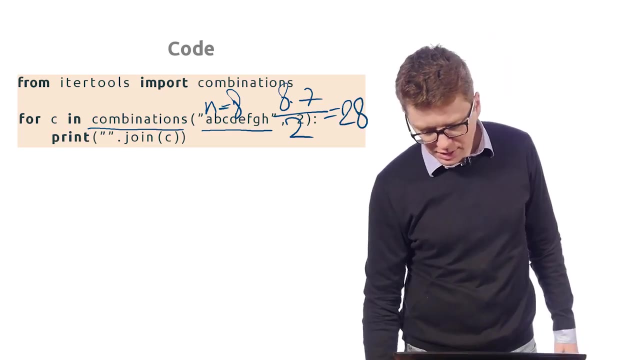 games between these eight teams. So what we expect to get is: N is equal to 8 in this case. So the formula gives us: 8 times 7, divided by 2, which is just 7 by 4,, which is nothing else, is 28.. Right, So let's run this script and indeed, 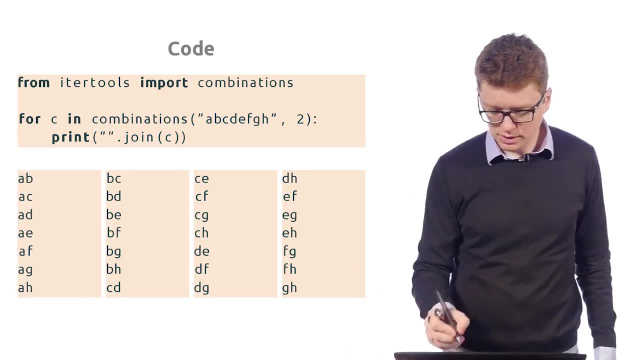 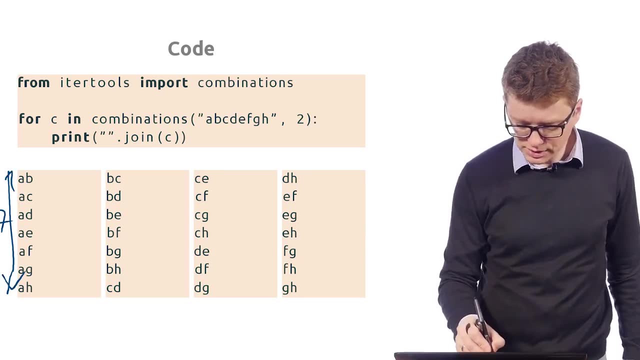 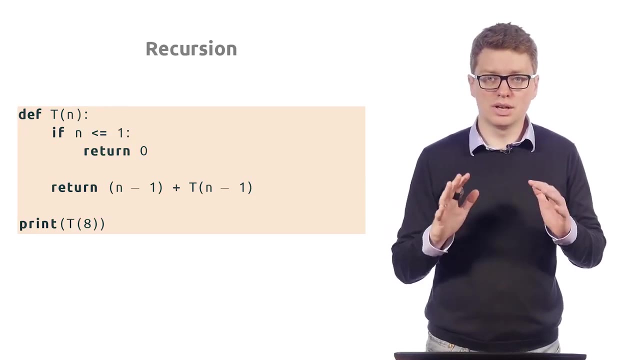 it produces all possible 28 silver teams. So we guessed that we will get that. everything should be equal to 7.. So such games. so the length of each list here is four, and there are four lists, okay, okay, and finally, let's, let's do the following: let's also show that the, our recurrent formula also produces exactly. 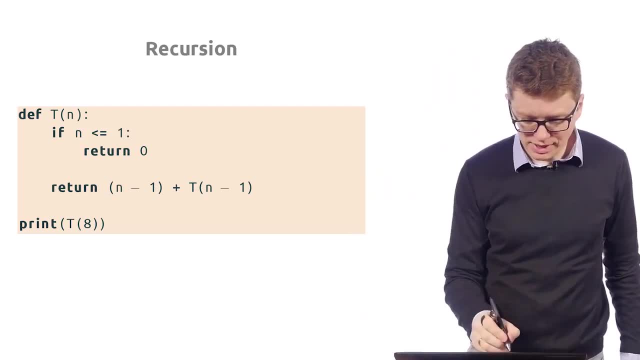 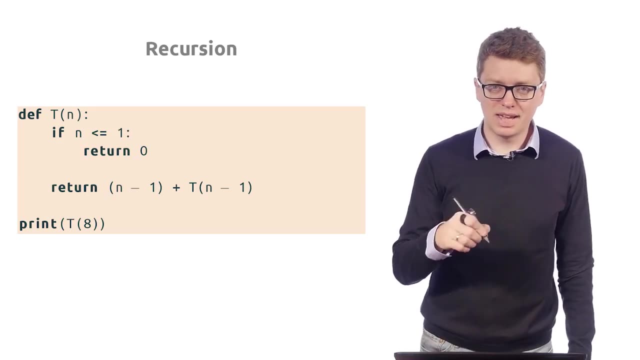 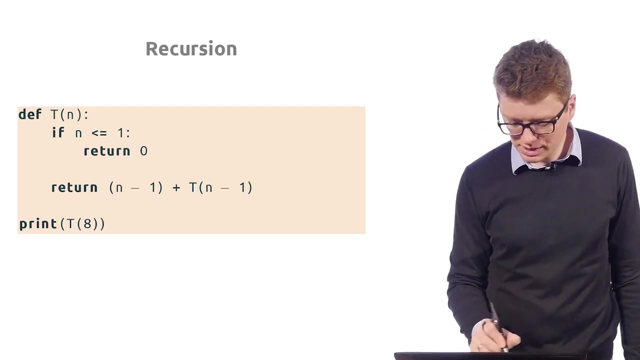 the same result, namely, this was, as you remember, when t of n was defined to satisfy. t of n was defined to be the number of games in a tournament with m teams, and we proved that it satisfies the following formula: it is equal to n minus 1 plus t of n minus 1, and this allows us to just 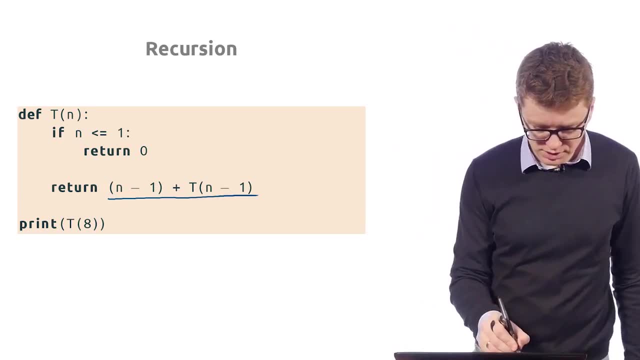 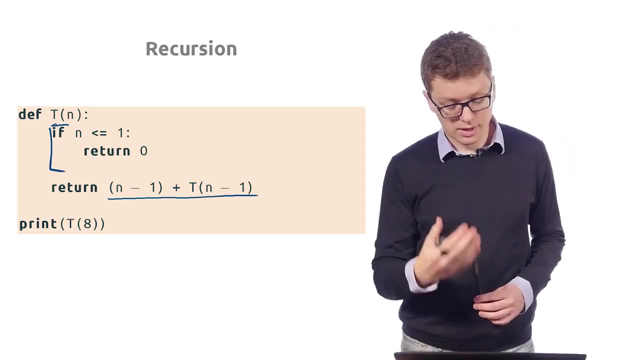 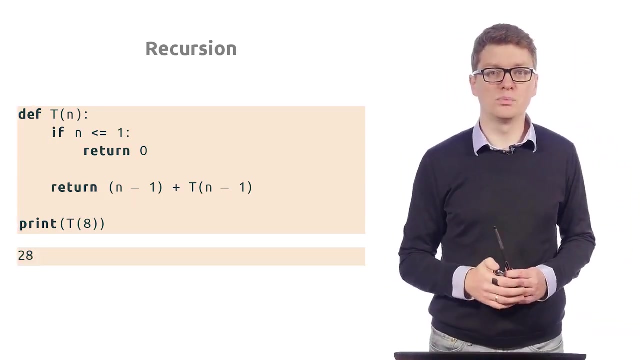 implement the following recursive procedure with with the following base case: when n is at most 1, we just return 0 immediately. so if we then implement this procedure and task it to compute t of a, then the output is going to be the same as the number of games in a tournament with n teams. 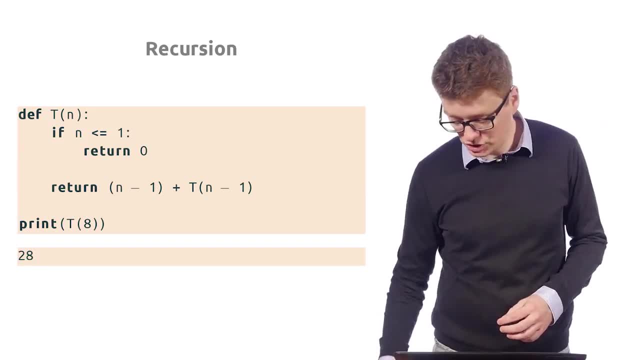 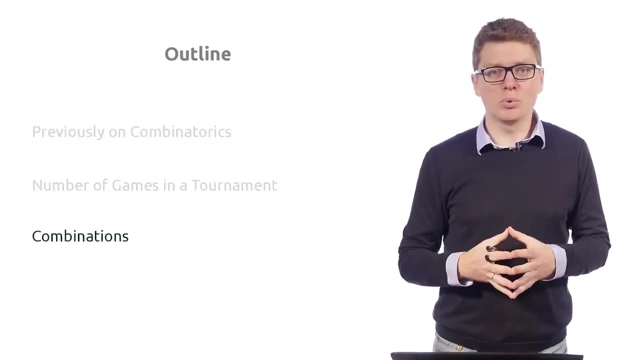 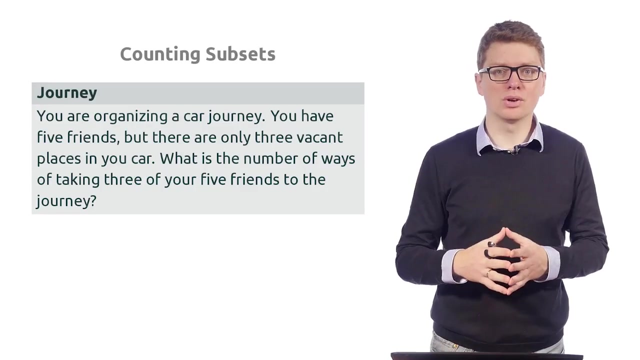 be as expected. 28, which justifies our previous formula. we are now ready to introduce an important combinatorial object called the combination. so imagine that you are going to a car journey and you have five friends, but unfortunately you have only three vacant places in your car. so what you? 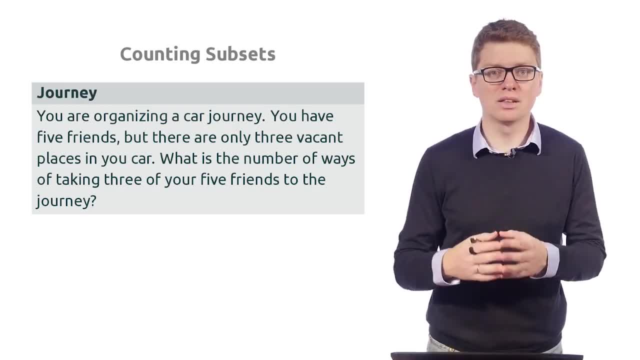 would like to compute is the number of ways of selecting the number of games in a tournament and the number of ways of selecting three of your friends out of five your that you are going to take with you to your journey out of five of your friends. okay, of course, in this case we don't care. 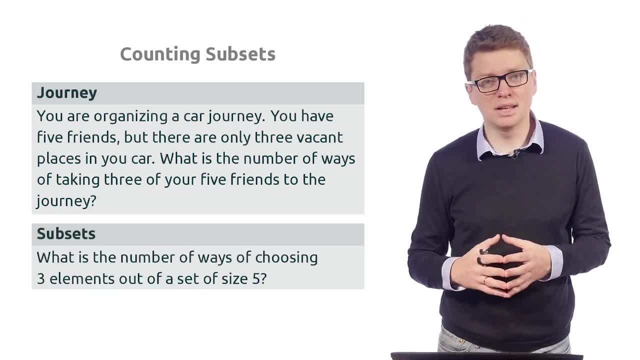 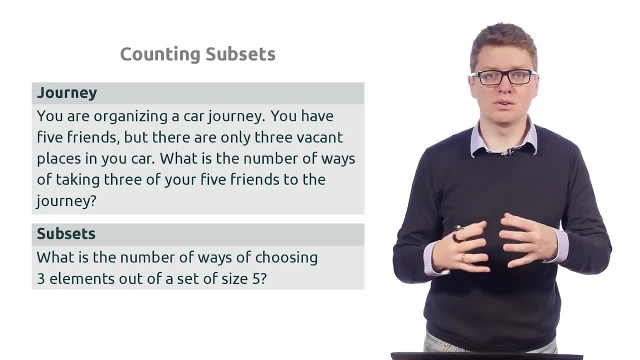 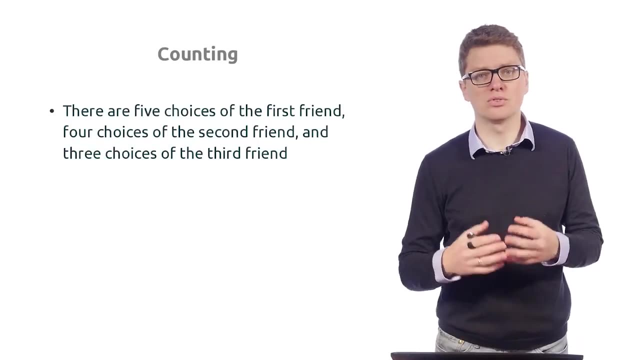 who of your three friends is going to sit where in in the car. so, basically, what we're looking for, uh, so speaking more formally, is what is the number of ways of selecting three elements out of five elements? okay, let's try to compute this number of ways. so you need to select three friends. there are five. 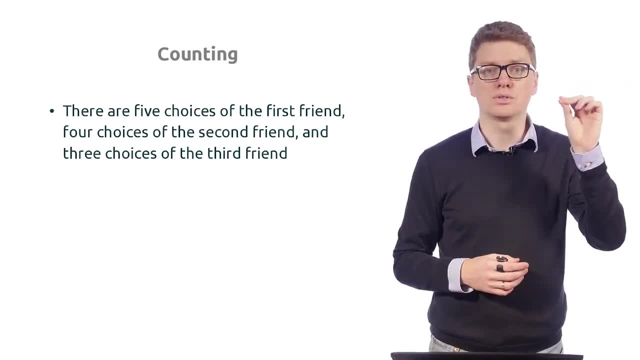 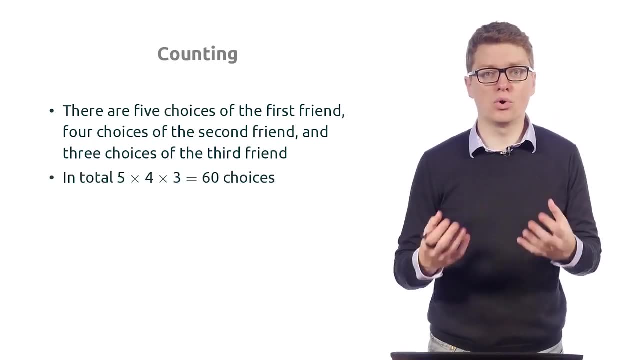 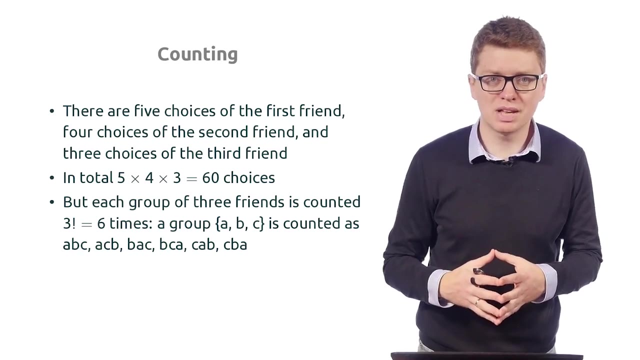 choices of the first trend, four choices of the second friend and three choices of the third friend. right? so this gives us four five times four times three, but, as we've seen already, this actually computes not the number of subsets of three friends, but the number of, uh, like three permutations, right? 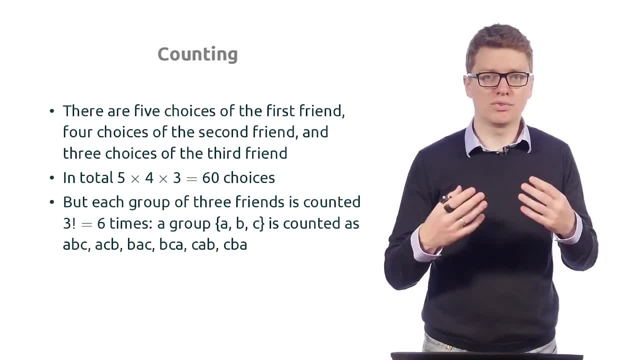 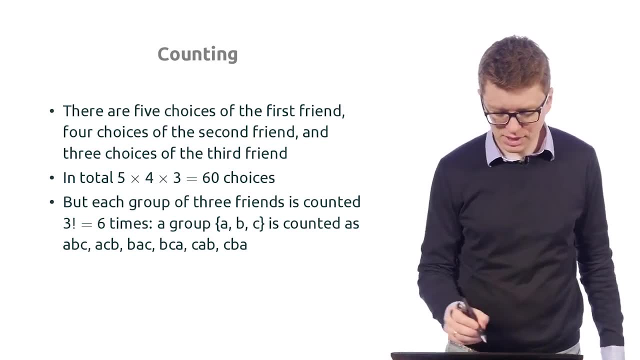 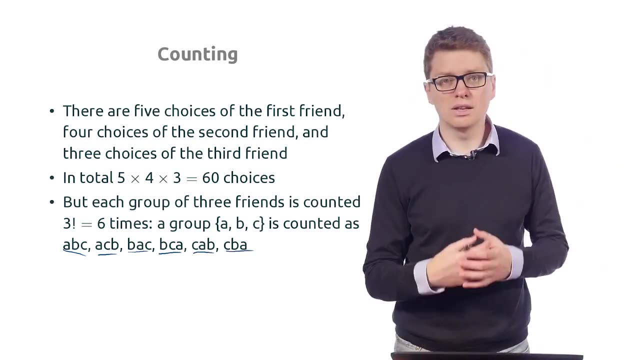 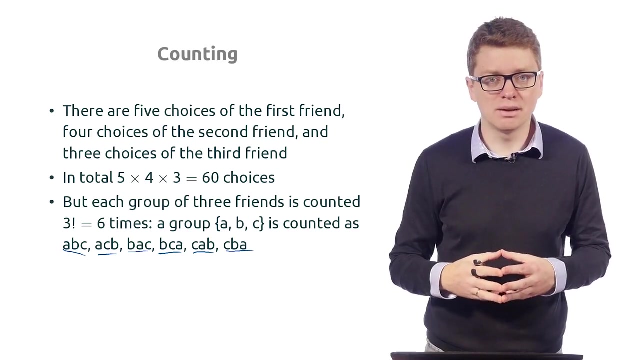 in particular, each subset uh, for example, of friends, abc was, uh- was counted six times. it was counted as abc, for example, as acb is, as bac, bca, cab and cba. but since we are not interested in the actual arrangement of these three elements, we need to divide everything by by six, right, uh? so we we. 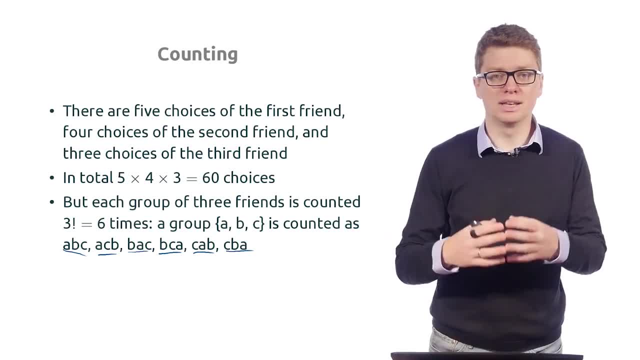 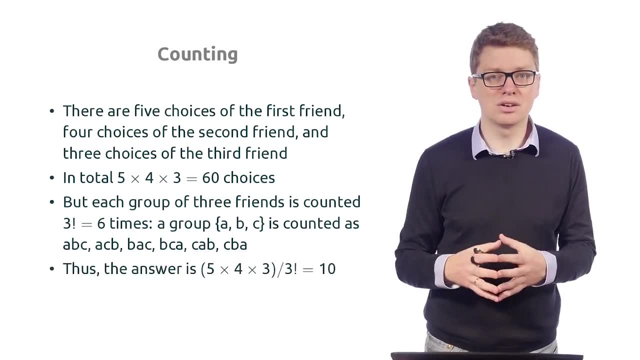 would like to count each subset exactly the same way. we would like to divide everything by by six, exactly once, while it- uh, you know, in our current estimate it was counted exactly six times. so the final answer is four is five- i'm sorry times- four times three, divided by three: factorial. 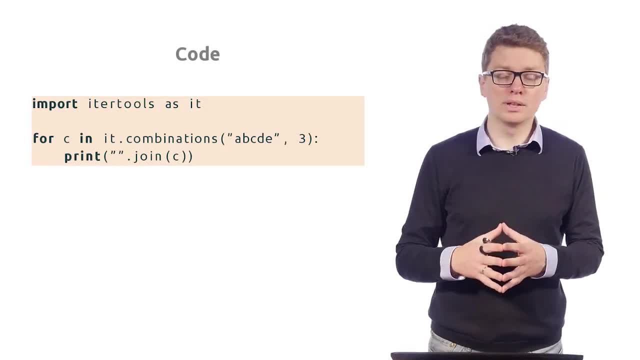 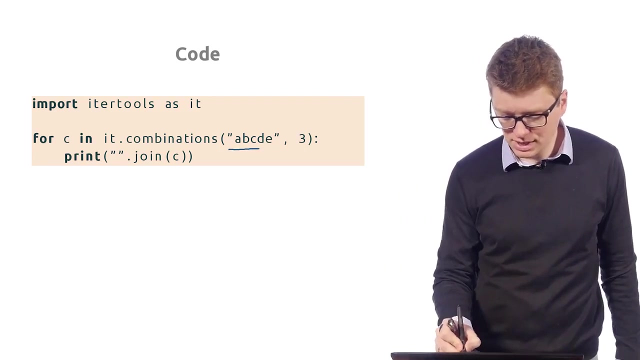 which gives us ten. so this is an important combinatorial quantity. let's also justify our count just by trying to to generate all such combinations. uh, namely, here we have five friends- a, b, c, d, e, and we we ask the combinations method to compute all possible. 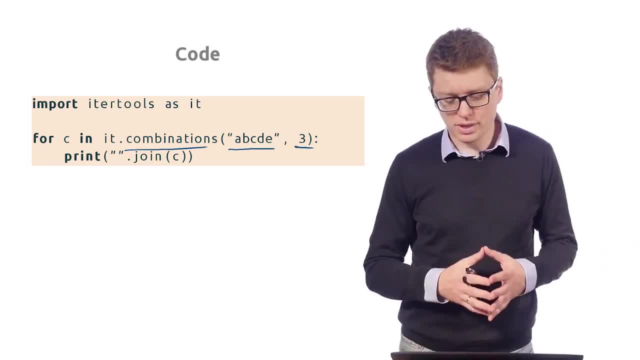 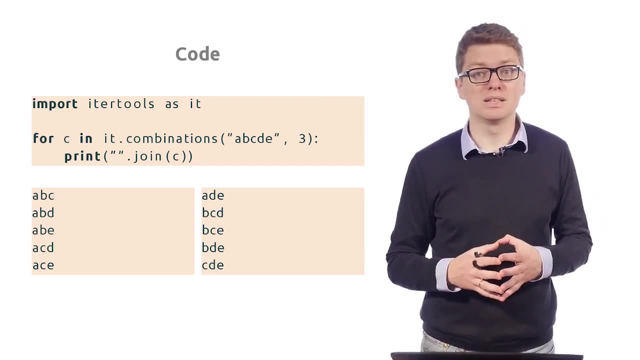 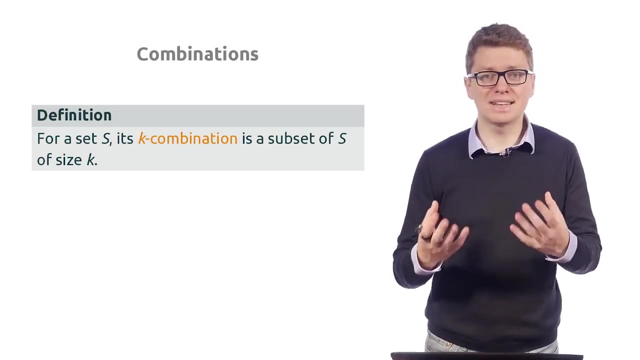 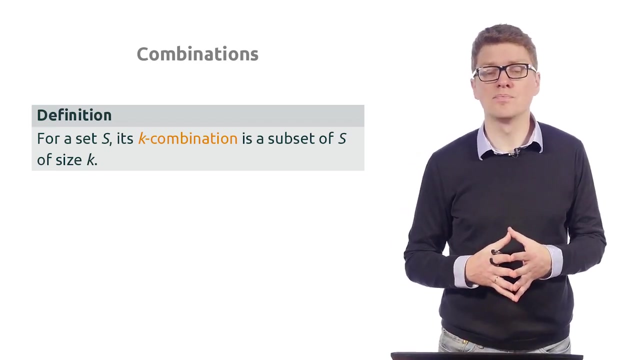 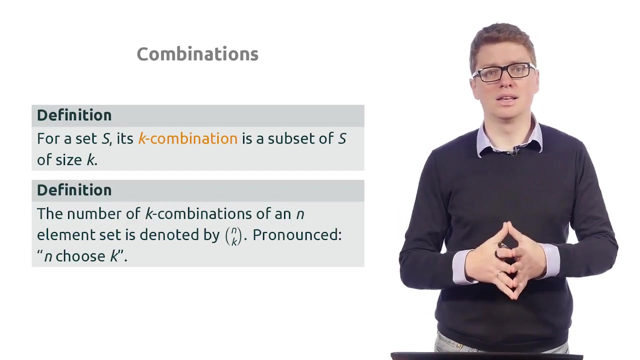 subsets of size three of of all these five letters. so what it gives us is exactly 10 such possibilities. okay, now we are ready to give a definition. so if we have a set s, then it's k combination is any its set of size k. okay, so, and the number of different such subsets of size k is uh is denoted by n choose. 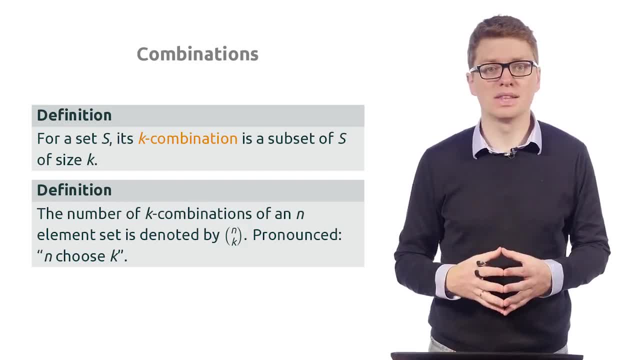 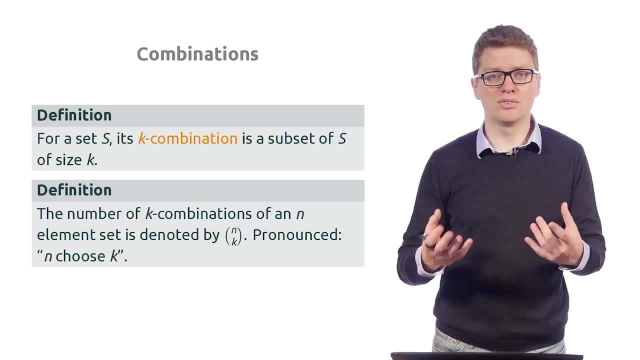 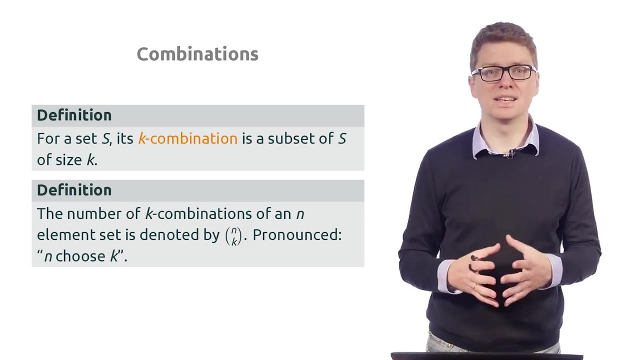 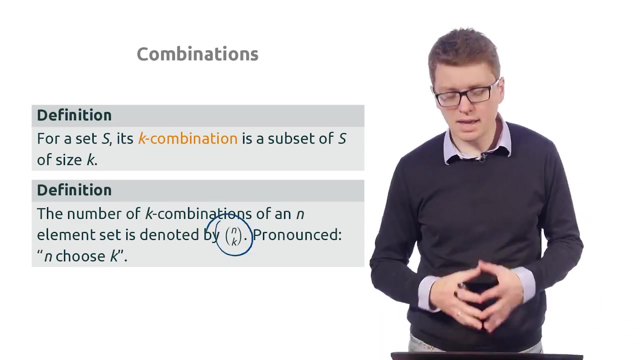 k. so where n is the size of the set s. so more precisely or more formally, n choose k is defined to be the number of different subsets of of size k of an n element set, and once again it is n choose k and it is written like like this: okay, so this is a very important combinatorial quantity. 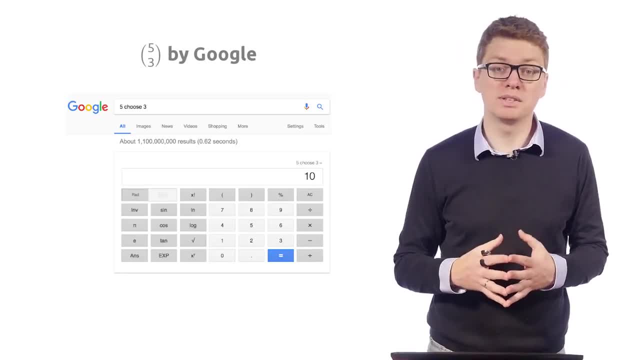 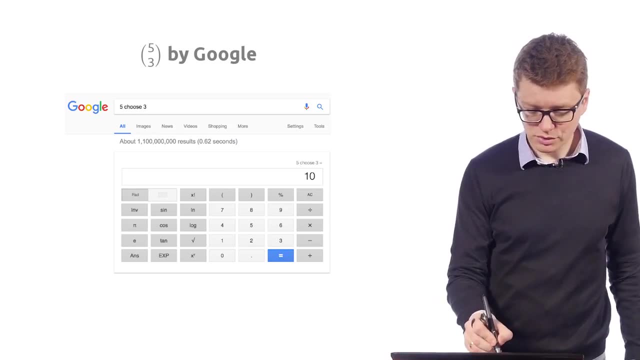 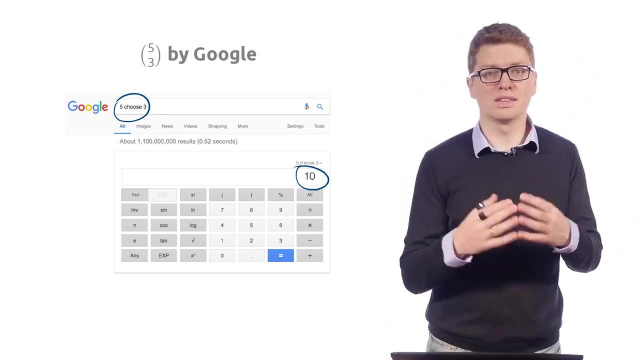 so, in particular, you can go to google and compute any such number. for example, if you compute five, choose three in in google. it will give you a result. okay, once again it is 10. so there are 10 ways of choosing, uh, three of your friends out of five of your friends. so that's the way to do it. 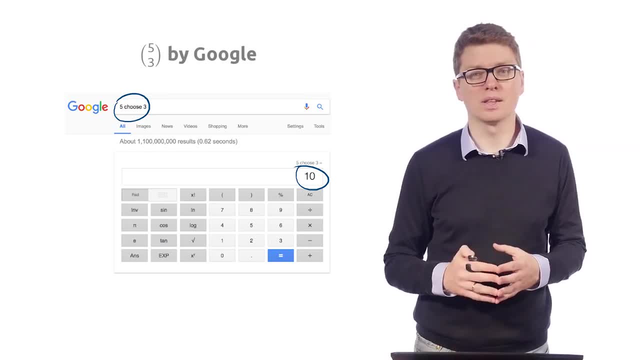 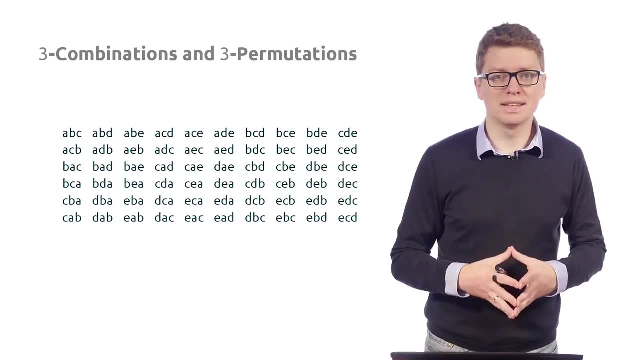 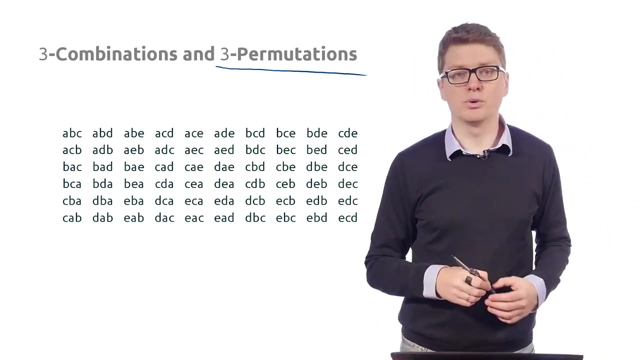 okay, now let's go to the next one. five, your friends. okay, now uh. before uh. before giving a formula, let's look once again at the difference between the uh, between the number of three combinations and three permutations. so let's list all possible three permutations. so recall that in a three permutation we just would: 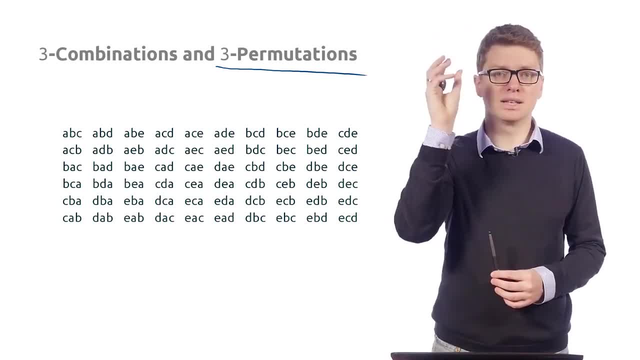 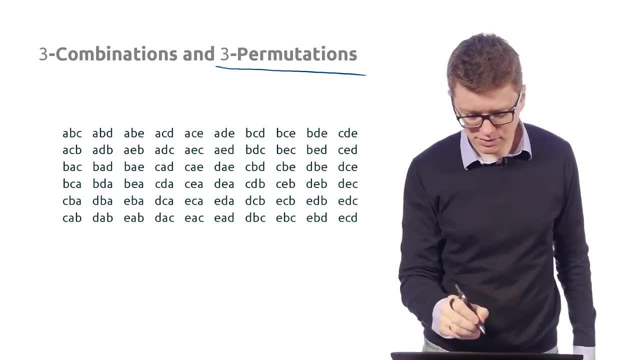 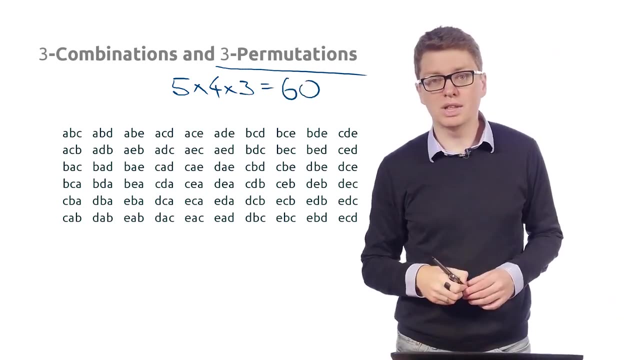 like to put one of your five friends to the first place, then one of the remaining four friends to the second place, and then one of the remaining three counts to the third place. so this gives us four, five times four times three, which is 60.. and all 60 permutations. three permutations are shown. 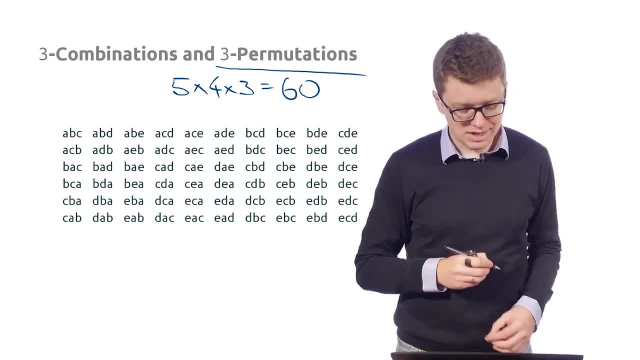 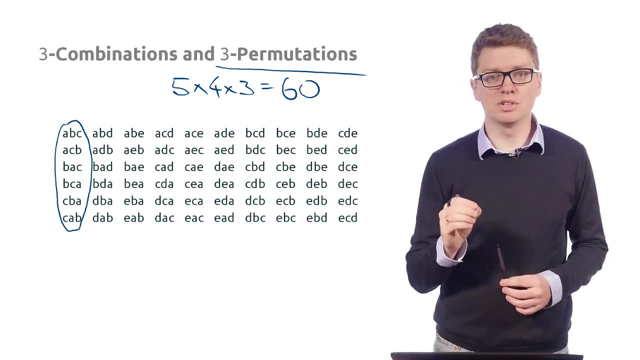 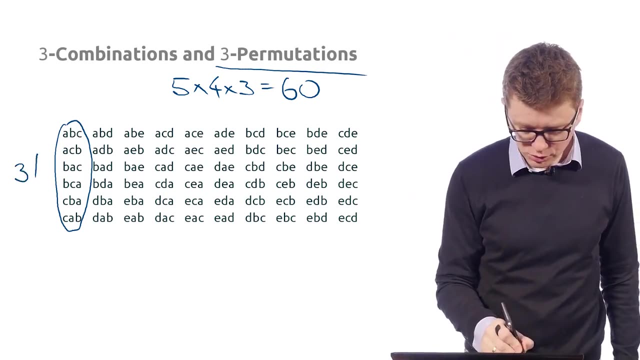 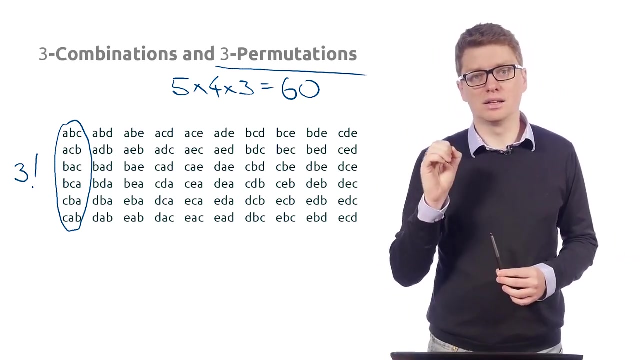 here on the slide, and they are arranged in a nice way such that, as you see, in in the same column we have exactly the same three elements permuted right and we know that for elements a, b, c, the exactly three factorial possible ways of permuter right. so in which means that, uh, the number of 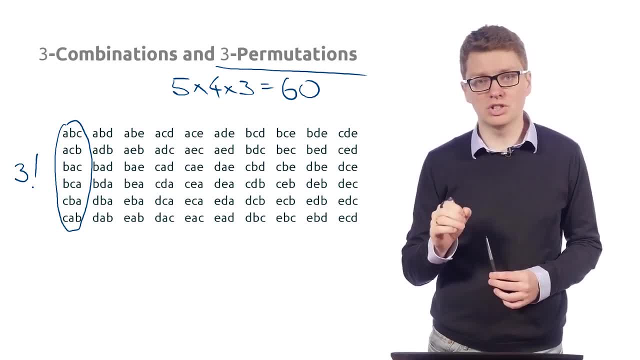 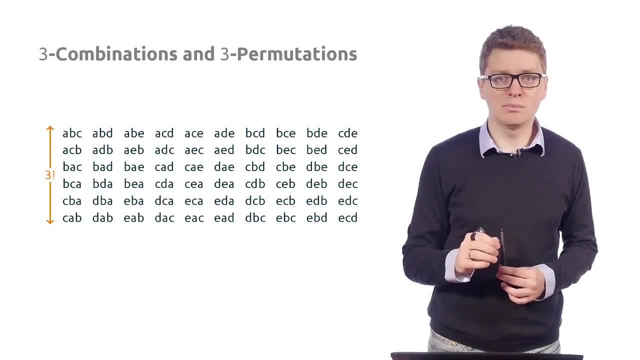 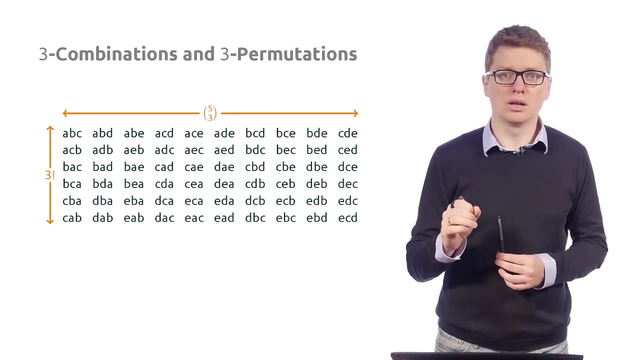 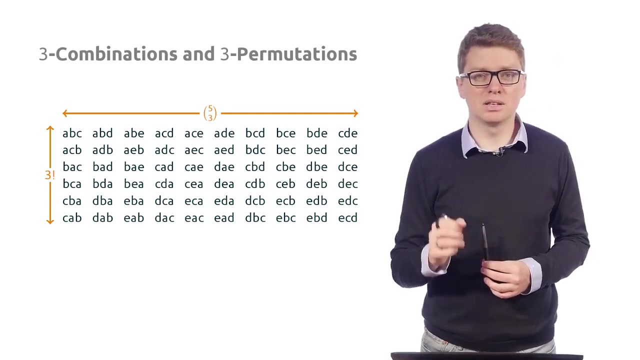 three permutations is three factorial larger than the number of three combinations. more precisely, what we see here is that, in this table, the height of this table is three factorial, while the width of this table is five choose uh, five, choose three. at the same time, the total size of the of the elements in this table is the number of three permutations. 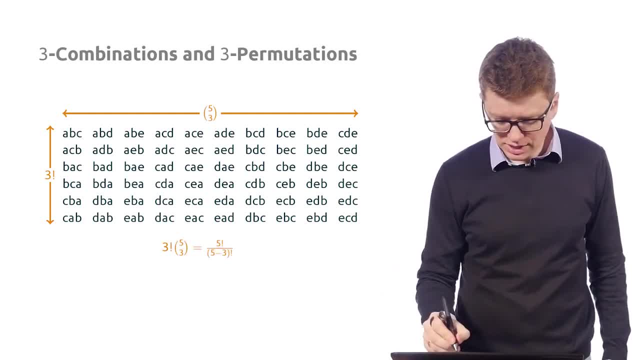 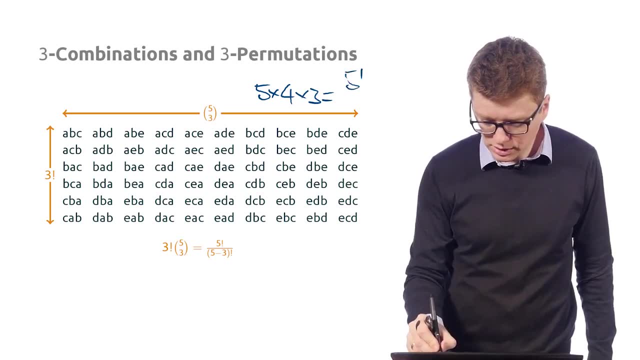 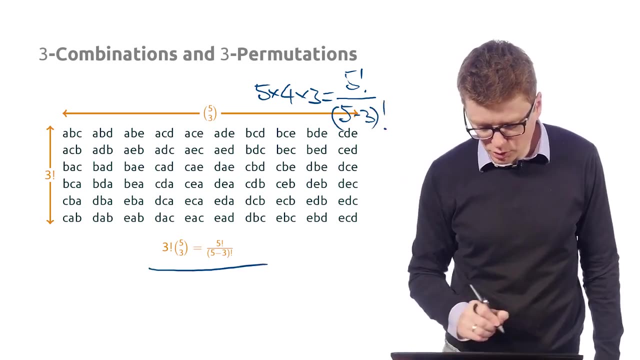 and we know how to compute it. the number of three permutations is five times four times three, which is nothing else as five factorial divided by two factorial, which is just five minus three factorial. so this gives us the following formula: the number of elements is is equal to the to the height of. 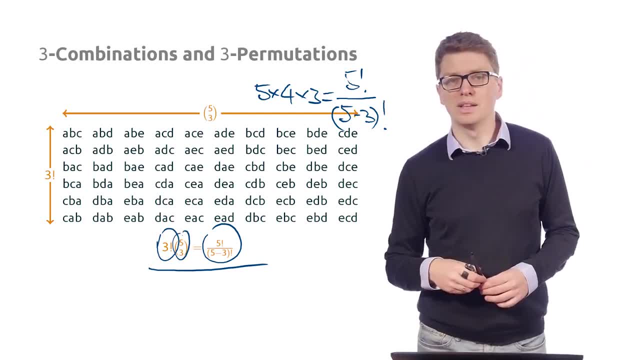 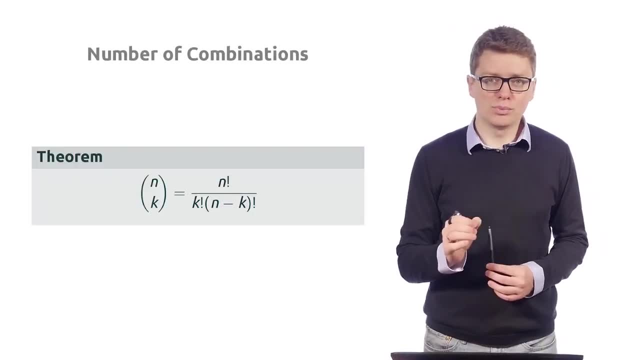 the number of three factorial times the width of this table. okay, and this will lead us, this observation will lead us to the general formula for computing n choose k. so the formula is as follows: n choose k is equal to n factorial divided by k factorial and divided by n minus k factorial. 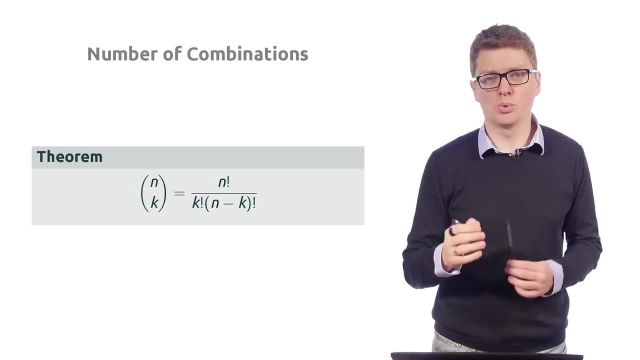 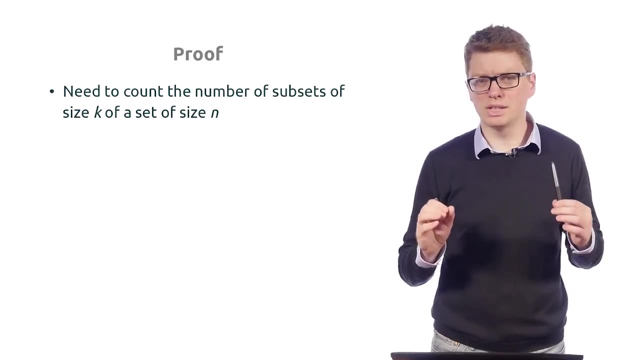 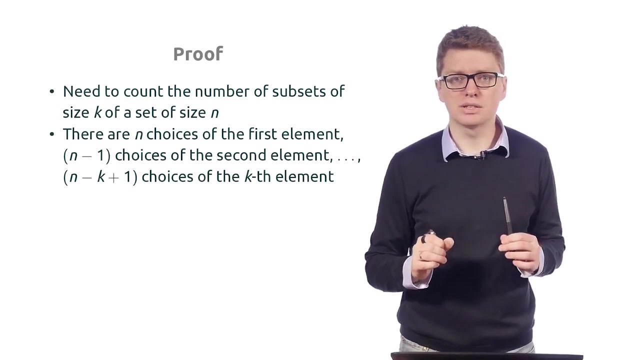 okay, so this is a formula, and now let's try to prove it. so we have actually everything, Okay. so first let me remind you that n choose k is the number of subsets of size k out of n elements. Okay, now, first let's count the number of k permutations. 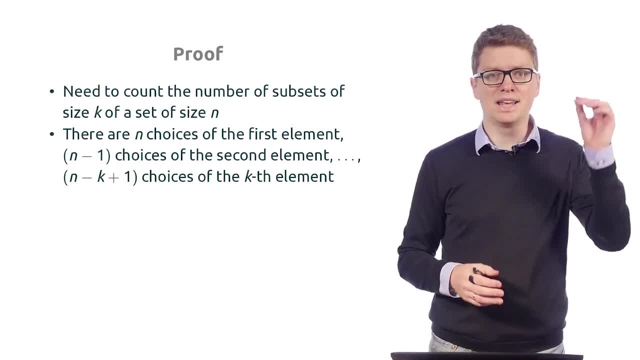 Okay, so for k permutations there are exactly n choices for the first element, Then there are n minus 1 choices for the second element, n minus 2 choices for the third element, and so on. n minus k plus 1 choices for the kth element. 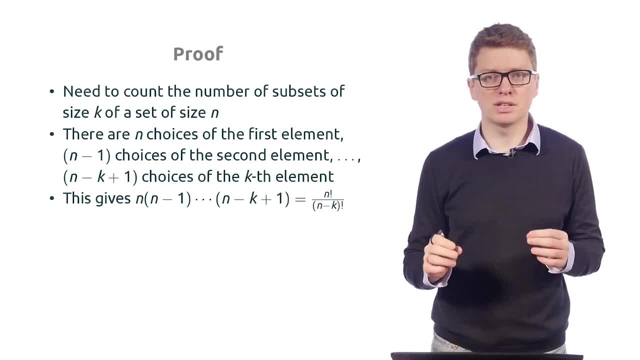 And this computes the number of k permutations and we know already that it is equal to n factorial divided by n minus k factorial, which is just a convenient way of writing the expression: n times n minus 1, times n minus 2, times n minus k plus 1.. 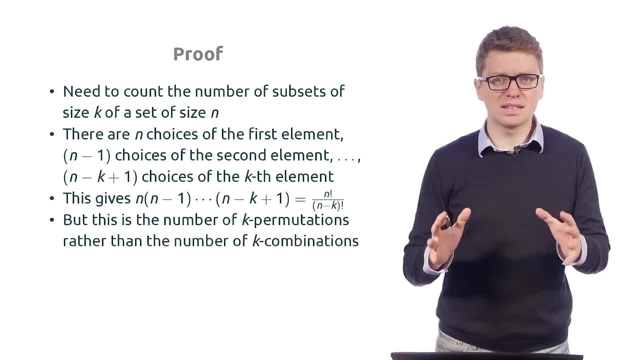 Okay, and this is as we've discussed already. this computes the number of k permutations, but not the number of k subsets, And the number of k permutations is exactly k factorial times larger than the number of k subsets. right? Why is that? 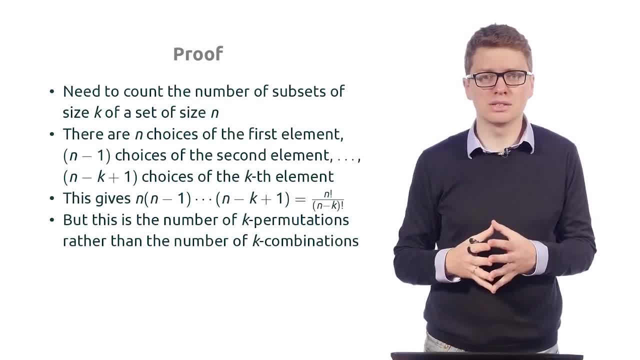 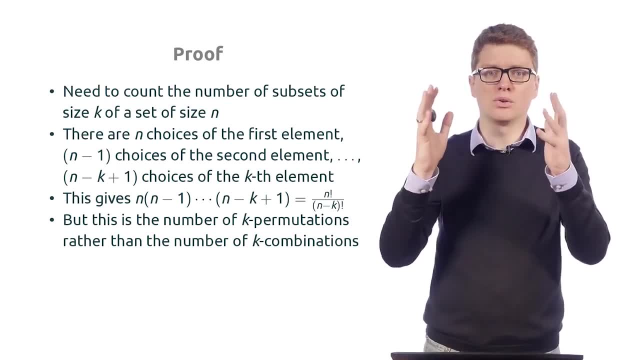 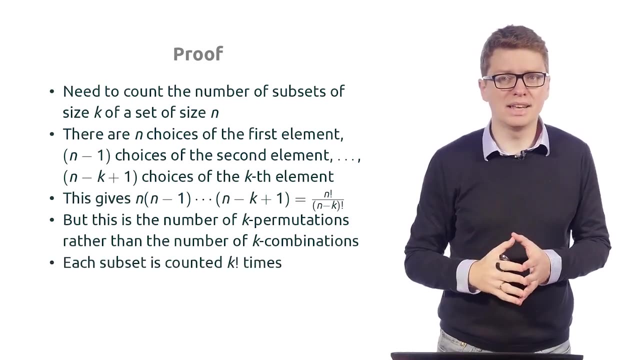 Well, because just when we count the number of k permutations, every subset is counted exactly k factorial times. Because if you have a subset of size k, there are k factorial ways of permutating, So you can think of it as permuting its elements, right? 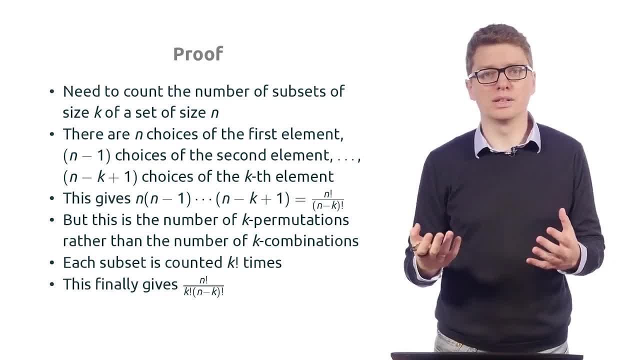 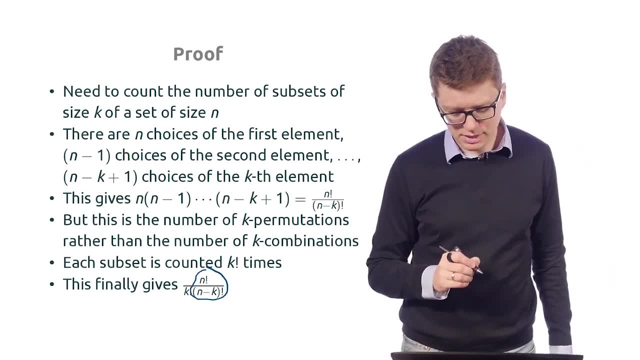 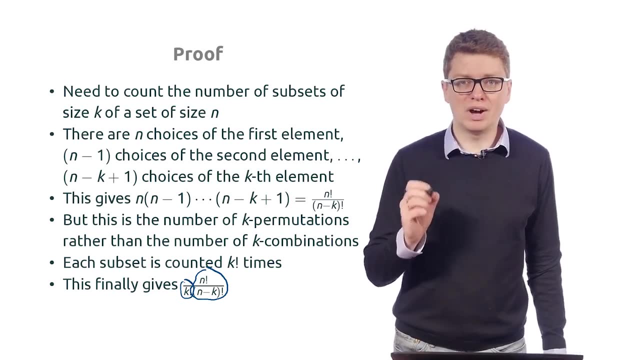 Which finally gives us the estimate n factorial divided by n minus k factorial. Let me remind you that this part, n factorial divided by n minus k factorial, is exactly the number of k permutations, and we need to divide it by k factorial to finally get the number of different k subsets. okay, 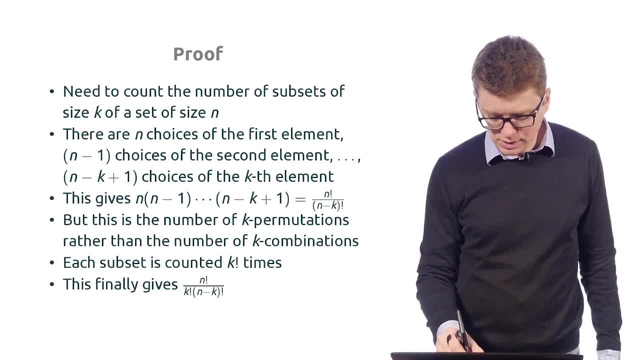 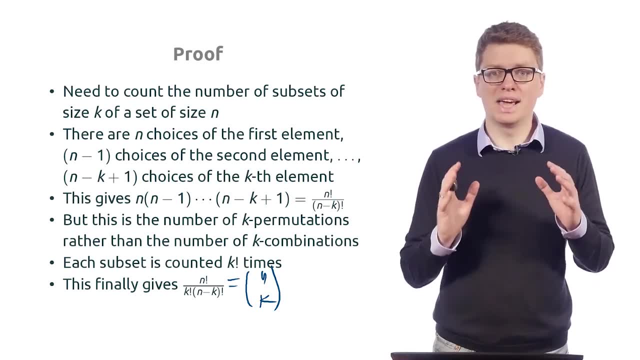 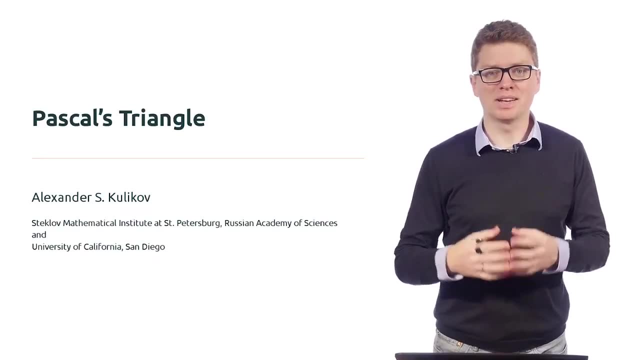 So once again, let me show you the result in a minute, an estimate. So n choose. k is equal to n factorial divided by k. factorial divided by n minus k factorial. Hi everybody, welcome back. In this video we are going to consider an elegant 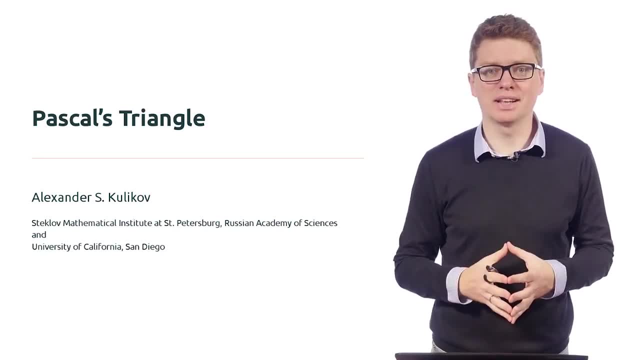 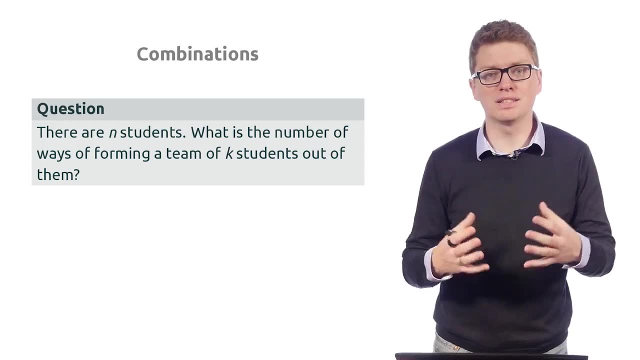 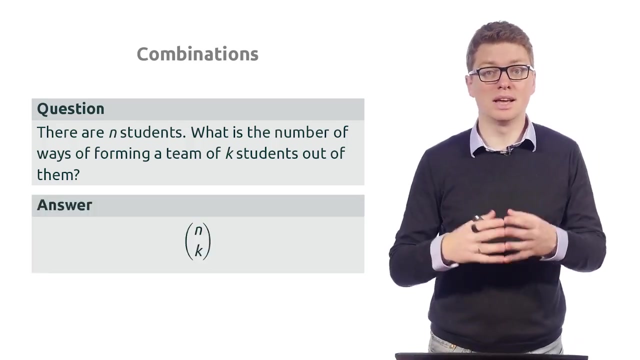 combinatorial structure called Pascal's triangle. Let's start with the following well-known question. I mean we have n students and we would like to form the sport team out of them, consisting of exactly k students. So what is the number of way of selecting such a team? So the answer is n choose. 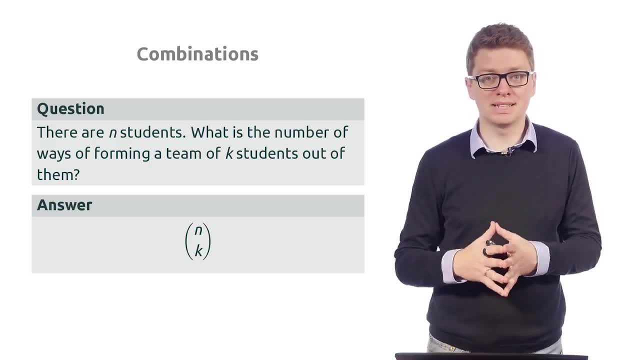 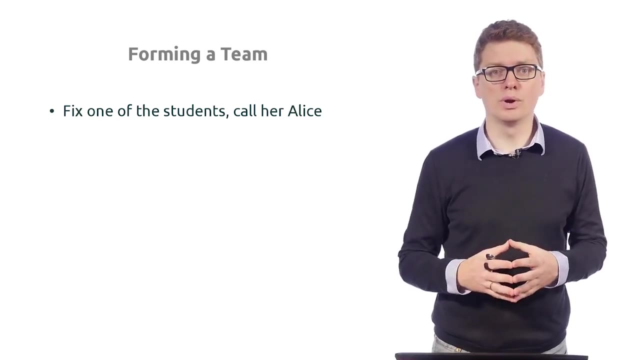 k. Well, why is that? Well, this is just because we are selecting k students out of n students. So, just by definition, this number is equal to n. choose k. Okay. at the same time, let's let's view at this number from a different viewpoint. let's just fix some. 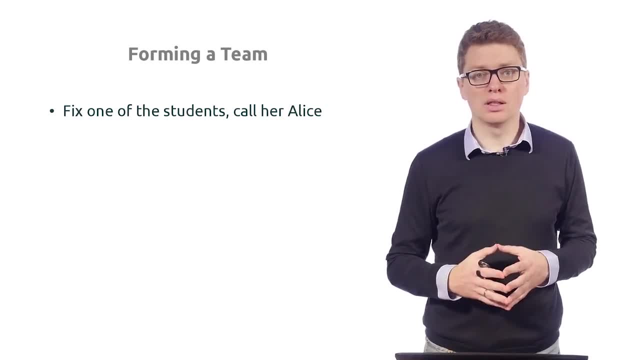 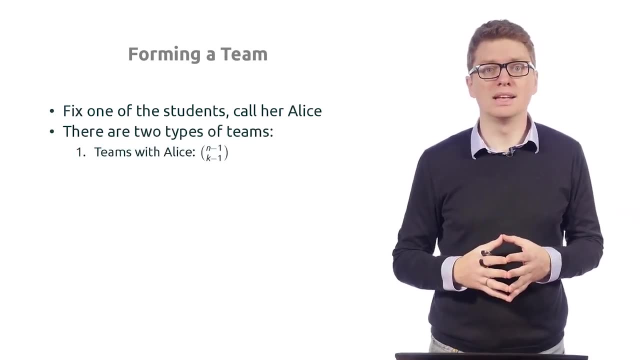 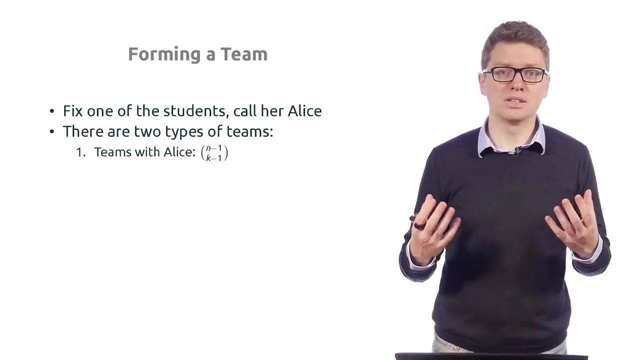 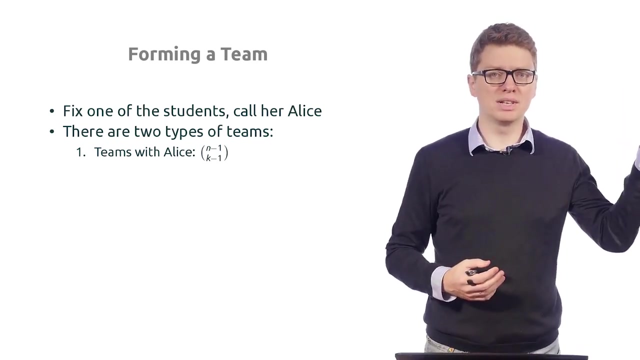 of the students and call her Alice, then all the possibilities are divided into two parts, naturally, first of all, there are teams with Alice, so first consider all the teams that that involve Alice. I claim that the number of such teams is equal to n minus 1. choose K minus 1. well, why is that? because we already decided. 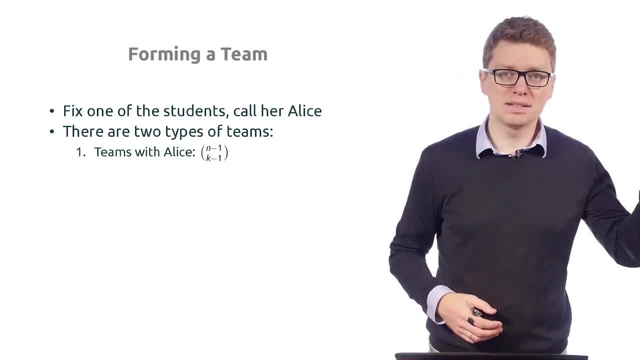 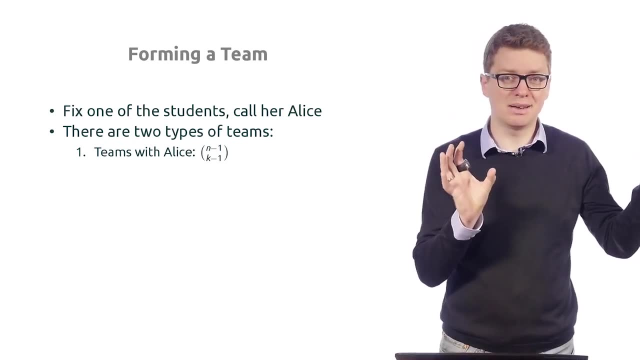 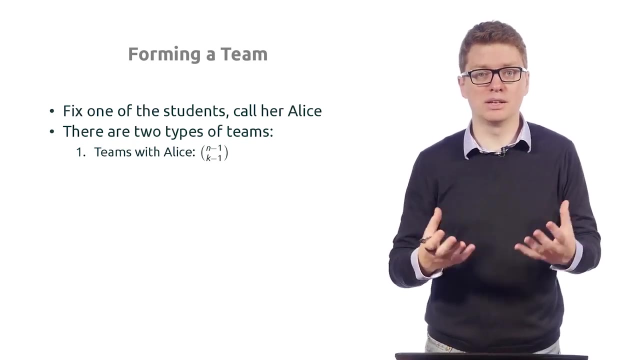 that Alice is in the team, okay. this means that we still need to select the remaining K minus 1 students, and we need to select them from the remaining n minus 1 students, and this is exactly this number of ways is exactly equal to n minus 1. choose K minus 1, okay. so once again, the number of teams with Alice is: 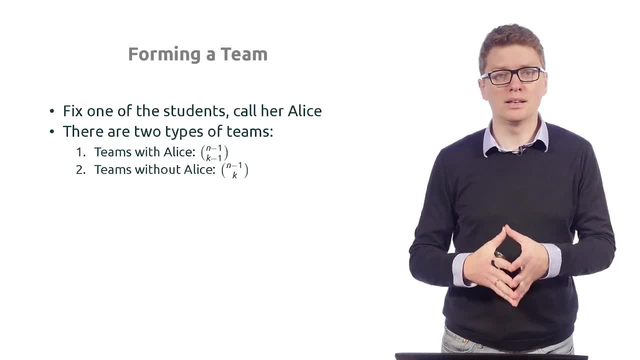 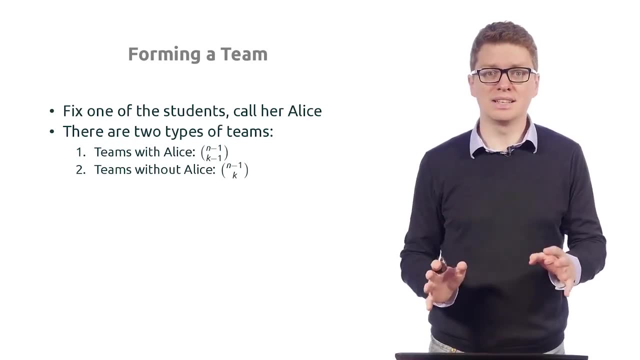 n minus 1. choose K minus 1. and now let's consider all other teams. there are teams without Alice, so we already decided that Alice is not going to be in the team. this means that we actually need to select the whole team, the whole K students from the 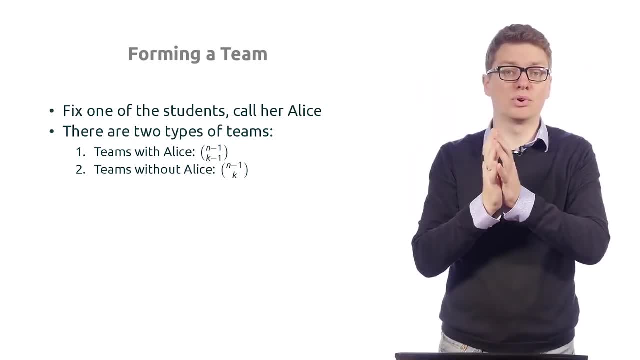 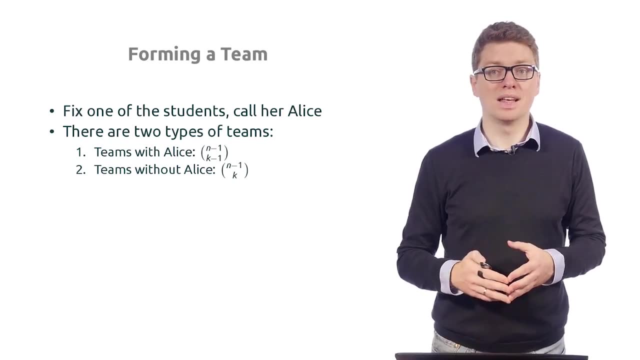 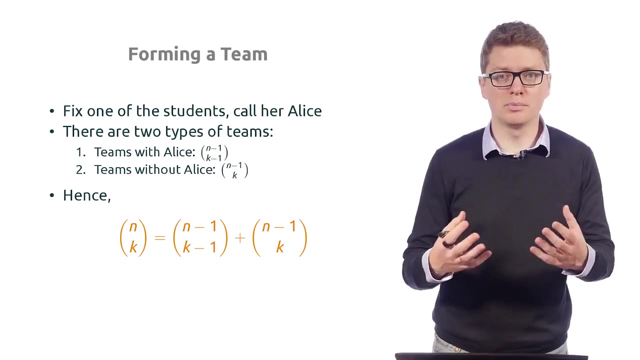 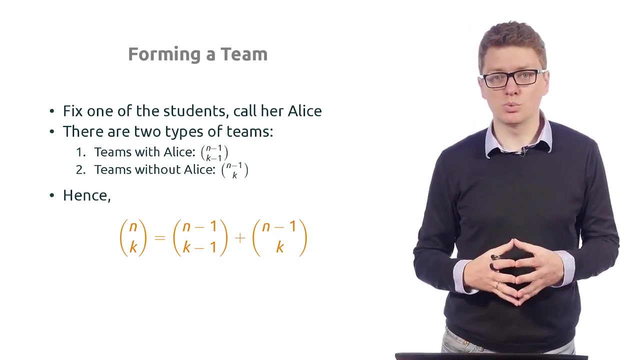 n minus 1. students, every, everyone except for Alice, right and again, just by definition, the number of such ways is n minus 1. choose K, and this is this gives us finally the following nice combinatorial property of the number of combinations: and choose K is equal to n minus 1. choose K minus 1 plus n minus 1. 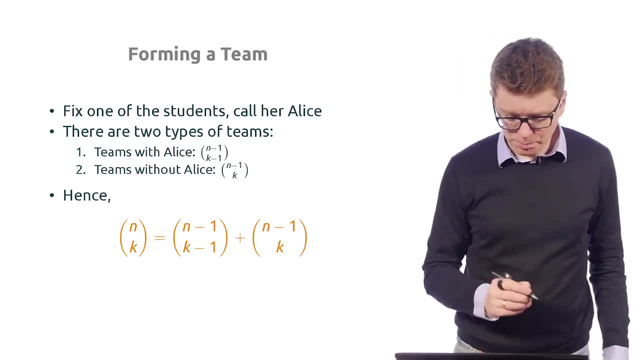 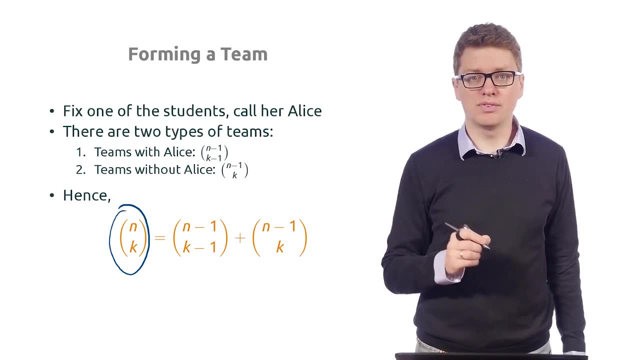 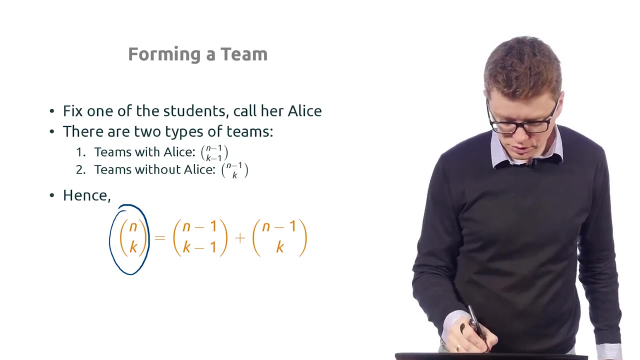 choose K. so once again, let me try to repeat this formula. this is a number of ways of forming a team. okay, of K, of K students, out of N students, and we represented this as naturally as two disjoint teams, and so this gives us the joint parts. so, first of all, this is a number of ways of forming a team with some fixed student. 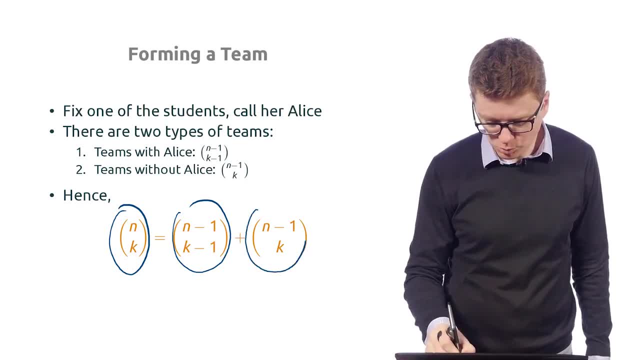 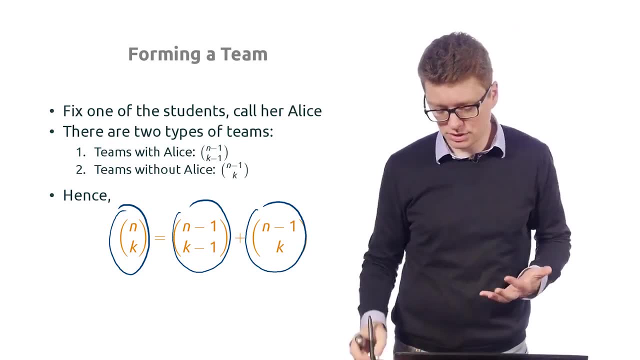 which we called alice, and this is the number of ways of forming a team without this student. so clearly, the number of ways of forming a team is equal to the sum of these two numbers, because this is just all the all the possibilities. okay, and this is a an important property of 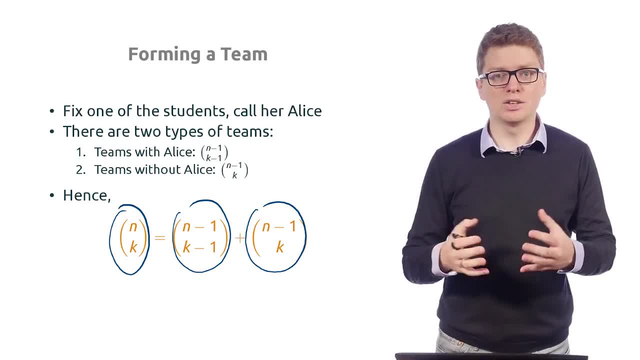 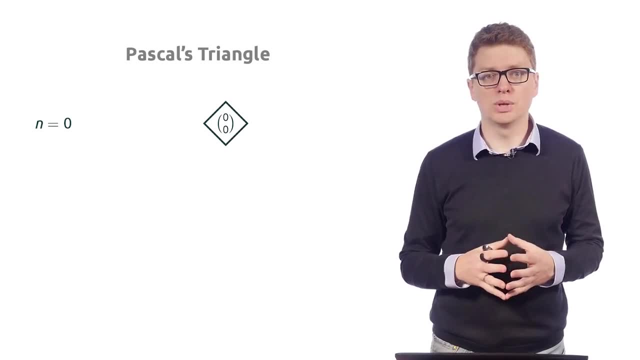 of this, of these numbers, and there is an elegant way of visualizing- uh, uh, visualizing this property. okay, so let's try to do the following: we're going to construct the so-called pascal triangle, which will contain a separate cell for every n and k. contain the value and choose k. so it is going. 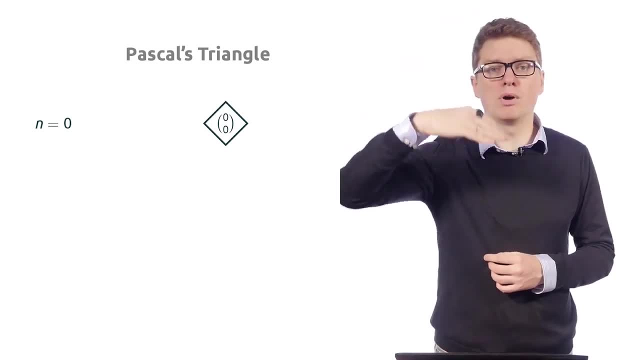 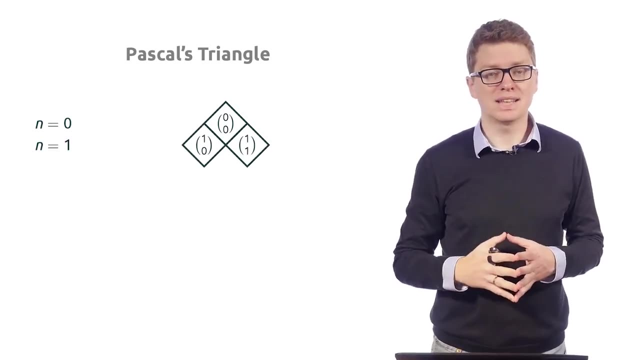 to be constructed from uh from top to bottom. so at the top we have just one cell containing the value zero, choose zero. the second row corresponds to n, equal to one, and it has two cells, one choose zero and one choose one. so in general at every row we have 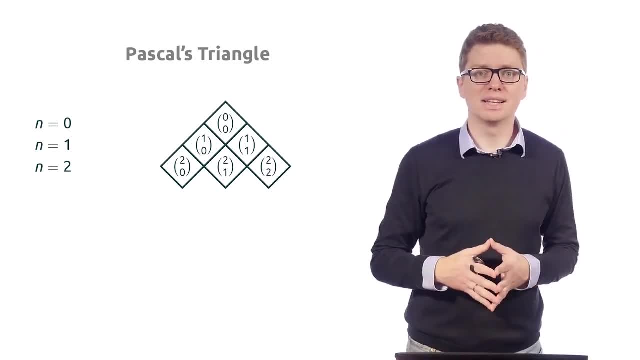 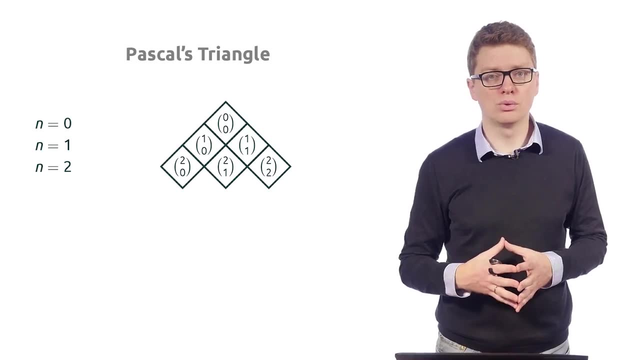 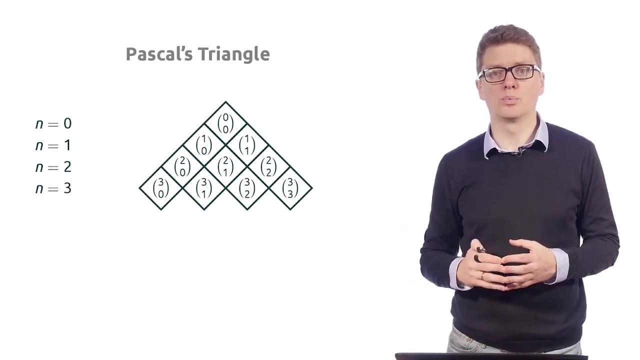 it corresponds to some fixed value of n and then it has all the values of n. choose k where k ranges from zero to n. so when n is equal to two, for example, k ranges from zero to two. so we have three cells. k is equal to zero, one or two. when n is equal to three, we have four such cells. 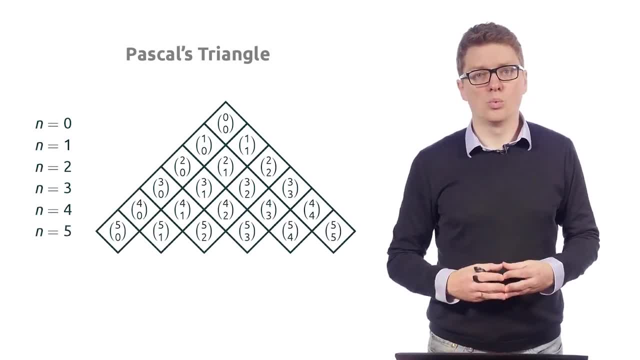 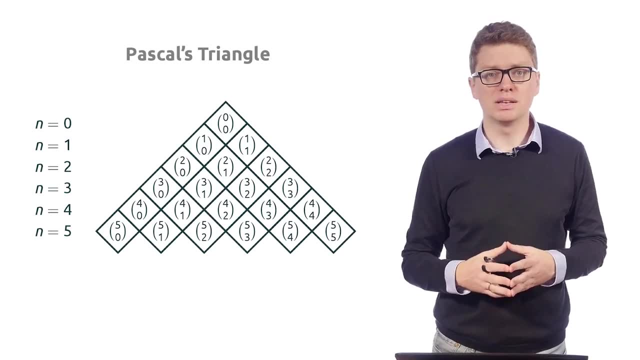 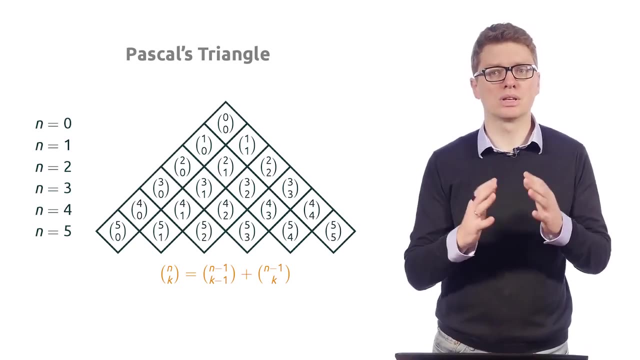 and so on. okay, now let's see: uh what, uh, uh what our uh. equality that we've just that, we've just proved, means in this triangle. so let me remind you this: equality and choose k is equal to n minus one- choose k. minus one. plus n minus one, choose k. so essentially it. 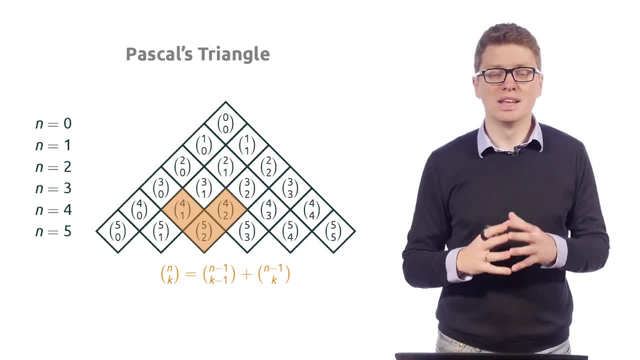 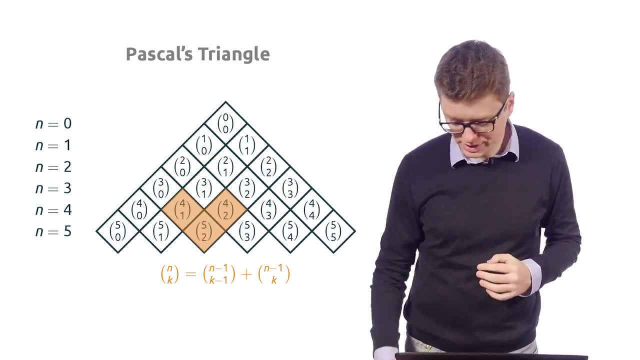 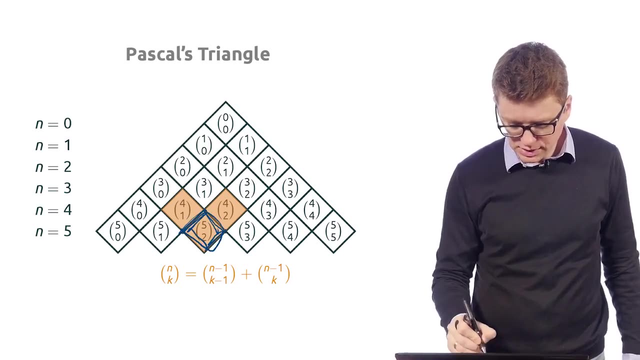 means that for every element in our triangle, its value is equal to the sum of its two top neighboring elements. so, for example: uh, what we know is that five choose two, so the value of this cell is equal to the value of this cell plus the value of this cell. so in this particular case, 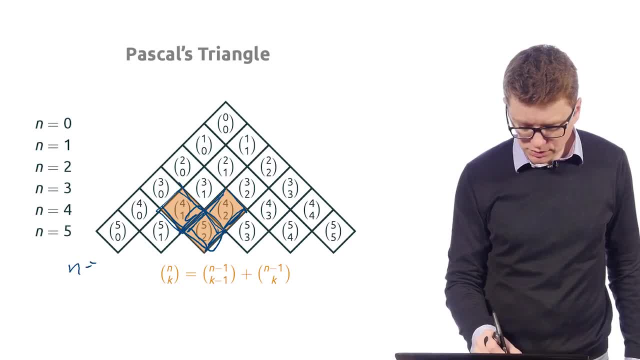 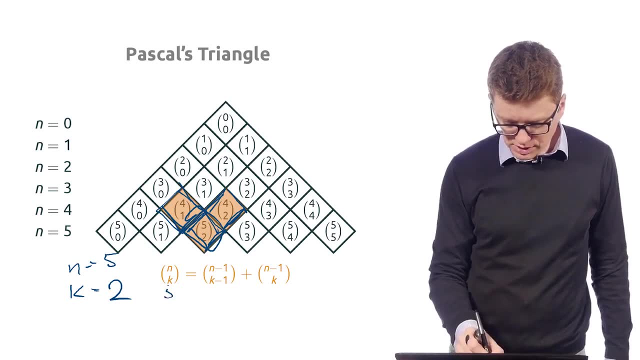 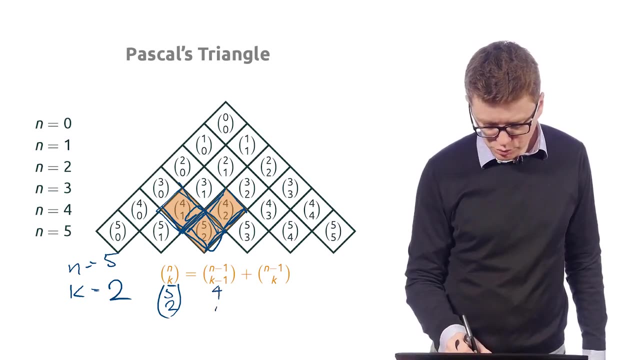 n is equal to five, and n is equal to five and k is equal to two. so by applying this formula, we have some in this case. so this is five, choose two, and n minus one, choose. k minus one is four: choose, choose one, which is exactly this cell. 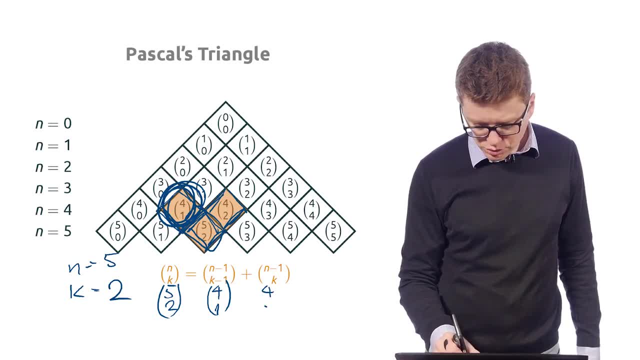 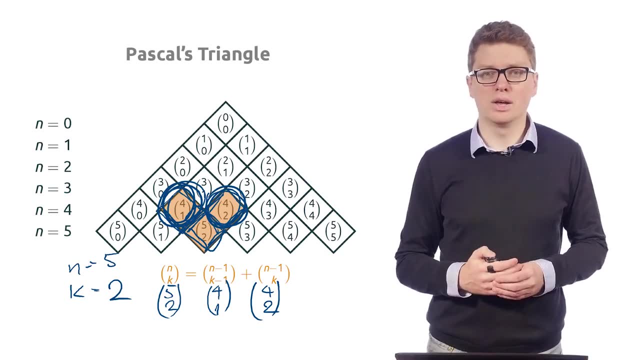 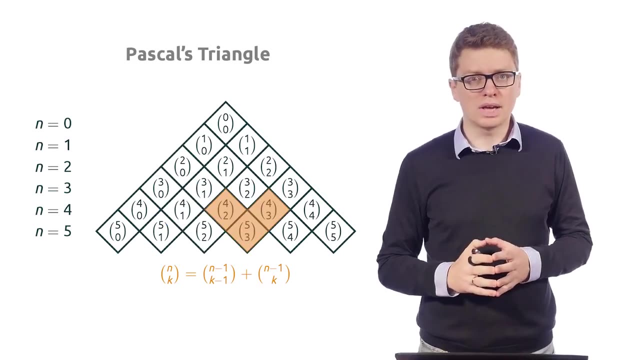 right, and then minus one, choose k is four, choose two. okay, which is exactly this, and this holds actually for for every, for every cell, you know, for every, to be formal, for every internal cell in our, in our table. okay, now, let me, let me replace all these, uh, all these numbers with the actual. 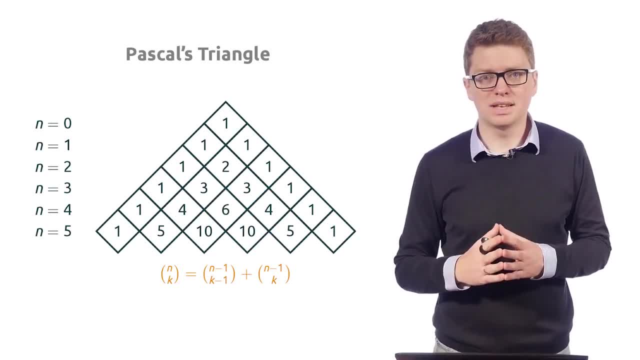 values. and let's take a look. so, first of all, we see that at the boundaries we have the value one everywhere. so why is that? well, just because at the boundaries we have- uh, we have- numbers like m- choose zero, or n- choose and choose n. so n- choose zero is always equal to one, so it is the number of 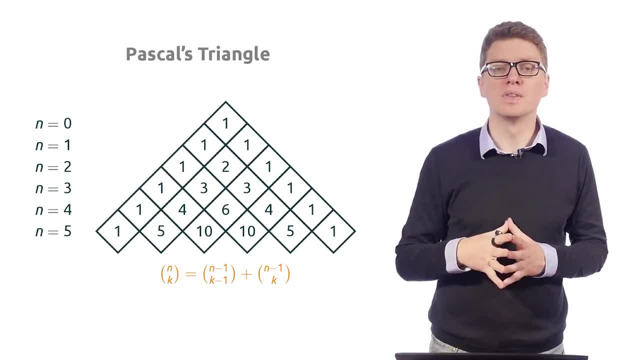 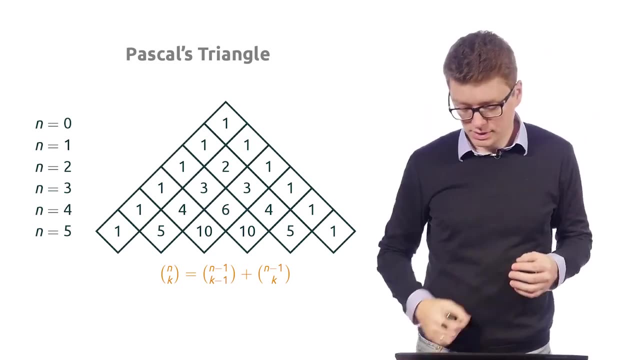 values of selecting an empty set. there is just one empty set, okay, and m choose n is all is also equal to one. well, this is just because m choose n is the number of ways of choosing a subset of size m, and there is exactly one such subset, of course. so at the boundaries we have ones ones everywhere. 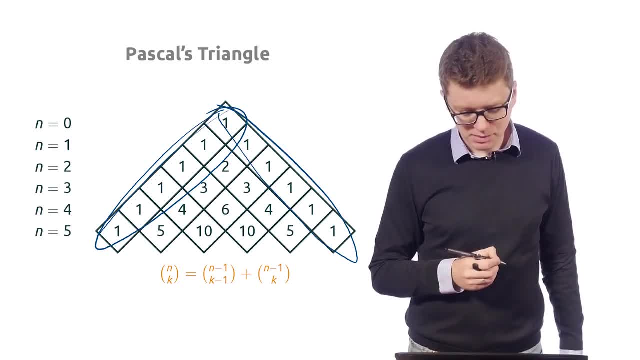 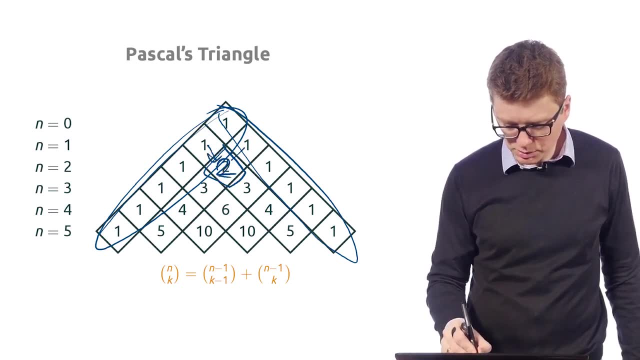 right, and then every other. every other element can be computed just by by computing the sum. so for the two here can be computed as the sum of one plus one. three here can be computed as 2 plus 1.. 4 here can be computed as 3 plus 1, 5 here can be computed as 1 plus 4, and so on. so 3 is computed as. 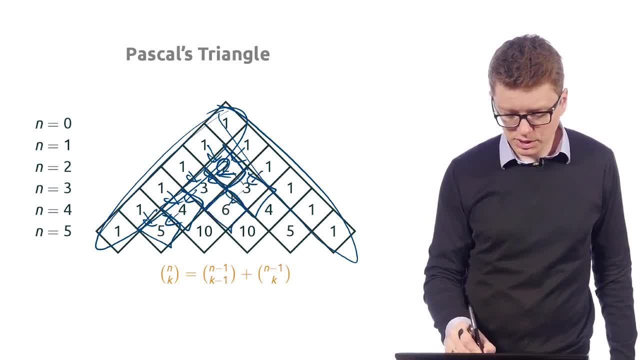 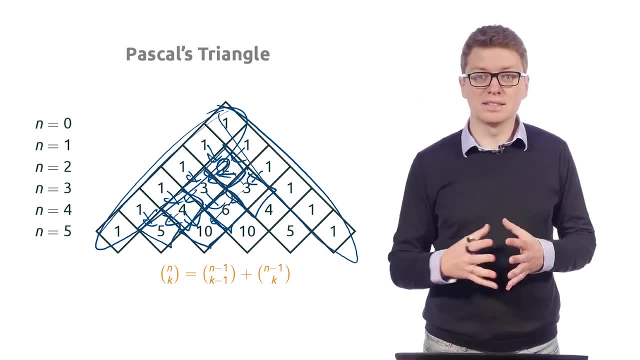 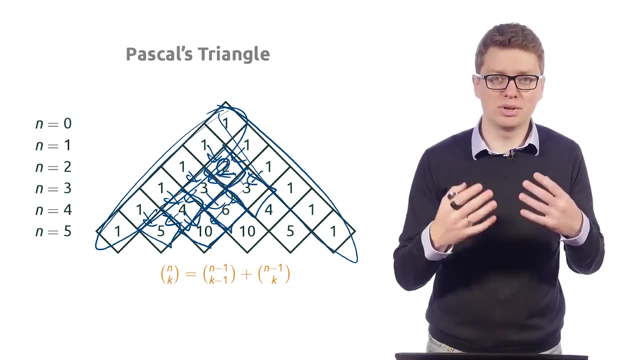 1 plus 2. 6 is computed as 3 plus 3, 10 is computed as 6 plus four and so on, and in fact this gives us, like another way of computing, the value of n. choose k. So if, for example, you have large numbers, n and k, 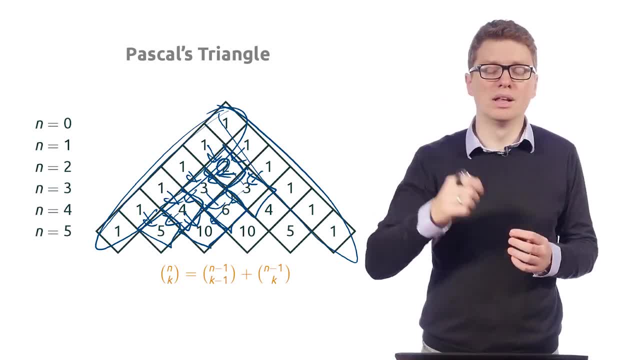 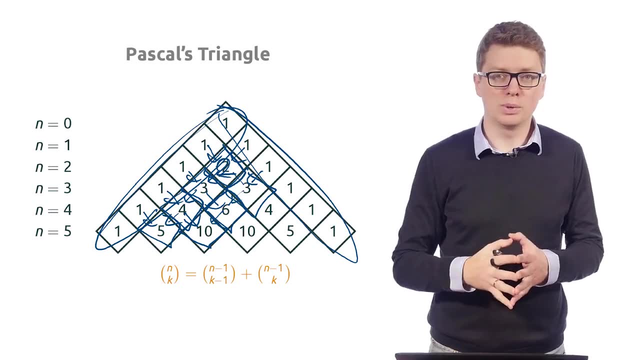 one way of computing n choose k is to compute n factorial, then divide it by k factorial, then divide it by n minus k factorial. So it involves many multiplications and many divisions At the same time. using Pascal's triangle, we can compute the value of n choose k. 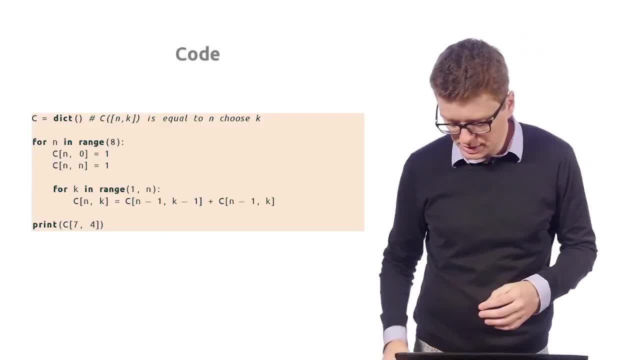 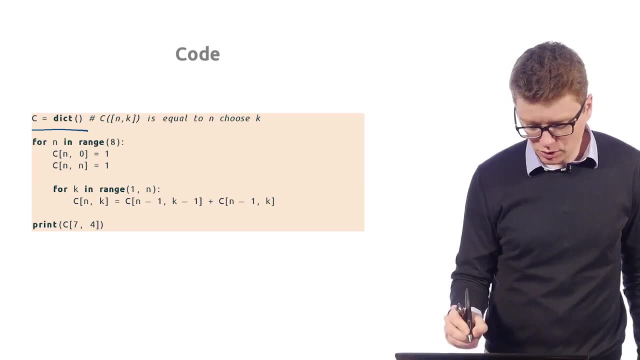 just by computing some sums. That's as usual. So let's just declare the dictionary c such that c of n, k is going to be equal to n. choose k. Okay, then we do the following: We range, we loop through all the values from zero to seven. 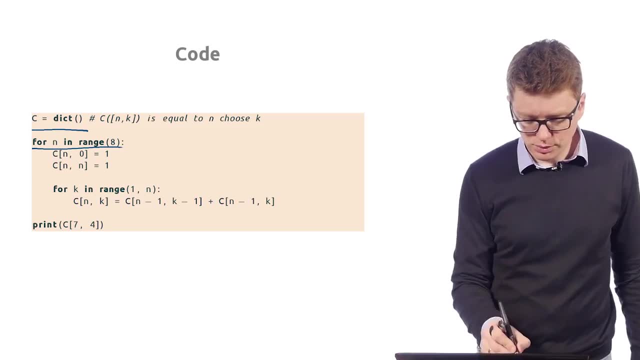 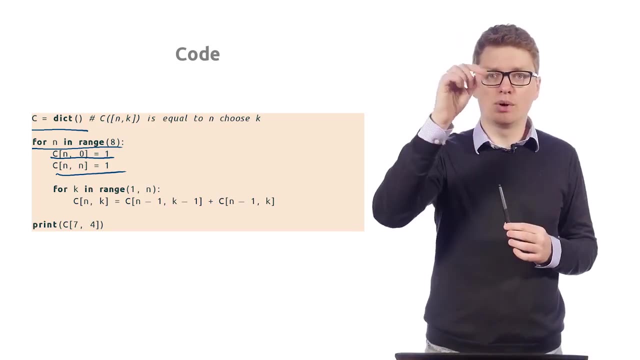 and we do the following: First, we say that n choose zero is always equal to one, and n choose n is also equal to one. In a sense, what we do here, we fill in our triangle, we fill it row by row. 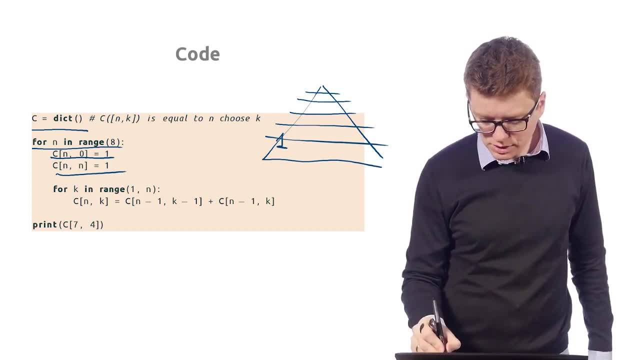 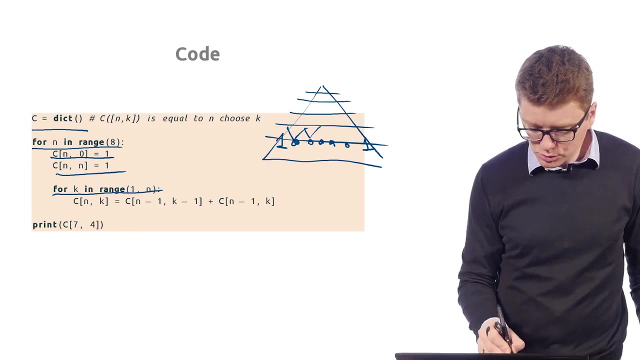 and at every row, we first say that the values at the boundaries are equal to one, And for every internal element in the row we compute it as a sum of two previous elements. right, And this is done here. So for all internal elements. 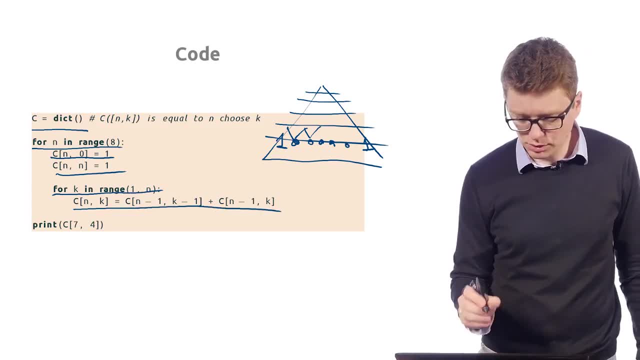 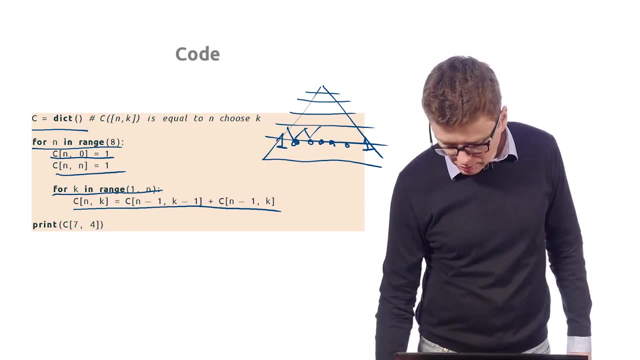 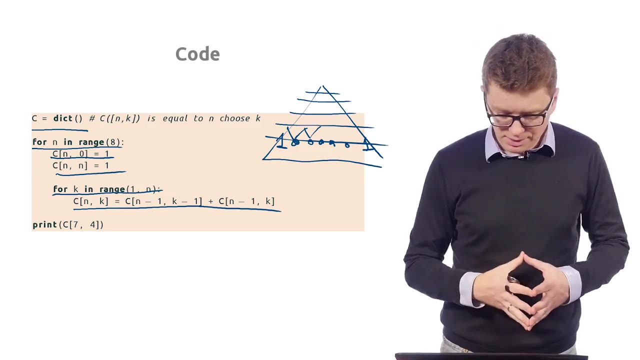 we apply our formula: n choose k is equal to n minus one. choose k minus one. plus n minus one, choose k. okay, So when n and k are large, so it uses a lot of space for computing n choose k, but still, I mean all the operations are just summations. 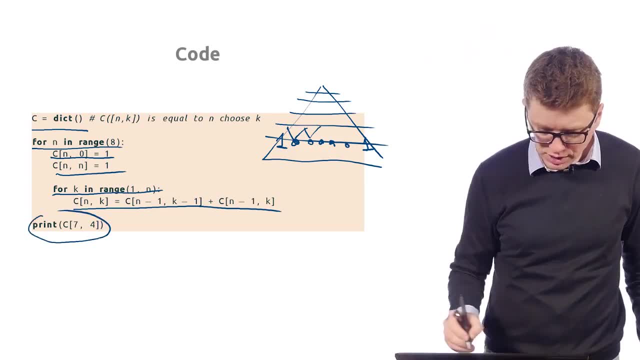 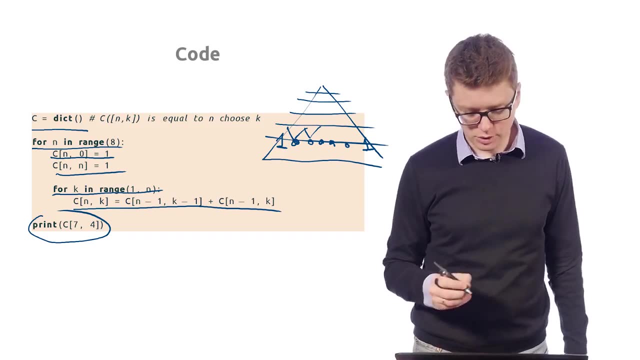 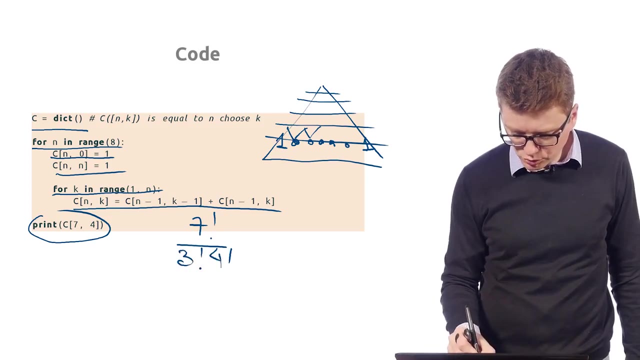 And now, in the end, let's just do a sanity check. Let's compute. let's compute this way. Let's print n: choose seven, choose four, I'm sorry. So what we expect is like: seven factorial divided by divided by three. factorial by four. factorial. 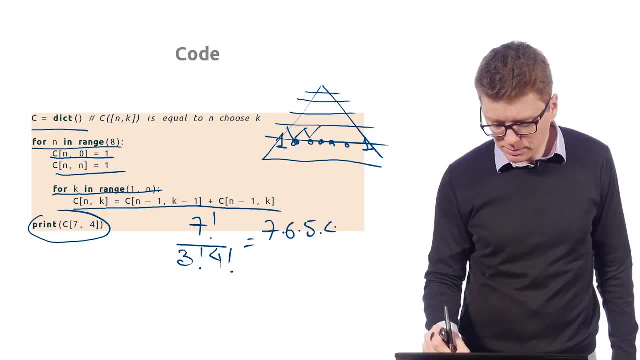 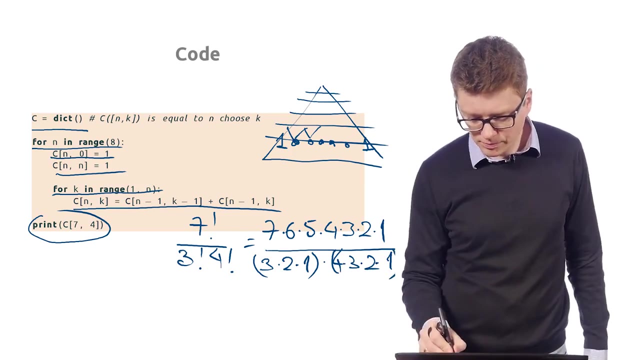 which is seven times six times four times times five times four times three times two times one. divided by three times two times one, This is three factorial. and divided by four times three times two times one, This is four factorial. We again cancel out this immediately. 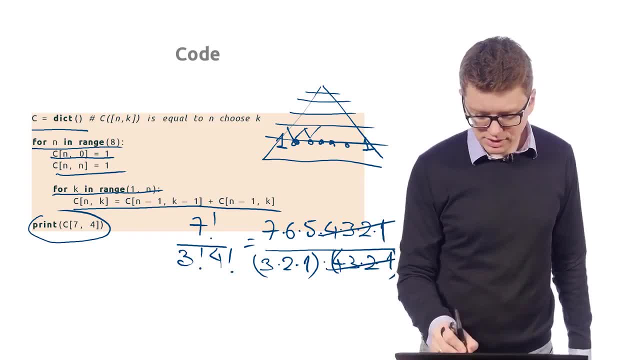 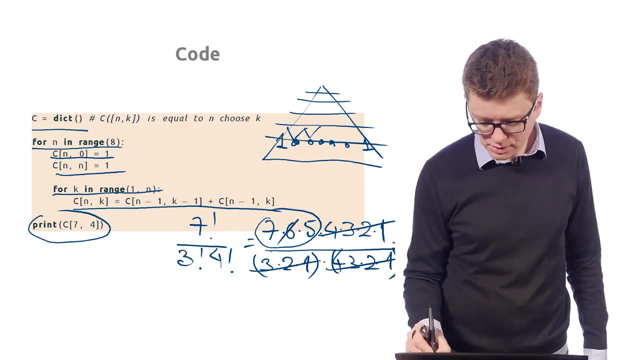 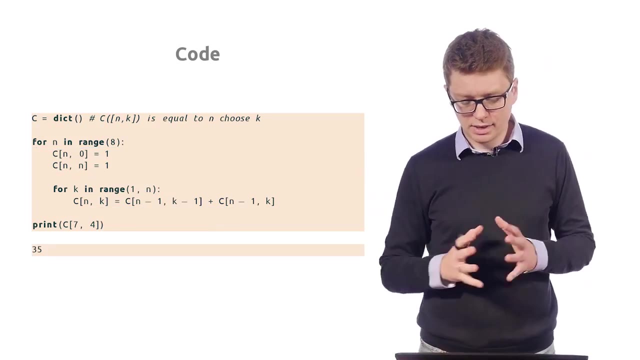 and then what remains is six times seven times six times five, divided by three times two times one. So six is also canceled, and what remains is 35. And the same, the same result is printed by our recursive precision. So once again, this Pascal's triangle gives us. 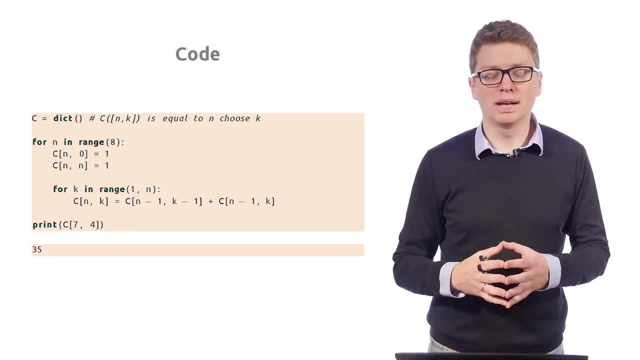 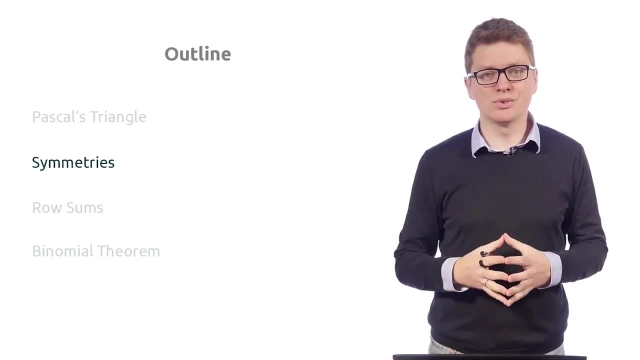 an alternative way of computing. of computing n, choose k. Let's now use the Pascal's triangle to prove another useful property of of n k. Let's now use the Pascal's triangle to prove another useful property of of n k. 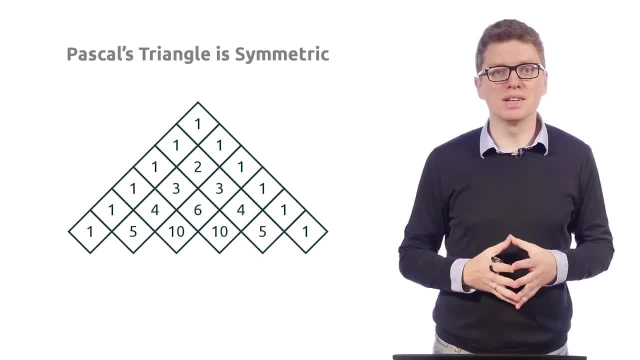 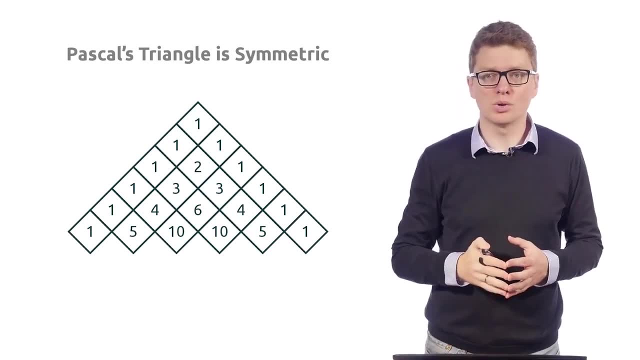 Let's now use the Pascal's triangle to prove another useful property of of n k. As you've probably noticed already, the Pascal's triangle is symmetric with respect to the center vertical line. So what does it mean? This actually means that if you start reading any row, 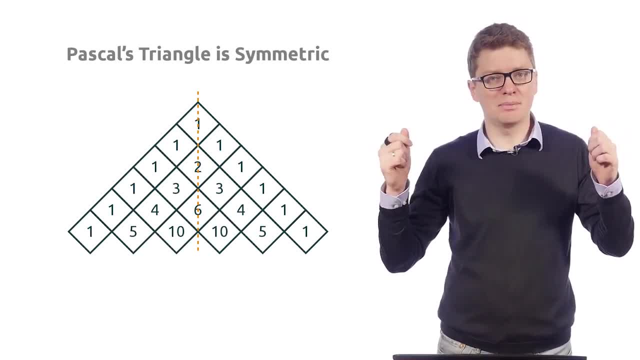 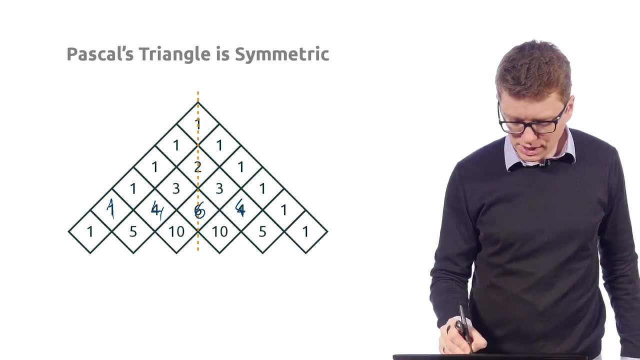 in this triangle from left to right, then you get exactly the same as if you read it from from right to left. For example, here we have one, four, six, four, one, And if you, if you read it from right to left, 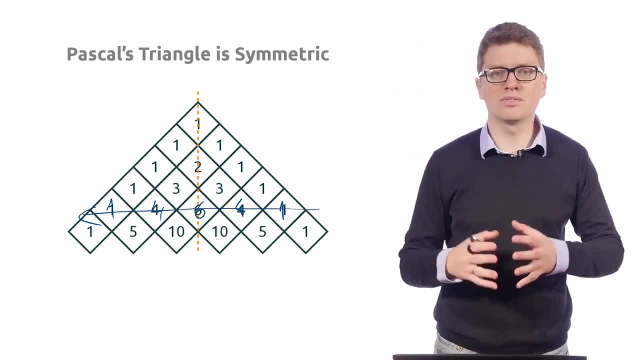 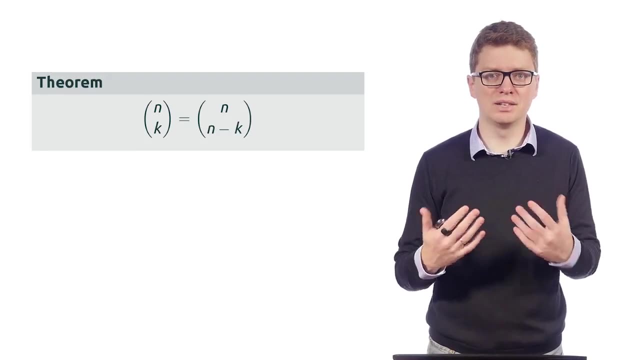 you get exactly the same sequence of numbers. So, in terms of n and k, this means the following: n choose k is equal to n choose n minus k. okay, So let's prove this, this formula, First of all. you can prove this directly. 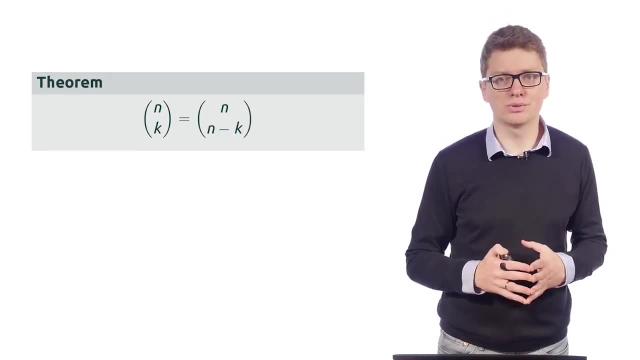 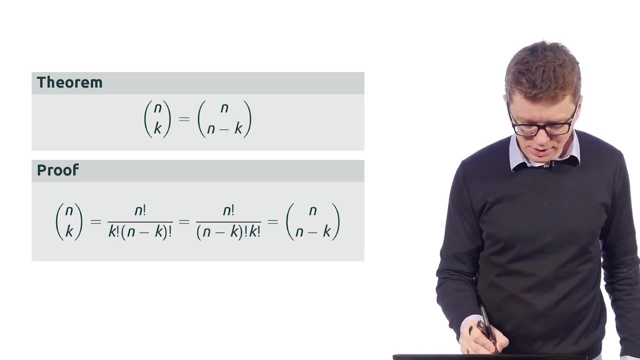 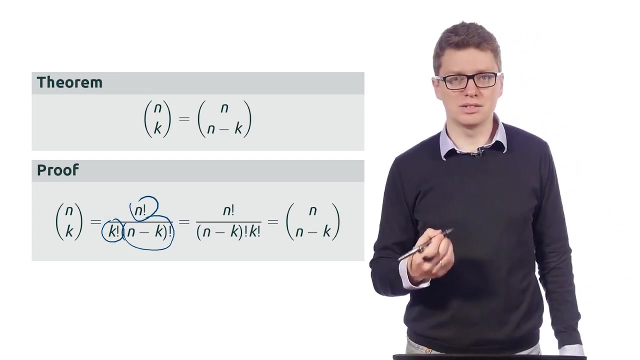 just by applying the known formula for: for n choose k. This gives you the following- well, slightly probably boring- proof: So we know that n choose k is equal to n factorial divided by k factorial divided by n minus k factorial. Okay, this is just a definite. this is just a formula. 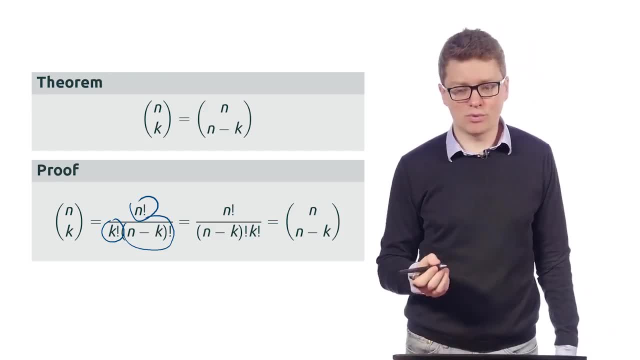 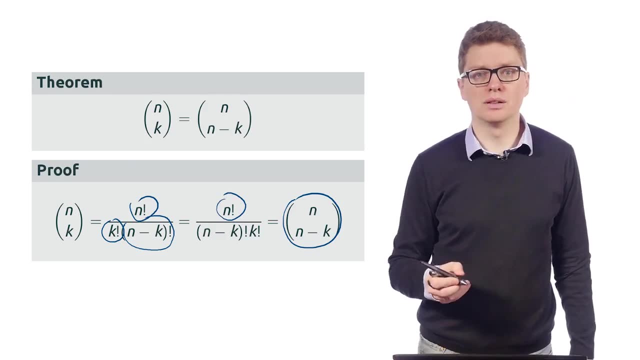 I'm sorry for n choose k. On the other hand, let's apply the same formula for n choose n minus k. So at the top we have n factorial, as usual. At the bottom we have first of all n minus k factorial. 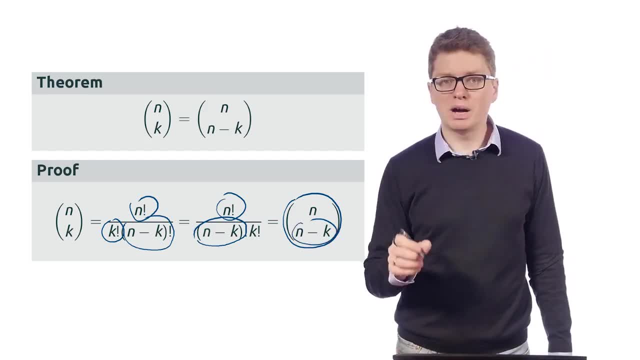 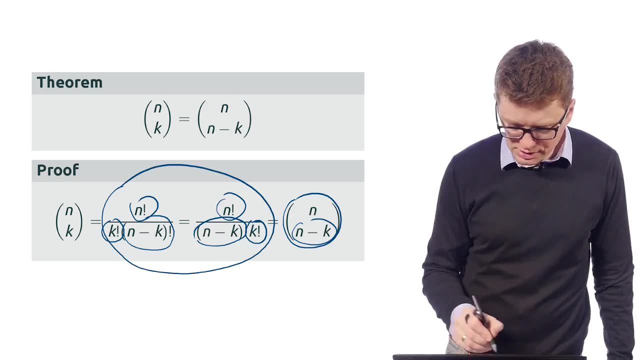 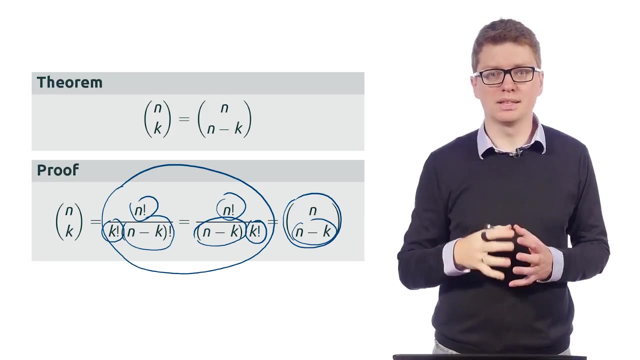 This is just repeated, this element, And then n minus n minus k, which is nothing else. This is just k factorial. Okay then then, just by comparing these two numbers, it is easy to see that they are exactly the same, just with two, with two terms swapped at at the bottom. 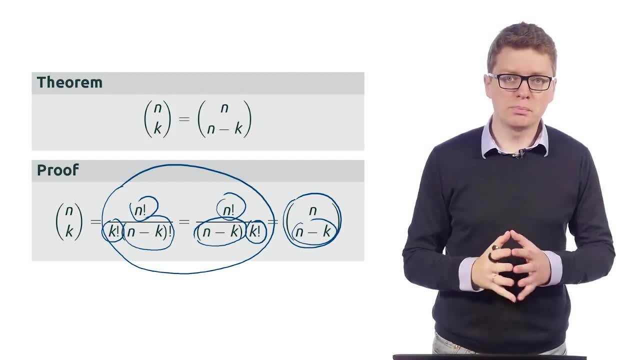 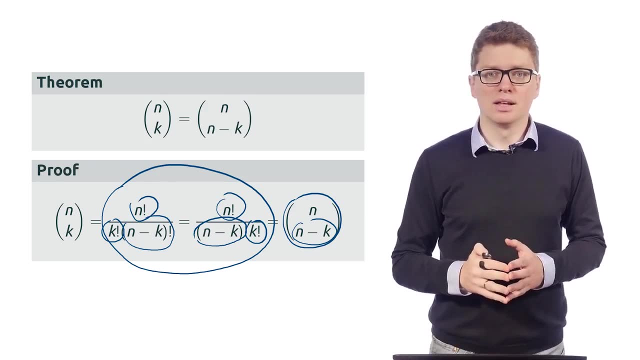 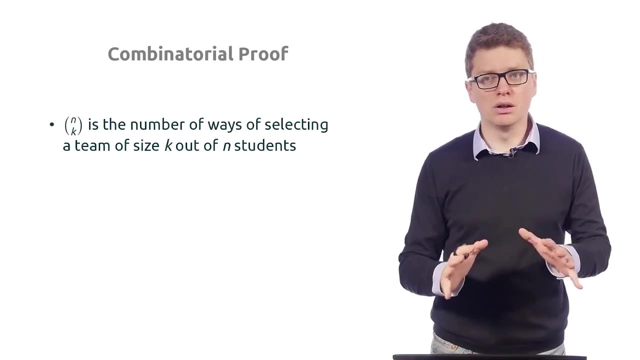 right of our fraction. Let's so this. this already proves this formula, but let's try to to find some combinatorial meaning of this equality, which is actually more nicely illustrates the nature of this equality. So let's recall that n choose k, just by definition. 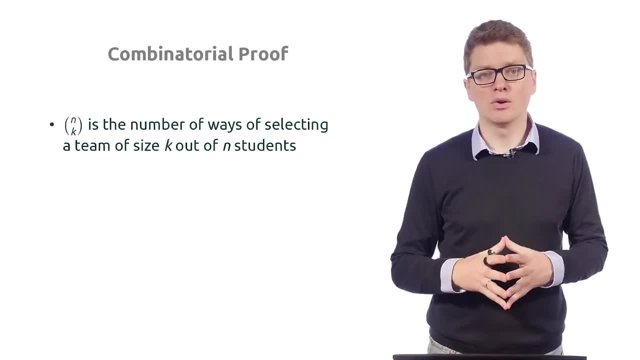 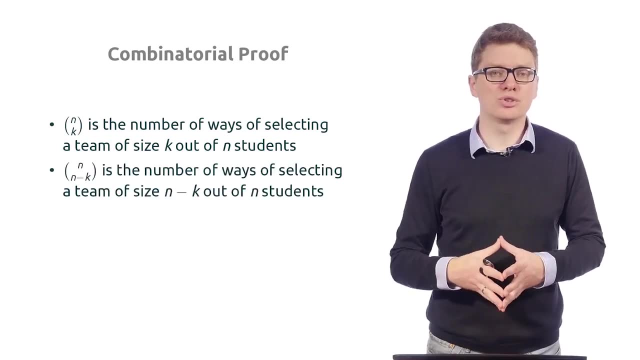 is the number of ways of forming a team of k students out of n available students right. On the other hand, n choose n minus k. is is essentially the same quantity, with the only difference is that in this case, we are forming a team of size n minus k. 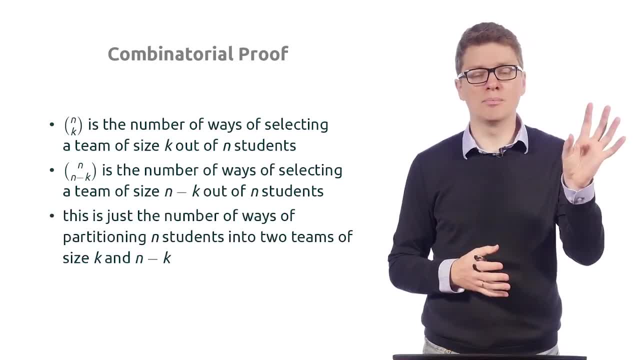 But at the same time, note that when we form a team of k students, what we basically do is just we divide all our n students into two parts, So there are k students that go into a team and there are n minus k remaining students. 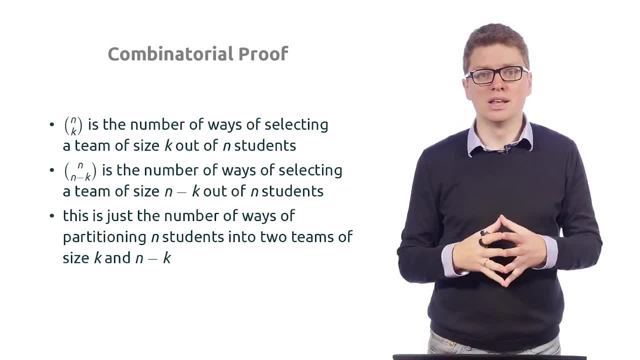 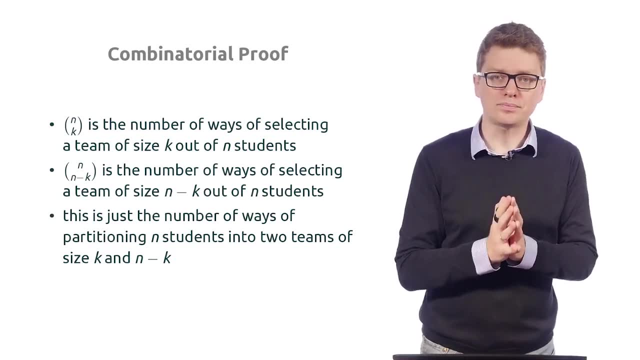 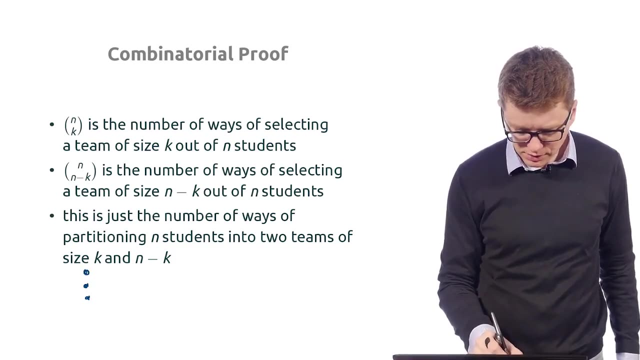 So that's why these two quantities are actually the same. So, more formally, the proof goes as follows: When you, if you would like to consider n choose k, you have these possibilities. okay, Each possibility is some subset of size k. 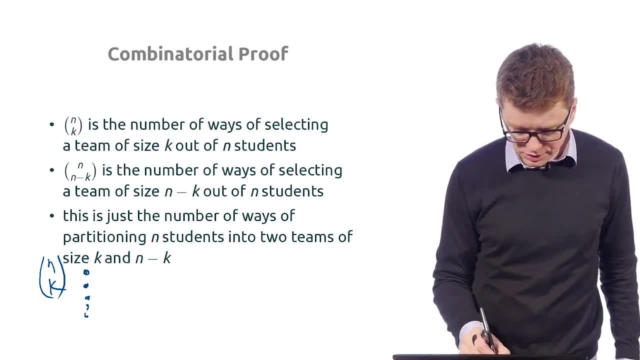 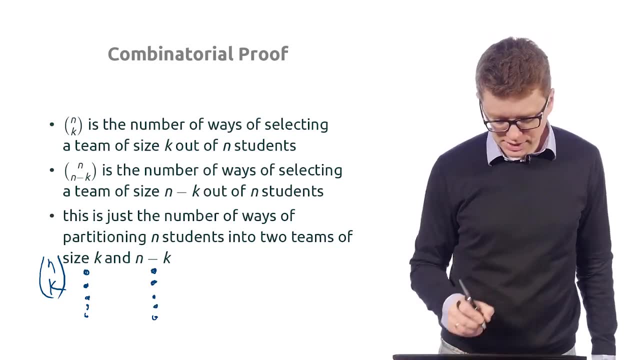 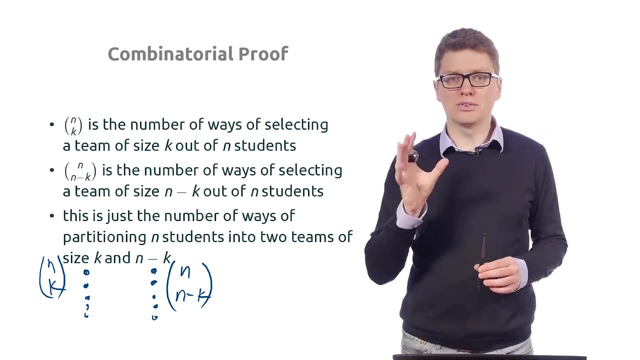 and there are n choose k of them, right? Then let's also draw here on the right, all possibilities of selecting subsets of size n, of size n minus k. So there are n choose n minus k of them And there is a one-to-one correspondence between them. 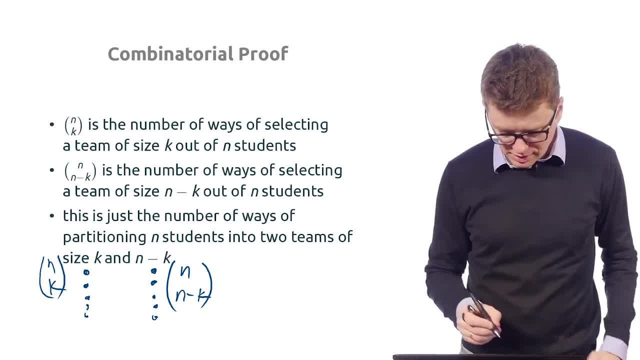 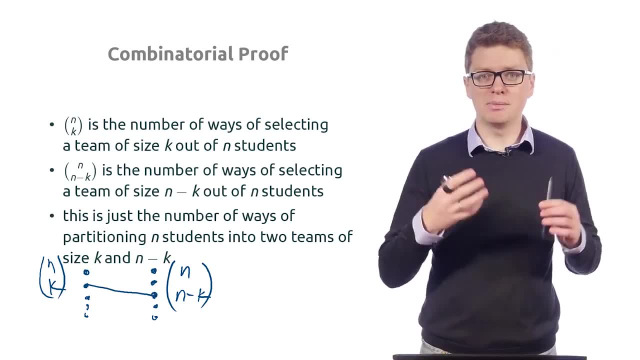 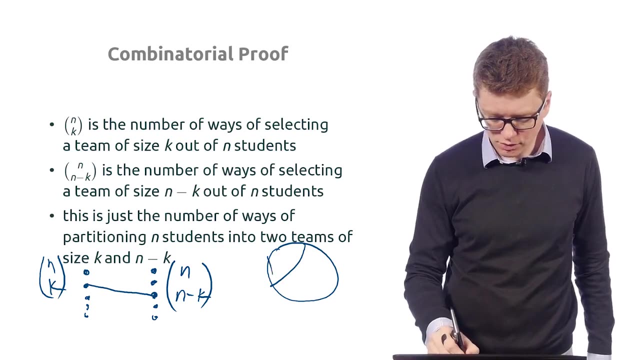 Namely, for each set of size k we can find a unique subset of size n minus k, Namely, this is just a complement of this set. So if we have a set of n elements and we selected k of them, then the complement, so this is the size of size k. 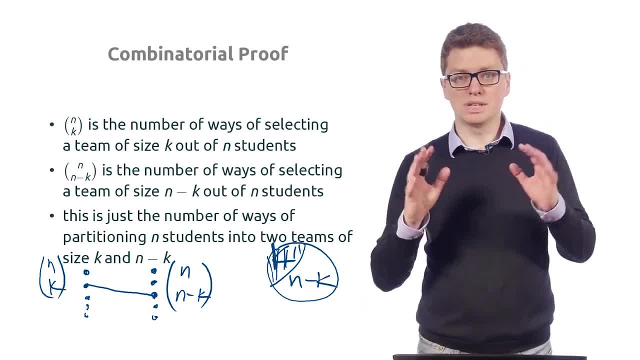 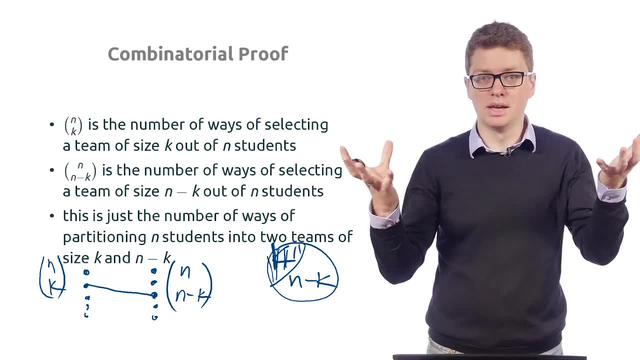 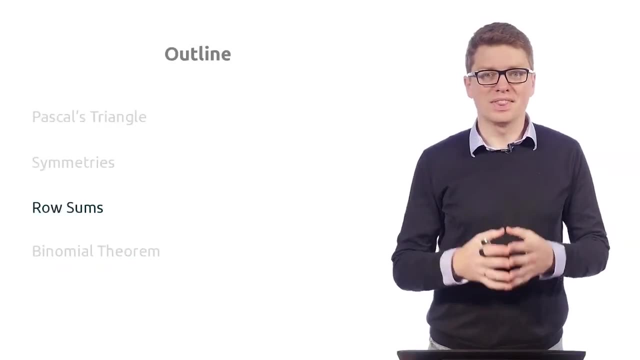 then the complement has size n minus k. So this establishes a one-to-one correspondence between sets of size k and sets of size n minus k, which basically proves that these two numbers are the same. We will now show that the symmetry is not the only remarkable property of Pascal's triangle. 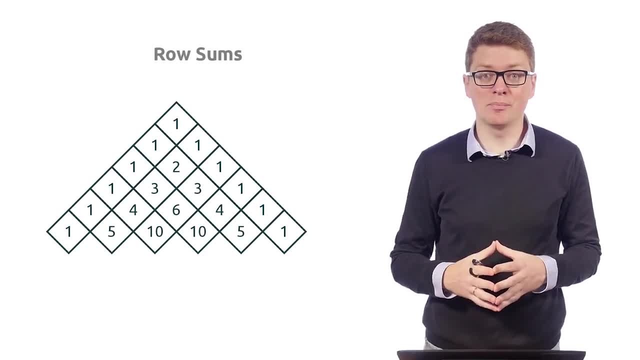 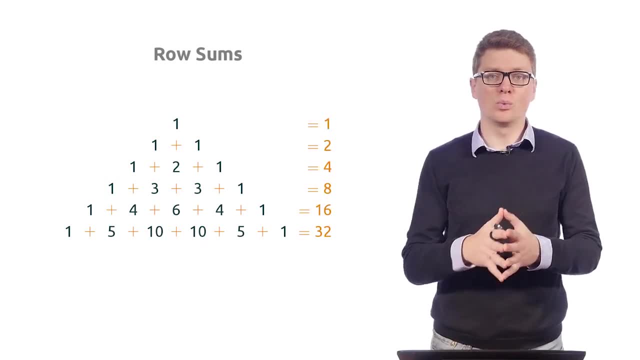 Mainly, let's do the following: Let's compute the sum of all the elements in every row of Pascal's triangle. okay, So what we see is that the sum in the first row is just one. There is a single element. In the second row, it is equal to one plus one. 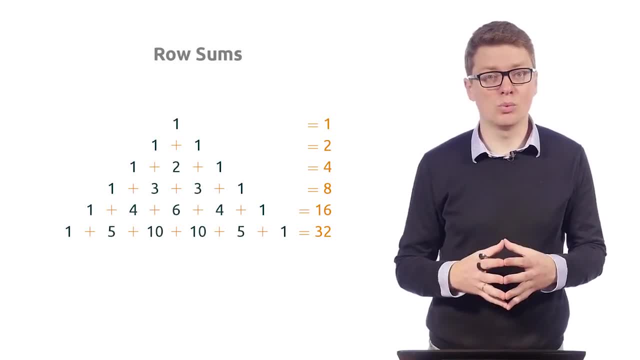 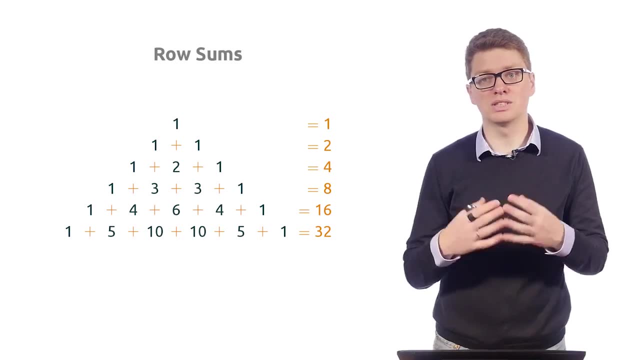 which is two. In the third row it is equal to one plus two plus one, which is nothing else as four. In the next one, it is one plus three plus three plus one which is eight, and so on. So you probably already see a pattern. 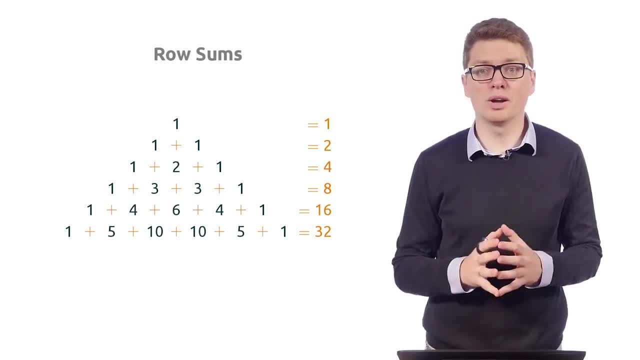 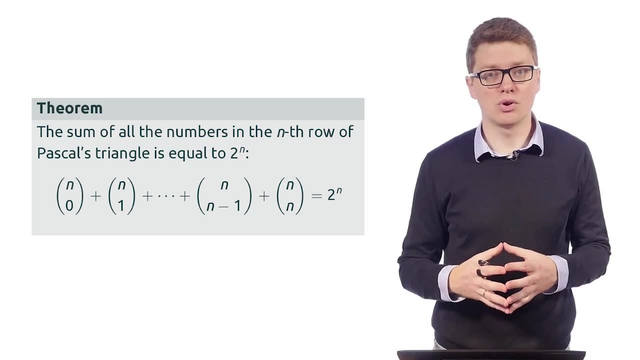 So these are just powers of two, and this is what we are going to prove now. So we are going to prove that the sum of all the elements in the nth row of the Pascal's triangle is equal to two to the n. We'll put it otherwise. 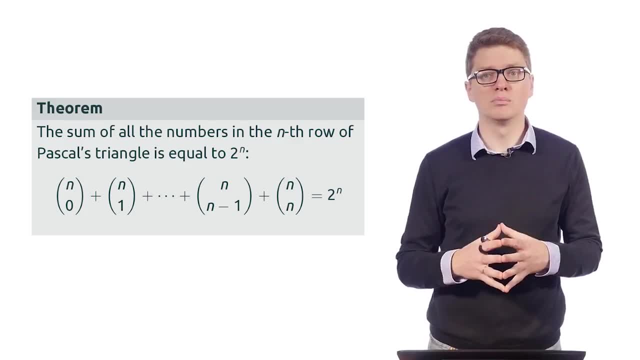 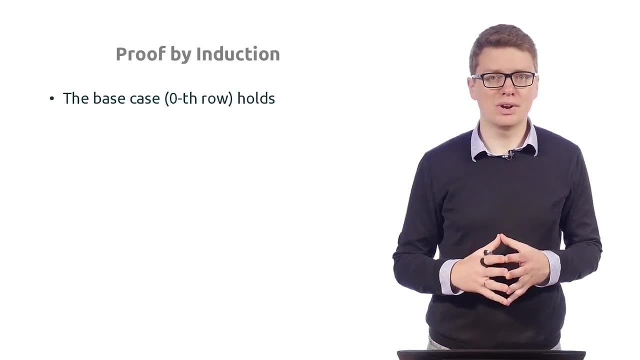 We're going to prove that n choose zero plus, n choose one plus, and so on. n choose one minus one. n choose n is equal to two to the n. okay, So there are again two proofs. One is slightly boring and it is completely formal. 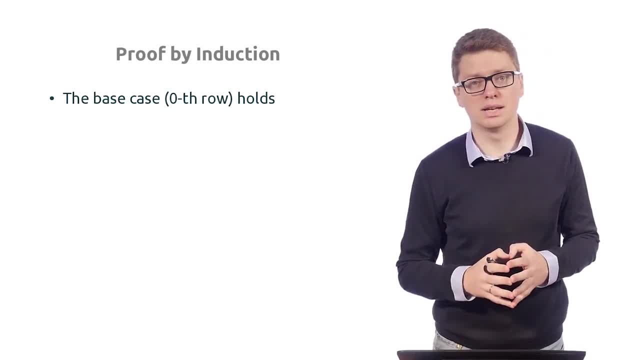 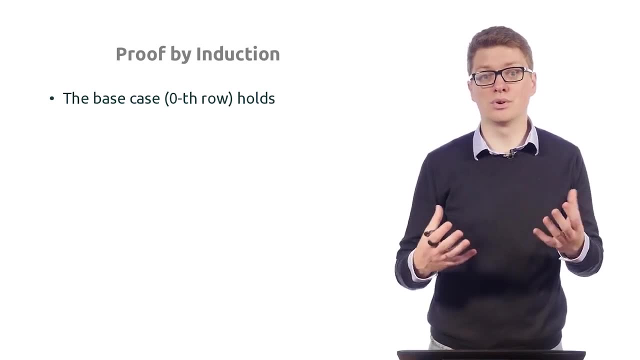 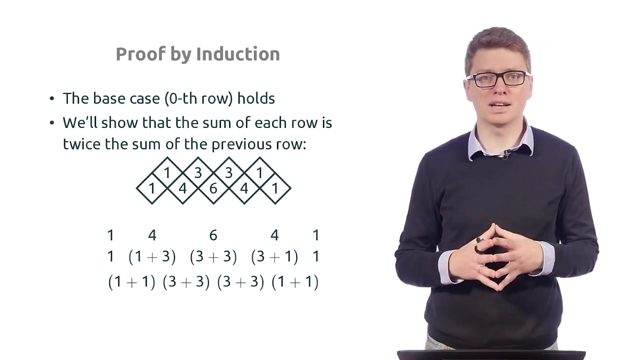 So we can show this just by induction on the number of rows. So it definitely holds for the first row and even for the several first rows, as we've seen already Right. On the other hand, if we would like to prove the step of our induction, 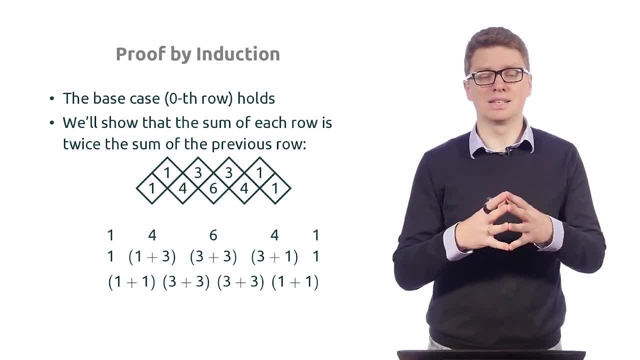 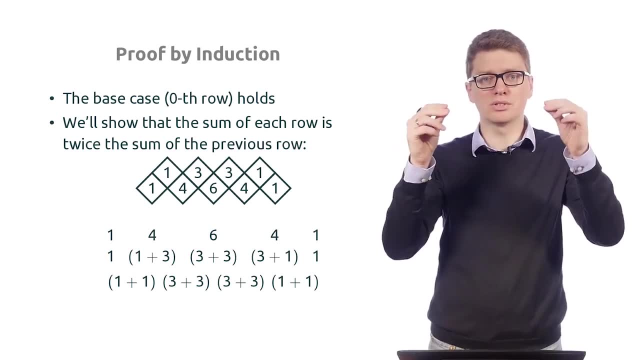 that is to prove that. if that we need to prove that for the nth row the sum is equal to two to the n, assuming that for the previous row the sum is equal to two to the n minus one, What we're going to show actually, 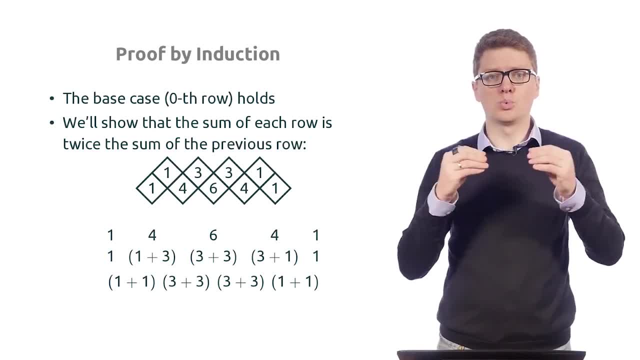 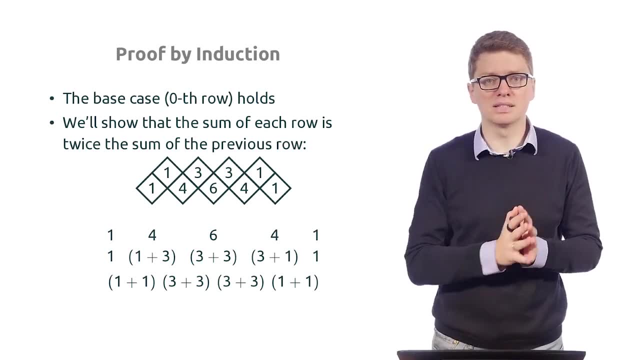 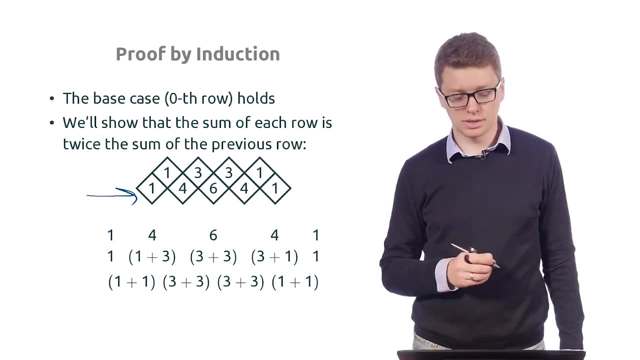 is that the sum in every row is twice the sum in the previous row, And we're going to show this just on a toy example To simplify things. So consider this row One, four, six, four and one, So the sum is the following: okay, 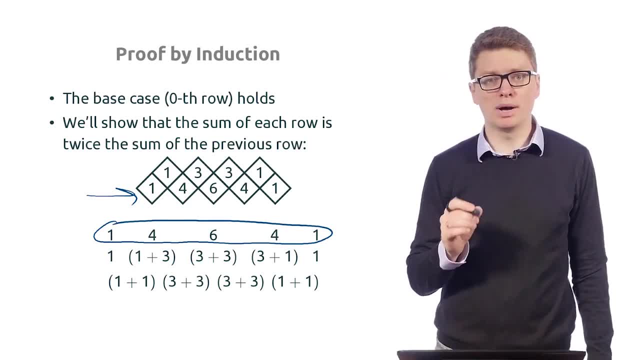 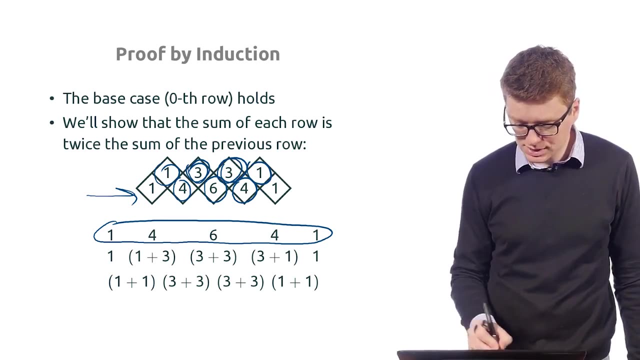 Now recall that this nice sum pattern in Pascal's triangle. So four is equal to one plus three. Six is equal to three plus three. Four is equal to three plus one. okay, Let's now represent four, six and one, Okay. 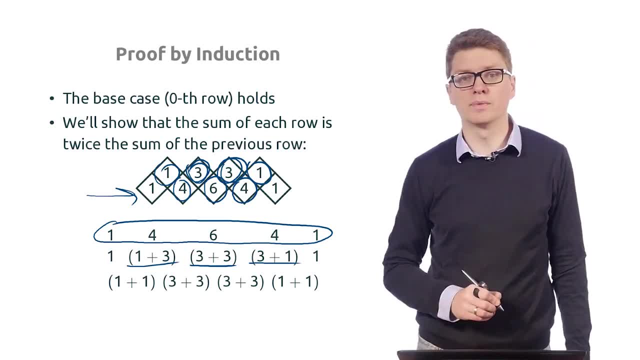 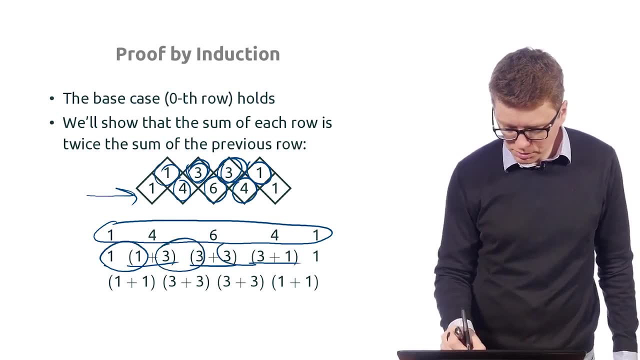 So six and four is one plus three, three plus three and three plus one. Okay, Now let's regroup all our terms. Then what we get is one plus one, three plus three, three plus three and one plus one. 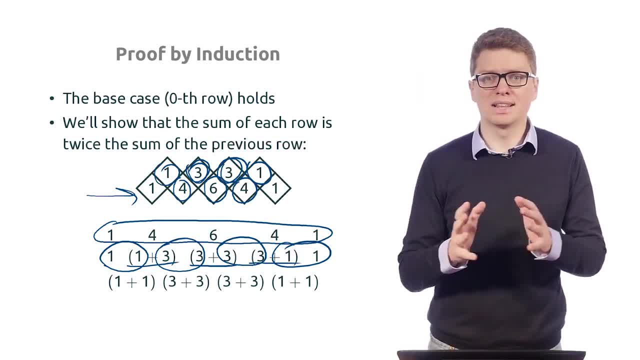 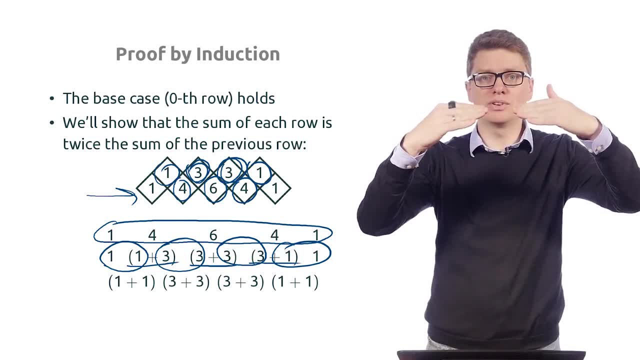 So, in fact- and this holds in general, So, in fact, if we regroup all the terms, if we express the sum in the current row via the sum in the previous row, then all the elements from the previous row appear exactly twice, which gives us okay. 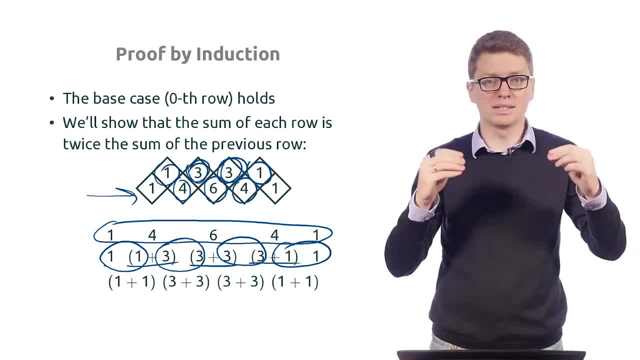 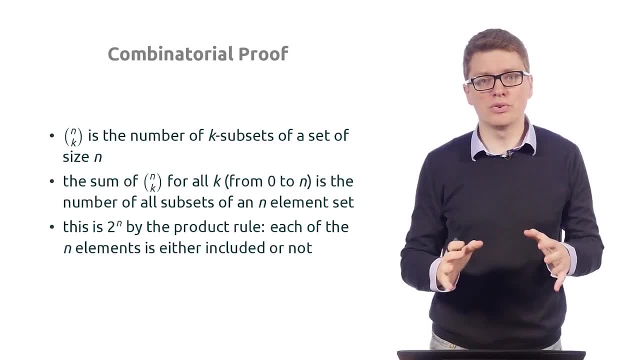 which gives us actually that the sum in the current row is twice the sum in the previous row, which concludes the proof by induction. But now let's focus on the combinatorial proof of this equality. So recall that n choose, k is usually the number. 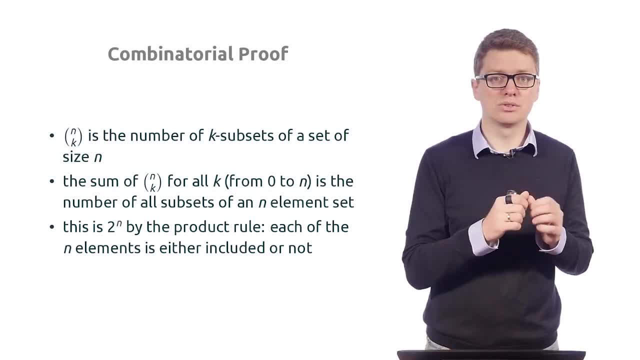 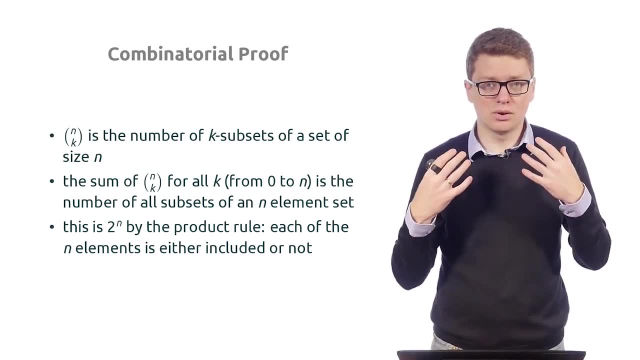 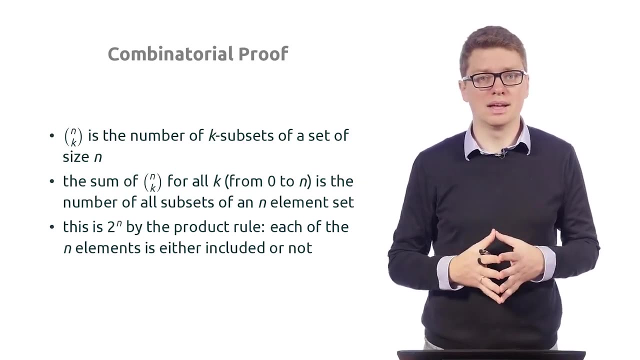 of subsets of size k. When k ranges through all the values from zero to n, we actually compute the number of subsets of all possible size from zero to n, right? So the sum of all n. choose k where k ranges from zero to n. 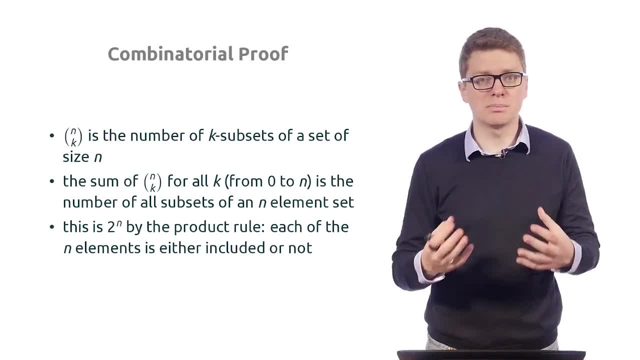 is actually just the number of all possible subsets of our n element set, And this is known to be two to the n, and actually it follows from the product rule, Since you would like to compute the number of ways of selecting a subset of our n element set. 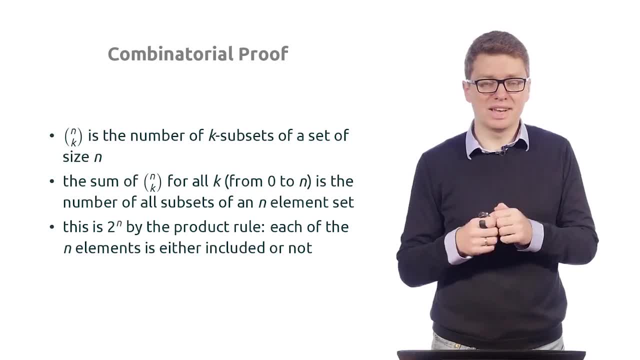 then, for each element, for each of the n elements, there are exactly two possibilities: You either take it into your set or you don't take it. Okay, so the resulting number is two times two times two times two. so n such terms. 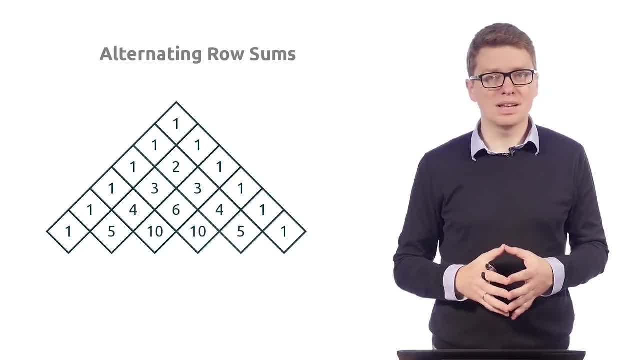 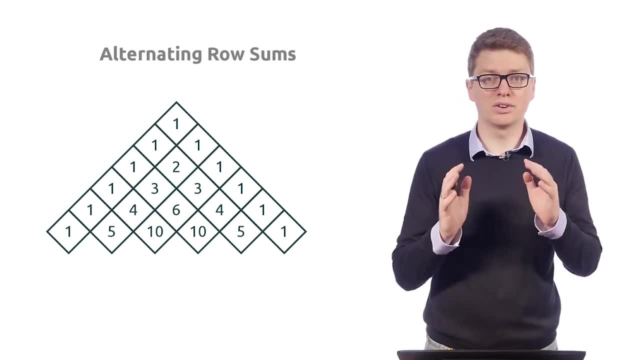 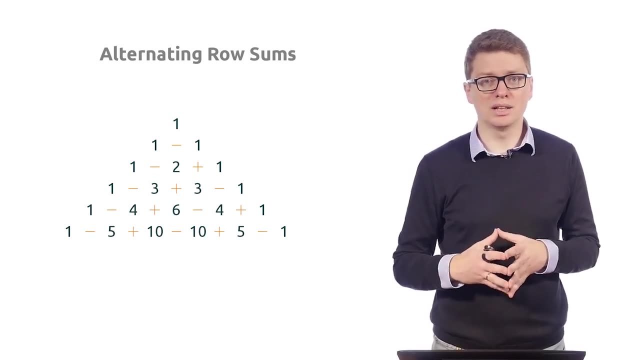 which is nothing else as two to the n. okay, So another nice property is the following: It is now not about row sums, but about alternating row sums. So instead of just computing the sum in each row, let's compute the following alternating row sums: 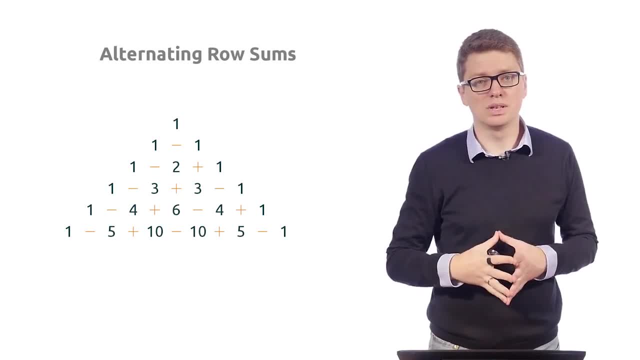 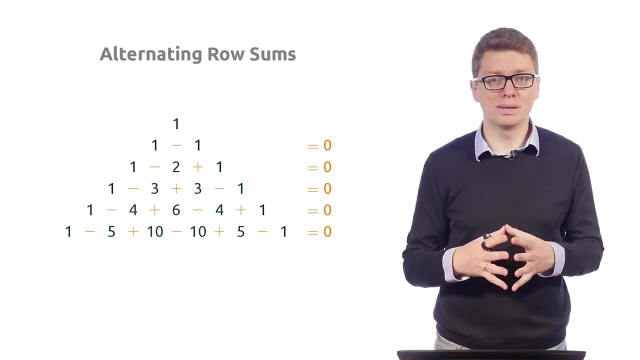 So each subsequent term is taken with either with plus or minus sign. okay, Then, for every row except for the first one, what we see is that such a sum is equal to zero. So in the first, in the second row, I'm sorry. 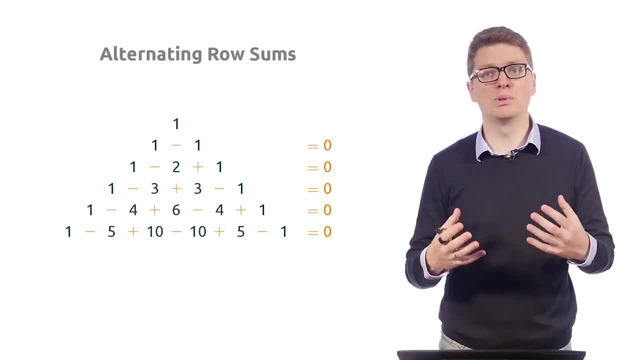 it is one minus one. In the next one it is one minus two plus one, which is zero. again In the next one it is one minus three plus three minus one, which is again zero. So for some rows it is immediate that it is equal. 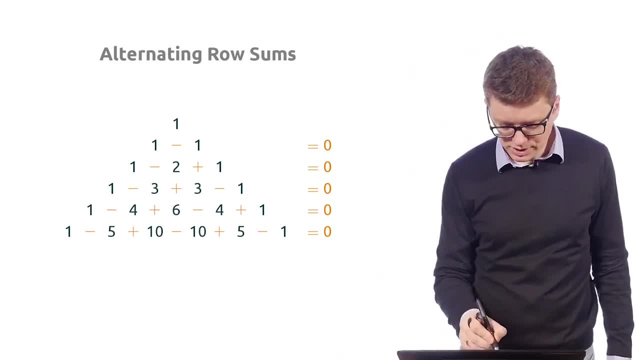 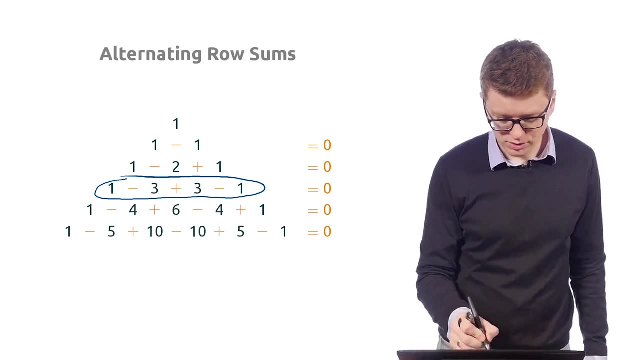 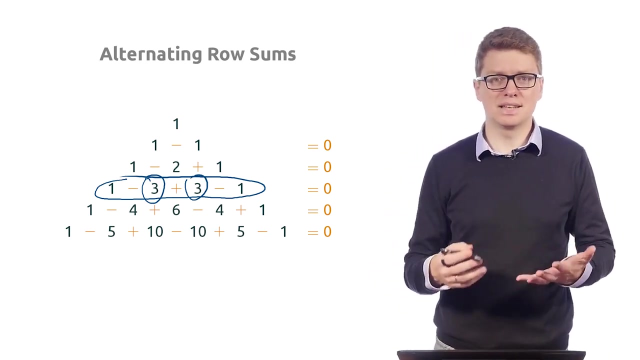 to zero just because they are symmetric. For example, this row is symmetric, So it has one, three, three, one And one of these. one of these two elements appear with plus and one appears with minus. So it is not surprising that everything. 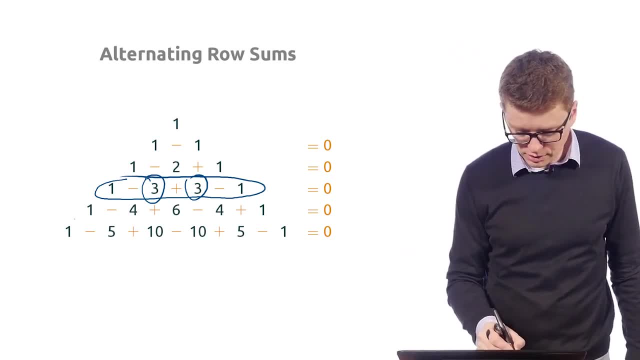 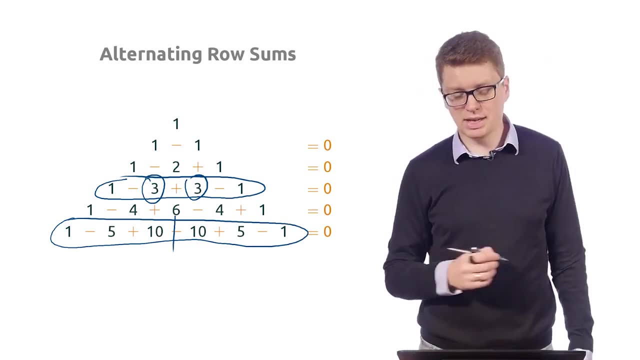 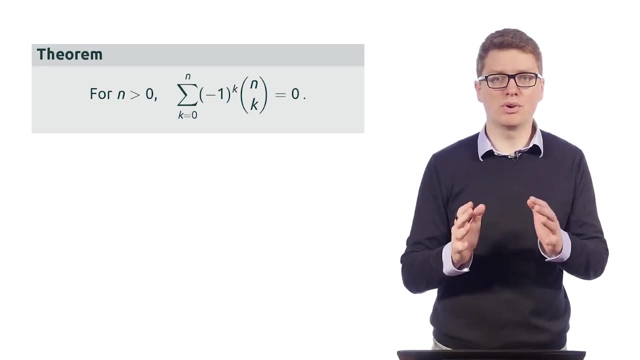 like telescopes or counsels, are For this row. it is also immediate. It is also a symmetric right And is taken with plus sign and with minus sign. For other rows it is not so immediate, but still it can be shown, And before this let's state it formally So for every row in our Pascal's. 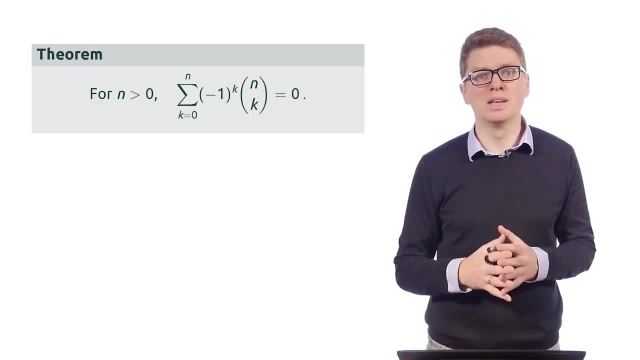 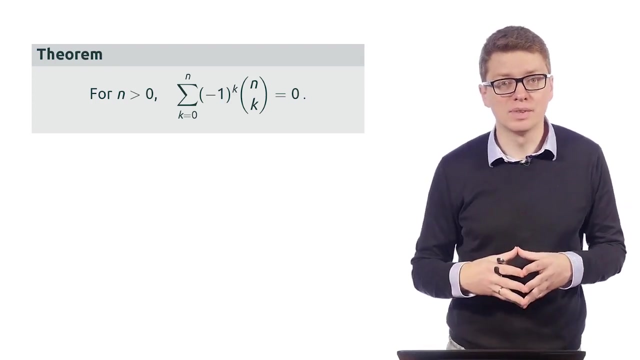 triangle, except for the first one, the alternating sum is equal to zero. The alternating sum can be represented as follows: So instead of computing just the sum of all possible n, choose k. we take and choose k with, with multiplier minus one to the k. So this is exactly so, minus one to the k. 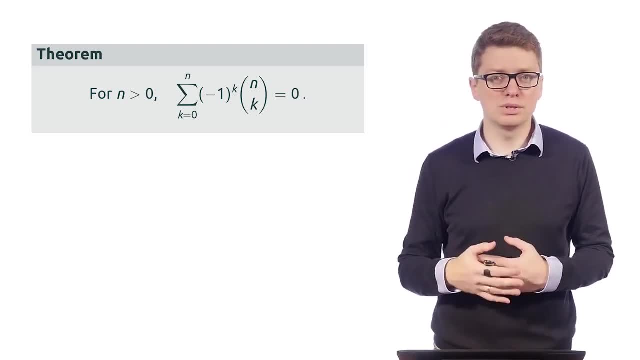 provides this alternating of sums. So when k is equal to zero, minus one is to the k is equal to one. When k is equal to one, minus one to the one is equal to one. So minus one to the k is equal to minus one when k is odd, and is equal to one when k is even. So that gives exactly. 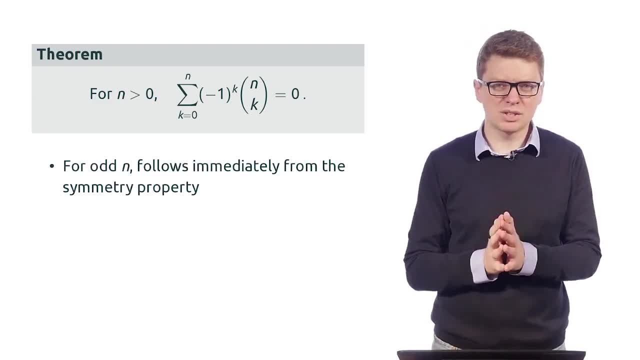 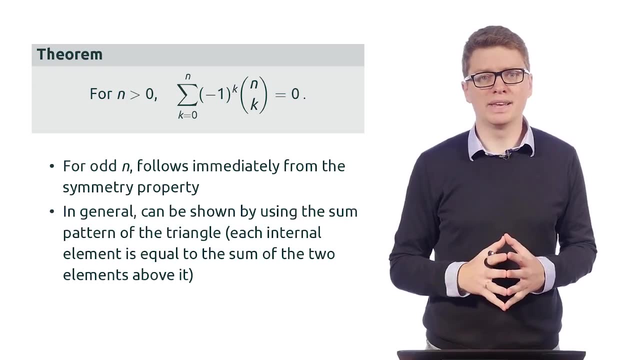 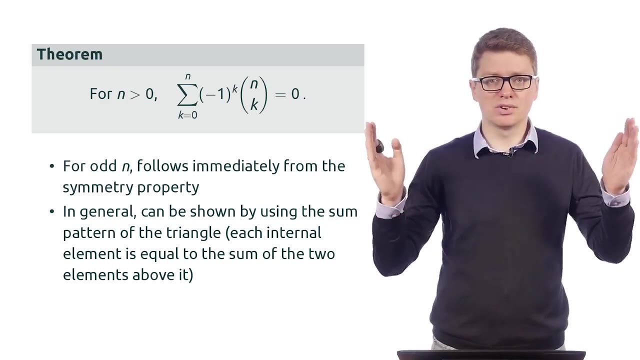 alternation. So, as we've discussed already, for some rows it is just immediate. For some other rows it also can be shown by by using this sum pattern of Pascal's triangle, Namely if you just represent this alternating sum of the current row via the previous row, I mean if you replace each element. 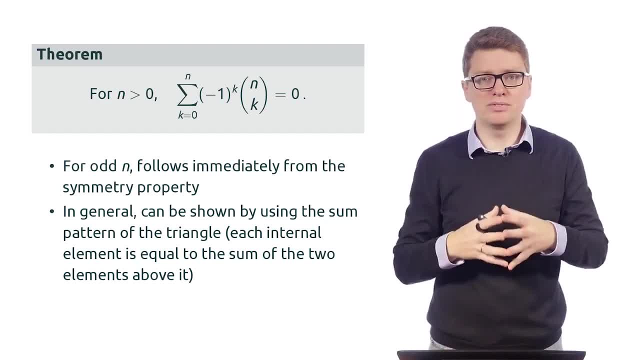 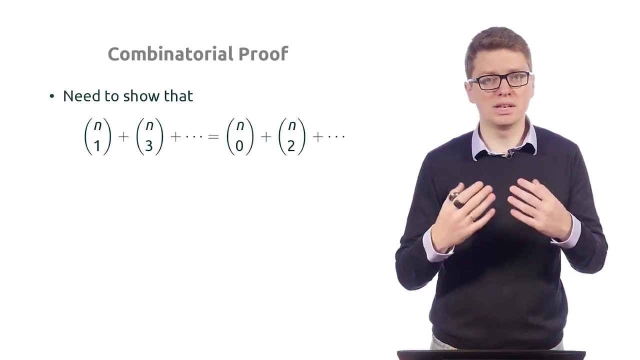 with with the sum of two neighboring elements from the previous row, you will see that each element from the previous row is taken once With with positive sign and once with negative sign, So everything cancels out. Okay, so this is just like a hand wavy formal proof, But let's instead again focus on combinatorial proof. So we 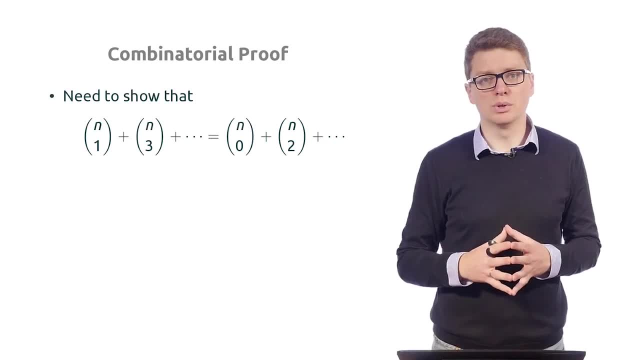 need to show that the alternating sum is equal to zero. If we take all, the all the elements with the negation sign to the right, Then what we need to show is that n. choose one plus n. take three and choose, and so on. all uh for all odd k is equal to n. choose zero and choose two, and so on. 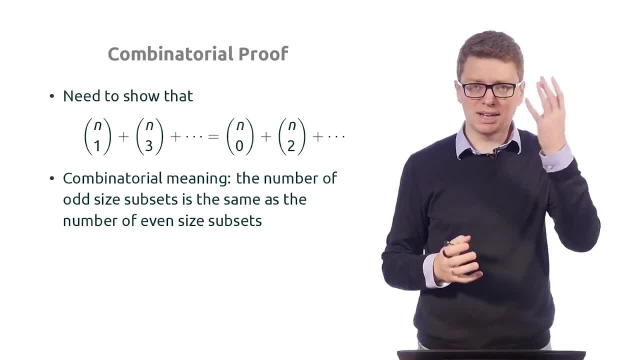 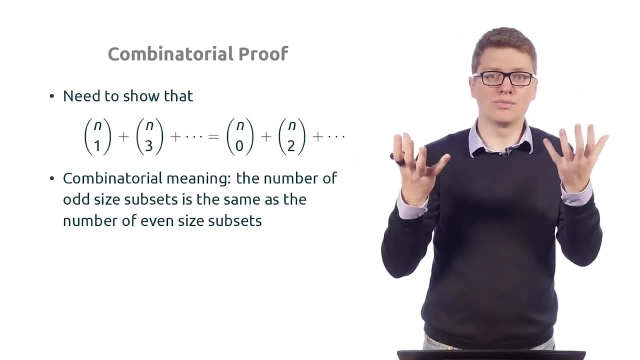 okay. so what basically we need to show is that what basically stays on the left is the number of subsets of even size, and what stays on the right is the number of subsets of odd size. so this is also another nice property. what we are going to prove now, the combinatorial meaning of 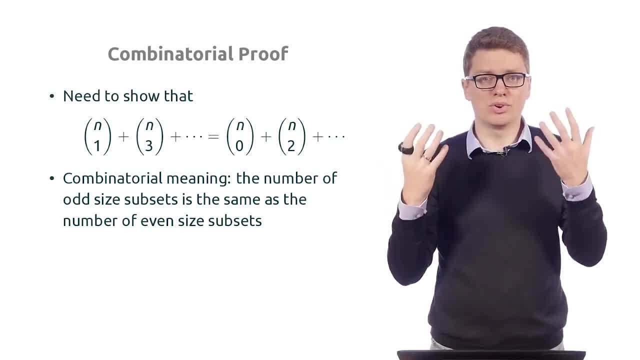 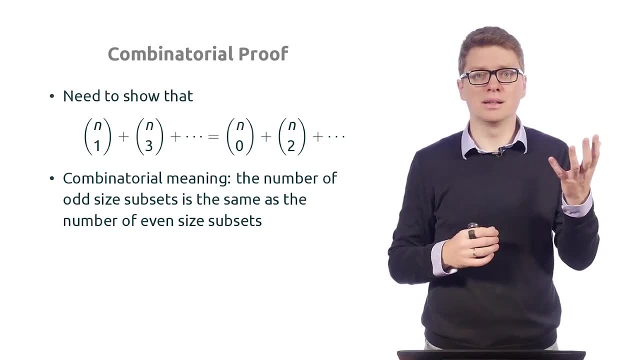 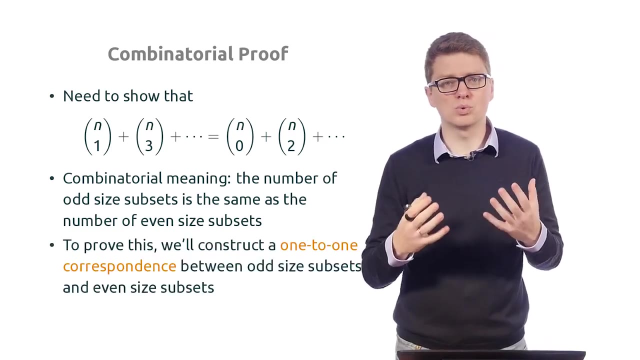 the equalities that we are proving is the following: that for every n greater than zero, an n element set has the same number of odd size- odd size subsets, i'm sorry- as the number of even size subsets. okay, so to prove this once again, we are going to establish one-to-one correspondence. 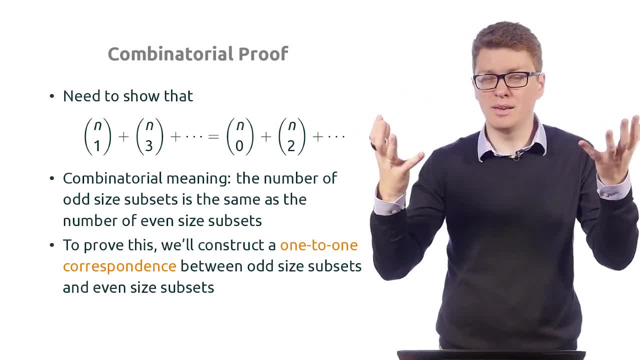 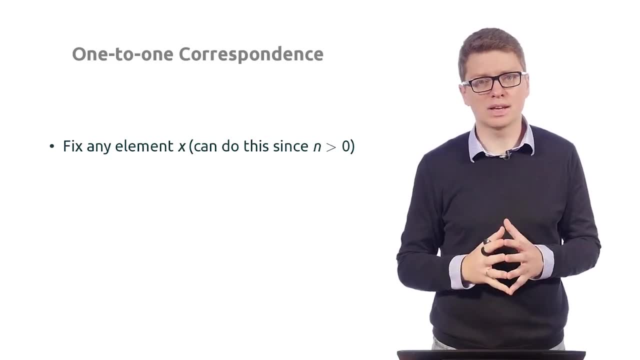 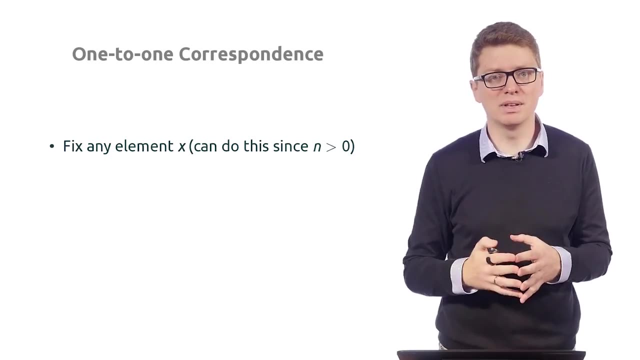 between all such subsets and all such subsets. okay, and for this we are going to do the following: let's fix any element, x, okay, and we can do this fixing just because n is greater than zero. so we have at least one element. now we are going to establish this one-to-one correspondence as follows: so: 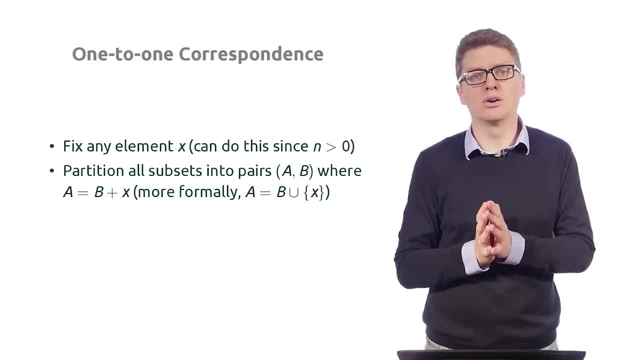 one-to-one correspondence is essentially like partitioning all the all the subsets into pairs, and we are going to form the pairs as follows. let's say that the subsets a and b form appear if they differ just by by the element x, namely if if one gets a by adding the element x to b. so what is written? 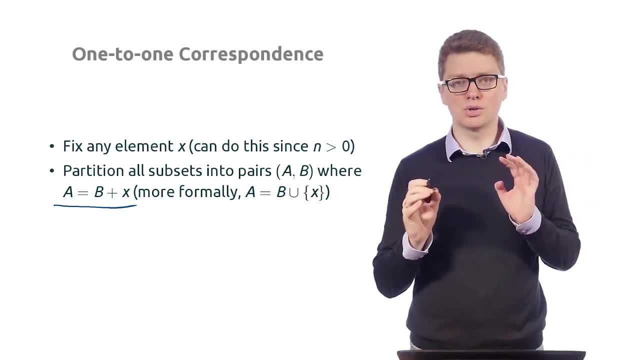 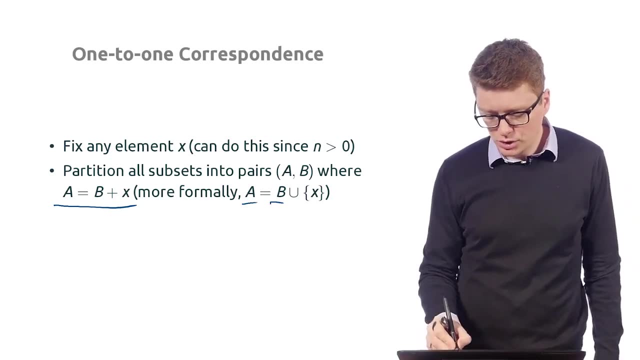 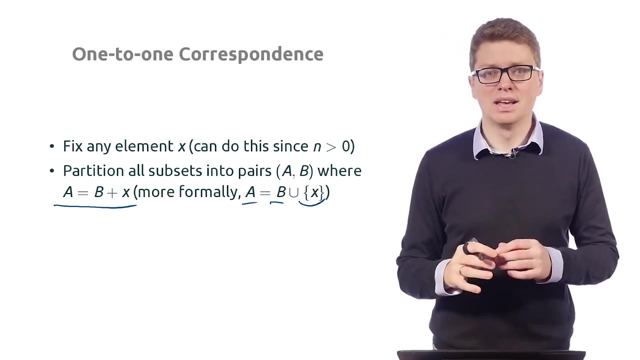 here is that a is b plus x. it is slightly informally, so more informally, in terms of, in terms of of sets, a is equal to b union, with the single element x. so this x embraces means that we're considering x, uh, as as a, as a set consisting of a single. 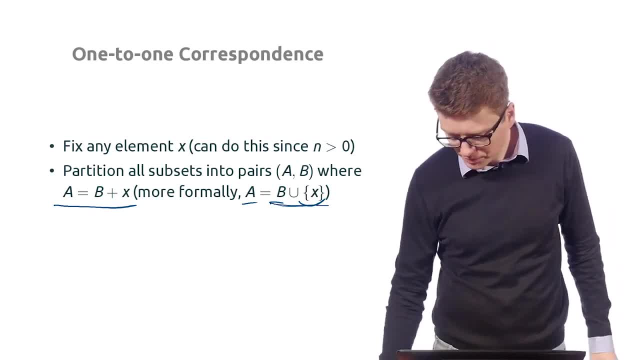 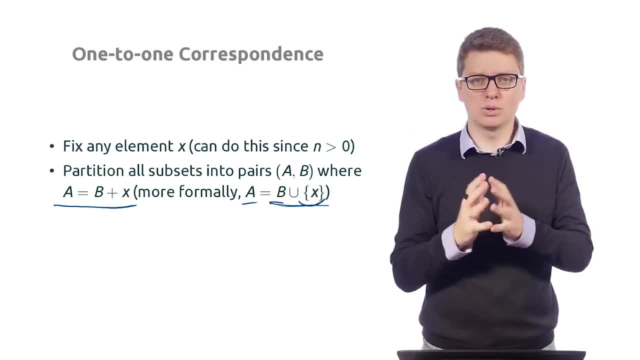 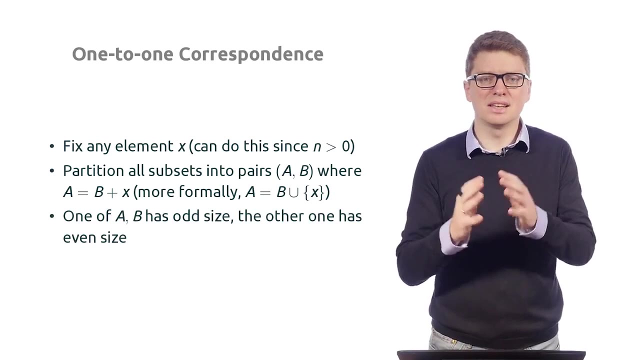 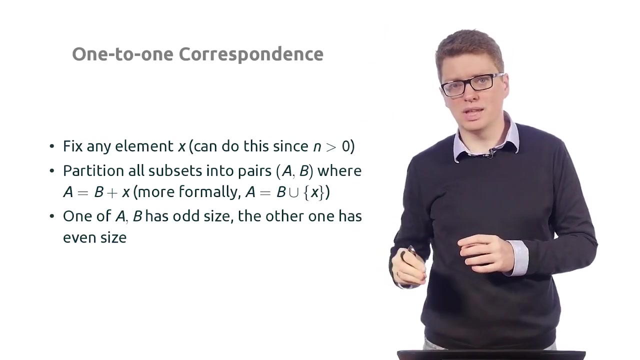 element x, and here we take a union of b and x. so for each uh, once again, so b is is- is a subset without x, and a differs from b just by adding x. so it is clear that this is indeed an one-to-one correspondence, right? so if uh, for we take all the subsets without x and by adding x to them we get 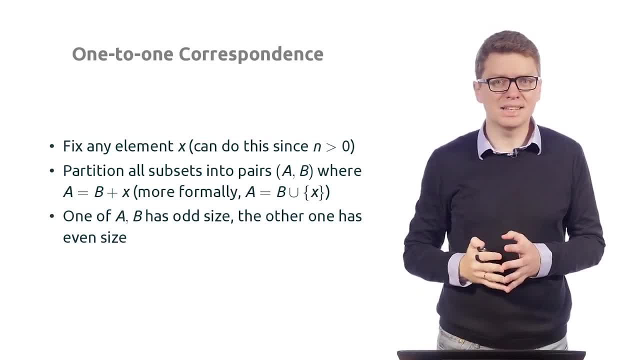 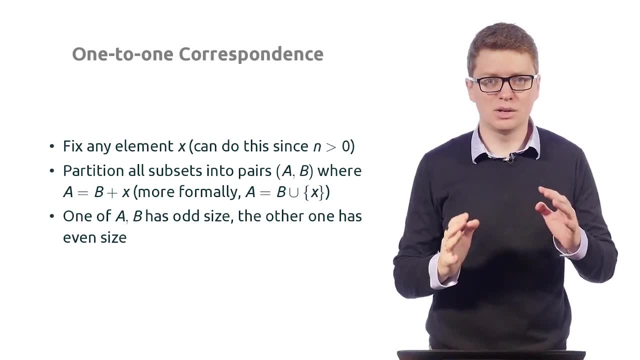 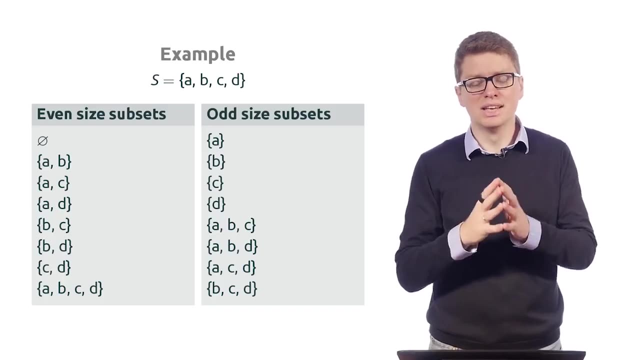 exactly the same number of subsets right. on the other hand, it is clear that exactly one in this pair of a and b has even size and exactly one of them has odd size right, because their size differ by one. so which means that we actually split all our, all our subsets into pairs and in each pair there is one subset of odd size. 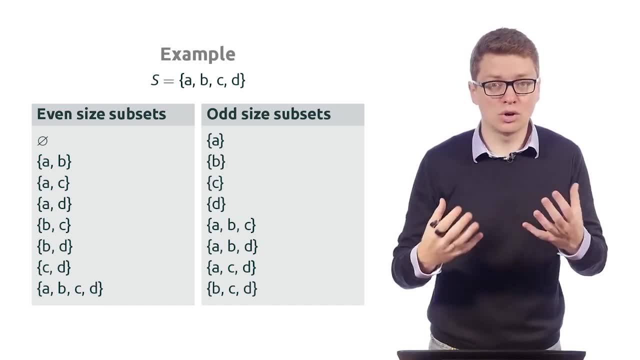 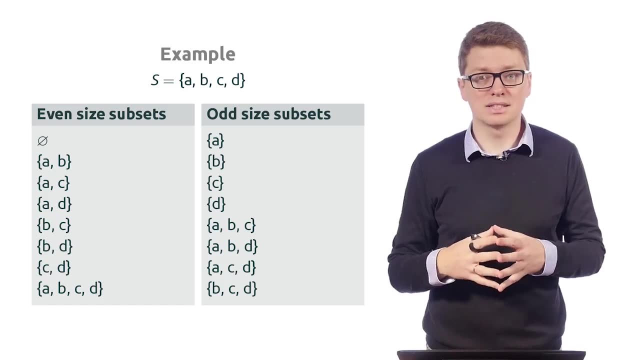 and there is one subset of even size, and this in turn means that there are the same number of odd size subsets as the number of even size subsets. finally, here we show an example: if we have, if our ground set denoted by s has four elements, then on the left we list all, uh all its subsets. 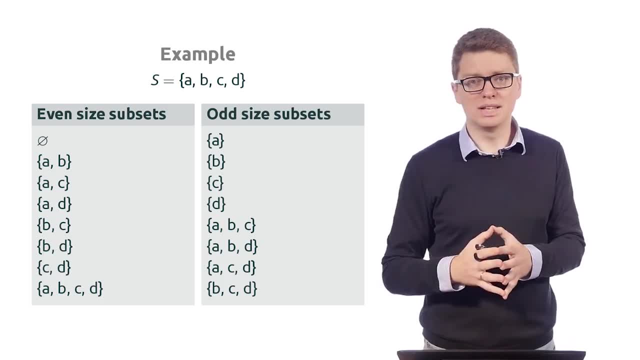 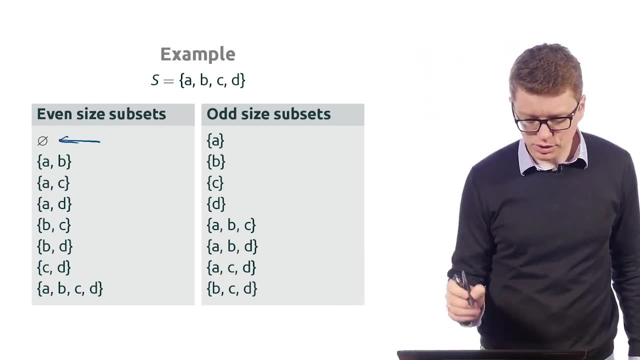 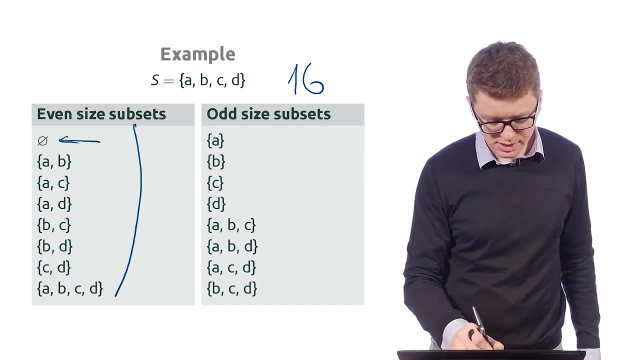 of even length, of even size, and on the right we list all its subset of port size. so note in particular that we also count the empty set, as usual. so the total number of subsets is is 16 and, as you see, the number of subsets of even size is 8 and the number of subsets of 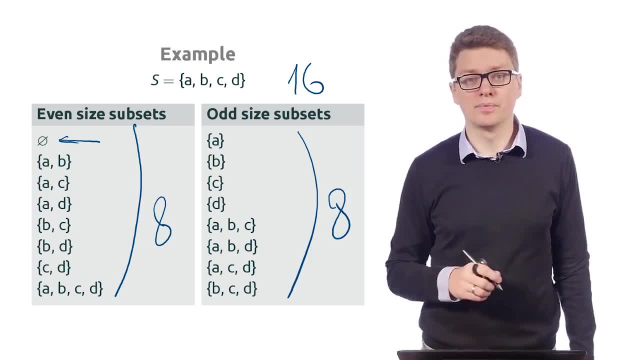 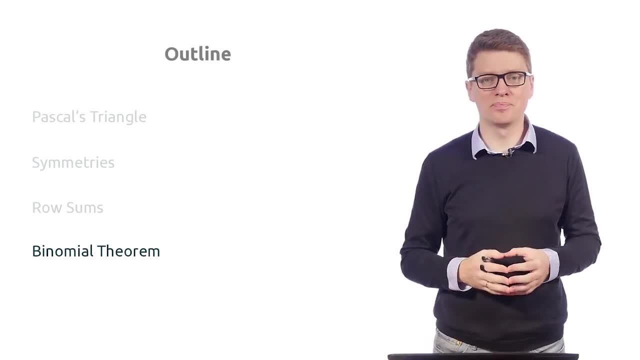 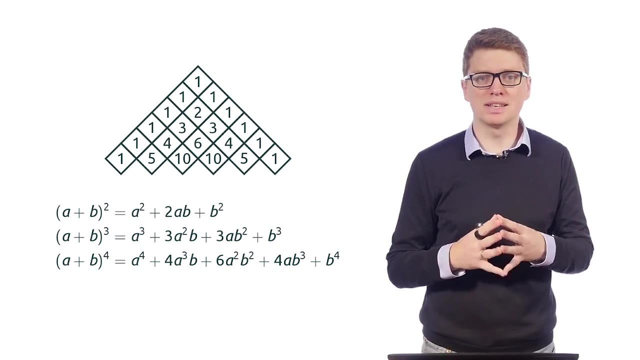 odd size is also 8.. we conclude the current lesson with the well-known binomial theory. so it states that, uh, the, the coefficients of all the monomials in the expression a plus b to the power of n, are actually the, the numbers from the nth row of pascal's triangle. so let's check this. 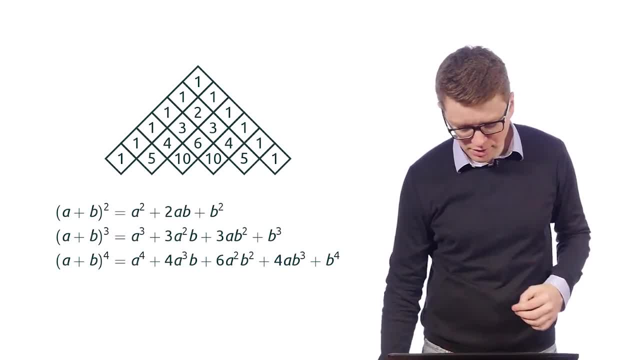 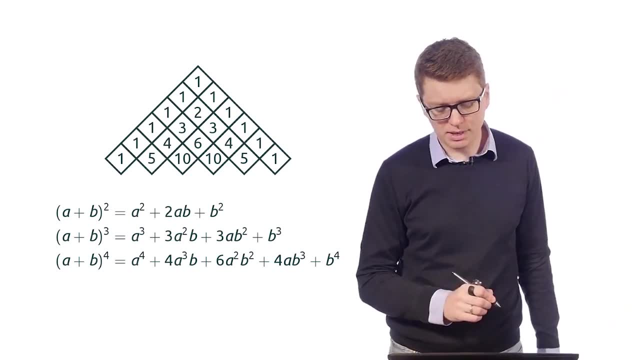 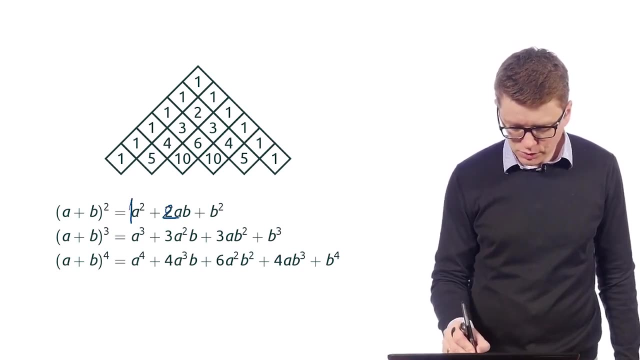 for for small values of m. okay, so if if one computes a plus b squared, then this is a well-known formula. it gives a squared plus two, a, b plus b squared. so essentially the coefficients for the monomials here are one, two and one, and these are exactly the coefficients from. 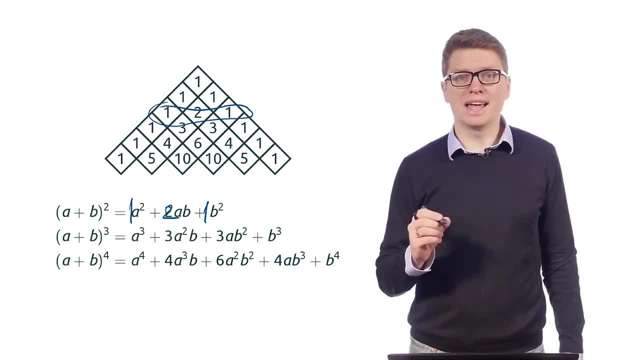 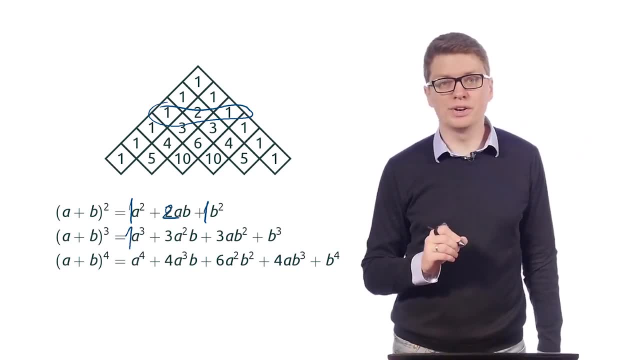 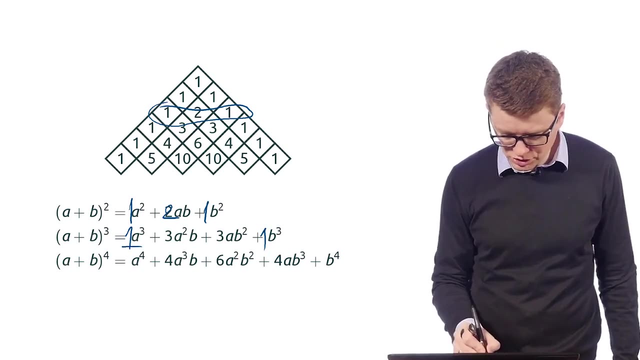 this row. another example: if we consider a plus b cubed, then it is 1 times a cube plus 3 times a squared b plus 3 times a b squared plus 1 times b cubed. so these coefficients- 1, 3, 3 and 1 are exactly. 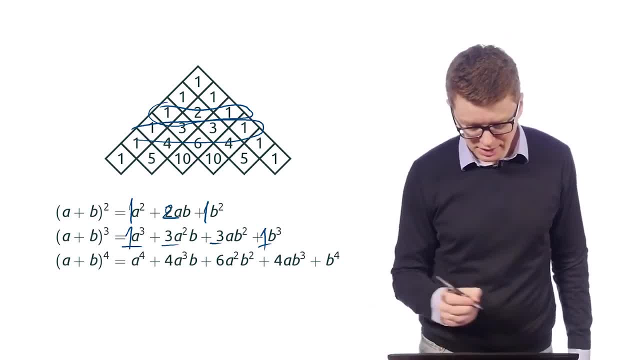 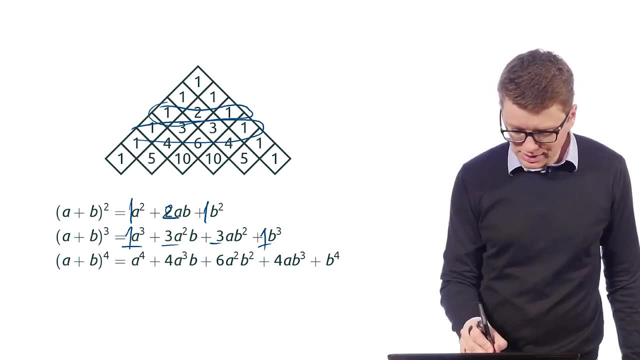 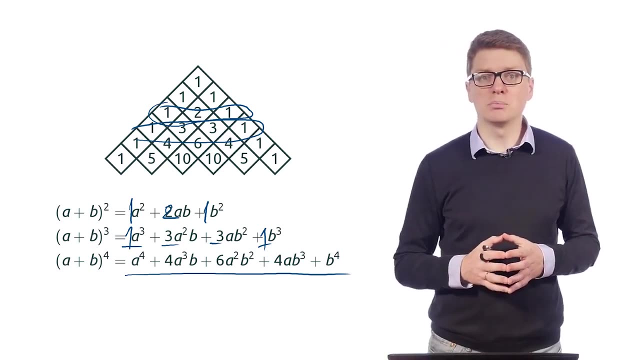 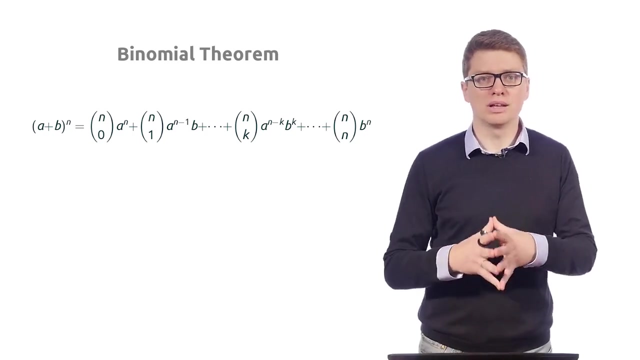 the coefficients from the pascal's triangle. okay, let me also omit just the example. for a plus b to these are 1, 1, 4, 6, 4. 1 are exactly the coefficients for for the next power of a plus b. so more generally, a plus b to the n is equal to n. choose 0 times a to the n plus m. choose 1 times n times. 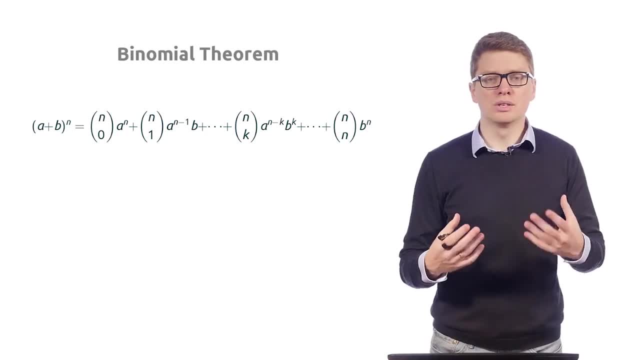 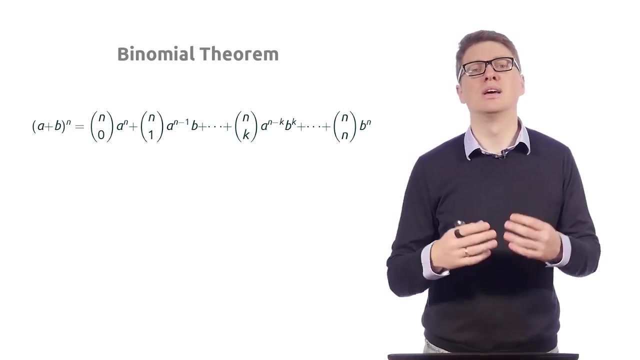 a to the n minus, 1 times b plus, and so on. so the general term in this expression is n. choose k times n minus k times b to the k, and so on. so the last term is then: choose m b times times b to the n. so 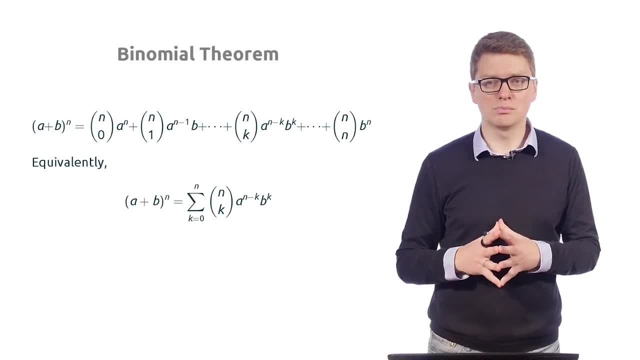 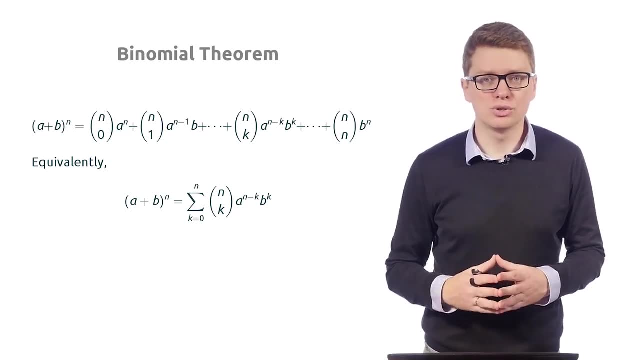 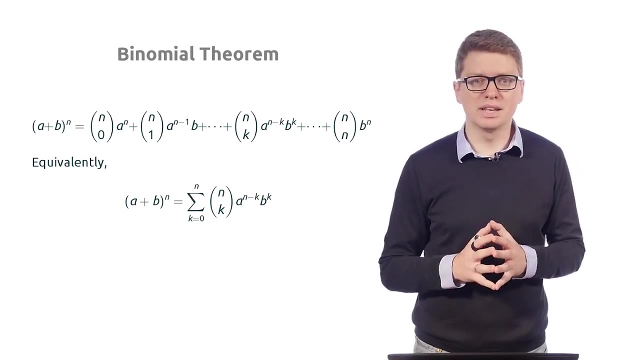 in terms of sum, it can be written as follows: a plus b is equal to sum overall k ranging from 0 to n of n choose k times a to the n minus k, b times b to the k. okay, for this reason, n choose k is called a binomial or binomial coefficient. 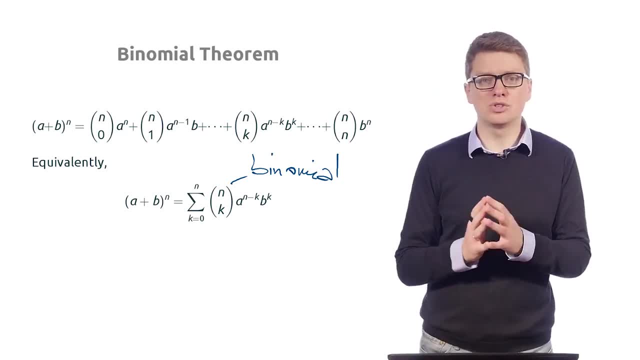 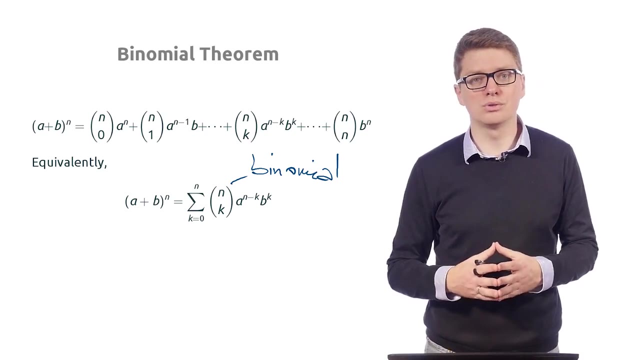 okay, so it also has. so on one hand, n choose, k is the number of ways of selecting a subset of size k out of a set of size n. on the other hand, it is also a coefficient of the monomial a to the n, minus k times b to the k in, if you open the expression. 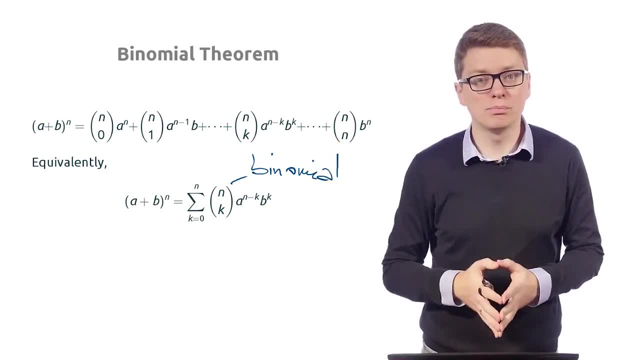 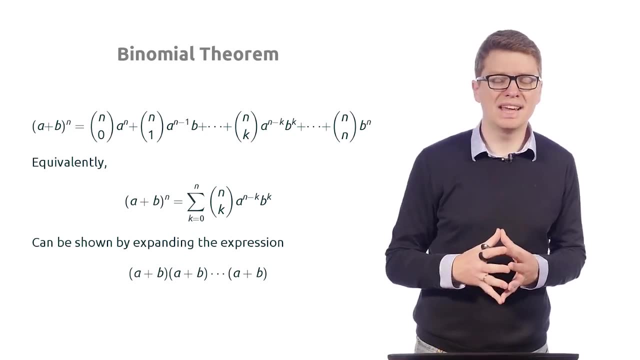 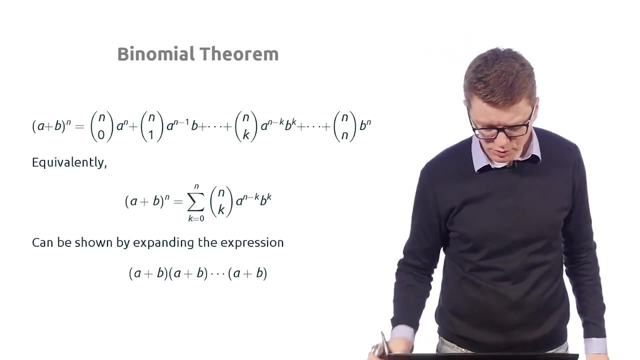 a plus b to the n, if you represent it just as a sum of monomials. okay, so the proof of this, of this theorem, is actually straightforward: a plus b to the n is just the product of a plus b, a plus b and so on: a plus b and times. so if you start opening opening this expression, then of course, 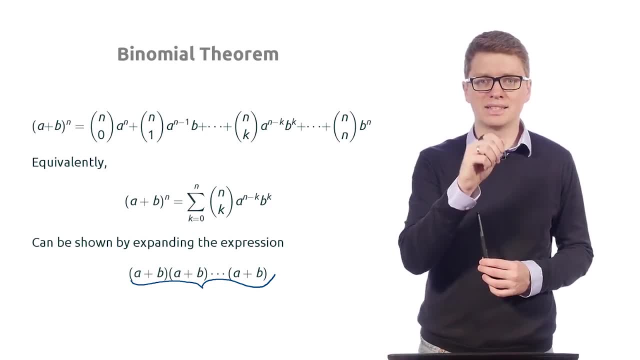 from every, from every term, you need to select either a or b right, and in particular, every monomial that you get has degree n. so you you take, for example, k, kb, and then you are forced to take also n minus k a's, and this gives you a monomial a to the n minus k, plus times b to the k. 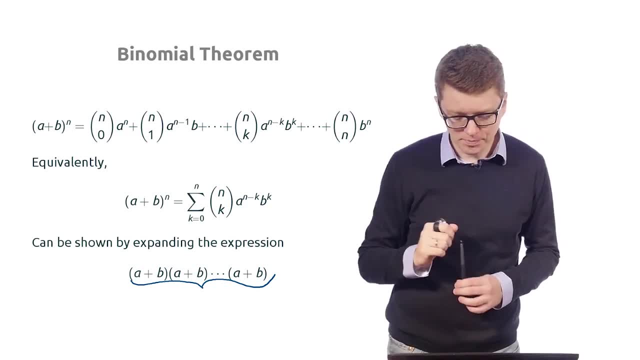 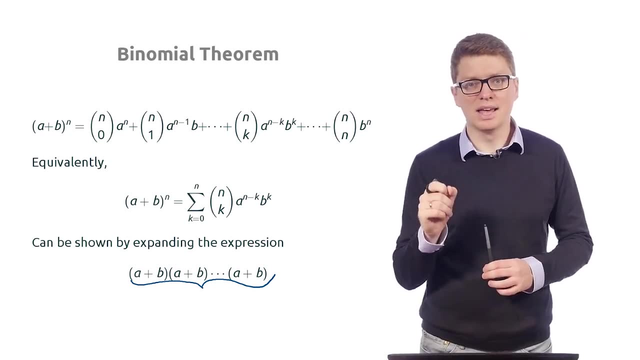 right. so the degree of this monomial is n okay. so, however, there are many, many ways of selecting k b's and n minus k a's right, and plus k squared, you get a more kitchen: 100. 2.cause so? but you also have a chance to do n minus k a's right, and then you do a tomorrow right, and then you, they, you pay p. x back and wave 14. all right so, but you still try to choose a, believe it or not, you do, and then you use k as v, as a degree. you do it, and then you have the boundary of this algorithm at the end of this. okay, so let's, maybe you'll say, although there are many, many ways you can choose kb's and n minus kz. 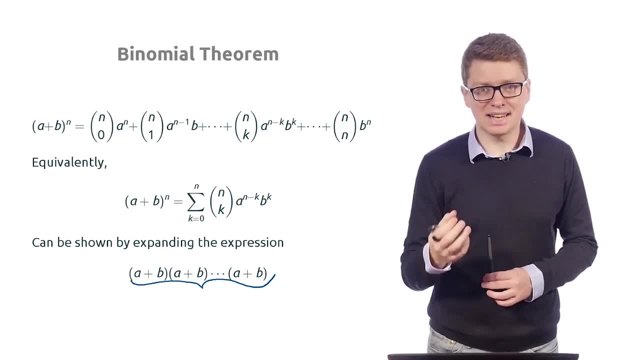 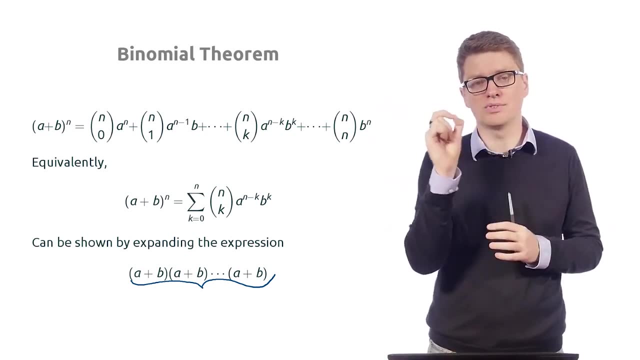 And the number of ways of selecting kb's is exactly n. choose k right. So you have n terms And out of these n terms, you are going to select k terms from which you are going to select b. So the number of these ways is n. choose k right. 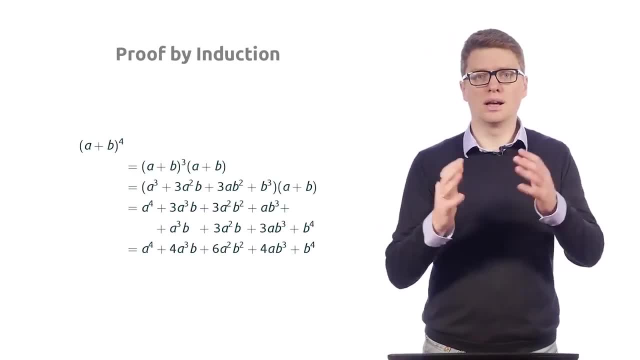 Exactly Okay. so this also can be proved by induction using the Pascal's triangle, So by induction on n, So for n equal to 0, or 1, or 2, or 3, or even 4, we've already checked this right. 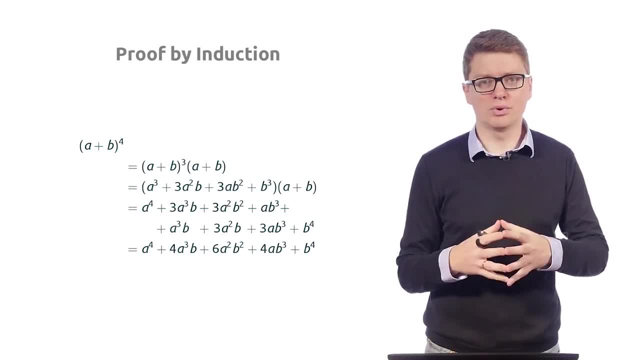 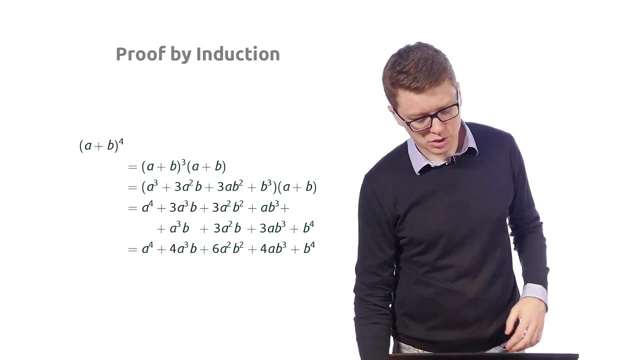 Now let me show you how the statement for n equal to 4 follows from the statement for n equal to 3.. And this actually shows a general pattern. So in fact it uses the sum pattern of Pascal's triangle. Okay, so a plus b to the 4 is of course equal to a plus b cubed. 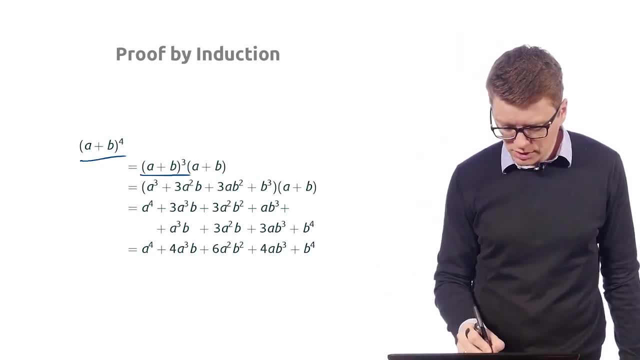 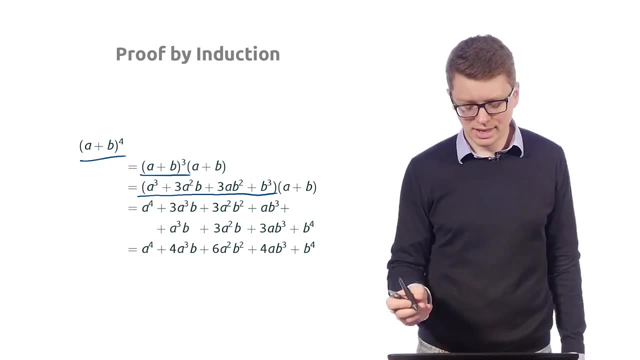 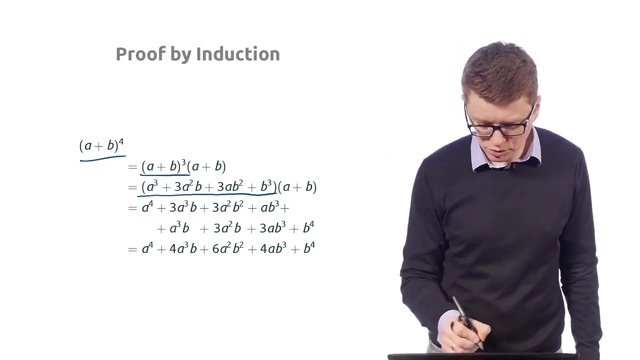 times a plus b. On the other hand, we already know the expression for a plus b- cubed, And I assume that we are proving this by induction. Then all the coefficients just go from the third row of the Pascal's triangle, And now we need to multiply this expression with a plus b. 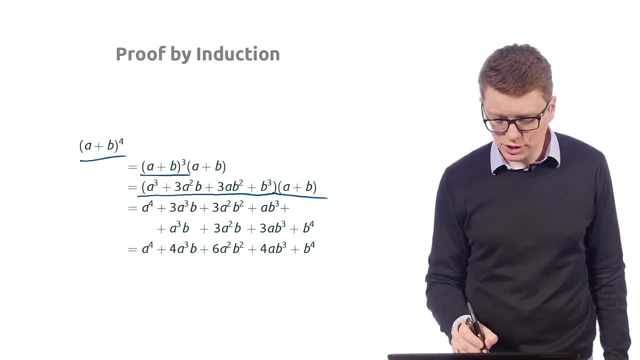 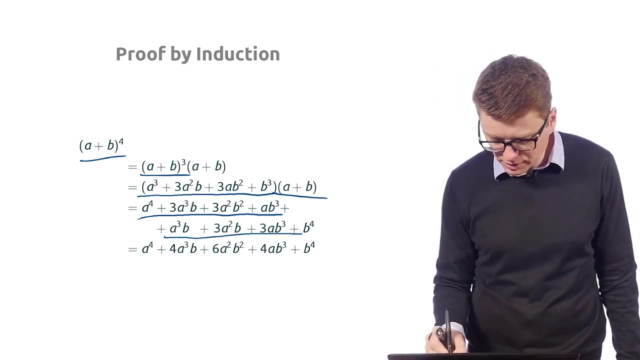 So let's just do this in a straightforward fashion. So a cubed plus 3a squared b plus 3ab squared plus b cubed. Multiply it by a, we get the following expression: Okay. Then, when we multiply it by b, we get the following expression: 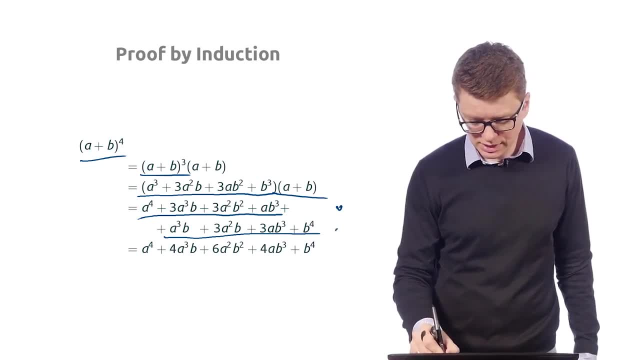 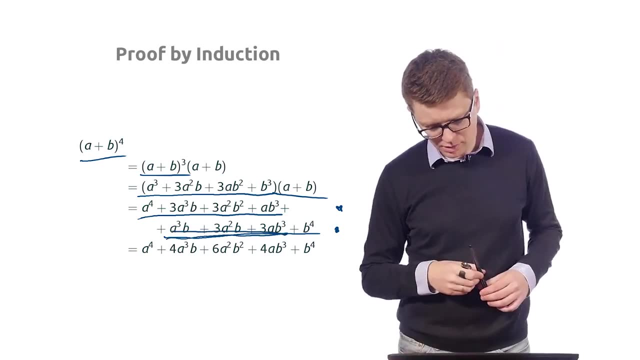 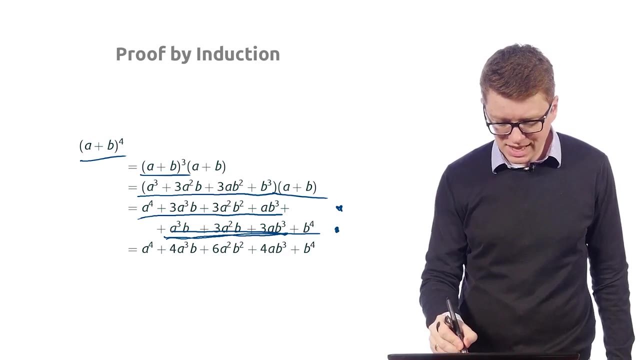 And they are aligned. Now, these two expressions are aligned so that we have these three terms here in the same columns. So, as you see, when you compute the sum of them, this is essentially the same as computing. So this 4 comes as the sum. 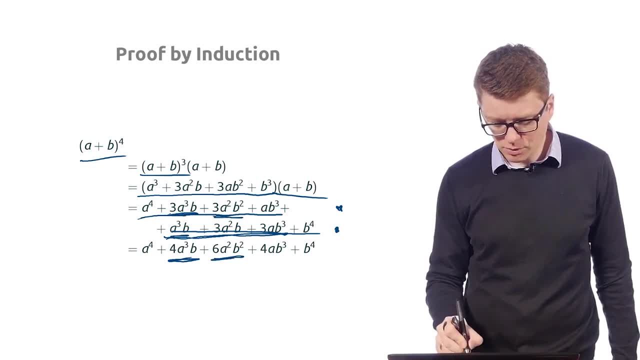 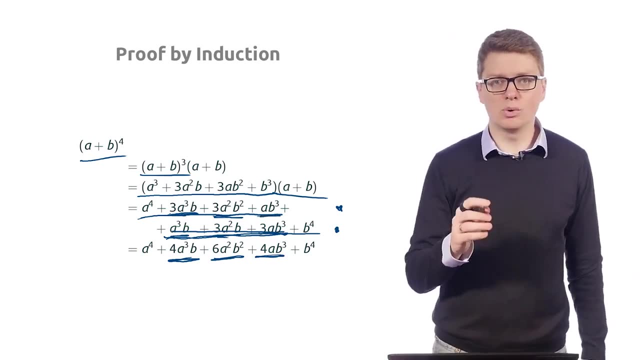 This 4 comes as the sum of 3 and 1.. This 6 comes as the sum of 3 and 3.. And this 4 comes as the sum of 1 and 3.. This is exactly the pattern in our Pascal's triangle. 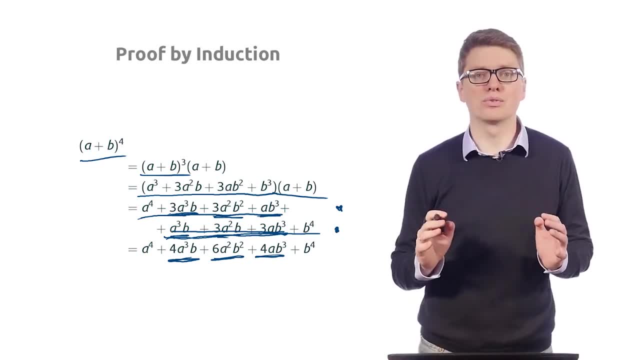 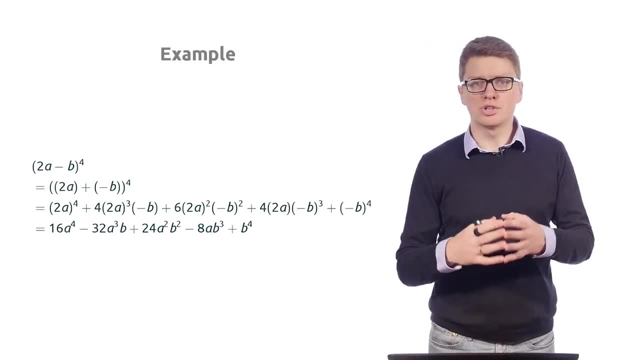 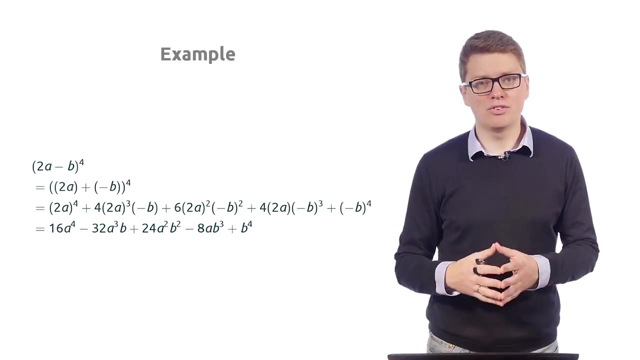 And this is true in general, not only for n equal to 4 and 3,, of course. So this is a way of proving the binomial theorem by induction. Okay, Now let me show you also some slightly more complicated example, just to show you that binomial theorem. 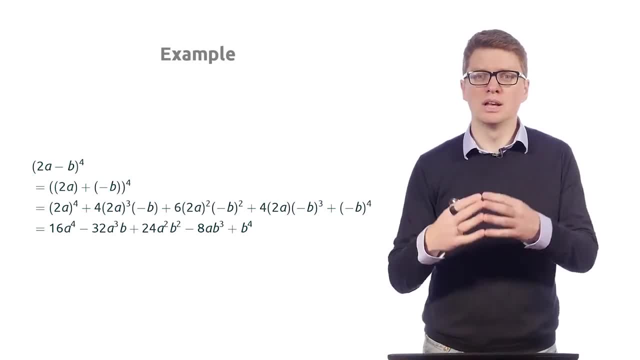 allows us to compute the coefficients of all the binomials, not only for the case when we have just a plus b. Instead, we might want to compute the sum of, I mean the force power of not just a plus b, but something like 2a minus b. 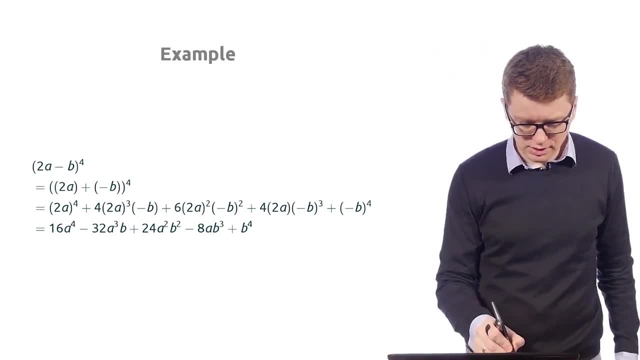 In this case, what remains to be done is just to consider 2a and minus b as our new a and b. So we consider 2a minus b as the sum of 2a and minus b, And then for this: 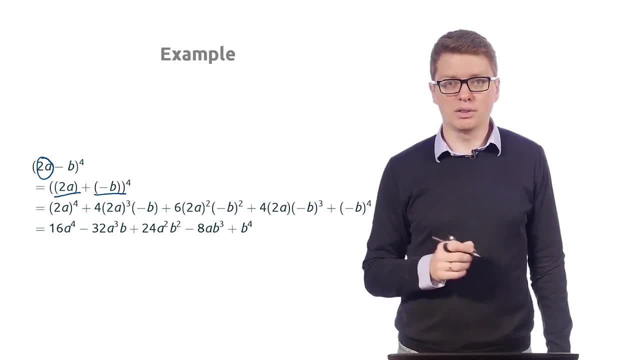 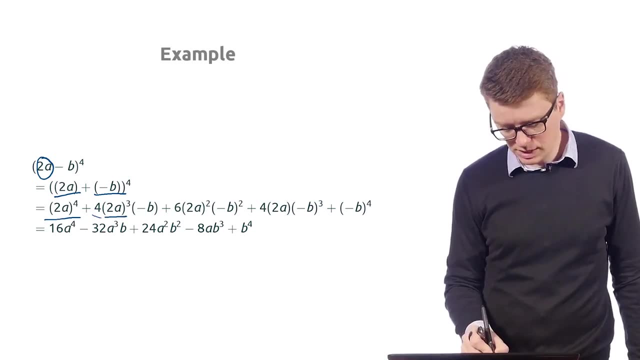 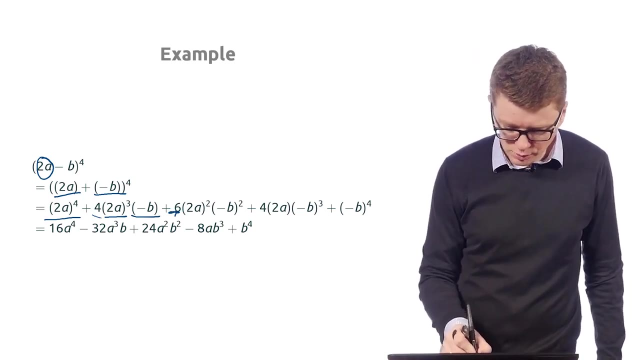 for the sum of these two guys we apply the binomial theory. This gives us 2a to the fourth, then 4 times 2a to the cube, times minus b times our second friend, then 6 times 2a squared times minus b squared, and so on. 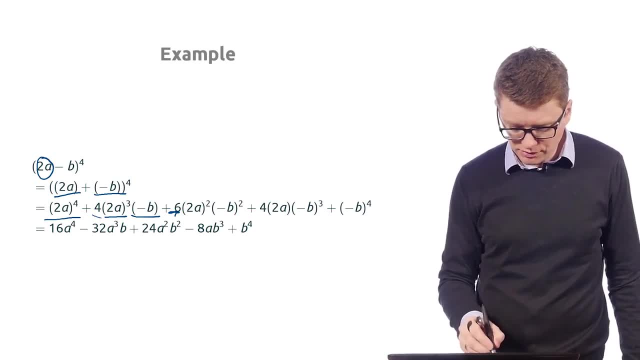 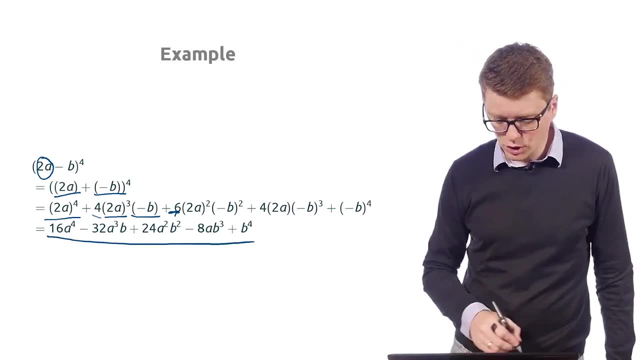 And then you just need to multiply these binomial coefficients with, with powers of 2 coming from 2a, Okay, and this finally gives you the following expression: So, in particular, if you have something like 2a minus b to the seventh, for example, you: 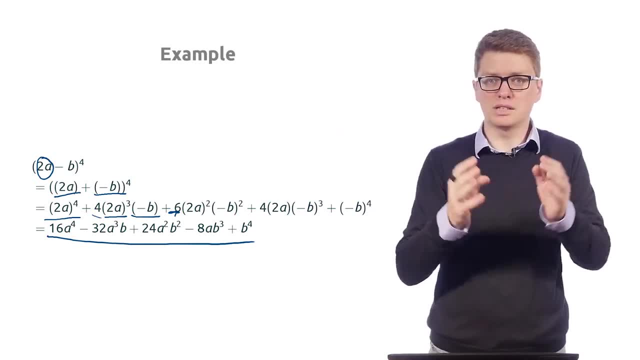 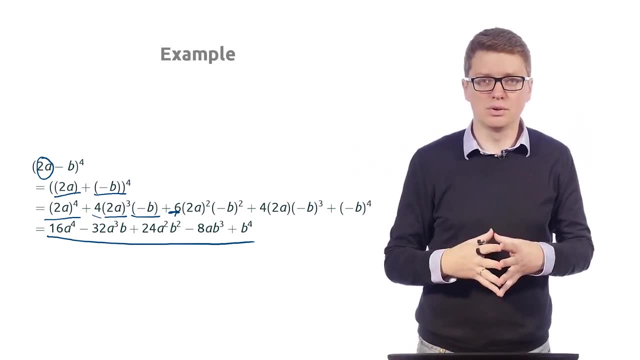 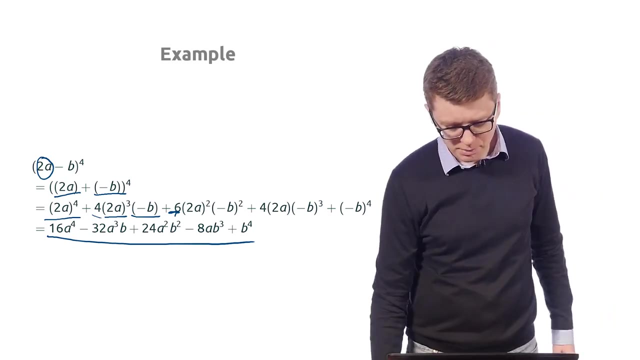 don't need to actually multiply many, many, many terms. You just need to to get the seventh row of Pascal triangle, and this will already give you all the coefficients. All what remains to be done is probably to multiply them with coefficients like 2 if, instead of 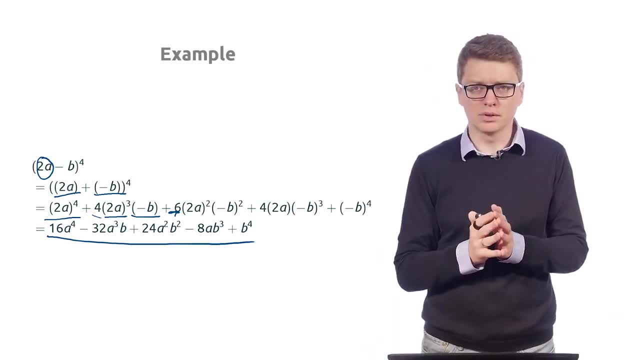 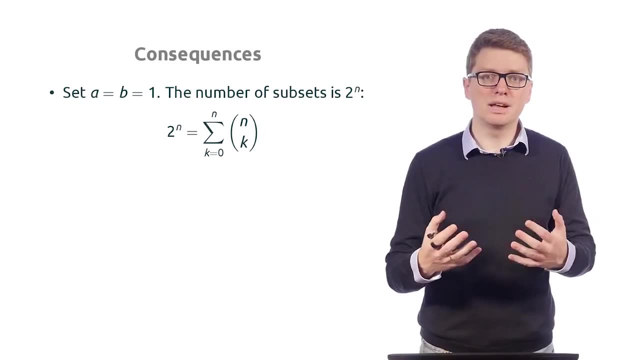 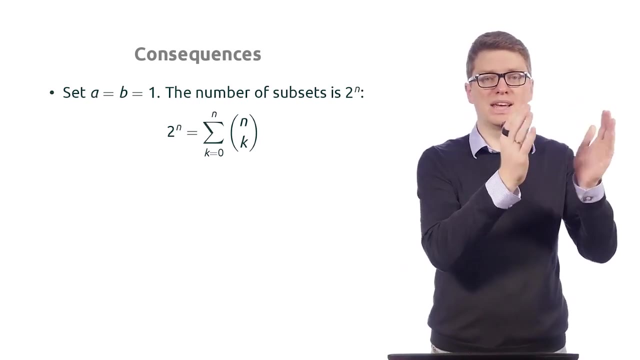 a plus b, you have something like 2a plus b. Okay, now let's also show several interesting consequences of the binomial theory. For example, if we set a and b equal to one, then what we get on the left- so instead of a plus b to the n, what we get is one plus one to the n. 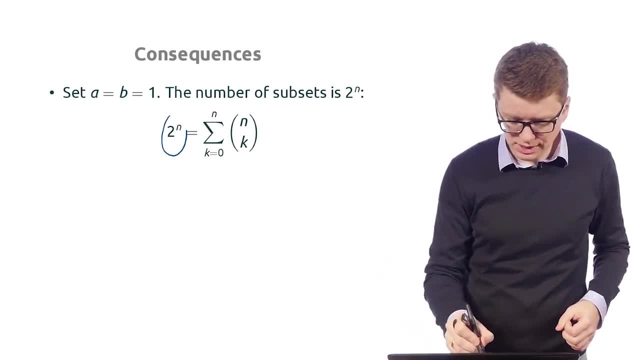 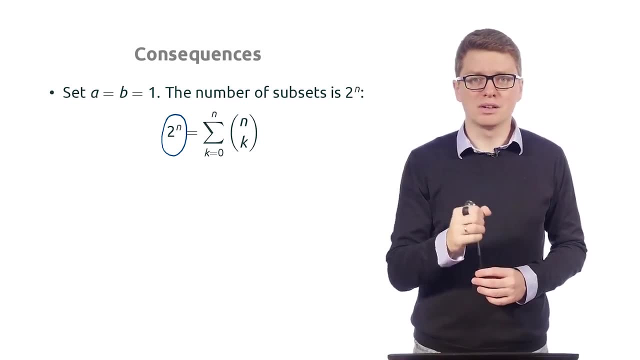 that is just two to the n. Okay, and this is what we get here. On the other hand, a to the k and b to the n minus k is always equal to one, because a and b is equal to one. So, on the right, what we have is: 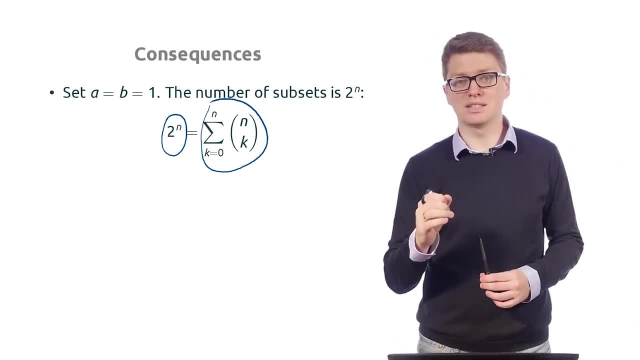 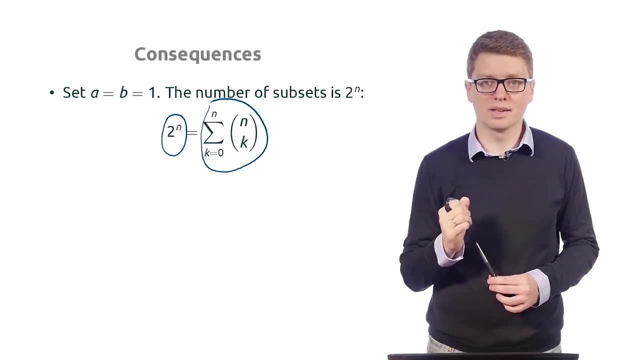 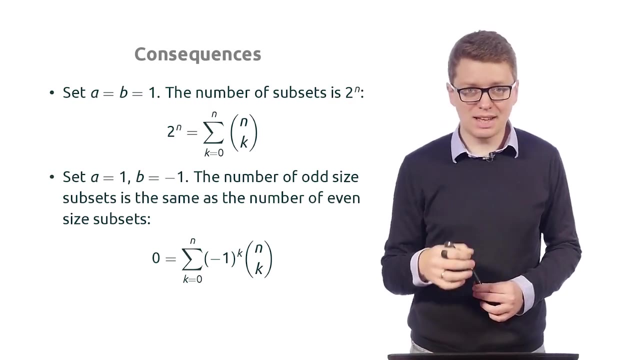 the sum of all binomial coefficients. So this gives us another proof of the fact that the sum of all binomial coefficients is equal to two, to the n. Okay. on the other hand, if we set a equal to one and b equal to minus one, and on the left we have zero, 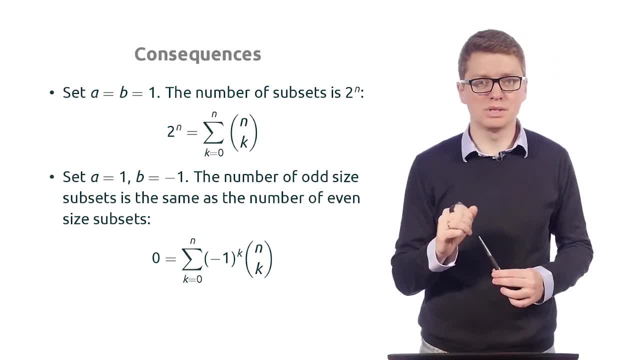 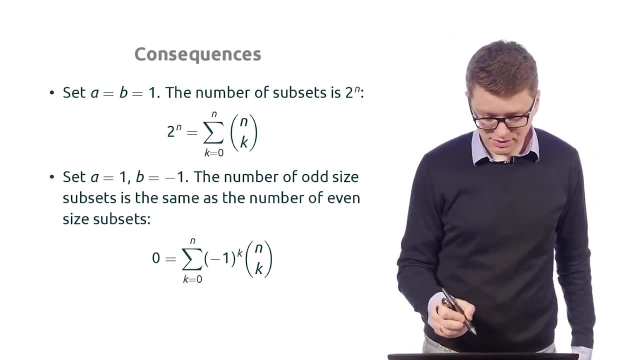 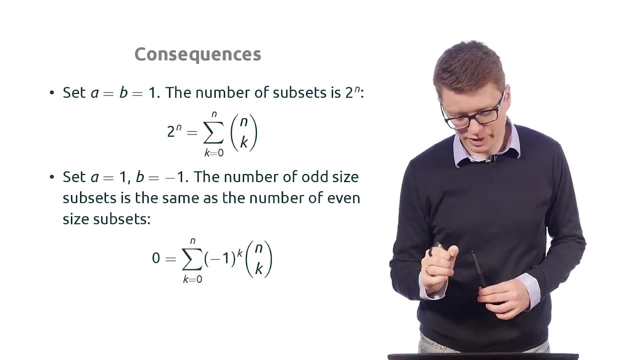 right, because we have one plus minus one to the n. On the other hand, on the right, what we have is just an alternating sum. Okay, so this gives us another proof of the fact that the alternating sum is equal to zero. And let me recall you: 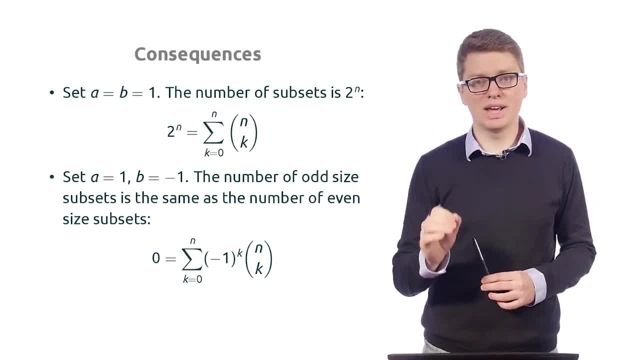 also the combinatorial meaning of that. This means that for any subset, for any n greater than zero, the number of odd size subsets is the same as the number of even size subset And the combinatorial meaning of the previous of the previous equation. 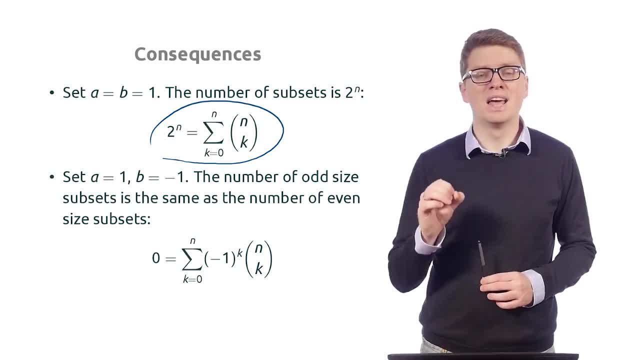 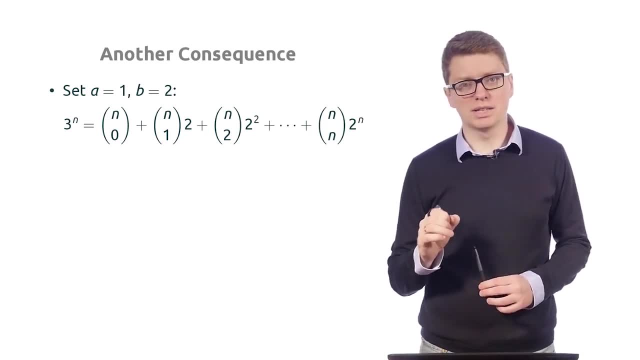 is number of subsets of an n-element set is equal to 2 to the n. Okay, finally, let me show you one more consequence, the one that we haven't seen before. So if we set a equal to 1 and b equal to, 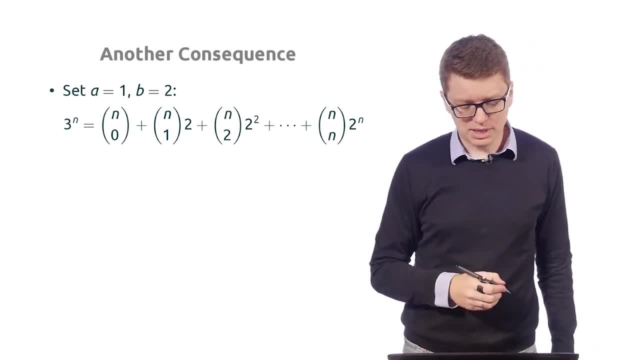 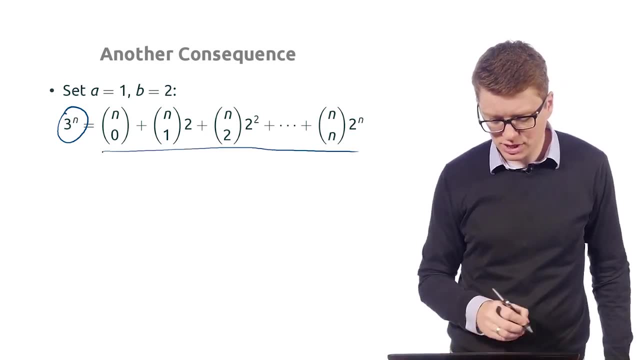 2, then what we get? on the left we have a plus b, which is 3, so 3 to the n, and on the right we have binomial coefficients and each binomial coefficient and choose k is multiplied by 2 to. 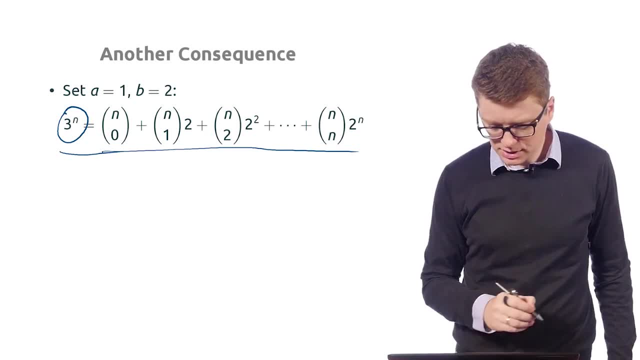 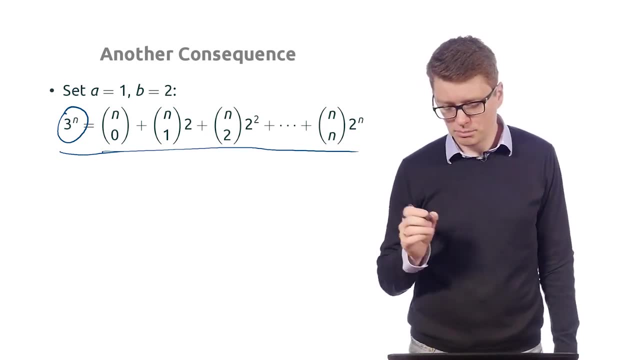 the k. Okay, so we have this nice, nice formula: 3 to the n is equal to n. choose 0 plus n. choose 1 times 2 plus n. choose 2 times 2 squared plus, and so on, and choose n times 2 to the n. So this is: 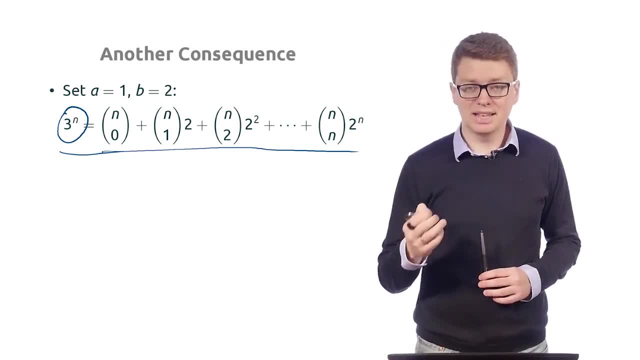 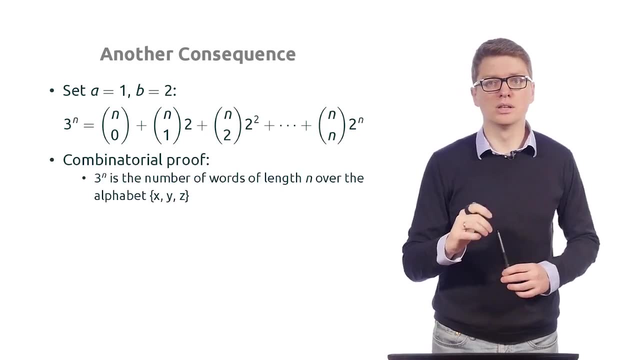 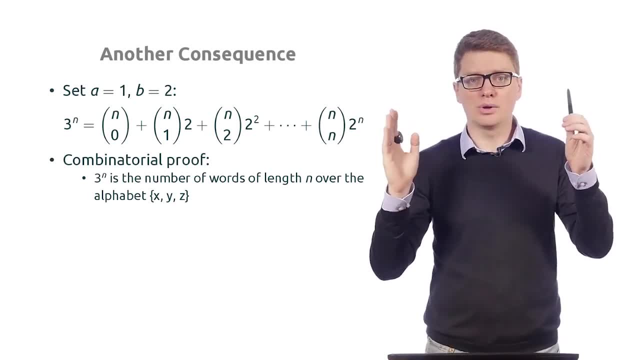 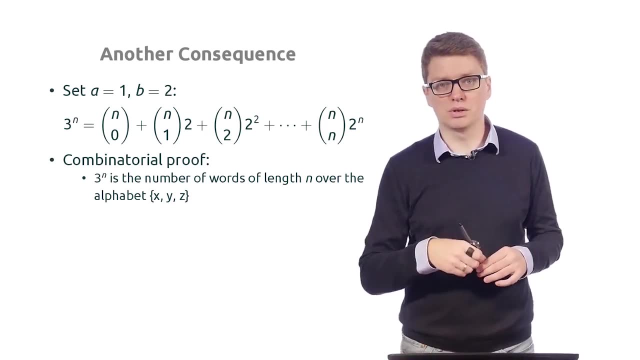 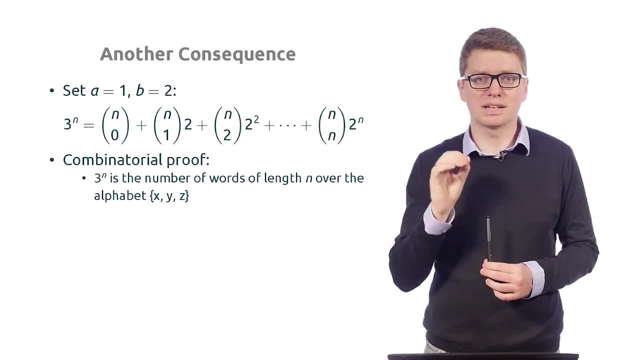 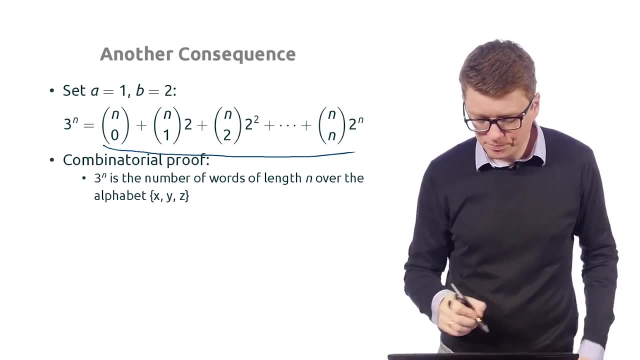 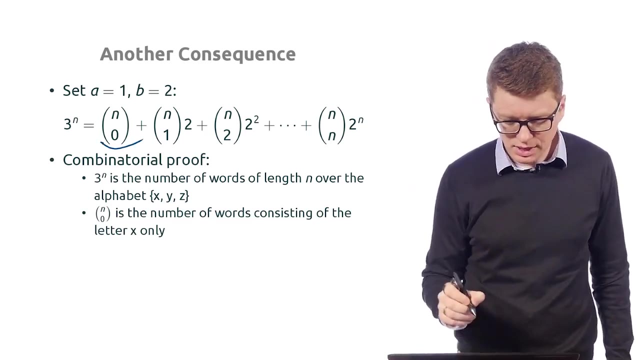 for every of N positions, you have three possibilities: X, Y and Z. So now our goal is to express this number of words as the sum, And this is what we're going to do now. So let's compute it as follows: So N choose, 0 is the set. 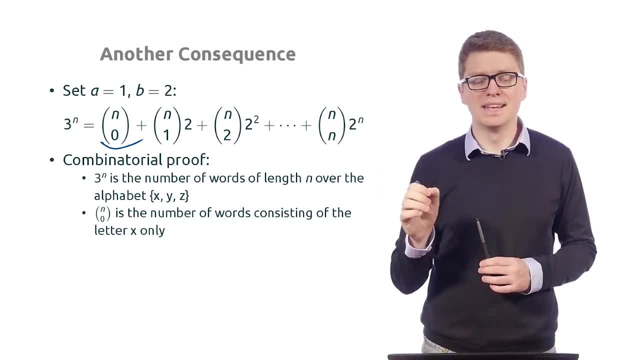 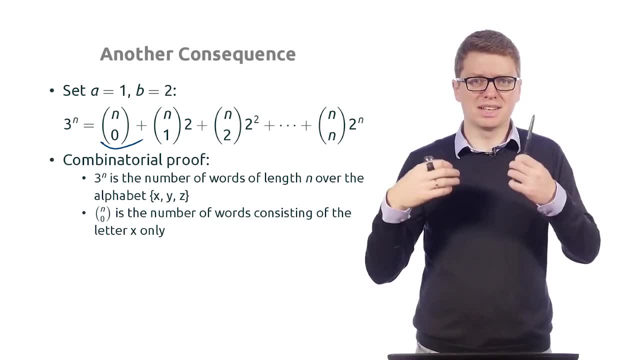 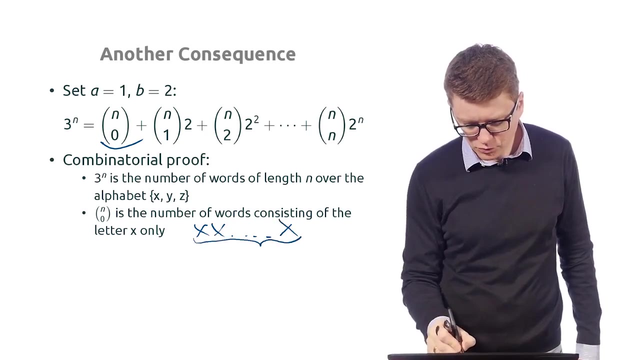 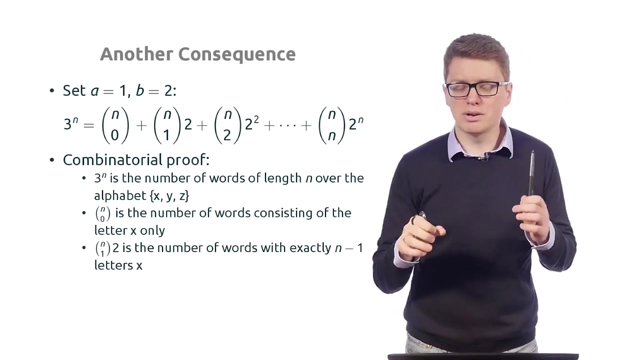 which is the number of all words of length N. that consists only of letter X, So N 0 is exactly the one that when there is exactly one such word, So you just XXX times, Right? Ok, so we justified this. Now what we are going to do of compute next is a number of 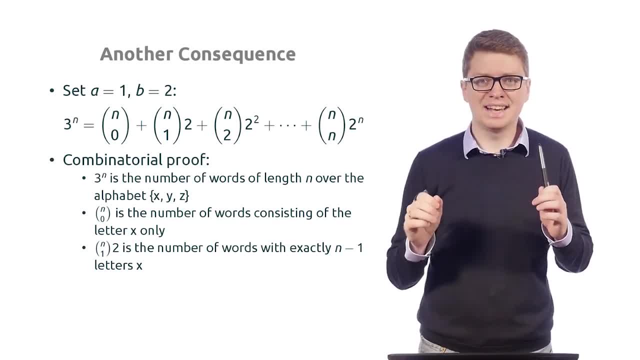 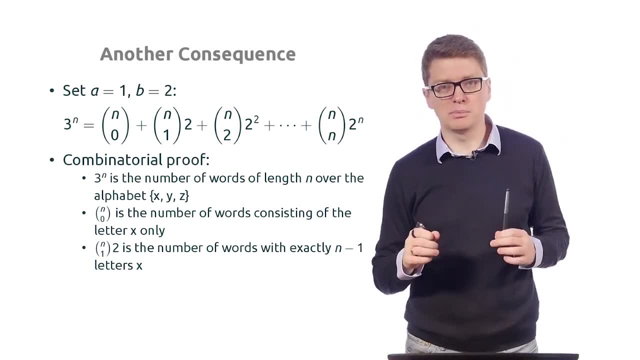 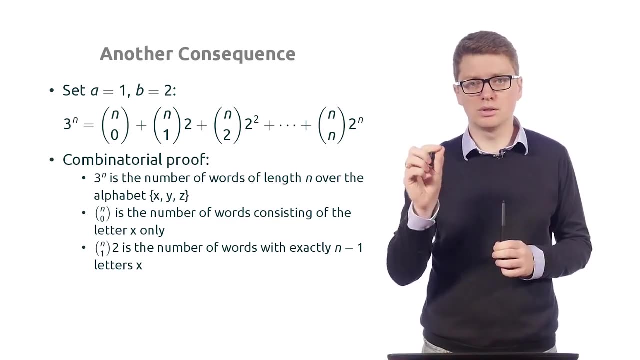 words containing exactly and minus 1 letters X. okay, so how to compute it and why it is equal to n. choose 1 times 2. well, it is equal to this expression because of the following fact: to compose such work, we first need to select exactly one position where X does not. 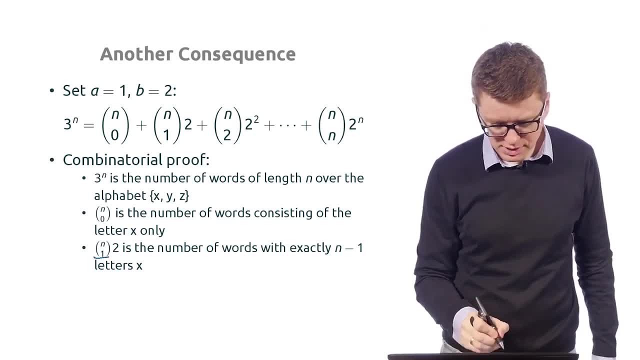 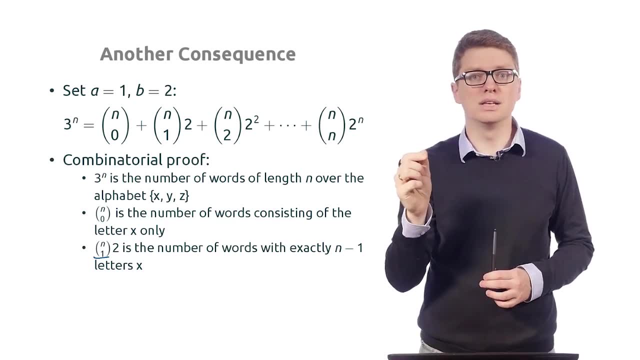 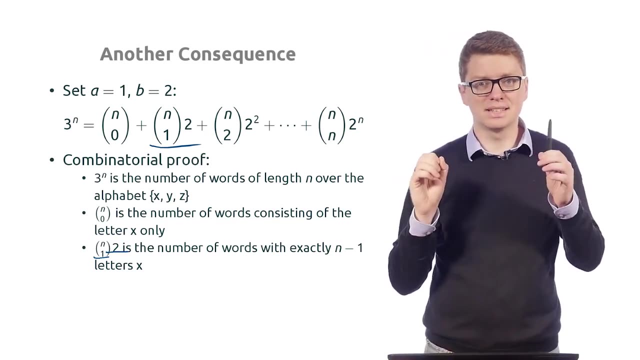 appear. so we can do this in in this many ways and choose one, and then for each, for this position, we need to choose either Y or Z, so we multiply it by 2. okay, so this is once again the number of words of length n that contain exactly n-1 letters X. 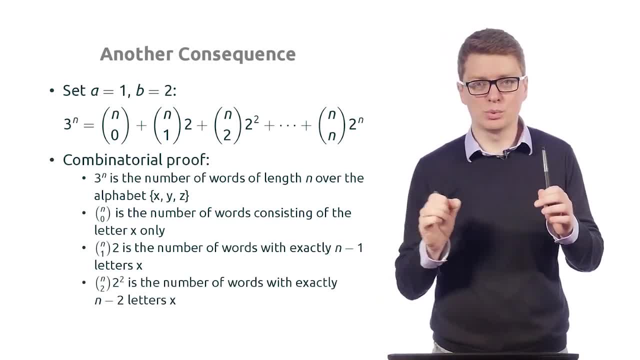 okay, let me finally show you the next one and the pattern will emerge. so this is, as you might guess already, exactly the number of words of length n that contain exactly n-2 letters, X, x. Why is that? Well, again, because to form such a word, we first need to select two places. 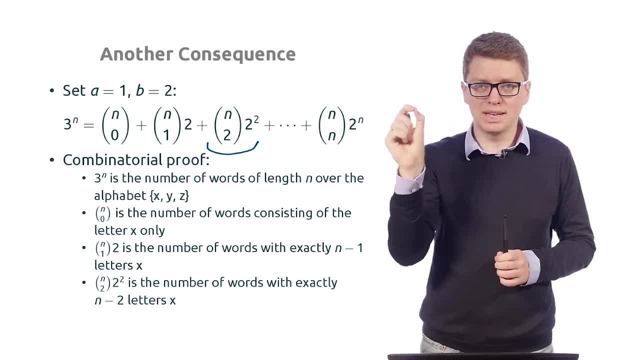 where there is no x, And for each of these two places, we need to select either y or z. So there are, first of all, there are n choose- 2 choices of these two places and then, for each of these two choices, we need to select either y or z. So it is 2, 2 times 2,, okay, And this gives us n choose. 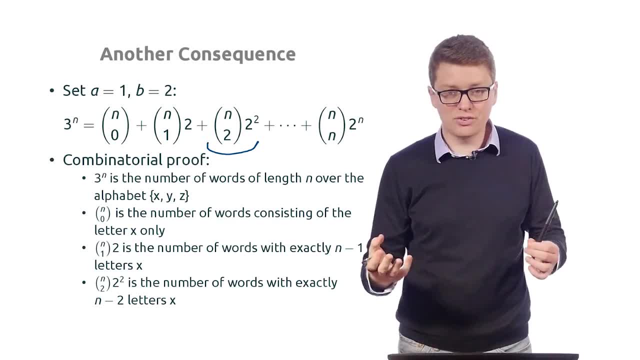 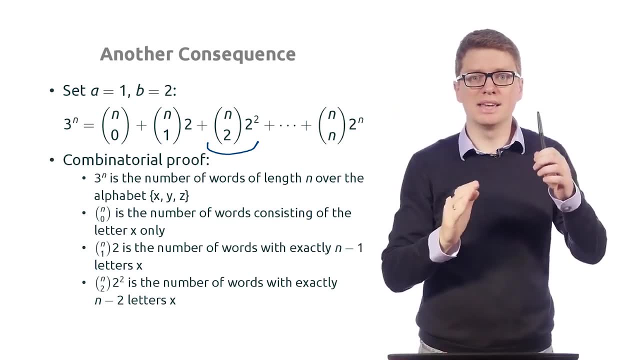 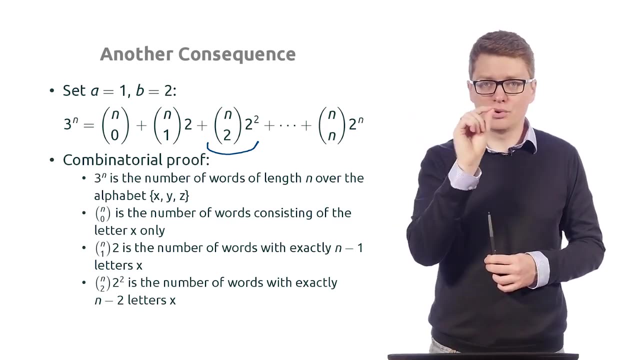 2 times 2 squared, And, in general, if we would like to compute the sum of the number of words that contain exactly n minus k letters x, then we first select k positions where k where x does not appear, And then for each of these k positions, we select either y or z. This gives us n. choose k. 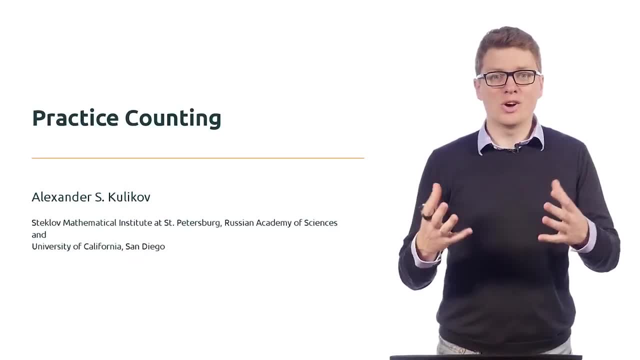 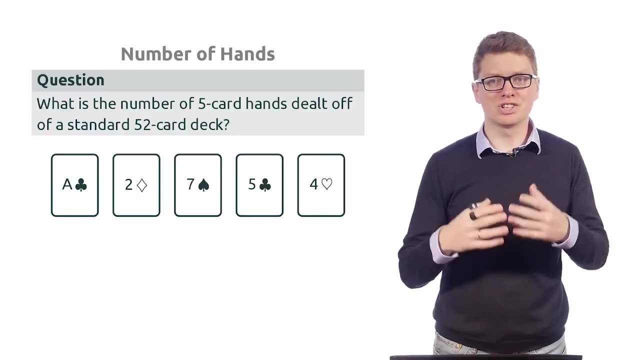 times 2 to the k. Now let's apply what we've just learned to solve the problem of n, choose 2 times 2 squared, And in general, if we would like to compute the sum of several problems. So the first problem is actually easy. So the question is: what is the number of? 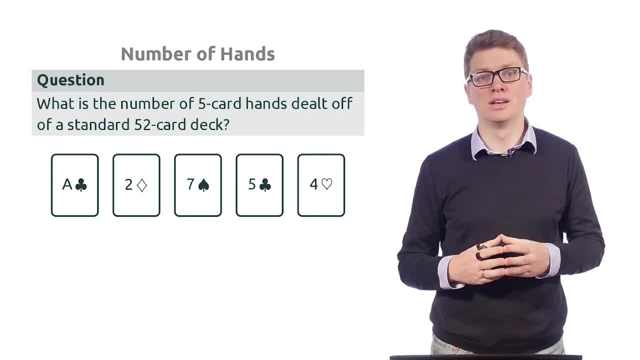 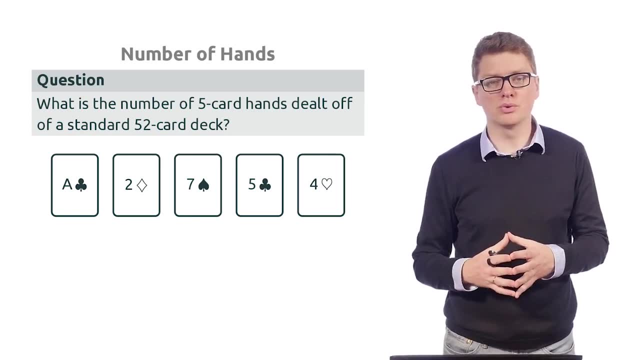 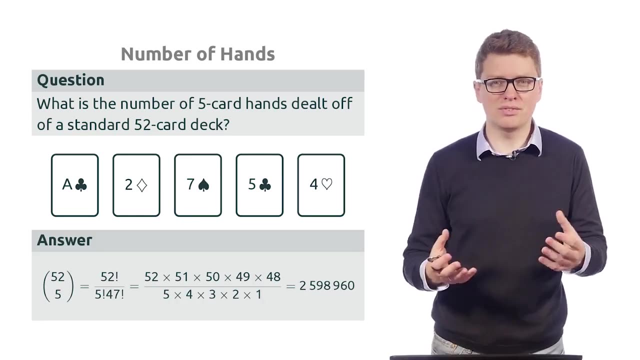 ways of selecting 5 cards out of 52 cards out of a standard deck consisting of 52 cards. So one such combination is shown here on the slide And the question is, of course it is just 52, choose 5, which is roughly 2 and a half million. okay, Now let's slightly. 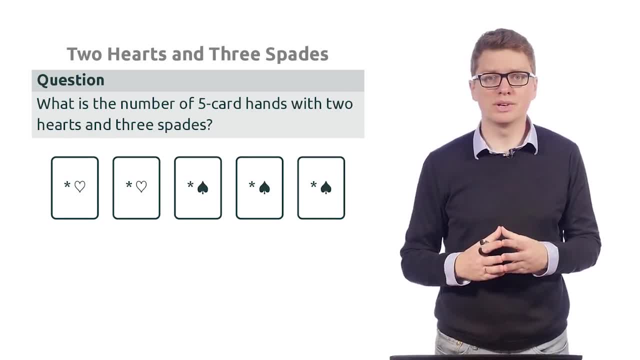 change the problem Now. we are looking for a number of ways of selecting 5 cards such that 2 of them are hearts and 3 of them are spades. okay, Now we see that we can arrange our 5 cards. 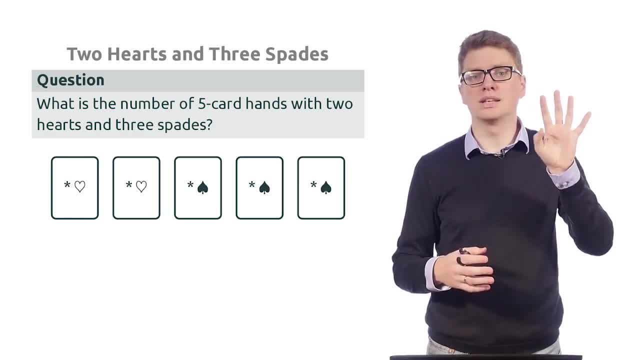 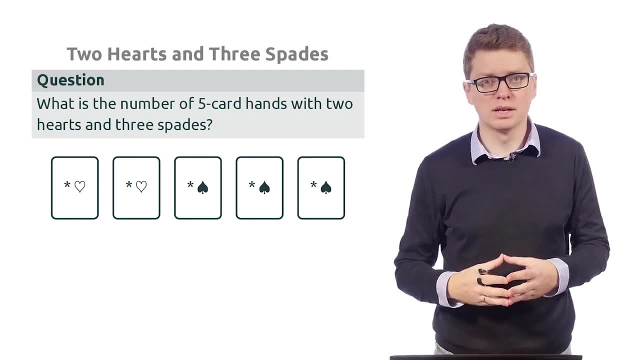 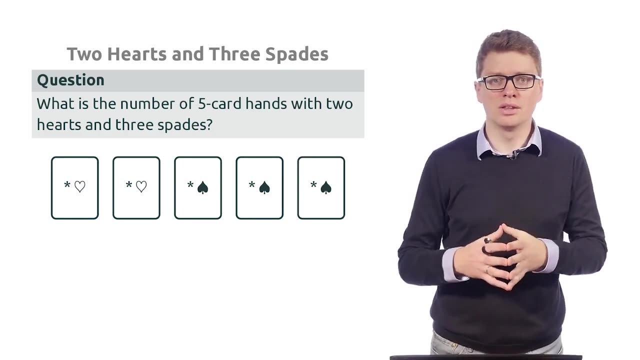 as follows, such that first we have 2 hearts and then we have 3 spades. okay, Then, to count such number of ways, we actually need to realize that we have a number of ways of selecting 5 cards. So for the first 2 cards, for each of the first 2 cards, there are 13 possibilities, all 13 hearts. 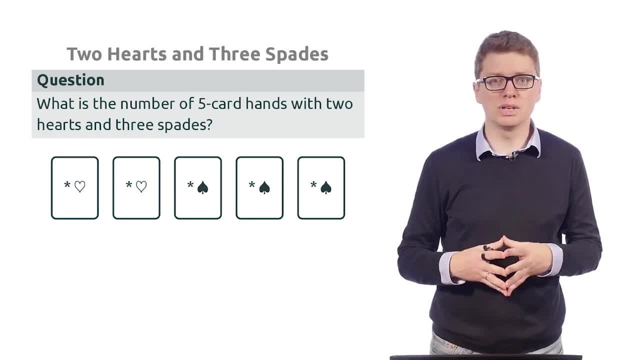 cards, right So? and among these 13 cards, we need to select 2.. And the same for spades: We need to select 3 spades from 13 possibilities. So by the product rule, the answer is just 13: choose 2 times. 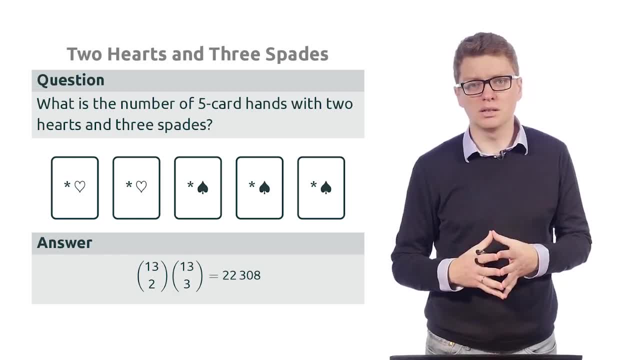 13, choose 3,, which is roughly 22.5.. So we have a number of ways of selecting 5 cards. So let's stomach it and begin to see what happens now. So we will go back to the storage就是. 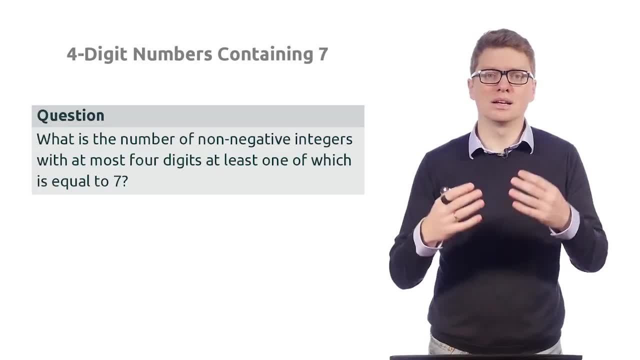 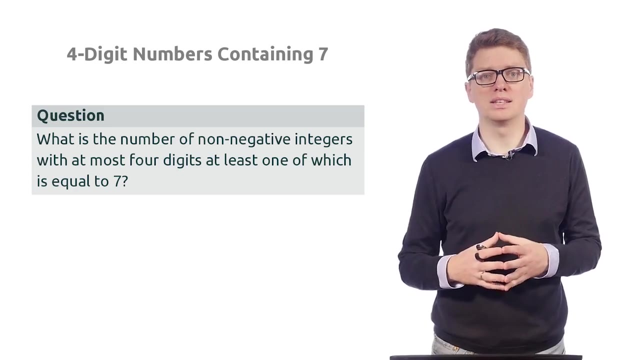 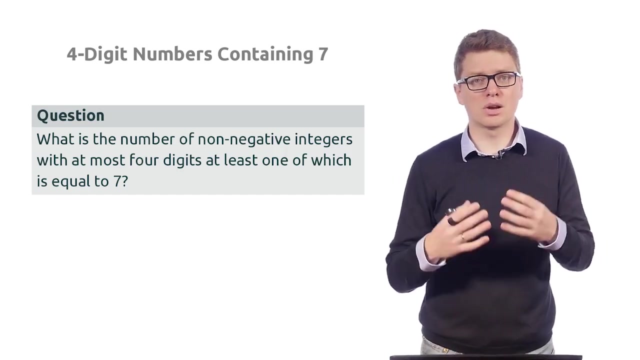 do another half second. this time we will go back to the storage. Now, when we are on a storage like this one, there is slice and we can set spoon class counting which meaning itemWhat一定要. we assume that it will like this sizehat of the same size as a word and this one. means 5, and we also need two. count these three times these, okay. So the next problem is about numbers. In this case we are interested in digit pie- am sorry, nonnegative integers with it, most 4 digits, such that at least 1 of their digit is equal to 7.So in this case, 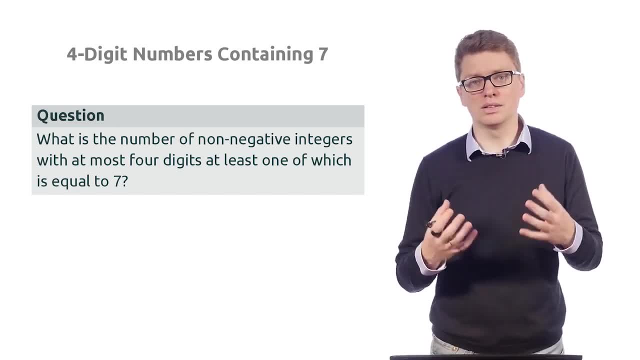 it turns out that it is easier to compute the compliment of what we need to compute, namely, let's compute a less than or add initially. 1 of them are hearts, which is the number of integers, of non-negative integers, with at most 4 digits that do not contain 7 as a digit. 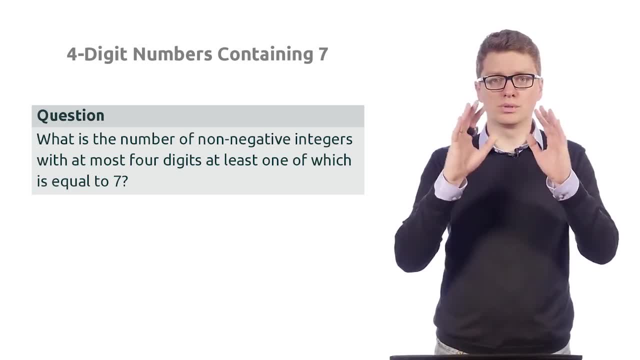 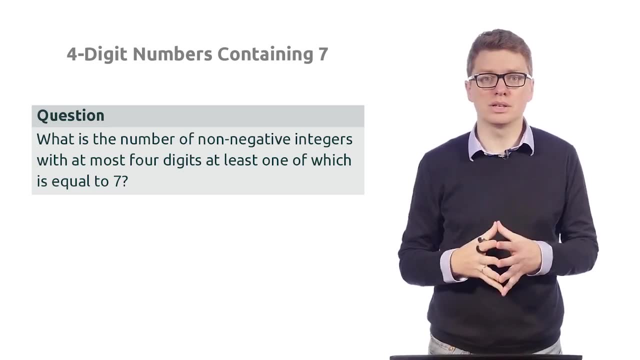 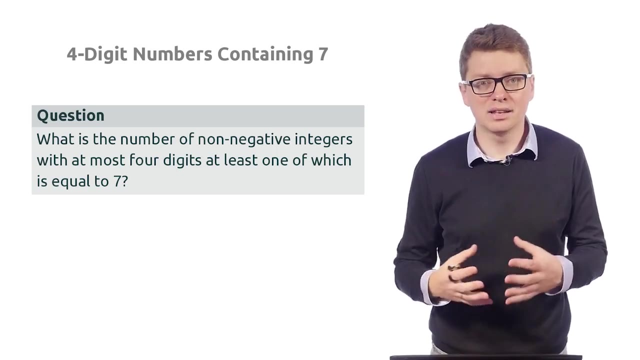 It is not difficult to compute. So there are 4 digits and for each of 4 possibilities we have just 9 choices. I mean all the 10 digits except for 7, which means that there are 9 to the 4 such possibilities. 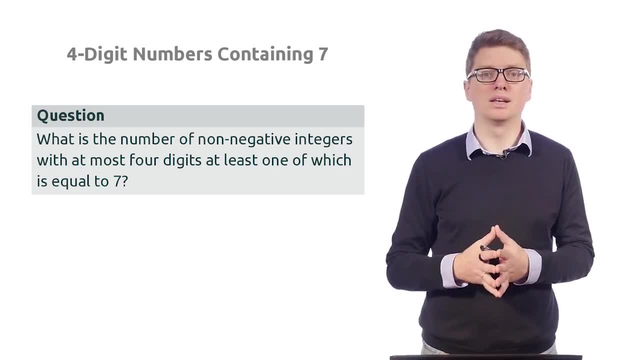 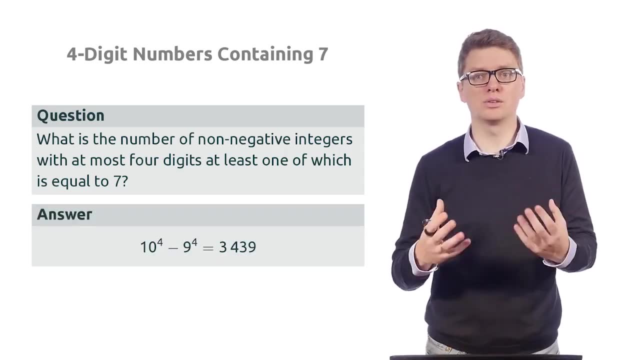 And the total number of 4-digit numbers- at most 4-digit numbers- is 10 to the 4,, which means that we need to subtract 9 to the 4 from 10 to the 4, which gives us something like 3000 and roughly half. 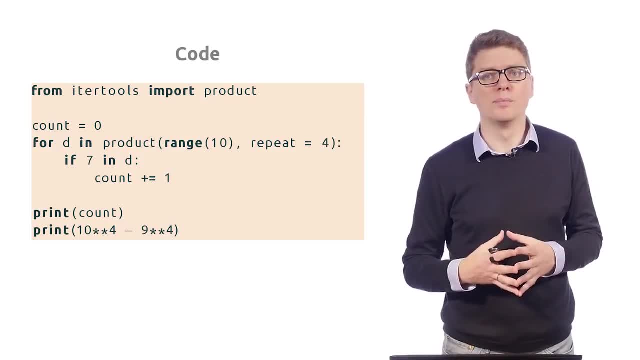 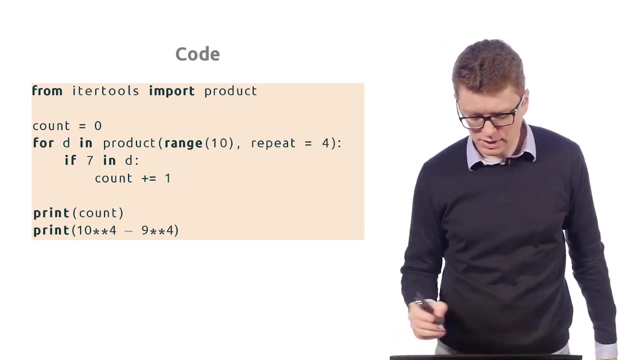 And we can double check this using a simple for loop in Python. So let's just consider all possible tuples of 4 digits and for each such tuple we check whether 7 is present in this tuple or not. If yes, we just increase our results in count by 1.. 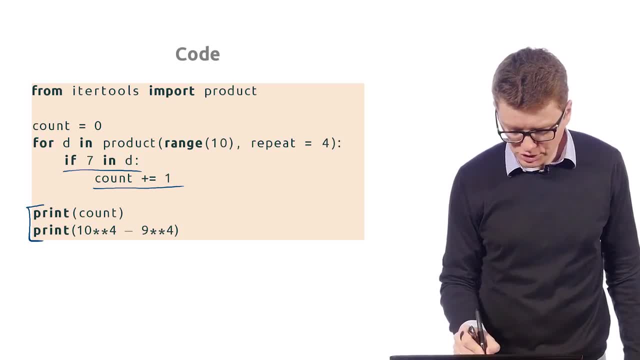 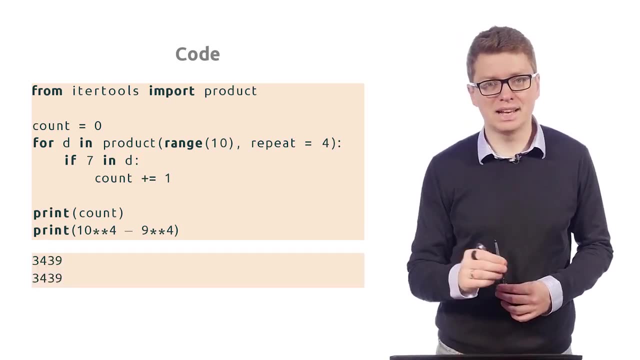 So in the end we print count and to double check, we print also the value of 10 to the 4 minus 9 to the 4.. So, as we see, this is exactly the same. So, as we see, this is exactly the same. 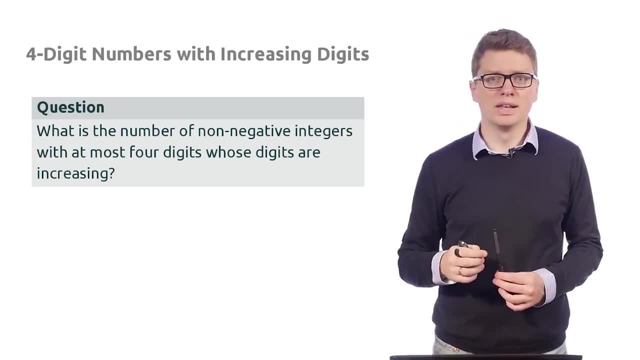 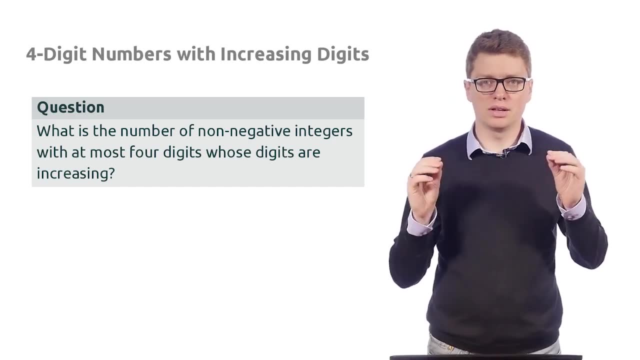 So, as we see, this is exactly the same, The same number. OK, So the next one is the following, also typical problem: We would like to compute the number of non-negative integers with at most 4 digits, such that the digits are strictly increasing. 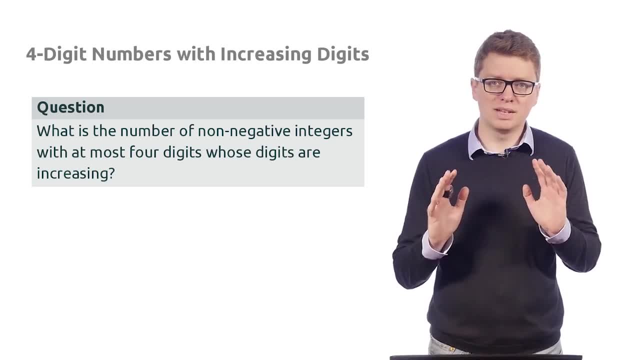 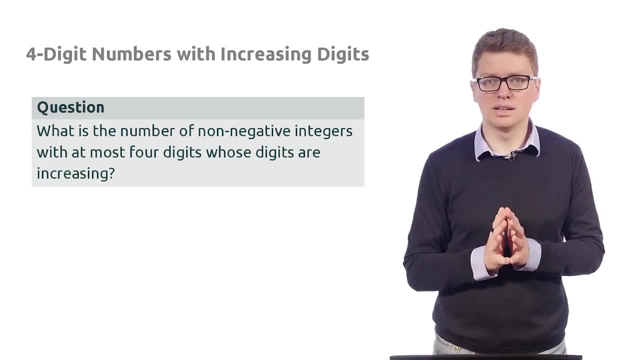 OK, So this is probably a slightly more complicated example. So in this case we need to realize that first, all the digits in our problem, in our all the four digits in our number are actually different. okay, but this in turn means that our goal is just to select four different digits out of ten. 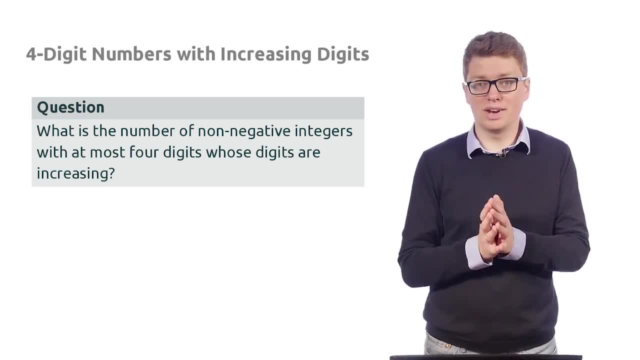 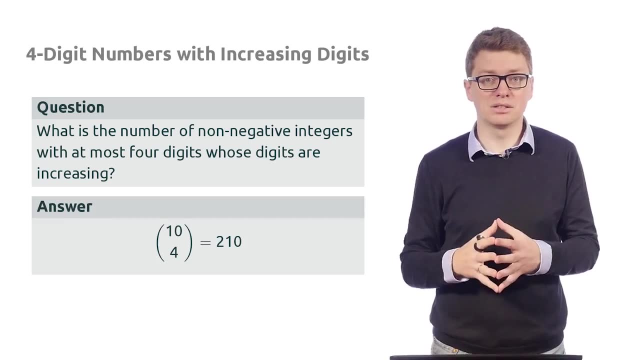 possible digits, and then what we need to do is to arrange them in increasing order. right, but this in turn means that the answer is nothing else as to is to choose four is ten, choose four, I'm sorry, which is equal to 210. once again, let's double check this. let's implement the following simple procedure, so it 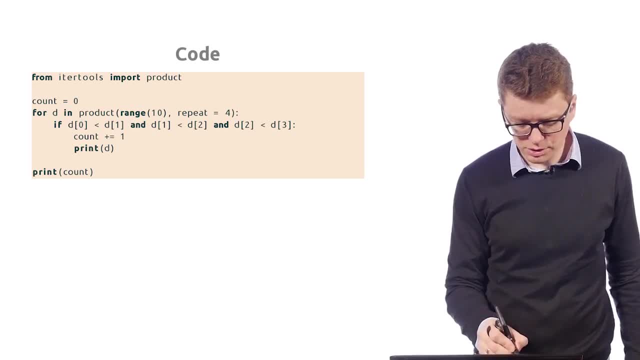 just ranges through all possible couples of four, of four digits, so through all possible four, and all the possibilities are digits from nine to ten. then if the first, if the zero digit is smaller than the first one, the first digit is smaller than the second digit is smaller than the first one. 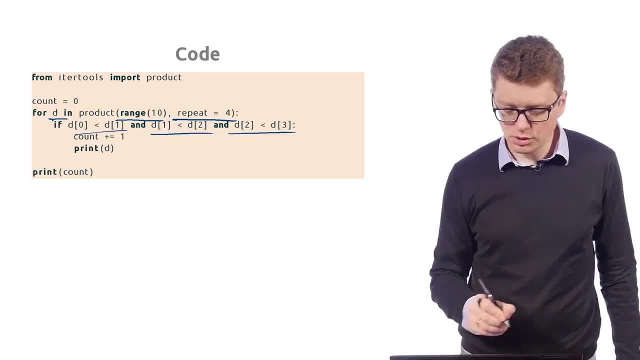 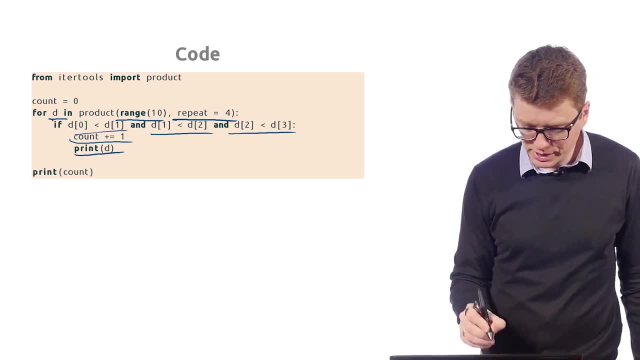 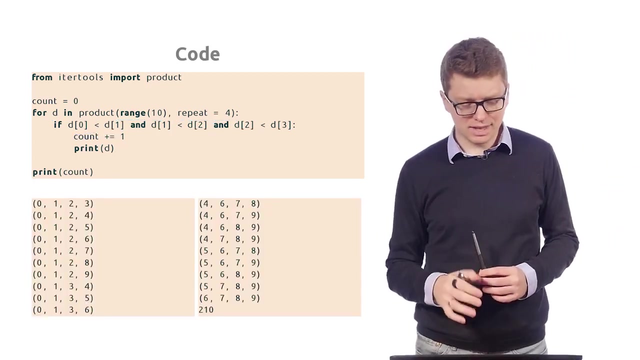 is smaller than the second one, and this and the second one is smaller than the third one, meaning that the digits are indeed increasing. then we increase the count and also we print the resulting number. in the end we print the count. okay, so then if we, if we run this program, then it will start printing. 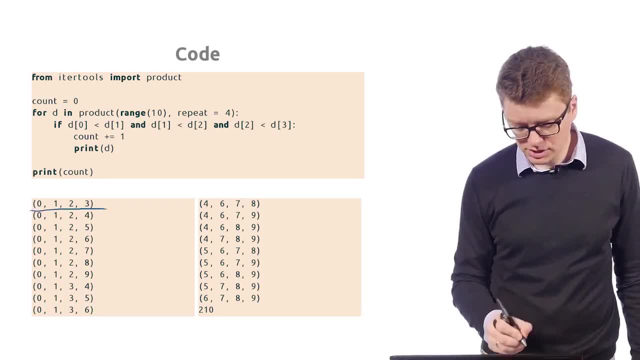 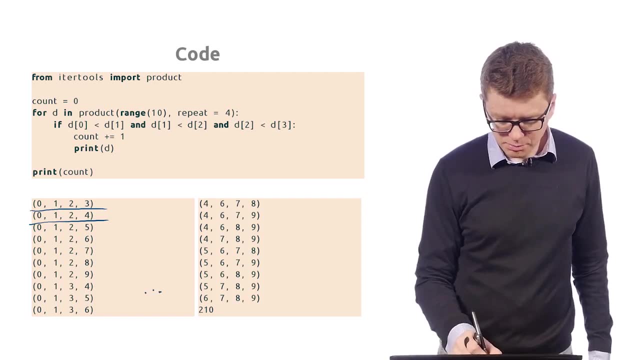 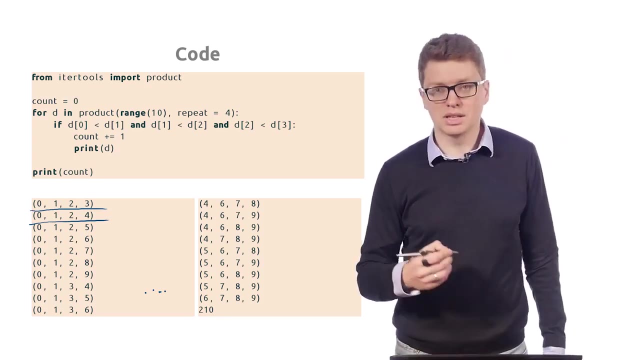 numbers like zero, one, two, three- I mean, these are just digits and not numbers- then zero, one, two, four and so on. so something is missing here in the middle of this list. and then the end of this list looks as follows: six, seven, eight, nine, which is kind of the the largest, uh. 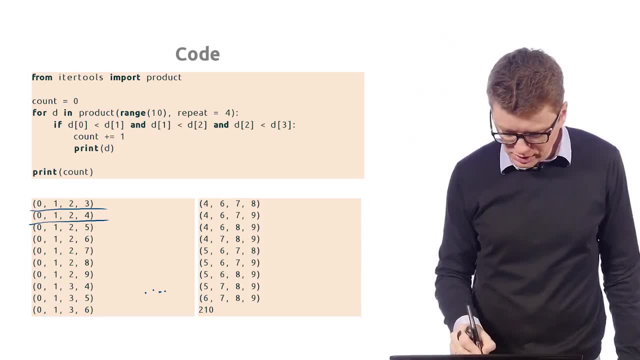 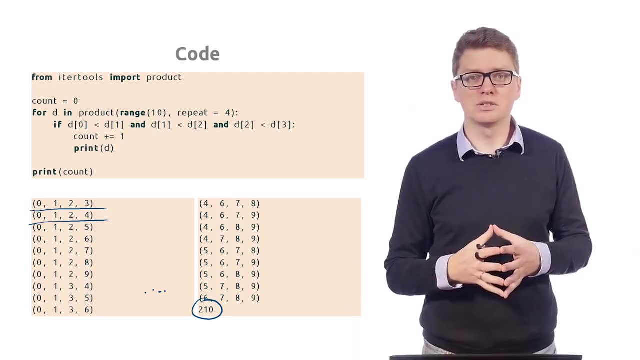 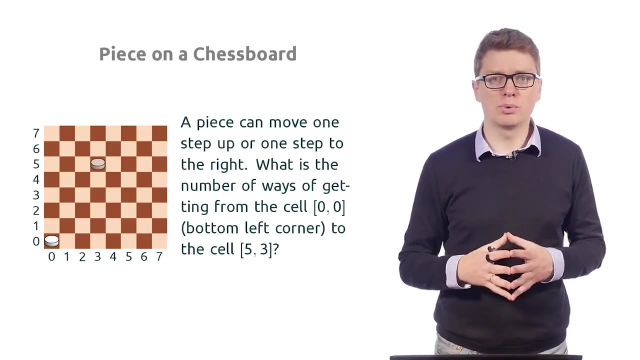 the largest, uh four digit number with increasing digit, and in the end we also print the count, which is indeed uh 210, which is nothing else. once again, as two, as ten, choose four. okay, finally, let's revisit the following problem. so we are given a board for 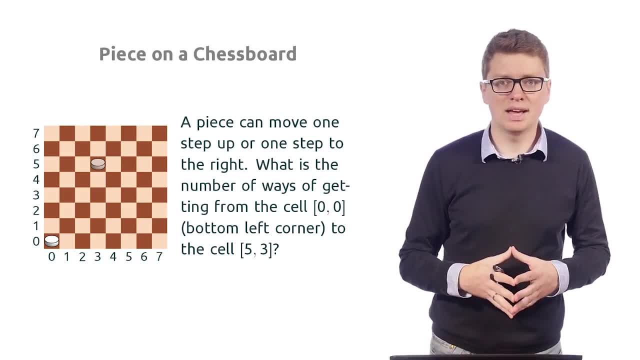 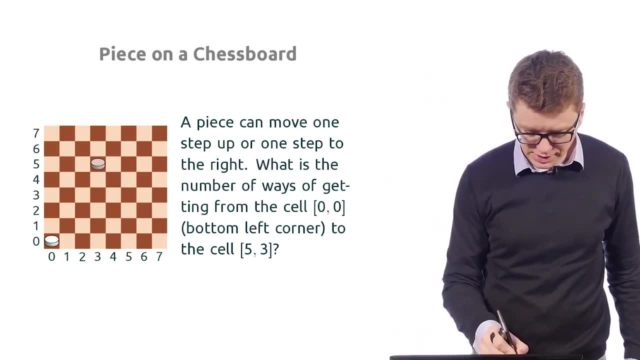 example, an eight by eight. uh, just work, and we have a piece uh whose initial position is at the cell zero, zero, and what we would like to do is to count the number of ways uh to get, for example, to the cell five, three, to the cell whose row is fifth one and whose column is the third one. so, uh, we 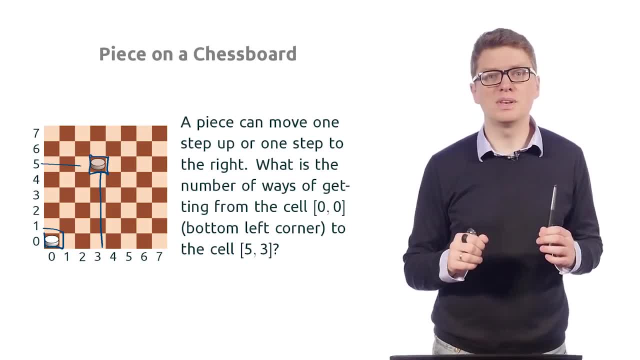 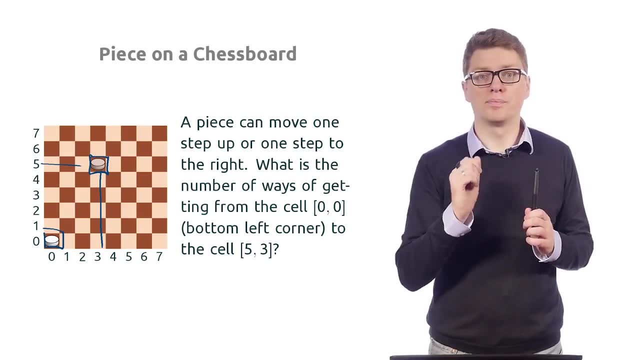 would like to count this number of of ways, assuming that, in a single move, uh, this piece moves either to the right or or moves up. okay, so, first of all, it is clear that, uh, the number of moves should be exactly eight, I mean in any possible movement from from this: 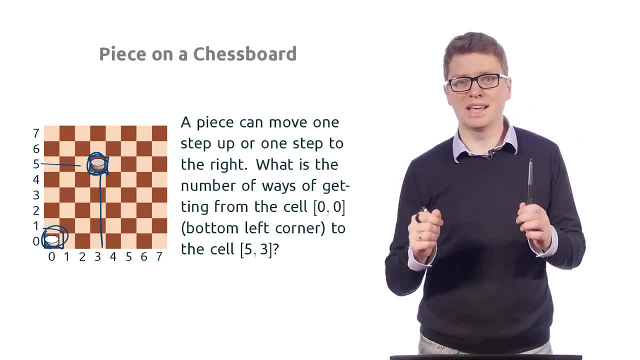 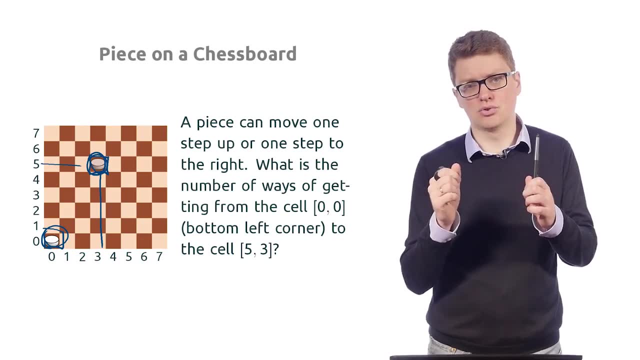 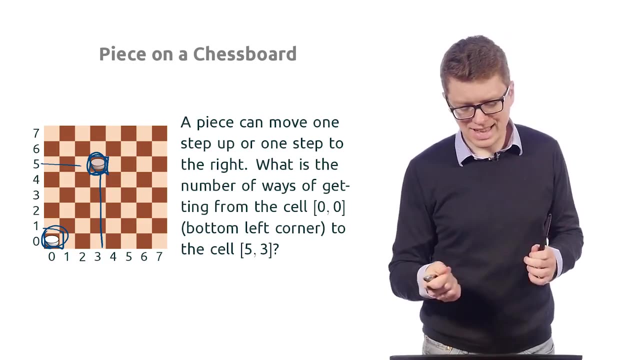 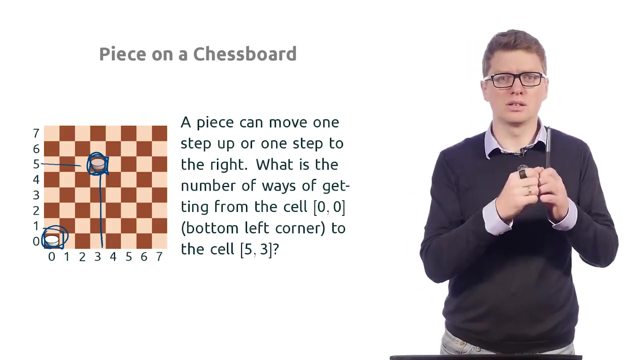 position. to that position, the piece should make exactly eight moves. why is that? well, just because each time we either increase uh, the the row number, or we increase the column number. initially, the row number and the column number is equal to zero, and in the end, the row number is equal to five, uh, and the column number is equal to three. so, at each with each. 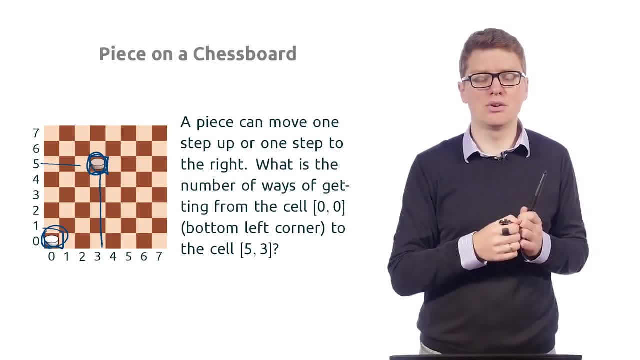 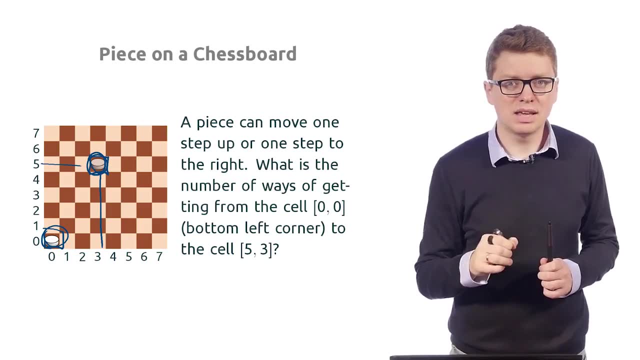 move, the sum is increased by exactly one. initially it is zero, in the end it is eight. so the number of moves must be equal to eight, and this gives us a hint. so we need to make eight moves. on the other hand, we know for sure that the number of moves to 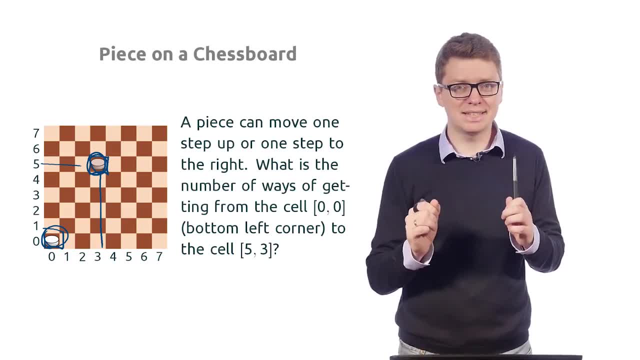 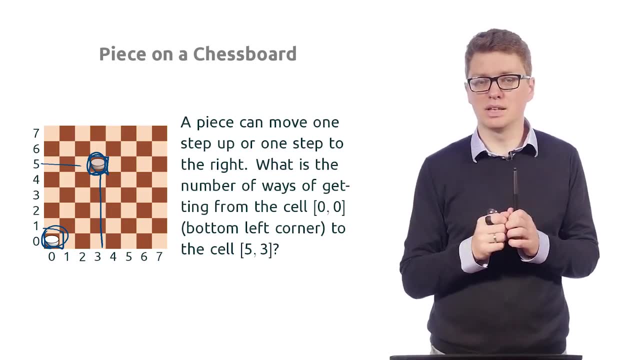 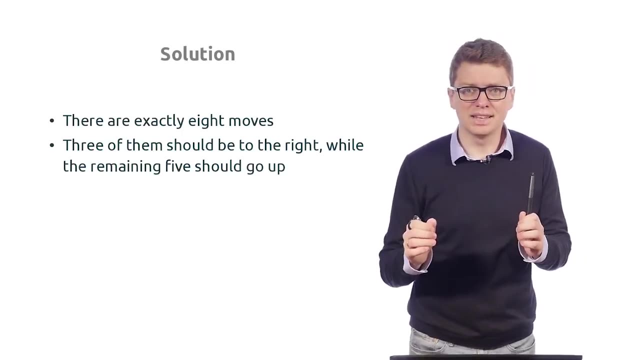 the right should be exactly three. if we make less than three moves to the right, then we will not be able to reach the third column. if we make more than three moves to the right, then we will not be able to return back to the third column. this is, on one hand, okay. on the other hand, if you consider, 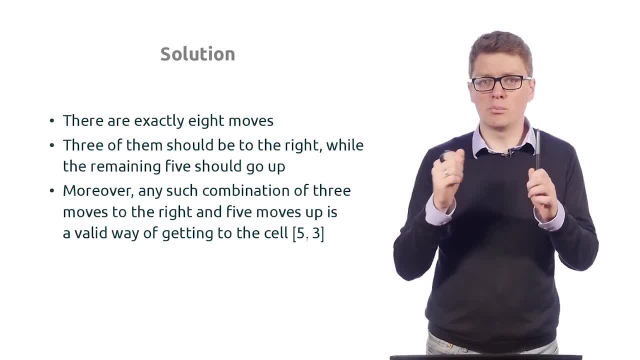 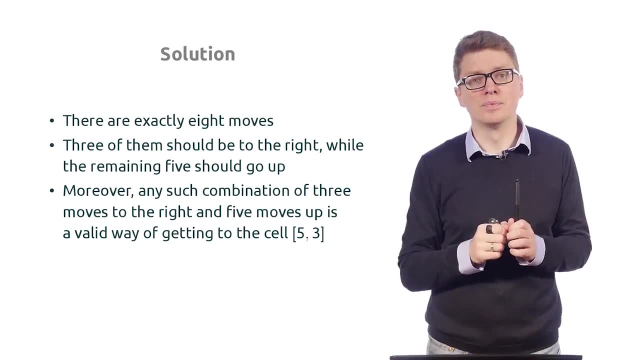 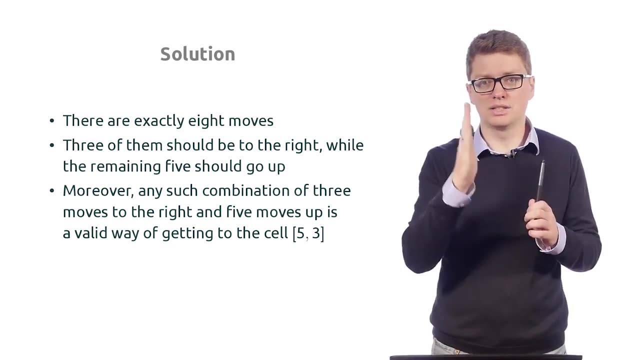 any such combination of eight moves, such that among these eight moves there are exactly three moves to the right, then we reach the position five, three. well, why is that? just because if there are exactly three moves to the right, this means that after this we are at the third column for sure. and since there are exactly three moves to the right, all the 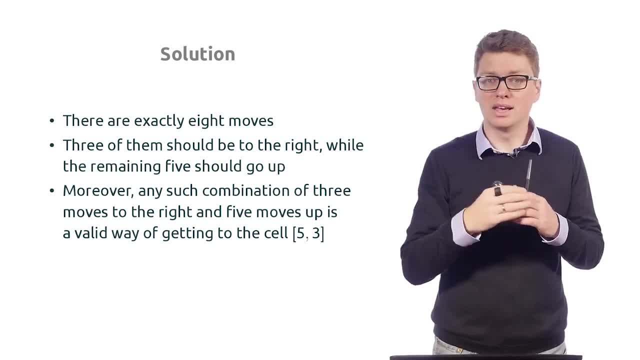 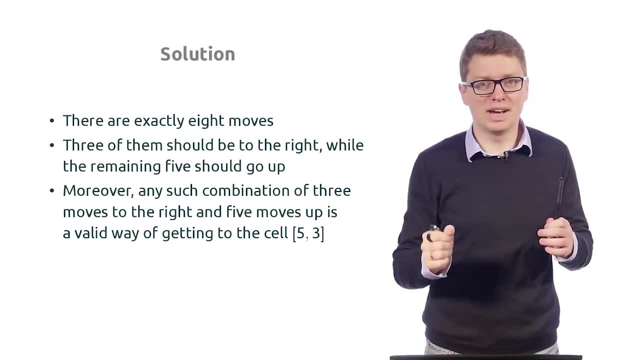 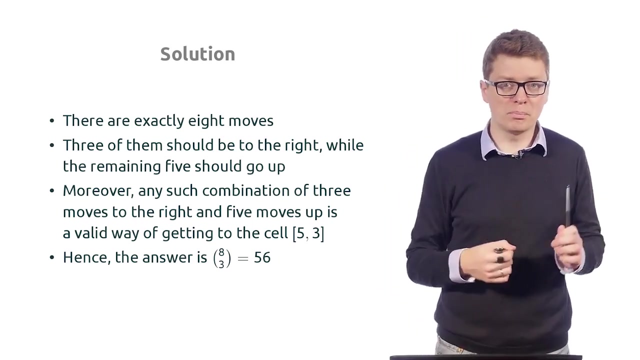 other moves are to the uh, uh, uh, going up, okay, and this in fact means that we we end up in the fifth, uh, in the fifth row, so exactly in our final position, and this all allows us to conclude that the number of such possibilities is eight. choose three, which is nothing else as 56.. well, it is also interesting to note that we could also: 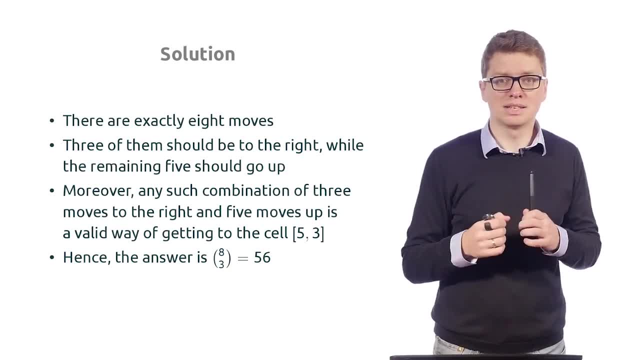 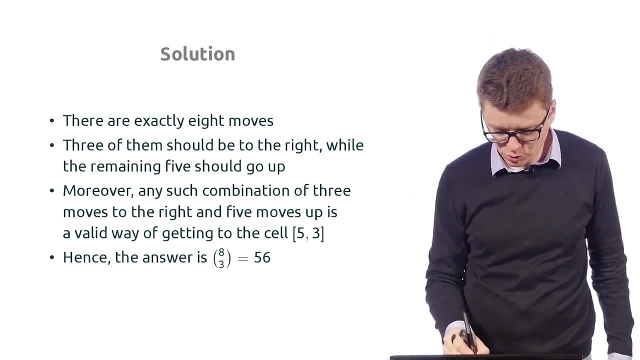 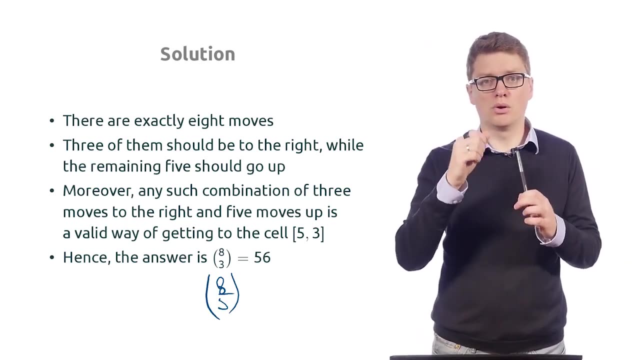 compute this number as the number of ways of selecting moves up. five moves up among eight possible moves. this will give us another solution, which is eight choose five. okay, so this is the same as selecting five moves up among all eight moves. at the same time, eight choose five is equal. 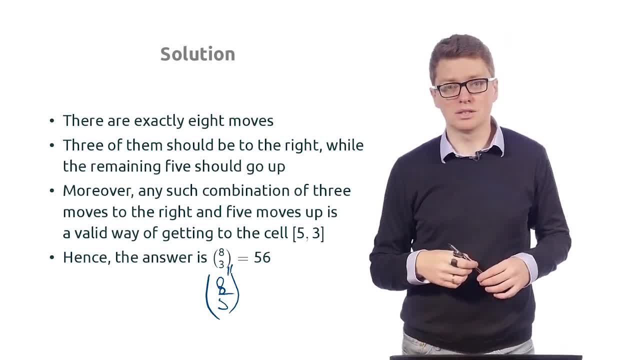 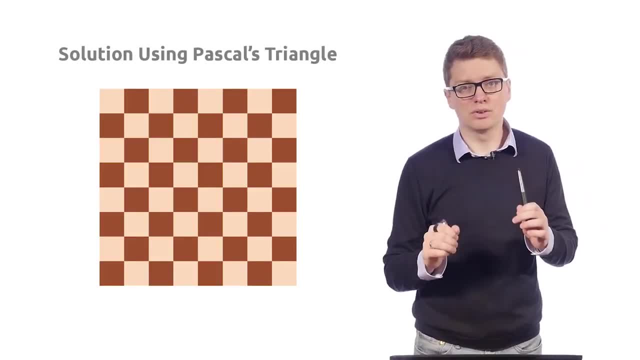 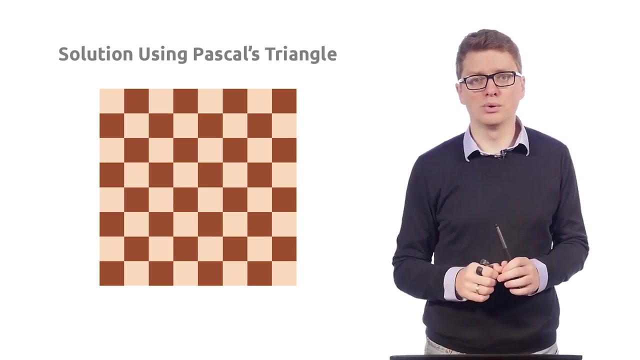 to eight, choose three, as we know already. right, this is a property of this binomial coefficients. finally, let me also show you that the same result can be achieved by uh, by drawing an analogy to the Pascal's triangle. okay, so now let's do the following: for every cell in our board, we are going to to compute the number. 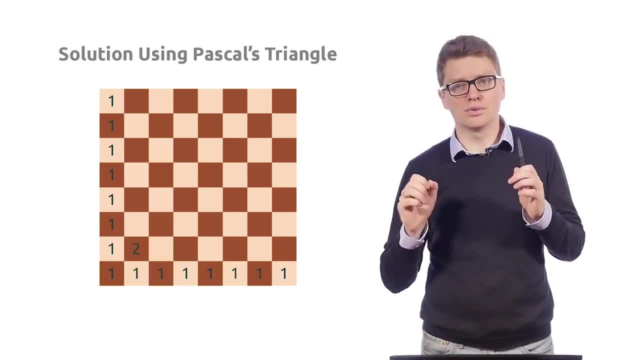 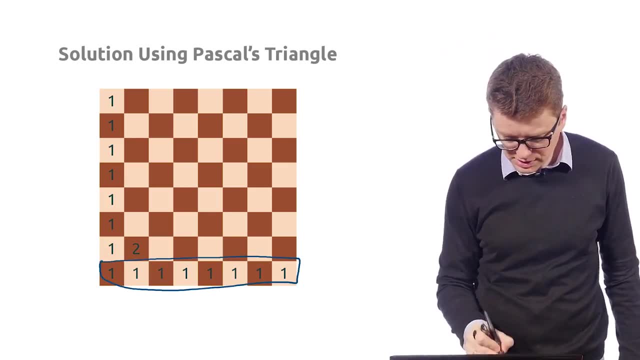 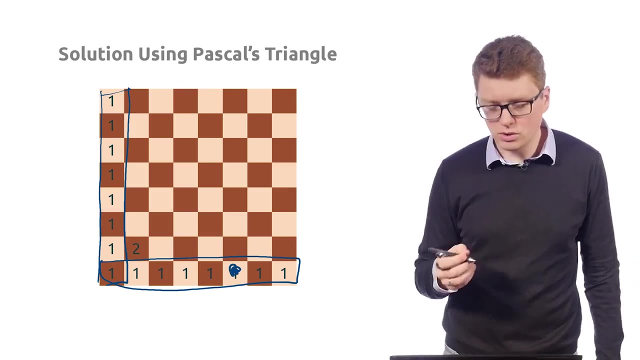 of ways of getting to this cell. first of all, for some numbers it is easy. okay, so we know that for all this, for all these cells, it is equal to one and for all these cells it is also equal to one, for example, for this cell. the only possible way, 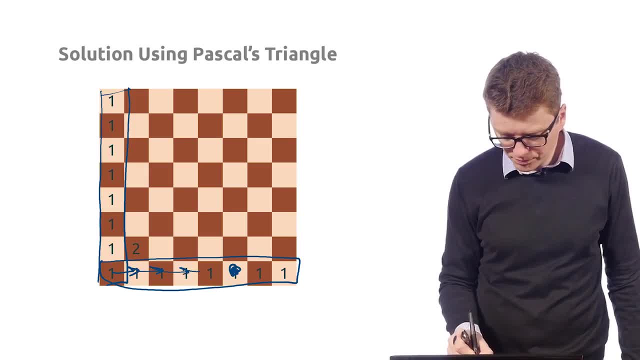 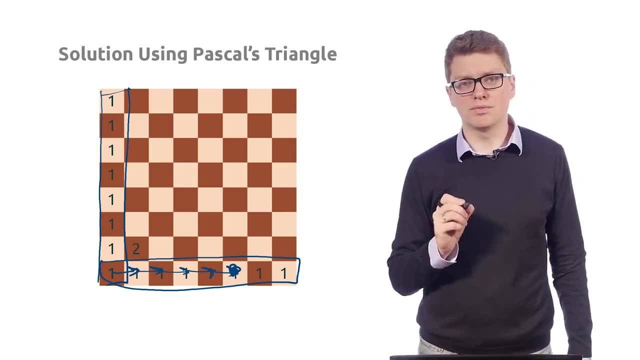 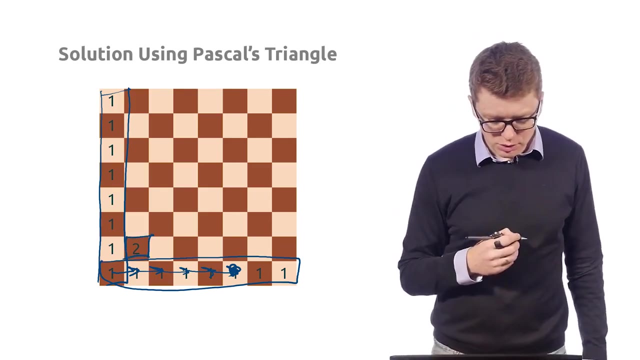 to get. to get there is to go to the right. okay, now let's do the following. let's start computing this number for all other cells. so, for example, we we show two here, Y is two. well, this is just because for every cell in our uh, in our board, there are two possibilities of the. 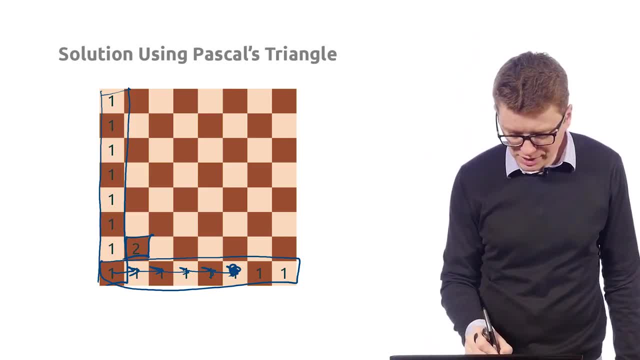 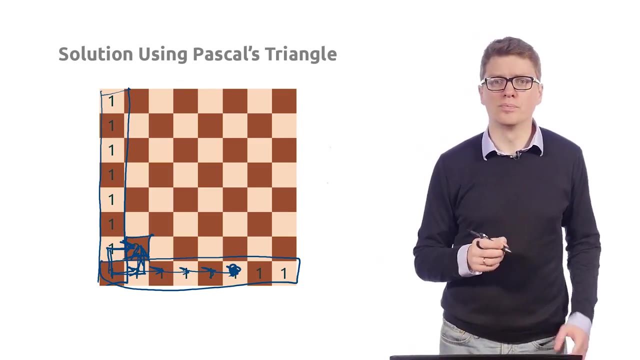 previous move before getting to this cell, so we might go there from this cell or from this cell. okay so, and in fact it is not difficult to see that we go either this way or we go either this way. so in this case it is easy to see- it is equal to two, but also- this is true in general- if we have 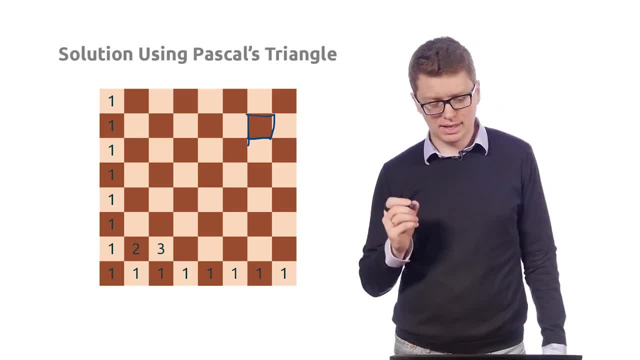 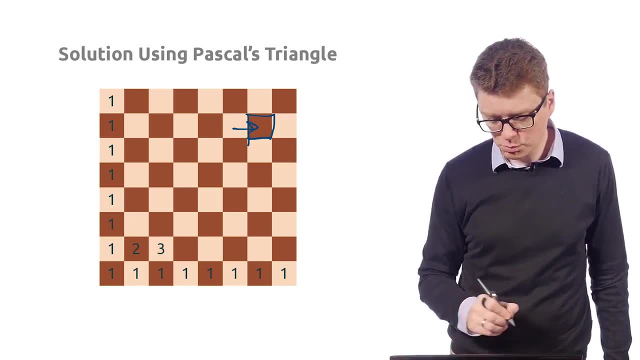 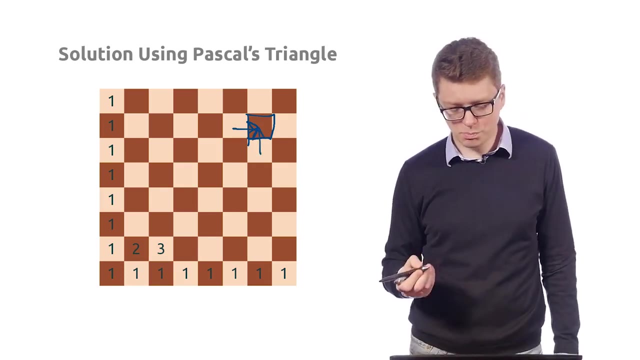 a particular cell here, for example, then any, any correct way of of getting to this cell, either its last, its last move, is either from this neighbor from the left or from, or the neighbor from below. okay, which basically means that if we have a number of ways here which is equal to B to, 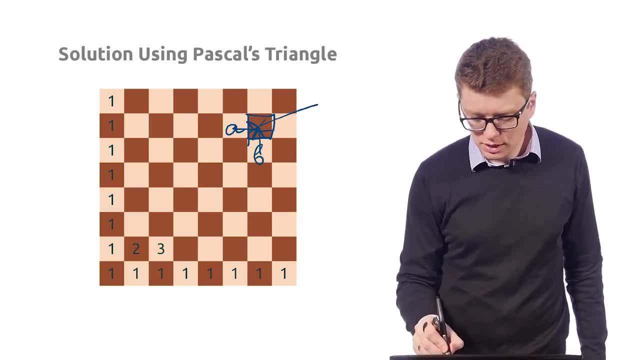 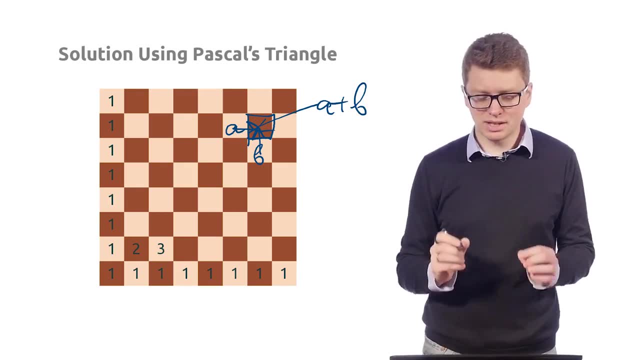 A and the number of ways here, which is equal to B, then the number of ways which we need to compute here is A plus B. so the numbers that we compute satisfy this nice property that in every cell the value is equal to the, to the value of its neighbor to the left and the value of its neighbor uh below. 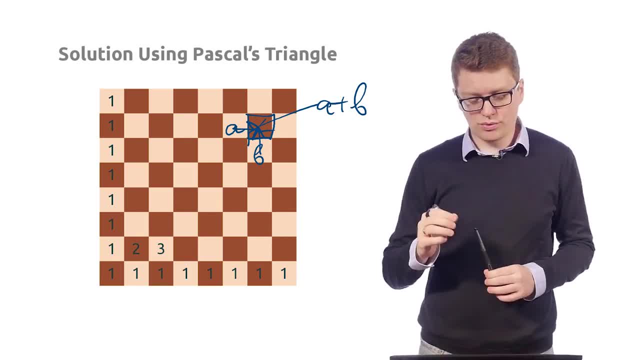 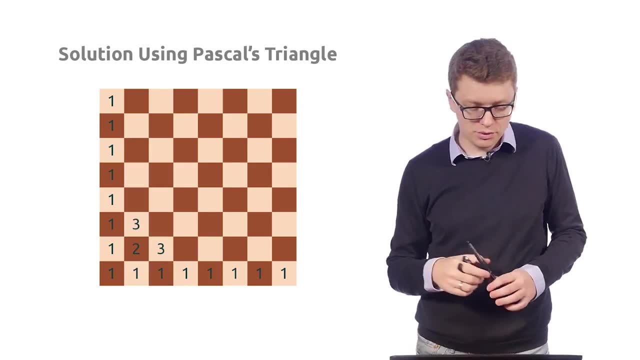 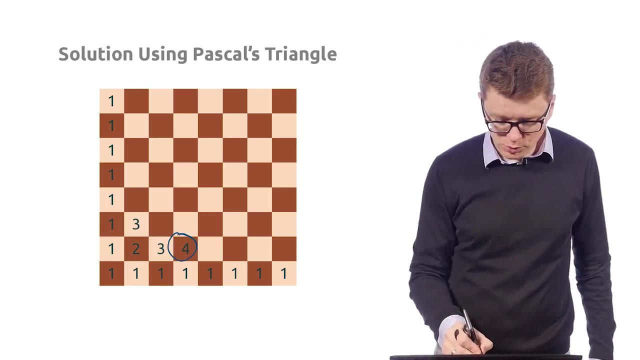 okay, and this is this allows us to to fill in this table as follows. so here we have three, just because it is the sum of two and one. okay, now let's continue filling in this table. so this three is equal to one plus two. okay, finally, this four is equal to the sum of one plus three. well, not, finally, I'm sorry, we're. 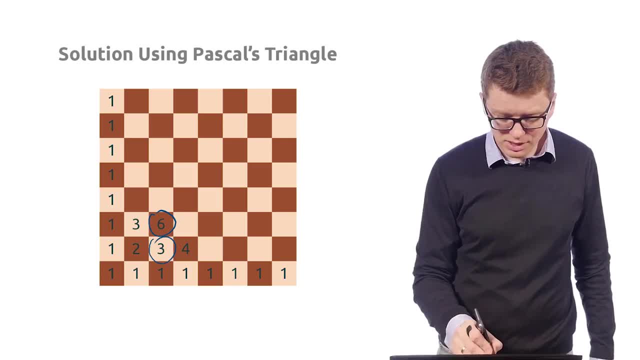 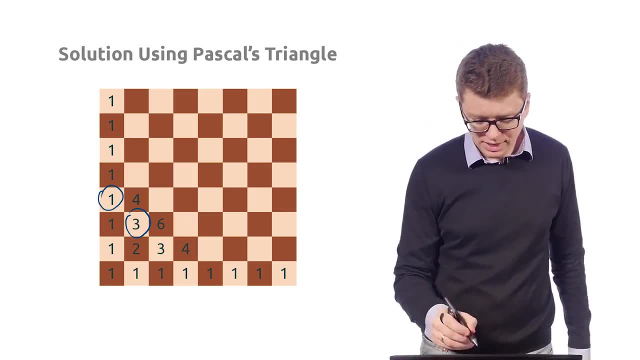 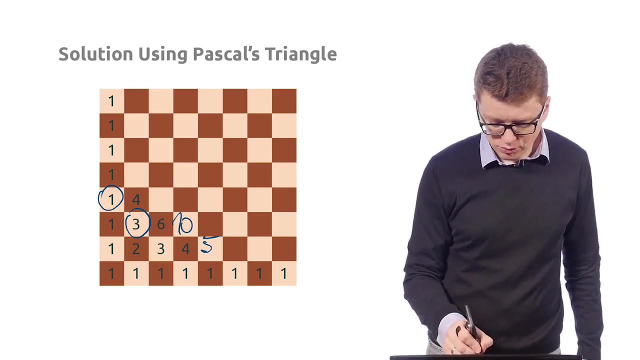 still going to fill in this table. so this six is equal to three plus three, and so on, this four is equal to one plus three. now let me continue doing this by hand. so here we we put five because it is four plus one. here we put ten because it is four plus six. here we put ten because it is four plus 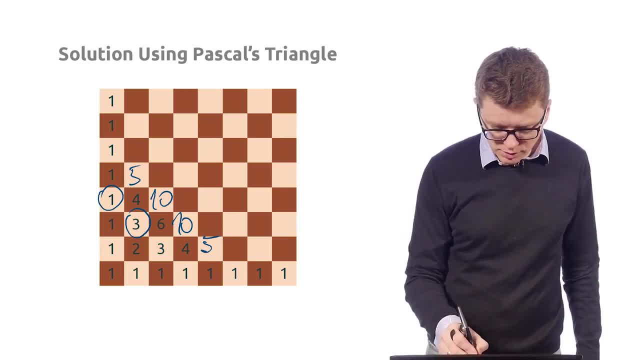 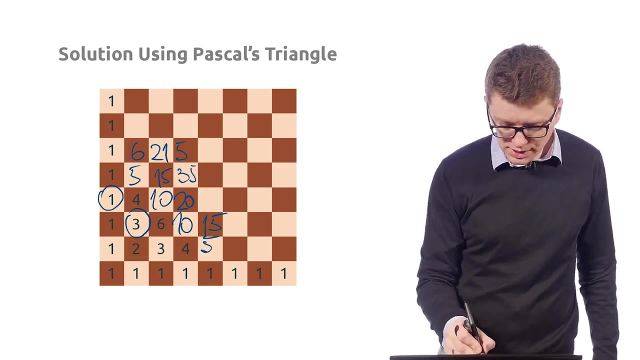 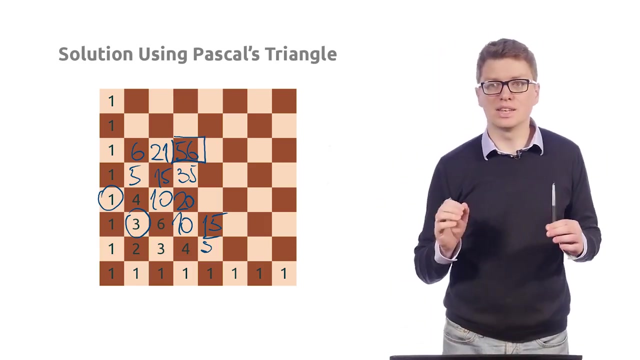 six, and here we put five, then here we put 15, here we put 20, 15 and also six, here we put 35, here we put 21, and finally, here we get 56. exactly so, for this cell that we were interested in, we get exactly the same. 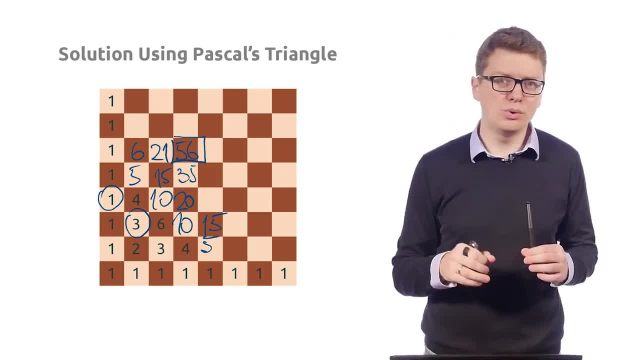 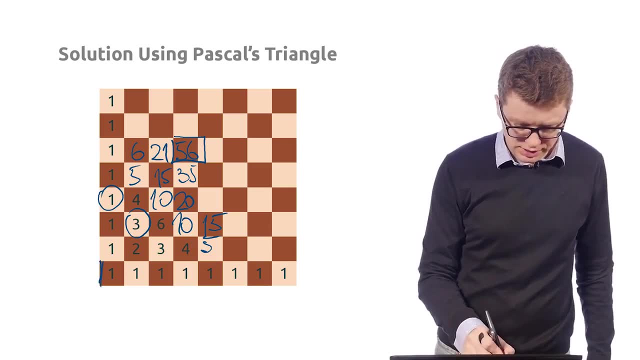 result, and you've probably already noticed that what we were doing is actually filling in the same result, and you've probably already noticed that what we were doing is actually filling in the triangle, whose uh, whose, uh, like top vertex was actually rotated to be here. so this is like the 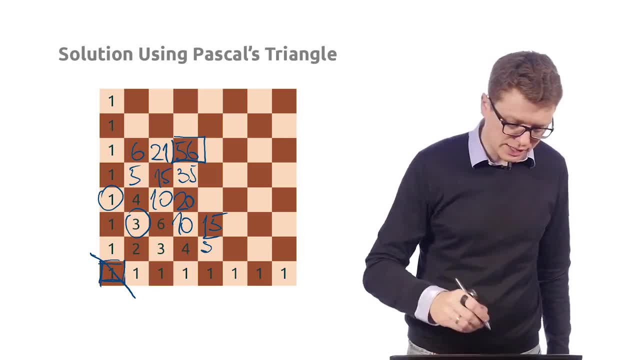 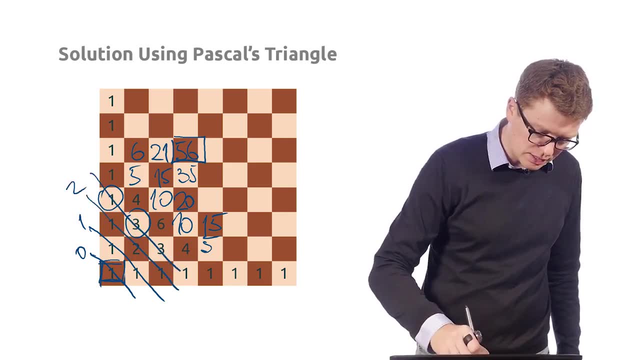 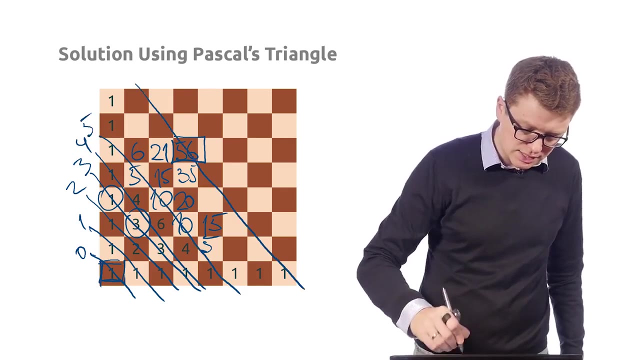 first the zeros row of Pascal's triangle. this is the the first row of Pascal triangle. so this is zero, this is first, this is second one, this is third one, this is fourth one, this is fifth one, and so on. so this, actually this cell, uh, five, three actually lies on the. 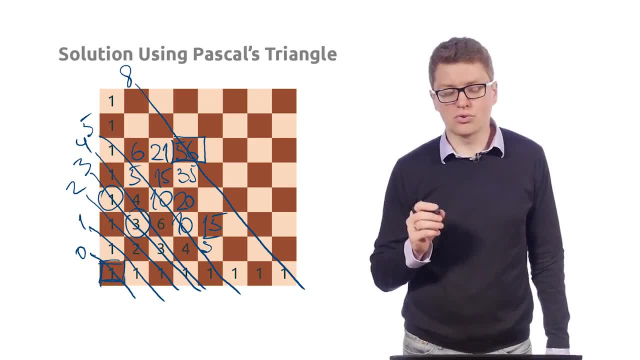 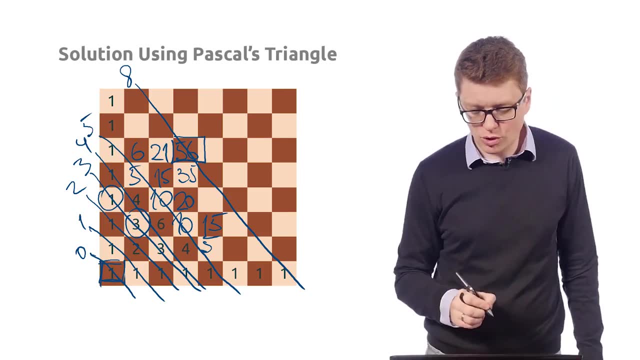 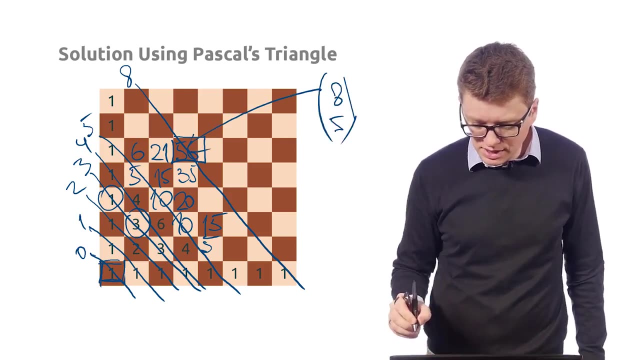 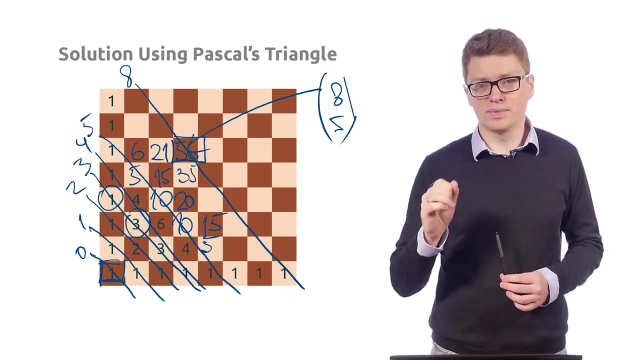 eighth, eighth, eighth row of Pascal triangle and we basically know that at eighth row, what all the values of the form eight choose something. so this particular cell is eight choose five. so this is another proof of the fact that to get to the cell five- three we need. the number of ways to do this is. 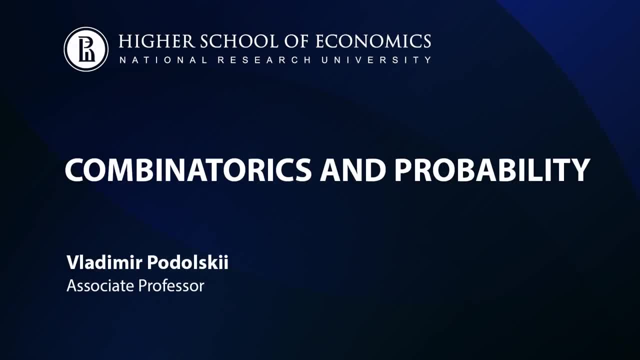 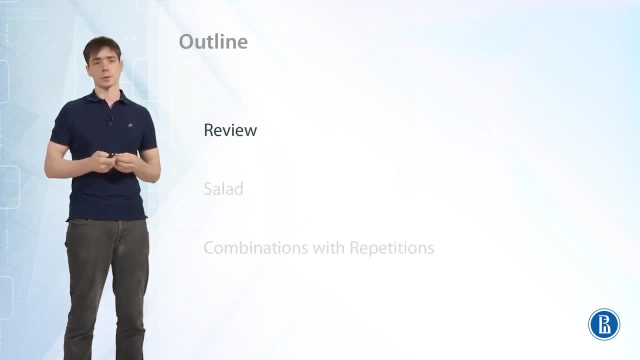 eight, choose five. hi, I'm Vladimir podolsky, and today we are going to talk about combinations with repetitions. let's review our knowledge. we have considered selections of key items out of n possible options and there are several variations to this model. we can consider ordered selections and unordered. 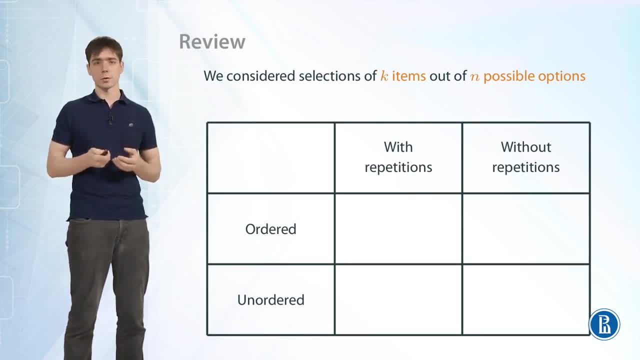 selections and we can can consider selections with repetitions and without repetitions. that is, we can allow to include the same option several times in the selection or and we can not allow to do that. so let's consider a simple example. suppose case two and there are three options: a, b and c. so the simplest case is the case of ordered selections with repetitions. 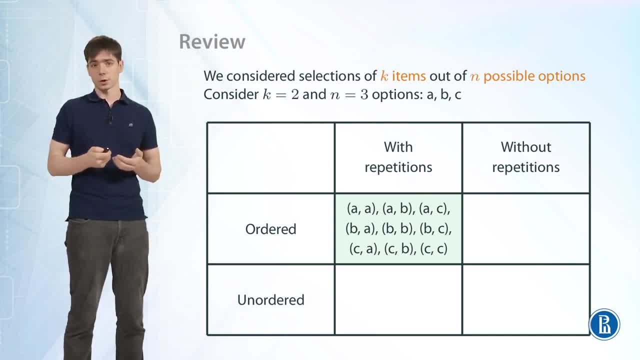 here we have nine possible selections. we can pick the first item in three possible ways and we can pick the second item in also three possible ways. next, we have considered ordered selections without repetitions. so now we have we can pick the first item again in three ways, but we can pick. 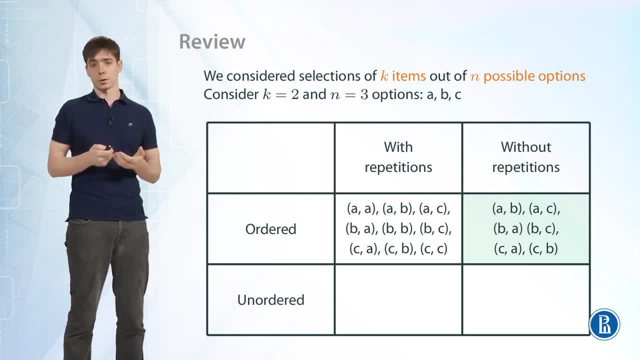 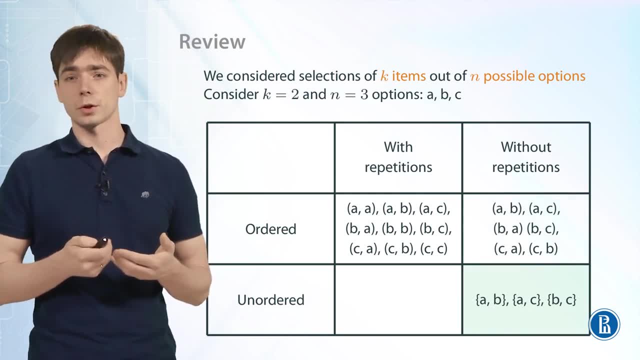 the second item only in two ways, because we cannot repeat the same, the same item twice. okay, next, we considered unordered selections without repetitions, and here we have three options: a, b, a c and b c. this is similar to the case above, but now we don't have order, so above we counted all of these pairs twice. 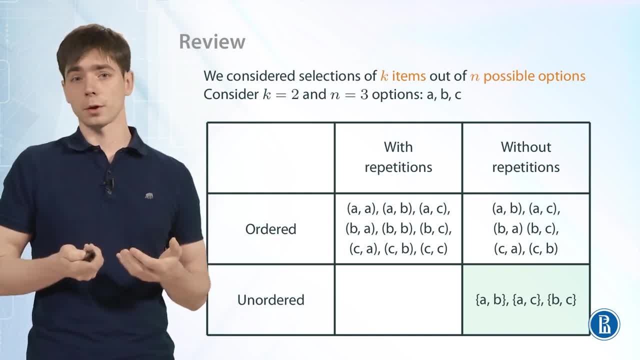 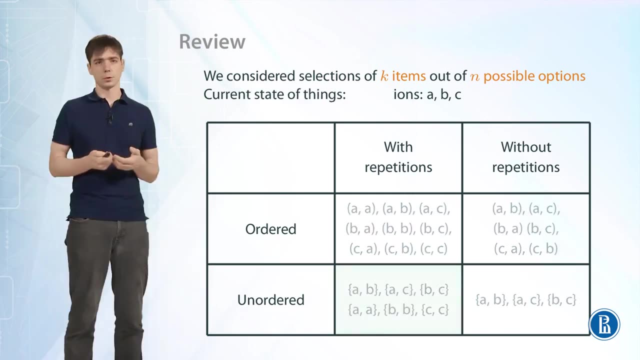 because the order okay, and now we have the fourth possible possible type of selections. we have unordered selections with repetitions. this is similar to the right case, but now we also allow selections where the same item is repeated twice. okay, let's review what we have learned so far. we considered: 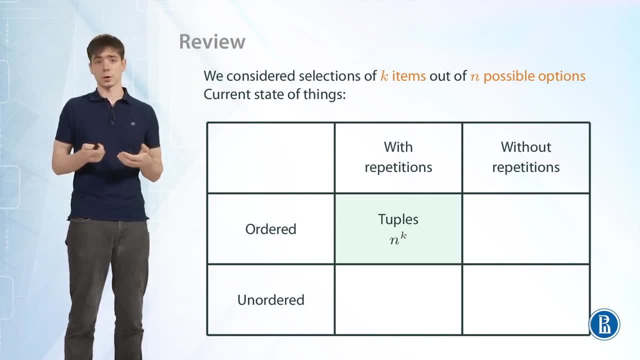 ordered selections with repetitions. these are just tuples. we can pick any item in n possible ways. there are key items, so we have n to the k possible selections. we also considered ordered selections without repetitions. these were k permutations now for the first time. then we have n options. for the second we have n minus one option. 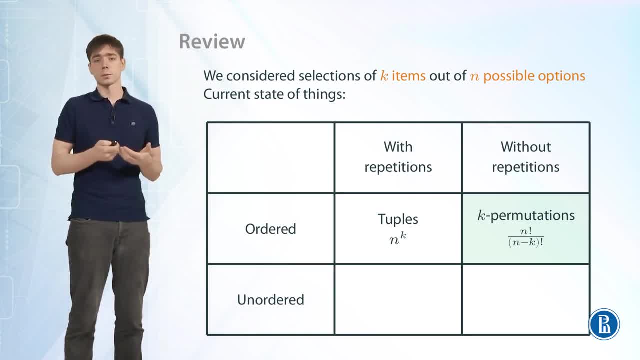 and so on. so the answer is n factorial divided by n minus k factorial. next, we considered unordered selections without repetitions. these are combinations and the answer was n choose k. and now we have the fourth, the fourth here, unordered selections with repetitions, and we haven't considered it yet. so this is this. 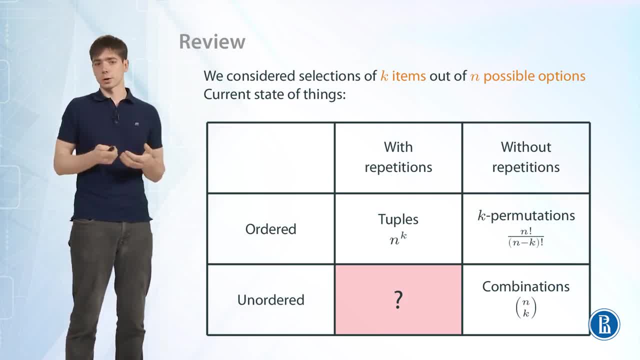 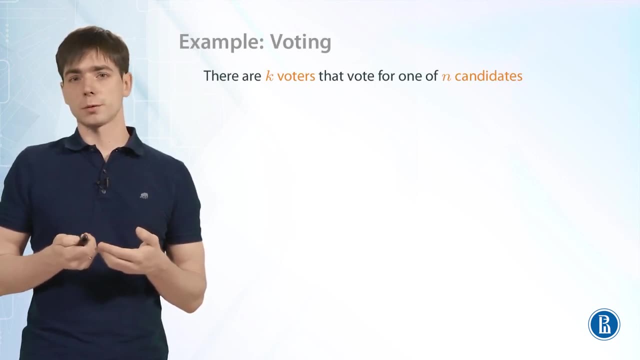 remains. this remains unclear. but before, before we start thinking about it, let's see. maybe it's, maybe it's not, not relevant, maybe this type of selections doesn't occur anywhere. let's consider the following example: there are k voters that vote for one of n candidates. so here is a ballot. this is: 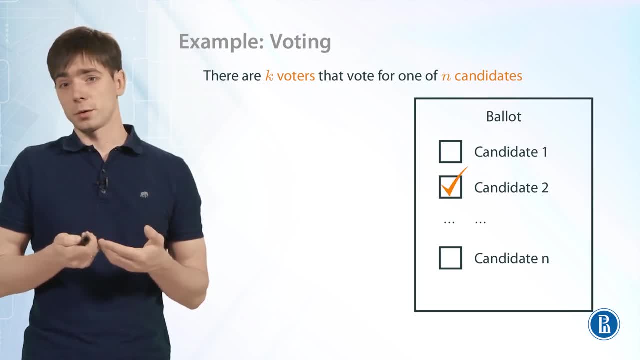 a candidate and each voter votes for one of the candidates. maybe candidate one, maybe candidate two, and so on. maybe the last candidate. so all votes equally matter. that is, it doesn't matter in which order votes are submitted. we can think of this as an unordered selection. also, candidates can be voted. 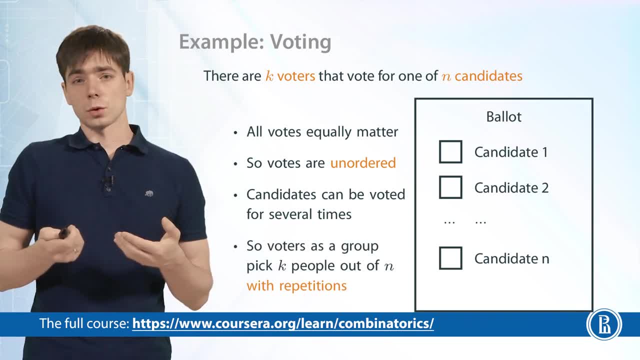 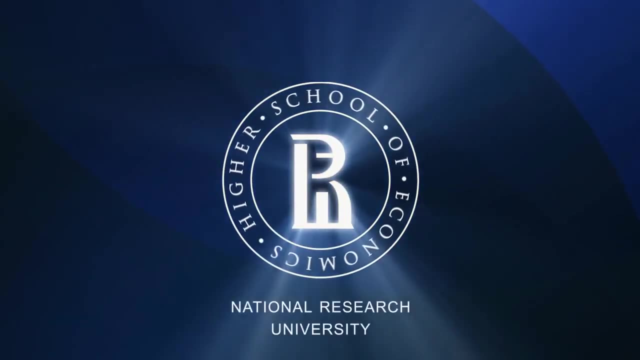 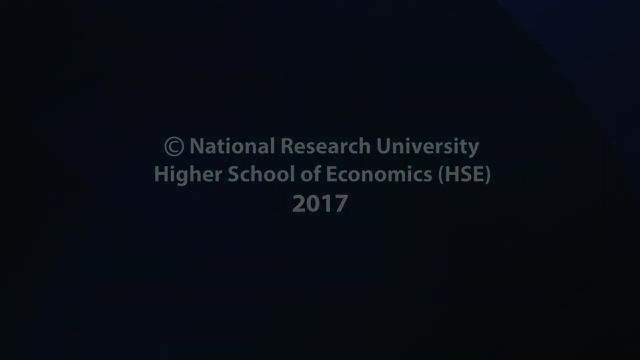 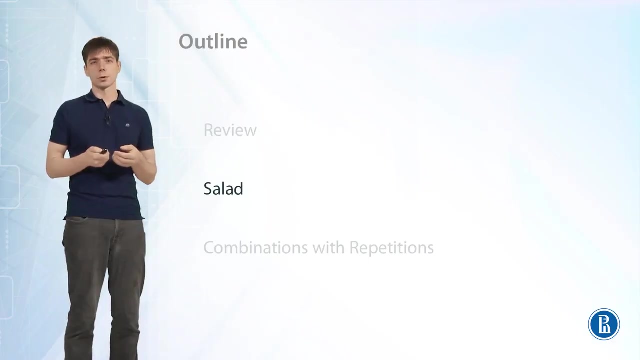 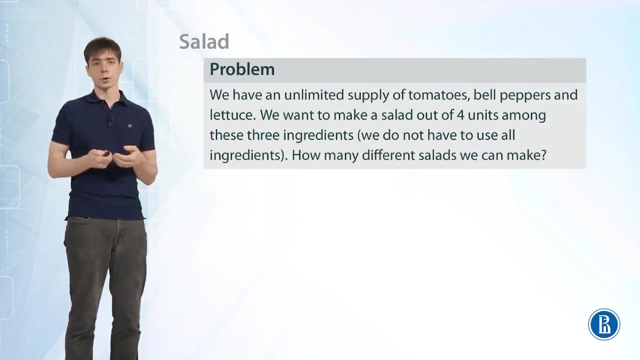 for several times by several different voters. so voters as a group pick k people out of n possibilities without repetitions. so this is this is our setting. let's consider the following problem: we have an unlimited supply of tomatoes, bell peppers and lettuce. we want to make a salad out of four units among these three ingredients. 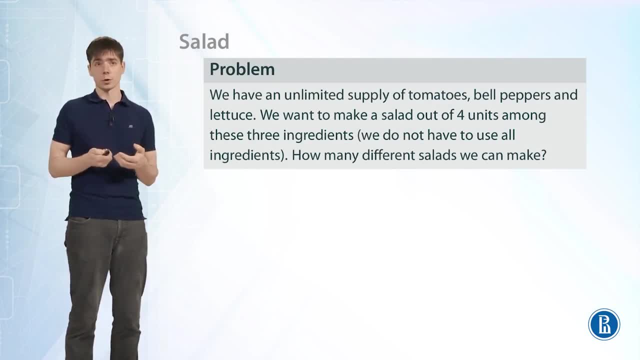 We do not have to use all 3 ingredients. we just have to pick 4 units among 3 options. How many different salads we can make. Let's see what we have in this problem. We pick 4 items out of 3 options, with repetitions. 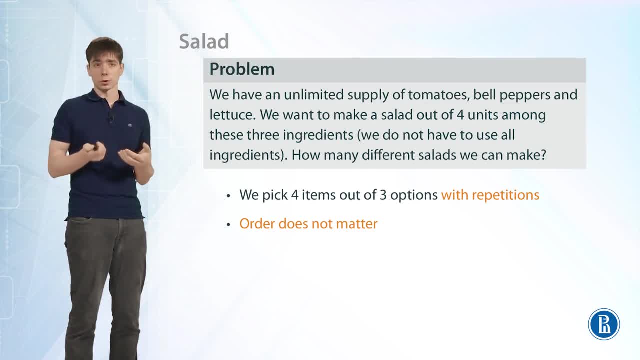 And the order doesn't matter. If we pick items in the different order, then this is still the same salad. So this is our setting: combinations with repetitions. Order doesn't matter, we allow repetitions of options. We still do not know how to compute the answer immediately. we do not have a formula. 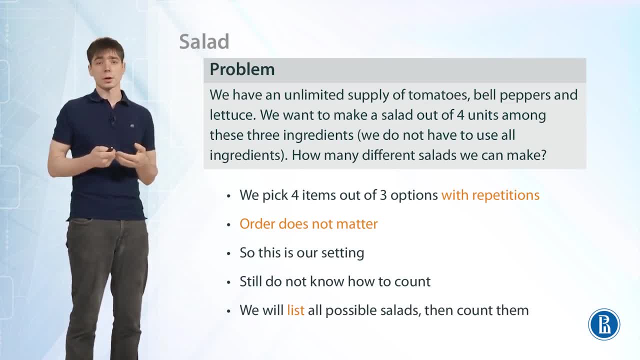 What we will do in this example. we will list all possible salads and then we will count them, But we would like to do it wisely. we would like to build up some intuition for the future solution of this problem in general. So let's look at the picture. 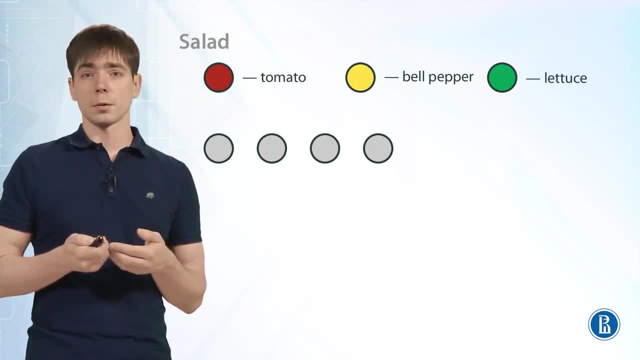 We will denote tomatoes by red circles, bell peppers by yellow circles and lettuce by green circles. So we have 4 ingredients and, for example, we can pick a salad like this, or we can pick a salad like this And note that these are just the same salads. order doesn't matter. 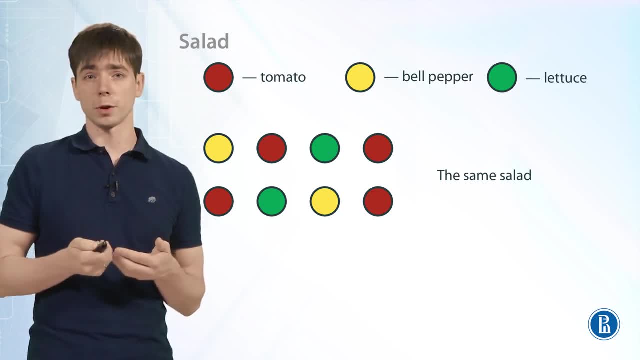 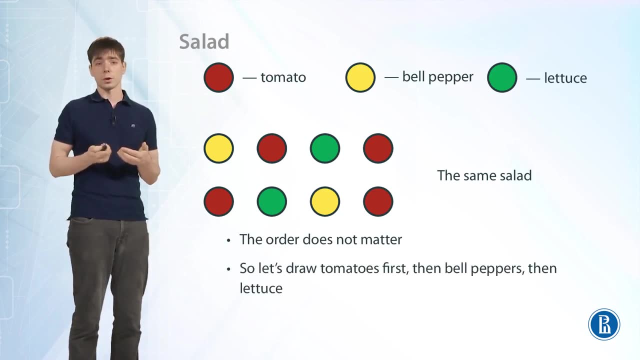 We have 2 units of tomatoes, 1 unit of bell pepper and 1 unit of lettuce. So since the order doesn't matter, let's do the following. Let's draw on our picture: tomatoes first, then bell peppers, then lettuce. 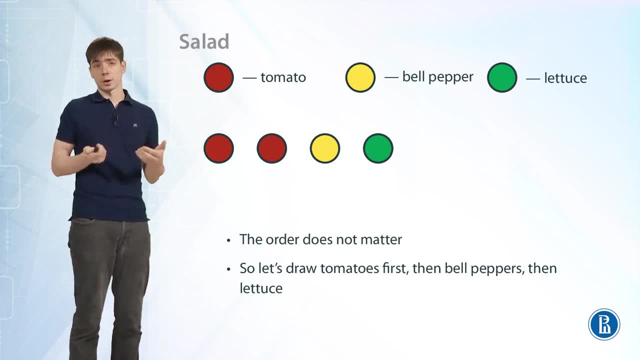 And let's do this always. So this way We will not count the same thing twice. So this is the same salad, but now we have ordered it. Okay, Now we have to list all possible salads, So we have to do it in some ordered way, in some reasonable way. 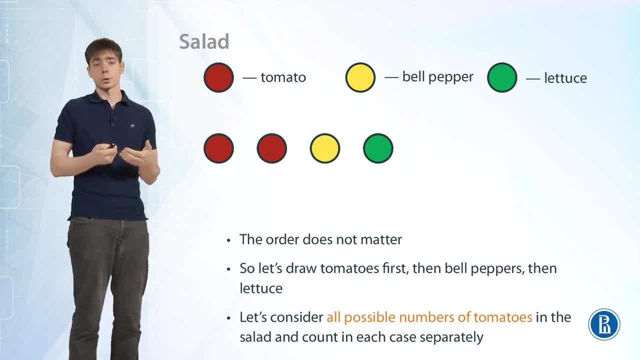 Let's consider, let's do the following: Let's consider all possible numbers of tomatoes in the salad. Let's consider all possible cases and we will count the number of salads in each case separately. Okay, Let's proceed to this. Here is our salad. 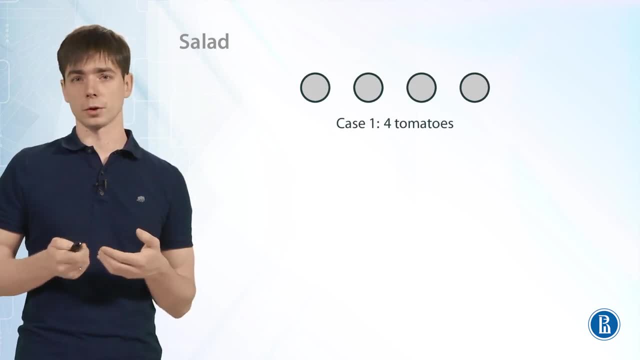 And let's start with the simplest case, The case of 4 tomatoes. Here it is, And there is only 1 salad with 4 tomatoes, because there is no room left for other ingredients. So 1 salad, Let's proceed to the next case. 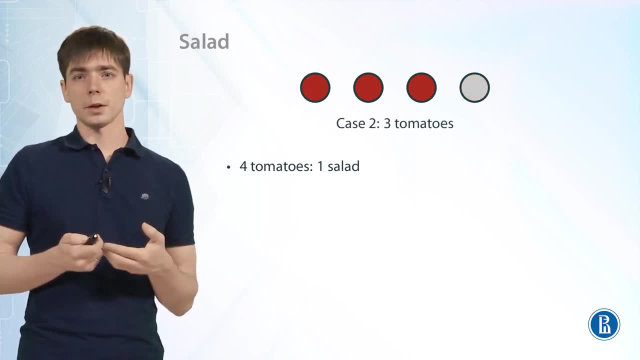 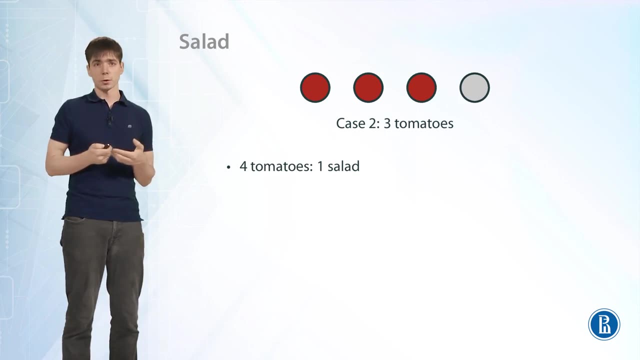 The case of 3 tomatoes. Now we have to pick the last ingredient. It cannot be a tomato, because we have only 3 tomatoes now, And so it can be either bell pepper or lettuce. Okay, Bell pepper Lettuce. 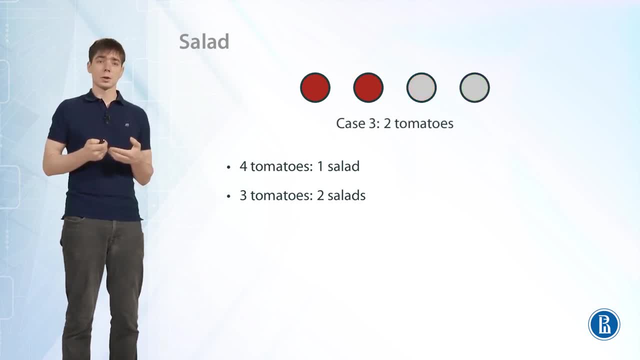 So there are 2 salads with 3 tomatoes. Okay, Next case: 2 tomatoes. Now we have 2 ingredients left, and they can be either 2 bell peppers, 1 bell pepper and 1 lettuce and 2 lettuce. 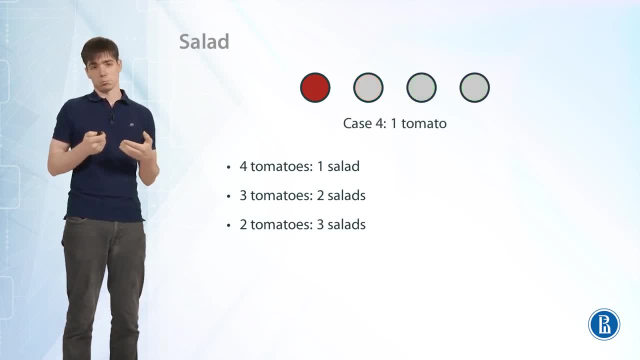 Okay, So we have 3 salads in this case. Now the case of 1 tomato. Now we have 3 ingredients left. It can either be all of them, can be bell pepper, 2 bell peppers and 1 lettuce, 1 bell pepper and 2 lettuce and 3 lettuce. 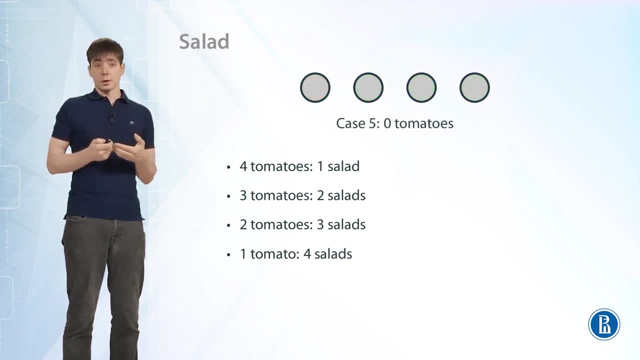 So there are 4 salads now And the last case, The case of 0 tomatoes, There are no tomatoes in our salad, Then either all ingredients can be bell pepper, there can be 3 bell peppers and 1 lettuce. there can be 2 lettuce and 2 bell peppers, 1 bell pepper and 3 lettuce. 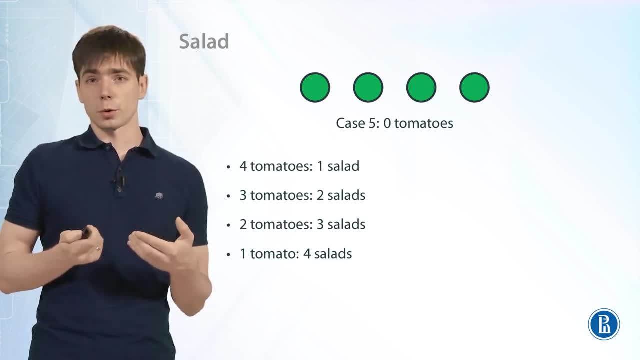 And all of them can be bell peppers. So these were 5 cases. So in case of 0 tomatoes, there are 5 possible salads. So we have considered all possible cases of the number of tomatoes And in total, if we sum this up, we will see that these are 15 salads. 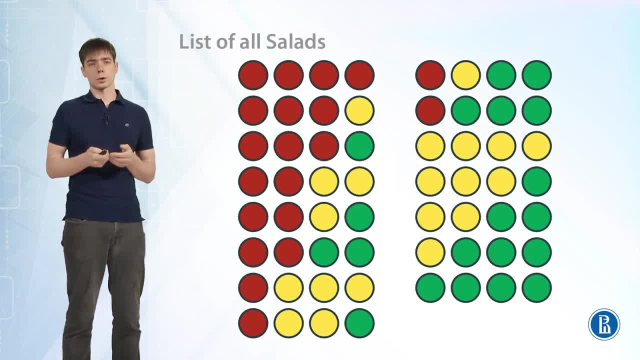 In total we have 15 salads. So here is the list of all of our salads. In the first column we can see 1 salad for 4 tomatoes, 2 possible salads for 3 tomatoes, Then 3 possible salads for 3.. 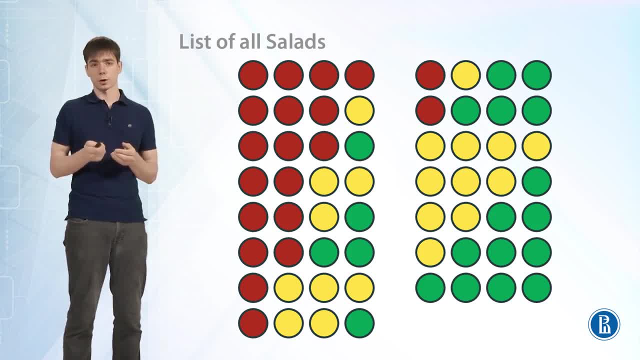 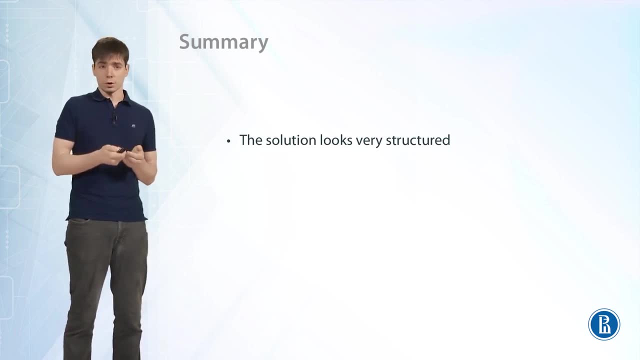 Okay, Okay, Okay, Okay, tomatoes. then four options for one tomato and finally five possible salads for zero tomatoes. So here we are all in the picture. there are 15 options in total and we are done. Okay, the solution looks very structured. For four tomatoes, we have one salad for three tomatoes. 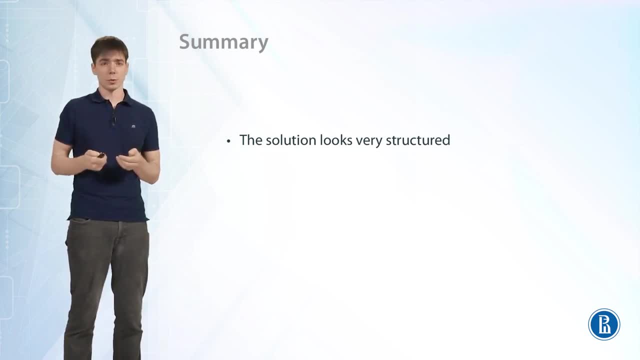 we have two salads, and so on. Each time the number of salads increases by one. If we increase the size of the salad but keep the number of ingredients the same, then the same structure holds. So the solution will have the same structure. But if we increase, 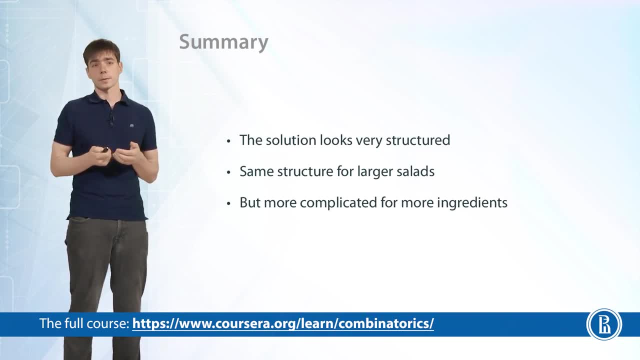 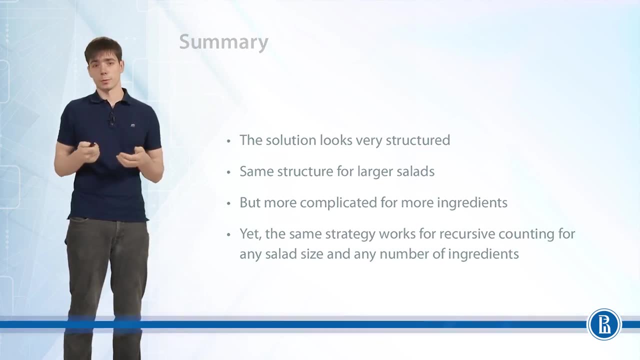 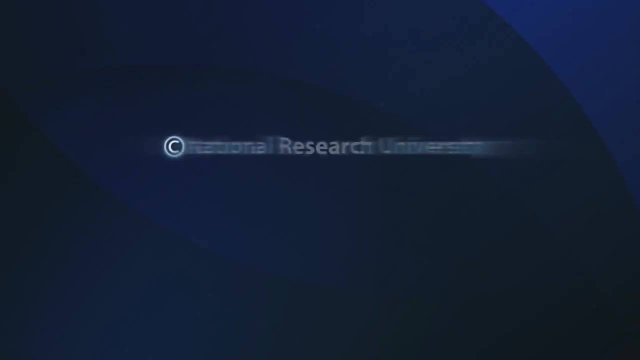 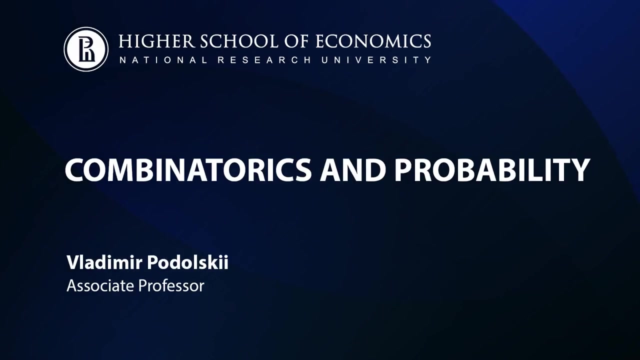 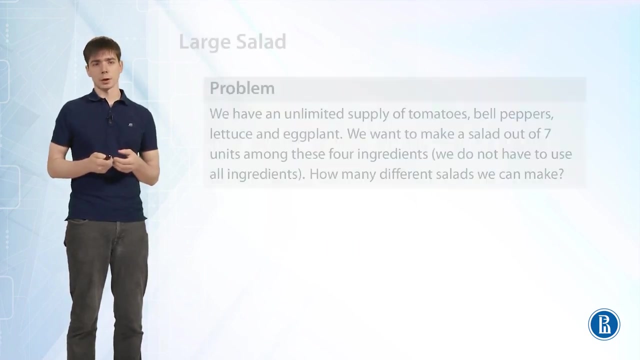 the number of ingredients, then the picture becomes more complicated. Yet the same strategy works. We can still count the number of salads in the same recursive manner. Let's consider the following problem: We have now unlimited supply of tomatoes, bell peppers, lettuce and eggplants, So we want to make a salad out of seven units among these four. 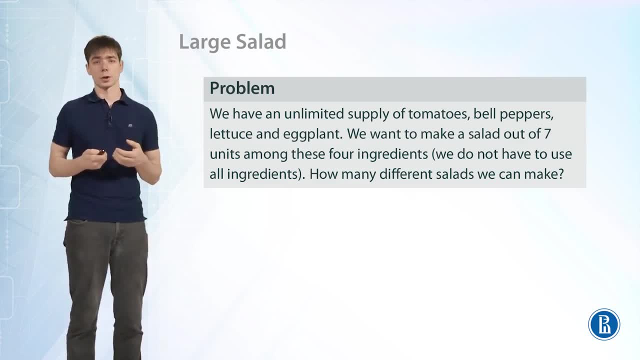 ingredients. Again, we do not have to use all ingredients. we just have to pick seven units among them. How many different salads we can make. Okay, we can use recursive counting here as well as in the previous problem, But now we would like. 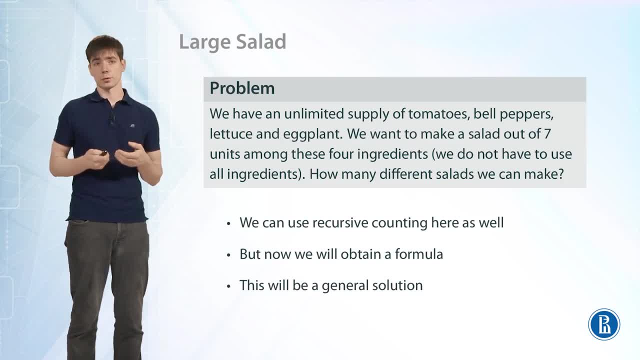 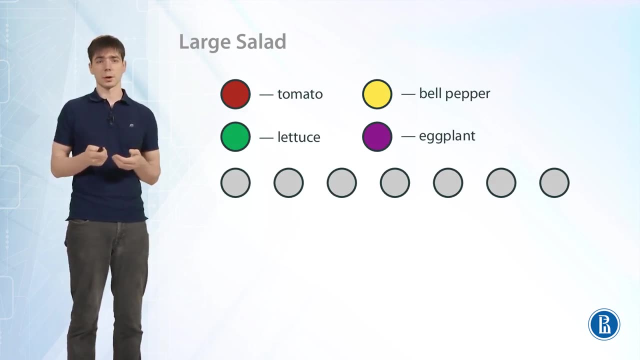 to obtain a formula, And this will be a general solution. Our solution will work for any number of ingredients and any size of salad. Okay, so here is the picture again Now: tomato is red, bell pepper is yellow, lettuce is green and eggplant is purple. 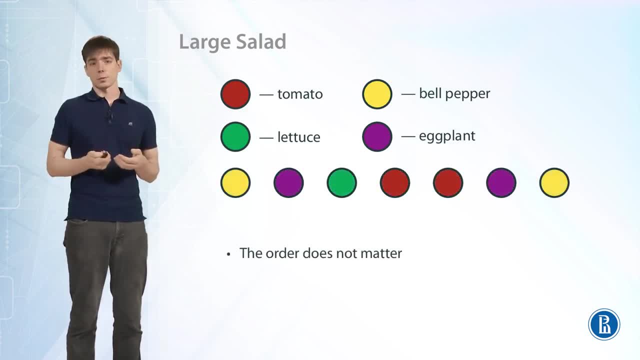 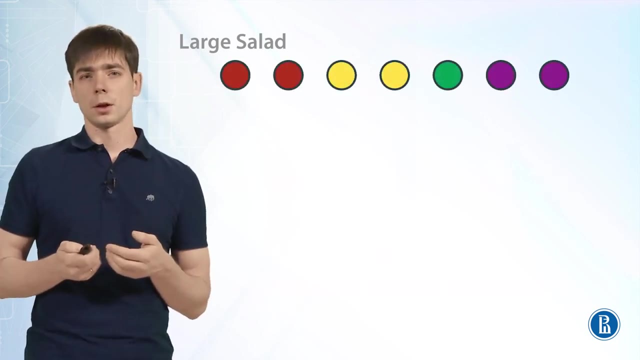 Okay, now we have seven ingredients. Here is an example of salad, but note again that the order doesn't matter, So for our convenience let's just list the tomato first, then bell peppers, then lettuce, then eggplants. So here is our salad, The solution to the problem. 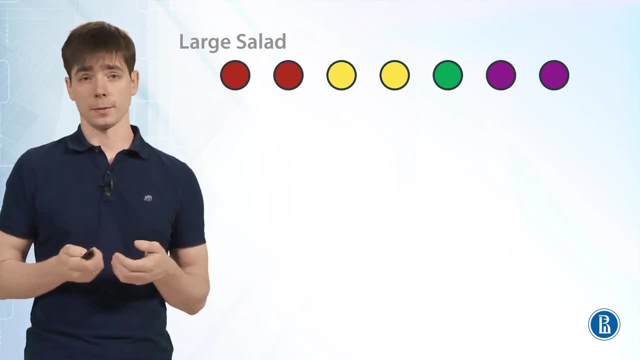 is non-trivial, So we will break it down to several simple ideas. Okay, the first idea: What information do we need to specify the list of ingredients? There are a large selection of ingredients for this order, so frequently we need to add various toda. Okay, the first idea. What information do we need to specify a list of ingredients? 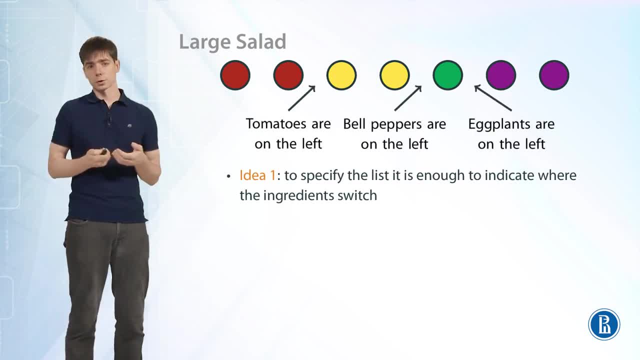 What is enough? Okay, it turns out that it is enough to say where, in this list, we switch from tomatoes to bell peppers, where, in this list, we switch from bell peppers to lettuce, and where we switch from lettuce to eggplant. So we can mark. 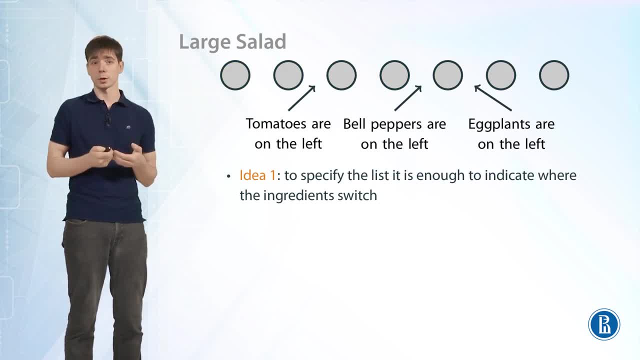 these places. and then this is enough information. We can forget about colors Now. we do not need colors. we can reconstruct them from what is on the picture. Okay, next second idea: We do not even need these text descriptions for tomatoes, bell peppers and eggplants. We can remove. 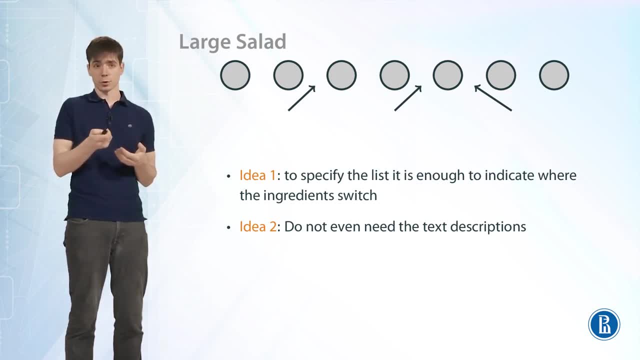 them, because we know that this first place corresponds to the switch from tomatoes to bell peppers. We have ordered ingredients in this way. The second corresponds to switch from bell peppers to lettuce and the last one from lettuce to eggplant. Okay, And finally, the third idea. We can represent these places of switches by 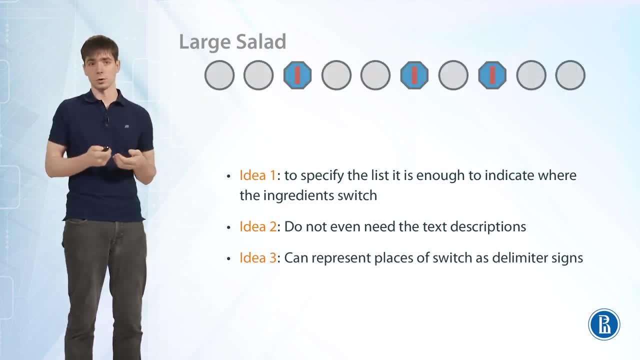 some special signs, some delimiter signs. Let's do it. Okay, we have done this. so now we have the first delimiter between tomatoes and bell peppers. This is after the second ingredient. Then the next delimiter is between bell peppers and lettuce, and the last. 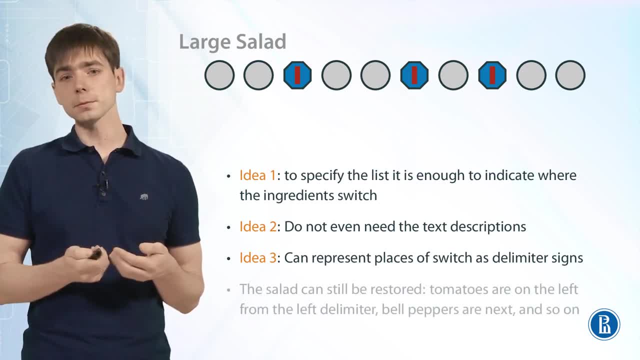 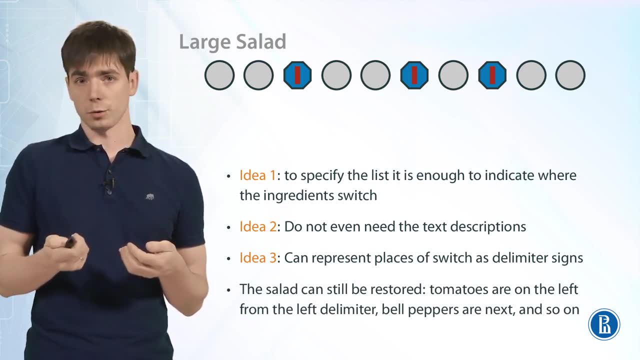 delimiter is between lettuce and eggplant. Okay, and note again that the first delimiter is between tomatoes and bell peppers and the last delimiter is between lettuce and eggplant. Okay, and note again that that the salad can be still restored from the current picture. 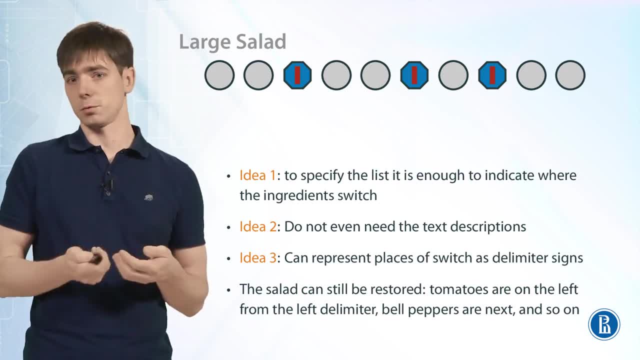 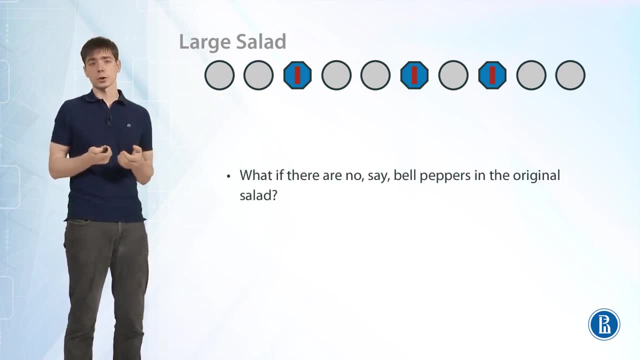 We can just color the ingredients as we described before, and we will restore the original salad from this picture. Let's do a small sanity check right now: What happens if in our salad there are no, say, bell peppers? So will the picture make sense? 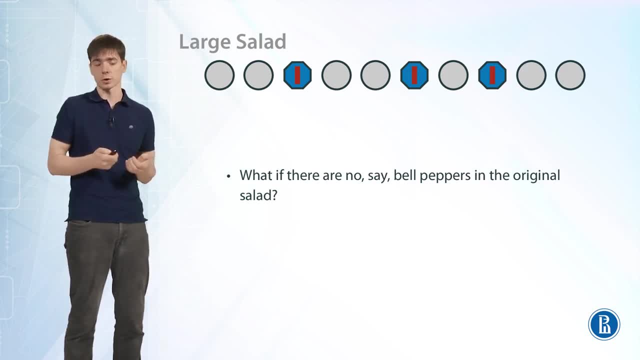 So how will it look like? Can we represent such a salad with such a picture? It turns out that this is fine. we will have a picture like this: The first and the second delimiter will be right next to each other. there are no ingredients. 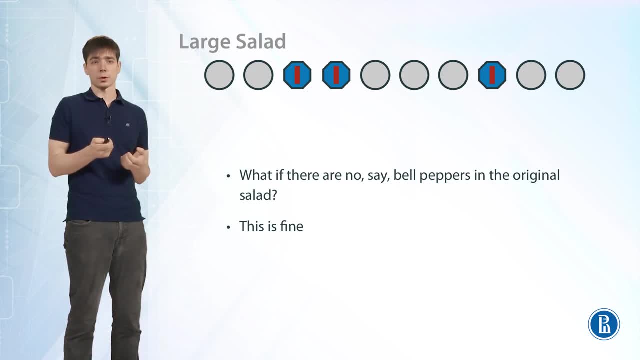 in between of them. So in case of this particular picture, we have salad with two tomatoes, three lettuce and two eggplants. So this is fine. our picture still represents such salads. Now let's proceed with the proof. What do we need to specify to fix a particular salad? 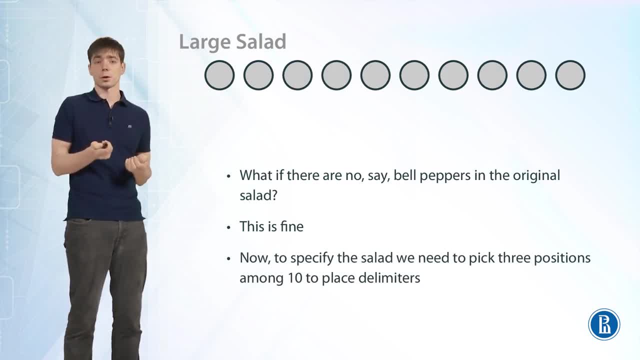 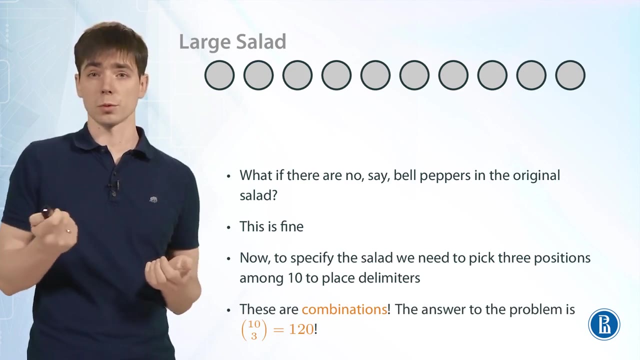 Now it turns out that this is simple. We need just to specify where to place three delimiters among these two positions. If we specify three delimiters there, then our salad is ready, And these are exactly combinations. So we have ten possible options and we have to pick three out of them, without order. 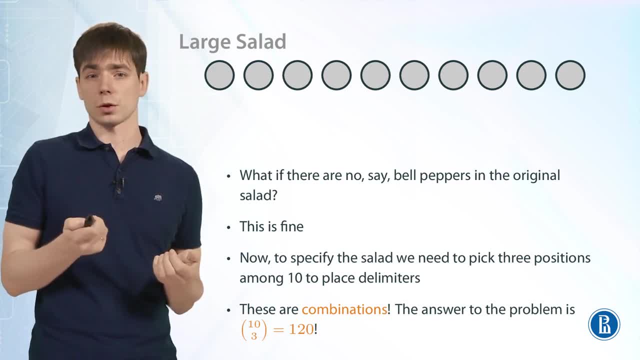 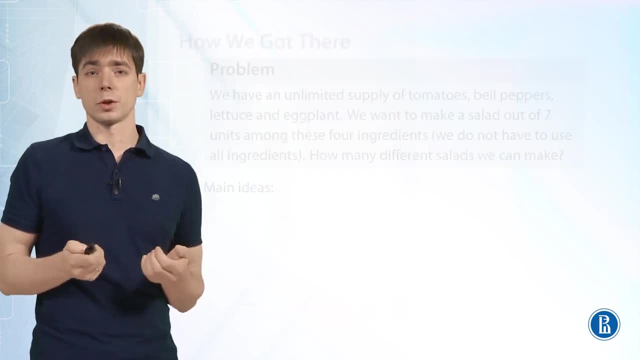 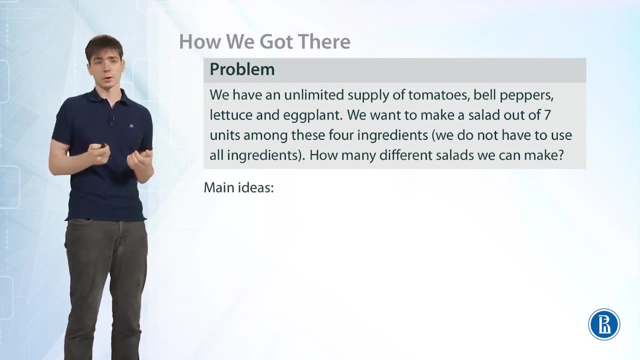 So the answer here is just n choose 3,, which is 120.. Note that this is 120, not 120 factorial, So the answer to the problem is 120.. Okay, let's review how we got there. Here is the original problem and let's review our main ideas. 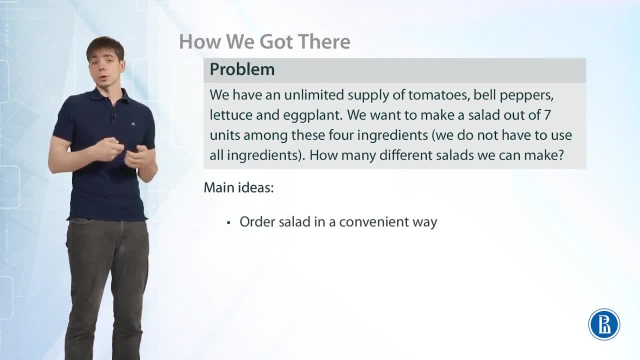 First order salad in a convenient way. Order doesn't matter, So we can order the ingredients in a way we like. So that turned out to be very useful. Next, salad can be determined by delimiters between types of ingredients. So we introduce delimiters. 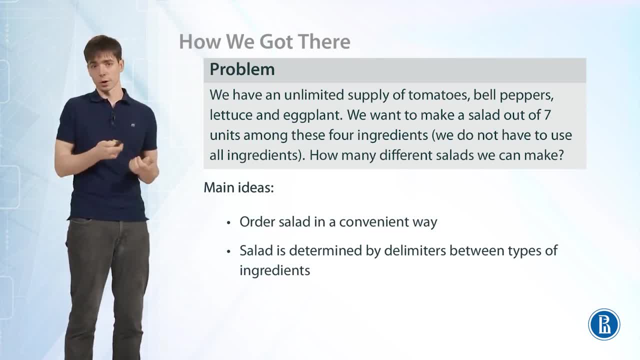 And once we introduce them, we do not have to provide any more information. We have delimiters, we know where ingredients change And final idea is to place delimiters in the line with our ingredients. And then we have a list of ten options: seven units plus three delimiters. 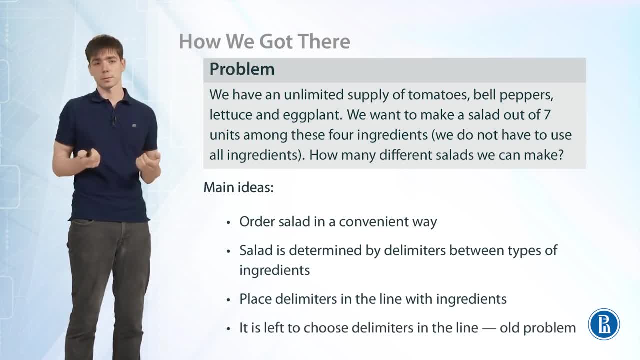 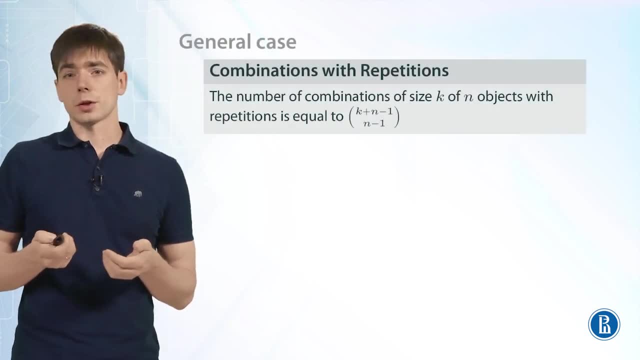 And we have to pick three delimiters among them, And that's what we already know: how to do. So if you consider number of combinations of size k out of n objects with repetitions, then the number of such combinations is equal to k plus n minus one. choose n minus one. 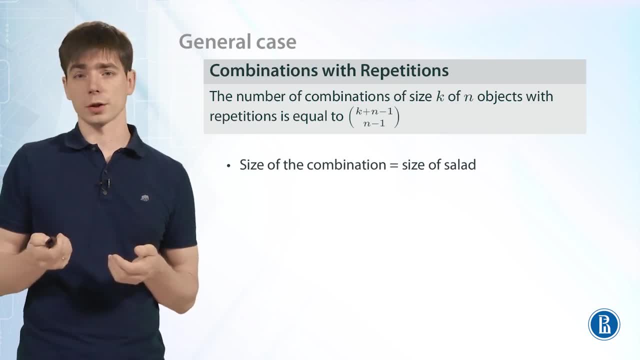 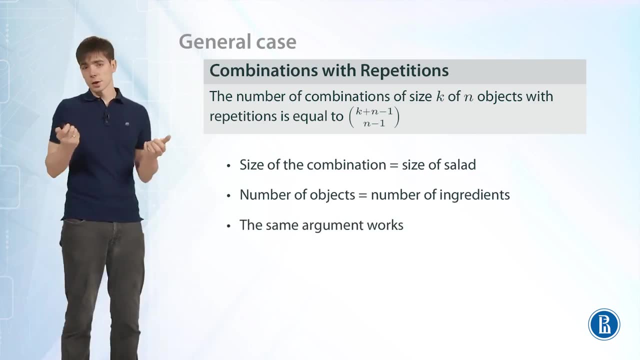 So here is the connection to the previous problem. Size of the combinations is size of the salad, Number of objects is the number of ingredients And the same argument works. So just our previous argument was general, So we can substitute seven and four. 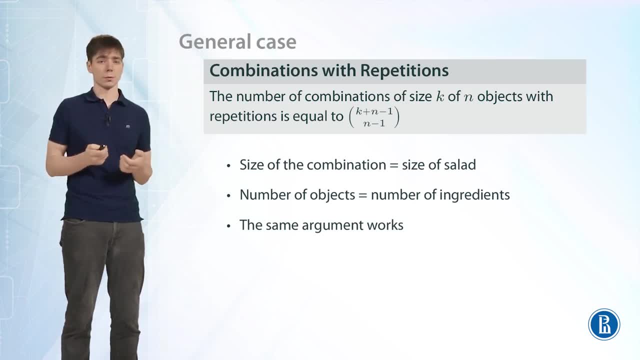 By k and n. and the same, just the same proof works. Let's just recollect briefly why we have k plus n minus one here and n minus one. Why not, for example, k plus n and n? Just so it looks natural? but instead we have k plus n minus one and n minus one. 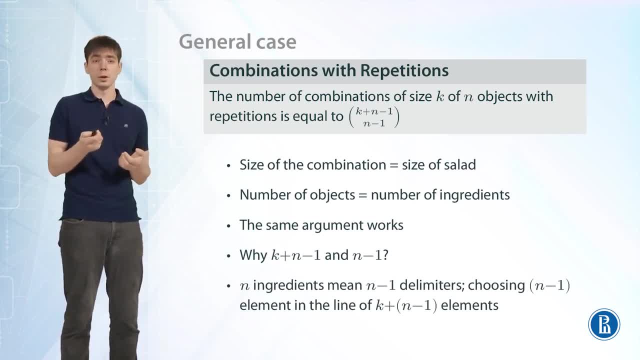 So recall that n ingredients in the salad mean that we need to place n minus one delimiters between them. So here is where n minus one comes from. So in the end of the solution we will have to choose n minus one positions in the line. 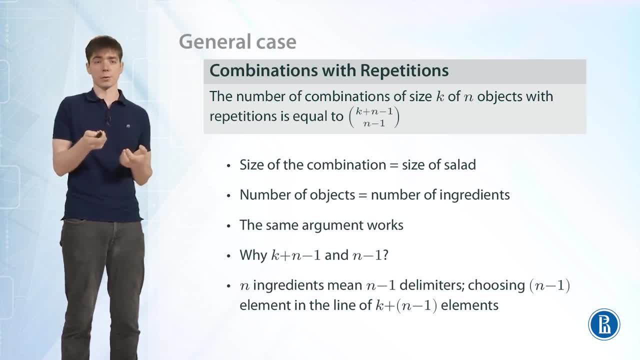 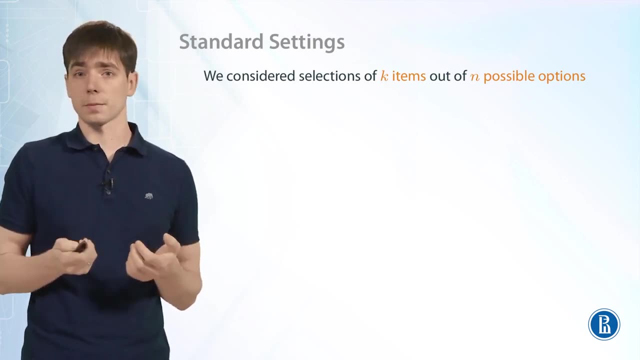 of k plus n minus one elements. k stands for the number, for the size of the salad, for the number of units of ingredients in the salad, And n minus one is the number of delimiters. Okay, now let's get back to our table. we had in the beginning of this lesson 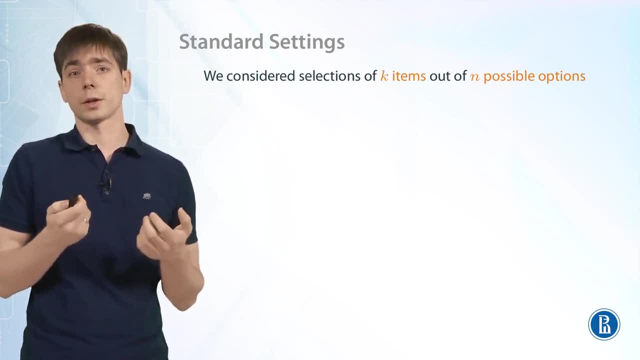 We can consider different variations of solutions. We can consider different variations of solutions. We can consider different variations of solutions. We can see several variations of example. If we have selected k items out of n possible options, we might start our solution, which is sleep, sleep, sleep. 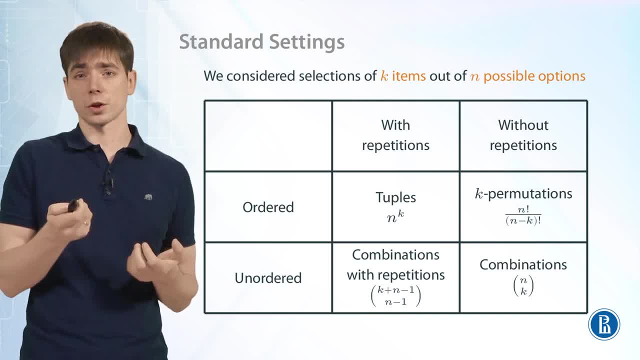 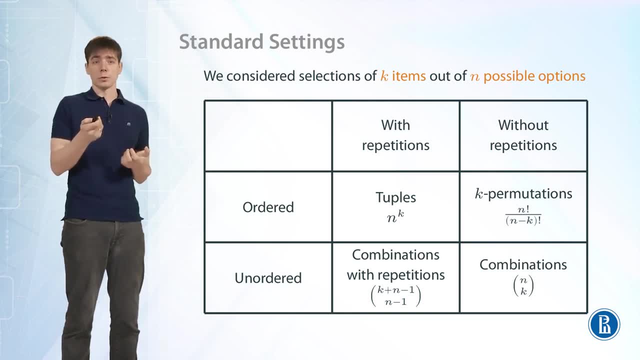 If we have selected k items out of n possible options, we might start the solution which is sleep, sleep, sleep. Selections removed without revolutions. Let's briefly review them now. So viise, or order n into k, are just tuples. Next, we can just filter k permutations. 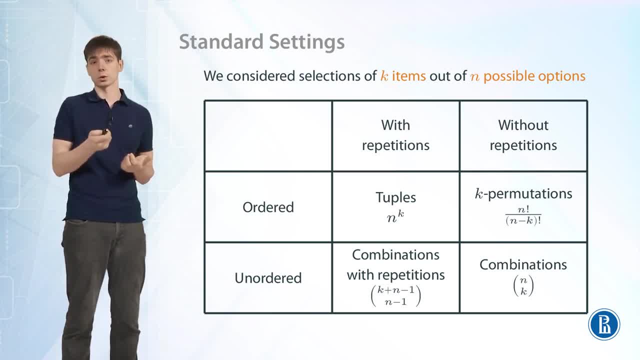 But the recيlections are surprising. selections, unordered selection without repetitions. They are combinations and there are n choose k of them. And in this lesson we consider the final cell of this table: unordered selections with repetitions. and it turns out that binomial coefficients helps here as well. So the number of combinations with 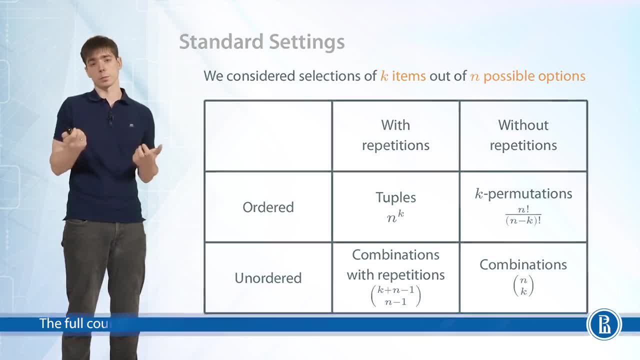 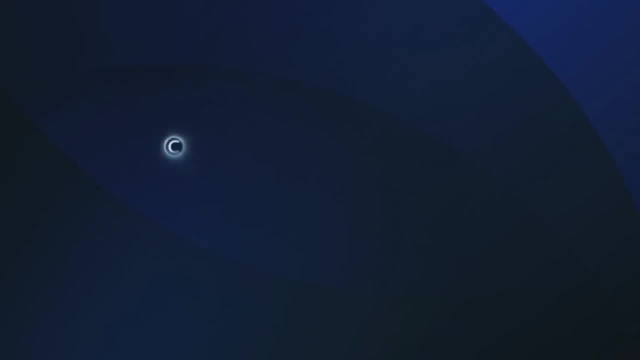 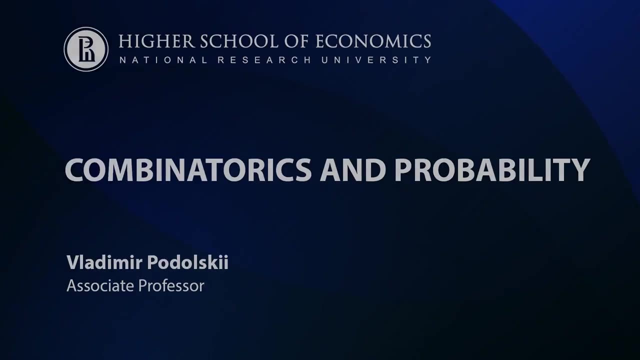 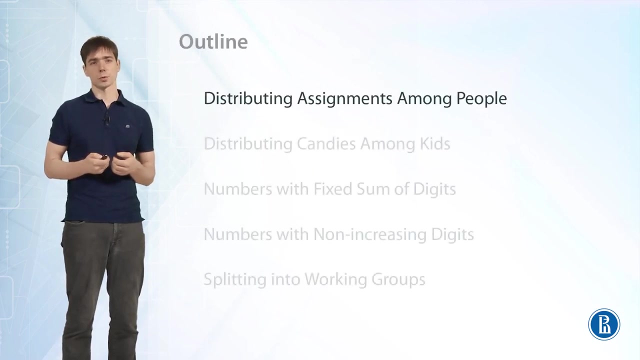 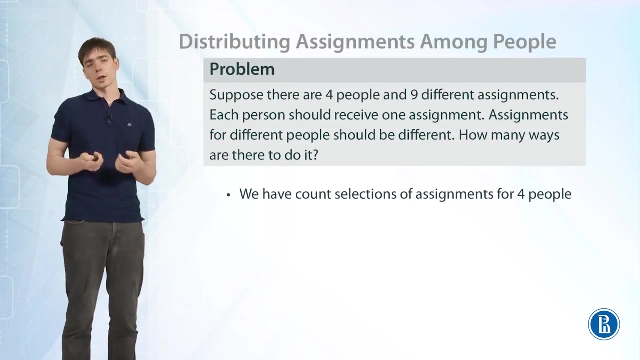 repetitions is equal to k plus n minus 1. choose n minus 1.. Hi, I'm Vladimir Podolsky, and today we are going to discuss various problems in combinatorics. Let's consider the following problem: There are four people and nine different assignments. We would like to assign each person one assignment. 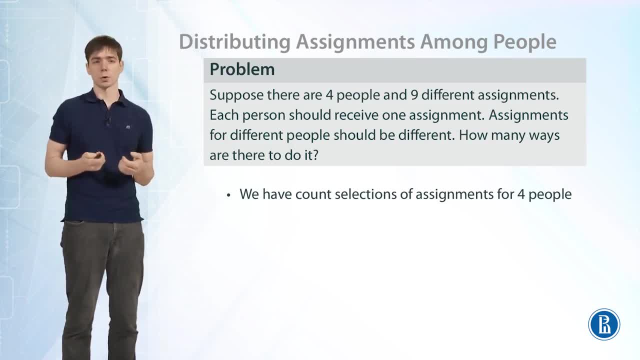 How many ways do we have to do it? Okay, in this case, we have to do it in the following way: In this problem, we have to count selections of assignment for four different people. People are different, so the selections are ordered And no. 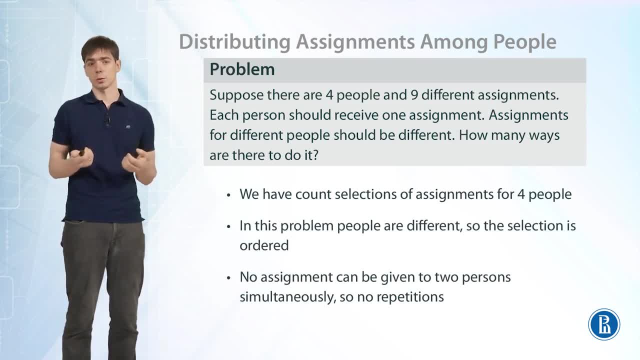 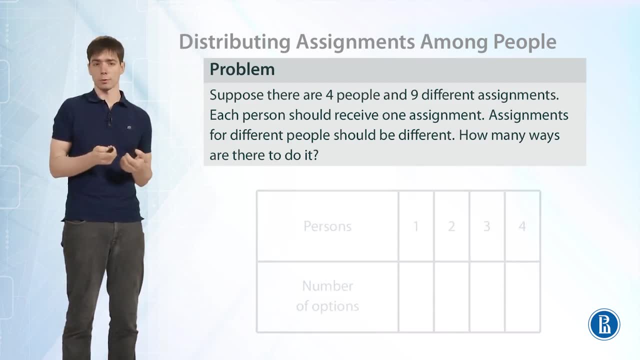 assignment can be given to two persons, so we do not allow repetitions, So we are just dealing with k permutations. Okay, let's consider the table. There are four persons. there are a number of options for them. For the first person, we can pick an. 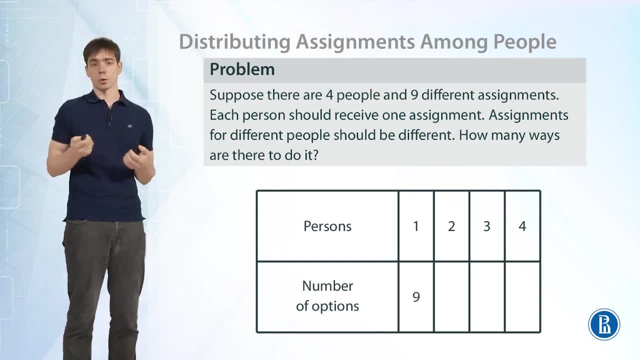 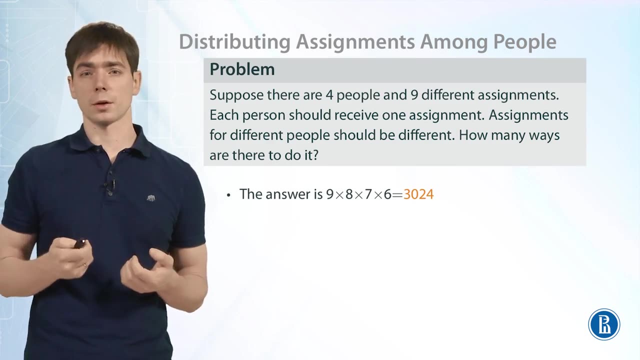 assignment in nine possible ways. For the second person, there are only eight options, for the third, there are seven possible options, and for the last person, there are six possible options. So these are just k permutations, Okay, and the answer is nine times eight times seven times six, three thousand twenty-four. Okay, and the problem was rather: 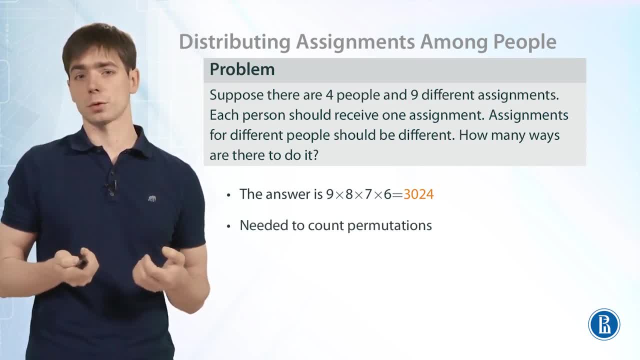 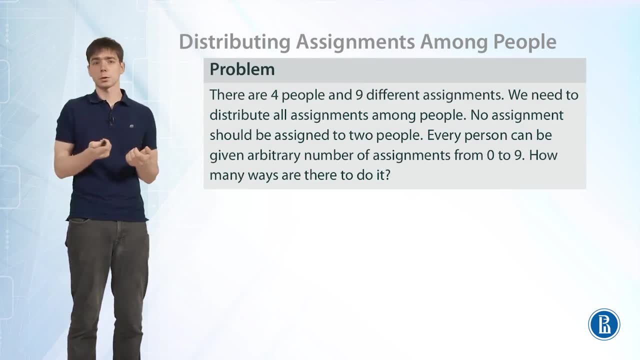 simple: We needed just to count permutations. The main difficulty was to understand that we need to count permutations. Now let's proceed to the next problem. Again, we have four people. Again, we have nine different assignments. Now we would like to distribute assignments between people, So each 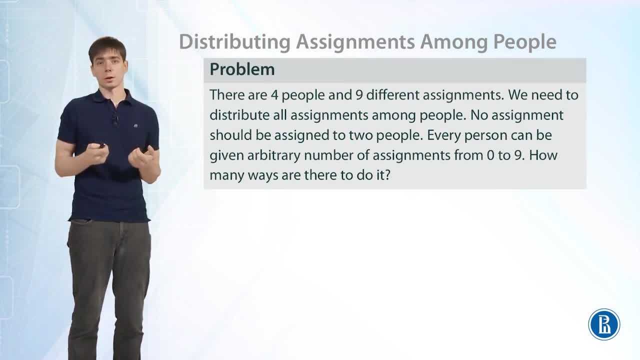 assignment should be assigned to one of the persons, and every person can receive arbitrary number of assignments, from zero to nine. How many ways do we have to do it? Okay, now, the difference is that the person receives several assignments in this problem. Let's try to solve this problem and we can try to look at. 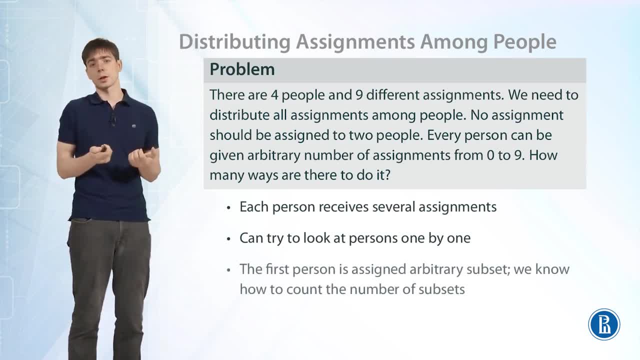 persons one by one. Okay, the first person is assigned an arbitrary subset of assignments. We know how to count the number of subsets. We have done this before. But if you look at the second person now, the number of options left for him depends on what we have chosen. 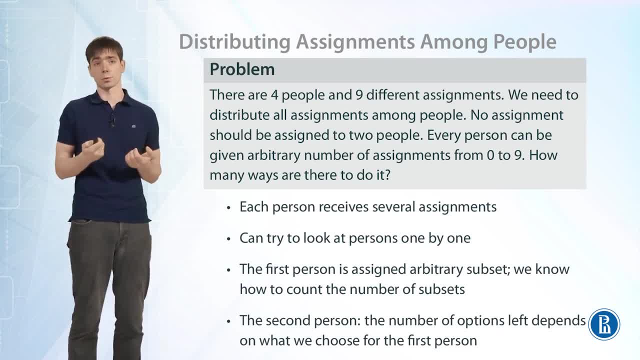 for the first person, how many assignments we have given to the first person. So now counting the number of options for the second person looks problematic. Okay, the problem seems tricky and we need some idea. And we have this idea. The idea is the following: 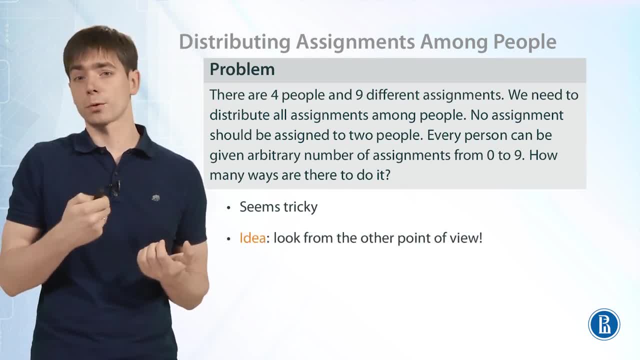 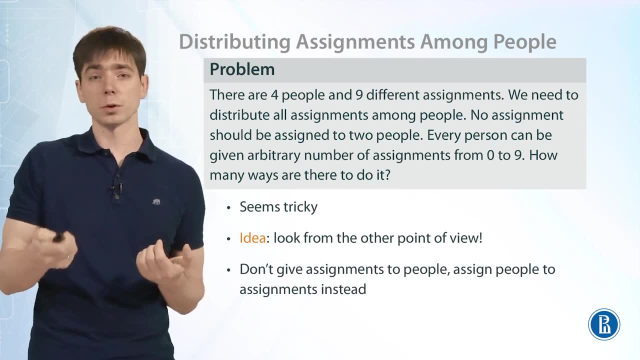 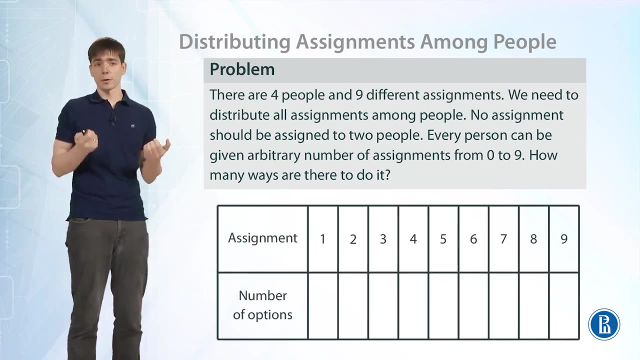 Let's look at this problem from the other point of view. Let's not give assignments to people, Let's assign people to assignments. Let's look from the position of assignments And then everything looks simple. So we have nine possible assignments and let's see what. 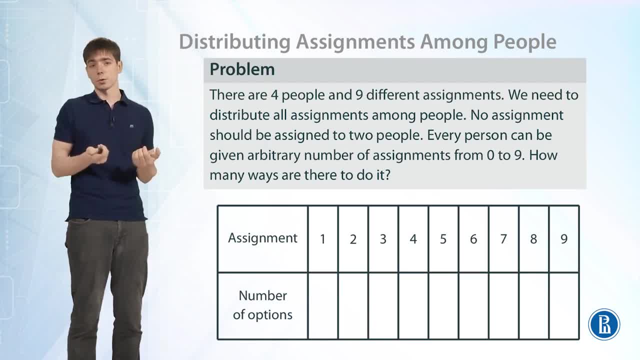 options do we have for each assignment? For the first assignment we have four options we can assign to any person. Let's look at this problem from the other point of view. Let's not give assignments to one person. For the second the same, And for the third one, And so on. So each assignment. 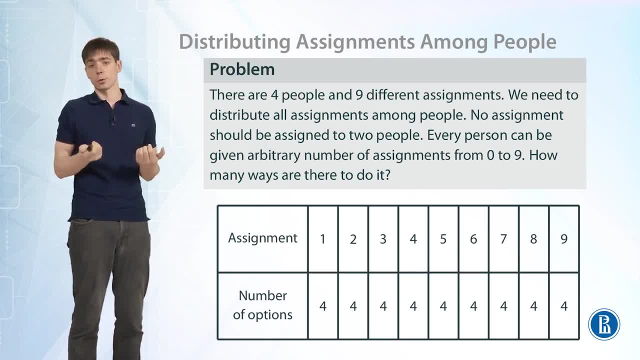 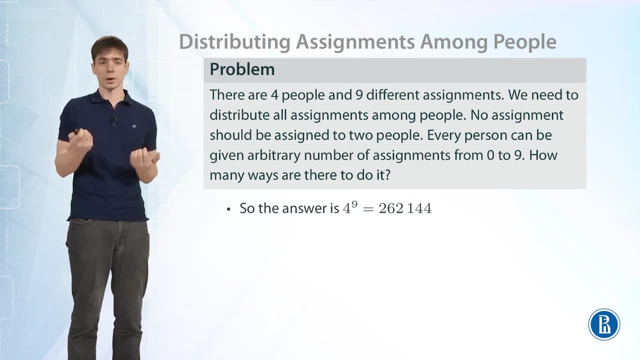 can be given arbitrarily to one of four persons. So in total we have four times four times four and so on, Nine times four to the nine, 262,144 possible ways to do it. And note that in this problem we just needed to count tuples. It turned out to be very simple. 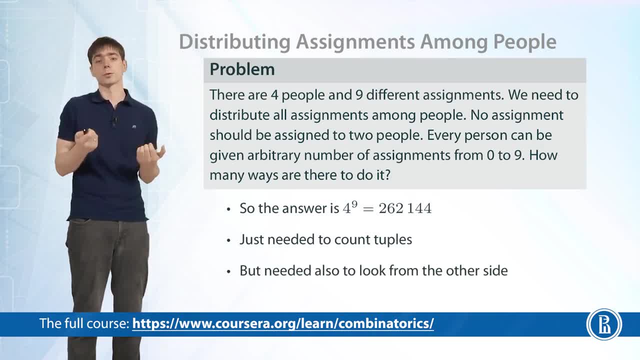 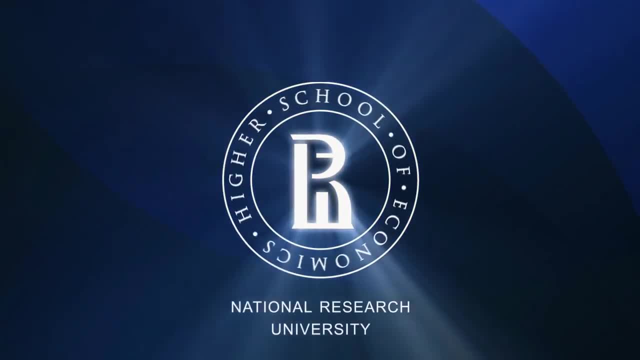 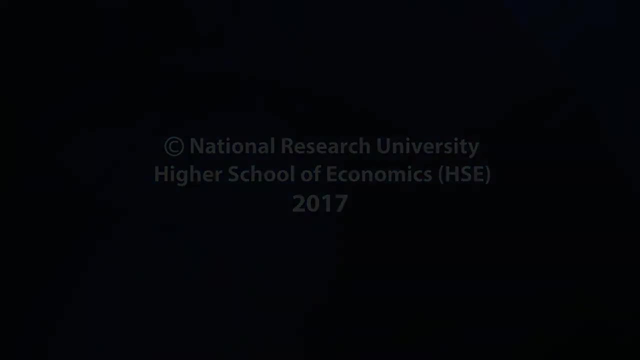 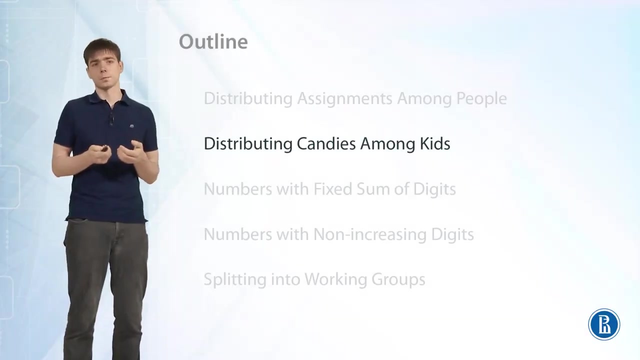 But it looked hard in the beginning, so we also needed to switch to the other point of view. Let's consider the following problem: We have 15 identical candies And we'd like to distribute them among seven kids. We'd like to make five babies. As a very simple example, we make 15 identical candies. We'd 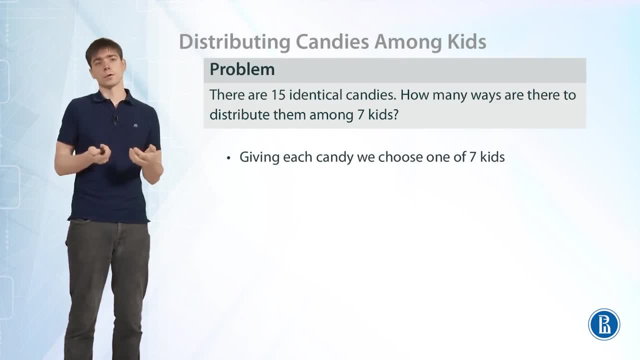 still like to make four babies, But let's see what we can bring them to the bag, Not How many ways do we have to do it. Let's look at the problem in the following way: Each time we give a candy, we choose one of seven kids. 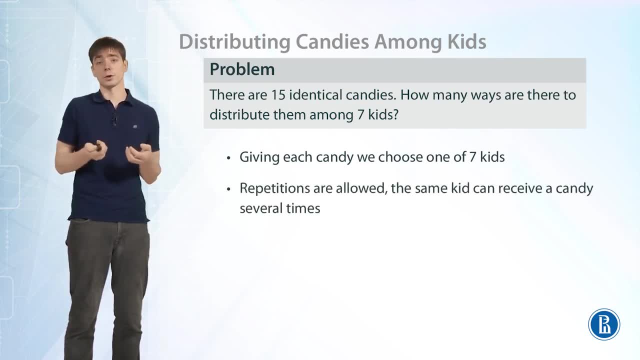 Okay, repetitions here are allowed. The same kid can receive more than one candy And in fact this is unavoidable. There are 15 candies and just only seven kids Candies are identical, so the order doesn't matter If some kid receives the 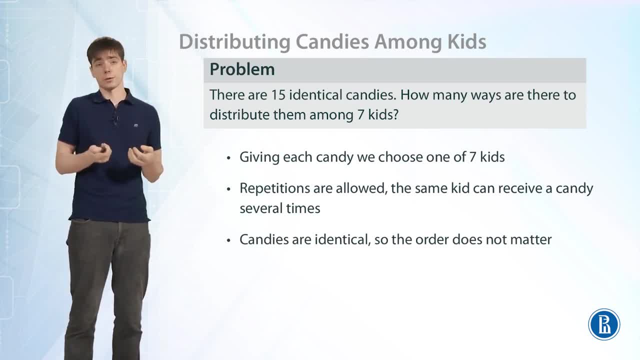 first candy or the second one, or the third one, it doesn't matter, They are all the same. so we don't care about the order here. So we are dealing with combinations, with repetitions. Order doesn't matter, Repetitions are allowed, And here the number of candies is the size of a. 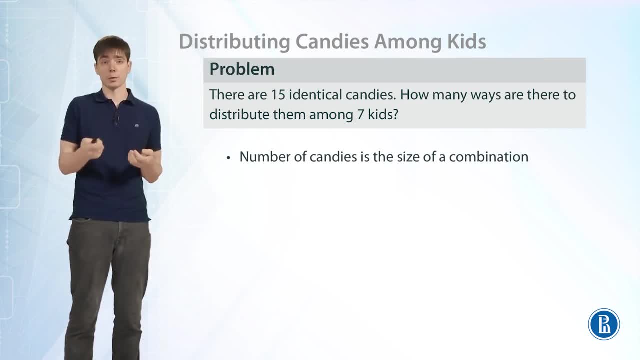 combination. So each time we give a candy, we pick one of the kids. So the size of our selection is 15.. And the number of kids is the number of our options. Each time we give a candy, we pick one of seven options, One of seven. 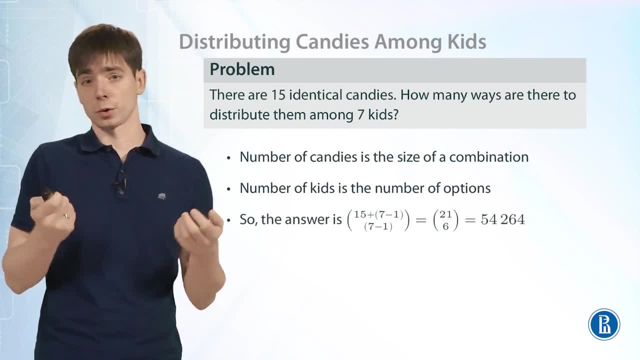 kids. So the answer here is obtained by a formula we already have. It's 15 plus 7 minus 1. choose 7 minus 1.. Which is 21, choose 6,, which is 54, 264.. Okay, Now let's consider a. 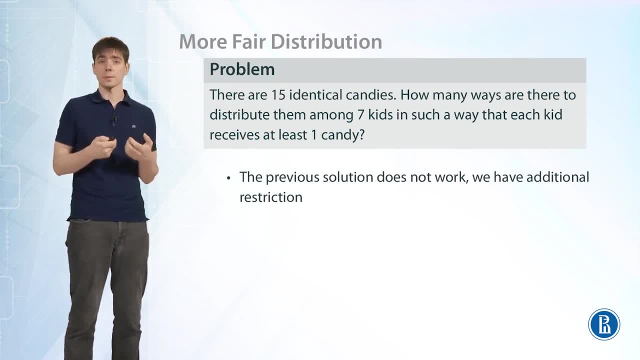 similar problem. Again, we have 15 identical candies. Again, we would like to distribute them among seven kids. but now we would like to do it in a more fair way. We would like each kid receives at least least one candy. Okay, the previous solution doesn't work, because now we 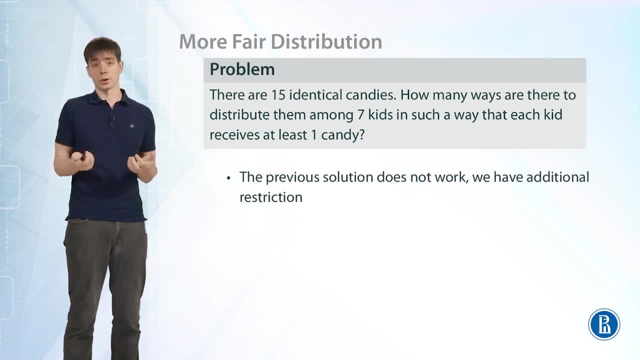 have an additional restriction. There are less combinations here and we have to do something else. The previous solution doesn't work directly, Okay, but so what we can do. It turns out that we can reduce the problem to the previous one. How we can do it? The idea is the following: We know we have a 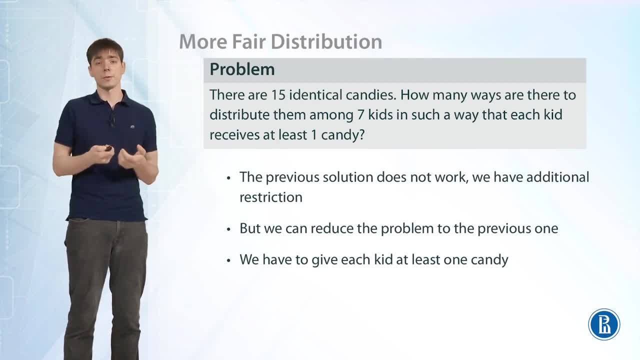 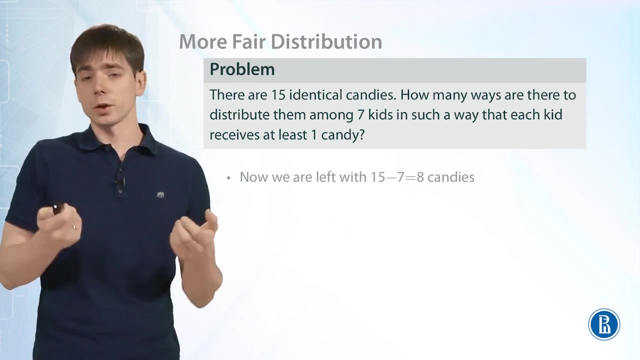 restriction that each kid has to receive at least one candy. so let's just do it. Let's just give each kid a candy and then proceed to give our candy, But let's just give each kid one candy and see what's left Now we are left with 15 minus 7, which is 8 candies, and now we have to. 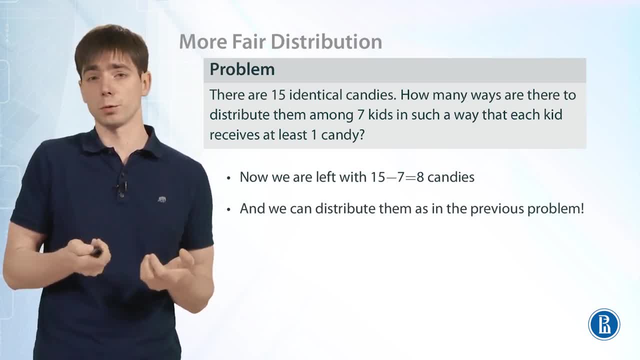 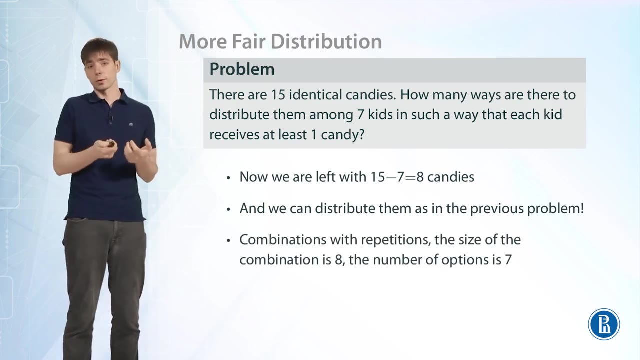 distribute them in the same way as in the previous problem. We've already satisfied our restriction. We've already given each kid one candy. We are left with 8 candies, and we have to just apply the same argument as in the previous problem. So again we have combinations with repetitions, but now the size of the combination is 8.. 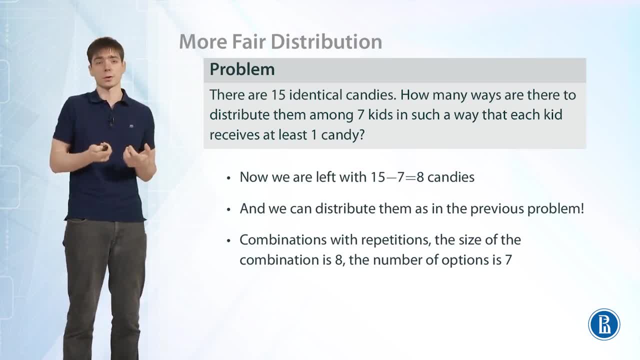 This is the number of candies that is left after we gave each kid a candy And the number of options. the number of kids is 7.. So the answer here is 8 plus 7 minus 1. choose 7 minus 1, which is 14,. choose 6,, which is. 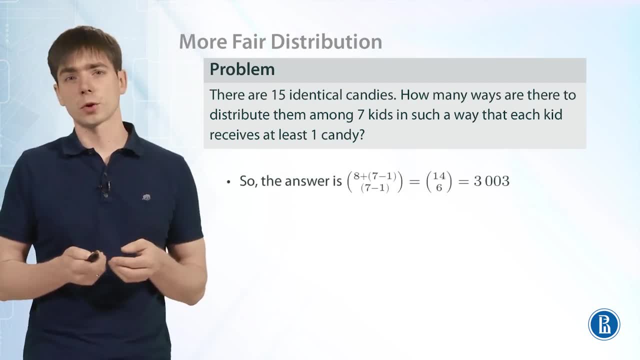 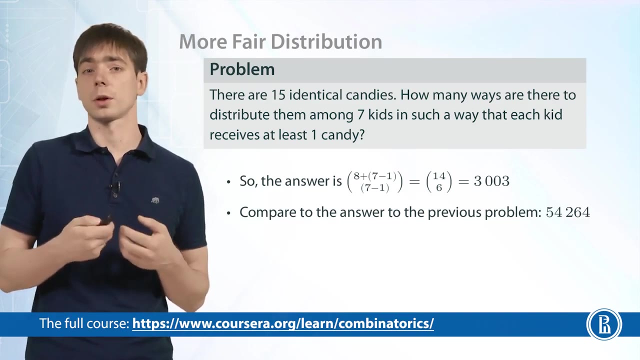 3,003.. It is interesting to compare the answer to this problem with the previous one. So here the answer is 3,003 and in the previous problem the answer was 54,264.. So there are a lot of ways to distribute candies between 7 kids. 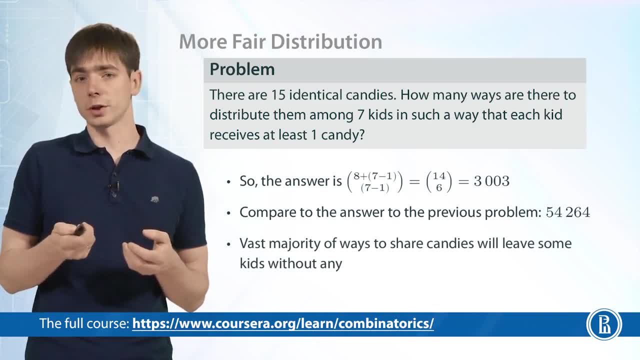 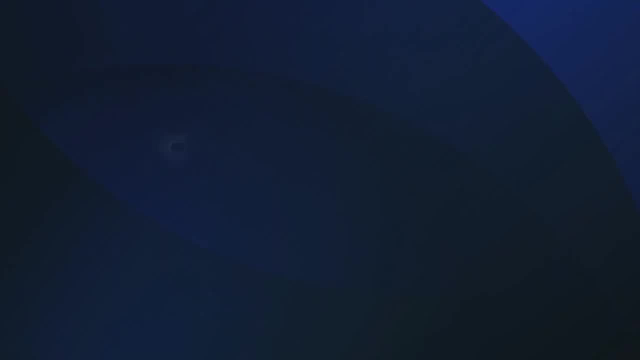 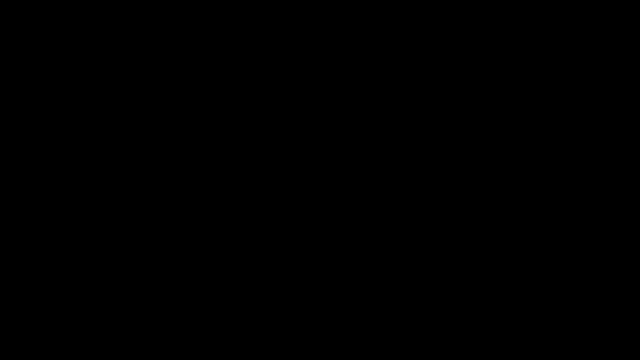 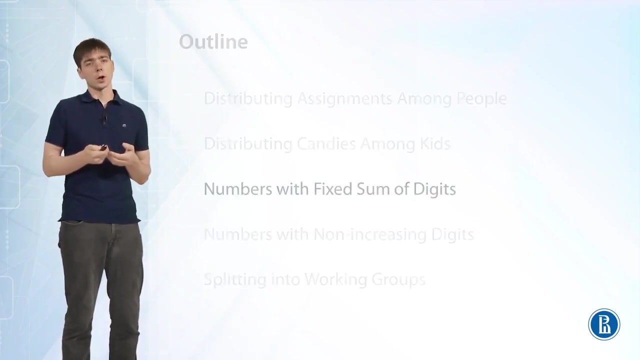 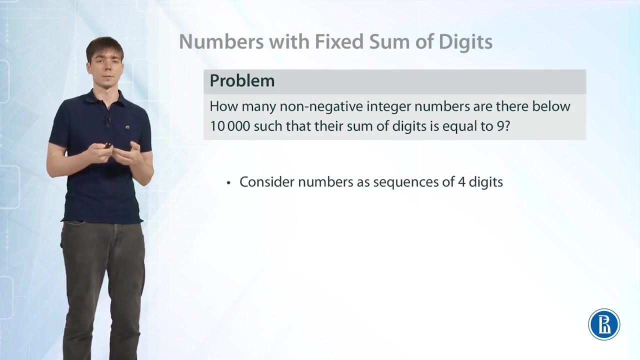 And only in a tiny fraction of them, each kid will receive at least one candy. Now let's consider the following problem: How many non-negative integers below 10,000 do we have, such that the sum of their digits is equal to 9?? 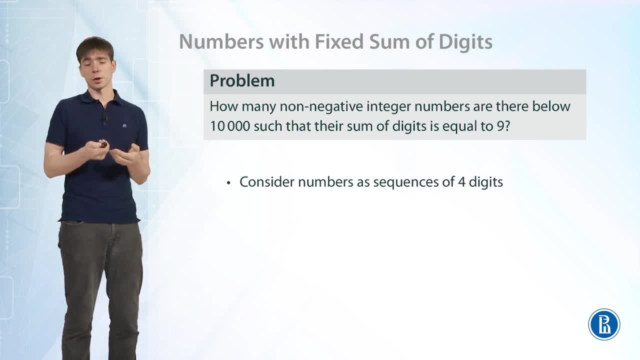 Okay, We can consider numbers below 10,000 as sequences of 4 digits and we can try to look at this problem. Let's consider the position of numbers. We can try to see how many options do we have for the first digit, for the second digit? 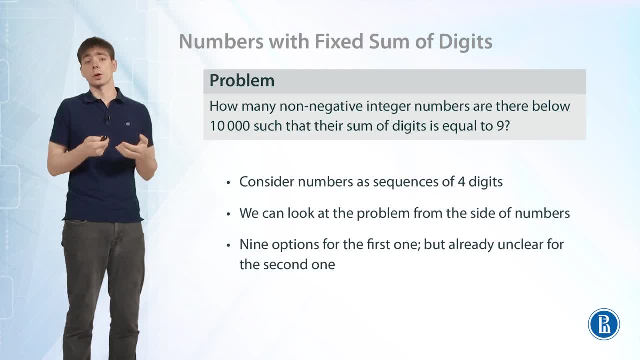 and so on. So for the first digit we have 9 options, But already for the second one this is unclear. If the first digit is, for example, 9,, then there is just one option for the second digit. If the first digit is 0,, then there are 10 options for the second digit. 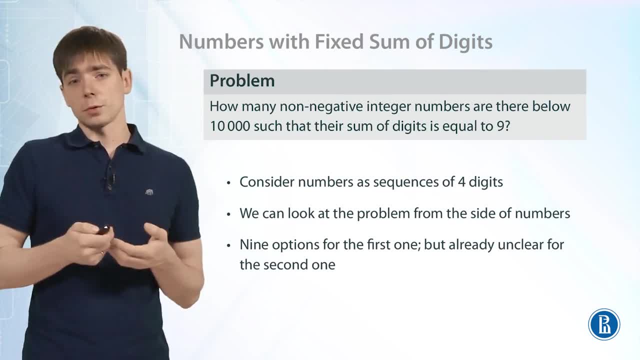 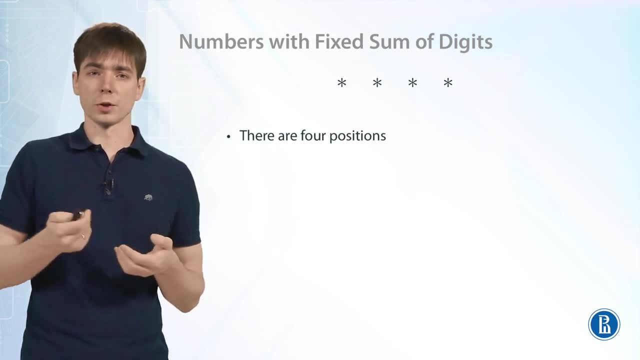 So this is unclear. This approach doesn't seem to work And instead we can try to do the following. Here is the idea. Let's look from the other side again. Okay, We have 4 positions and we would like to distribute weight 9 among them. 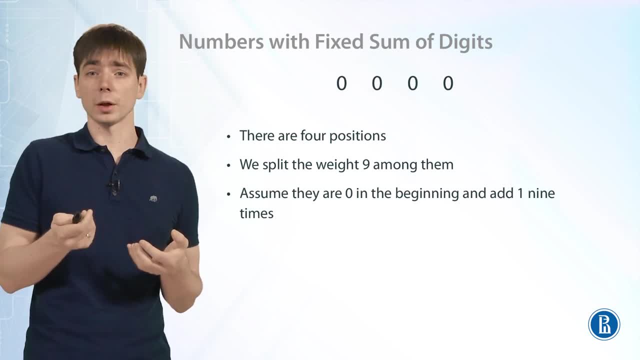 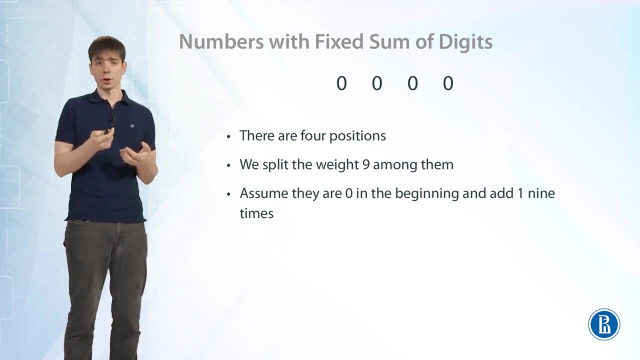 So we assume that initially, in the beginning, all positions are 0, and then we add 1, 9 times, And this way we will obtain all possible 4-digit combinations with sum of digits equal to 9.. Okay, Uh, Order doesn't matter. 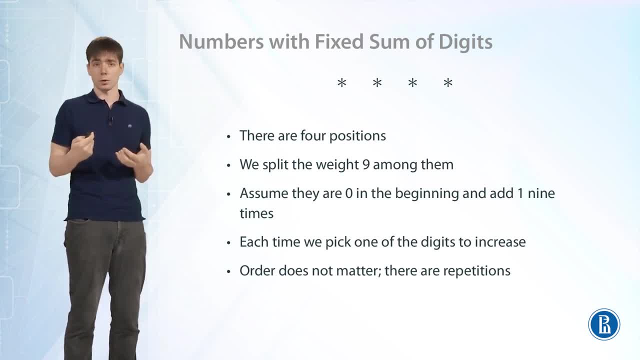 So if we add 1 to some position on the first step and on the second step, it doesn't matter. So we still add 1 to the same position. Also, repetitions are allowed. So here we are dealing with combinations with repetitions of size 9 among 4 options. 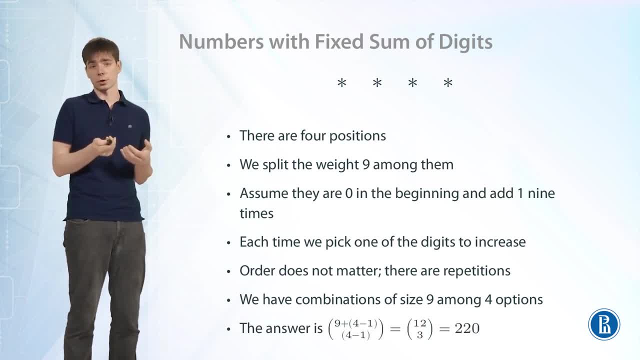 Okay, And we know how to count them. The answer is 9 plus 4 minus 1.. We have 4 options, so we have 4 minus 1 here. 9 plus 4 minus 1. choose 4 minus 1, which is 12. choose 3, which is 220. 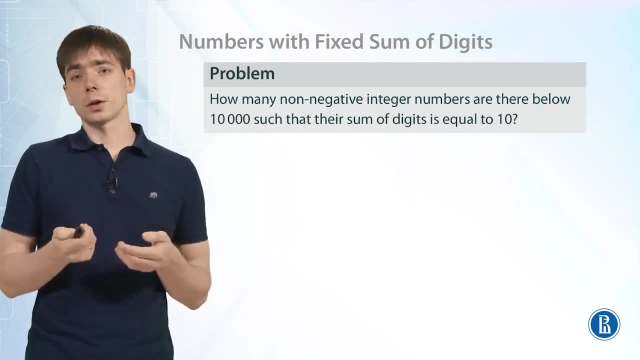 Now let's proceed to a very similar problem. How many non-negative integer numbers do we have below 10,000, such that the sum of their digits is equal to 10?? In the previous problem we had 9.. Now the sum is equal to 10.. 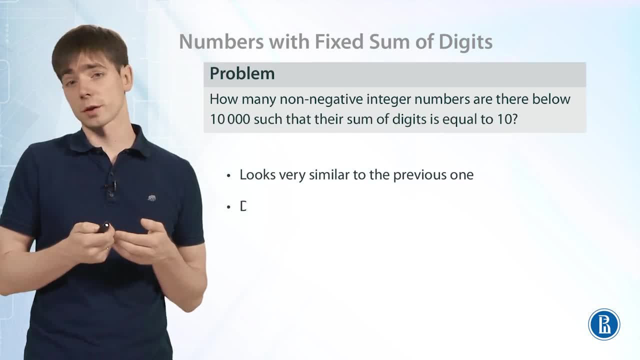 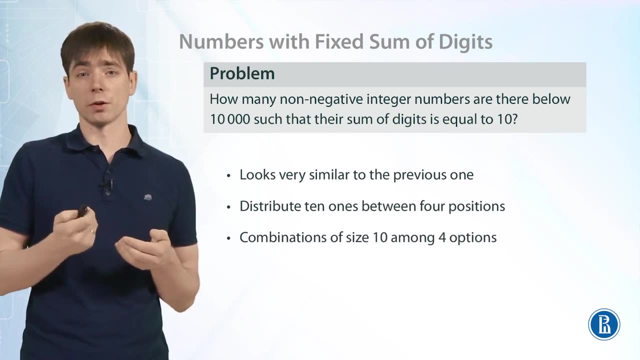 The problem looks very similar to the previous one, So probably we should just try the same approach. Now we have to distribute 10 ones between 4.. Again, we have combinations with repetitions of size 10 among 4 possible options And the answer is 10 plus 4 minus 1. choose 4 minus 1, which is 13. choose 3, which is 286. 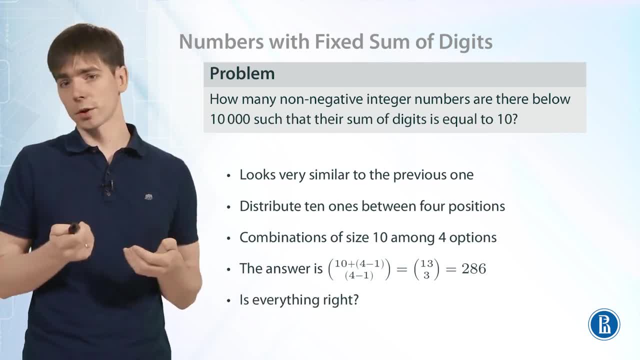 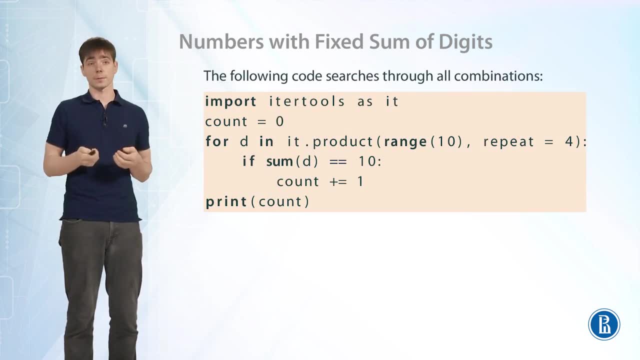 Okay, Is everything right? So have we done everything correctly? So let's just check. Let's count all of these combinations directly. So for this we can just run the following code: This combination is equal to 10.. This code goes through all 4-digit combinations and increases the counter if the sum of all 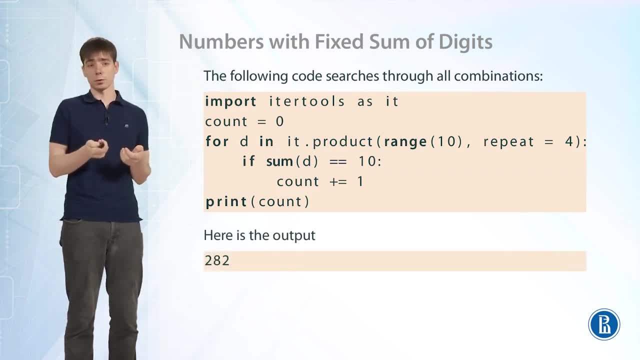 digits is equal to 10.. And if we run this code, we obtain the following result: 282, which is not equal to our answer. Our answer was off by 4, not by 4, factorial, by 4 exclamation mark. So what went wrong? 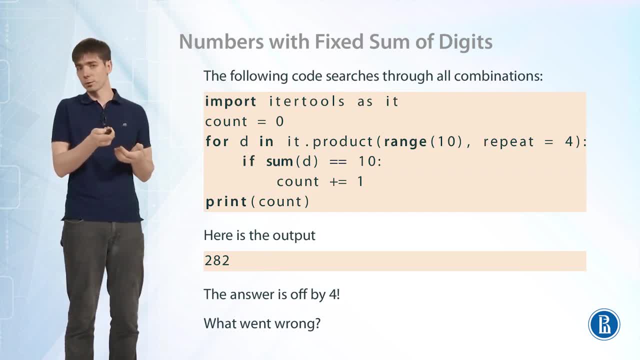 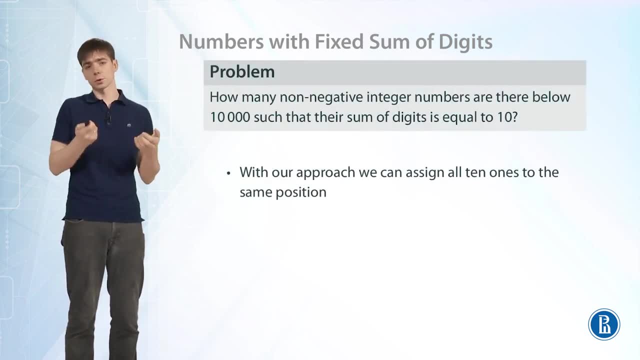 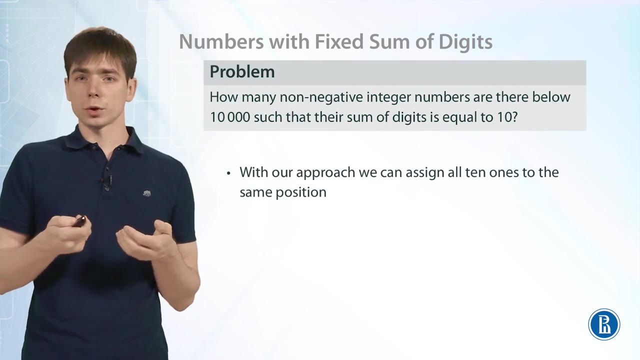 What we have done wrong, What happened This code we have from comparing this code to our solution, And it is not hard to see if we know that there is a problem, it is not hard to see where it is. When we applied our approach, we also counted the following: 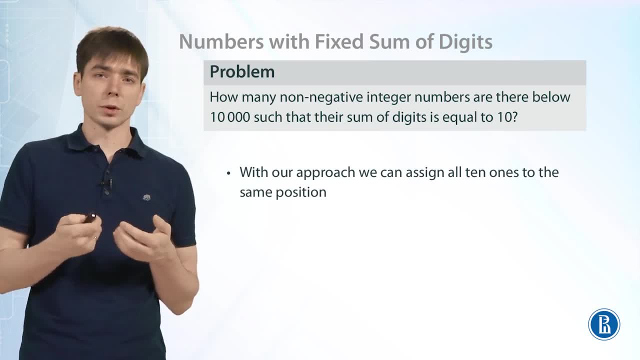 We counted cases in which we assigned all 10 ones to the same position, And this is not allowed in digits. Digits ranges from 0 to 9.. So we shouldn't have counted this. So what should we do next? What should we do now? 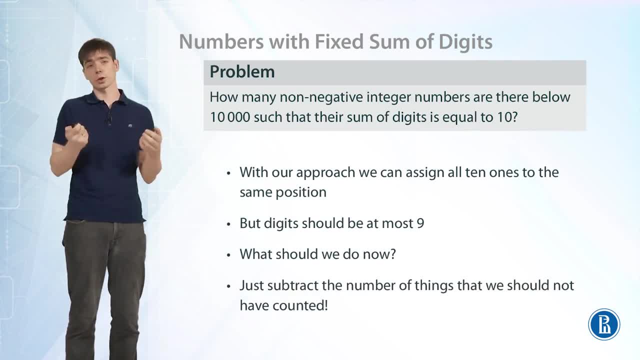 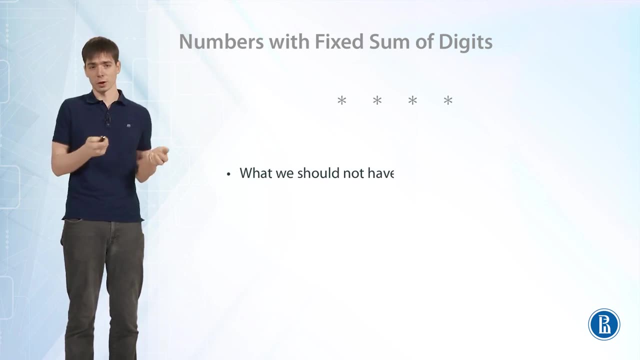 The idea is simple. We can just fix our old solution. Let's just subtract the number of things we shouldn't have counted. Let's count them. Let's count the wrong combinations we had before and let's subtract them. What exactly we shouldn't have counted? 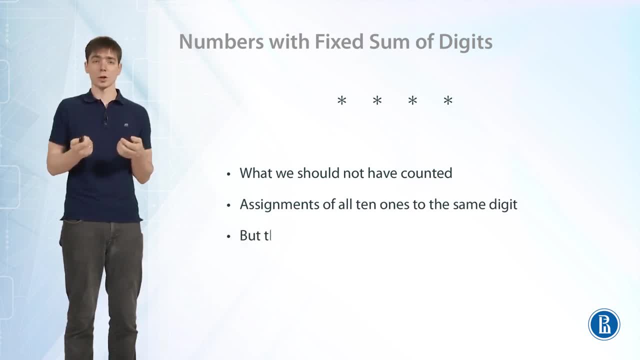 We shouldn't have counted assignments of all 10 ones to the same digit. And what should we do next? What should we do next? There are just four of them. We can assign all 10 ones to the first position, to the second one, to the third one and to: 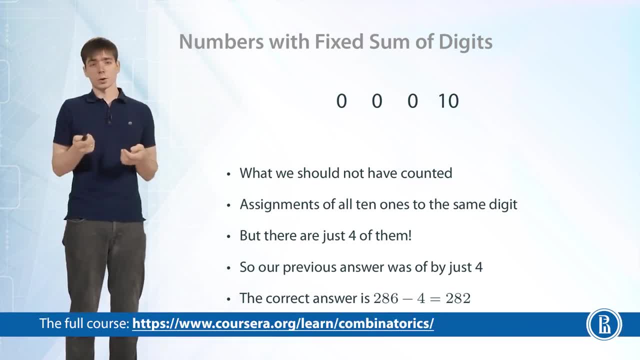 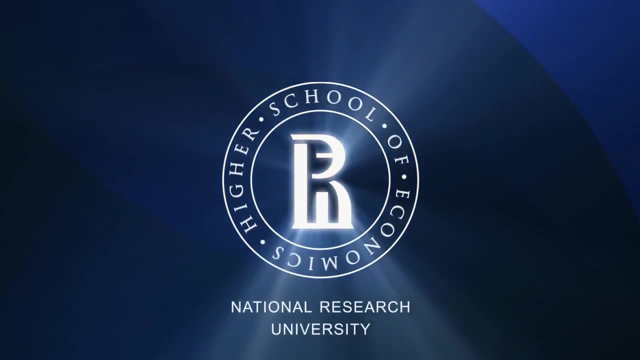 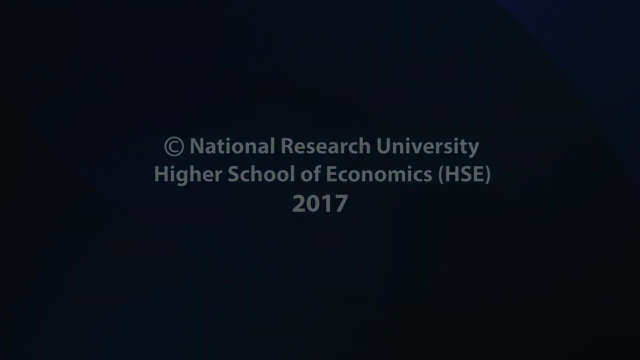 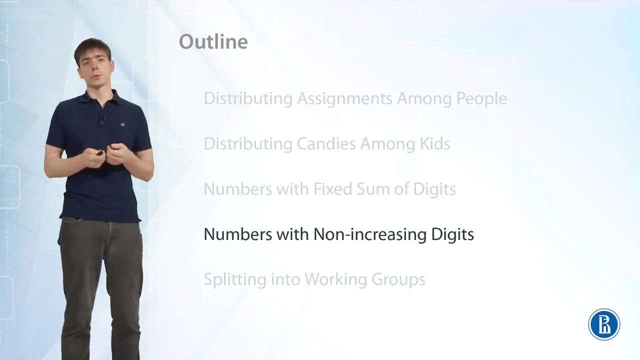 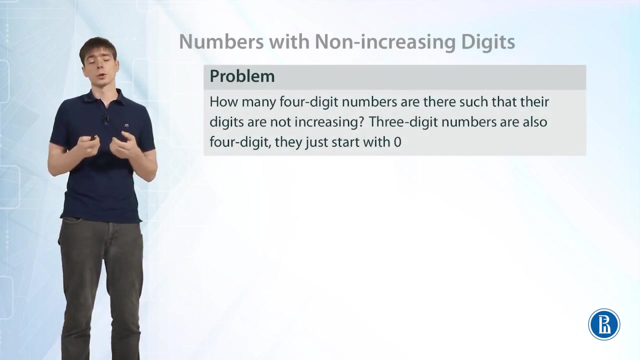 the fourth one. So there are just four of them, and the correct answer to this problem is 286 minus 4, which is 282, which now coincides with our experiment. Let's consider the following problem: We would like to count how many 4-digit numbers do we have, such that their digits are not? 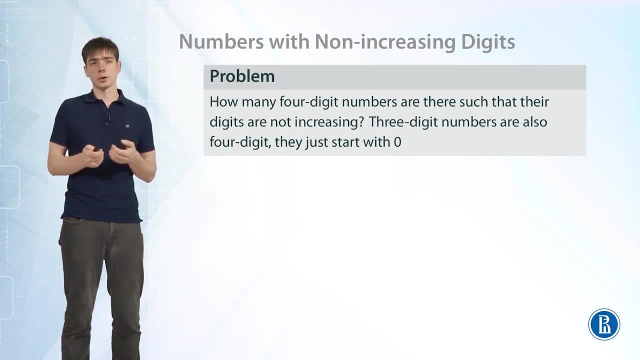 increasing from left to right And in this problem we assume that 3-digit numbers, 2-digit numbers, 1-digit numbers are also 4-digit numbers. We just start with 0.. Okay, We can try to look from the side of positions. 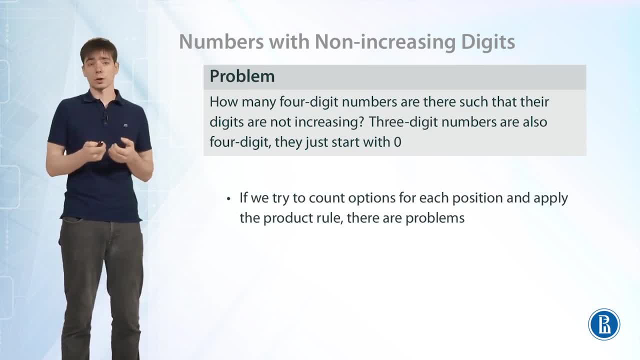 Let's start with 0.. Okay, Let's try in the numbers. We can try to count options for each position and then apply product rule to solve this problem, But it turns out to be complicated. This approach doesn't work. We have 10 options for the first position, but if we already consider the second position, 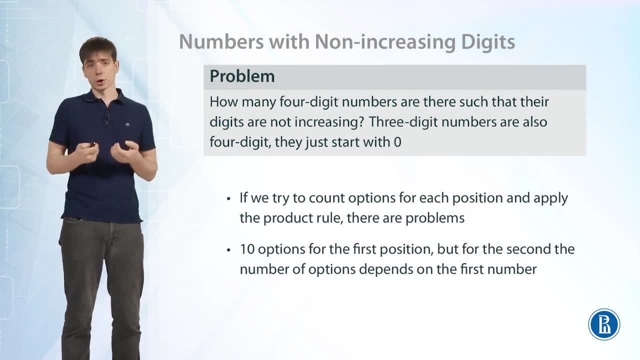 since the number there should be at most the number in the first position. the number of options depends on what we have chosen for the first position. So this approach doesn't work And we have to do something else. And the idea is again to look from the other side. 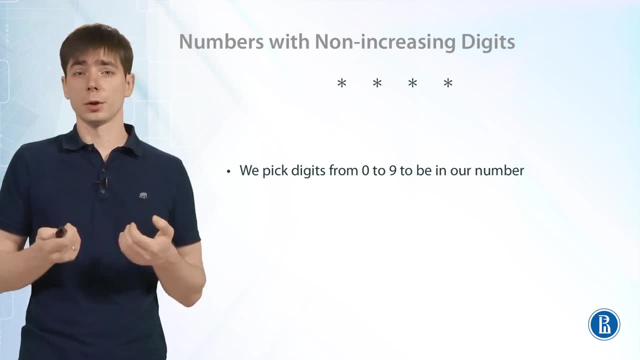 Okay, Again, we have 4 digits and we pick digits from 0 to 9 for each position. And okay, Note that once we picked 4 digits to place to these positions, our number is uniquely determined. Indeed, Suppose we have picked 4 digits. 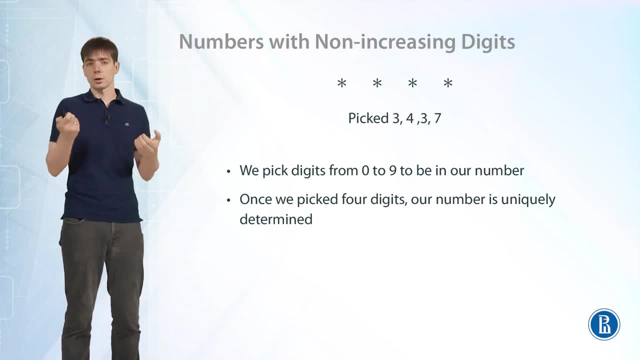 3, 4, 3, 7.. Then we can position them in this position And we have to do something else, And the idea is again to look from the other side. Okay, So we can position them in these 4 digits in a unique way. 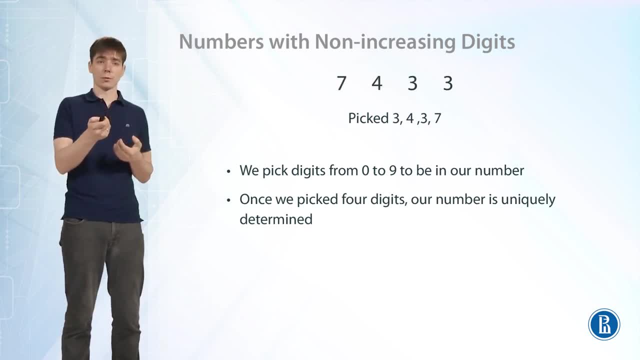 We can place 7 only on the first place, 4 only on the second place and then 3 and 3.. The reason is that the digits in the number should not increase, So there is a unique way to place 4 digits in our positions. 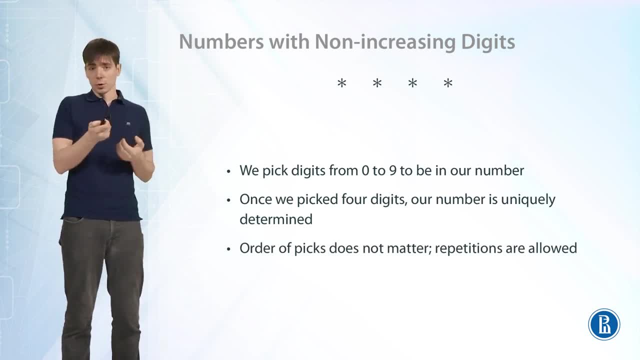 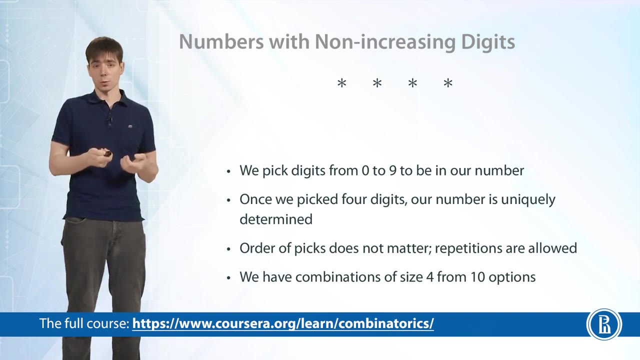 And note that order of the picks doesn't matter. So anyway, we will have to reorder numbers And repetitions are allowed. So again, we are dealing here with combinations with repetitions of size 4 from 10 options. So we need to pick 4 numbers from 0 to 9.. 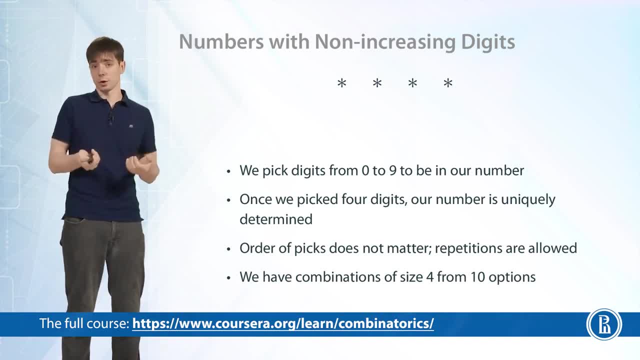 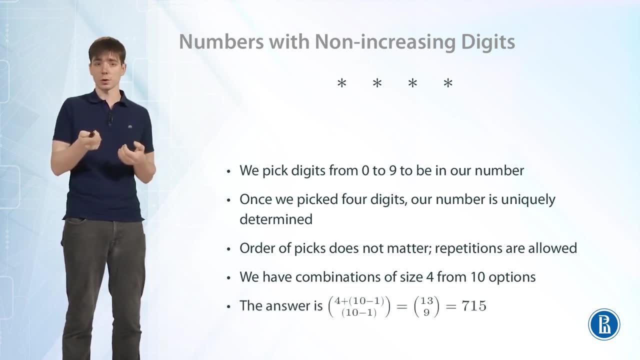 And the order doesn't matter And we allow repetitions. Okay, And the answer is known to us. The answer is 4 plus 10 minus 1.. Choose 10 minus 1, which is 13.. Choose 9,, which is 715.. 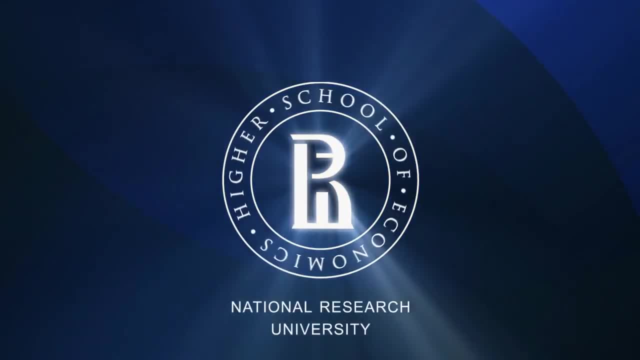 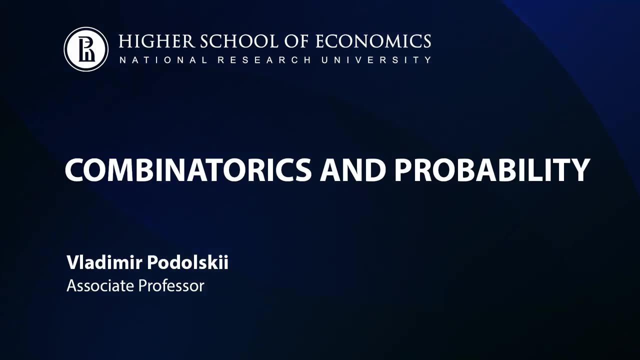 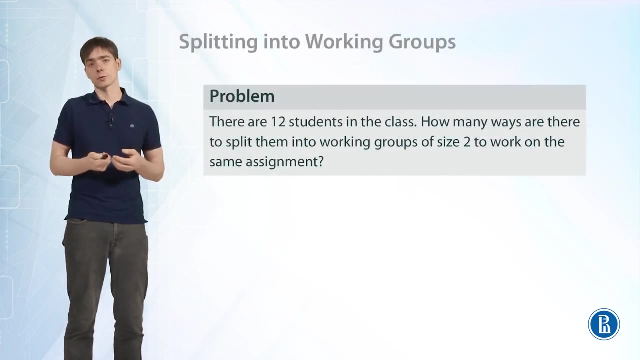 Choose 0. And if the answer is no, then we need to apply the same rules ourselves. Consider the following problem: We have 12 students in the class and we would like to split them into working groups of size 2 to work on the same assignment. 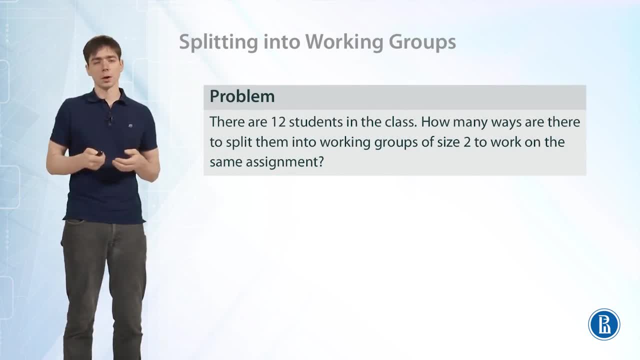 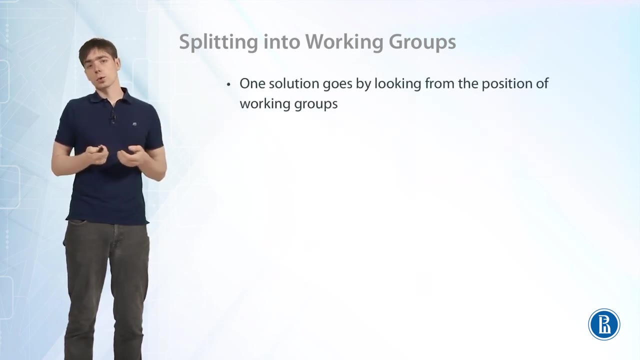 How many ways do we have to do it? Okay, This problem is more tricky than previous problems. There are several ways to solve it, But anyway, we need to combine several ideas we had before. Okay, One of the solution goes by looking from the position of working groups. 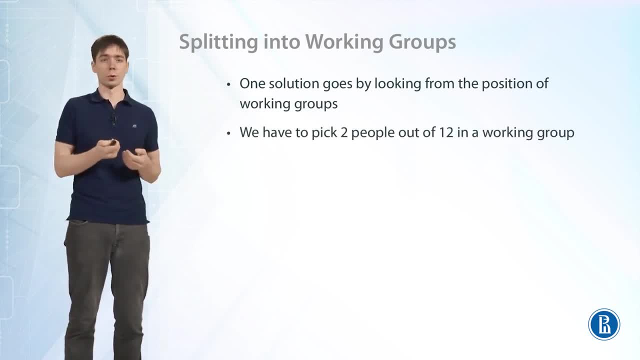 We have to pick. Let's just pick the first working group. We have to pick two people out of twelve into the first working group, And order in the group doesn't matter. So we are dealing with combinations. So there are twelve. choose-two ways to do it. 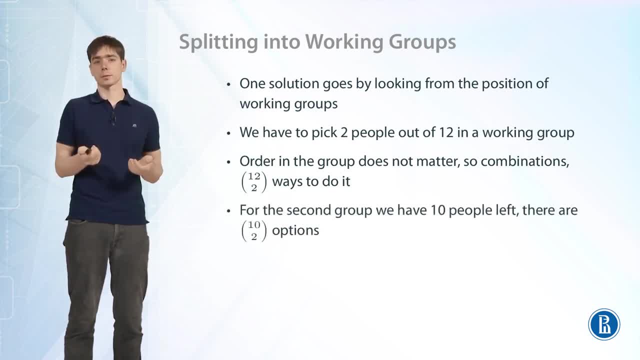 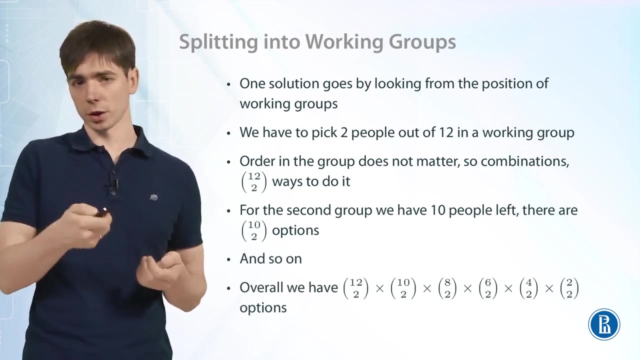 Okay, Now let's proceed to the second group. We have ten people left, And again the order doesn't matter, Again combinations, and there are ten choose-two options there, And so on. If we go through all of the groups and each time we have to. 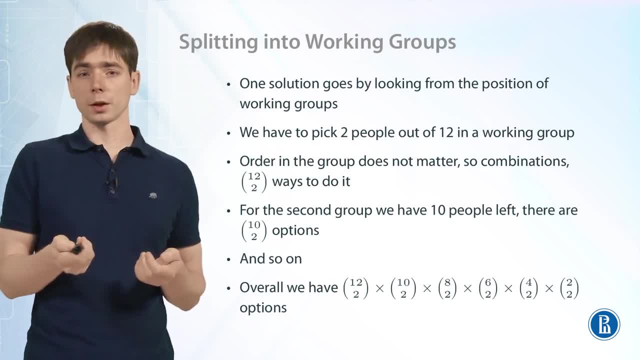 So in total, we have to multiply options for each group. Then we have twelve choose-two times ten, choose-two times eight, choose-two times six, choose-two times four, choose-two times two, choose-two options. Okay, So we obtain this. Is this all? Are we done? 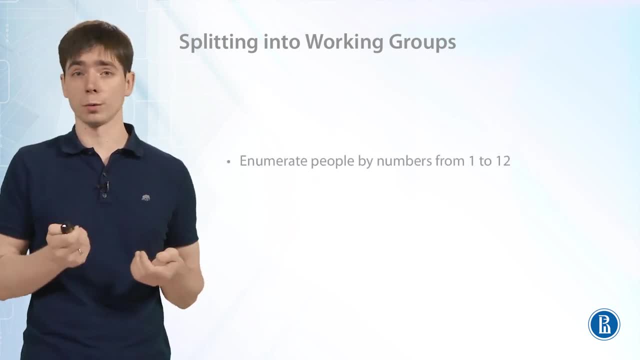 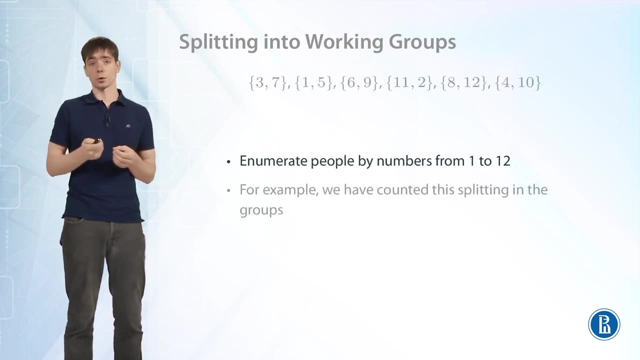 It turns out that no, we are not. And let's see what is the problem. Let's, for our convenience, enumerate people by numbers, from one to twelve, And let's consider, for example, the following splitting into groups. Here is the first group, of size two, then one and five, the second group, and so on. 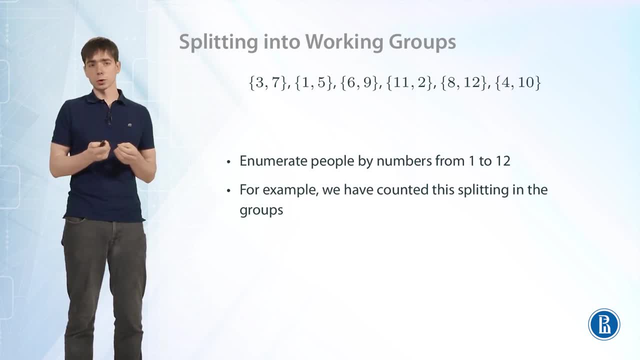 And we have counted this splitting And we have counted this splitting into groups, but also we have counted this splitting into groups separately And note that the difference is only in the first two groups. They are just switched between each other. But note that the order between groups doesn't matter, It's still the same splitting into groups. 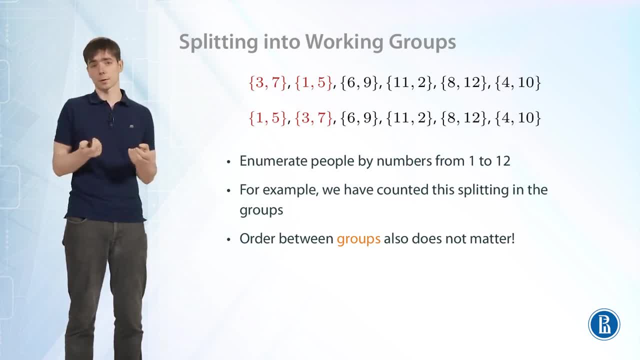 So we have counted the same splitting into groups twice. Okay, our solution is wrong. So what do we have to do now? Should we start from the beginning? Okay, it turns out that we do not have two. We can just figure out the order. And then we have the same splitting into groups twice. 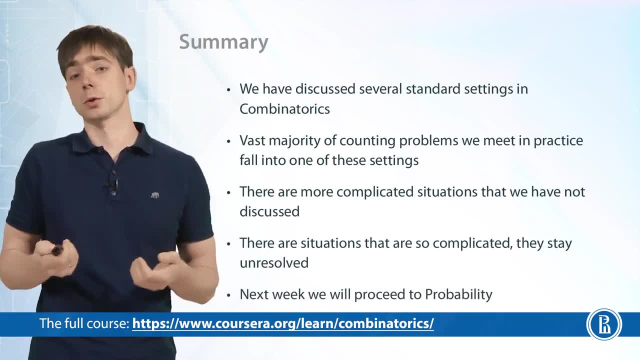 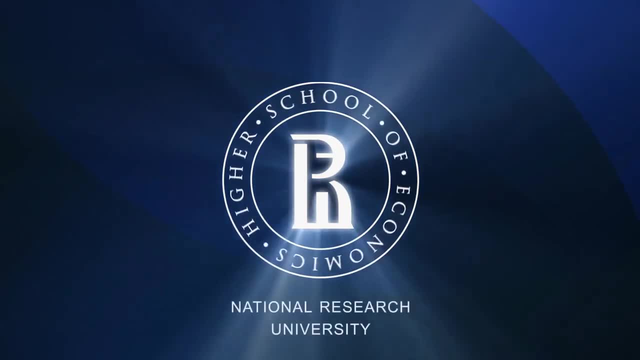 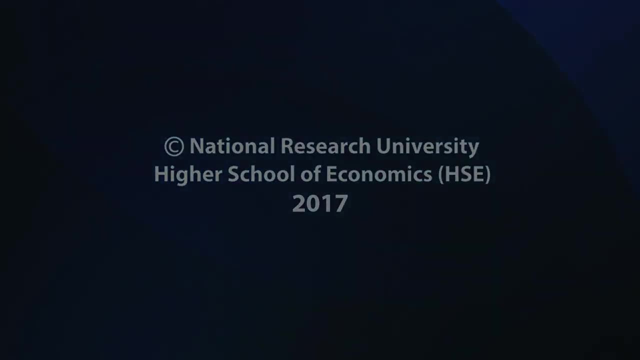 We can just figure out the order And then we have the same splitting into groups twice. Next week we will proceed to probability, where, in particular, we will need the knowledge we obtained in combinatorics. We start this part of our course devoted to probability theory. 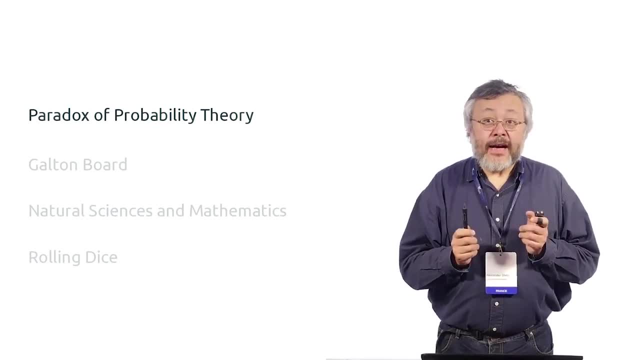 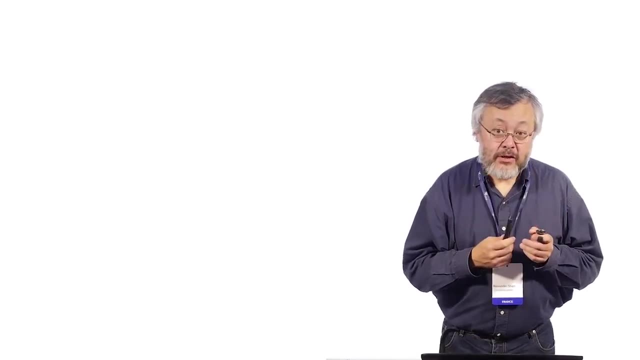 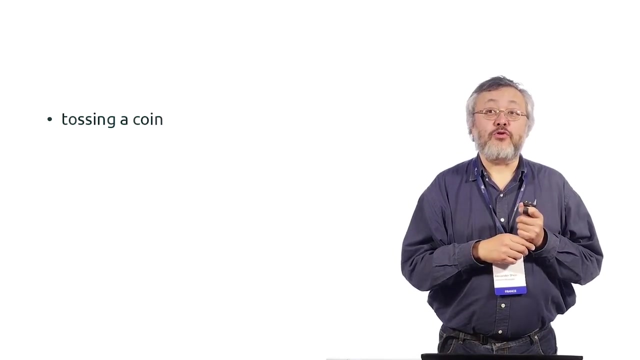 And I would like to start with some general remarks. Actually, probability theory is rather strange. Actually, probability theory is rather strange. It tries to predict the unpredictable. So, for example, a standard object of probability theory is coin tossing. So imagine you go to a restaurant. You want to decide who will pay. 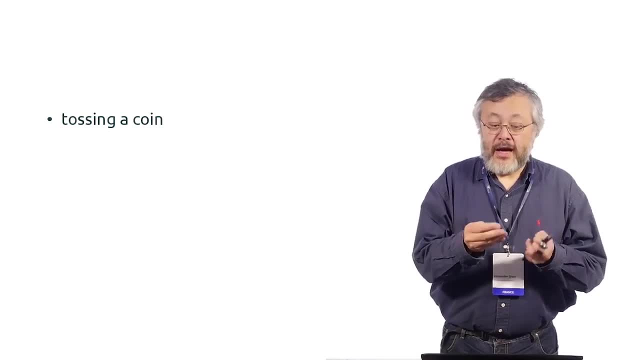 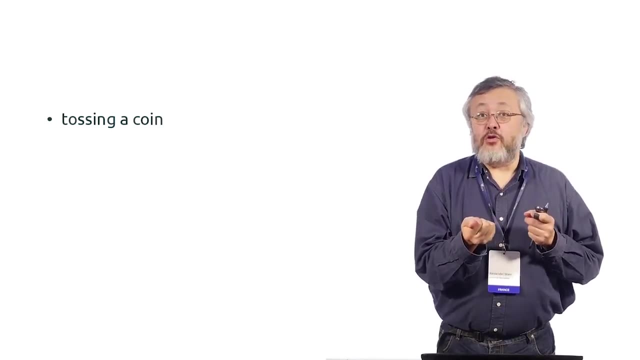 And so if you, you can take a coin and toss the coin, And then you the idea that nobody can predict this. So somehow you don't know in advance who will pay. So somehow you don't know in advance who will pay. 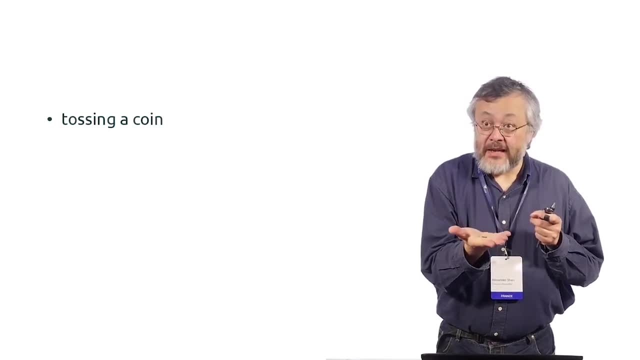 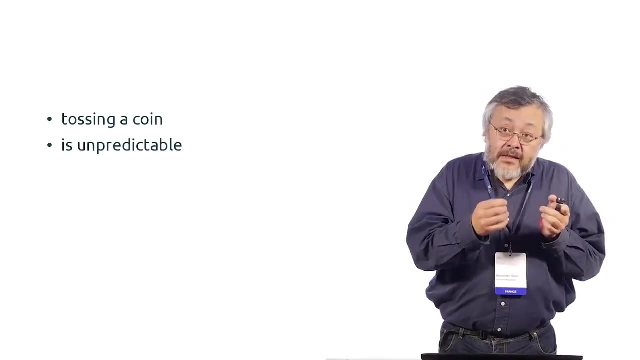 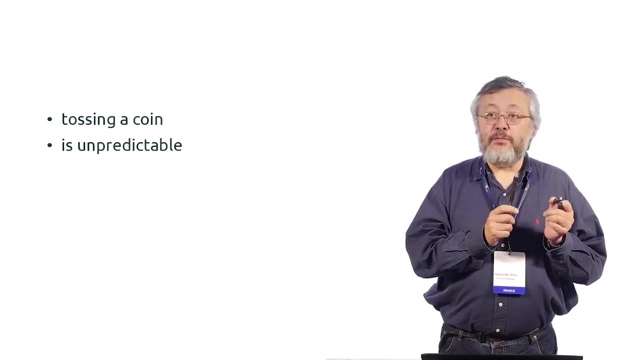 somehow equal chances to pay. So you see that this is tail and then you decide who pays And the idea still the idea of probability theory, somehow, that you can predict. you can something, predict something about the coin tossing. Let me explain. So imagine we do not. 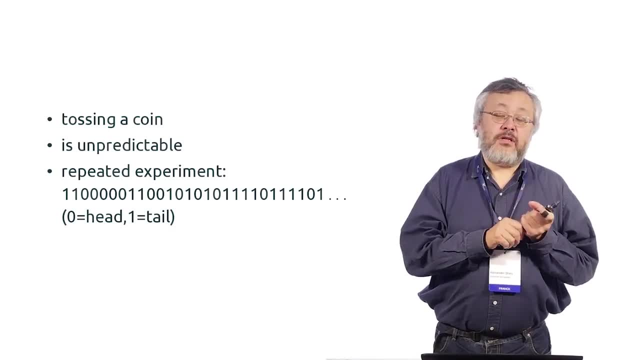 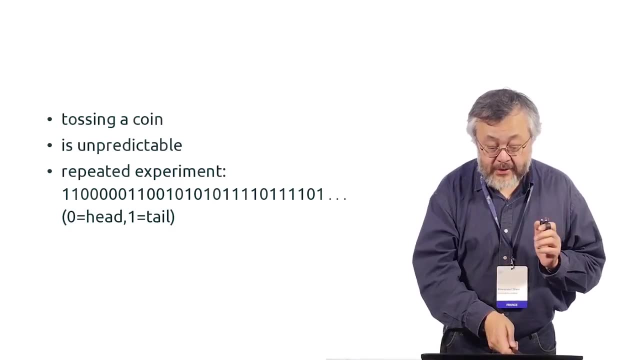 the one coin tossing, but many of them. So we toss it many times and we record the results. For example, if one is tail and zero is head, here is this tail, tail, head, head, head, head, head, and so on. 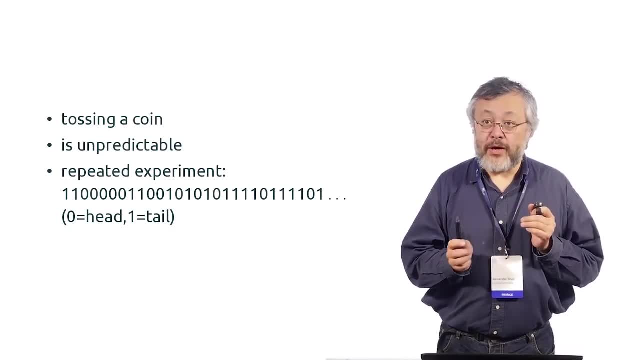 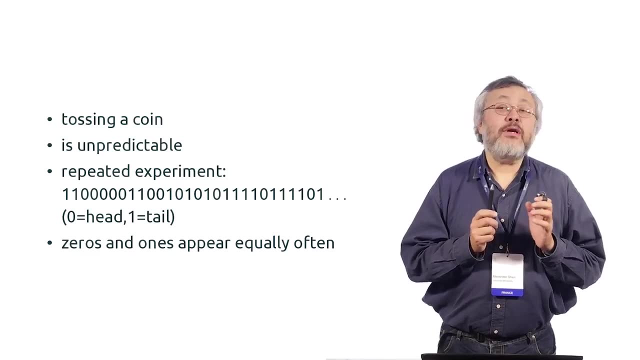 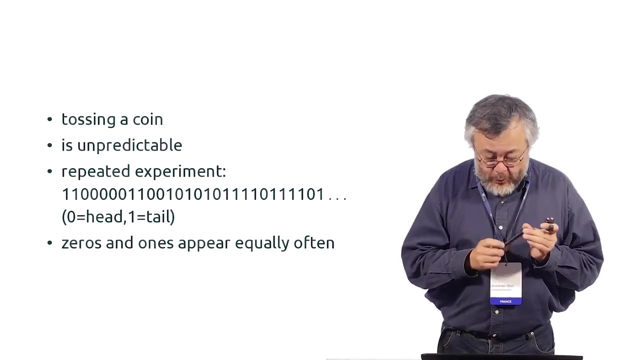 So we can count how many heads and tails we have in this sequence And it turns out that usually zeros and ones appear equally. not exactly equal equal number of zeros and ones, But actually they are quite close. So let's look at this example. We have one, two, three, four. 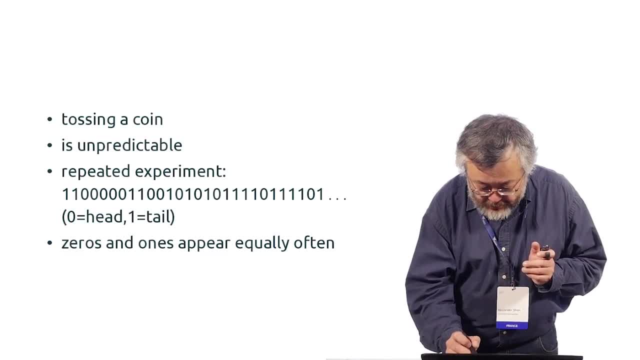 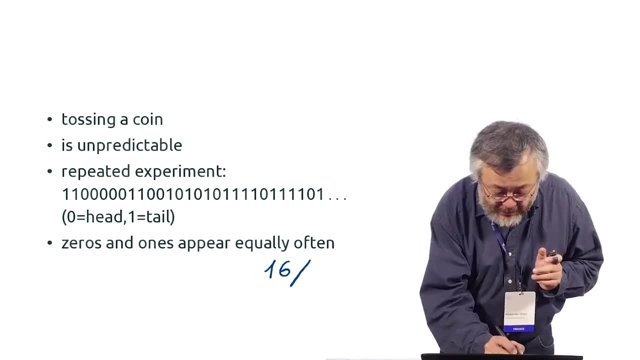 five, six, seven, eight, nine, ten, Eleven, twelve, thirteen, fourteen, fifteen, sixteen- Hopefully I am correct- but sixteen- And the total number is one, two, three, four, five, six, seven, eight, nine, ten. 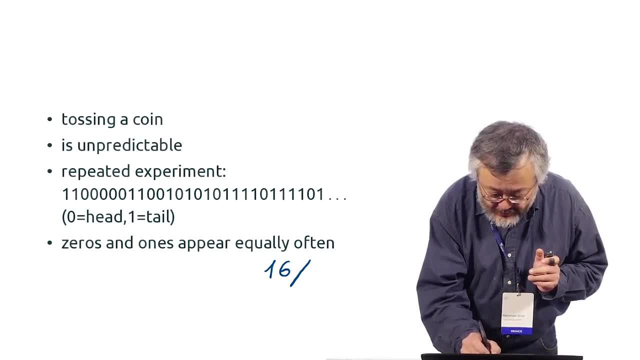 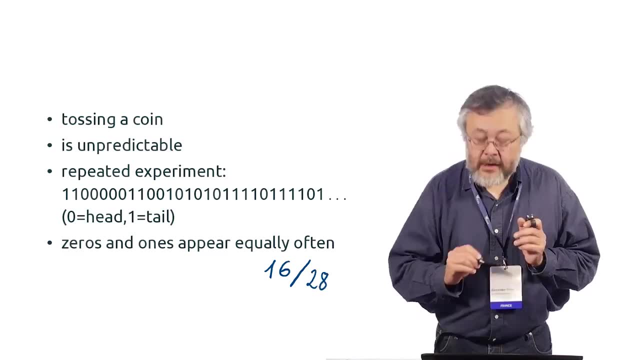 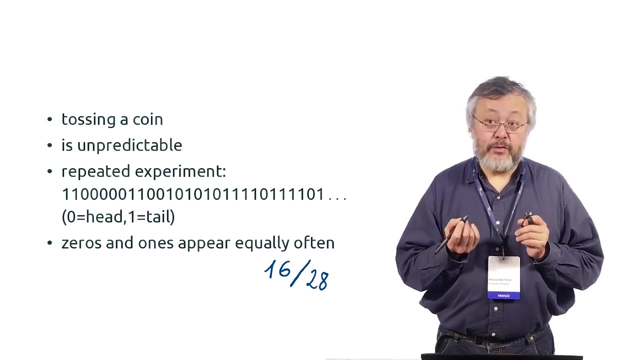 Eleven, twelve, thirteen, fourteen, fifteen, sixteen, sixteen, seventeen, eighteen, nineteen, twenty, Twenty-one, two, three, four, five, six, seven, eight. So it's sixteen of twenty-eight. It's not exactly half, because half will be fourteen of twenty-eight. 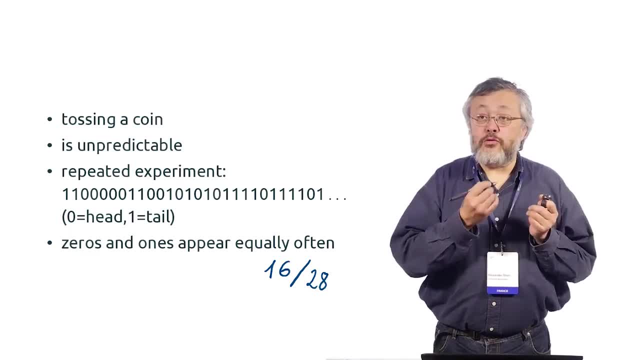 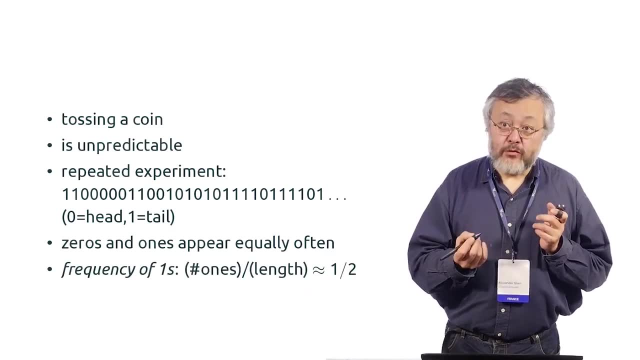 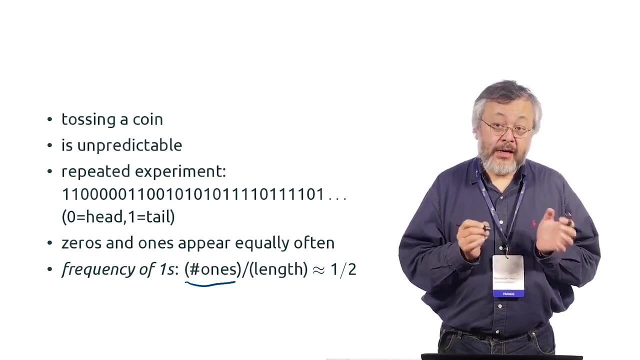 But quite close, And we can try to make these computations for different number of coin tosses and compute the frequency of ones. The frequency of one is the number of ones divided by the total length, And the prediction of probability theory is that it should be close to one-half. 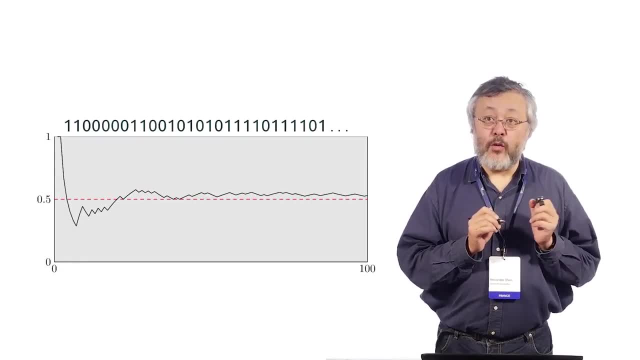 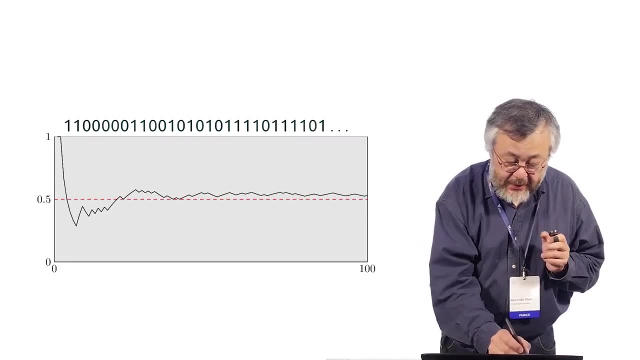 And here let's do it actually, and one can draw a graph. So you see, this is one, one, zero, zero. And here is the number, And here is the number of experiments, And here is the frequency. So you see that we start with ones because there are two ones. 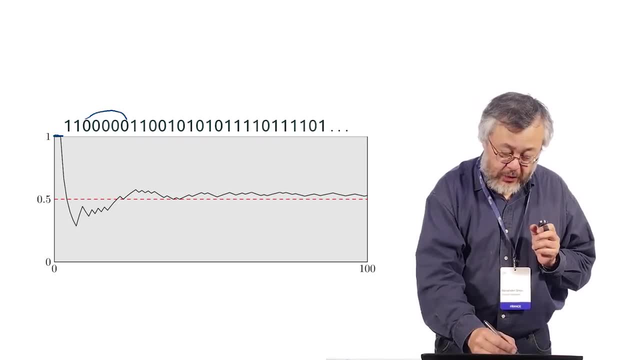 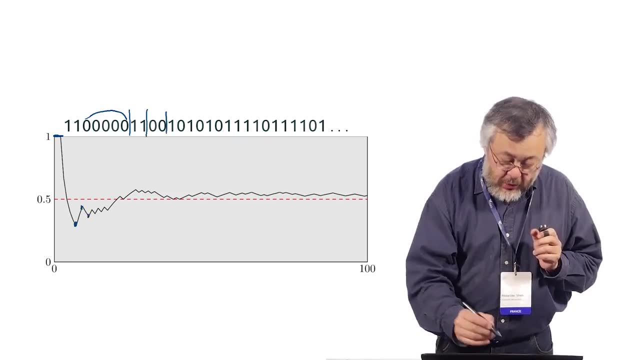 And here, then there is a long series of zeros and frequency goes down. So now we are here, Then there is two ones, we are here, two zeros, and so on. So there are some oscillations, But at the end the oscillations are small. 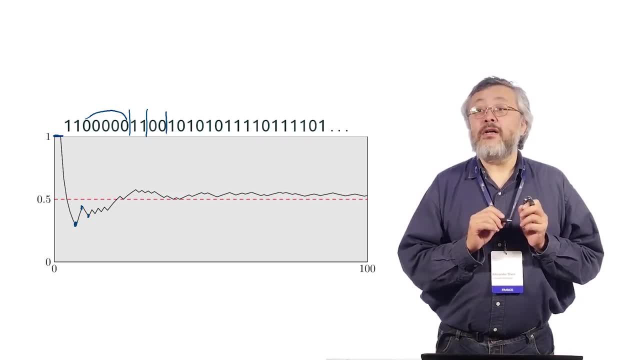 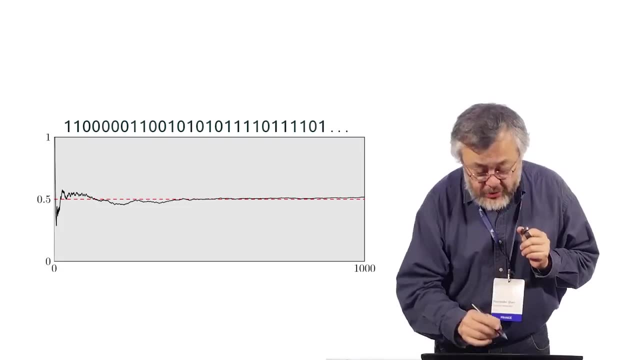 And after hundred, hundred coin tossing, we are close to one-half, A bit more, So let's see what happens later. Ah, four thousand, And you see, this initial part is somewhere here. So there were oscillations, But then the oscillations become smaller. 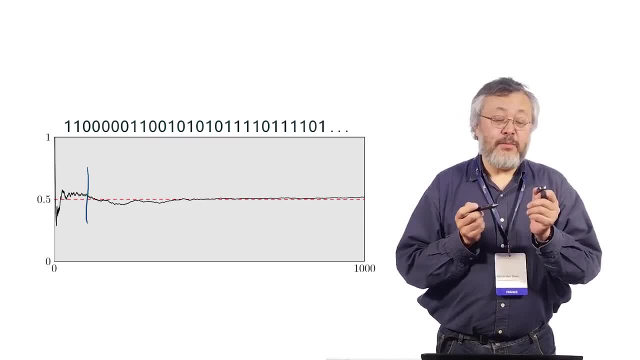 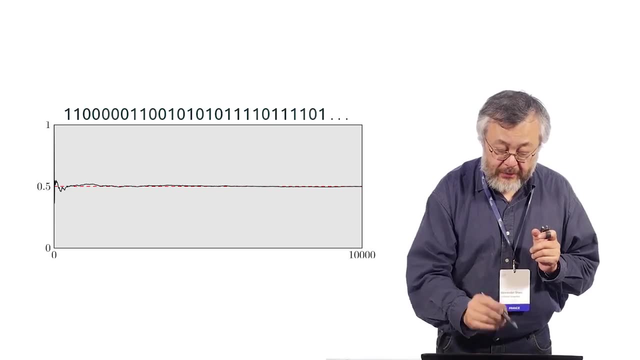 And at the end they are rather close to one-half. And if we make ten thousand random experiments, you see that it's even better. So now the oscillations are very, very small part of the picture And at the end we have almost one-half. 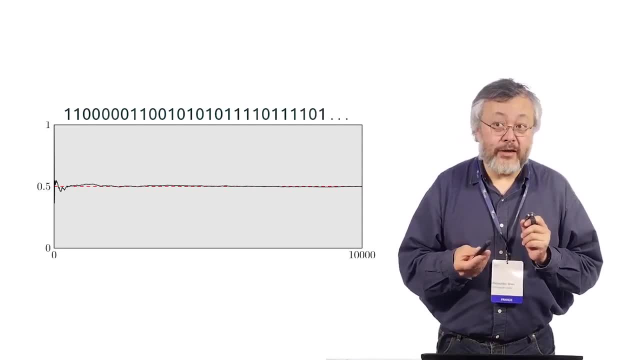 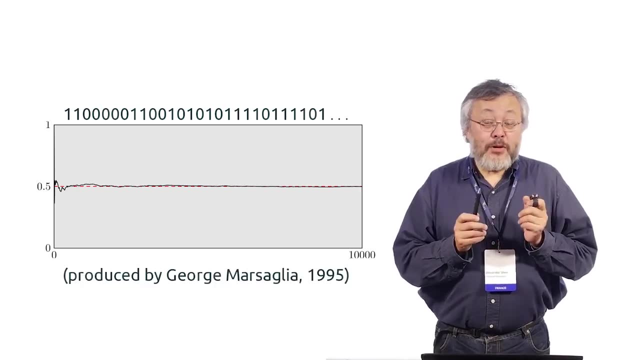 It's even hard to see whether it's more than one-half or less. So for ten thousand the frequency is very close to one-half. Probably you won't believe me that I make ten thousand coin tossing, And indeed this is not real coin tossing. 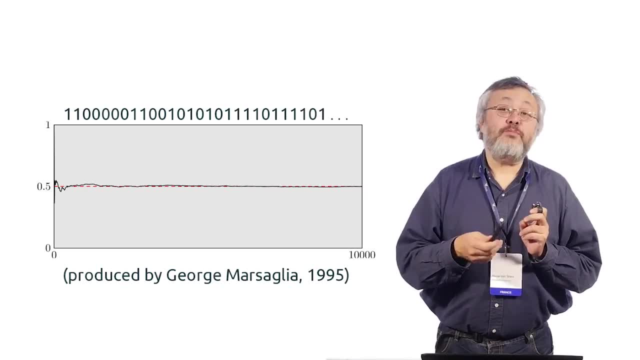 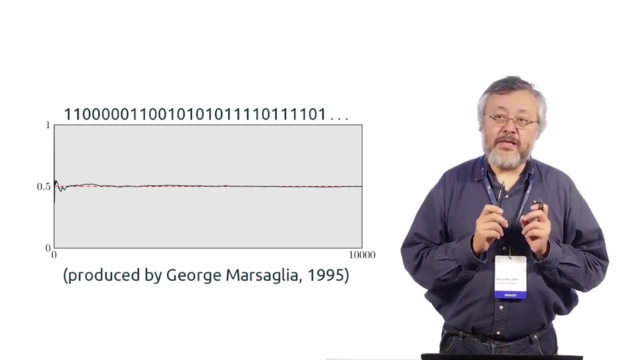 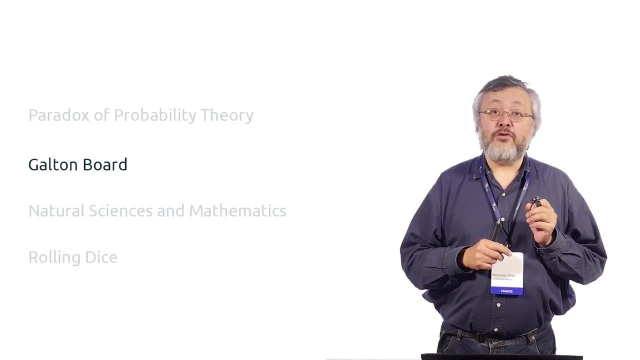 This is some experiment, physical experiment which should behave in the same way. It was produced specially for long sequence of bits which behave like coin tossing. It's random bits, so to say. Another physical device to show the laws of probability theory. 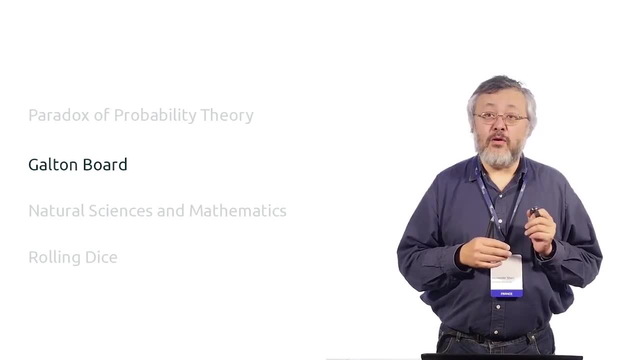 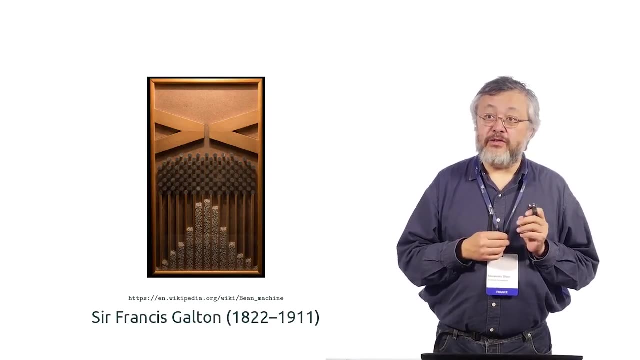 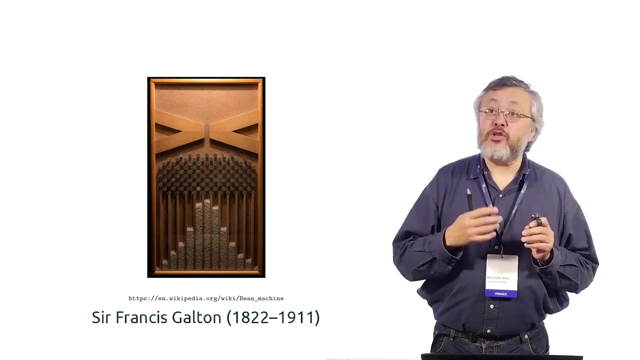 It was designed specially for this. This is what is called Galton board And also the other name is Bean machine. So if you look at Wikipedia page, it's called Bean machine. What it is? It's a vertical thing. You see the picture, I think, of a real machine from Wikipedia. 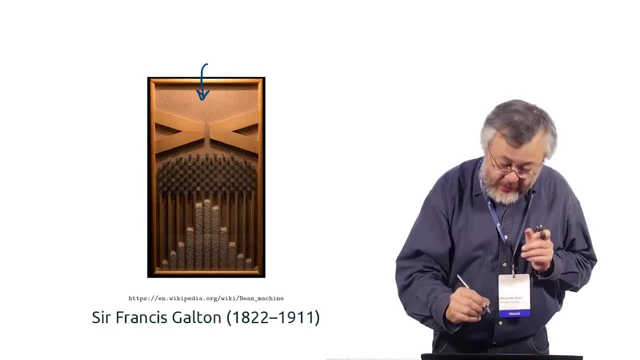 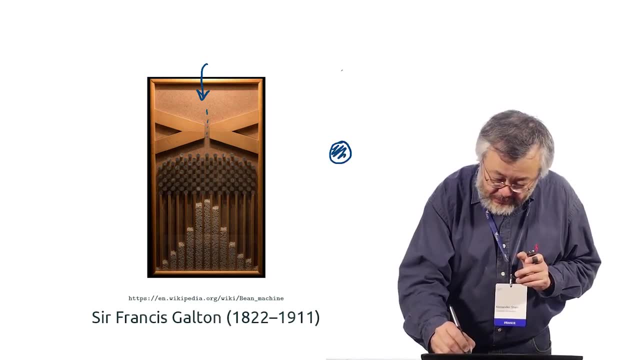 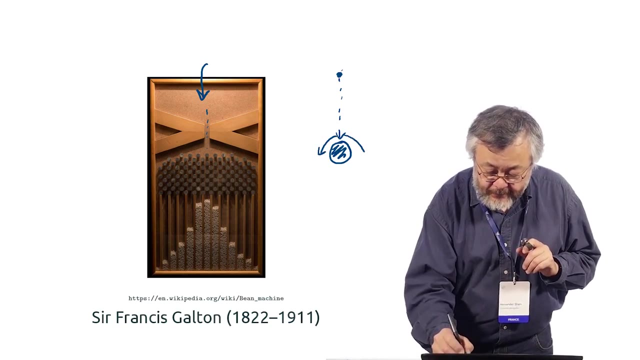 And what is happening? Beans go here and then they fall down through this hole And there is some kind of cylinder and beans go down. And what is random here? they can go left or right And the idea is that you cannot predict for individual bean whether it will go left or right. 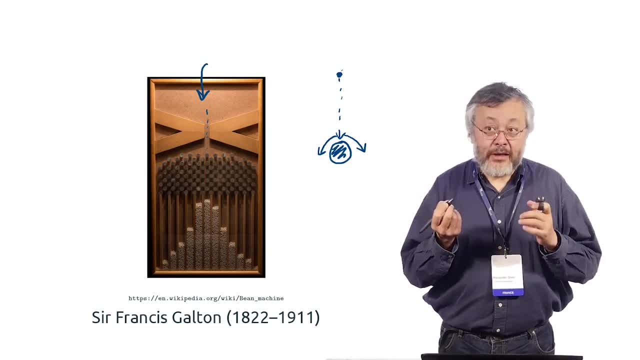 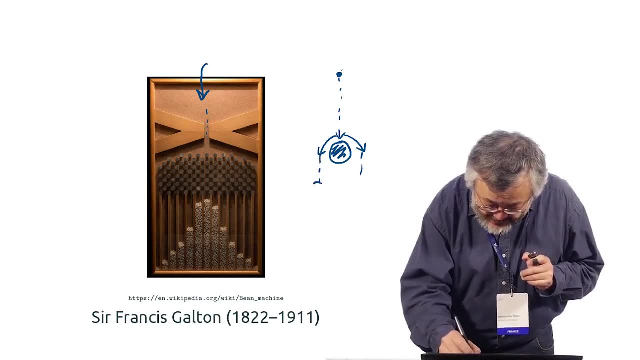 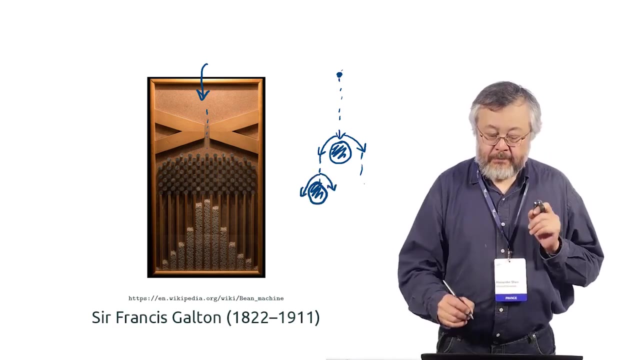 But half of them normally will go. Approximately half will go to the left and then another half will go to the right, And after that they fall down and they meet another cylinder And in this cylinder again they can go left or right. 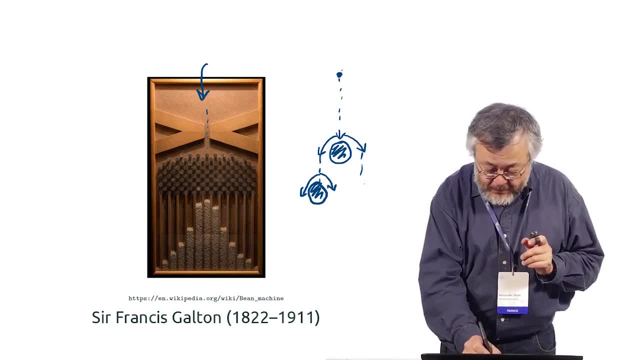 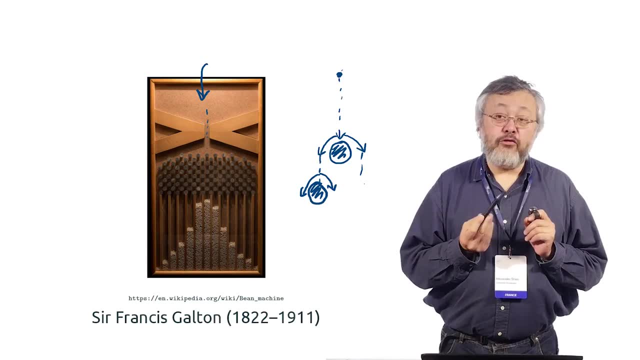 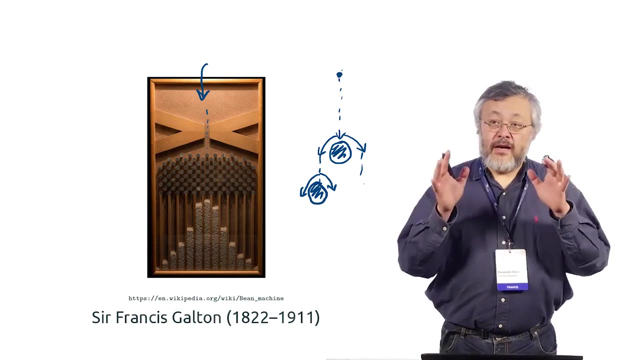 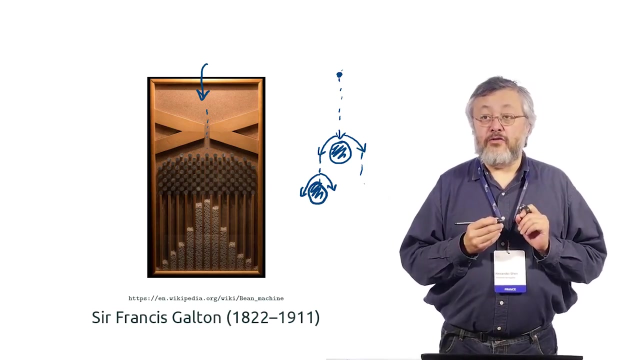 So at the end they are collected in these boxes, And what is interesting here is that the central boxes are full and the boxes far from the center are almost empty. So there is some kind of concentration effect. The beans have a tendency to concentrate near the center of the machine. 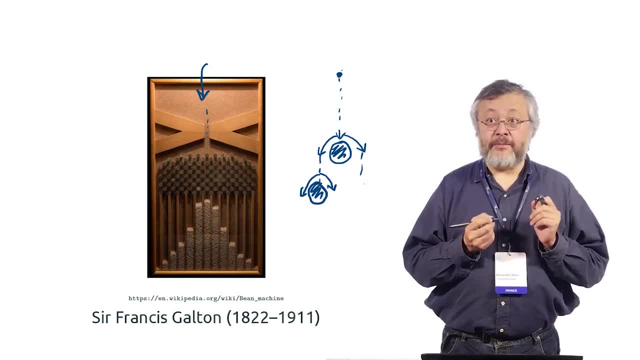 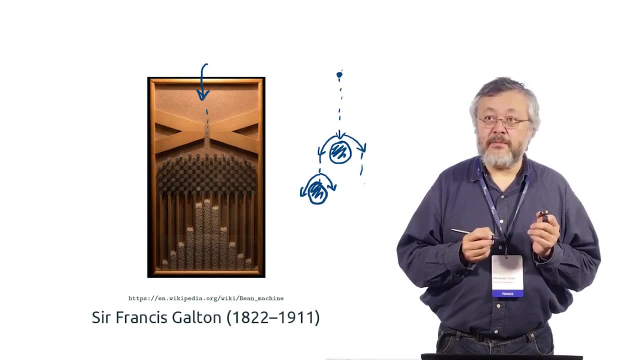 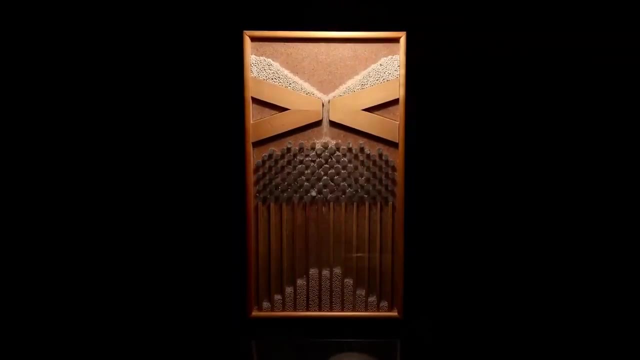 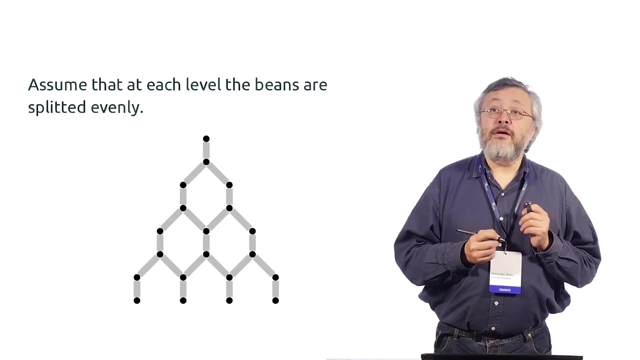 This is the effect, which should be explained. You can also look at the video. A Wikipedia page has a nice video how it works. Now the analysis of this machine. So we assume This is an assumption about the real world. We assume that at each level beans are split evenly. 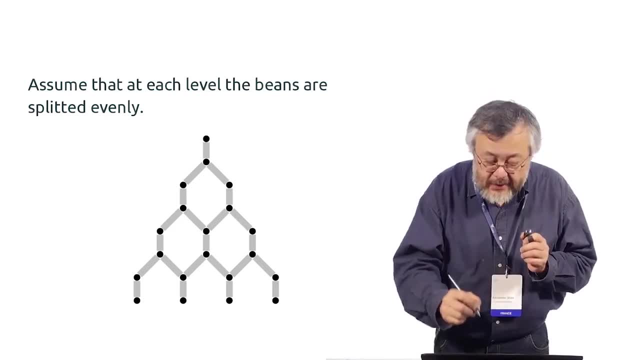 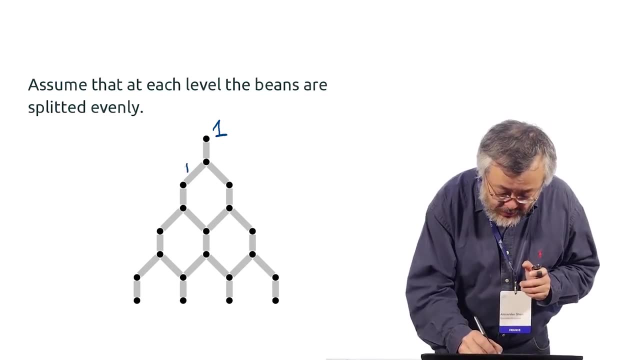 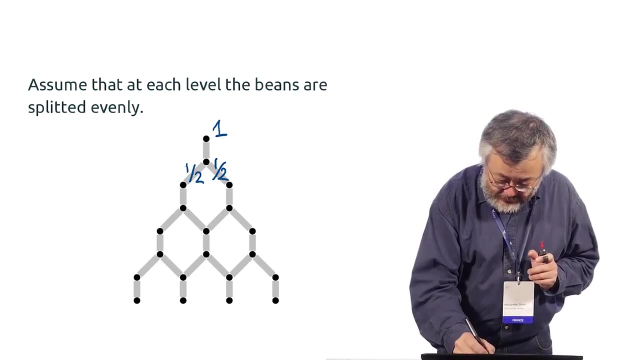 So here, if we take the total number of beans we denote as one, then half of them goes here and half of them goes here, And then they go here. OK, here is also one half and one half, And here we get one fourth and one fourth. 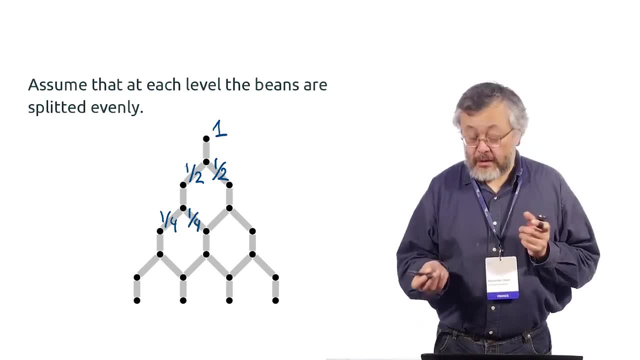 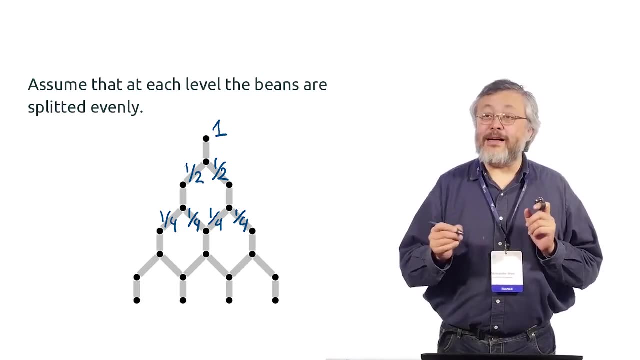 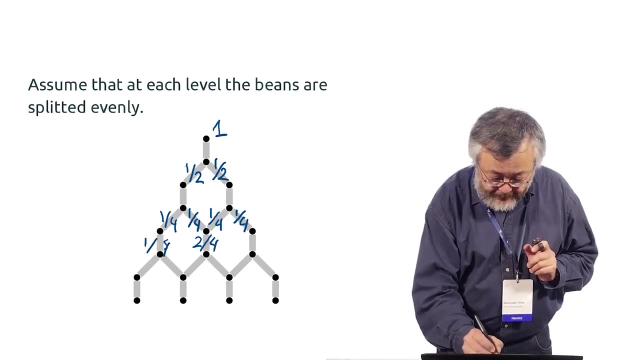 Just this one half is split into two equal parts, And here we also have one fourth and one fourth. What is new on the next level is that these two things combine So together. we have two fourths here and only one fourth and one fourth here. 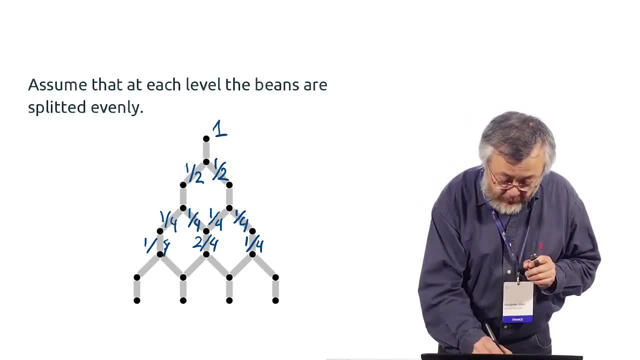 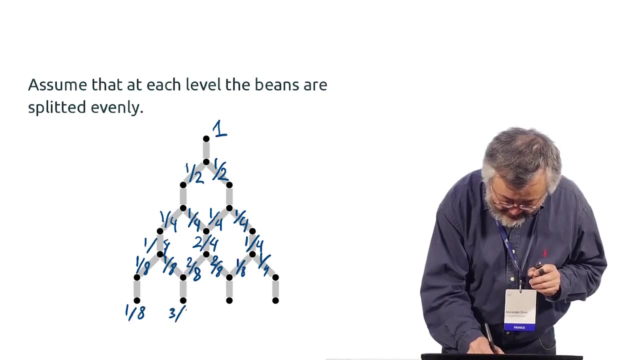 On the next level, the same thing happens. This one fourth is split into equal parts, And two fourths are also split into two eighths And one eighth and one eighth, And we have a combination. Let me write here: It's one eighth, three eighths, three eighths and three eighths. 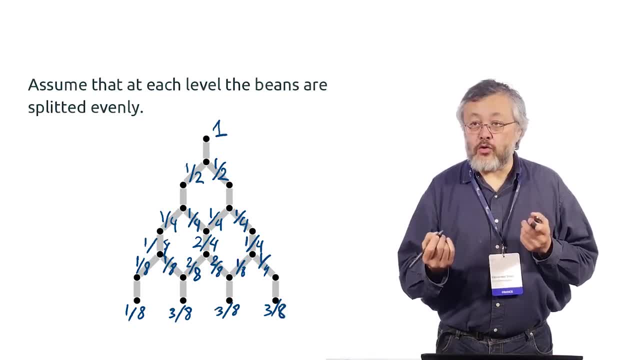 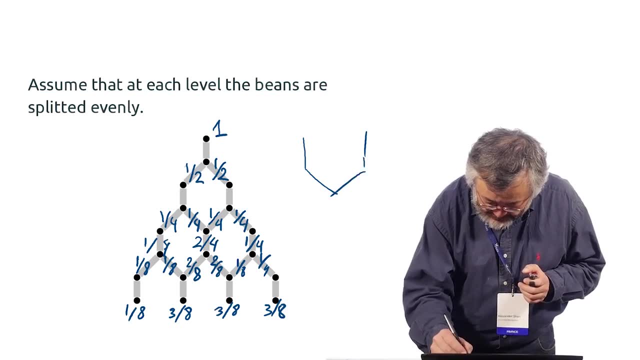 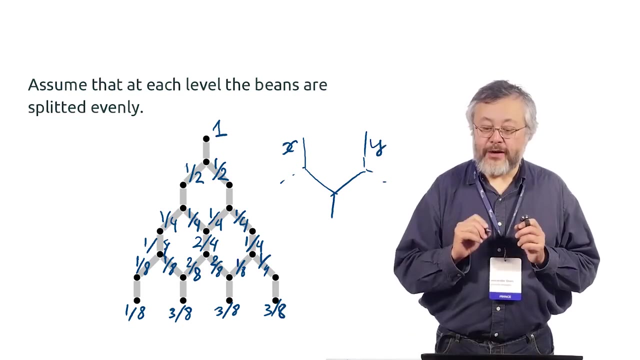 So there is some general rule how we fill the table. So if, For example, let's Imagine we look at this place, So imagine we have some- I don't know- x, And here we sum y fraction, Here we have x over 2 and y over 2.. 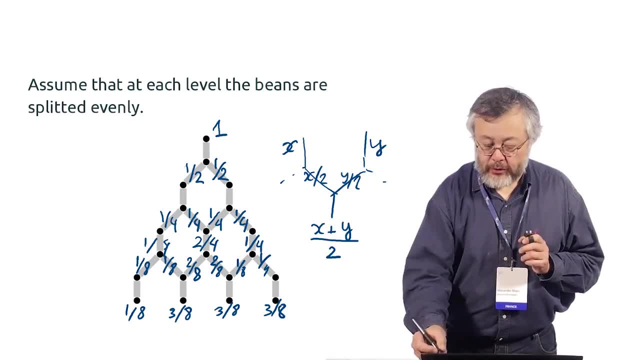 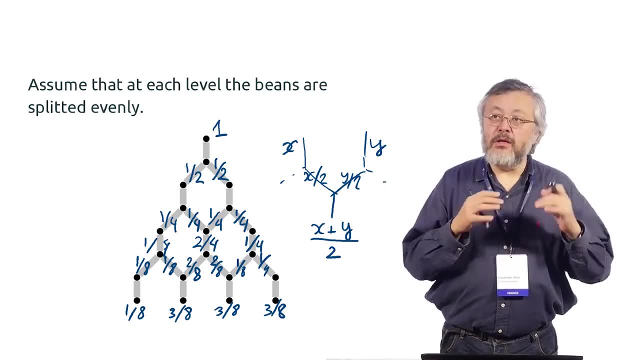 And here we have x, the sum, and get x plus 1 over 2.. So we assume that at each splitting the flow goes into equal parts. This is the rule. So you can easily. You can easily fill the table. 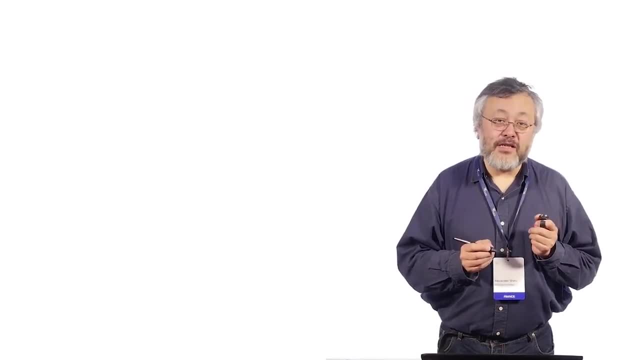 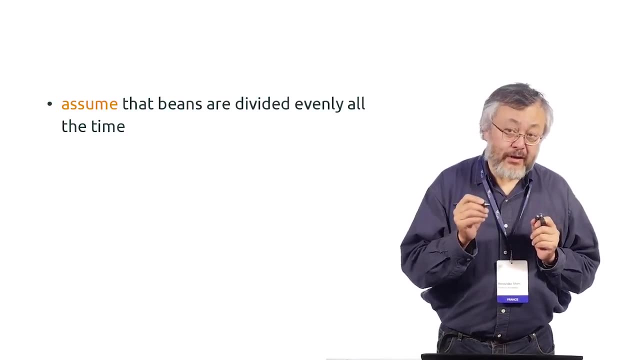 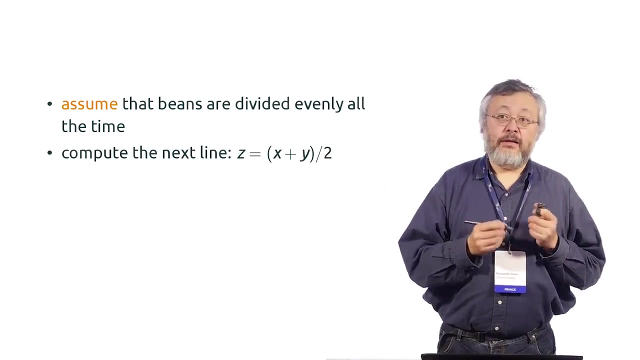 And probably you see that this table is similar to the thing which you should know, Pascal triangle. So, assuming that beans are divided evenly, is this assumption about real world? But then, after that, we have mathematical computation, And this is the rule that we used. 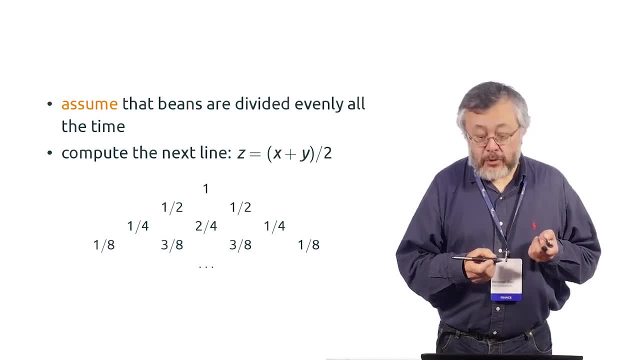 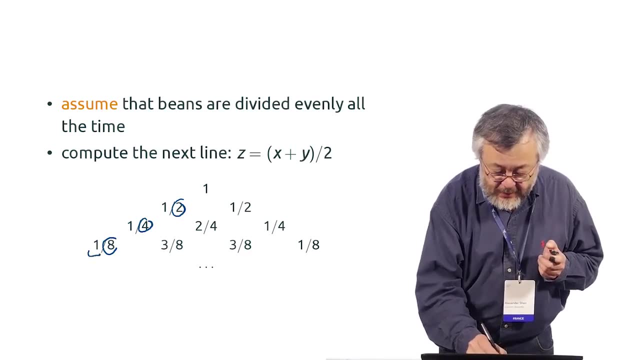 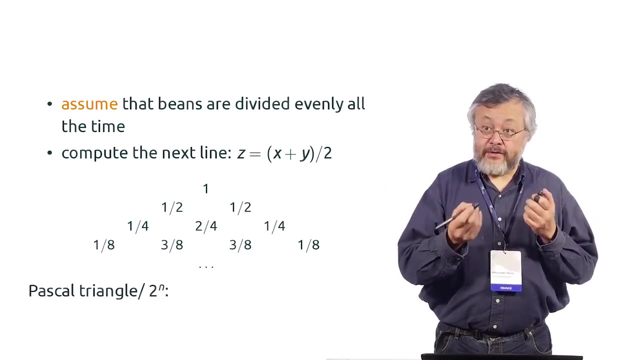 And this is the table that we got. And this table is just, You see, this is the power of 2.. 1,, 2,, 4,, 8.. And these things are like in Pascal triangle, And this is Pascal triangle divided by powers of 2.. 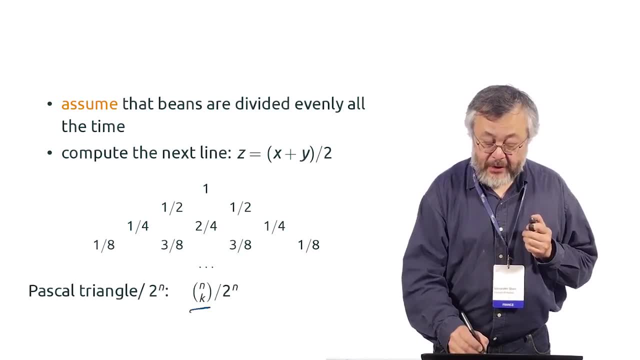 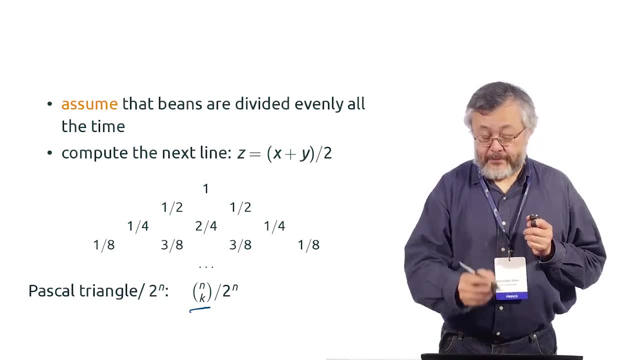 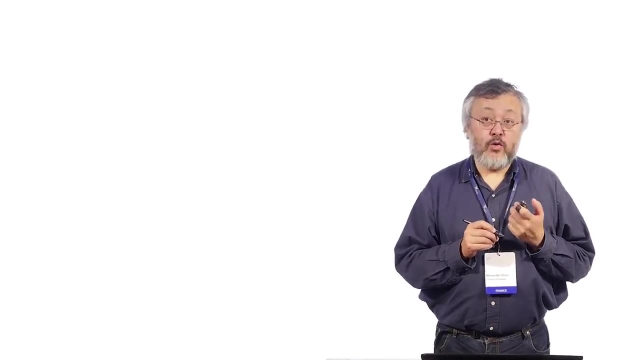 And if you want to write a formula, it's like this: It's binomial coefficient K is the number in the line And 2 to the n is the number of the line itself. And this concentration effect now can be estimated quantitatively. 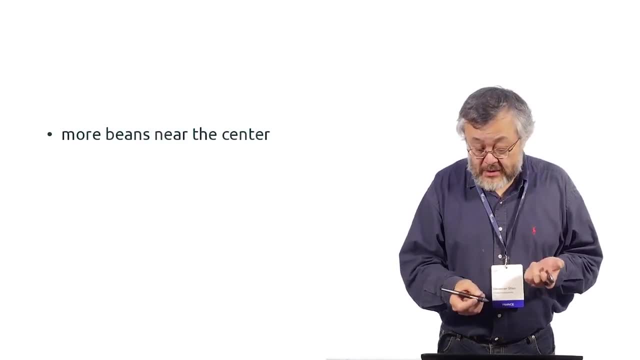 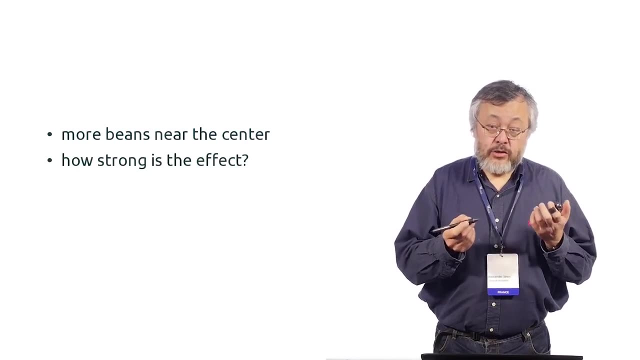 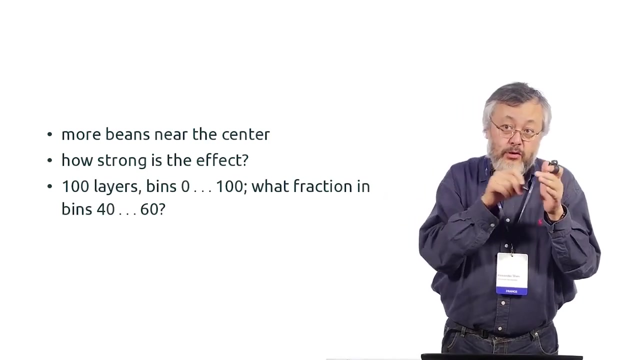 You can just compute and see, really, if the model is correct, which fraction of the bin should be near the center, And you can find just a number. So you can take 100 layers, Then the bins are from 0 to 100.. 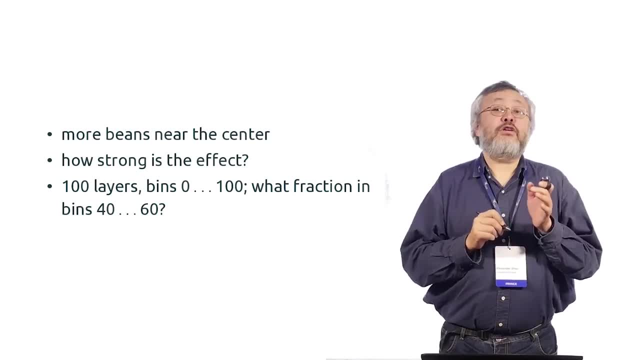 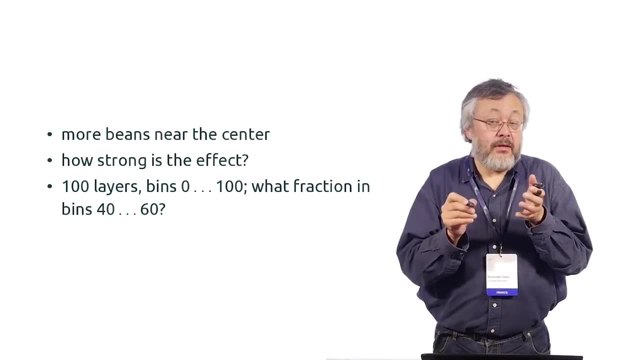 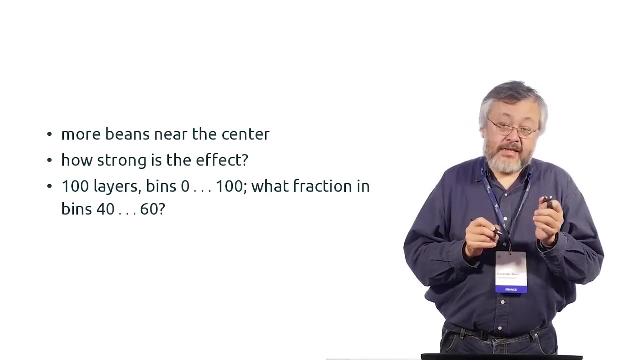 This K is from 0 to 100. And if you decide, for example, that center is between 40% and 60%, you can just compute with an easy program What fraction of these bins goes into the center part. And if you compute the same for 1,000 layers? 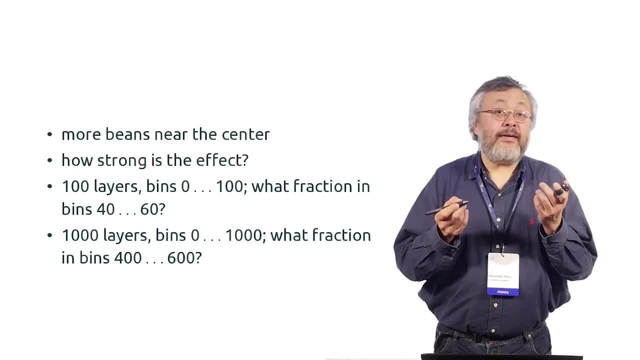 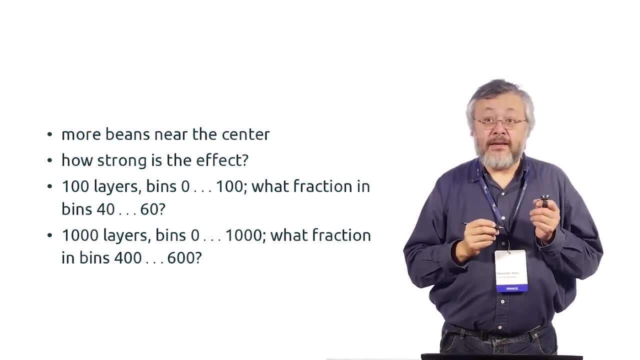 it's also not very difficult for a computer. You need an array of size 1,000.. You don't need to fill the entire table. You should just go from top, filling line by line, And if you do this then you see what fraction is here. 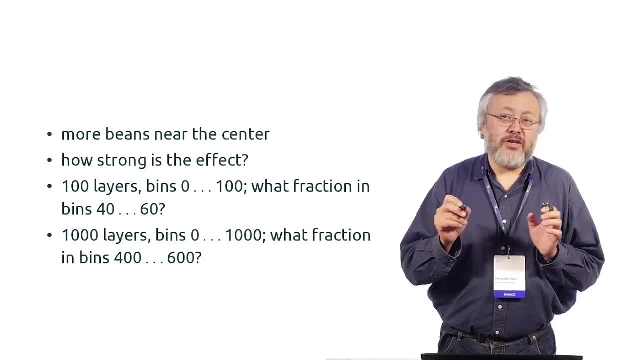 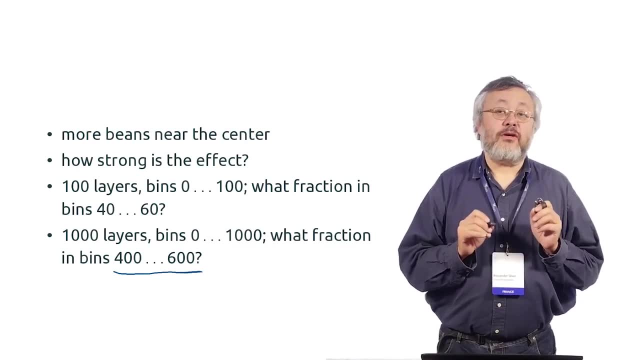 And you will see. I promise you. I don't remember the numbers, but I promise you that for this part, the concentration effect is much stronger. Almost all the bins will be near the center. So this is the same effect, somehow, that we observe with frequencies. 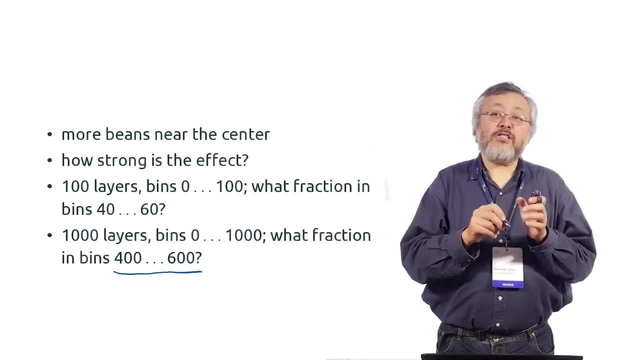 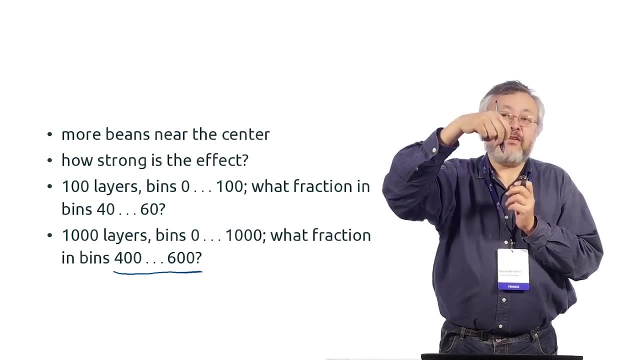 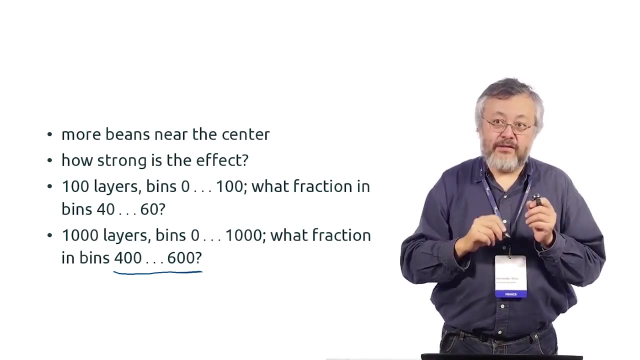 But now it's not for one sequence, It's just we look on many. Each individual bin somehow has some individual trajectory And we count the number of trajectories going and ending at different places. I want to say more things about the division of probability theory. 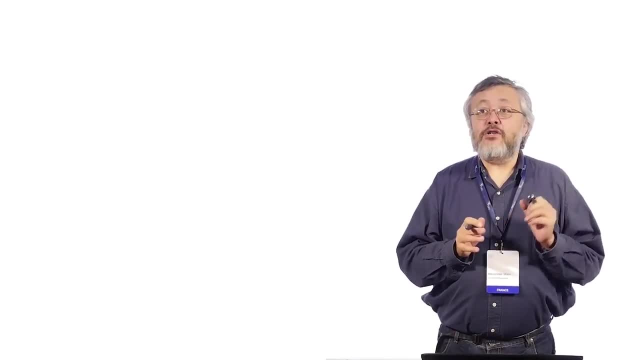 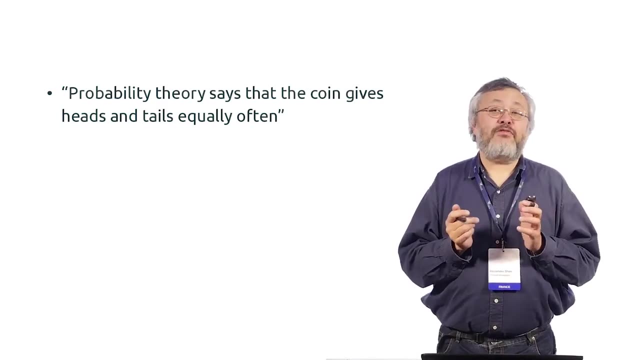 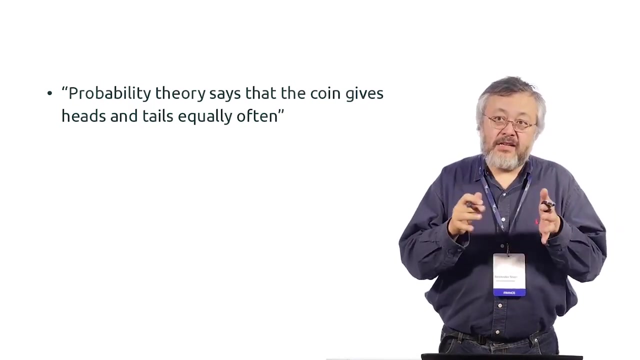 between natural science and mathematics. So if you ask some people on the street what is probability theory, maybe some of them will tell you that the probability theory says that the coin should get head and tail equally often, But actually, strictly speaking, it's not the case. 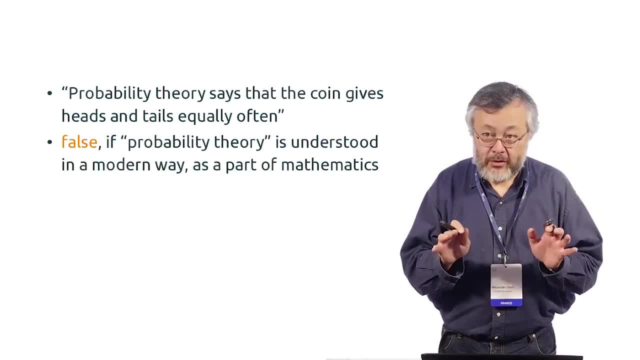 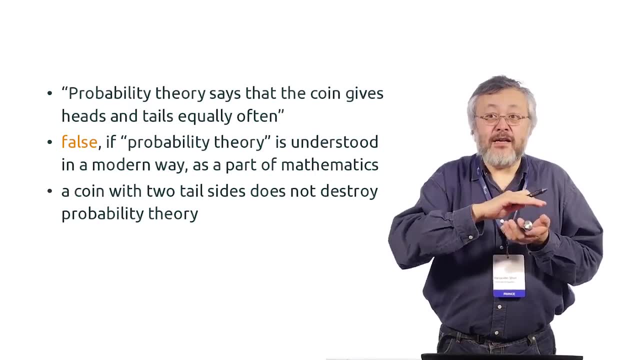 Mathematical probability theory doesn't care about the coins at all. It's just a part of mathematics, And if somebody makes a coin which has two tails on both sides, of course this person will not destroy mathematical probability theory. And just a coin is bad. 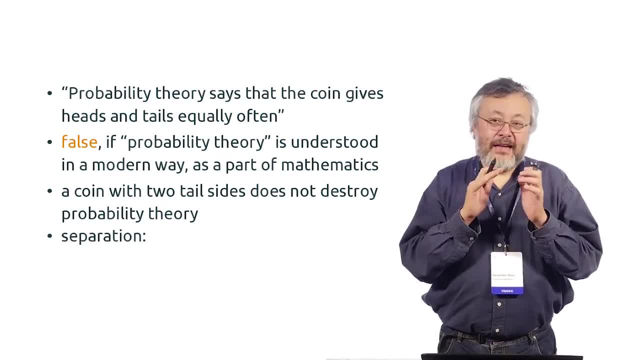 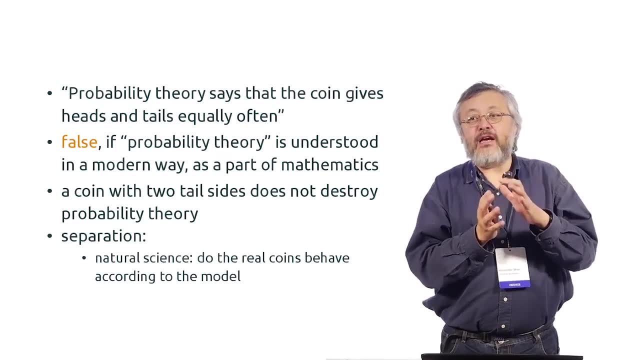 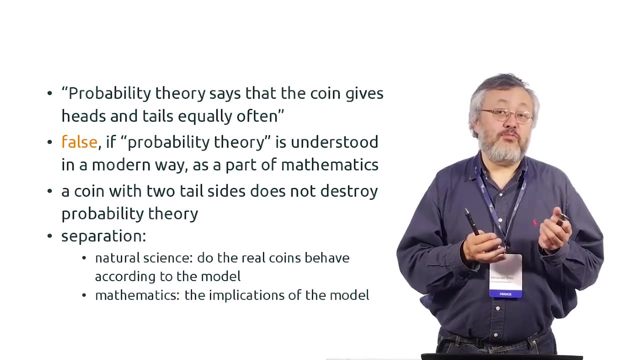 But theory is good. So again, let's see what is the separation line. So natural science cares whether the real coin behaves according to this equal head and tail model, And mathematics studies the implication of this model. For one coin tossing is not much to study. 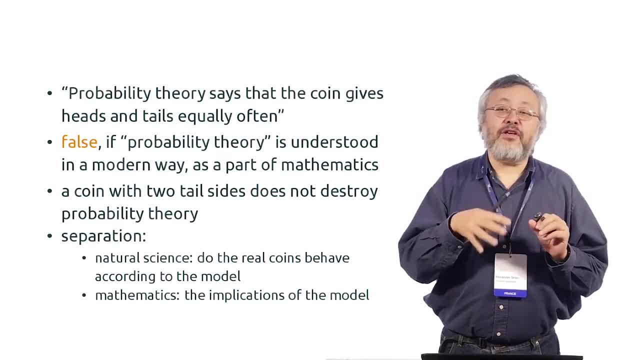 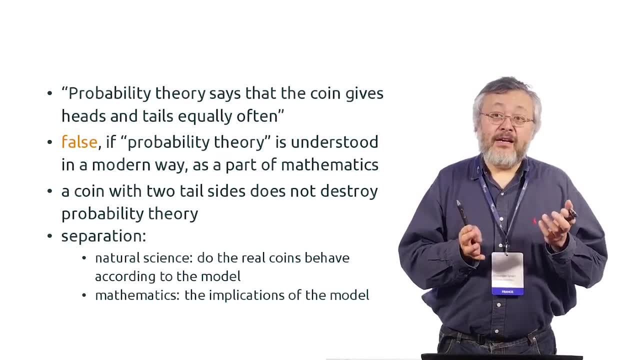 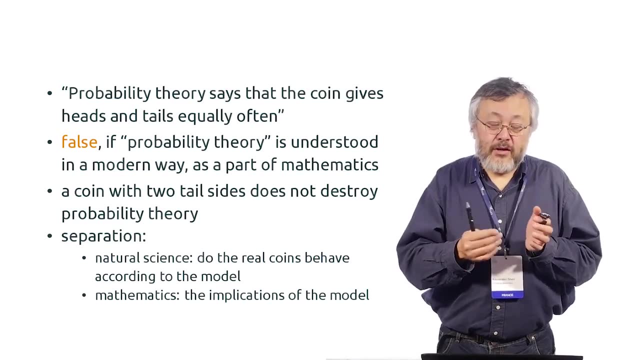 But still, mathematics starts with the model and then finds what are the consequences of this model. Of course, normally mathematicians work together with some other scientists, So if the model is not good, they found this and they try to suggest a different model. 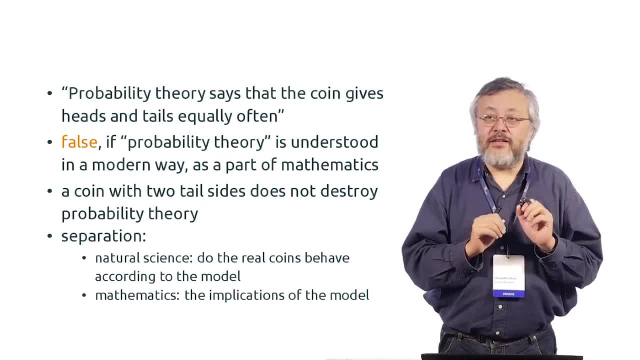 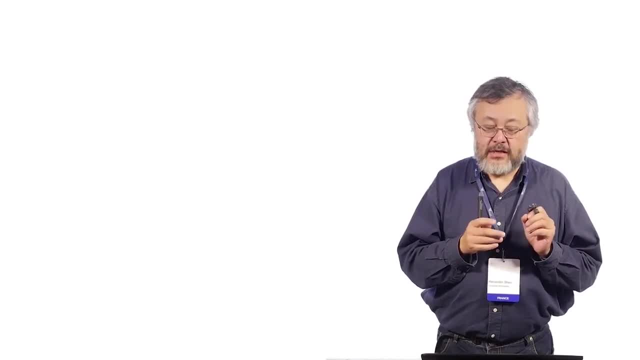 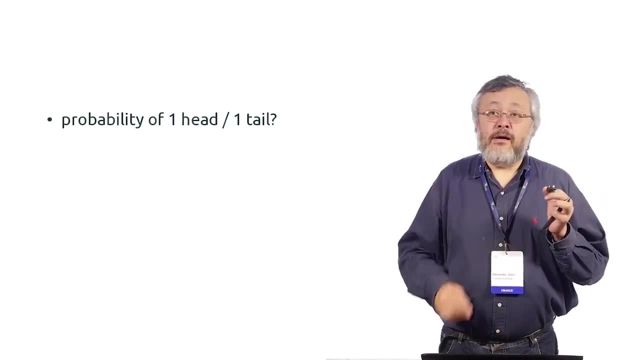 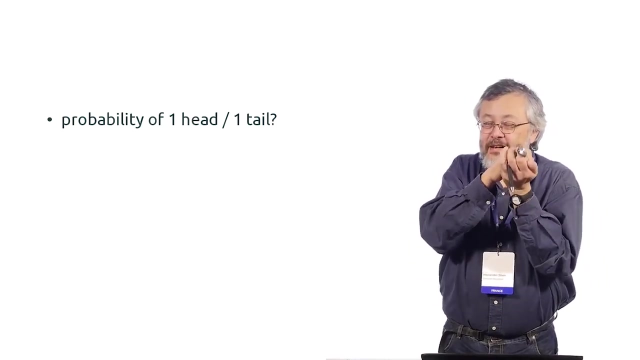 and so on, But purely theoretical. there is a division like this. Let's look at some special case when this illustrates this division. So imagine we toss two coins And, for example, you can just take two coins and do something like this: 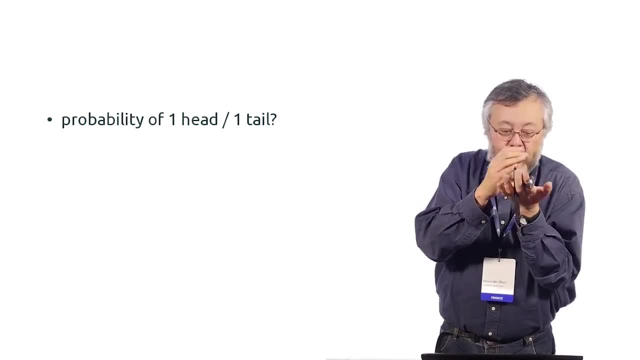 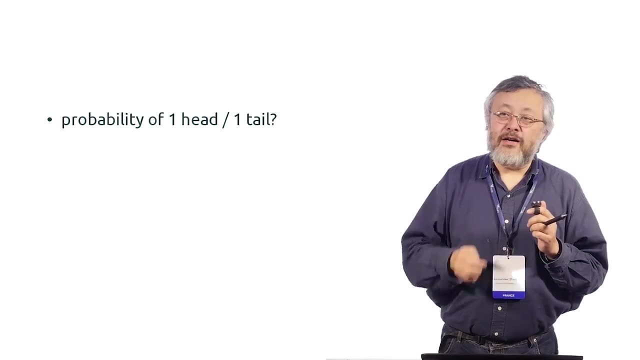 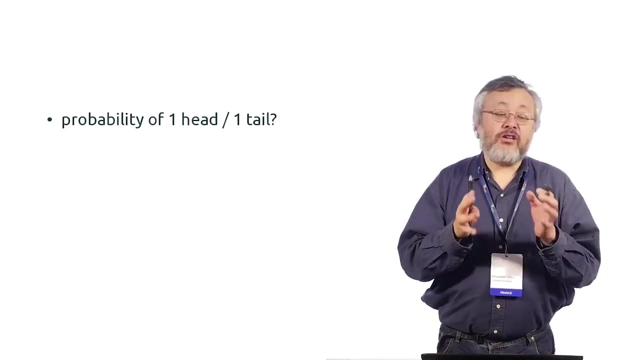 And you see something. What do we see? Oh, now we see two tails. But the question we want to ask is: what is the probability to have one head and one tail? And just imagine a discussion. This question is asked And then Alice says something like that: 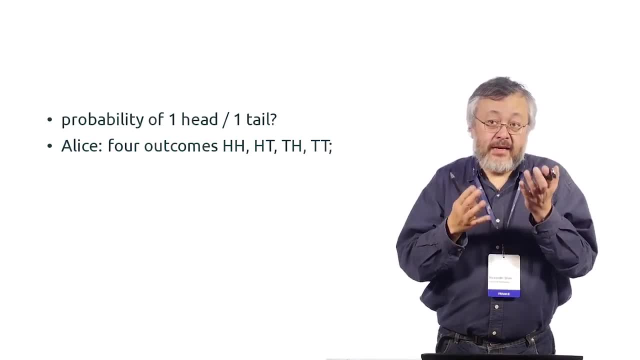 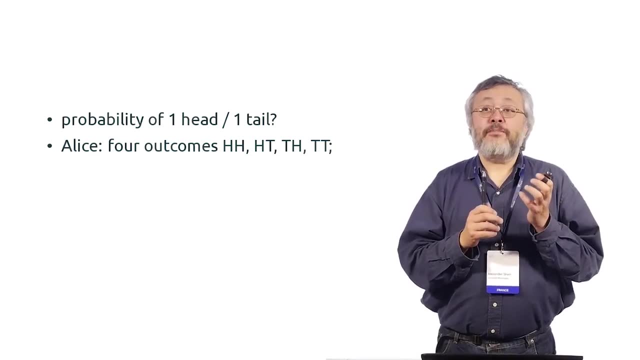 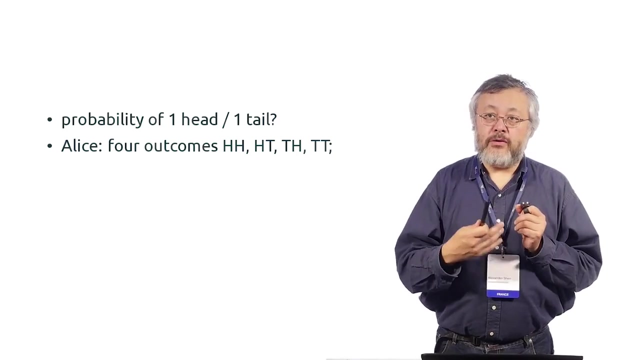 There are two coins, So the first can be head and the second can be head, Or first head, second tail, Or first tail, second head, Or two tails. So there are four outcomes And we are interested in which fraction of the coin experiments. 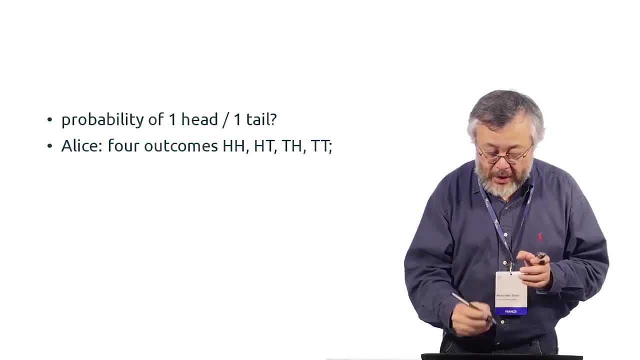 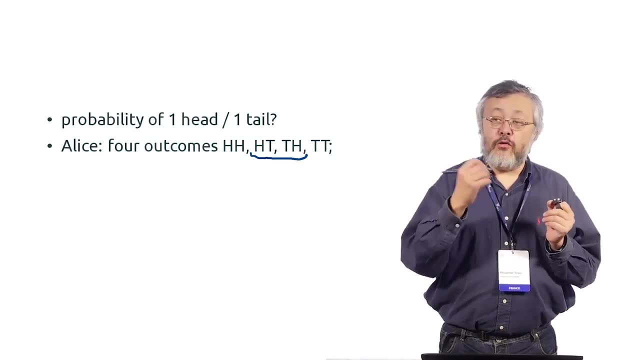 we will have one head and one tail. So if all four outcomes are equally probable, there are two of them, which corresponds to one head and one tail. The probability is two of four, So it's one half. This is what Alice says. 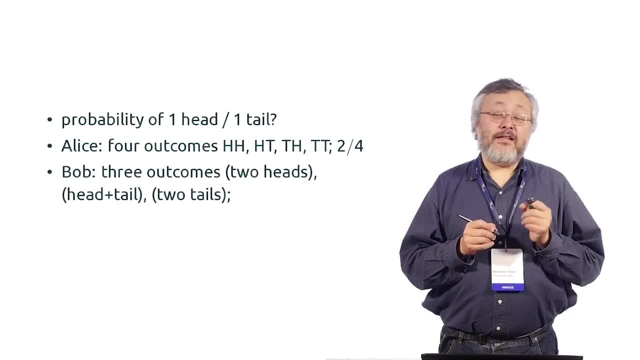 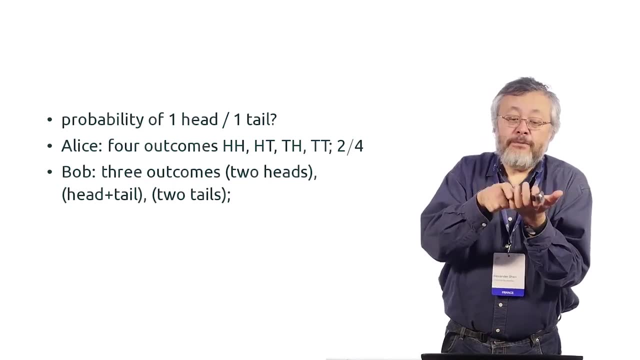 But now some other guy comes, Bob, and says: look, you see why there are four outcomes. You have two coins, You toss them And when you look you don't know where is the first coin and where is the second coin. 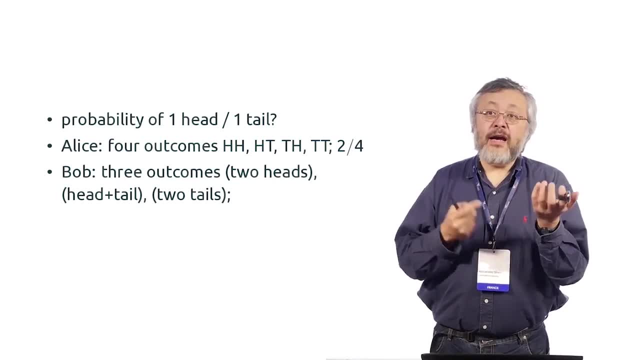 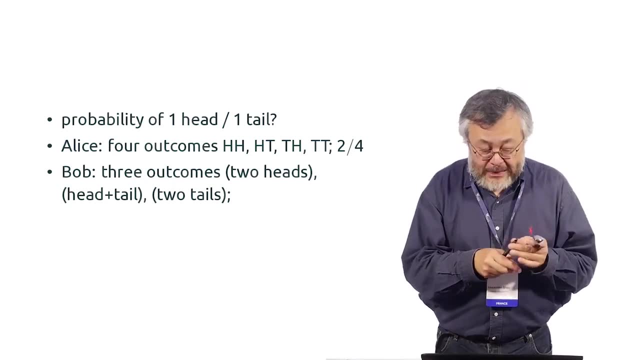 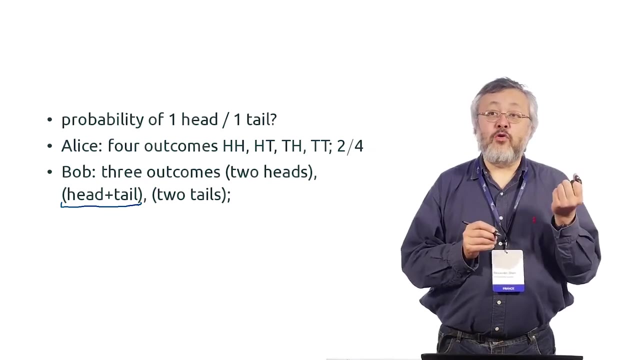 So essentially, there are three outcomes: Two heads, head plus tail and two tails. And so if we assume that these three outcomes appear equally often, then the probability of this outcome is one of three. And so who is right here? Then a pure mathematician, Charlie, comes. 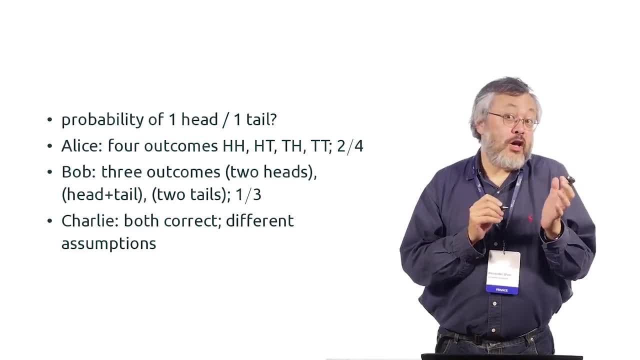 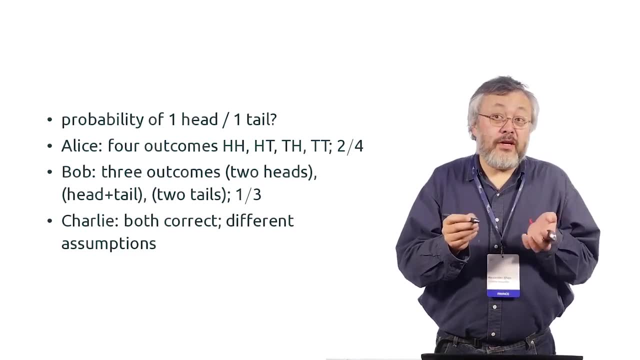 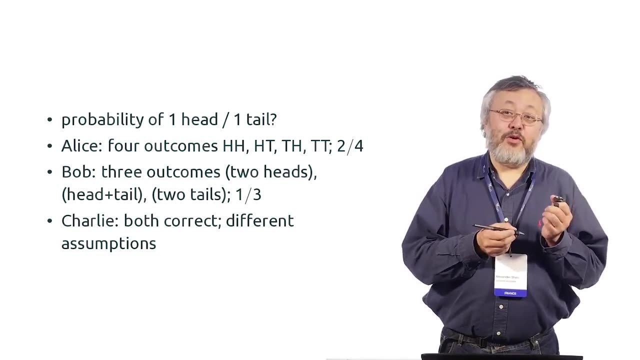 and says: you are both correct. You just have different models And I don't care about real coins, but if you want, you can consider this model or that model, Why not? They are just different assumptions And, of course, if you want to know what happens really. 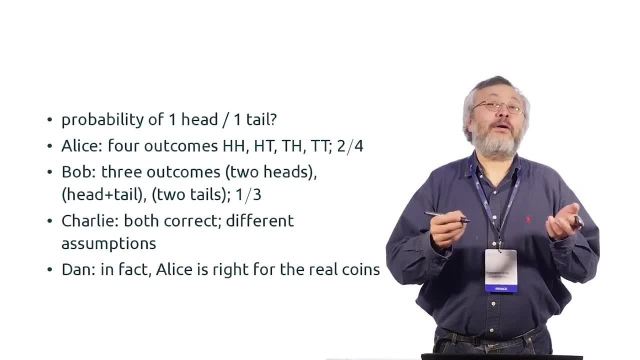 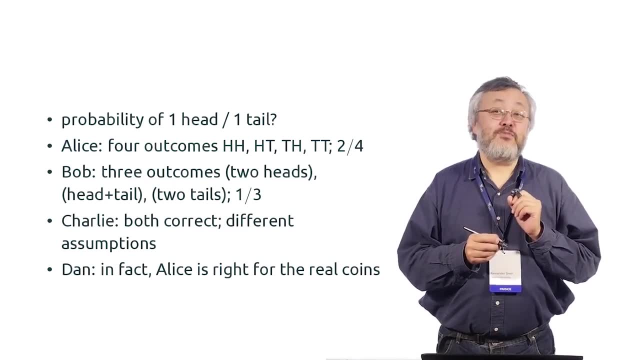 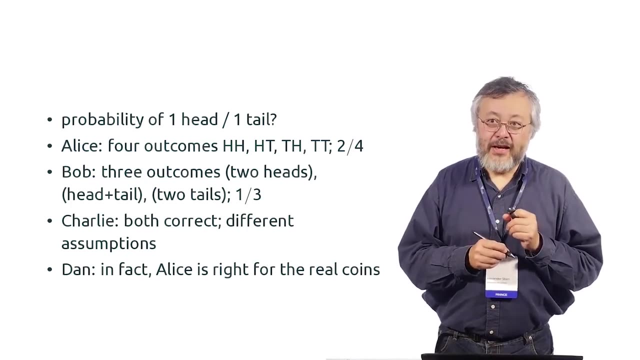 it's not the mathematicians who should be asked. We should consider some natural scientists or physicists then, And he will tell you that, indeed, Alice is more right. So for the real coins- just it's an experimental observation- These four outcomes have the same probability. 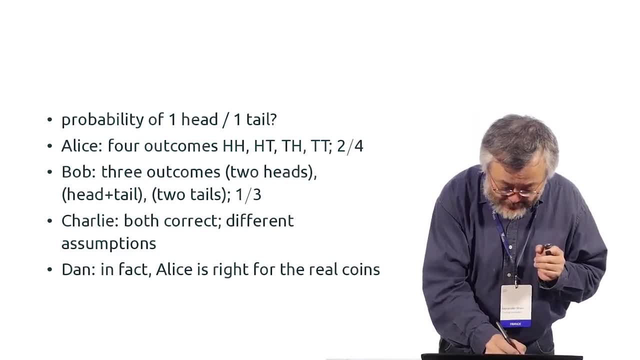 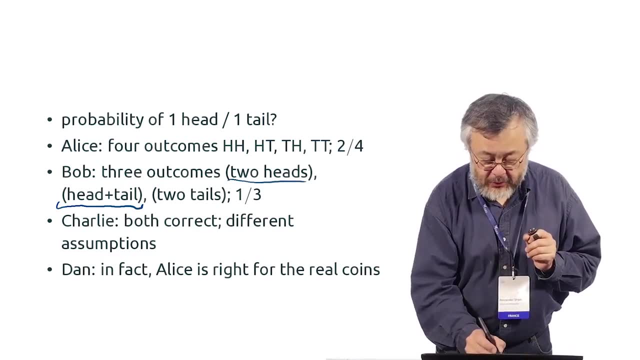 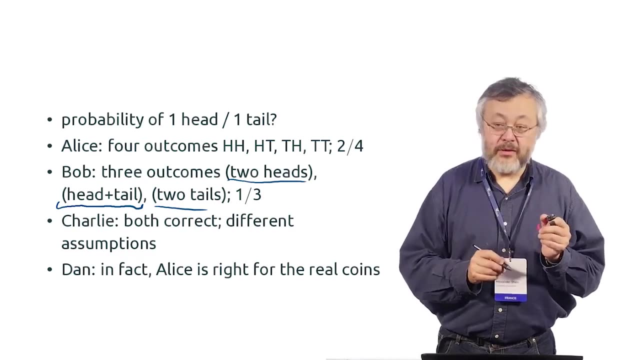 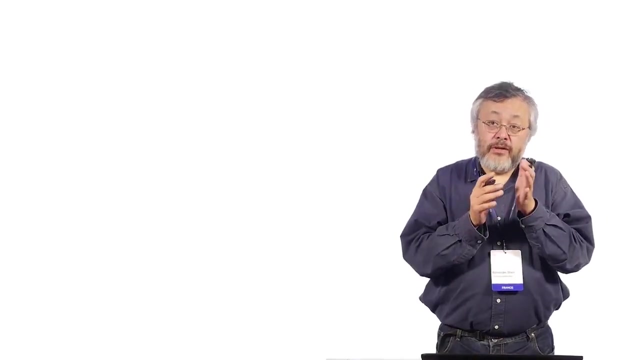 And so, if we classify things according to Bob's scheme, this outcome will appear twice more often than this or this, Because in this model there are two cases, which corresponds to one case in this model Again. so this is the distinction between. 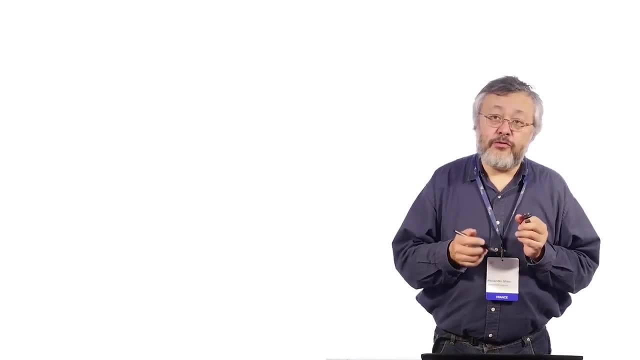 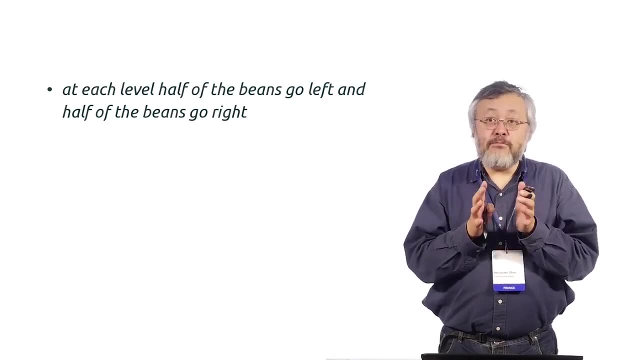 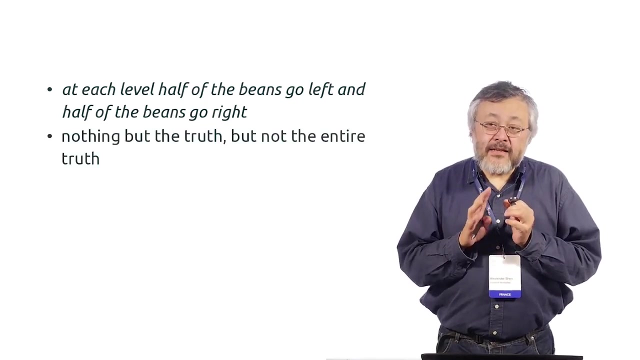 mathematics and natural science. Let's look from this viewpoint on Galton board. What would we assume really? So one can say that the assumption is that each level, half of the beams go left and half go right, And it's yeah, of course. we assume this. 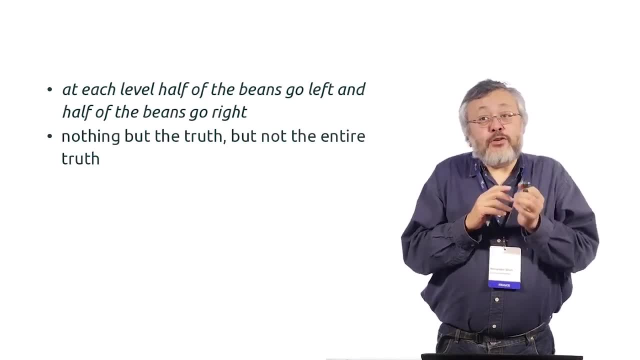 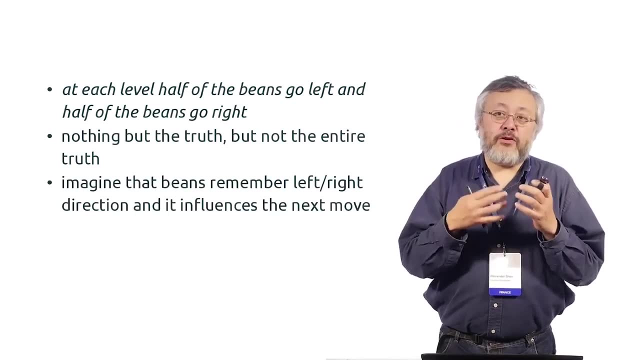 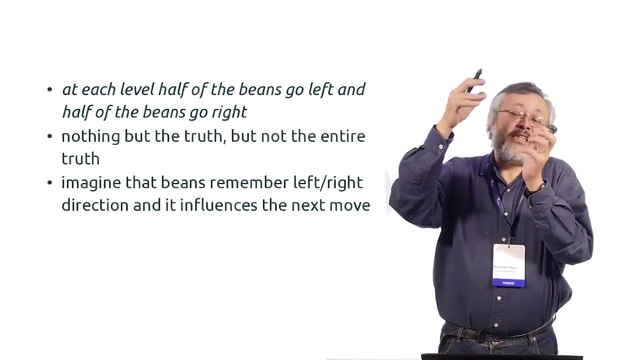 but that's not all, Because you can imagine, for example, if a board, just depending on the board construction, maybe the beams actually when they make a first move they get some velocity, And if they go to the left in the next move. 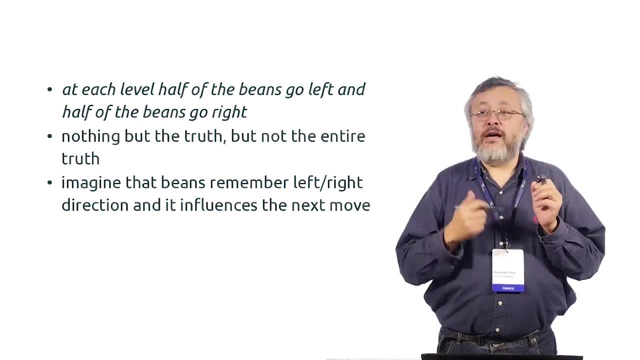 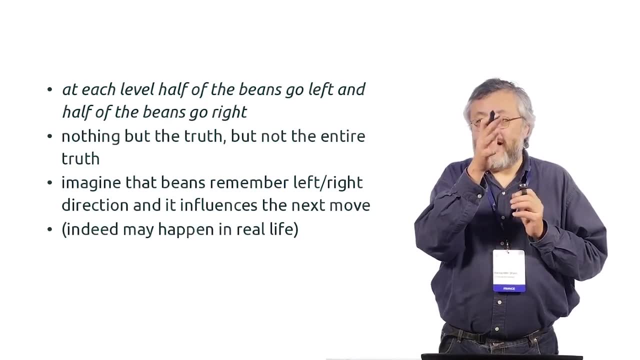 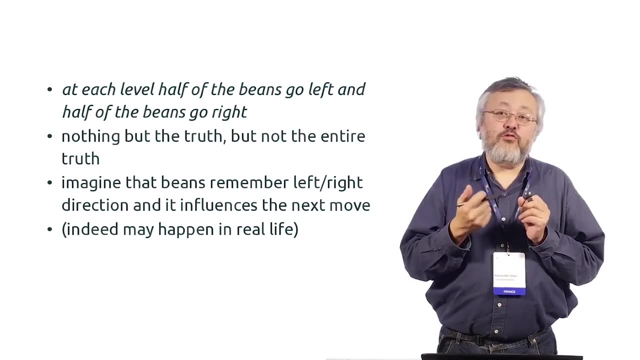 they will also go to the left because they already have this direction. So maybe in the physical world it can happen that some decision on the level k influences the decision on the level k plus one. For example, going left makes the next left move more probable. 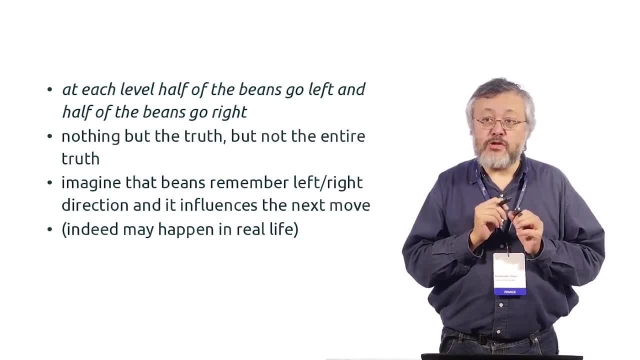 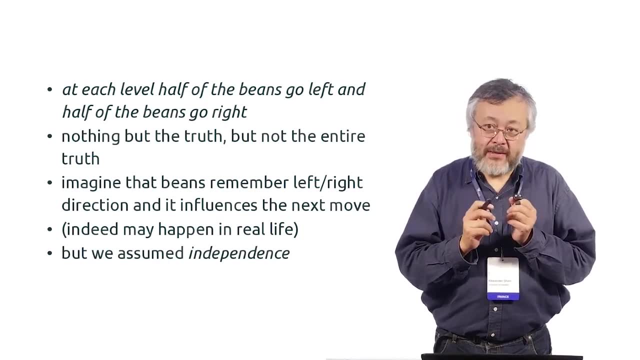 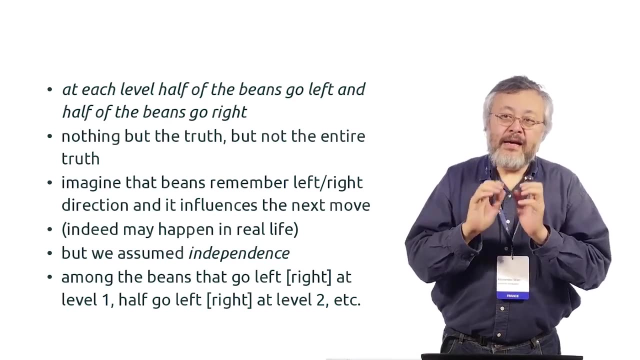 But we assume our assumption, our computation was based on the assumption that this doesn't happen. So we assume that probability theory, language theory, language is independent. We assume that among the beams that go left, if we consider only the beams that go left at level one, 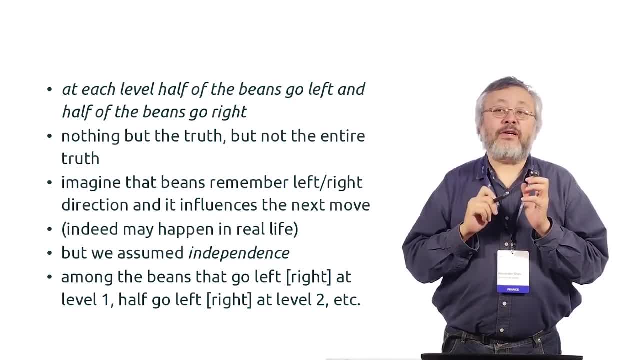 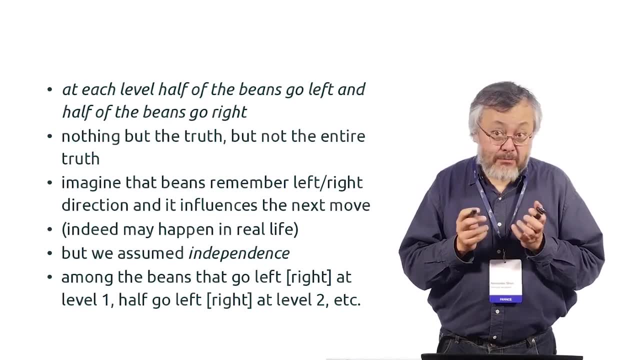 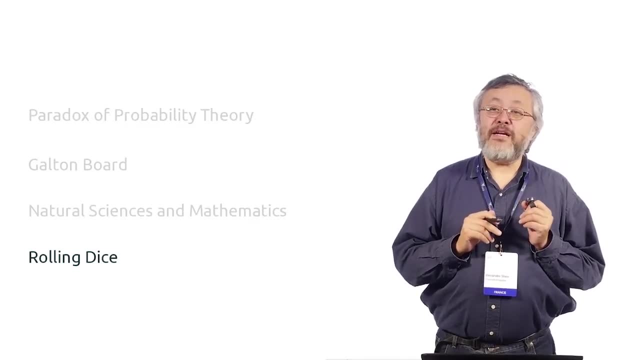 half of them will go left at level two and half will go right at level two. So the second decision is somehow independent from the first one. This was our assumption and we made computation based on it. Now we switch to another experiment, which is rolling dice. 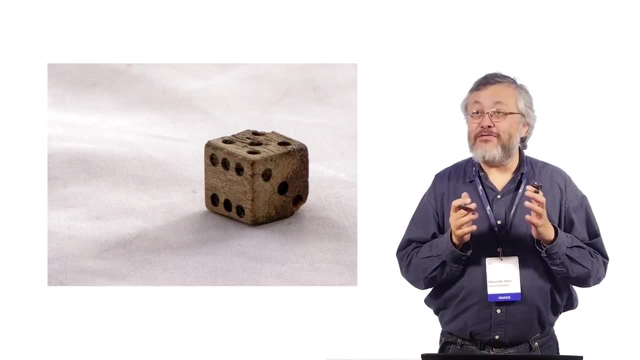 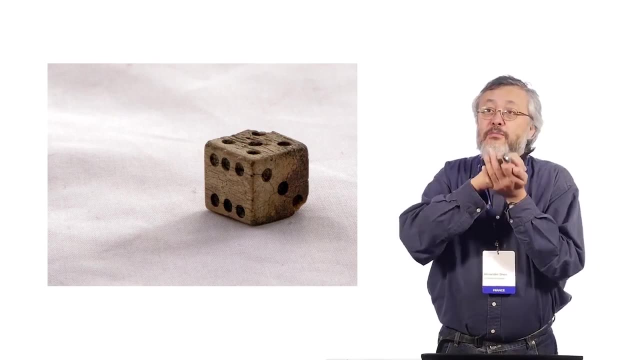 So actually, unfortunately I don't have dice now, so I can only show you a picture, but probably you have seen it, So you can also toss it and roll it, or roll it like this or whatever, And you can get a number. 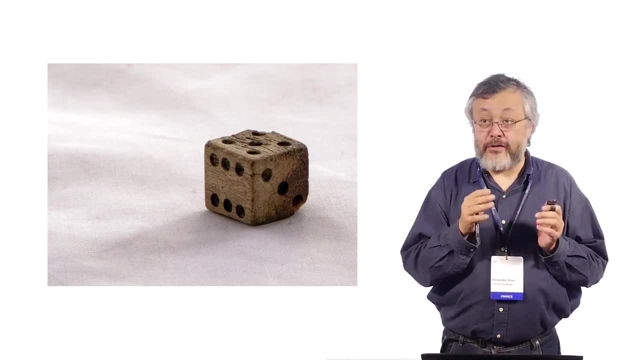 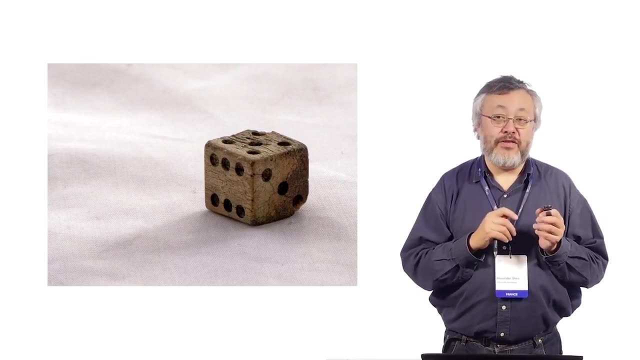 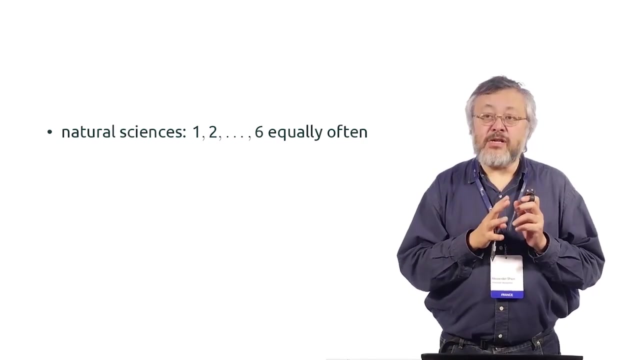 which is between one and six: one, two, three, four, five, six. So it's very useful if six people go in a restaurant and can decide who of them pays, And the natural science part is that these six outcomes appear equally often. 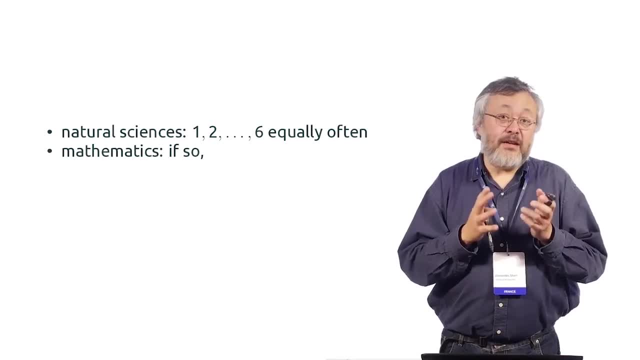 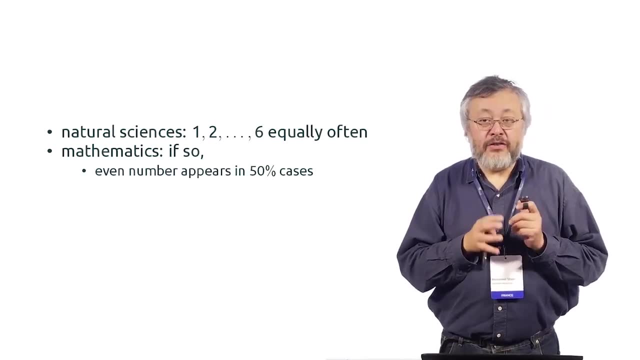 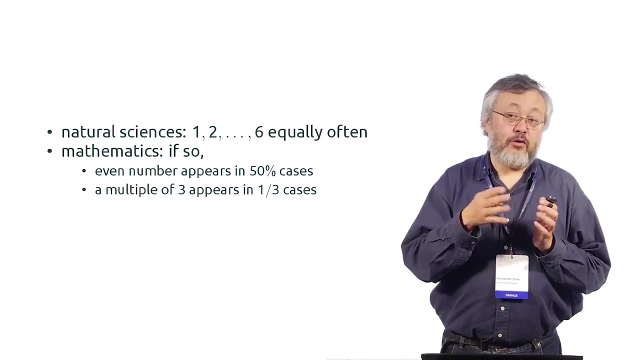 It's an observation And mathematics can make some conclusions, But of course what we will say, this is our trivial conclusion. So, for example, we can conclude that even number two, four, six appears in 50% of cases And a multiple of three or three or six. 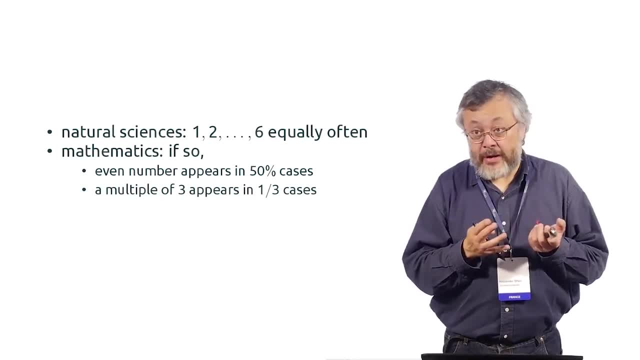 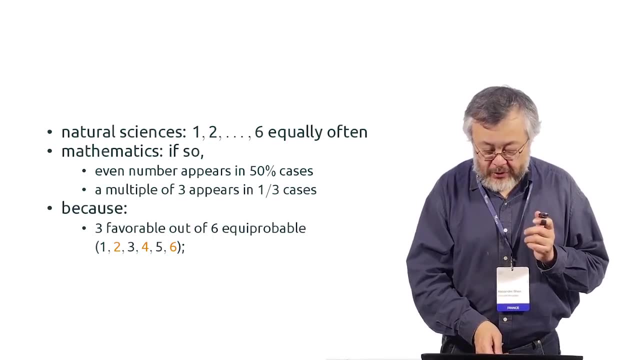 appears in just one third of cases. Why? Because it's very easy. We have just six outcomes: It's one, two, three, four, five, six. And if we want to get an even number among these six outcomes, 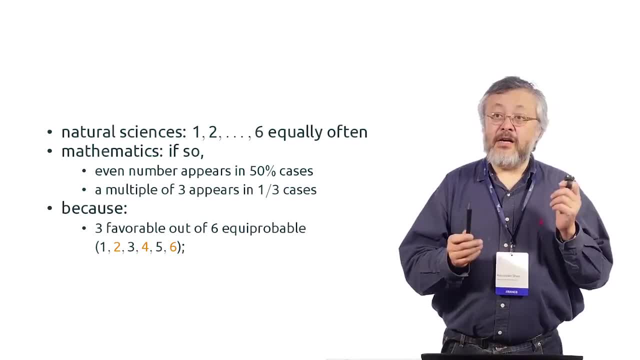 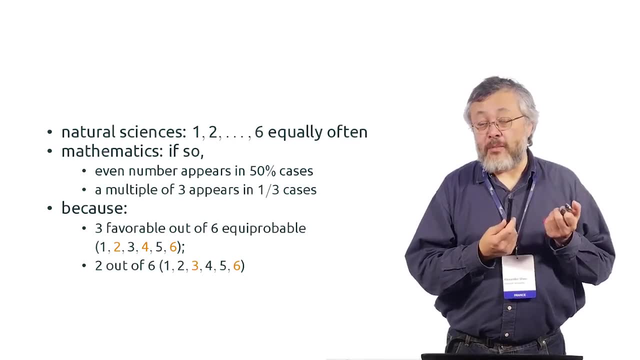 there are three favorable outcomes: two, four and six, So we have three over six, which is 50%, And for multiple of three, we have two over six. We have two favorable outcomes, three and six, So we get one third. 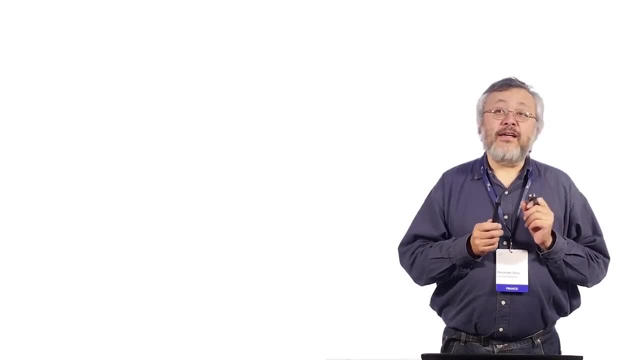 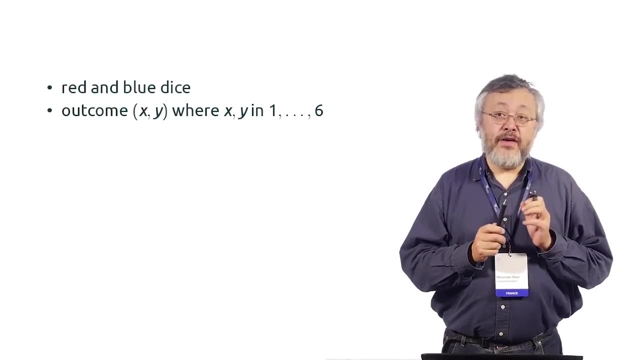 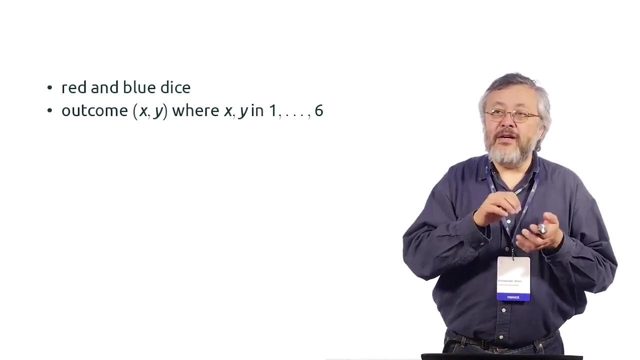 Trivial. What is not so trivial, it's what happens if we roll two dice. So imagine we have red and blue dice And then if we roll them or if we do some other way, make them produce random numbers. then we get an outcome. 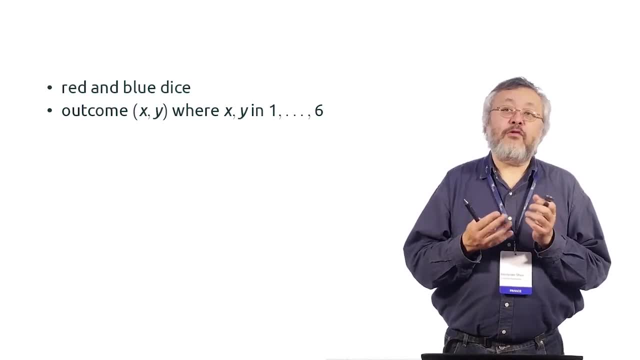 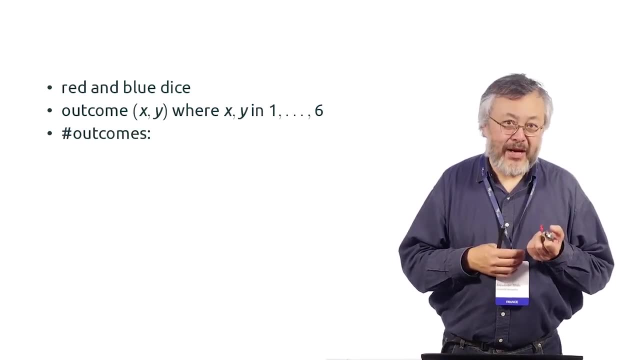 which is a red number and blue number. Each of them, for example, x is red and y is blue, And each of them is between one and six. And how many of them do we have? If you remember something from combinatorics, 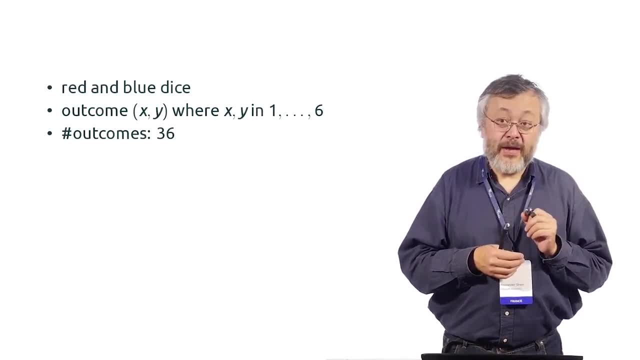 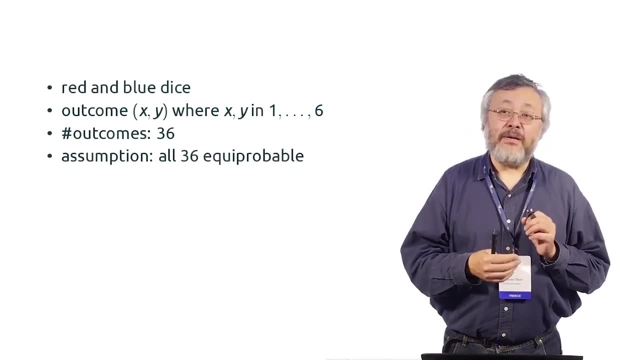 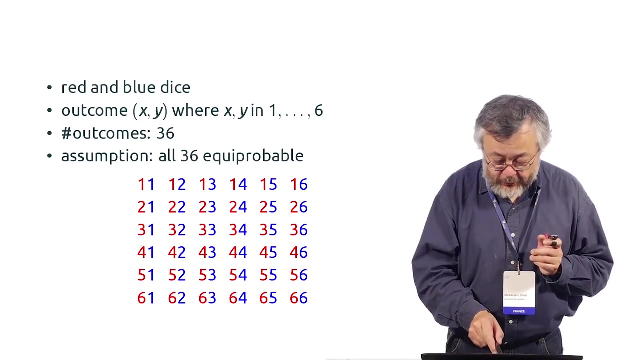 part of the course, you will tell immediately that it's 36.. And even if you don't remember, you can just write all 36 outcomes and believe that they are equi-probable. So this is a table So red. you see this, for example, 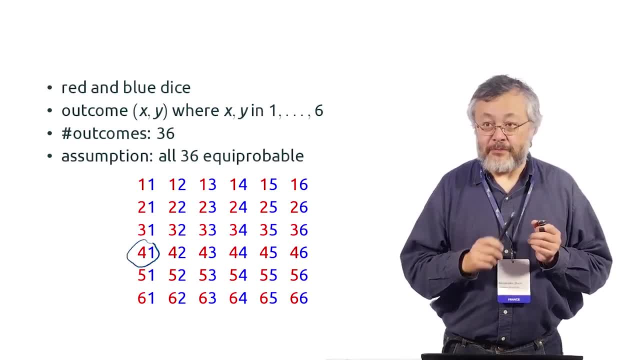 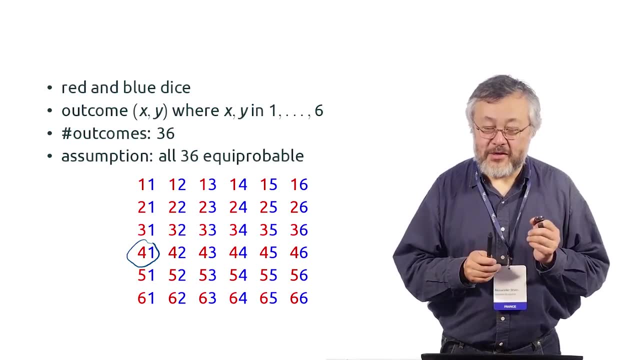 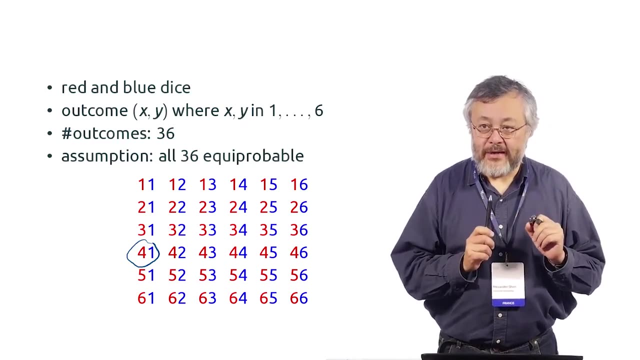 four on the red dice and one on the blue dice or whatever. There are all possible combinations. If you don't believe me, you can count all the numbers here and you get 36. And the assumption is that they all appear equally often in the real world. 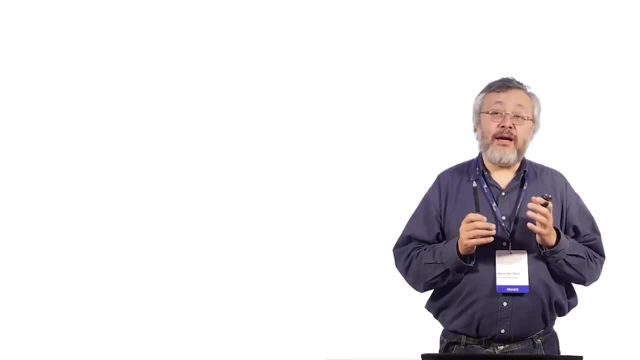 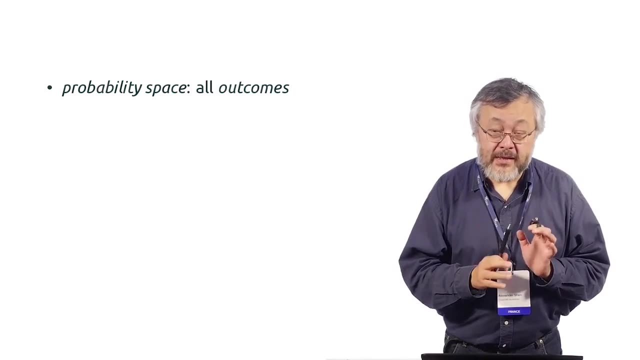 So if we assume this, we can compute the probability. So let me explain the language of probability theory. So there is something which is called probability space. It's just the set of all outcomes. So in our case we have 36 outcomes. 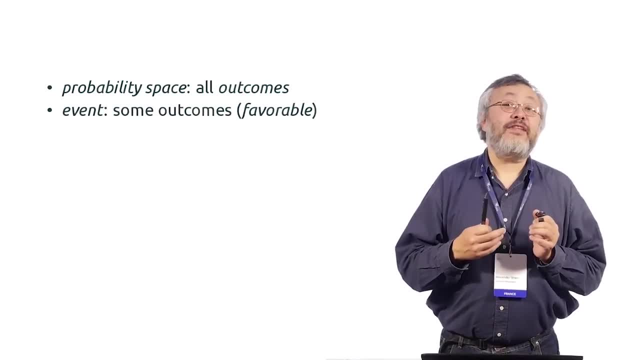 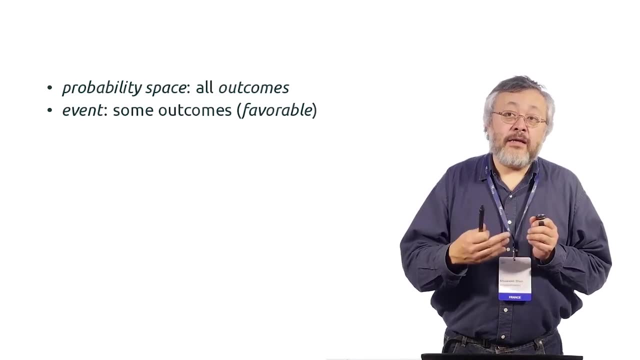 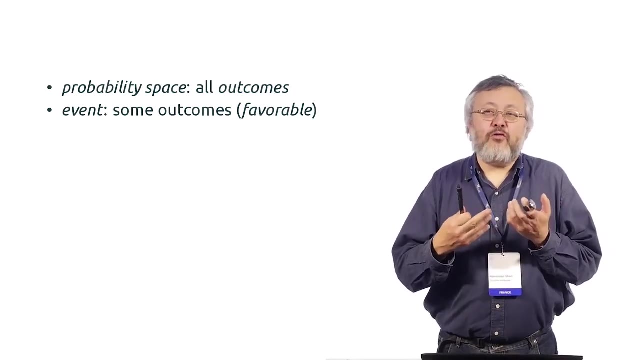 and they form probability space. Also, there is some event, something. this is a property of outcome. It may happen or not, And it's a set of outcomes, And these outcomes are called favorable. That's what we want, somehow, Of course. 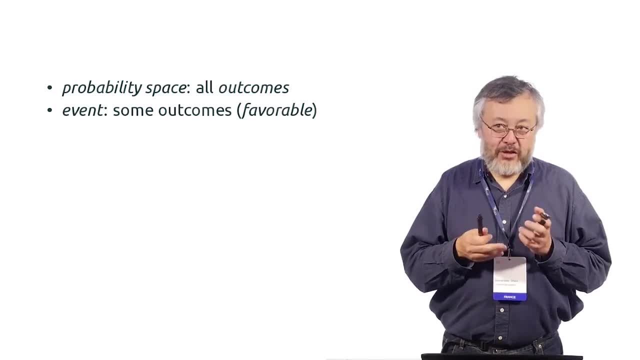 we can consider probability of undesirable events, So it will be an unfavorable account. But just this is a kind of language used. So if we have an event, we call the outcomes from this event favorable. So for example, imagine we have an event. 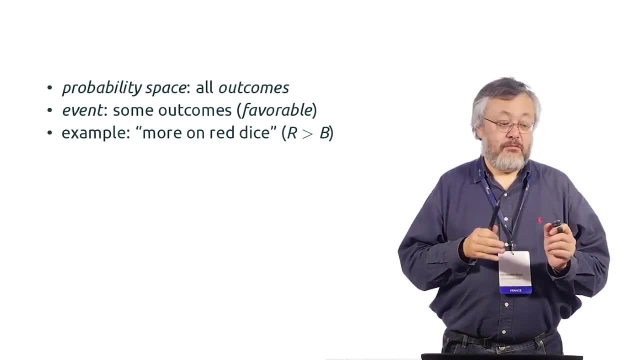 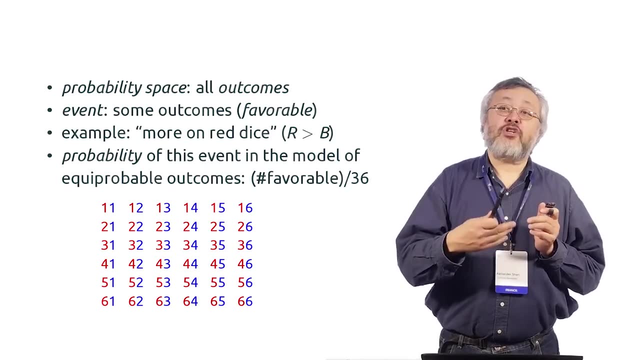 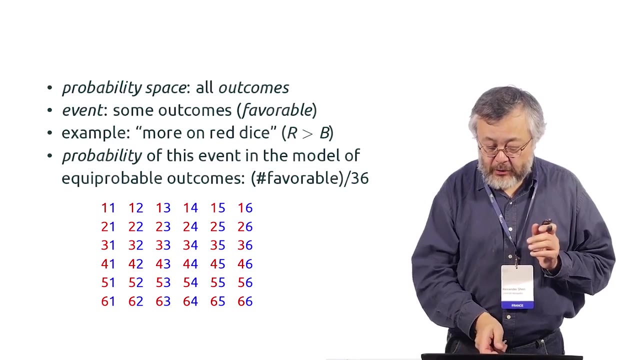 that the red number is bigger than the blue number And we want to compute the probability of this event. And probability is just the fraction of these outcomes in a long series. So if we believe that all 36 will appear with the same frequency, 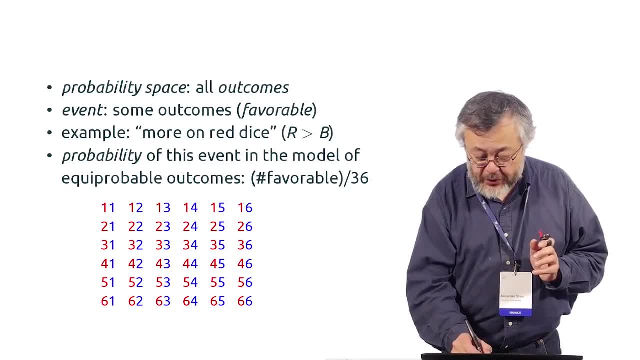 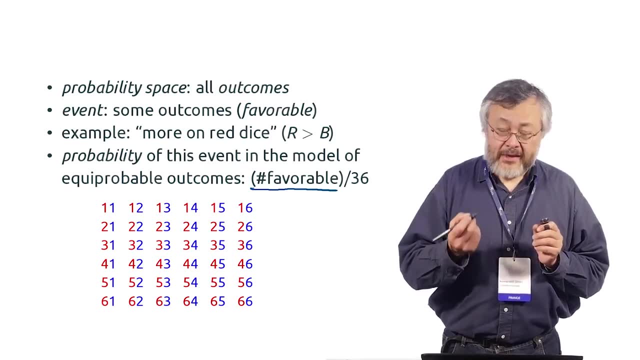 we just want what we should do: we should compute the number of favorable outcomes and divide by 36.. So where are favorable? where the red is bigger, red number is bigger. So here, here, here, here, they are equal. 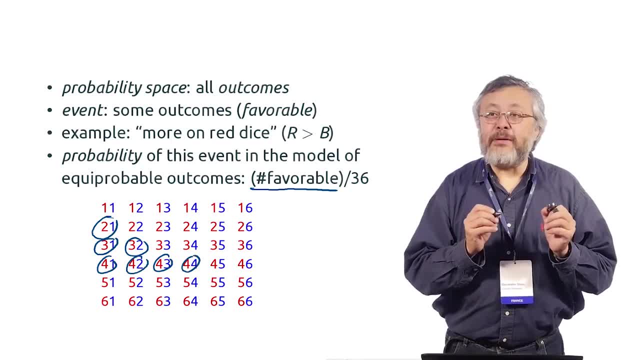 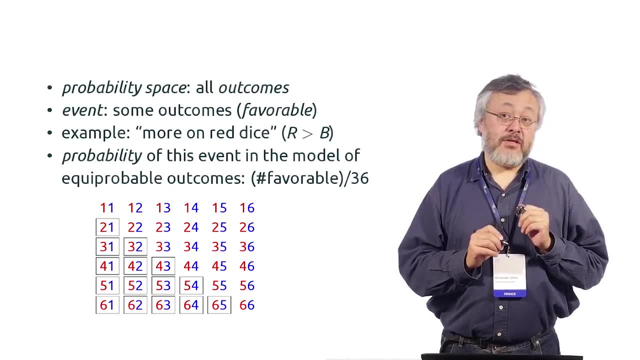 So this is all of this. No, I think I prepared a nice picture, Yeah, With boxes. So these boxes show favorable outcomes, And then you can count them: 1,, 2,, 3,, 4,, 5,, 6,, 7,, 8,, 9,, 10,. 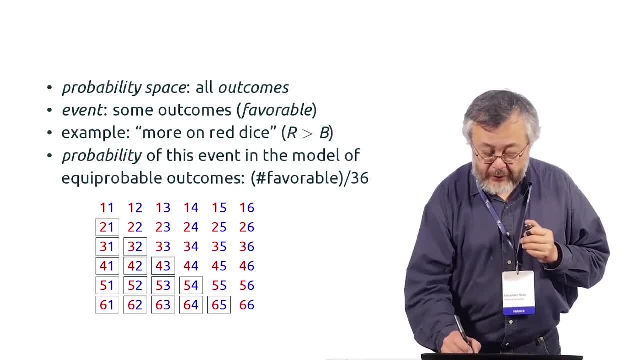 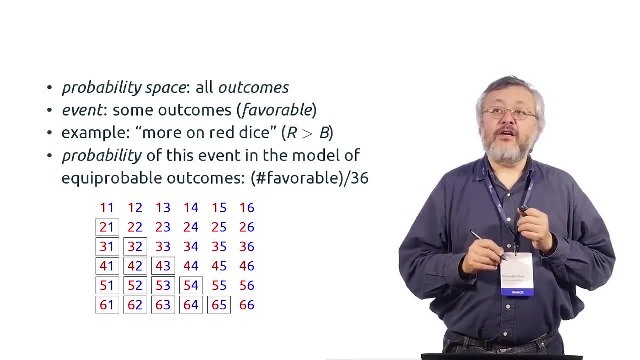 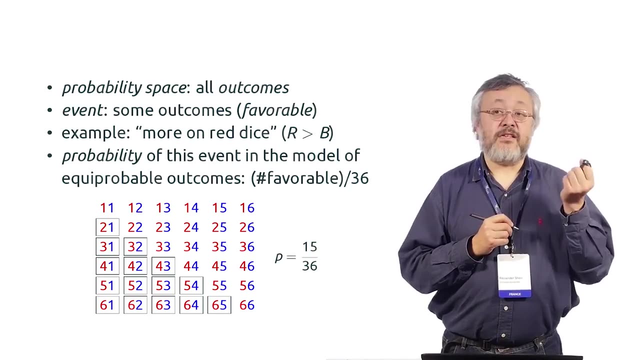 11,, 12,, 13,, 14,, 15.. And so we get 15 over 36.. We know that favorable outcome will in the long run form 15 over 36 fraction. This is called the probability of the event. 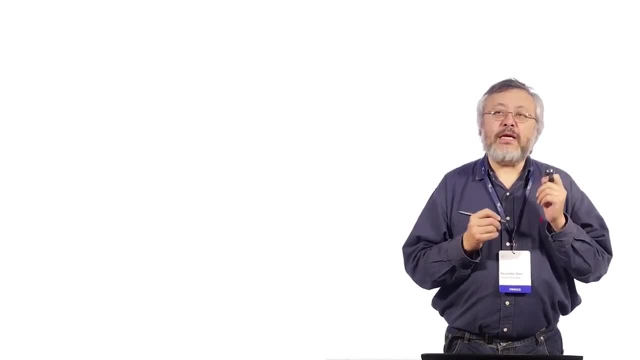 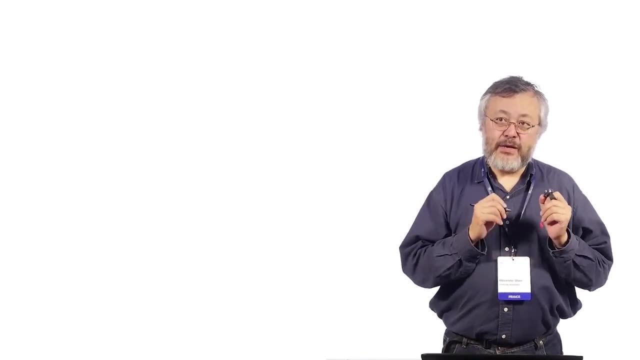 What is very important, that somehow we we can. it's called independence. We assume that red and blue dice are independent. Let me explain what does it mean. So we have 36 outcomes and we believe that they are appear equally often. 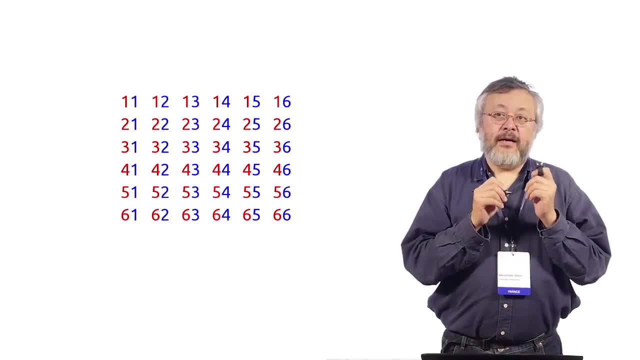 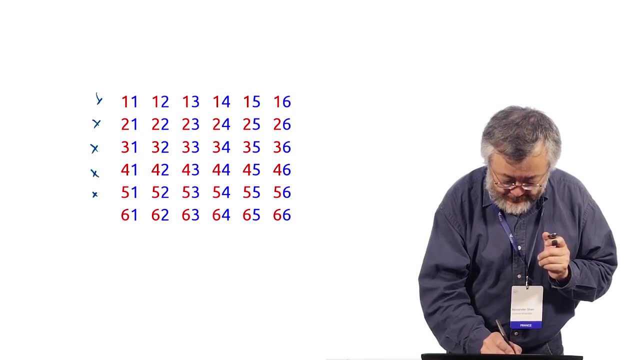 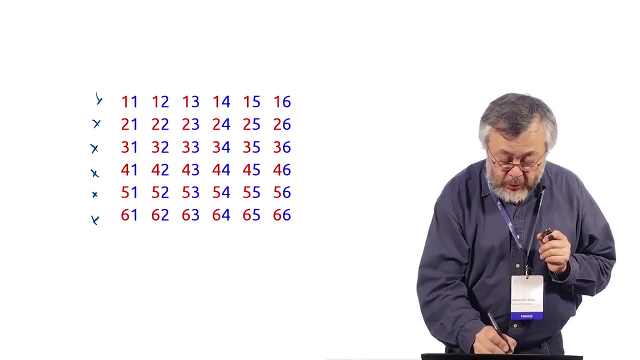 So red dice can give 1,, 2,, 3.. So there are this rows, We can have 1,, 2,, 3,, 4,, 5, 6.. It's equally often, And also blue dice appears with 1,, 2,, 3,, 4,, 5, 6.. 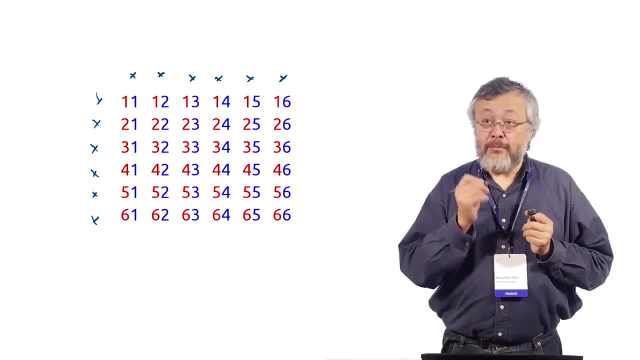 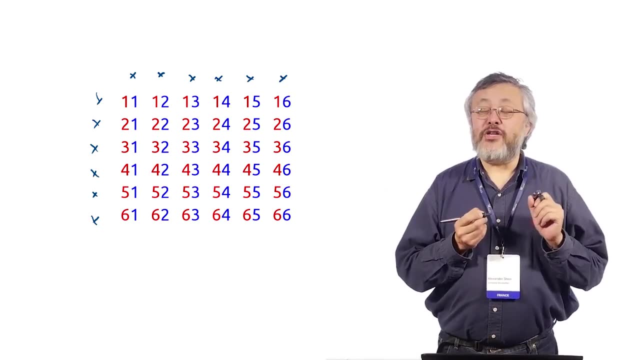 And this, this is, these cases are equally often, But this is not only. it's very important things that they are also independent. For example, imagine some magic, magic dice which always, for some strange reason, red and blue show the same thing. 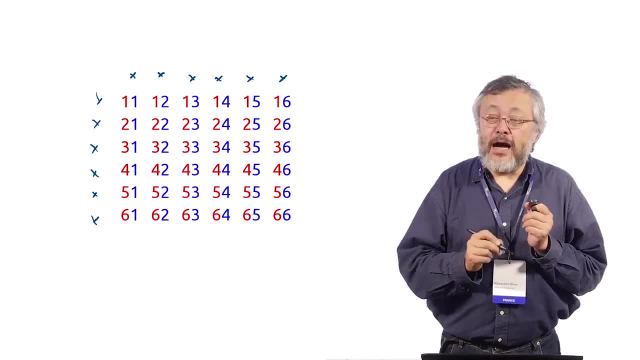 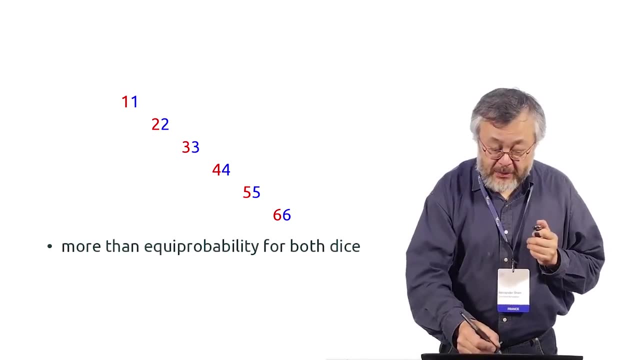 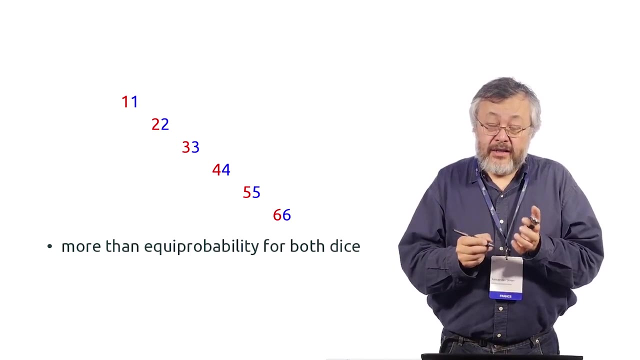 And then, of course, we almost all the outcomes disappear. What we have is something like this: This is the only six possibilities, And these six possibilities are equally probable. And then, indeed, the red coin, the red dice, is okay in isolation. 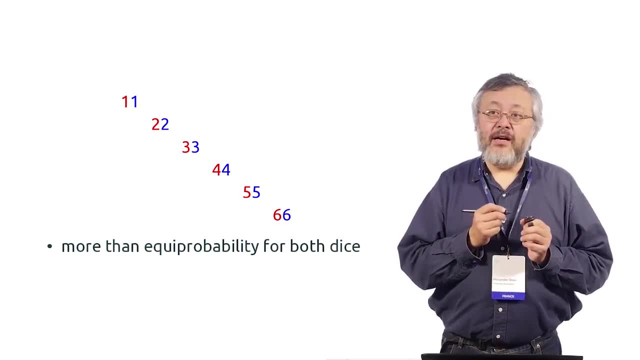 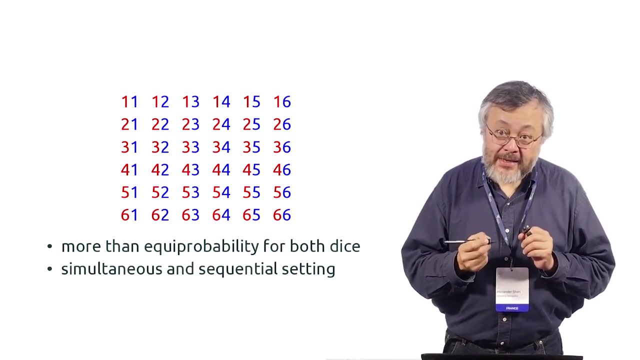 and blue is okay in isolation, But of course all our theory doesn't work because they are somehow dependent. That's the language of all the theory. We will return to this dependence question later. So independence is somehow more than its probability for both dice. 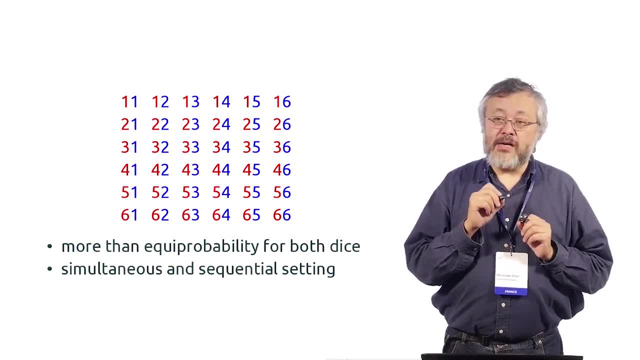 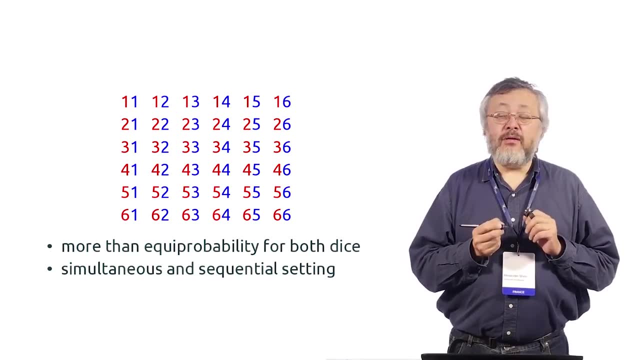 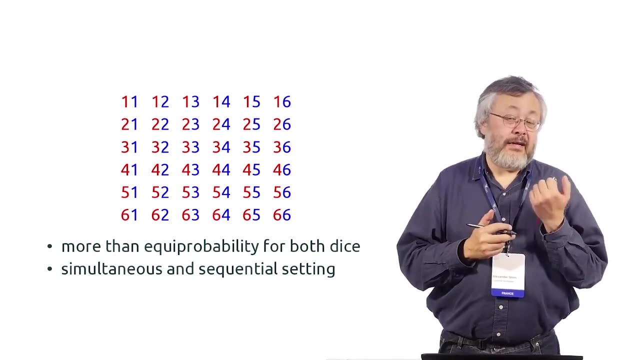 We assume that all 36 outcomes are the same, have the same frequency And it actually happens in the real world for many settings. For example, you can toss the two roll the two dice at the same time, Or another thing you can do. 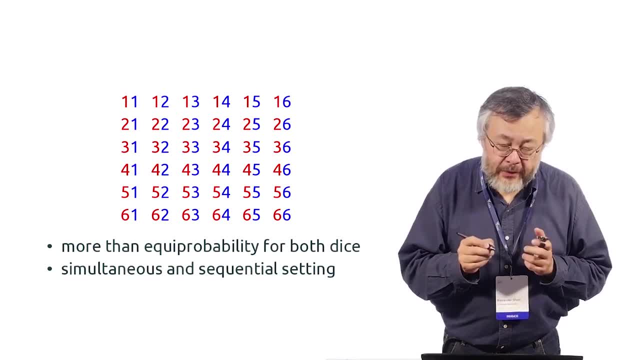 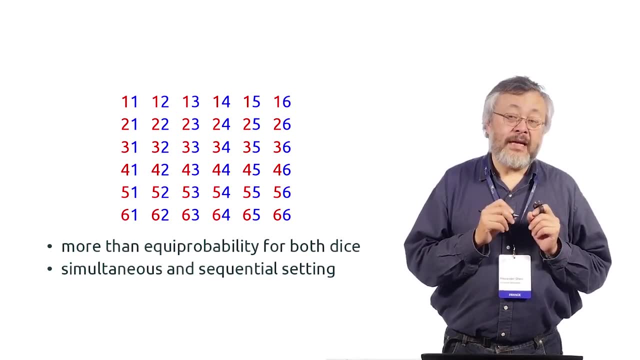 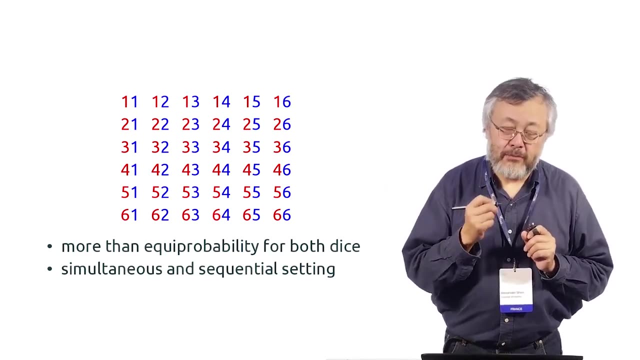 is, you can take first you can roll the red one and then the blue one, Or even you can do even more: You can take one dice and roll it twice And you first. first you get the red number and then you get the blue number. 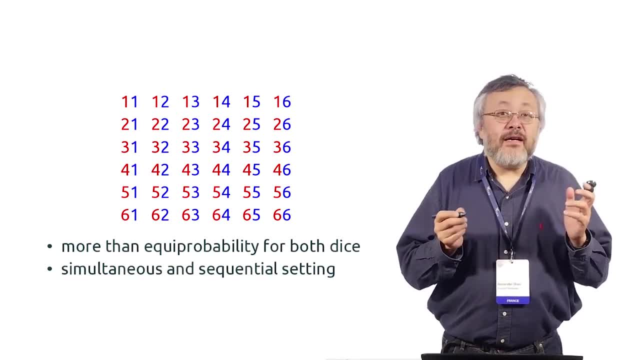 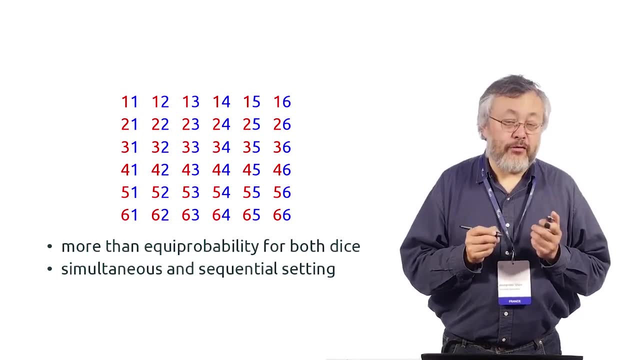 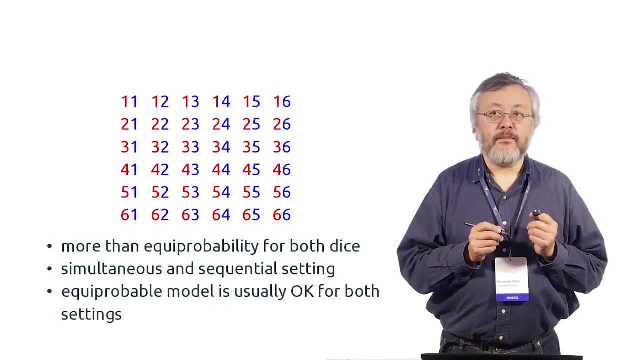 And in all three settings actually. in fact, in the real world all combinations will appear equally often. This is observation about the real world, But then we can compute the probabilities as we have done in our example. So you can. this is again the division. 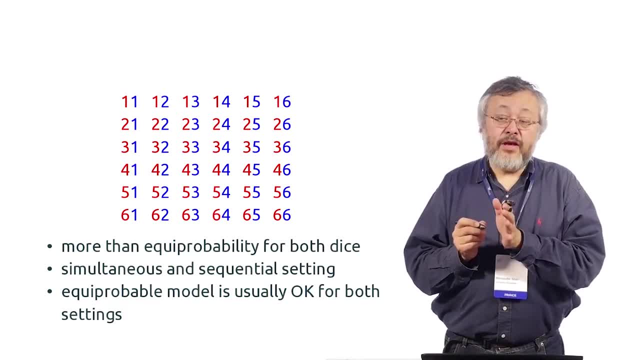 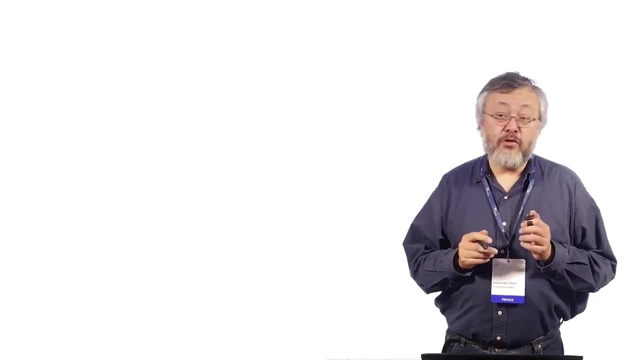 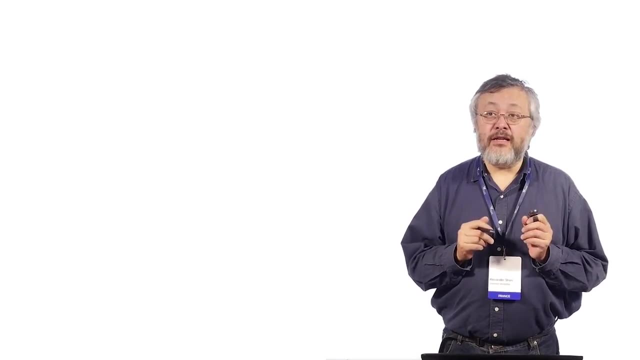 Equiprobable model happens in the real world And then mathematicians use it for computation of probabilities. Now we consider other examples of probability spaces. We will have more later, But just to illustrate the notions let me show some. So first is the sequence of coin tosses. 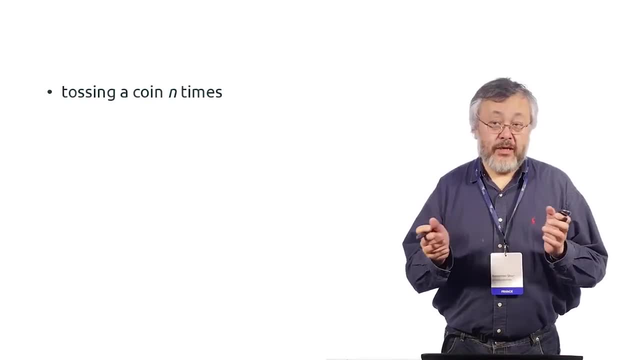 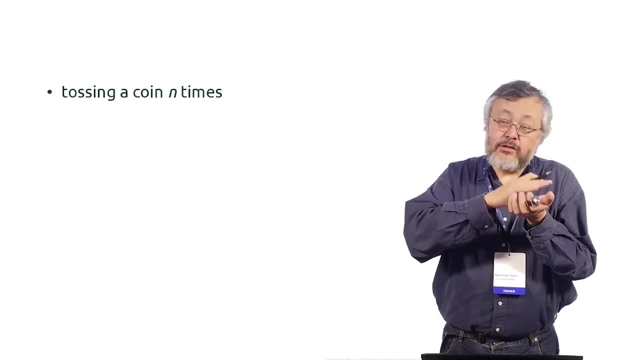 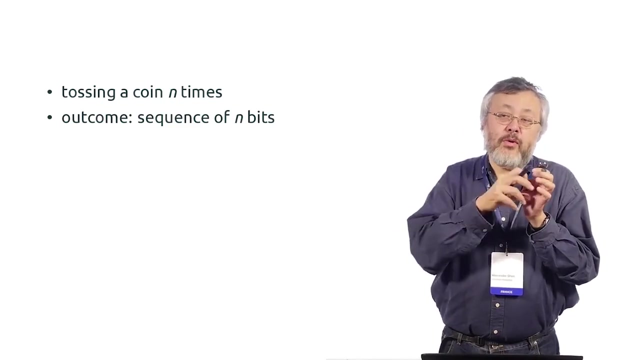 So imagine we toss a coin n times. n is some probably large number. So what is then the outcome? We just write down heads and tails of zeros and ones. So the outcome is just a sequence of n bits which show the outcome of first, second and so on. 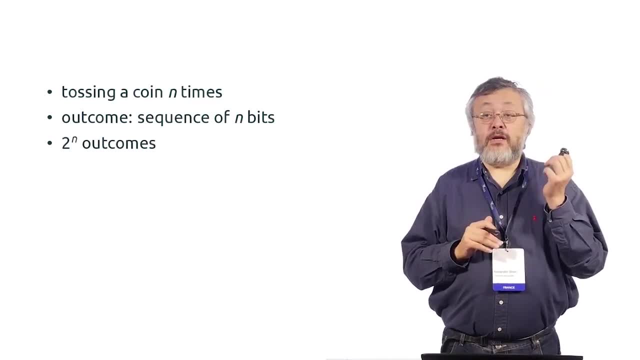 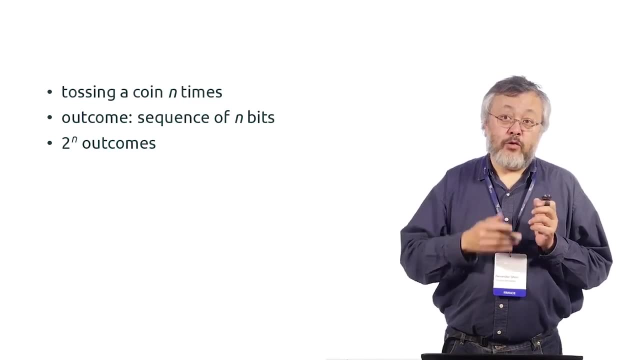 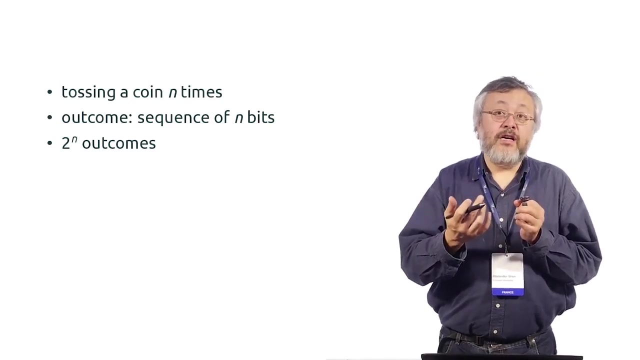 coin tosses And how many we have of them. If you remember combinatorics, you know that it's 2 to the n, So each new bit increases the number of possibilities twice. So you had in total you have 2 to the n. 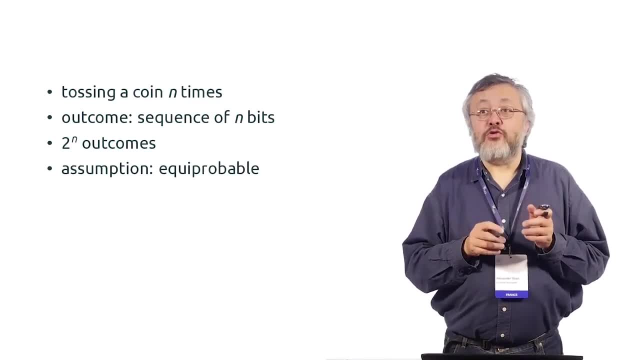 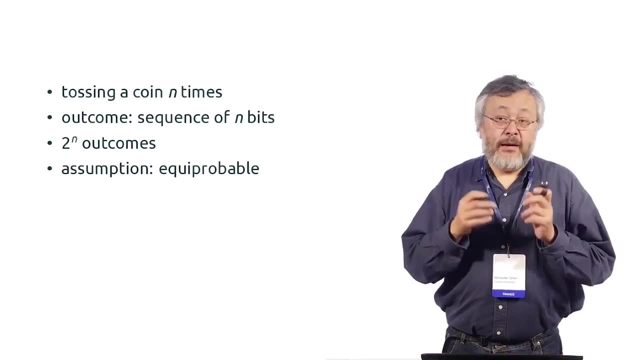 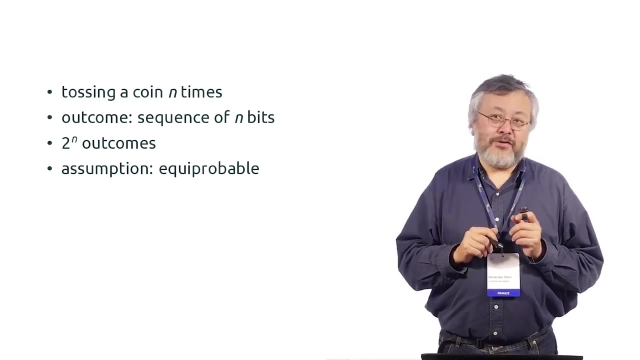 And the assumption which usually is used in probability theory that all 2 to the n outcomes have the same probability appear with the same frequency in a long series of experiments. And it's not so obvious really, Because imagine we toss, I don't know. 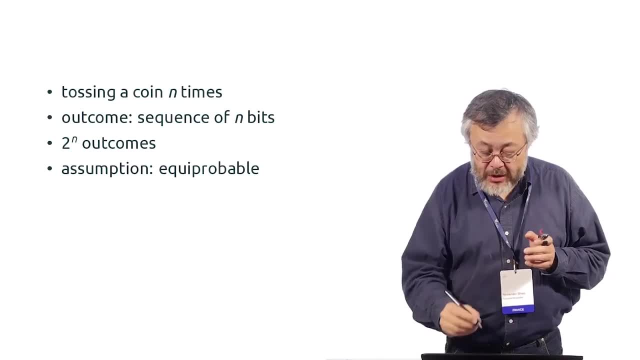 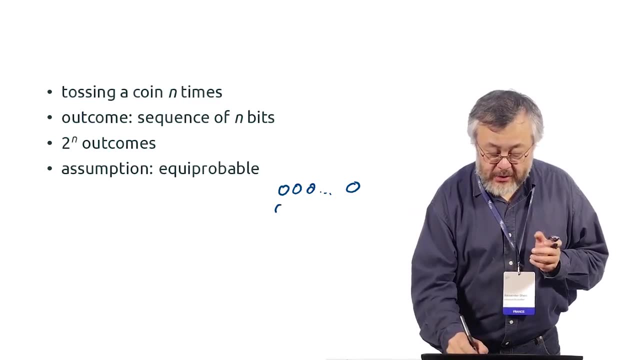 the coin 10 times And one of the possible outcome is just 0, 0, 0, 10 zeros, And another one is something like I don't know: 0, 1, 1, 1, 0, 1, 1, 1, 0, 0,. 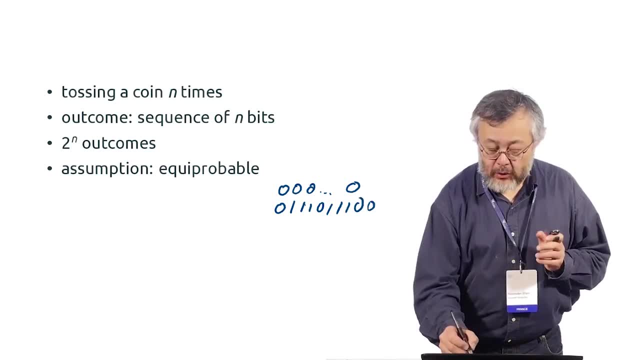 1, 2, 3, 4, 5, 1, 2, 3,. yeah, So this account 10 zeros and this, So what do you think Is which of them will appear more often? 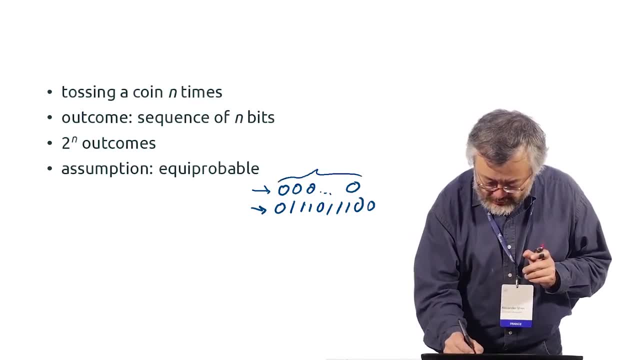 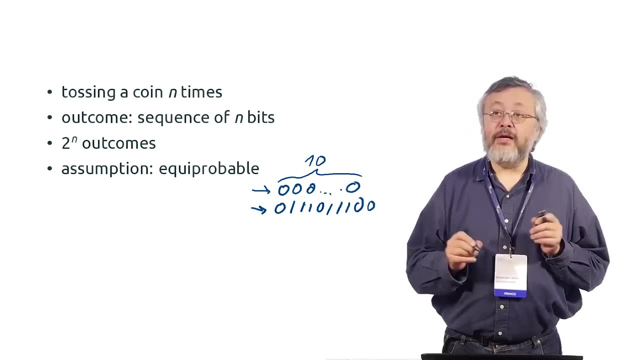 No, it's 10 zeros, So you should. this is the dots are for zeros only. So there are 2 specific outcomes: 10 zeros and this one. So which of one will appear more often in the real life? And you know. 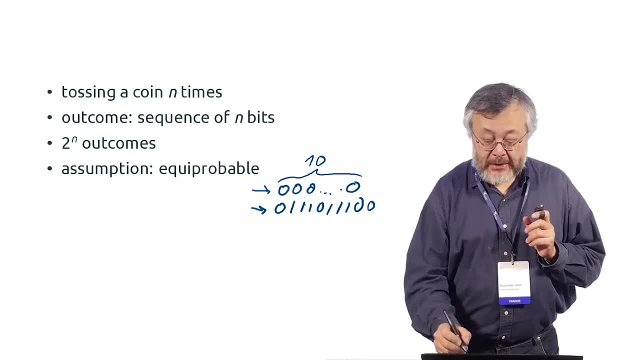 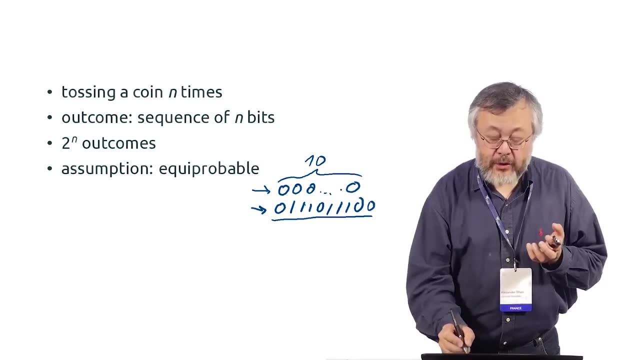 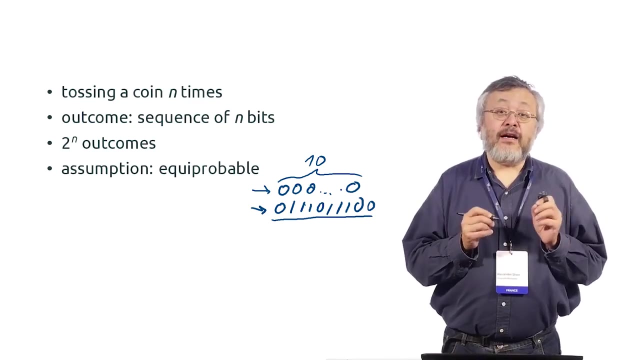 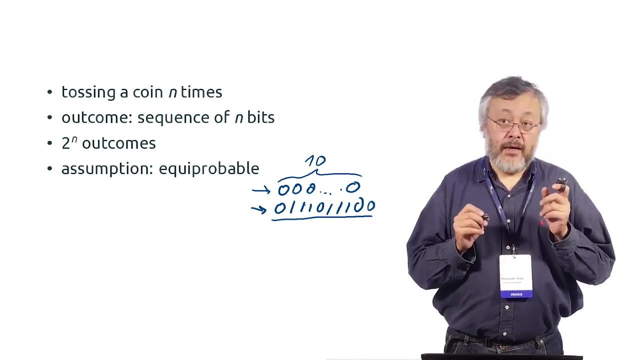 maybe some people believe, probably, that this is more probable because, you know, zeros is something strange. You have y, always 0. But actually the current understanding of the real world is that these 2 outcomes will appear equally often In the real world. 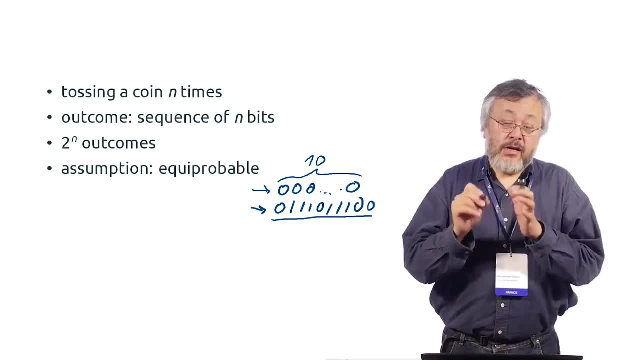 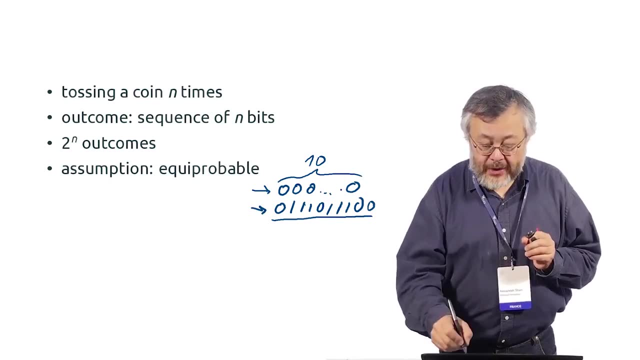 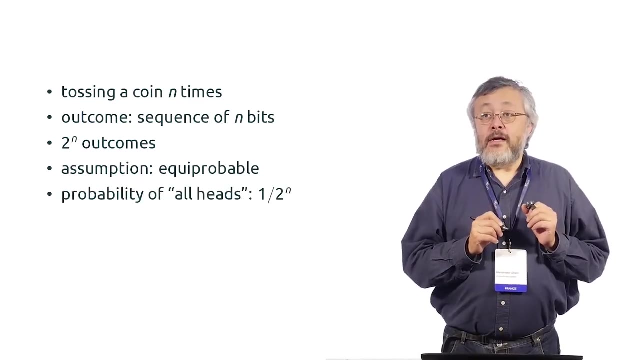 But this is about real world and mathematic assumption starts here. So we agree in advance, before computing some probabilities, that they are all the outcomes are equally probable, appear equally often. So, for example, probability of all heads for n bits: it's just 1 over 2 to the n. 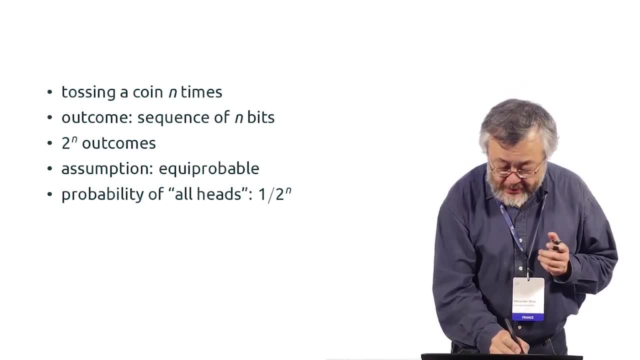 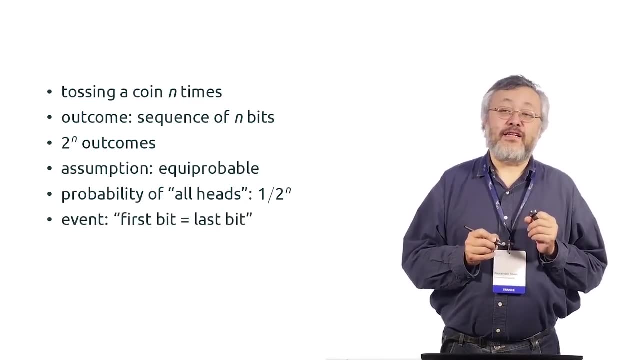 When n is the number of coin tossing and we have 2 to the n out. what comes in bit are interesting when we do 1 and 1.. You can consider more interesting events. Imagine this event is the first bit is equal to the last bit. 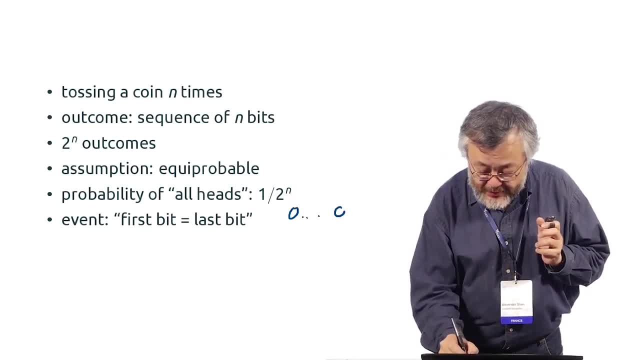 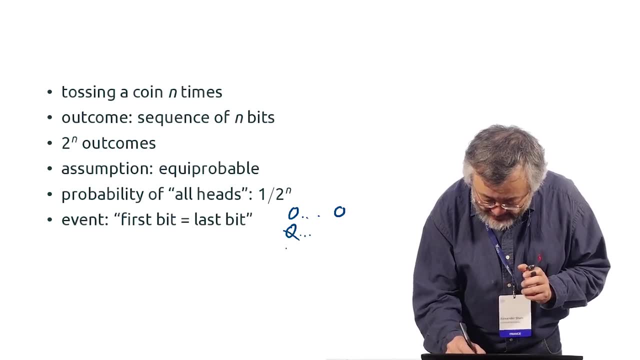 So, for example, this event happens if we start with 0 and end with 0, and also happens when we start with 0 and start with 1, sorry- and end with 1.. So what is the probability of this event? 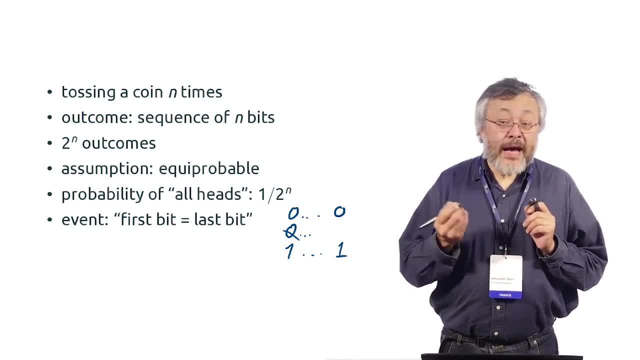 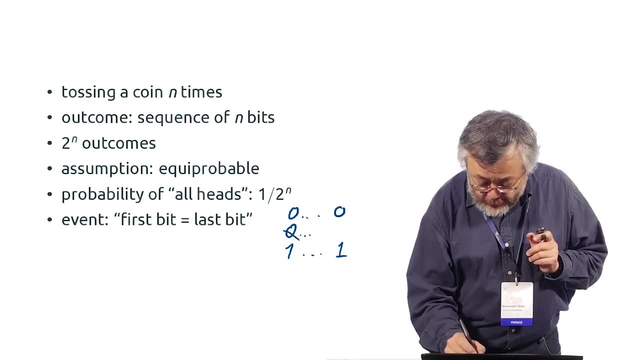 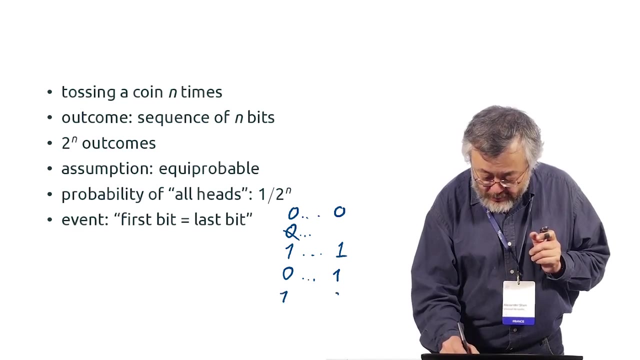 What do you think? Actually, it's easy to think that it's one half. Why? Because there are actually four possible groups. You can have 0, 0, 1, 1, 0, 1, and 1, 0.. 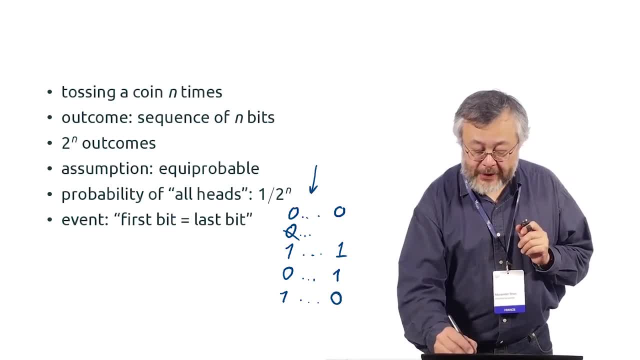 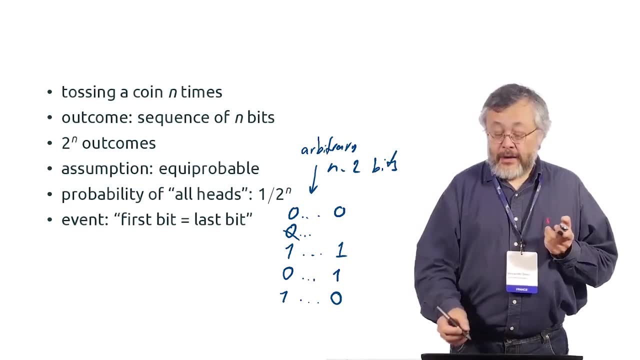 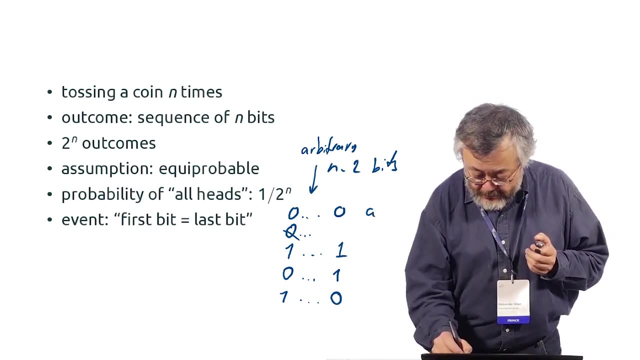 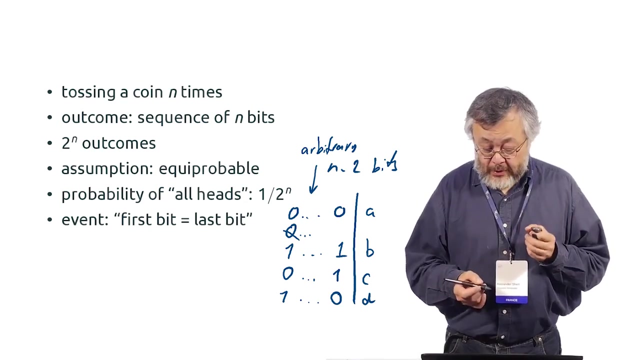 And here in all four groups you have arbitrary n minus 2 bits. So we divide all the outcomes into four groups And these four groups- A, B, C, D- have the same number of outcomes. So each of them 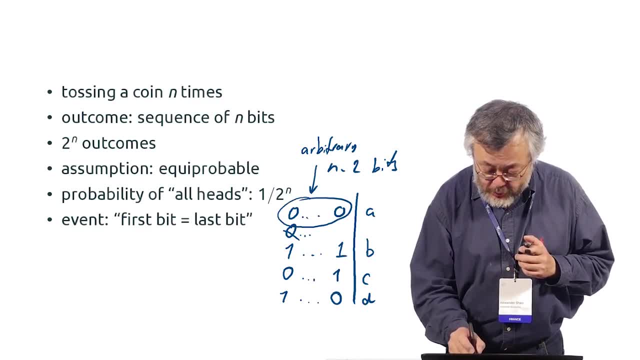 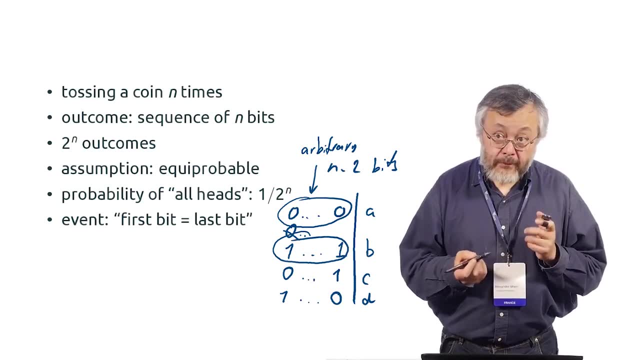 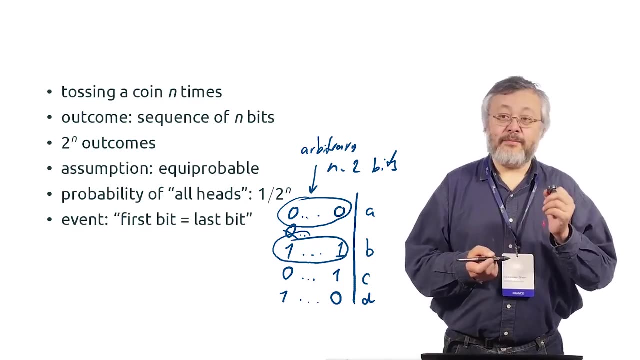 is one fourth of all possible outcomes. So our groups here is just one half. Together it's two fourths. So this event has the probability one half. If you remember combinatorics part, probably you will remember computation like this. And then another question: 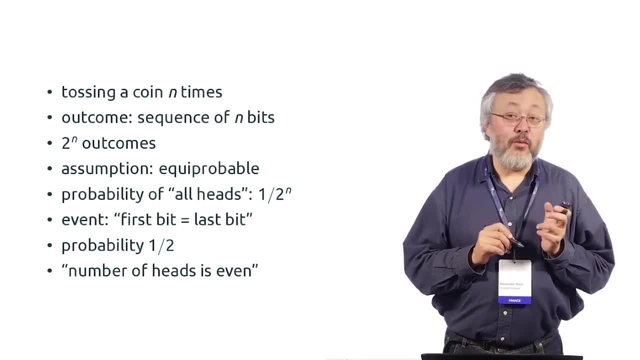 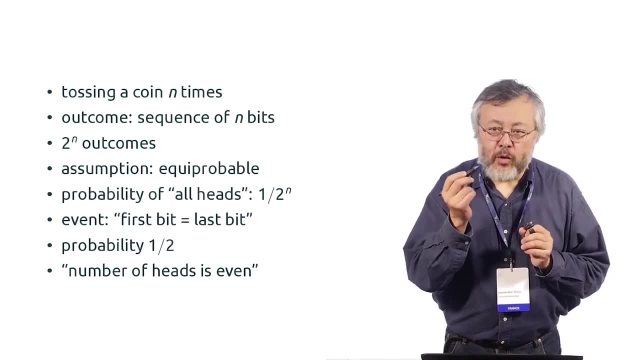 So for this it's probably one half. Another question more difficult, and I will not tell the answer so you can think about it. So the event is that number of heads is even. So if we sum all the 0s and 1s. 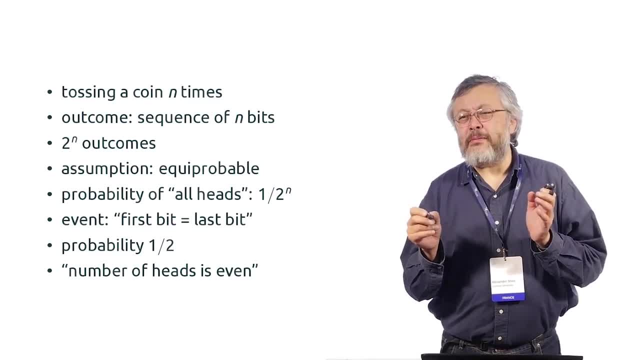 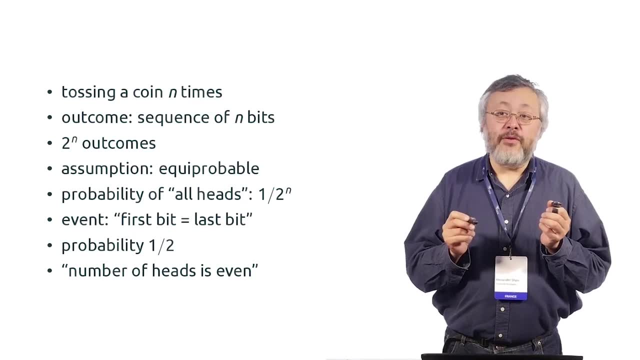 we just have a number or I don't know. maybe it's number of tails. Anyway, it doesn't matter. So the number of heads is even. What is the probability of this event? I will tell you the answer: one half. 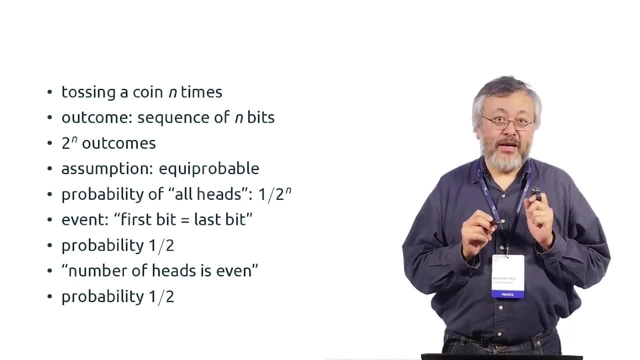 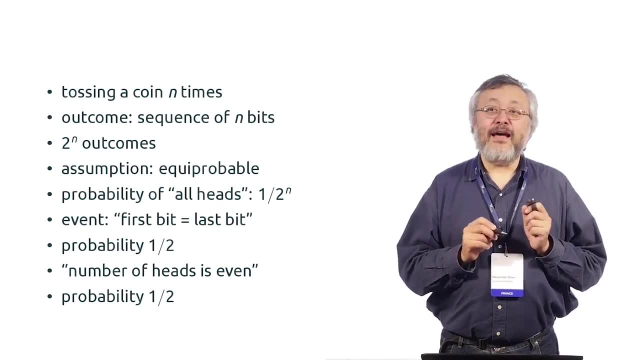 Yeah, it's one half. But what I won't tell you is why it's one half. But maybe you remember something from combinatorics and you can see it immediately. If not, think a bit and you will get. I hope you will get. 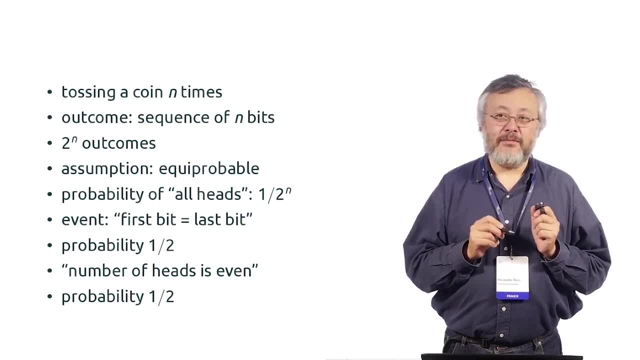 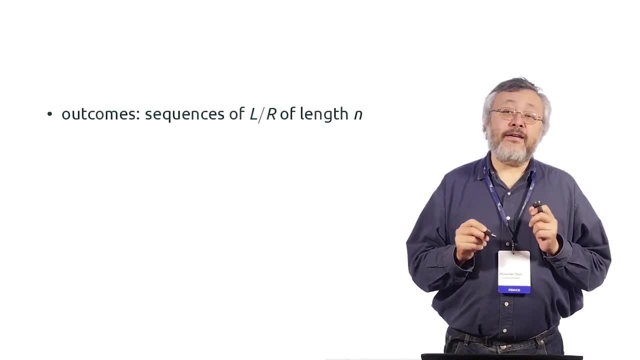 the idea why it happens Again, we can also look at Galton board, And here the outcomes are very similar. It's the sequences of not 0s and 1s and heads as they just left and right, Of course. 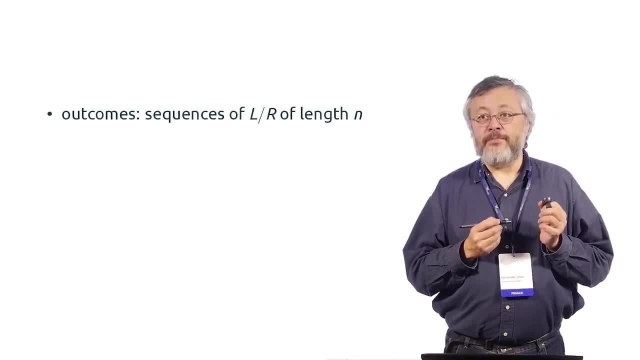 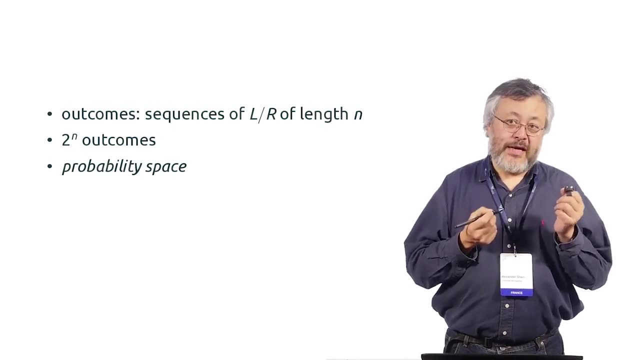 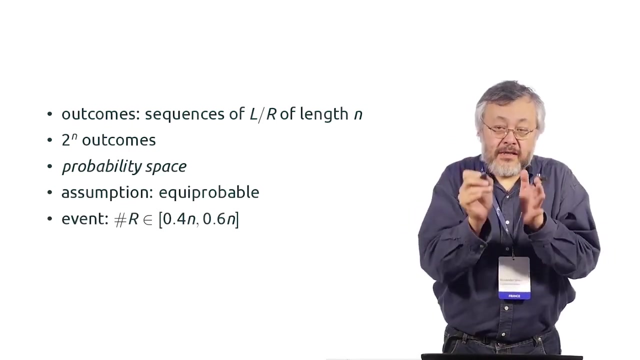 you can use any notation. And again we have 2 to the n outcomes And the probability space is made of all of all these outcomes And if we are interested, they assume to be equiprobable And if we are interested in the concentration event, 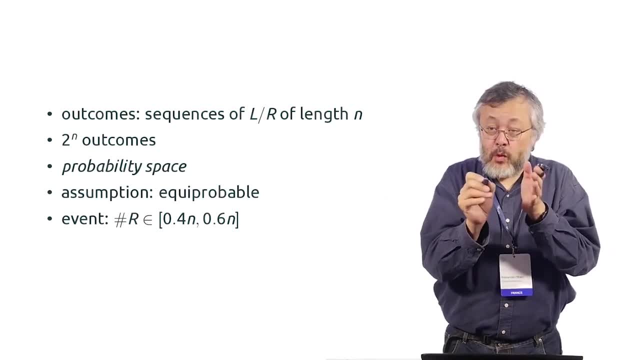 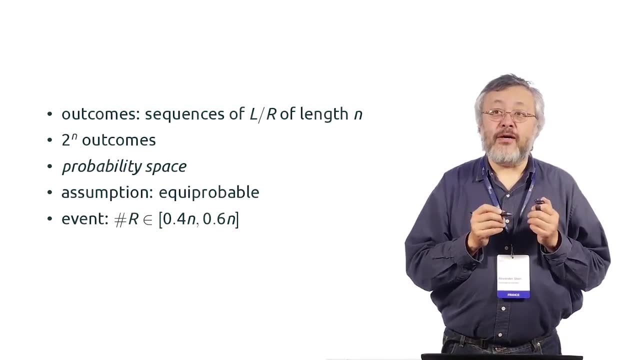 if we want to compute the probability that the bean will end in the middle, we just consider the event that the number of rs in the sequence is between 40% of n or 60% of the total number, And so this is an event. 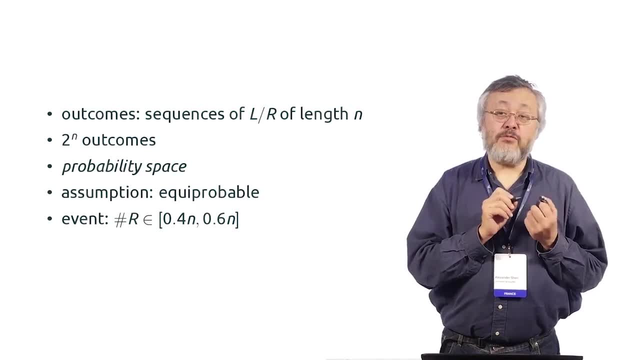 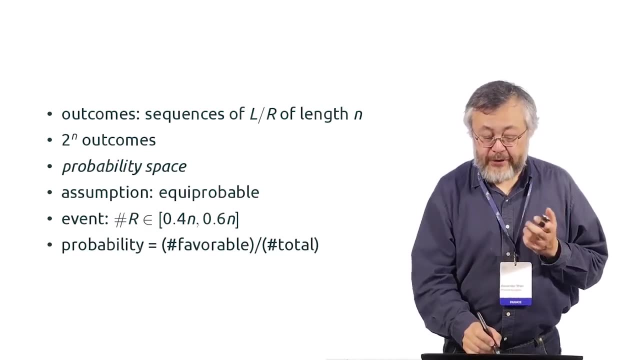 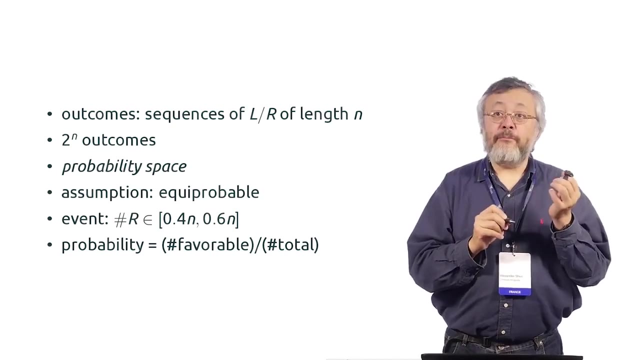 So we need to compute how many outcomes are in this event and divide by the total number of outcomes. So, according to general formula, favorable outcomes are just the outcomes where the number of rs is between 40% and 60%, And so this is the formula. 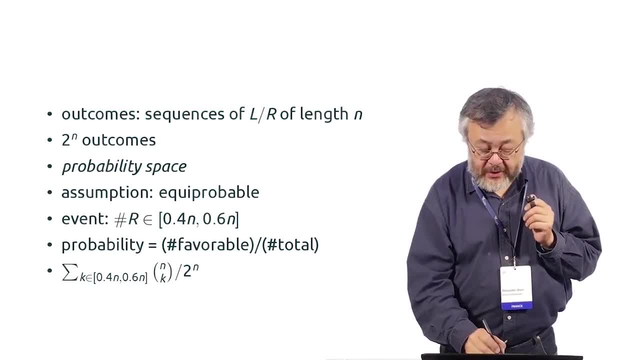 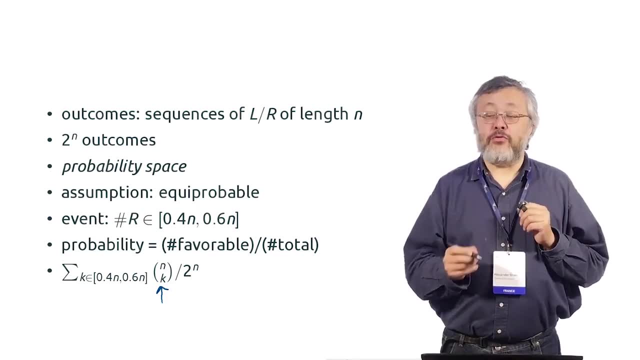 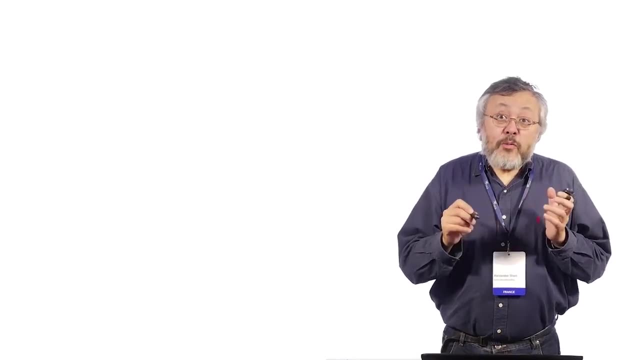 It's the same formula you have seen. This is the number of outcomes with exactly k letters r, And then we make a sum and divide the sum by 2 to the n, And that's what we wanted. So now you probably will say: 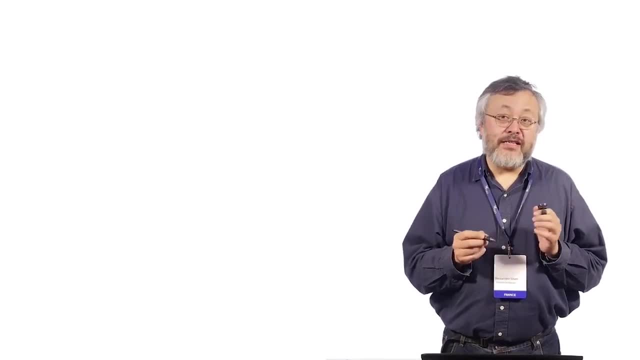 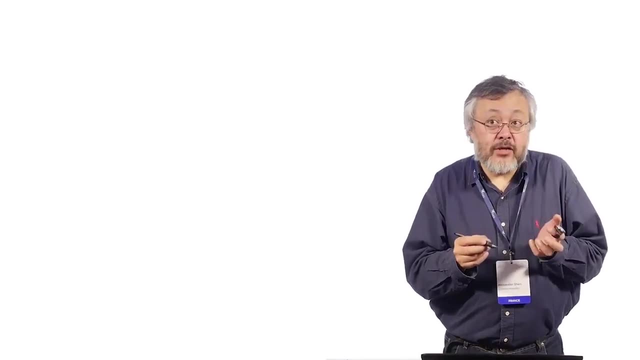 that. why should we learn probability theory? It's just combinatorics in disguise. You can ask about probability of something, or you can just ask about the number of outcomes, And this is essentially the same question in different language. And it's true, and it's mostly true. 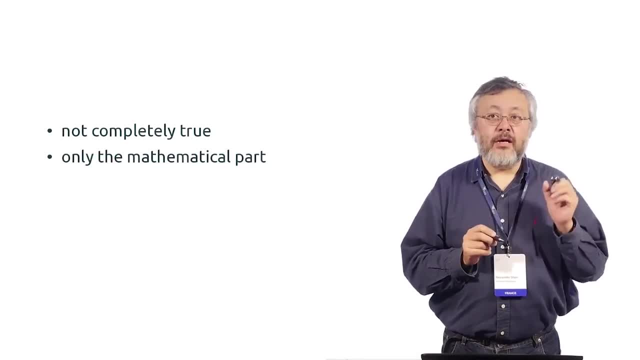 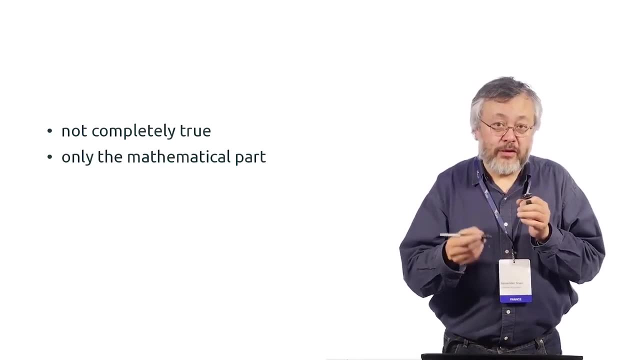 in our course, but it's not completely true in general. So first we speak only about mathematical part. So there is also a question of natural science, which models are good or bad. But we decided it's not probability theory. So for us, 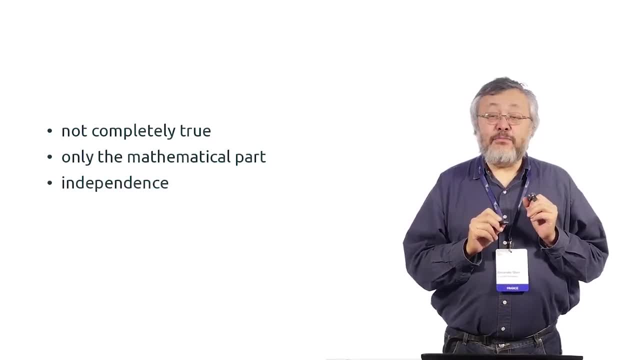 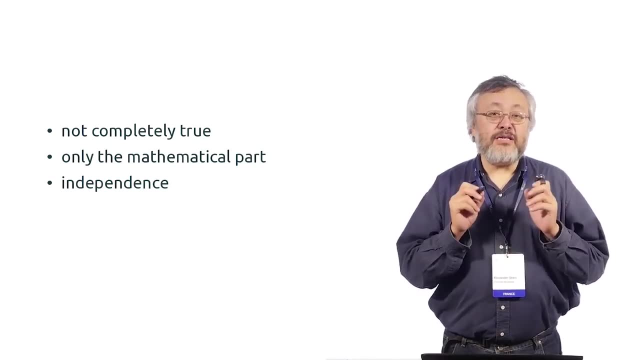 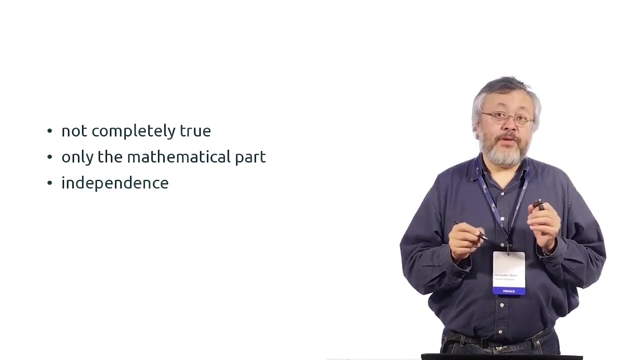 we consider the mathematical part, And mathematically still there are important things. So probability theory cares a lot about this independence thing, And in combinatorics we usually don't speak about independence, We just count things. So if we concentrate, 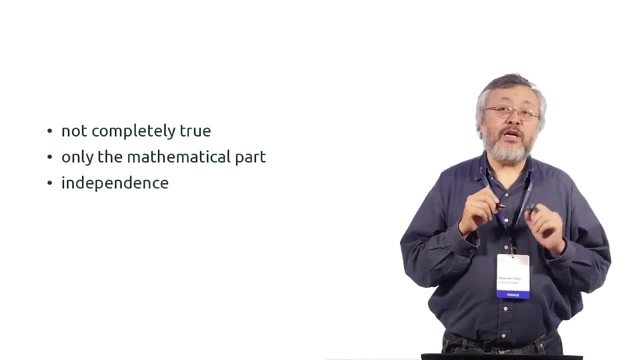 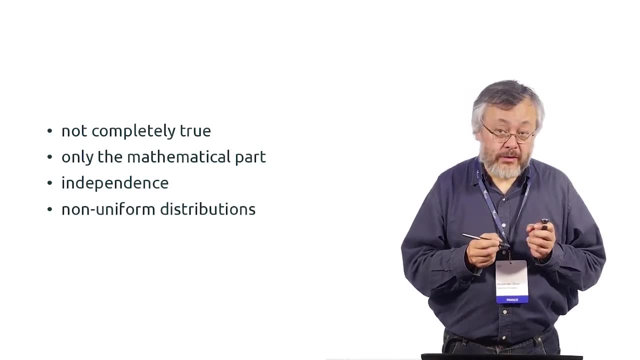 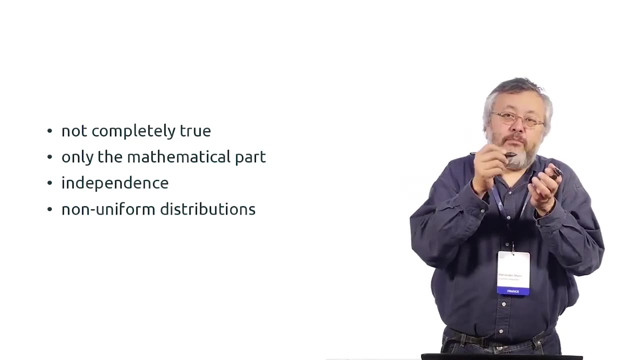 on whether some events are independent or not. this is more about probability theory. Also, if we are interested in finding model for real world, for example, a coin may be different and non-symmetric, or dice can be not, could be one part. 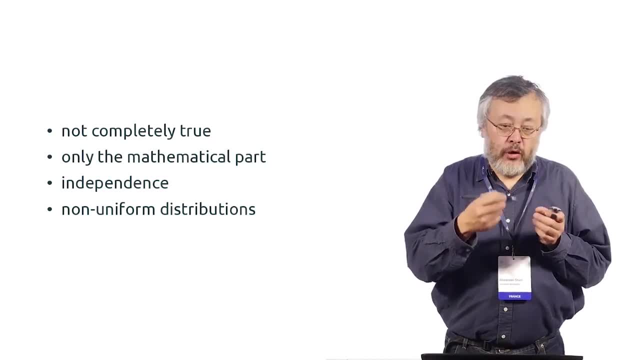 could be here. So then, of course, the thing, not our assumption- that all the outcomes- one, two, three, four, five, six- appear equally often is wrong. So we should somehow consider another models, which are called non-uniform distribution. 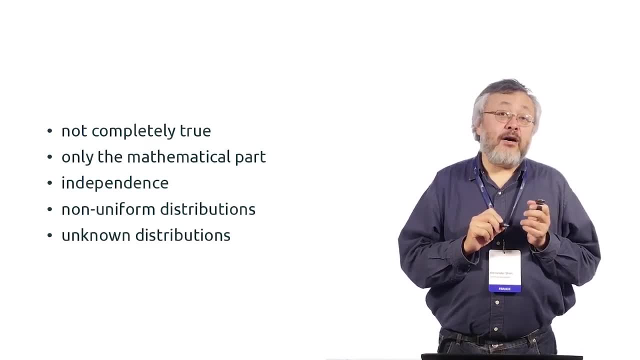 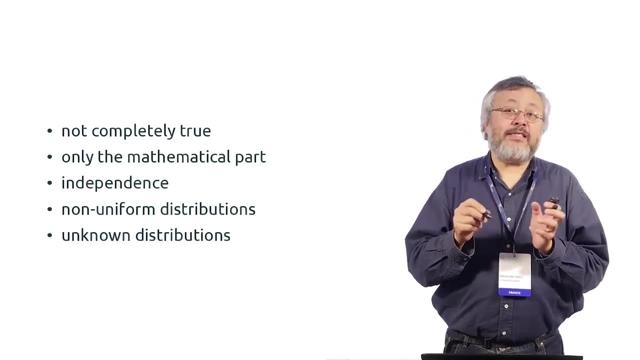 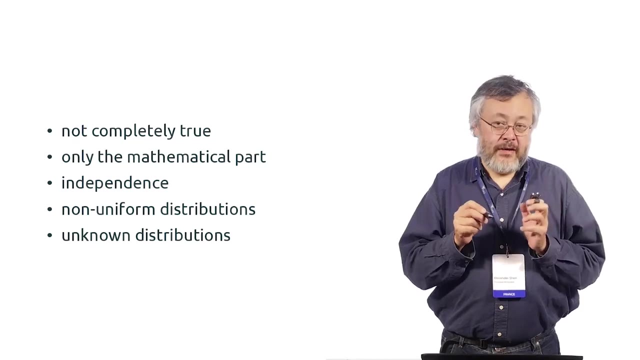 We will speak about this And sometimes we don't know. we want to speak about probabilities of different event, even if we don't know exactly the underlying distribution. So the simplest example: imagine that some event A has some probability. So then we consider: 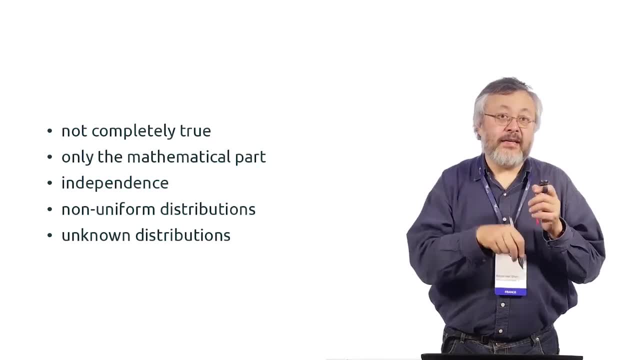 the negation of A, the event saying that A didn't happen. And what is the probability of this negation? Of course negation happens in cases when our event doesn't happen. So it's just the complement. So the probability is: 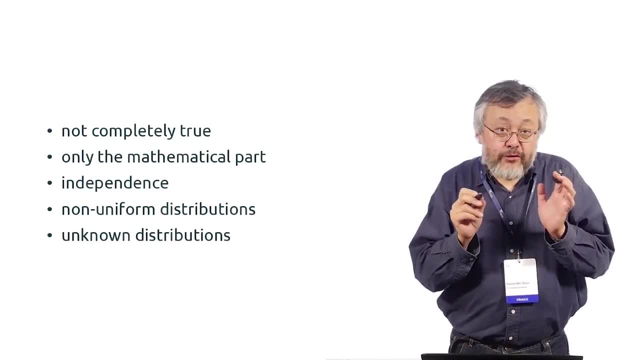 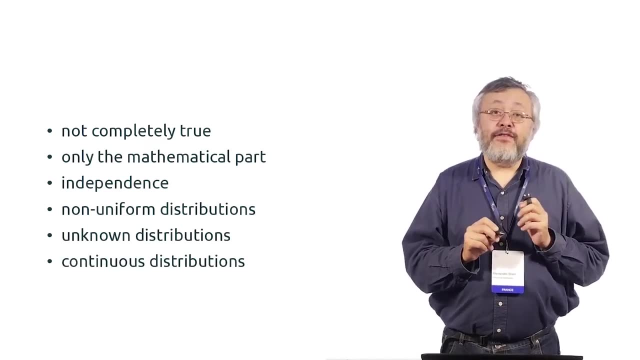 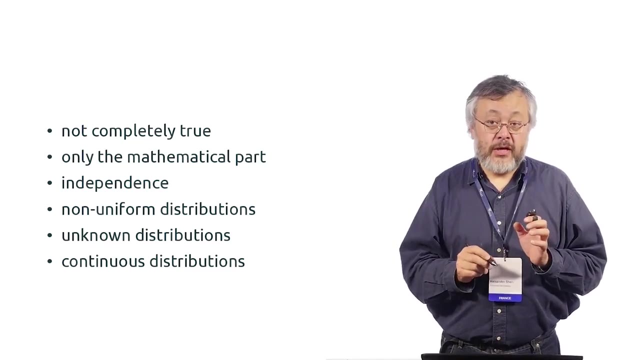 one minus probability of the event. And for saying this we don't need to know anything about underlying distribution. And finally, there is a part of probability theory very important which we completely ignore in our course. It's about continuous distribution. Let me just say one thing. 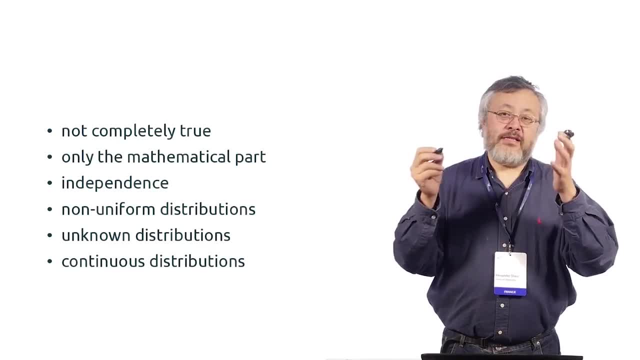 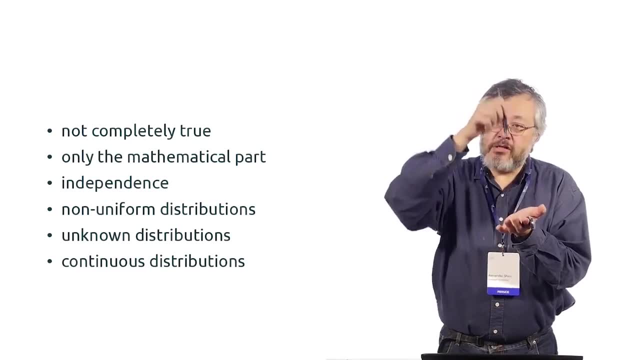 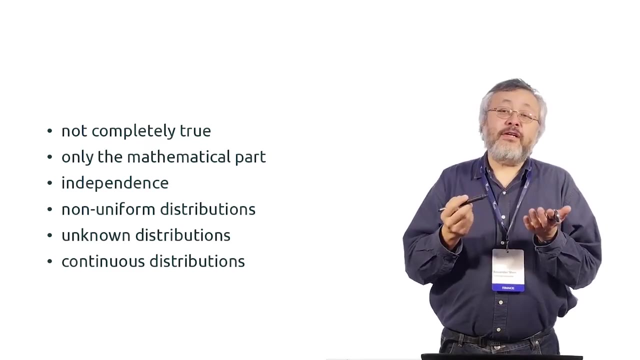 So imagine, I don't know, there is a rain outside and you go with a piece of paper and you see where the first drop falls, And it can fall at any position, But you are interested in cases when it falls into some region. 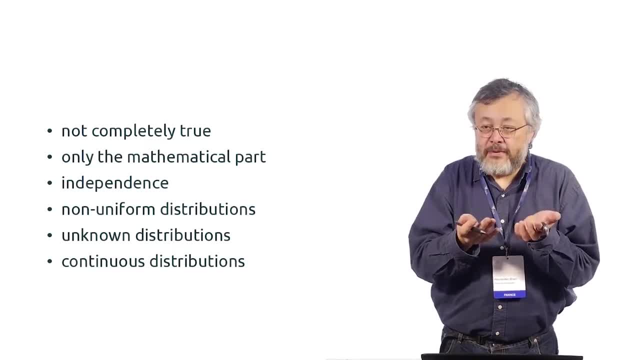 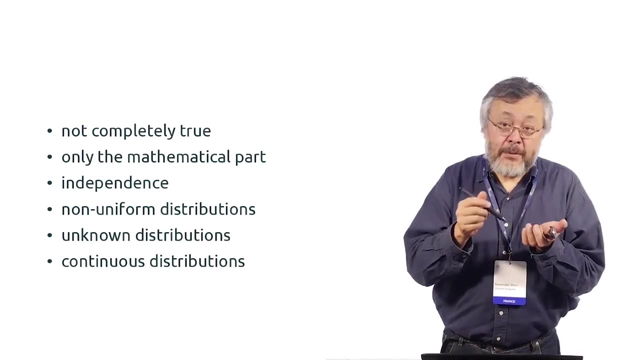 You draw a picture on this paper and you see whether it goes inside the figure or outside, And of course then outcomes are not. there are infinitely many of them. The drop can go in any point on the paper, So you cannot count them. 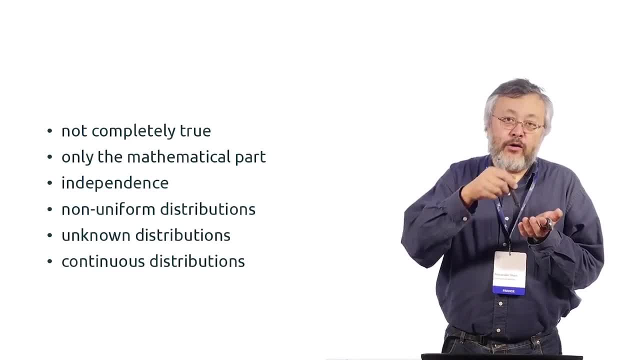 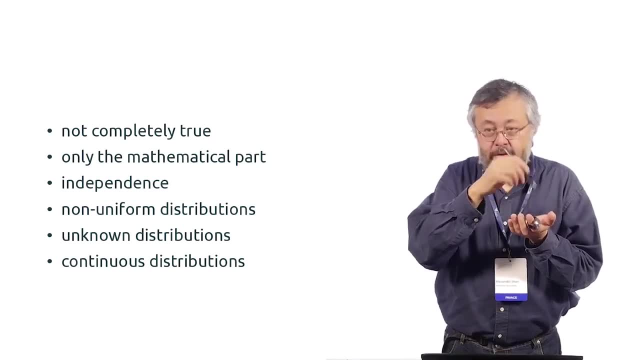 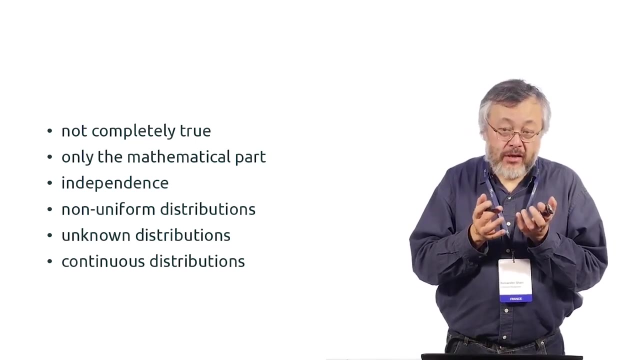 But what you do instead? you just look at the area of this thing And the empirical fact is that the fraction of cases when it goes inside the zone is proportional to the area of this zone. So it's kind of mathematicians say measure. 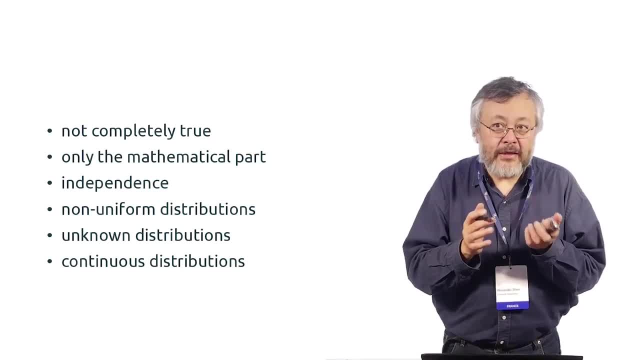 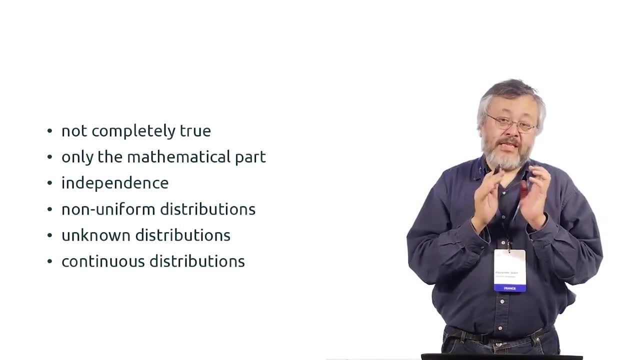 for areas and similar things. So the probability theory is a part of measure theory and a part which deals a lot with independence, But it's a complicated thing. You need to know how to the notion of integral, So we will not go into this. 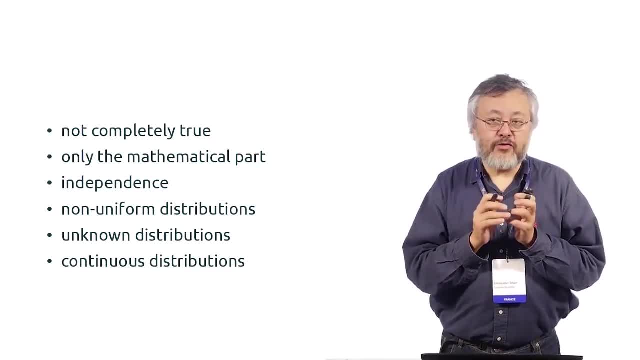 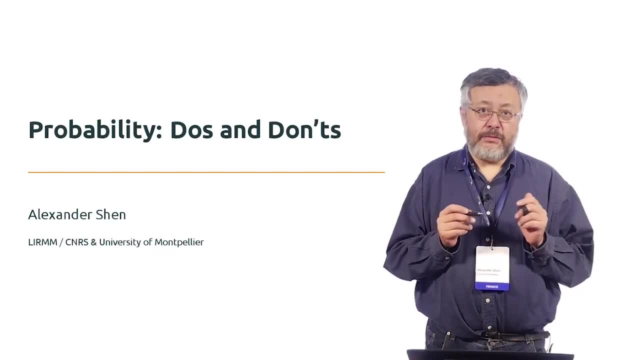 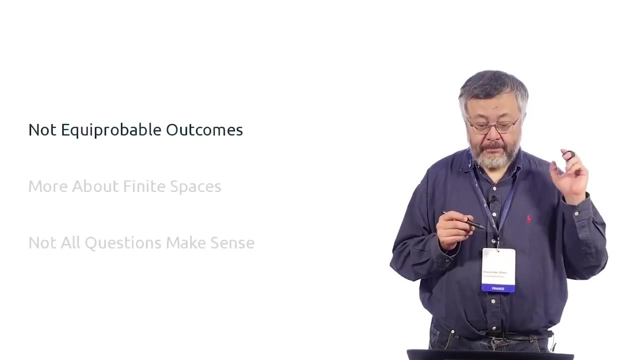 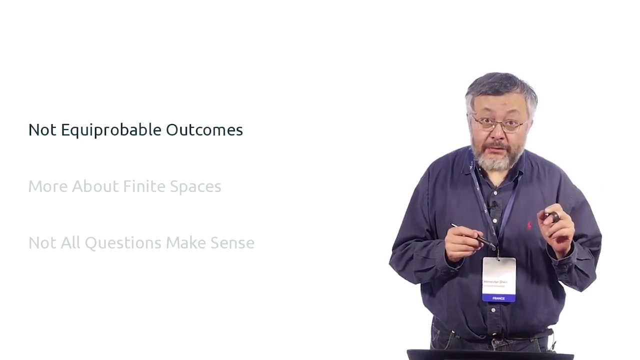 and consider only discrete distribution when the number of outcomes is finite. Now we start to discuss the limitations of probability theory, What is possible to do and what is not possible to do. So let's start. First thing is just the notion of finite probability space. 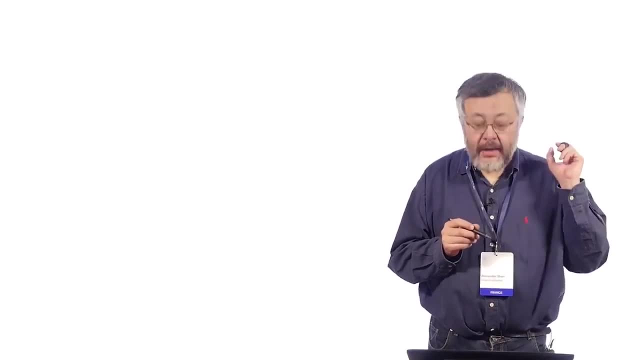 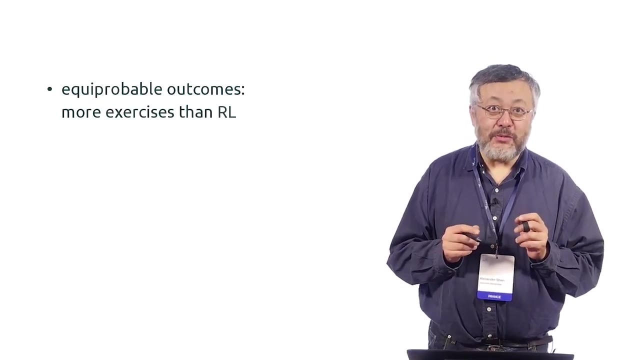 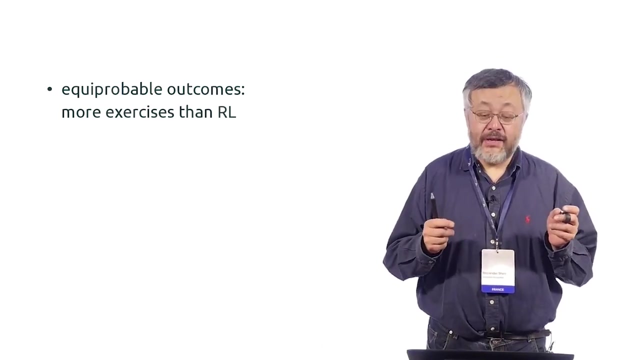 where not all outcomes are equiprobable. And you know, the equiprobable outcomes are more for exercises in textbook or probability theory than in real life. Most probability theory is not applied to dice or to coins, And even a real dice may be asymmetric. 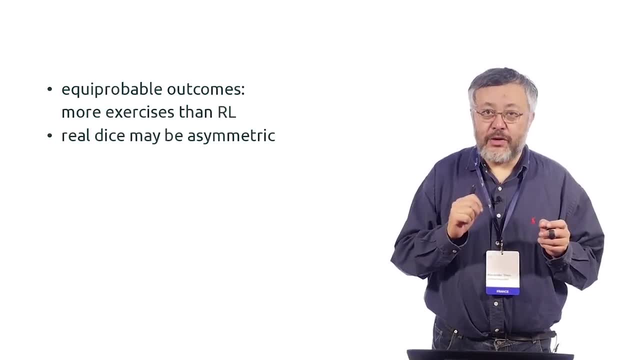 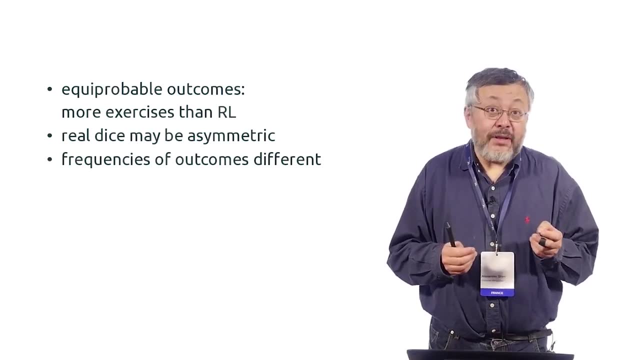 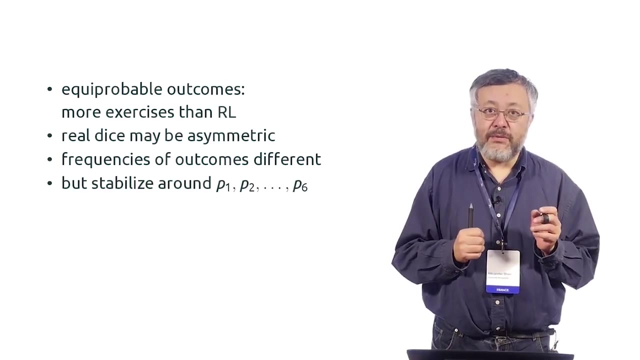 A coin can have one side that could be more heavy and fall more often, But this makes the frequencies of different outcomes different. But this is not a problem as soon as this frequency still stabilizes around some values. So if we have a long series of experiments, 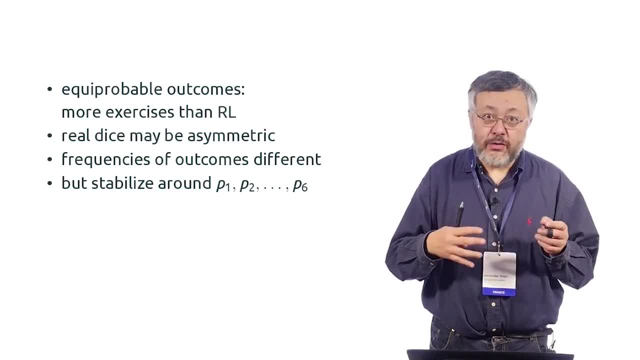 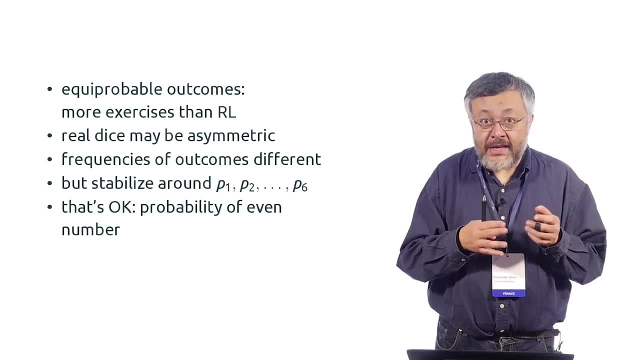 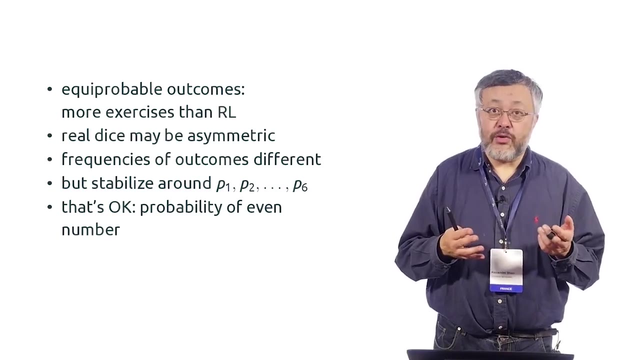 then we should have some limit values of frequencies, which could be called probabilities, And then, for example, if we know that for a dice there are some limit frequencies- p1,, p2,, p3 and so on- And we want to know how often the even number would appear, 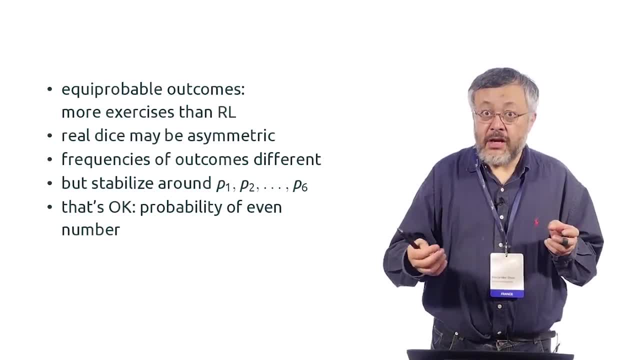 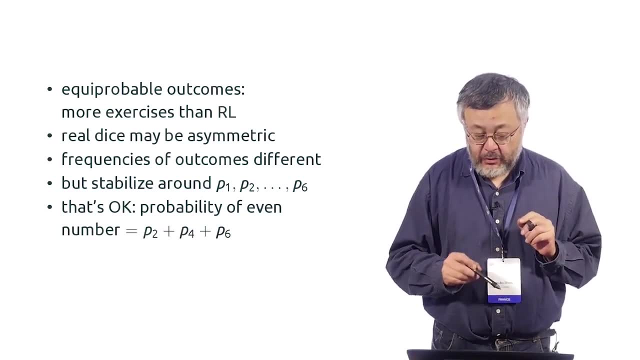 It's a combination of three cases of 2, of 4 and of 6.. So we should add these three numbers to get the probability of an even number. So here is the formula, And then you can be sure that in a long series, 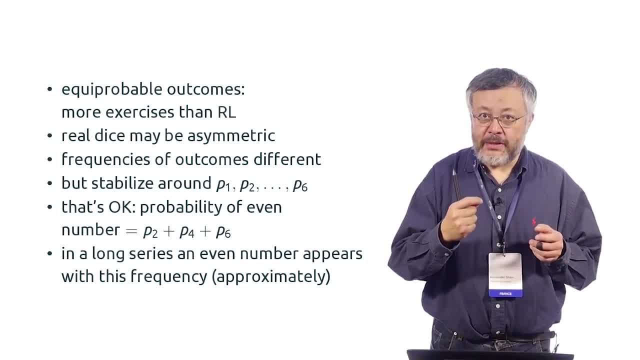 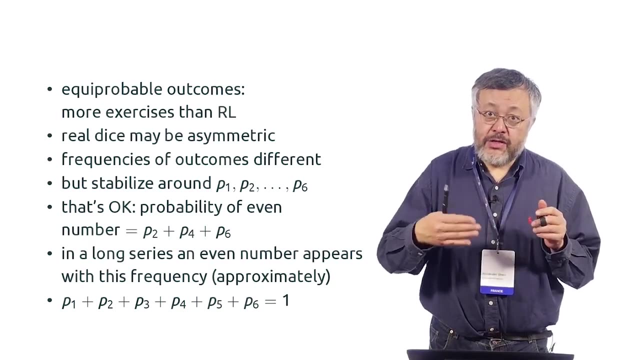 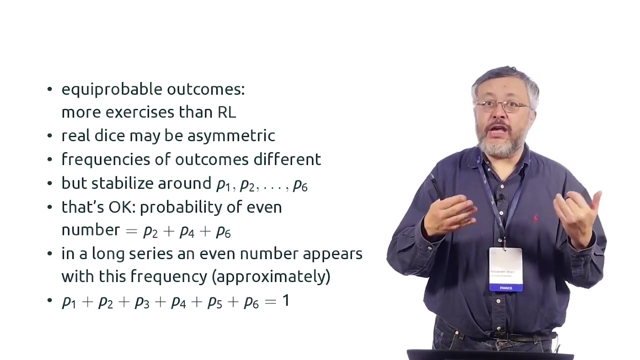 if the individual outcomes will have stable frequencies around the probabilities, then this combined event will also have the required stable frequency. And the last thing which you should know is that if the frequency of individual outcomes is a stable frequency, it should give some 1, because at each stage, 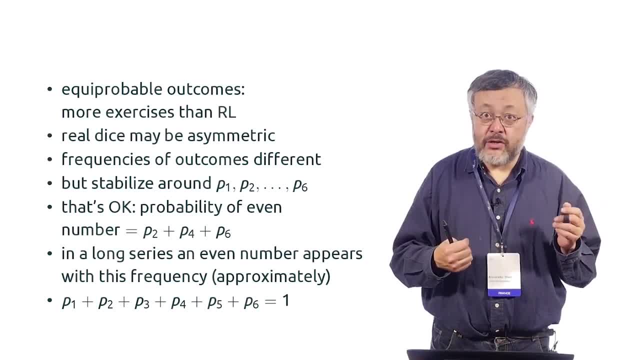 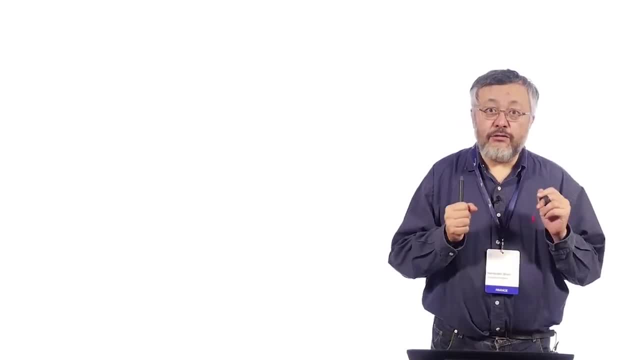 it is the case. So if things stabilize, it will also be the case after the stabilization. Okay, now we can give a special slide for a formal definition of finite probability space. So let's look at it. So we have a finite set of outcomes. 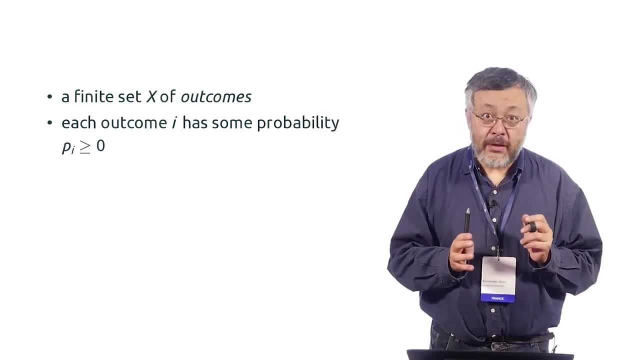 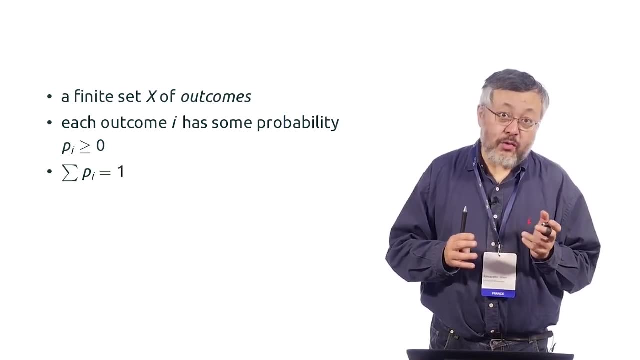 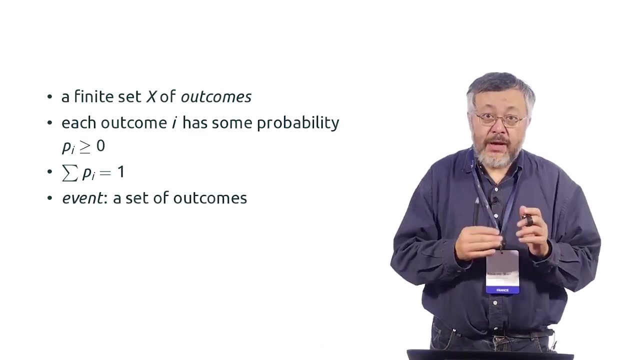 and each outcome has some probability. It's a number, a real number, which should be non-negative, and the sum should be 1.. So all the numbers should be between 0 and 1, therefore, And we know what is an outcome, and event is just a set of outcomes. 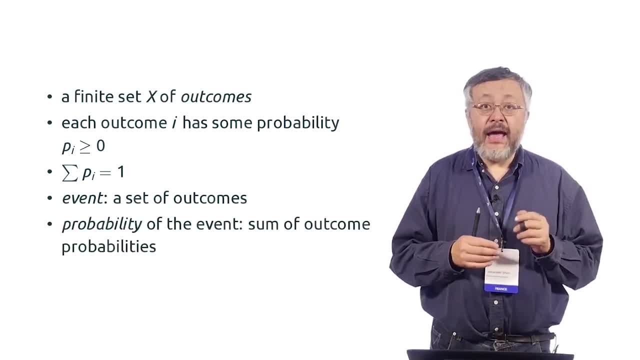 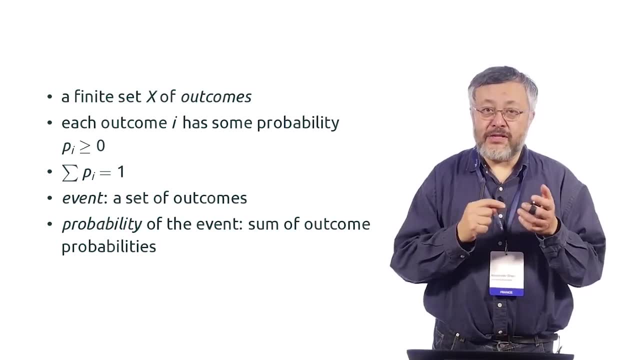 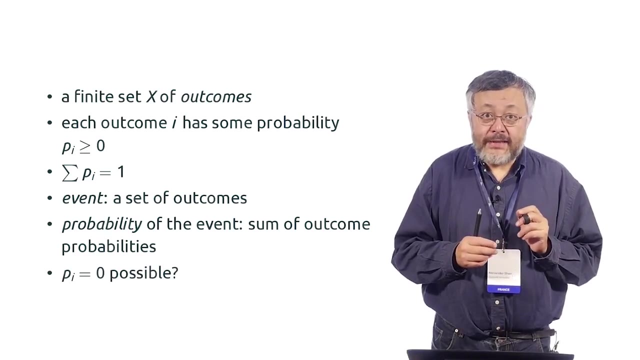 Any set of outcomes is considered as an event and the probability of this event is defined as the sum of probabilities of outcomes that form this event. Just what was in our example, but in a general setting. Last small technical details: whether some PI could be 0.. 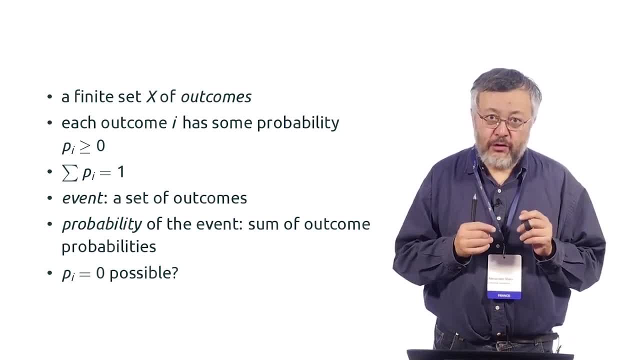 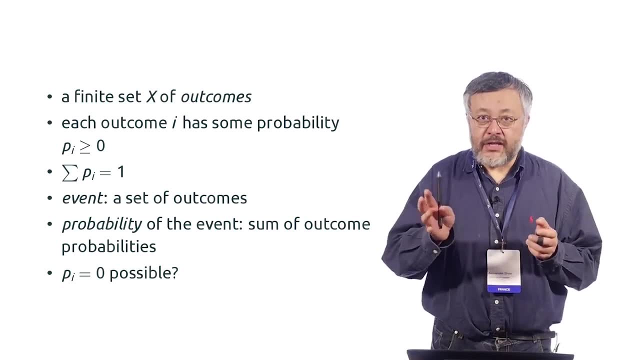 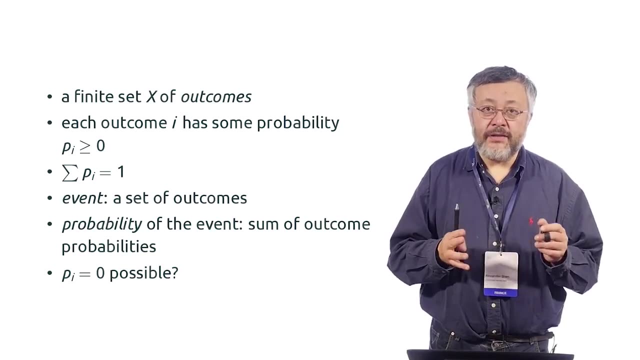 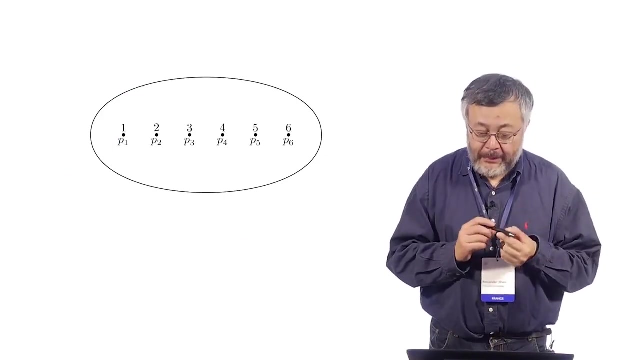 It's not that important. We allow this formally, but these outcomes actually, if they have 0 probability, they can be ignored and we can delete them from the probability space, probability space. So here is the formal definition and now we look at an example. I prepared an example. 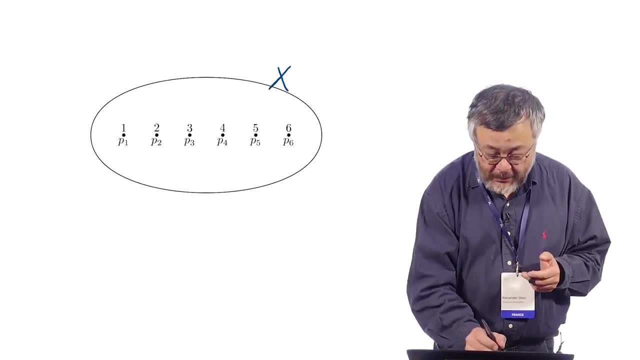 so here is the probability space x. it consists of 6 outcomes- 1,, 2,, 3, 4, 5, 6- and they have individual probability: p1, p2, p3, p4, p5, p6. 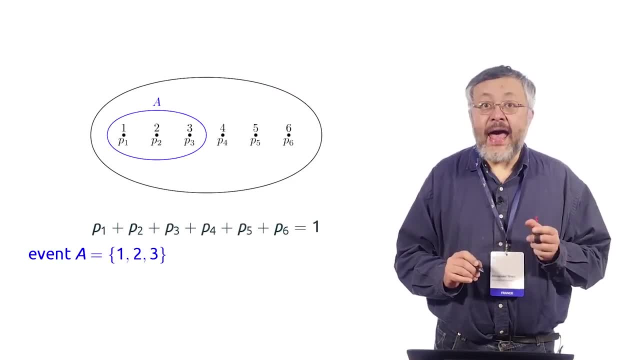 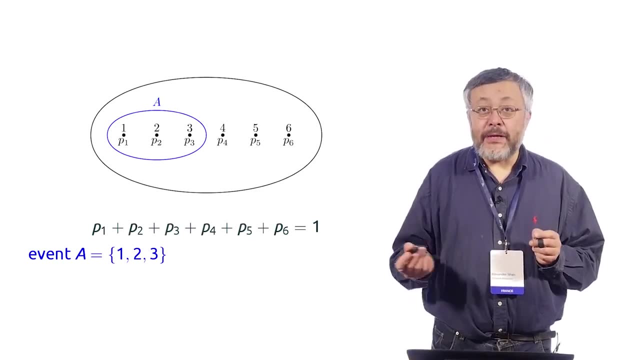 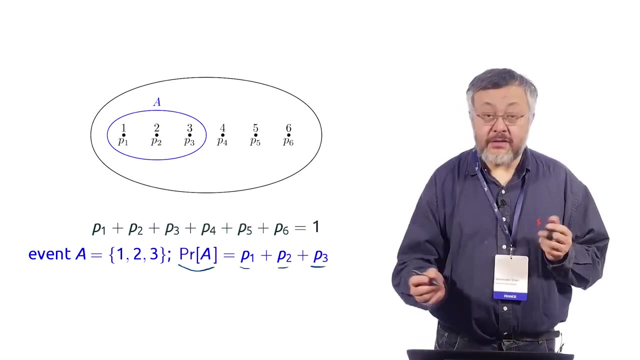 and if we have some, the sum should be 1. and if we have some event now, here is this event. a consist of 1,, 2, and 3, and its probability is the sum of probabilities of these events. probability of a is the sum of individual probabilities. 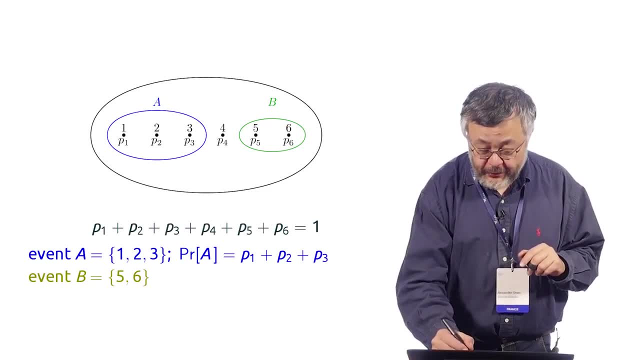 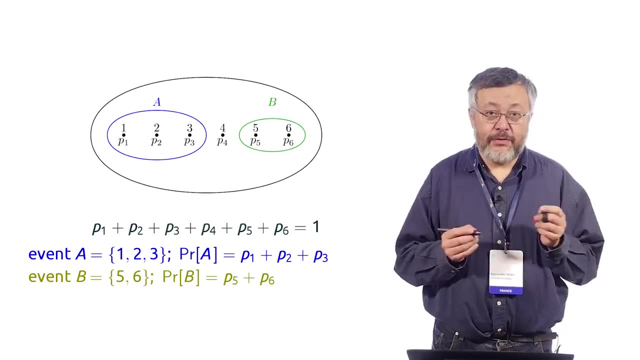 as we have said, and if we have another event b, then it's now made of 5 and 6 and the probability of p5 and p6, of course, the probability is the sum of p5 and p6 and now we can consider the combined event. 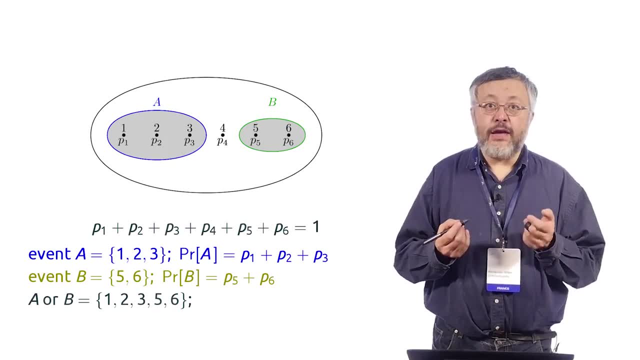 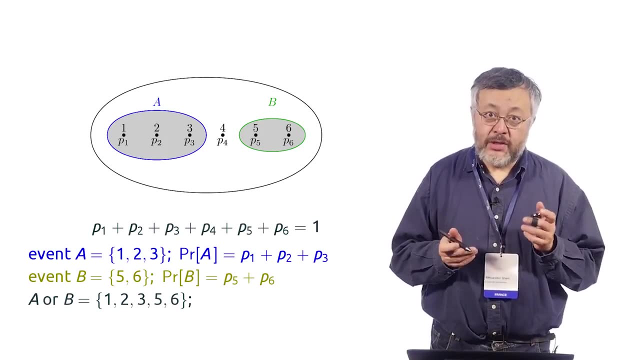 in set theory we say the union of the logical terms is the event a or b. so it happens when a happens or b happens. in our case it's not possible together, but just a or b is 1,, 2,, 3,, 5,, 6. 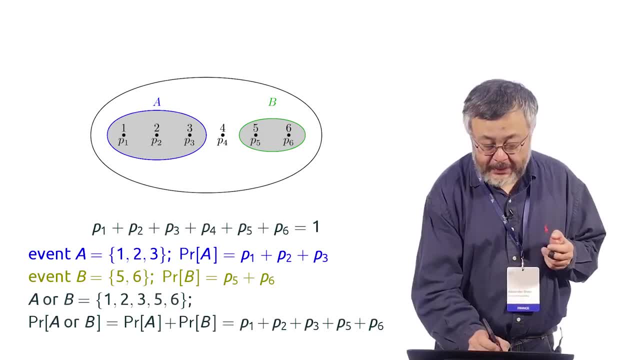 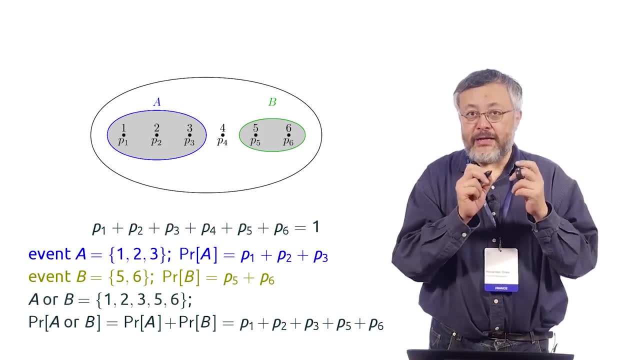 and, of course, the probability of this event is just the sum of these probabilities- 1,, 2,, 3,, 5, 6- and they can be split into two groups in probability of a is one group and probability of b is another group. 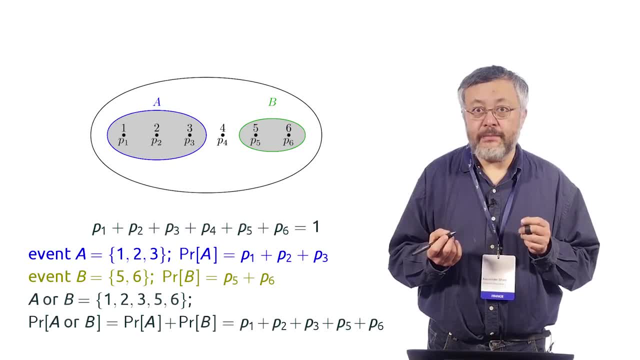 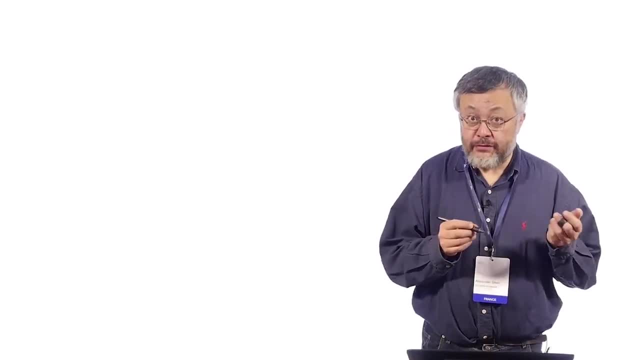 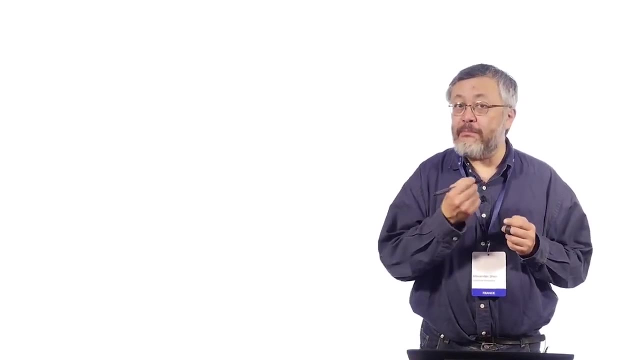 so we have this formula for the general case. a bit later now let's speak more about finite spaces and let's start with. what we finished with is what is called the mutual exclusive event and the formula for the probability of sum probabilities. so the event is a set of outcomes. 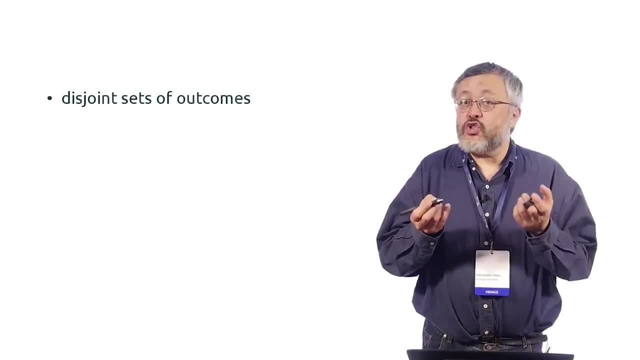 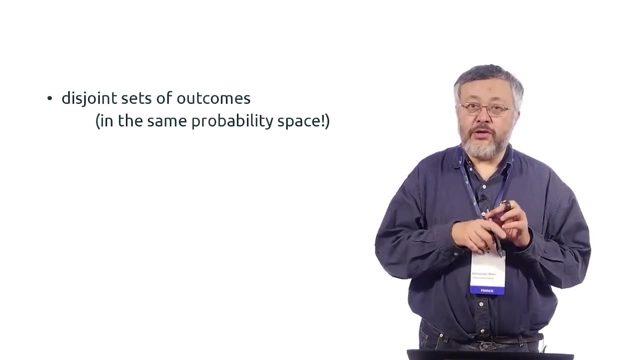 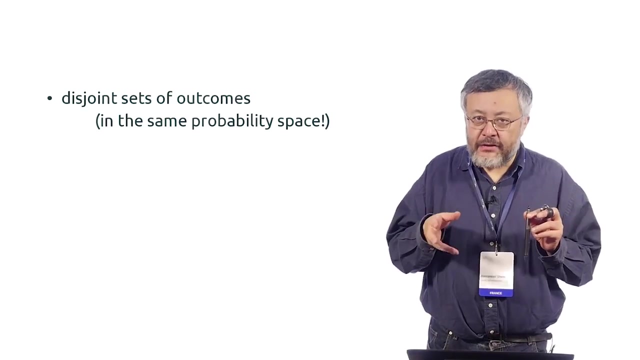 and the mutual exclusive event are just this joint set of outcomes. but there is an important thing. so imagine somebody asks you: I toss a coin and get I don't know head, and another time I roll a dice and get 3. so are these outcome events? 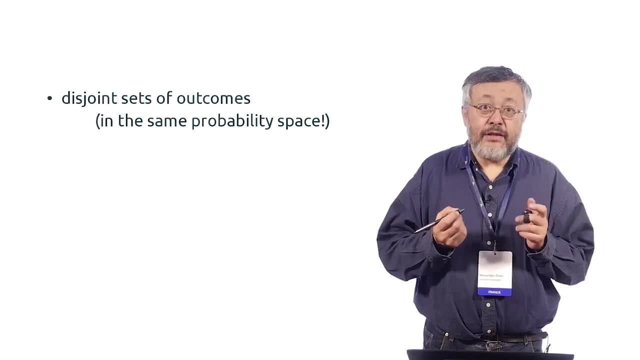 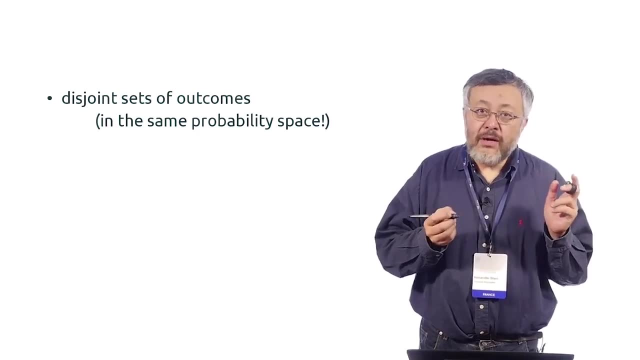 are they mutually exclusive? and the correct answer is not yes or no. the correct answer is that they are not defined on the same probability space. so there is no, the question has no meaning. it's often the case in probability theory: when the question has no meaning, 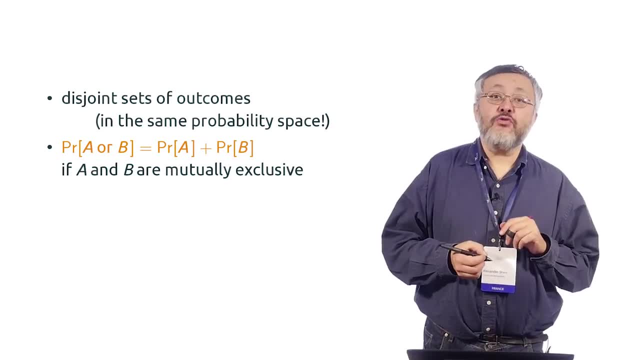 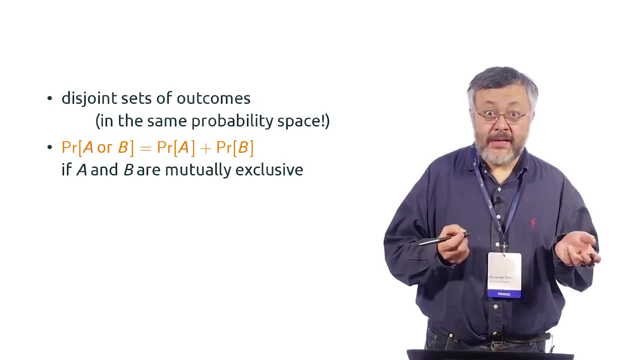 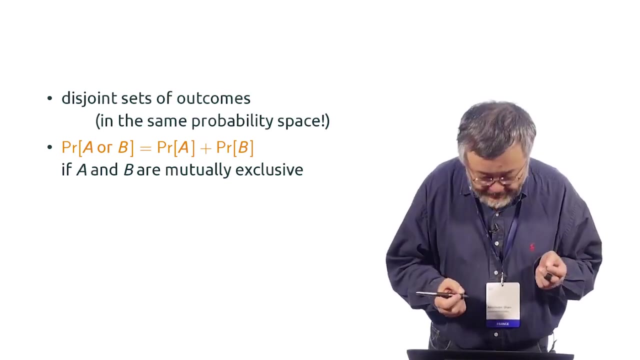 anyway, if there are two mutually exclusive events, then the probability of their union, a or b, is the sum of probabilities. that's what we have seen. we have seen for a specific example, and this will happen in the general case as well. a special case of this rule is: 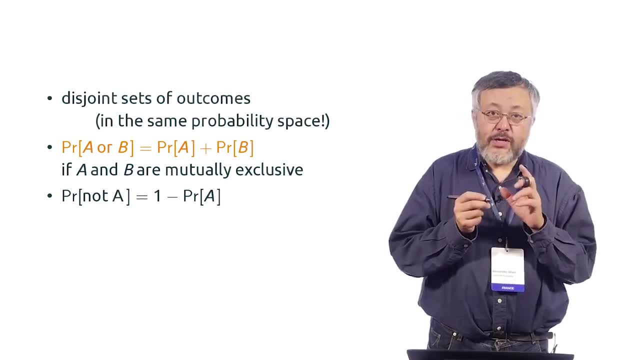 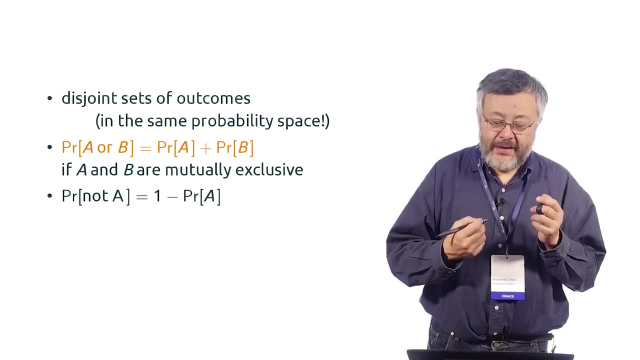 with this mutual exclusive event are complementary. so imagine we have some event, a, then it defines another event called not a. this event happens when a doesn't happen. in terms of set theory, it's the complement of the set which form the event and a and not a. 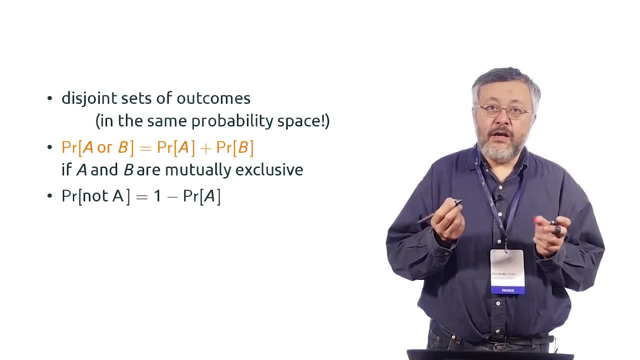 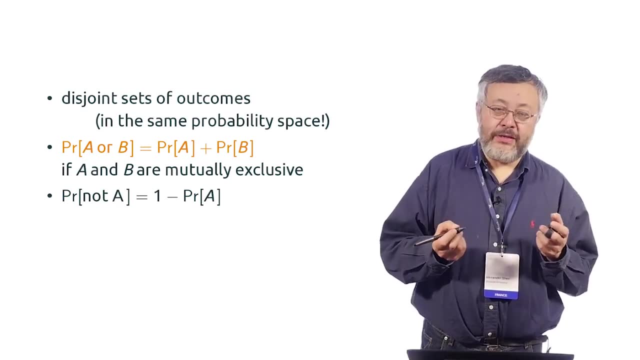 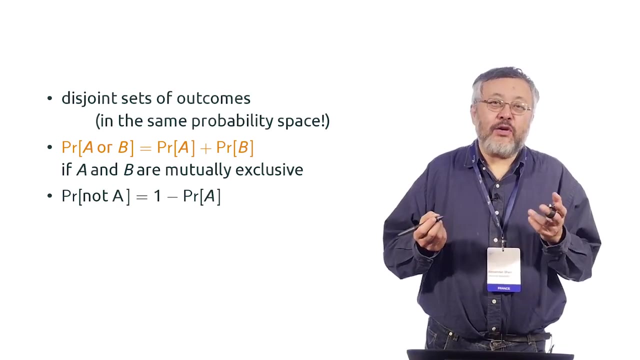 are mutually exclusive events and together they can cover the entire space. so the sum of probabilities should be one. so the probability of not a is one minus probability of a. so if you believe that probability- I don't know to see a crocodile- is one third, for whatever reason. 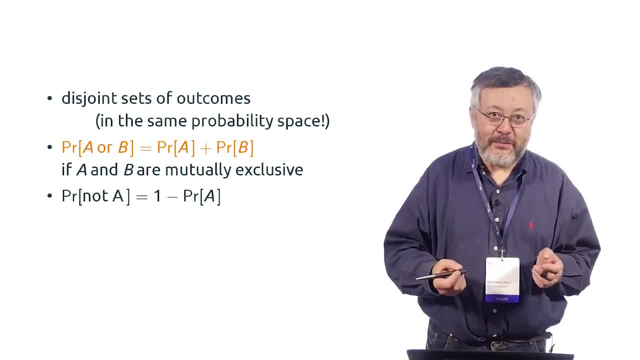 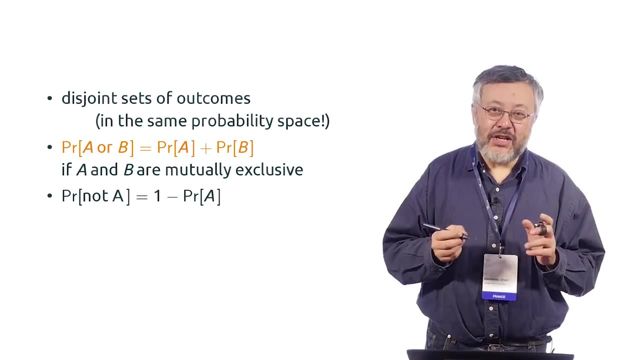 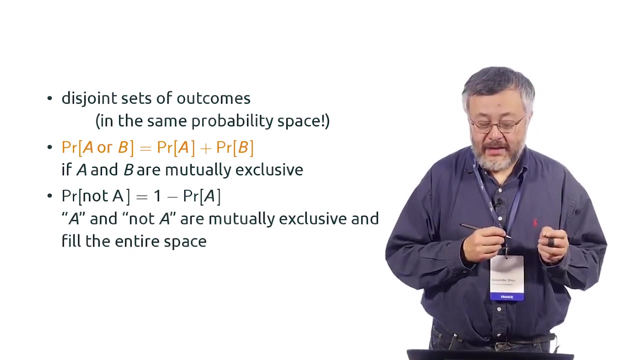 then you should agree that probability not to see it is two third at the same experiment. okay, there is no reason or probability space here, but okay, just it's a simple rule. this is the explanation why it happens, because they are mutually exclusive, so we can apply the sum rule. 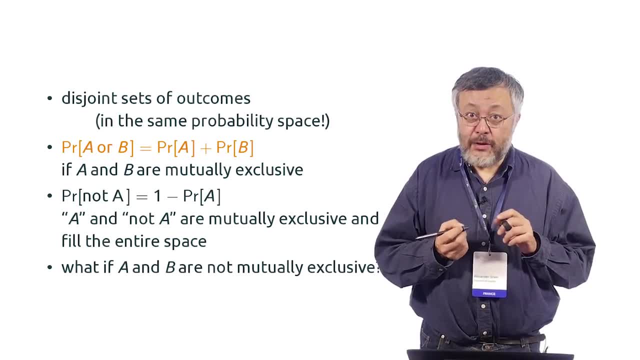 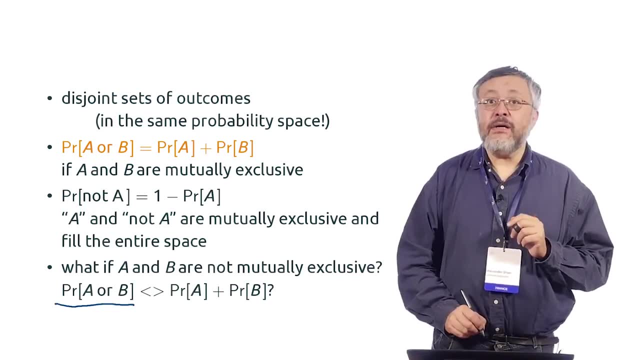 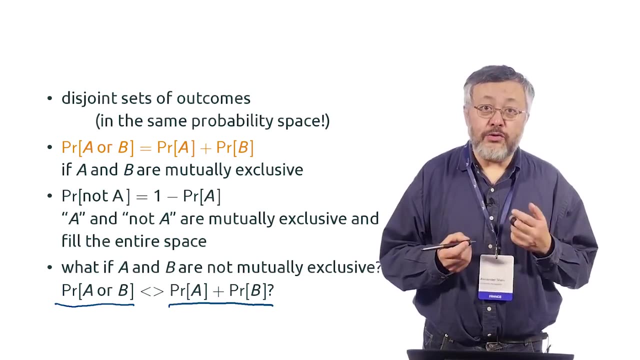 and the last thing we want to discuss is the probability of two events. what if they are not mutually exclusive? so then, this probability of a or b is not, maybe not equal to sum of probabilities. but now the question is, is it bigger or smaller? what do you think? 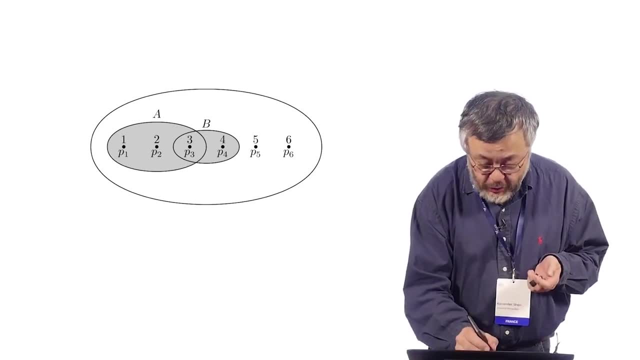 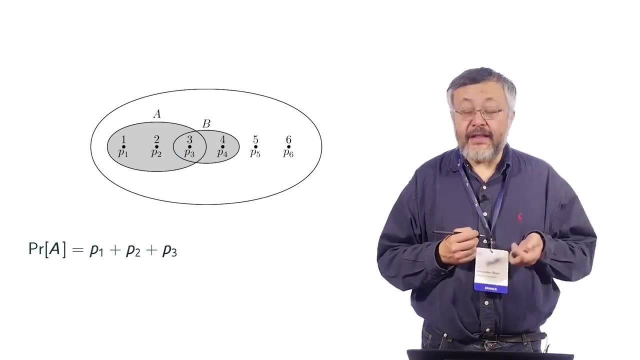 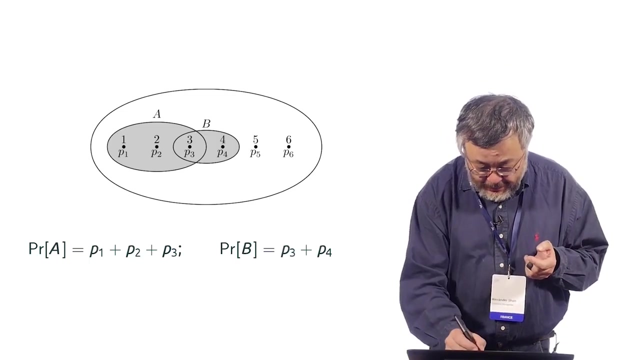 and let's see an example and we will see the answer immediately. so imagine we have two events, a and b, and they are not mutually exclusive, and then probability of a is p1 plus p2 plus p3 and the probability of b is p3 plus p4. 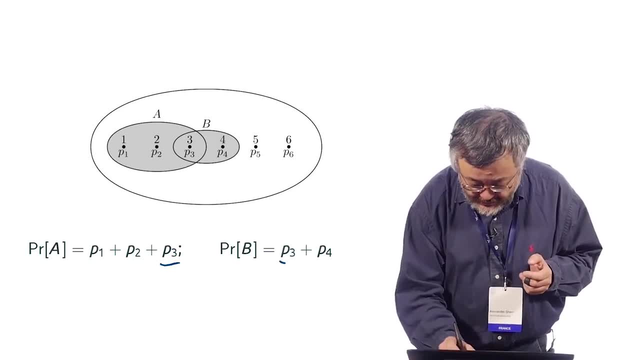 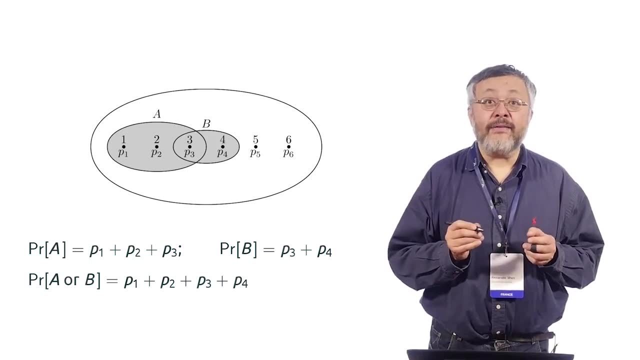 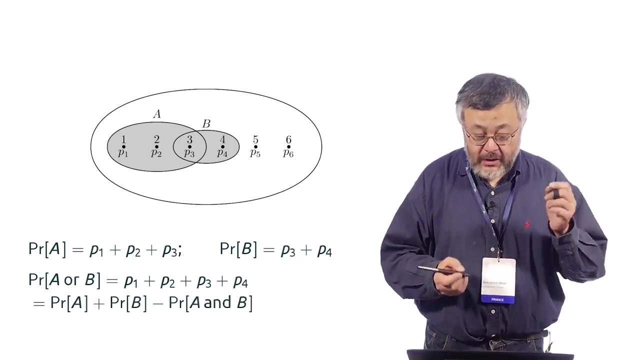 now there is common p3 here. so if we look at the union, a or b, it's just p1, p2, p3 and p4, and if we add these two probabilities, look, we will count p3 twice. so to get the correct answer we should compensate. 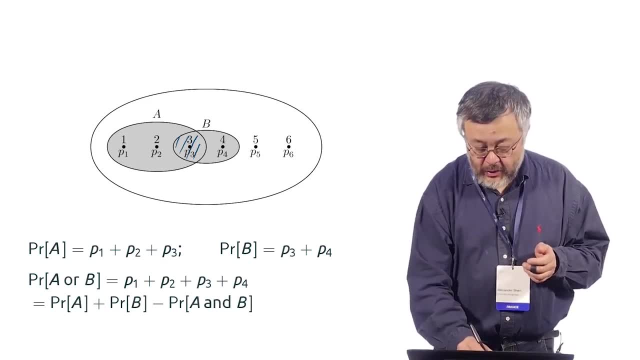 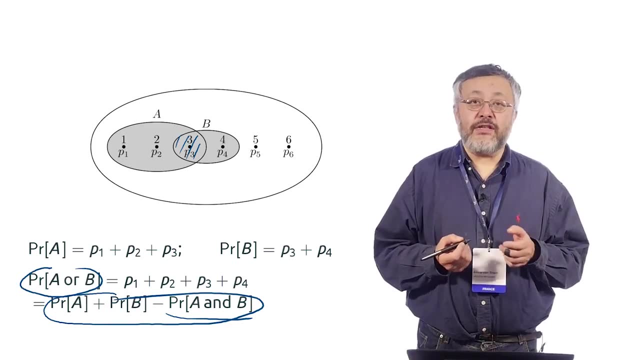 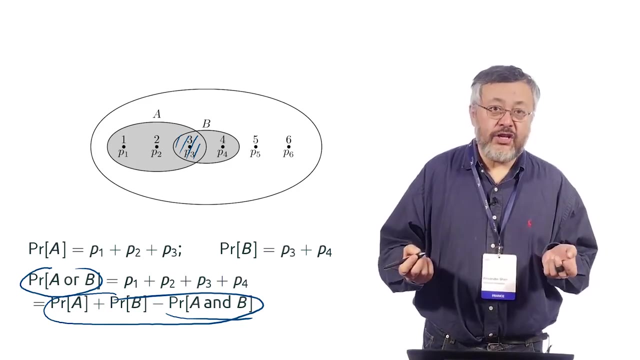 and subtract this intersection of these events, which is now only one: p3, and this rule, this rule- probably you see this, you have seen this in combinatorics, it's inclusion and exclusion formula and it's true for general probability spaces, not only for the equiprobable outcomes. 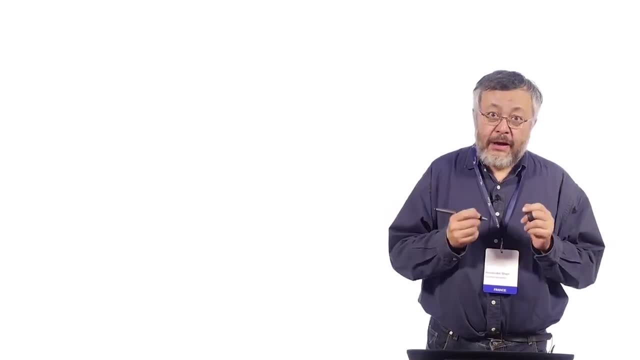 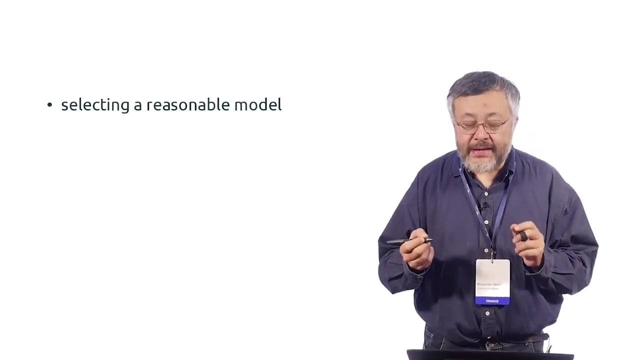 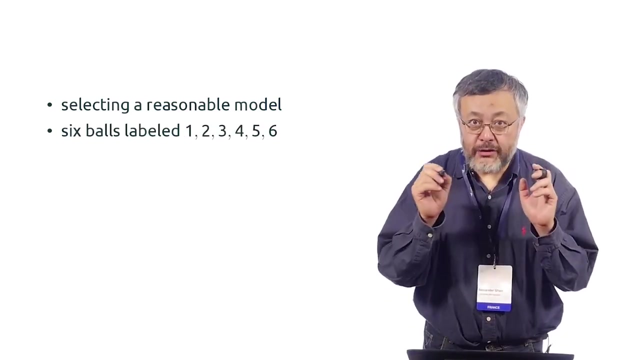 another story when a general probability space with non-equal probability of outcomes appears. it's what is called sequential choice. let me explain. so there is some prepared example. the question is how to select a reasonable probability model for some experiment, and the experiment is like this: we have six balls: 1, 2, 3, 4, 5, 6. 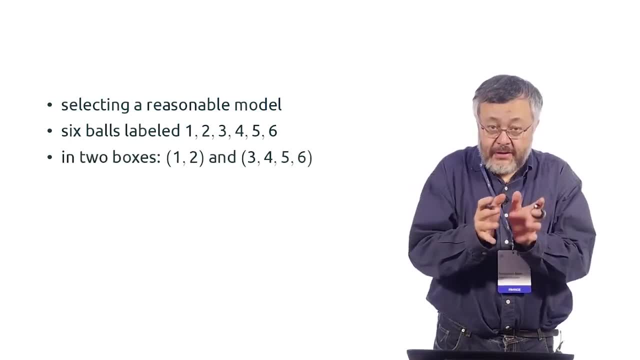 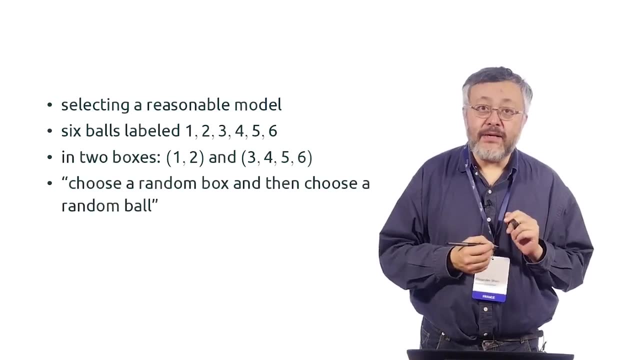 and we have two boxes and the balls 1 and 2 are in one box and 3, 4, 5, 6 is in another box. and then the probability experiment is described as we choose a random box and then choose a random ball in the box. 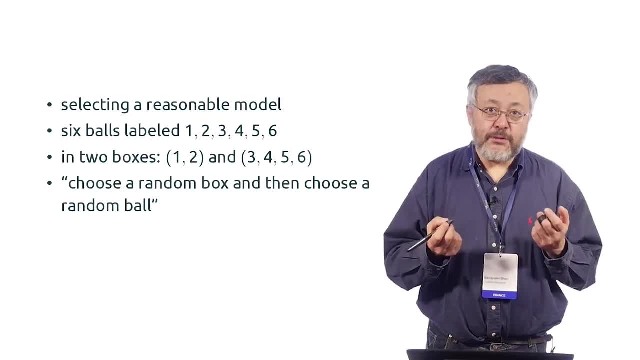 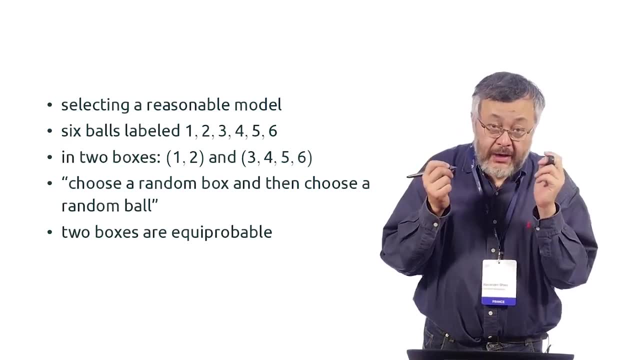 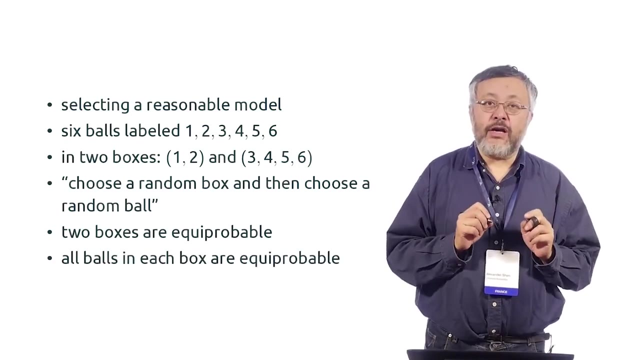 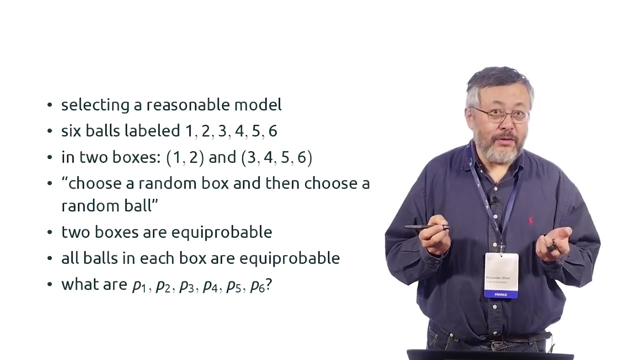 so the question is what probability space reasonably corresponds to this process and what. we assume that the boxes have equal chances to be selected and in each box all the balls have equal chances to be selected and we want to decide the probabilities of all six outcomes. probably you can say the answer immediately. 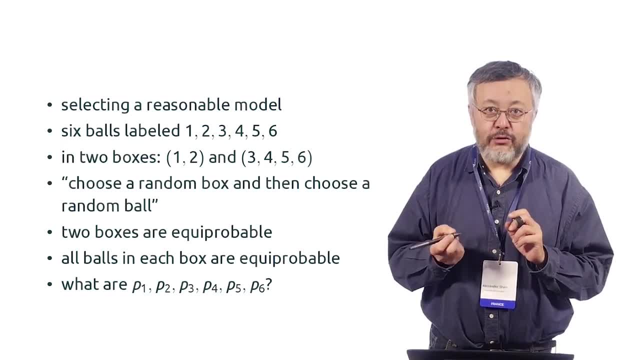 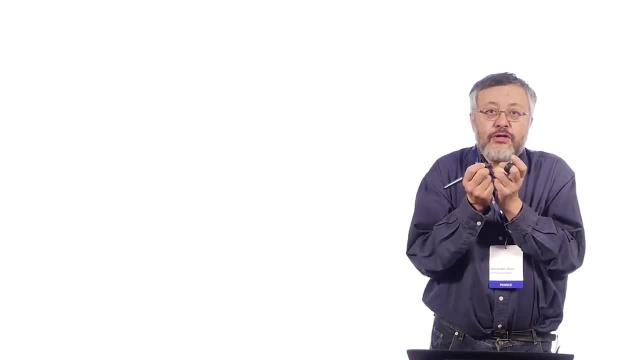 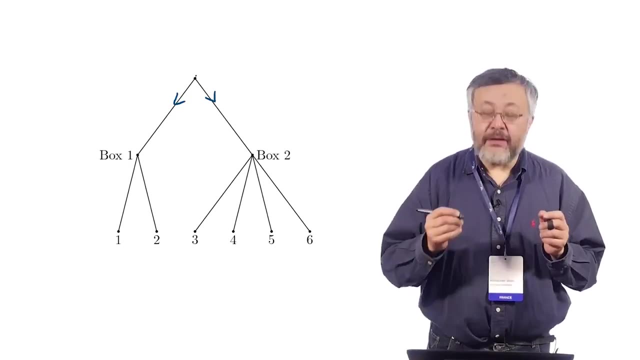 but still, I prepared some slides to explain this, so just keep it if it's obvious. but it's useful to represent what is happening in a kind of a tree. so we have a tree and this is the first choice, whether we take box 1 or box 2. 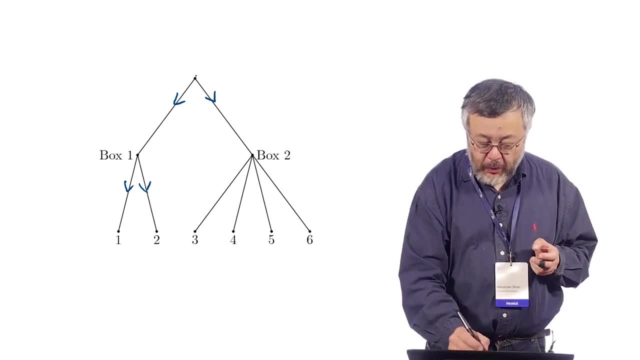 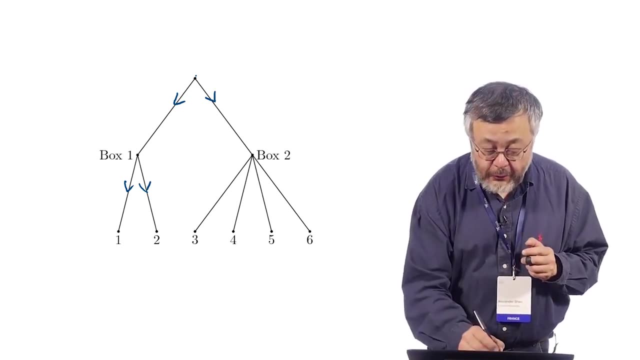 and here we made the second choice: when we take one ball, either 1 or 2 if it's box 1, or 3, 4, 5, 6 if it's box 2. so in half of the cases we will go left, in half of the cases. 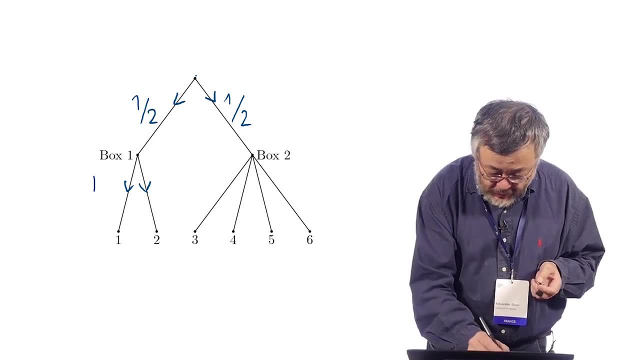 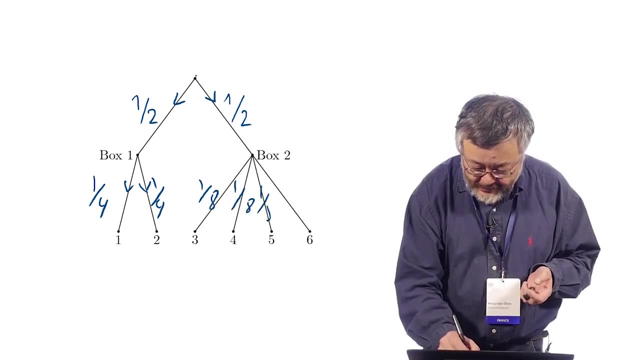 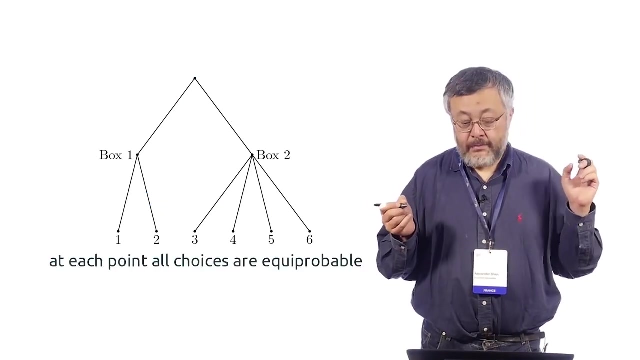 we will go right, because the boxes are equi-probable, and here then we can go in: half of this, half we go here, and half of this, half we go here, and here we have one of the eight. so this is how we get the probabilities for six outcomes. 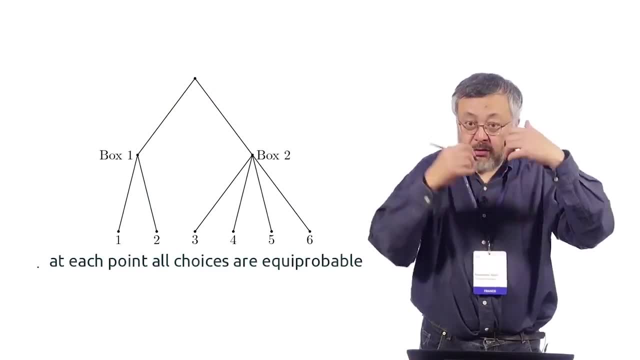 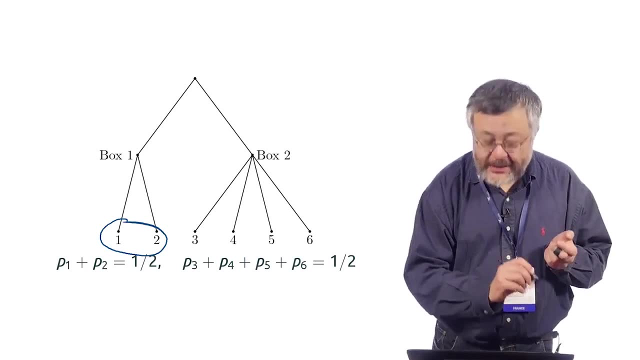 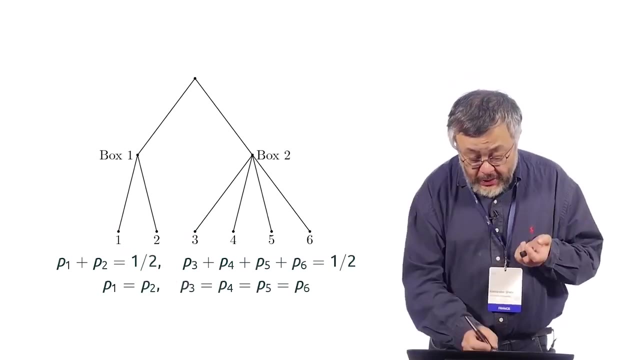 and using the fact that at this point all choices, all father choices, are equi-probable. and then is another explanation. so here is just the event we select box 1 and here is the event we select box 2, and they should have probability 1 half. 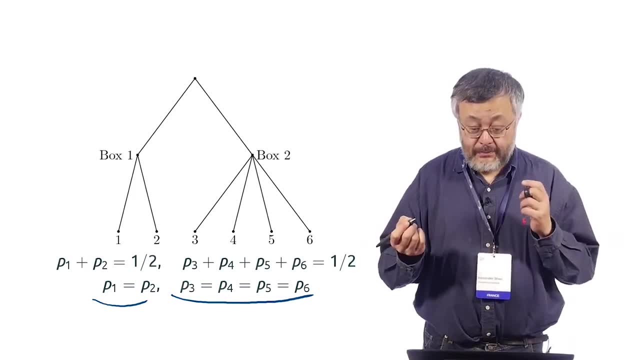 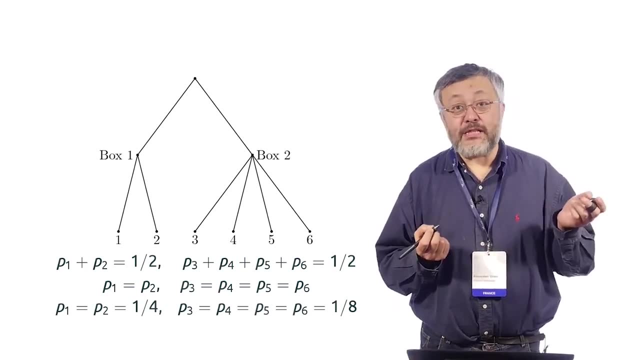 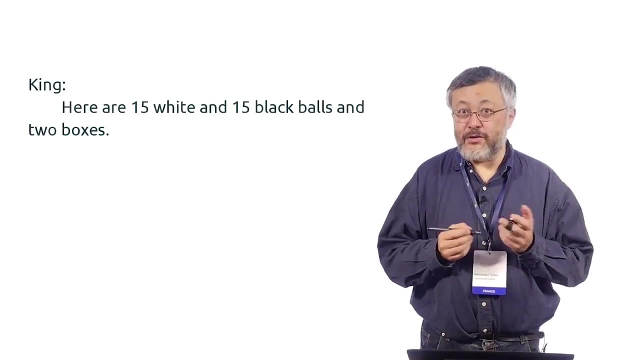 and also this individual probability inside the boxes should be also equal. so there is only one possibility for that and it's written here: it's exactly the same numbers. in this part we have some puzzle or some tale, and the tale is about a prisoner and a king. 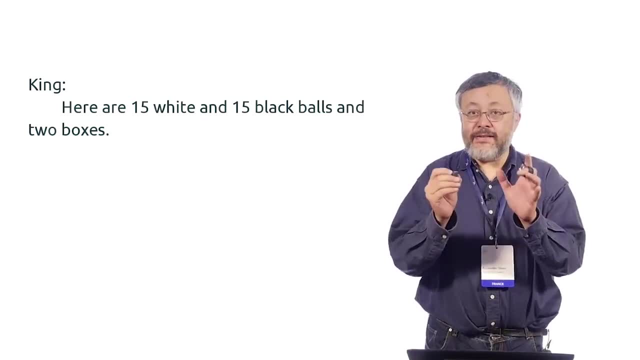 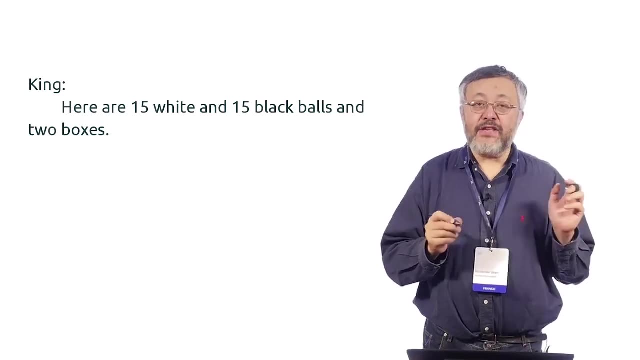 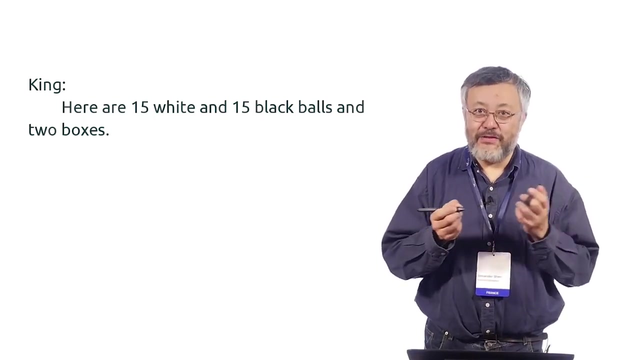 so the king calls the prisoner and tells that, look here we have 15 white balls and 15 black balls and these balls will be used to determine your fate. you know, the king can determine the fate of everybody and what the prisoner can do. the prisoner is allowed. 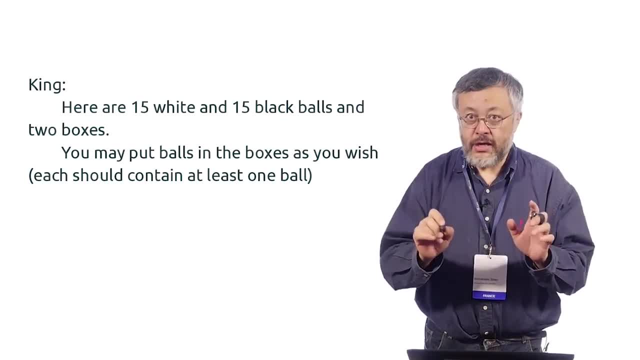 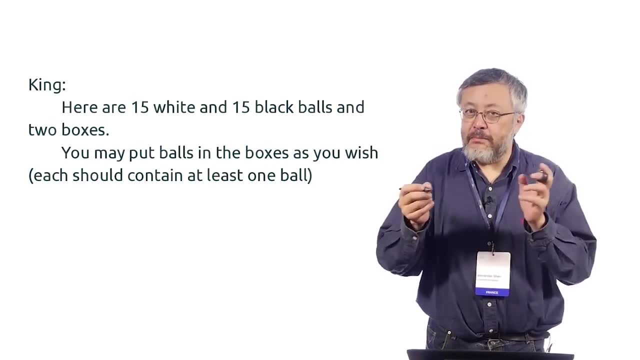 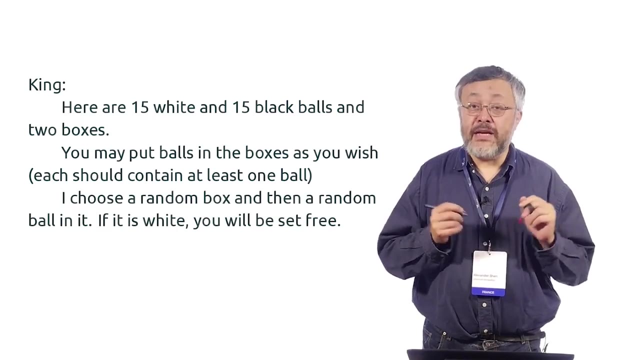 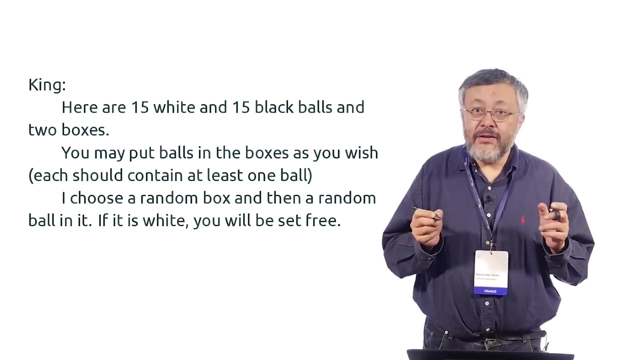 to put the balls in the boxes in any proportion. so each box should be non-empty, but he is not. he is able to put black and white balls as he wishes, and then king promised that he will choose one of the boxes randomly and then he will take a random ball. 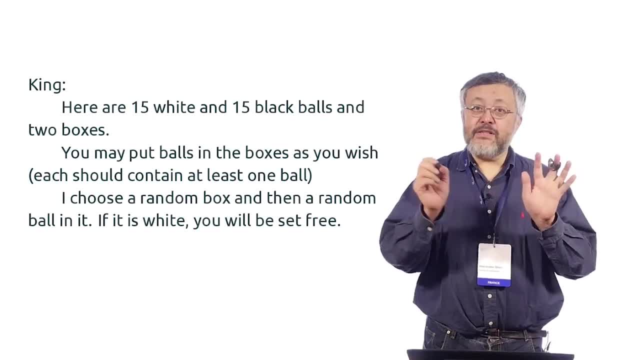 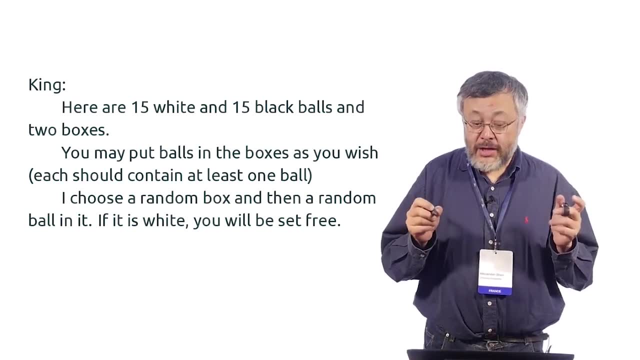 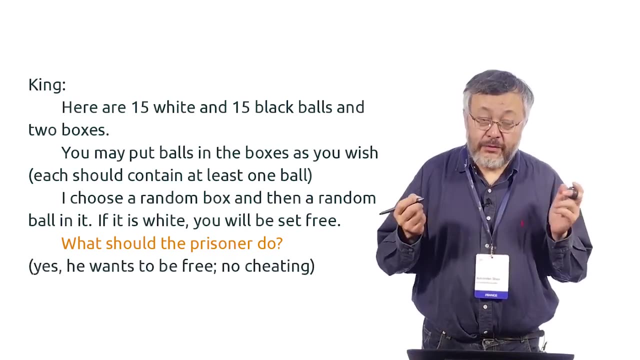 from this box and if this ball is white, then the prisoner is set free, and if it's black, something bad happens. so imagine that prisoner wants to increase his chances to be set free. he wants to be free and there is no cheating. the prisoner cannot just throw away. 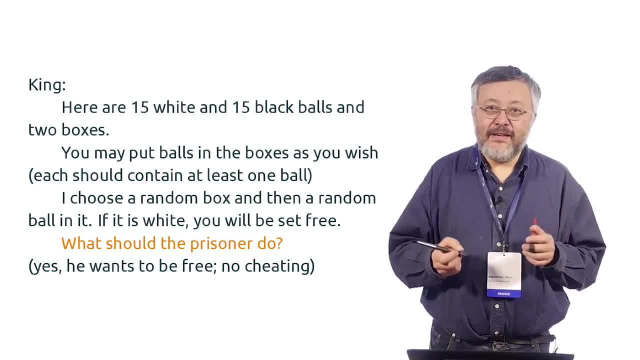 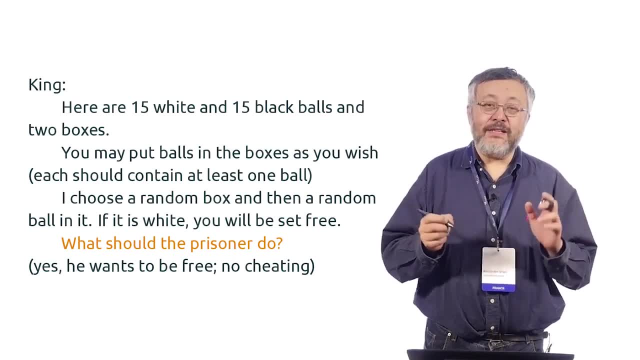 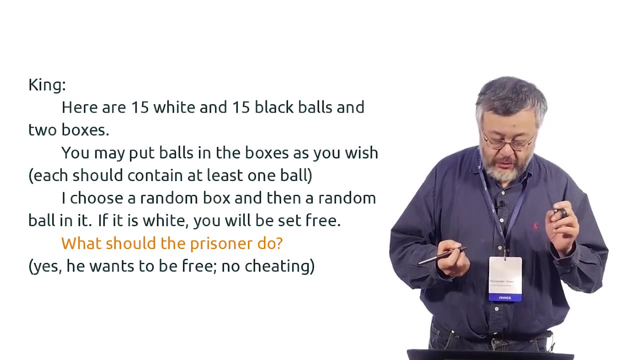 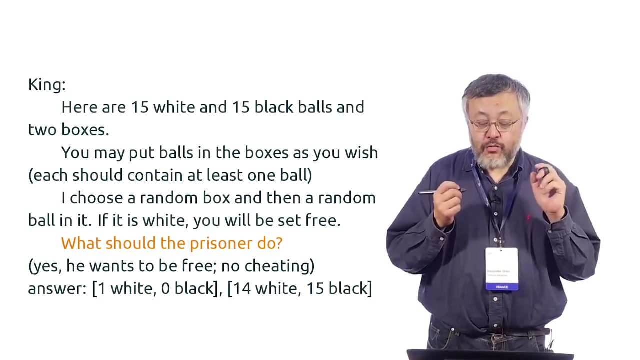 all the black balls, or the king cannot kill them. the ball is white, so everybody follows the protocol, but still the prisoner should maximize the probability of being set free. what should the prisoner do? and here is the answer. the answer is that you should have one white in one box. 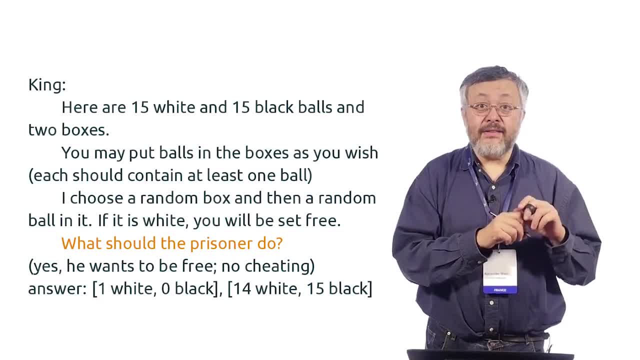 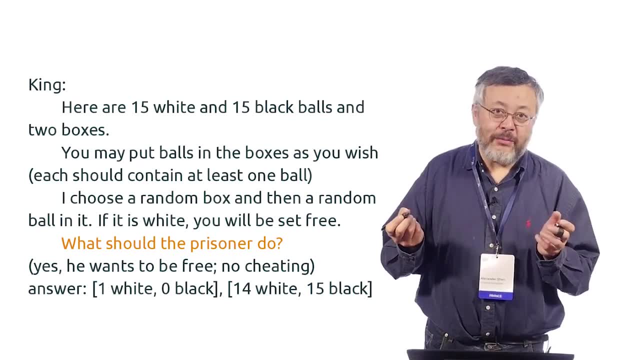 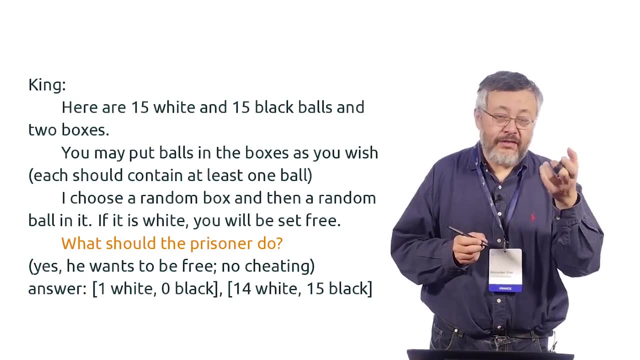 the prisoner should put just one white ball, and in the other box he should put the rest of white balls, 14 white balls and all the black balls. so what does it give if the king took the box with only one white ball? then the prisoner is guaranteed to be free. 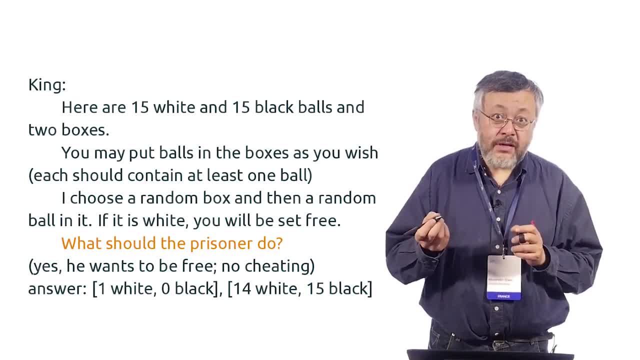 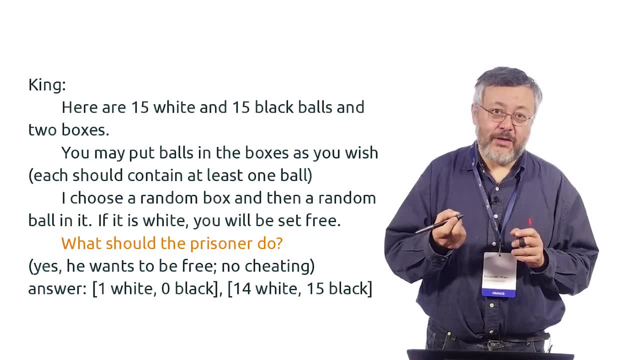 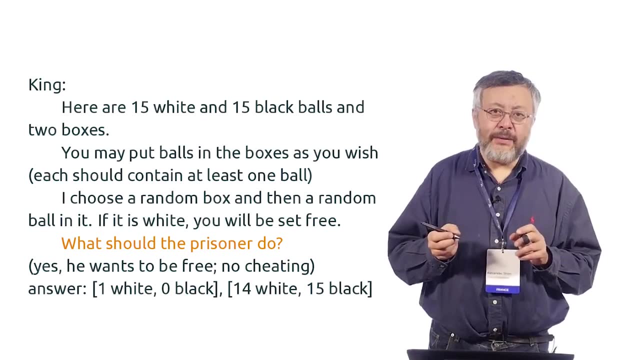 but if the king selects another box, then still the prisoner has some reasonable chances. it's just a bit smaller than 1 to 1, 14 to 15, because there are only 14 white and 15 black, so it's a bit less in total. 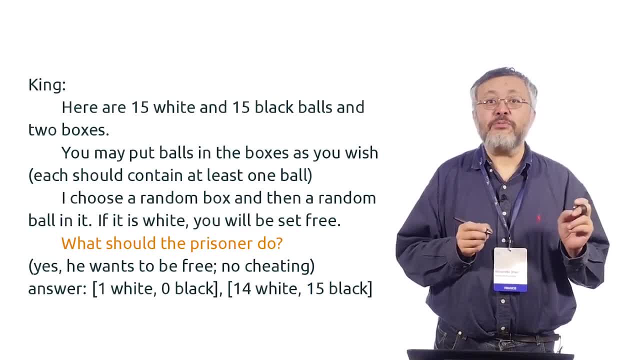 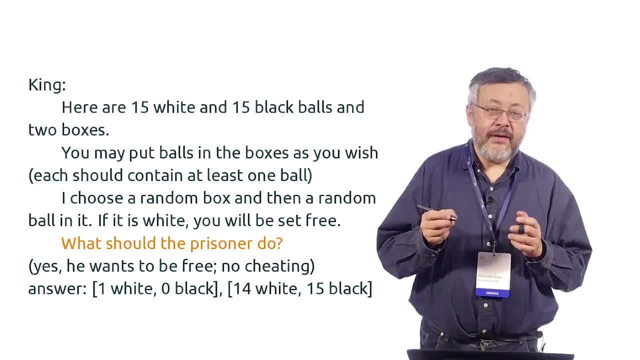 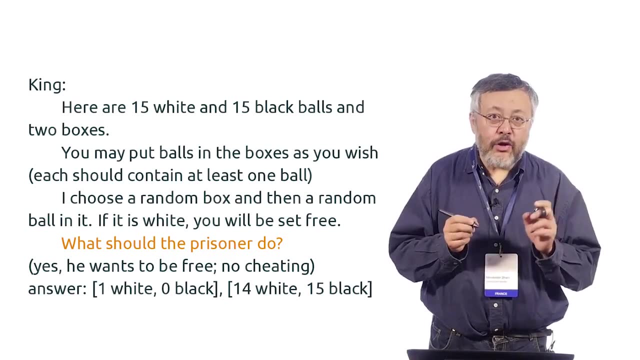 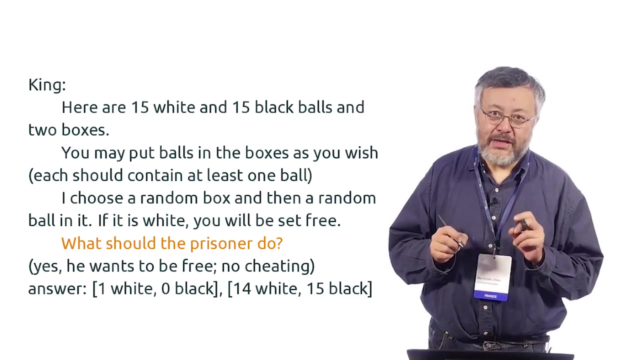 but I claim that this is optimal and it's not very easy. it's somehow obvious if you think, intuitively obvious. but mathematical proof is not so trivial and I will not explain it completely formally with all the formulas, but it's a really valid mathematical proof, just explained in an informal way. 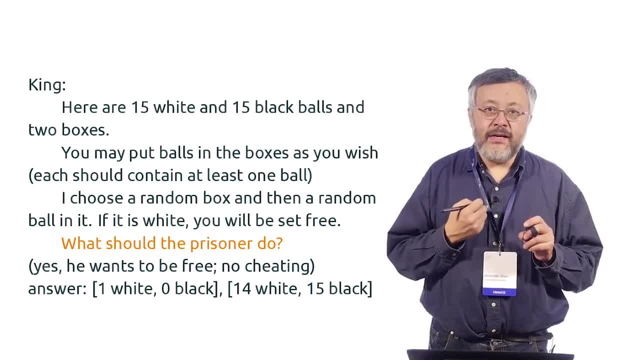 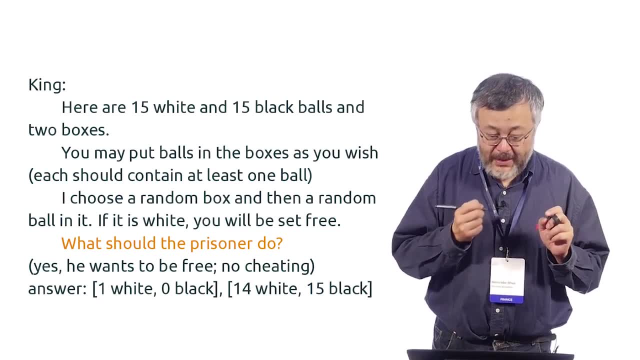 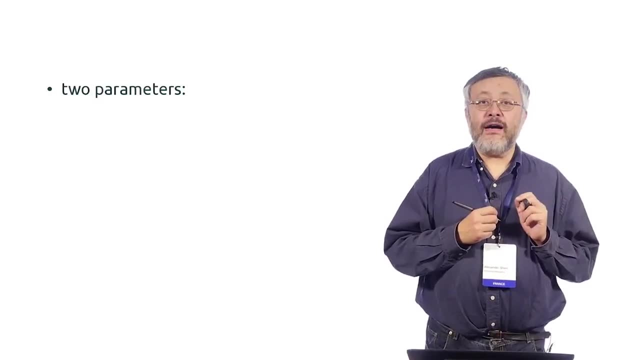 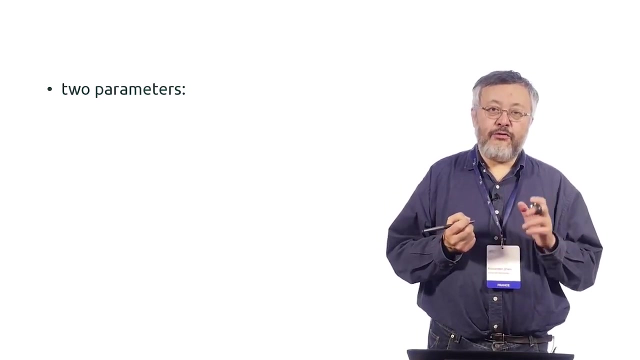 so you can think about it. if you retell it in a more formal way if you feel it's necessary, ok, so now the proof it should be prepared. yeah, so actually the prisoner has somehow two-dimensional space of choices, so first he should decide, it's not. 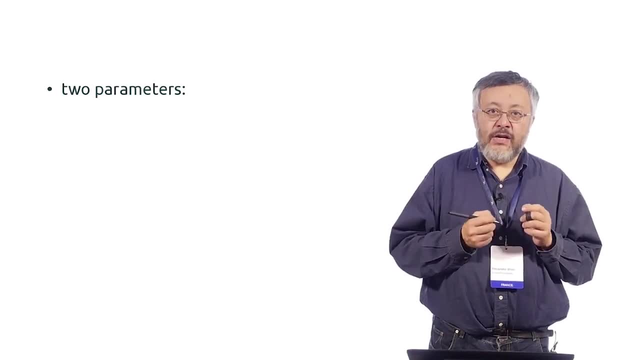 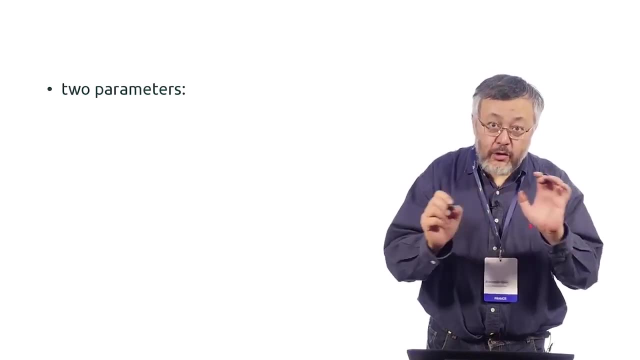 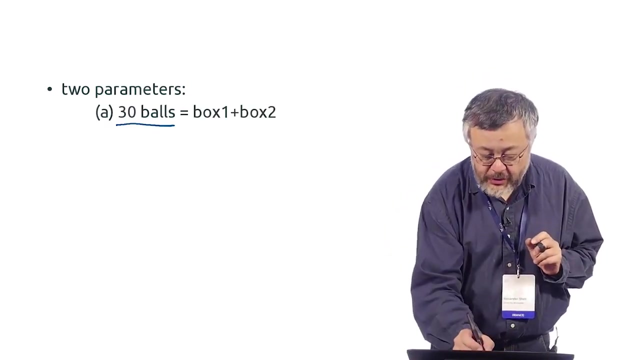 just, we describe this choice this way: first he decides how many balls will be in the one box and how many balls will be in the other box, ignoring the colors. so first he decides just the numbers and then. so this is the splitting of 30 balls into two boxes. 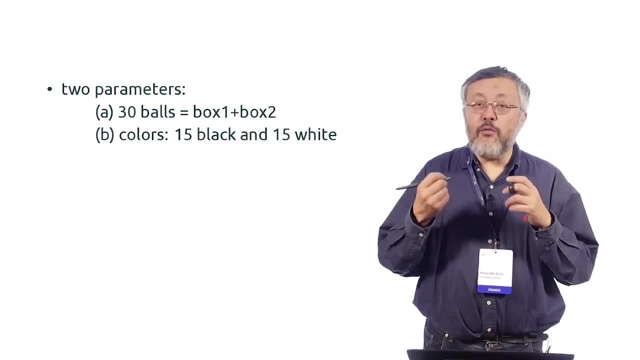 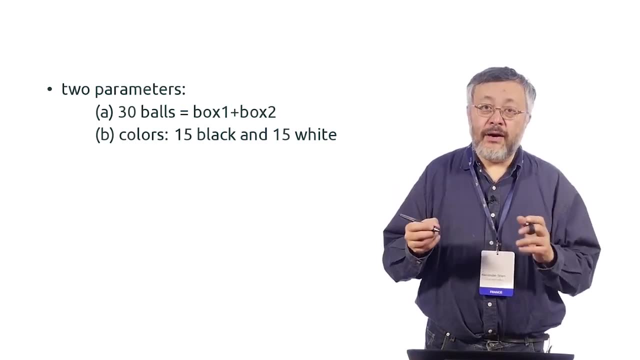 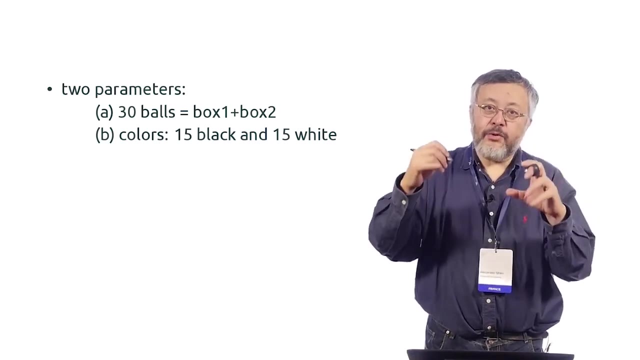 and second, he decided how the colors are distributed, so how many black balls we have in the first box and in the second box. so this is the second decision. the total number is fixed. the prisoner can modify the numbers, but he should balance things, so the total number should be. 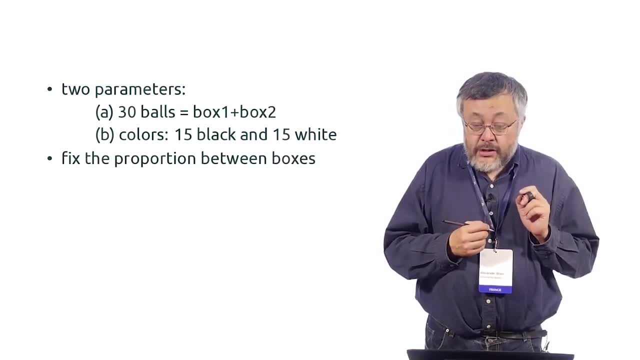 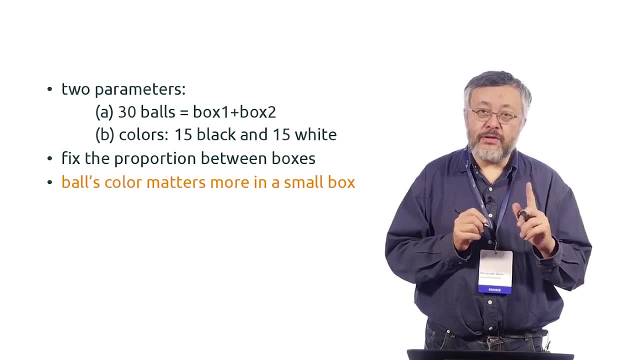 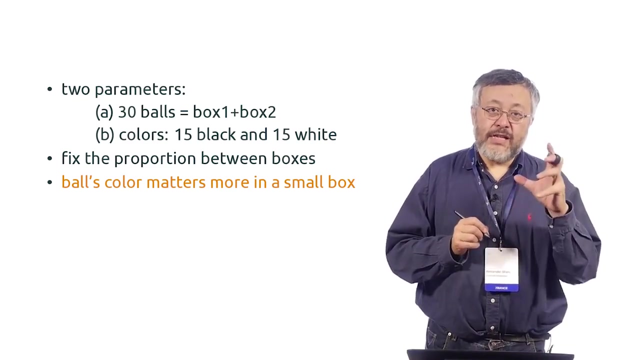 as prescribed. so let's look at the second stage, when the proportion between boxes is fixed, and this is the most important informal which can be made formal, informal remark that the color of the ball in the box when there are fewer balls. so if a small ball, look, imagine you have a small. 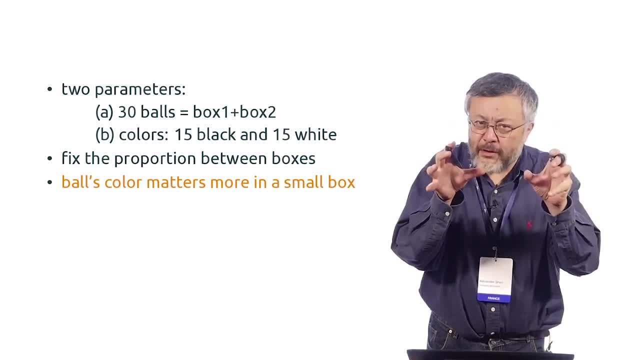 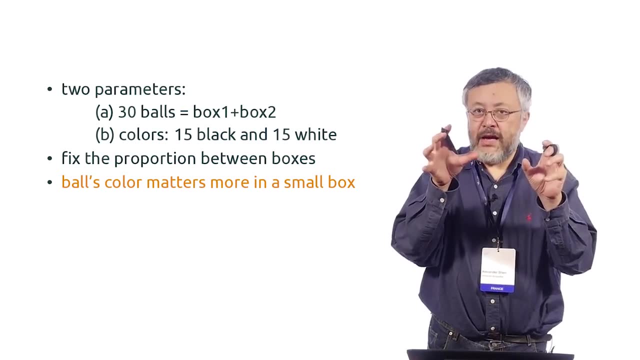 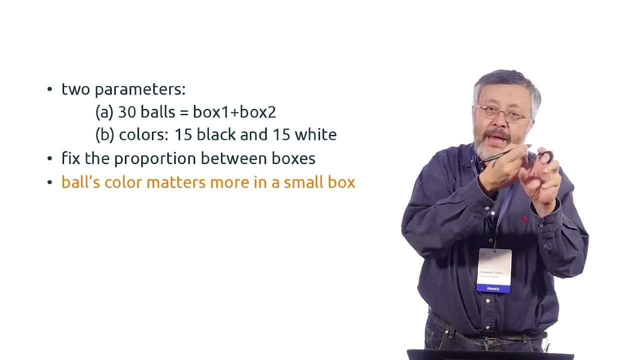 small box and big box. no, a box with small number of balls and big number of balls. so, and then you can vary, change the number of black balls and white balls, so you can add. you can make one black ball white in a small box, but you have to pay. 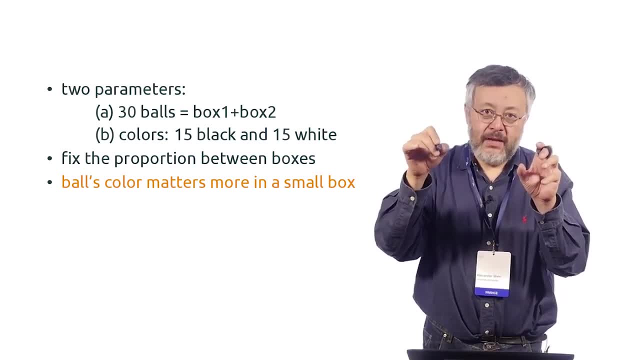 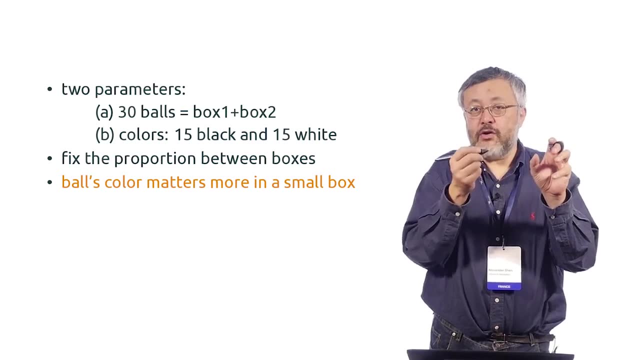 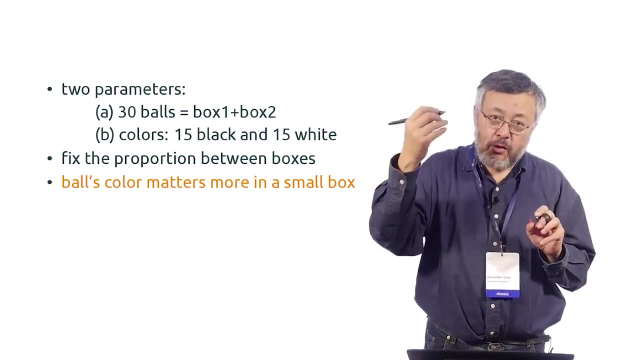 and make one white ball black in the big box. but the increase in probability in the small box is more important because the denominator is smaller. so if the total number of balls is smaller then each ball means more, and for box with a large number it means less. 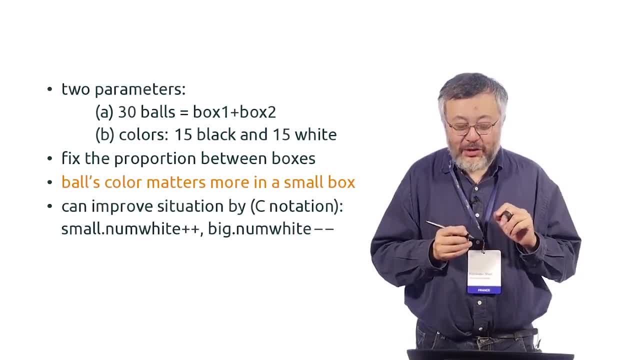 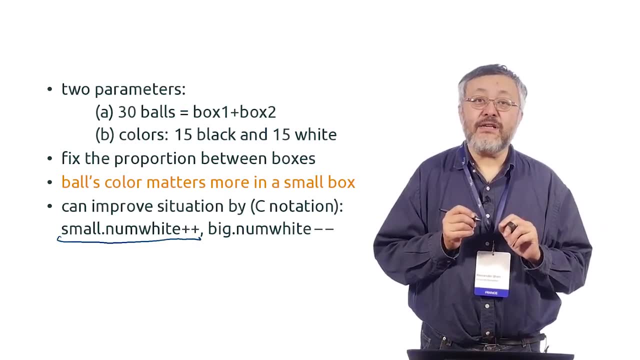 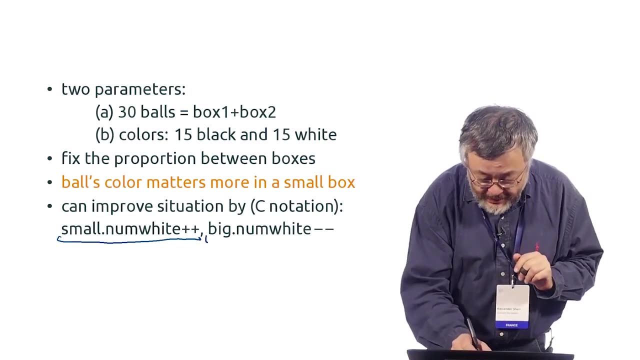 so we use a strange C notation just for fun. so this means that in small box the number of white balls is increased by one and the number of black balls will decrease to keep the total number the same and in the here to compensate in the bigger box. 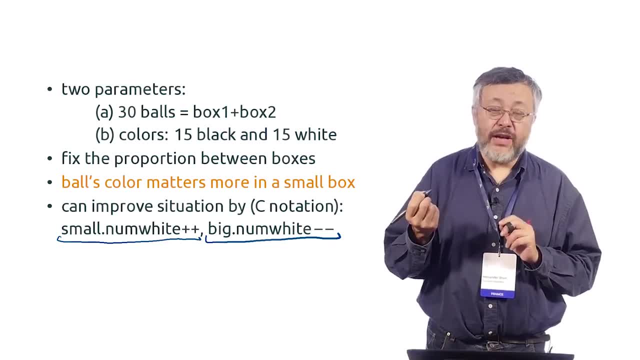 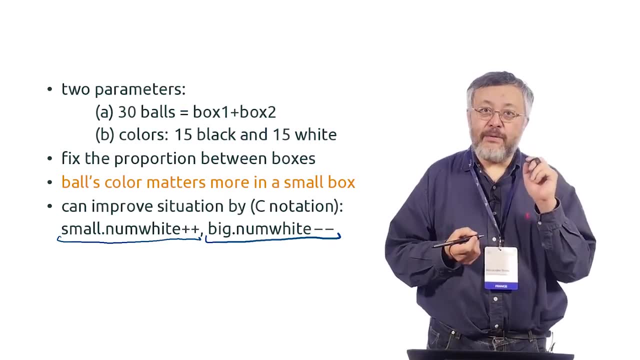 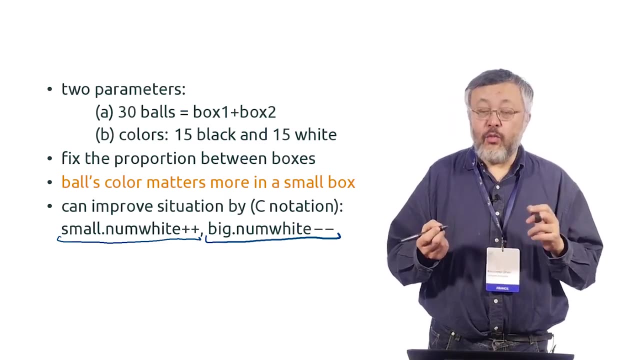 with bigger number of balls, we should decrease the number of whites by one, and what I am saying is that is profitable, because in the smaller box each ball costs more, so to say, and so we can do this, repeat this until we have all the white, all the balls, in the small box. 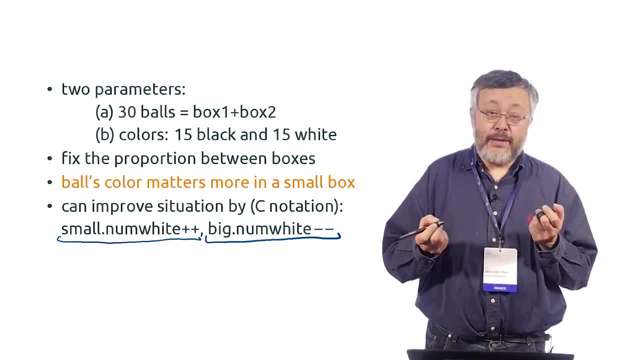 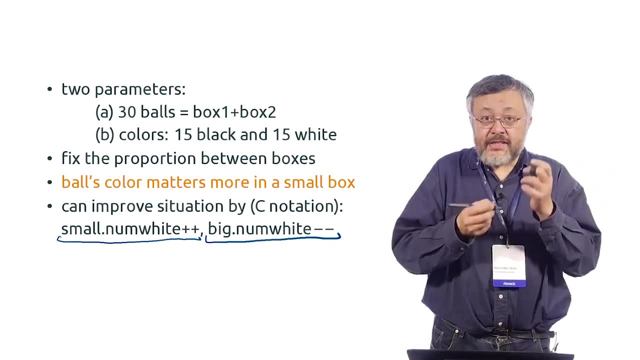 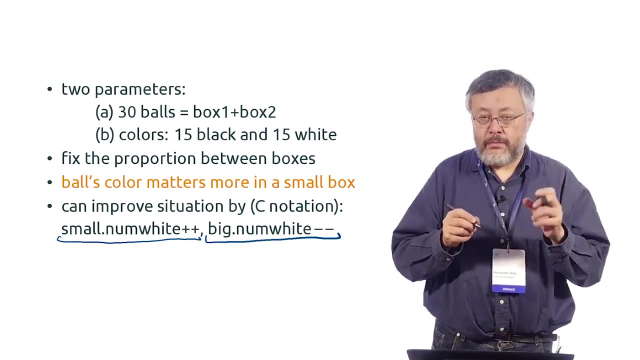 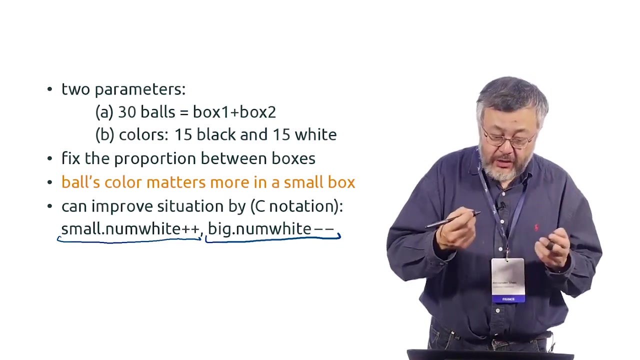 are white now and it is enough white balls because it is smaller box- at most 15. ok, so we see that situation can be improved. whatever we start with, we can improve the situation by adding making balls in the small box white, but then imagine we continue this until it is possible. 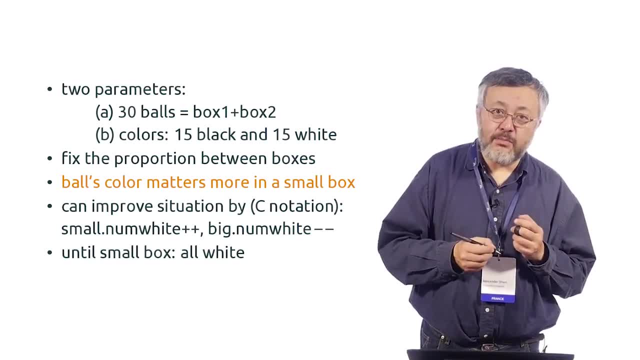 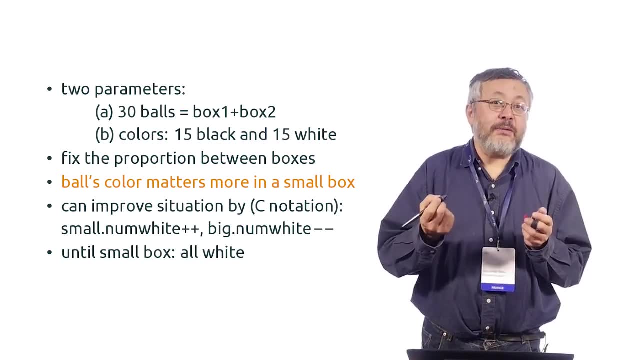 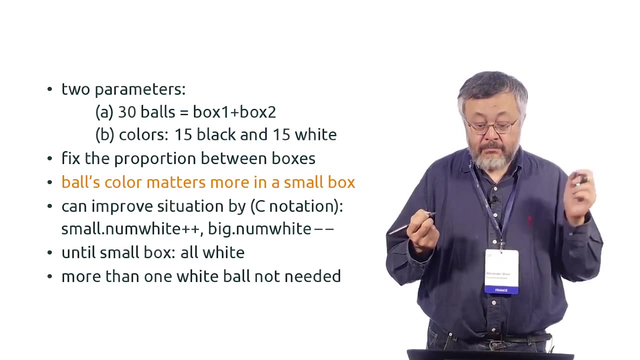 when we finish with all white balls in the small box. but then it is easy to observe that we don't need that many, so one is enough. it is still probability one, and still the other balls can be used to increase our chances for the other box. so we get exactly. 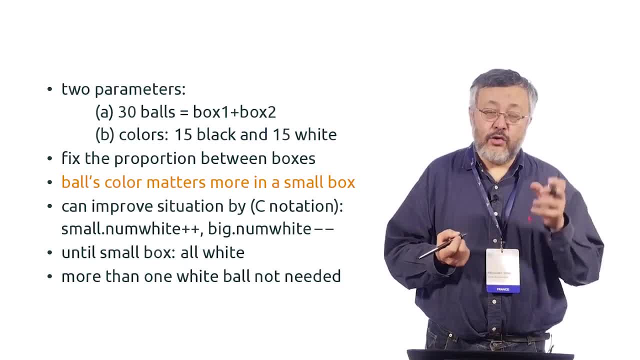 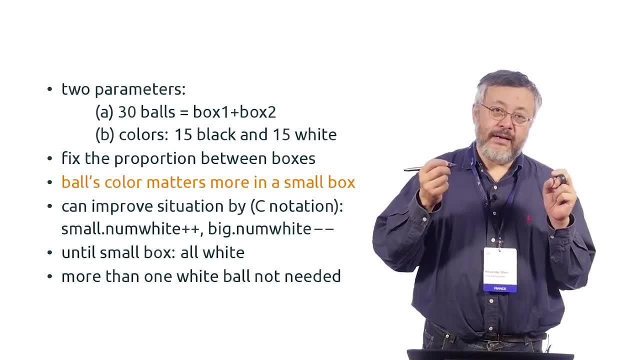 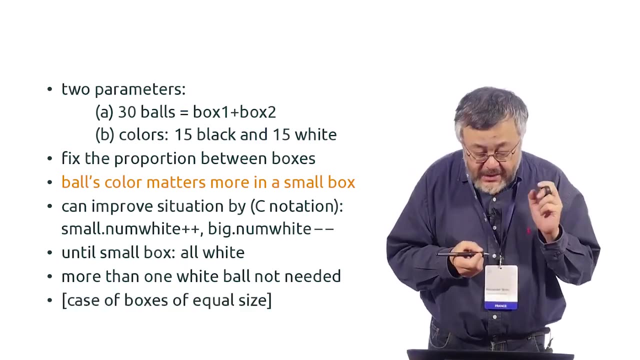 exactly the same the answer we claimed. so in the small box we have one ball- white ball- and all the rest, all the white balls and all the black balls- are in the other box. just exactly what we said. there is a small technical detail that when we say small and big box here, 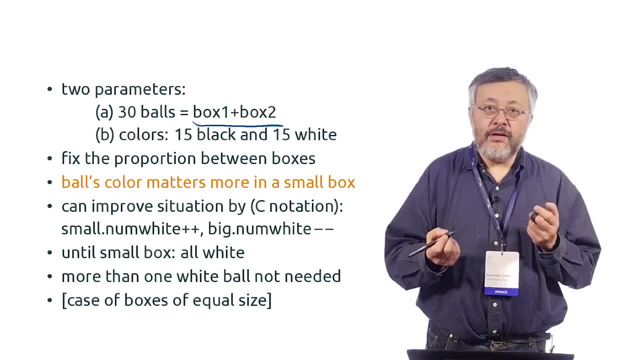 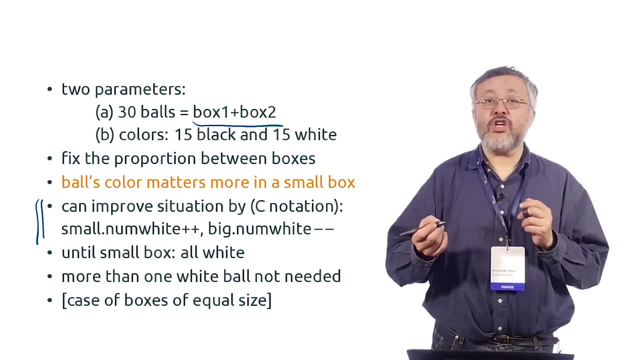 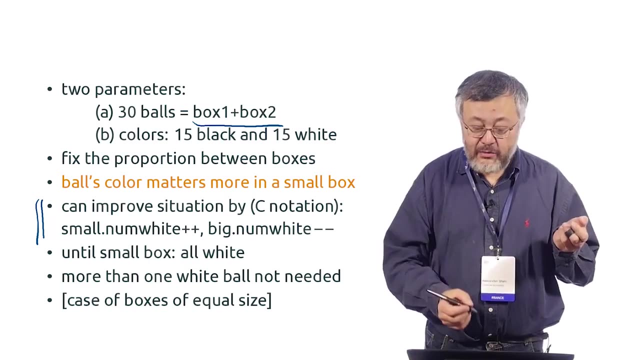 we assume that one implicitly forgot the case when they are equal. but then, of course, if they are equal, then this first stage doesn't change, doesn't make things better, but also doesn't make them worse. so we can do it anyway. and then we came, improving, to this optimal case. 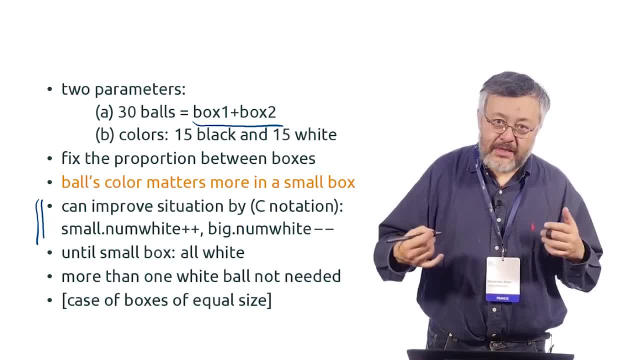 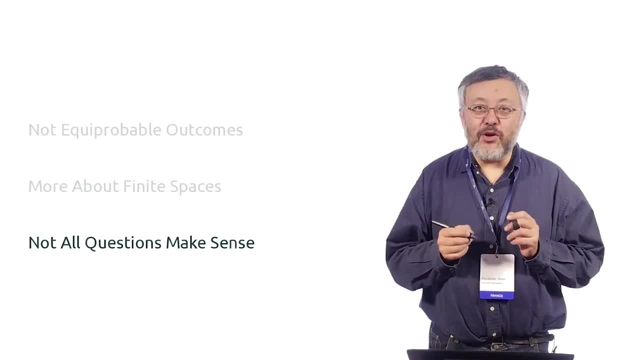 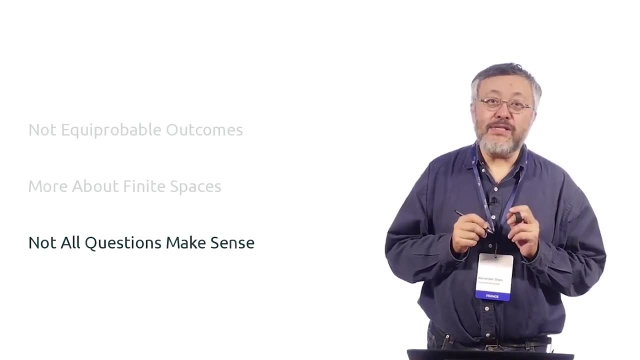 so this case can be obtained from any other, and so optimization ends here. so it is optimal. you can complain that I am telling more what you should not do after hearing this section, but it is very important, because the most dangerous probability theory is not that you cannot compute something. 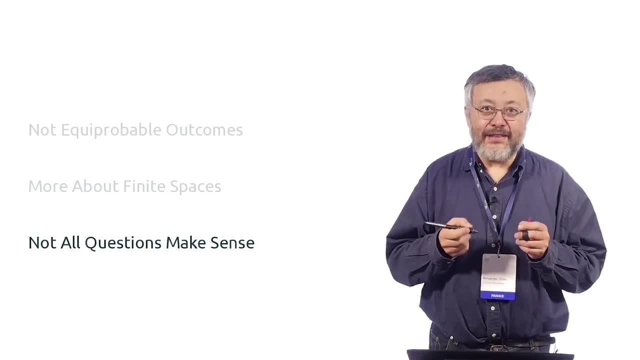 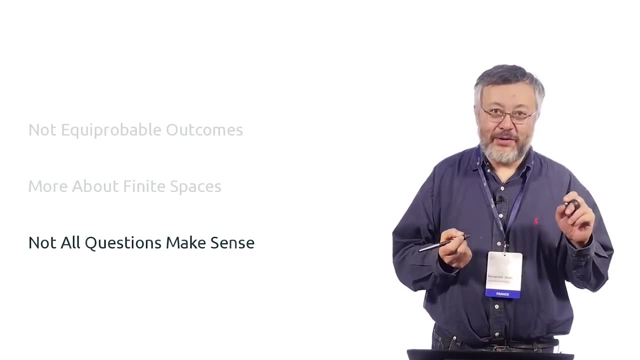 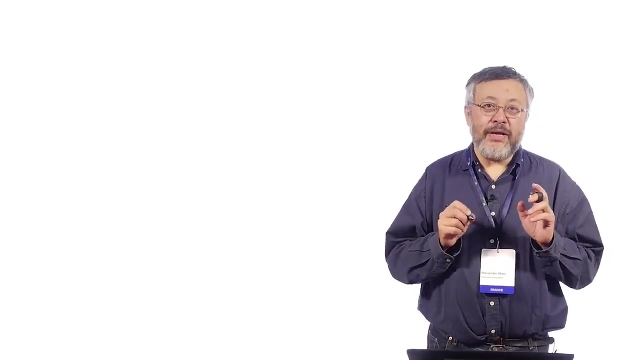 the danger happens if you believe that you have computed something and this is wrong, you make a wrong decision, thinking that it is based on probability theory. so let me say something about what you should not do. the first thing you should be very careful is the probability of the past events. 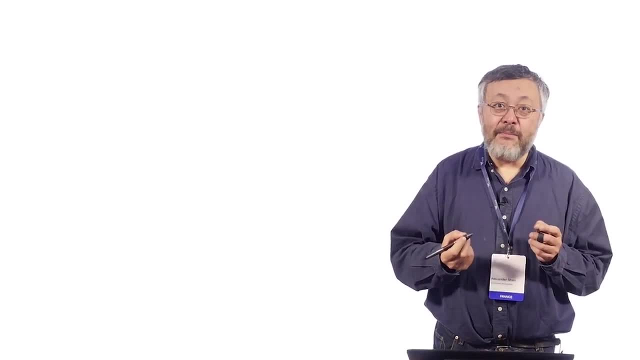 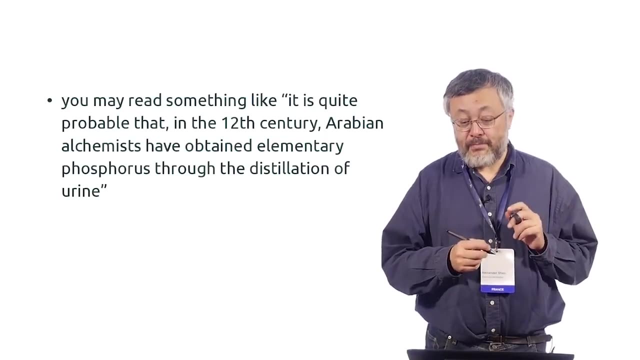 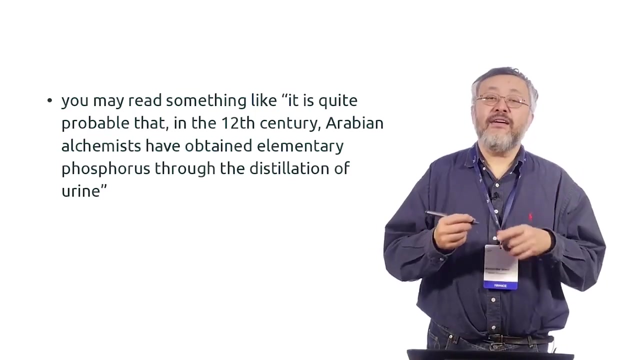 events in the past. so I looked in some to get an example. I looked, just googled- for some historical statement and that is what I found. it is from actual, actual historical historical paper and it is quite probable that in 12th century something happened and but 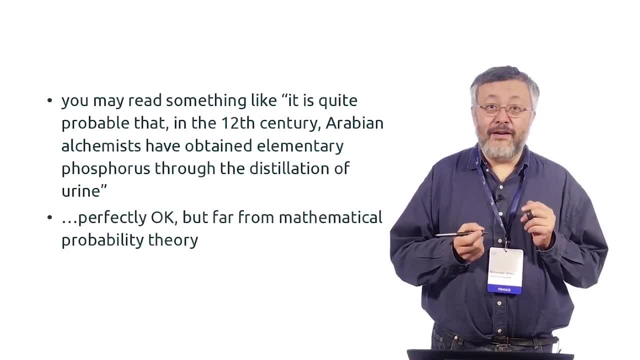 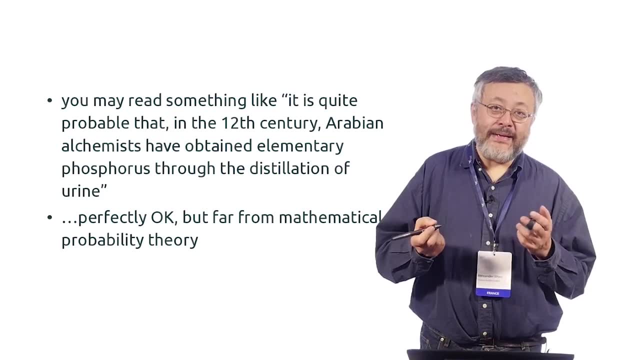 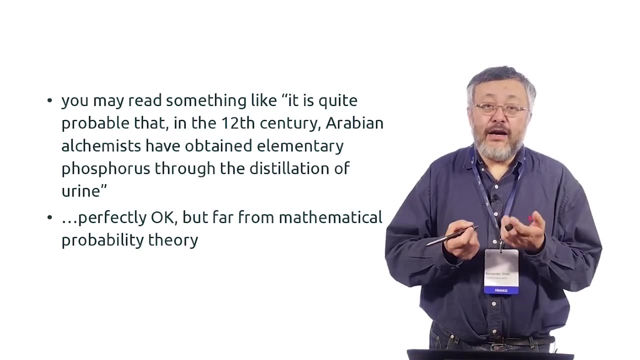 ok, you can say it is quite probable. but if you, it is not mathematical probability. if the other guy asks what you think is the probability greater than two-thirds or smaller than two-thirds, probably this has no meaning, because two-thirds means that if we repeat the experiment many times, 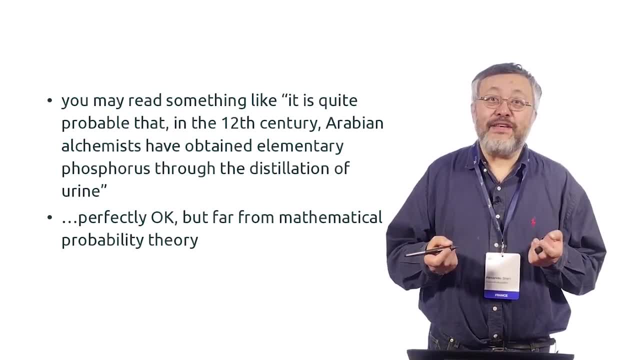 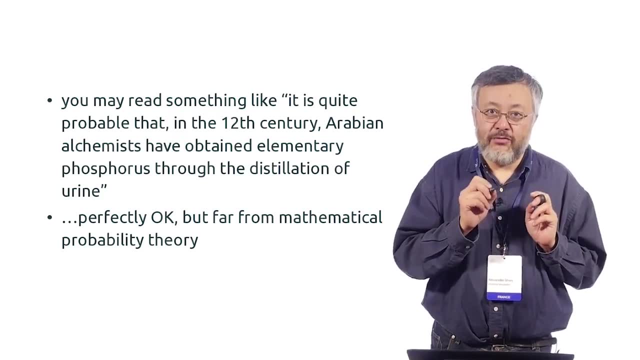 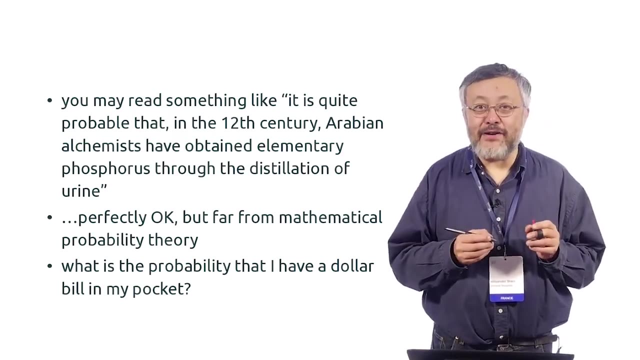 we will get something, but you cannot repeat the experiment, so the numerical value for this probability is something very strange. you should avoid this. another example more clear. so imagine I ask you what is the probability that I have a dollar bill in my pocket and you may start to guess this? 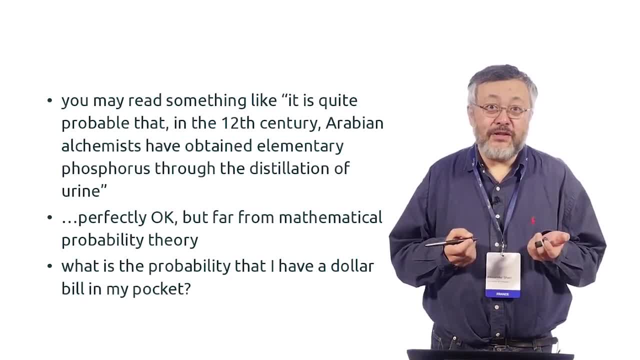 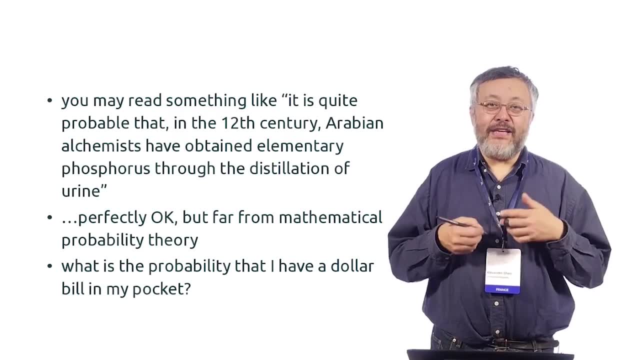 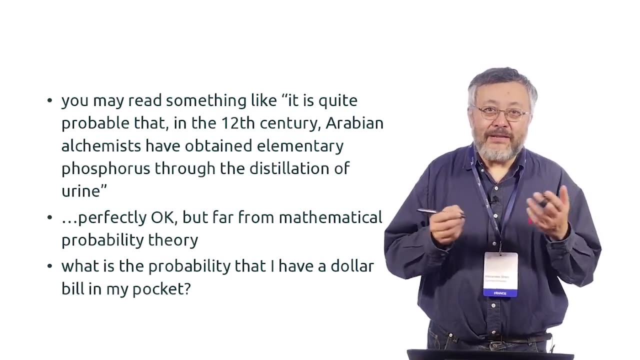 but it is not the correct thing to do, because I either have it or I don't have it, and it is not clear what the probability could mean. there is no. if each day I come with the dollar bill or without the dollar bill, you can compute the fraction of the days. 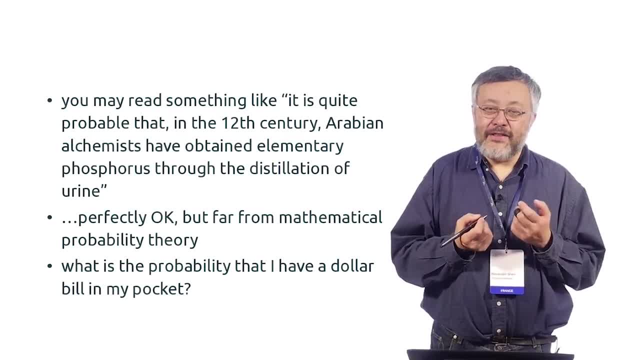 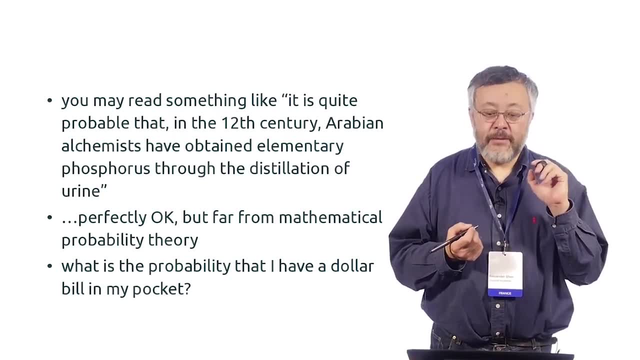 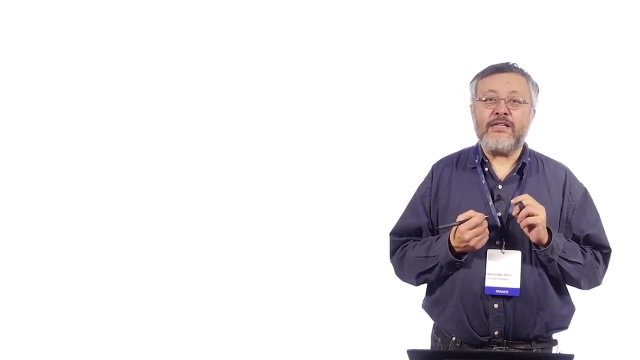 when I come with it, but in one isolated case the question has no meaning. we will see later something when it still can have a meaning, but a different meaning. ok, there is one very clear example of this case, and it is. let me tell you, so you know, that. 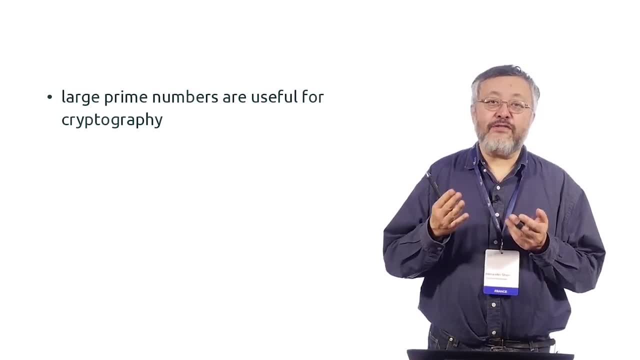 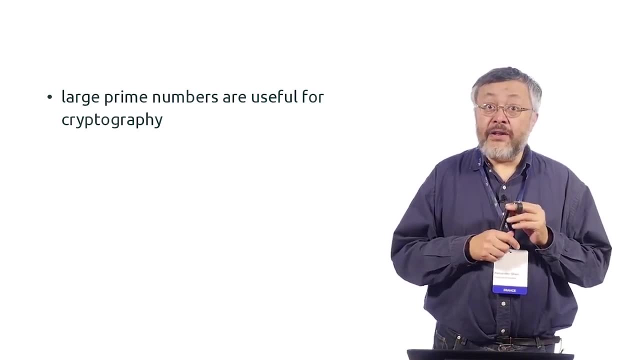 first prime number. prime number is a number that cannot be factored. so I don't know. 5 is a prime, but 6 is not, because it is 2 times 3, so a prime number. you cannot factor it and big prime numbers are rather important. 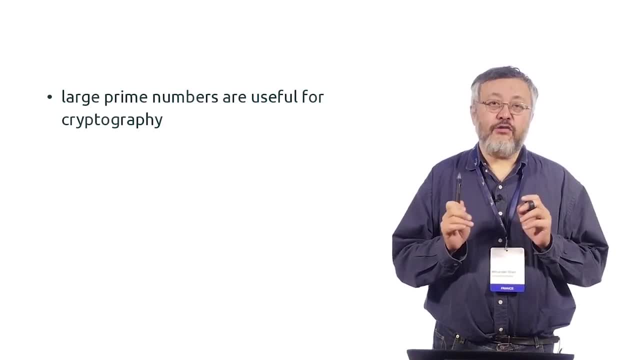 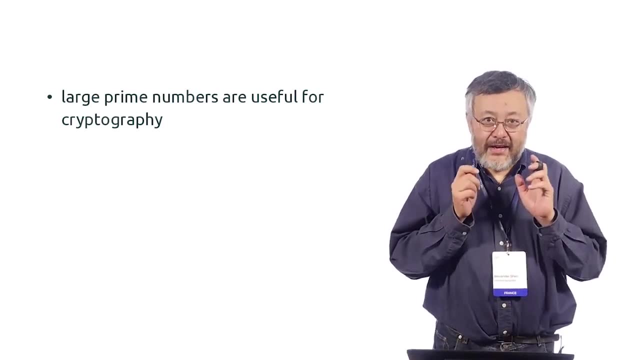 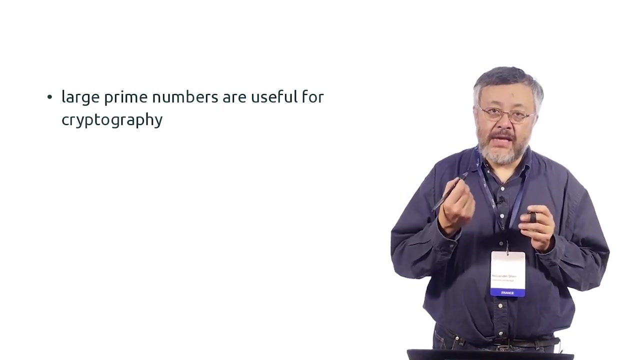 because we will see this later. they are used for cryptography. for cryptography, you take two large, big prime numbers, you multiply them and nobody can factor back. but anyway, you need the big prime number and there are algorithms which are used to decide whether a number is really prime or not. 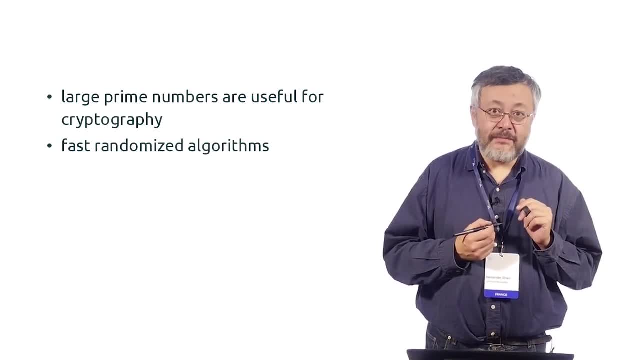 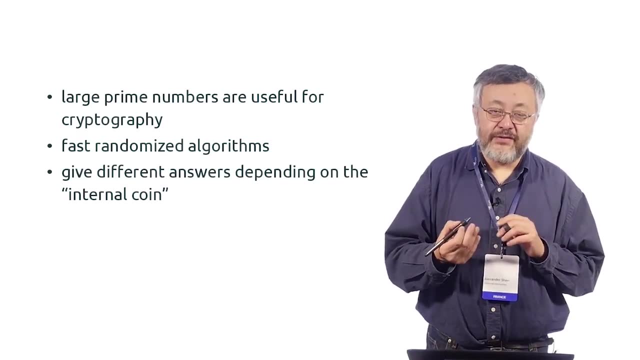 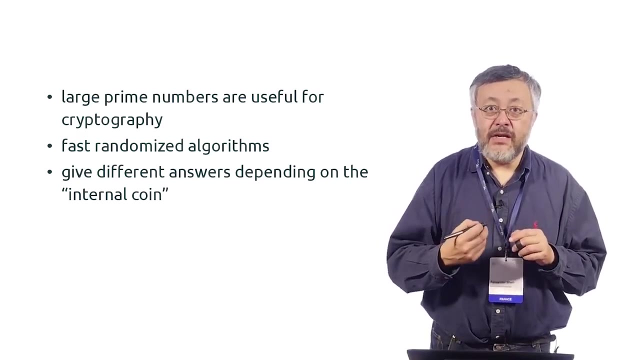 but the fastest algorithms are randomized. what does it mean? the algorithm uses some internal coin. it is not a coin actually. it is some other physical device or some prepared random bits, but the answer of the algorithm depends on the values of these random bits. so if we apply this, 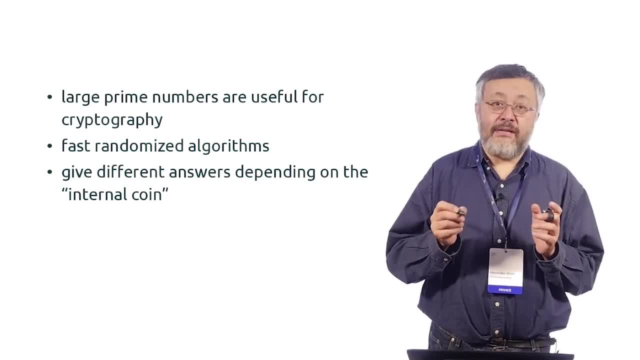 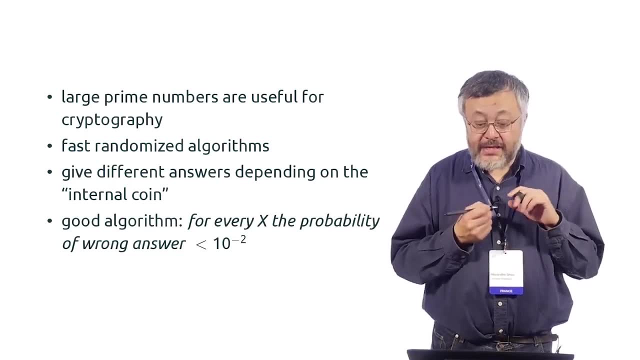 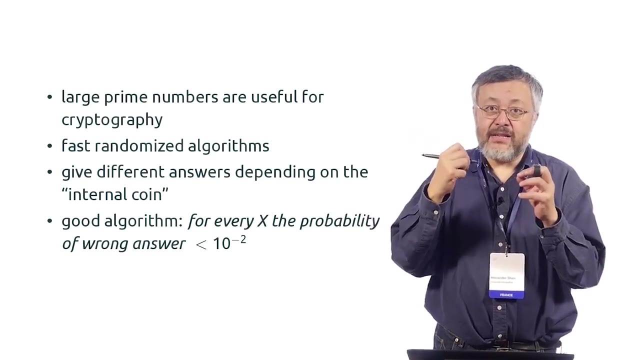 this algorithm many times to some number, then it can get different answers and there is a proportion of correct answers. and if you write a good algorithm you can prove, for example, that for whatever number you take, if you repeat the same algorithm on the same number but with different random bits, 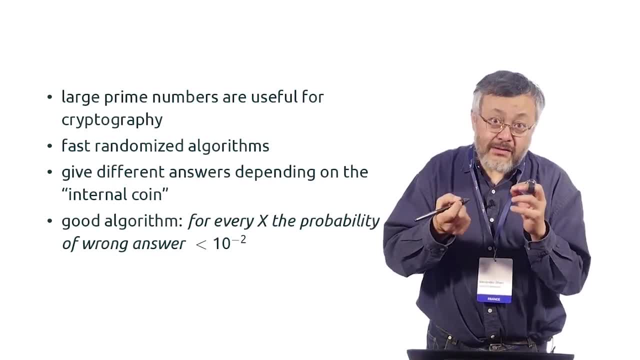 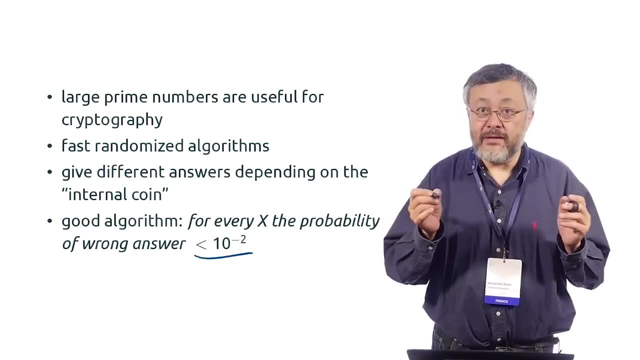 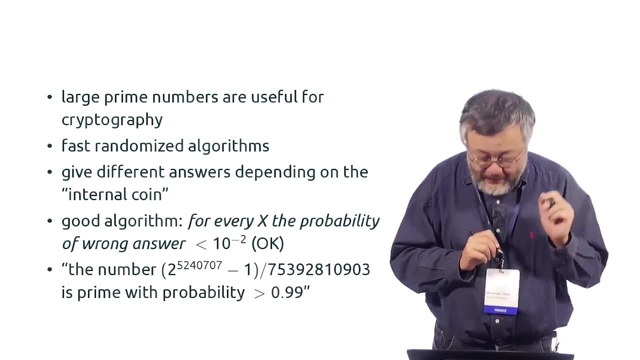 you will get different answers, but most of them will be correct. the probability of wrong answer is, say, less than 1%. okay, this is perfectly good. this is a good statement. what is not good if you say something like this? imagine you tried this algorithm for some number. 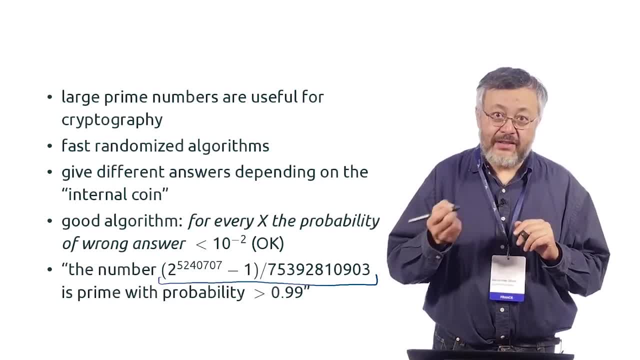 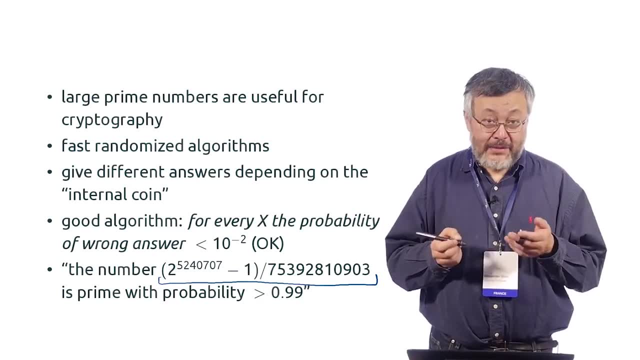 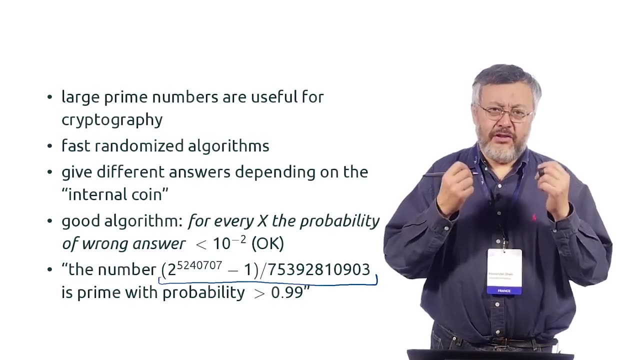 so I choose some number which was actually people don't know whether it is prime, so they try this randomized algorithm. so imagine you tried your good algorithm on this number and the algorithm says it is prime, as it did for this number, and then you say that, look, this number is prime. 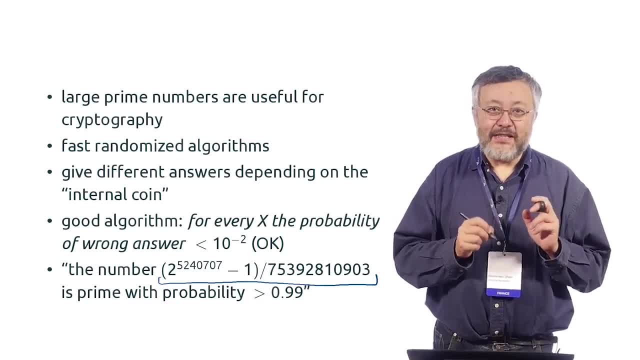 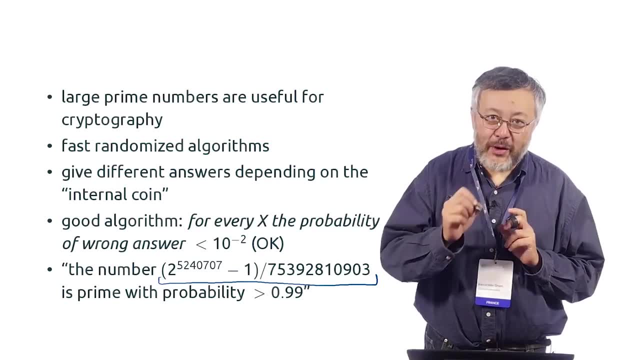 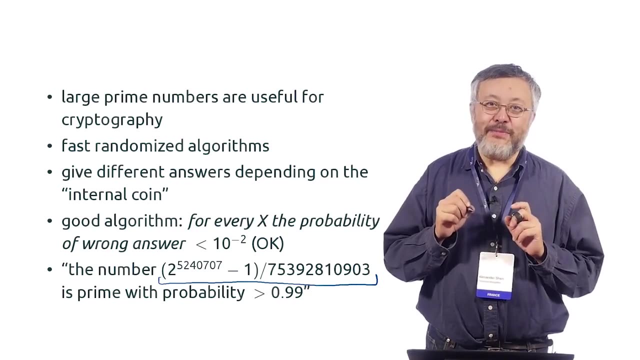 with probability at least 99%. this is complete nonsense. this number is either prime or composite. it is not prime with any probability. so you should avoid such a statement and you should see when somebody else makes such a statement and you should be very careful about the knowledge of probability. 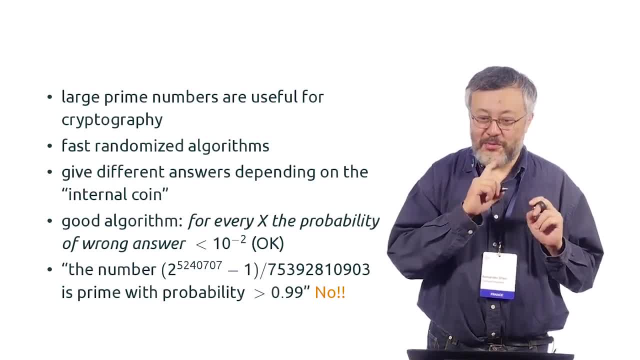 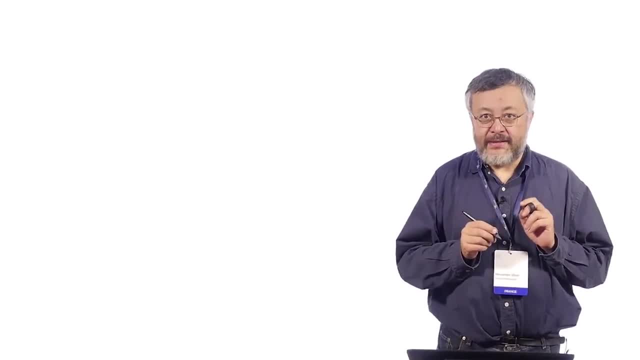 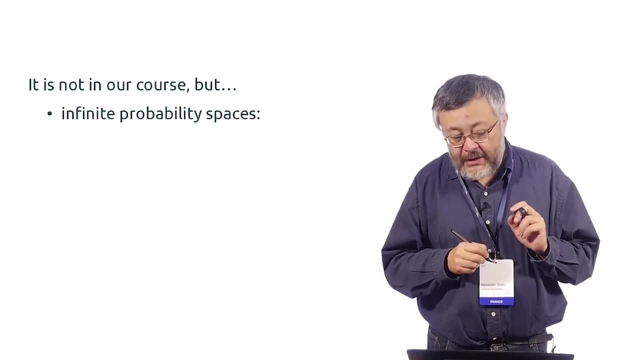 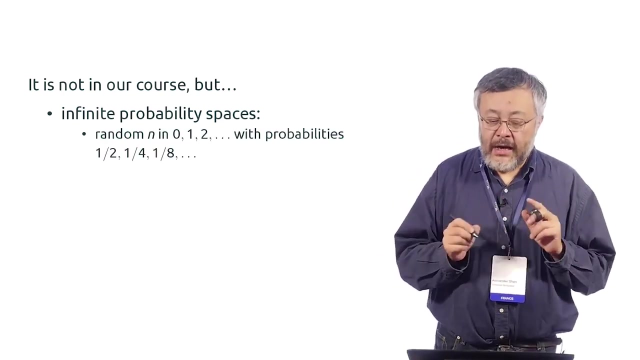 for this guy who says this, this you should not do. now let me say about what probability theory, how it can be extended, and first the simple thing which I already have said, that is, infinite probability spaces. so, for example, the meaningful setting. if, for example, we want to take 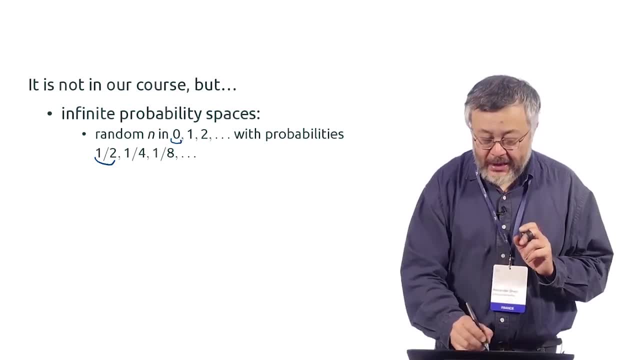 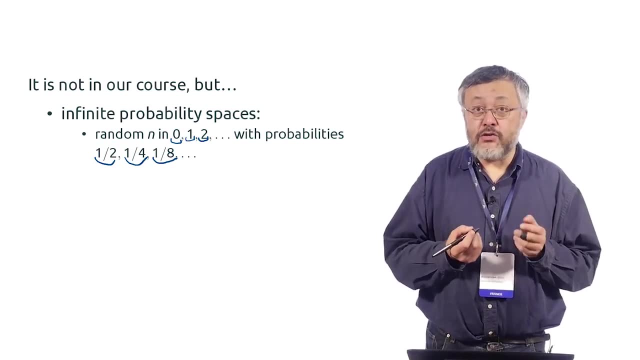 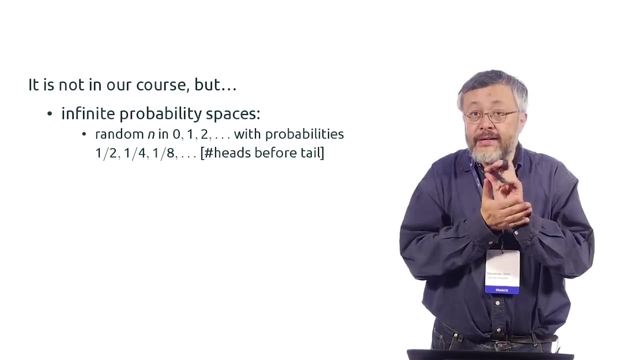 random natural number, and we agree that 0 should appear with probability 1 half, 1 with probability 1 fourth, and 2 with probability 1 eighth, and so on. it is even easy to imagine an experiment which produces this, so, for example, you can toss a coin. 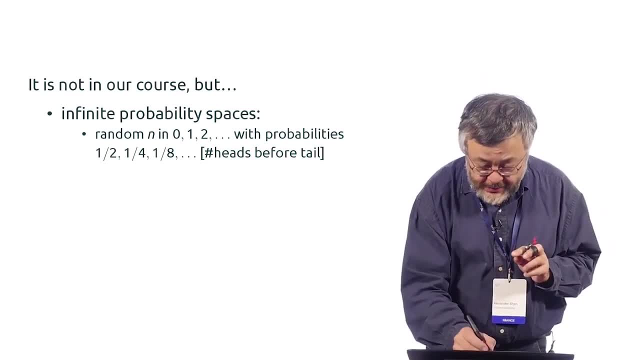 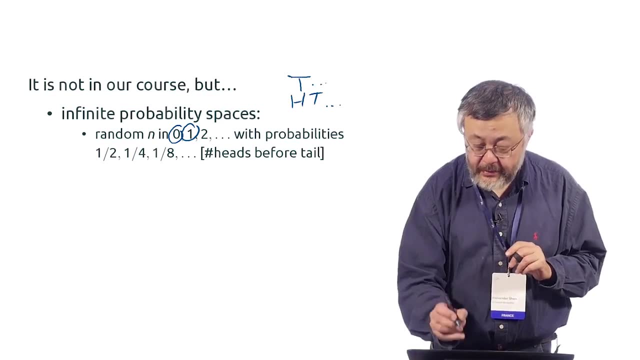 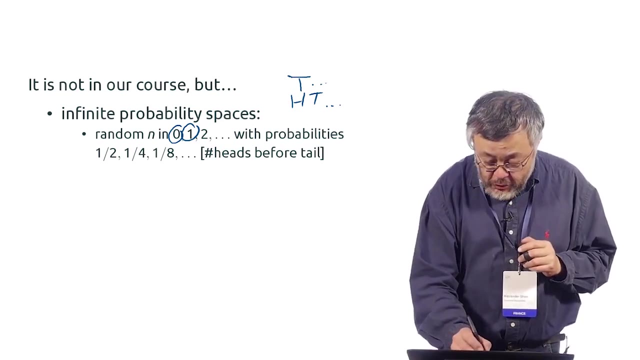 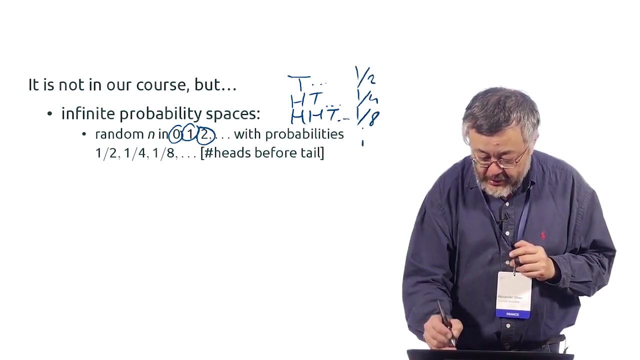 and count the heads before the first tail. so you say 0 if you get a tail immediately, you say 1 if it is head tail and something you stop coin tossing here. but anyway, if it is 2, it is still and the probabilities are exactly 1 half. 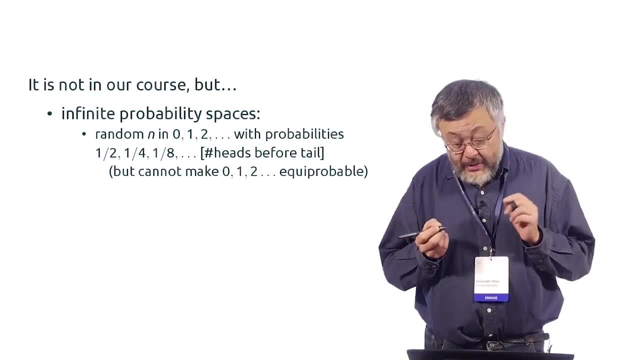 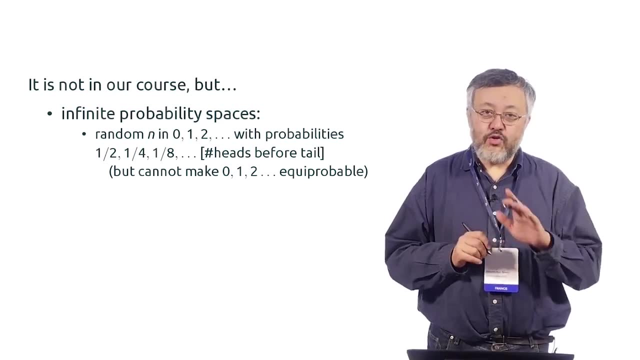 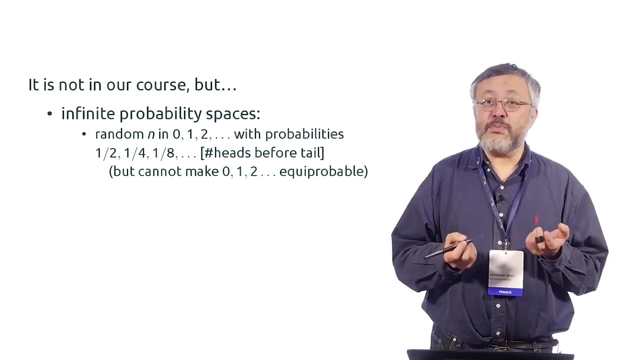 1 fourth, 1 eighth and so on. so it is kind of a reasonable thing to consider such a space. but if somebody says that take a random integer and make all of them equally probable, then you should immediately complain and this has no meaning, because if they are equally probable, 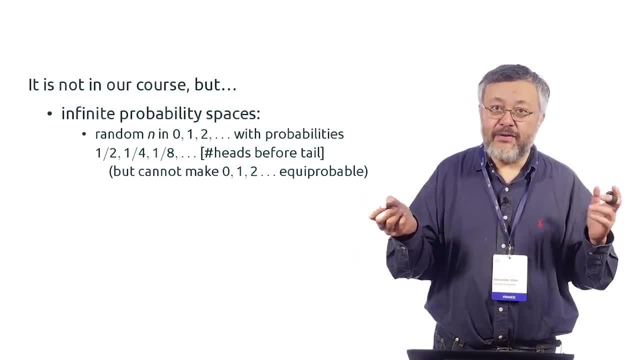 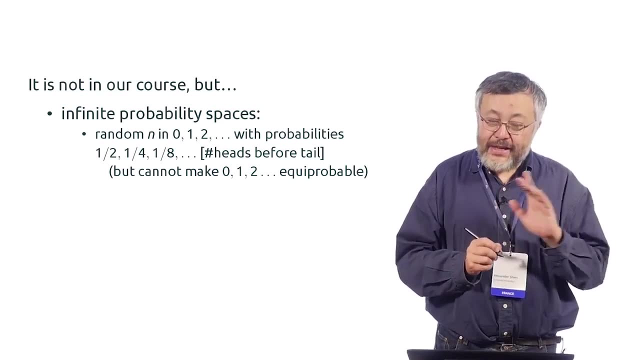 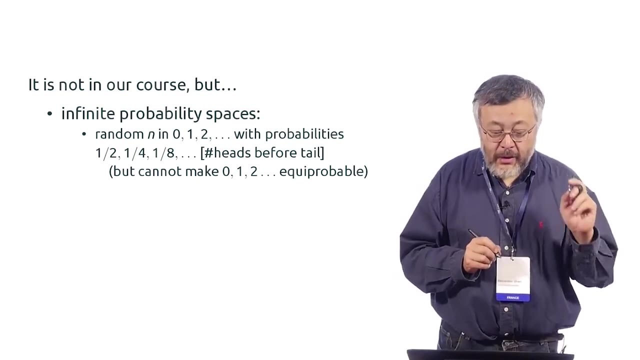 then what is this probability? if it is positive in the initial segment, so the probability should be 0. and if all probabilities are 0, what does it mean? so equi-probable integers is something impossible. ok, this is the first remark and the second case we also mentioned. 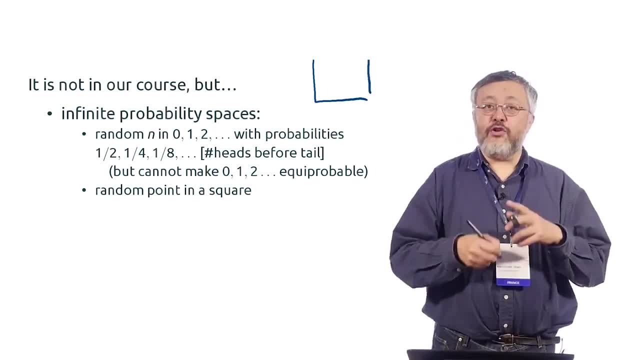 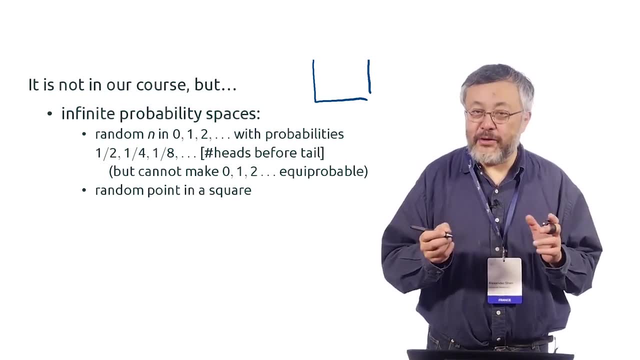 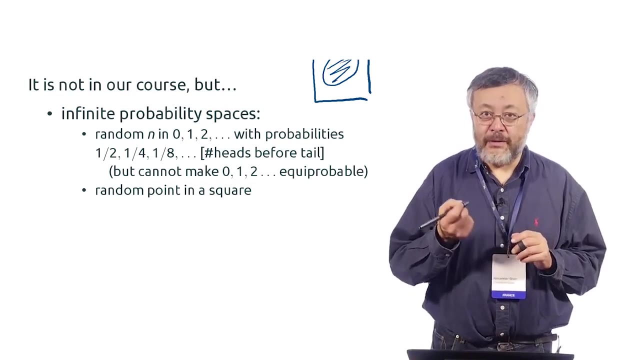 and when we take. we can find a random point in a square. if you go on the street and wait until a drop falls somewhere, it is a random point in a square and the probability to get it inside some zone is proportional to the area of the zone, and so on. 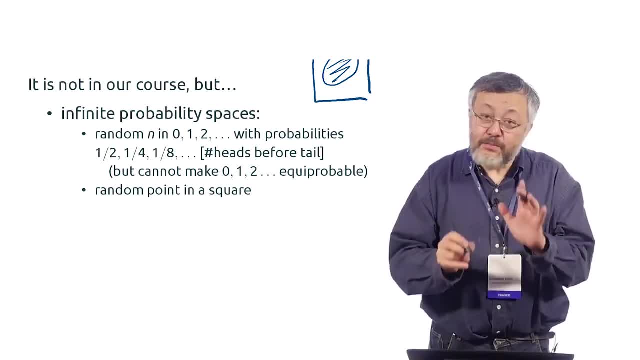 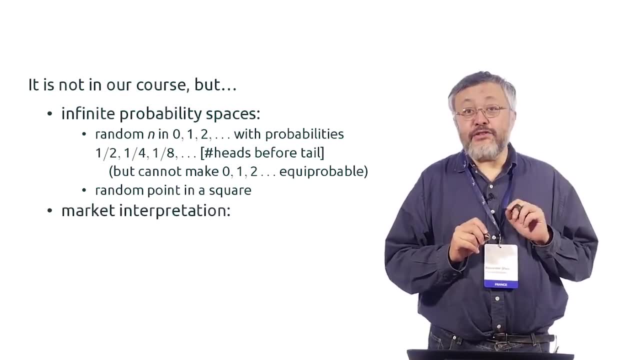 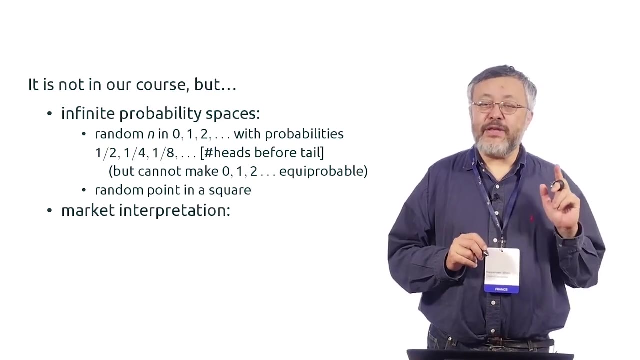 so infinite probability space are dangerous, but not that dangerous. in many cases it is a reasonable thing. and another thing which somehow even the probability of individual event, which I told you that you should not consider, sometimes they can be considered, so to say. so imagine that we want to ask. 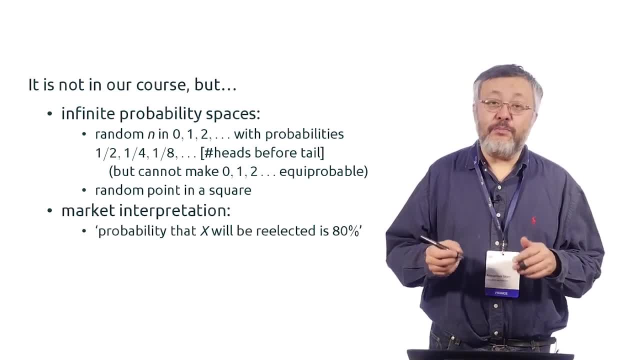 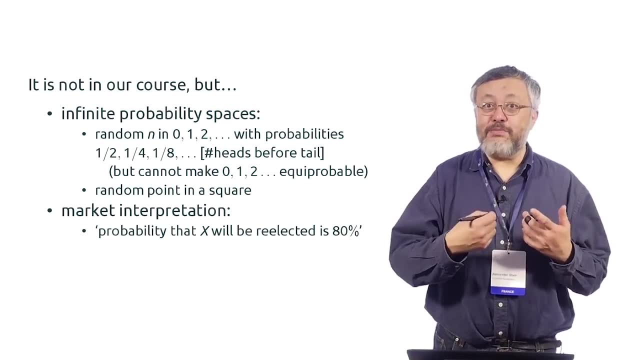 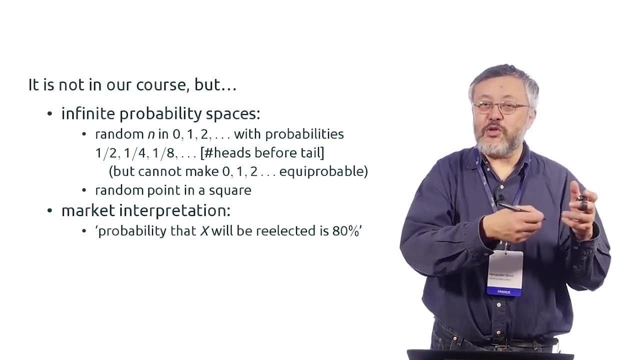 what is the probability of some guy, politician X, to be re-elected? and you can say the probability is 80%. what does it mean? of course you cannot repeat the experiment. you don't have many worlds with the same guy in each of them and see how many of them. 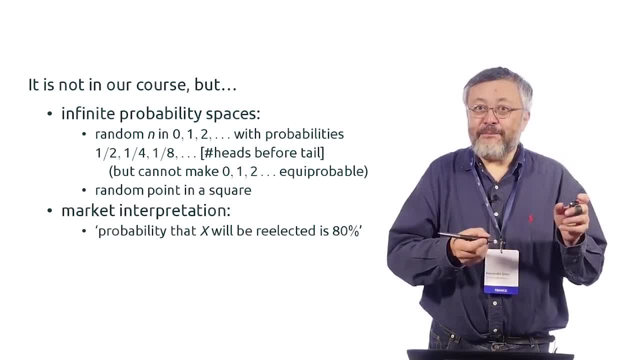 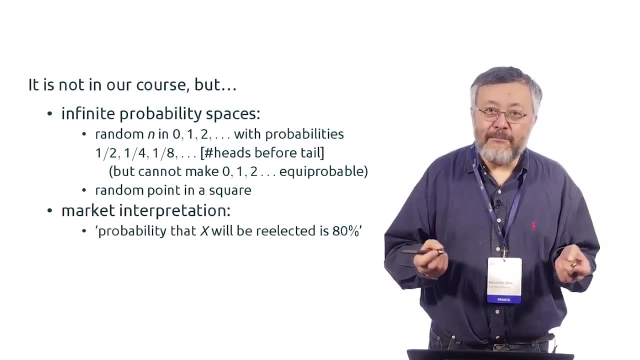 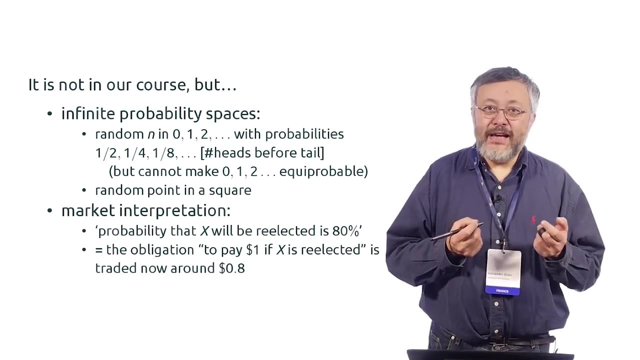 in which proportion are the worlds when he is re-elected, and so it looks like something stupid and non-existent. but still imagine that some people don't like this guy to be re-elected and they want some insurance. the insurance is just a paper that guarantees you that if he is re-elected, 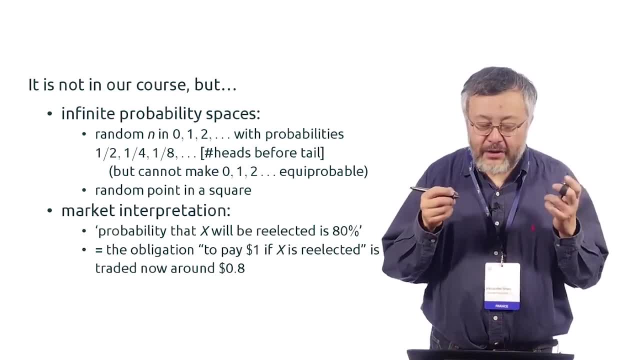 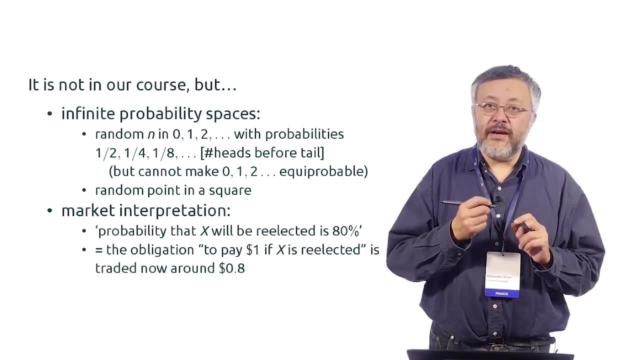 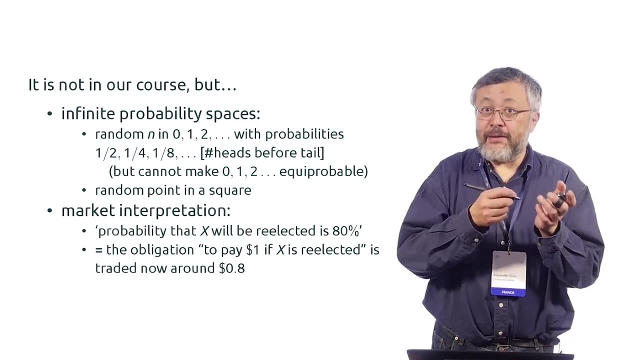 the insurance company will pay you, I don't know, one dollar or any other amount, and the question is the market price of this insurance paper now. so if there is a market for such a thing and if the selling price is close to buying price, then you can say that. 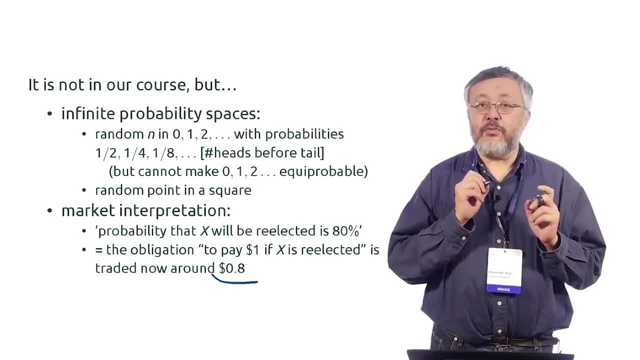 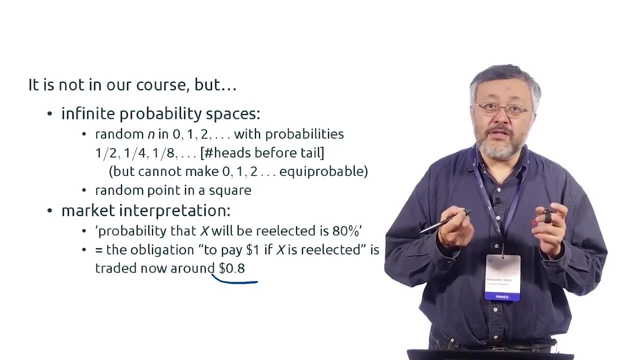 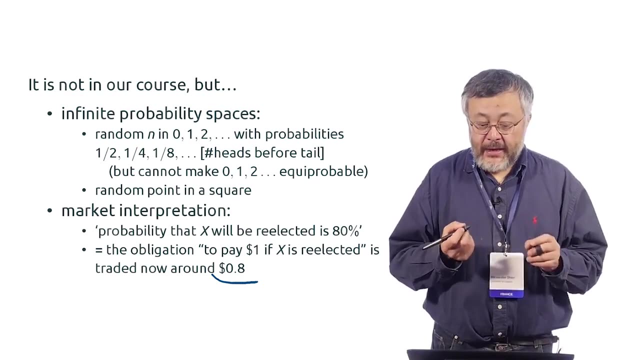 if it's, for example, around 0.8 dollars, then you can say the probability of being re-elected is 80%. of course it has no statistical meaning, but still this number obeys some rules of probability theory and you can even prove the sum rule. 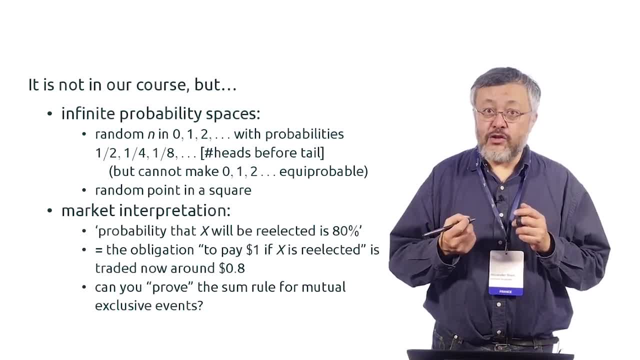 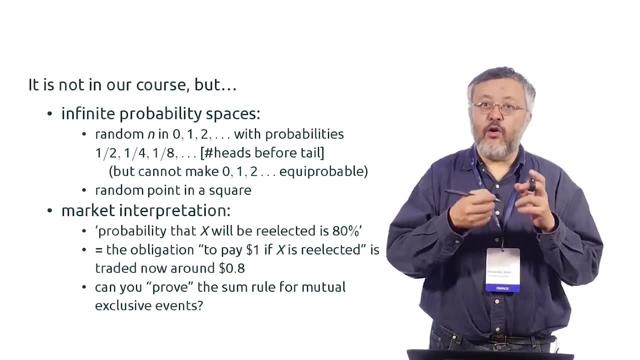 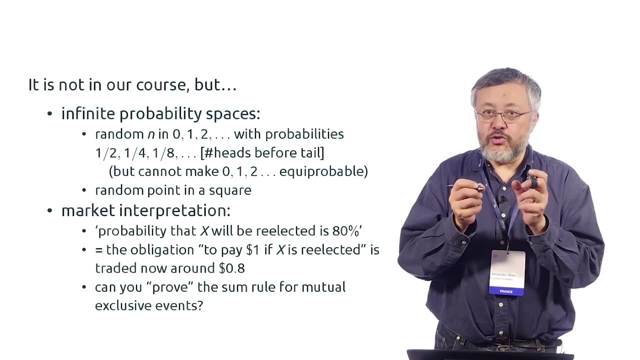 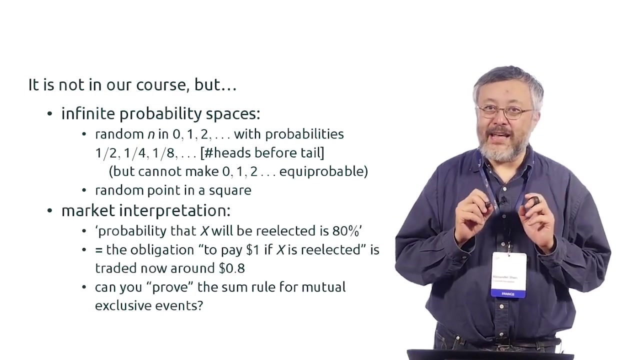 for disjoint events. so, for example, if you want to consider the probability of A being re-elected and B being re-elected and the probability of A or B being re-elected, and there is some reason why the insurance paper for all three cases should have matching probabilities, the last one should be: 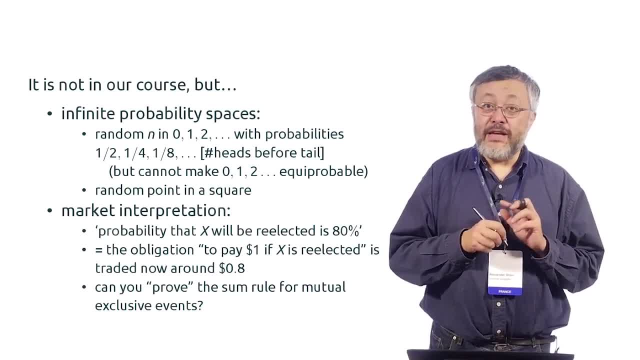 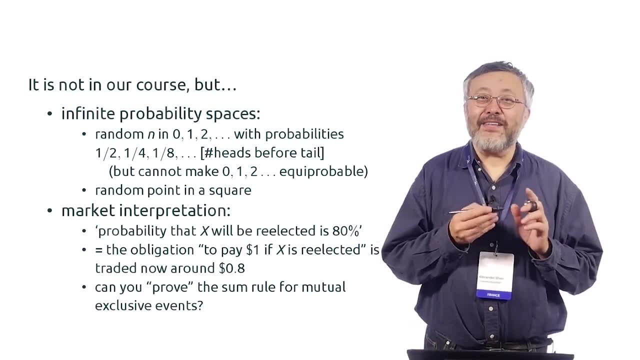 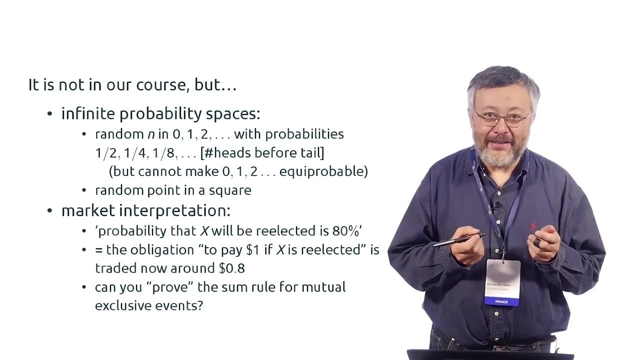 the sum of the previous two and why it happened. so if the problem with my pocket has a dollar in it- no, there is no dollar actually. so the problem with this insurance is that nobody will sell or buy insurance on this, so there is no market. but for more important event, 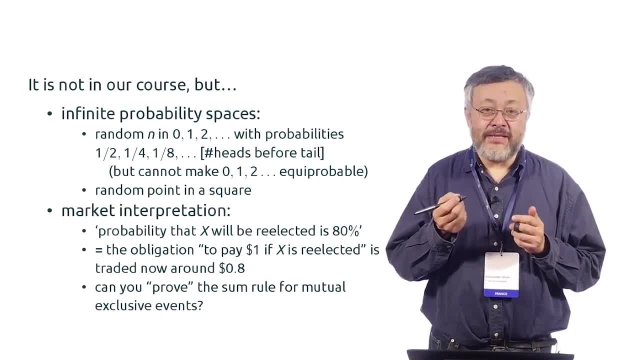 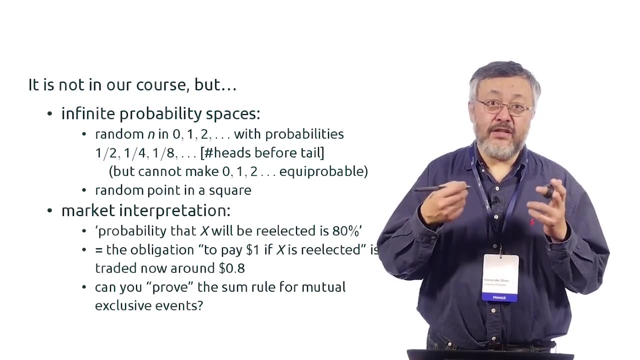 there is a market. and if there is a market, actually you can bet. in some countries it's legal. you can bet for political events. the market price can be considered as a definition of probability for individual events, and then we also get somehow a probability space, even if there is no repeatable experiment. 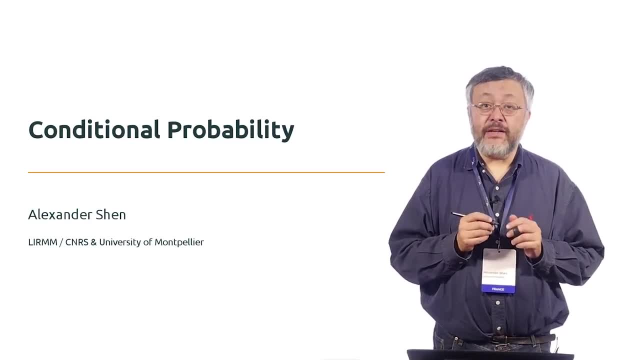 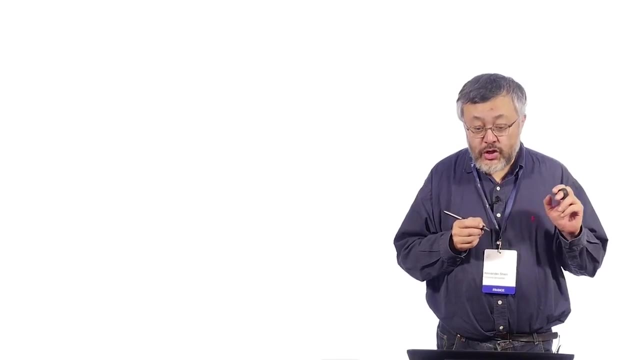 so now we switch to a topic which somehow is central in probability theory, which is distinguishing from measure theory or combinatorics: the conditional probabilities and independence. so first, conditional probability is some example which just some kind of demographic example, which has nothing to do with probability theory. 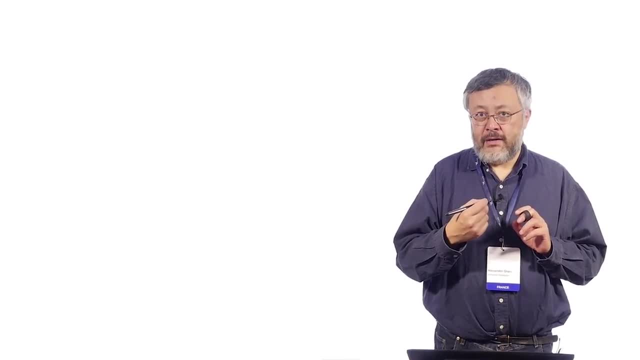 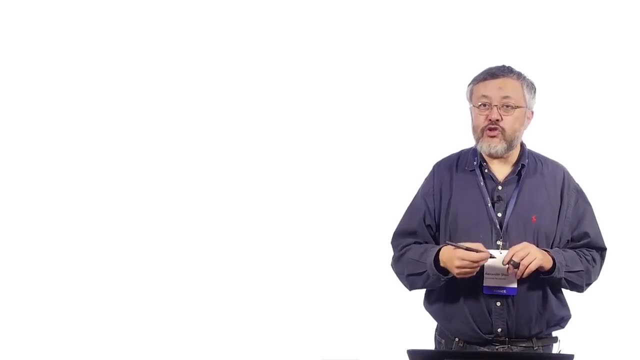 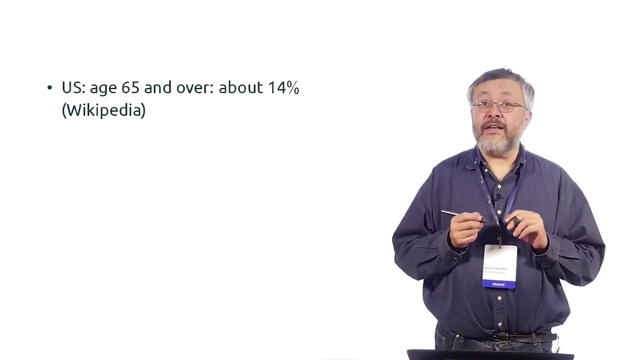 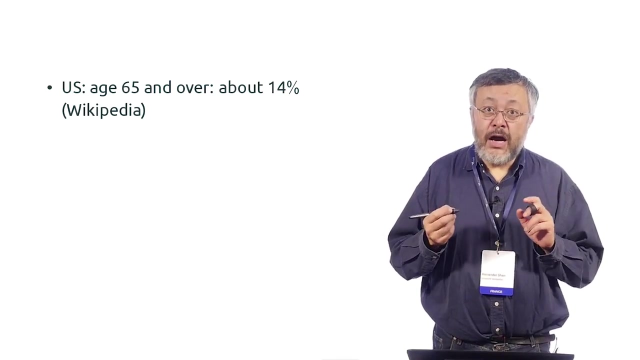 I just want to illustrate the language, probability theory language, by comparing this, by retelling the same story both in normal language and probability theory language. so let me explain. so this is just statistical data taken from Wikipedia. if you look at United States population, then you look how many people 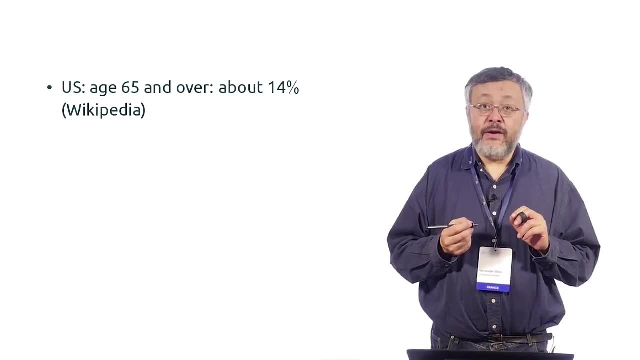 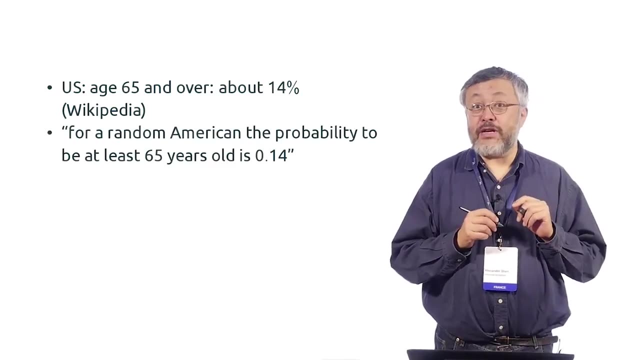 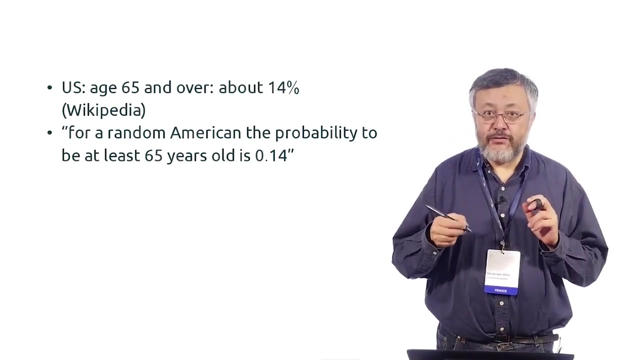 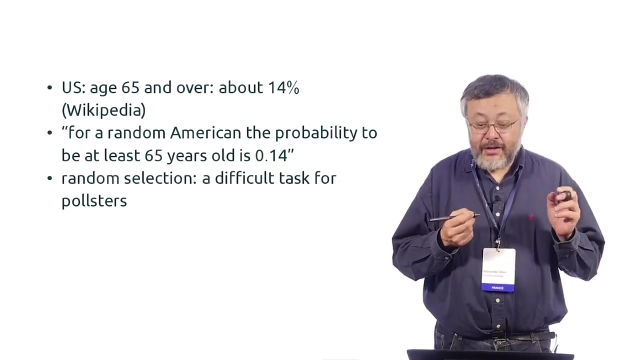 are of age 65 or over 65, then it's 14- 14%, and sometimes you can say in language probability theory that for a random American the probability to be of age 65 or bigger is 0.14. of course it's strange. 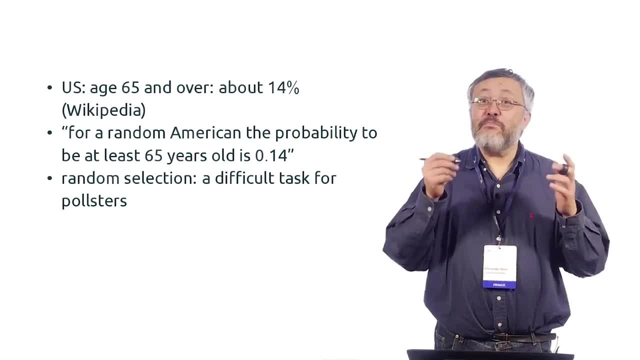 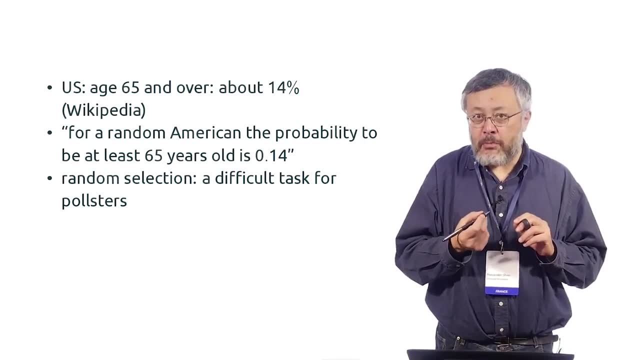 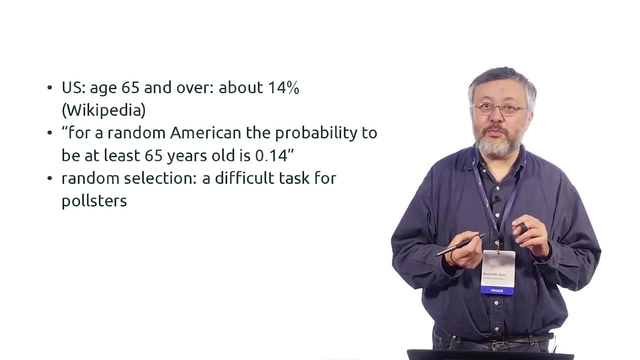 how do you select a random American? somebody comes and picks a random American mystically and it's a real problem. if you make a statistical a poll, you would like to select a random American, but there is no procedure which does this, so it's a big problem for pollster. 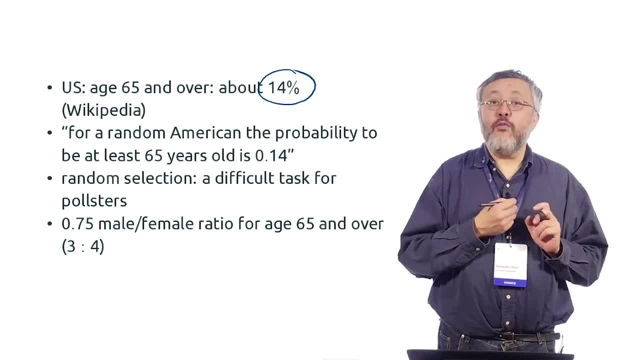 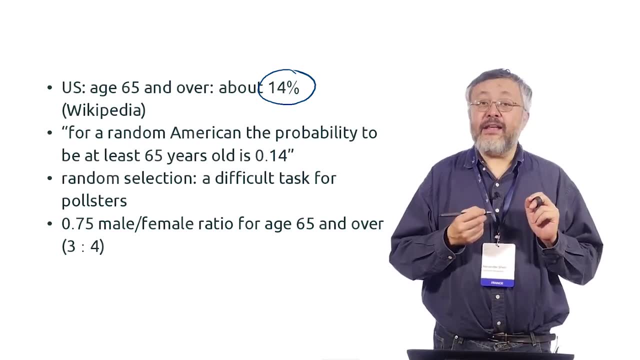 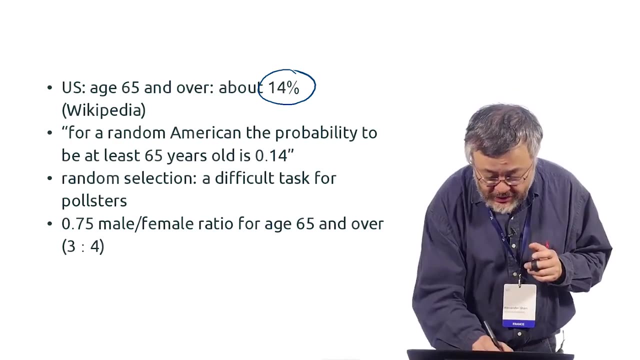 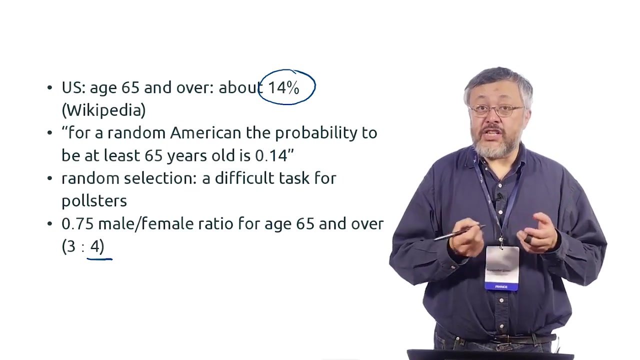 anyway, we agree on this 14%. but now we look at the male-female ratio for age 65 in this group- 65 and over- and actually the women have bigger life expectancy, so there are significantly more of them. 3 to 4. so 3 to 4 is just 3 out of 7. 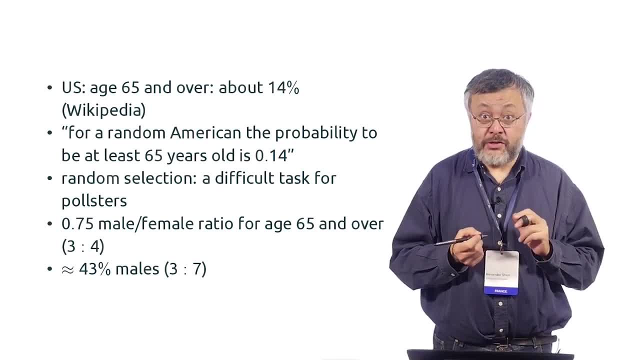 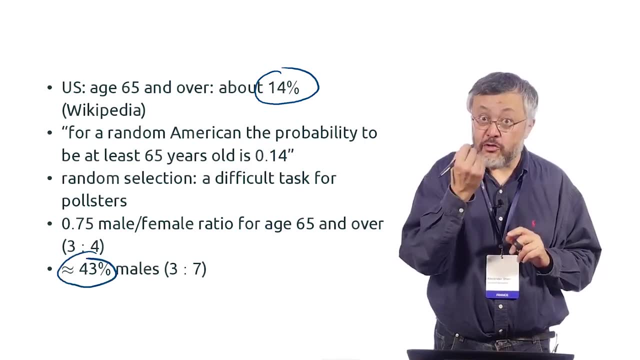 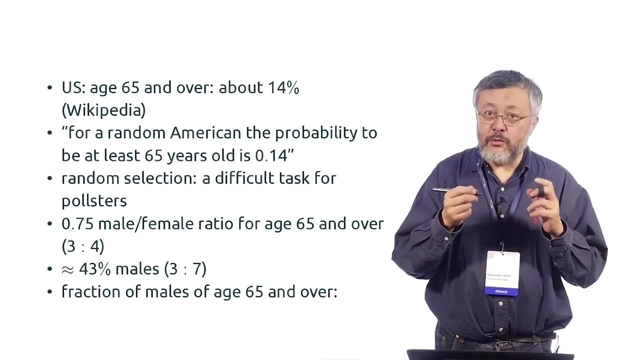 and it's about 43%, and so among this 14% there is 43% of male in this group. only so we can just, if we want to compute the total in total, how much, how many we have males over 65, then we can compute. 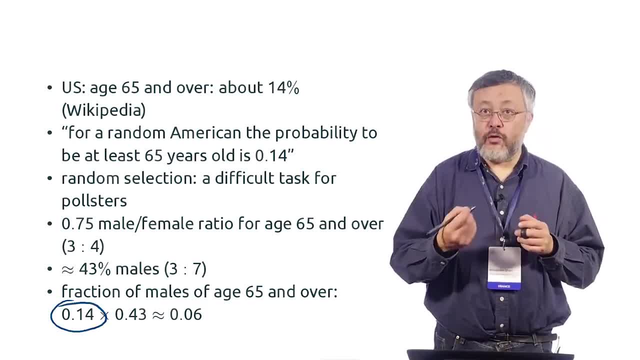 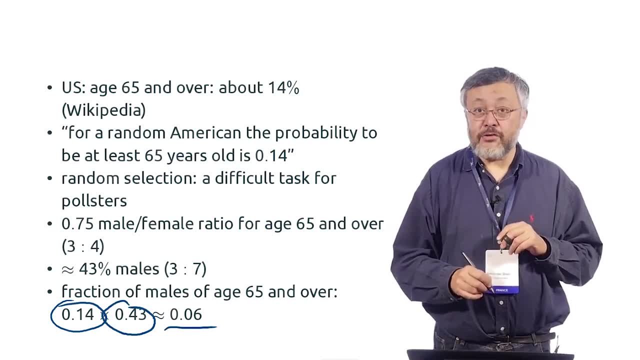 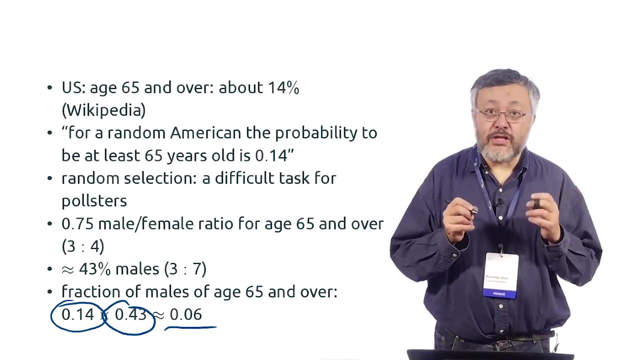 this by: first we take the 14% of old people and then the fraction of males among the old people and we get something like 6%. of course it's not exact computation, but the data are just approximate, I guess. ok, so this is all trivial. 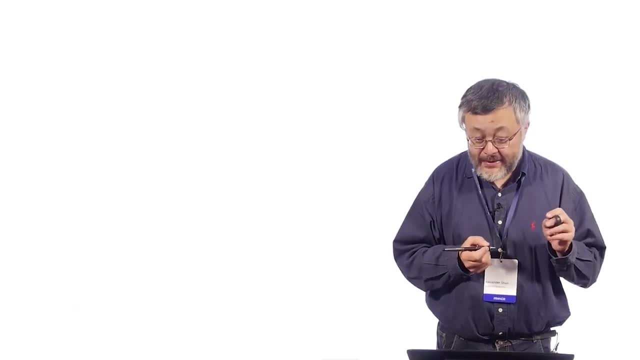 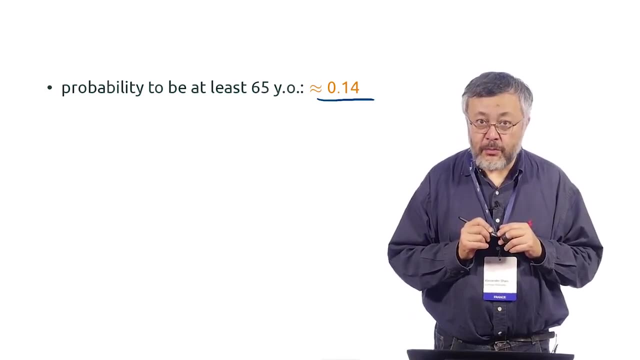 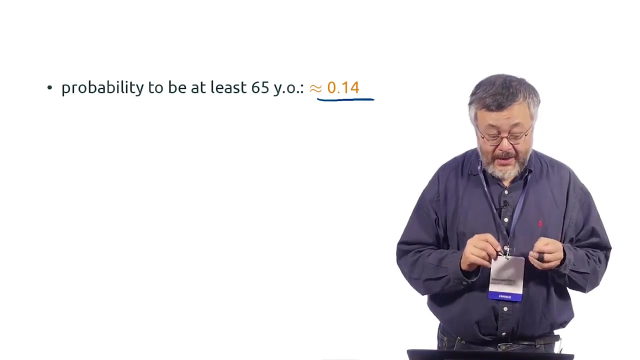 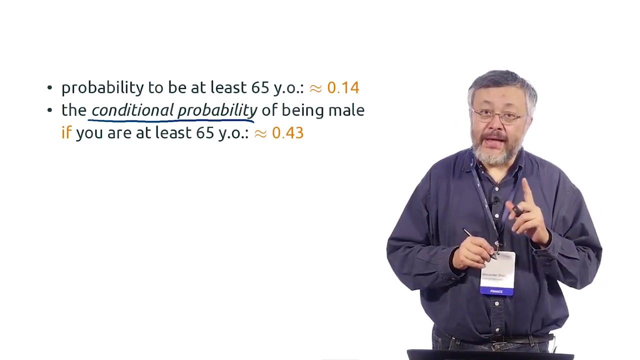 and explained in the language of probability theory. and first, first thing, we have said this: 16, 0.16, it's the probability for a random American, this mystical random American, to be at least 65 years old. and now, what is important, then, the fraction of males. 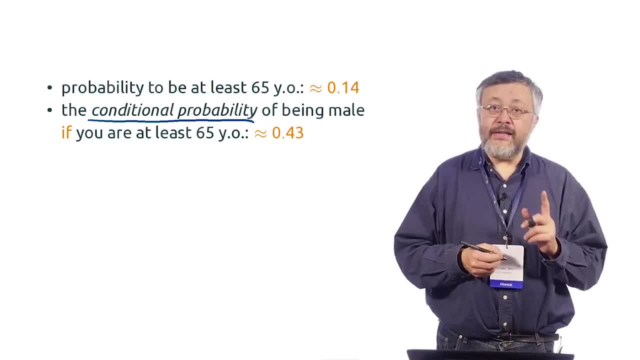 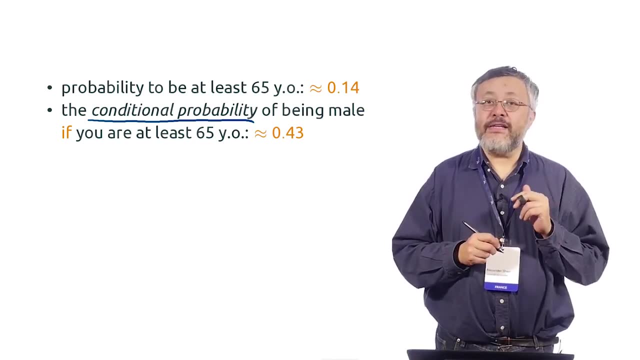 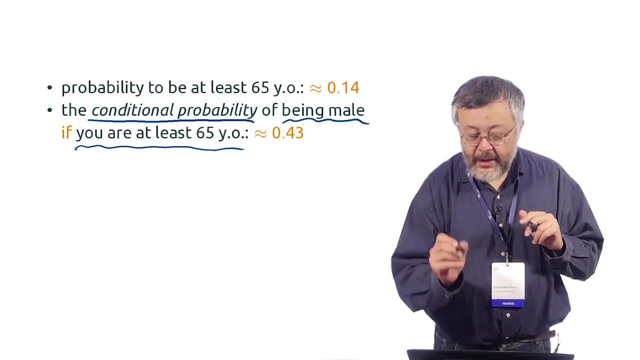 among the people who are of age 64 or more. what conditional probability? the conditional probability of being male under the condition that you are at least 65 years old. so there is a condition and there is the event event of being male and you look at the conditional probability. 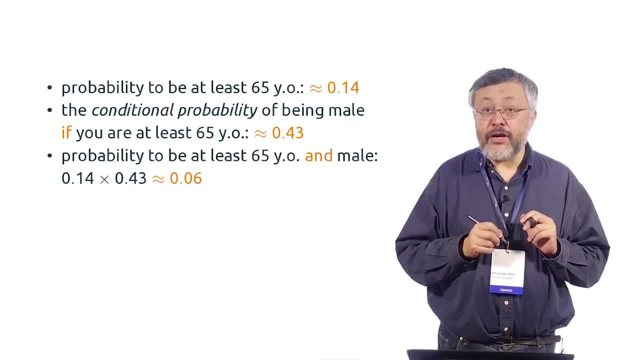 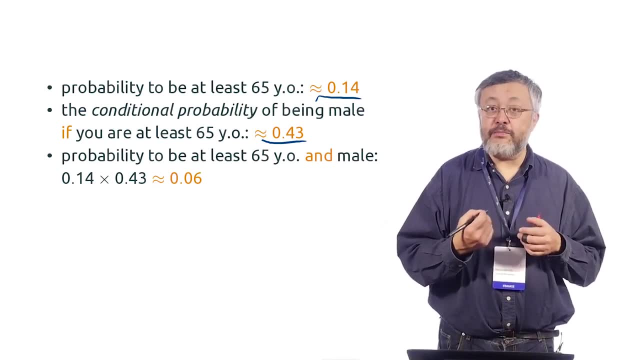 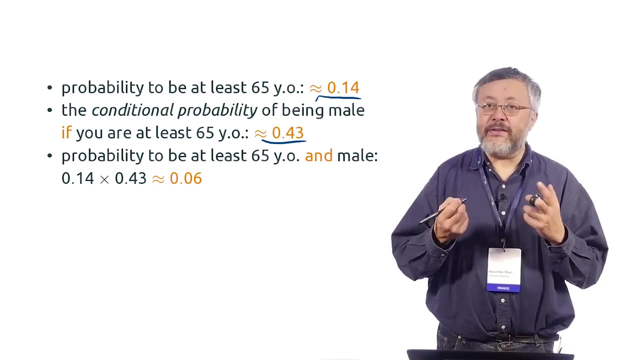 of this event. so it's a fraction inside some group and you can use if you know this fraction. and you know this fraction, you can compute the total probability of being 65 years old and male. that's not total, just probability of this combined event and this is the product of these two probabilities. 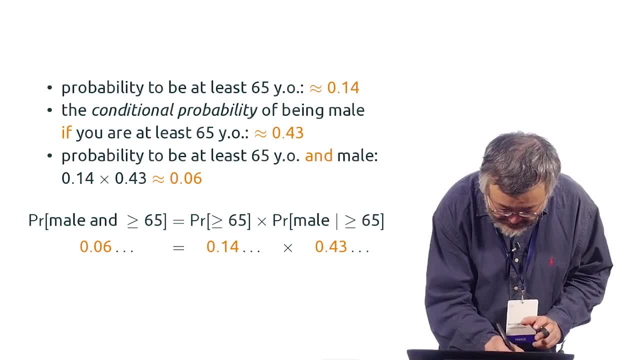 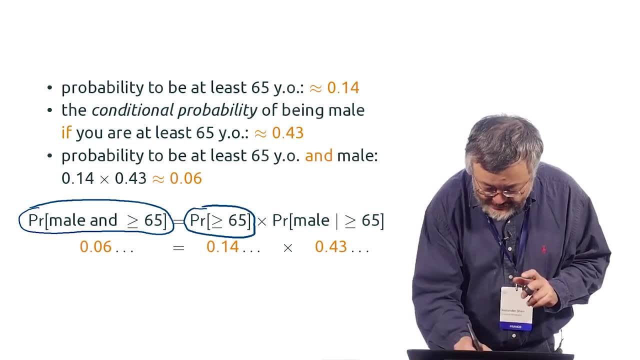 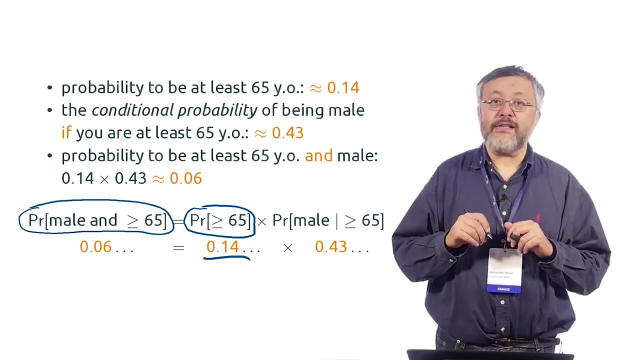 so I write it again. so probability of being male and at least 65 is a product. first, the probability to be at least 65 is 14%, and the conditional probability of being male is 45 or older. it's here and this is 43%. 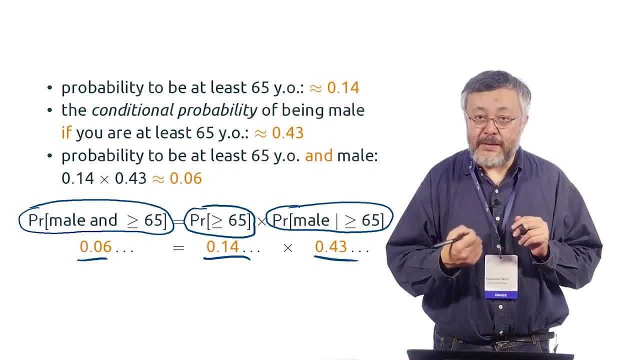 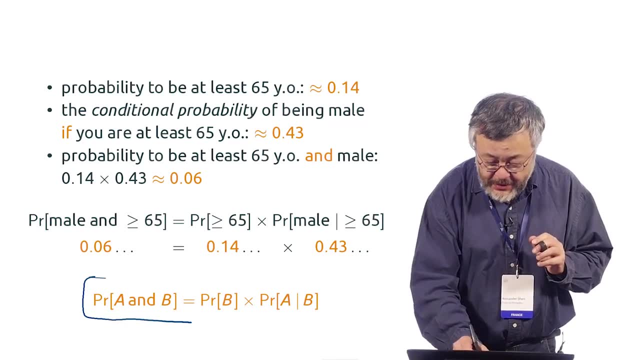 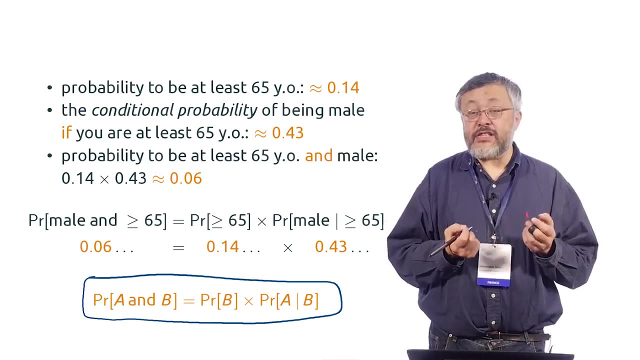 so the product is 6% approximately. so this is the same computation but repeated in probabilistic terms and general general statement: the probability of A and B is just the product of probability of B and conditional probability of A given B, and actually it's just a definition. 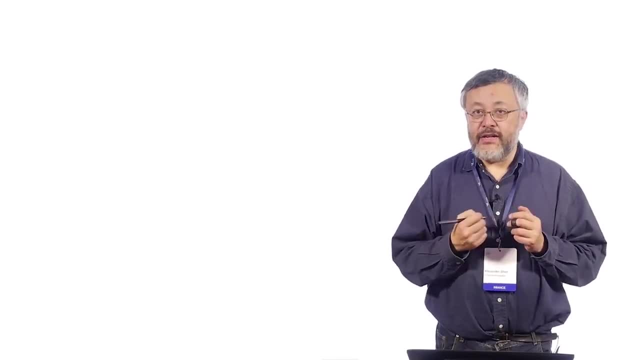 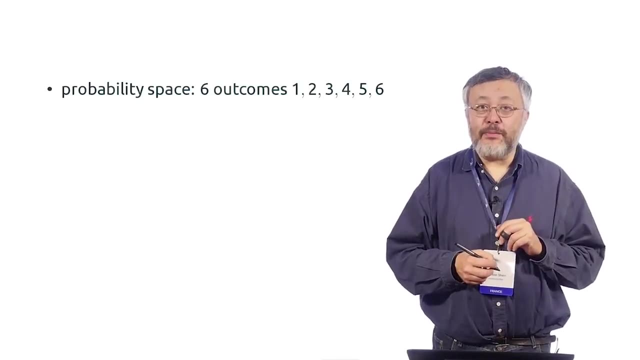 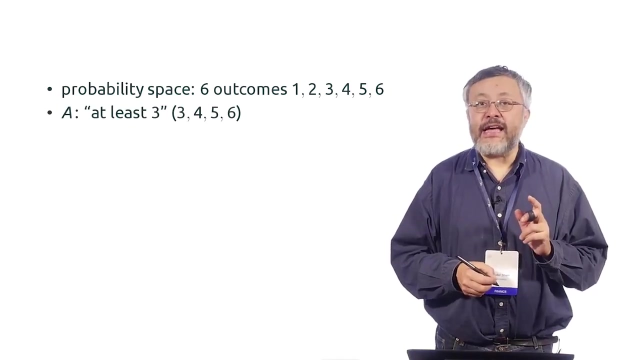 of conditional probability. so you see this definition in the next example more close to our standard probability theory. so now we have probability space with 6 equi-probable outcomes: 1,, 2,, 3,, 4,, 5,, 6, and A is at least. 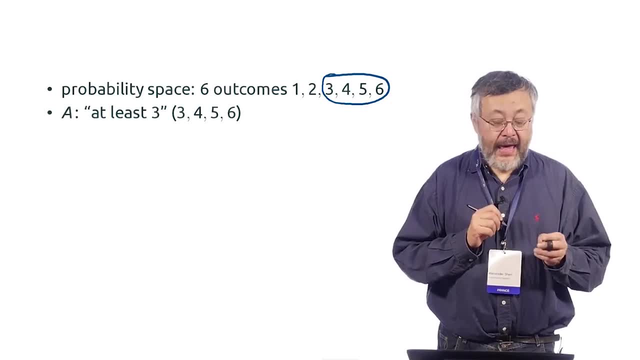 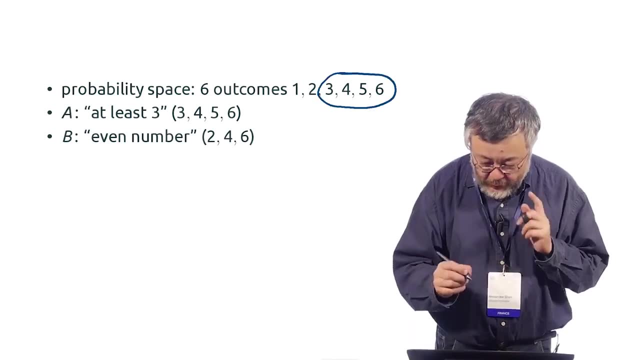 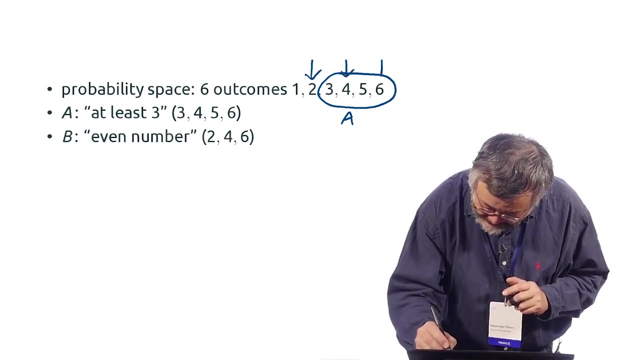 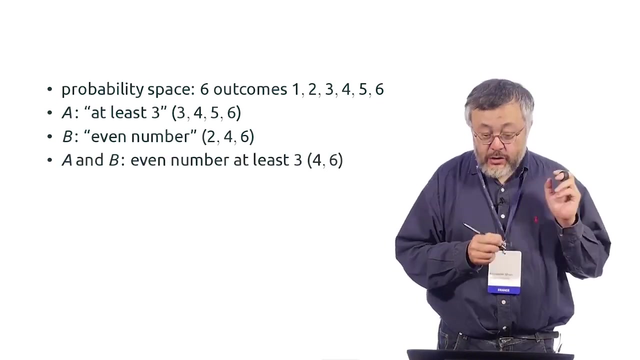 event, at least 3, so there are 4 outcomes and B is the event to be. even so, inside this event? no, not inside this event. this is A, so this is B, and now we can consider all these things conditional probabilities for this special case. so A and B. 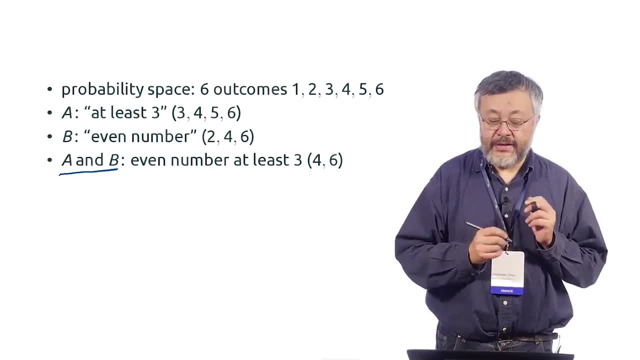 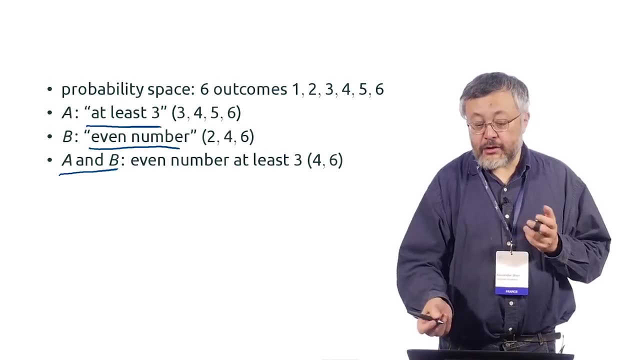 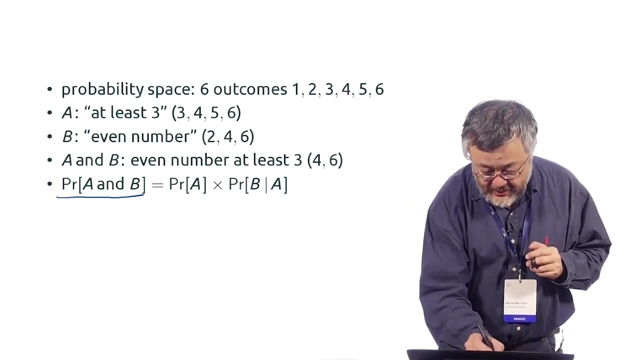 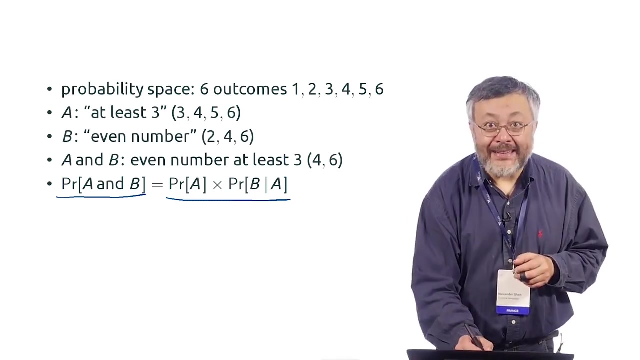 is to be first, we consider the conjunction, the end event. so A and B is just the even number, which is at least 3, and there are 2 of them. we want this product. so we can say the product of being even at least 3 is a product of being at least 3. 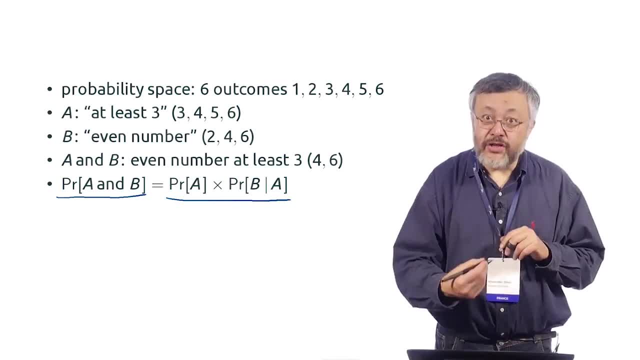 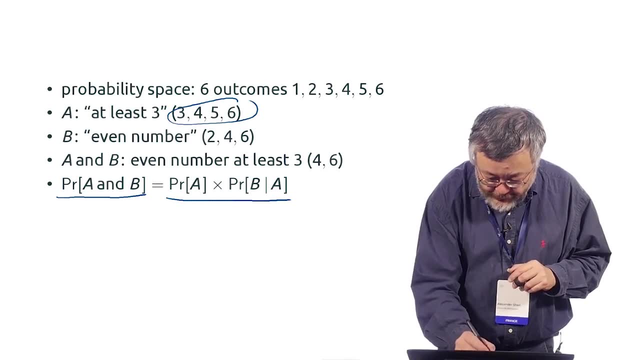 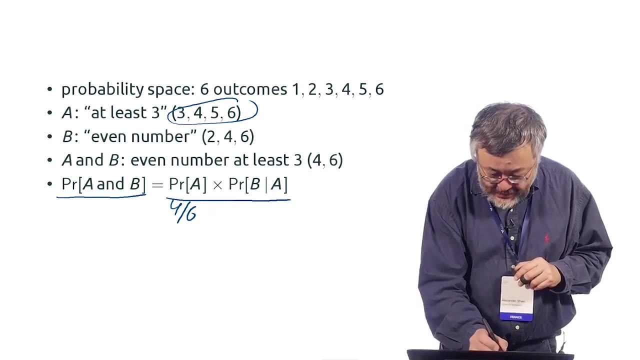 times the product of being, even under the condition that you are at least 3, so just the probability of being at least 3 is 4 out of 6, and out of this 4 there are B, A and B. there are only 2 of this. 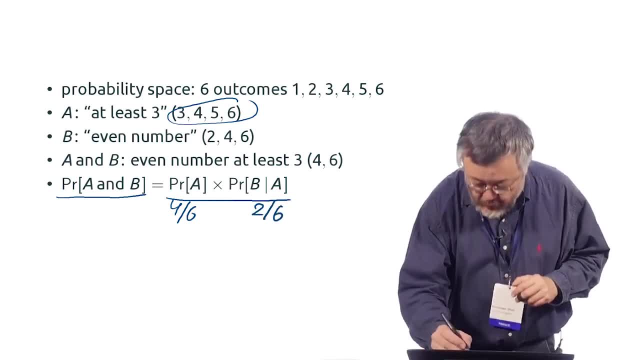 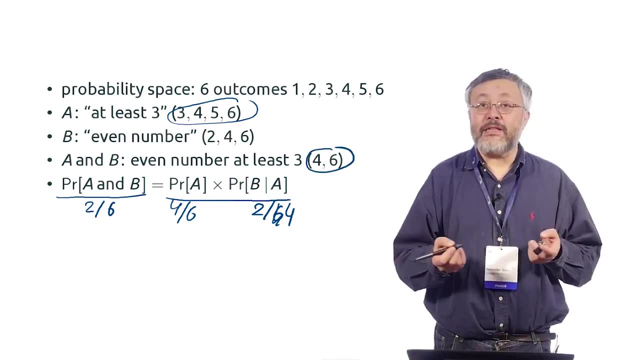 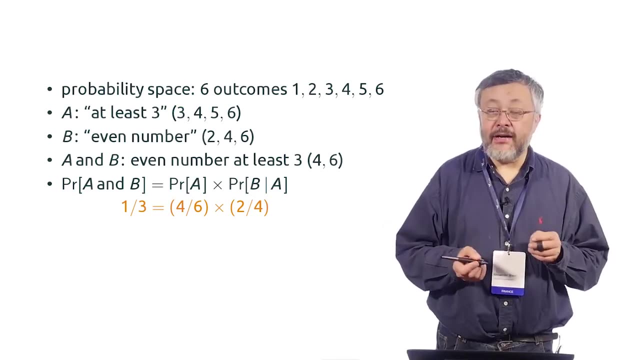 2 of this 4, so we get not 6, sorry, 2 of this 4, and the product is, of course, 2 out of 6. 2 out of 6, so it is the probability of being A and B together trivial. yeah, here is this. 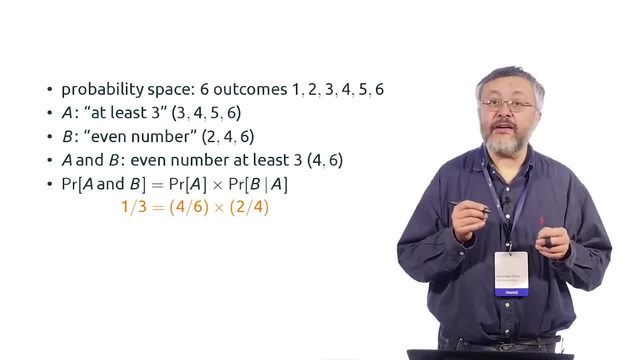 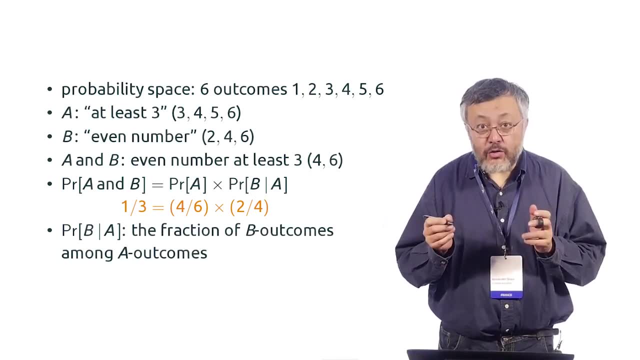 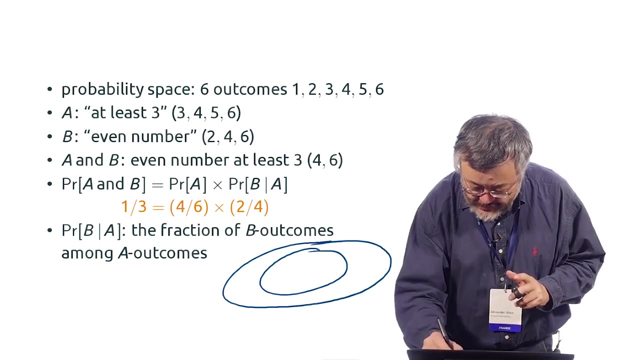 1. third is the product of this: 2 things: 4 out of 6 and 2 out of 4. as I have said again, this is the condition of B outcomes among A outcomes. so it is in the picture. you have the entire space, you have event A. 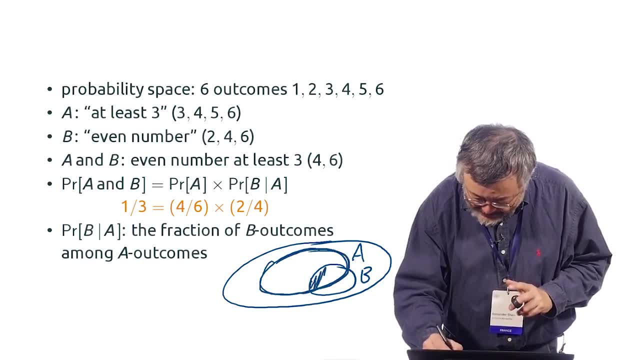 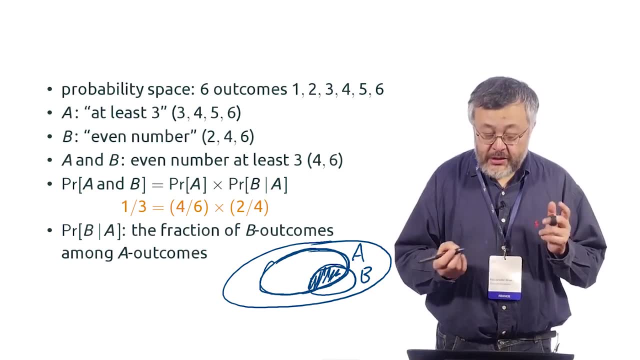 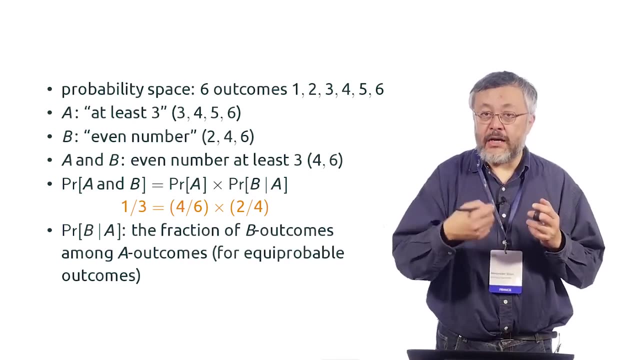 you have event B and now you look only inside A. so B forms some fraction and you look how big this part is inside A. so this is this condition of probability and this is for equal probable outcome. all the numbers and you can, in general case you can just define by this equation. 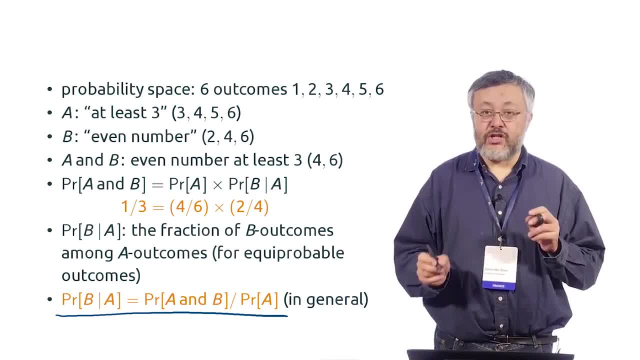 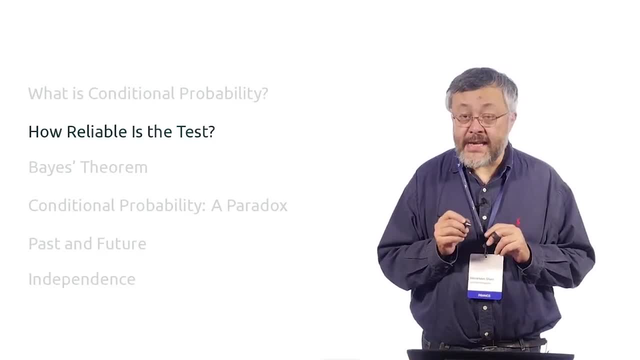 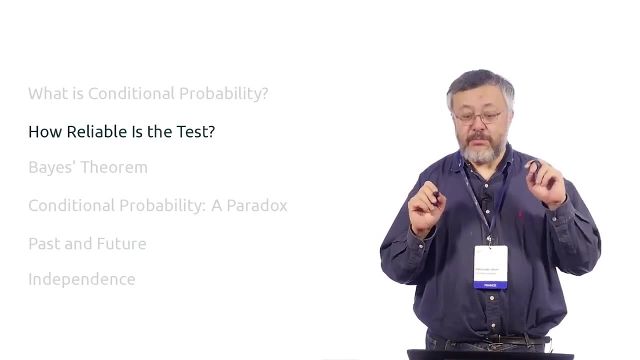 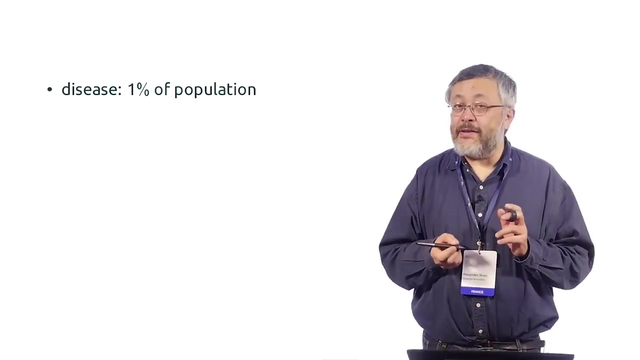 this is ratio, this is definition of conditional probability. in this part we consider a somehow counterintuitive test example which is related to conditional probability, just a test and disease example. so let me explain what I mean. so imagine there are some disease which is not rare but rather rare. 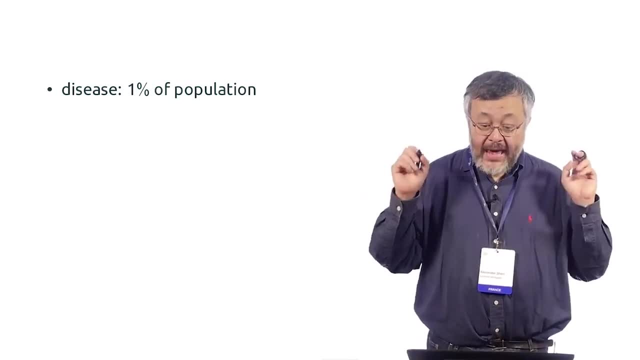 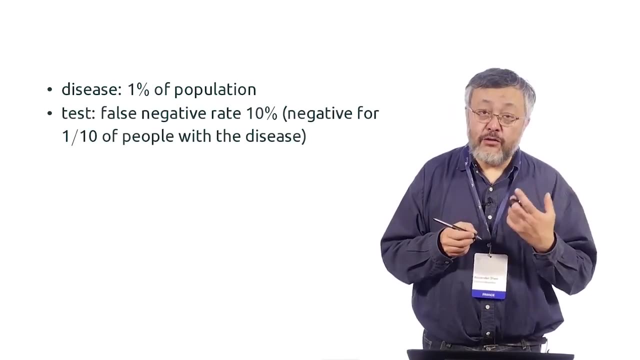 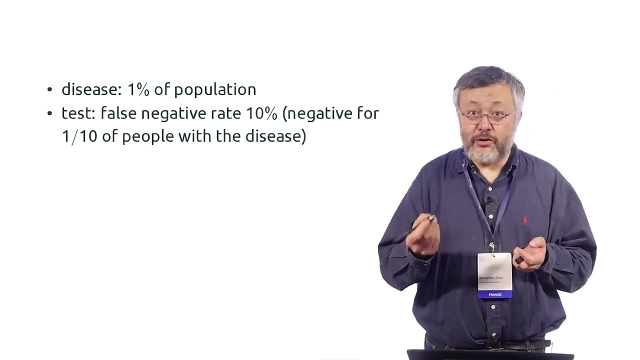 1% of all people in some population have this disease and you have a test for this disease and every test can give false positive and false negative. so false negative: the test is negative while you are ill. and false positive: the test is positive if you are not ill. 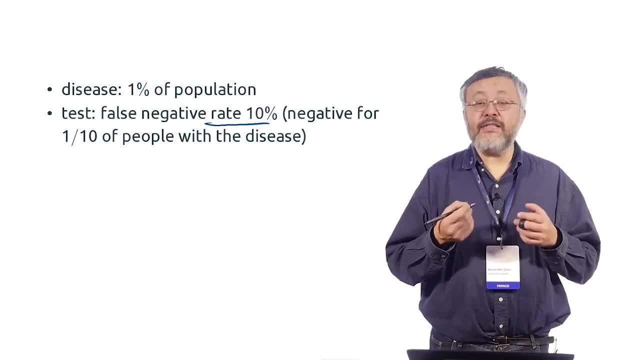 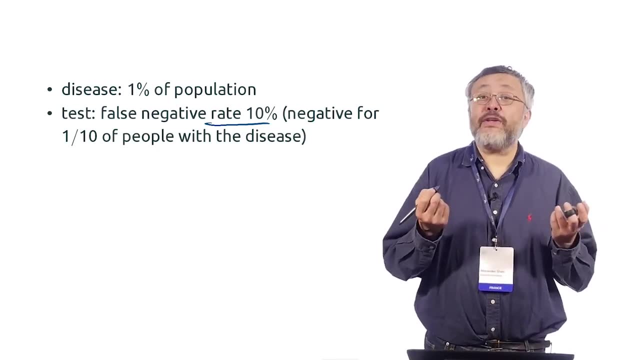 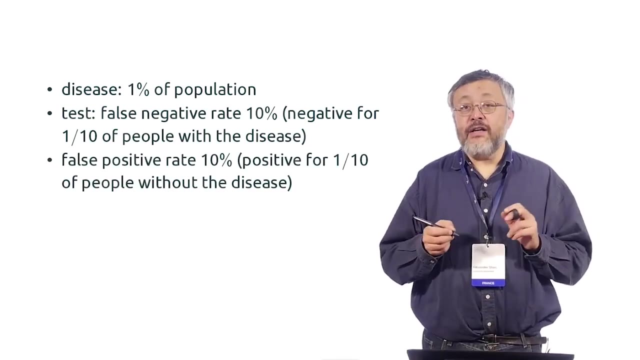 so the rate means that 1 tenth of all people who have the disease get negative test. no, it's not so. it's somehow 90% reliable. and also for false positive rate is equally small. if you are positive, then 90% if you are not ill. 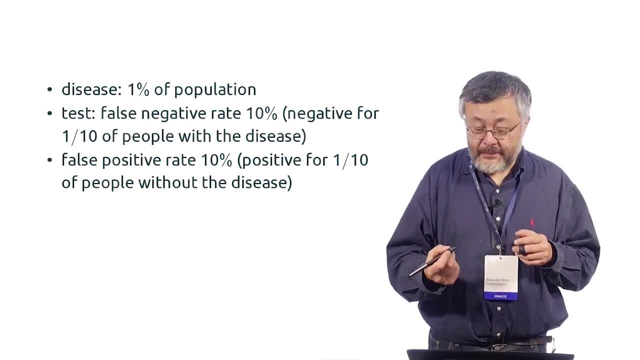 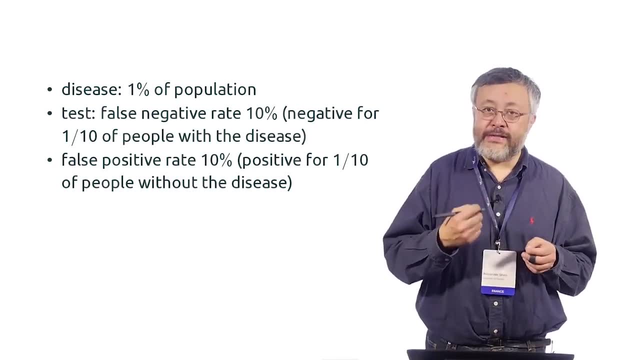 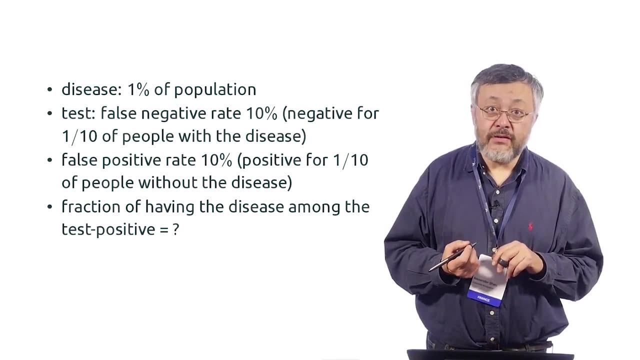 then probability to get a false positive test is 1 tenth. so again, 90% people have correct, correct, are classified correctly. and imagine that now you are informed that your test is positive and the question is, how much should you be worried? of course you should be. 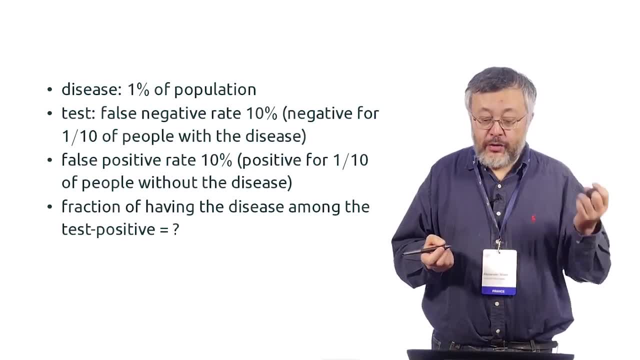 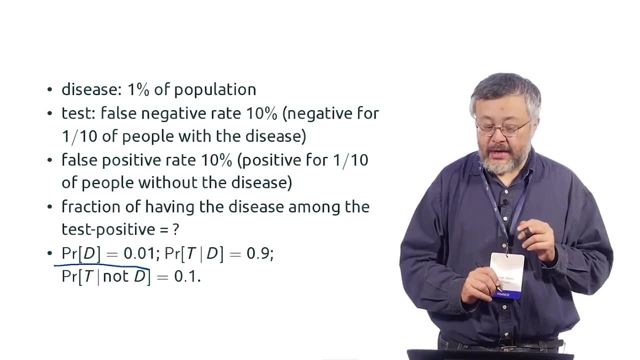 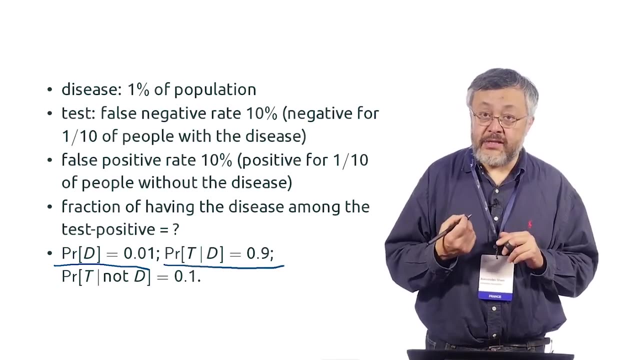 but what is the probability that you are really ill? so in terms of our probability theory we can say like this: so the probability of the disease is 1 over 100 and the conditional probability of test if you really have the disease is 90%. so this is. 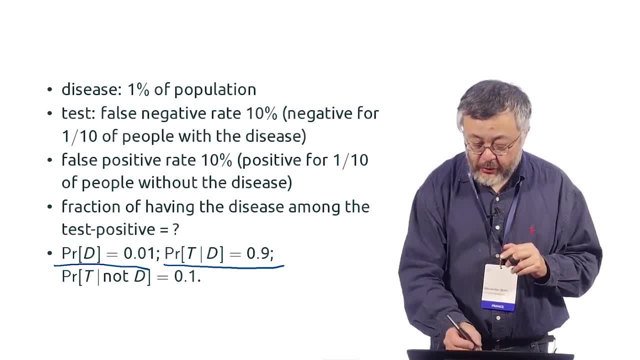 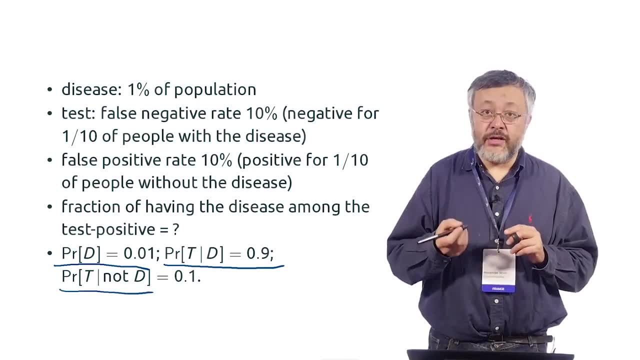 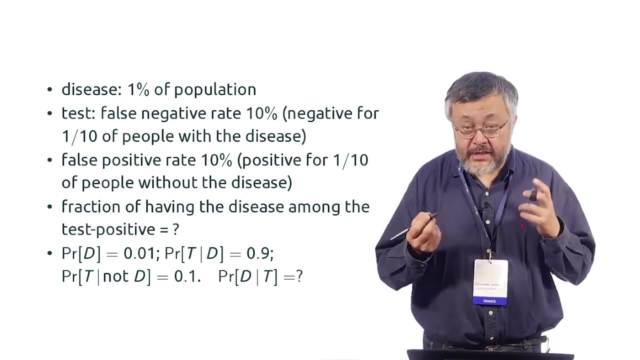 false negative. so to say false negative if the test doesn't show you. so this is the compliment, and here is false positive. you are not ill, but you get a positive test and this happens probability 1 tenth. ok, and this is what is given. and the question is: 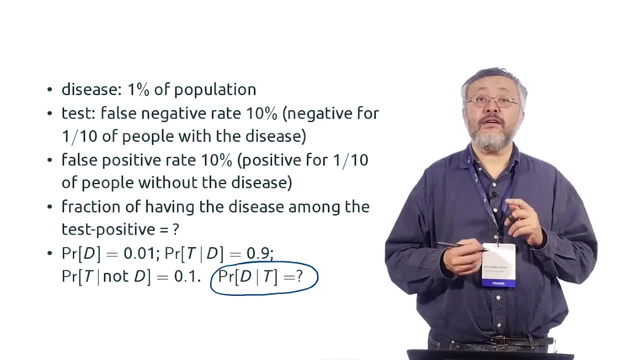 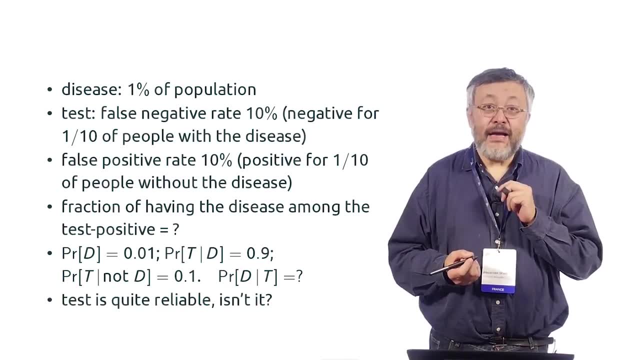 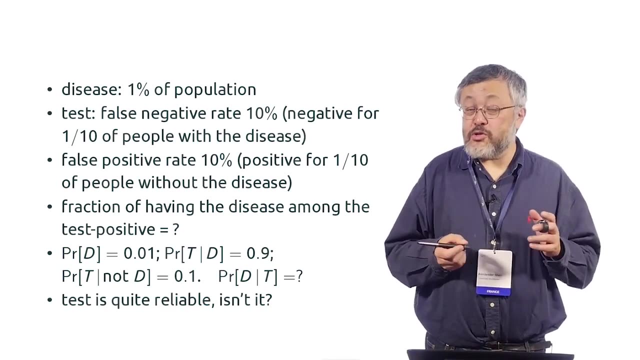 what is the conditional probability of having a disease? is it? what do you think? is it high or not? I think that many people will say that look, test is quite reliable. 90% is almost in most of the cases it's correct. so most probably I have the disease. 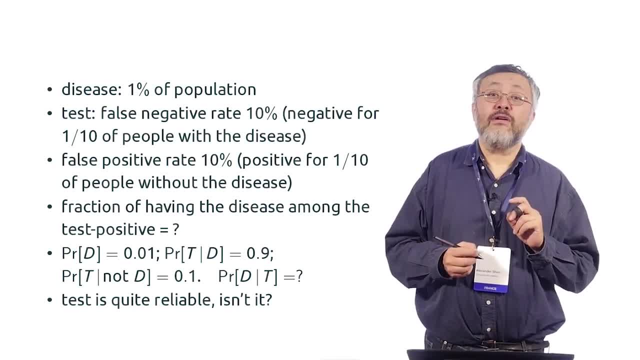 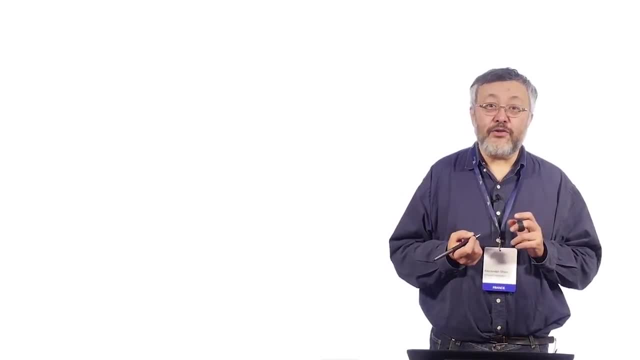 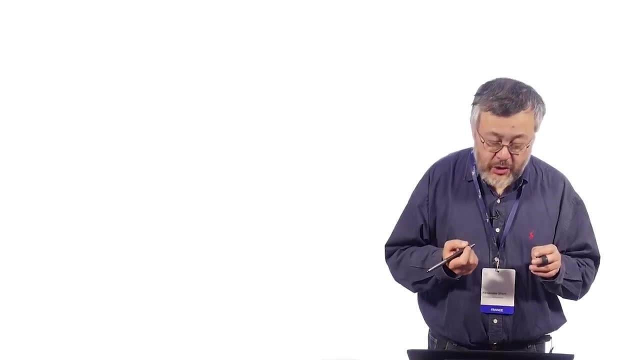 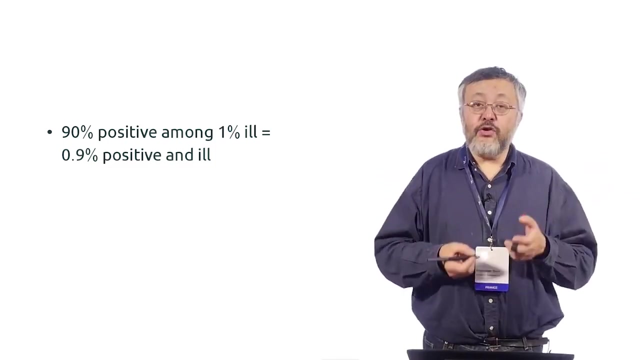 many people will think so, but it's a wrong, wrong understanding. so you should, before going into panic, you should think a bit and compute a bit, and then you understand the situation better. so let me tell you what I mean. so just, we compute things slowly, so there is 1%. 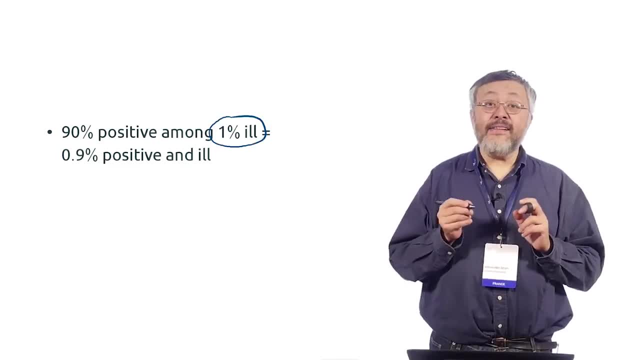 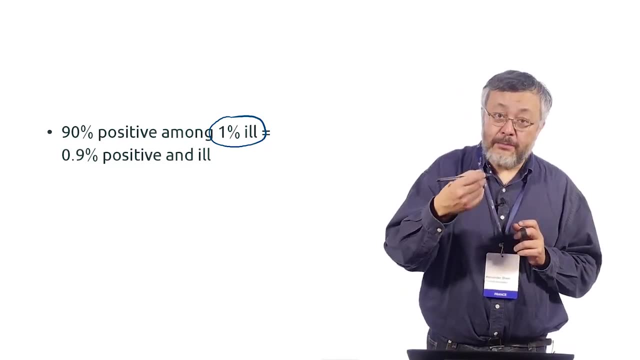 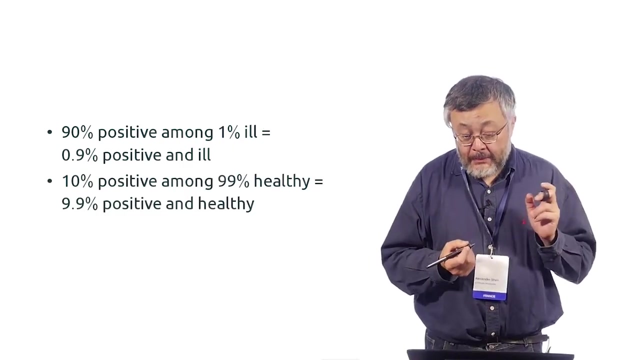 of ill people here, and 90% of this ill people are positive. so it's 90% of 1%. so it's just 0.9% positive and negative and ill. but also there is 99% of healthy people and some of them are also positive. 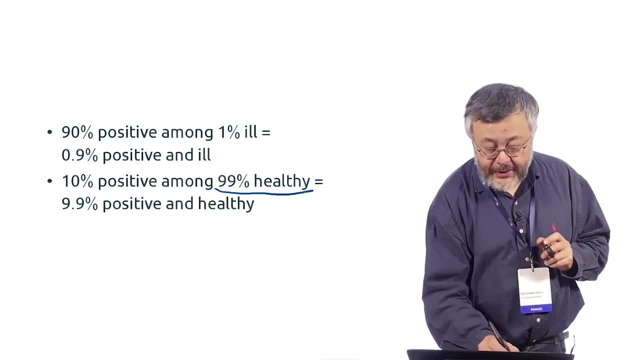 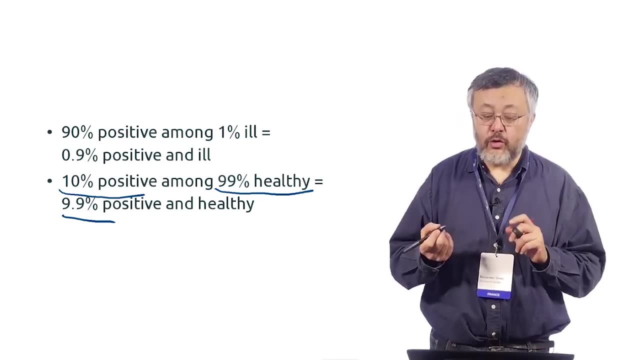 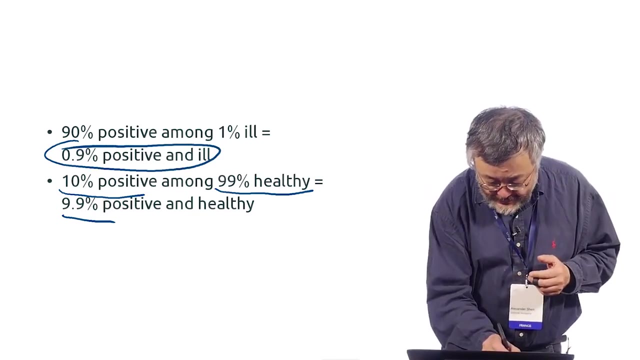 just 1 tenth of them are test positive. so there are 10% of this, and so we have 9.9% in the population of people who are positive but healthy. and now you see, positive and ill is much smaller than positive and healthy. it's just in proportion. 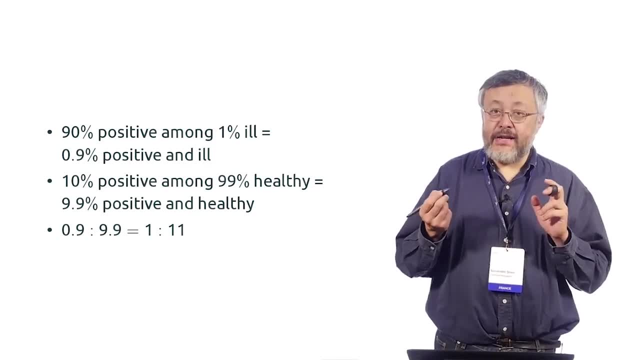 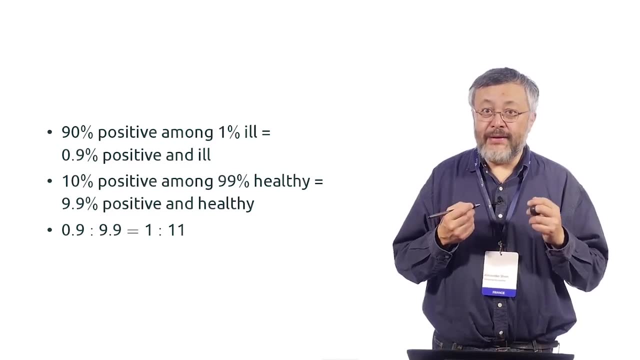 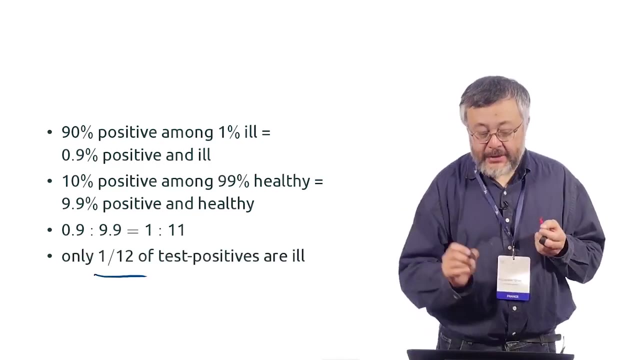 1 to 11. so if you look at all positive people and find 1 of every 12 positive people, 1 is really ill and 11 is healthy. so it's not so bad. only the probability to be ill- assuming you are test positive- is 1 over 12. 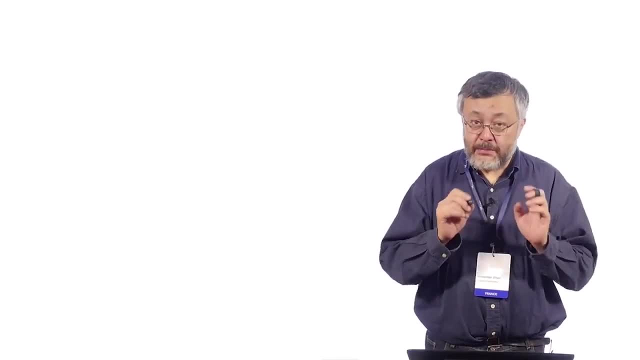 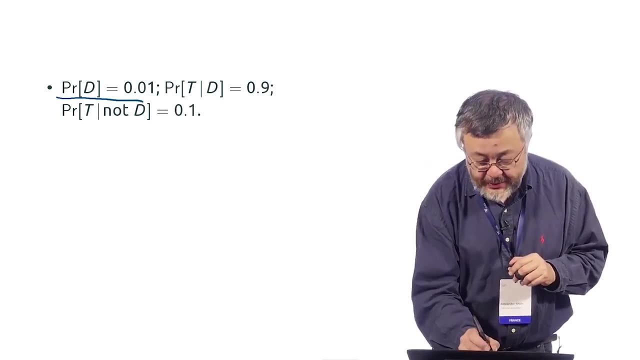 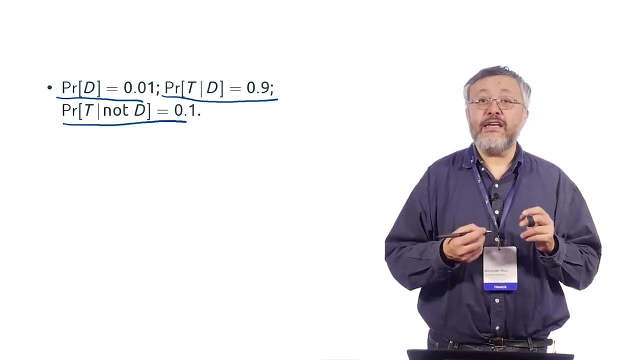 and the same computation can be done in terms of probability theory, slowly again. so here is what we start with: the probability of the disease, the conditional probability of positive test if the disease happens, and the probability of test if the disease doesn't happen. and this is what is given. 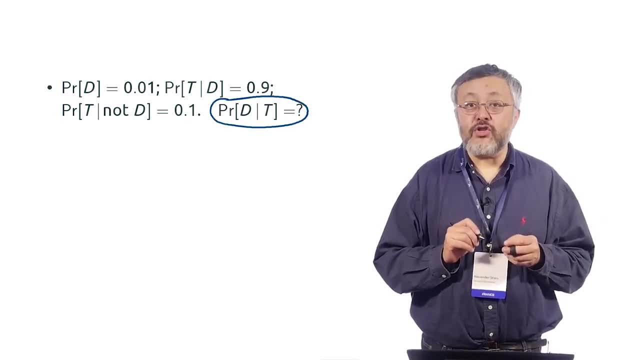 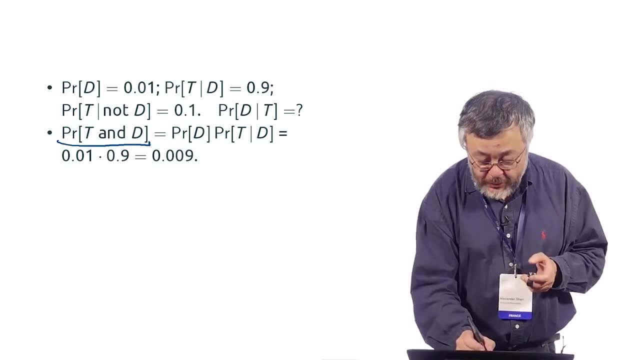 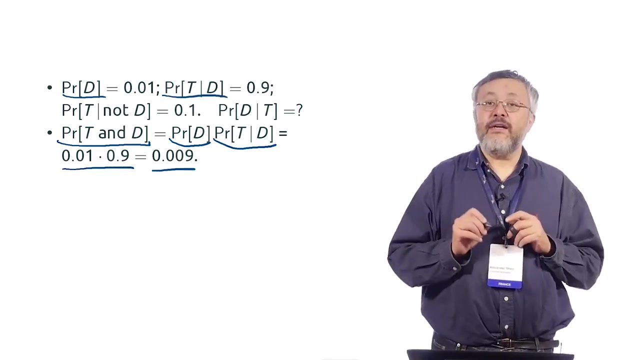 so that's what we want to compute, and now we make the computation. so first we start probability test and disease, and the formula is the probability of disease by the conditional probability, and so we get this, and this is 9 out of 1000. and if you 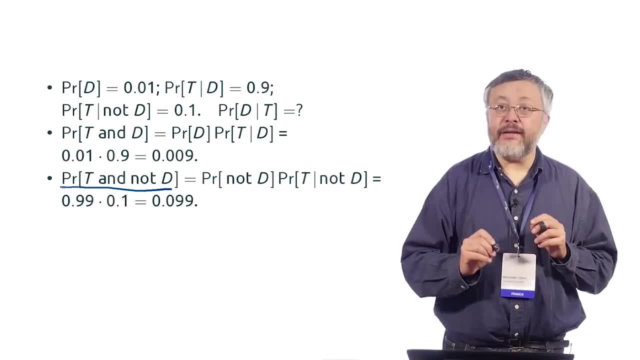 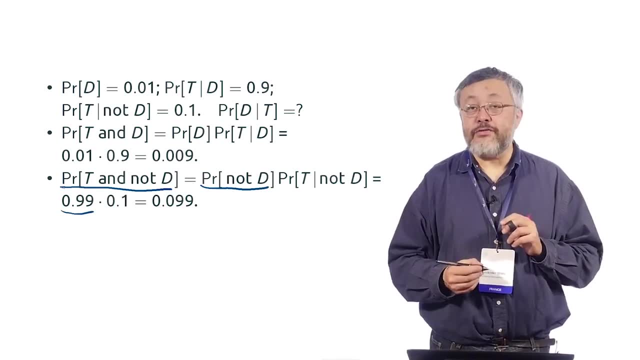 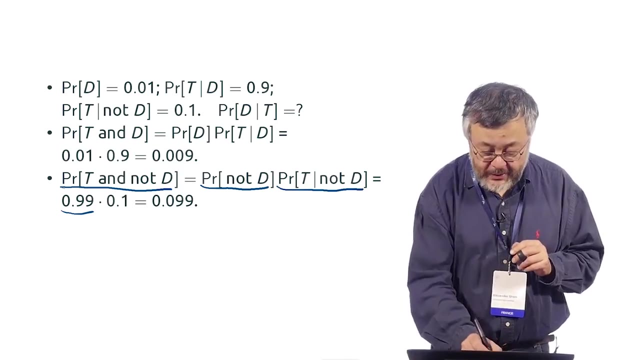 compare this with test and not disease. test and healthy. we also do the same. we have 99% of people who have no disease, not this disease, and among them there is 1 tenth who are test positive. so we get this number and then we can. 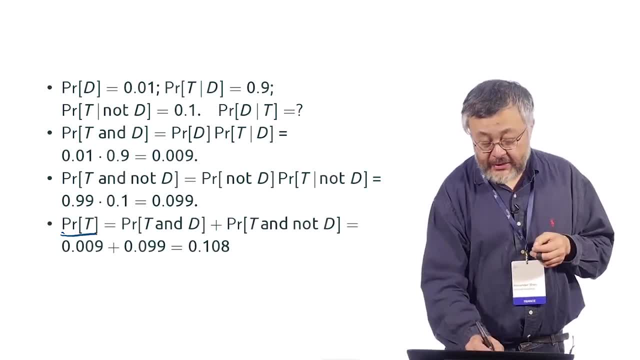 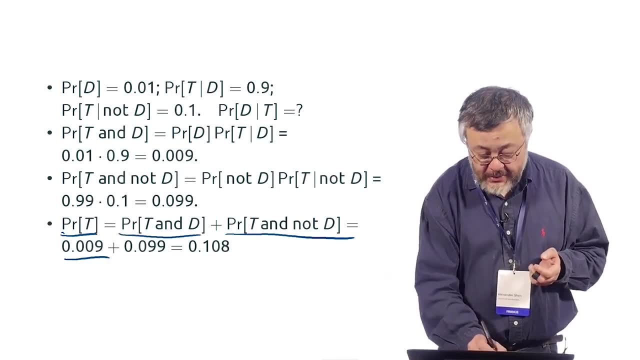 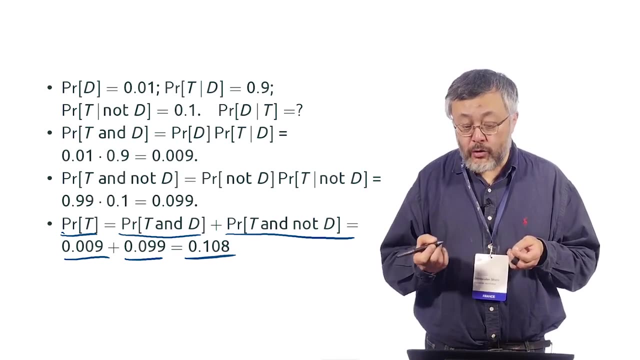 just compute the probability of being positive. it's just two cases, two disjoint cases, so the sum of probabilities works and we can just add these two numbers and get the sum. and now we can just compute the conditional probability according to the definition, so the probability that you have disease. 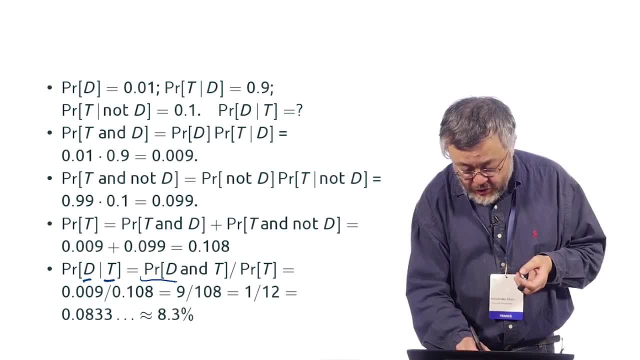 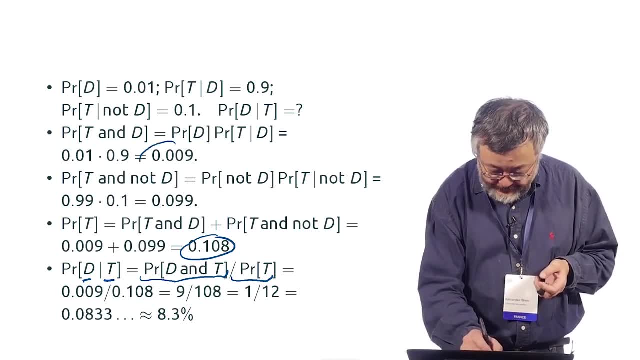 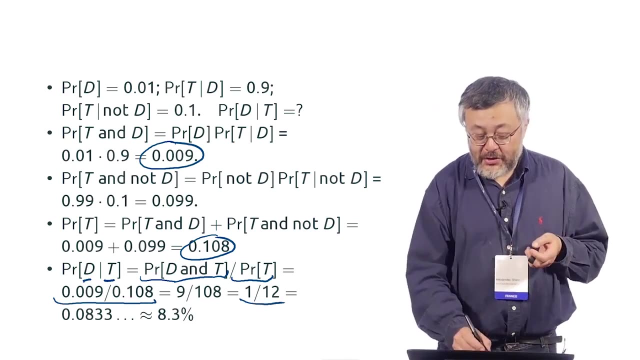 under the condition you are test positive is, by definition, the ratio of these two probabilities, and you know both of them. this is this one and this is this one. so you divide this and you get 1 over 12, as before, of course. as before, we do the same. 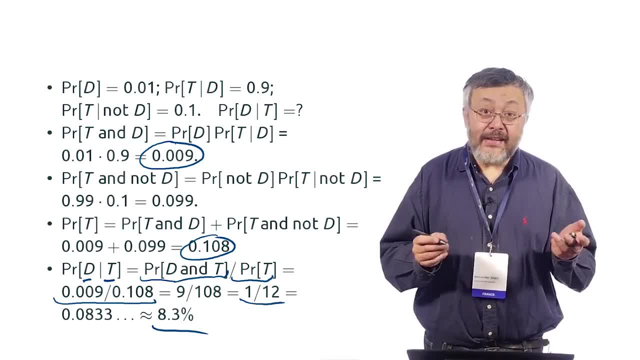 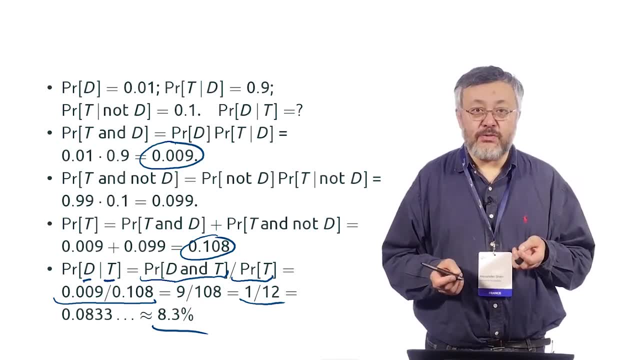 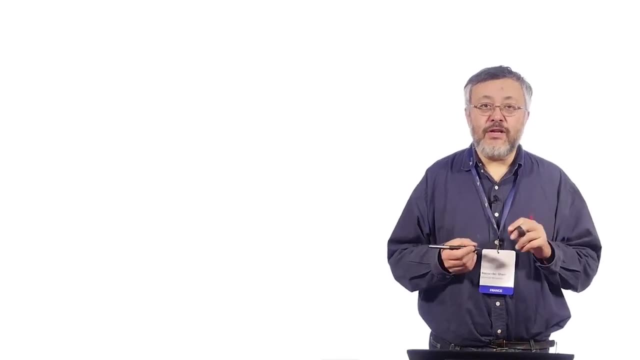 so it's like 8.3% and it's not so big. so this is counter intuitive, but now probably it's not so strange as before. let me say we used. we used something which has a serious name, the law of total probability, but actually it's a trivial thing. 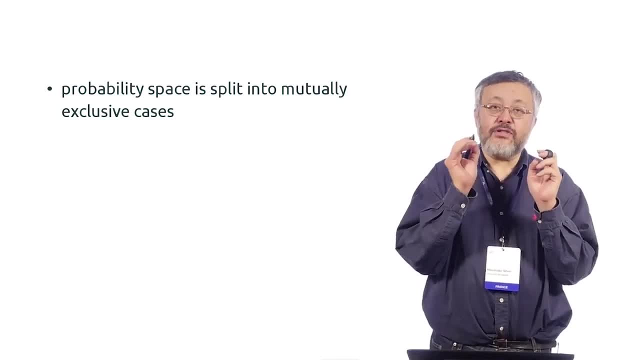 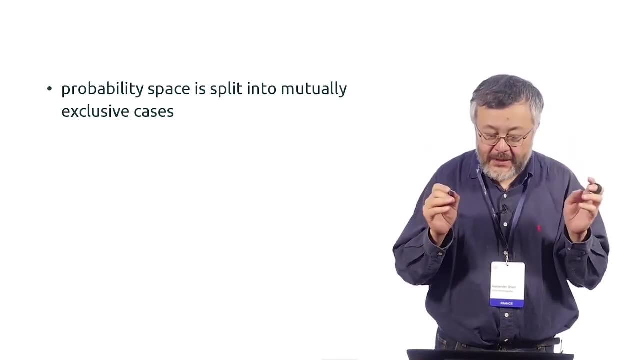 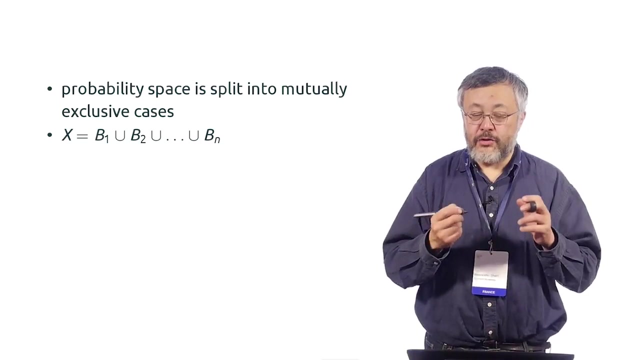 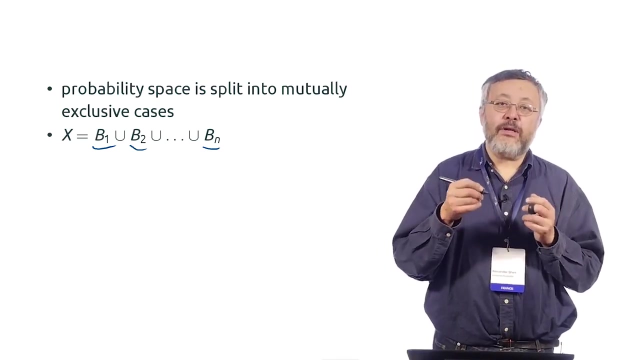 and imagine the probability space is split into some subsets, disjoint subsets, which form the entire space, so they are mutually exclusive. and exhaustive list of cases: b1, b2 and so on: bn, so there are n events. they are mutually exclusive. one and all, in every outcome, belongs to one. 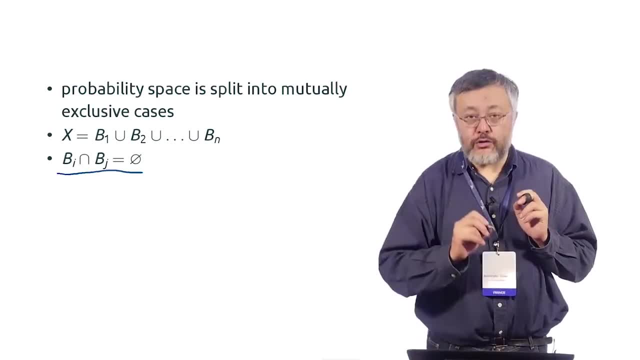 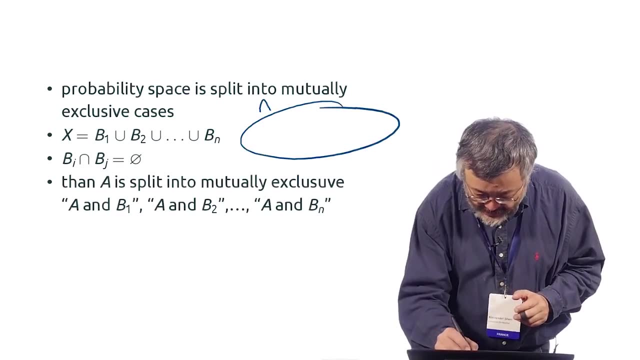 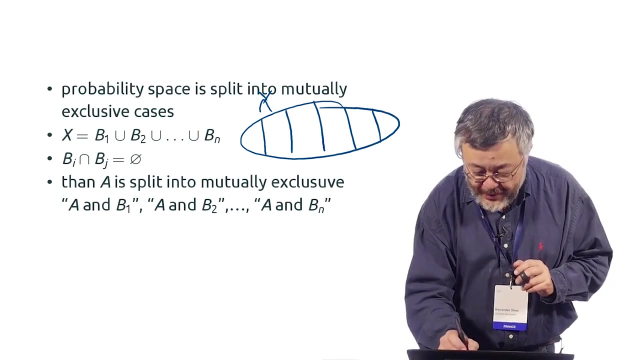 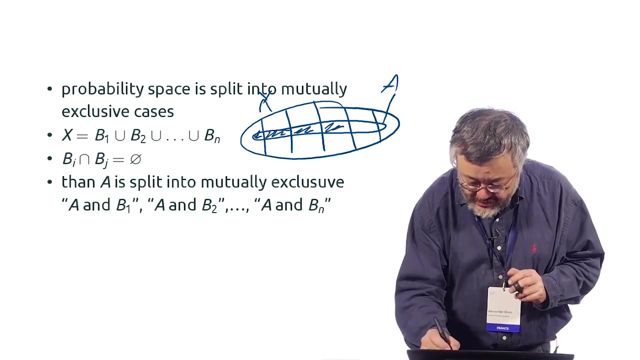 and only one of them. there is a language of set theory, mutually exclusive events, and then, if we let me draw something so a, the entire space is split into this events and then we have a, some subset, and it also is split into events, smaller events here a and b1. 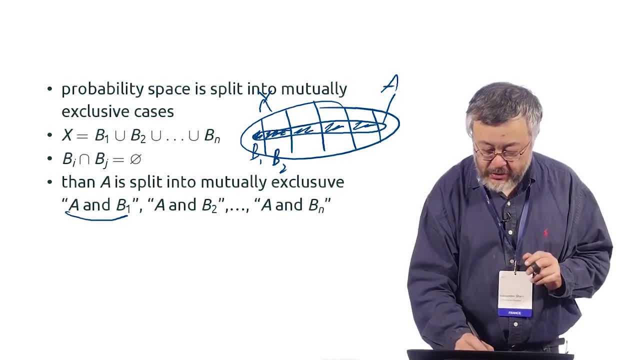 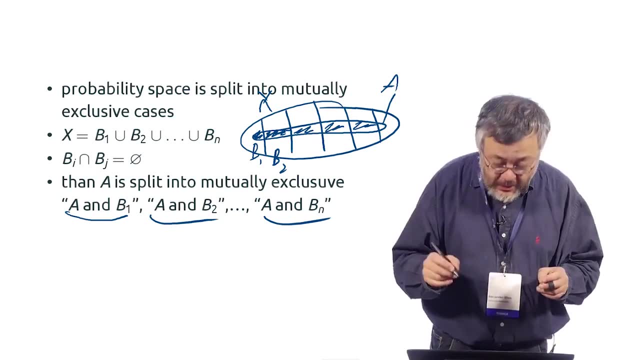 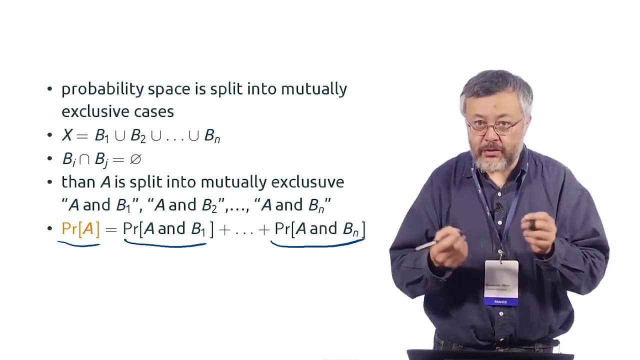 so this is b1, this is a and b1, b2, a and b2 and so on. so our a is split into mutually exclusive events. so we can compute the probability of a as a sum. probability of a is the sum of the probability of this individual events. 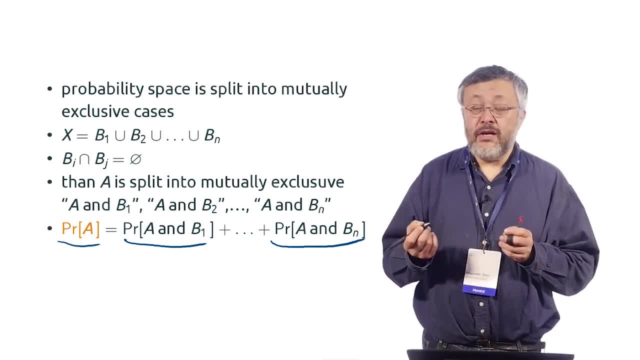 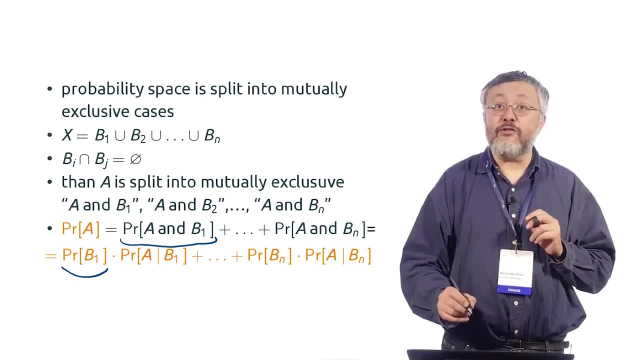 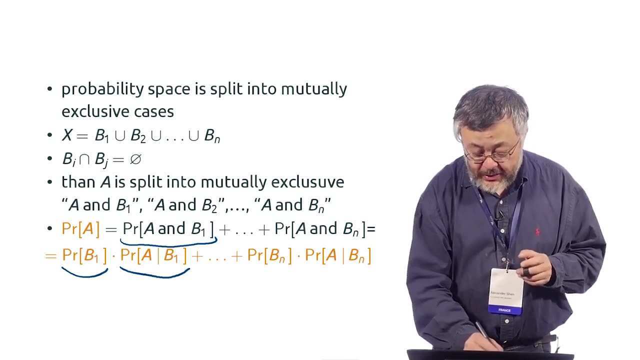 a and b1, a and b2 and so on, and each of them can be computed according to the definition of conditional probability, like this: the probability of b1 and the probability of a under the condition b1, and so on. we just get this formula, and this formula is called. 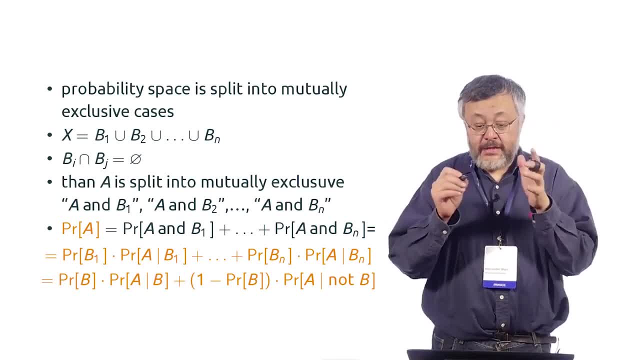 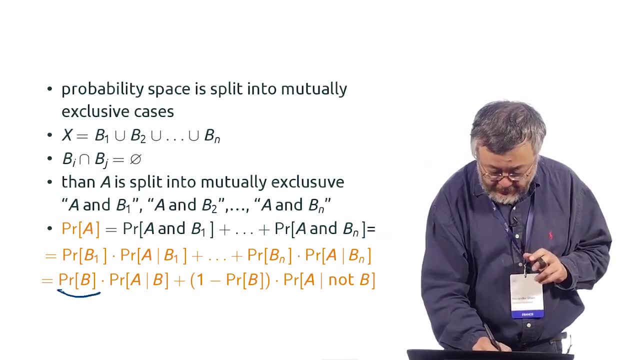 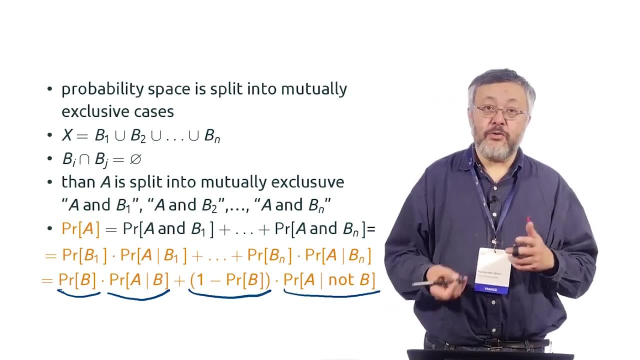 the law of total probability and for the case when we have two, this b1 and b2, only two events, we have somehow b and not b. here is what is the same: it's probability of b times the conditional probability. this is probability of not b and this is the conditional probability. 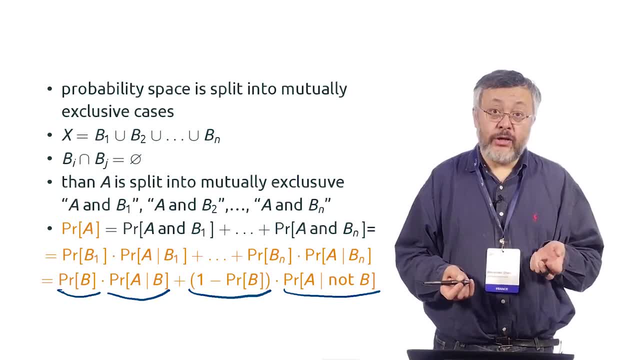 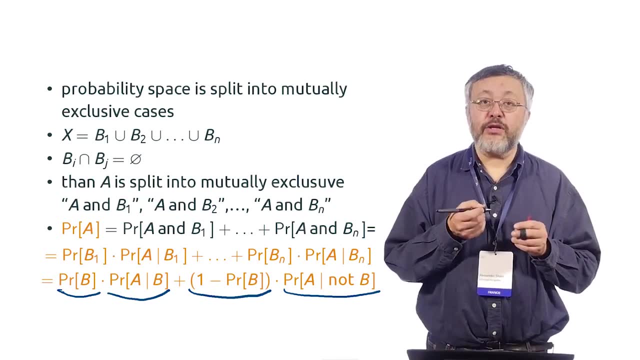 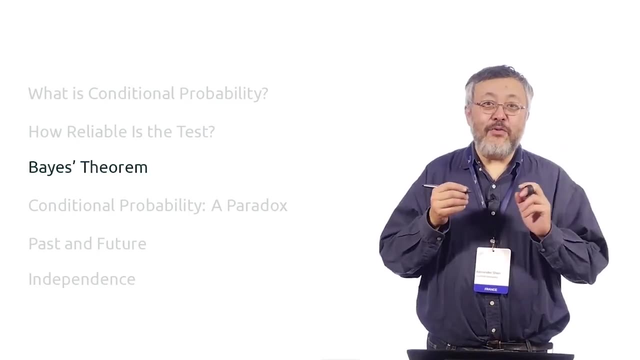 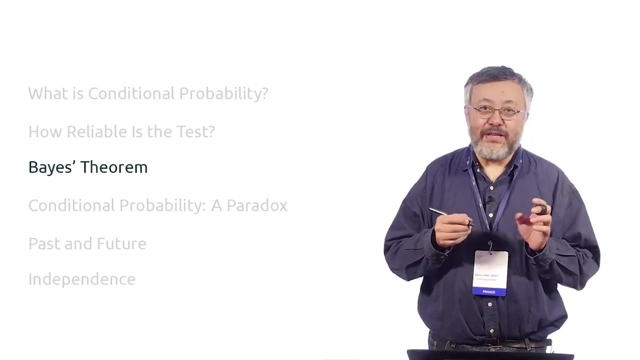 we have just a special case. that's what we did actually in our computation, so we apply this law of total probability in the case when we have only two. now we start considering some very famous thing which is called bias theorem. actually, like other things we discussed now, it's something trivial. 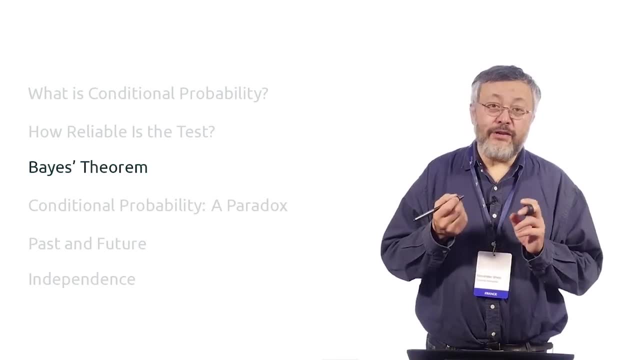 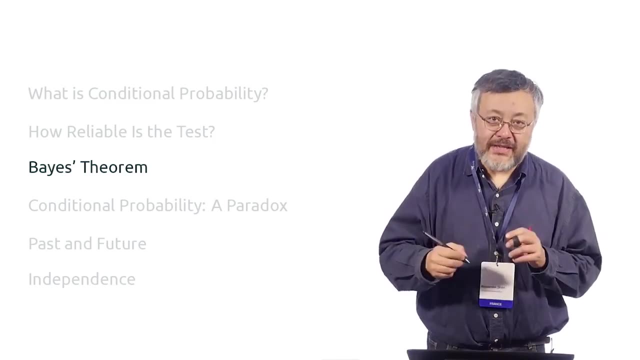 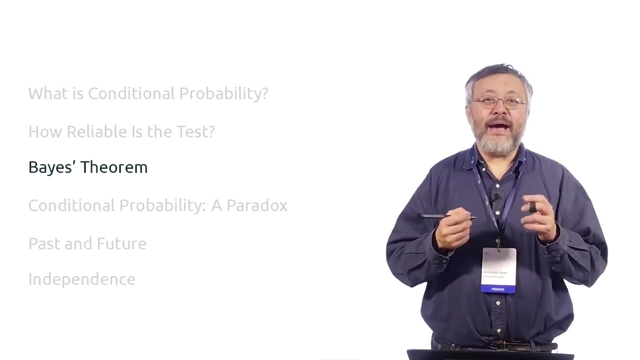 but it's very popular and very important. it's how somehow say something about the reasoning. what kind of probabilistic reasoning is good? so there is a special name, bias and statistic or bias and argument or whatever. but the formula is very simple. let's go to it. 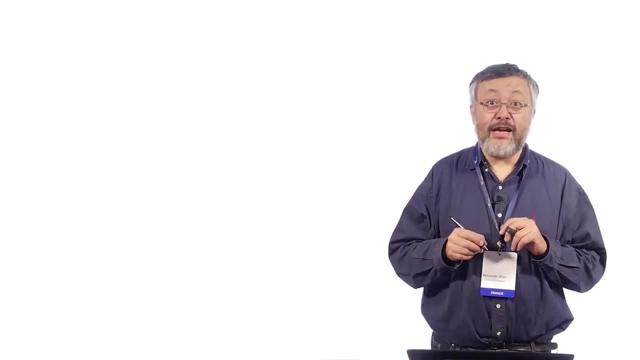 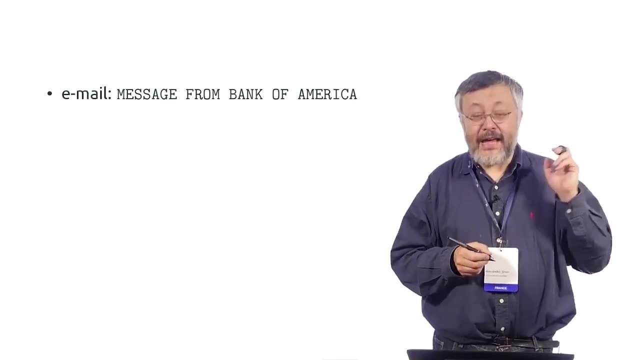 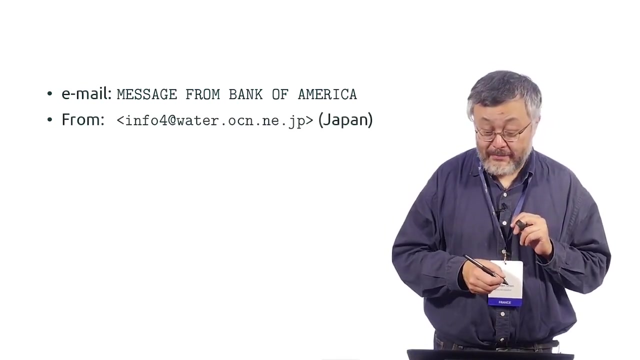 but still, I want to start with a real life example. actually, several weeks ago, when I prepared the slide, I looked in my mail that I have a message from Bank of America, but strangely this message has an address in Japan. you see, this is Japan, and I thought 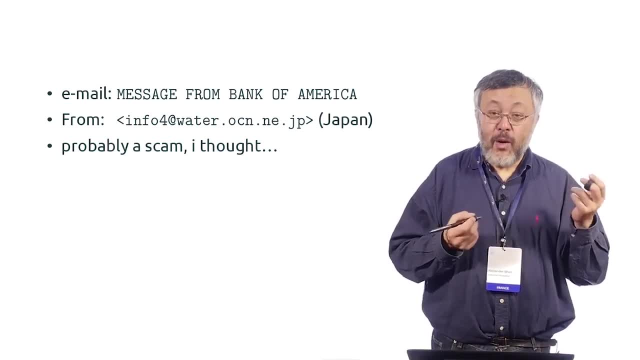 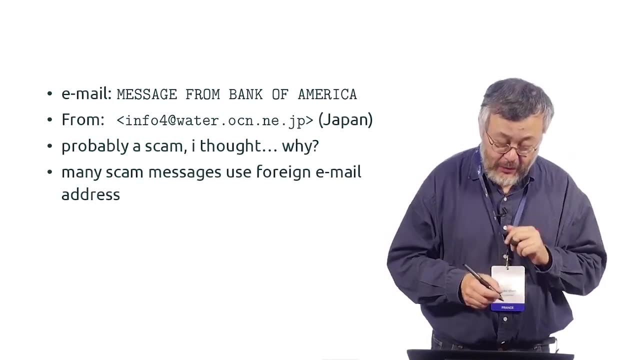 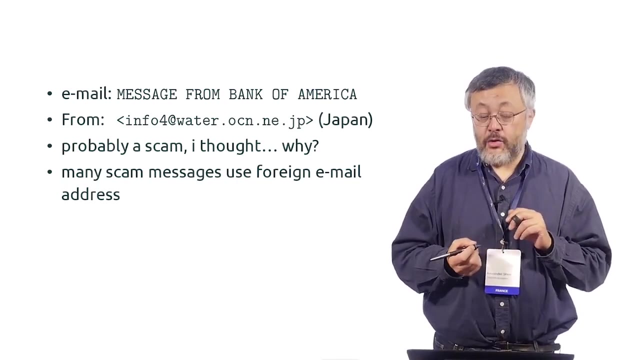 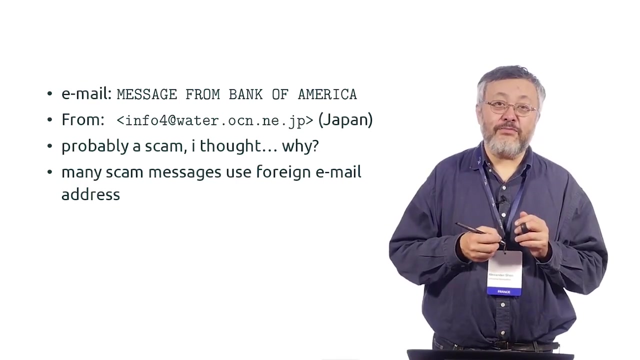 that it's probably a scam, and why? what are the reasons for that? and the reasons are following. first, I know by experience that many scam messages have foreign address because people don't want to be caught, so it's convenient for them to use their address in a foreign country. 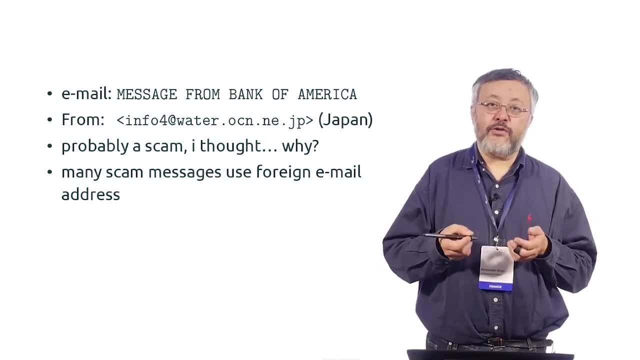 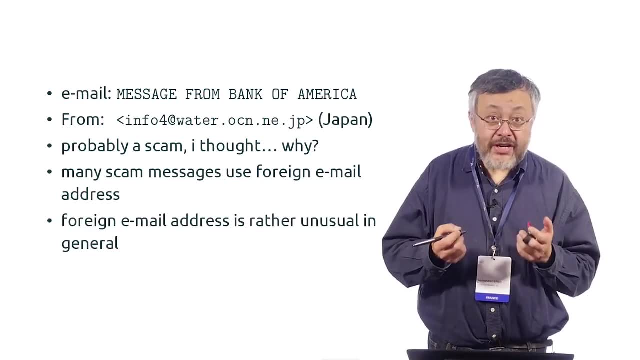 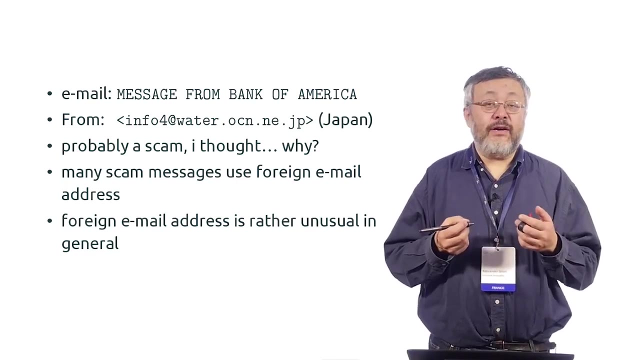 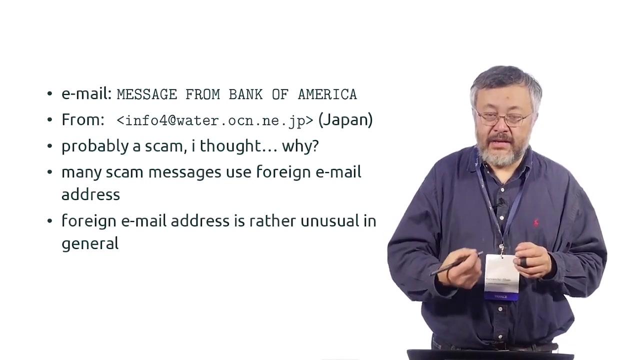 so it makes the search for who really uses the address more difficult. anyway, it's just observation. another observation, just in general. if we look at all messages, this foreign address are not so common things. it's not often there is a clear contradiction between the place when the message comes. 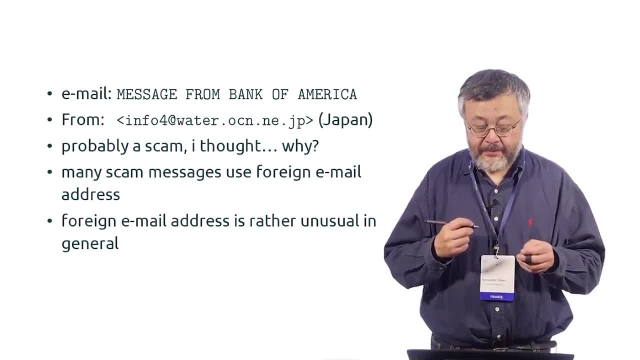 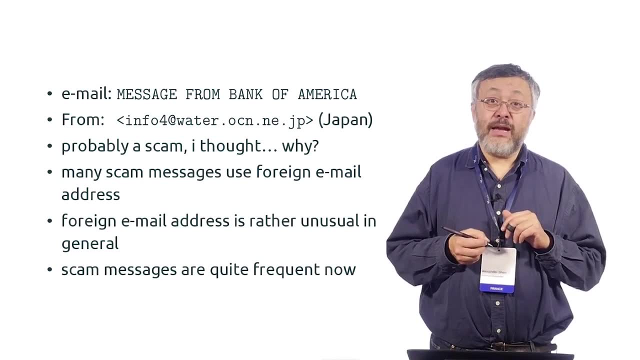 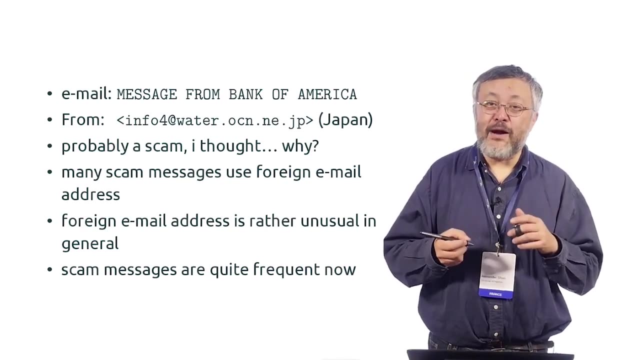 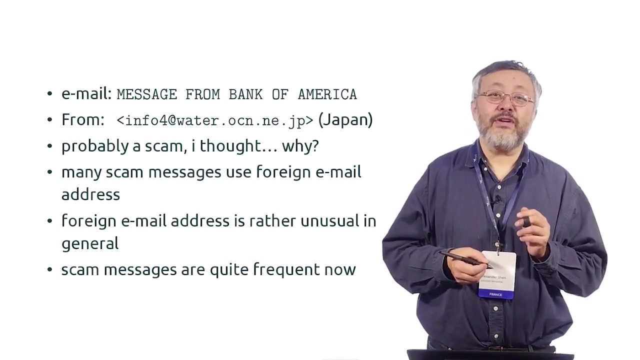 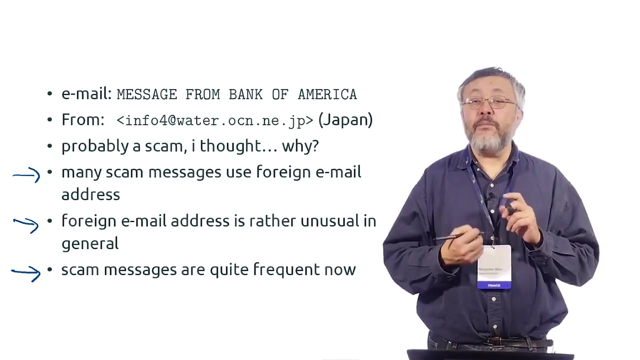 the name of the person and the location of the person and the address. and another third observation, unfortunately, that the scam messages are rather often so people try to somehow to prevent them or to prosecute the people who send them. quite often, unfortunately. and these three reasons are just three components. 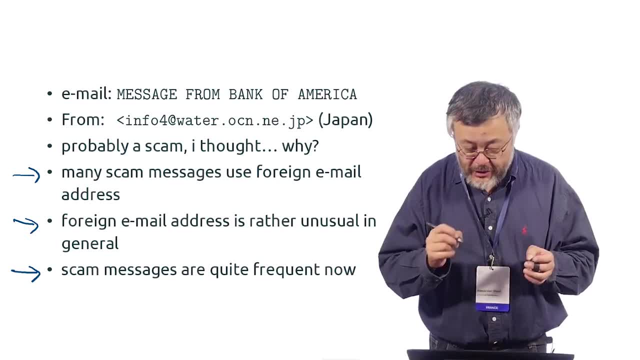 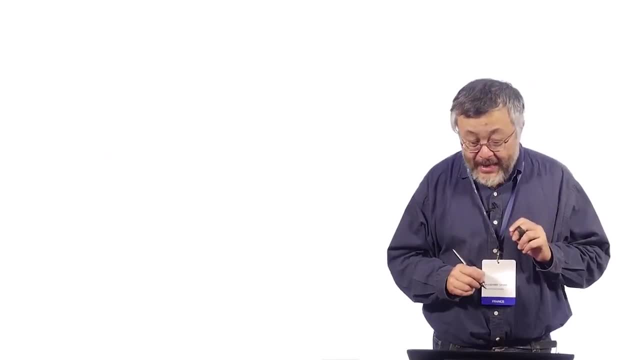 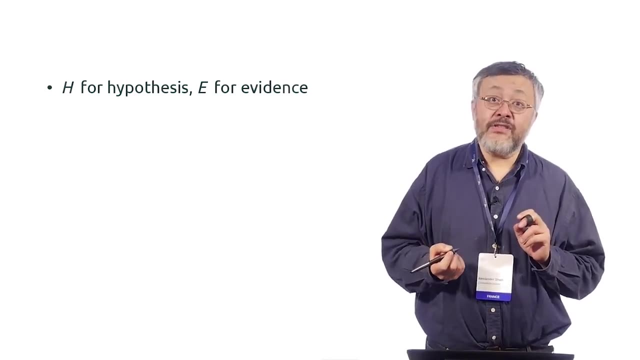 of bias and reasoning. I will tell you. try to explain what do I mean in the next slide. so there are three components of bias reasoning and here is the formula. so it deals with two events. they are called hypothesis and evidence, but just any two events. the names are: 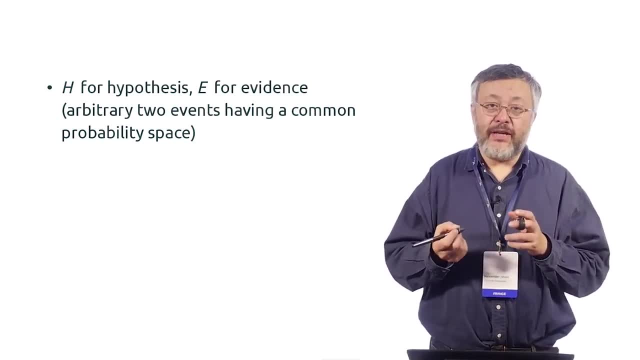 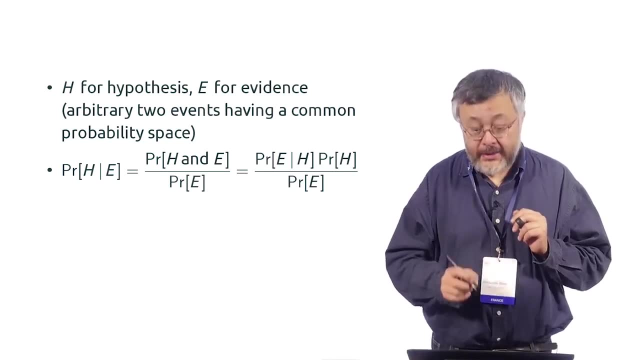 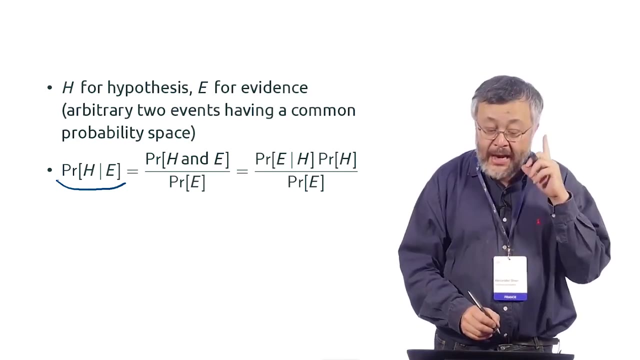 but of course they should be in the same probability space. so for example, we can consider the event H and E. so recall the definition of conditional probability. so the conditional probability of H under the condition E, the probability of hypothesis. it's somehow counterintuitive, the probability of hypothesis. 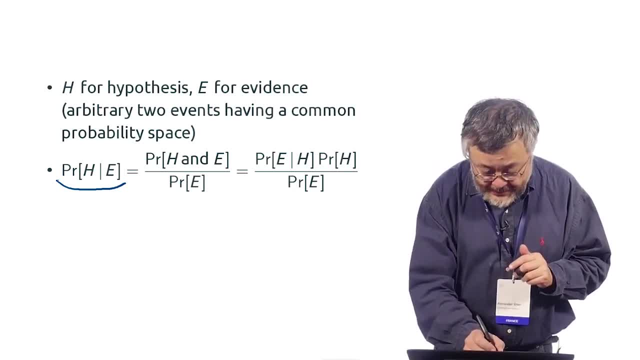 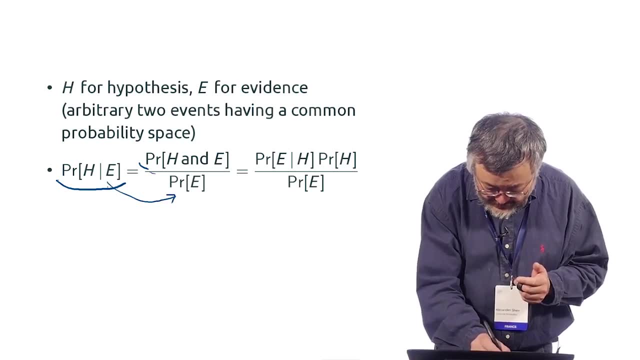 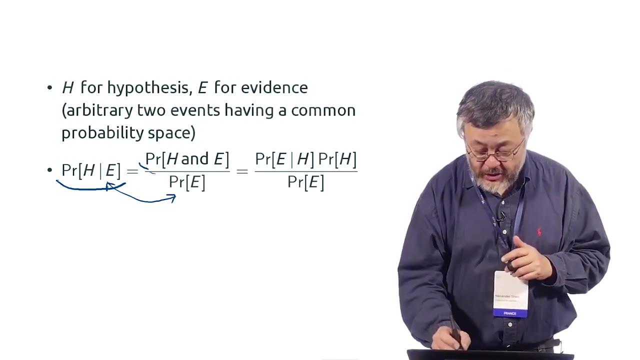 under the condition that event happens is, by definition, just a fraction. this together divided by probability of the condition, and then we can use the same formula, the definition of conditional probability, in other direction. we can start with H and use the other conditional probability. you see that it's in different order. 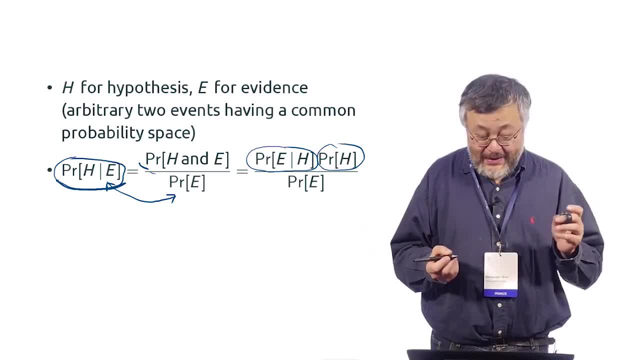 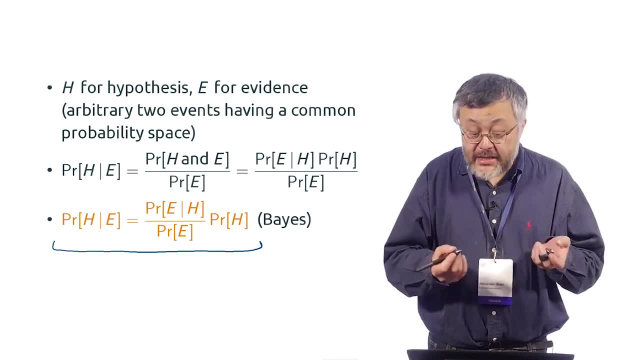 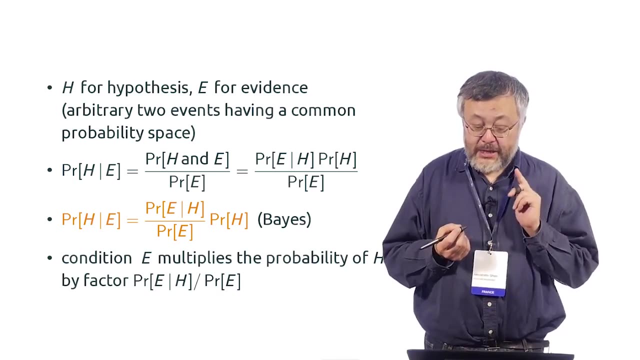 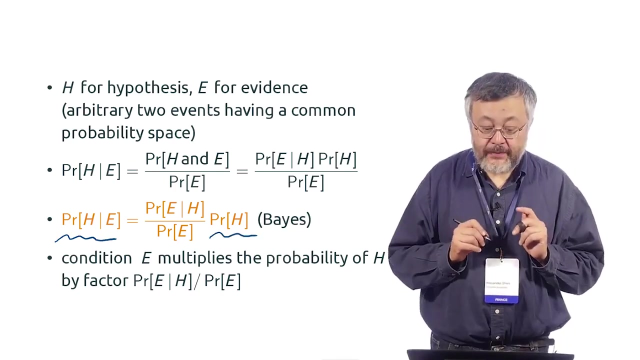 okay, so what? we can rewrite it even like this, and it's trivial computation, but it has some meaning, and the meaning is can be explained like this. so we are comparing the probability of H with condition E or without this condition, and with condition E somehow it multiplies the probability. 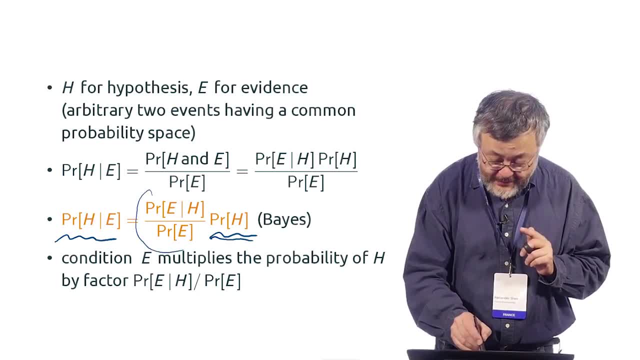 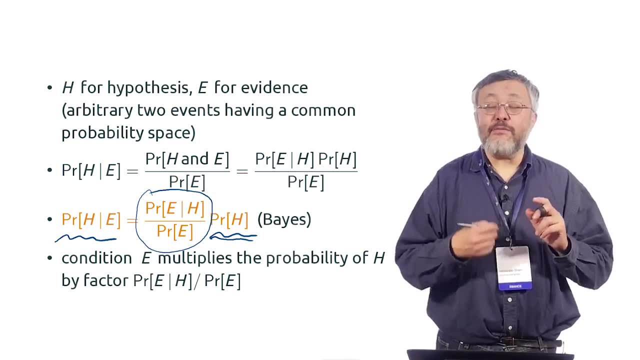 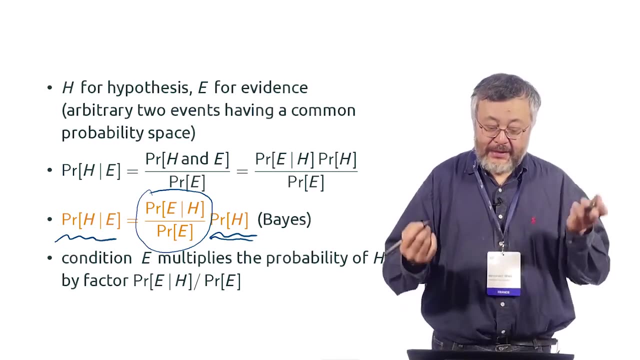 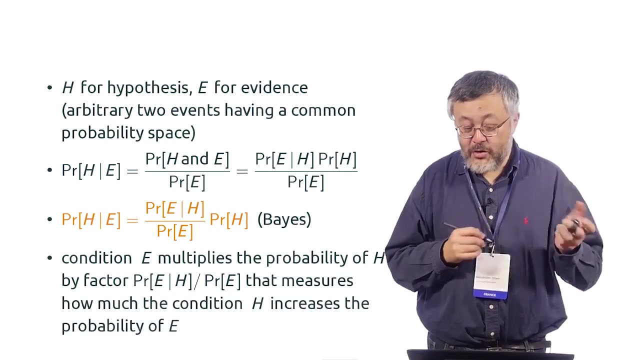 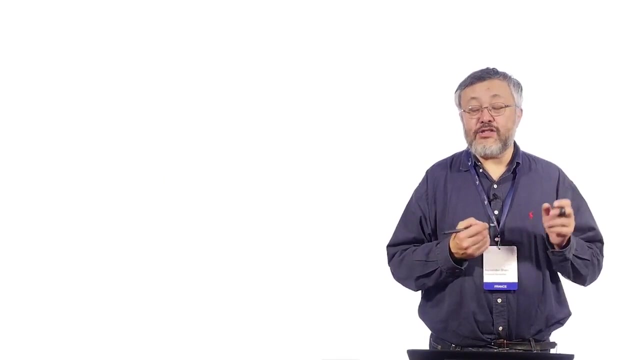 without the condition by some factor, and this factor shows how much. how much E becomes more probable if we add the condition H. so the condition multiplies probability by some factor, which is another ratio. so it's kind of explanation of this factor. we will see this as an example. 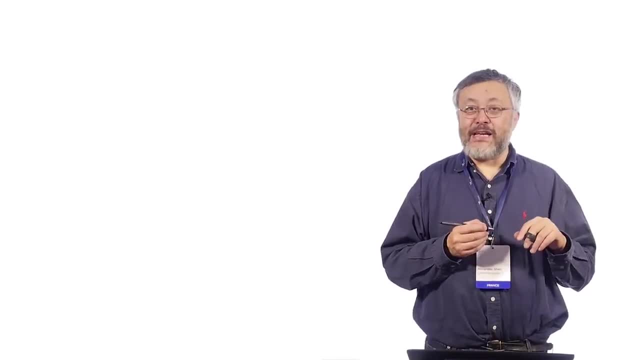 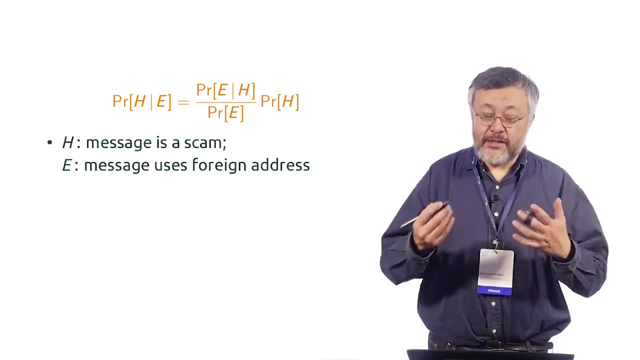 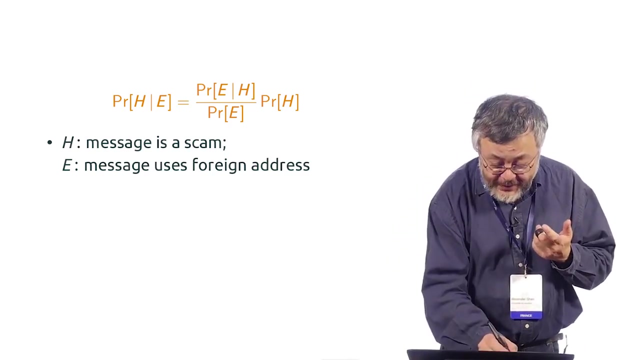 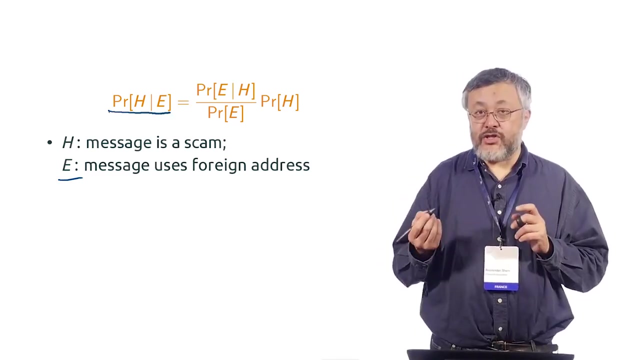 so let's compare our theory and our practice, our example, with this email. so this is the bias formula and what is the interpretation? so H, the hypothesis is that the message is a scam and the observed event is that message uses a foreign address. so how probable is that the message is a scam? 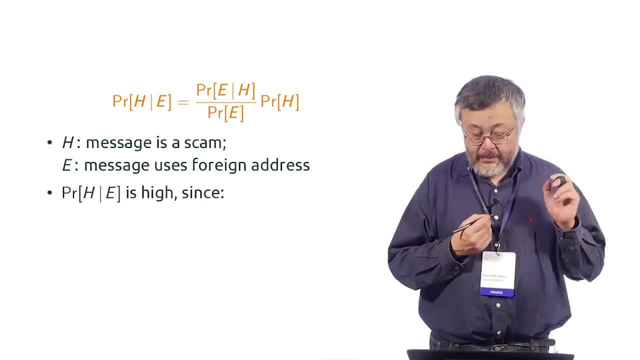 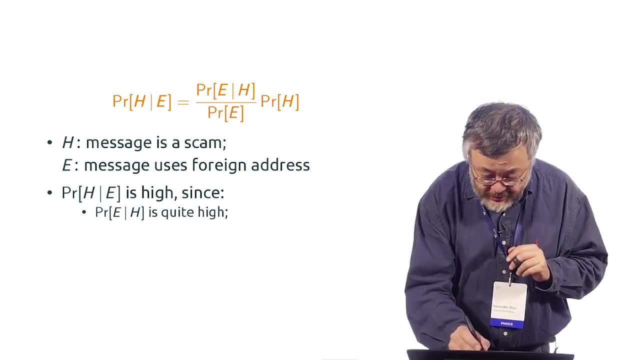 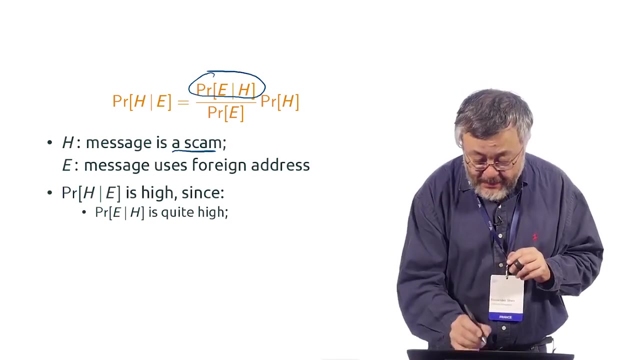 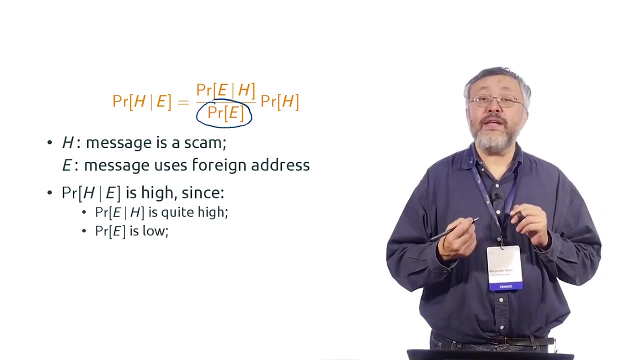 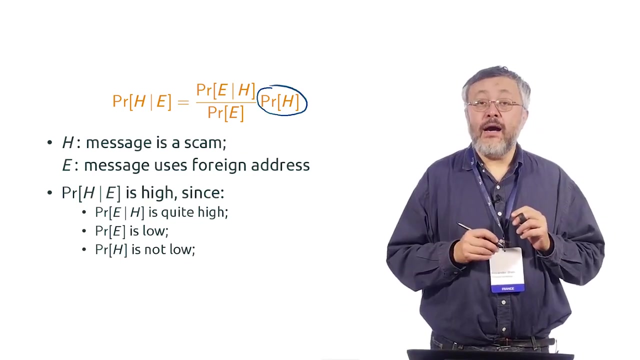 assuming that it has a foreign address, and my reasoning was that this probability is rather high because, first, this thing is quite high, which means that many scam messages use foreign address, and this is pretty low, that not many messages in general have foreign address, and this is not very low. 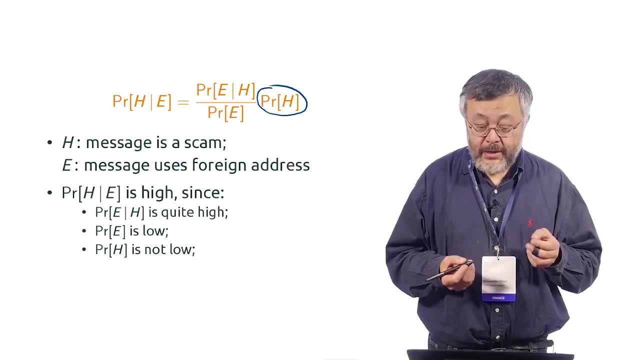 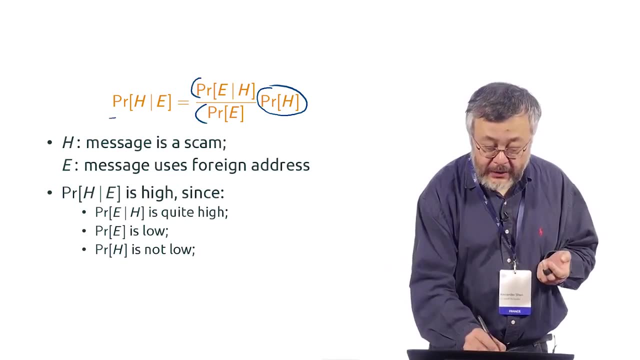 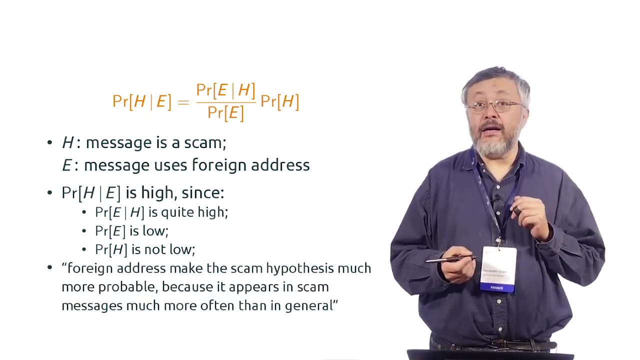 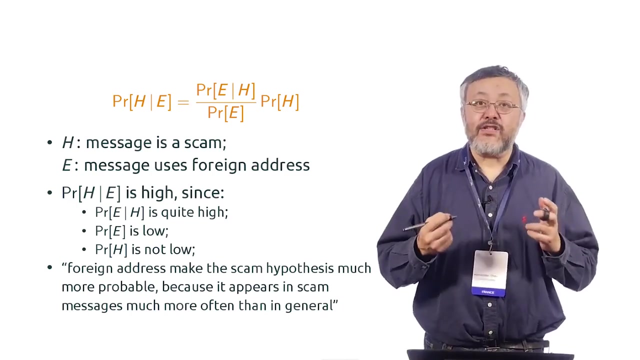 nowadays there is a lot of scam, so we have: this is rather high, this is low and this is not very low. this thing is high and this was the reasoning why I decided that this is a scam. so I tried to write this just in one sentence, the reasoning. 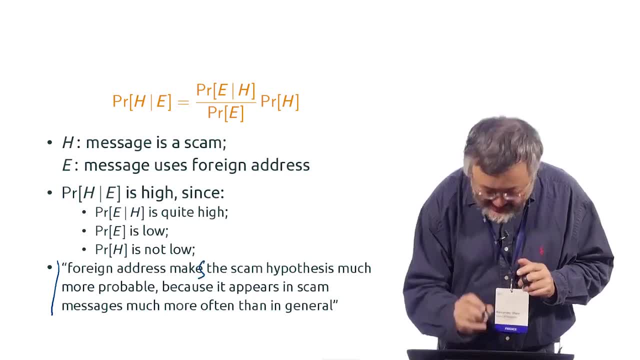 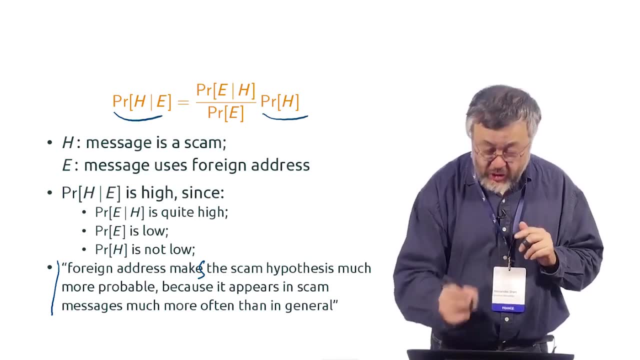 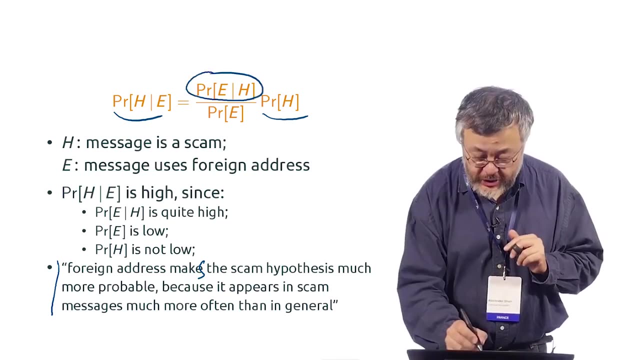 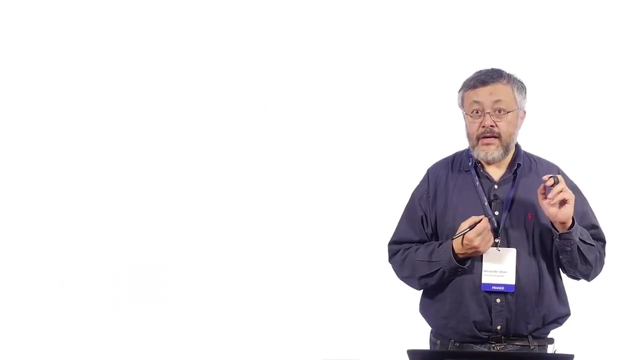 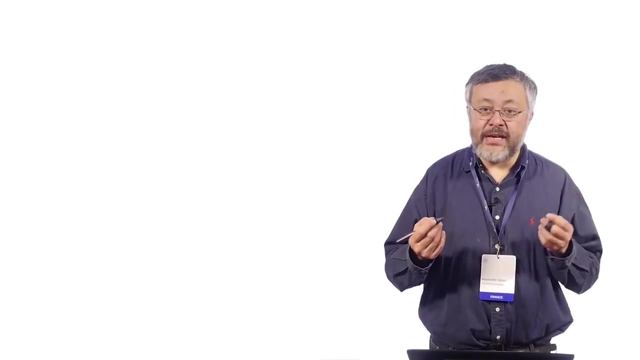 it's written here. so foreign address makes the scam hypothesis much more probable compared to original probability, because it appears in the messages much more often than in general. so this is a reading of bias formula for our special case. and let's now look on our example with disease. 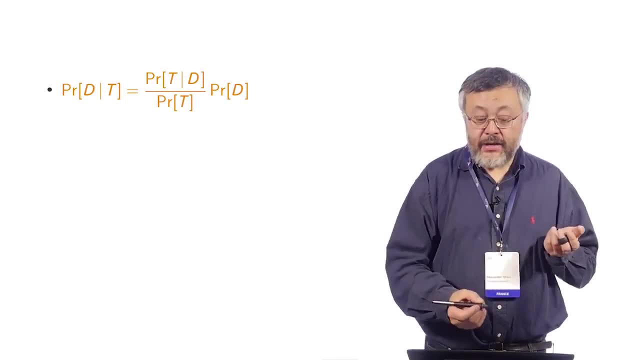 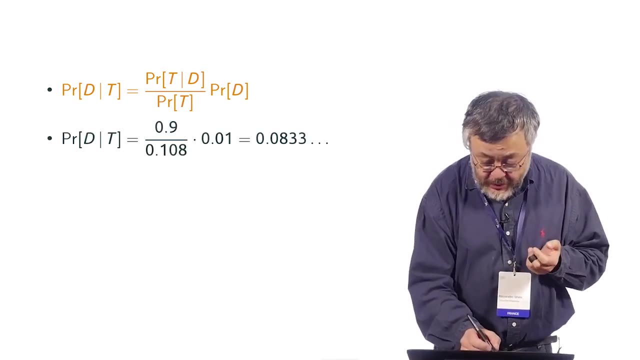 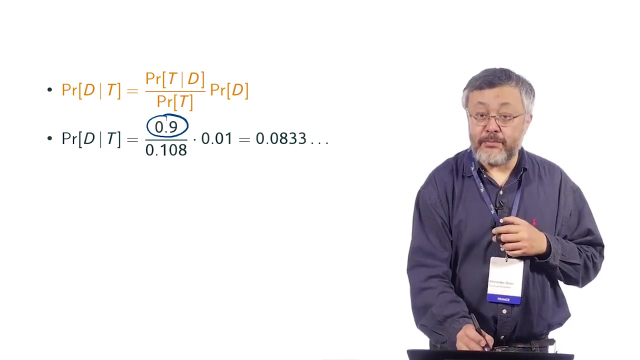 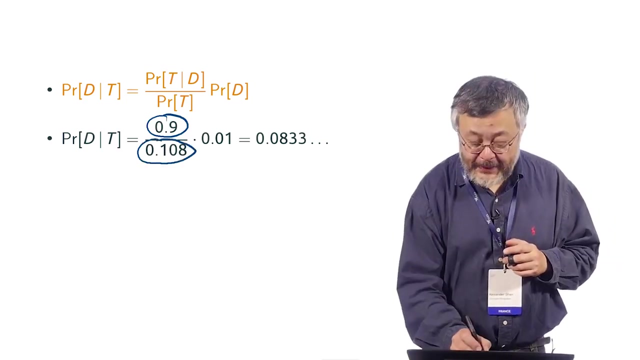 when somehow similar reasoning doesn't work, why the formula doesn't give things. so again we have this computation. so probability of test for people having disease is 0.9. the probability of having the positive test we computed using the formula of total probability is this: and here is the probability. 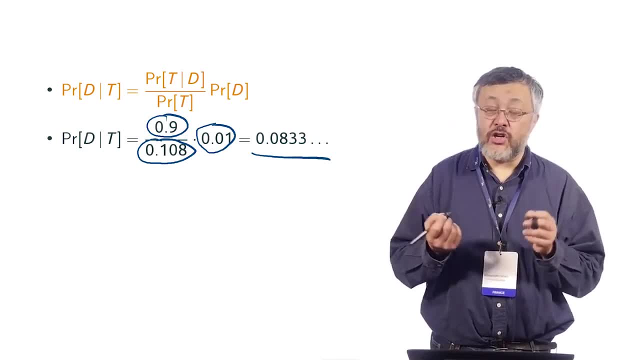 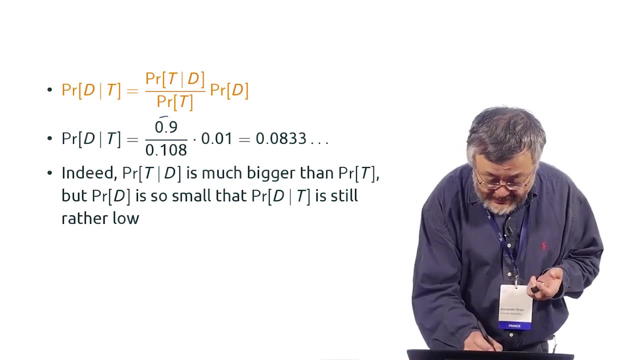 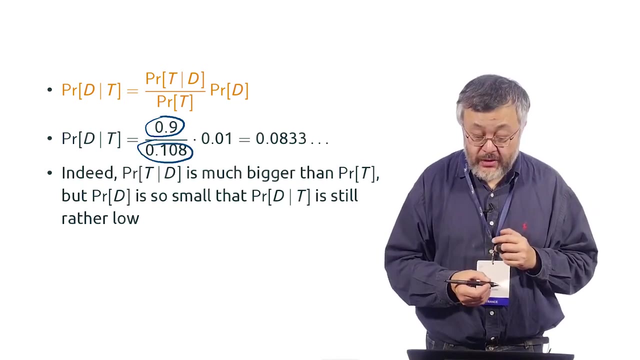 of the disease and we get. when we compute things, we get only 8%. so why don't we get such a big number of tests? for people having the disease is much bigger than the probability in the general population, but this probability of the disease is small. 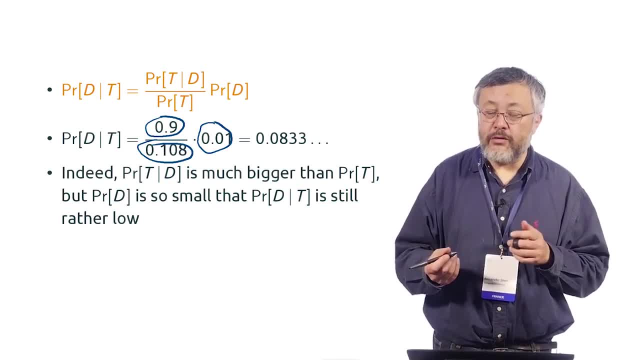 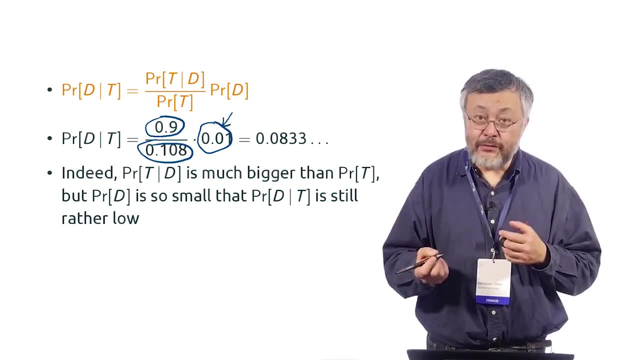 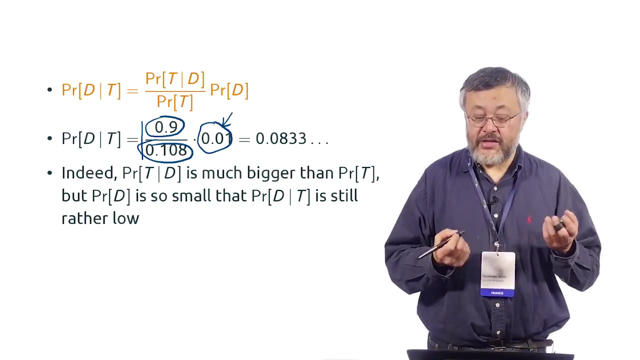 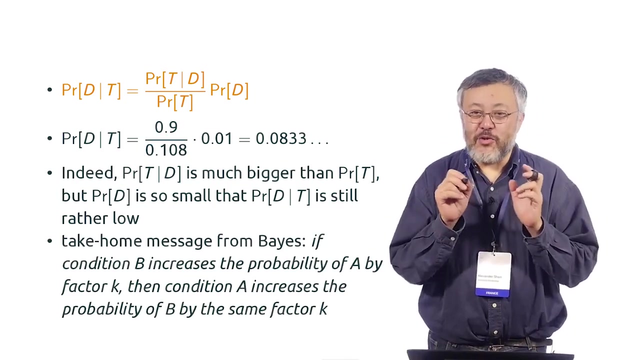 very small. so even the product is not very large, only 1 over 12 actually. so here the hypothesis was so improbable by itself that even the increase in the probability because of the bias theorem is what happens in our example. ok, Coursera wants all the time. 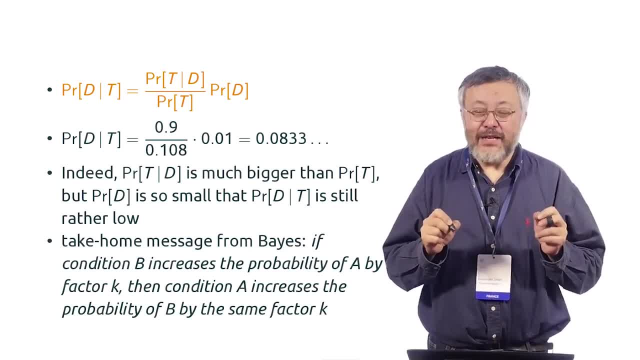 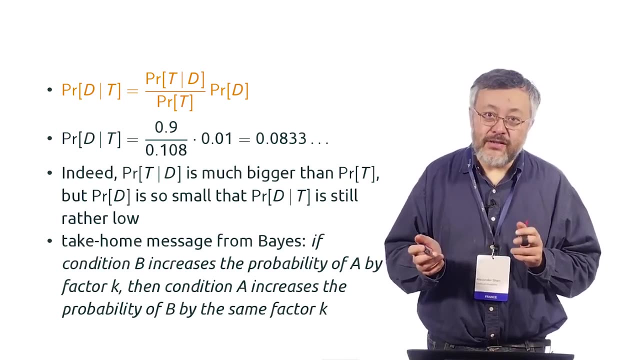 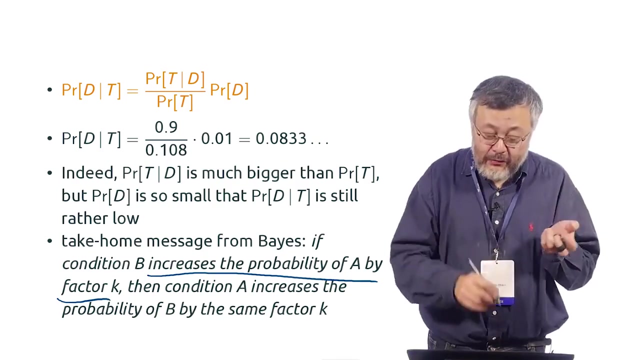 take home messages and repeating the main learning objective. ok, so here the learning objective is to understand the meaning of bias formula and see the cases when you apply this reasoning in the real life. so this is the message: when we consider the probability of some event by some big factor, 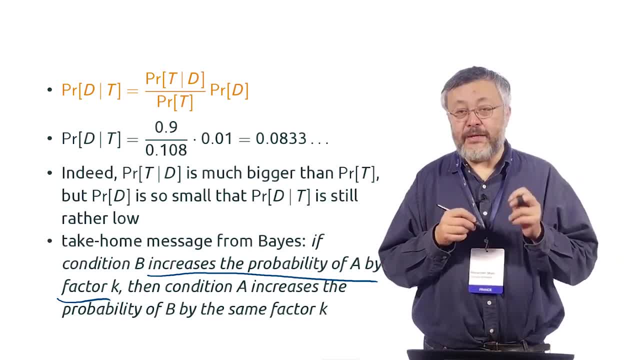 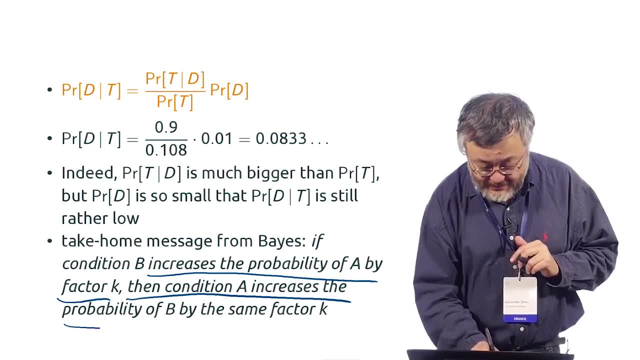 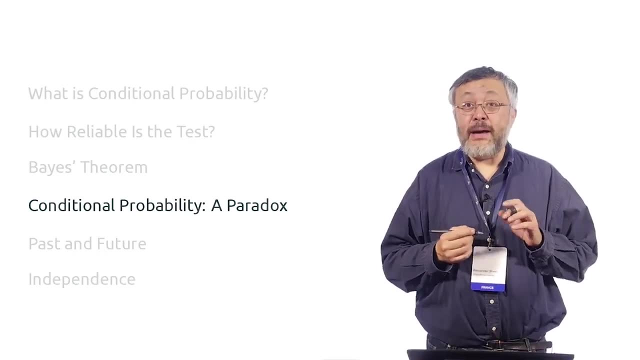 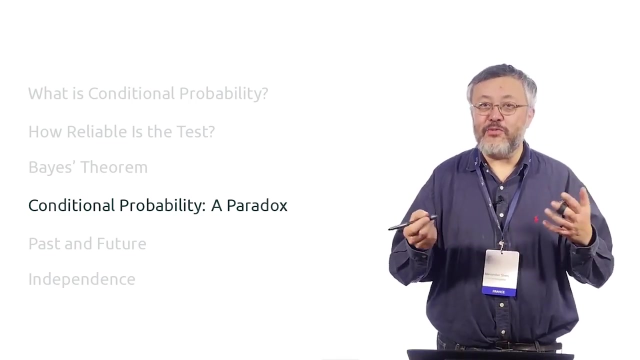 of course it's true for any factor, but it's interesting for big factors. so if condition B increases the probability of A, then symmetrically condition A increases the probability of B by the same factor. and you should. there is a kind of a conflict between reasonings. 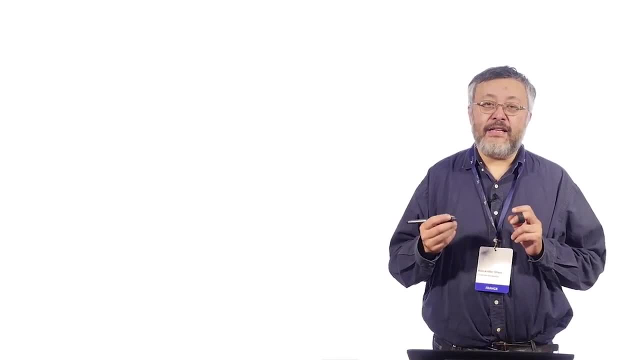 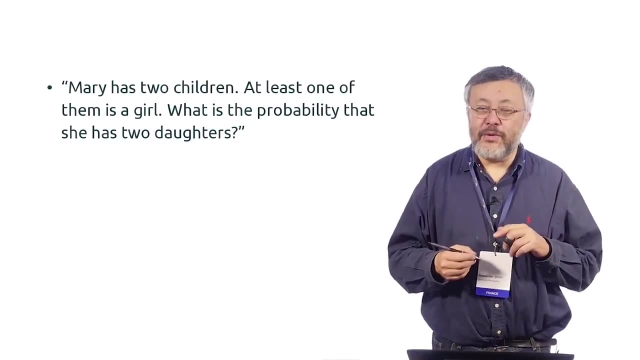 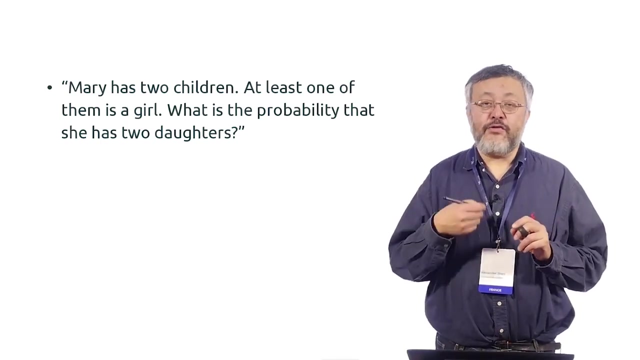 two different ways of reasoning. so this is known, the paradox is known in the setting with children. but so imagine, some woman has two children and you know that at least one of them is a girl. so what is the probability that there are two girls? the other child 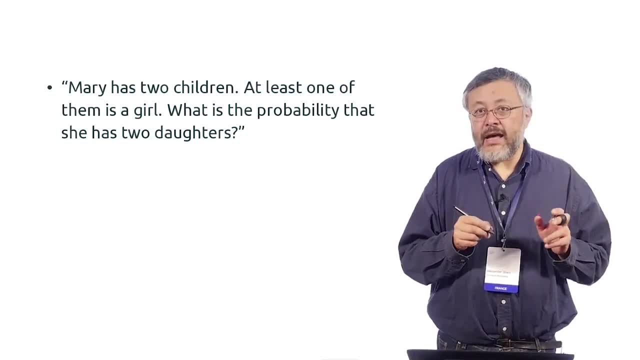 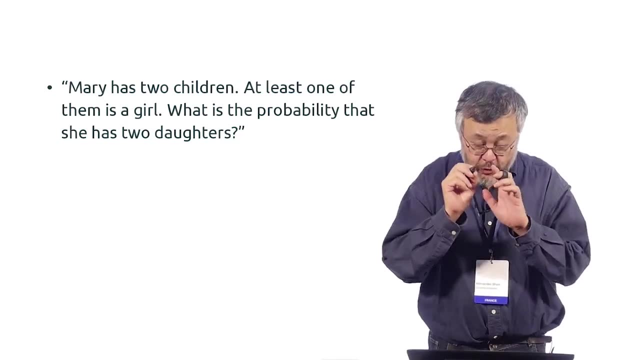 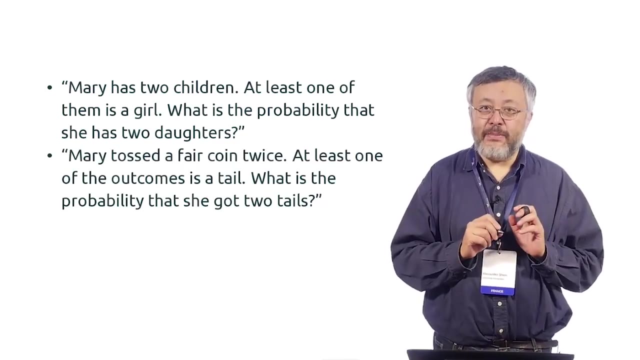 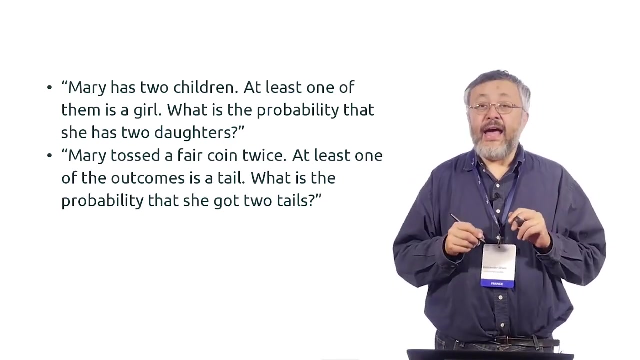 ok, this is a biological question and whether the dependent, the sex of the two siblings, is dependent or not. but just to ignore this problem, let's consider the cleaned formulation, without any biological information. so, Mary, just make two times, two times. and it's known that at least one of outcomes 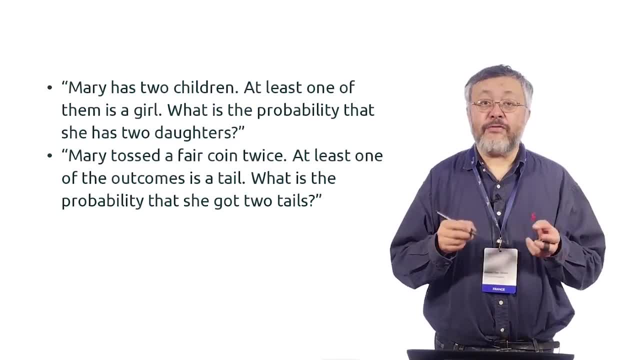 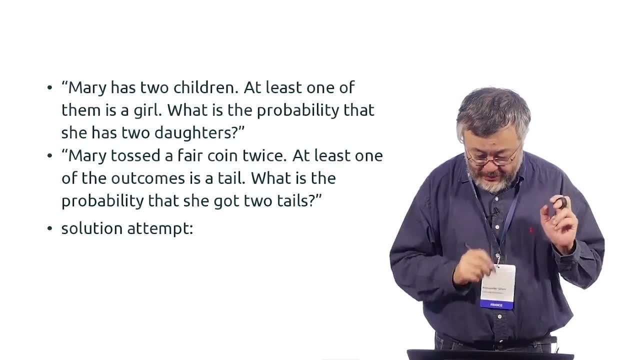 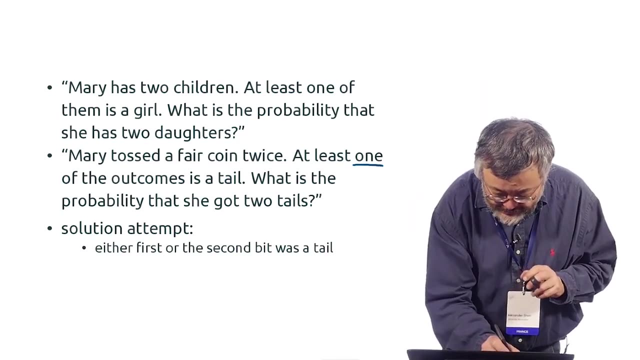 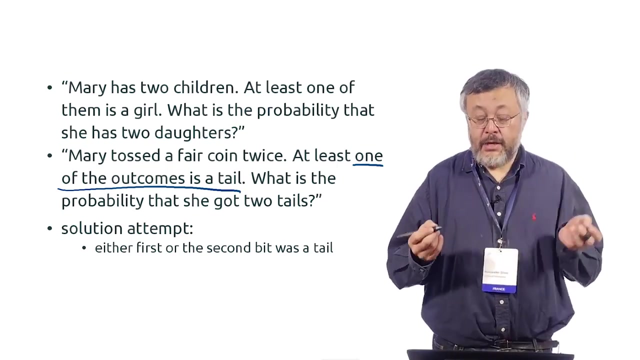 is a tail. and so what is the probability to have two tails? and I will show you two arguments which give different answers. the first argument, first solution, of course, if there is one of the outcomes is a tail, then there are two cases either. the first bit is a tail, 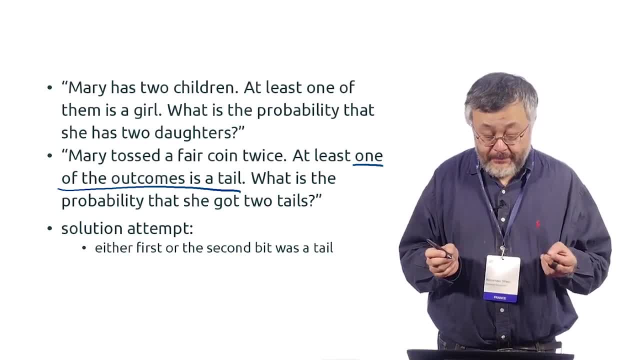 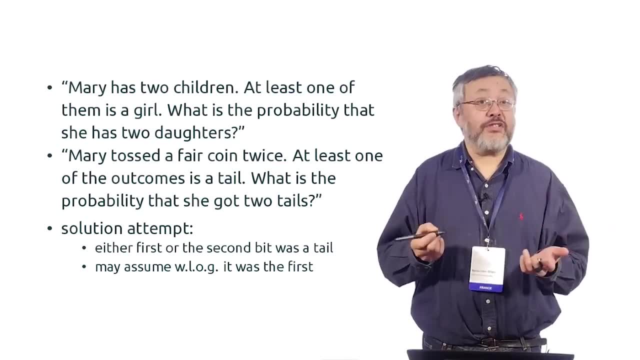 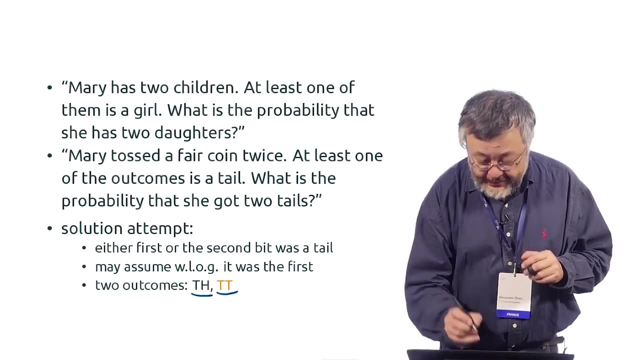 or the second bit is a tail, and of course we may, they say, we may assume, without loss of generality, that it was the first case. for example, first bit is a tail and then there are two possible outcomes: tail head and tail tail, and this is a favorable outcomes. 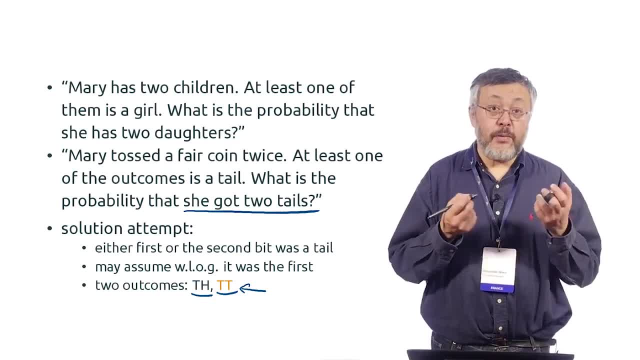 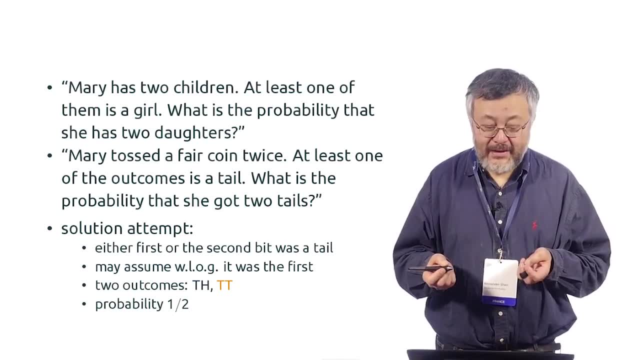 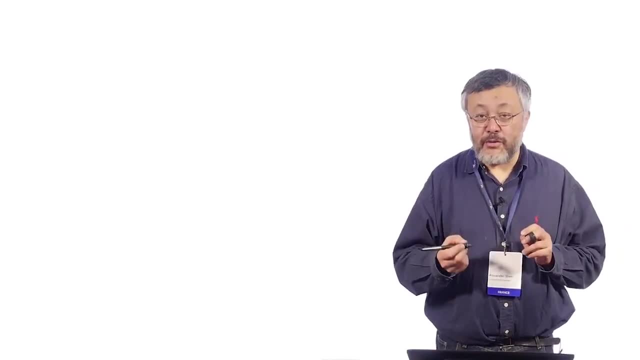 when we have two tails. so there are two outcomes equiprobable, and one of them is favorable. so the probability is one half. so are you convinced? what do you think? let me, let me show you another solution. it's more formal, without this loss of generality. stories. 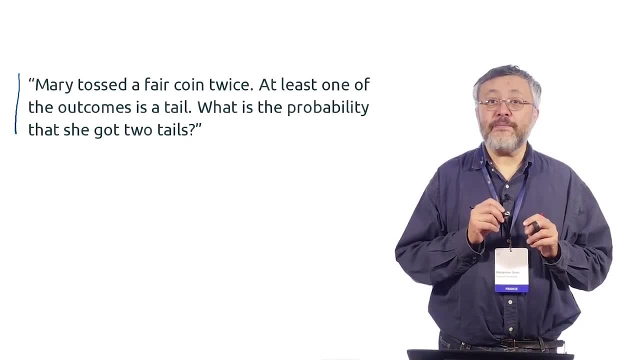 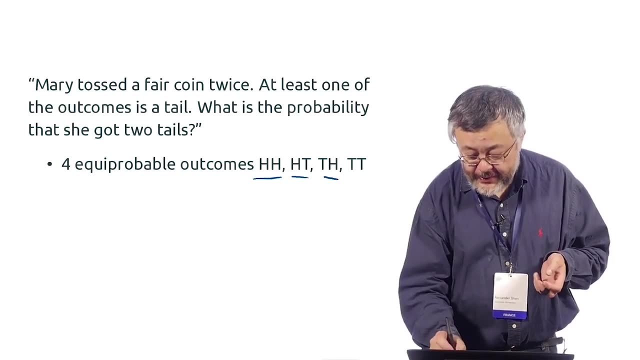 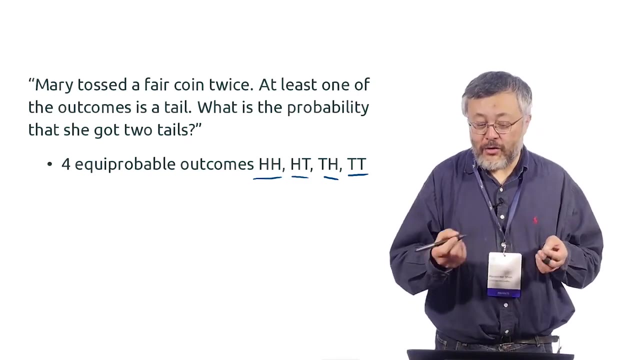 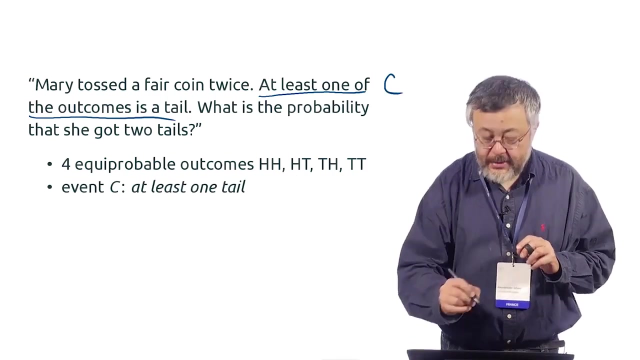 here is again the question. and now we just consider four equiprobable outcomes: head, head, head, tail, tail, head, tail, tail- and just do the boring thing. we just look at all the, all the events. so event here, this event C, at least one tail. where is it? 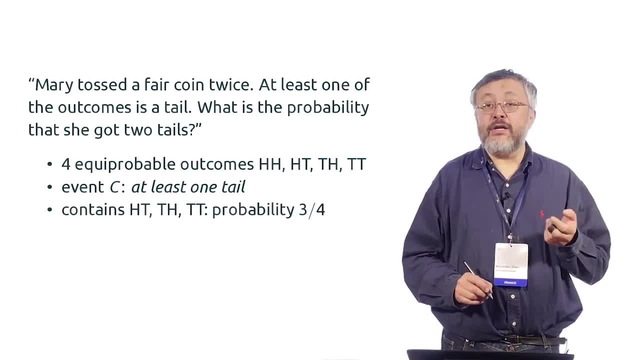 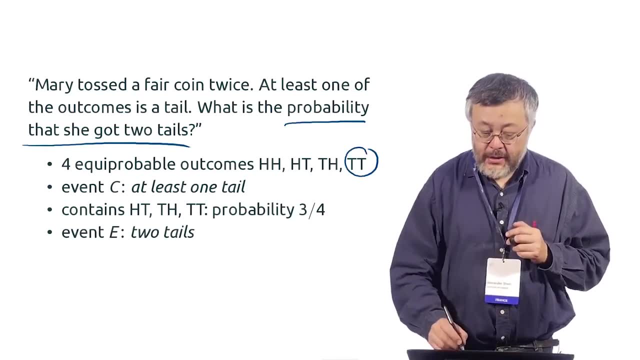 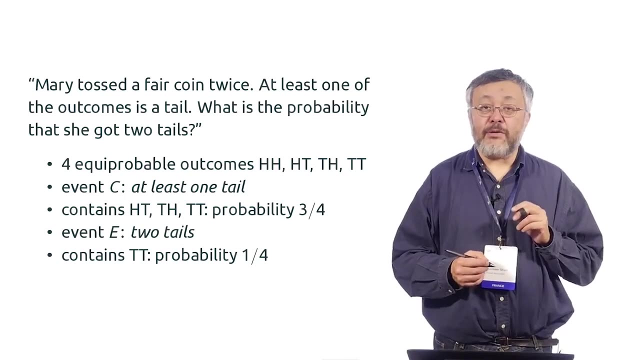 here, here and here. so it's probability three over four and this event probability of two tails. this is just this one. so among these three events, we have only one event. E is two tails, it's only one outcome and probability one over four, and actually it's now. 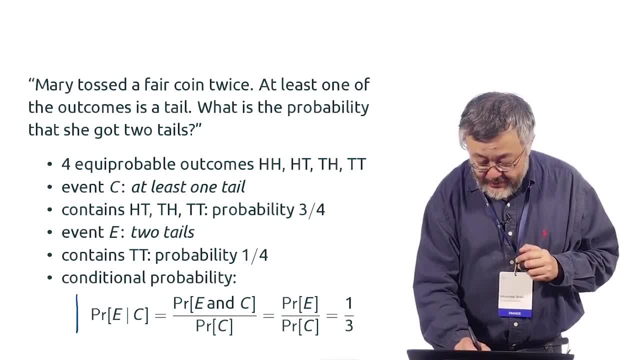 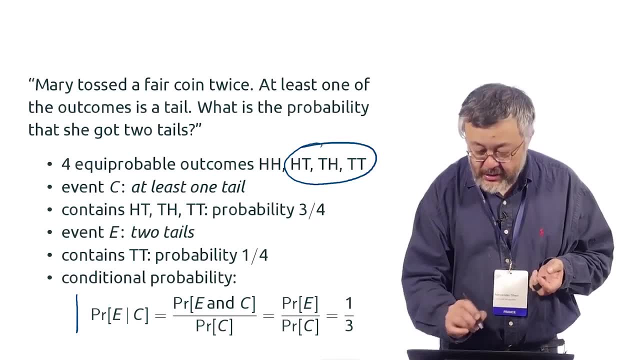 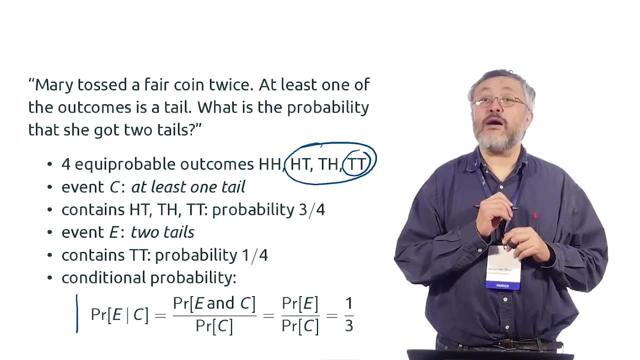 easy to compute. the conditional probability here is: it is one. fourth over three, fourth is one over three. or we can say that the condition is this and the event is this. now, event is a part of the condition. so out of three possible outcomes, our event selects one. 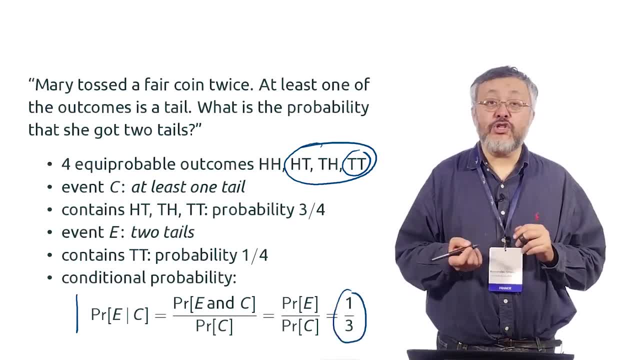 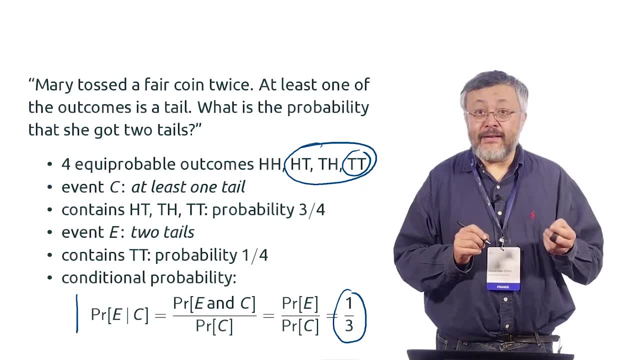 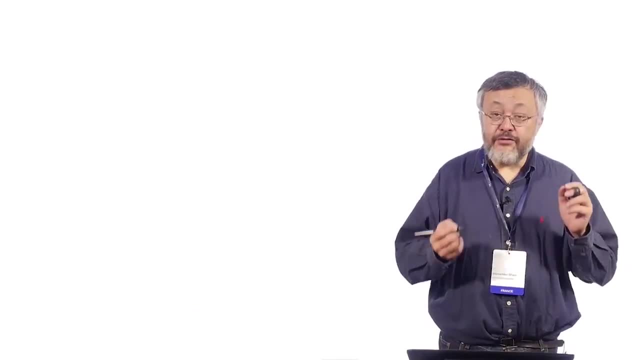 so it's one over three. so what do you think? which argument is correct? actually, the second one is correct, and to understand what is the error in the first argument, we should look at a picture and first we should read the problem statement and parse the problem statement. 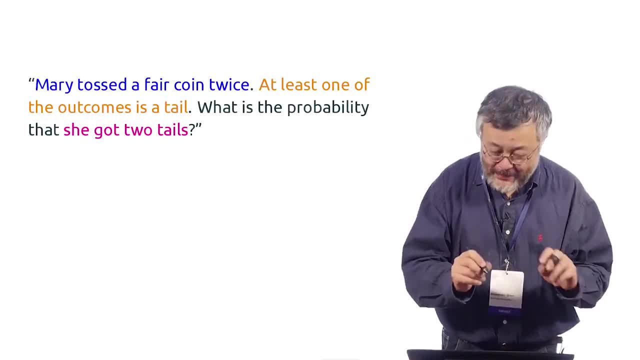 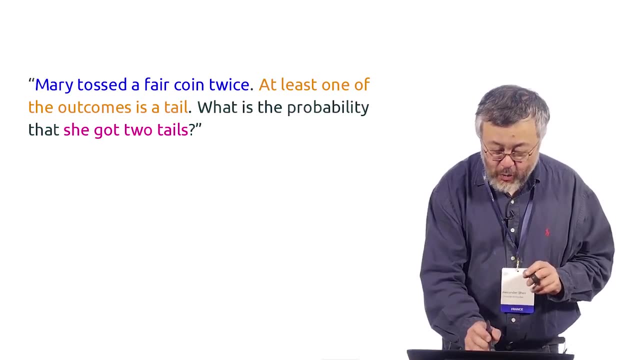 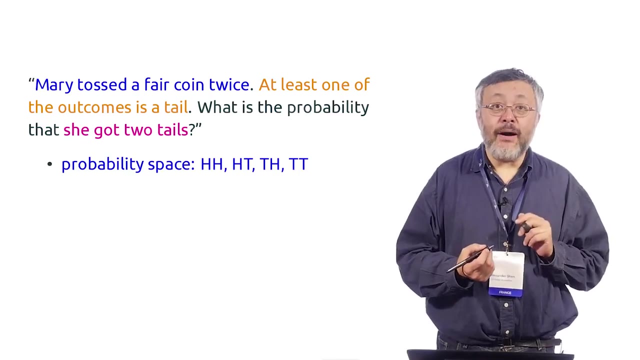 so to say so, here are shown in colors. I prepared this slide, so it's just the same statement, but there are three parts: the blue one, this one, yellow one and the red one or magenta one. ok, what is the role of these three parts? the first part is just sets the probability space. 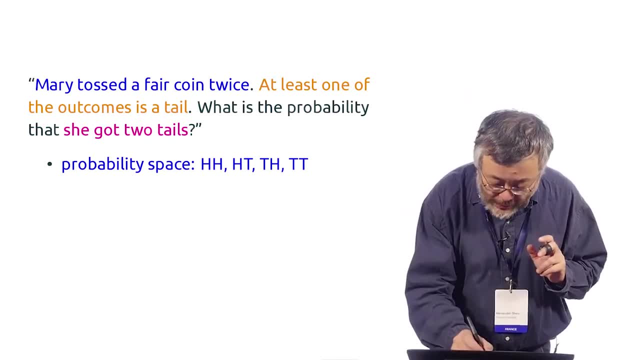 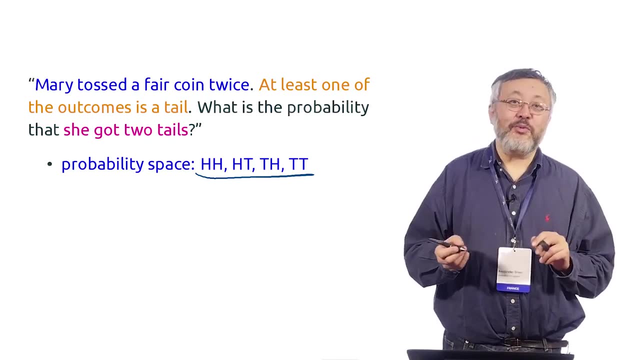 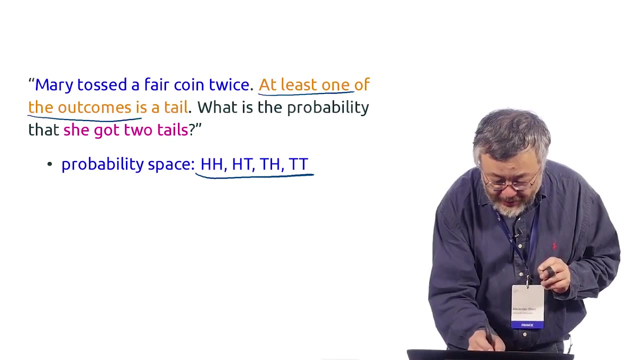 Mary tossed a fair coin twice means that there are four outcomes and they are equi-probable. oh, this is not set explicitly, but if you are in probability theory textbook you always assume this, even if it's not set explicitly. and then here is the condition: at least one of the outcome. 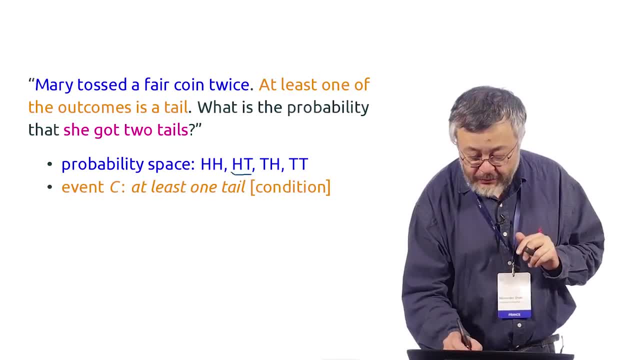 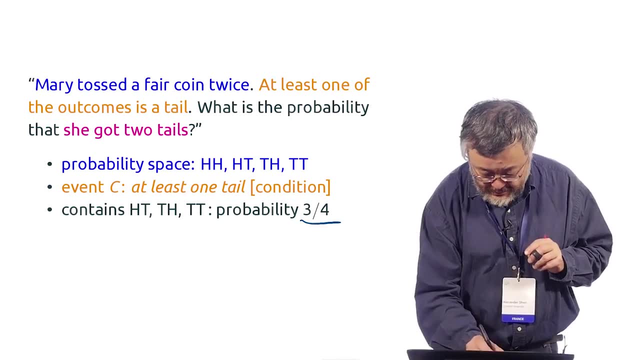 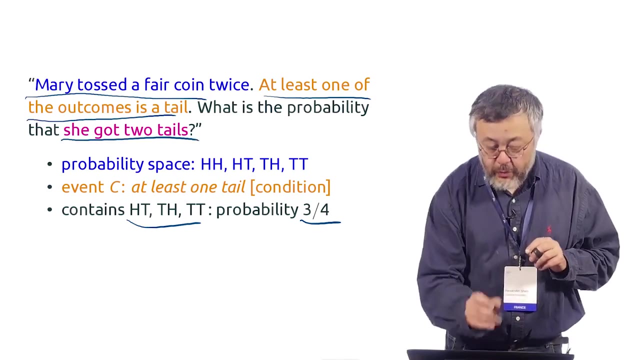 is a tail, so it's a condition, which is event made of three outcomes, and the probability of this event is three over four. here it is, and so there is the space, the condition and now the event we are interested in. so event E is two tails and this is one is part of this. 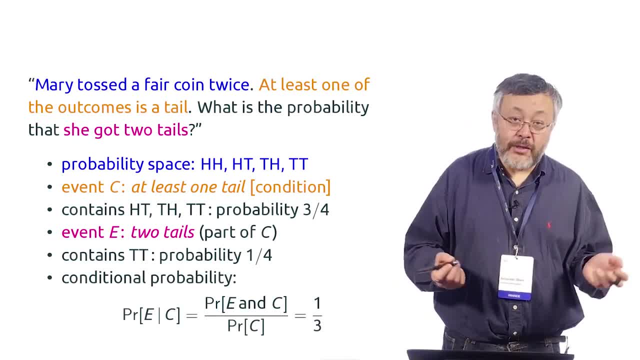 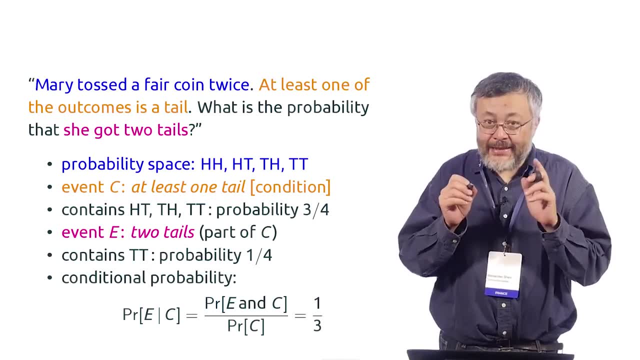 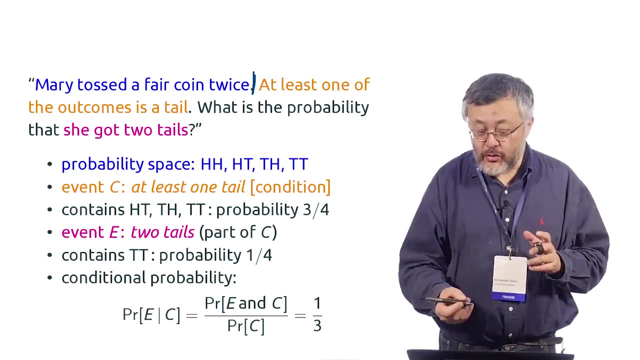 and this has probability one fourth and the condition of probability is one over three. so I just repeated the second argument. but the only difference is I clearly separated here the setting of the probability space and the condition. when you read this it's not clear. just Mary tossed a coin. 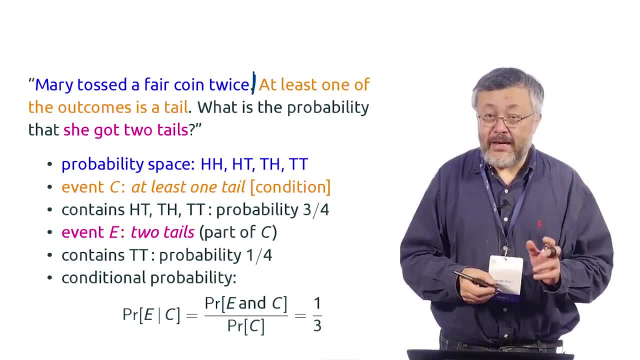 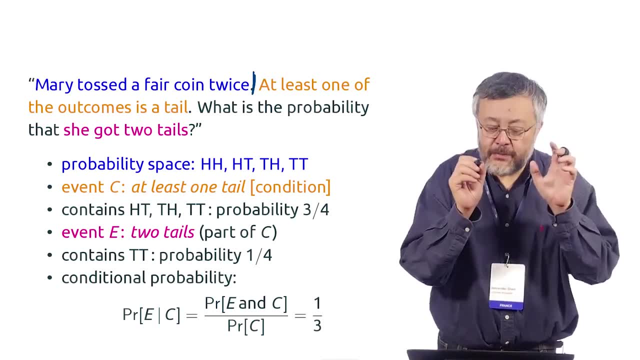 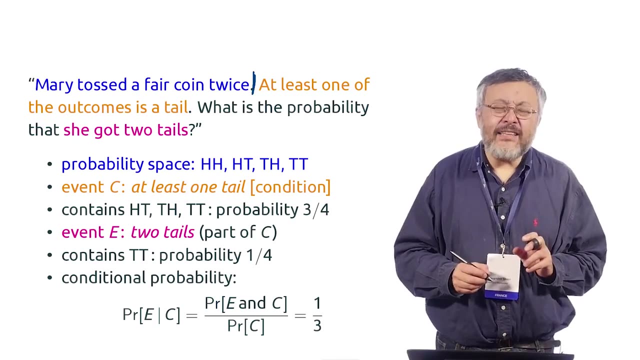 at least of the one of the outcomes, like kind of story. but if you want to ask a probability question you should clearly see, clearly distinguish the probability space and the condition. and actually it was the source of many errors. I think that just in 19th century, 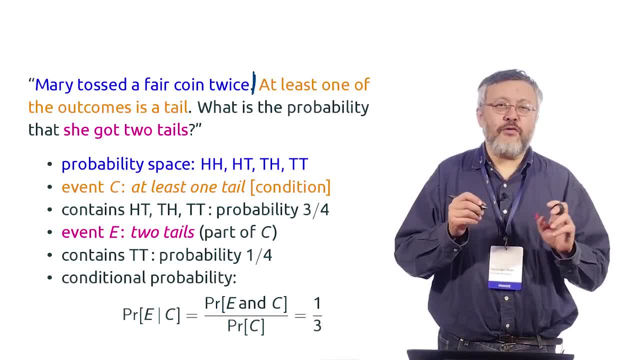 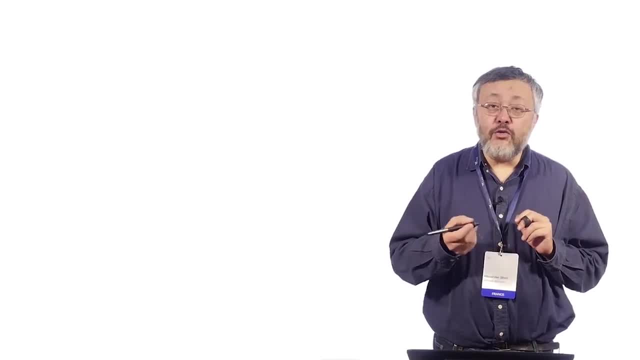 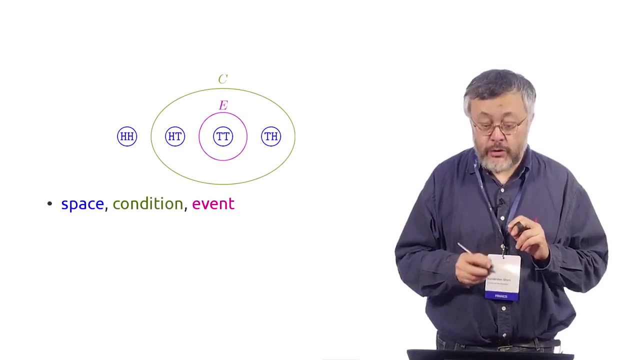 people do not understand this clearly and this was a source of many paradoxes and so on. so hopefully now people are better in this and we can look in the first solution- wrong solution, what we really did there, and there is a picture. this is a picture for the correct solution. 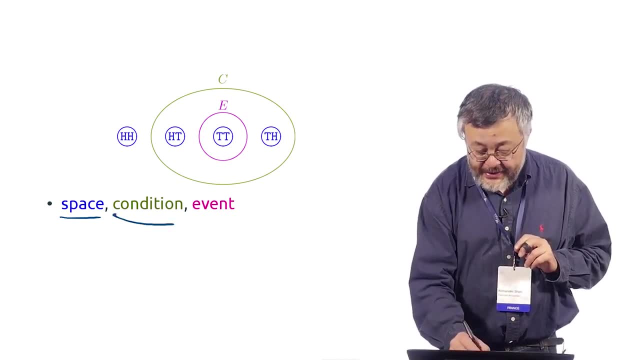 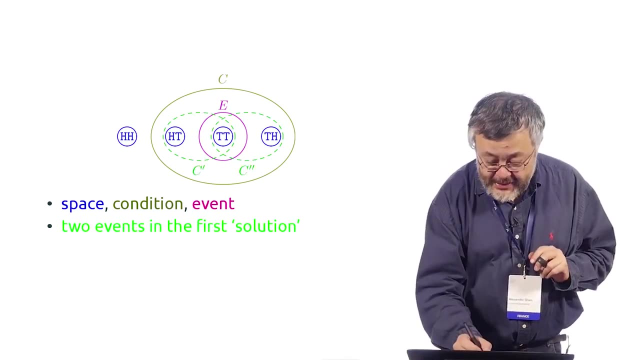 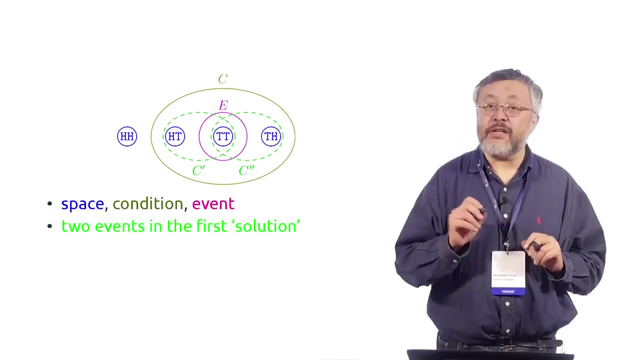 we have the space, this blue one, condition, this olive one, and event, this is event. so what we did in the first solution, we consider two other events, C prime and C double prime, and this is the event in the second tail, second tail, and this is the first tail. 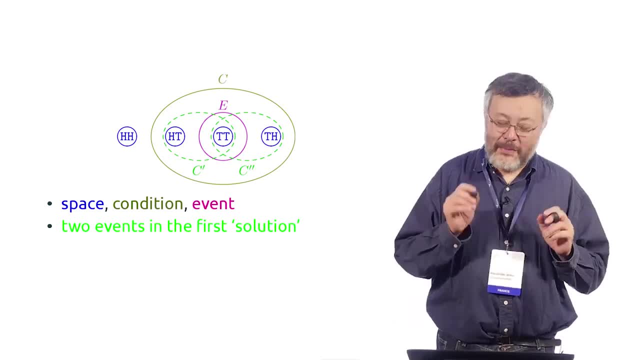 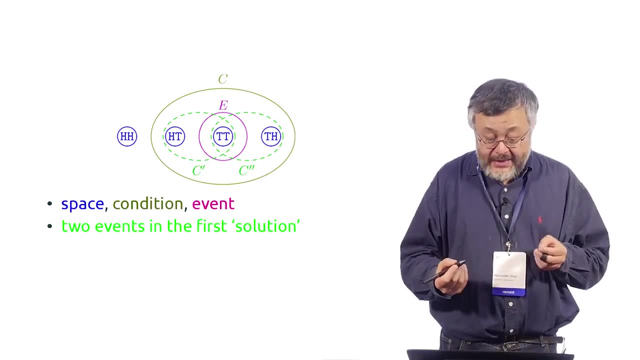 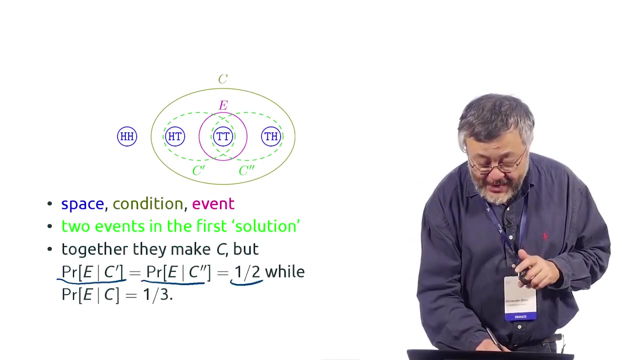 or maybe they should be denoted in other way. but anyway, there are two events and together they make the condition C, but for each of them the conditional probability is different. it's one over two and for the entire condition it's one over three. so when we say, without loss of generality, 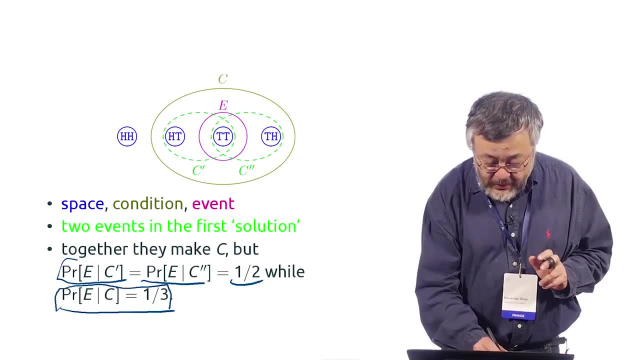 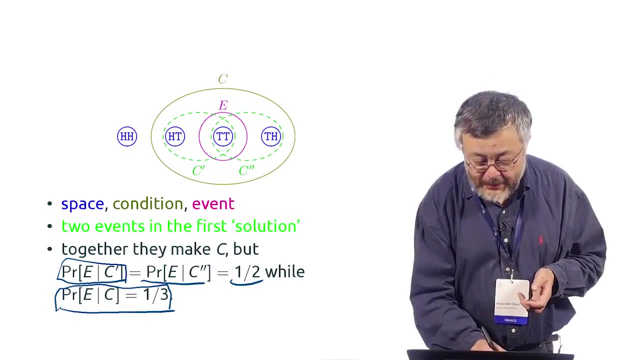 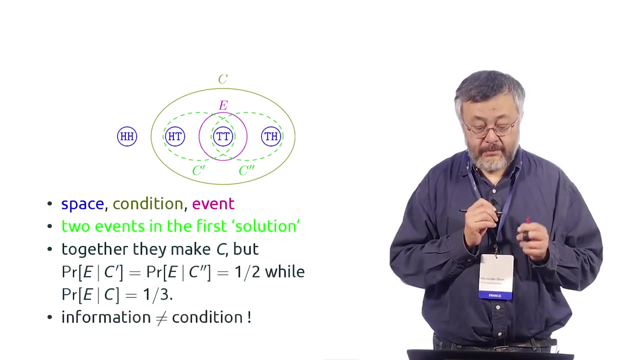 we do a very bad thing. we replace this by this only because this event C is a union of these two symmetric events, C prime and C double prime- but for each of them the conditional probability is different. so you cannot replace this and kind of take home message. 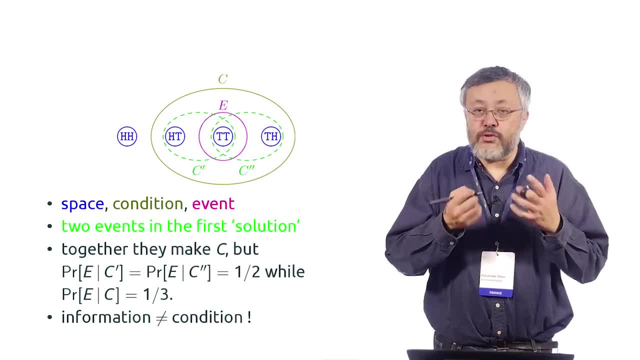 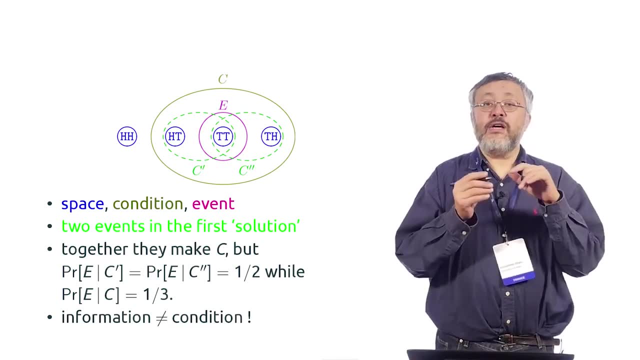 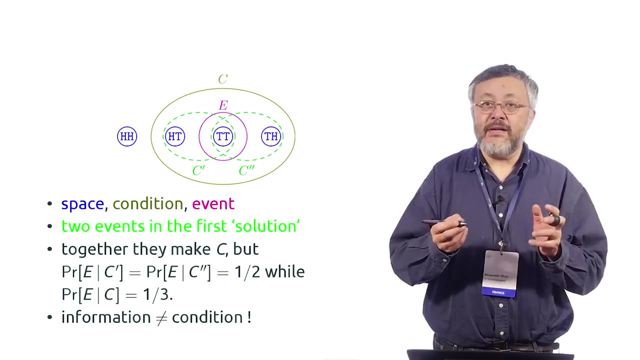 that information is not always. you should distinguish between information which explains the space and the condition, which is part of the problem, and explain what the probability space is, and then you say the condition and the event and then the problem is set. and if you just make some kind of a story, 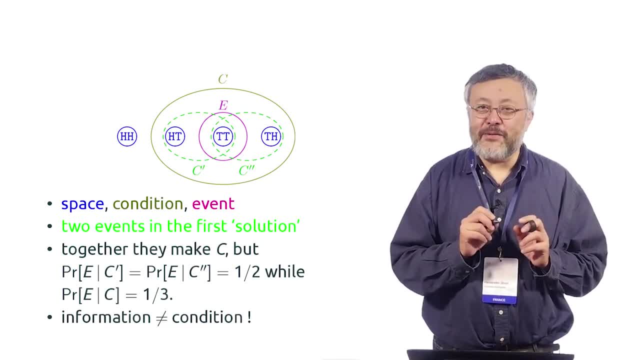 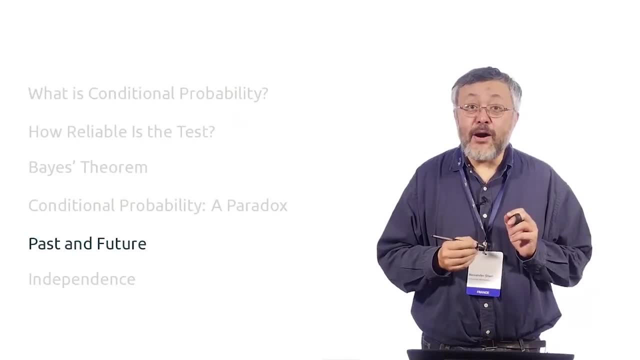 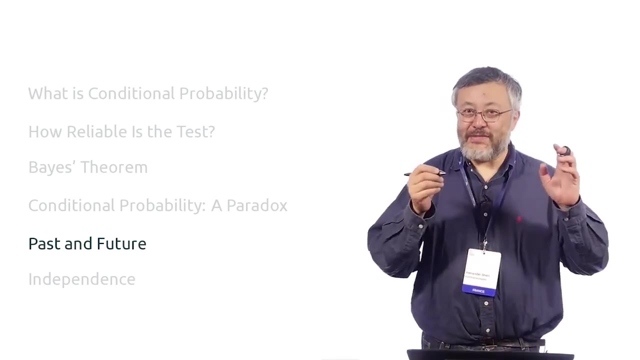 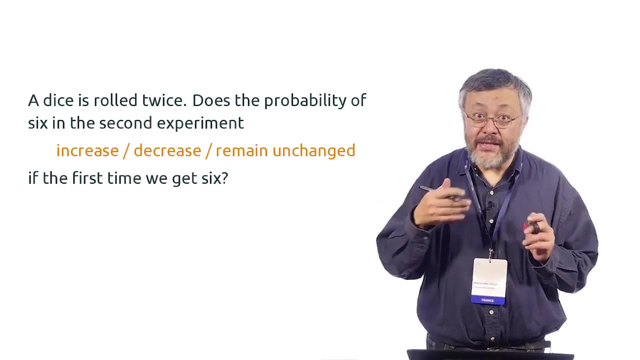 it always. it's a very easy way to get into trouble. you should avoid this and be clear. it is about informal questions: how the past, can the past influence the future. but ok, it's very philosophical. it's not clear. so imagine that a dice, you have a dice. 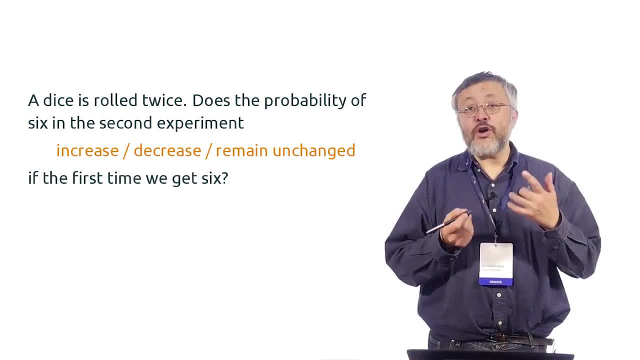 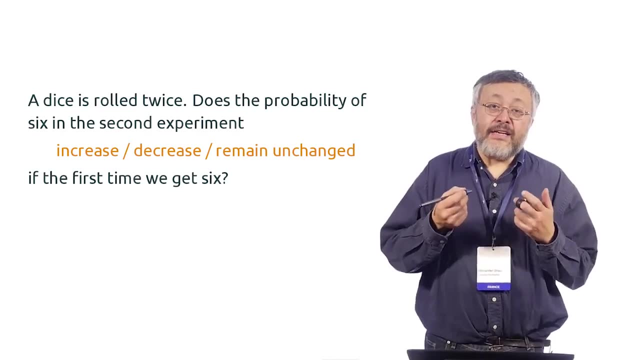 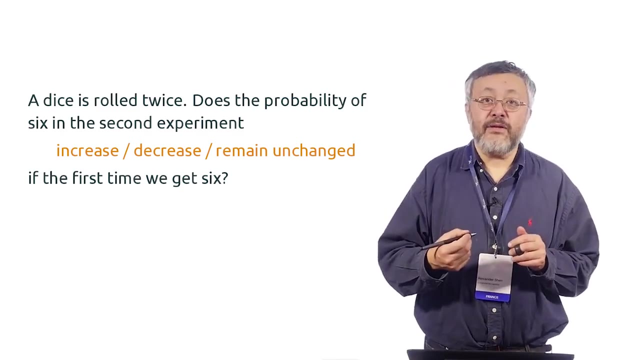 and you roll it twice and you are asked: how probable is 6? and imagine you have seen 6 in the first experiment and does this observation? does it increase, decrease or leaves unchanged the probability of getting 6 in the second experiment? you can do it easily. 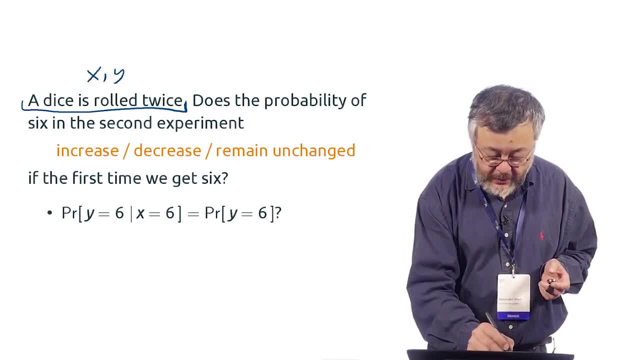 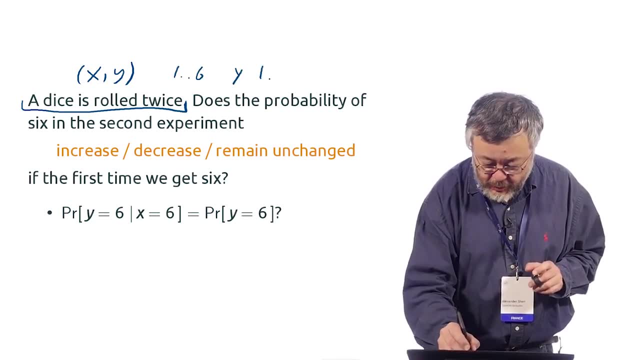 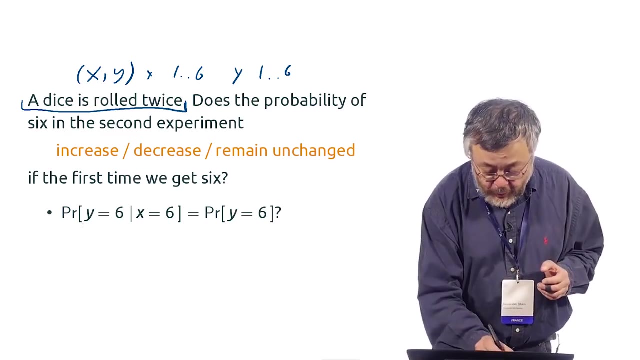 so here the space is just a pair of x and y inside x is 1 over 6, and y is also between 1 and 6, and all combinations have the same probability, and so we can compute: the conditional probability of y equals to 6. 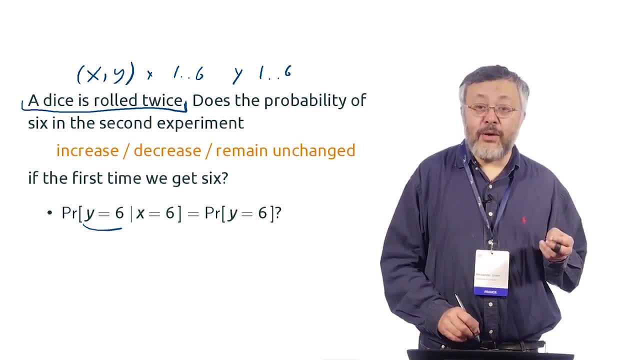 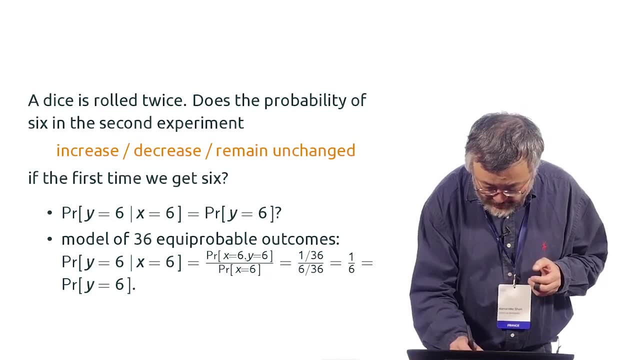 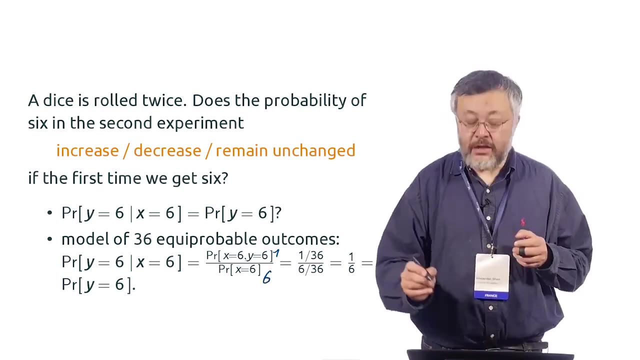 under the condition that x is equal to 6 and without the conditions, and it's easy to do this. so here we have 36 equiprobable outcomes and here we have only one outcome. so there is a fraction. so here we have only one outcome out of 36. 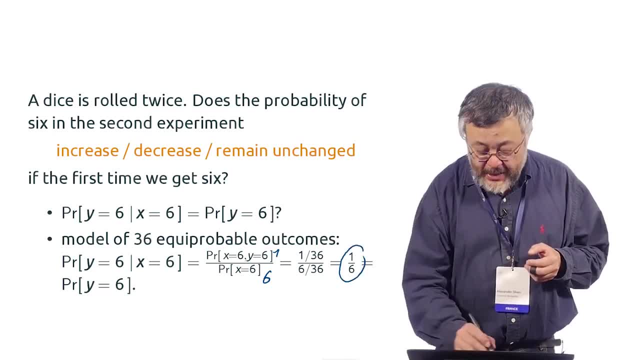 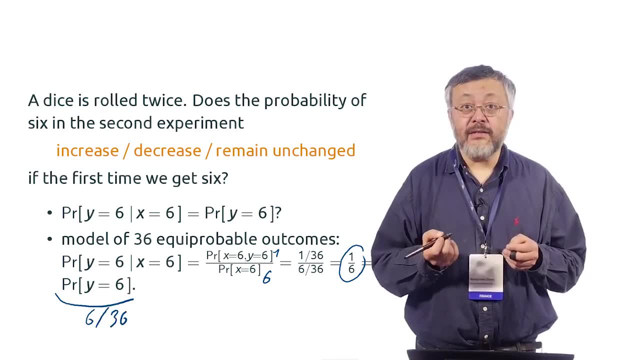 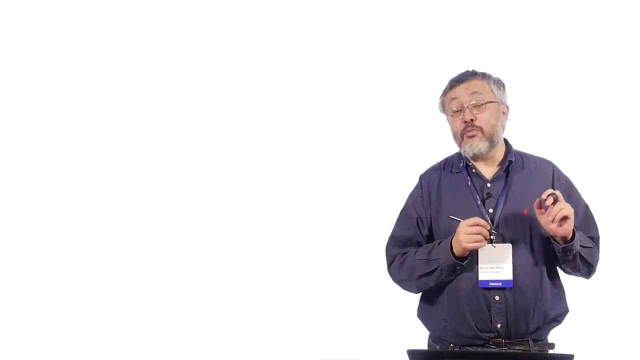 and here we have 6 outcomes for all possible values of y. so we get 1 over 6, and this is exactly. this is also 6 over 36 because there are 6 possible values of x. so in our model the condition doesn't change the probability. 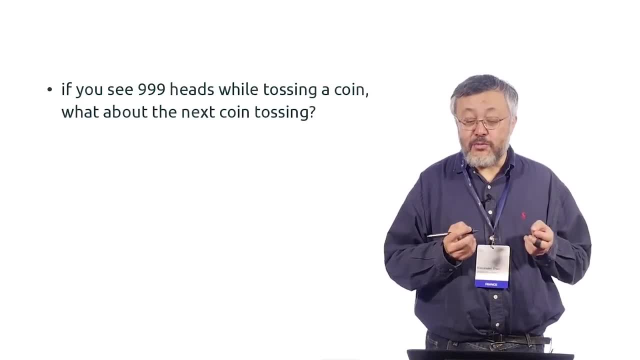 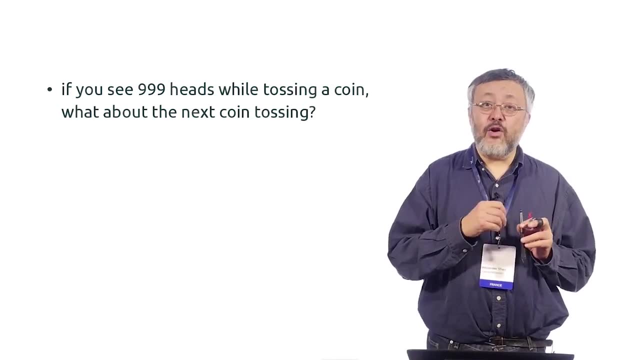 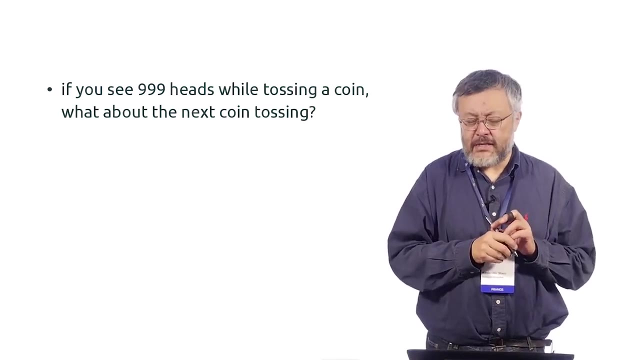 because model and real world is real world. so imagine there is a movie- Rosencrantz and Guildenstern are dead, I think it's called- and this movie starts with a long scene when one of these two guys make a coin tossing many times and it's always head head. 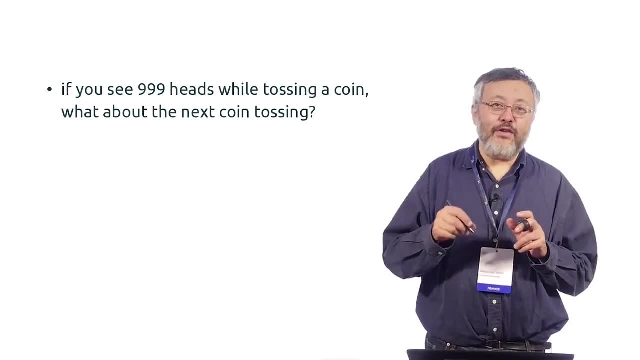 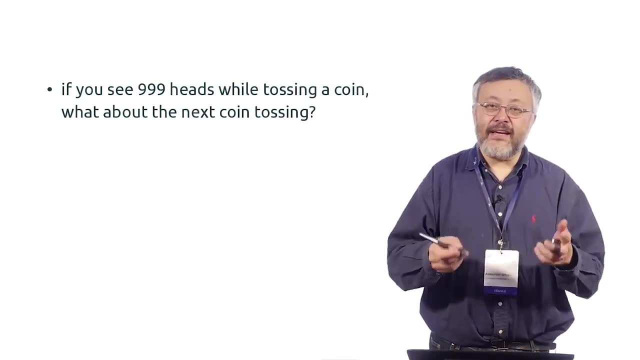 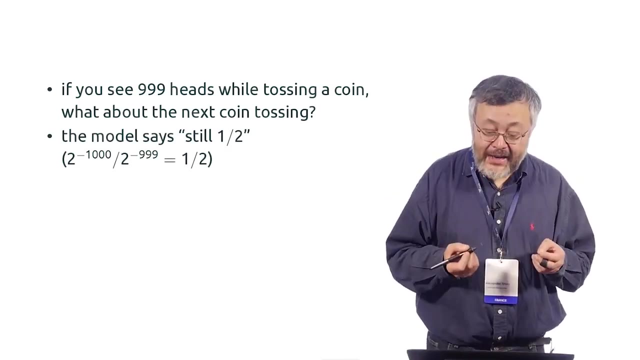 or maybe tail, but just the same result many times. and he becomes worried and you watch this movie and you see that it's head, head, head and so on. so the model still says that after you see 999 heads, the probability of the next head. 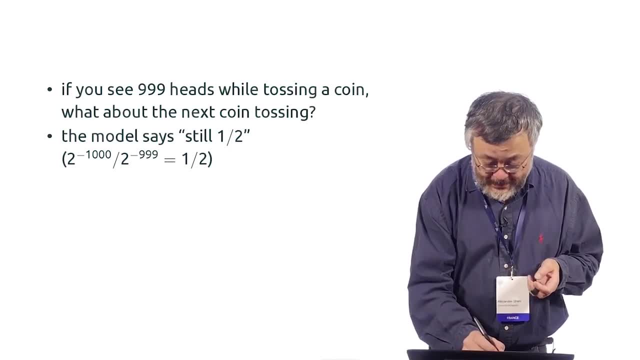 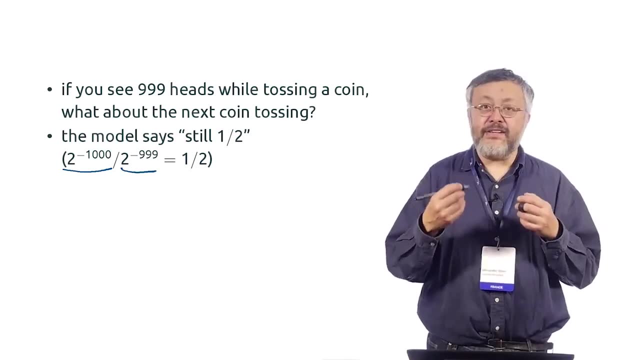 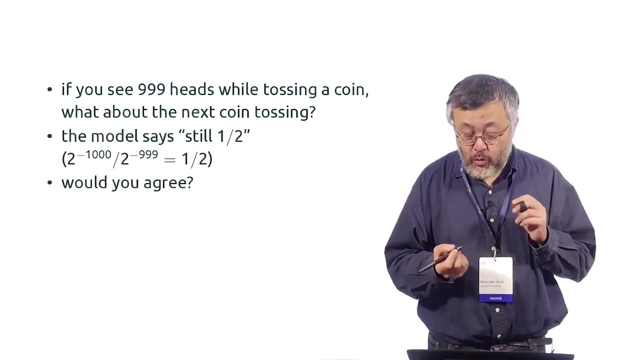 is just 1 over 2 because you can compute the probability of 1000 heads and this probability to have 999 heads. so it's still 1 over 2. but in the movie probably you will have different feeling. why you have this feeling, why you disagree with the model. 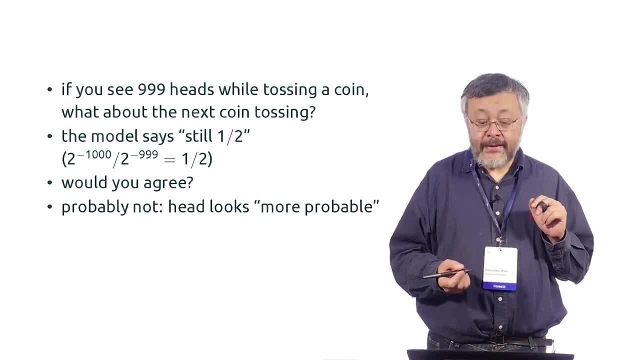 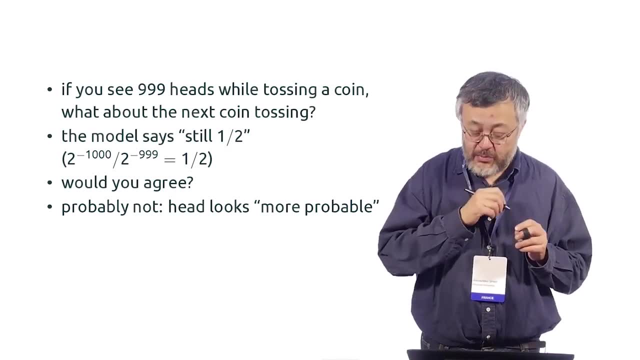 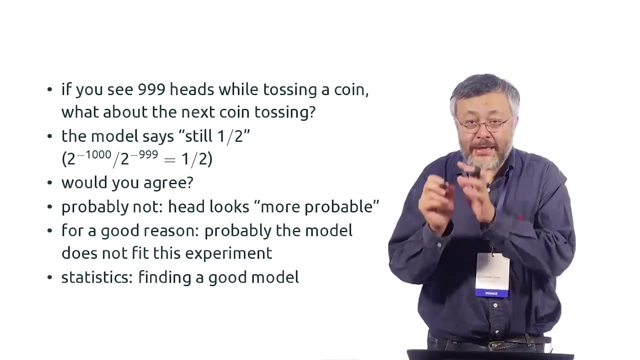 probably you will disagree, and the reason why you think that the head looks more probable is not because in the model it's more probable. it's because you've been starting to think that the model doesn't fit the experiment. so there is probability theory and there is statistics. 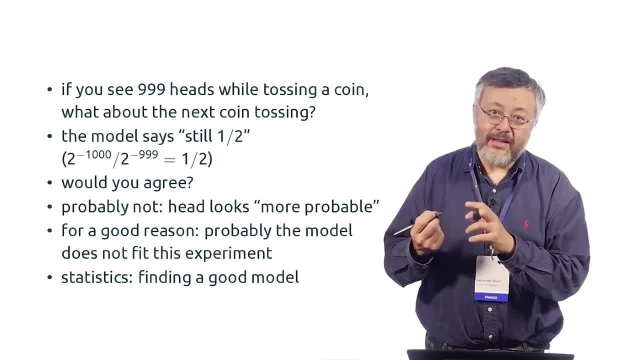 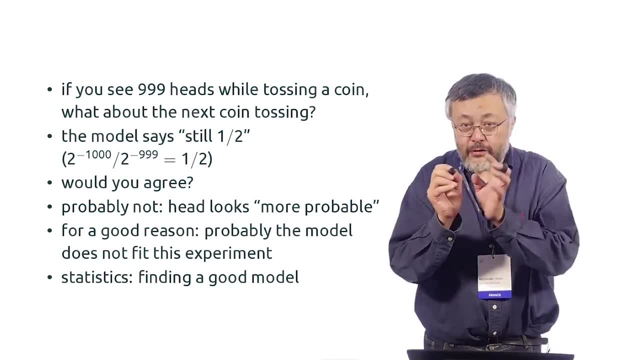 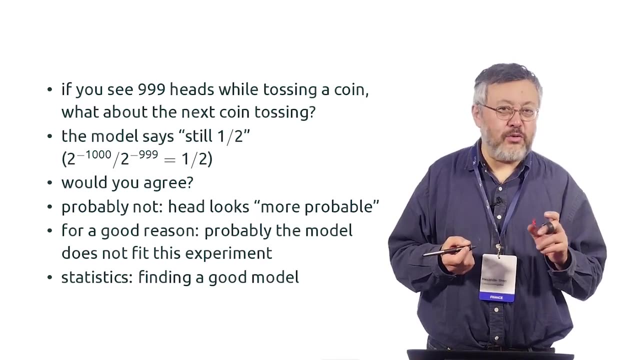 so probability theory somehow studies what are consequences of a given model and statistics tries to find a good model for experimental data. so there is a kind of separation between them. so in this case statistician would say the model of fair coin is not a good model, you should look for a better one. 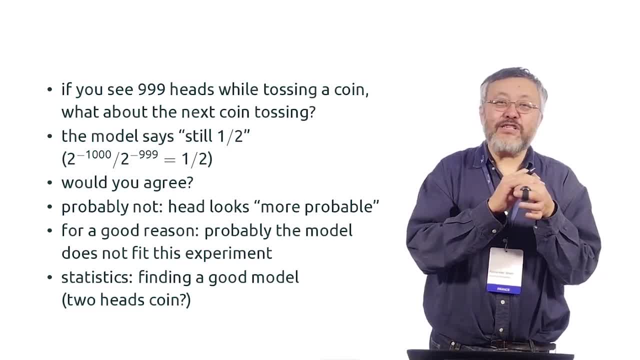 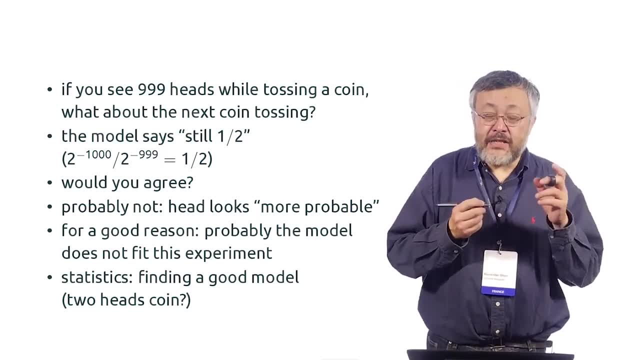 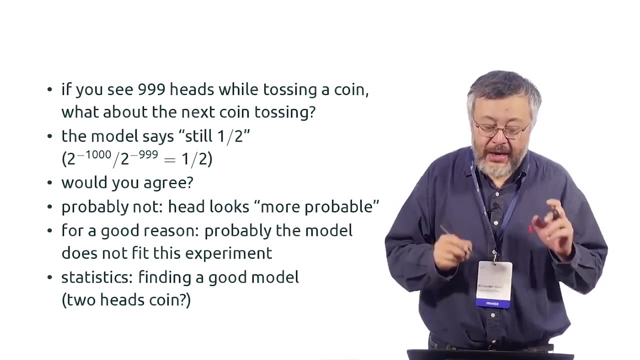 and the better one is. just the coin has two heads. I don't remember whether in the movie somebody tried to check, probably not, and this is a bit strange. so statistician will try to find a better model. but if we assume that, if we assume this model, 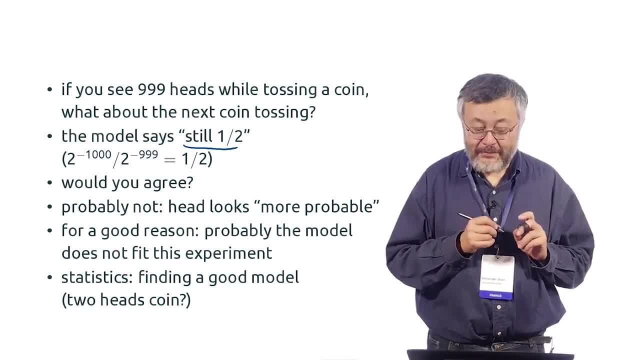 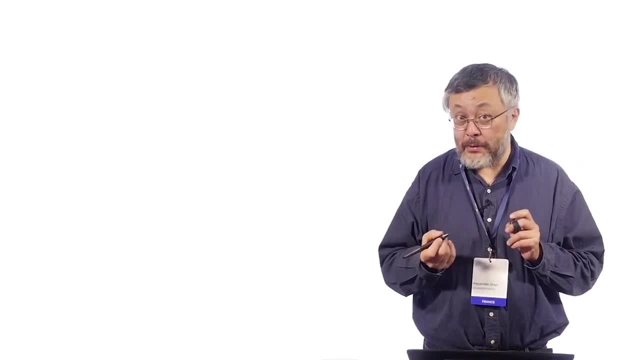 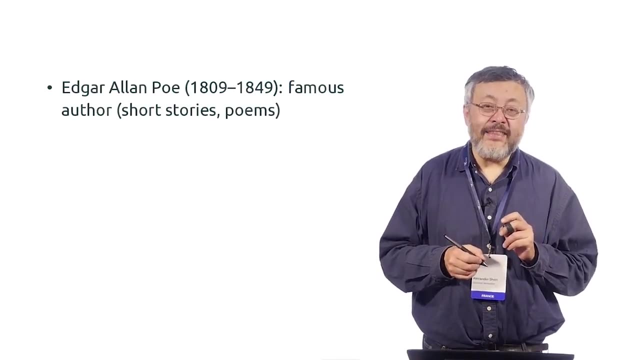 in this model we have still probability one half. and now there is a very strange story about an American writer. probably you know him. it's from 19th century. he is famous author of short stories. I think he was one of the first authors of detective stories. 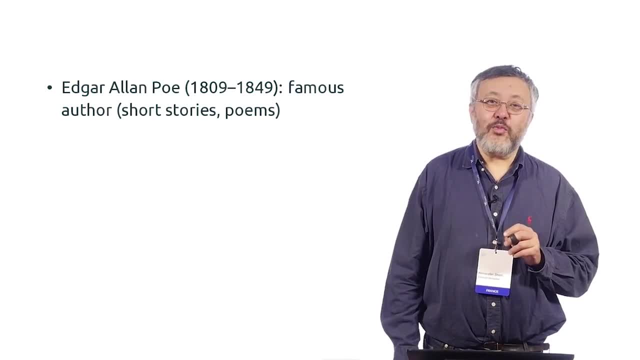 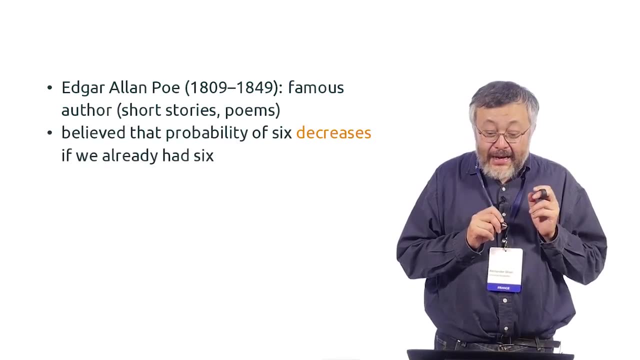 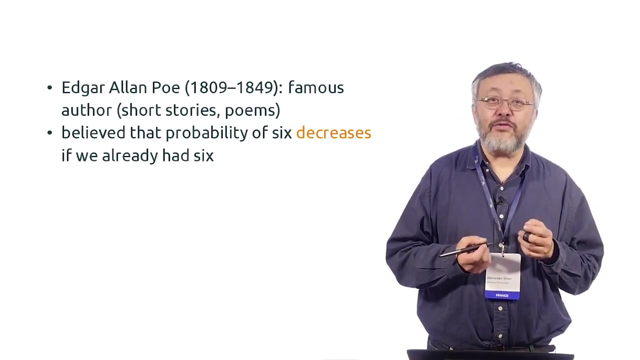 and also he is well known for a poem about a raven which always says: nevermore, independently of what you ask this raven, and it seems, at least if we believe, if we take seriously what he writes in one of the stories, it seems that he believed 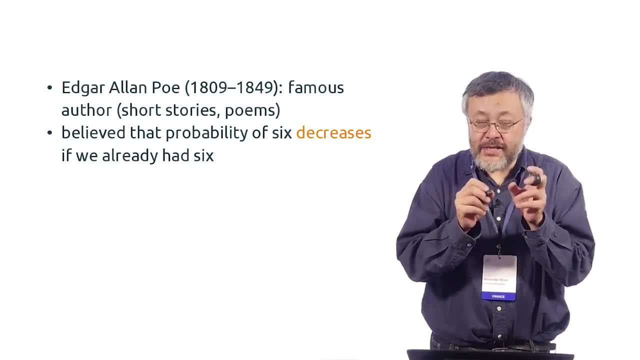 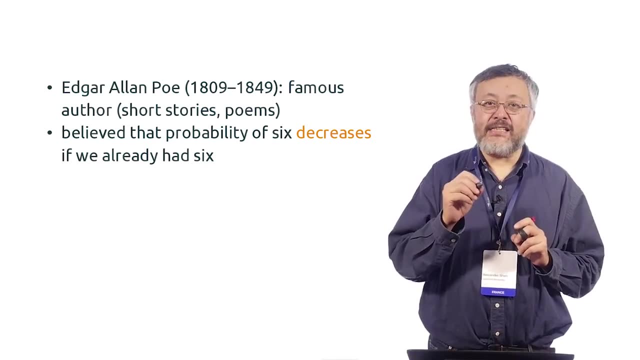 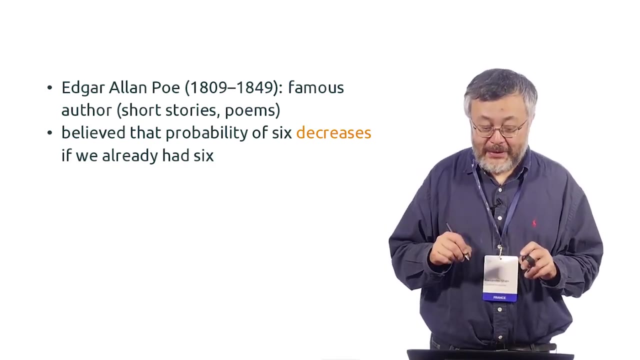 that if you see some probability of six, if you see six already, it decreases the probability to get it another time- not increases, as in our story about coin, but he believed in the opposite direction- and decreases the probability. and what is even more strange, maybe kind of mystification. 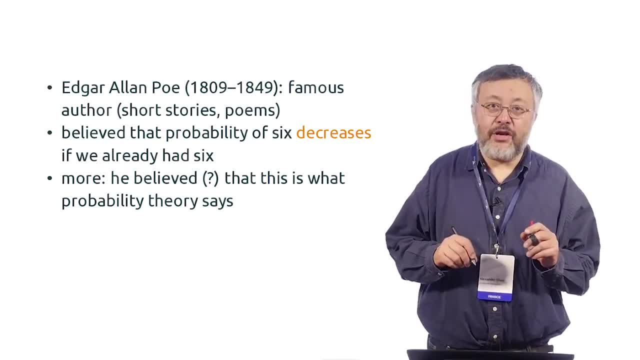 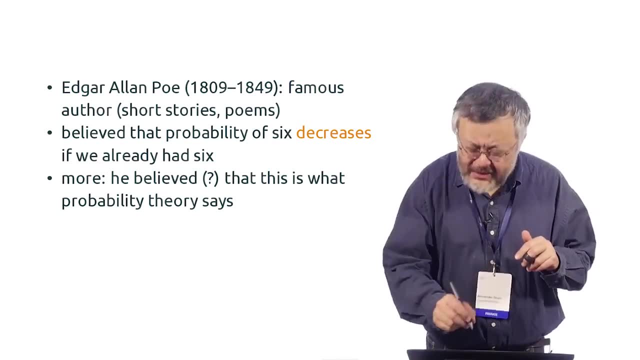 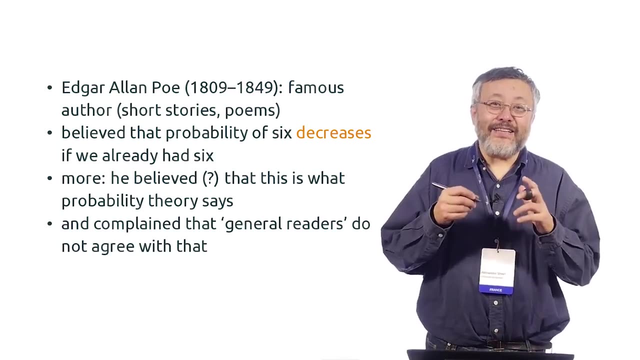 I don't know, maybe just a joke, but in the story it's written quite seriously. I will show you the quote. but it seems that he believed that this increase, this decrease, is just what probability theory says and he complained that the general readers, as he says this: 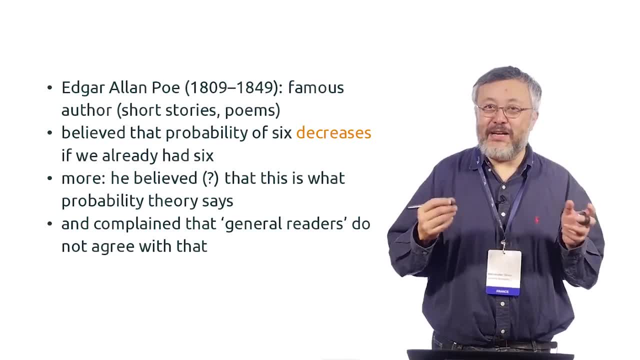 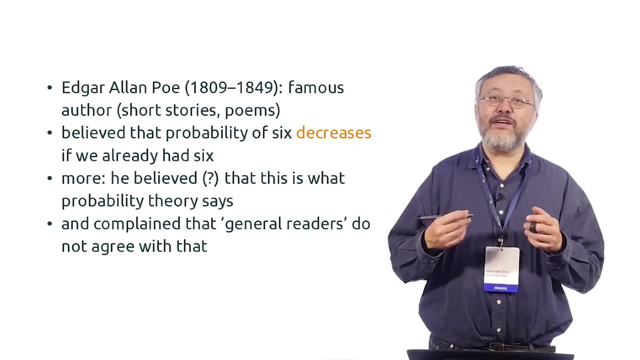 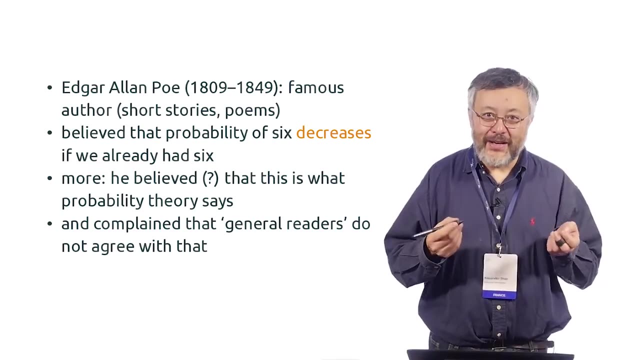 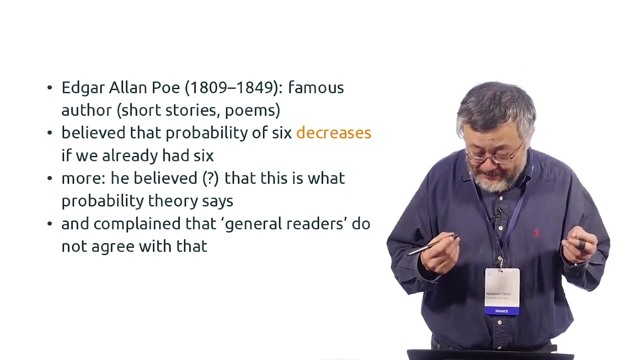 is just what probability theory says. so everything was mixed in his explanations. so the correct understanding was considered as something what general readers believe, because they are not aware of mathematical theory and some wrong thing was claimed to be a result of mathematical theory. it looks very strange, but it also reminds. 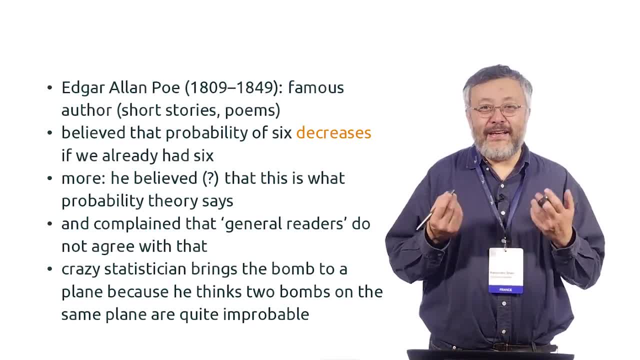 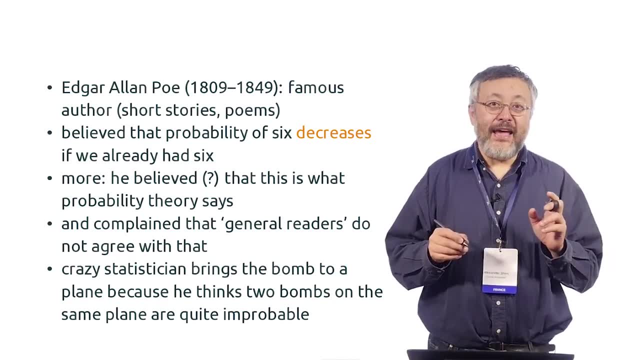 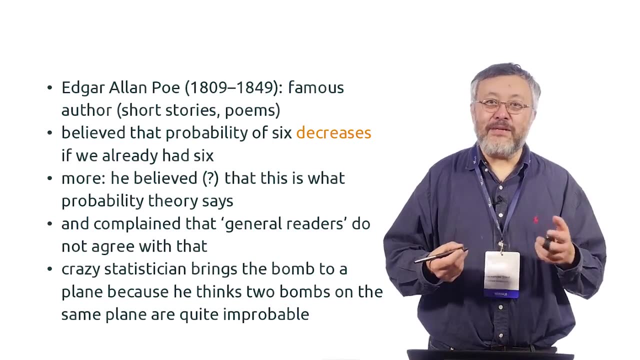 a joke that a mathematician who computed the probability to have two bombs in a plane and decided that probability is extremely small, it can be ignored. and then he decided that you can bring one bomb yourself and then just keep it, and then the probability to have another bomb. 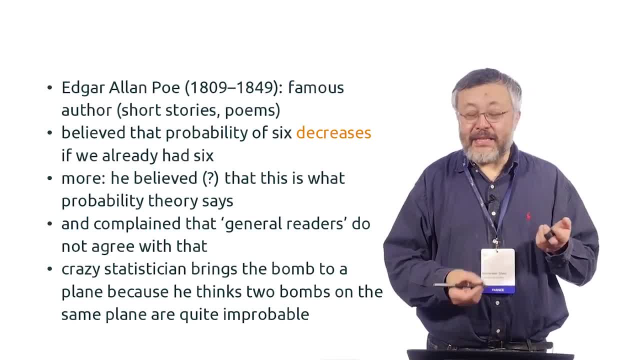 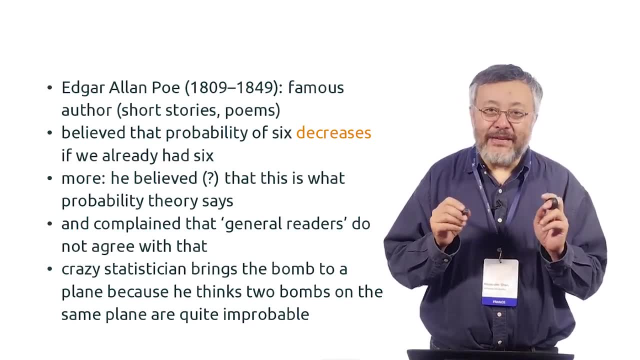 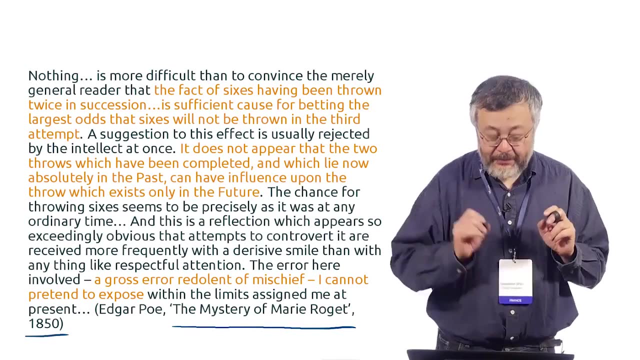 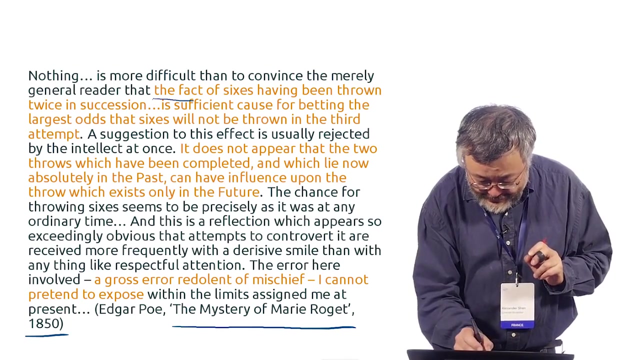 and to be in danger is extremely small, but of course it's a wrong reasoning. but now I don't want you to believe me, I just want to show you the quote. so this is for this, for the story, a detective story. and here is this statement, the fact. 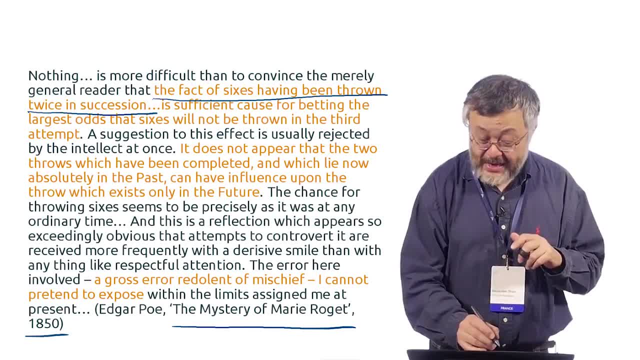 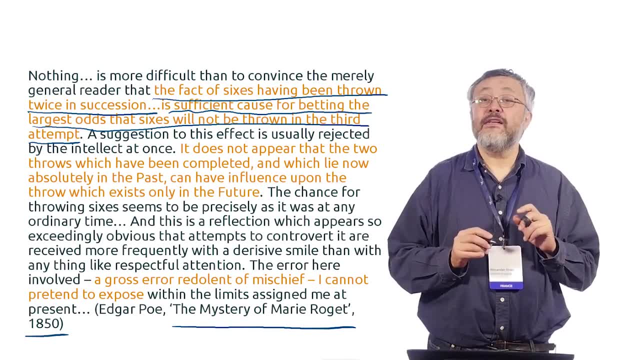 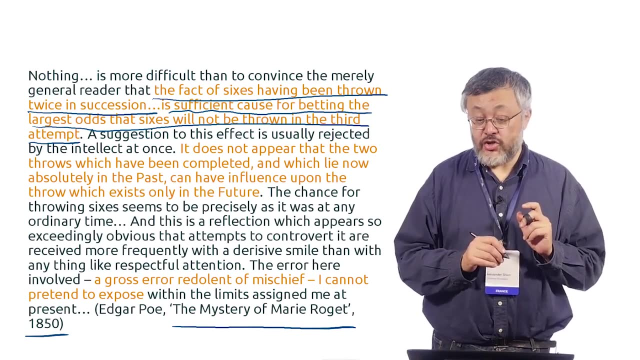 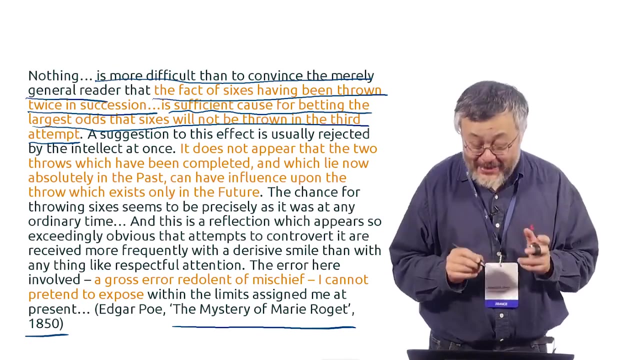 if you see already twice six, then, says Mr Poe, it's a reason to believe that third six will not appear. sixes is the reason to bet against the third six. strange, moreover, he claims it's difficult to convince the general readers and indeed he explains why the general readers. 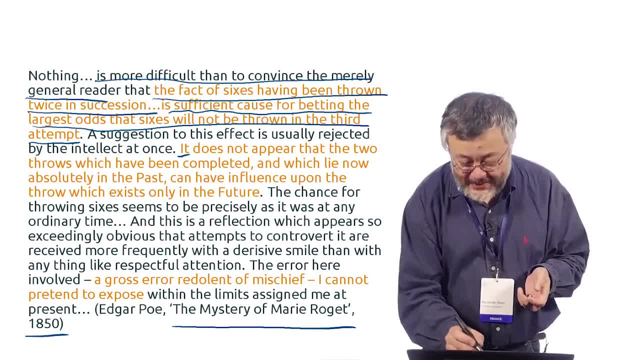 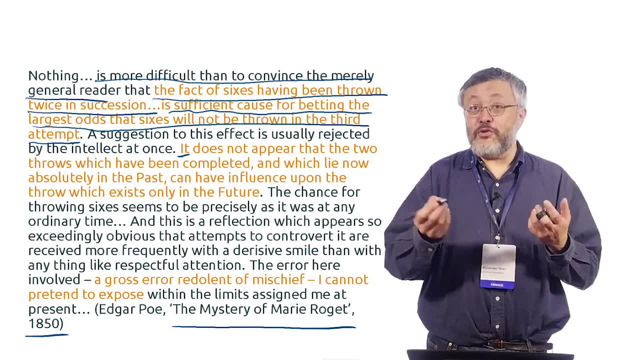 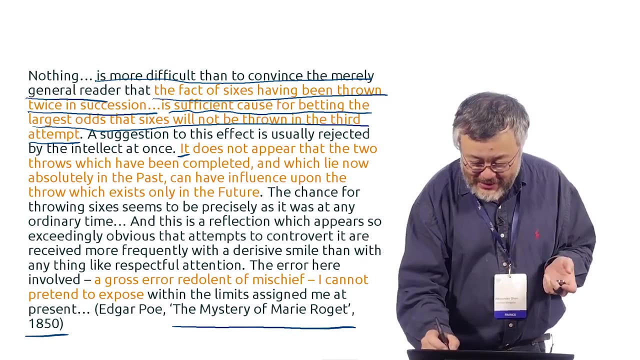 do not believe in this. and he says that if you make two dice, two sixes, they are in the past, so to say, and then you make a new experiment and why the previous experiment can influence the new one. so this is explained very convincingly, but strangely. 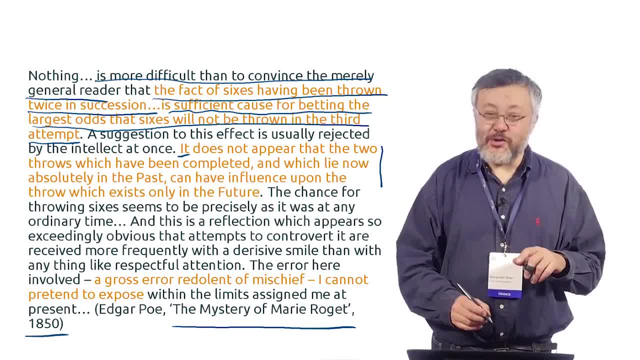 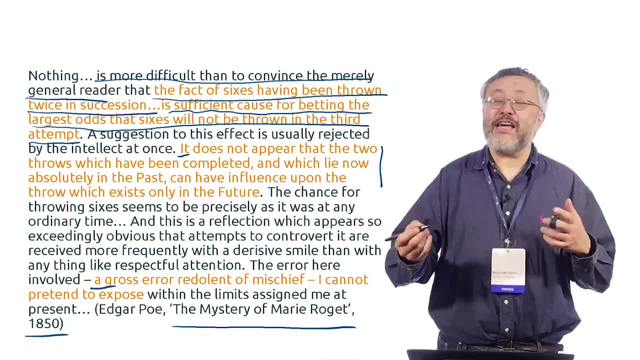 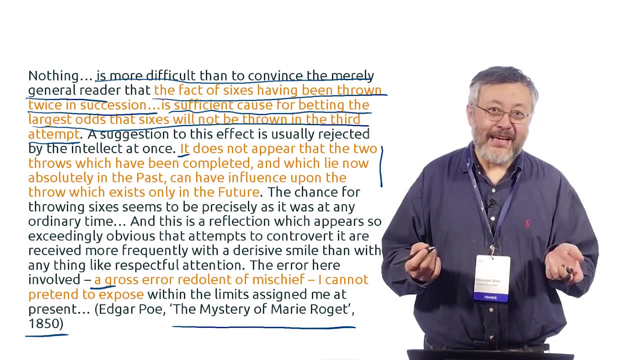 Poe believes that this explanation is an error and of course he cannot explain. I don't know. he doesn't want to explain it and he just says that look, theory says it's an error. I have no space to explain it and often when people say things like this: 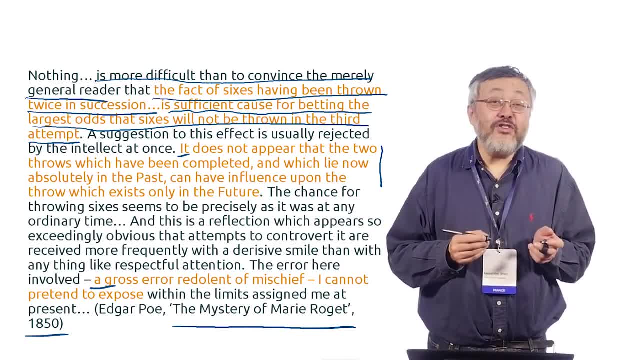 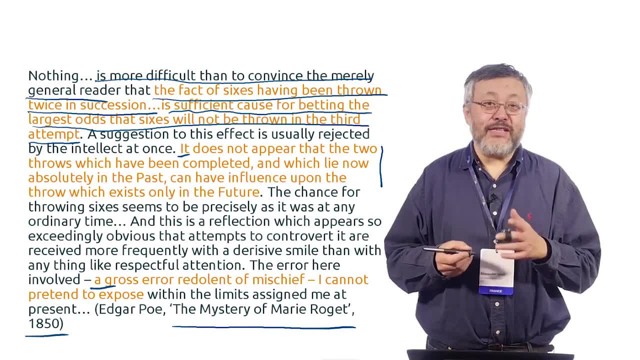 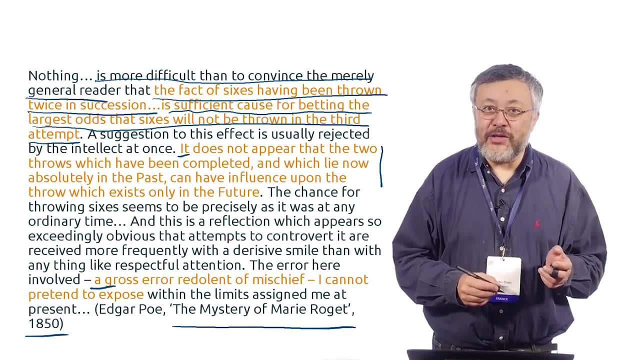 it's just because they cannot explain it and everything is mixed here and I don't know what the serious scholar thinks about this. was it a joke or did he really believe in this? anyway? but I just found this while reading the novel and it's funny and so I showed it to you. 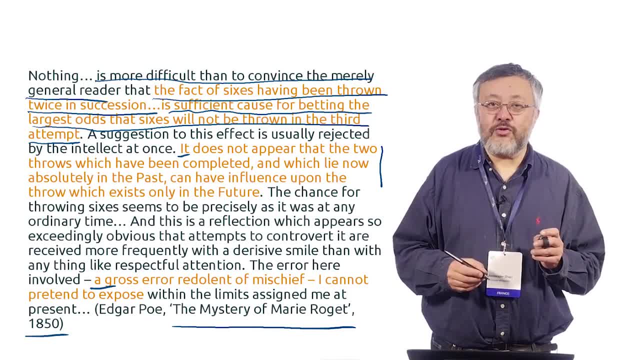 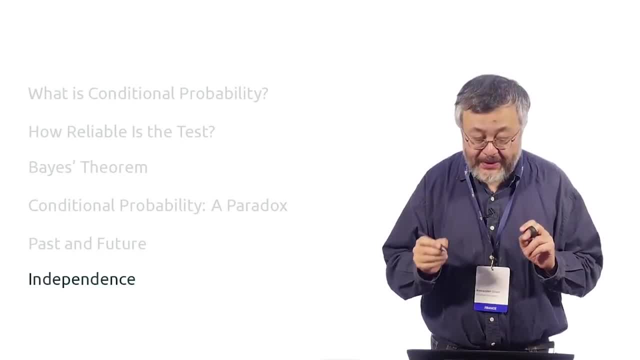 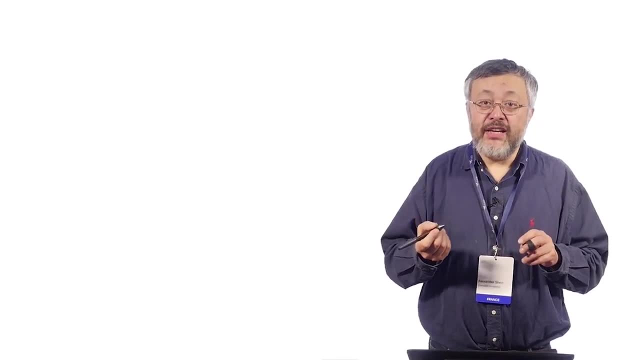 but I don't know what really this all should mean. now we came to our goal, so to say, in this part: the notion of independence. this is a mathematical notion of independence, and this word is used in the normal language in many different ways and they are not identical. 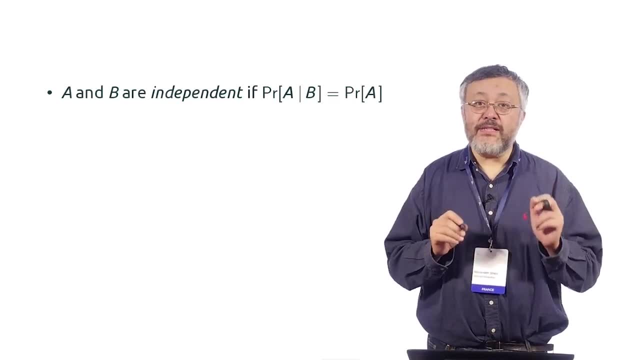 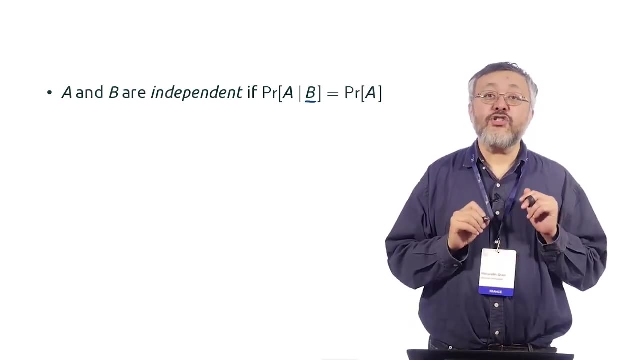 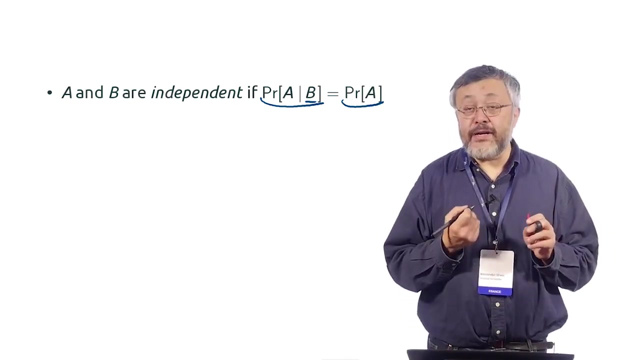 with the mathematical notion. I will try to explain so. first, the mathematical definition: a and b are independent. when we use b as a condition it doesn't change the probability of a, so the conditional probability is equal to unconditional probability. and if we recall the definition of conditional probability, 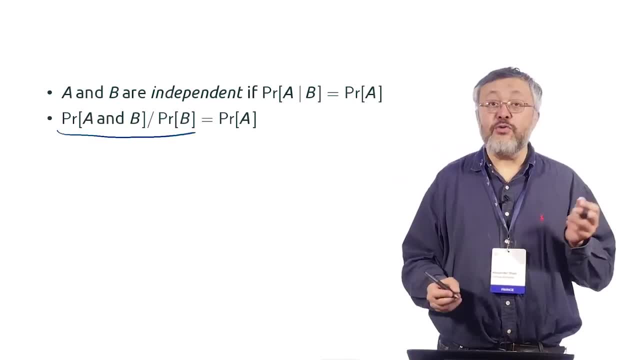 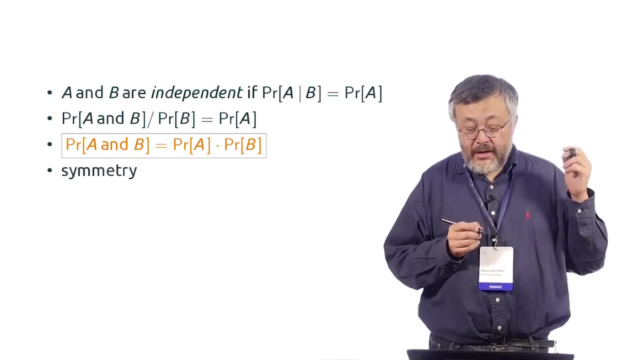 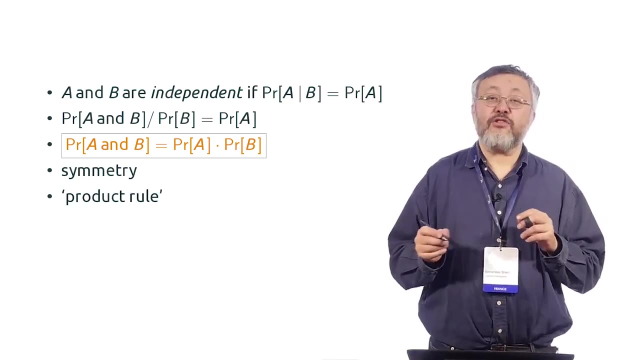 this is a fraction, this is the fraction, and we can rewrite now like this: and this is symmetric and this is called the product rule and the probability of a and b is the product of probability of a and probability of b. but it's actually somehow misleading because it's not a rule. 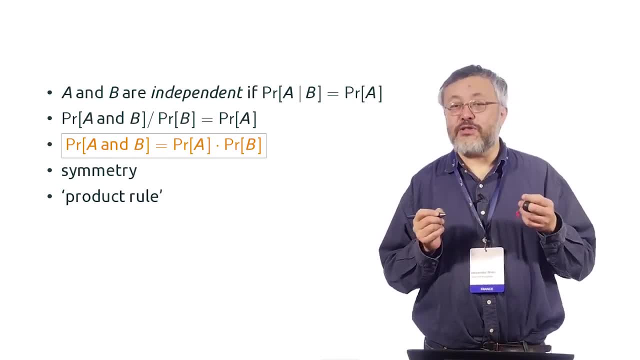 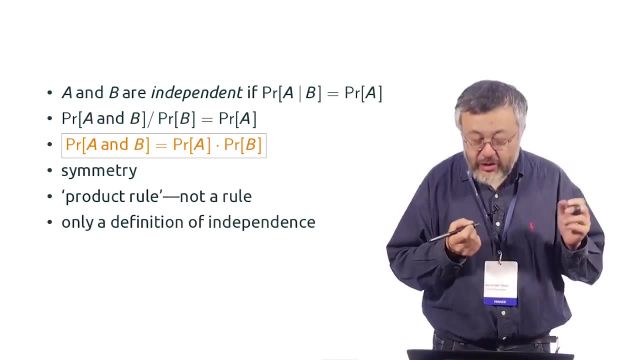 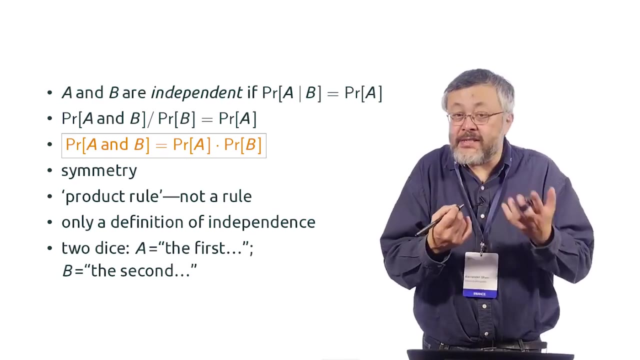 it's a definition. so if this happens, then the event a and b are called mathematically independent, and if this happens, then it doesn't happen nothing bad. so it's not a rule, actually a definition of independence. and for example, if we make, but it's somehow consistent. 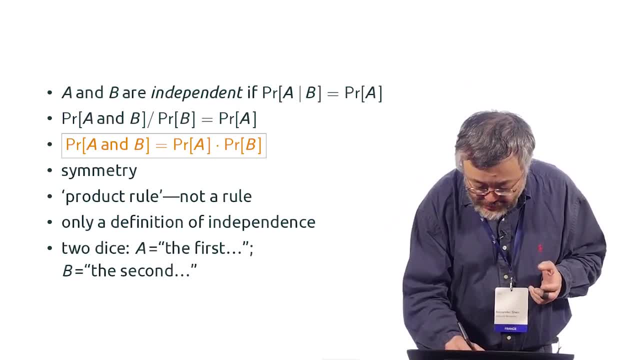 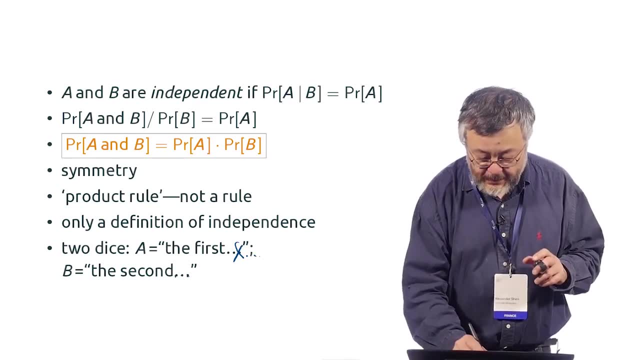 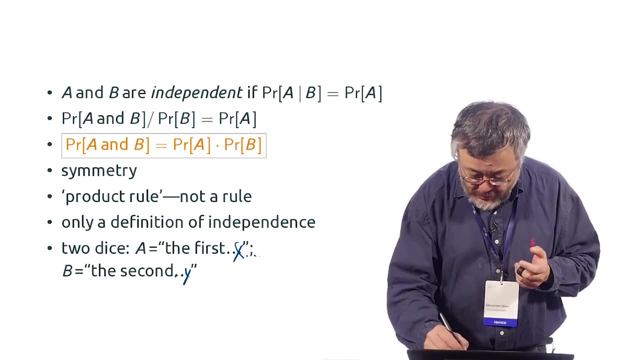 with the language used in some cases. so imagine we have two dice. a is some event about the first dice, I don't know this x something and b is an event about the second dice. you can check that they are mathematically independent in terms of our table. 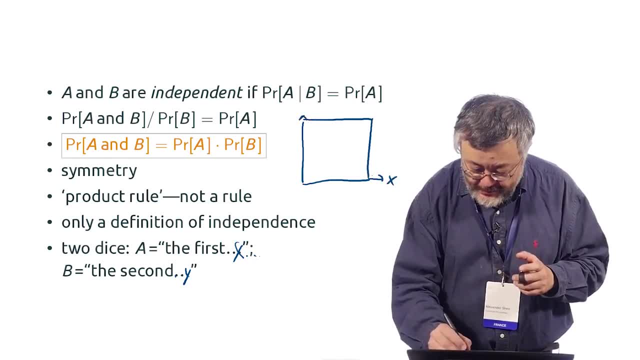 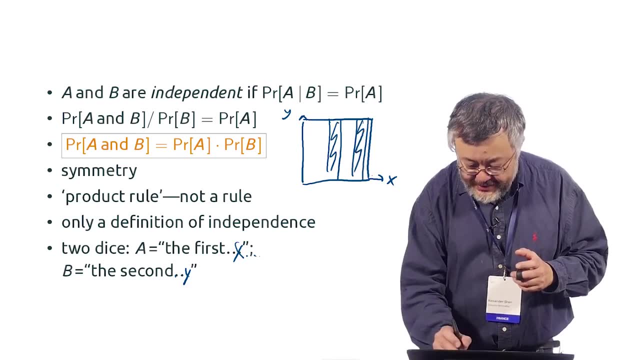 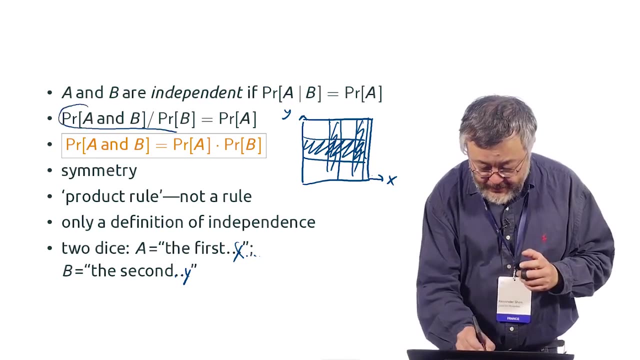 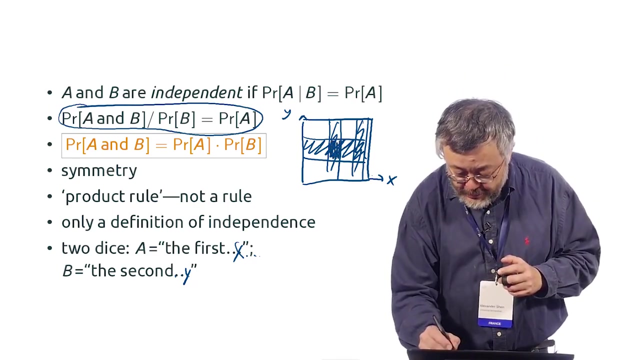 we can make a table for x and y, so events that say about x are just kind of. we select some columns and events about b, we select some rows and what is written here, that if we look at the fraction of a inside b, the fraction of these things, 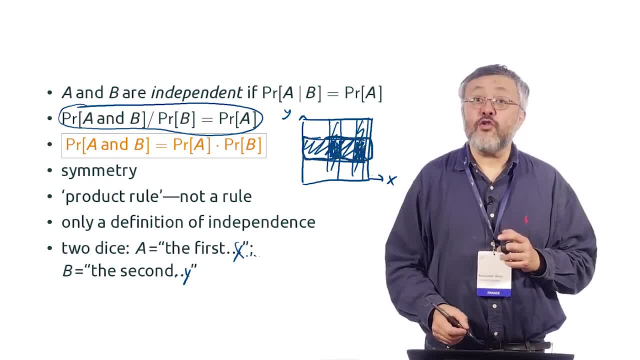 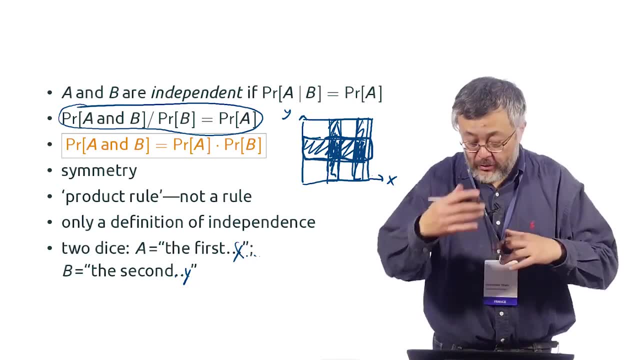 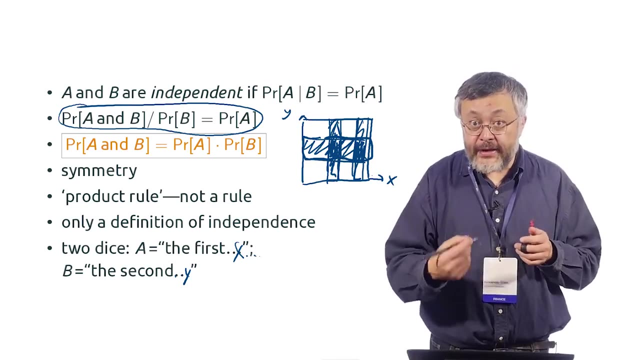 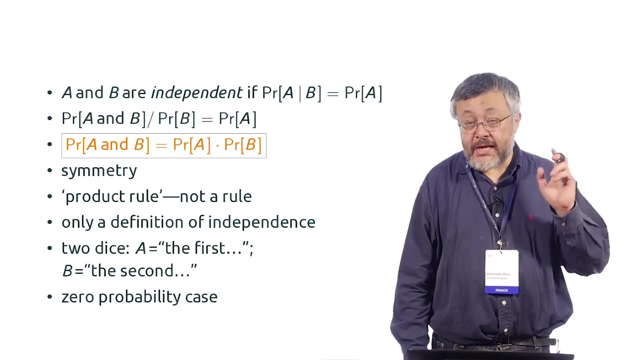 inside this it is of course the same as a fraction of b and the big columns inside the big things. so everything is proportional. so if two dice are independent in the natural sense, they give also mathematically independent events. ok, and also let me say again this strange zero probability case. 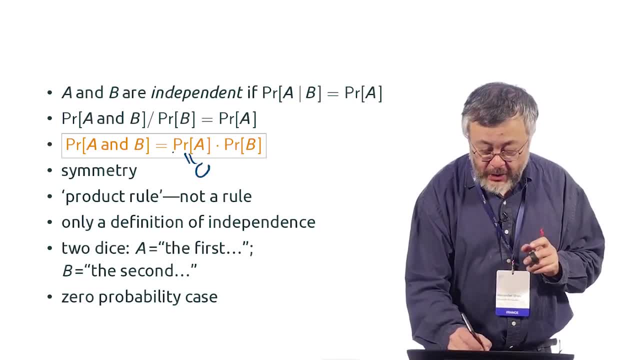 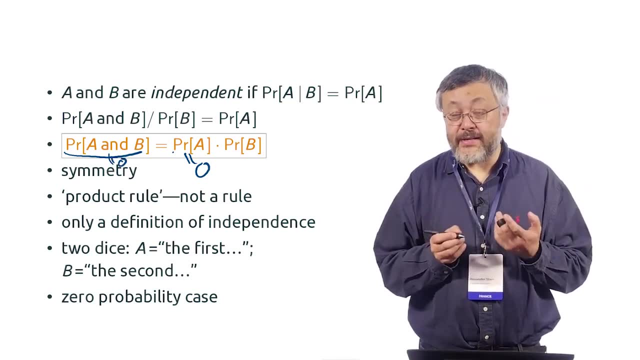 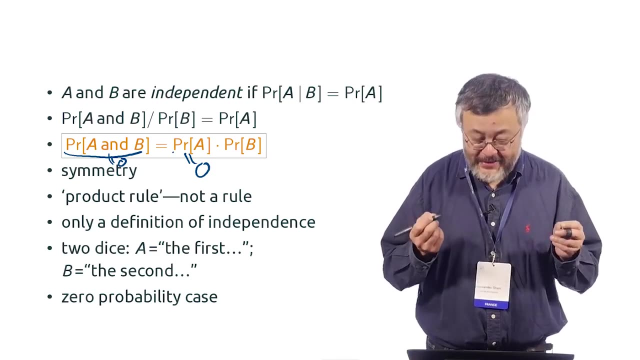 which we can ignore. but if one of the events has probability zero, then of course the end is a part of it, so it also has probability zero. so the formal definition of independence is satisfied, so the impossible event is independent with any other event, and we can look. 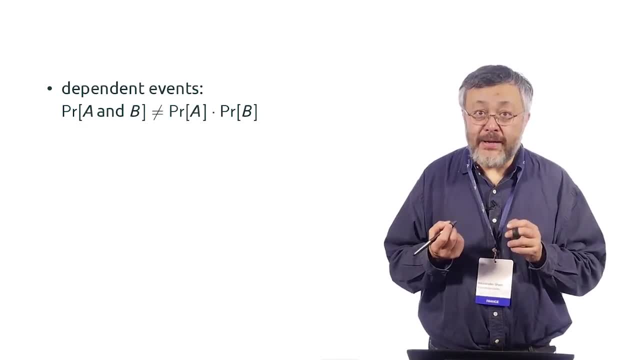 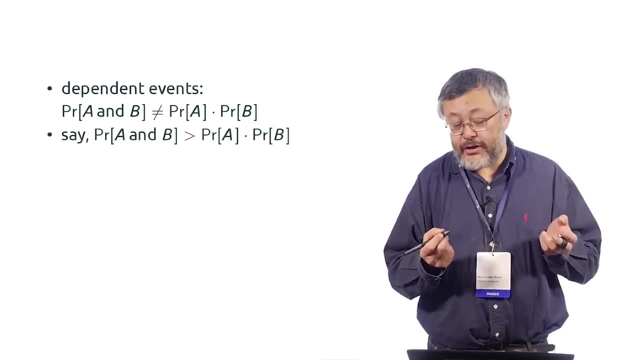 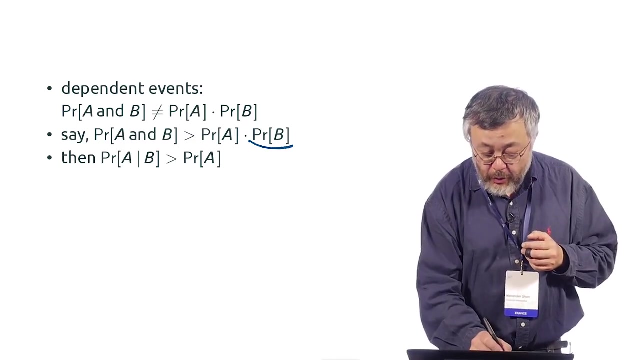 at the bias formula. so if the events are dependent, this means that this probability is not a product and it can be bigger or smaller. let's, for example, consider the case when it is bigger, which means that if we divide this by probability of b, we see that the conditional probability of 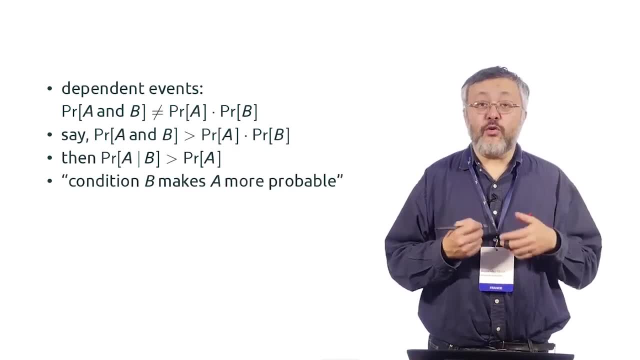 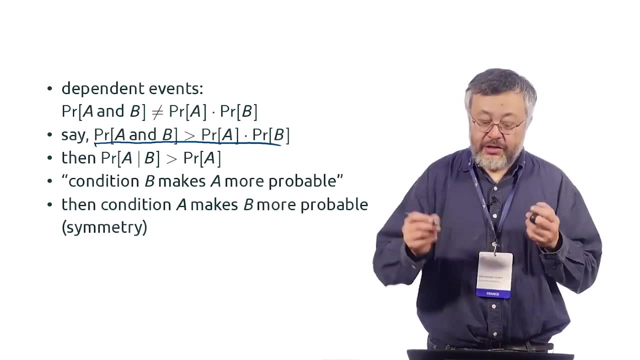 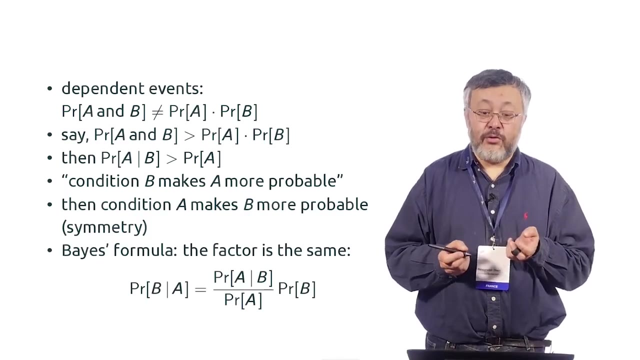 a given b is bigger, so condition b makes a more probable. and then the symmetry says: this is a symmetric thing. so the symmetry says that condition a makes b more probable. and this is exactly what we discussed in bias formula, because the factor that changes the probability is the same. 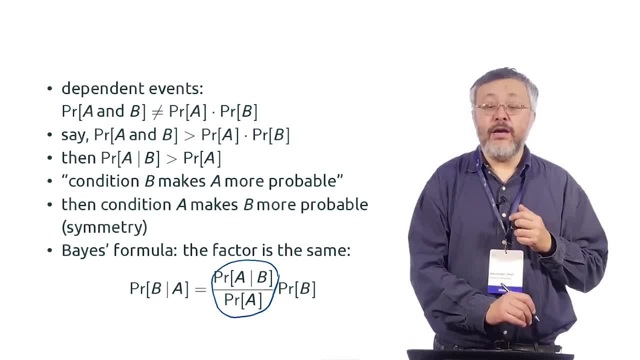 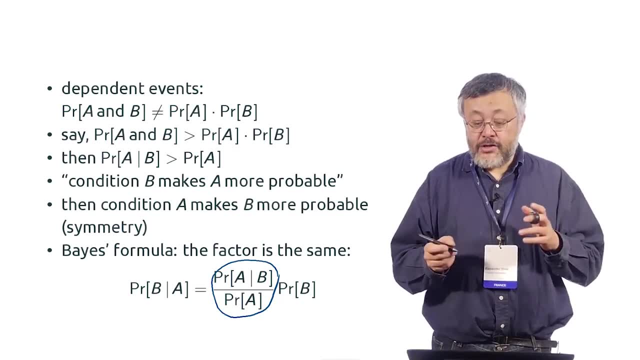 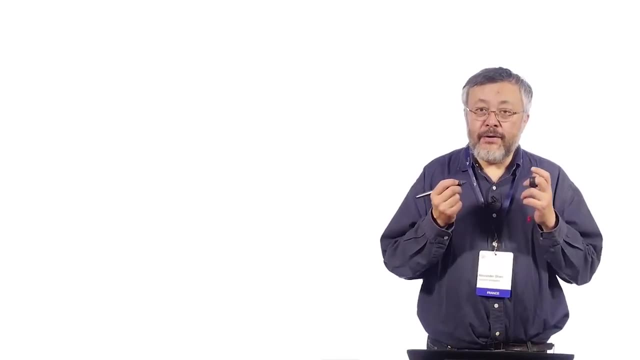 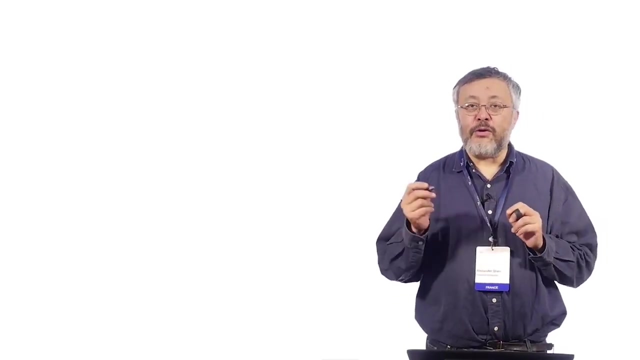 so the same factor, how b increases the probability of a, shows how a increases the probability of b. so it is just the bias formula again. so we can- now we can clearly see the mathematical notion and also we should clearly understand that it is not identical to our. 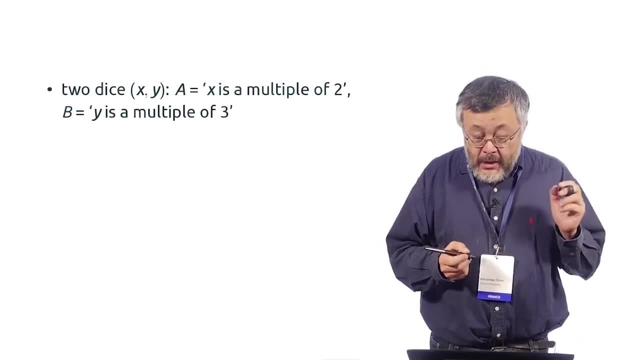 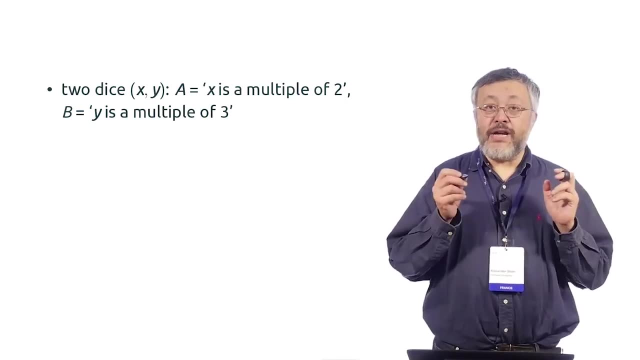 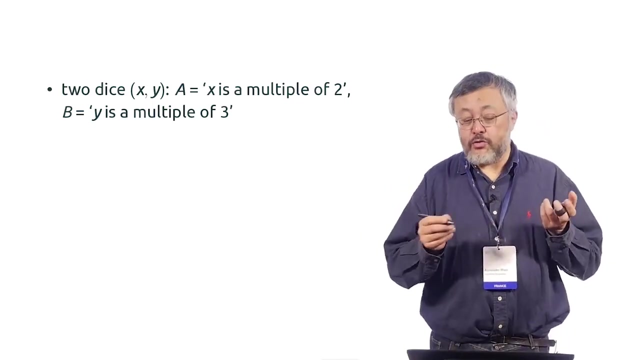 life, our language and normal life. so in both directions it is possible. so let's start with a good case. we already considered we have two dice- x and y, two numbers- x and y- appearing while rolling a dice twice or two dice, and there are two events. 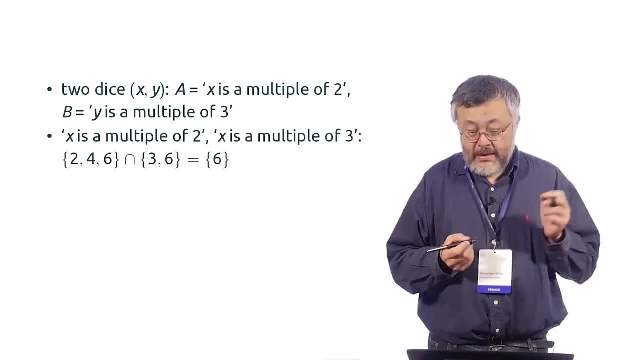 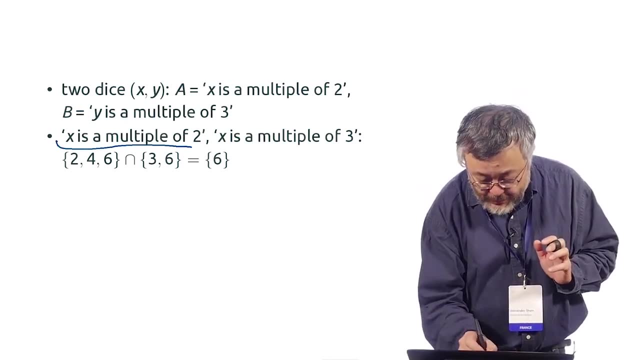 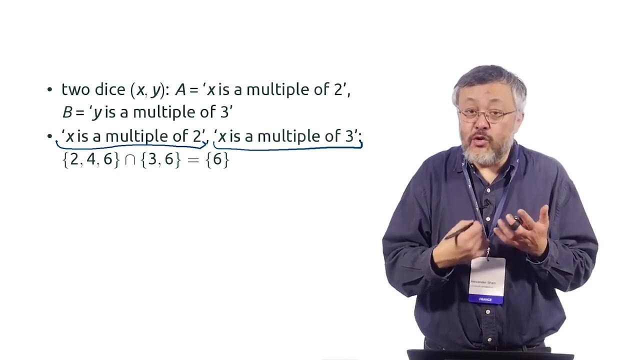 x is a multiple of 2 and y is a multiple of 3, so they are independent. only forget about the second dice. so just event: x is a multiple of 2, x is a multiple of 3 and they are also independent. they refer to one. 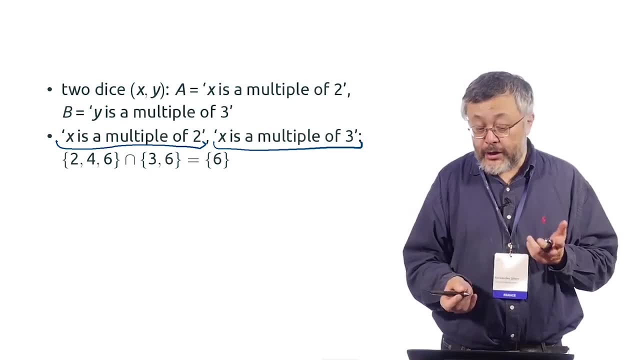 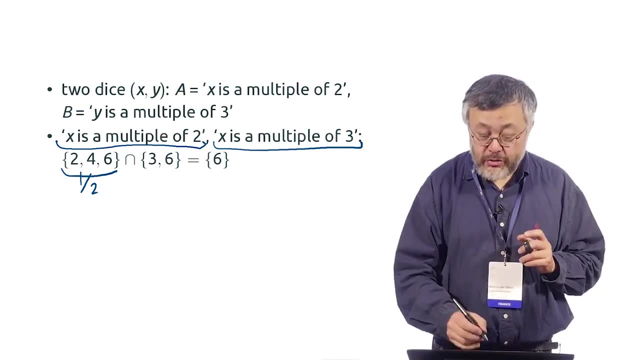 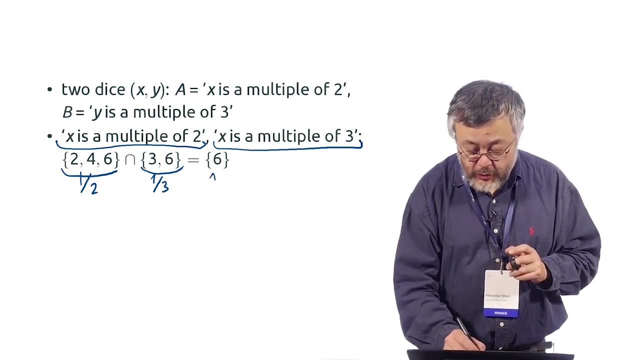 there is no reason why they should be independent, but in fact they are, because multiple of 2 is three numbers, probability is one half. multiple of 3 is two numbers, probability is one third, and the intersection is one number. so perfectly fits, perfectly well. so there is a mathematical independence. 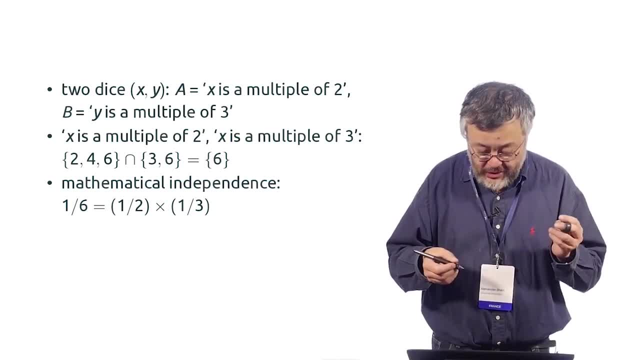 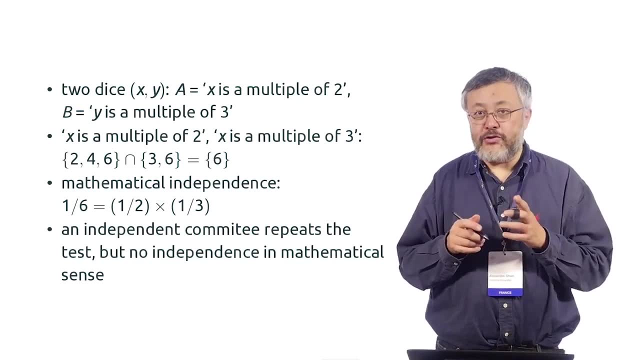 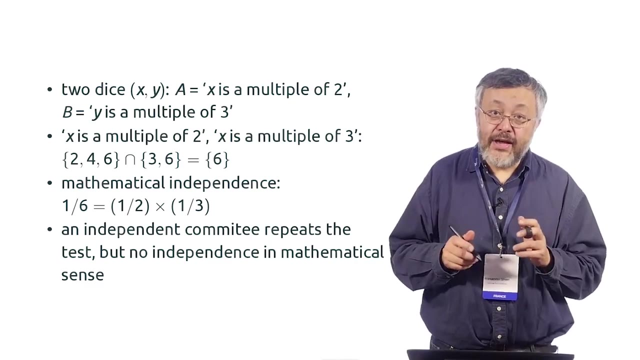 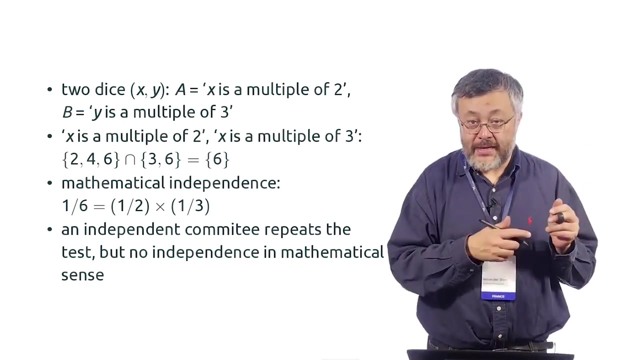 but no real life independence. and another example: when we have a real life independence. so imagine you want to pass some English proficiency test and you take it once in some organization and then you want to check the results and you go to another independent organization which repeats the test. 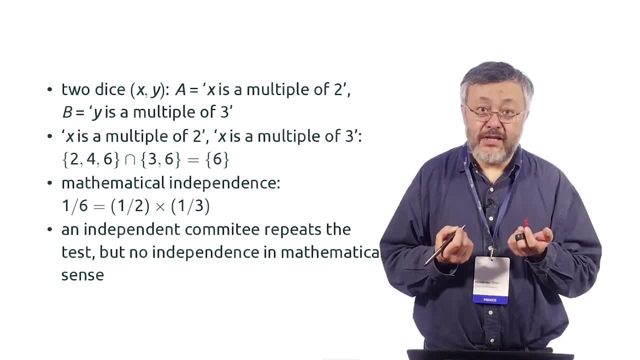 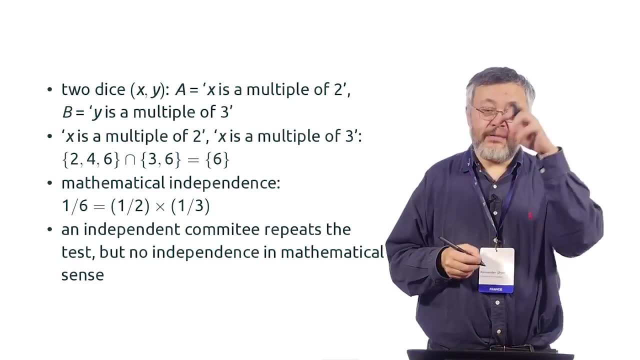 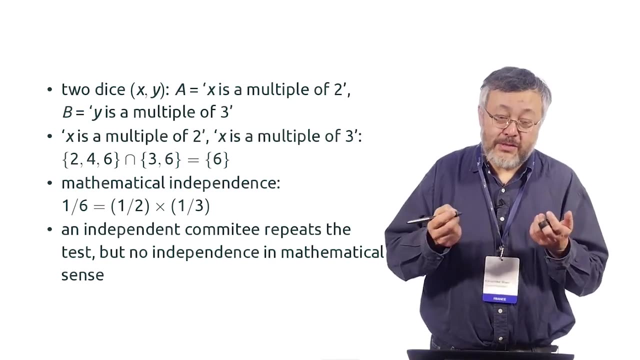 and this organization is independent in the real life sense. but of course, if you just take the statistic, if you look at many people and see whether they passed the first test or the second test, normally most of the people who passed the first test will pass the second test also. 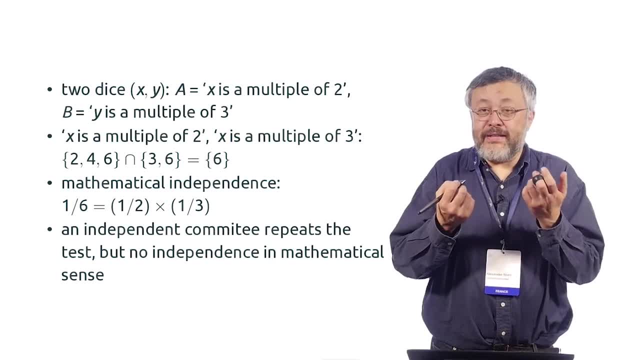 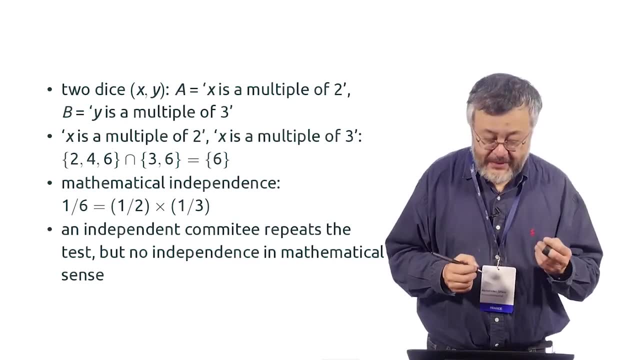 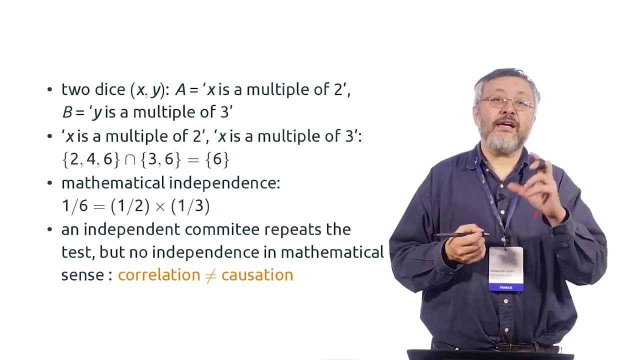 and vice versa. so even if the test is independent in the real life as a mathematical event, for a random person, taking both tests is independent and somehow it's called, it's explained as correlation. so these tests are correlated, but correlation is not causation, none of them. 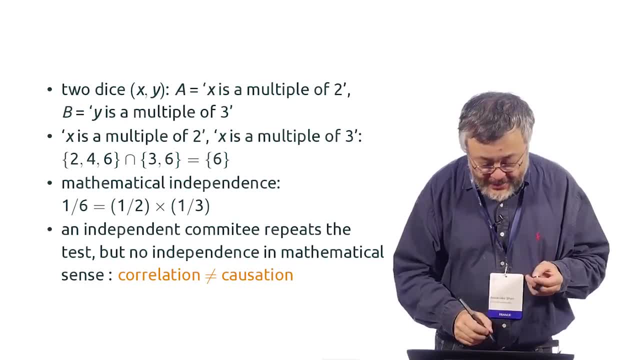 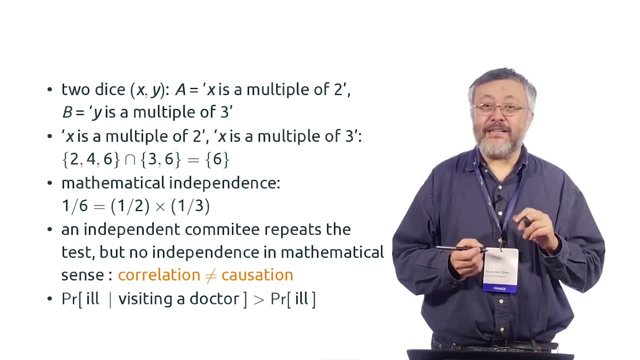 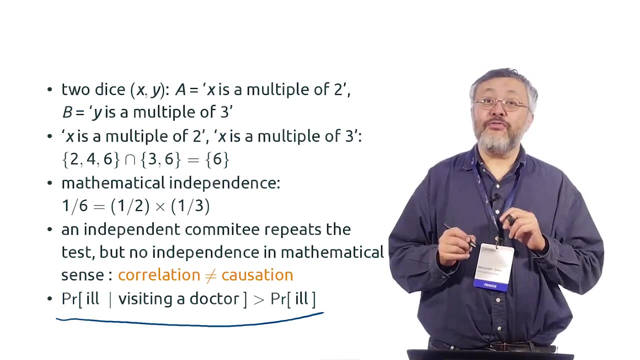 influences the other in any way. and there is a joke about a statistician- a crazy statistician- who decided that visiting a doctor makes you ill because he just computed the conditional probability of being ill if you visit a doctor with the condition of visiting a doctor and this probability 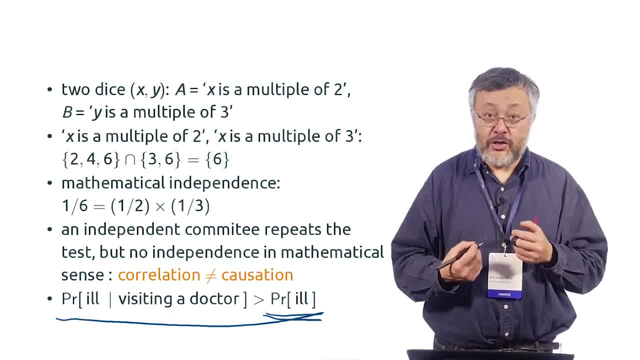 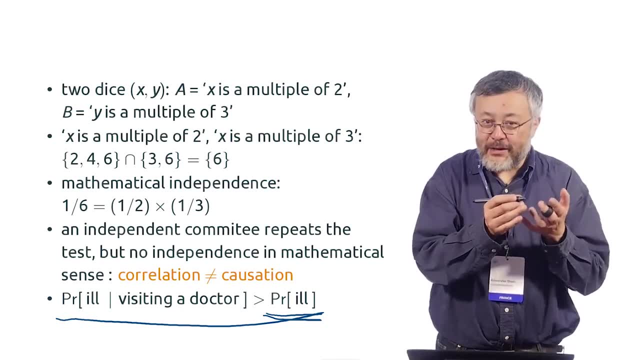 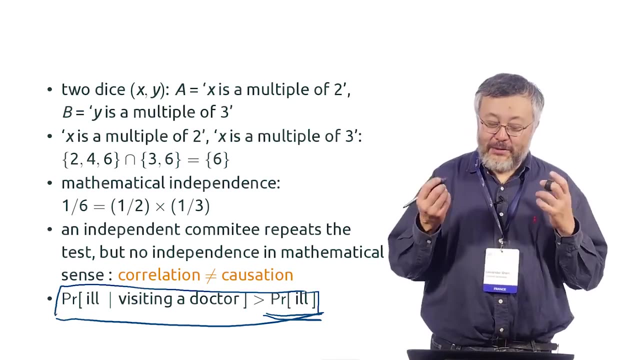 is bigger than being ill in the general population. of course, if you look at the people who come to the doctor, more of them are ill, a bigger fraction of them is ill. so it's true, but you should not. so it's true mathematically, but you should not. 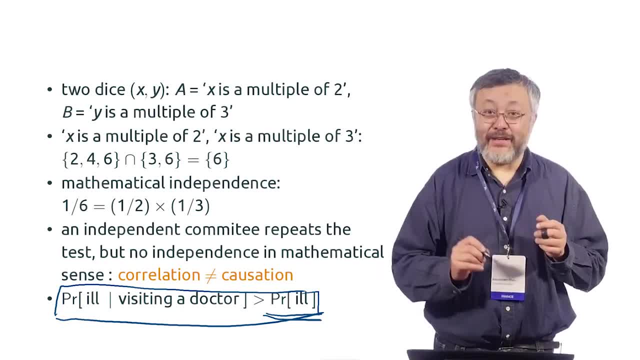 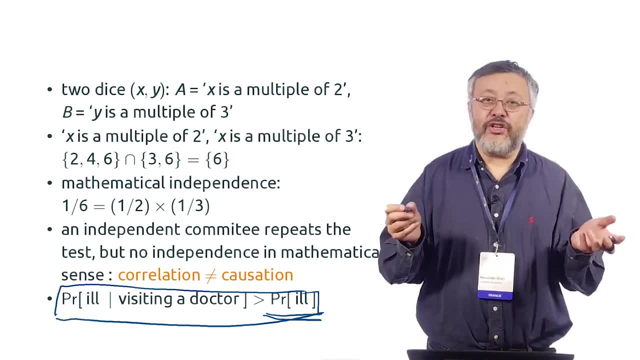 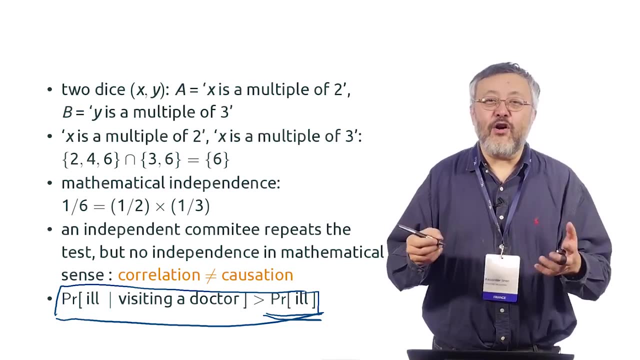 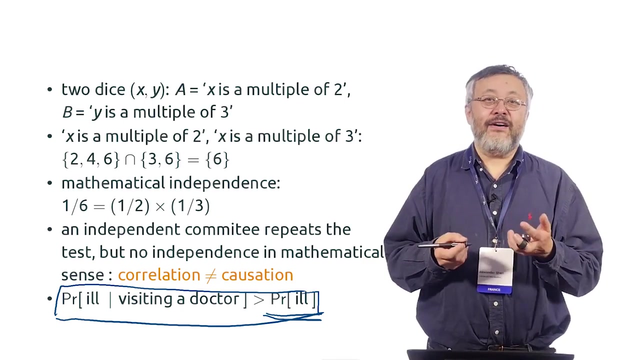 make a conclusion that visiting a doctor makes you ill, and it's actually quite often in the real life. let's consider some imaginary example. you read in the newspaper: drinking coffee increases your life span, which means that if you look at the people who drink coffee, then they live longer. than the average, but it may well happen. I don't claim anything about coffee. it may happen just because old people like coffee, so the old people make a significant part of the coffee drinking population. but that doesn't mean that one is the reason of the other one. 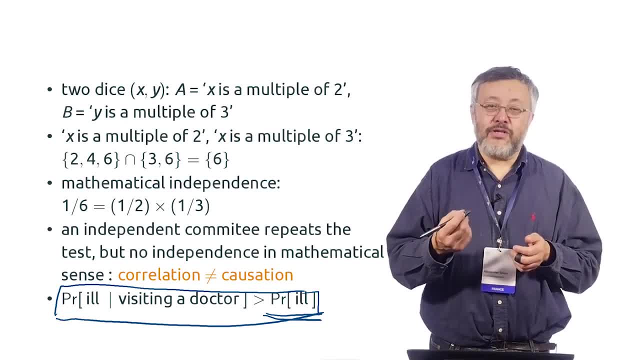 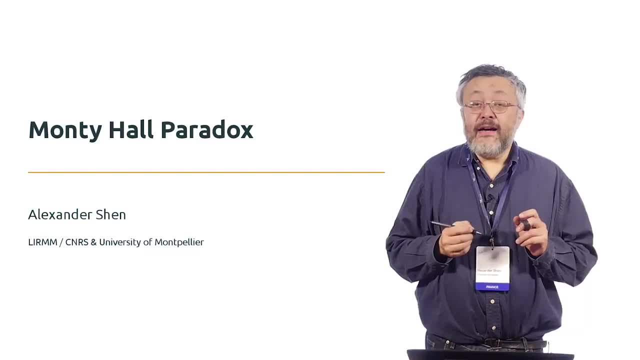 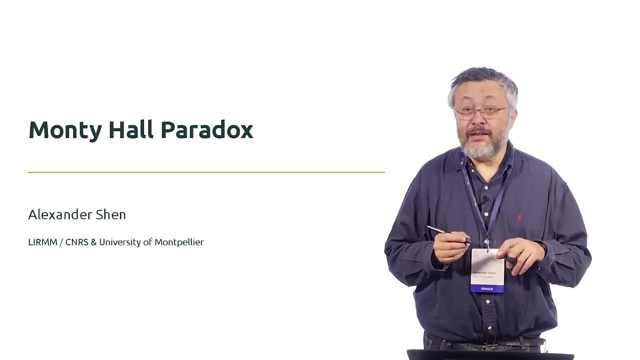 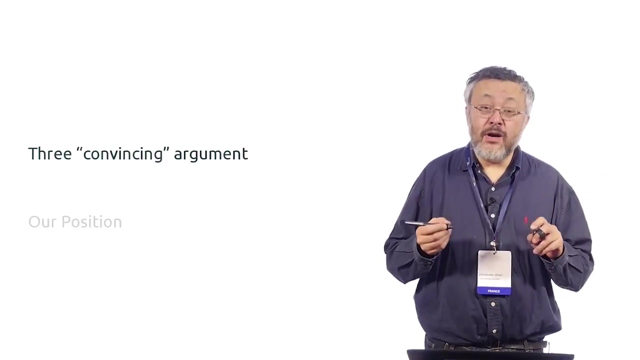 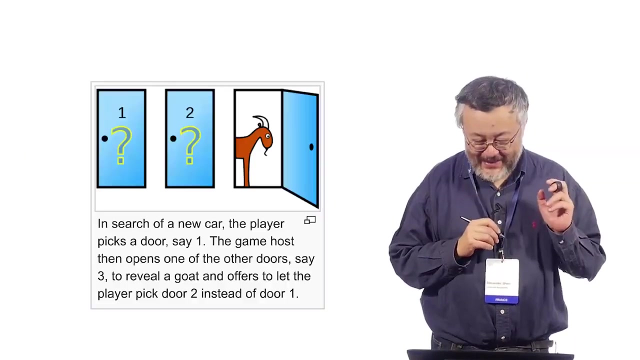 and still there is a correlation but not causation, as one can say. again this take home message. now we consider a famous, known paradox. it's called Monte Hall paradox or Monte Hall problem, and the name is because of some show of this name when this paradox appeared. 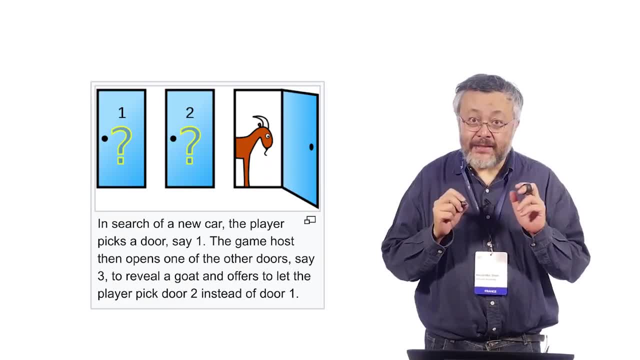 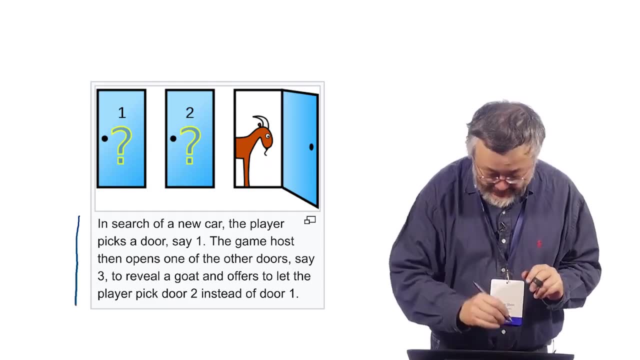 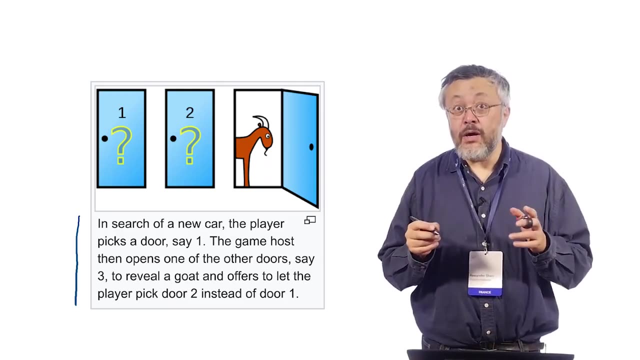 and I start with a short description just extracted from Wikipedia. there is a picture. you see this picture and you see the short description here. the story is like this: so there is a show and the player which comes to the show sees three doors and he wants to find a car. 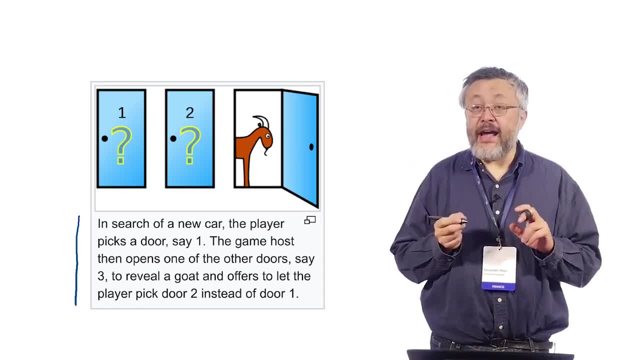 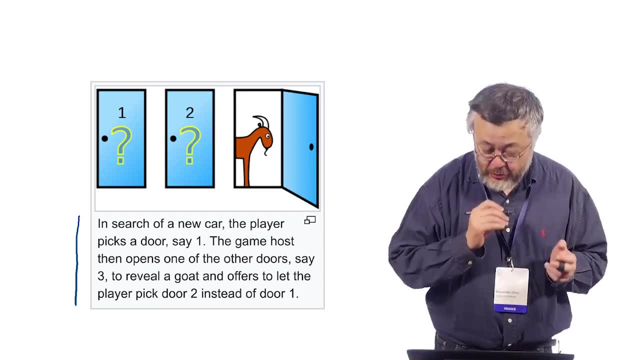 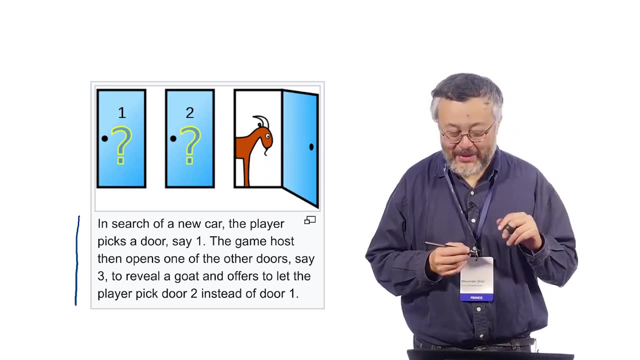 which is behind one of them and he picks a door and the game host opens one of the other doors and for example the third door, and there is no car, there is no prize for one of the participants. so then the host asks the player whether the player 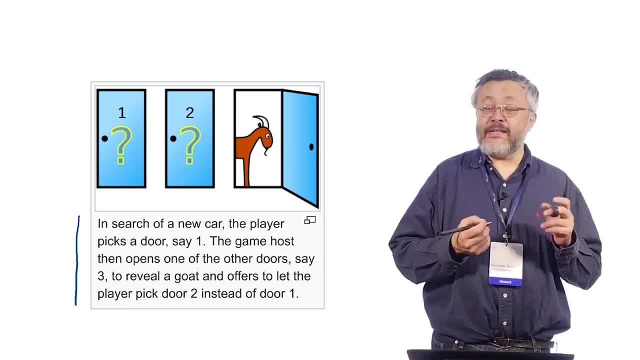 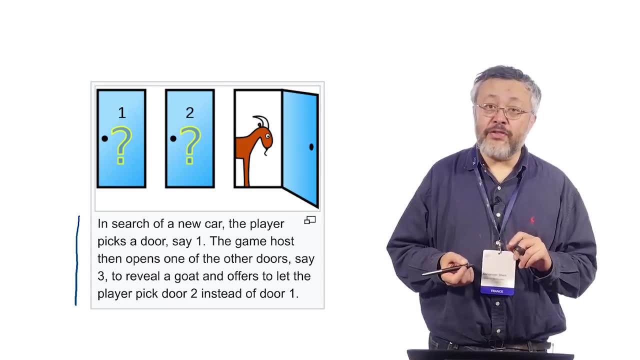 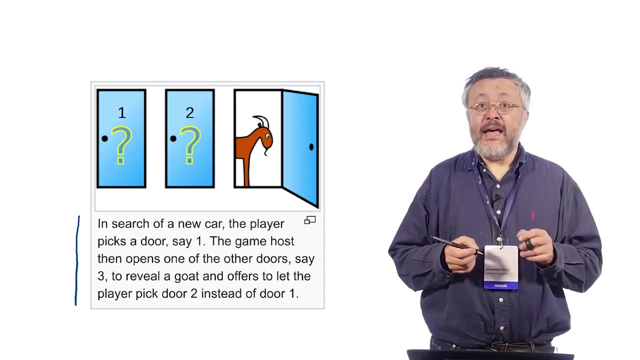 wants to keep the guess or change that. so the player is now allowed to rethink and choose not the door one but door two, and the question is whether the player should do this or what is the best strategy for the player and to make the game more clear. 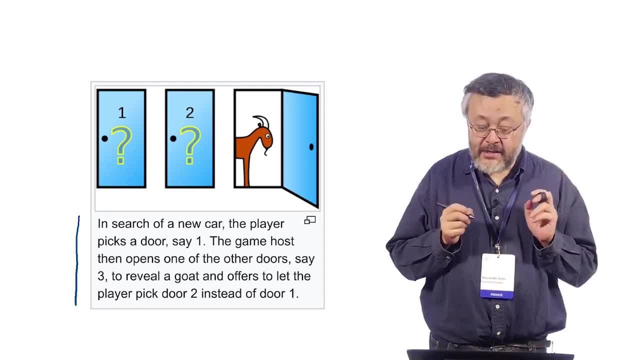 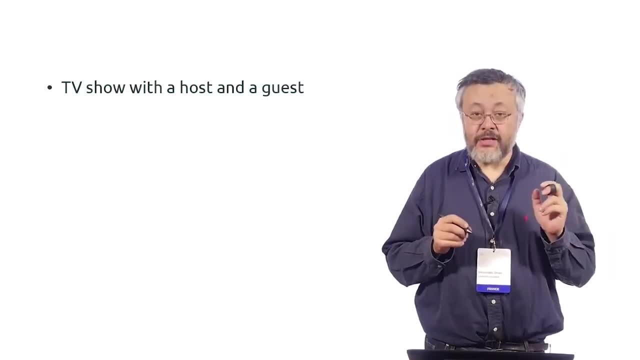 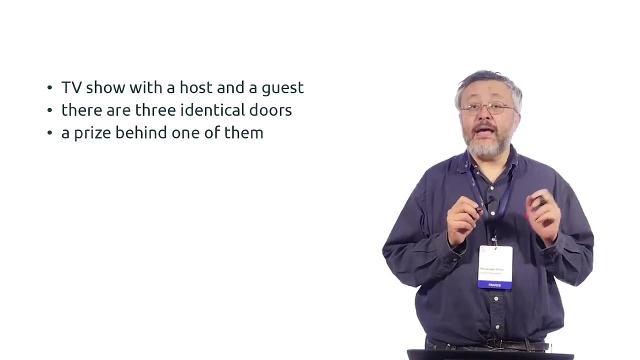 and modify the protocol more exactly, and this is very important, as we will see later. I prepared a slide with things in detail. so first there is a TV show, there is a host and a guest and there are three identical doors- one, two, three- and there is a prize. 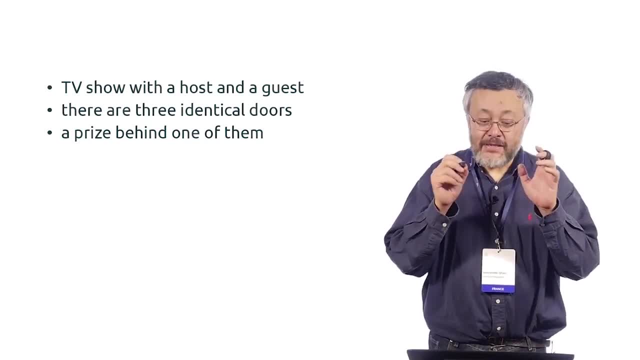 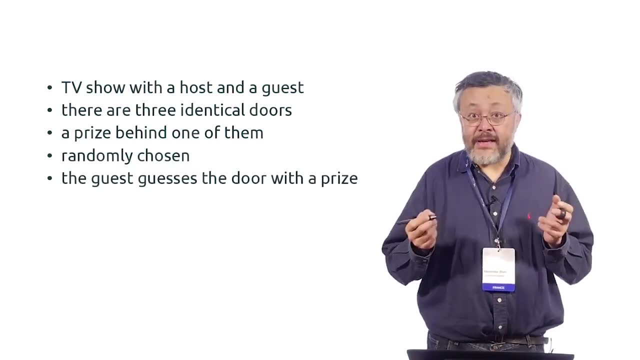 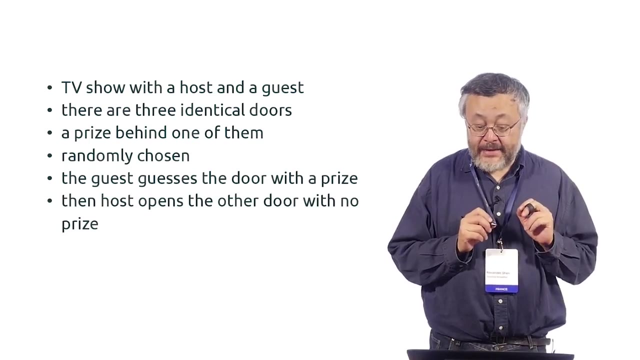 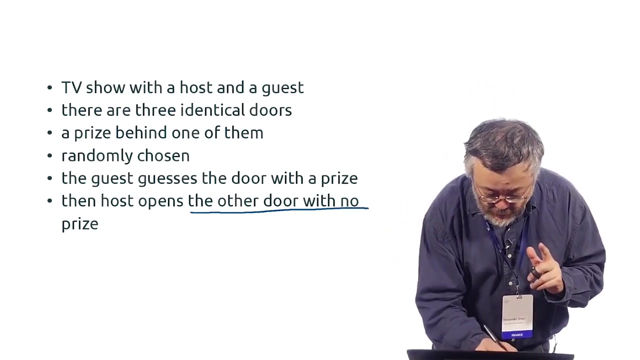 behind one of these doors, so forget about goals. and there is a prize- a car- behind one of the doors, and this door is randomly chosen. the guest makes a guess where the prize is, also randomly, and then the host looks open the other door with no prize. so there is one door with a prize. 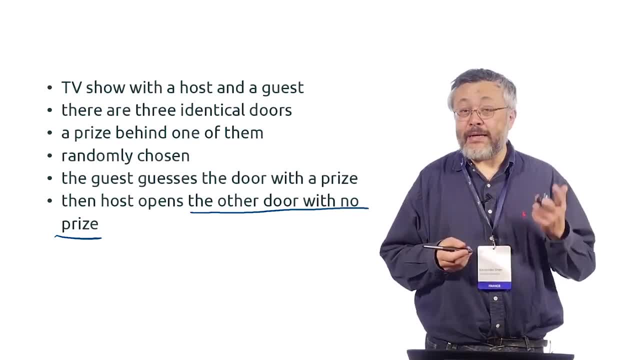 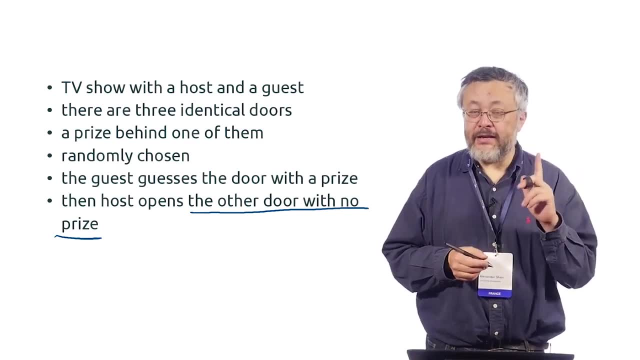 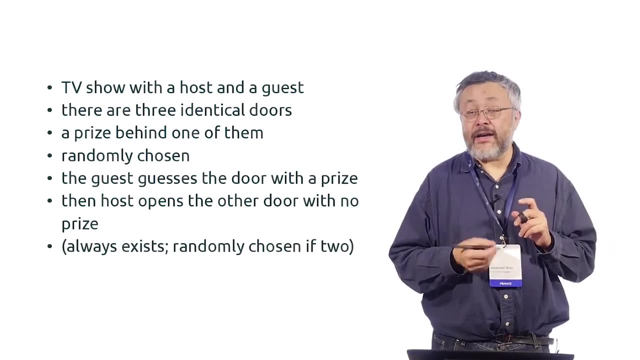 and one door chosen by a guest, maybe the same one, but in all cases there is another door which is not chosen by the guest and also which is not. there is no prize there. so the host opens this door and if there are two possibilities, the host chooses. 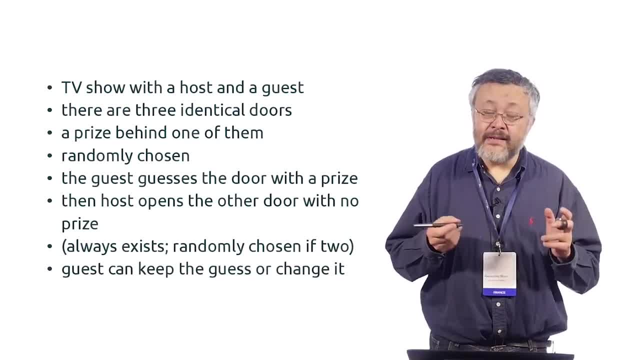 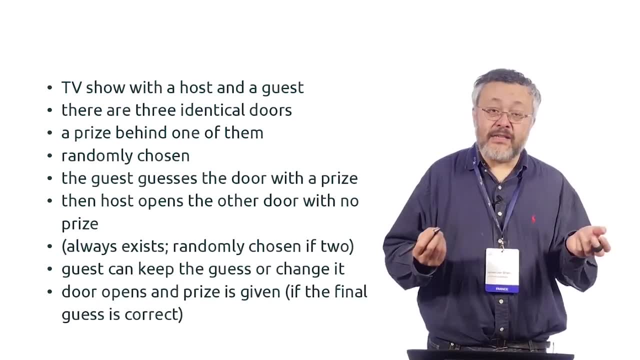 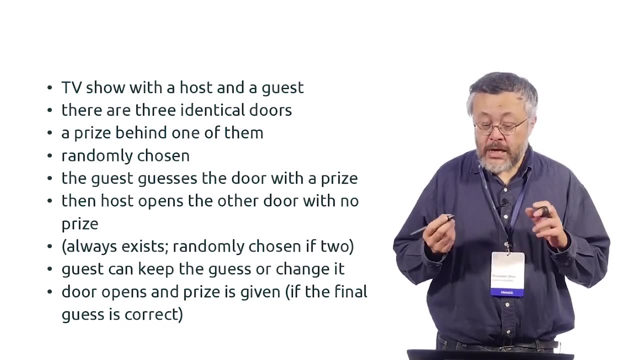 the random one, and then the guest is allowed to keep the guess or to change the guess, and then the door is opened and the prize is given or not given, depending on the final guess. if the final guess is correct, the player gets the prize. so this is the game setting. 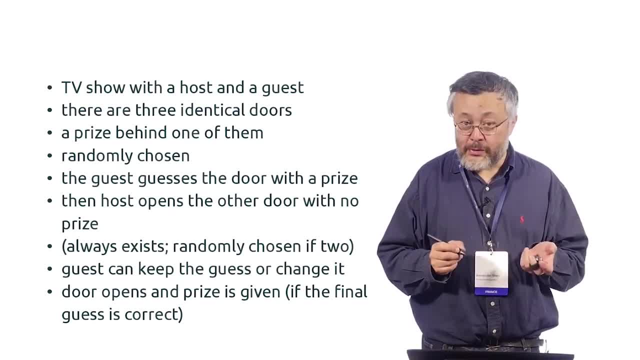 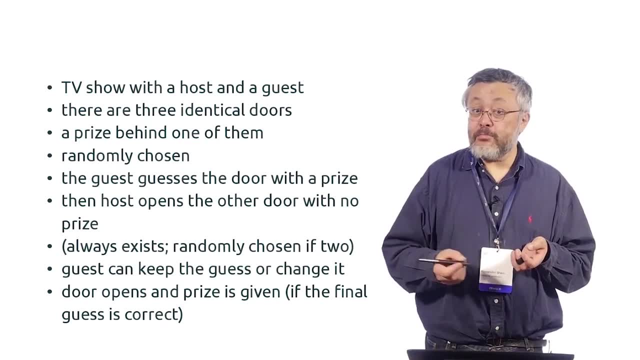 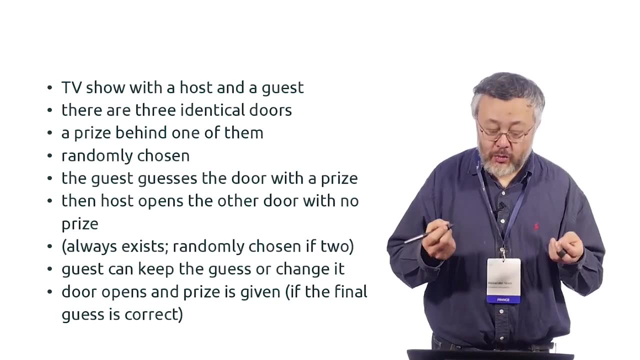 in full detail, I hope. and now you can think about this question. so what should you do as a guest in this show? should you keep your guess after the door is opened, or should you change it, or should you make a new random choice, or whatever? and now I'll try to present. 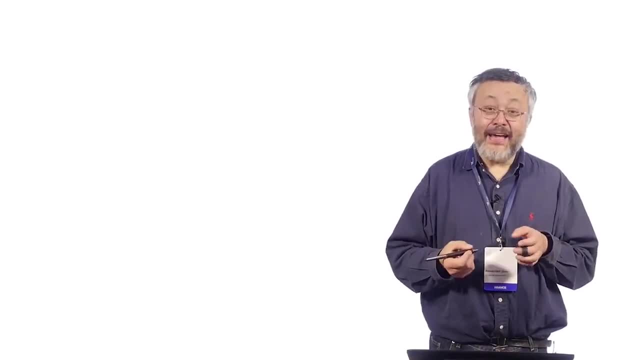 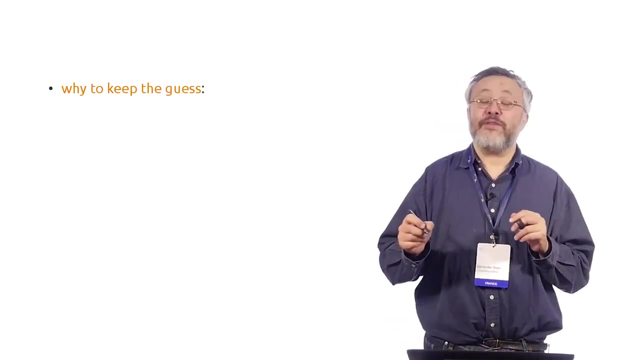 several arguments in favor of different theories, and I want to present it in a very convincing voice so you would be convinced. but then let me try. so why? why you should keep the guess? what is the argument why you should keep the guess? and the argument is like this: 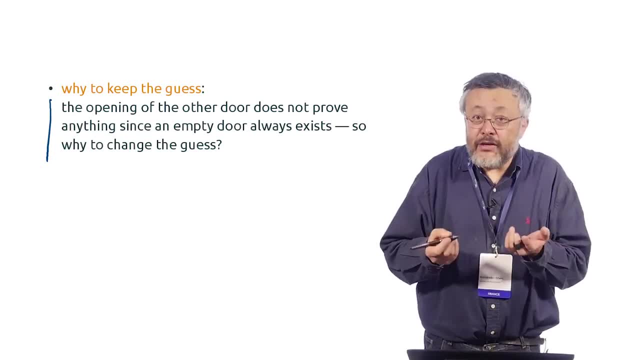 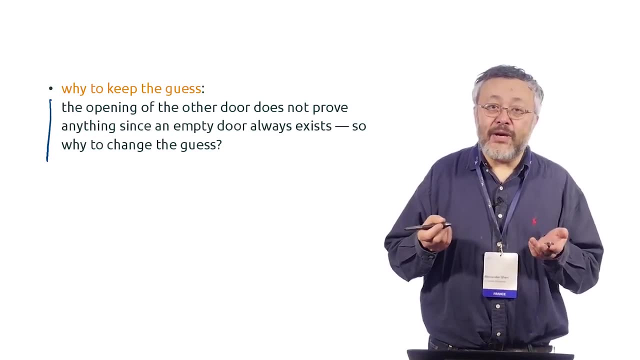 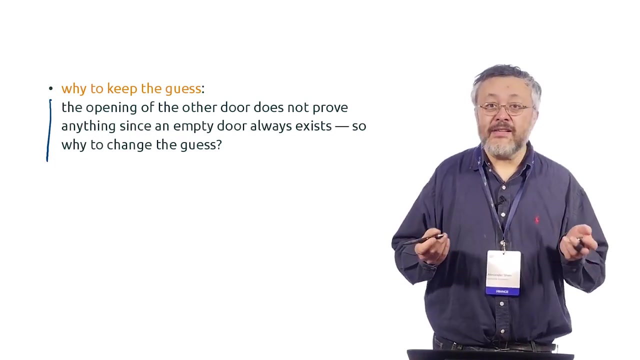 so you know, opening the other doors it's always the host opens the door. there is no prize. so opening this door doesn't really give you, doesn't prove anything about the original door. new events do not prove anything, so you should keep the old guess because there is no. 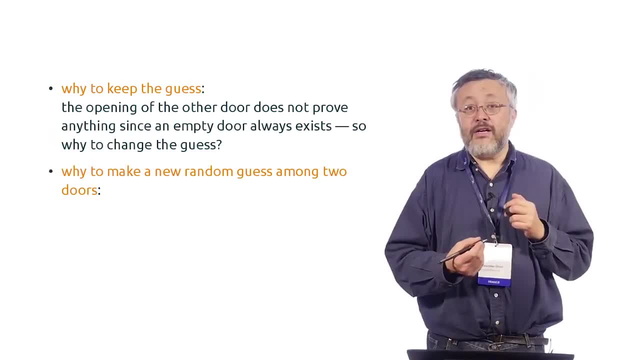 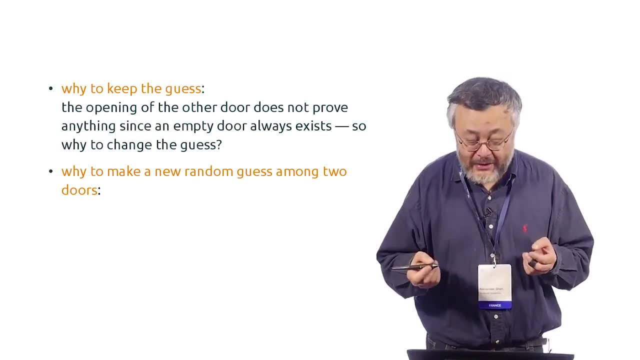 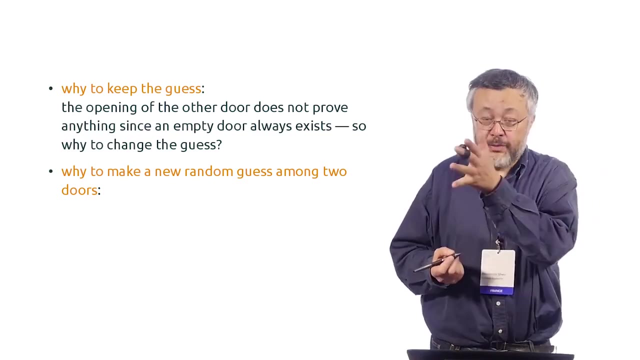 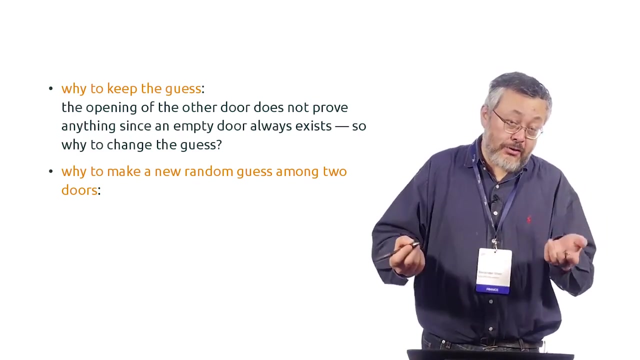 significant new information or why to make a new random guess among two doors. another recommendation, and this is supporting evidence. so now, after one door is opened, you can have a prize behind this or behind that door. the best way- it's a random event, so the best way you can behave. 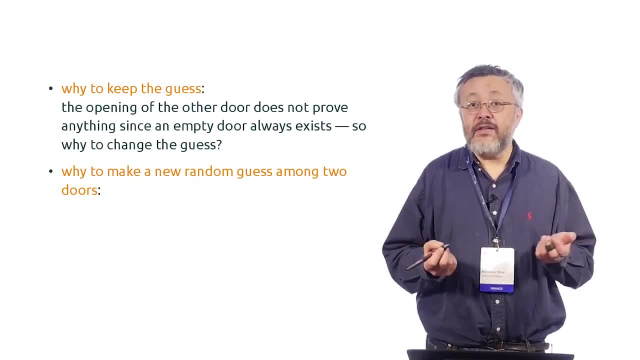 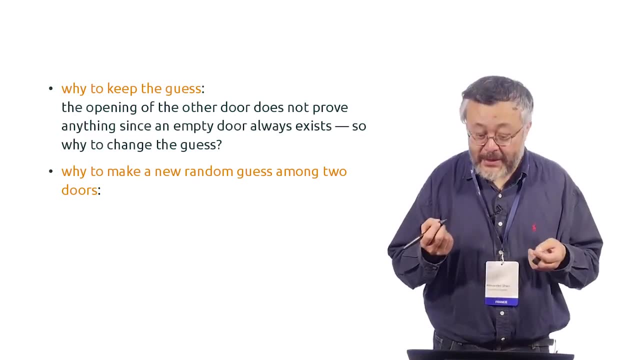 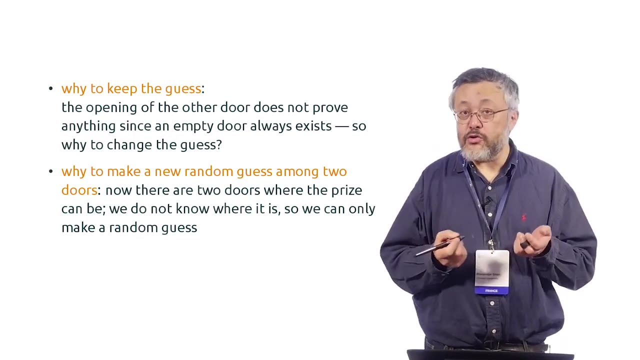 is also to make a random choice and choose the random door between two, and then you get the car with the probability one half. so it's a new random guess. it makes things better. so here is the reasoning. so there are two doors. you don't know what is the correct one. 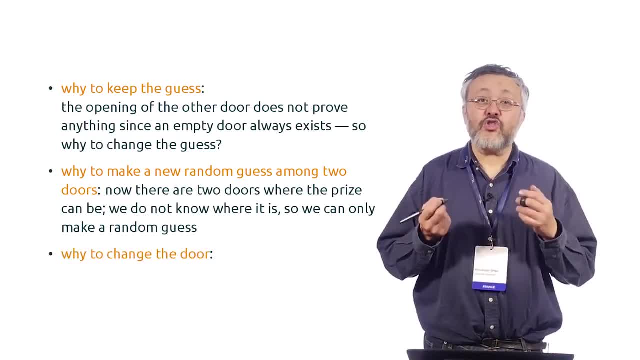 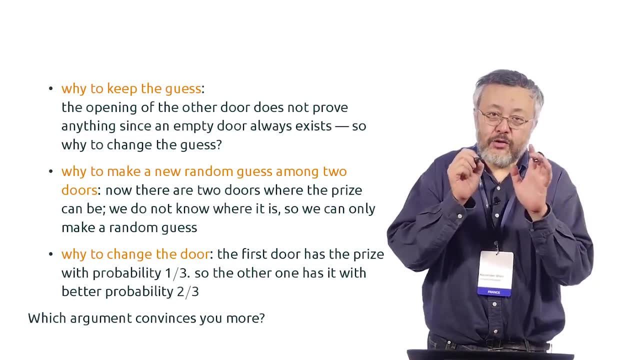 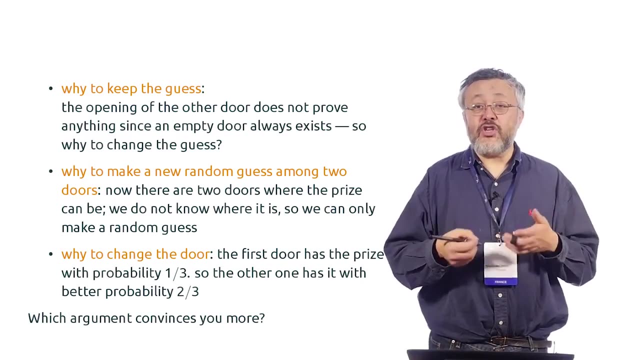 but you can make a random choice and finally you choose the door, and the argument is like this: the first door if there was no second part. the first door has a prize probability one third, and so the second door is just a complement, is not an event, which is not. 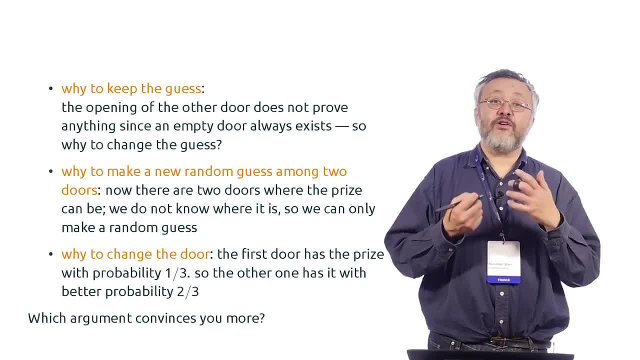 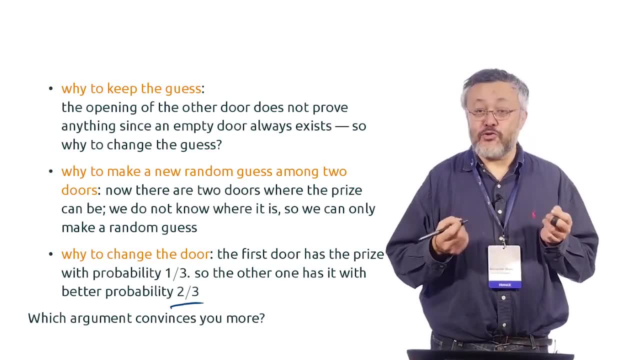 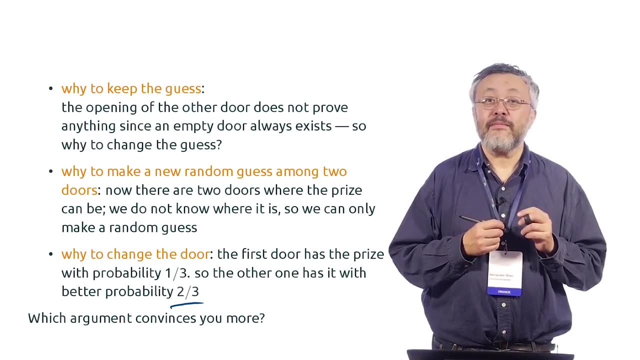 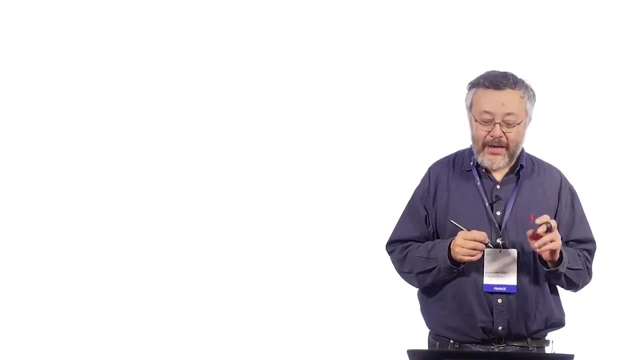 the first door does not have the prize, so the complement has the probability two. third, because there is a rule, so there is a better probability. you should do this. so which argument is more convincing for you? and let me now try to move you in other direction, explaining why the arguments 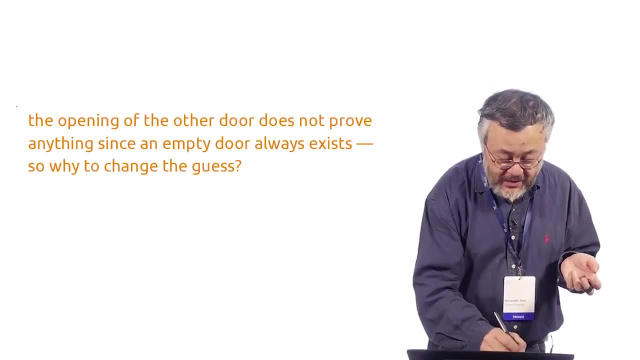 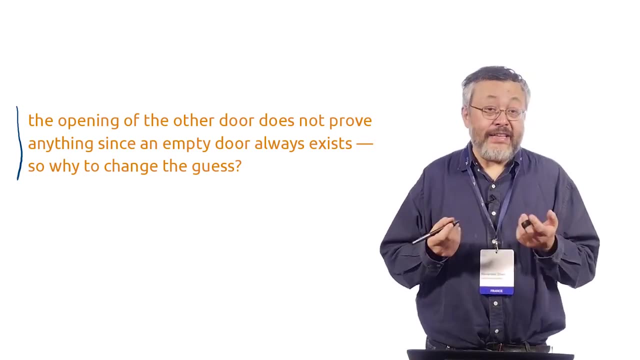 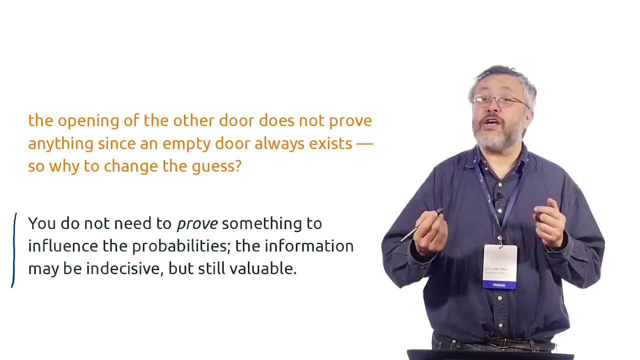 are not convincing. so in the first argument here is it? the opening of the door by the host doesn't prove anything, indeed it doesn't prove. even this information is not decisive. it can change the probability, so why should you ignore this? so this is the refutation of this argument. 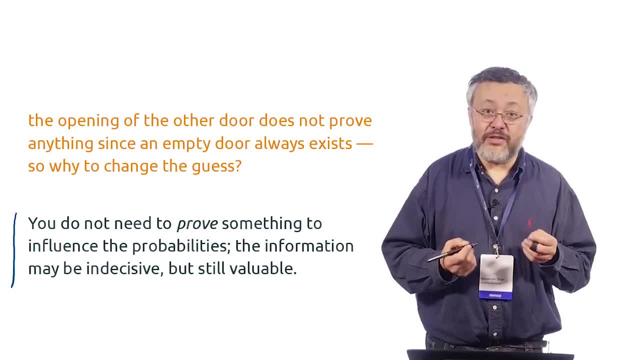 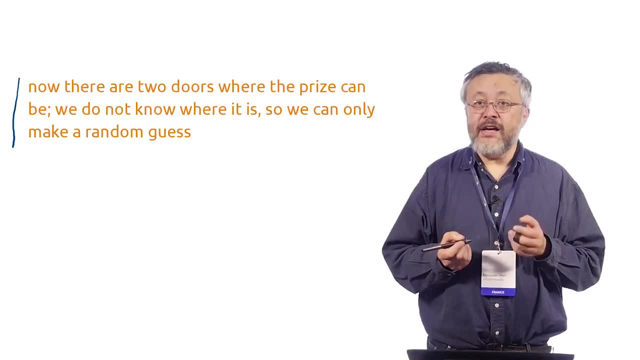 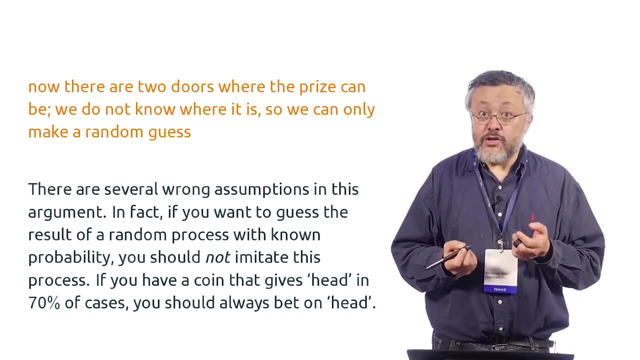 it is valuable information, but even if it is not decisive for the second argument. the second argument says that, since you don't know where the car is, the only thing you can do is just to take a random door, which can be contested here. so, for example, the idea that if there is some random process, 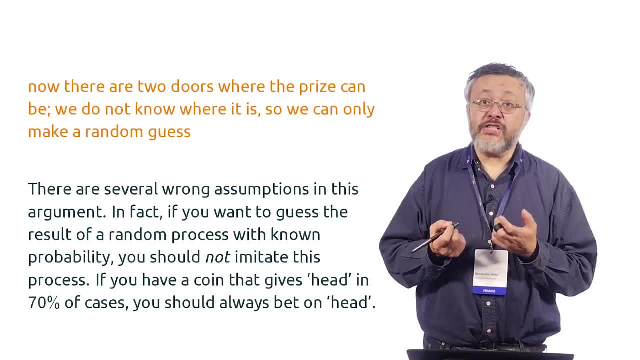 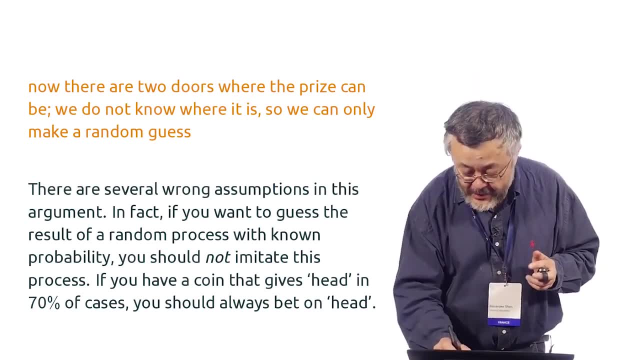 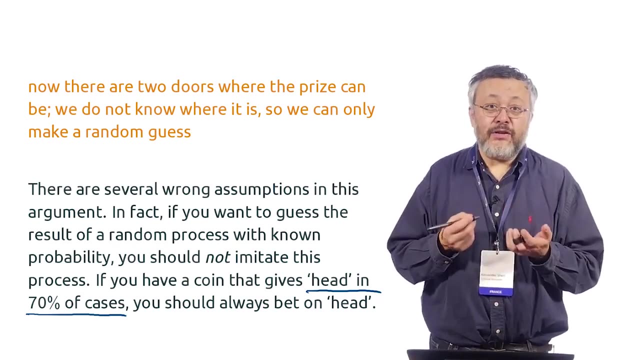 to get the best chances, you should simulate the process. it is just a wrong assumption. imagine we have a coin which is more often false head, so it gives head in 70% of cases- and you want to bet against this coin and it. the wrong idea is to imitate the coin. 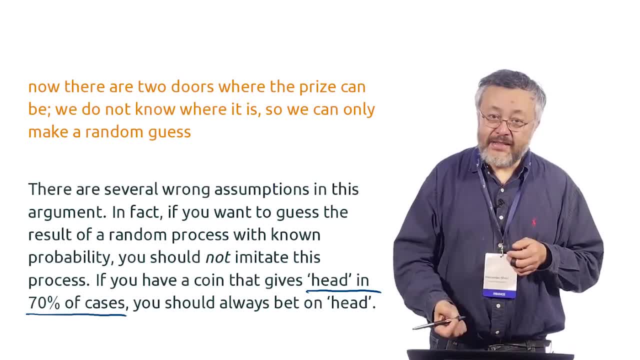 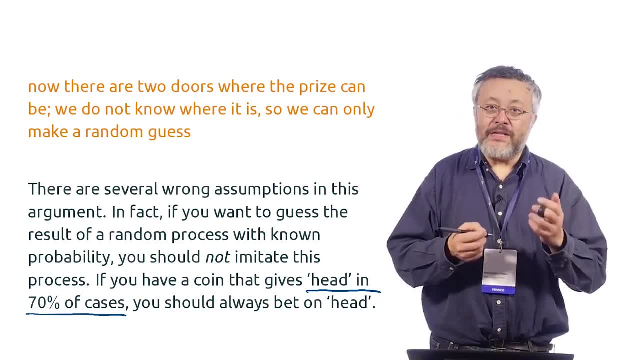 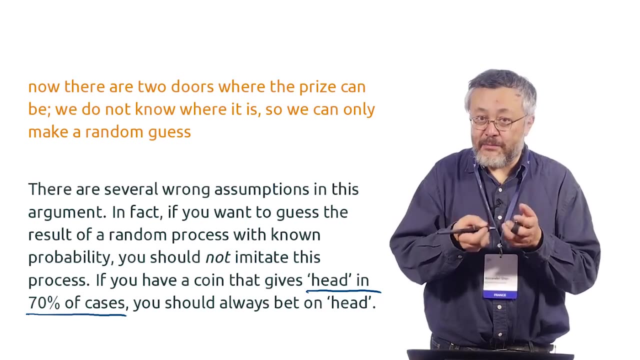 is to try to say head in 70% of cases and tail in 30%, and you will win more if you play a game with this coin and you always say head, of course, because there are more chances if you say tail in some case in some trial. 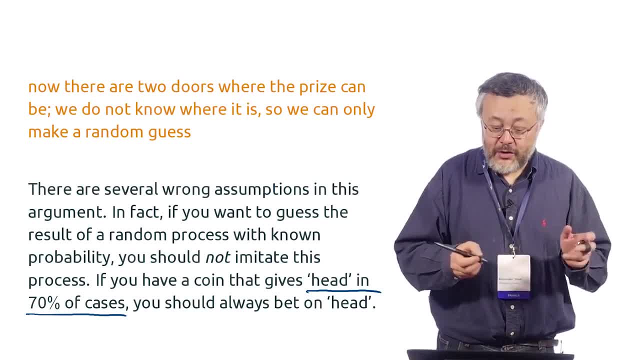 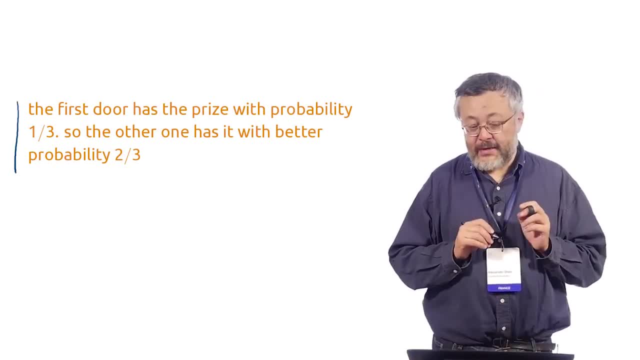 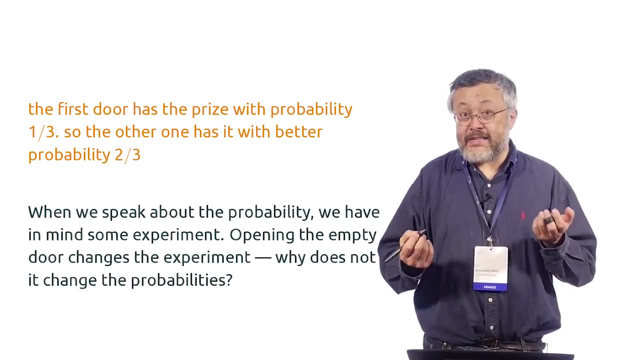 then you decrease your chances in this trial, so why do this? so this is why the second argument is bad and the third argument. then the probability is one third and the complement is: probability is two thirds and it is an error which we discussed, because this probability one third, 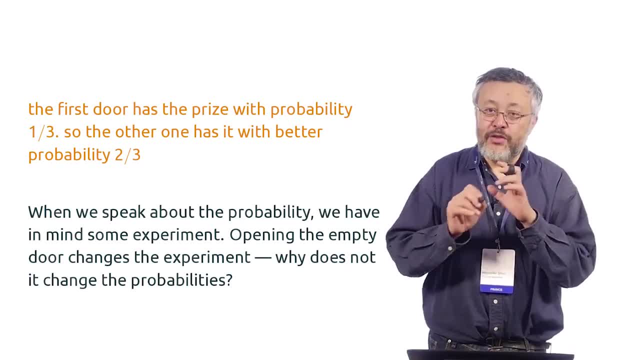 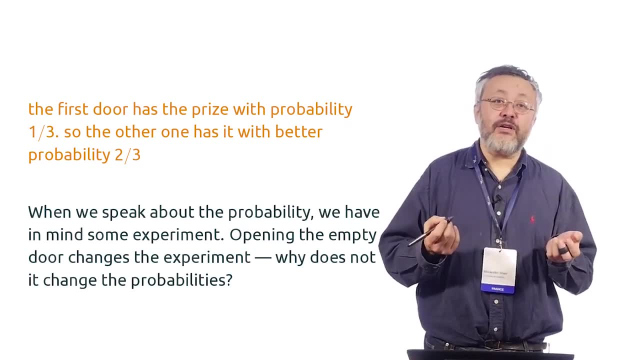 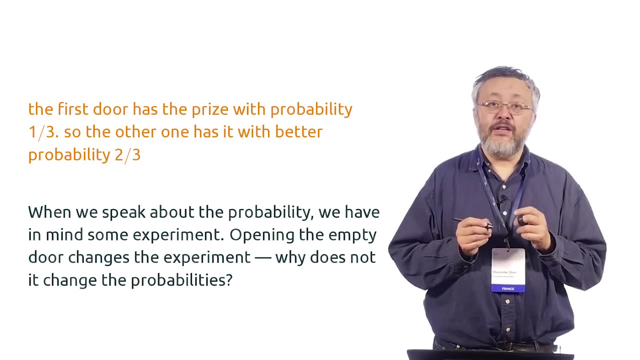 was for the one experiment, for the first experiment, without this change, opening the door part, and then we change the experiment. we have a new experiment now, so new probability is just a probability in a new experiment and we cannot apply the formula for the sum of probabilities because they were for. 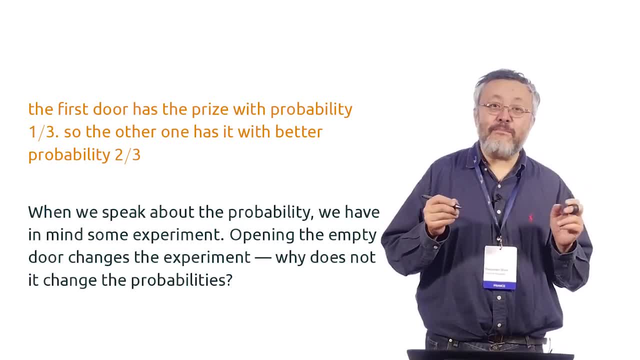 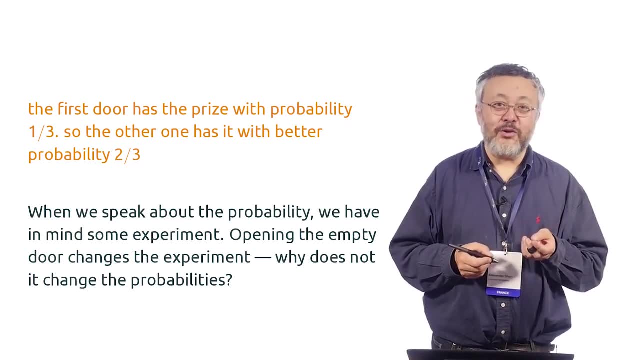 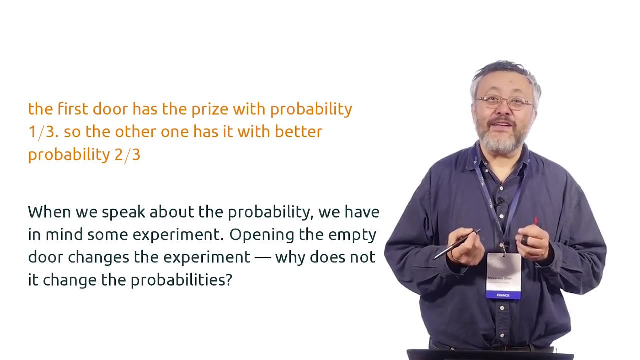 events in the same space. ok, so now I tried my best to make to say convincingly what are the argument for and the argument against. so where are you now? what do you think about this question and what is the correct answer? stop here if you want to think. 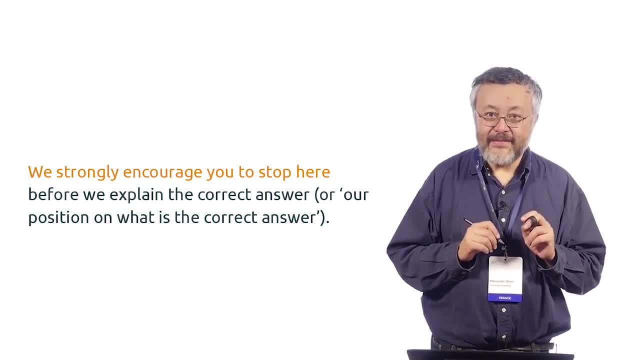 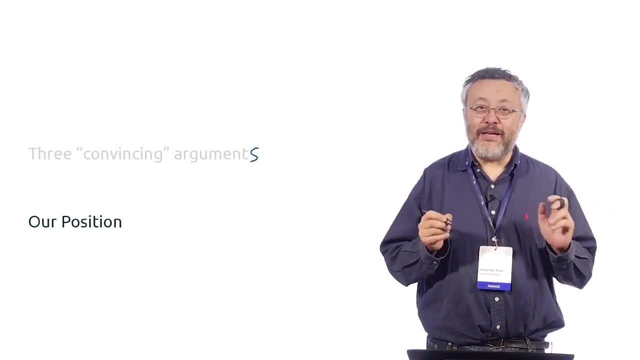 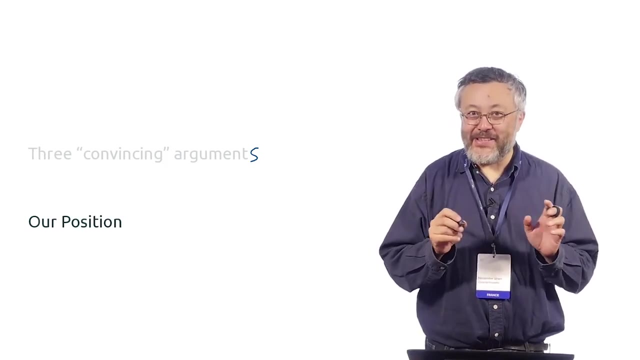 and we will give the answer later. so we have three convincing arguments and now we want to explain the correct answer. or if we are in a postmodern world, it is not politically correct to say what is the correct answer. we should say it is our position about this problem. 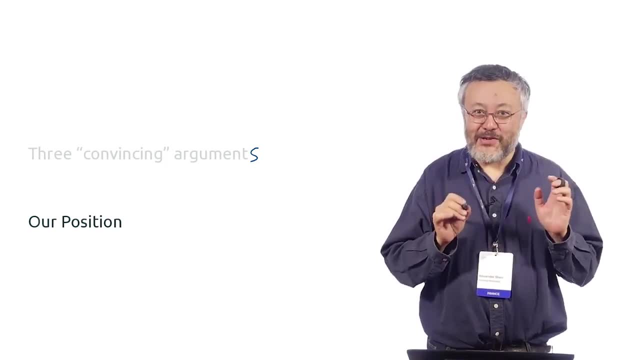 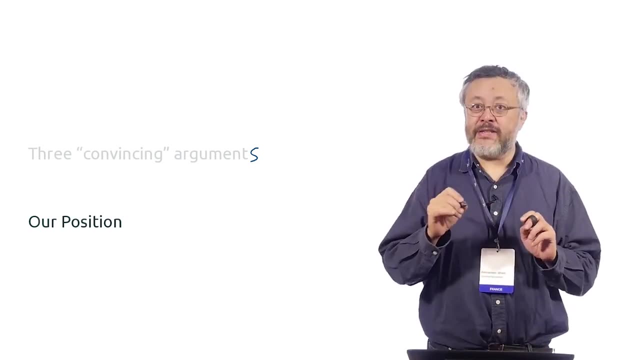 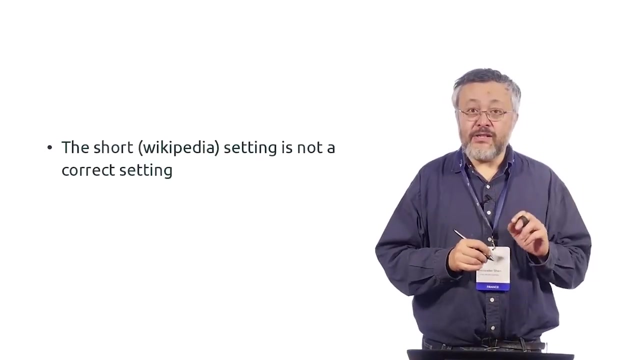 and other people have different positions. we don't make any claim, but if you want to be serious, I will try to explain the correct answer and also explain why the short setting is not good. ok, so what do we think about this problem? first, the short setting is not. 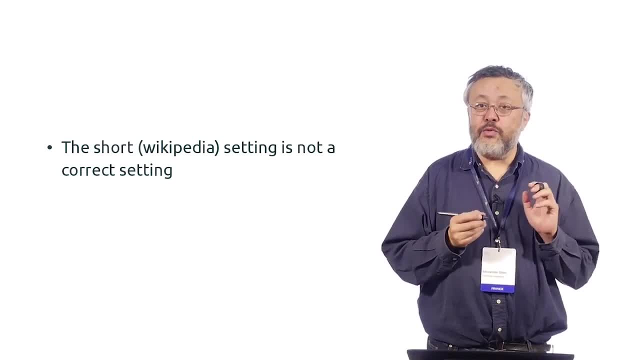 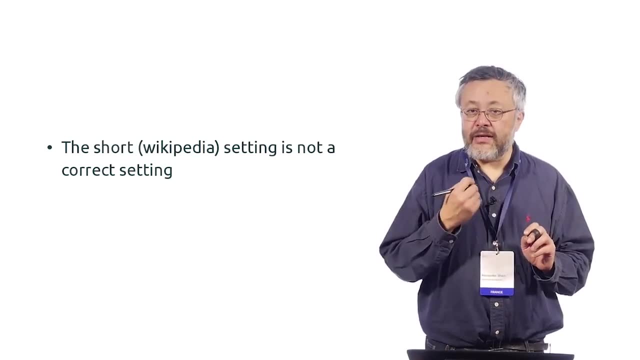 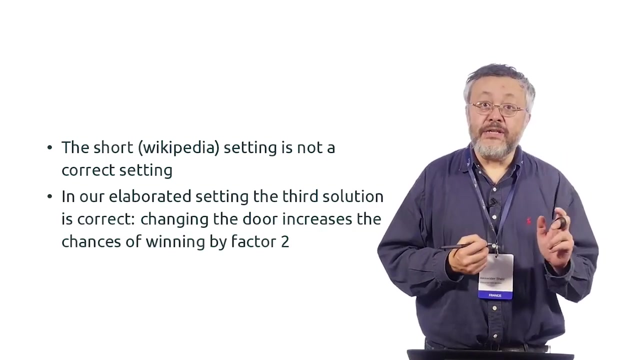 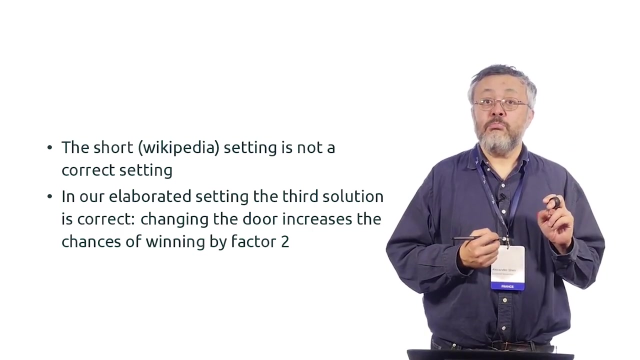 if we just say the short story, then we don't have any. we cannot say what is the best strategy, because the situation is not clear and, in our elaborated setting, the correct solution is the third one. so, indeed, changing the door by a factor, winning chances by a factor of two. 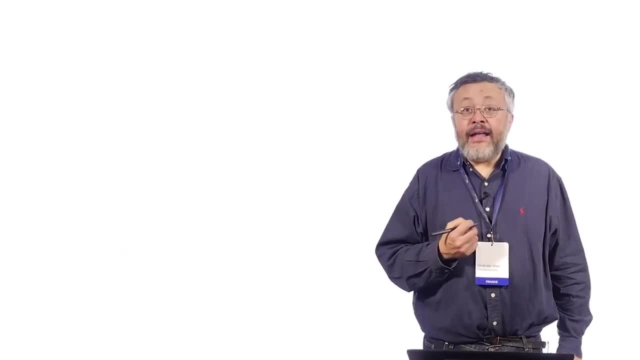 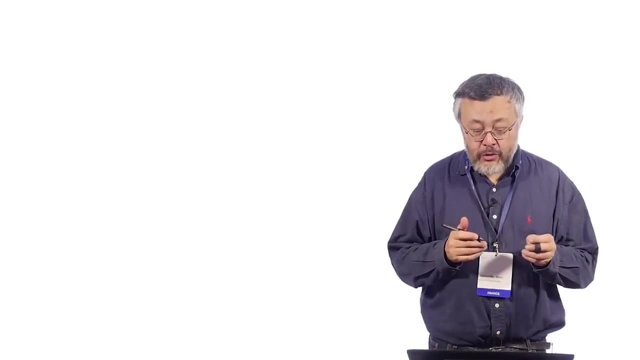 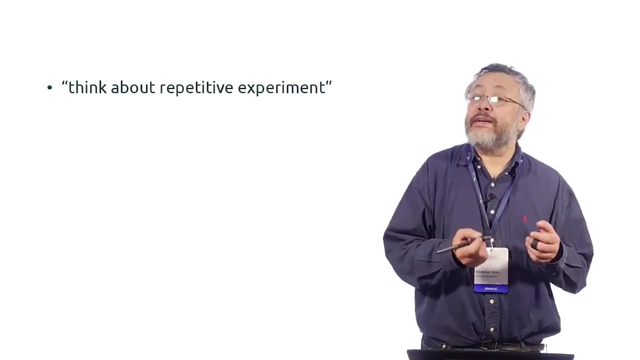 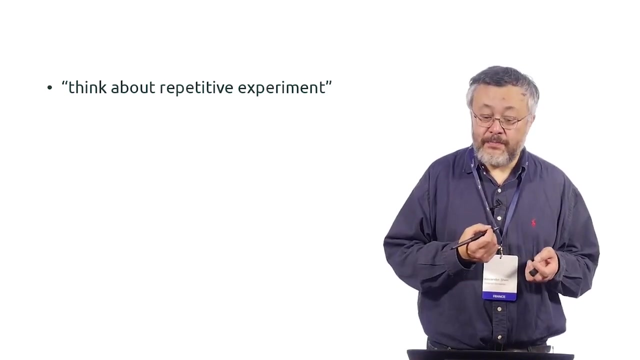 so why is all this? and there is some general advice: how to deal with paradoxes and probability theory. you should think about a repetitive experiment. so if there is not no repetitive experiment, it is not clear what is this experiment? then the question should be posed. but if there is a repetitive experiment, 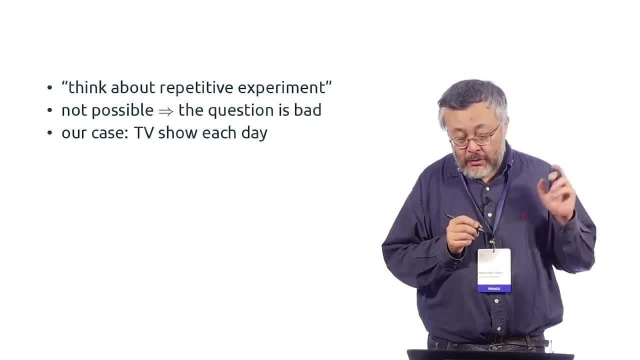 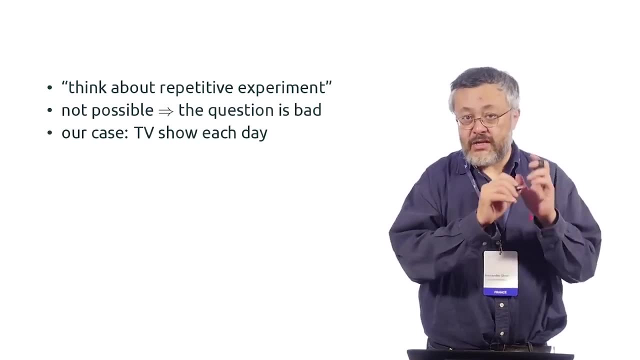 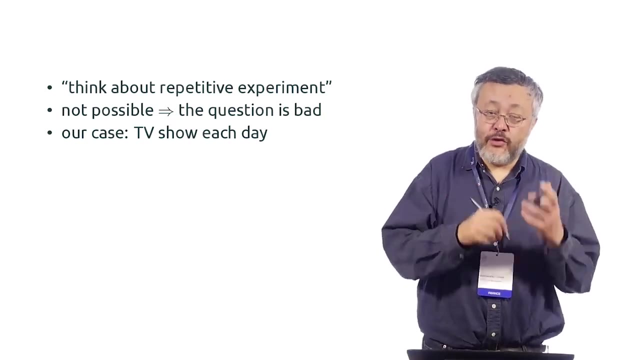 and you imagine it, things become more clear. so in our case there is no problem in repetitions. you can make this show every day and can make the random choices every day, and then you should imagine that the guest follows the first strategy, the second strategy or the third strategy. 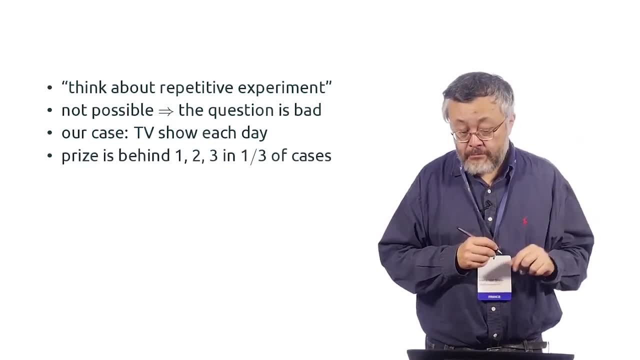 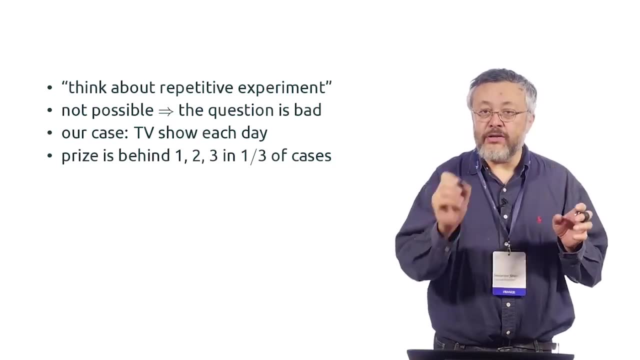 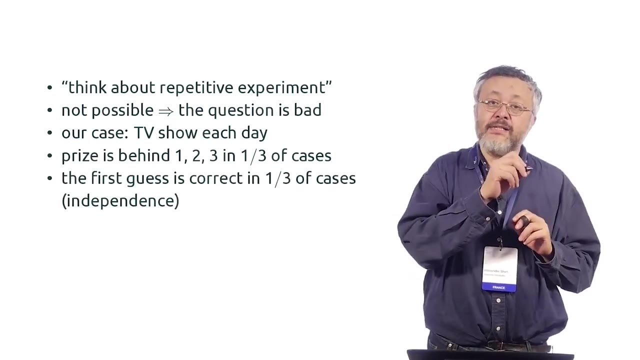 and look at which percentage of cases the guest will win. so let's look at this. so, by assumption, our price is behind the door one, door two and door three in one third of all cases and in each of the third cases the guest makes independently the guess. 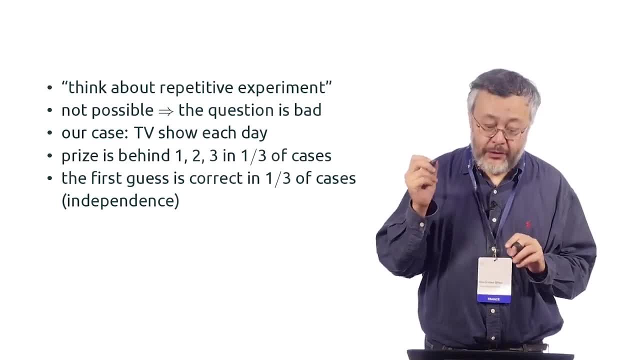 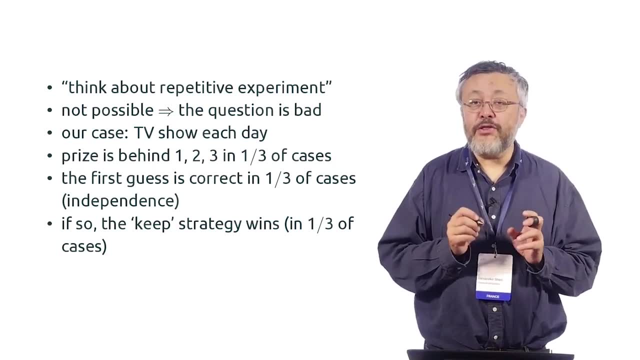 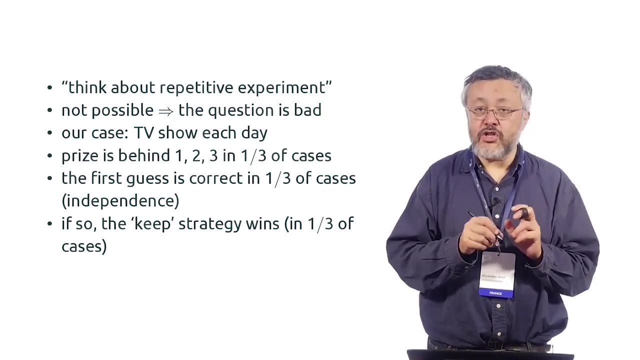 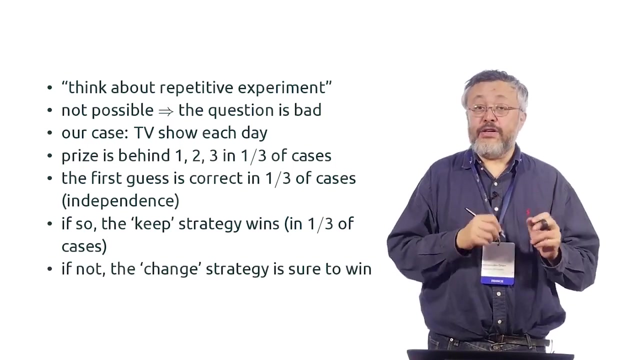 and so this guess is correct, with probability also one third. so this is enough to say that the keep strategy will win in one third of the days. so if a guest always follows the keep strategy, she will win in one third of the days, but in other third of the days she will lose. 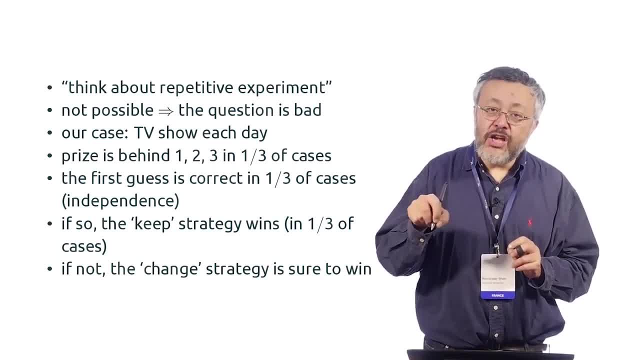 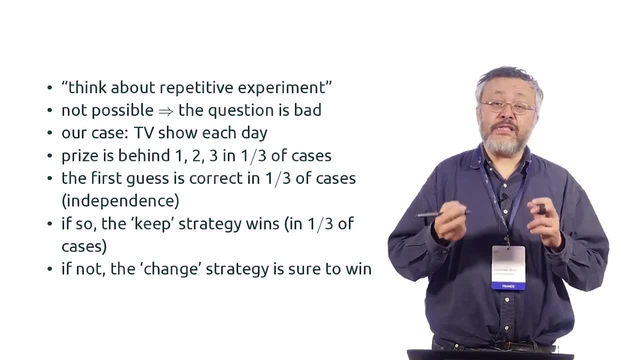 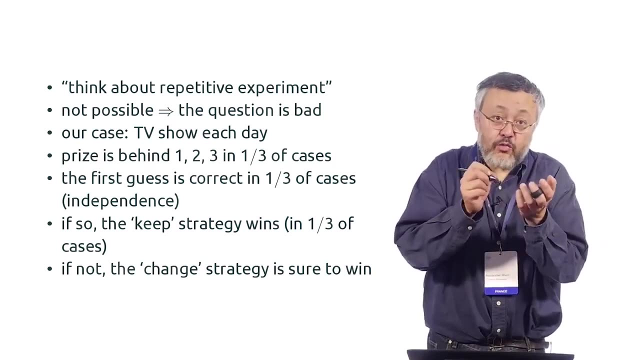 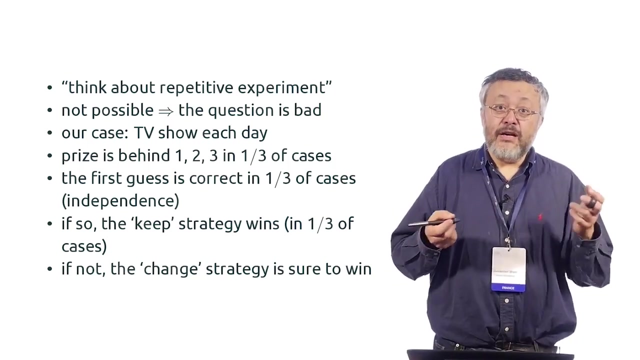 but if she would use the change strategy, then she would win exactly in the other cases. so in fact this event can be considered as events in the probability space, because we just have an experiment in one part for one strategy, the experiment. the rest is not important, but still. 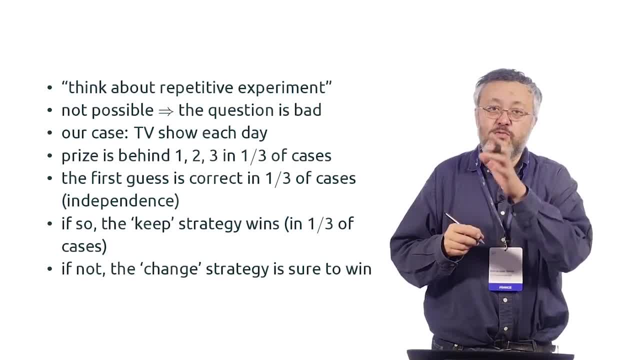 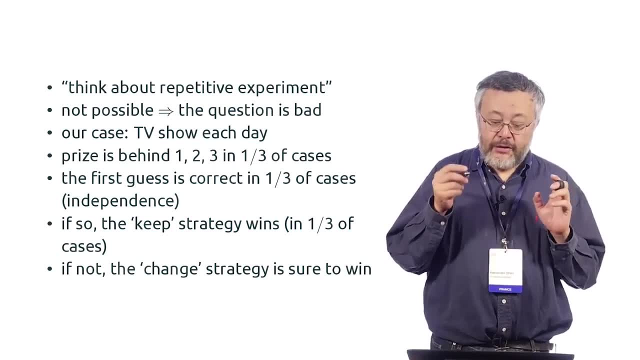 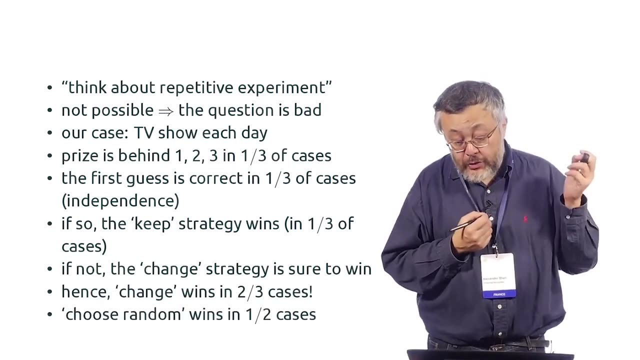 we have the same setting and there are cases when the keep strategy is good and when the change strategy is good. there are complementary cases, so the change strategy is sure to win, with probability two over three, and we can also say that the random choice strategy will win. 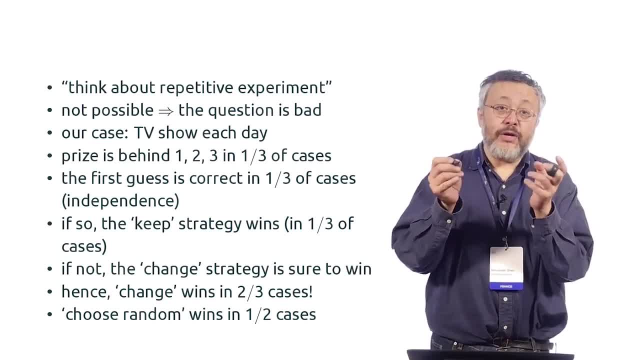 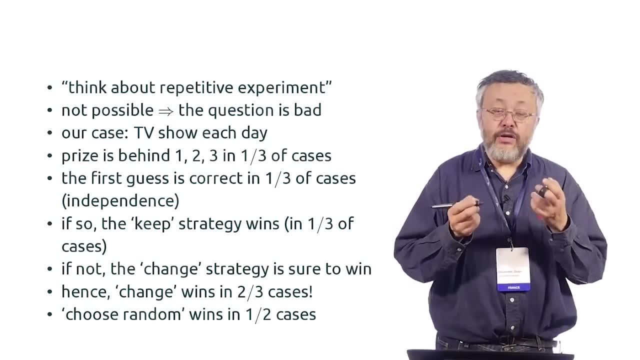 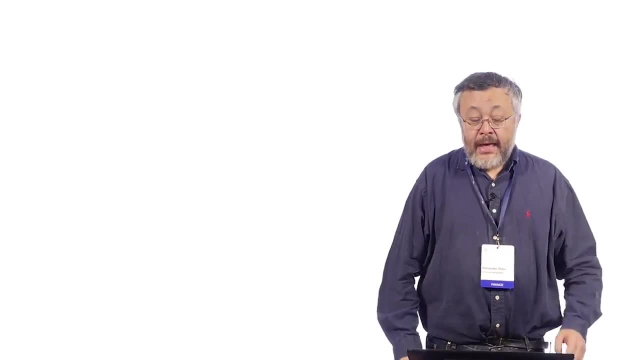 in half of the cases because new random choice will be correct in half of the cases by definition of independent random choice. so now we know the probabilities for all three strategies and see that the third strategy is the best one. and now let me explain why. the short setting. 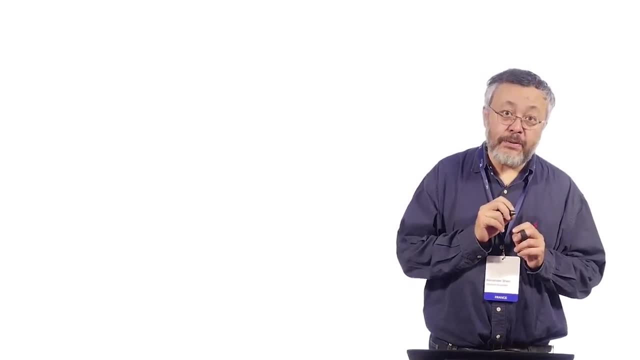 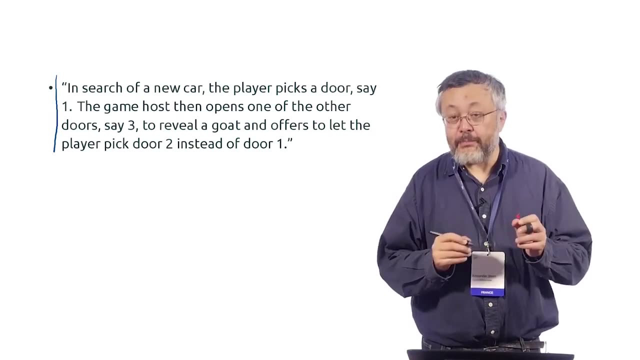 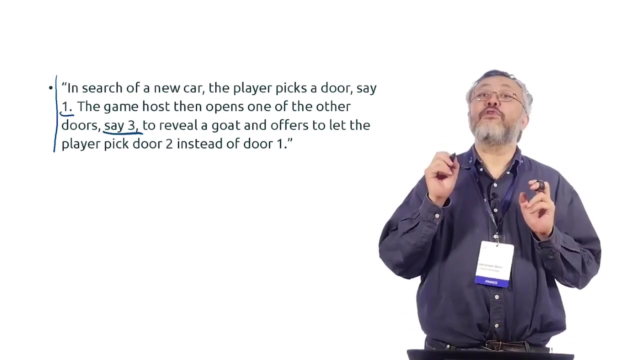 as the story below the picture in Wikipedia is not enough, why you should not hear the story, I repeat it. in search of a new car. the player picks a door, say door number one. the game host then opens one of the other doors, say door number three, and there is a goat. 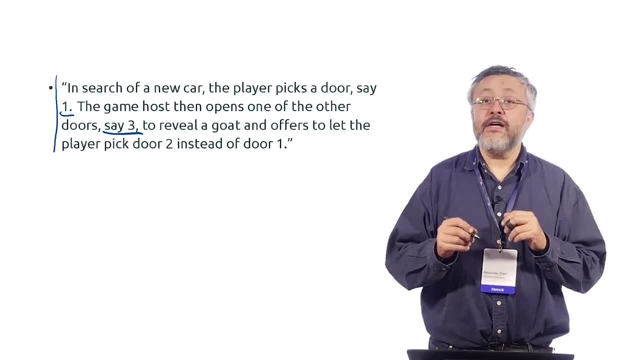 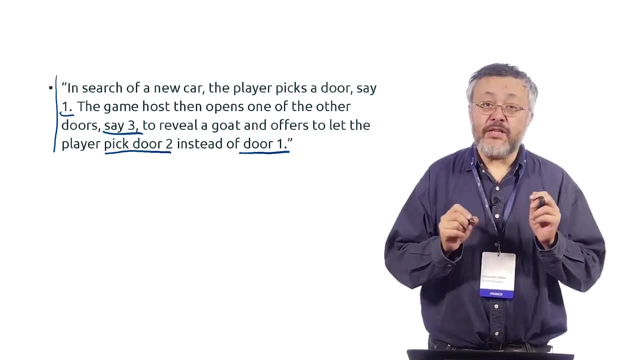 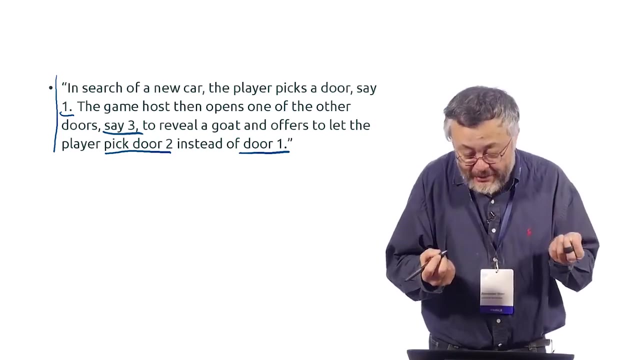 and then the player has a chance to change the guess and pick door two instead of door one. so this doesn't tell you what is the repetitive experiment. this tells you only what happened once, and this, this information, is just not enough. so this is a sequence of events. 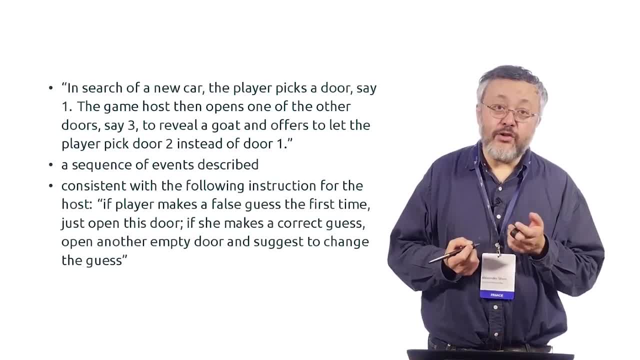 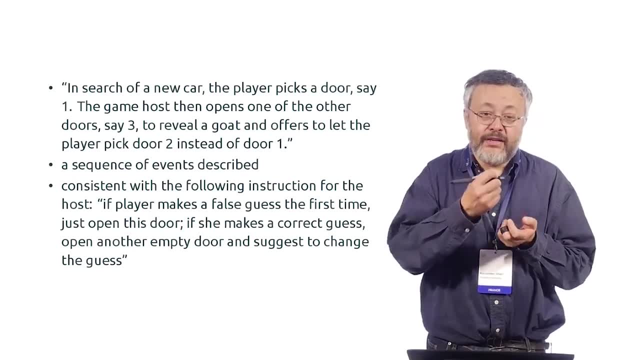 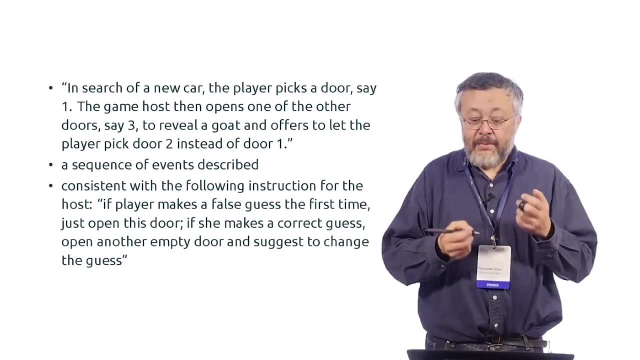 in one case, and to see why it's not enough, imagine that the host of the show probably in advance knows, has some instructions what to do. maybe they are given or whatever. but imagine the instructions like this: first you let the guest to make a guess and if 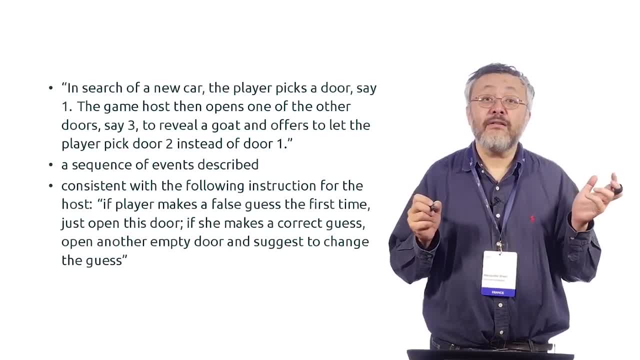 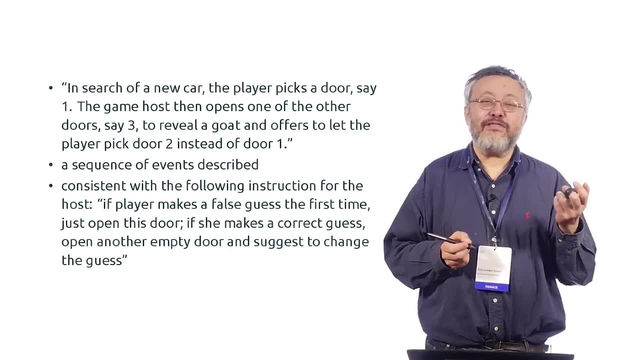 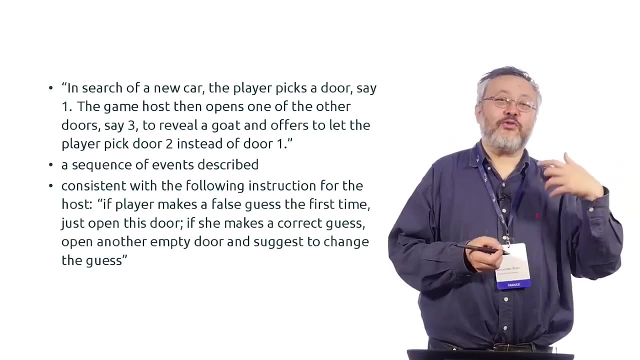 the guest is incorrect, then you open the door immediately and guess: you save the money. and if the first guess is correct, you still want to save the money. you want to somehow to confuse the guest and so you say, okay, I open this door and now you can change. 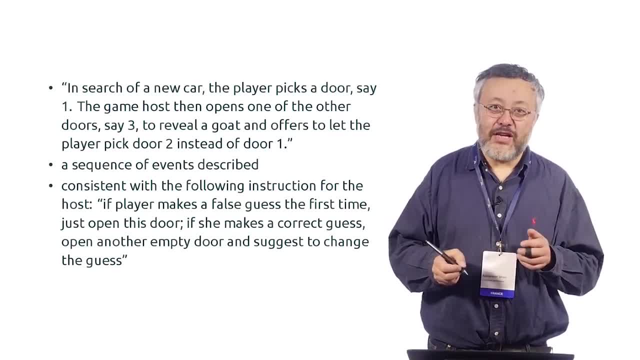 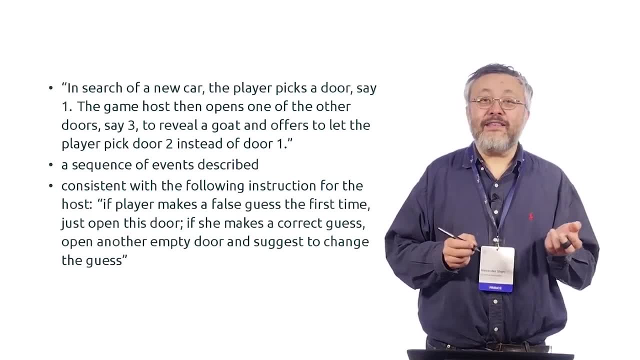 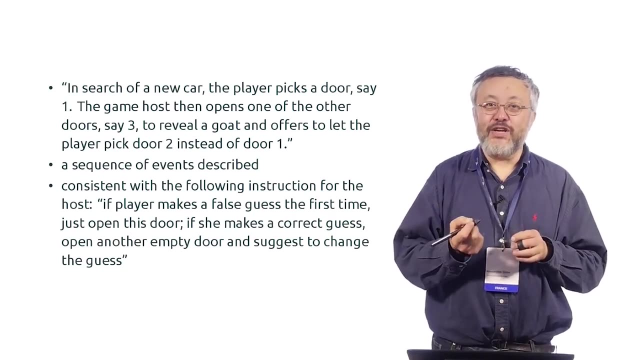 maybe the guest will change and then you save your money because the first guess was correct. so the host follows this protocol and in this case it's obvious that if the host suggested to change the door, it's a clear indication that the door was the guess was correct. 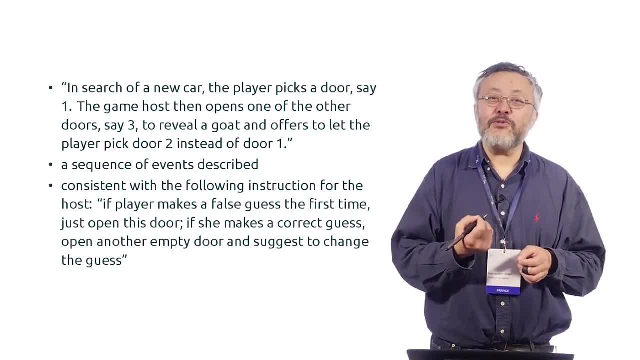 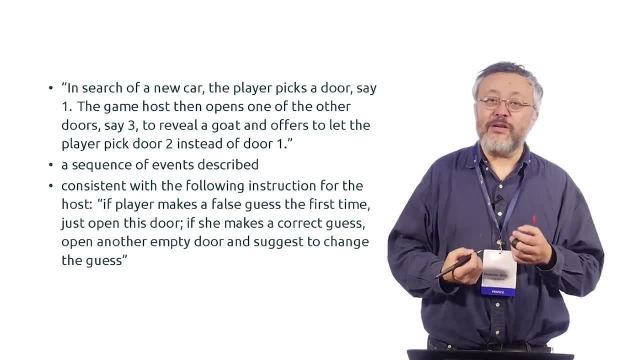 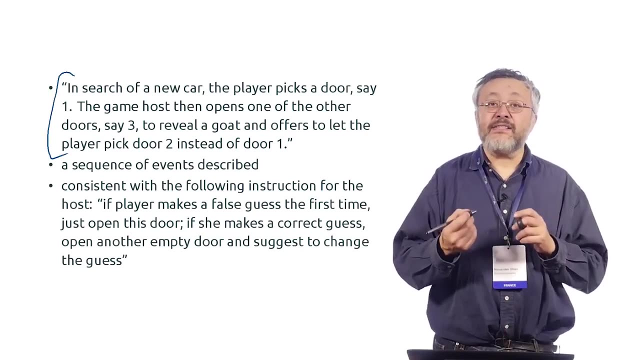 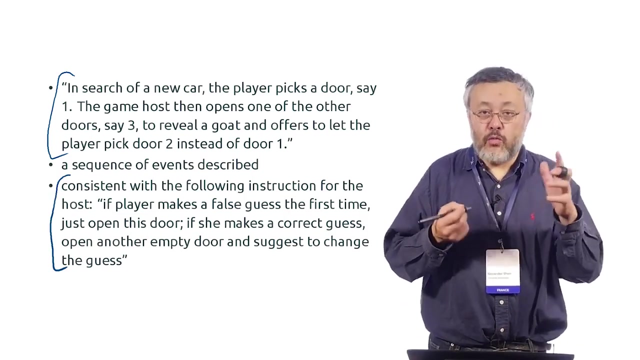 so you should keep it. of course, in this setting, the keep strategy will win with probability one in the cases when it's applicable, and you should always follow it. so the story, this story is consistent with both descriptions, with this one and our original description, so we cannot distinguish between. 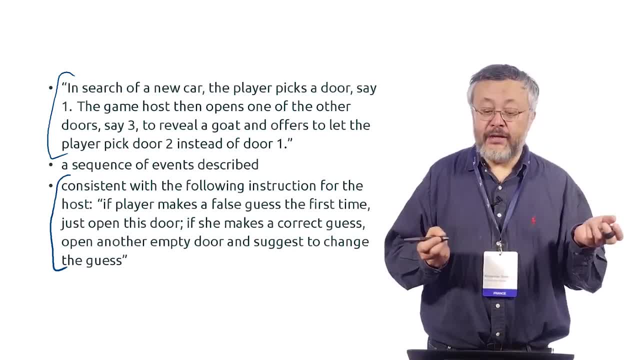 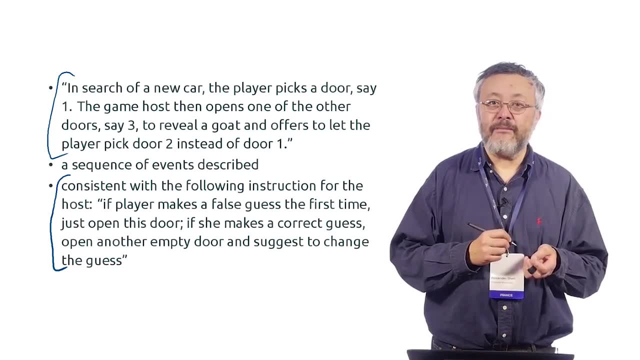 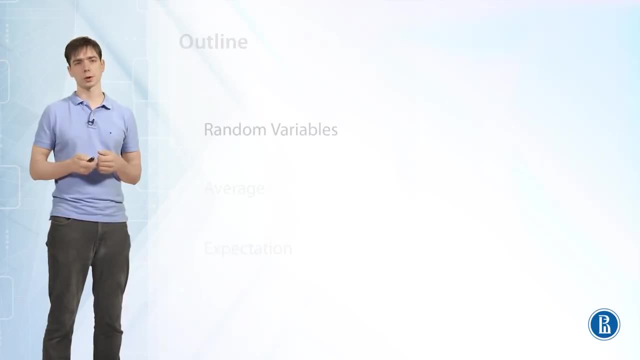 what is happening behind the scene, and the recommendations depend on what is happening, so this short description is not enough to make an informed decision about best strategy. Hi, I am Vladimir Podolsky and I will be your host for this week in this series. we will discuss: 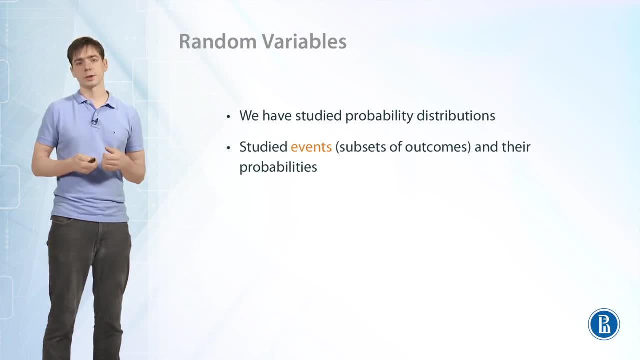 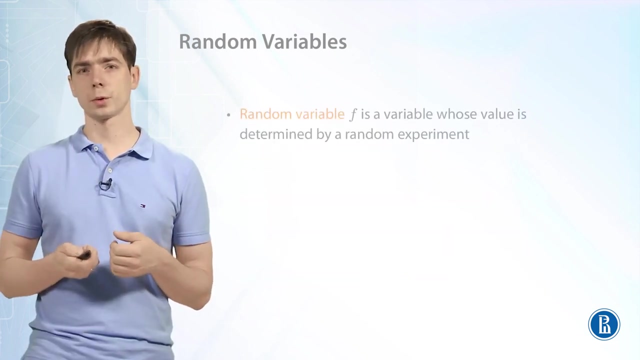 probability distributions and the probability distribution of random variables and their expectations. on the previous week we have studied probability distributions. we have considered events which are just subsets of outcomes and their probabilities. note that an event is a yes or no question, so we have a probability distribution on some finite set, x. 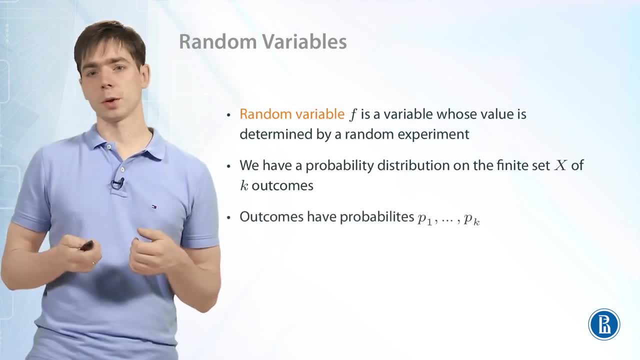 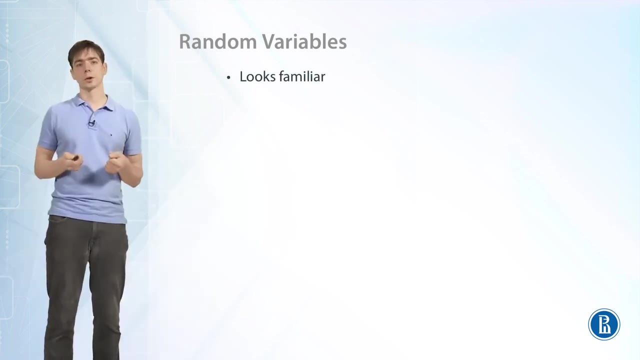 with k outcomes, outcomes have probabilities p1 and so on, pk, and to define a random variable, f, we have to assign a number, a sub i, to each outcome, and then f has a value, a sub i, with probability, pi. this looks familiar and indeed we have already seen this before. 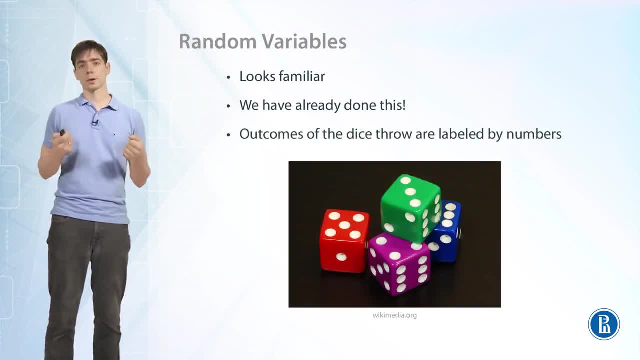 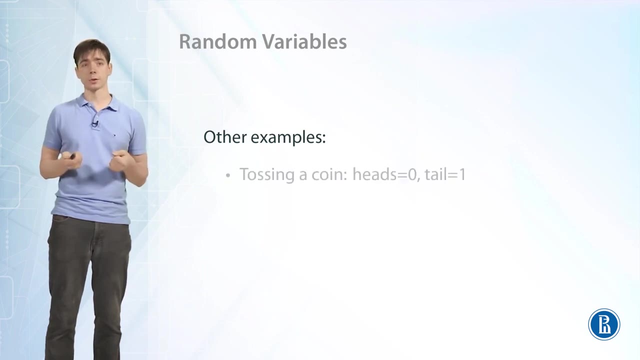 for example, if we consider an outcome of a dice throw, then we label each face of a dice by a number and in this case we already have a random variable. to each outcome we assign some number. there are other examples we have seen and there are other examples in real life. 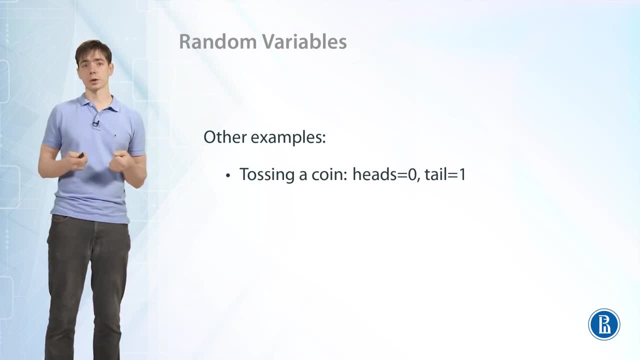 for example, if we toss a coin, then we can assign 0 to heads and 1 to tails. we have done this in the previous lecture. if we consider a random person in the class, then the age of a random person is a random variable we assign to each outcome. 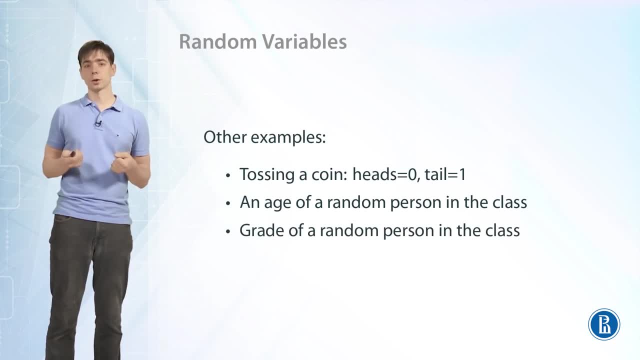 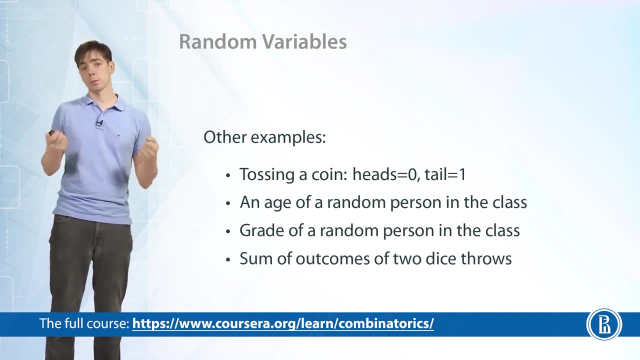 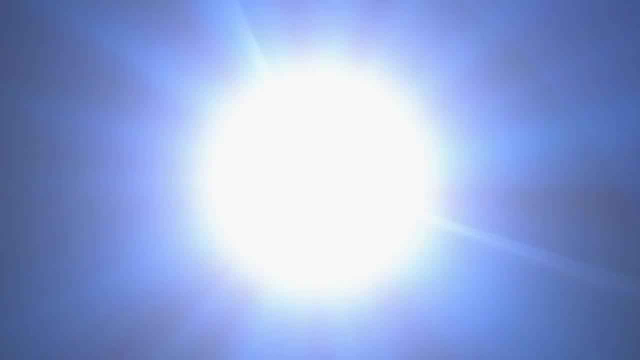 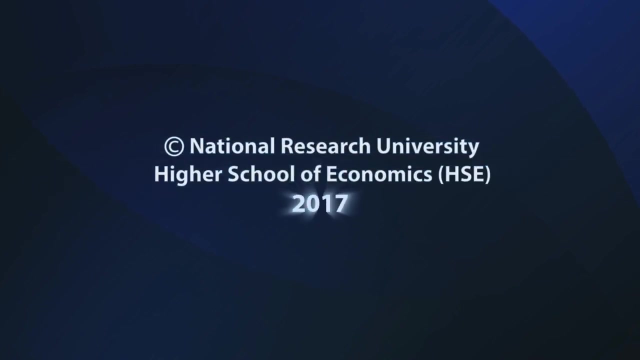 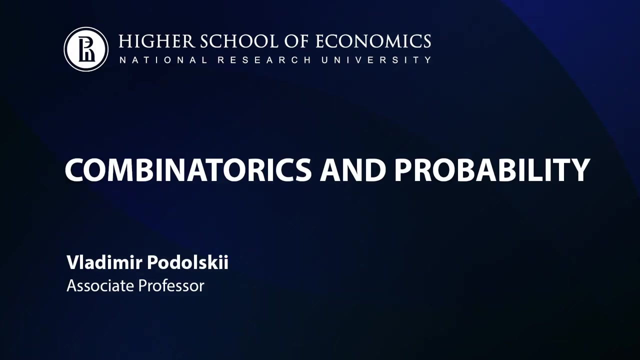 some value. a grade of a random person here in the class is a random variable. there are some other random variables that arise, for example, in some games. for example, sum of outcomes of two dice throws: this is also a random variable. before we discuss expectations of random variables, 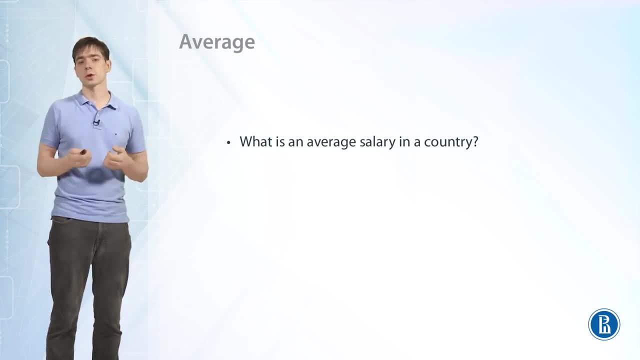 we will discuss the notion of average. so what is an average salary in some country? ok, this is the total salary of all population divided by the number of employees in this country. so this is the standard notion of average which is used everywhere. in mathematics it is called arithmetic mean. 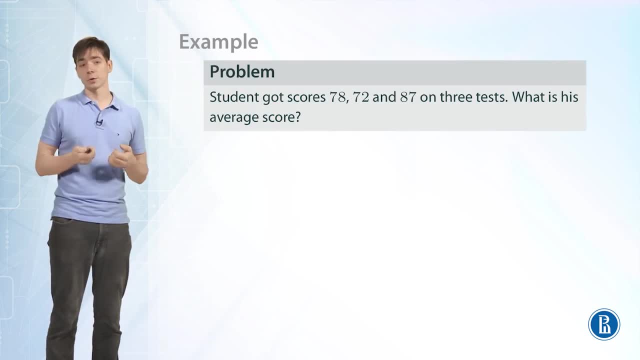 ok, let's consider the following example: we have a student and he had 3 tests and he got scores 78,, 72 and 87. what is his average score on these tests? ok, to compute average, we need to do the following: we need to add all the scores. 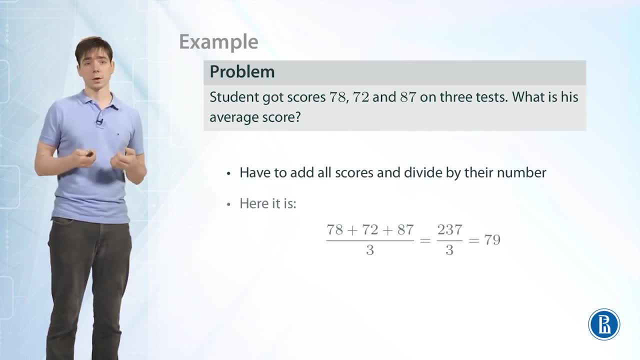 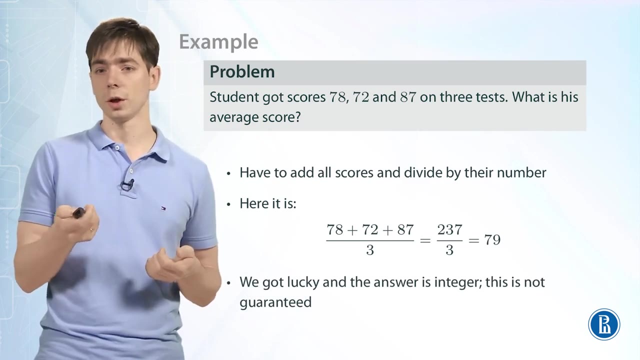 and divide by their number. so we have to add 78, 72 and 87, divide by 3. there were 3 tests, so we have 79. note that in this case we got lucky and the answer is integer. in general, this is not guaranteed. 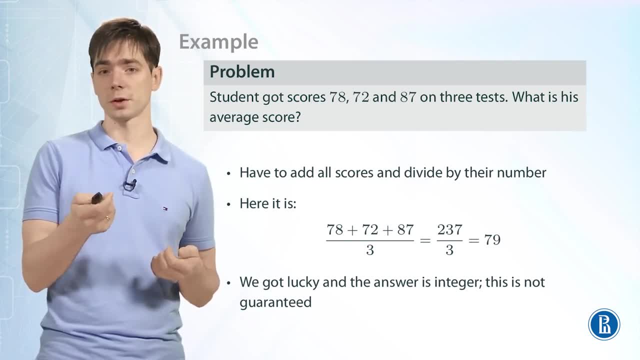 for example, if we reduce instead of 87, we consider 86. there we will not obtain an integer number. we will have 78 and 2 thirds. so this is not always the case, but in this case we have an integer number. let's consider one more example. 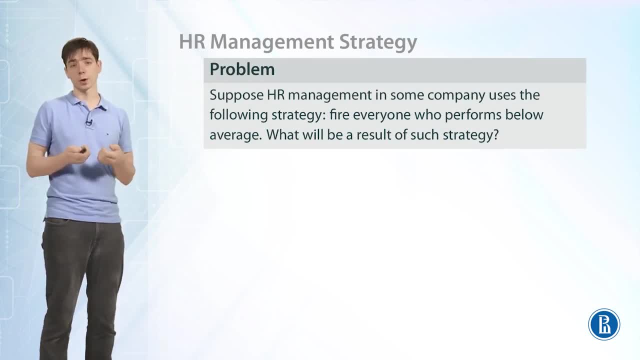 related to the notion of average. suppose we have a company and there is HR management in this company and they use the following strategy: we look at everyone's performance and they fire everyone who performs below average. so what will be a result of such a strategy? ok, this might sound reasonable. 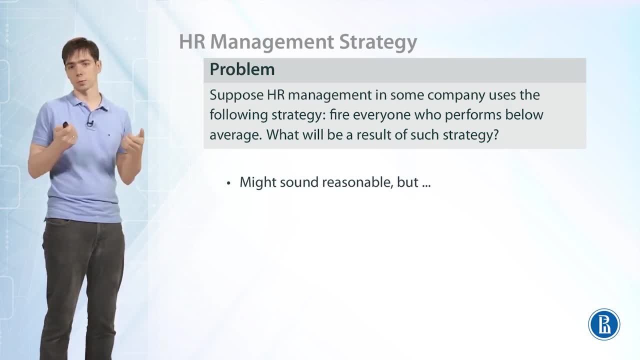 if someone works below average, probably the company should fire him. ok, but note that unless everyone works equally, which is an extremely rare case- it's very rare that two persons perform equally if we measure their work by some number. if it doesn't happen, if it is not the case that everyone works equally, 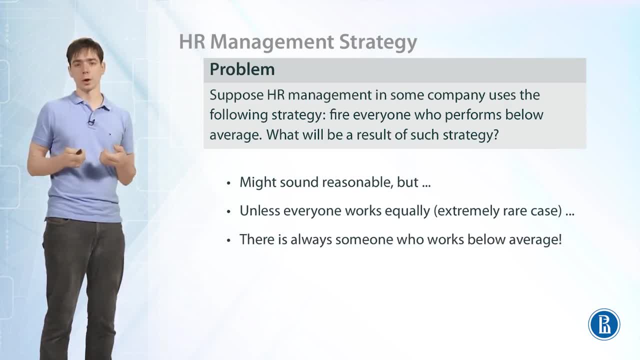 then there is always someone who works below average. average is something in the middle, so someone works better, someone works not that good, so there is someone below average because average is somewhere in the middle. so if we fire them, then the average performance will grow. we fired people who work below average. 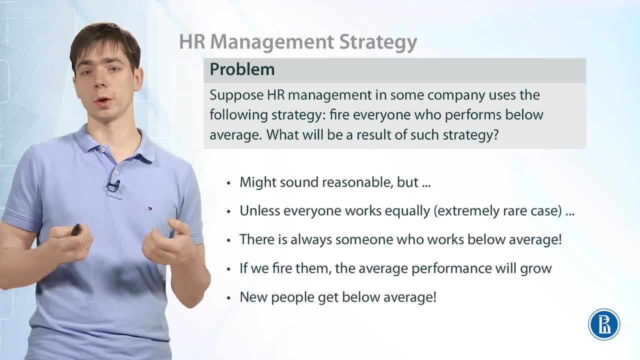 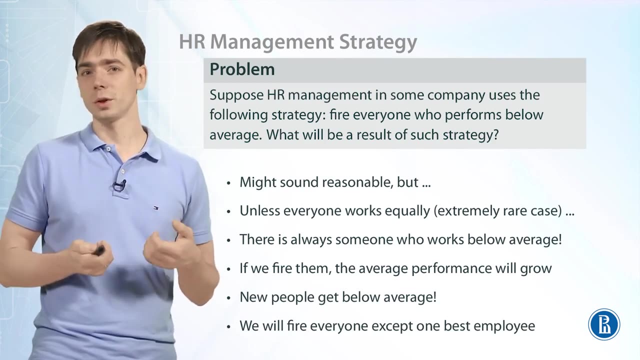 so the average will grow and then we will have new people below average, because if everyone doesn't work equally, then there is someone below average. if we repeat it several times, we will just be left with just one person who was the best employee. but is it good? 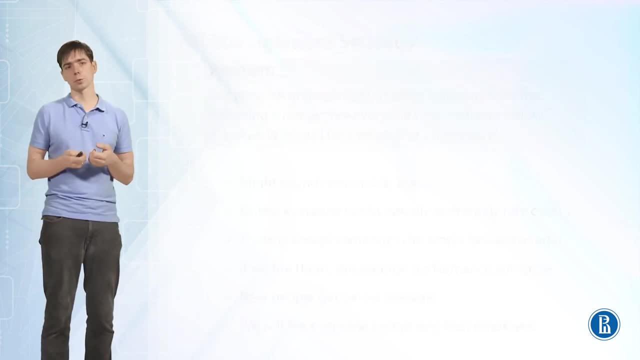 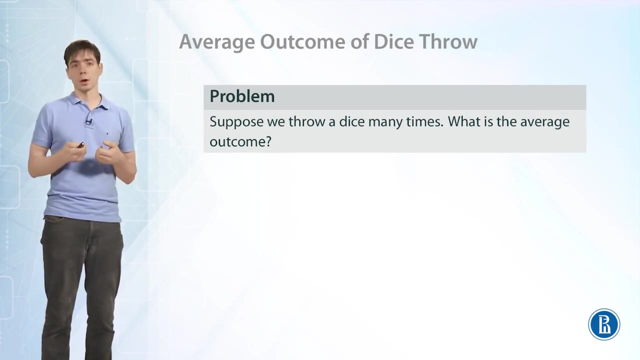 that we have only one person left. ok, let's move on to problems that are more related to random variables. suppose we have a dice and we throw this dice many times, and each time we have some outcome. what is the average outcomes of all of these throws? ok, can we give a precise answer? 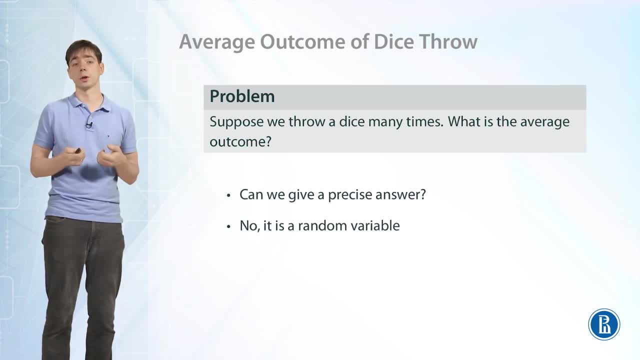 no, we cannot, because this is a random variable. if each time we have as a result 6, then the average outcome will be 6. this is quite improbable, but this is possible. if, on the other hand, each time we have 1, then the average will be also 1. 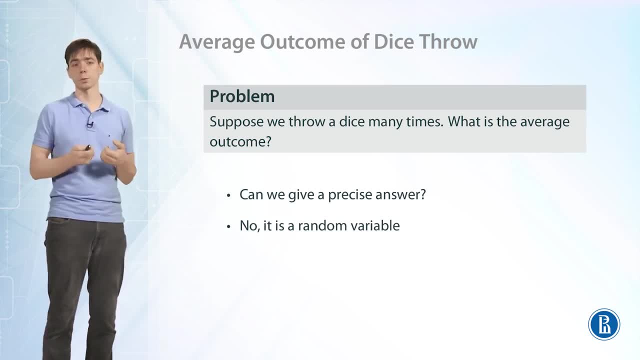 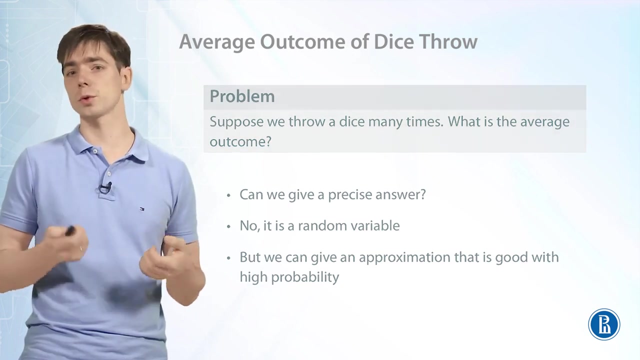 this is again improbable, but this is also possible. so there is no possibility to give some precise answer, which will be always the case, but what we can do. if we give an approximation to an average outcome, that will be a good approximation with high probability. ok, let's see what we can do. 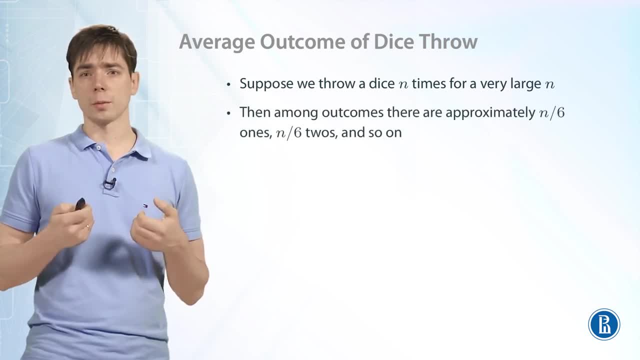 suppose we throw a dice n times and n is very large. then among outcomes there are approximately n over 6 ones, n over 6 twos and so on. so each outcome has probability 1 over 6. so in approximately 1 over 6 fraction of all cases 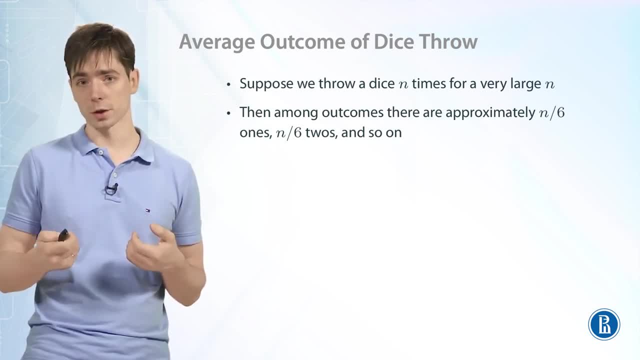 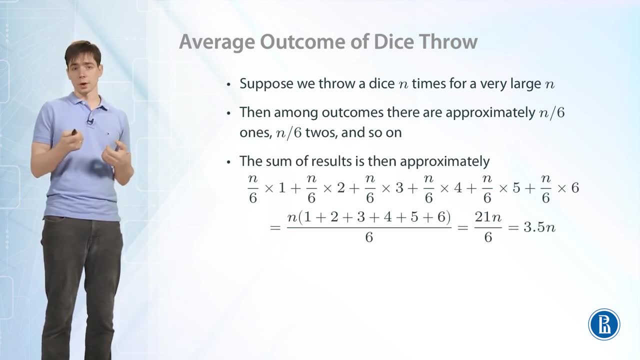 we will have 1 fraction of all cases. we will have 2, and so on. then now we are ready to compute the average, we have to sum up all of the results. so we have 1 over 6 times 1. so we have 1 n over 6 times. 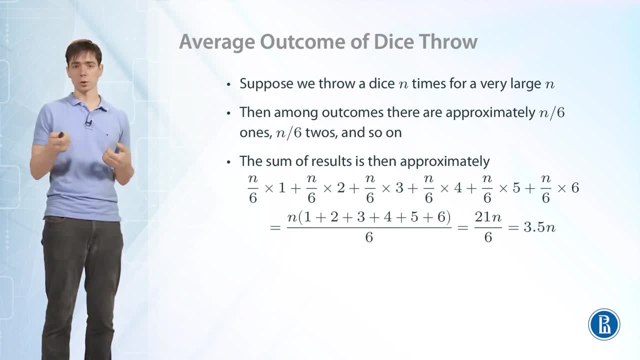 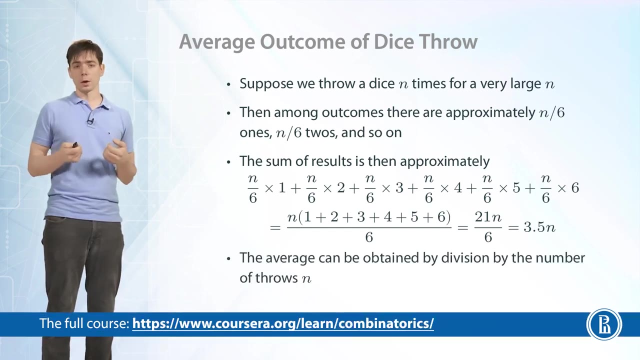 we have n over 6 times 2, and so on. so we sum all of this up, we can move n outside of the brackets and then we have 3.5 times n. this is the sum of all the results, approximately. ok, and now to obtain the average. 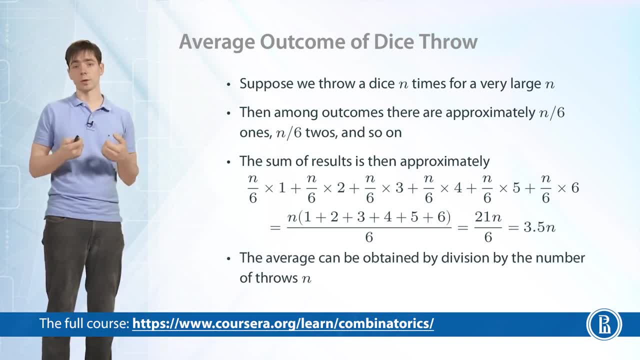 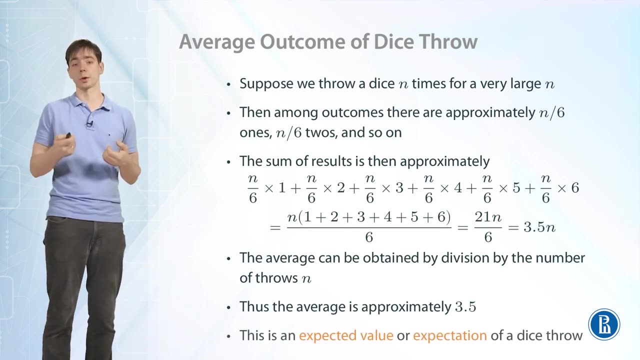 we have to divide by the number of experiments, we have to divide by n. we threw the dice n times, so we have to divide by n, so the average is approximately 3.5. ok, and this is called an expected value or an expectation of a dice row. 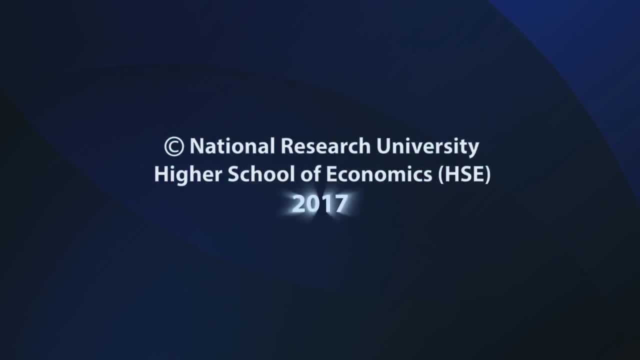 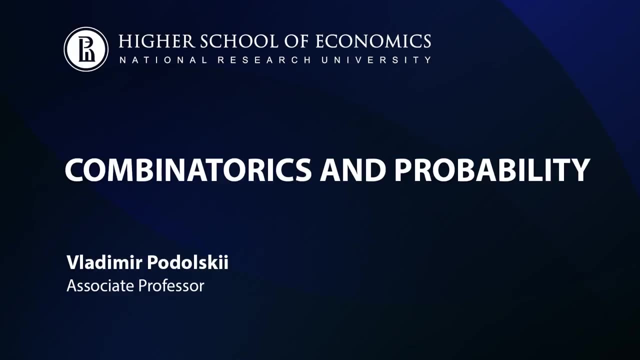 let's consider the notion of expectation in the general case. suppose we have a random variable and, for simplicity of presentation, let's assume that this is a random variable on the probability space of size 4. so there are 4 possible outcomes. the probabilities of our outcomes. 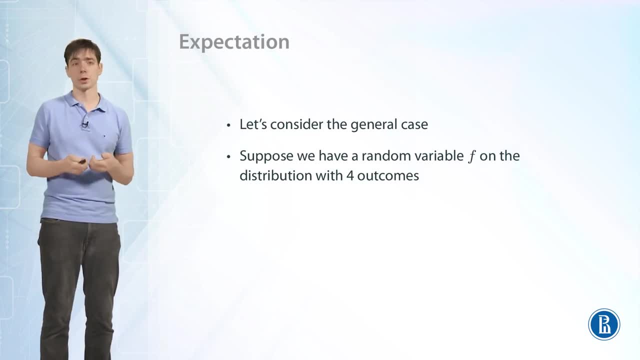 are denoted by: p1 is equal to p2 is equal to p3 is equal to p4 is equal to p5 is equal to p6 is equal to p1, p2, p3 and p4 and the values of the random variable on these outcomes. 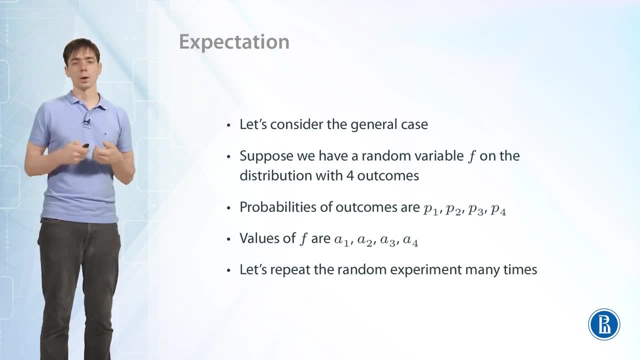 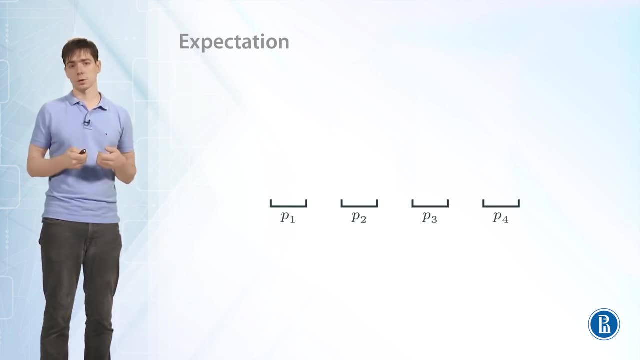 are a1, a2 and a3 and a4. ok, let's repeat the random experiment many times so we have these outcomes. let's run our experiment and, for example, the outcome was this one. then in the next experiment, the outcome was the first one. 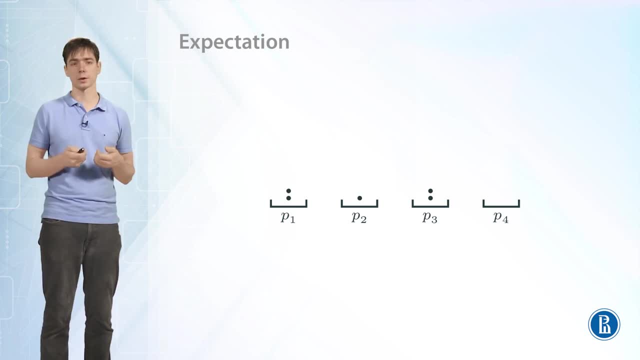 then again the third one, then the second one, the first one, the third one, again the fourth one, so we can run an experiment many times and in the end we will obtain some results. so we have repeated the experiment n times and n is some large number. ok, 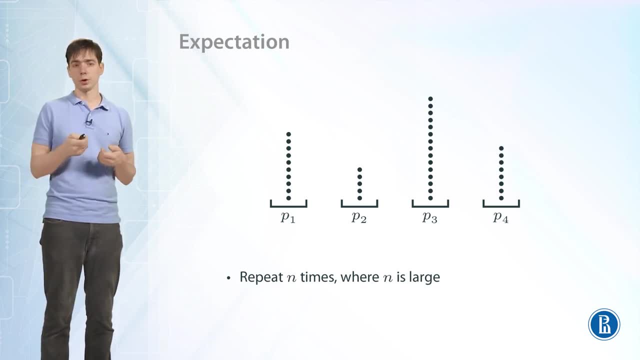 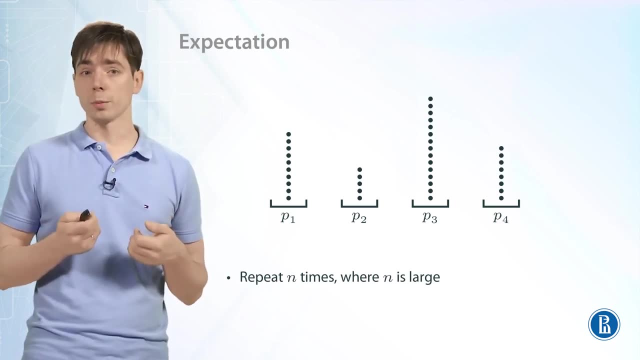 how many outcomes do we have in each of these piles, in each of these columns? we cannot say for sure, but we can say approximately the approximation will be good, with high probability, since each outcome, since each experiment ends up in the first outcome with probability p1. and we run n experiments. 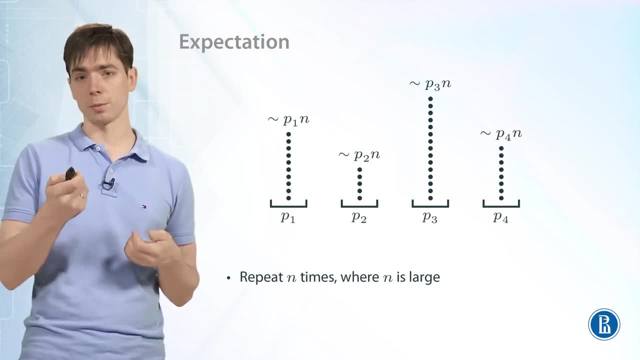 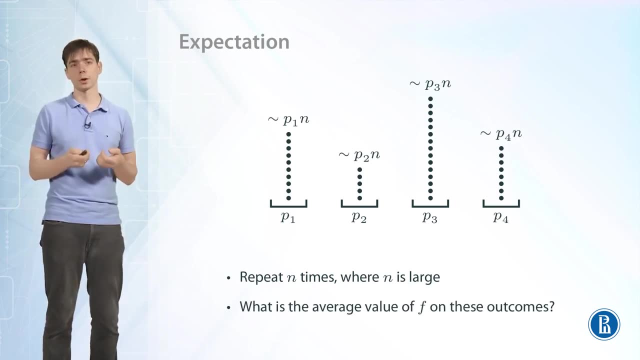 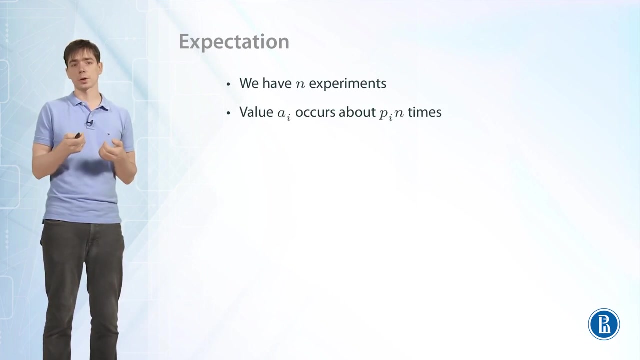 so we have approximately p1 times n in the first column, we have p2 times n in the second column, and so on. ok, let's see what is the average value of our random variable on all of these outcomes. so we have n experiments and an outcome, a sub i. 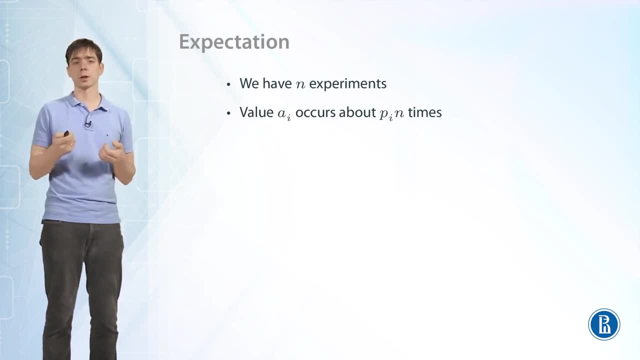 happens about p sub i times n times. so this is the number of times approximately that a sub i will occur among the results of our experiments. so to compute an average we have to add up all the results and divide by the number of values. so we have n experiments. 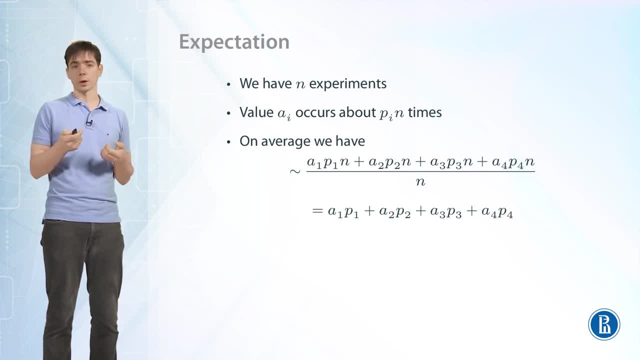 so we have n in the denominator, in the numerator we will have a1, approximately p1 times n times, a2, approximately p2 times n times, and so on. so we add all of these ups, we obtain this expression and note that n cancels out. so as a result, we have: 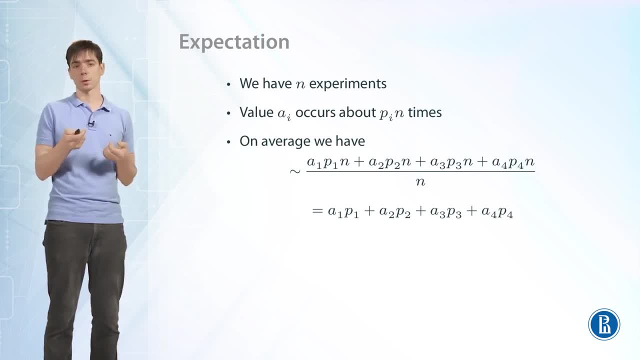 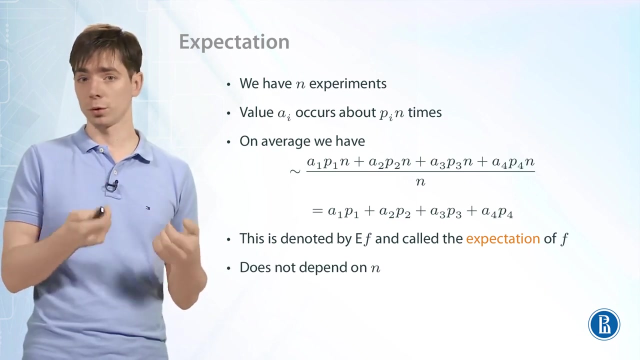 the following expression: a1 times p1 plus a2 times p2, and so on. ok, this value is called the expectation of f and is denoted by ef. note that this value doesn't depend on n we have. during the whole argument, we had n as the number of experiments. 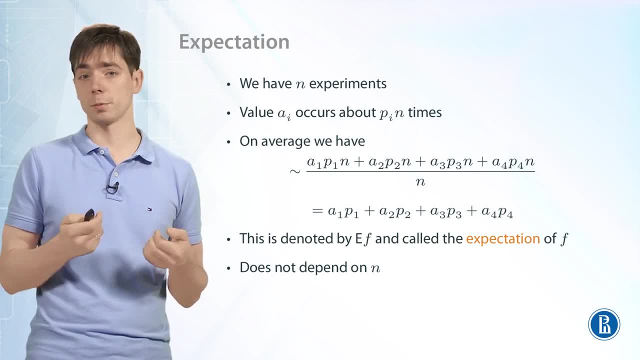 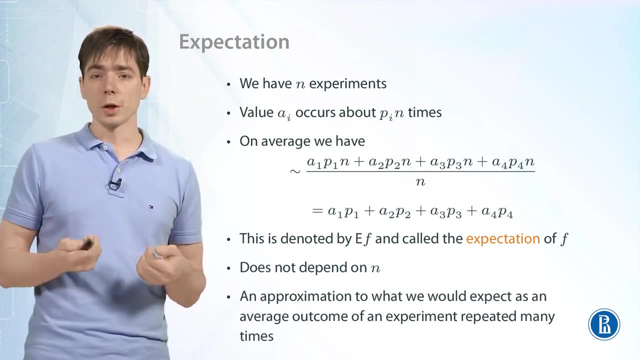 but in the end it cancelled out. so this number doesn't depend on n, it depends only on the random variable. and what is this number? this is an approximation to what we would expect as an average outcome. if we repeat our experiment many, many times, the same construction works in the general case. 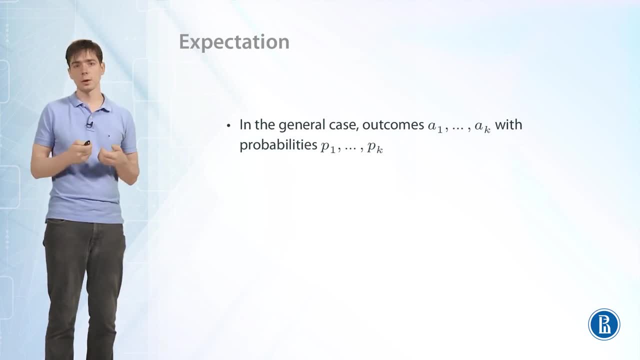 so if now our random variable has k, the values are a1 and so on and the probabilities are p1 and so on, then to compute the expectation we have to multiply ai times pi, for all i, and we have to add up the results from 1 to k. 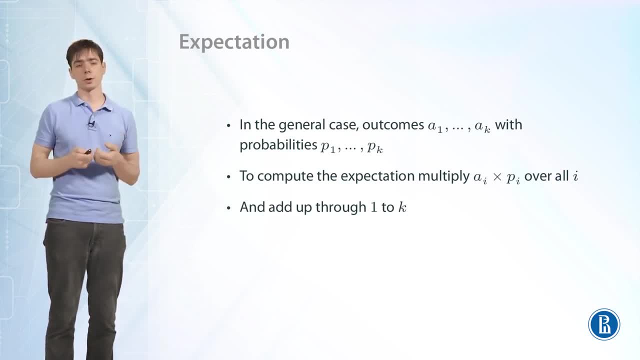 this will result in the expectation of our random variable. why expectations are important? first of all, expectation is a number, so it is a numerical characteristic of a random variable, and this is important and convenient. we can compare numbers, we can add up numbers. we can do a lot of things. 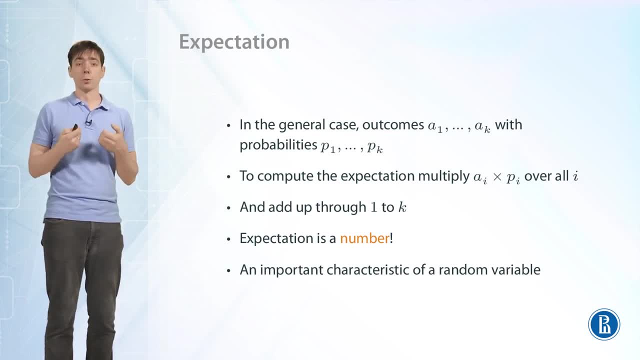 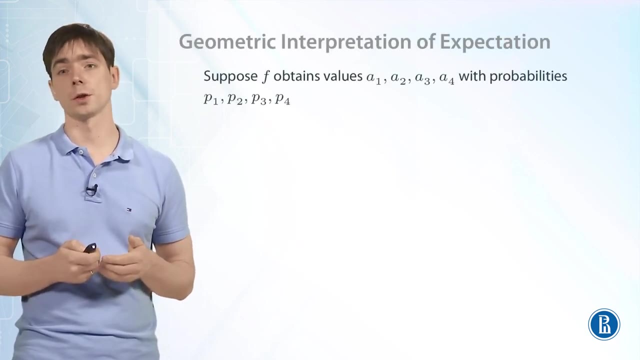 with expectations and, on the other hand, this is an important characteristic of a random variable. this is the average value and it reflects important properties of a random variable and it is very useful to get more intuition about expectations. let's also discuss geometric interpretation of an expectation of a random variable. 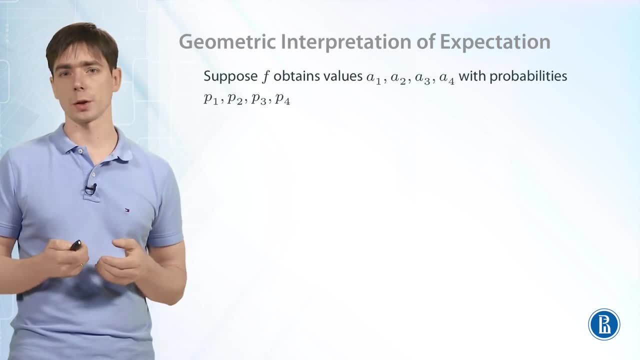 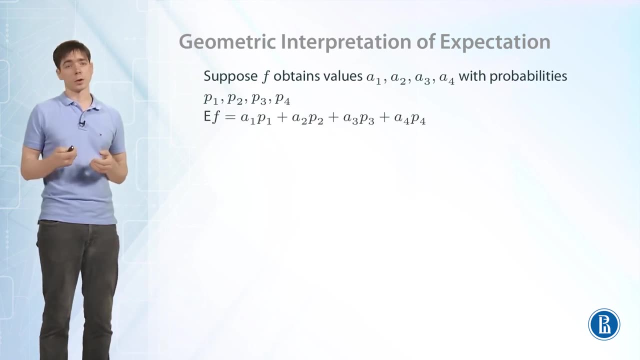 suppose we have a random variable f with four values- a2, a3 and a4- with probabilities p1, p2, p3 and p4- and its expectation is equal to a1 times p1 plus a2 times p2, and so on. ok, let's do the following. 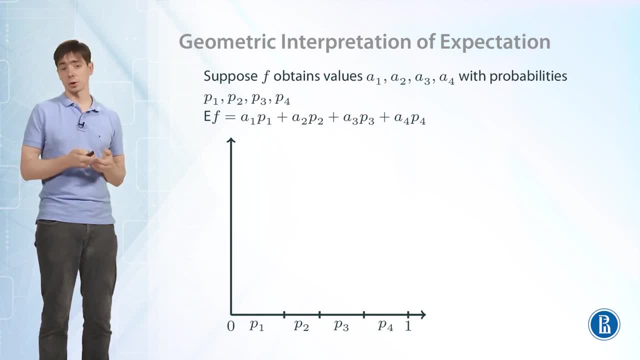 let's consider a system of coordinates and let's consider, on a horizontal axis, points 0 and 1 and let's consider interval between 0 and 1. now recall that the probabilities p1, p2, p3 and p4 add up to 1. 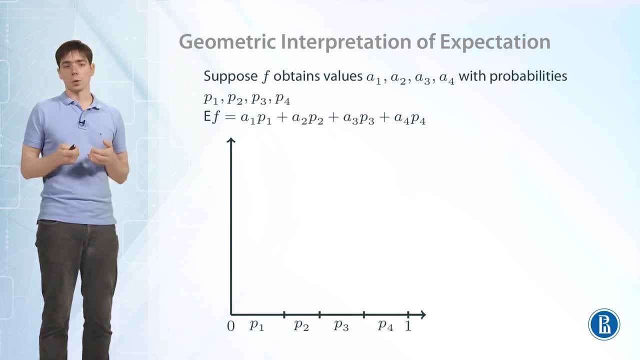 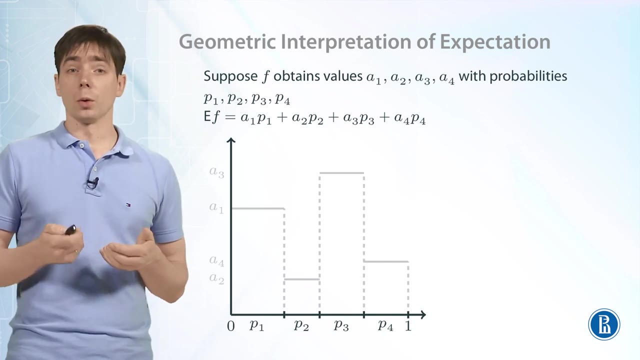 the probabilities should always be equal to 1, so we can do the following. we have an interval from 0 to 1 of length 1. let's break it into four intervals of length: p1, p2, p3 and p4 respectively. now let's consider the following. 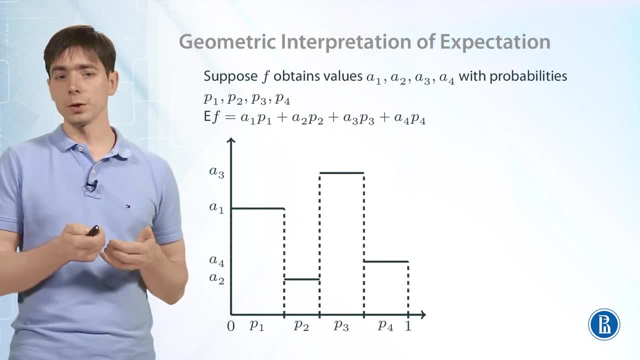 graph of some function. on the interval p1, the function is equal to a1. on the interval p2, the function is equal to a2, corresponding to the vertical axis. on the interval p3, the function will be equal to a3. on the interval of length p4, the function will be equal. 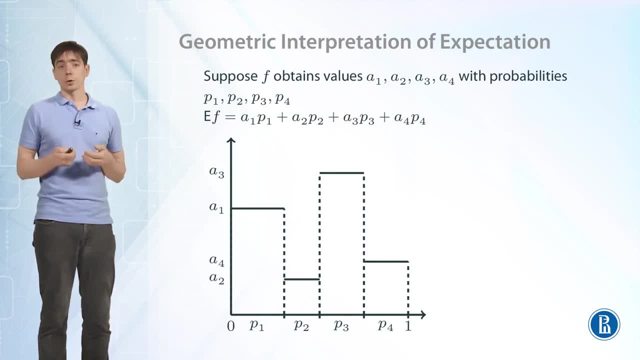 to a4. there is an intuitive correspondence between this function and our random variable f. just intuitively, let's say that that we throw a point, a random point, in the interval from 0 to 1. this is not a formal explanation, this is just an intuition. 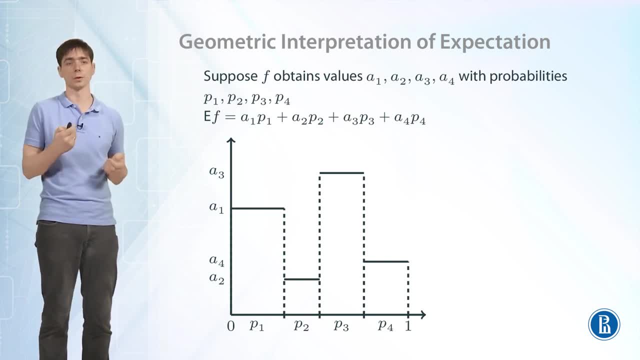 because formally we do not know what it means to throw a point into an interval. but let's intuitively say that we throw a point into an interval from 0 to 1 and all positions of the points are equal, so we do it uniformly. then what is the probability to get? 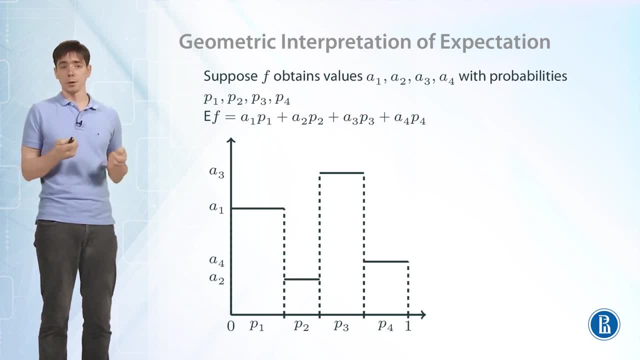 into the first interval. this probability will be p1. it's the fraction that the first interval takes into the large interval from 0 to 1. since the interval from 0 to 1 is of length one, then this fraction is just a length of the first interval. 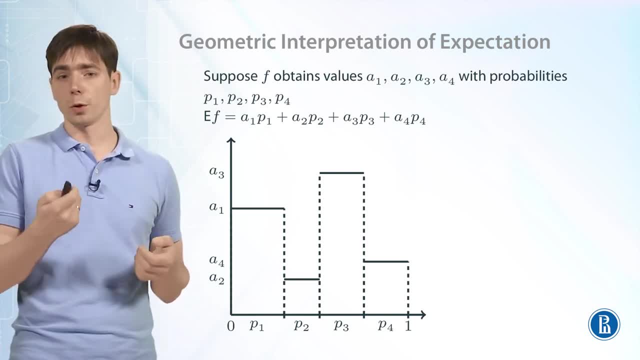 so it's p1. with probability p1, our point will get into a first interval. with probability p2, our point will get into the second interval. with probability p3, it will get into the third interval. p3 will get into the last interval. now let's look at the values of this function. 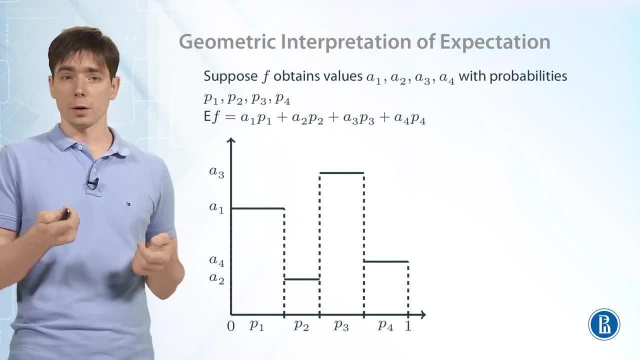 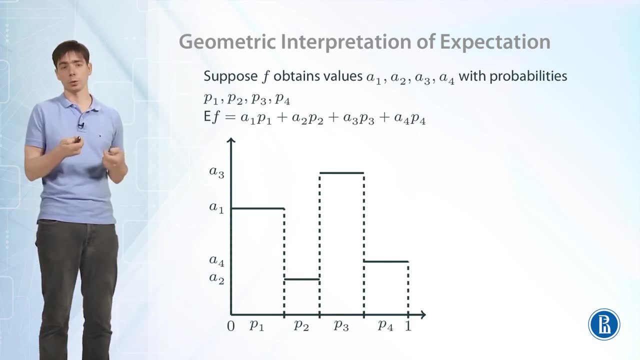 random point. In interval p1, this function is equal to a1.. So with probability p1, our function will be equal to a1.. With probability p2, our function will be equal to a2.. With probability p3, our function will be equal to a3.. And in the last interval, with probability 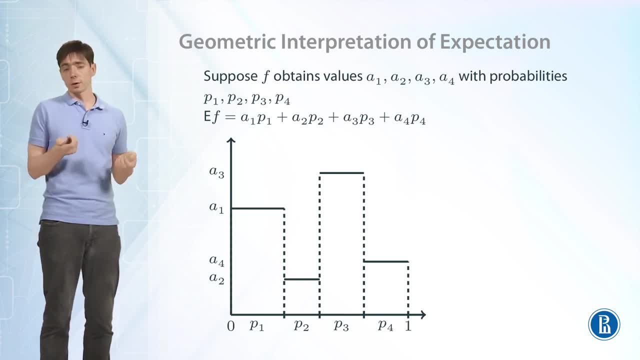 p4, our function will be equal to a4. So this function behaves on this random point which we throw into this interval, exactly in the same way as our function f. So we can speculate that this is a graph of our function. Of course this is just an intuition. 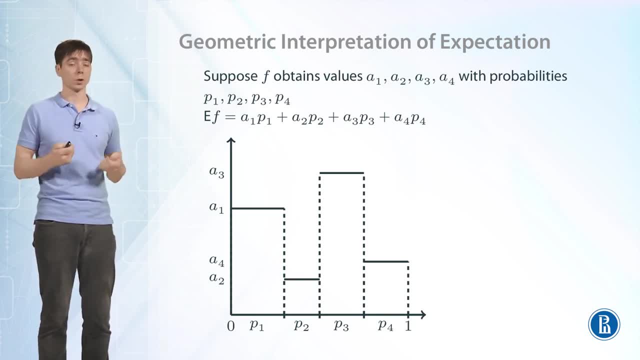 this is not a formal argument, But we can think of this picture as a graph of our function. Now, where is the expectation on this graph? And it turns out it has some very specific meaning. on this graph, It turns out that the expectation is the area below this graph. some of the areas of 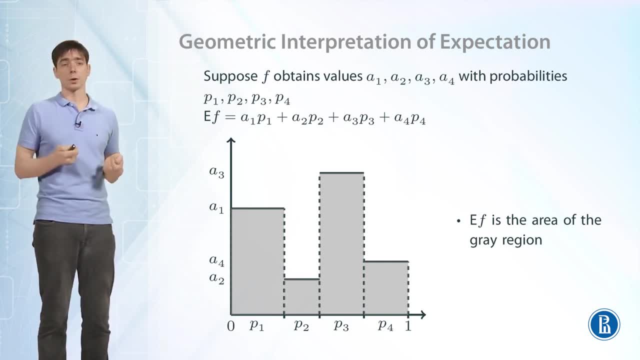 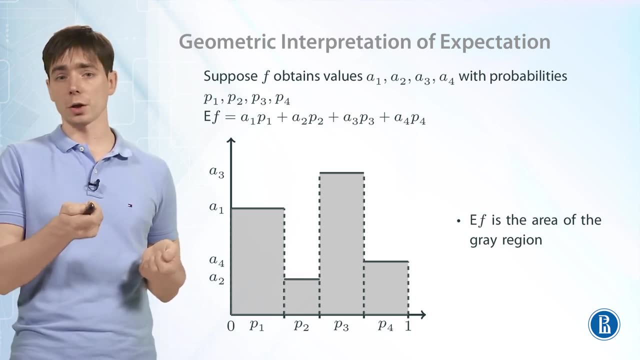 this four rectangles, And it is easy to see if we look at the definition of the expectation. Note what is the area of the first rectangle. Its dimensions are p1 and a1.. So the area is the product a1 times p1. And this is the first moment in the expectation For the second rectangle. 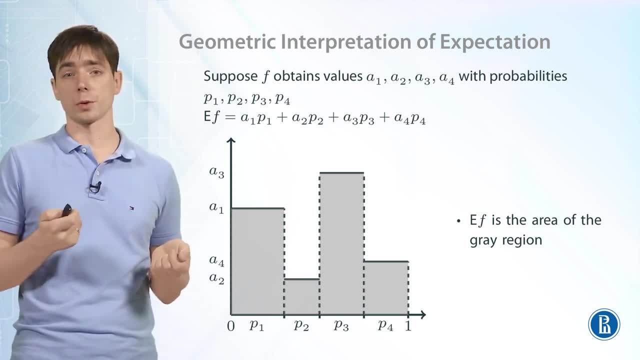 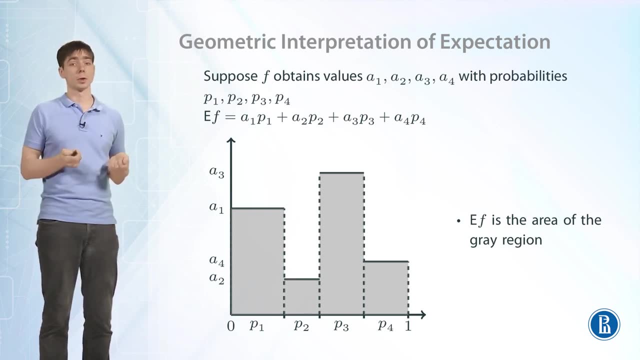 Its area is p2 times a2, and this is the second summand in our expectation And we proceed in the same way. so the sum of areas of all these rectangles is equal to the expectation of f. So if we think of f as a graph of this function, then the expectation is the area below the. 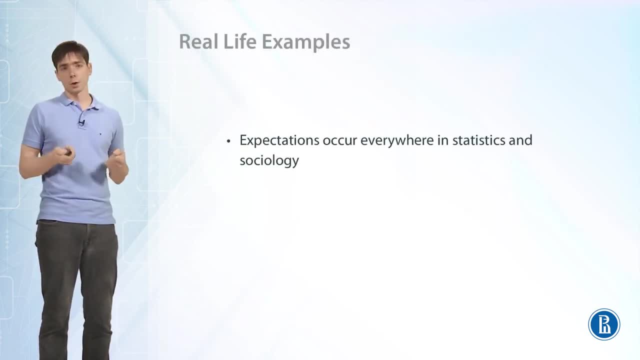 graph of this function. Okay, we have discussed expectations and actually they are used a lot in various fields. For example, they are everywhere in statistics and sociology. If we hear something about average age in some country or life expectancy, these are actually just expectations. these are expected values. 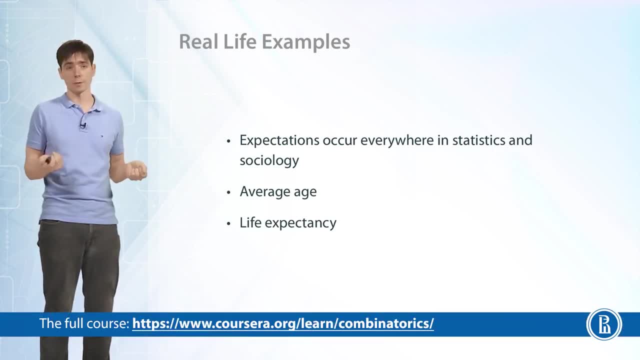 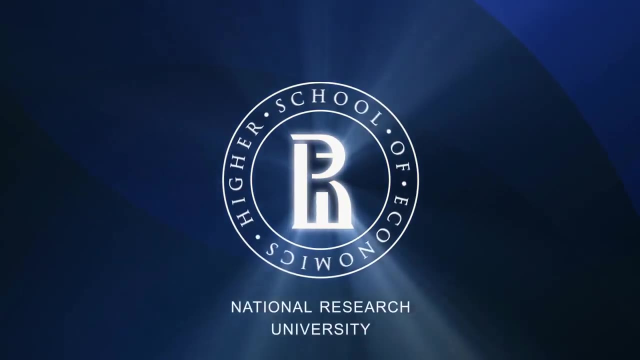 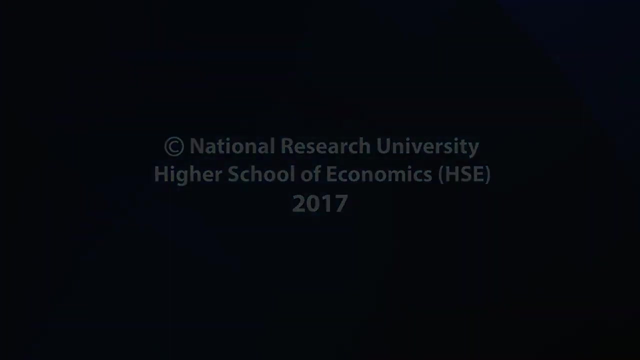 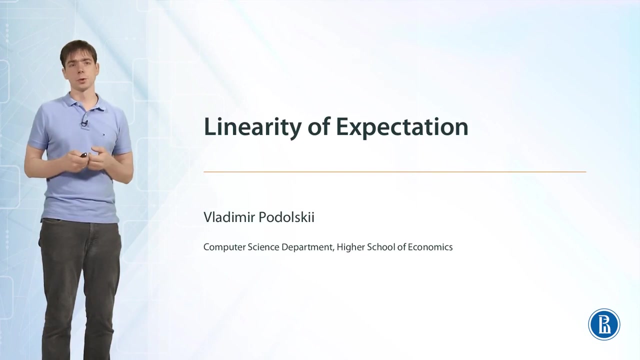 We pick a random person and see its age, so this is a random variable, and average age is the expectation of this random variable. So the same with average grades or average evaluations of students. Hi, I'm Vladimir Podolsky, and today we are going to discuss an important property of 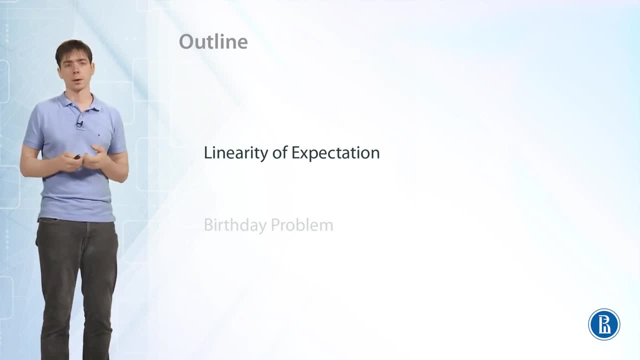 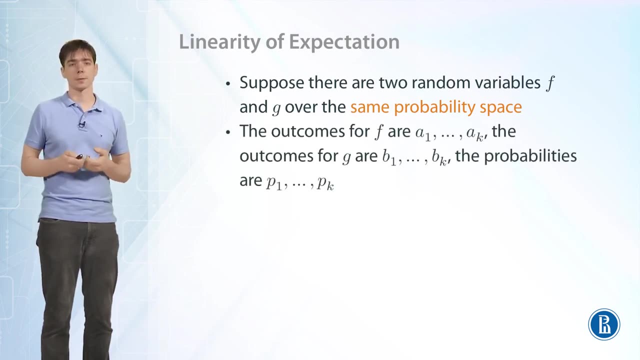 expectations of random variables – linearity. Suppose there are two random variables over the same probability space: two random variables, f and g. Suppose the outcomes of f are a1, and so on, ak and the outcomes of g are b1, and so on. 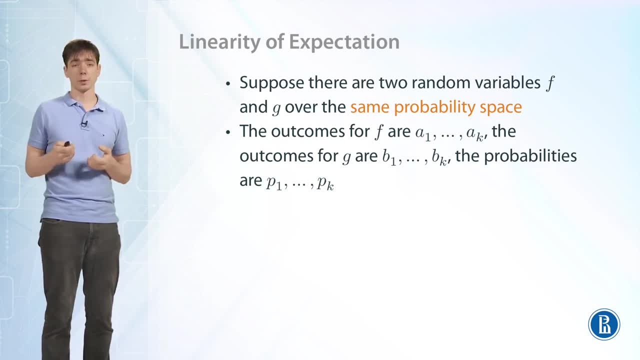 bk, and the probabilities of these outcomes are p1, and so on, pk respectively. Okay, now let's consider f plus g- And note that it is also a random variable- and again over the same probability space, The outcomes here are a1 plus b1, and so on ak plus bk and the probabilities again. 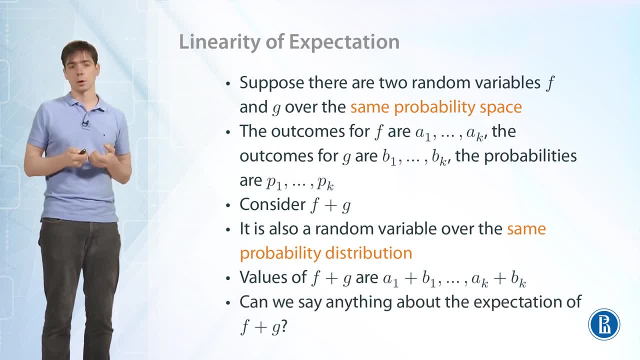 again IP1 and so on, PK. Now can we say something about the expectation of F plus G? F plus G is a new random variable. Can we say about its expectation at least anything? It turns out, yes, we can, We can do it. So it turns out that the 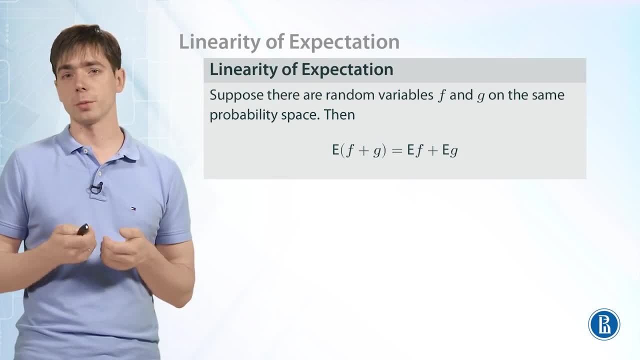 following holds: If you have two random variables, F and G, on the same probability space, then the expectation of F plus G is equal to the expectation of F plus the expectation of G, And this property is almost immediate. The proof is very simple, Indeed, So let's just use the definition of expectation and let's 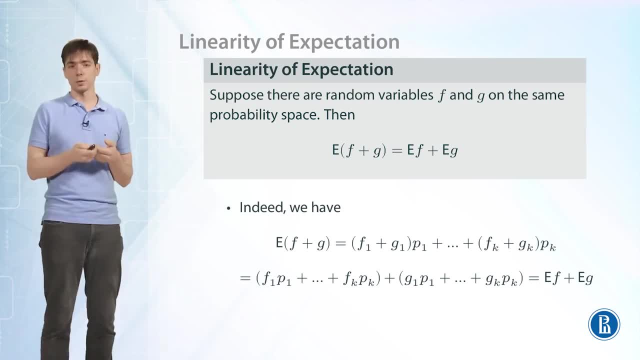 just write down the expectation of F plus G. If we do it, then we see that it is equal to F1 plus G1 times P1. So the value on the first outcome times the probability of the first outcome plus, and so on, plus FK plus GK. 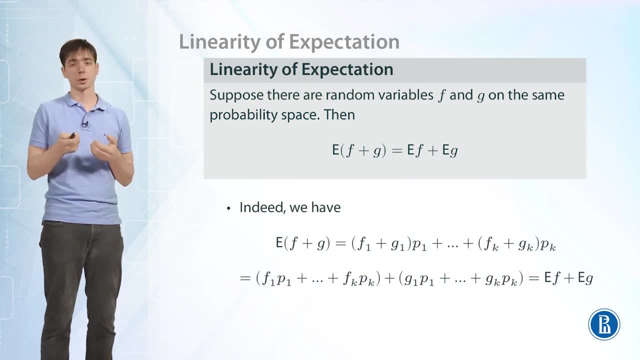 times PK. So the value on the last outcome times the probability of the last outcome. Now we can split this sum into two parts. In the first part, we will include all summands that contain F1 and so on, FK, And then the second part, we will include all summands that contain 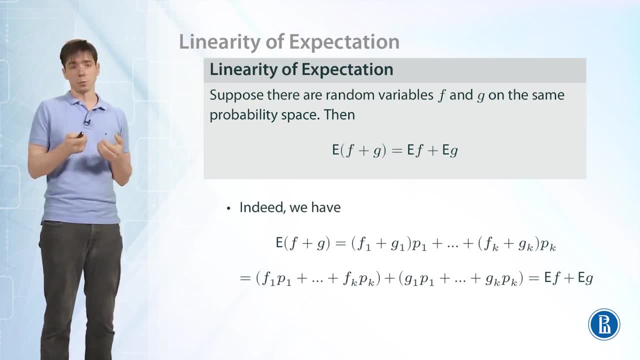 G1 and so on GK, And then the first part will be F1 times P1 plus and so on, plus FK times PK, And the second part will be G1 times P1 plus and so on, plus GK times PK. And now note that: 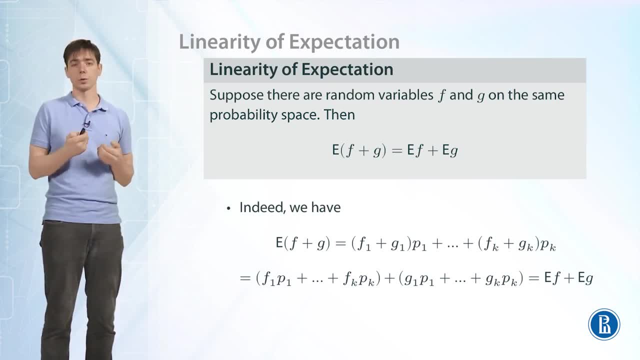 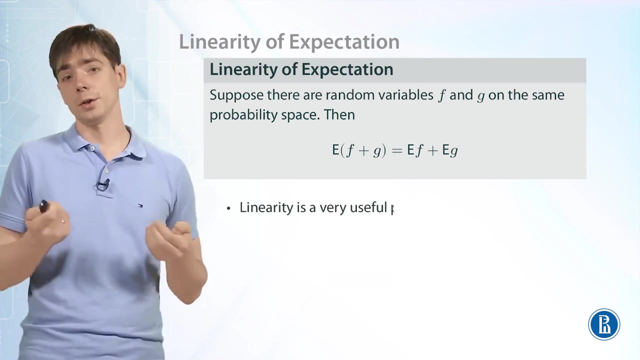 by the definition. if you look at the first part, it is equal to the expectation of F and the second part is equal to the expectation of G. So we obtained that the expectation of F plus G is equal to the expectation of F plus the expectation of G, which is what we needed to show. Now, linearity is a very 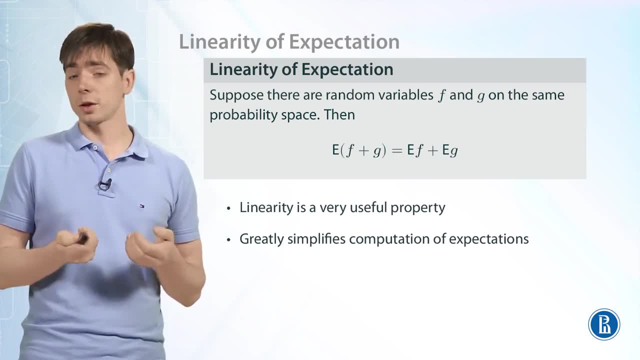 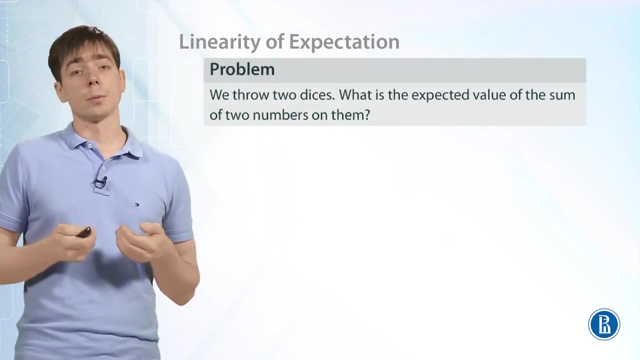 useful property and the idea is that it allows us to compute expectations of more complicated random variables through computation of expectations of more simple random variables, and this helps a lot. Let's see a couple of examples. Suppose the first, so let's consider the following problem: we throw 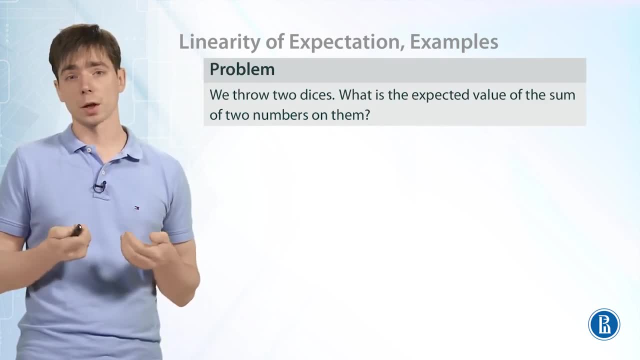 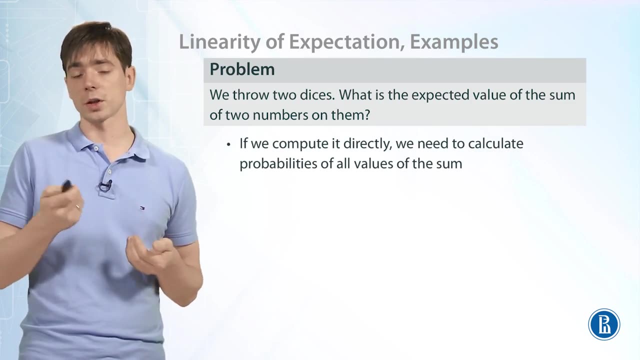 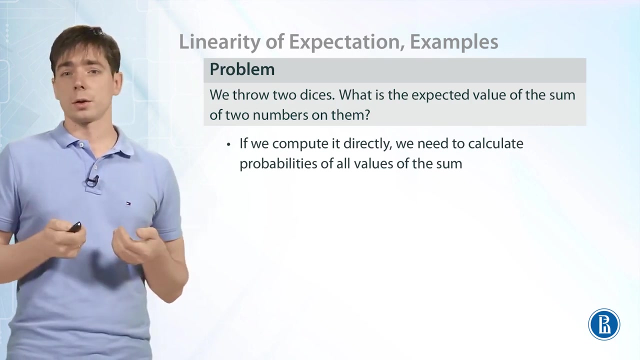 two dices, what is the expected value of the sum of two numbers on them? Okay, we can compute it directly. be throw two dices, there are six times six outcomes, so only thirty six possible outcomes. We can compute, just compute expectation directly. We can even not consider all 36 outcomes, we can just compute. 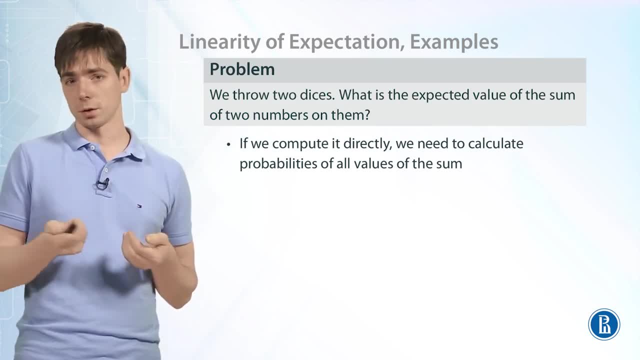 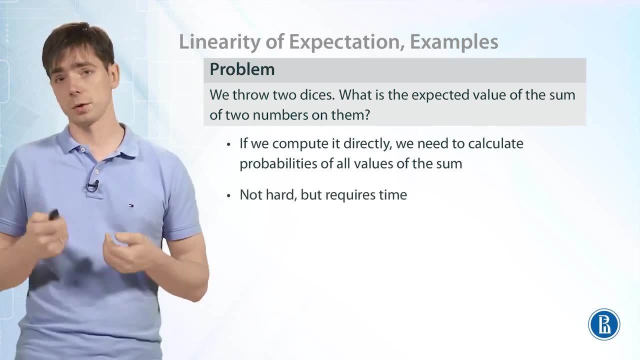 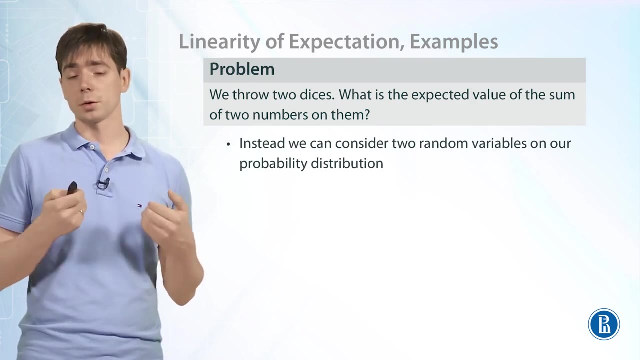 the probability of each value of this sum and write the expression for expectation. But this requires some work. This is not hard, but it requires to do something. But we will show. on the other hand, instead we will use linearity and we will show the same. so we will compute. 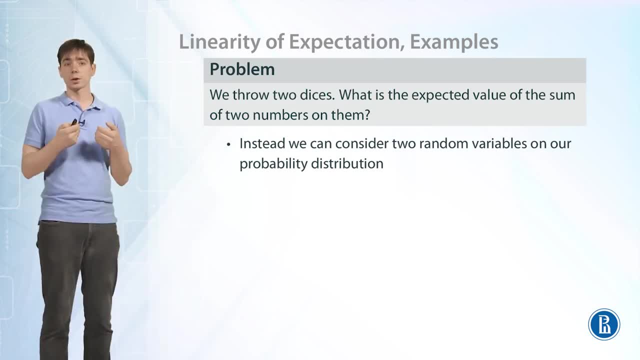 the expectation. almost immediately, We can, instead of this one random variable, the sum of values of two dices. we can consider two random variables on the same probability distribution. The first one is the value of the number on the first dice and the second random variable. 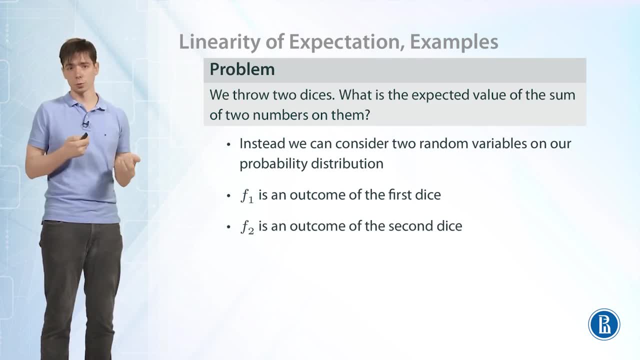 is the number on the second dice. So these are: we throw two dices and the first random variable is the number of the first dice, the second is the number on the second. So now we have two new random variables and note that we would like to actually compute the expectation of the 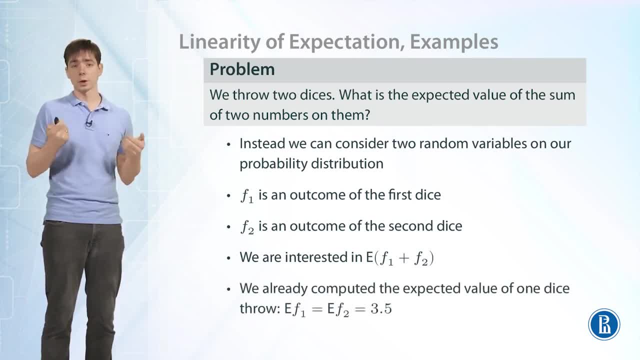 sum of these random variables And instead we can compute the expectation of each of them. And it is, first of all, it's very simple to do and, moreover, we have already done this, So we know that the expectation of each of these random variables is 3.5, and thus the 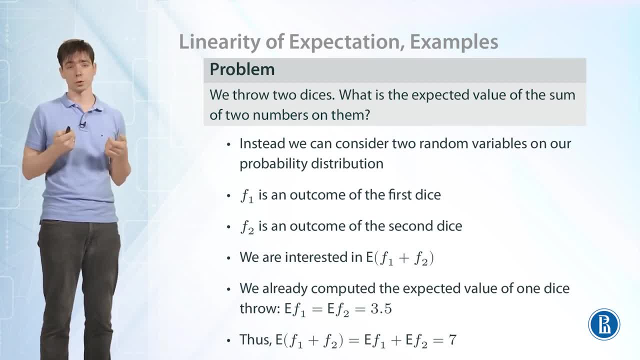 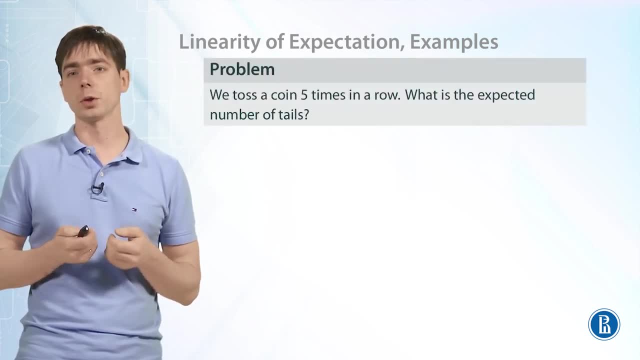 expectation of sum of two numbers on two dices is 7.. So let's consider one more example. Suppose we toss a coin five times in a row and we are interested in how many. what is the expected number of tails in these five tosses? Again, we can compute it directly From combinatorics we know. 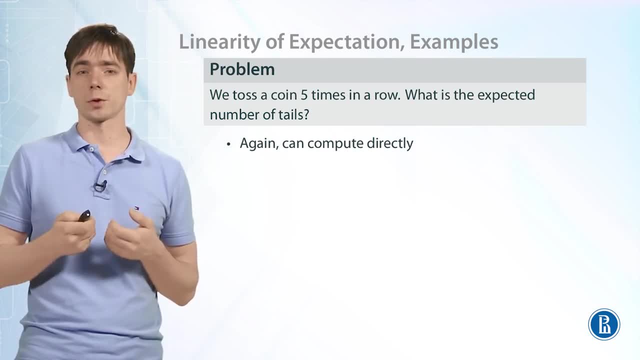 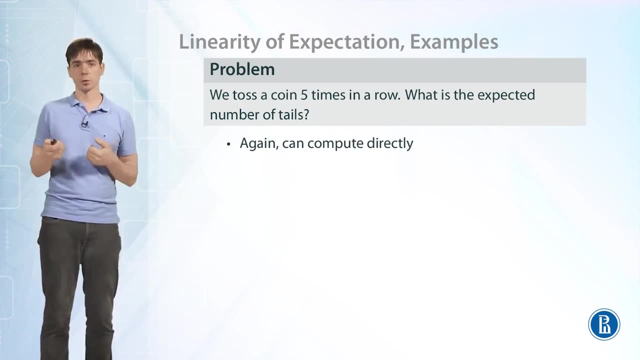 that there are two to the five possible outcomes. There are two possibilities for the first coin, two for the second, one and so on. So we have two times two times two, and so on. Two multiplied by itself, five times. So these are 32 outcomes, and we can just list them all and compute the. 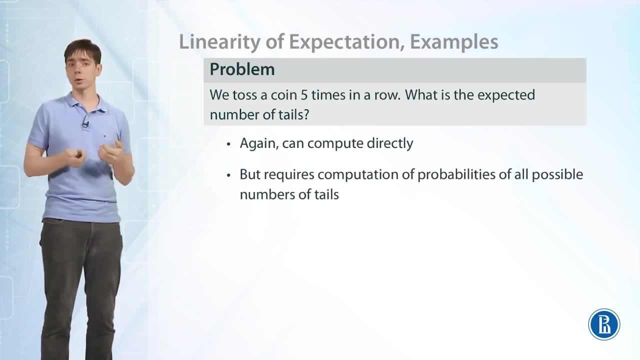 expectation directly by the definition. Okay, we can even do something more smart. We can try all possible values of this random variable of the number of tails. Possible values are from zero to five and we can compute the probability of each of them. This will require also some use of combinatorics. We will 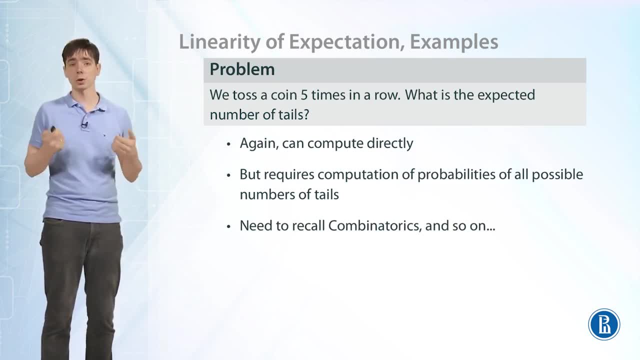 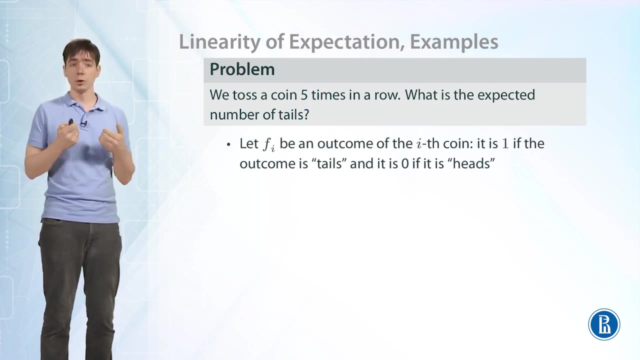 need to compute the number of combinations, So this requires some work in both of these approaches. Instead, we can use linearity and obtain the answer almost immediately. Indeed, let's introduce new random variables. Let phi i, f sub i be the outcome of the if coin, So f sub 1 is the outcome. 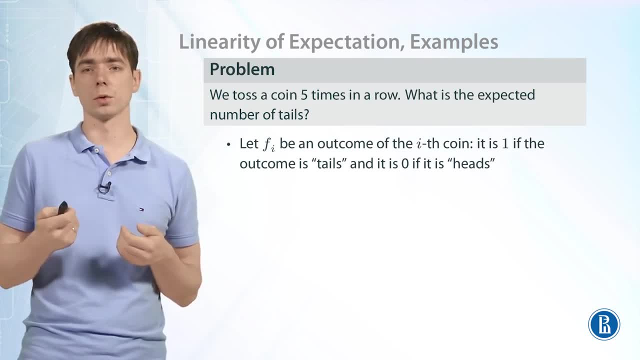 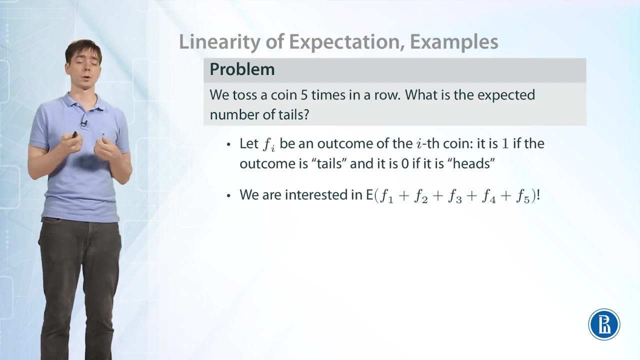 of the first coin, f2 is the outcome of the second coin, and so on. These values are equal to 1 if the outcome is tails and they are equal to 0 if the outcome is heads. Okay, to compute the number of tails, we have to sum up all these random variables. 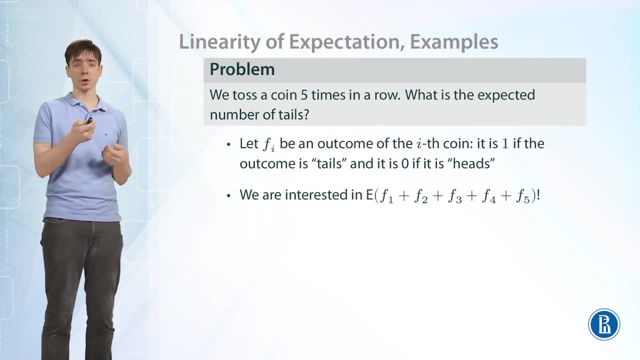 And now we are interested in the expectation. We are interested in the expectation of sum f1 plus f2 plus f3 and so on. So that's what we need to compute. And again, we can use linearity readily, So we can just compute the expectation of each of these random variables and add the results. 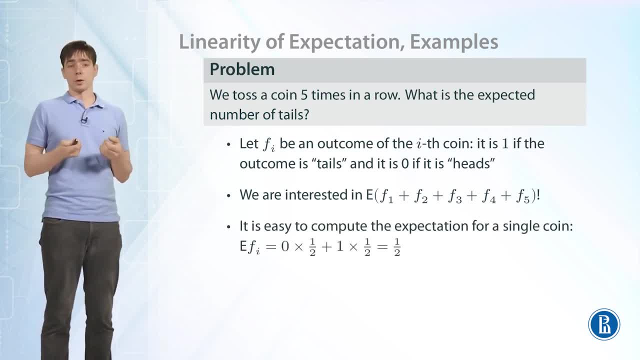 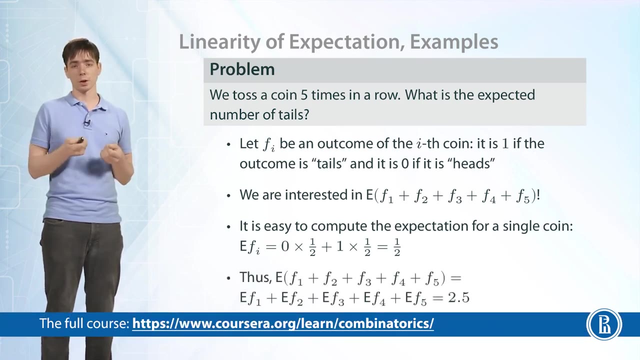 Okay, so what is the expectation of each of these random variables? The value, the output of this random variable is zero with probability one-half, and it is one with probability one-half. So overall, the value of this expectation is equal to one over two. And if we sum this up, 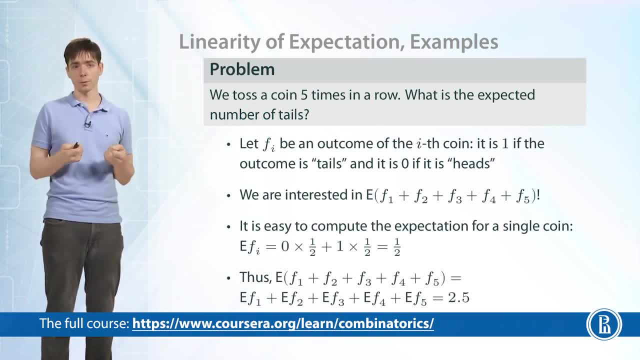 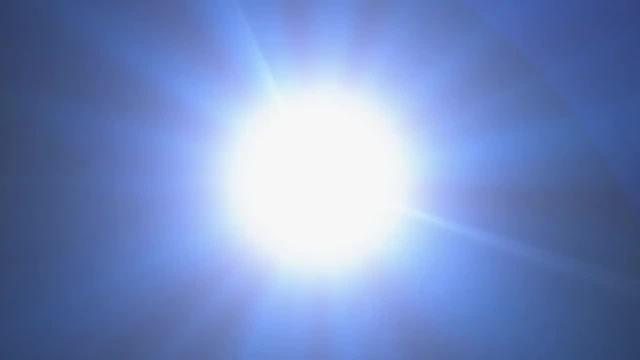 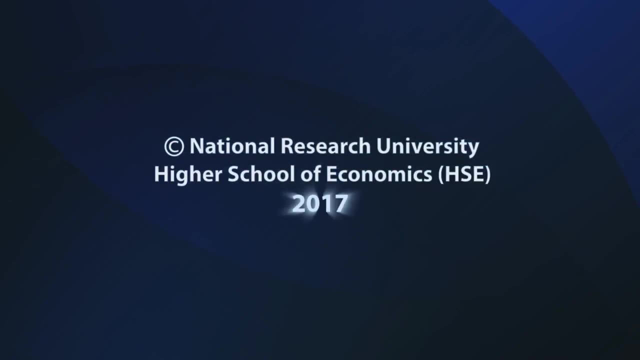 then we will have that. if we have five coin tosses, then the expected number of tails is 2.5. And that is equal to 0.5 times f1 plus f3 plus f2 minus f2, times f3 plus f3 minus f2.. 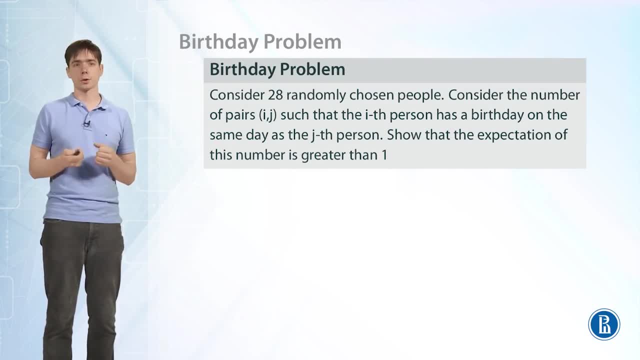 Consider the following problem: There are 28 randomly chosen people and we are interested in the following pairs: Pairs i- j, such that a person with no i has a birthday on the same day as the person with no j, And we are interested in the number of such pairs. 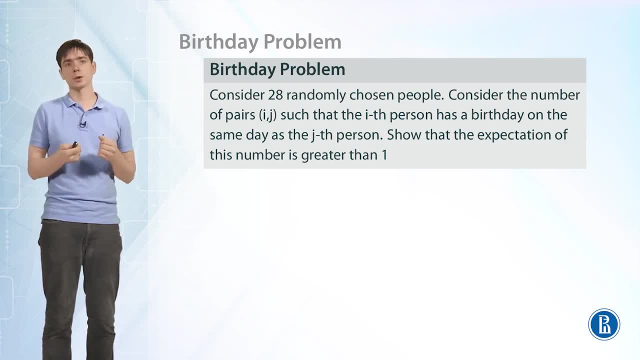 that the expectation of this number is greater than one. That means that, on average, we will have at least one pair of people with the same birthday. Okay, let's discuss in more details what are these pairs and what are we computing If there are two people with the same birthday? 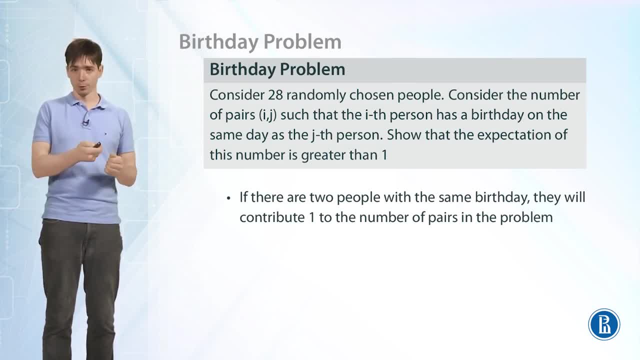 then they form a pair of people with a birthday on the same day. So they contribute one to the number of pairs we are interested in. If there are three people with the same birthday, they will form three pairs. If we have three people, then there is a pair of the first one and the second. 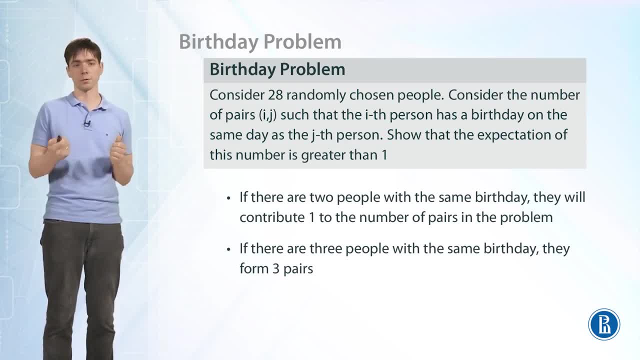 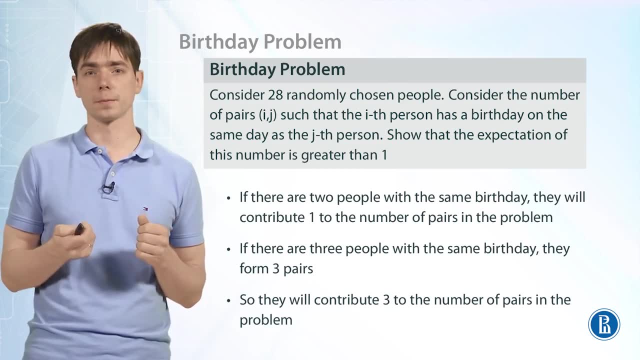 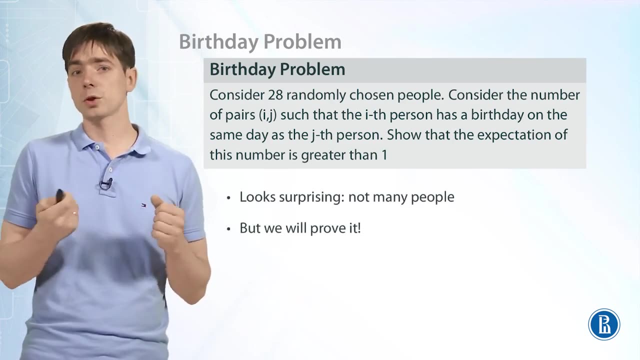 one, the second one and the third one, and a pair of the first one and the third one. So these people will contribute three to the number of pairs we are interested in. So that's what we are going to compute. Okay, the problem looks a bit surprising. So there are just 28 people and we are saying that. 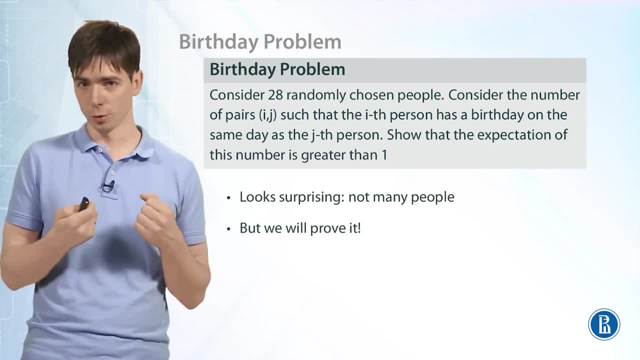 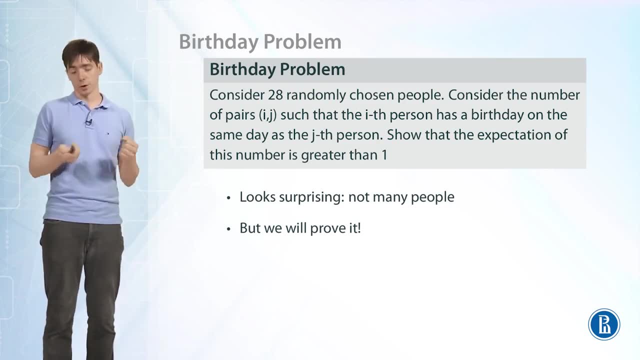 it is fair to expect. it will be good to expect that there are two of them with the birthday on the same day, But we will show that this is indeed the case. Okay, on the other hand, we have to formalize the problem. On the other hand, we have to formalize the problem. On the other hand, we have to formalize the problem. 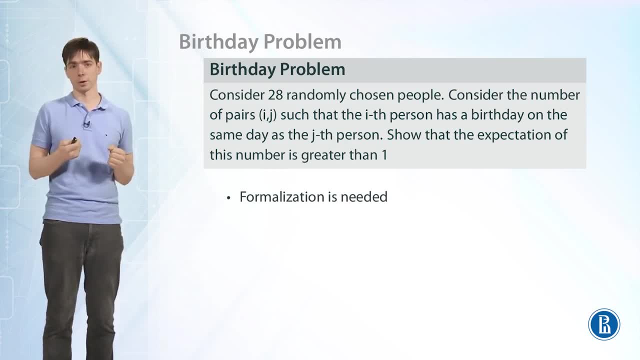 a little bit, So the current statement is not completely formal. We assume for this problem that birthdays are distributed uniformly among all days of the year And we assume that there are 365 days of the year. for simplicity, We will not discuss it. but 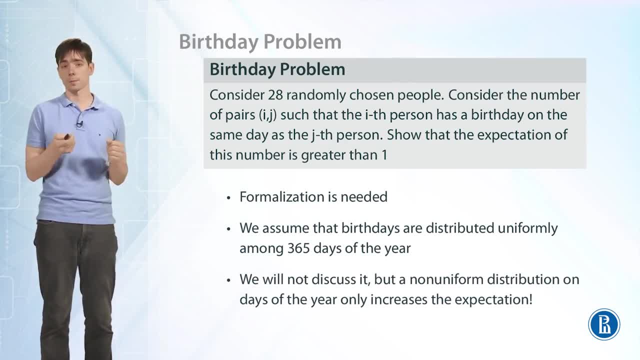 actually, if the distribution of birthdays among days of the year is not uniform, which is the case in real life, then this expectation will only increase. But for simplicity, we consider it a uniform distribution among all days. Also, we have to specify that we 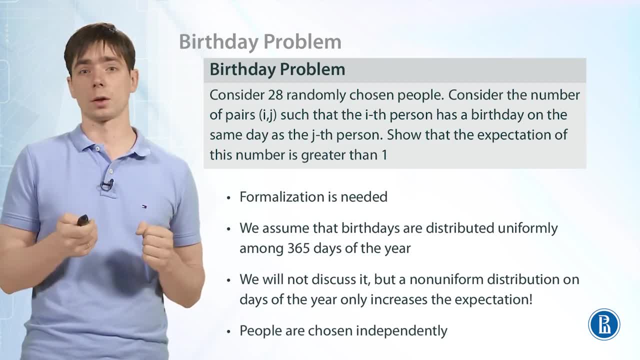 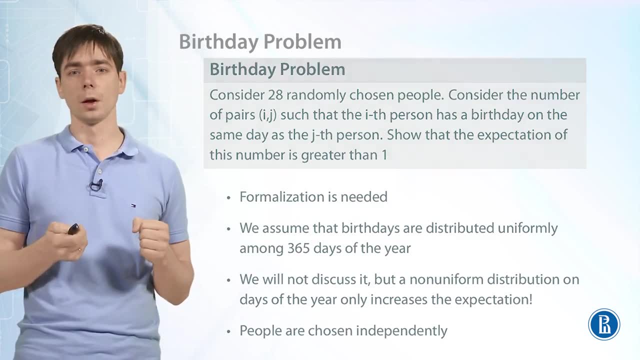 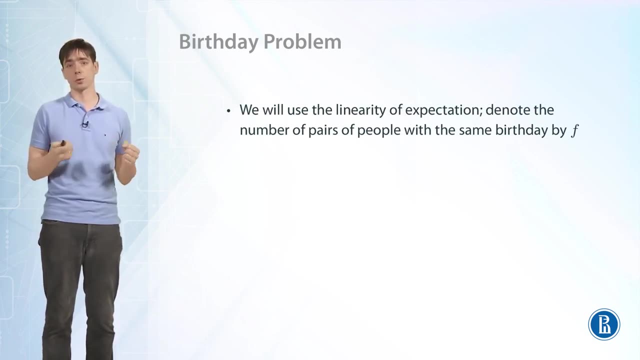 choose people independently and uniformly. Randomly here means that we just pick random people with random birthdays. Okay, let's proceed to the proof. Of course, we will use the linear approach before making any changes. use the linearity of expectation here to compute, to have a bound on the expectation we are. 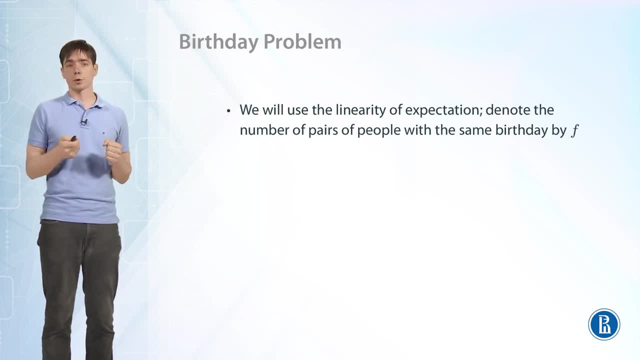 looking at. Let's denote the number of pairs of people with the same birthday, the number we are looking at by f. This is a random variable And let's introduce more random variables. Let's enumerate people from 1 to 28.. 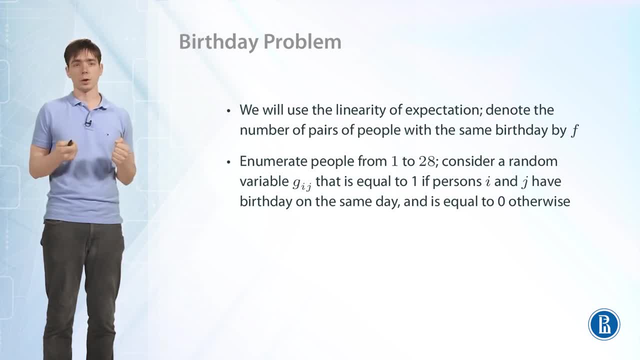 And let's consider a random variable: g sub ij. It will be equal to 1 if persons i and j have a birthday on the same day, and otherwise it will be equal to 0.. And now an important observation: f is equal to the sum of all gij over all unordered pairs of i and j. 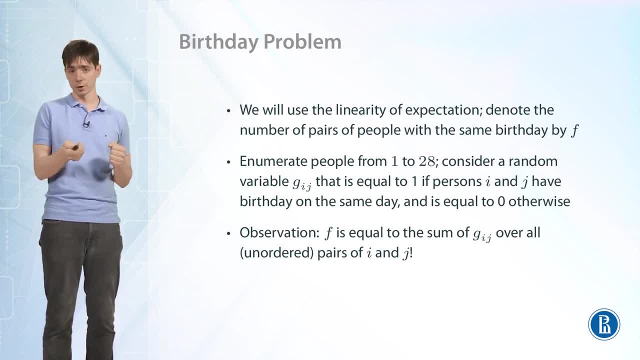 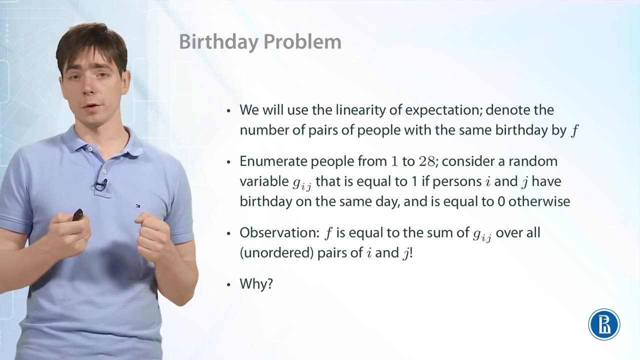 That's an important observation we will make, And note that this is the observation that will help us to use linearity. We break our complicated logic. We break random variable f into the sum of more simple random variables. But let's see why this is true. 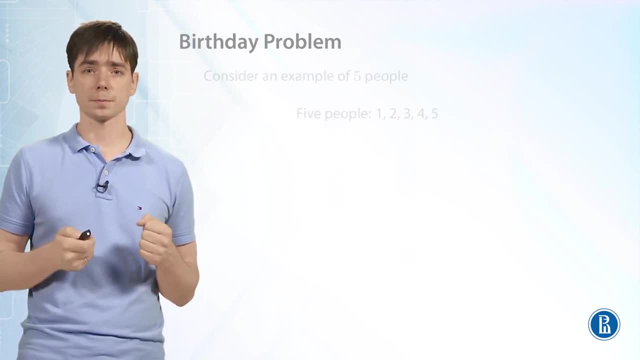 Why f is equal to the sum of all of these random variables. And let's consider an example. It's easier to see an example. Suppose we have 5 people: 1,, 2,, 3,, 4,, 5.. 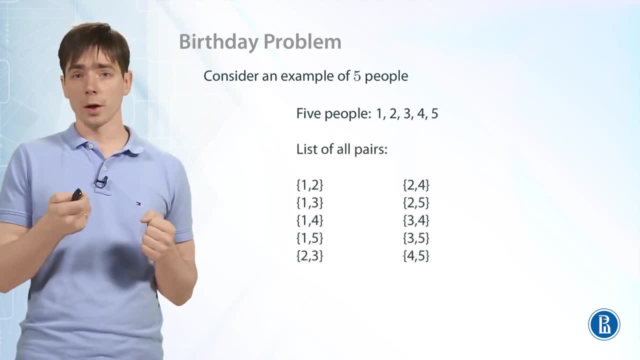 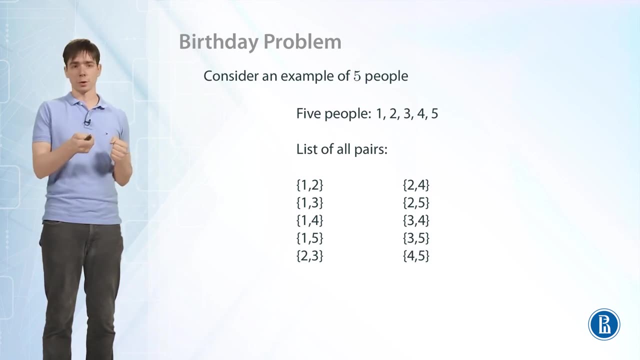 And let's just list all of the pairs. There are 5. choose 2 pairs, which is 10.. And here they are all listed. First we have 5. We list pairs which contain person number 1.. Then we list pairs that contain person number 2.. 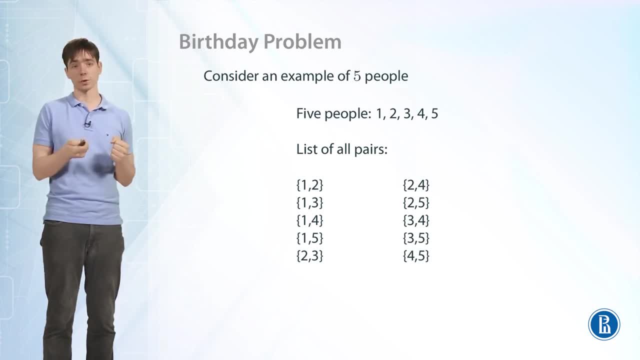 Then we list pairs that contain person number 3 and that wasn't counted before. And there is finally one pair that doesn't contain anyone among persons 1,, 2, and 3. This is a pair 4 and 5. So we have 10 pairs. 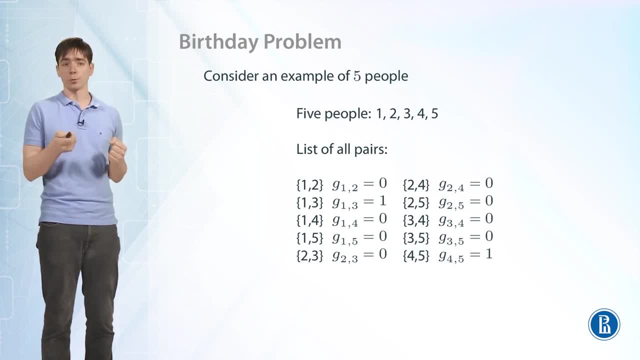 And suppose the following happens: The first person and the third person have the same birthday, And the fourth and the fifth person have the same birthday. So then the values of our new random variables are like this, So they are all zeros except two cases. 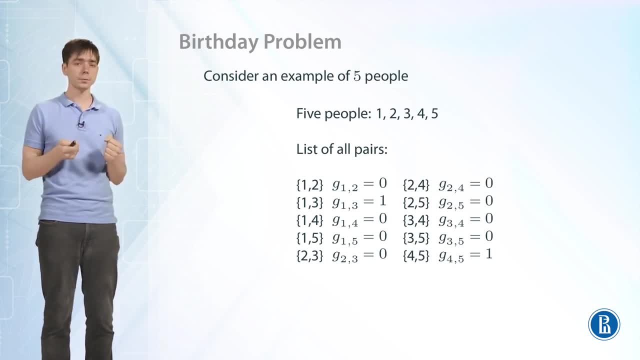 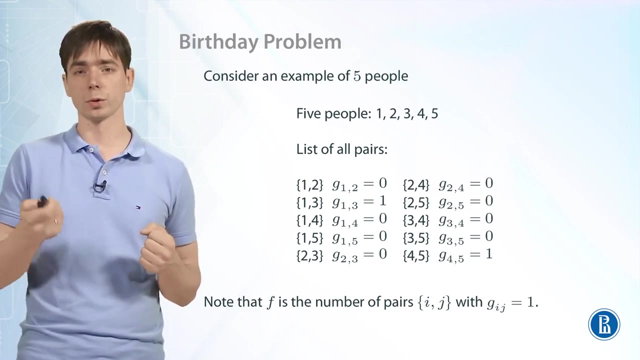 Except g and g. Note that f in this case, is equal to 2.. There are 2 pairs of people That have a birthday on the same day, And note that, on the other hand, the sum of all g is also equal to 2.. 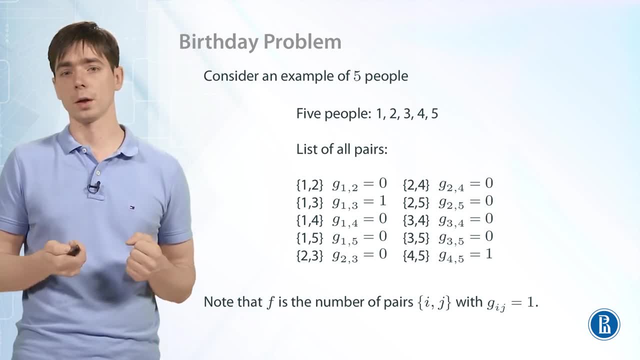 Because exactly two of them are equal to 1 and others are equal to 0. So in this case it is easy to see that f is equal to the sum of all g. It is just the number of pairs, such that g is equal to 1.. 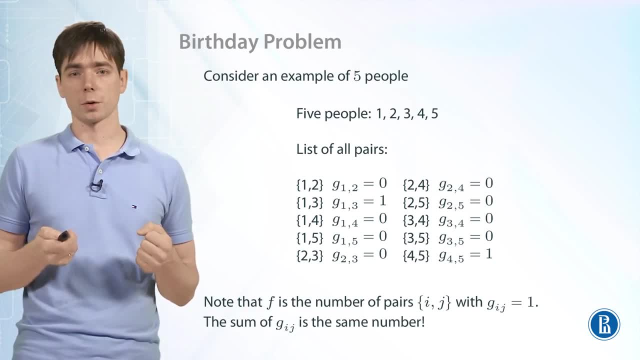 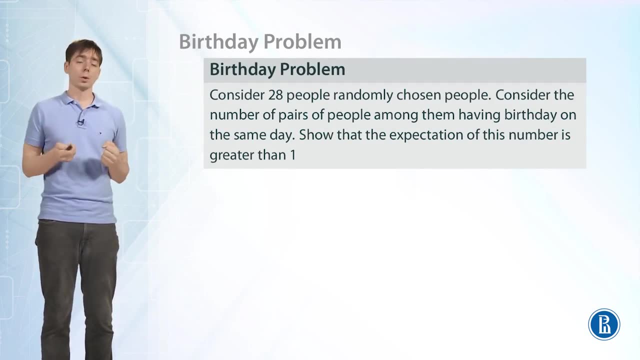 And if we sum up all g, we will obtain exactly the same number. So that's why we have this. So that's why we have this. We have our property we will use. Okay, now let's get back to the proof. 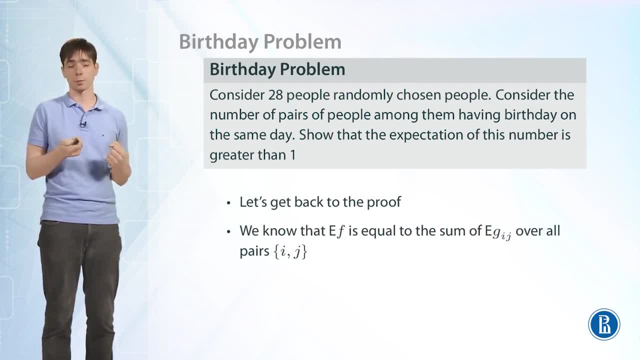 We know now that the expectation of f is bilinearity, is equal to the expectation, to the sum of all expectations of all g over all pairs, And there are two things left. We need to compute these expectations, These expectations of simple, random variables. 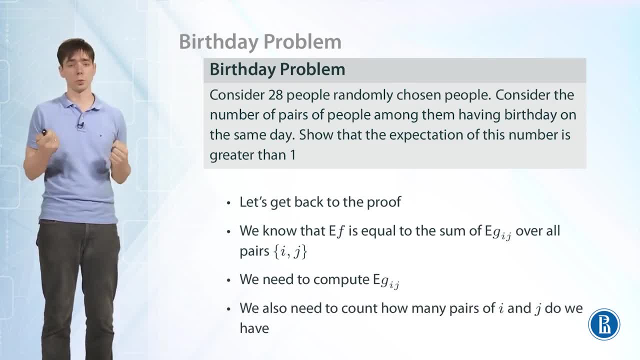 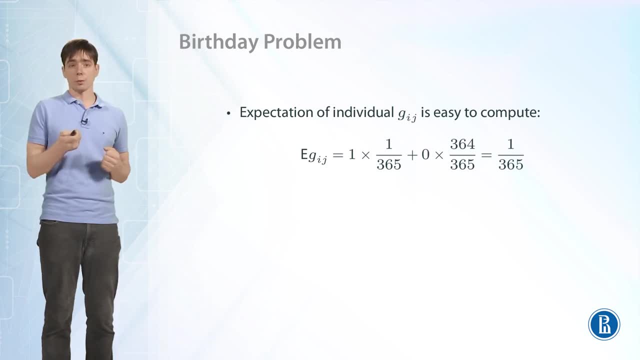 And second, We need to count how many pairs of i and j do we have. Okay, let's proceed to the first task. Let's compute the expectation of individual g, And it is very easy to compute Because this value has only two outcomes. 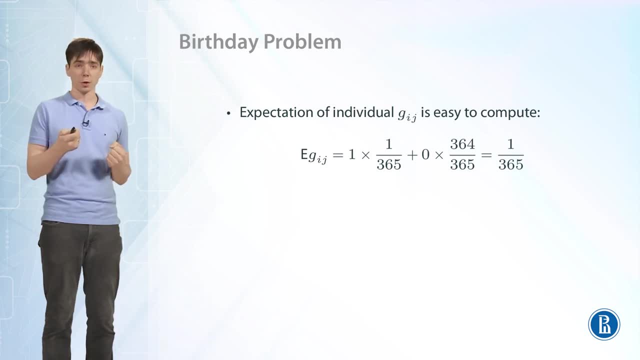 One and zero, And the first outcome happens with probability 1 over 365.. And the second one happens with probability 1 minus 365.. But it doesn't matter, Since the value of this outcome is the second outcome. The second outcome is zero. 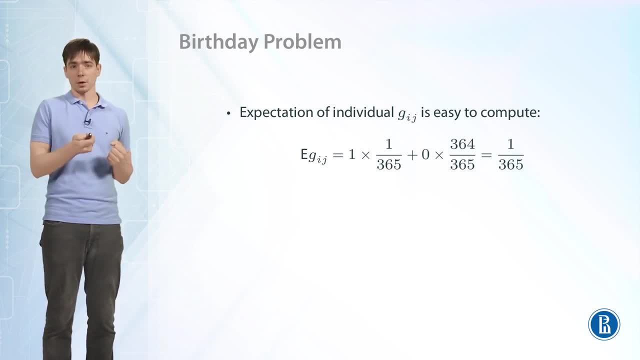 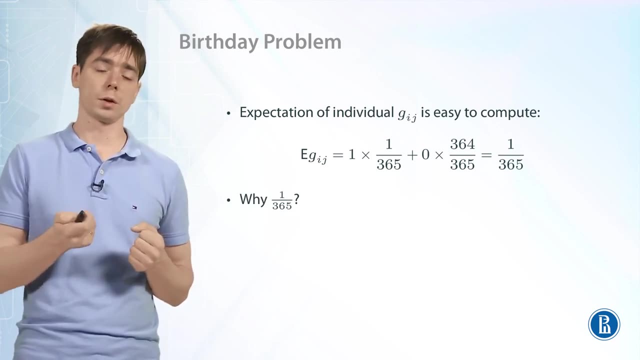 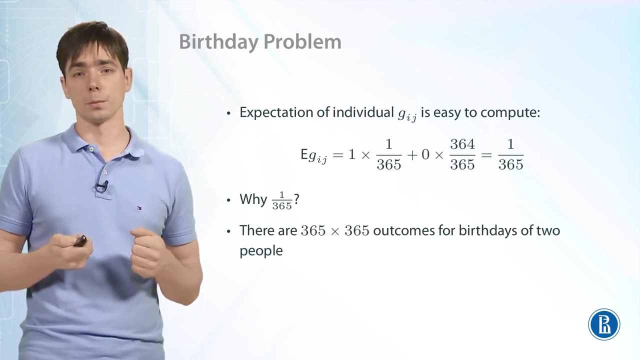 So it doesn't matter by which number we multiply zero, And the expectation will be 1 over 365.. So now why the probability of value 1 is equal to 1 over 365? We can just compute it directly: How many possible outcomes are there for the birthday of two different people? 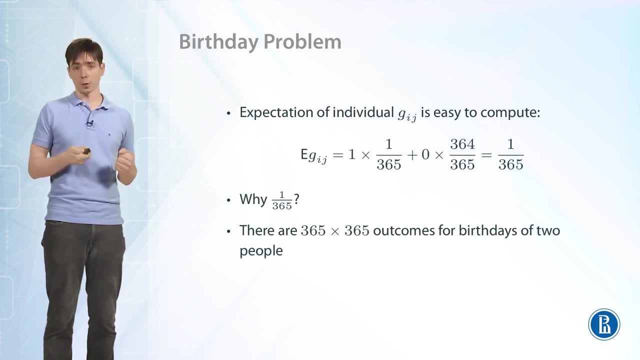 Each of them can have a birthday. Okay, One of 365 possible days. If you have a pair of people, Then there are 365 times 365 possible outcomes, And note that only 365 outcomes are good. There are only 365 possibilities for them to have a birthday on the same day. 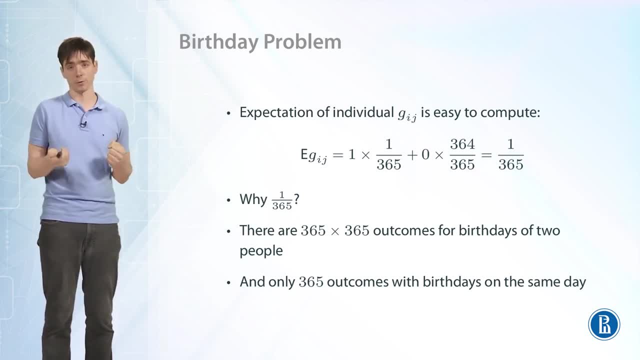 We have to pick one day And then we have to have a birthday. Both of them should have a birthday on this day. So we divide 365 by 365 squared And we obtain our probability. So we have computed the expectation of Gij. 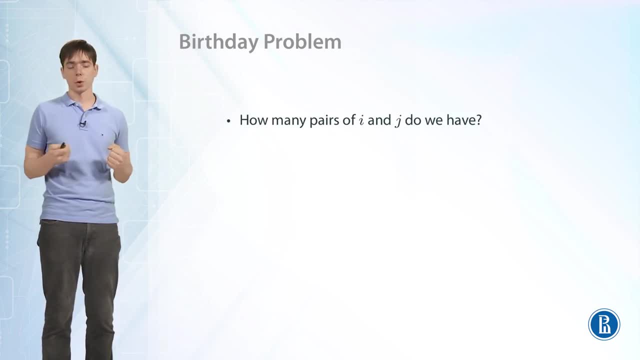 And now we can proceed to the second part. How many pairs of i and j do we have? So there are 28 people in total, And we are interested in unordered pairs of people. These are combinations, And there are 28 people. 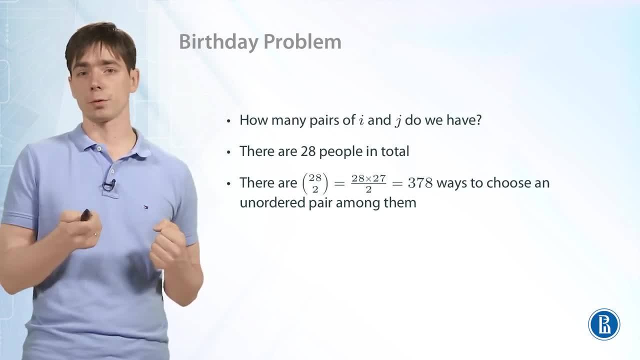 28 choose-to pairs. This is 28 times 27 divided by 2, which is equal to 378.. So there are 378 possible pairs of 28 out of 28 people. Let's briefly recollect why it's 28 choose-to. 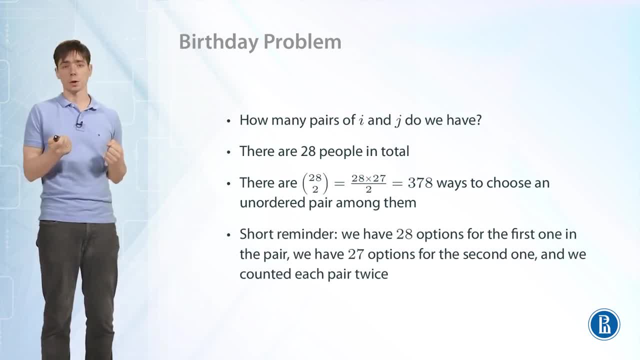 Here is a short reminder. For the first person, we have 28 options And there are 28 possible people. Now we would like to have a pair of different people, So for the second person, there are only 27 options left. 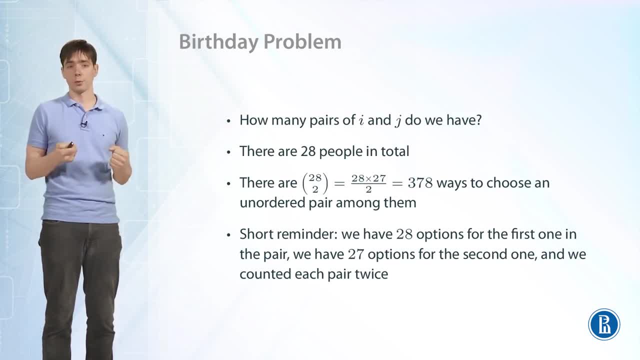 And finally, we have counted each pair twice. If we have a pair of the first person and the second one, we have counted twice. First is when we pick the first person first and the second person second, And the second time we picked the second person first and the first person second. 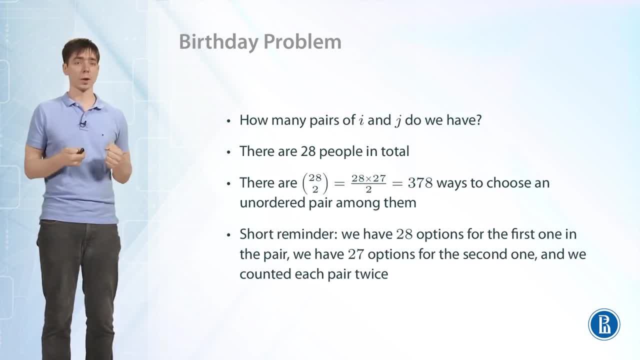 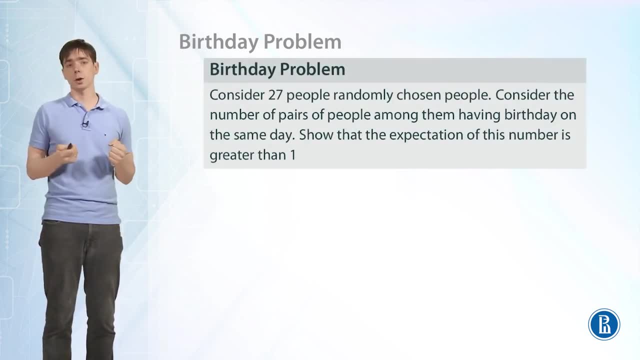 So we counted each pair twice, So we have to divide by 2. And here is why the number of pairs is equal to 28, choose-to, OK. Now let's get back to our proof and finally we have everything we need. We know that the expectation of f is the sum of expectations of gi for 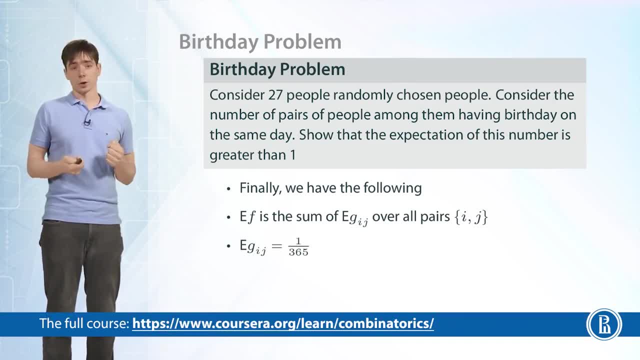 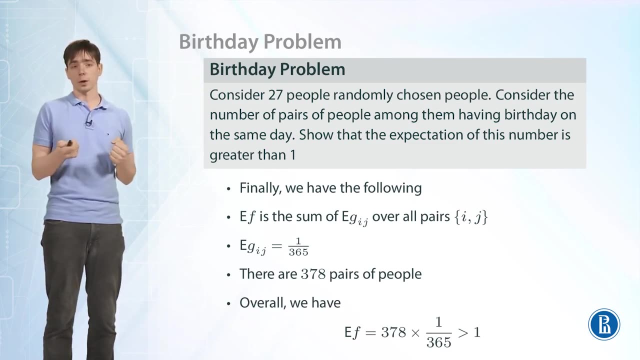 all pairs of i and j. We note the expectation of each gi. It is equal to 1 over 365. And know that there are 378 pairs of people. So overall we have to add up 1 over 365, as many times as there are pairs of people. So overall we have 378 divided by 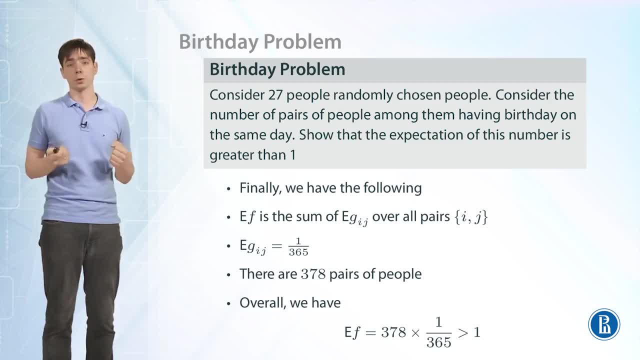 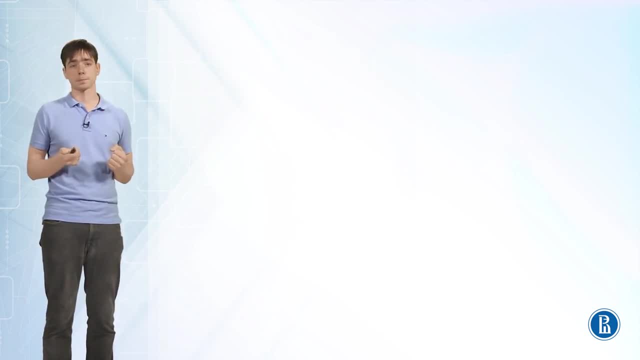 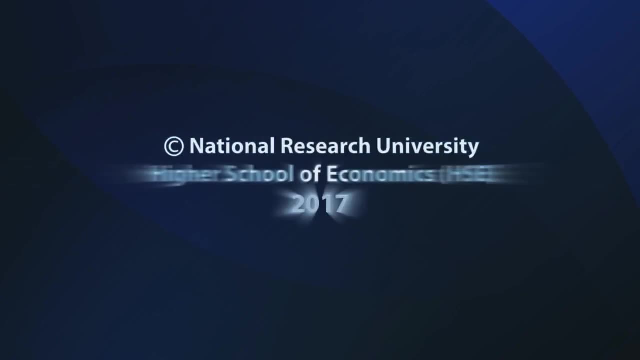 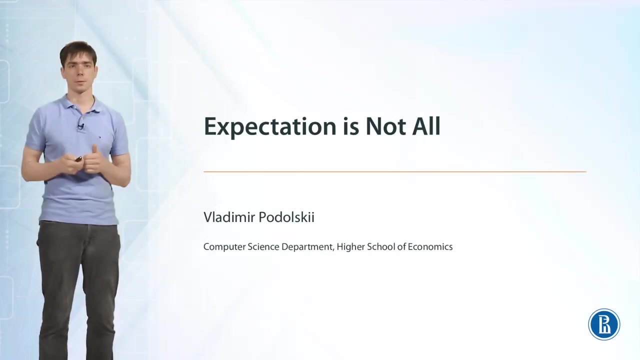 365,, which is greater than 1.. That's what we needed to show, So we computed the expectation of our number and it turned out to be greater than 1.. Hi, I'm Vladimir Podolsky, and today we are going to discuss that expectations. 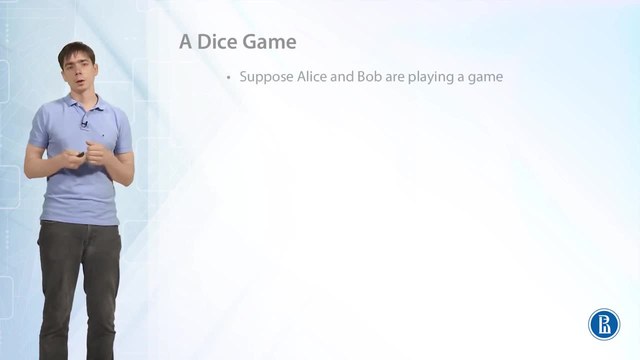 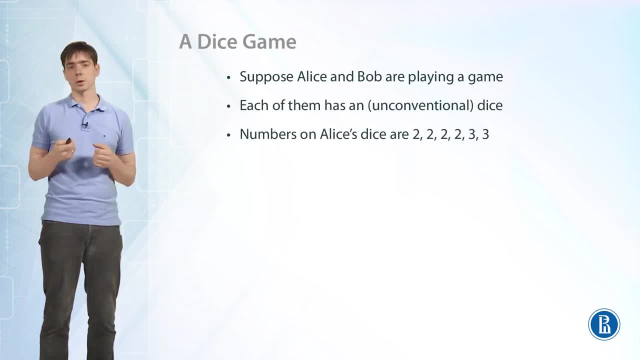 For Alice's dice contains the following numbers on its faces: It contains number 2 four times and number 3 two times. The dice of Bob contains the following numbers: It contains number 1 four times and number 6 two times. Okay, now they do the following: 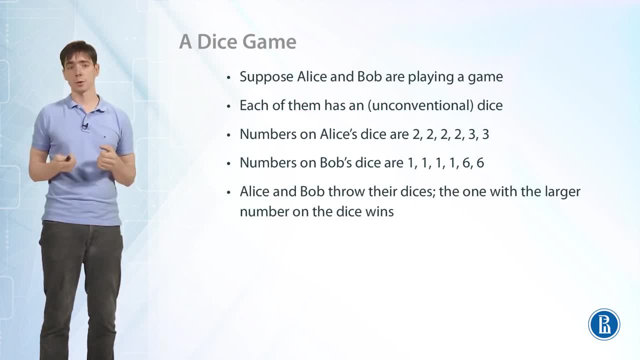 Both of them throw their dices and the one with the large number wins. Okay, and let's see what happens if the players play these games many times. Who will win more often? Okay, so here is a picture. There is Alice and Bob and these: 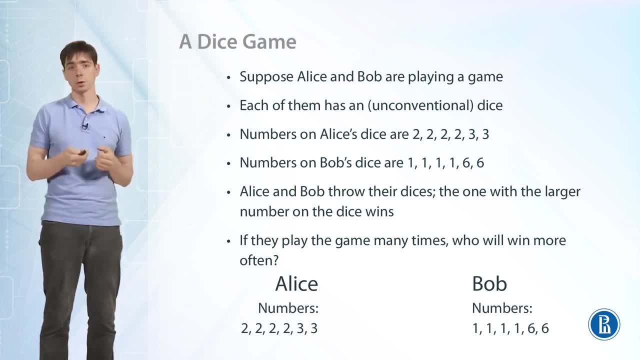 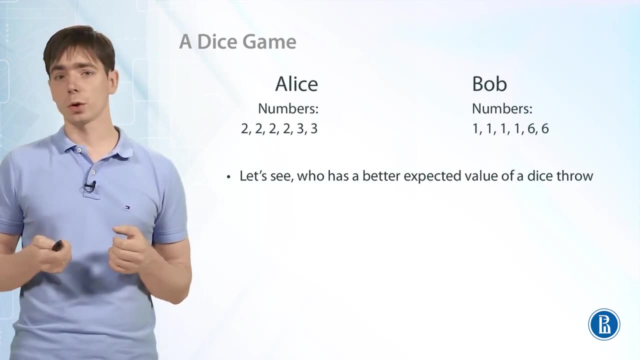 are their numbers. All numbers are equi-probable. and suppose they play this game. Alice throws two, Bob throws six- He's somewhat lucky- and Bob wins in this game. Okay, so this is the game, and let's see. Let's see first of all who has a better. 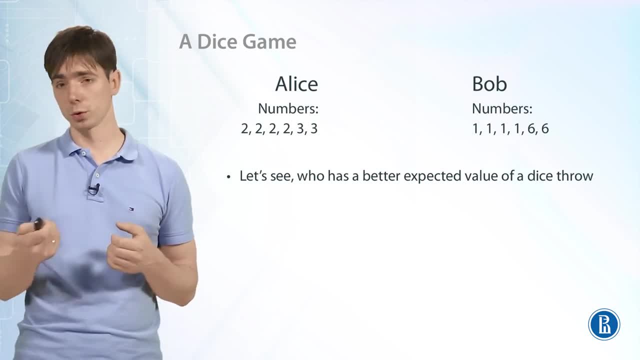 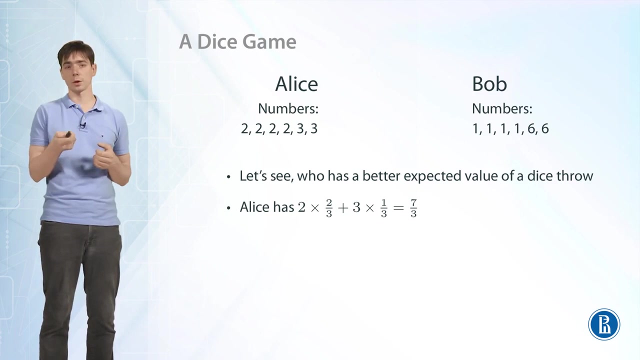 expected value of a dice struggle. It is good to have better expected value because on average you throw larger numbers. Let's see the dice of Alice. It has two, the outcome 2, with probability two thirds, and it has 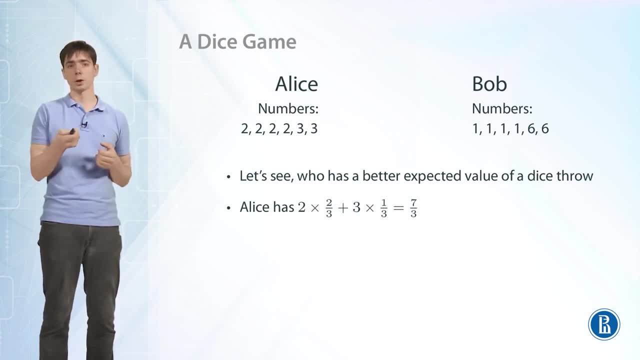 outcome: 3 with probability one third. So the expectation is here and the expectation is 7 or a higher probability, or 2x6.. 7 over 3, which is slightly more than 2.. Now let's proceed to Bob. 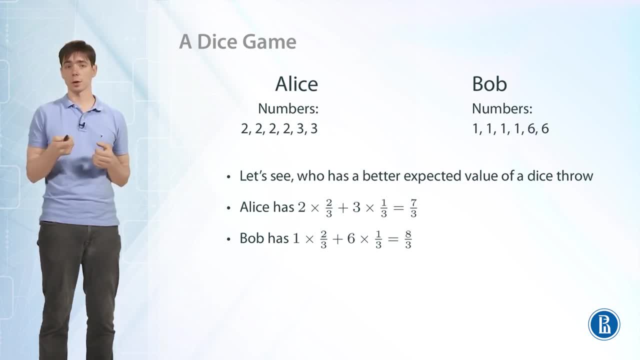 His dice has 1 with probability 2 thirds, and he throws 6 with probability 1 third. So here is the expectation, and the expectation is 8 over 3.. So Bob has a better expectation. Bob has a better expected value on his dice. 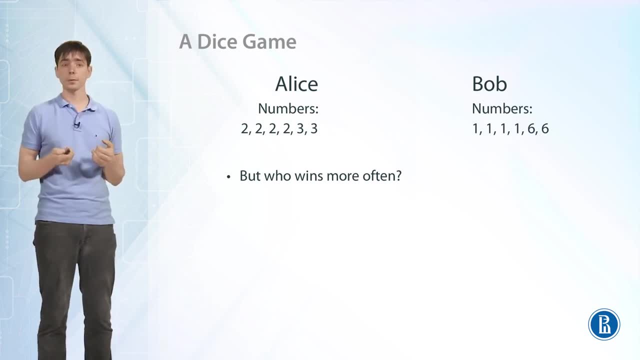 But who wins more often. So let's see who wins in this game And note that actually the game is rather simple. The winner depends only on the throw by Bob. It doesn't matter what Alice throws. Note that if Bob throws 1, then he definitely loses. 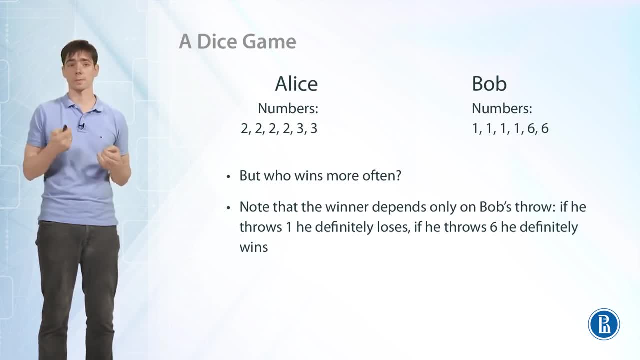 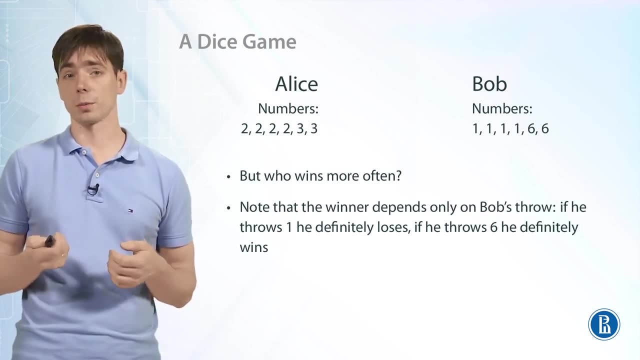 1 is smaller than all numbers that Alice has, And if Bob throws 6, then he definitely wins Because 6 is greater than all the numbers. Bob throws 1 with probability 2 thirds, So he will lose the probability 2 thirds. 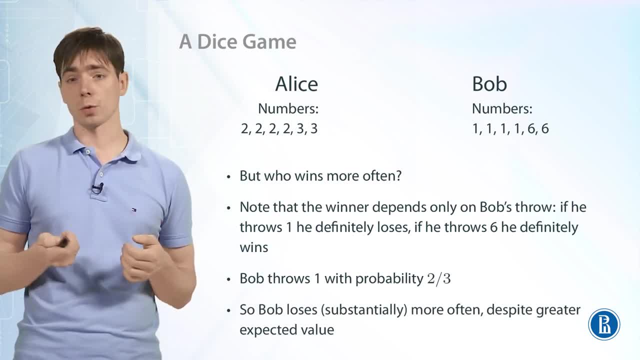 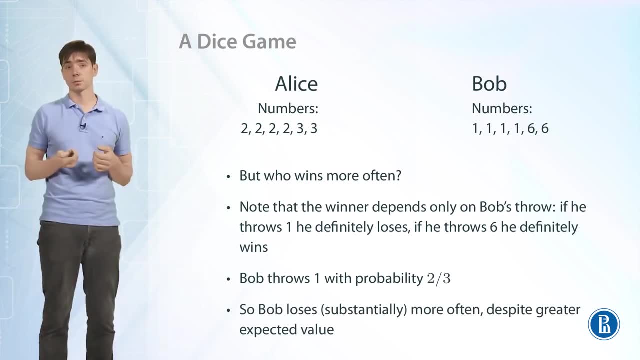 So Bob loses more often, substantially more often. 2 thirds is much greater than 1 third, And this is despite greater expected value. So the dice of Bob has better expected value, but Bob loses more often. Let's see why this happens. 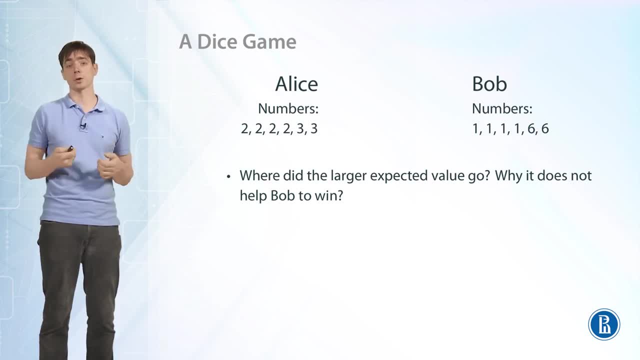 So what happened Where the large expectation of Bob's dice went? So what happened? Note that when Bob wins, he wins by far. 6 is much greater than 2 and 3 that Alice can throw. On the other hand, if Bob loses, he loses slightly. 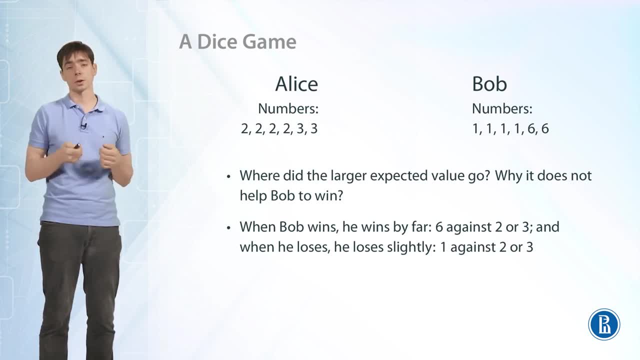 1 is just slightly less than 2 or 3 that Alice has. So here is where the expectation goes. So if Bob loses, which is not very probable, but if Bob wins- this is not very probable, but he will gain more in the expectation than Alice. 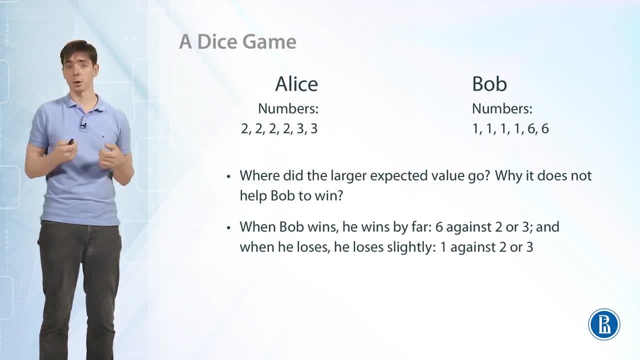 Much more. And if Bob loses, this is probable- but he will get slightly less than Alice. But note that Bob doesn't get any credit for difference between numbers in this game. He either loses or wins. The difference between numbers doesn't matter. 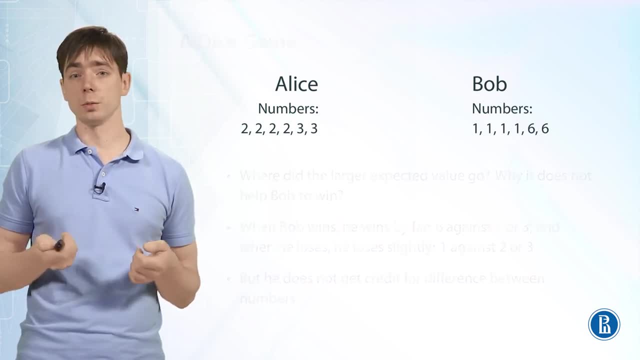 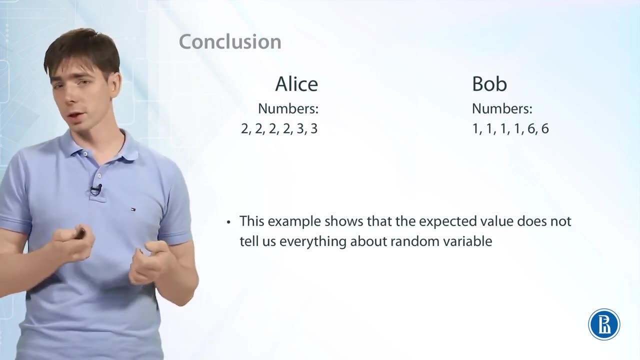 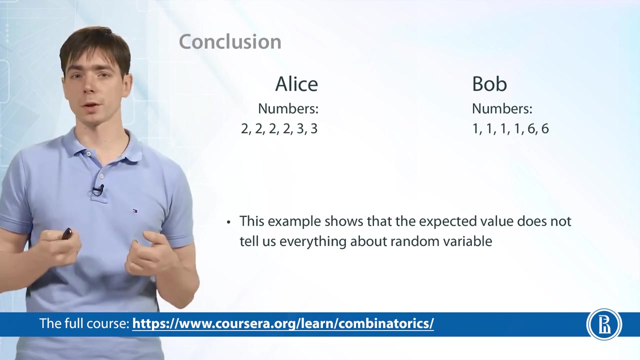 So that's why the expectation is not extremely relevant to this game. Okay, This example shows that the expected value doesn't tell us everything about a random variable. It might be that the expectation of a random variable is better than for the other random variable. 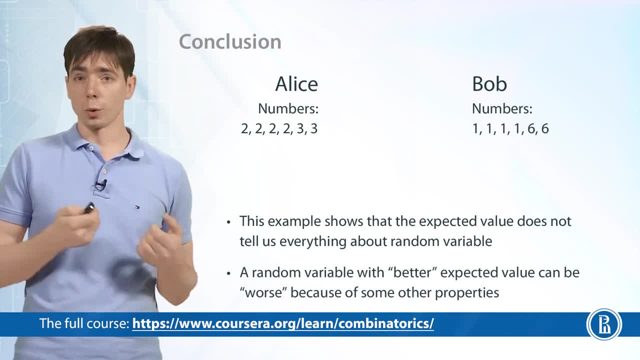 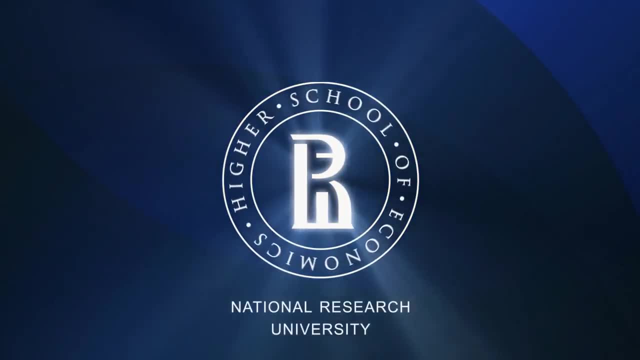 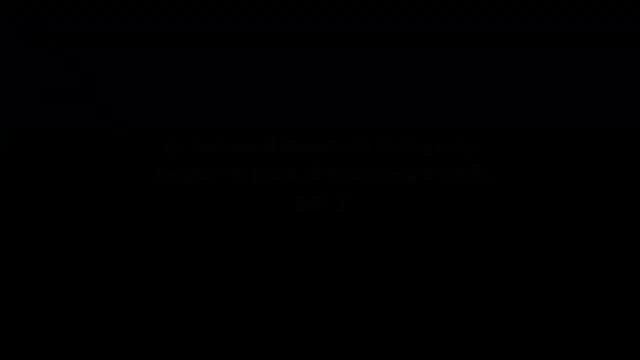 But on the other hand, the random variable is worse because of some other properties And one of these properties is that it is less than or equal to 100. So the bet in the bet and the luck in the bet is more than or equal to 100 or the expected. 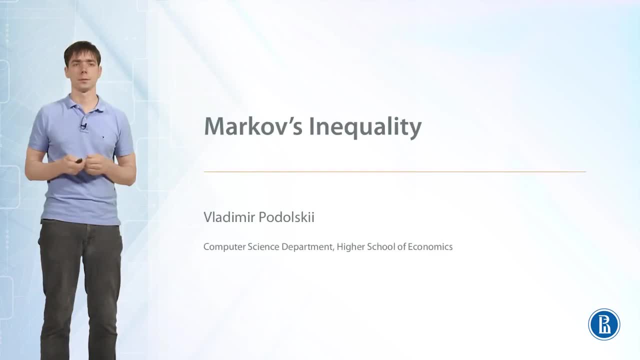 value And we will see that in the next lesson. Thank you for your attention And see you in the next lesson. Bye, See you, Bye, Bye. Hi Hi, I'm Vladimir Podolski and today we will discuss Markov inequality. 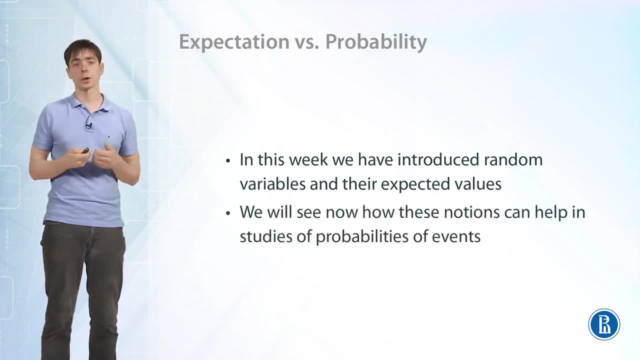 In this week we have introduced random variables and their expected values, And now we will see how these notions can help us in studying the Maxwell equation of random variables. The deduction numbers are shown in the graph. Here we have a two-dimensional line probabilities of events that we have discussed in the previous week. 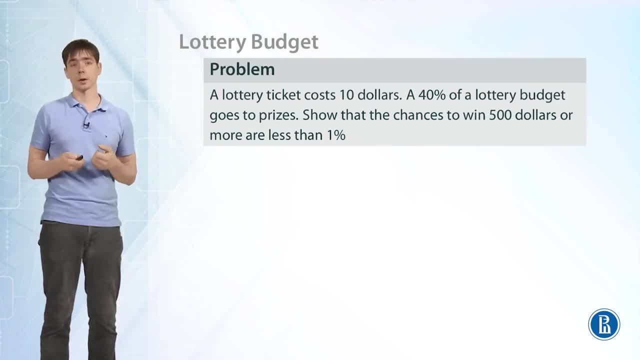 Consider the following problem. Suppose there is a lottery and a ticket costs $10 and it is known that 30% of the budget of the lottery goes to prices. We need to show that the chances to win $500 or more in this lottery is. 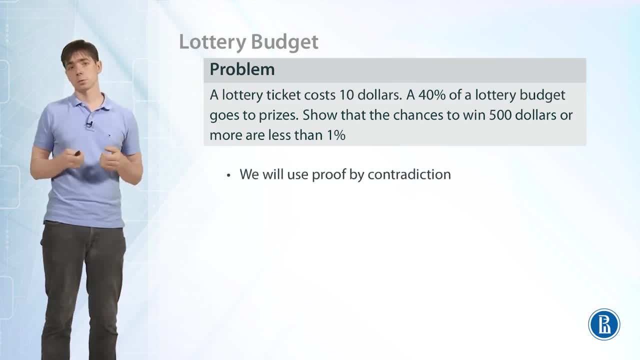 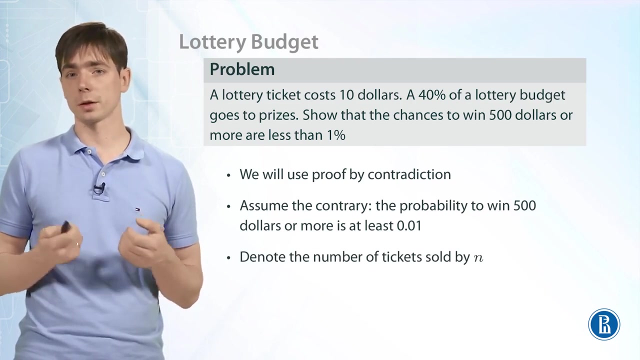 less than 1%. Ok, first of all, we will use proof by contradiction. We will assume that this is not true, that chances are to win $500 or more are at least 0.001.. Ok, denote the number of tickets sold by N, and then we 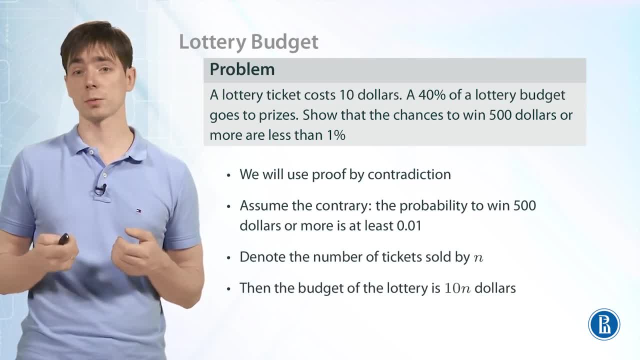 can say what is the budget of the lottery? The budget is ten times N dollars. Now we know how much money the lottery spends on prices. It is 40%. so this is 10 times n times 0.4, which is 4 times n dollars. 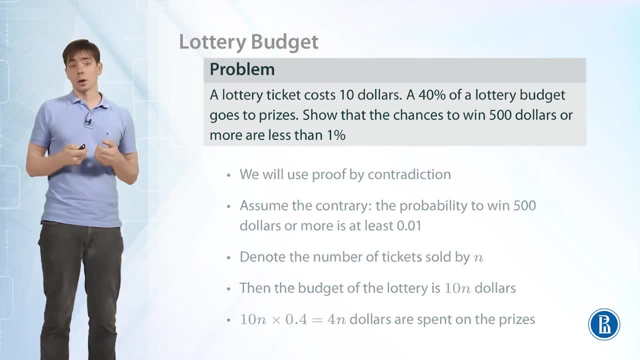 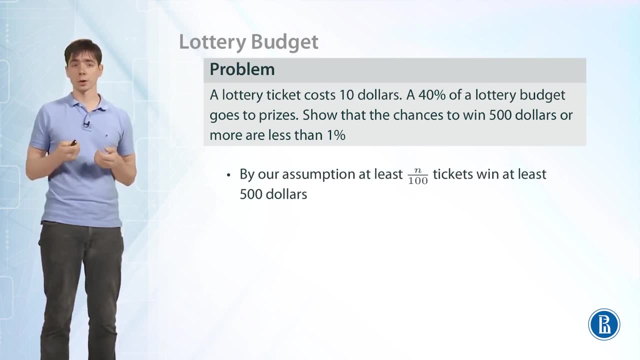 This is the money that is spent on prices. Now, by our assumption- recall that we argue by contradiction- by our assumption- at least n over 100 tickets, at least 1% of tickets, win at least 500 dollars. So in total, these tickets win at least n over 100 times 500, that is, 5 times n dollars. 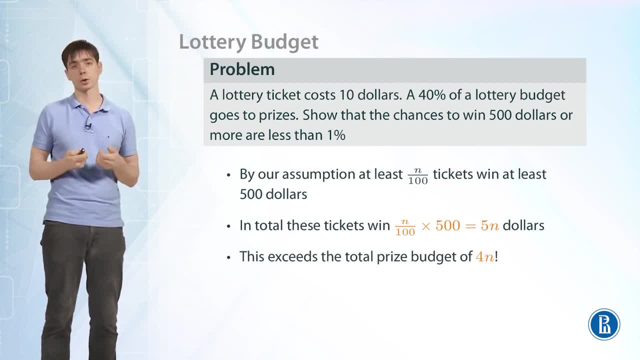 And this is a contradiction. This is more than the total budget on prices in this lottery, The total budget was 4 times n dollars And we have obtained that, And only by these tickets with large prices we have 5 times n dollars. we can win 5 times. 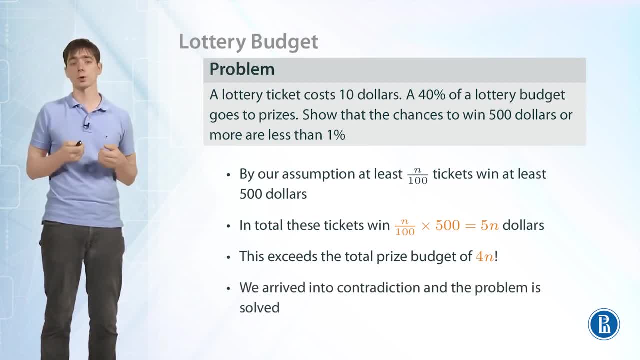 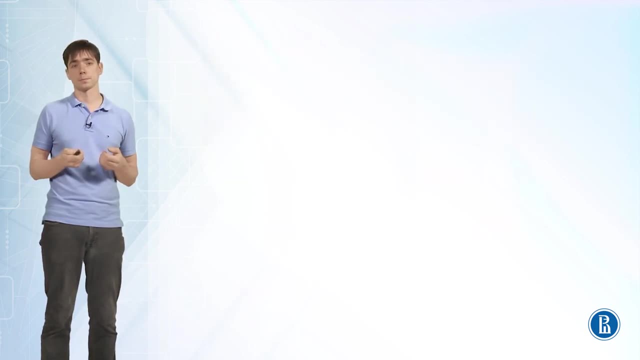 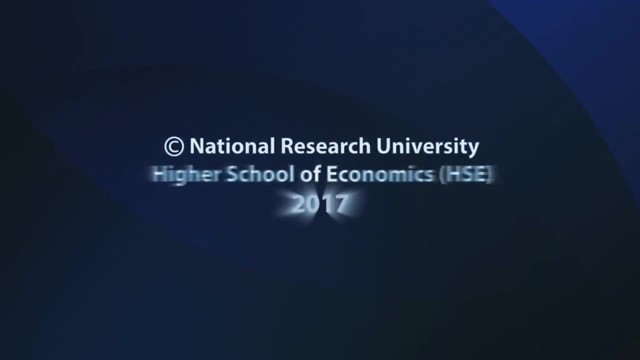 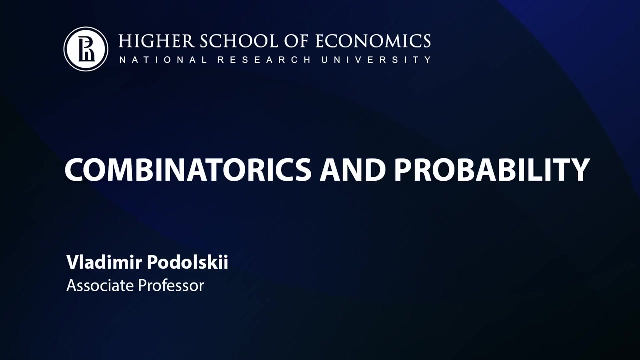 n dollars in total. So this is a contradiction. so our assumption is wrong and we have shown that the statement of the problem is true. The chances to win 500 dollars or more is less than 1%. Now we proceed to Markov's inequality. 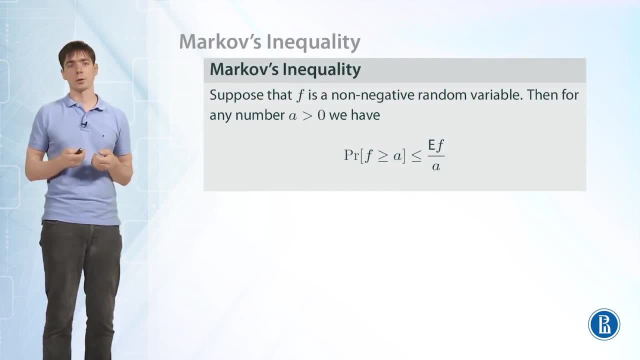 Suppose there is a non-negative random variable, f, that is, f obtain only non-negative values. Then for any positive number, a, we have the following: The probability that f is greater or equal than a is at most 1.7 times n. 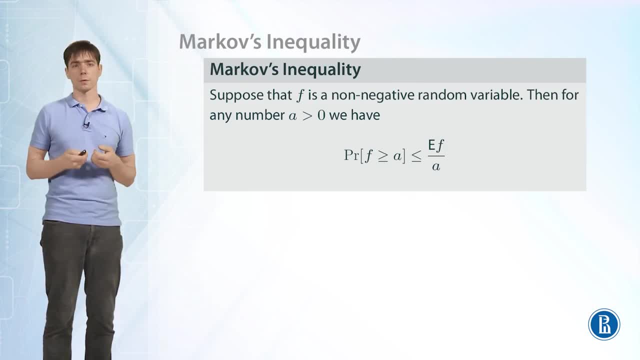 ippost times, 1.4 times n, And for any positive number, a, we have the following: The probability that f is greater or equal than a is, at most, 1.7 times n, most the expectation of F divided by A. This is a useful inequality and we can use it in. 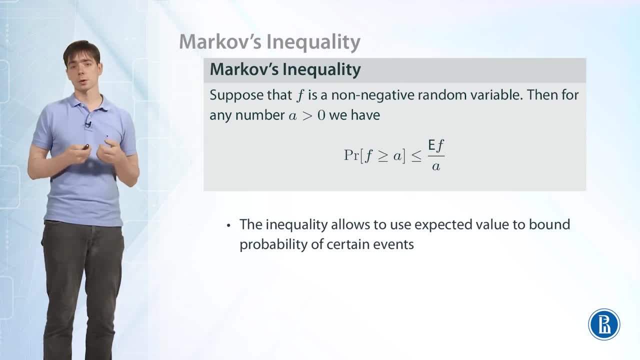 the following way. It allows us to bound probabilities to show that probabilities are not too large using the expectations. We have discussed how we can compute expectations, so now we can use this to bound some probabilities For the proof of this inequality. it is convenient. 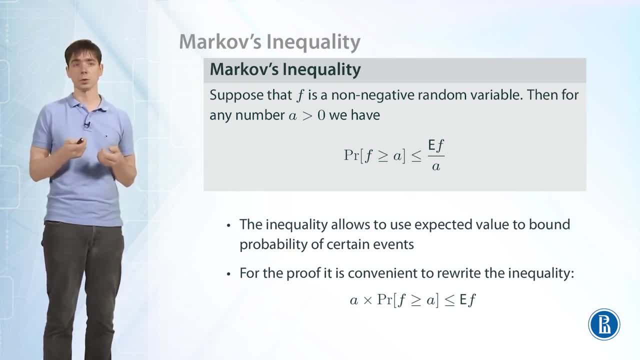 to rewrite it. It is convenient to multiply both sides by A Note that A is positive, so we can do it, And we will show that A times the probability that F is greater or equal than A is at most the expectation of F. So we need to show this inequality And for this 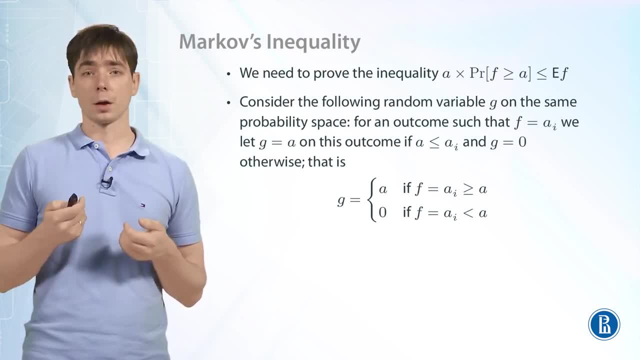 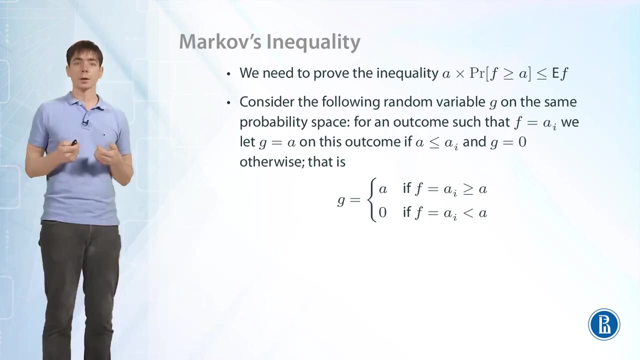 let us consider the following new random variable, g. So it is a random variable on the same probability space and it is defined in the following way. So consider some outcomes and the value of F on this outcome is AI, then if AI is at least A, then g is equal. 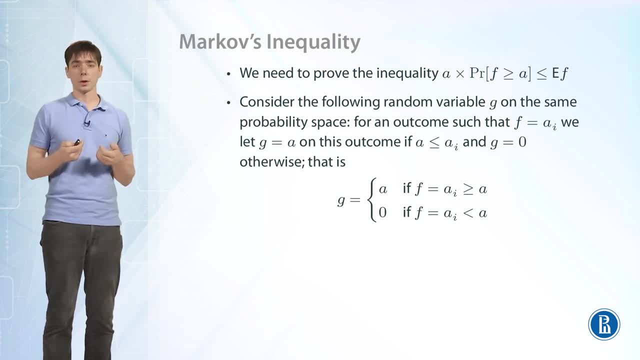 to A on this outcome. And if AI is less than A, then g is equal to 0 on this outcome. So g indicates a certain event. g indicates the following: if on some outcome the value of F is at least A, then g is. 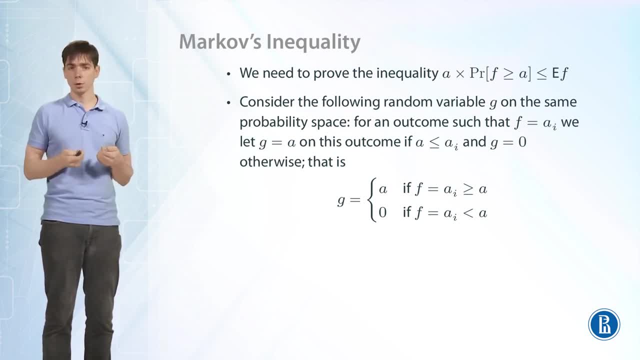 a, a, Otherwise it is zero. Okay, Note that g is always less or equal than f on each outcome, Since it is always on all outcomes, at most f. then the average value of g is also at most average value of f. So we have this inequality: The expectation of g is at most expectation of f. 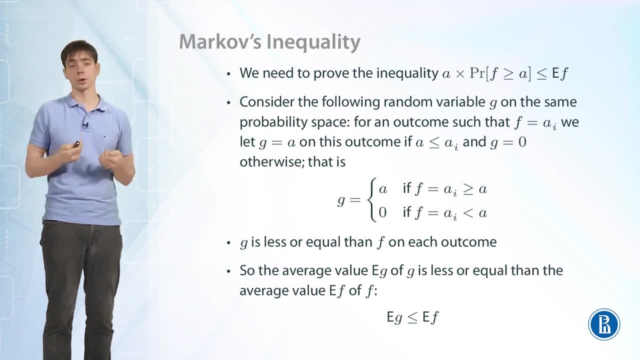 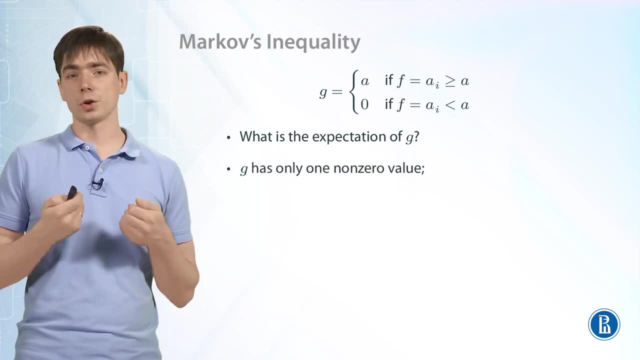 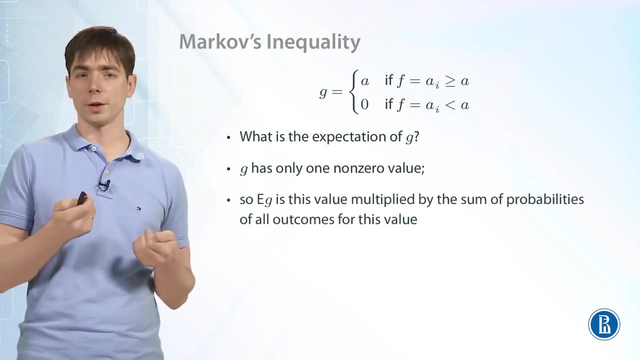 Again, this follows, since g is at most f on each possible outcome. Okay, Now, what is the expectation of g? Note that g has only one non-zero value. If we write the definition of expectation, then we see that the expectation of g is this value multiplied by the sum of probabilities of. 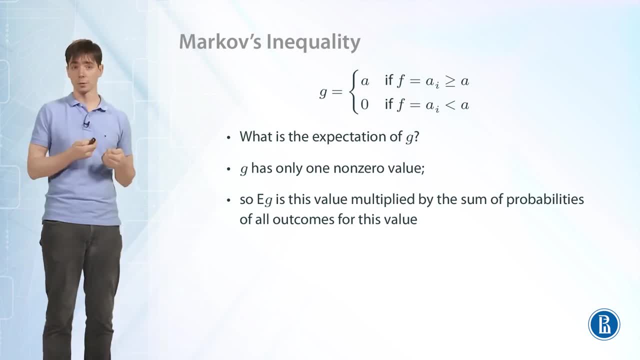 outcomes for this value of g. Now we have to see what are these outcomes. Note that these outcomes are exactly the outcomes of the following event: f is at least a. G is equal to a, if, and only if, f is at least a. So these are the outcomes of the event: f is at least a. 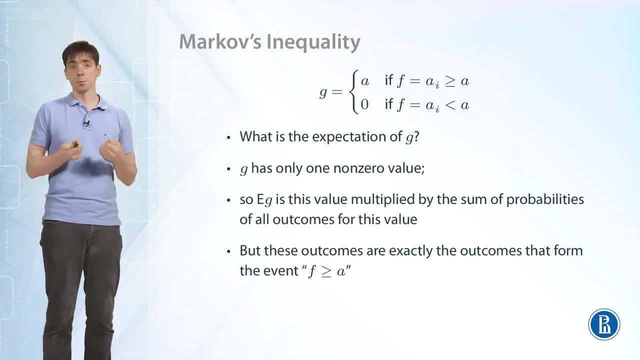 The sum of probabilities is, by the definition, when f is at least a. So the sum of probabilities is f. whatever f is at least a, probabilities of this outcome is just exactly equal to the probability of the event. f is at least a. And so now we know what is the expectation of G. We have to multiply a by the sum of. 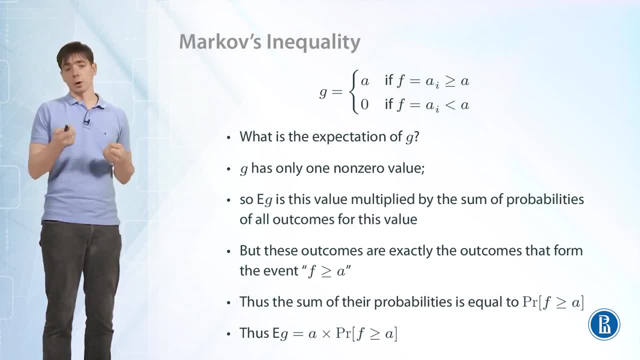 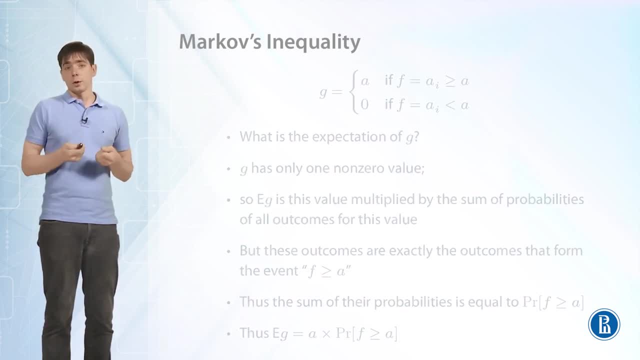 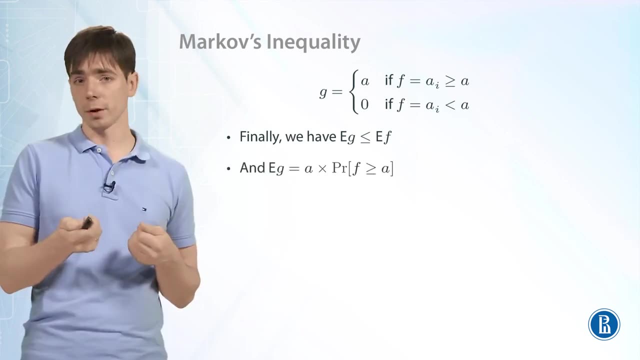 probabilities of these outcomes, and this sum is equal to the probability that f is at least a. So here is the expectation of G. Now let's sum up what we already have. We have that the expectation of G is at most the expectation of f, and, on the other hand, 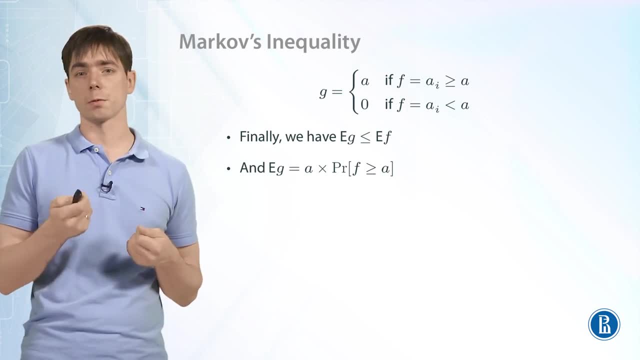 we have already computed the expectation of G. It is equal to a times the probability that f is at least a. So if we combine this, we see that the expectation of f is at least a times the probability that f is at least a. 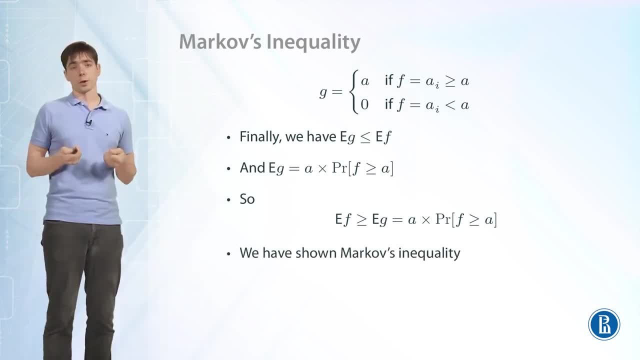 And this is exactly what we needed to show, And we have shown Markov inequality. So the idea was that we substituted f by a smaller and simpler random variable, and this way we have bounded, We have obtained the bound between expectation and the probability of the event we are interested. 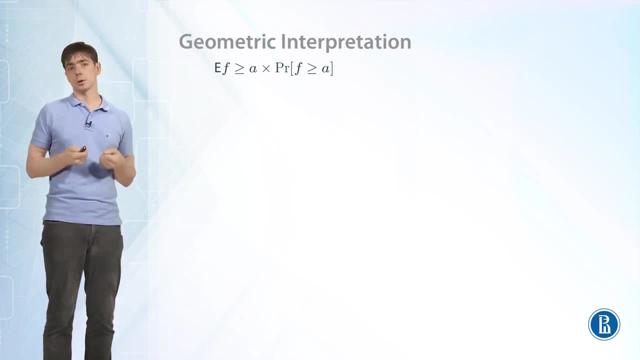 in. Okay, Now let's see. just to get more intuition, let's see geometric interpretation of this inequality. Now we have this inequality we would like to show And suppose, for simplicity of the presentation, suppose that f obtains four values: a1, a2,. 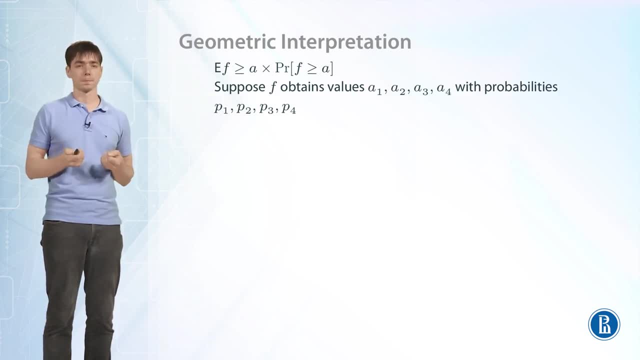 a3 and a4, with probabilities p1, p2, p3 and p4.. Now again recall that we can represent f in the system of coordinates. We can split the interval from 0 to 1 into four intervals of length: p1, p2, p3 and p4. 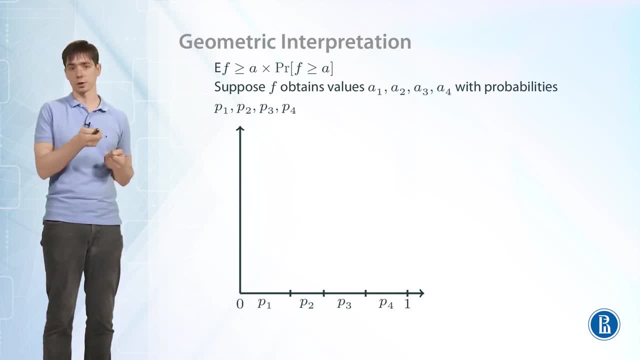 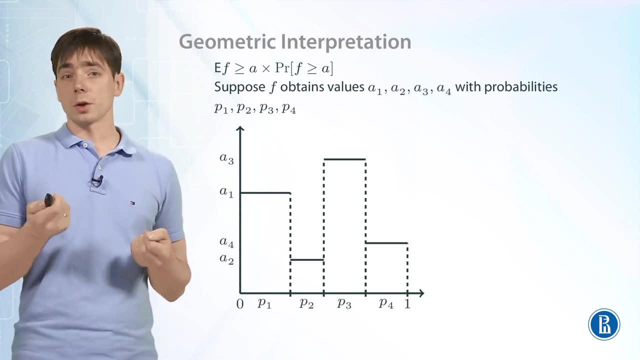 Recall that p1 plus p2 plus p3 plus p4 is exactly 1.. So we can split the interval of length 1 into these parts. We can consider the following graph, which correspond to the function f, If we throw a point, informally speaking, if we throw a point from interval from 0 to. 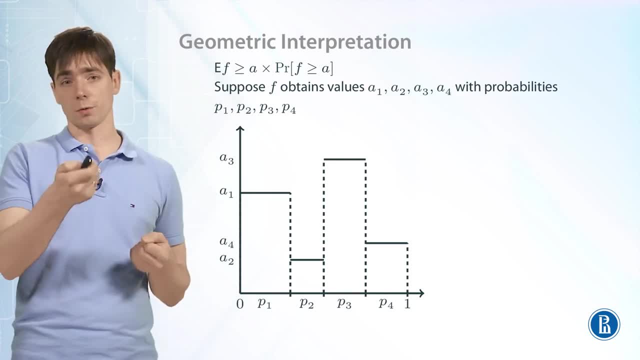 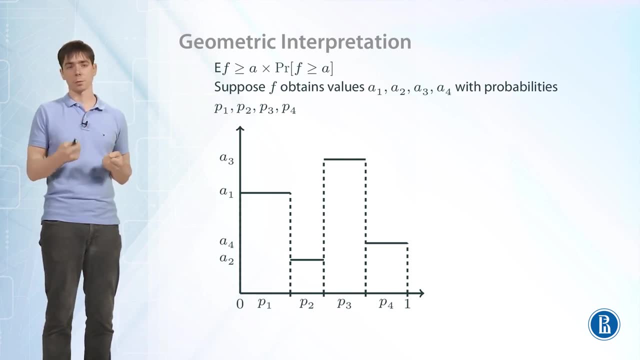 1, then with probability, and see the value of the function with this graph in this point. then with probability p1 it will be equal to a1, with probability p2 it will be equal to a2, and so on. This is exactly our random variable f. 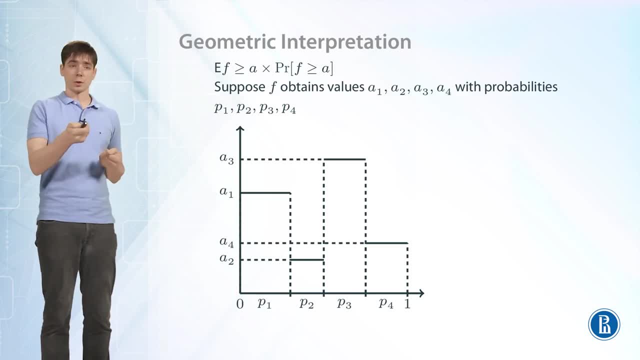 So here is the graph, Here is how it corresponds to vertical axis And here is a from the inequality on the top of the slide, And recall that the expectation of f is just the area of the gray region. On the other hand, we can also see a times the probability that f is at least a in this. 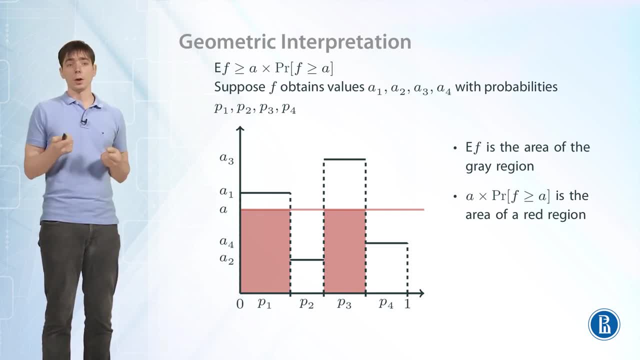 picture It is the area of the red region, Indeed. So f is at least a on two outcomes on this picture: On the outcome a1 and on the outcome a3. So the probabilities are p1 and p3.. So this product, a times probability of that a, is at least a breaks in two parts. 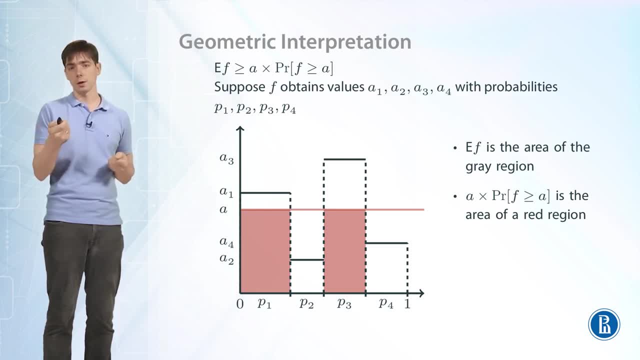 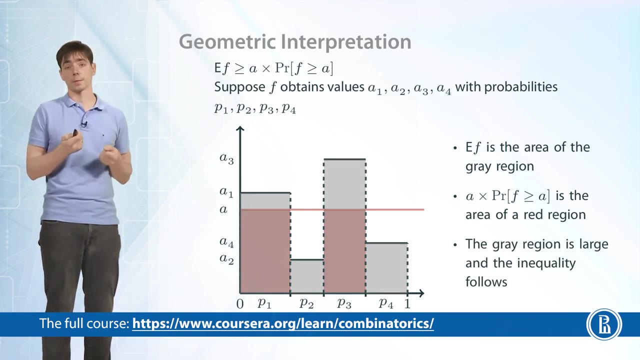 It's a times p1 plus a times p3. And these are exactly errors. So we can see that f is at least a on two outcomes on this picture. So the probabilities are p1 and p3. So it's a. Now it is just observed that the gray region is larger than the red one. 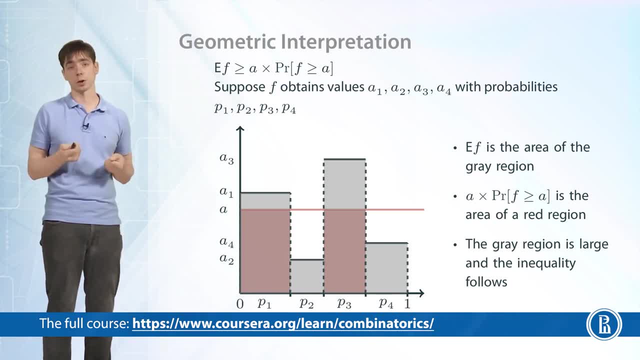 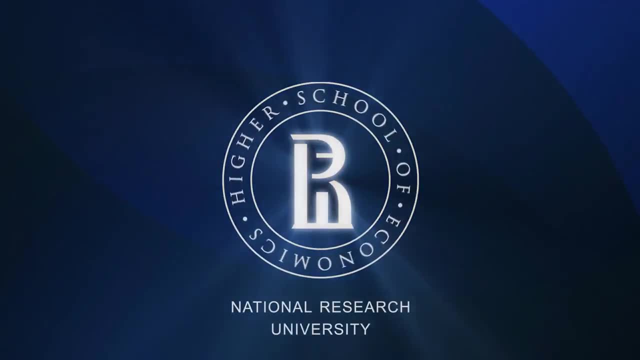 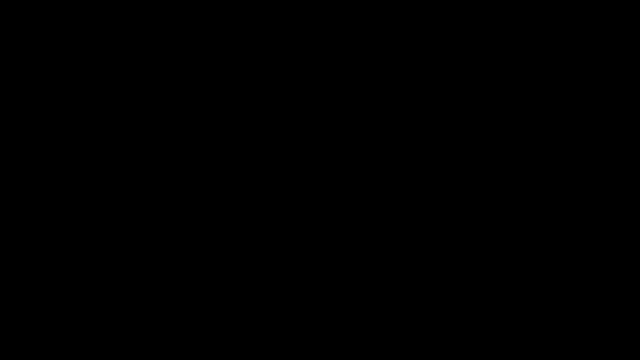 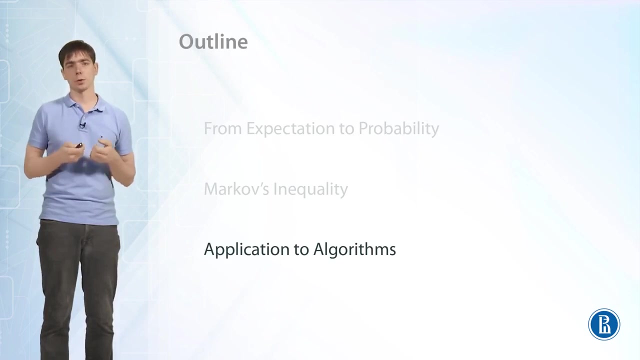 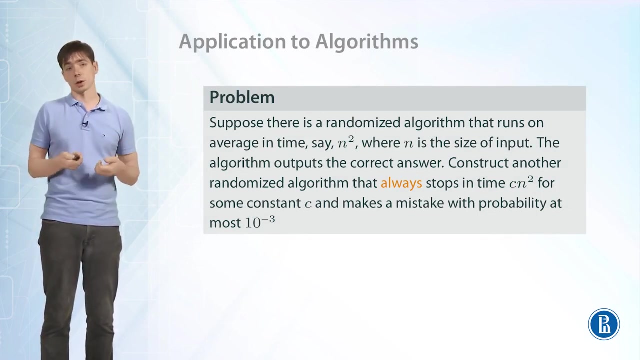 So that's the intuition behind the geometric intuition behind Markov's inequality. Now we will see an application of Markov's inequality. Consider the following situation: Suppose we have a randomized algorithm that uses randomness in some way, Then running time of this algorithm is a random variable. 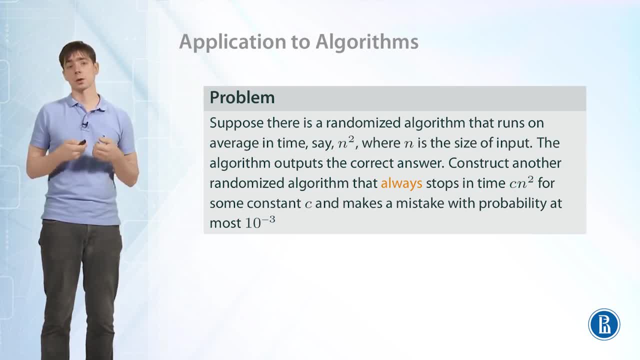 And suppose that on average algorithm runs in time n squared where n is the size of input, Then algorithm outputs the correct answer always. Now we are not happy that our algorithm runs in n squared on average, but in some rare cases it might take a long time and we are not happy about it. 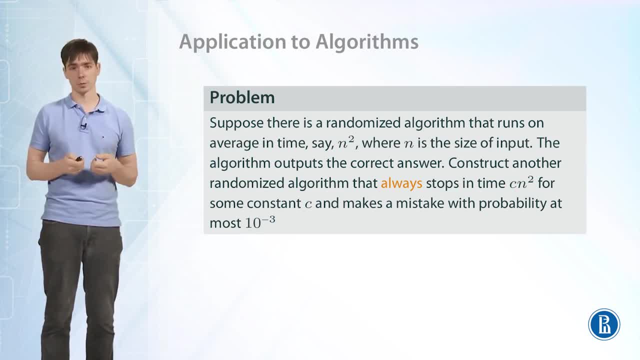 For some reason, it would like to stop after a certain number of steps, And so we would like to construct a new algorithm, again randomized, that always stops in time, some constant times, n squared And we are ready to sacrifice something. We are ready to say that, ok, let our new algorithm to make a mistake with very small probability. 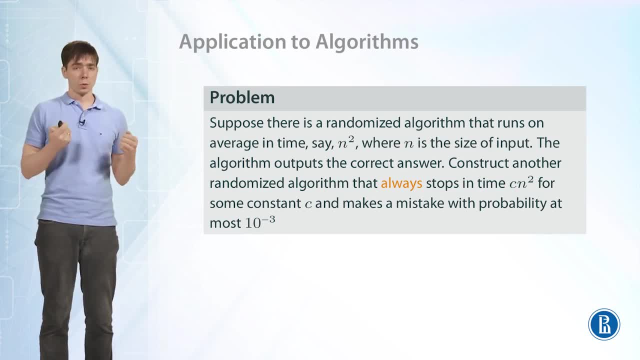 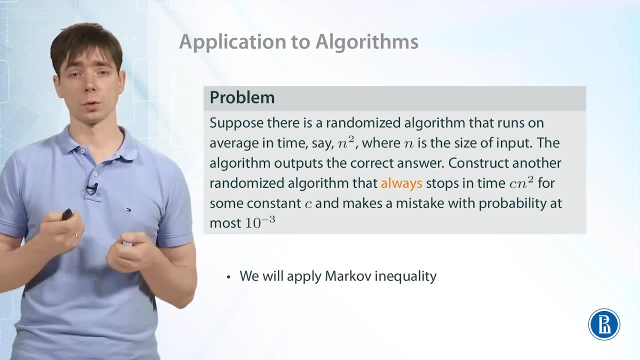 For example, with probability 1 over 1000.. So can we do it or not? Ok, it turns out that we can do it, and we will just apply Markov's inequality to this. Ok, let's proceed to the proof. 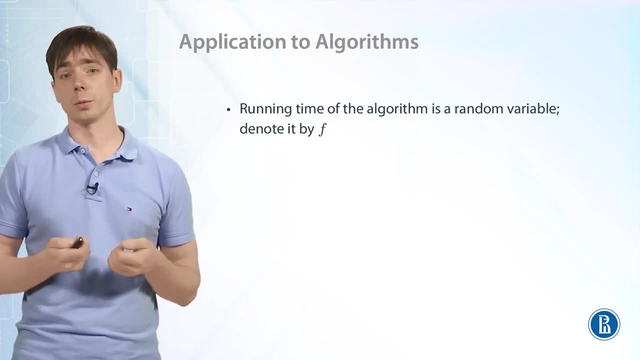 The running time of our algorithm is n? squared And we are ready to sacrifice something. So our algorithm is a random variable that is denoted by f And we know that on average, the algorithm runs in time n squared, which means that the 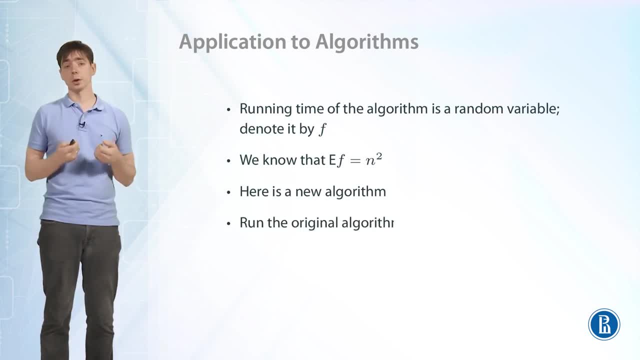 expectation of f is n squared. Now here is a new algorithm. We run the original algorithm for 1000 times n squared steps And then, if it stops, good, we also stop. our new algorithm stops, But if it doesn't, the original algorithm doesn't. 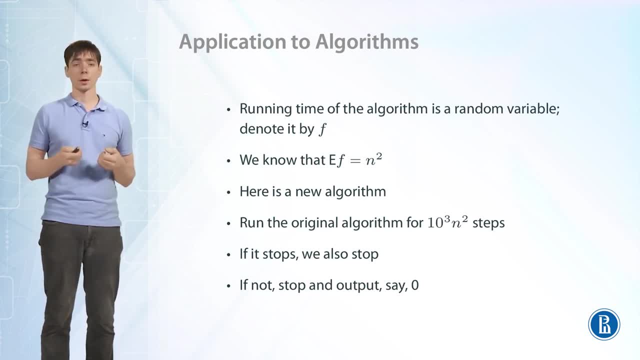 It is not guaranteed to stop after these number of steps, And if it doesn't stop, we stop it and output something. It doesn't matter what. Let's say output 0. It doesn't matter if it makes sense or not, So just output, arbitrary output. 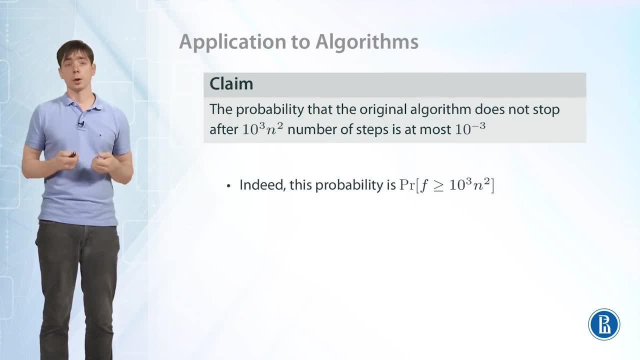 Ok, now we claim the following: The probability that the original algorithm doesn't stop after 1000 times n squared steps is at least 1.5.. Ok, At most 1 over 1000.. And this in particular means that our algorithm makes a mistake with probability at most 1. 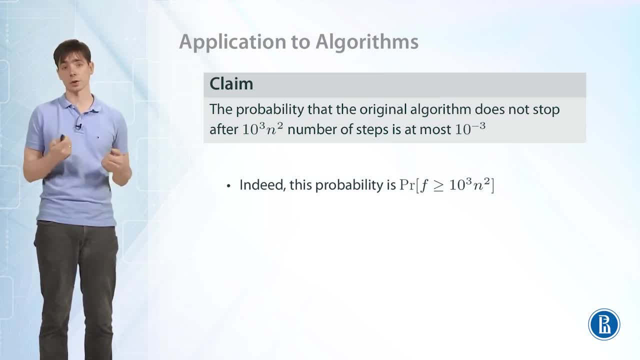 over 1000.. It can make a mistake only if the original algorithm doesn't stop after these number of steps. Ok, Why is the claim true? Indeed, note that the probability, our probability, is the following: The probability that f, our random variable, the running time of the algorithm is at least. 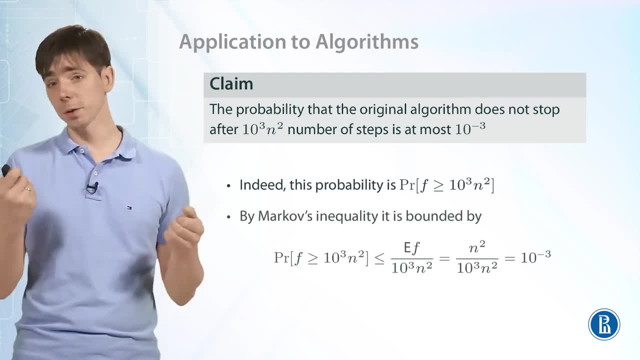 f squared And by Markov's inequality. recall that f is a non-negative random variable. its running time of the algorithm can be negative. so this probability is at most the expectation of f divided by this number in the inequality inside of the probability. so it's divided. 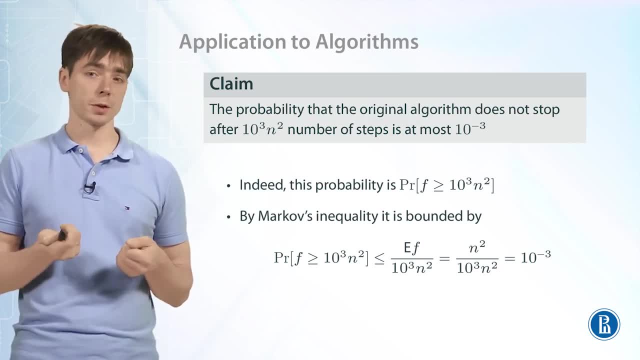 by 1000 times n? squared, We know that the expectation is n? squared, so it's n? squared divided by 1000 times n squared. n squared- cancel out. n squared- cancel out. And so we have that this probability is at most 1 over 1000.. 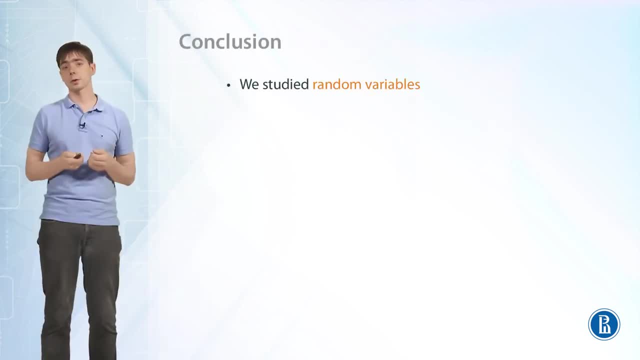 And that's exactly what we needed to show. So in this week we studied random variables. They are very useful, for they allow us to study quantitative aspects of randomness. Also, they allow us to use many analytic tools to study probability, to apply more mathematics. 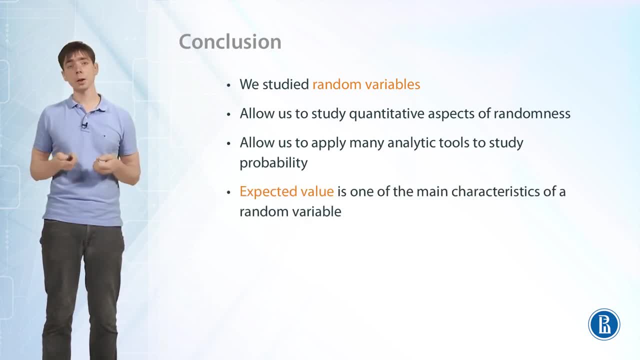 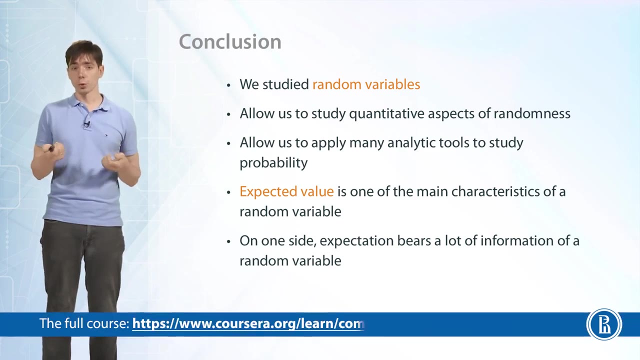 to study probability. Next, we considered one of the most important problems, One of the most important characteristics of random variables. they are expected values And they are also very useful, and there are two reasons for that. On one hand, expectation bears a lot of information of a random variable. 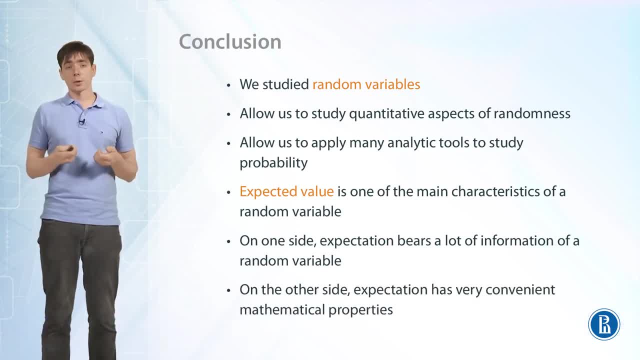 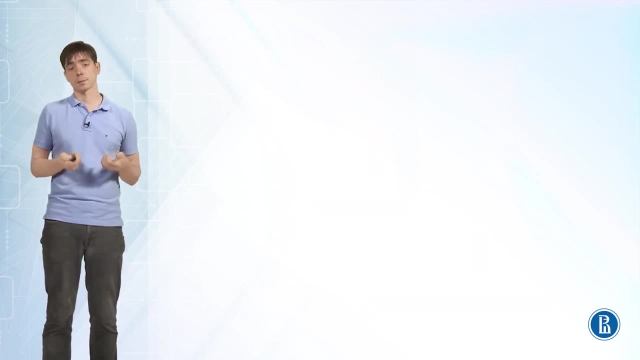 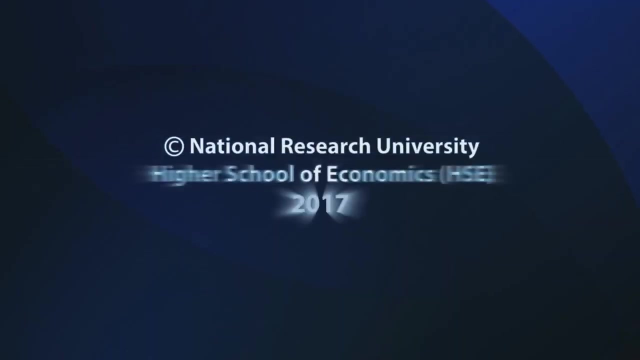 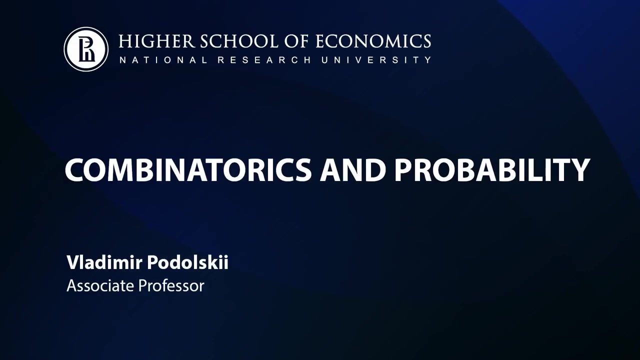 It tells us a lot about random variables. On the other hand, expectation is a very convenient thing to study. It is a number And it has very convenient mathematical properties like linearity, which makes it often very easy to compute. Hi, I'm Vladimir Podolsky, and today we are going to discuss a certain dice game. 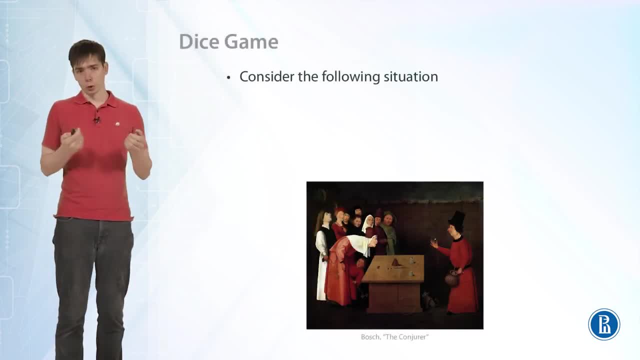 Consider the following situation. Let's start with a very simple one. You are in some shady neighborhood of some city and there is a shady person on the corner of the street who offers bypassers to play a game with him. And here is the game. 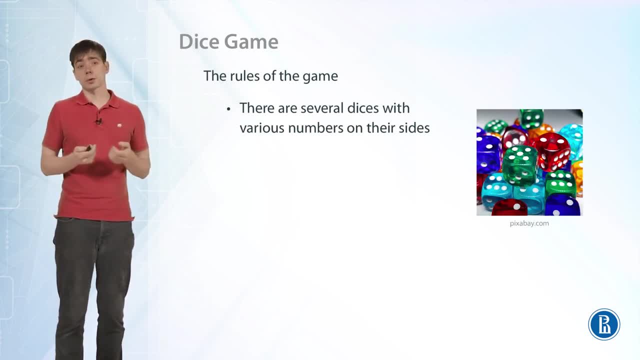 There are several dices with various numbers on their sides. These are not just standard dices with numbers 1,, 2,, 3,, 4,, 5, 6. These are dices with some other numbers possibly, and they are different, so lots of various. 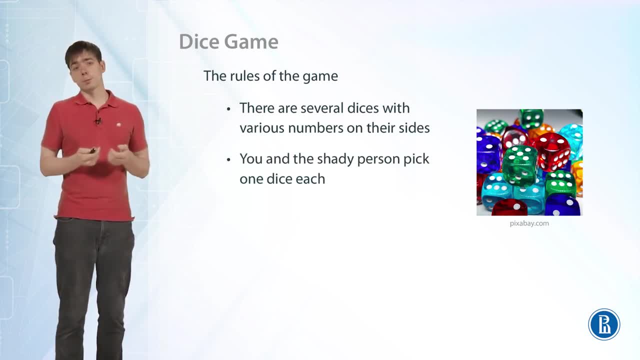 dices. You pick one dice each And then you throw. both of you throw your dices and whoever has the larger number on his dice wins And the winner gets one dollar from the loser. And the shady person is eager to play this game a lot, so you can repeat the game and 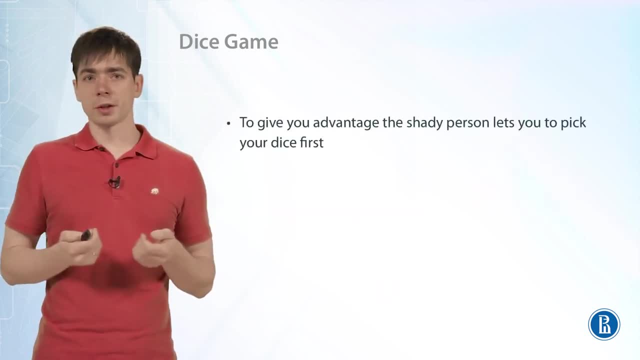 so on, Okay, And the only thing that is unclear is that who picks his dice first? Maybe you just would like to pick the same dice, and then what? Okay, And for this the shady person tells you, okay, to give you an advantage he would like. 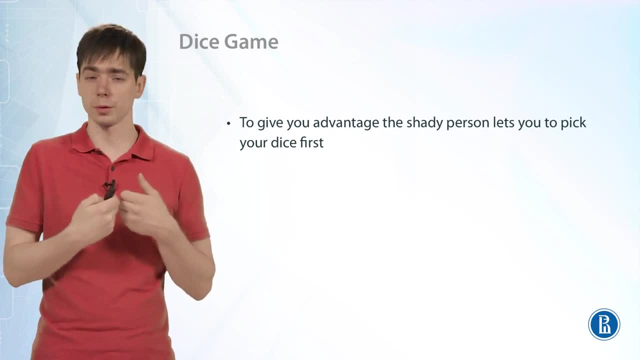 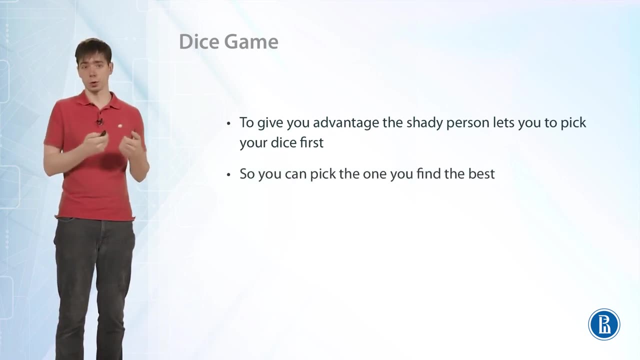 to give you the opportunity to pick your dice first. So he lets you pick your dice first, and so you can pick the best dice there is. So you can pick the one that you find best, And the shady person will have to pick among other options. no other choice for him. 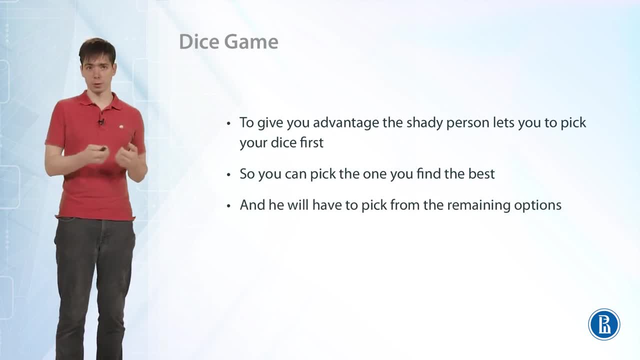 So you are not allowed to pick the same dice. You pick your dice, Then he will have to pick from other options. Okay, And now this looks- we start to look strange. So now the game seems to be favorable to you, So you have an advantage clearly. 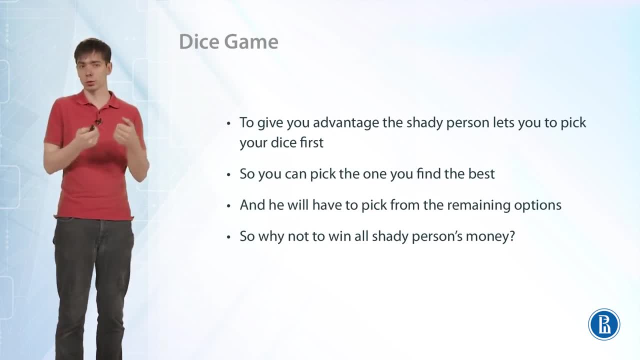 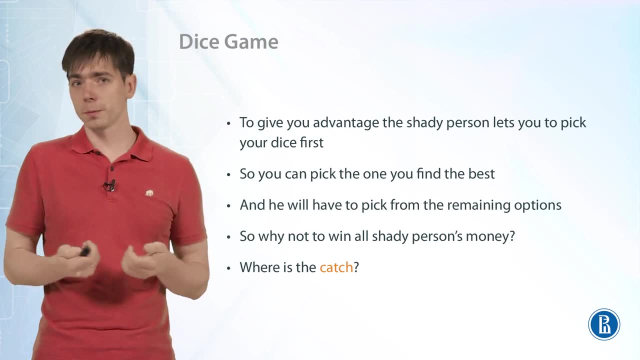 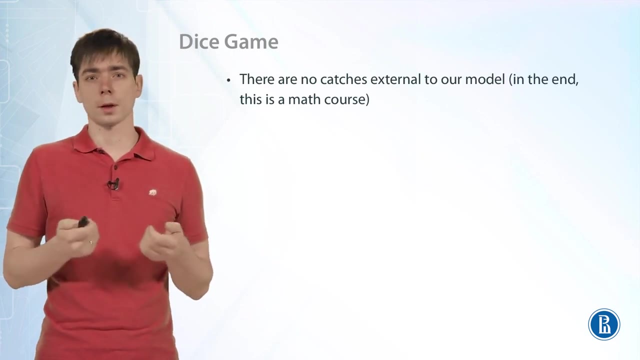 And why not? to spend an evening and to win? not to win all shady person's money. What is the catch here? And note that in our problem, there are no catches that are external to our model. Okay, And don't forget that we have a math course. 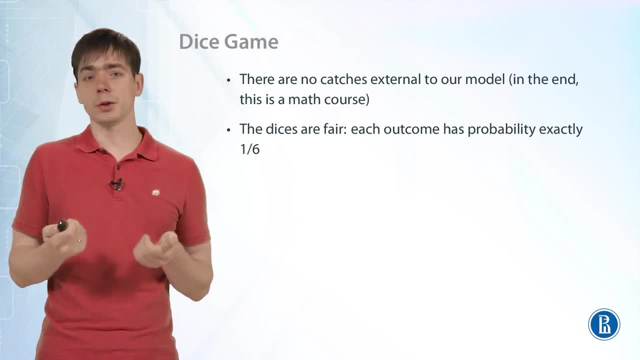 So, in particular, the dice is a fair. each outcome has probability exactly one over six. Also, no one will hit you on the head from behind during the game And no one will pick your pocket, And this is a good time for a disclaimer. 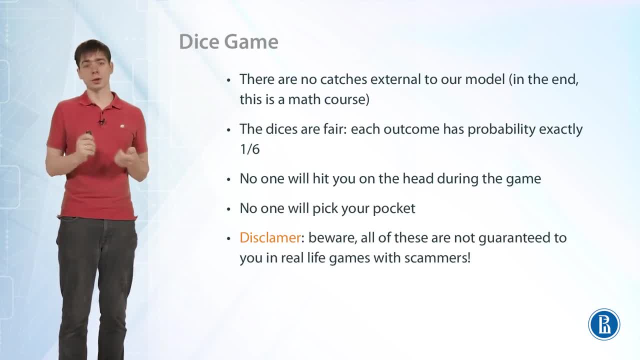 Note that all of these are not guaranteed to you in real life- games with cameras, So you probably should avoid these games in real life. But in our problem, the shady person is not cheating. The game will be played exactly as we described it. 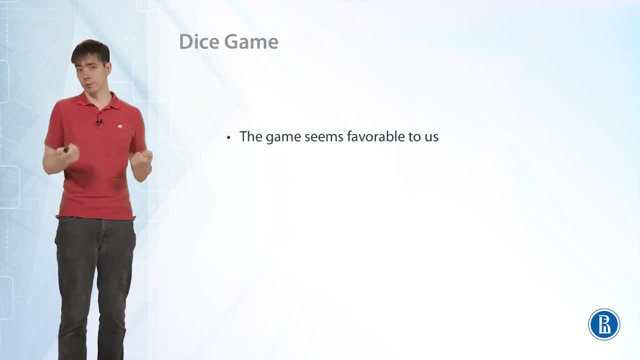 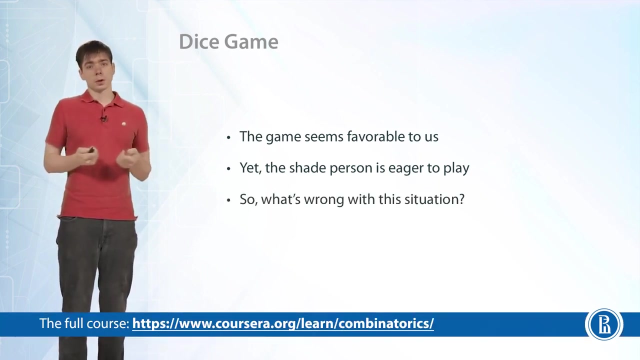 So now, what do we have? The game seems favorable to us, So we have an advantage. And yet there is the shady person who is eager to play this game with us for a long time and with many other people as well, And that's his job. 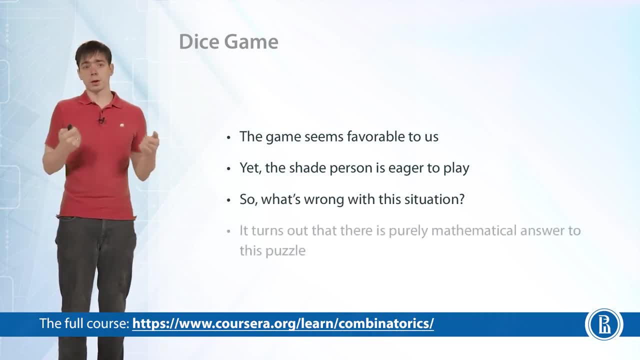 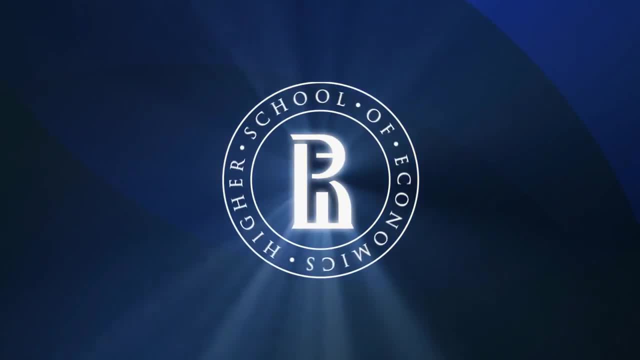 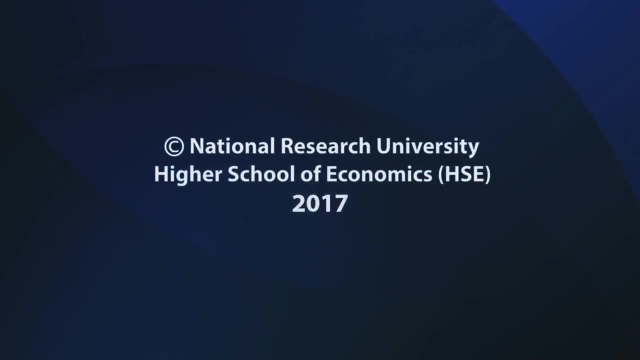 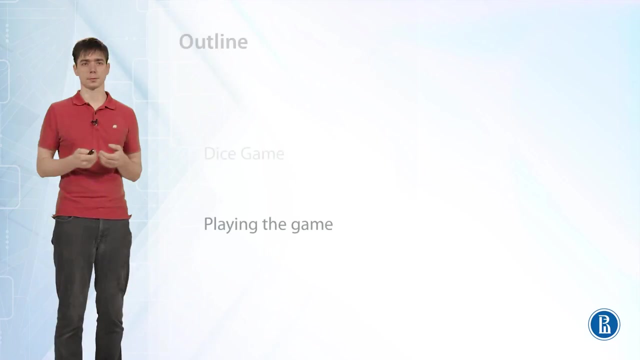 And it turns out that there is a purely mathematical answer to this problem. And it turns out that there is a purely mathematical answer to this problem In the antithetical phenomenon of this world. we may not have the answer to this puzzle. So once we come closer to the shady person, we can see that he has just 3 dice. 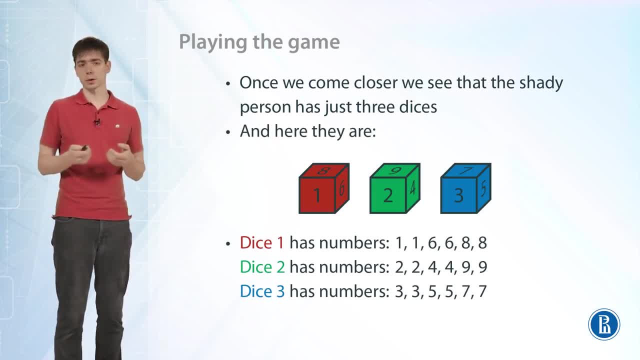 And there they are. The first dice has numbers 1, 1,, 6,, 6 and 8, 8 on its sides. The second dice has numbers 2,, 2,, 4,, 4,, 9, 9.. 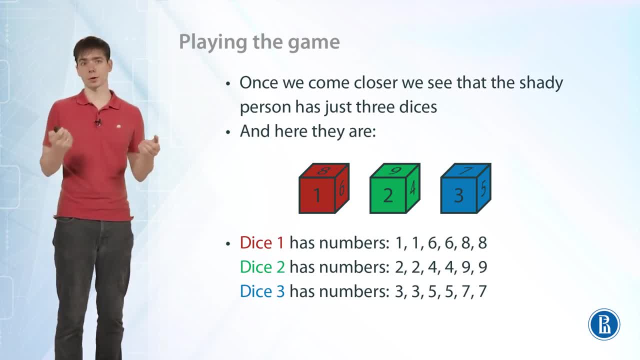 And the third dice has numbers 3,, 3,, 5,, 5,, 7,, 7.. So these are just three dices. Everything is very simple, Okay. so which of the dices should we pick if we play this game? 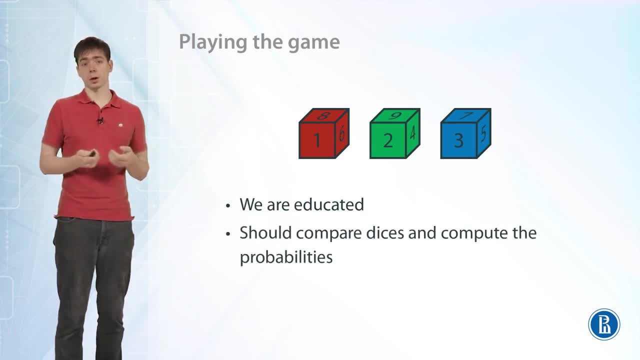 Now we are educated, We know something. now We know that we should just compare dices between each other, compute probabilities and see which of the dices is the best. So let's just do it. Let's start, for example, with dice 1 and dice 2.. 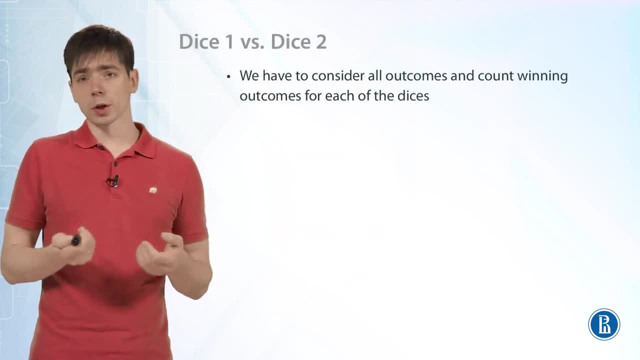 So what should we do? We should consider all possible outcomes and count winning outcomes for both of the dices, for the first dice and for the second one, And we will see which one is better. Okay, so here is the list of all outcomes. 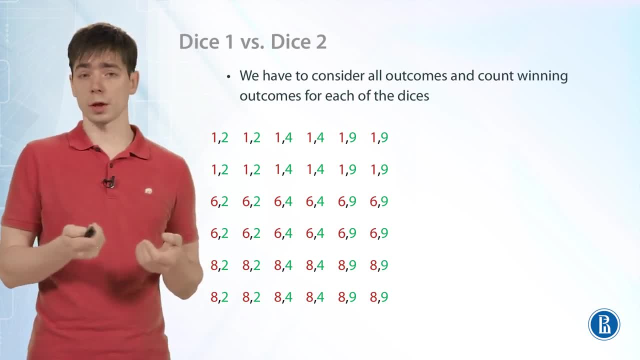 There are six outcomes of the first dice, and rows of this table correspond to outcomes of the first dice, And there are six outcomes of the second dice, And columns correspond to outcomes of the second dice. So the dice that has a larger number wins. 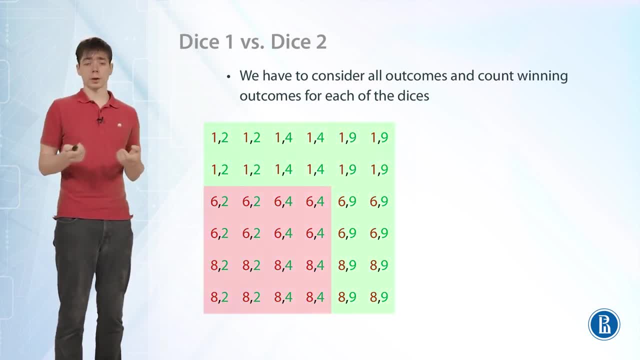 So we can see from this picture that Okay. so here are winning outcomes for both dices And we can count that dice 1 has only 16 winning outcomes and dice 2 has 20 winning outcomes, So dice 2 wins the probability. 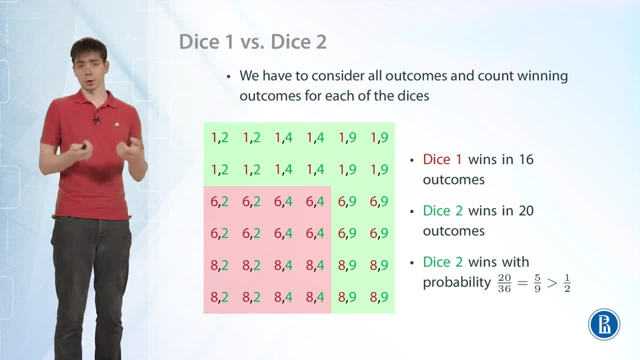 Five over nine, which is greater than one half. If we have to choose, if we are playing with dice 1 against dice 2, we will win in approximately five out of nine games, And if we play this game long enough, we will start winning. 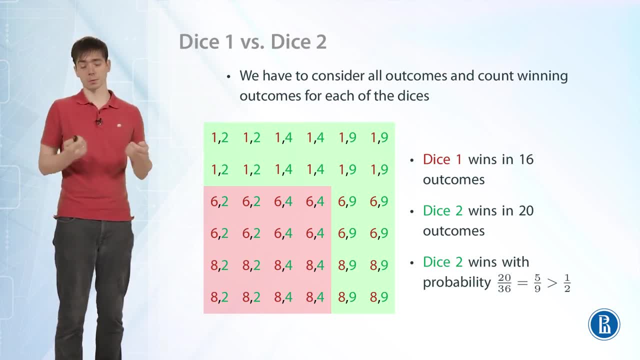 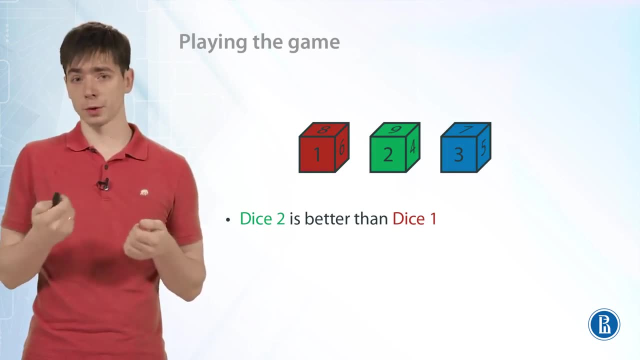 We will start gaining some profit. So dice 2 turns out to be better than dice 1.. And so if we play a game with dice 2 against dice 1, we will, on the long run, we will- start to win. 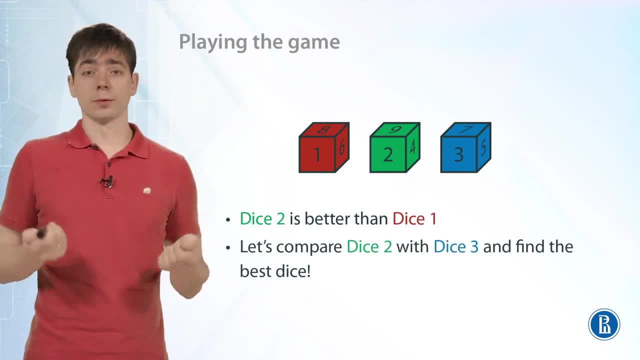 Okay. so now let's compare dice 2 and dice 3, and we will find the best dice. Dice 2 is better than dice 1.. If we compare to dice 3, we will know which one is the best. Okay, again, we have to consider all outcomes. 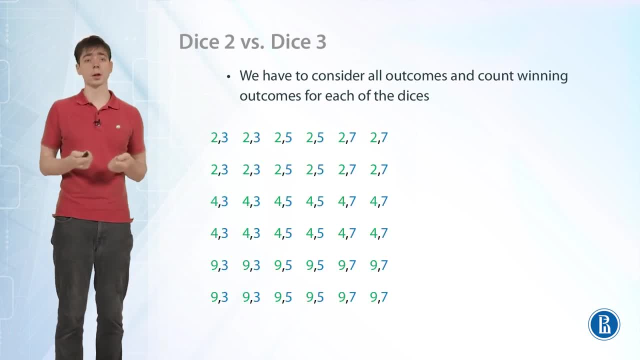 and we have to count winning outcomes for each of both dices. Here is the table again. So now, rows correspond to outcomes of dice 2.. Columns correspond to outcomes of dice 3.. And again, the dice that has larger number wins in this specific outcome. 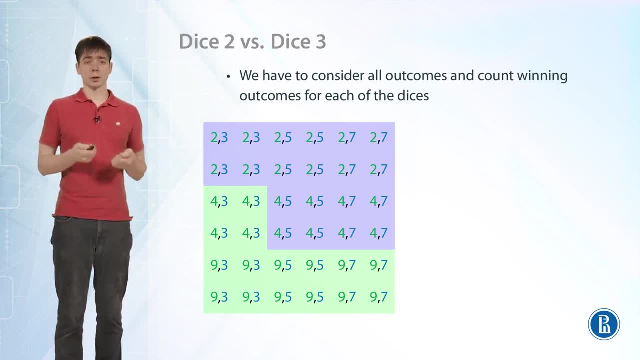 So here are winning outcomes for dice 3 and winning outcomes for dice 2.. So dice 2 now has only 16 winning outcomes, and dice 3 has 20 winning outcomes. Again, as in the previous case, something similar happens. 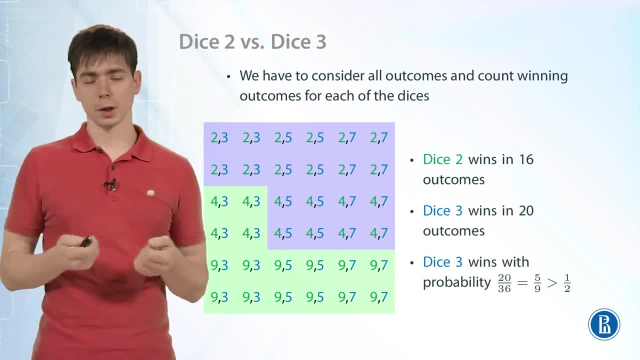 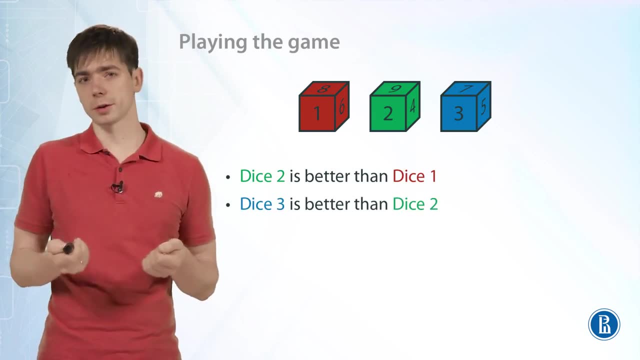 Dice 3 wins with probability 5 over 9.. So dice 3 is better than dice 2, and overall we have the following: Dice 2 is better than dice 1.. Dice 3 is better than dice 2. And so clearly, dice 3 is better than dice 1,. 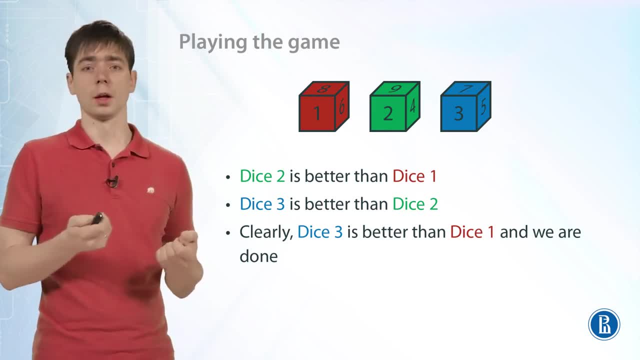 since dice 3 is better than dice 2.. Dice 2 is better than dice 1. And so dice 3 should be much better than dice 2.. And we are done. We should pick dice 3 to play this game. 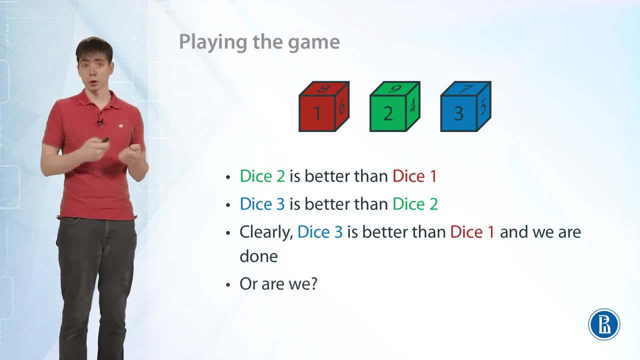 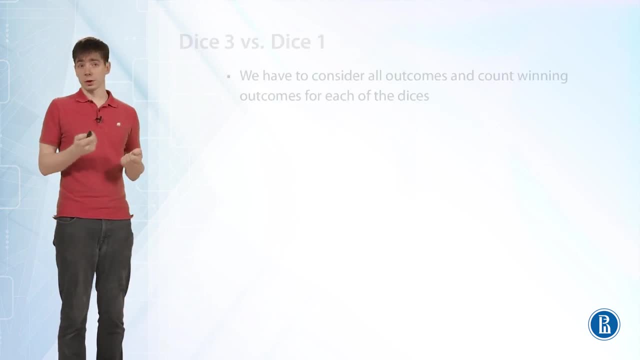 Or are we? Is everything correct? Recall that we are playing with a shady person. We should be careful here. So let's just check just to be sure. Okay, let's compare dice 3 and dice 1.. Again, we have to consider all outcomes. 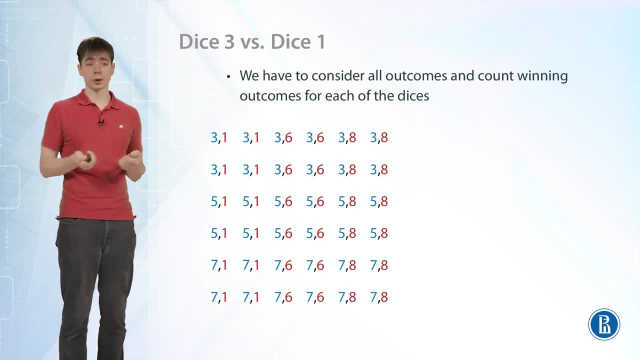 Again, we have to count winning outcomes for each of the dice. And here is the table now. Rows correspond to outcomes of dice 3.. Columns correspond to outcomes of dice 1. And the dice that has larger number wins in a certain outcome. 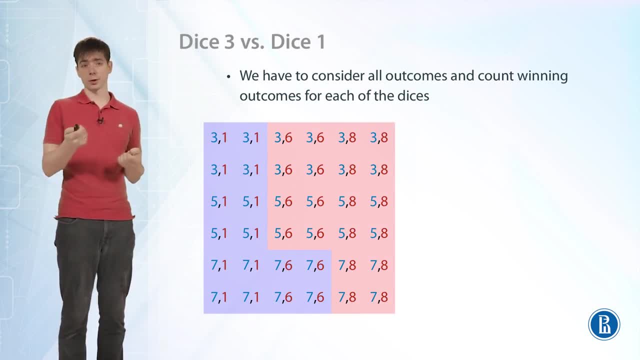 So Here we can see that here are winning outcomes for dice 1. And here are winning outcomes for dice 3.. And we can see that there are only 16 winning outcomes for dice 3. And there are 20 winning outcomes for dice 1.. 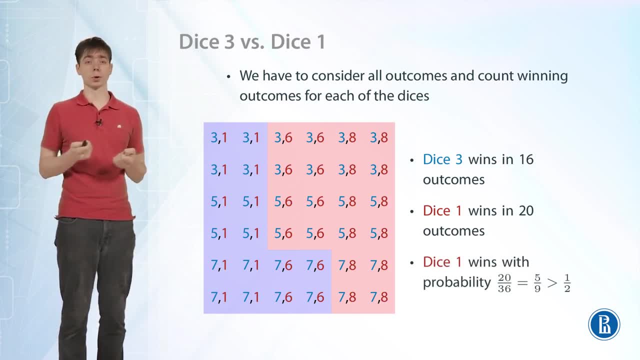 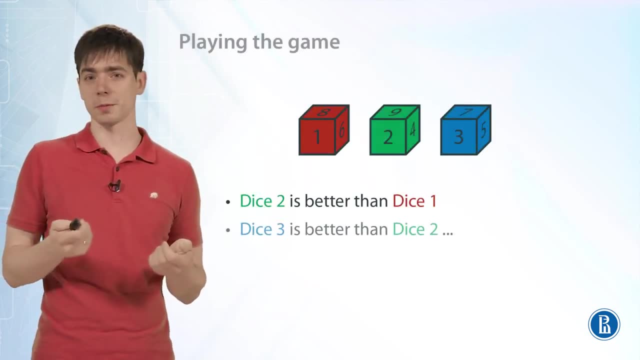 And so dice 1 wins with probability 5 over 9, which is greater than 1 half. So let's summarize what we have: Dice 2 is better than dice 1.. Dice 3 is better than dice 2.. We have showed both of these. 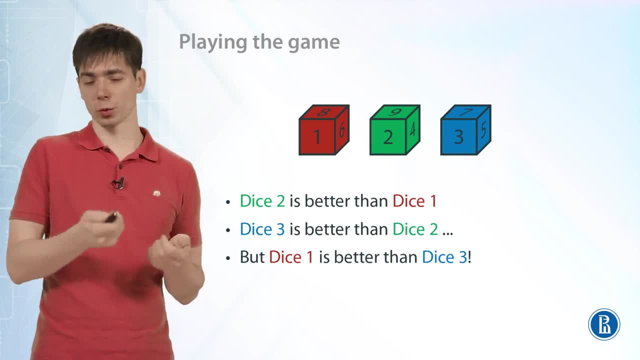 But it turns out that dice 1 is better than dice 2.. Dice 2 is better than dice 3.. So we did the calculation in all of three cases. So all of this is true. So how is this even possible? What is going on? 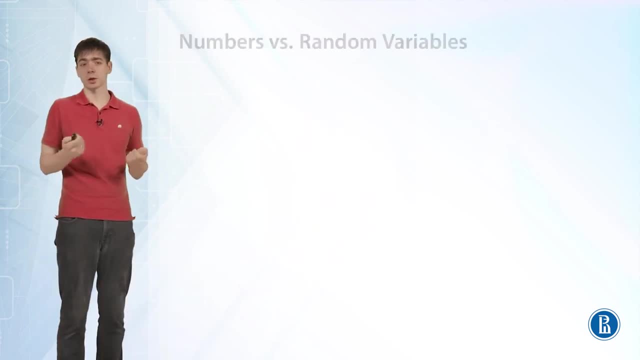 So what is happening? And here is some explanation. We are used to compare numbers. We do it a lot. We do it in real life constantly. This is a very common thing we do And we are used that certain properties hold for numbers. 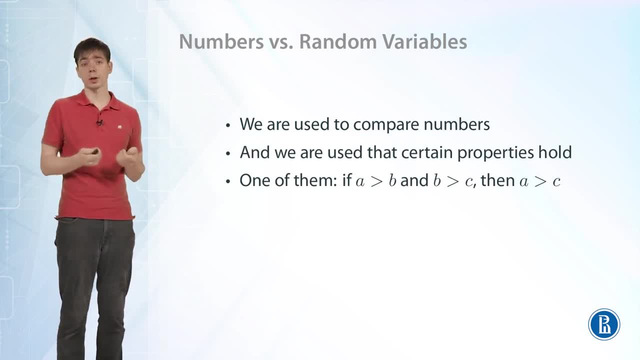 For example. here is one of them: If some number, a, is greater than some number b and b is greater than c, then a should be greater than c. This is a very common property. In mathematics it is called transitivity, So we are very used to it. 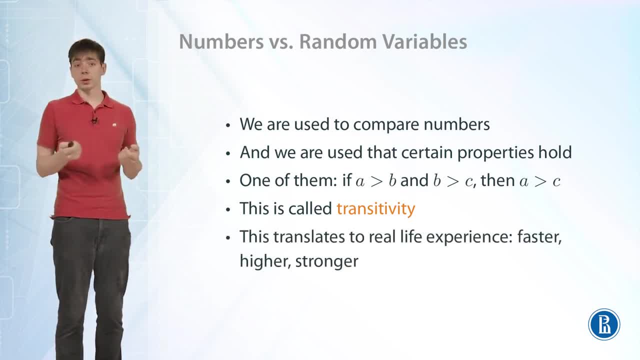 We use it constantly And it translates to real life experience again constantly. So here is an Olympic motto, for example: Faster, higher, stronger. In all of these we are mostly used that transitivity holds If someone is faster than someone else and this second person is faster than the third person. 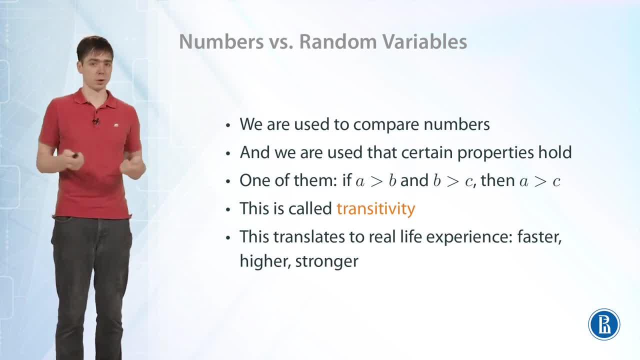 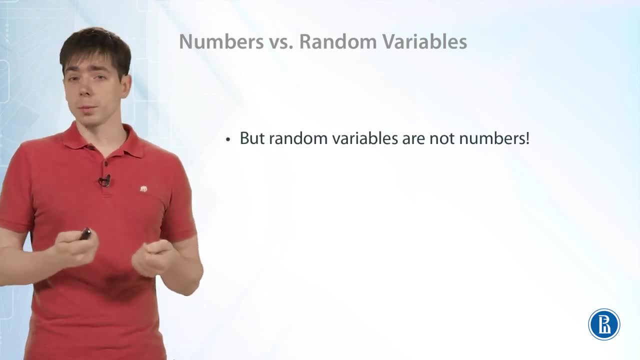 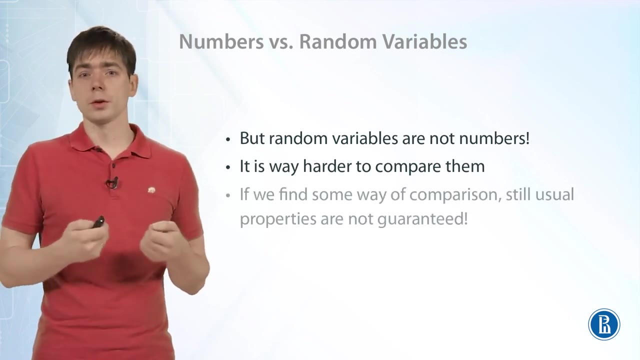 then the first person is faster than the third one. So this is very typical and this is very standard. But note that random variables are not just numbers. They are more complicated And it is way harder to compare random variables And even if we find some way to compare them, 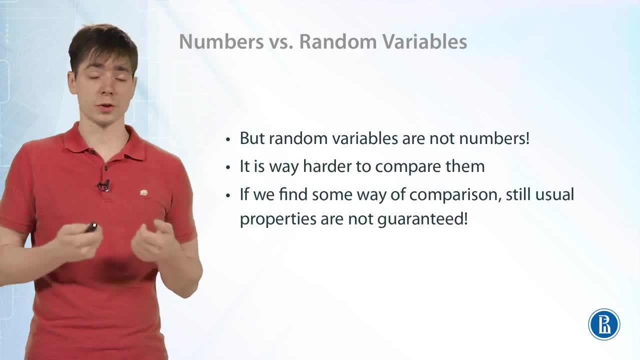 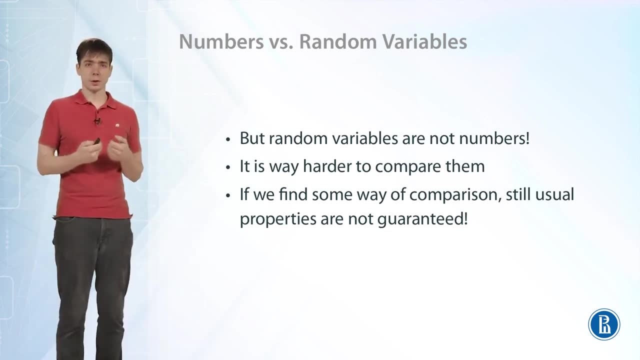 like in our game, we compare some random variables in a certain way. If we find some way to compare random variables, we are still not guaranteed that properties we are used to are still holding for random variables, And so this is the problem in our puzzle, in our game. 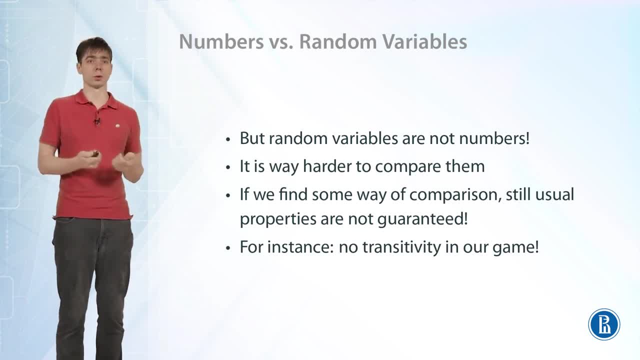 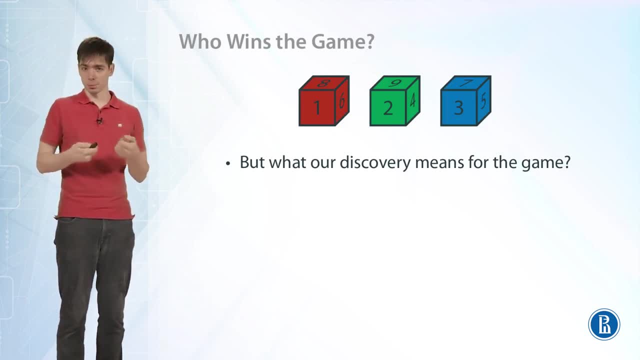 For instance, transitivity in our game doesn't hold, And that's what we have shown. Okay, but what does it mean? What does our analysis give us for the game with the shady person? What does it tell us? So let's recall what we have. 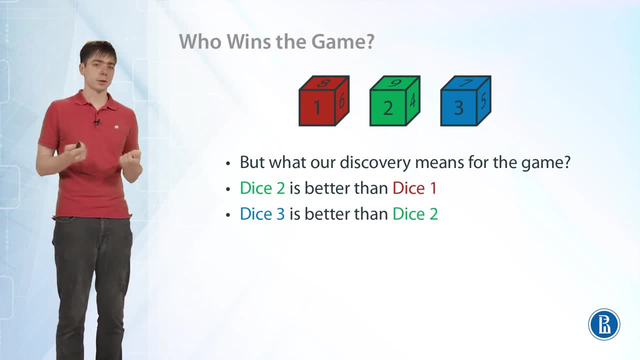 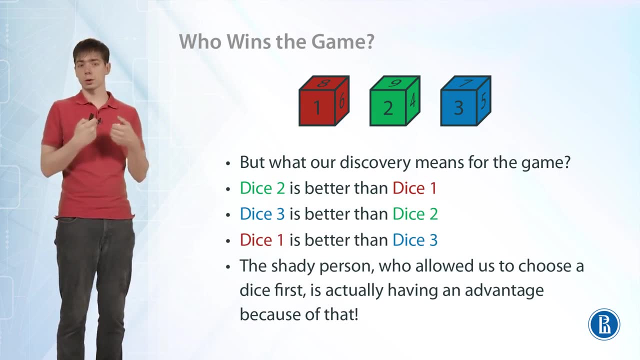 Dice two is better than dice one. Dice three is better than dice two. Dice one is better than dice three. And now note that the shady person who tells you that, to give you an advantage, he will allow you to choose your dice first. actually, in this specific moment, he is gaining an advantage. 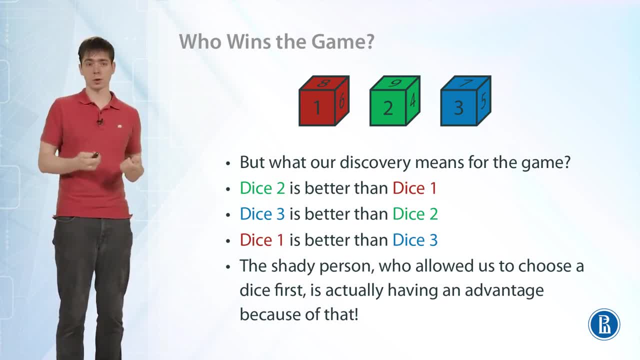 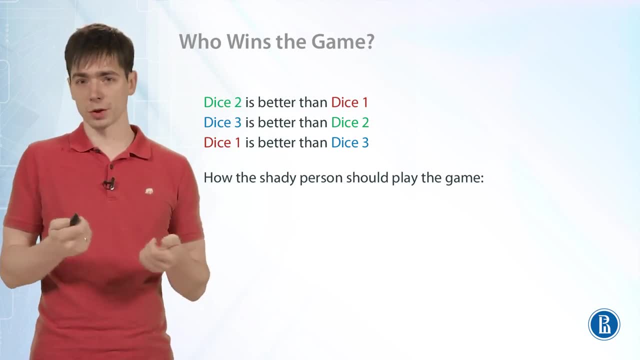 He is gaining an advantage because you choose your dice first. So let's see how the shady person will play his game. He should play his game this way, And he certainly will, because that's his job. Dice two is better than dice one. 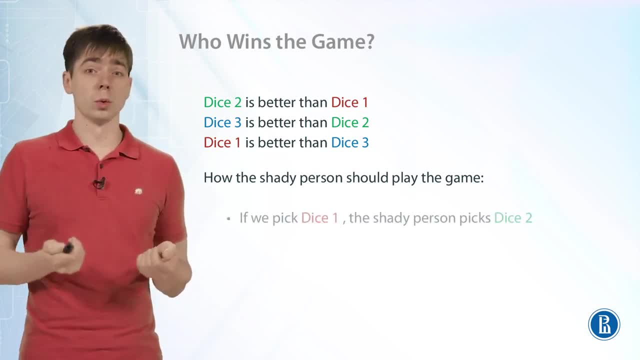 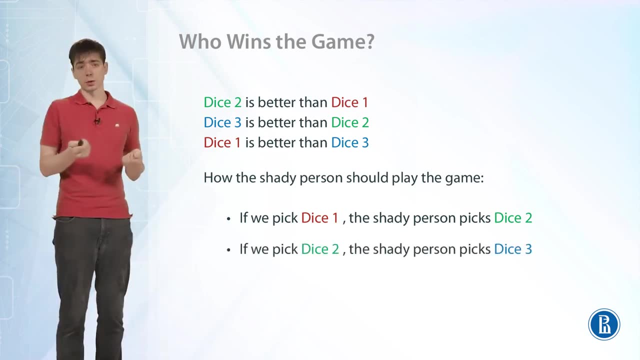 Dice three is better than dice two. Dice one is better than dice three. So if we pick dice one, the shady person will pick dice two And on the long run he will start winning. If we pick dice two, the shady person will pick dice three. 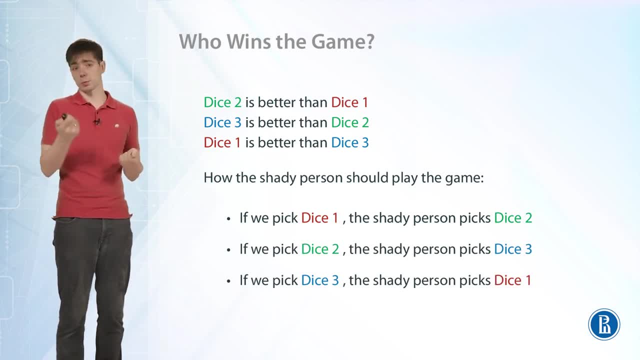 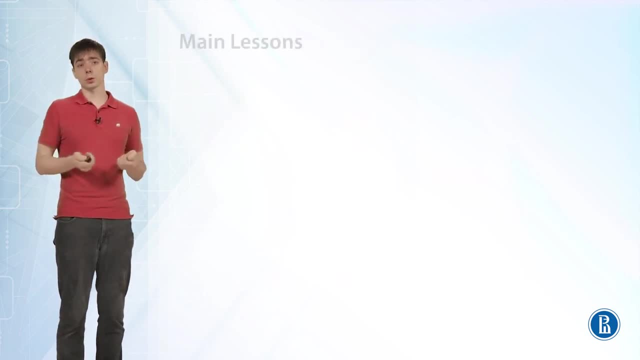 And if we pick dice three, the shady person will just pick dice two, which is better than dice three, And that's the whole strategy for the shady person. Okay, so let's review the main lessons we have seen in this video. The probability is tricky. 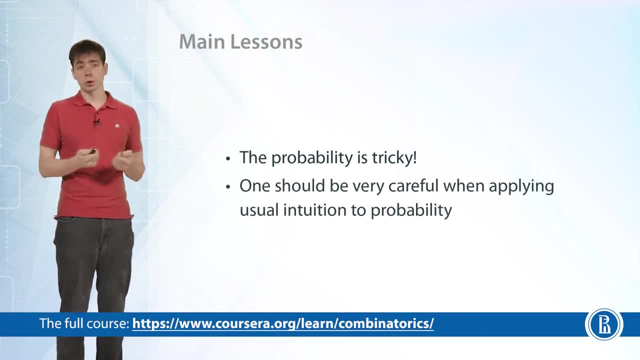 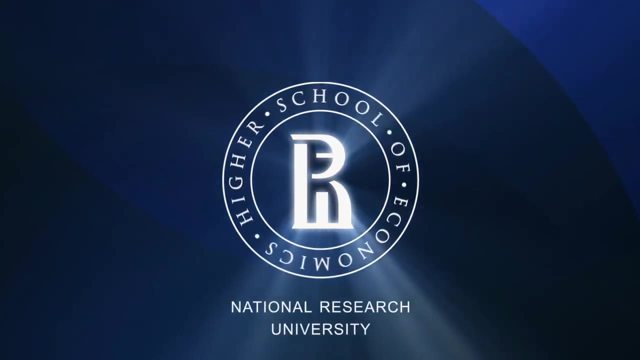 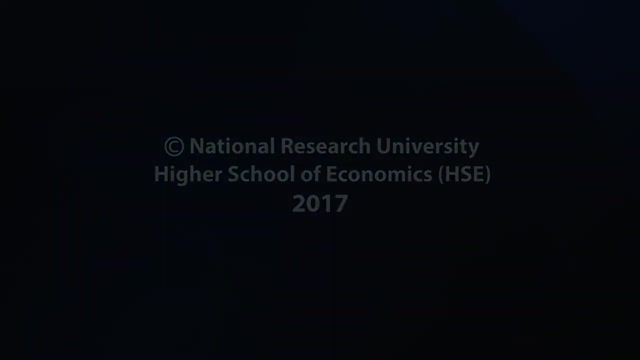 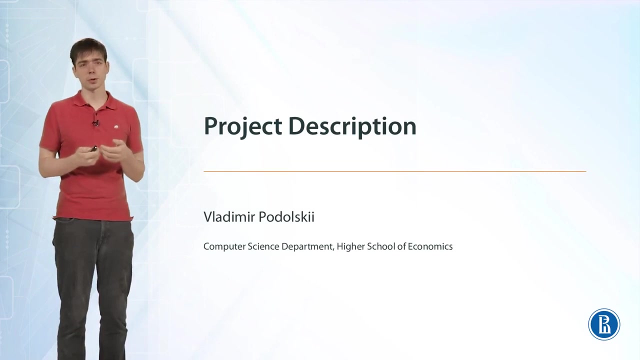 We should be very careful when we apply our usual intuition to probability. It is very tricky and very complicated, Sometimes very counterintuitive, And one more lesson we should probably avoid – scam games. Hi, I'm Vladimir Podolsky, And in this video we will discuss the project of our course. 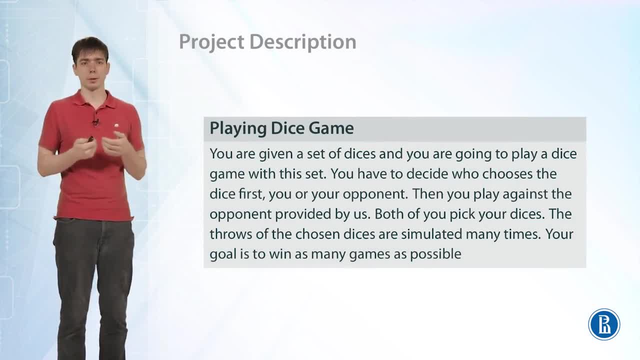 So in this project you will create a program that plays the following game. You are given a set of dice And you are going to play a dice game with this set. First, you have to decide who chooses his dice first – you or your opponent. 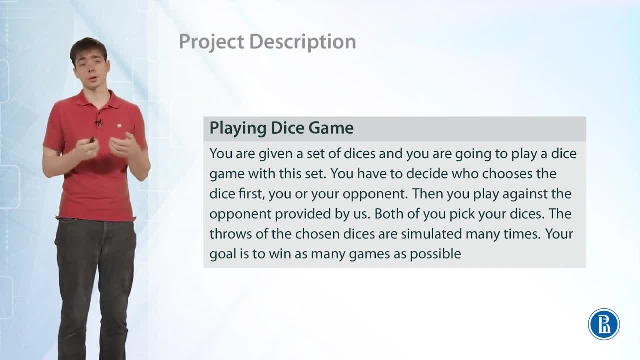 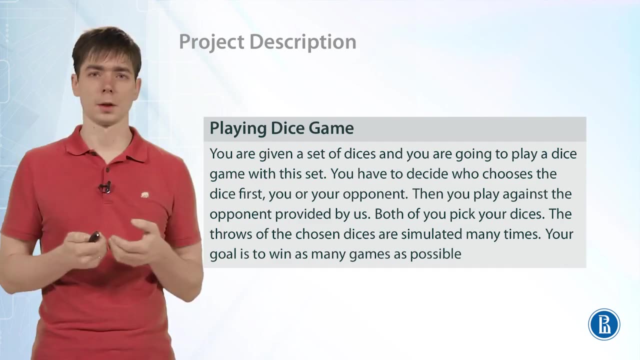 And then you will play a game against an opponent provided by us. So you and your opponent will choose your dice And then the throws of the chosen dice will be simulated many times, And your goal is to win as many games as possible. So, since you can choose whether you pick your dice first or not, 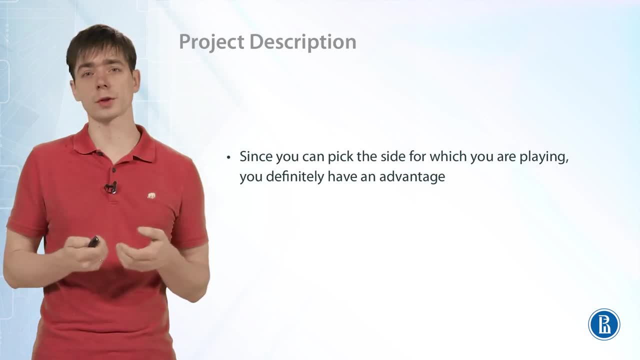 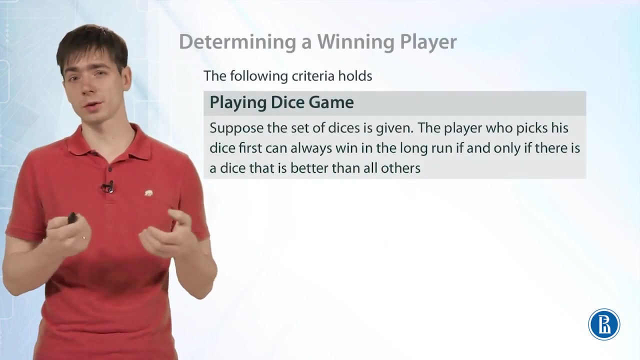 so you are choosing the side for which you are playing. you definitely have an advantage in this game, And the key is to pick the right side, of course. So how should one do that? And it turns out that this simple criteria holds. 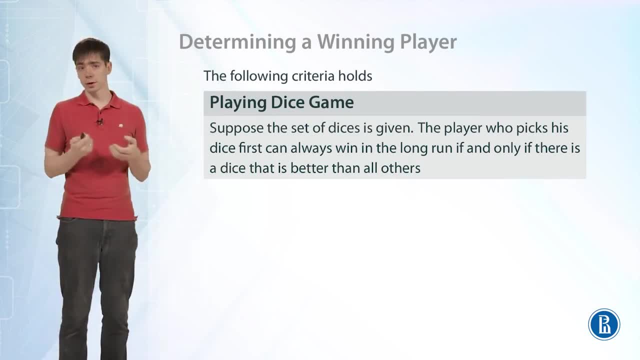 So suppose there is a set of dice given to you And the player who picks his dice first can always win in the long run If, and only if, there is a dice that is better than all other dices. Okay, so let's see why this statement is true. 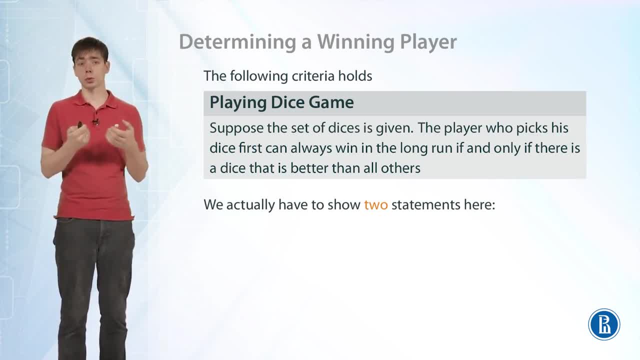 And to show this statement we need actually to show two things. First, if there is a dice that is better than all others, then the first player wins, But the converse is also guaranteed, so it should be a criteria If there is no dice. 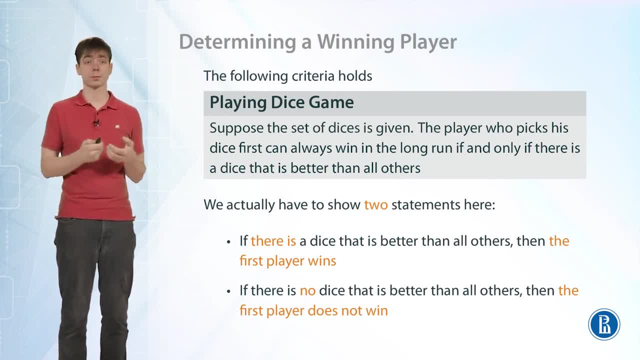 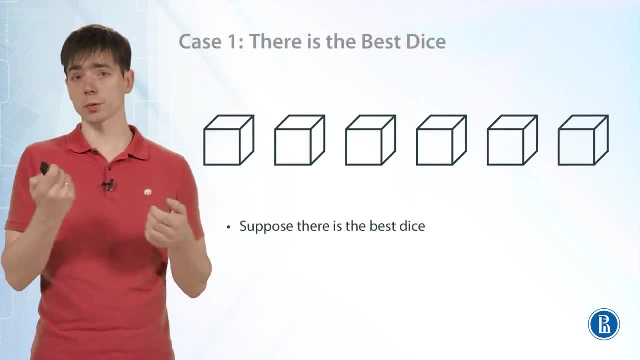 that is better than all others, then the first player doesn't win. So we have to show these two statements, And let's show them one by one. Let's consider two situations. The first one is: there is the best dice, So here is our set of dices. 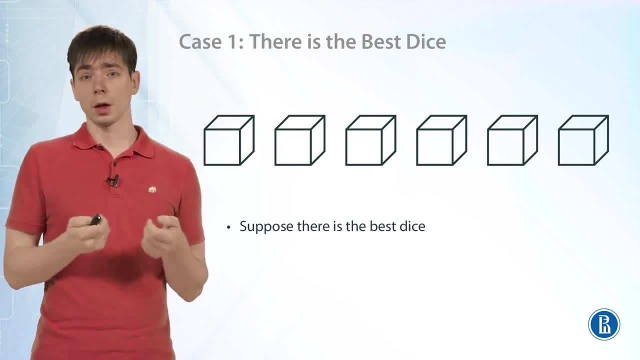 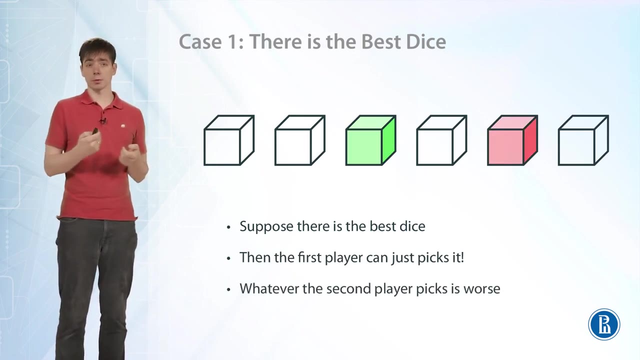 And there is one that is better than all others, And then we will show that the first player wins. And the strategy is very simple: The first player should just pick the best dice And then the second player should pick some other dice, And since the dice of the first player is better than all others, 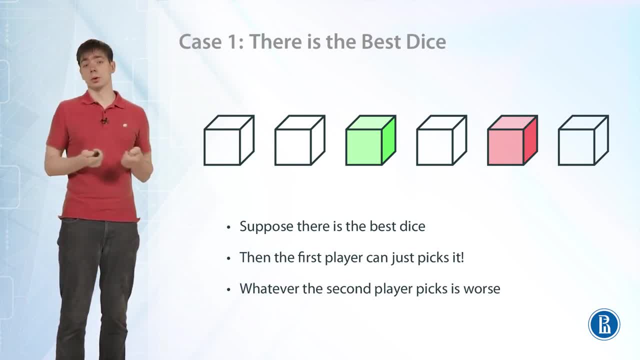 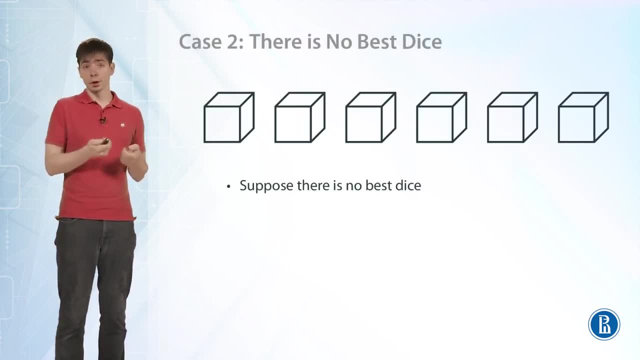 it will be better than the dice of the second player, So the first player will win on the long run. Okay, and now the second case. There is no best dice in this set. So we are given a set of dices and there is no dice that is better than all others. 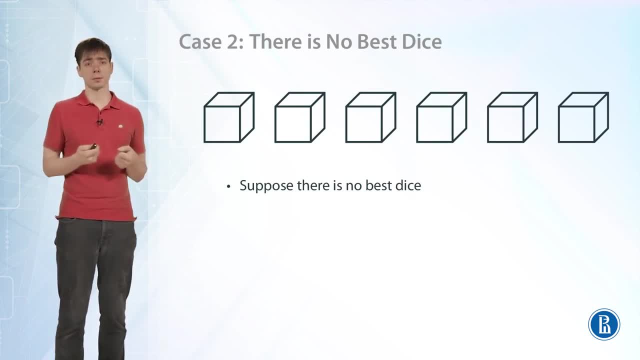 We have seen an example of such set of dices in the previous video. So now what's going on? Since there is no best dice in this set, it means the following: For any dice, there is some other dice that is not worse than it. 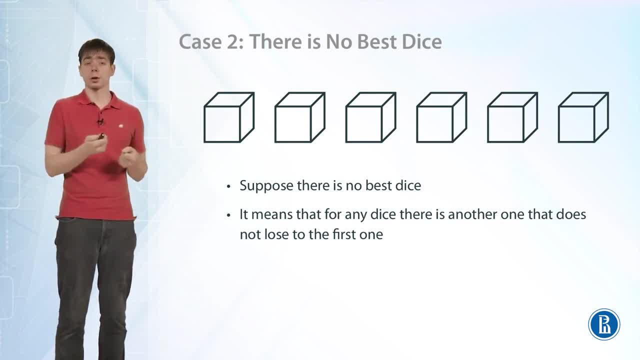 That doesn't lose for the first one. In the worst case they will be equal, So they will have probability one half each, And otherwise for each dice there will be just dice that is better than all others, And that's the winning against it. 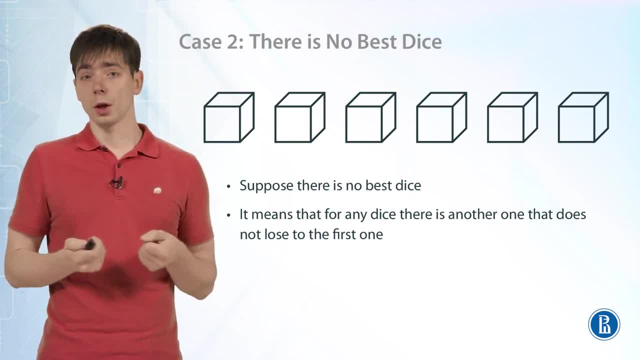 And now the second player turns out to have a winning strategy. So suppose the first player picks one of the dices and then the second player will just So, since we know that for each dice, and in particular for this red dice, there is another dice that is better than this one. 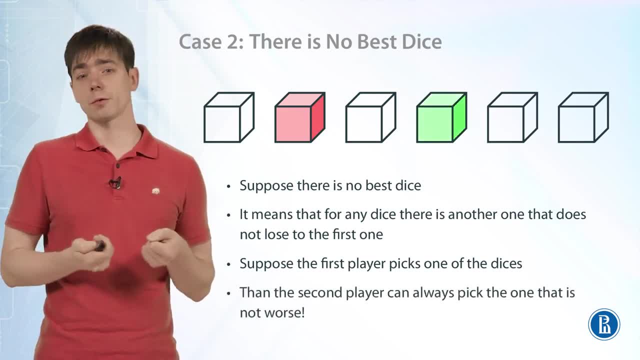 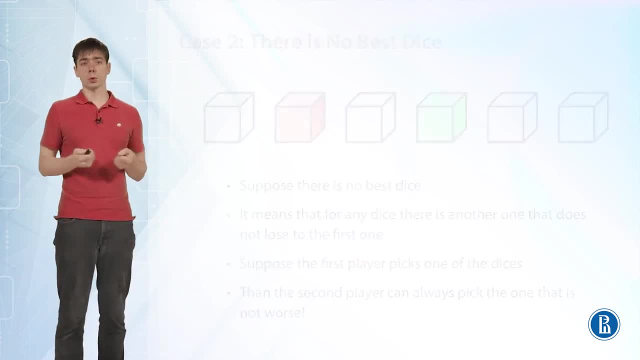 or at least not worse. so the second player will just pick the dice. that is not worse than the red one, And that's the whole strategy. So it's also very simple. Okay, so now how should your program play this game? 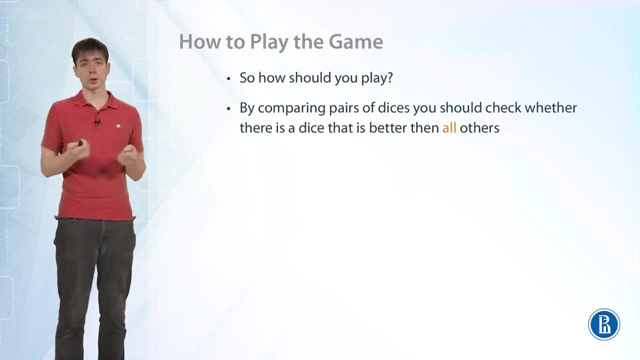 Okay, we need first to compare all pairs of dices and we should check whether there is a dice that is better than all others. We will check our criteria And if there is such a dice, okay to win as many games as possible. 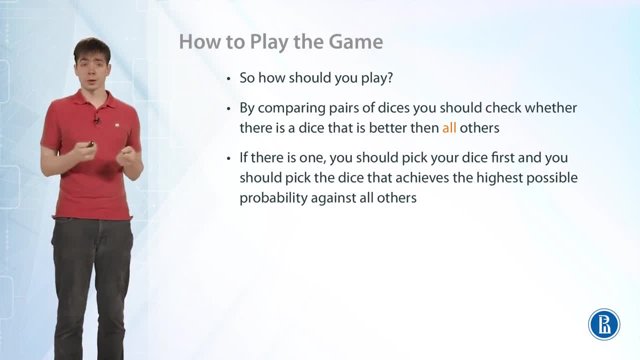 one should pick the dice that is better than all our dices with highest possible probability, So that wins against all our dices with highest possible probability. And if there is no such dice, one should find for each dice the one that is best against it. 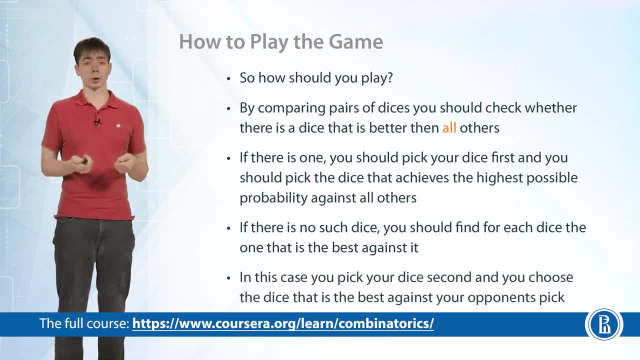 and then choose the role of the second player And then, once the first player picks his dice, then we choose the dice that is better than the dice of the first player by as large probability as possible. 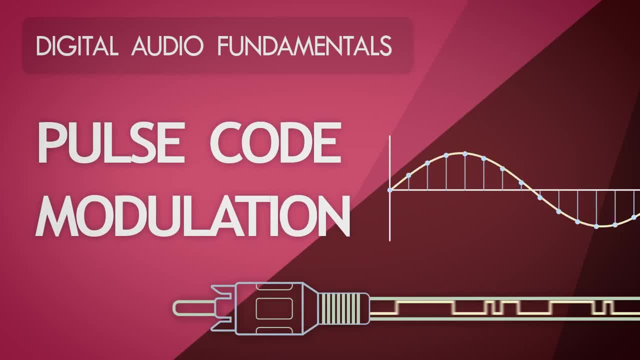 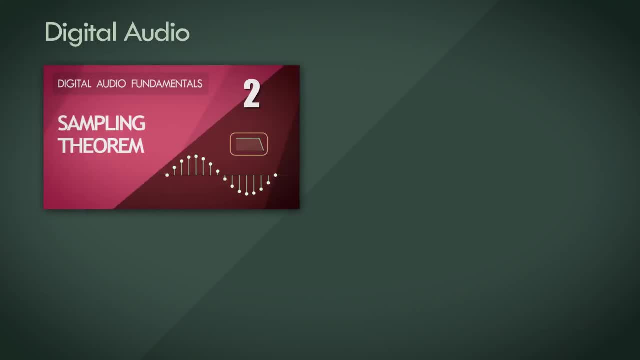 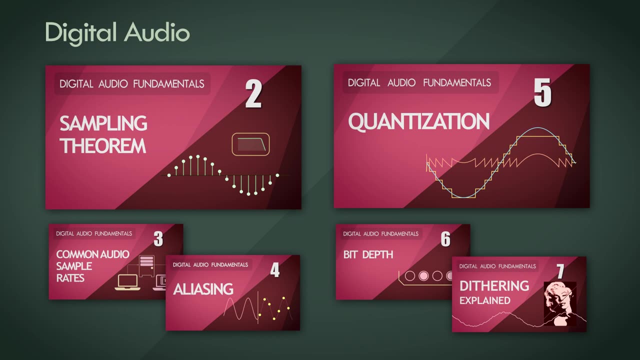 We've been talking about digital audio for a while now. We've talked about sampling, quantization and several nuanced topics along the way, all in isolation, all hinting at a topic in the future where they may be combined together to get a form of audio in the digital. 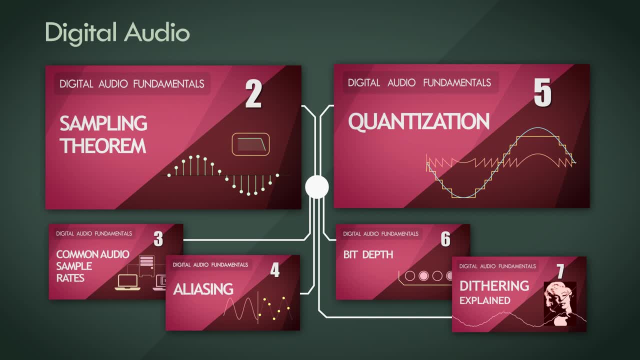 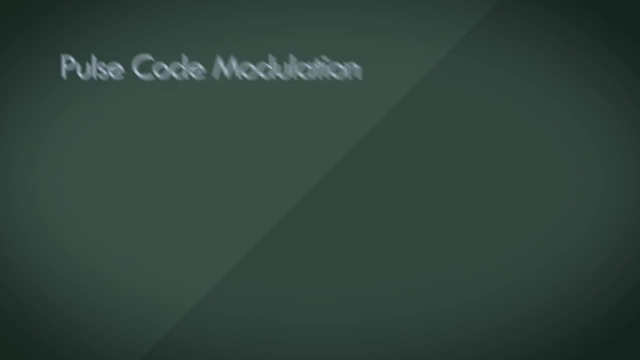 domain that can be transmitted and stored and used in the real world. This is that topic, the final piece that lets us piece together all these digital transformations. The final piece is encoding a way of digitally representing sampled and quantized data. The title of this video is Pulse Code Modulation, and Pulse Code Modulation is a specific type. 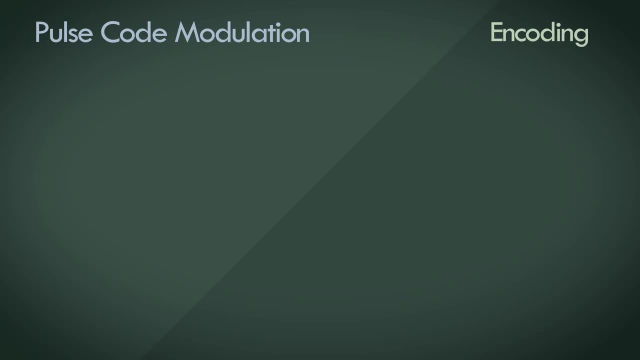 of encoding strategy. The reason why we are talking about Pulse Code Modulation, or PCM, specifically is because it's the most common encoding scheme in news, the easiest to understand and a classical method that's been around since the dawn of digital audio. I'll have you note that there are several different alternative encoding. 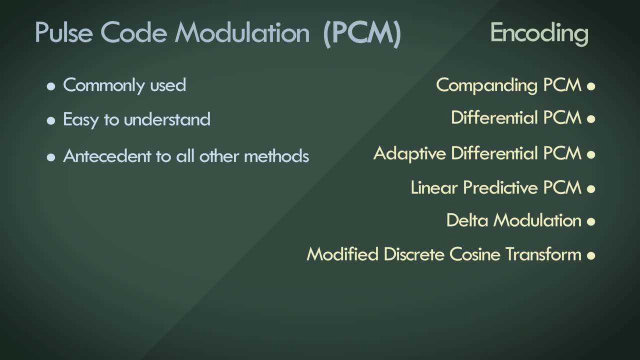 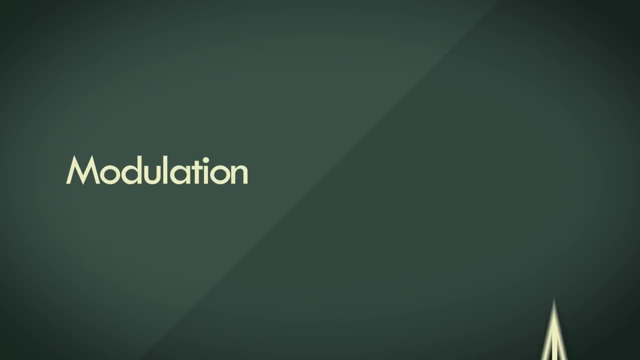 schemes with benefits and drawbacks of their own, and we'll describe a few here and go over them in more detail in future videos. But we'll start from scratch and build up to why PCM is a viable encoding strategy. You've all heard of FM before in the context of radio transmission. 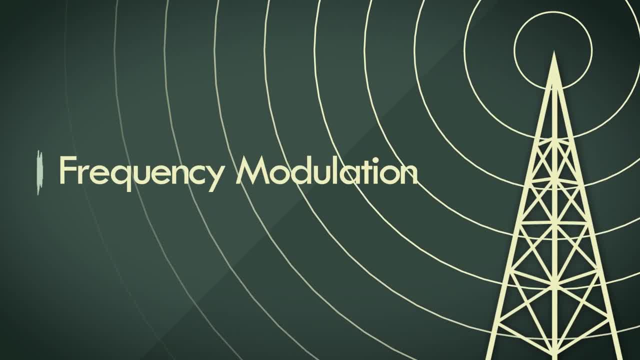 FM is Frequency Modulation. Let's say you have a piece of music or speech and you want to transmit it wirelessly across large distances. You'll find that doing this directly, transmitting the audio signal directly, is very limiting and you won't get very far. 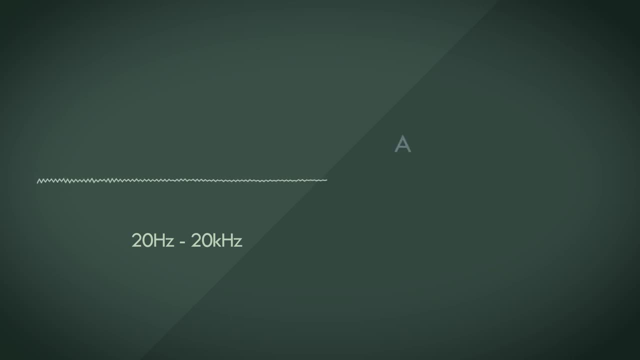 For starters, the audio band between 20Hz and 20kHz just doesn't have enough power and would need a lot of amplification to be transmitted even short distances, And if you receive it on the other side and try to play it back, you'll end up with a very short distance.